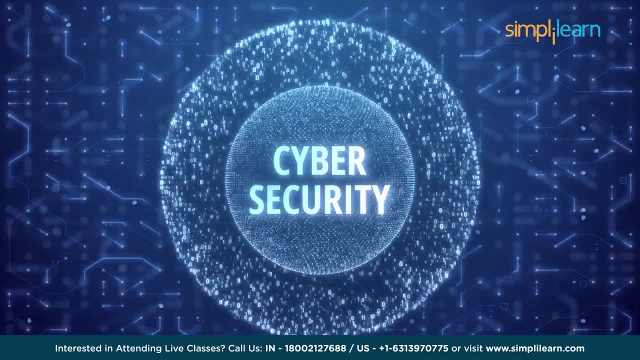 have a solid foundation in cyber security and seek to expand their knowledge in specialized areas. Our advanced Cybersecurity course goes beyond theory. Throughout the course, a considerate especialist is in the get-go phase to address the expertise question In order to fill in. 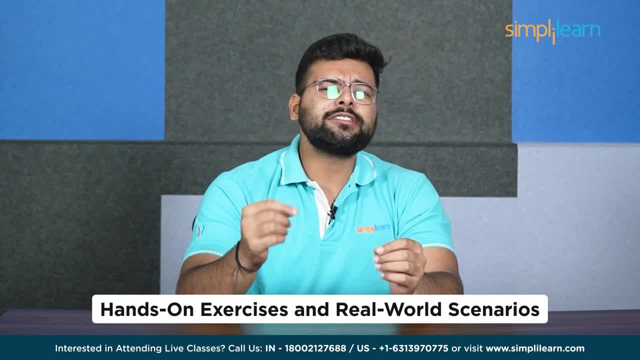 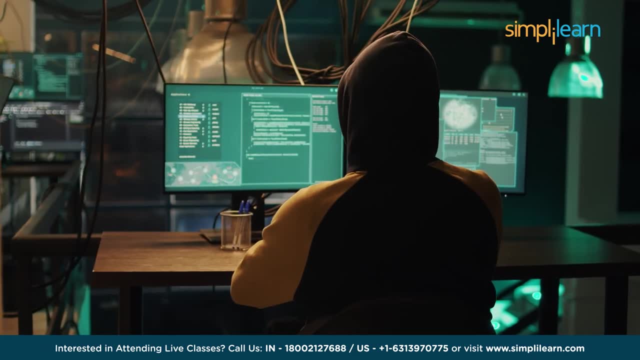 In this full course, you will have access to practical hands-on exercises and real-world scenarios. You will work on simulated environments, conduct vulnerability assessments and develop incident response plans, gaining valuable experience in a safe learning environment. And now we will break down the topics: what we have to learn in this full course. 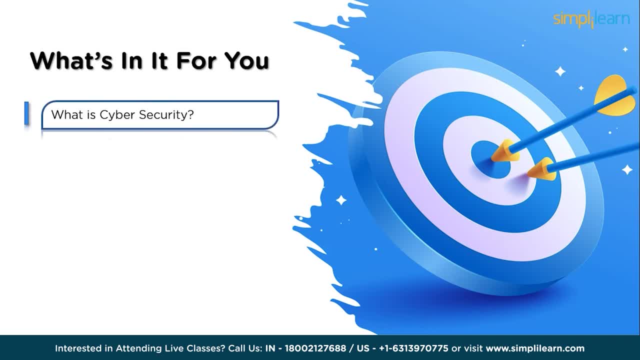 And here we will start with what is cyber security? that is introduction to the concept of cyber security and its importance in today's digital world. and after that we have what is ethical hacking? that is, exploring the role of ethical hackers in identifying vulnerabilities and improving security. 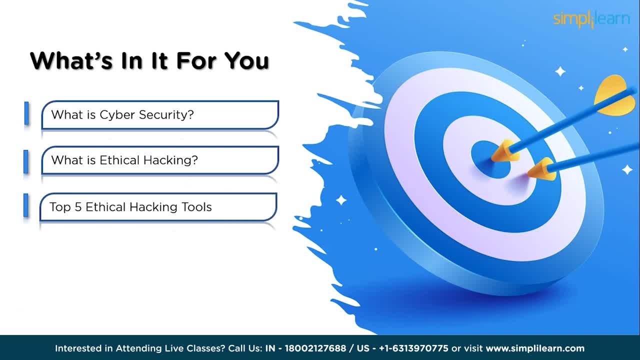 Then we will have a look on top 5 ethical hacking tools. that is introduction to some popular tools that is used by ethical hackers for vulnerability assessment and penetration testing. Then we have ethical hacking and penetration testing. that is, understanding the fundamentals of ethical hacking and the process of penetration testing and phases of penetration testing. 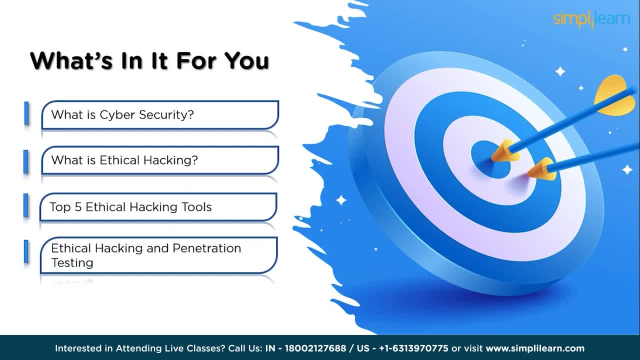 Then we will understand the functionalities and application. Then we will understand the application of Metasploit, that is a powerful framework for conducting attacks. Then we will have an exploration on VPN, that is, virtual private network. that is, explaining the concept of VPN and how it provides secure and private communication over the internet. 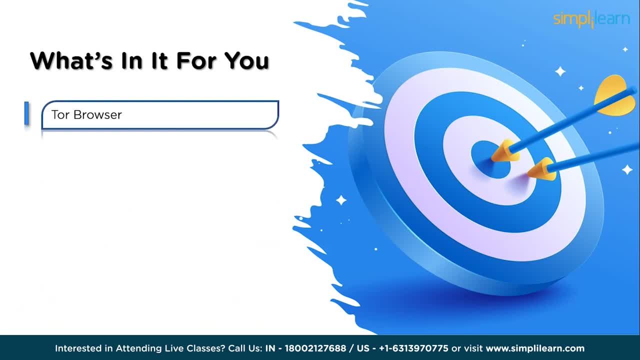 Then we have Tor browser, that is, we will introduce the Tor browser and its role in maintaining anonymity and privacy online. Then we will explore firewall, that is, understanding the purpose and functionality of a firewall in protecting network. Then we will understand what is ransomware, that is, we will explore the threat of ransomware. 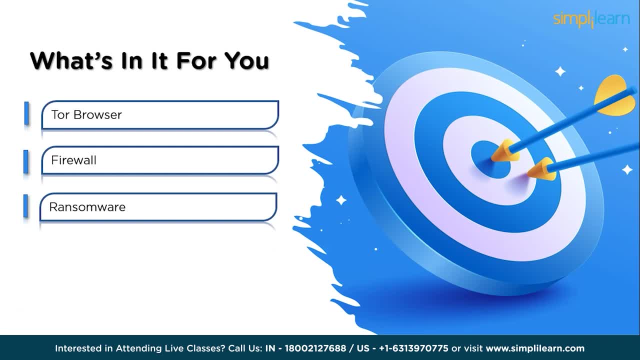 its impact on individuals and organizations and preventive measures. Then we will have a look on malware, that is, defining malware and its various forms, as well as discussing strategies to detect and mitigate malware attacks. Then we will learn what is SQL injection and explaining the concept of SQL injection. a 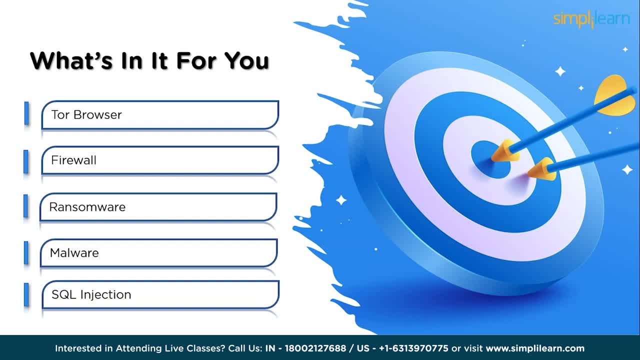 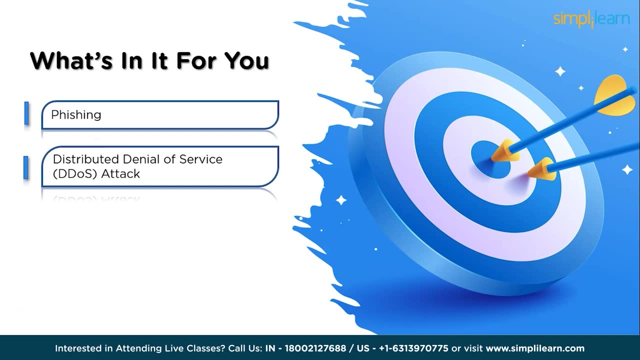 common web application: vulnerability and methods to prevent it. Then we have phishing: Understanding phishing attacks, how they deceive users and best practices to avoid falling victim to them. Then we have Distributive Denial of Service, that is, DDoS attack. Discussing the DDoS attack method, its impact on networks and mitigation techniques. 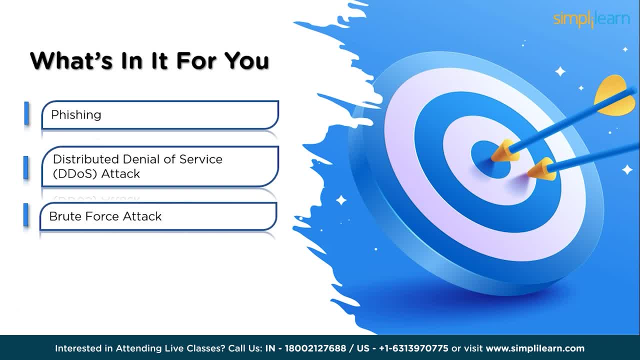 Then we will learn what is brute force attacks, Exploring brute force attacks and the methods used by attackers to gain unauthorized access to systems. Then we have botnet: Defining botnets, their role in conducting cyber attacks and strategies to detect and mitigate cyber attacks. 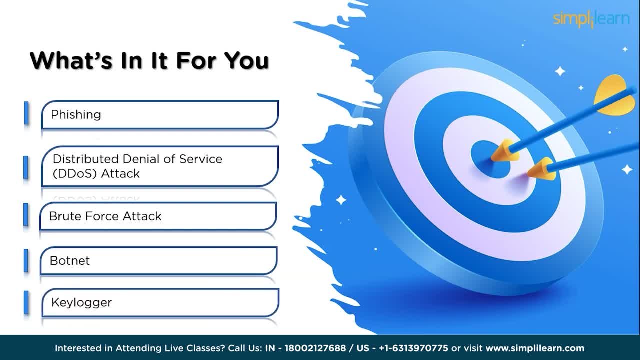 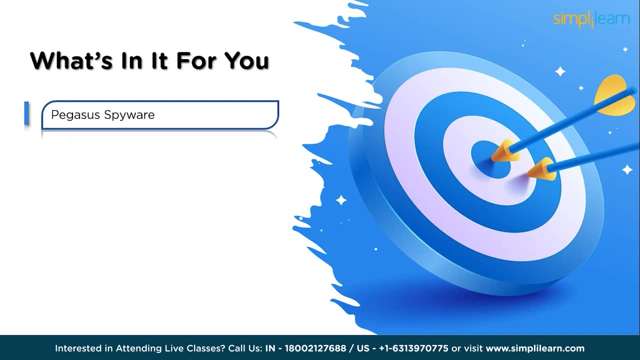 And to detect and disrupt them. Then we will understand what is keylogger, That is, understanding keyloggers, how they work and preventive measures to protect against keylogging attacks. Then we have Pegasus spyware: Analyzing the infamous Pegasus spyware and its implications on user privacy and security. 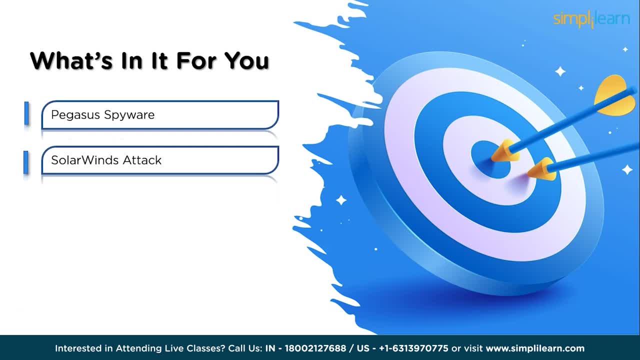 Then we have SolarWinds attack: Examining the SolarWinds attack, a high-profile supply chain attack, and its lesson for cybersecurity. Then we will see what is cyber war: Exploring the concept of cyber warfare, its implications and the role of cybersecurity. 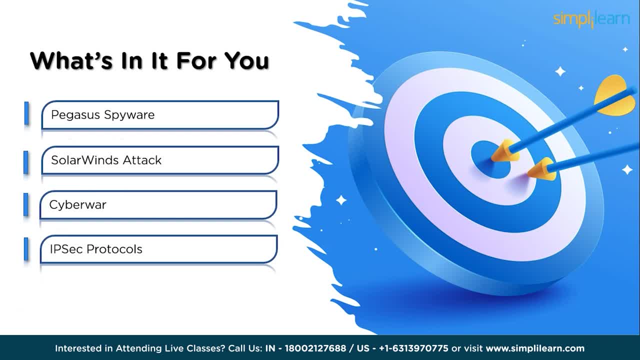 in defending against it. Then we have IPSec protocols. Introducing IPSec protocols and their use in securing network communication, Then we will understand what is network security, Understanding the fundamentals of network security, including network segmentation, firewalls and intrusion detection. 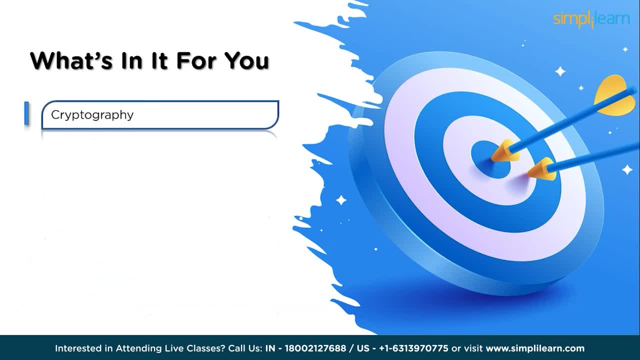 Then we have cryptography, Exploring the principles of cryptography and its role in securing data and communications. Then we have symmetric key cryptography, Exploring the principles of cryptography and its role in securing data and communications. Then we have key cryptography, Discussing symmetric key cryptography algorithms and their applications in securing data. 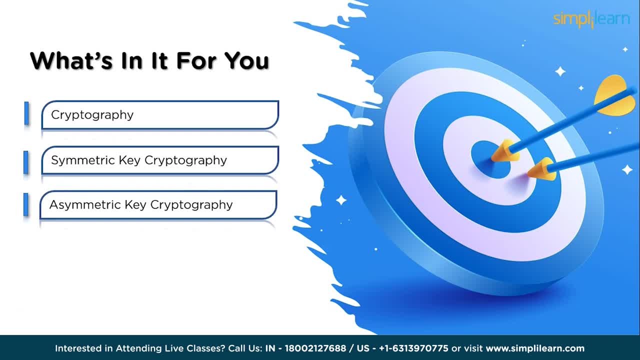 Then we have asymmetric key cryptography. That is explaining asymmetric key cryptography algorithms, including their use in encryption, digital signatures and key exchange. Then we have hashing, That is understanding hashing algorithms, their role in data integrity and their applications in password storage. 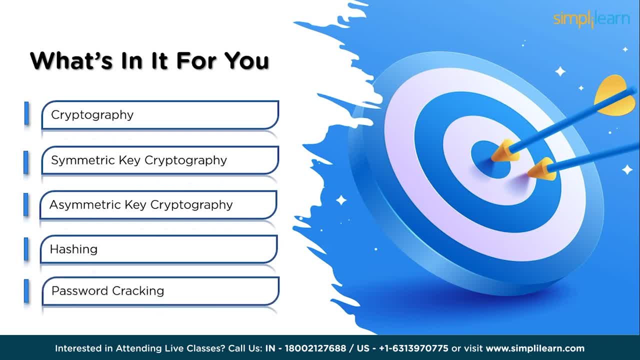 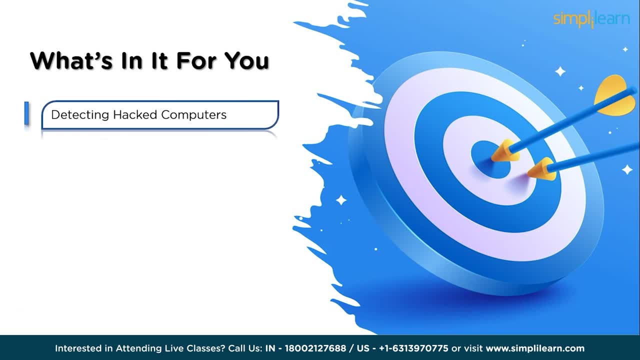 Then we have password cracking: Discussing common methods used by hackers to crack passwords and strategies to create strong, secure passwords. then we have detecting hacked computers: we'll explore science and techniques to identify if your computer has been hacked. then we'll secure whatsapp from hackers, that is, we'll 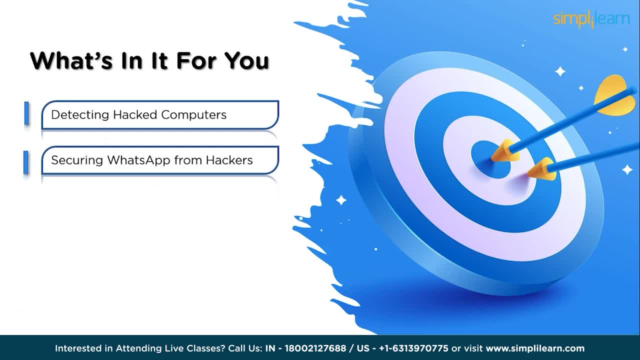 see the best practices and tips to keep your whatsapp account safe from hacking attempts. then we'll see the kali linux installation. that is a step-by-step guide to installing kali linux, a popular operating system for ethical hacking and penetration testing. then we have parrot security os installation. that is a step-by-step guide to installing parrot security os and alternative. 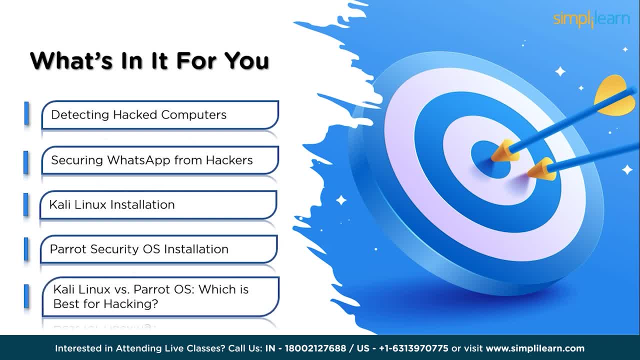 operating system for cyber security professionals, then we'll have a differentiation, that is, kali linux versus parrot os. which is best for hacking. a comparison of kali linux and security os, helping you choose the right operating system for your needs. then we have nmap tutorial for beginners. 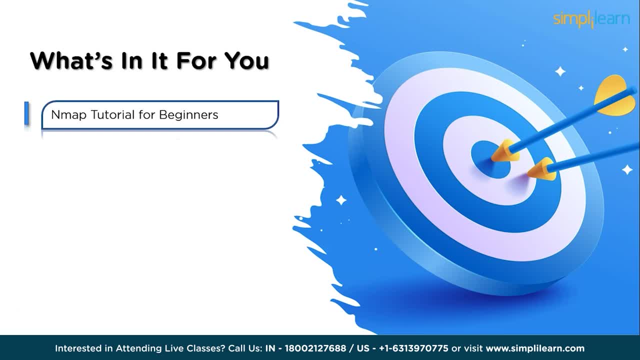 that is a beginner friendly tutorial on using nmap, a powerful network scanning tool. then we have ubuntu versus debian. which one should you use? that is a comparison between ubuntu and debian, two popular linux distributions, to help you make an informed decision. then we have intrusion detection systems, ids. that is exploring the concept of ids and its role in detecting and preventing. 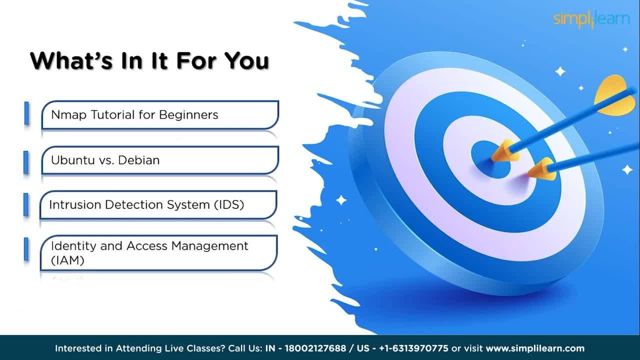 unauthorized activities in computer system. then we have identity and access management- iam. in this we'll understand iem system and their significance in managing user identities and controlling access to resources. then we have password cracking and after that we'll have cyber security certifications. that is an overview of various 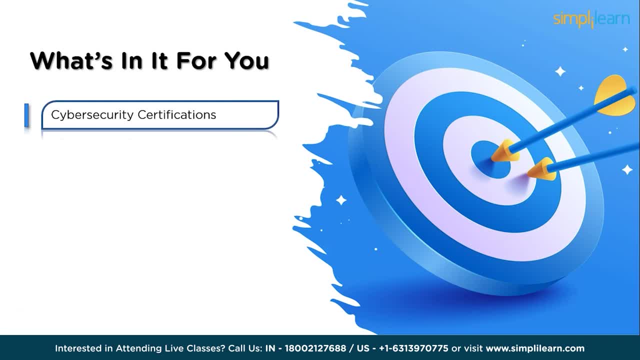 cyber security certification, their requirement and their value in the industry. then we have chat gpt in cyber security. that is discussing the role of ai powered chatbots like chat gpt in assisting with cyber security task and providing information. and that's it for today's video. if you find this, 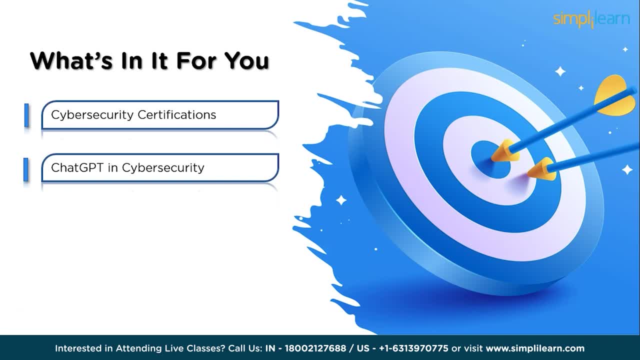 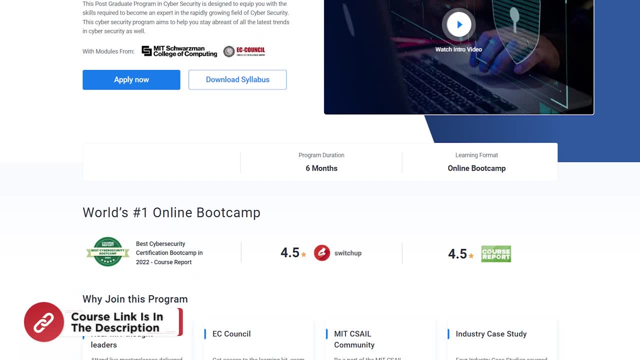 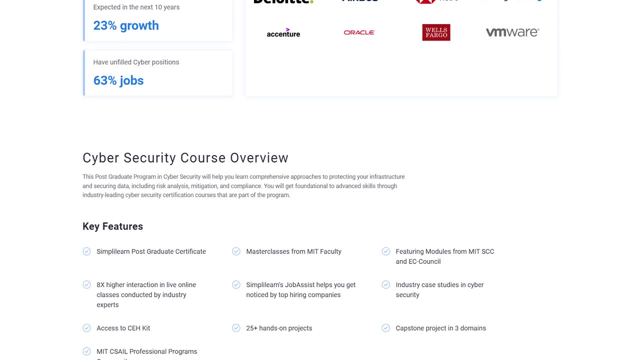 information helpful. don't forget to give this video a thumbs up and subscribe to our channel for more cyber security videos. and if you are someone who is interested in building a career in cyber security, that is, by graduating from the best universities or a professional well assets to switch careers with cyber security by learning from the experts. 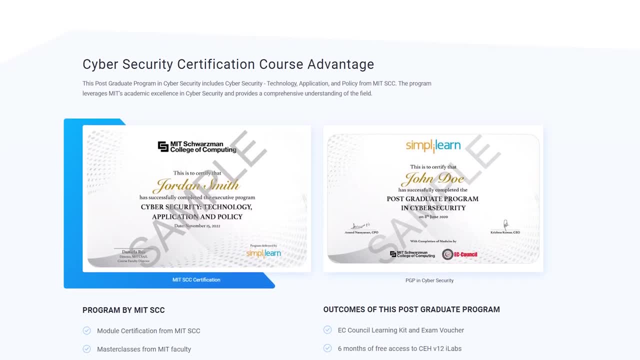 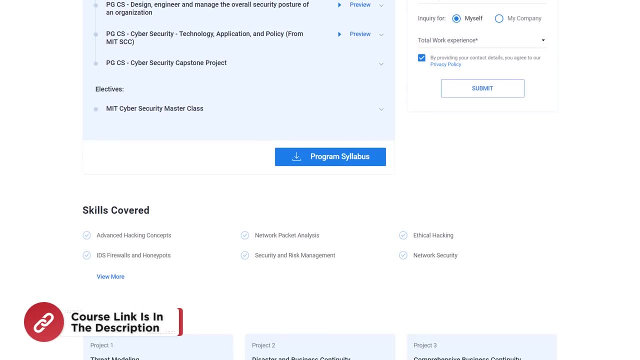 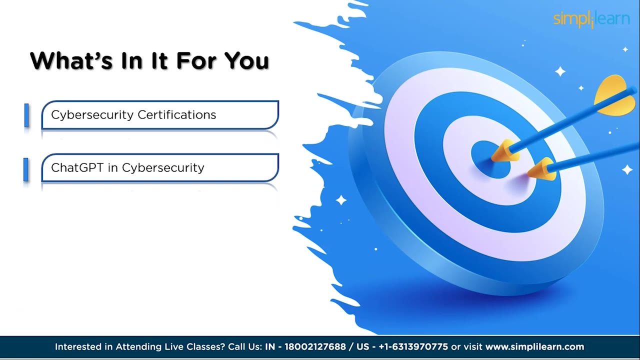 then try giving a shot to simply learn postgraduate program in cyber security with modules from the mit schwartzman college of engineering, and the course link is mentioned in the description box. that will navigate you to the course page, where you can find a complete overview of the program being offered. and now let's take a minute to hear from our learners. 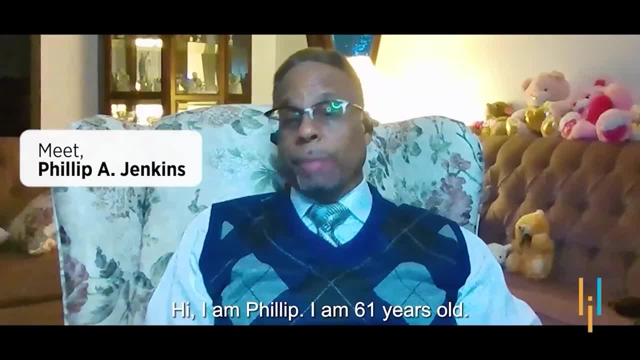 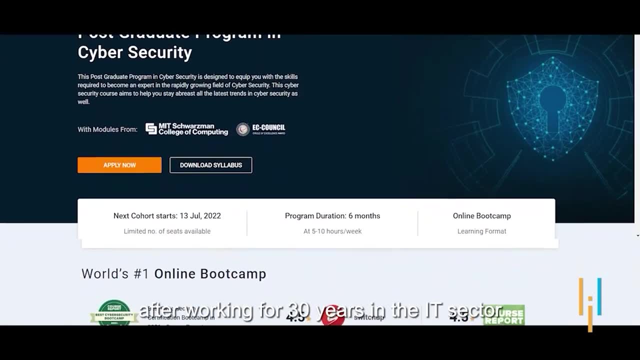 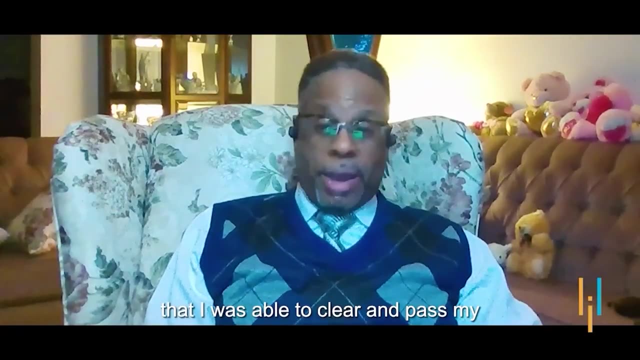 who have experienced massive success in their careers. hi, i'm philip. i'm 61 years old and last year i upskilled with simply learn's postgraduate program in cyber security. after working 30 years in the it sector in various different profiles, i'm happy to tell you that i was able to clear and pass my cissp and ccsp certification exams. 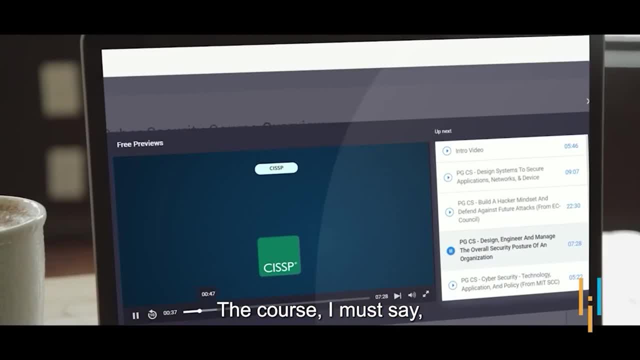 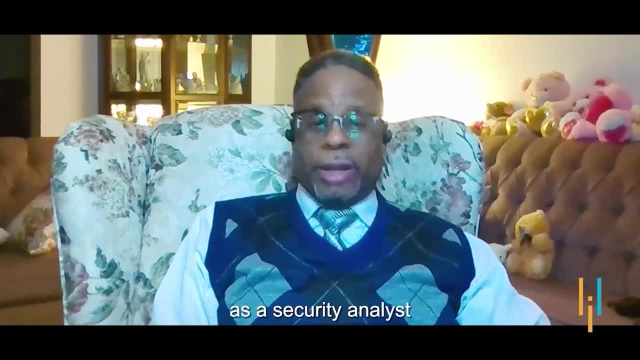 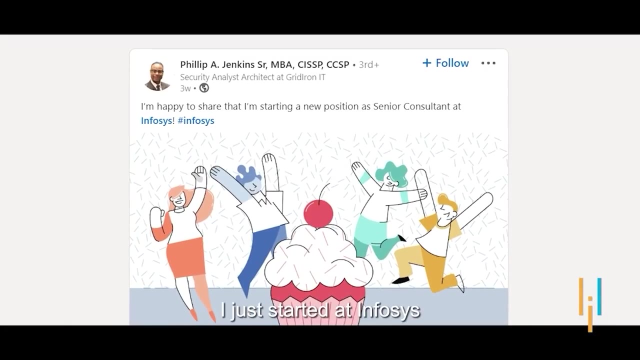 on the first attempt after taking the course, course, i must say, was packed with practical examples. it was led by highly skilled certified instructors with many companies before, security analysts and the architect on a contract basis. but i needed some stability, which i got with the job i just started with. 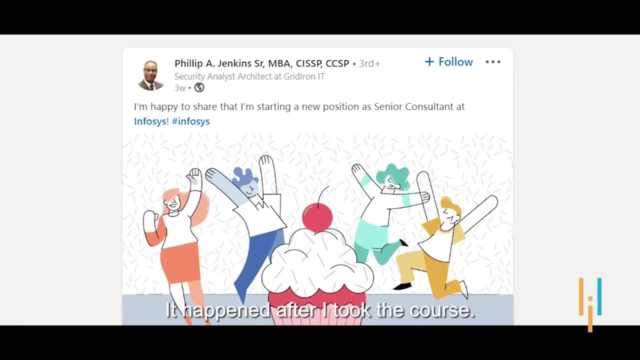 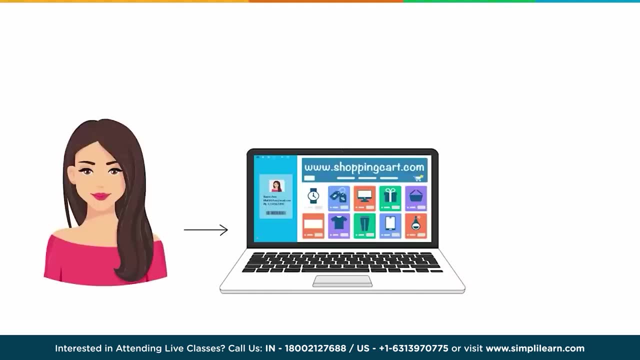 infosys as a cyber security consultant happened on a first meet ann. she often shops from wwwshoppingcartcom. she has her information, like email id address and credit card details, saved on the website to enable a faster and hassle-free shopping experience. the required information is stored in a server. 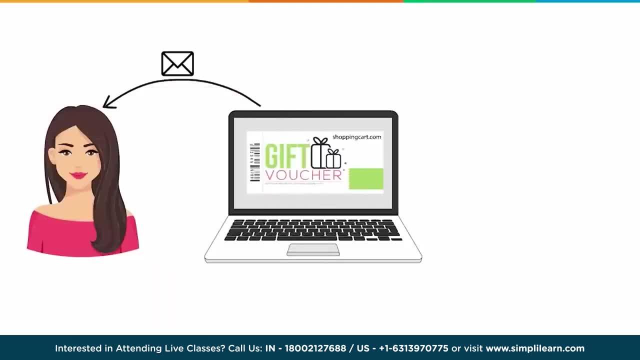 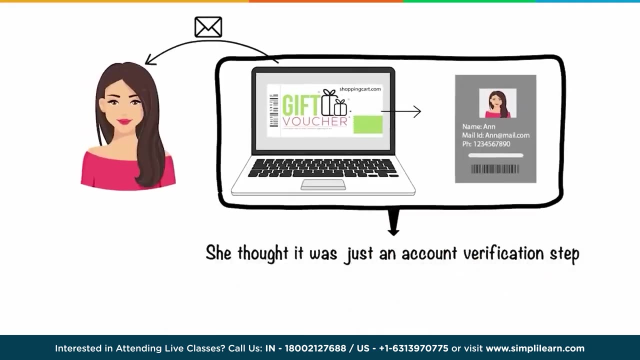 and an email with a written question mark as the email address and a free email for learning the process from the source. she then sent her two students to the cyber security agency where they would get a free, free newsletter each day for the school of business and finance. this process were scheduled to finish on monday and 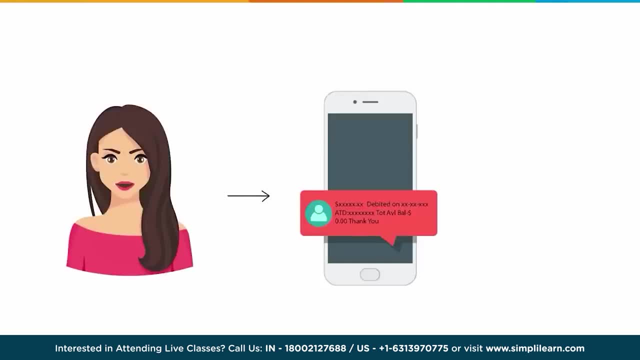 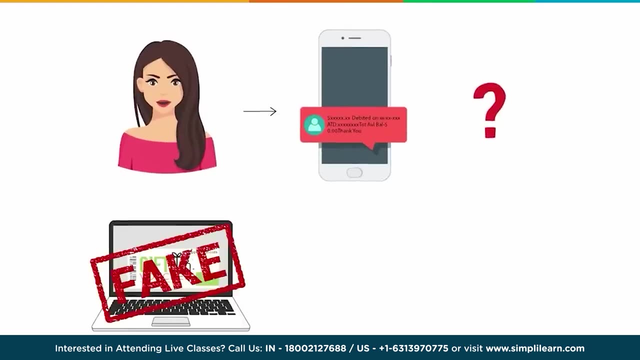 received an email which stated her eligibility for special discount voucher from shopping cartcom. in order to receive the coupon code, she was asked to fill in her shopping cartcom account credentials. happened, Well, yes, the email she received was fake. Ann's shoppingcartcom account witnessed unauthorized access from a third party. This 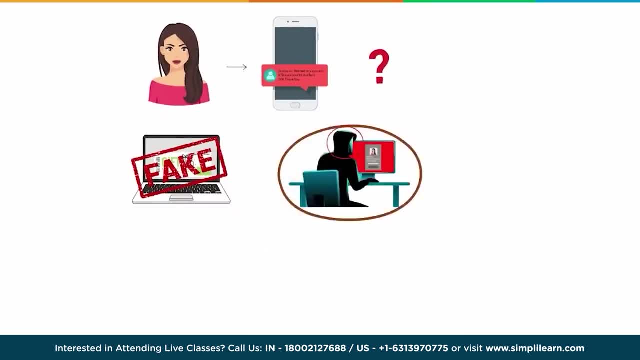 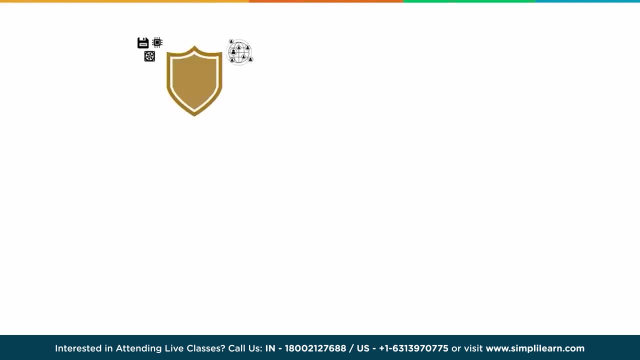 type of attack is known as a cyber attack, and the person who carries it out is called a hacker. Could Ann have prevented this attack? Indeed, she could have with the help of cybersecurity. Cybersecurity involves techniques that help in securing various digital components, networks, data and computer systems from unauthorized 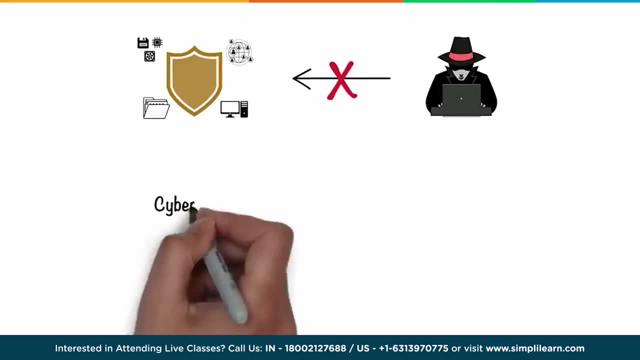 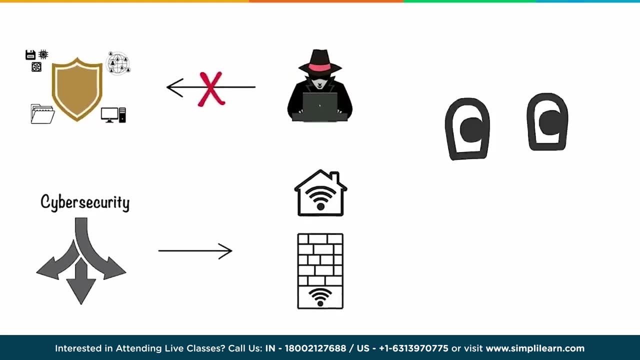 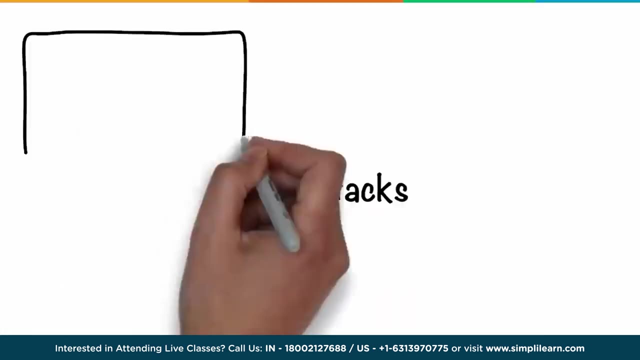 digital access. There are multiple ways to implement cybersecurity, depending on the kind of network you are connected to and the type of cyber attacks you are prone to. So let's take a look at the various cyber attacks that Ann could have been exposed to. One of the most common types of cyber attacks is a malware attack like Trojan, Adware and 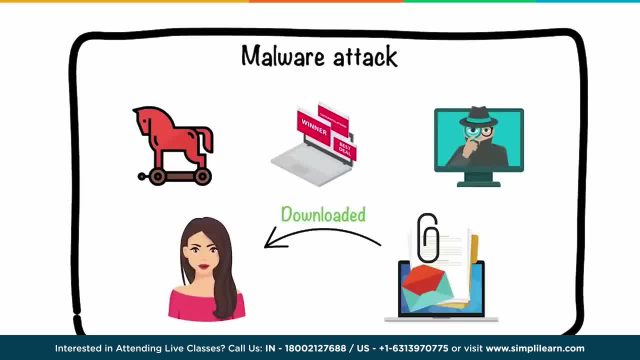 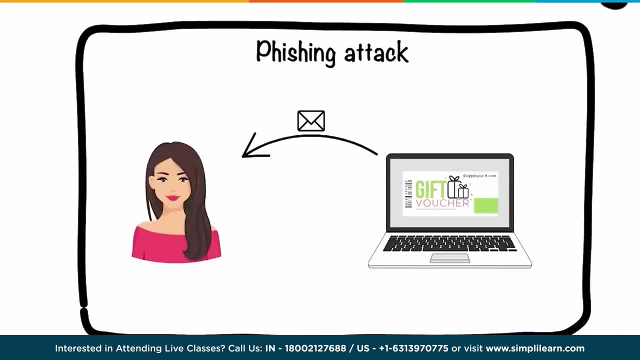 Spyware, to name a few. Had Ann downloaded any suspicious attachments online, her system could have gotten corrupted by certain malicious viruses embedded within the attachments. Next is a phishing attack, the type of cyber attack which Ann experienced Here. the hacker usually sends fraudulent emails which appear to be coming from a legitimate source. This 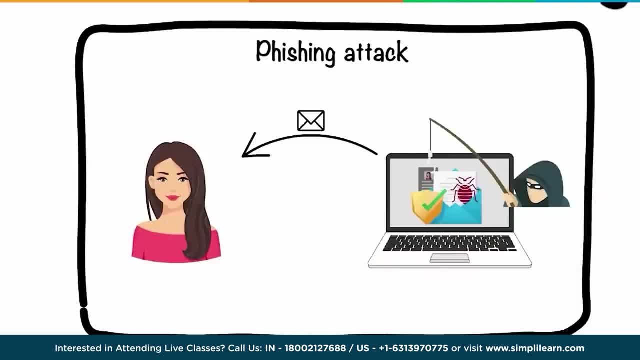 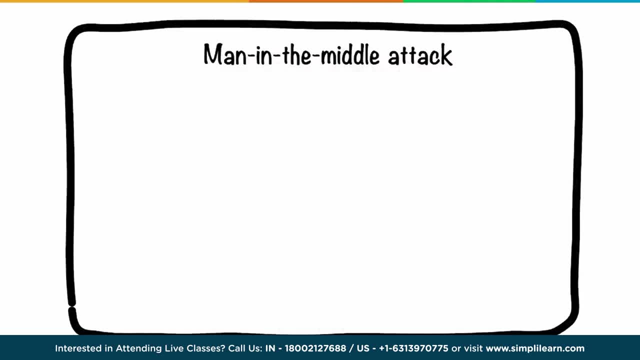 is done to install malware or to steal sensitive data like credit card information and login credentials. Another type of attack is the man-in-the-box attack. This is the type of cyber attack that Ann has been exposed to since she was a child. Here, the hacker gains access to the information. 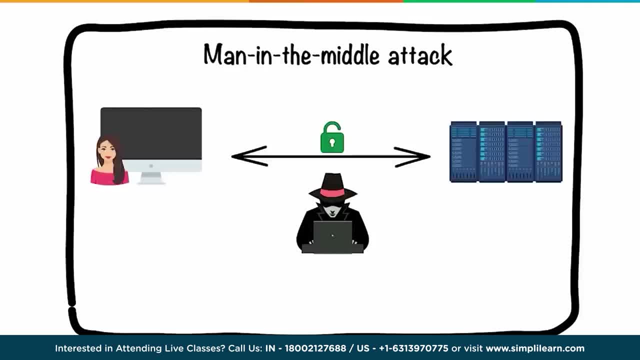 path between Ann's device and the website's server, The hacker's computer takes over Ann's IP address. By doing so, the communication line between Ann and the website is secretly intercepted. This commonly happens with unsecured Wi-Fi networks and also through malware. 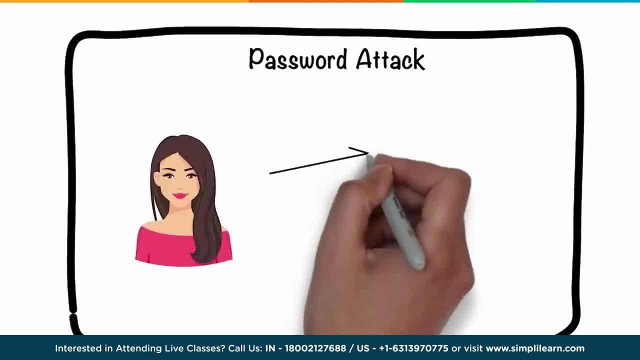 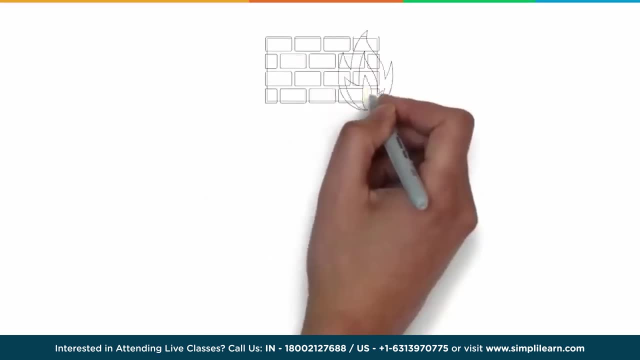 Password attack is one of the easiest ways to hack a system. Here Ann's password could have been cracked by using either common password or a secret password. To prevent future cyber attacks, Ann sought to implement a few cybersecurity practices. First, she installed a firewall. As the name suggests, it is a virtual wall between Ann's 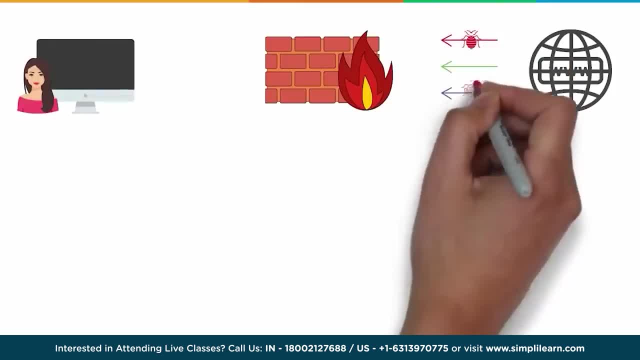 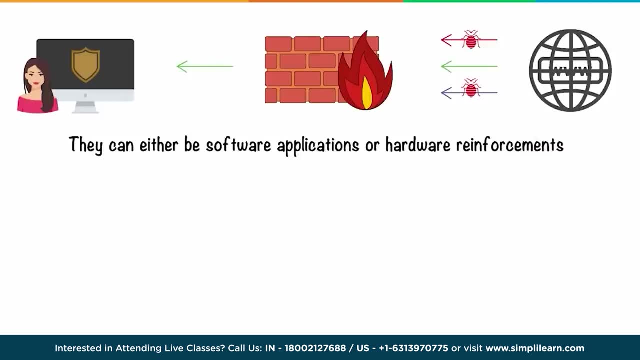 computer and the internet. Firewalls filter the incoming and outgoing traffic from your device to safeguard your network, and they can either be software applications or hardware reinforcements. Secondly, Ann implemented honeypots. Just like how flowers attract bees, dummy computer systems called honeypots are used. 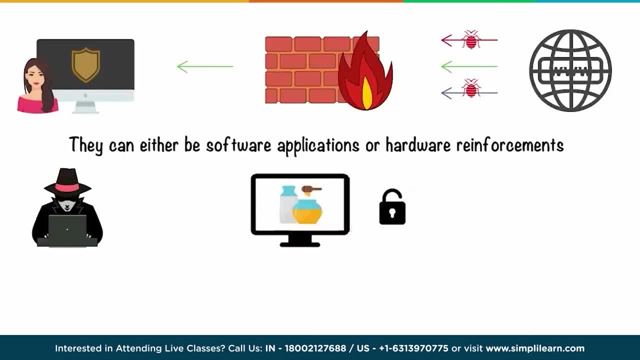 to attract attackers. These systems are made to look vulnerable in order to deceive attackers, and this, in turn, defends the real system. In addition to these, she also decided to use unique alphanumeric passwords, antivirus software and started avoiding mails from unknown senders. 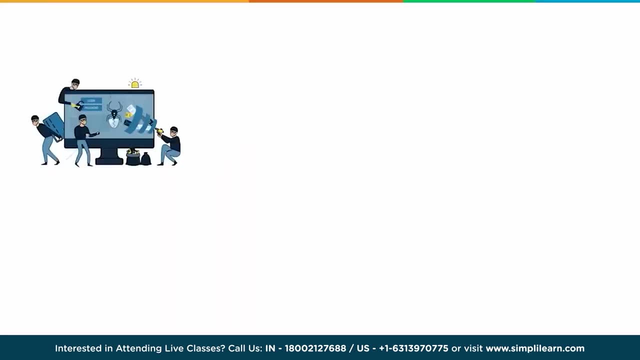 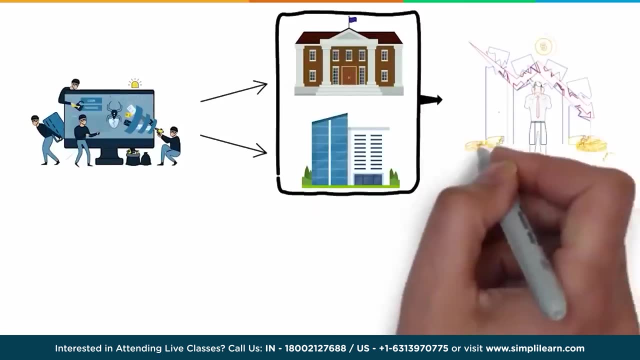 That was Ann's story. Cyber attacks are not just confined to individuals. They can also be used as a means to protect people from the threat of cyber attacks. The cyber attacks carried out in such places are more deadly and they result in colossal losses. 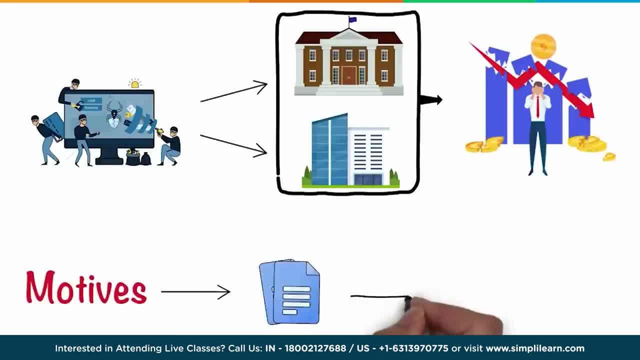 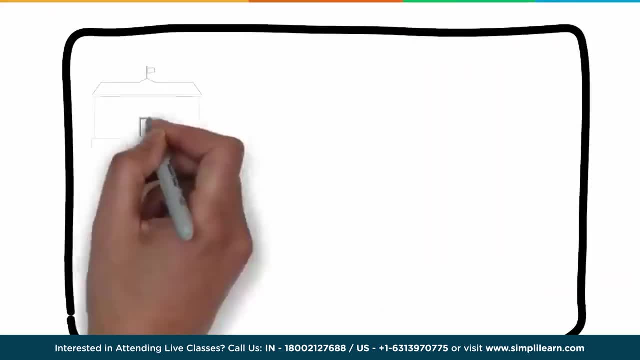 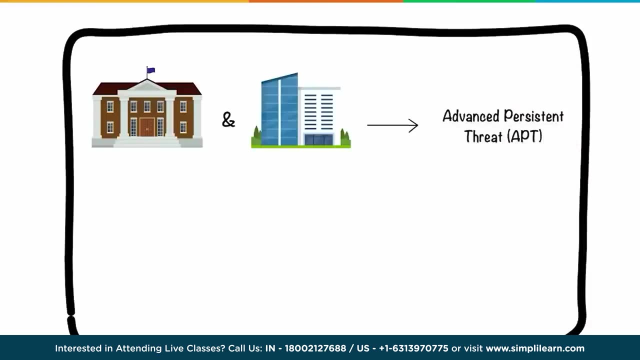 Motives of such attacks are many, starting from tampering with crucial data to monetary gains. Let's have a look at a few of the cyber attacks that companies are subjected to. Various public sector organizations and large corporations face the Advanced, Persistent Threat In this form of attack. hackers gain access to the internet. 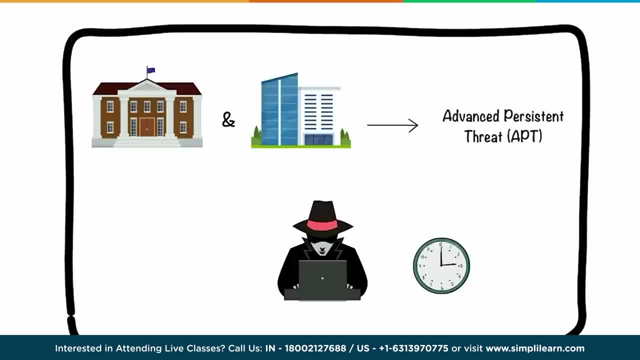 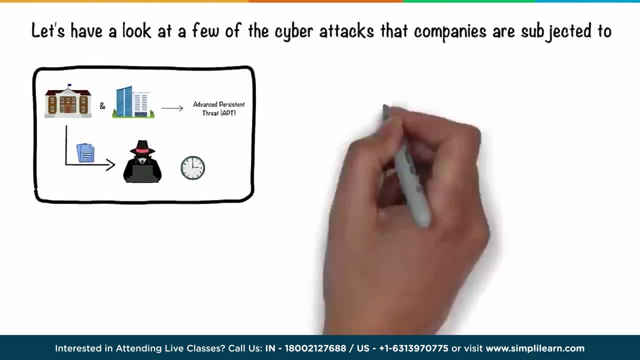 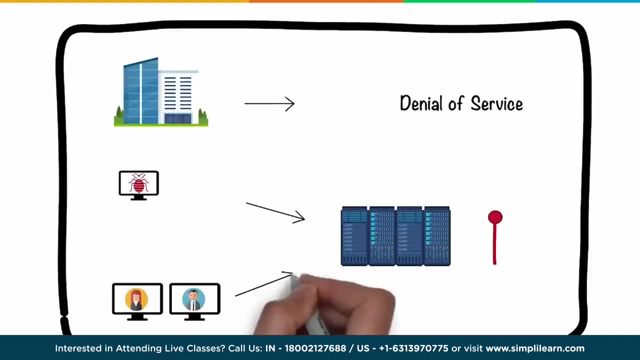 for a prolonged period in order to continuously gain confidential information. Companies also witnessed the denial-of-service attack, where networks are flooded with traffic, which, in turn, leaves legitimate service requests unattended. A variant of this is the Distributed Denial of Service attack, when multiple systems 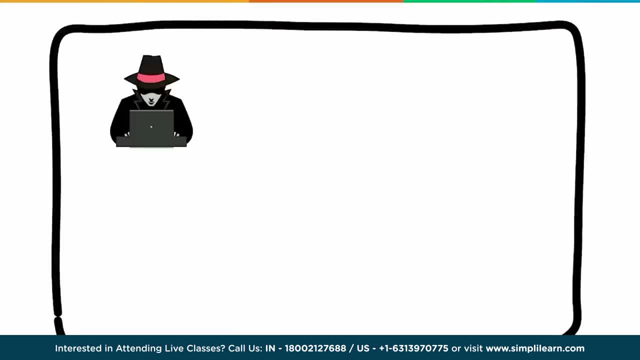 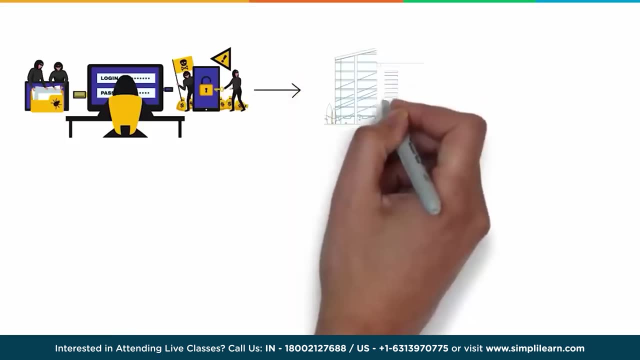 are used to launch the attack. When a hacker manipulates a standard SQL query in a database-driven website, it is known as an SQL injection attempt injection attack. By doing so, hackers can view, edit and delete tables from databases. Amidst a plethora of cyber attacks, it is indeed a challenge for organizations with 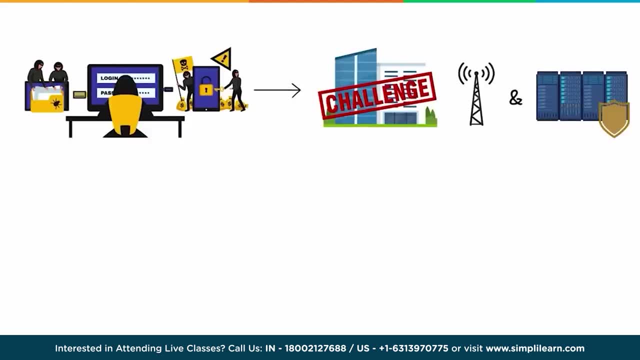 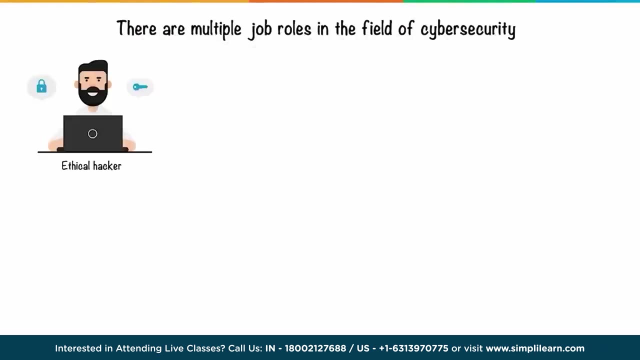 several networks and servers to ensure complete security. This is not an easy task, and to help with this, cybersecurity professionals are hired to work on identifying cyber threats and securing a company's network. There are multiple job roles in the field of cybersecurity If hacking fascinates. 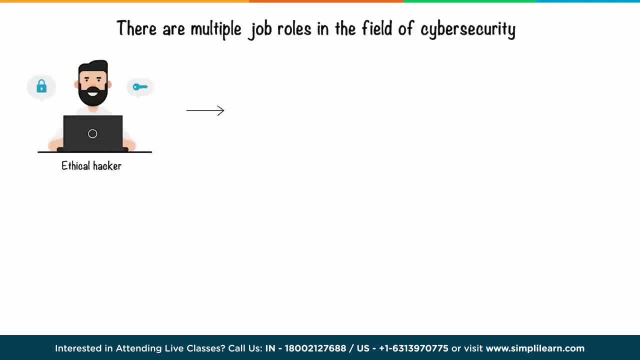 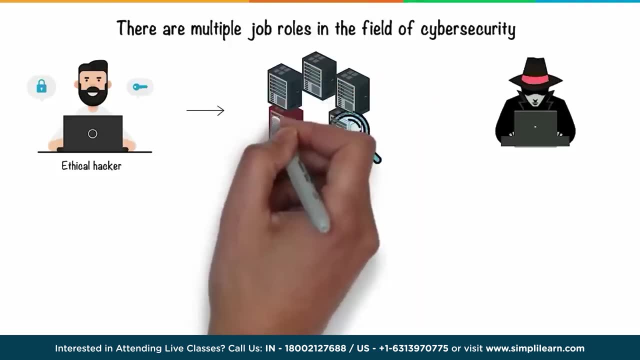 you, then the role of an ethical hacker is something to be explored. Such professionals try to explain a network's vulnerabilities just like how a hacker would do, but only to identify those vulnerabilities and resolve them for protection against an actual cyber attack. But if you are looking to design robust security structures, then the role of a security architect. 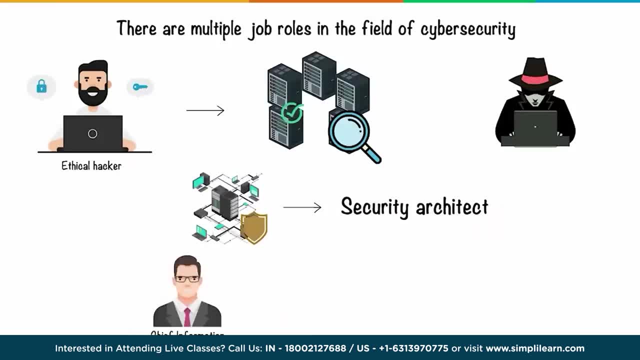 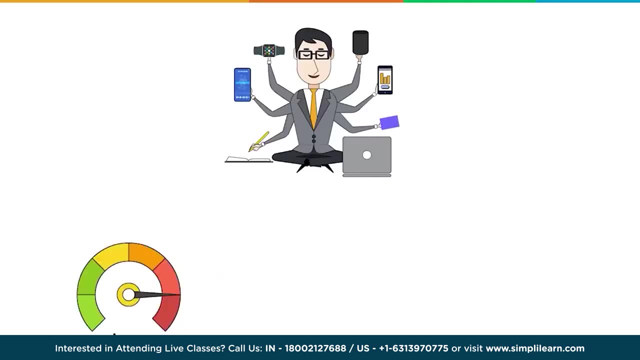 is more apt. A chief information security officer, CISO, plays a crucial role in enterprise security and is entrusted with the role of a security architect. We humans are highly tech-savvy in today's times, With the extensive use of the internet and modern. 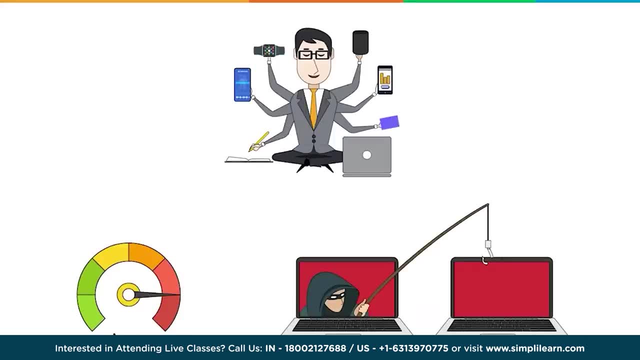 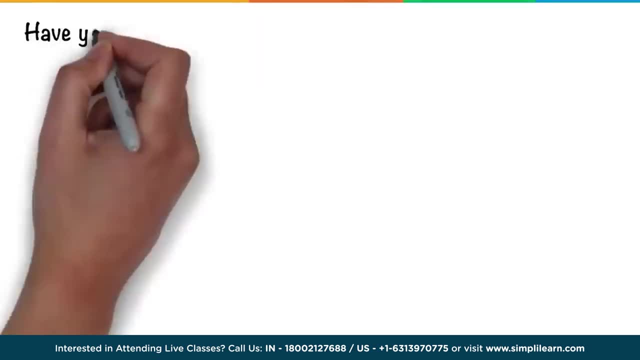 technologies. there is a massive challenge in protecting all our digital data, such as net banking information, account credentials and medical reports, to name a few. Have you heard about the deadly WannaCry ransomware attack? The attack happened in May 2017 in Asia. 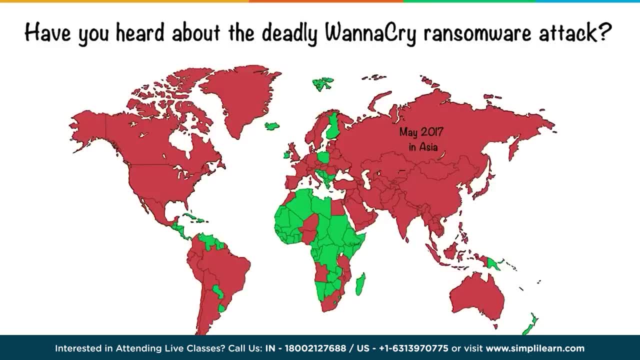 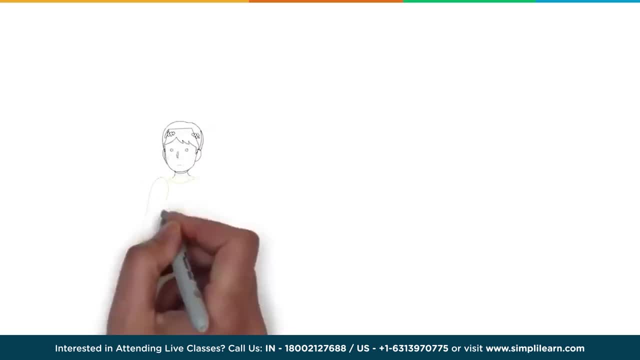 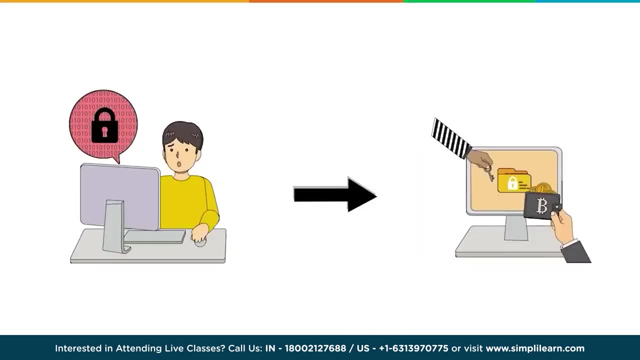 and then it spread across the world. Within a day, more than 230,000 computers were infected across 150 countries. The WannaCry cryptoworm encrypted the data and locked the users out of their systems. For decryption of the data, the users were asked for a ransom of $300 to $600 in Bitcoin. 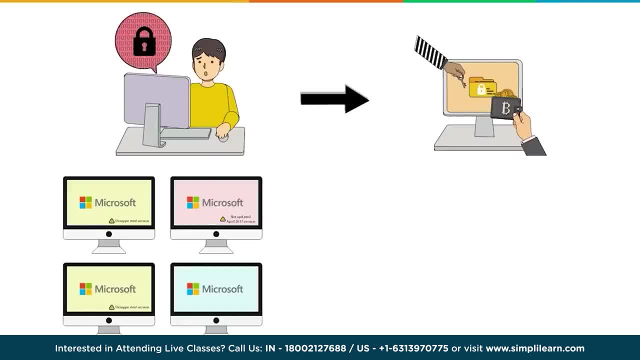 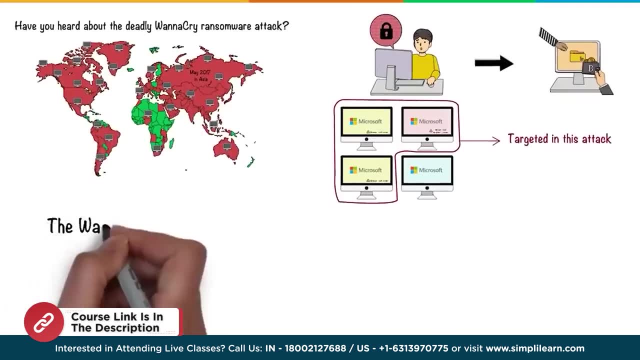 The users who used the unsupported version of Microsoft Windows and those who hadn't installed the security update of April 2017, were targeted in this attack. The WannaCry attack took the strike and it took a toll on every sector: Top tier organizations like Hitachi, Nissan. 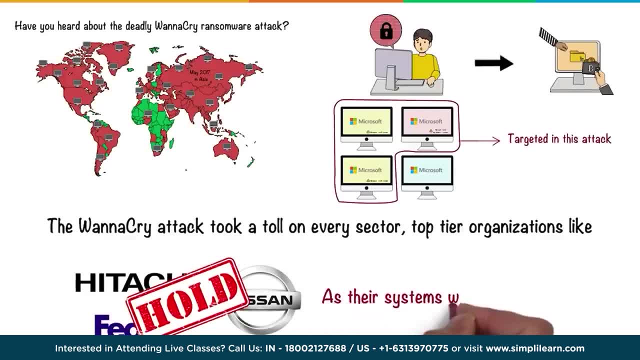 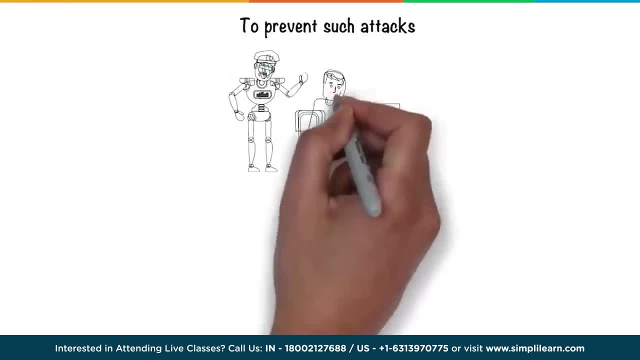 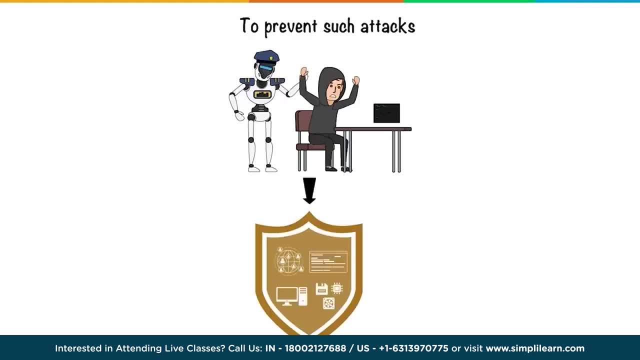 and FedEx had to put their businesses on hold, as their systems were affected too. Now this is what you call a cyberattack. To prevent such attacks, cybersecurity is implemented. We can define cybersecurity as the practice of protecting networks, programs, computer systems and their components from unauthorized 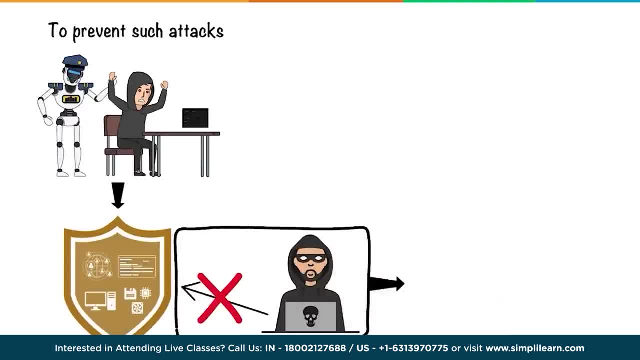 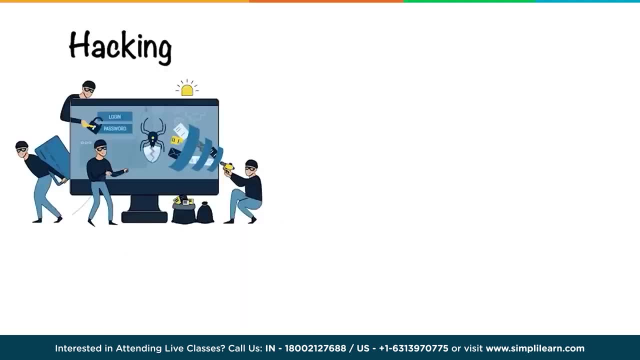 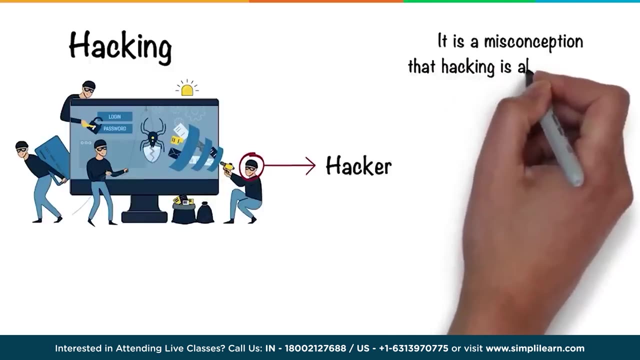 digital attacks. These illegal attacks are often referred to as hacking. Hacking is a. Hacking refers to exploiting weaknesses in a computer network to obtain unauthorized access to information. A hacker is a person who tries to hack into computer systems. This is a misconception that hacking is always wrong. 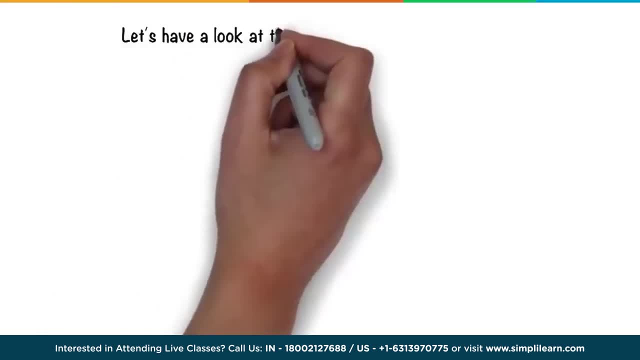 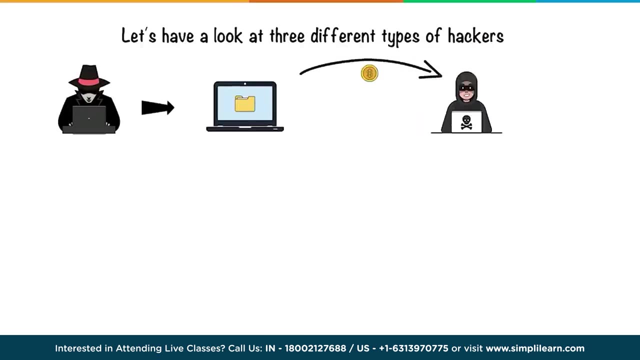 There are hackers who work with different motives. Let's have a look at three different types of hackers. Blackhat hackers are individuals who illegally hack into a system for a monetary gain. On the contrary, we have whitehat hackers, who exploit the vulnerabilities in a system. 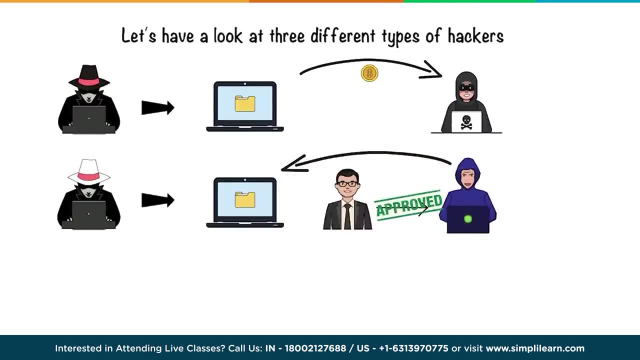 by hacking into it with permission in order to defend the organization. This form of hacking is absolutely legal and ethical. hence they are also often referred to as ethical hackers. In addition to these hackers, we also have the greyhat hackers. As the name suggests, the color grey is a blend of both white and black. 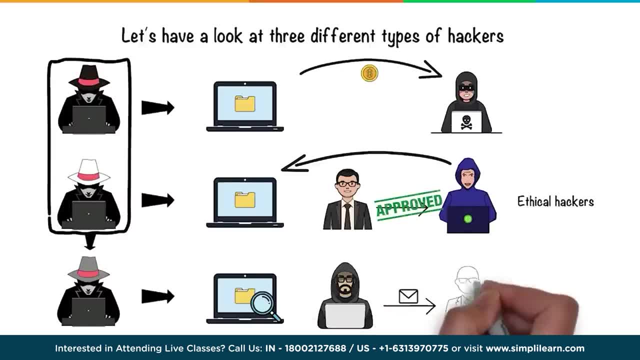 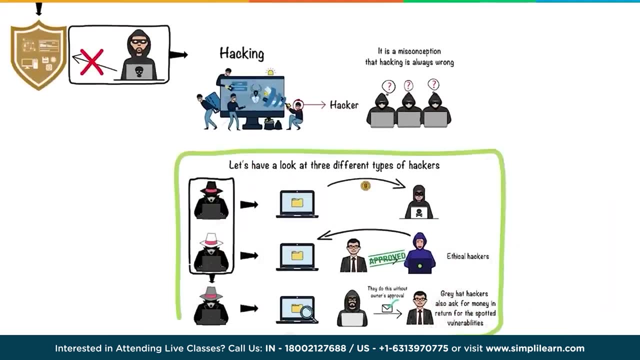 These hackers discover vulnerabilities in a system and report it to the system's owner, which is a good act, But they do this without seeking the owner's approval. Sometimes, greyhat hackers also ask for money in return for the spotted vulnerabilities. Now that you have seen the different types of hackers, let's understand more about. 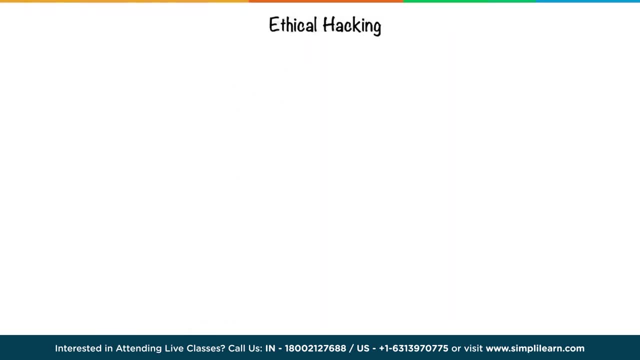 the hacking that is legal and valid ethical hacking. through an interesting story. Dan runs a trading company. He does online trading with the money his customers invest. Everything was going well and Dan's business was booming until a hacker decided to hack. 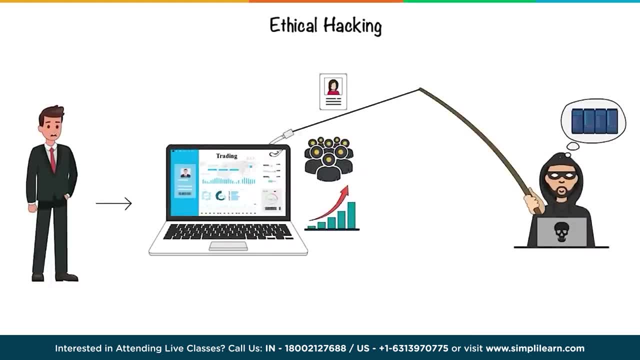 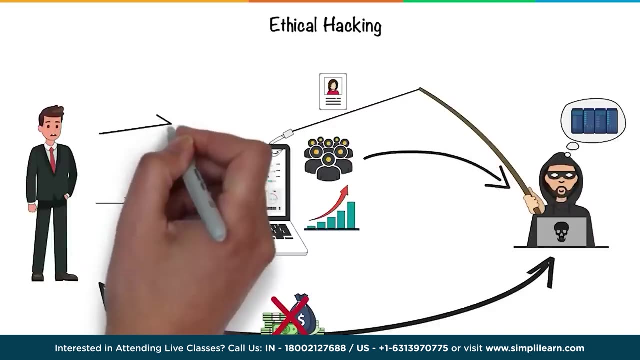 the company's servers. The hacker stole the credentials of various traders. He asked for a lump sum ransom in exchange for the stolen credentials. Dan took the hacker's words lightly and didn't pay the hacker. As a result, the hacker withdrew money from various customers' accounts and Dan was. 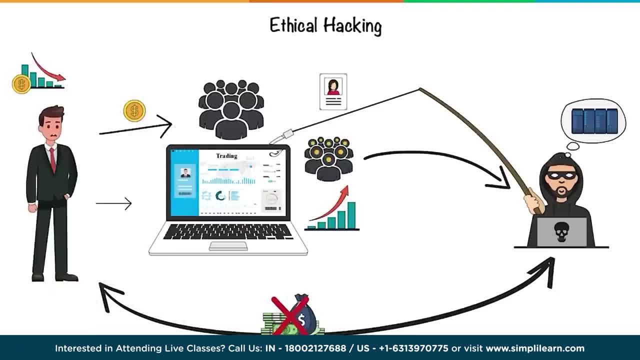 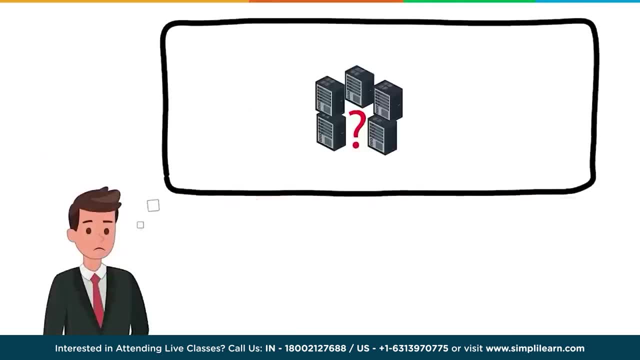 liable to pay back the customers. Dan lost a lot of money and also the trust of his customers. After this incident, Dan gave a lot of thought as to what could have gone wrong with the security infrastructure in his company. He wished there was someone from his company. 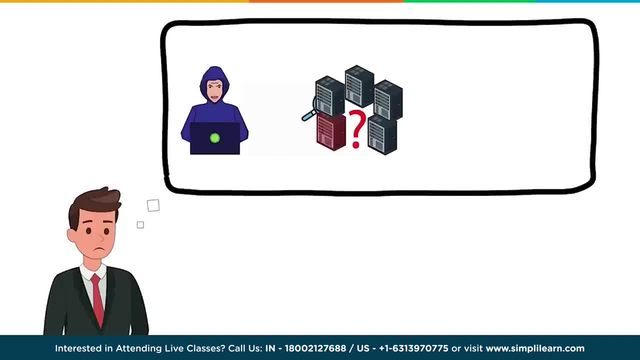 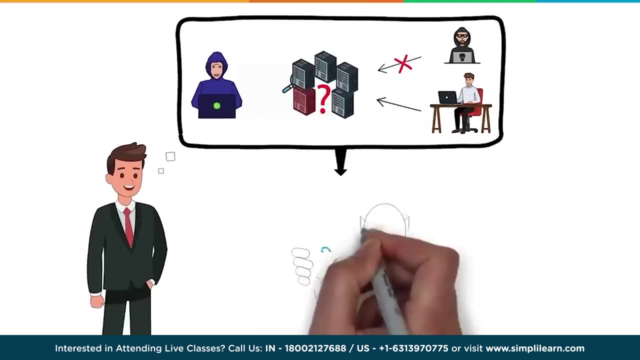 He could have run a test attack to see how vulnerable his systems were before the hacker penetrated into the network. This was when he realized he needed an employee who thinks like a hacker and identifies the vulnerabilities in his network before an outsider does. To do this job, he hired an ethical hacker, John. 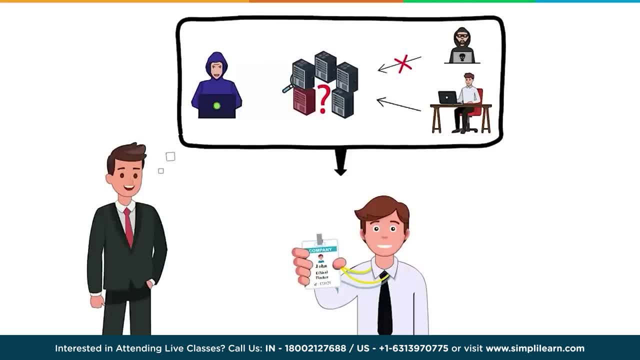 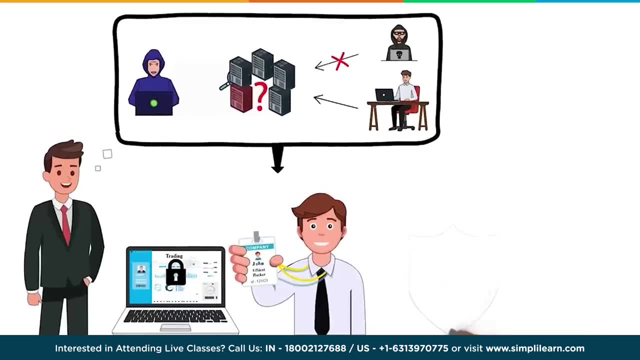 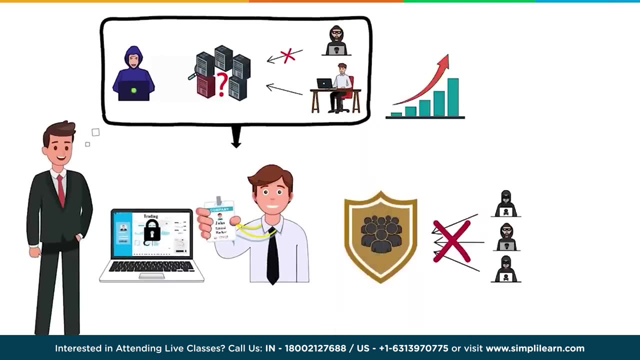 John was a skilled professional who worked precisely like a hacker. In no time he spotted several vulnerabilities in Dan's organization and closed all the loopholes. Hiring an ethical hacker helped Dan protect his customers from further attacks in the future. This, in turn, increased the company's productivity and guarded the company's reputation. 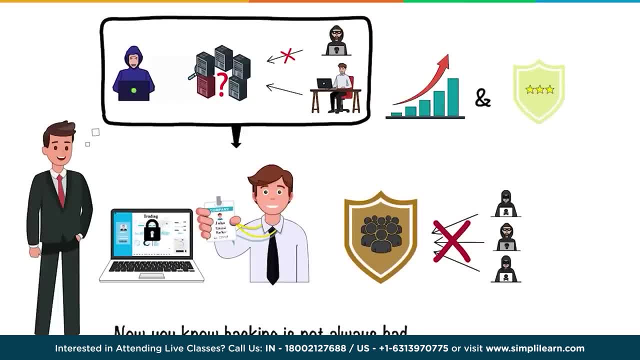 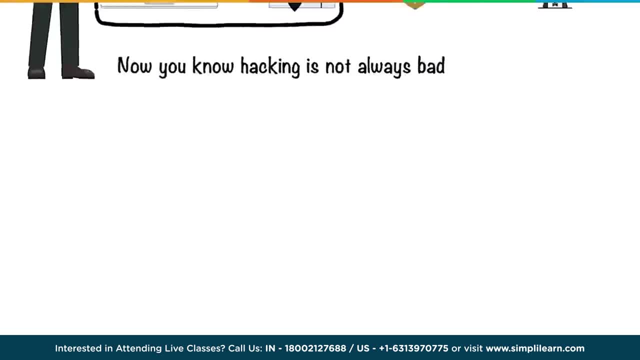 So now you know hacking is not always bad. John, in this scenario, exposed the vulnerabilities in the existing network, and such hacking is known as ethical hacking. Ethical hacking is distributed into six different phases. Let us look at these phases step by step. with respect to a hacker: 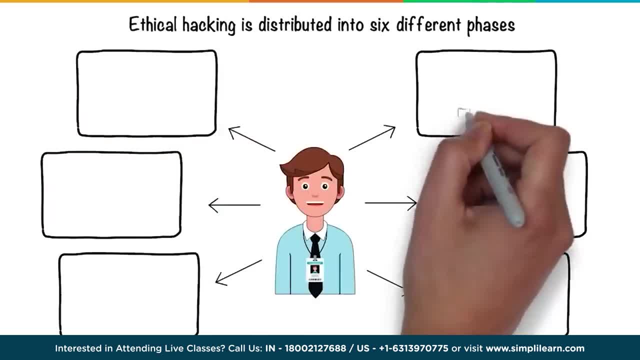 Before launching an attack, the first step John takes is to gather all the necessary information about the organization's system that he intends to attack. This step is called reconnaissance. He uses tools like Nmap and HPing for this purpose. John then tries to spot the vulnerabilities, if any, in the target's system using tools. 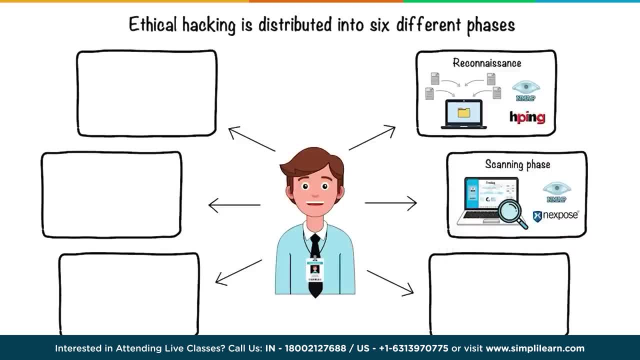 like Nmap and Expose. This is the scanning phase. Now that he has located the vulnerabilities, he can start scanning. He then tries to exploit them. This step is known as gaining access. After John makes his way through the organization's networks, he tries to maintain his access. 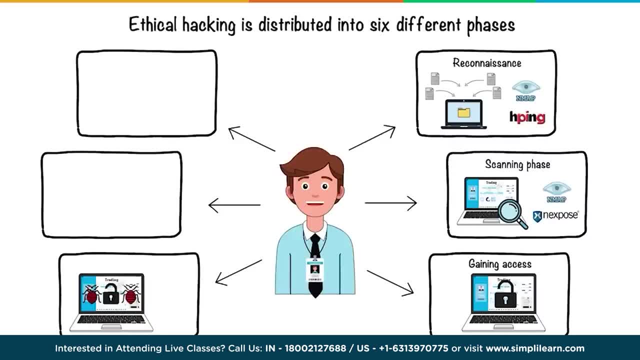 for future attacks by installing backdoors in the target's system. The Metasploit tool helps him with this. This phase is called maintaining access. John is a brilliant hacker, Hence he tries his best not to leave any evidence of his attack. 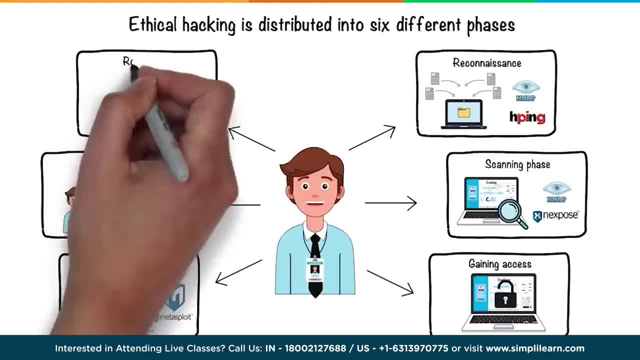 This is the fifth phase, Clearing tracks. We now have the last phase, that is, reporting. In this phase, John documents a summary of his entire attack, the vulnerabilities he spotted, the tools he used and the success rate of the attack. 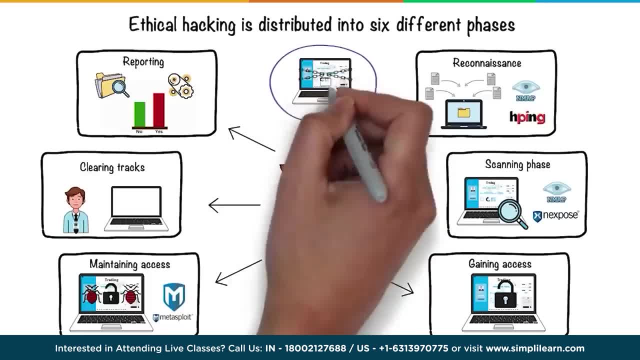 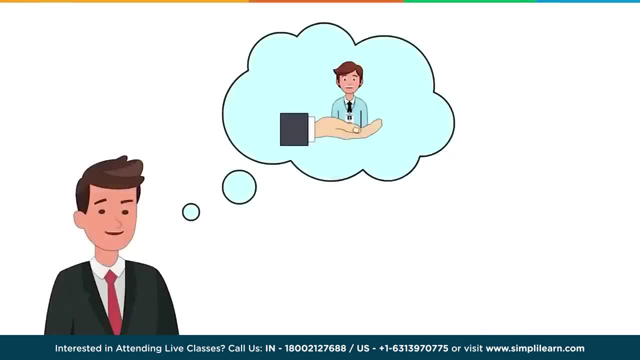 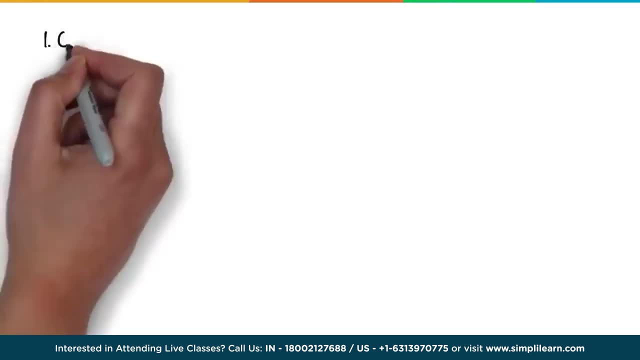 Looking into the report, Dan is now able to take a call and see how to protect his organization from any external cyber attacks. Don't you all think John is an asset to any organization? If you want to become an ethical hacker like John, Then there are a few skills that you need to acquire. 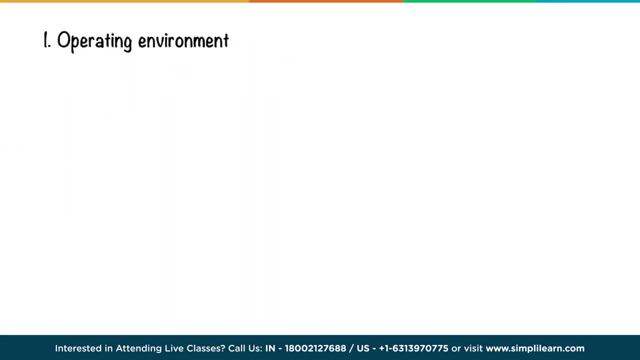 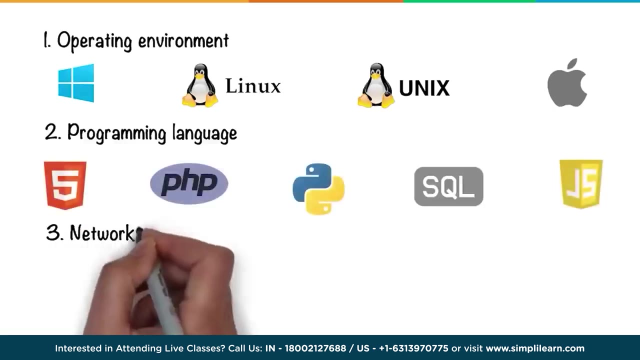 First and foremost, you need to have a good knowledge of operating environments such as Windows, Linux, Unix and Macintosh. You must have reasonably good knowledge of programming languages such as HTML, PHP, Python, SQL and JavaScript. Networking is the base of ethical hacking. 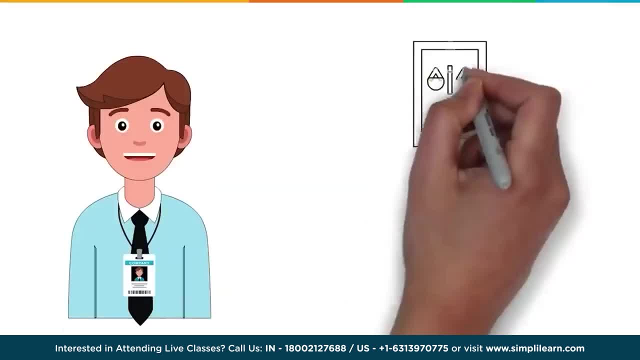 Hence, you should be good at it. Ethical hackers should be well aware of security laws so that they don't misuse it. This is the first step. Then there are a few skills that you need to acquire. First and foremost, you need to have a good knowledge of operating environments, such as: 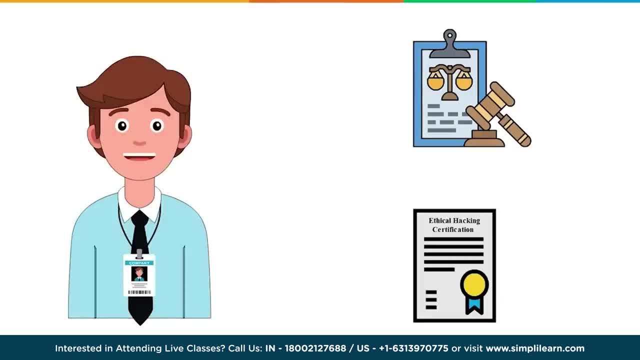 Windows, Linux, Unix and Macintosh. Then there are a few skills that you need to acquire. This is the first step. Then there are a few skills that you need to acquire. This is the first step. Then there are a few skills that you need to acquire. 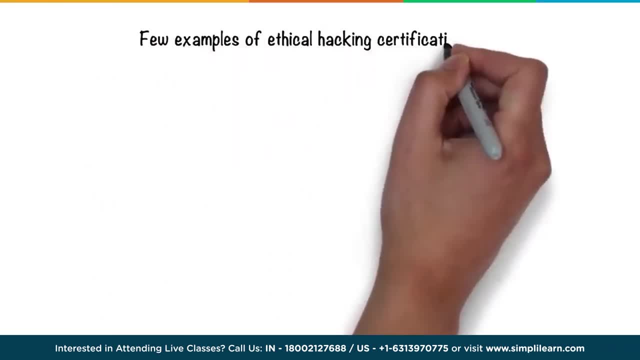 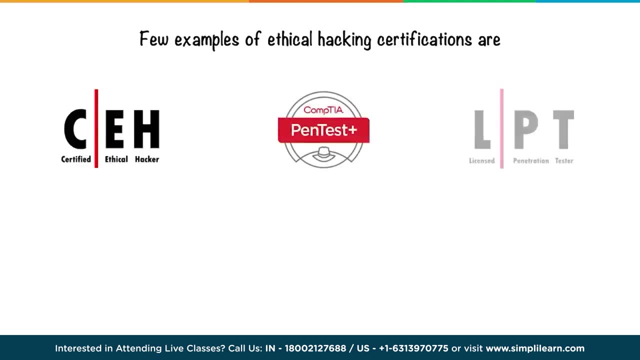 This is the first step. Finally, you must have a Global Certification on Ethical Hacking to successfully bag a position of an ethical hacker like John Few. examples of Ethical Hacking Certification are: Certified Ethical Hacker Certification, CompTIA PenTest Plus and Licensed Penetration Tester Certification. 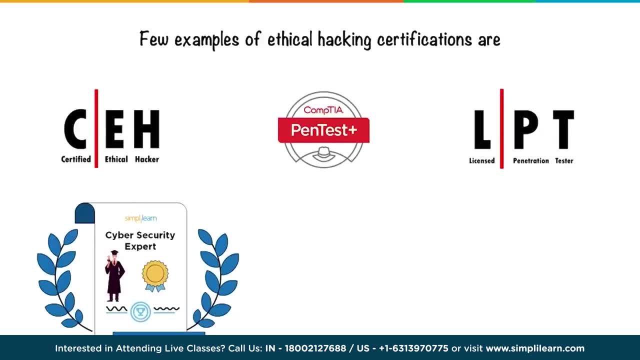 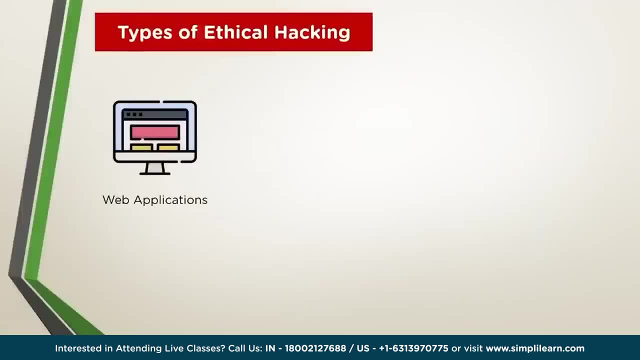 to name a few. SimplyLearn provides a Cybersecurity Expert Master's program that will equip you with all the skills required by a cybersecurity expert. When it comes to web app hacking, it generally refers to the exploitation of applications via HTTP, which can be done by manipulating the applications via its graphical user interface. 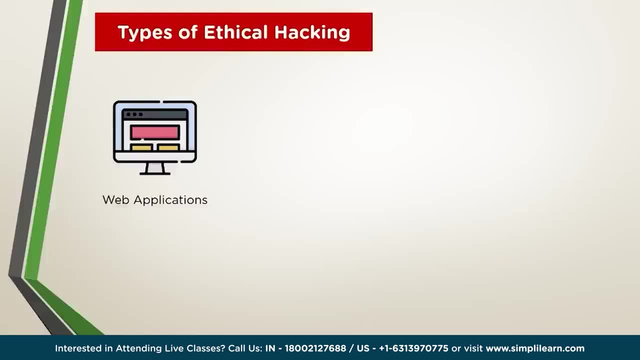 This is done by tampering with the Uniform Resource Identifier, also known as a URI, or tampering with the HTTP elements directly which are not a part of the URI. The hacker can send a link via an email or a chat and matrix the users of a web application. 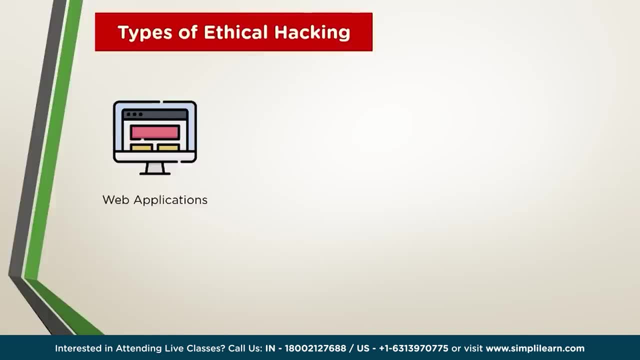 into executing actions. In case the attack is on an administrator account, the entire web application can be compromised. Anyone who uses a computer connected to the internet is susceptible to the threats that computer hackers and online predators pose. These online villains typically use phishing scams, spam email or instant messages, and 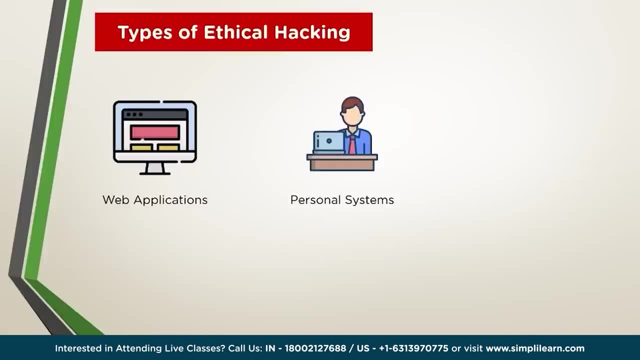 bogus websites to deliver dangerous malware to your computer and compromise your computer security. Computer hackers can also try to access your computer and private information. In case the hacker is on an administrator account, the entire web application can be compromised. The hacker can also try to access your computer and private information directly. if you are 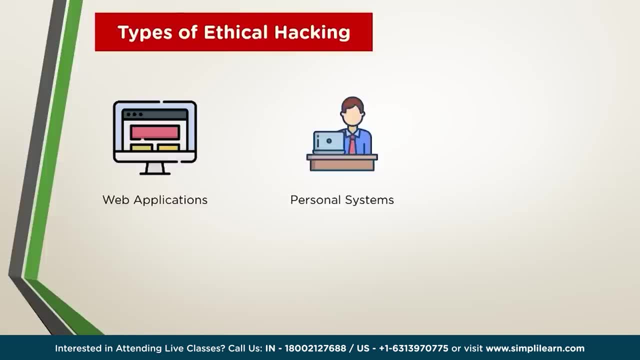 not protected by a firewall. They can monitor your conversations or peruse the backend of your personal website. Usually disguised with a bogus identity, predators can lure you into revealing sensitive personal and financial information. A web server, which can be referred to as the hardware, the computer or the software. 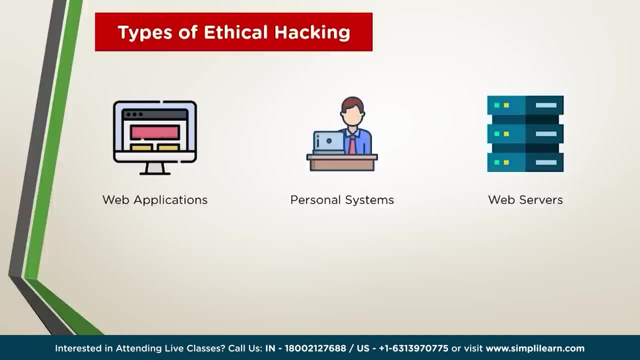 which helps to deliver content that can be accessed through the internet. The primary function of a web server is to deliver these web pages on the request to your clients using the hypertext transfer protocol or HTTP, So hackers attack the web server to steal credential information, passwords and business. 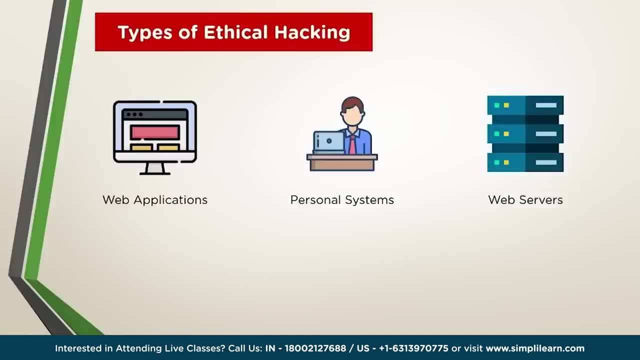 information by using different types of attacks like DDoS attacks, SYN flooding, ping, flood, port scan and social engineering attacks. In the area of web security, despite strong encryption on the browser's server channel, web users still have no assurance about what happens at the other end. 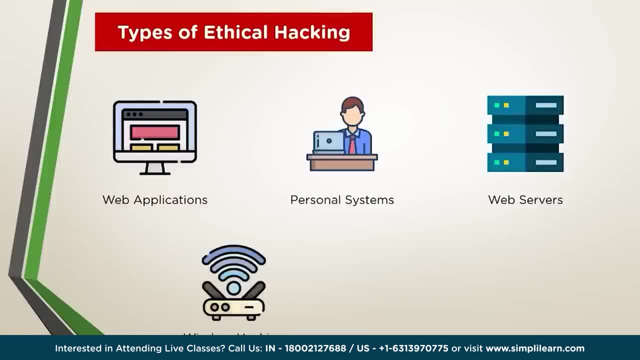 In the area of web security. despite strong encryption on the browser's server channel, web users still have no assurance about what happens at the other end. Although wireless networks can be used to protect users, they can also be used to protect other users. 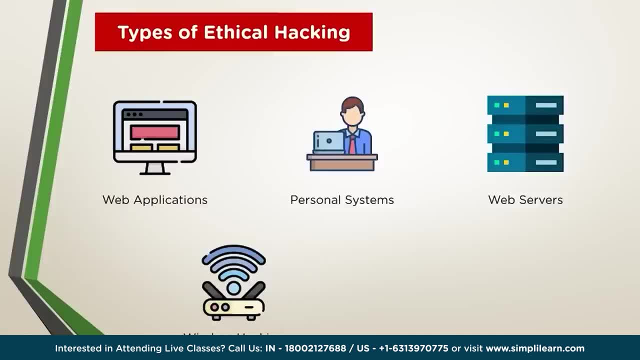 While wireless networks offer great flexibility, they have their own security problems. A hacker can sniff the network packets without having to be in the same building where the network is located. As wireless networks communicate through radio waves, a hacker can easily sniff the network from a nearby location. 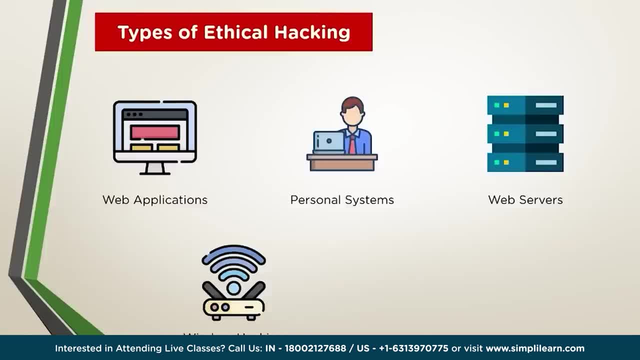 Most attackers use network sniffing to find the SSID and hack a wireless network. An attacker can attack a network from a distance and therefore it is sometimes difficult to collect evidence against the main hacker. Social engineering is the art of manipulating users of a computing system into revealing 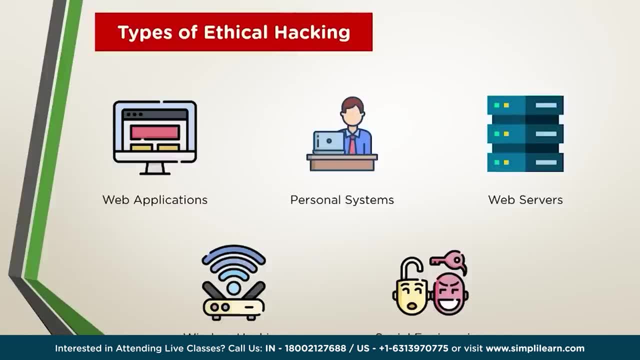 confidential information which can be later used to gain unauthorized access to a computer system. The term can also include activities such as exploiting human kindness, greed and curiosity to gain access to restricted-access buildings, or getting the users to installing backdoor software. Knowing the tricks used by hackers to trick users into releasing vital login information. 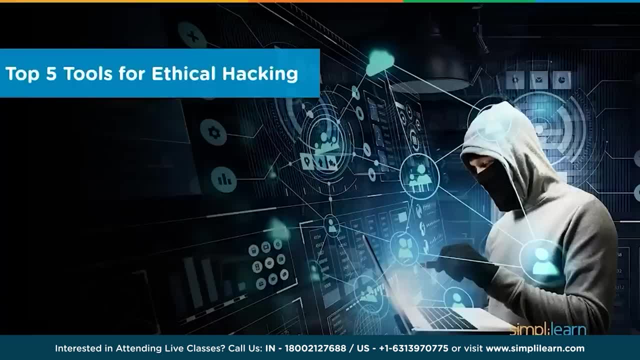 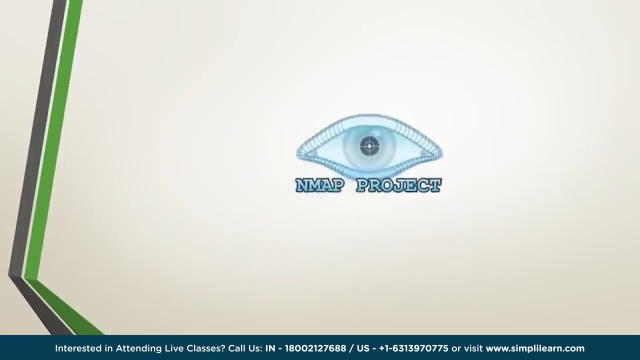 is fundamental in protecting computer systems. Coming to our main focus for today, let us have a look at the top 5 most essential ethical hacking tools to be used in 2021.. Nmap: At the top of the chain lies Nmap. Nmap, which stands for Network Mapper, is a free and open-source utility for network discovery. 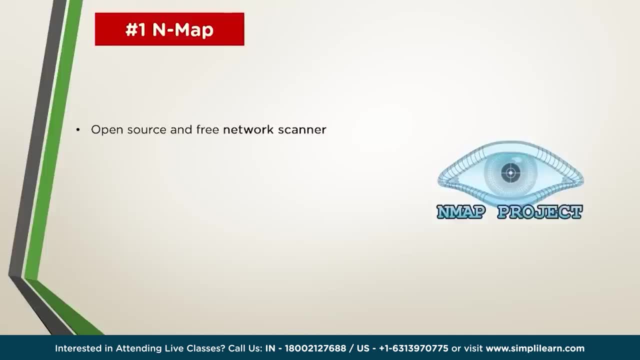 and security auditing. Nmap is a tool that can be used to track and track the security of your network. Many systems and network administrators also find it useful to track and track the security of your network. Nmap can be used to track and track security of your network. 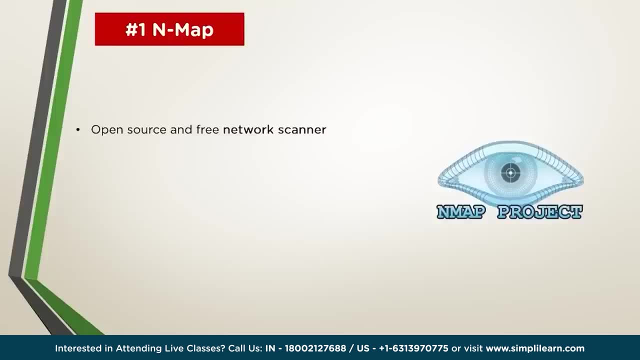 This tool is useful for tasks such as network inventory, managing, service upgrade schedules and monitoring host or service uptime. It is most beneficial in the early stages of ethical hacking, where a hacker must figure the possible entry point to a system before running the necessary exploits, thus allowing 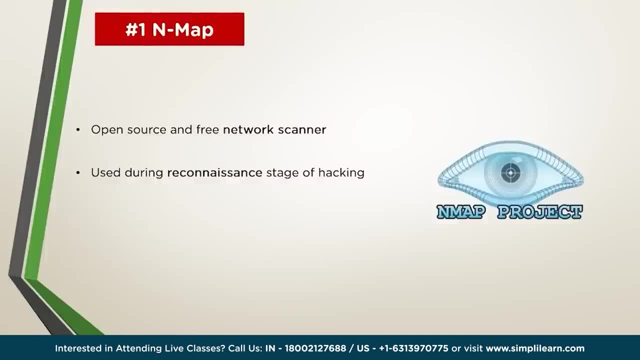 the hackers to leverage any insecure openings and thus breach the device. Nmap uses raw IP packets in novel ways to determine what hosts are available on the network, what service they are running and how much data they need to be used to track data. 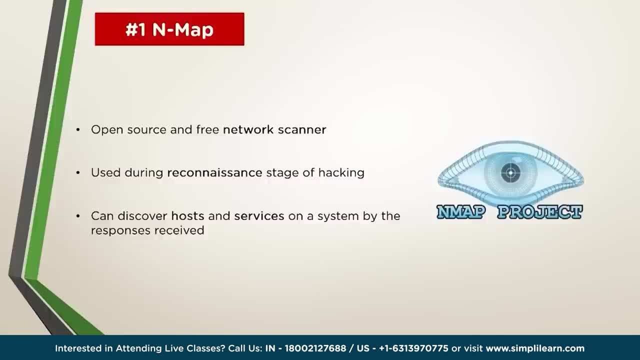 what operating systems are installed, what type of packet filters and firewalls are in use, and dozens of other characteristics. It was designed to rapidly scan large networks, but works fine against single host as well, Since every application that connects to a network needs to do so via a port. the wrong. 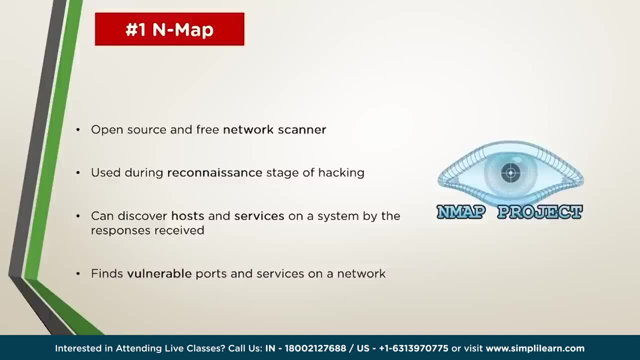 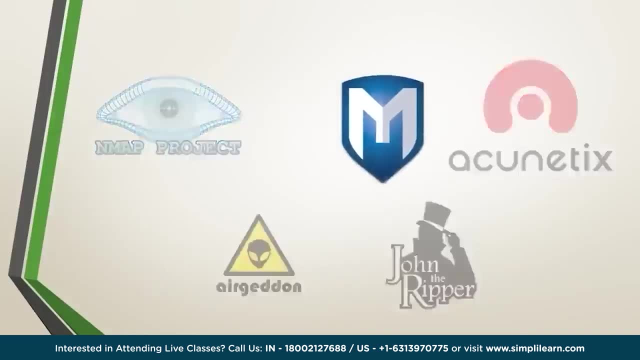 port or a server configuration can open a can of worms, which lead to a thorough breach of the system and, ultimately, a fully hacked device. Next on our list we have Metasploit. The Metasploit framework is a very powerful tool that can be used by cyber criminals as 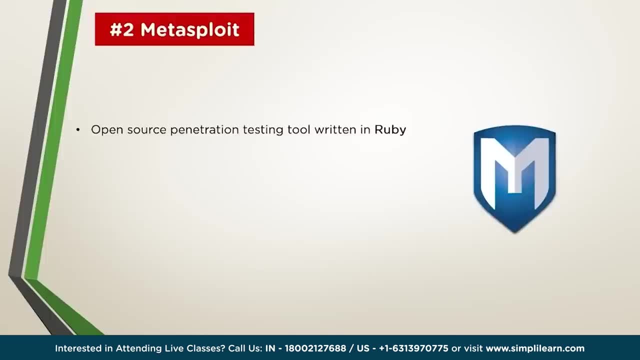 well as ethical hackers, to probe systematic vulnerabilities on both networks and servers. Because it's an open source framework, it can be easily customized and used with most operating systems. With Metasploit, the ethical hacking team can use ready-made or custom code and introduce. 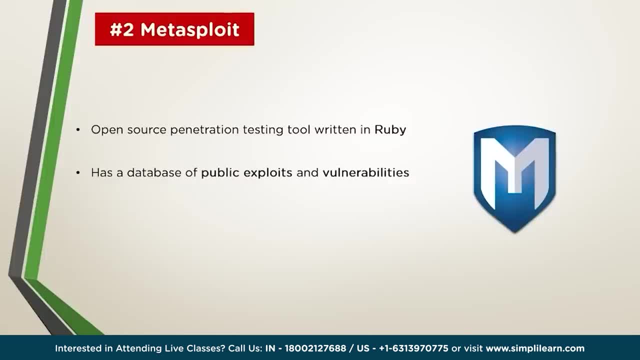 it into a network to probe for weak spots As another flavor of threat hunting. Once the flaws are identified and documented, the information can be used to address systemic weaknesses and prioritize solutions. Once a particular vulnerability is identified and the necessary exploit is fed into the 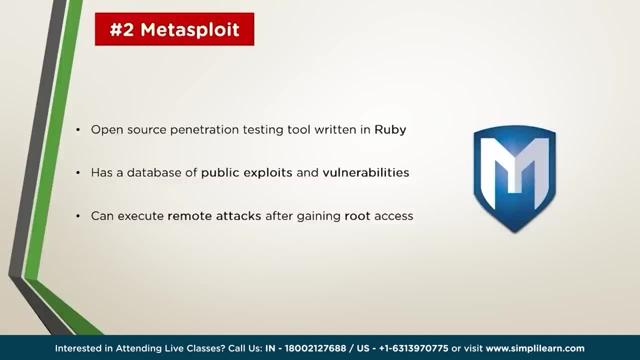 system. there are a host of options for the hacker, Depending on the vulnerability. hackers can even run root commands from the terminal, allowing complete control over the activities of the compromised system, as well as all the personal data stored on the device. A big advantage of Metasploit is that it's easy to use. 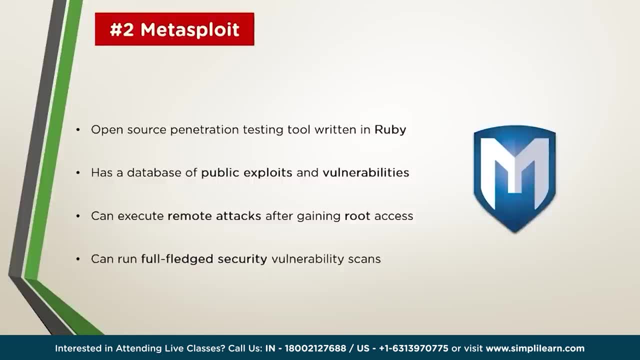 The advantage of Metasploit is the ability to run full-fledged scans on the target system, which gives a detailed picture of the security index of the system, along with the necessary exploits that can be used to bypass the antivirus software. Having a single solution to gather almost all the necessary points of attack is very 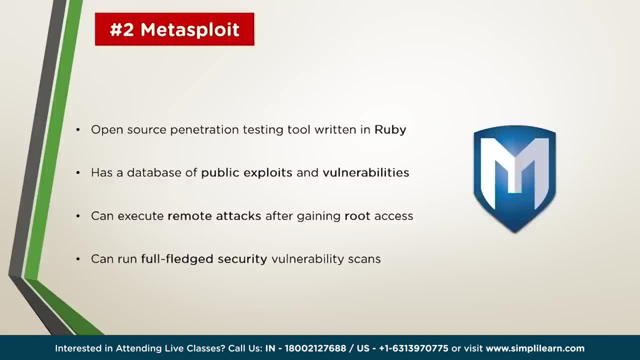 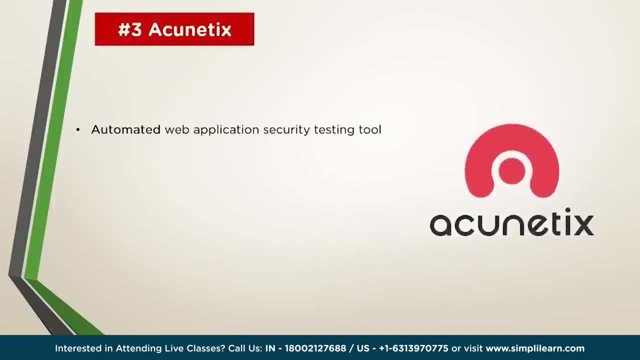 useful for ethical hackers and penetration testers, as denoted by its high rank in the list. Moving on, we have the Acunetix framework. Acunetix is an anti-hacker. It's an end-to-end web security scanner which offers a 360-degree view of an organization's 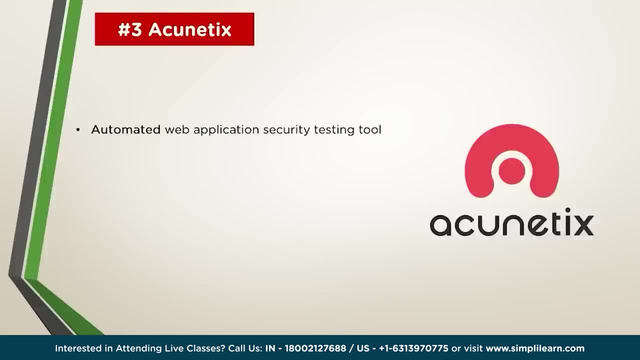 security. It is an application security testing tool that helps the company address vulnerability across all their critical web assets. The need to be able to test applications in-depth and further than traditional vulnerability management tools has created a market with several players in the application security space. 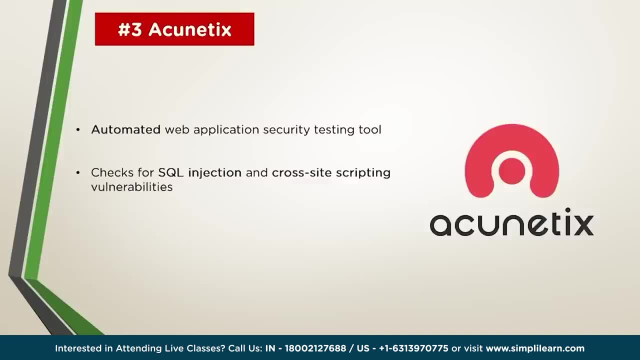 Acunetix can detect over 7,000 vulnerabilities, Including SQL injections, cross-site scripting, misconfigurations, weak passwords, exposed database and other out-of-band vulnerabilities. It can scan all pages, web apps and complex web applications running HTML5 and JavaScript. 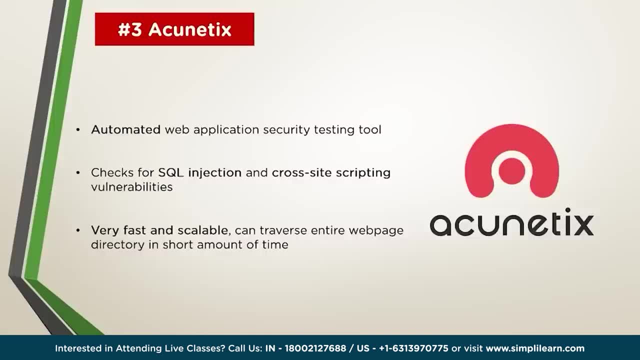 as well. It also lets you scan complex multi-level forms and even password-protected areas of the site. Acunetix is a dynamic application security testing package. It has a lot of features. It has a lot of features. It has a lot of features. 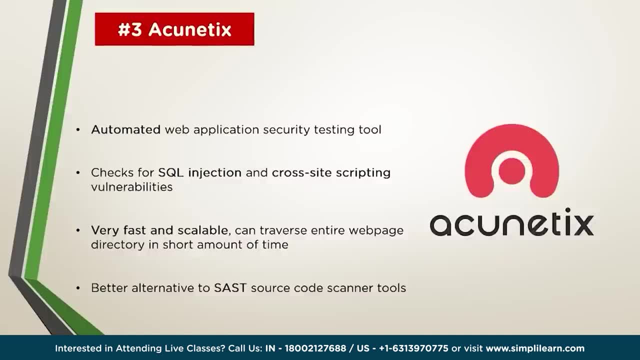 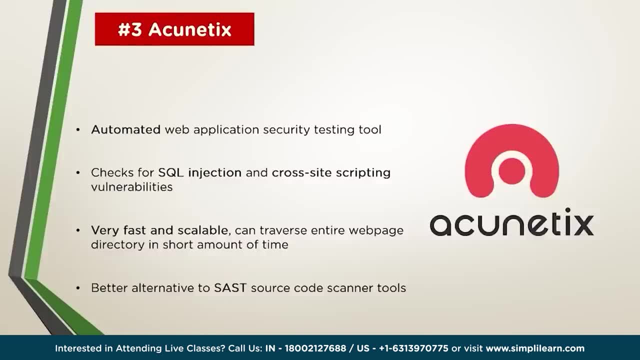 STores, the hooks over status, application security testing frameworks, which are also known as SAST scanners. SAST tools only work during development and only for specific languages, and have a history of reporting a lot of false positives, Whereas dynamic testing tools, also known as DAST, have the ability to streamline testing. 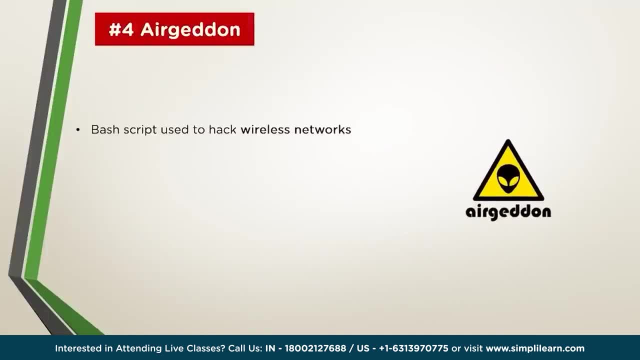 from development to deployment with minimal issues. Next on our list we have taergeddon. Next on our list we have taergeddon. games have installed a multi-use Bash totally within its cript systems to hack and audit wireless networks like our everyday Wi-Fi router and its counterparts. 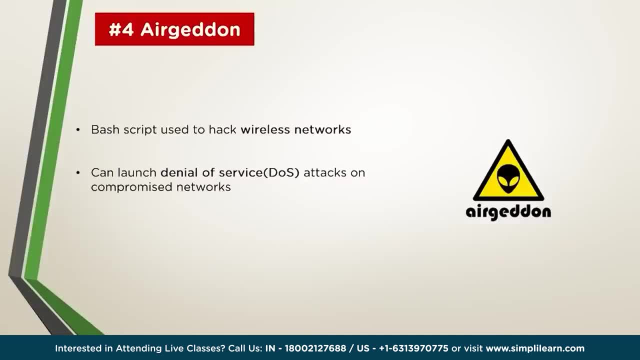 Along with being able to launch denial-of-service attacks on compromised networks, this multipurpose Wi-Fi hacking tool has very rich features which support multiple methods for Wi-Fi hacking, including WPS hacking modes, WP attacks, handshake captures, evil twin and so much more. 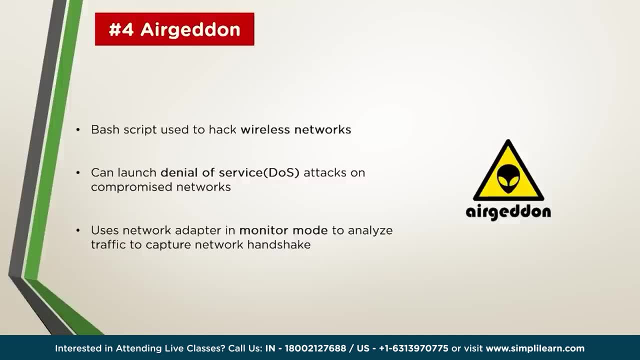 It usually needs an external network adapter that supports monitor mode, which is necessary to be able to capture wireless traffic that traverse the air channels. Thanks to its open-source nature, AirGarden can be used with multiple community plugins and add-ons, thereby increasing its effectiveness against a wide variety of routers, both in 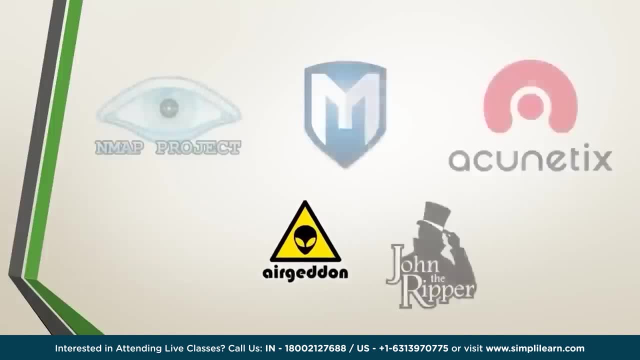 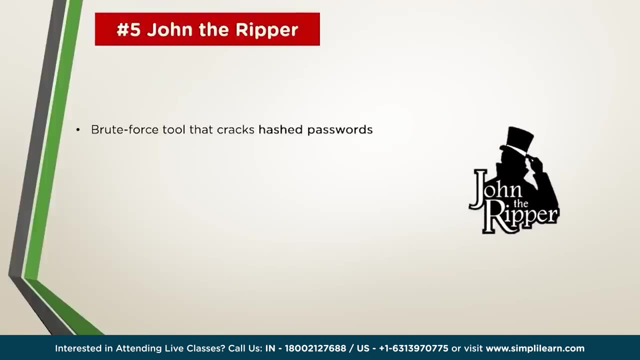 the 2.4 GHz and the 5 GHz band. Finally, at number 5, we have John the Ripper. John the Ripper is an open-source password security auditing and the password recovery tool which is available for many audits. John the Ripper Jumbo supports hundreds of hash and cipher types, including for user passwords. 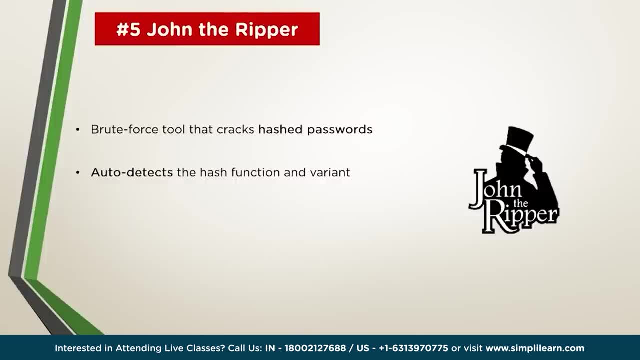 of operating systems, web apps, database servers, encrypted keys and document files. Some of the key features of the tool include offering multiple modes to speed up the password cracking, automatically deselecting the hashing algorithm used by the passwords, and the ease of running and configuring the tool to make password cracking easier. 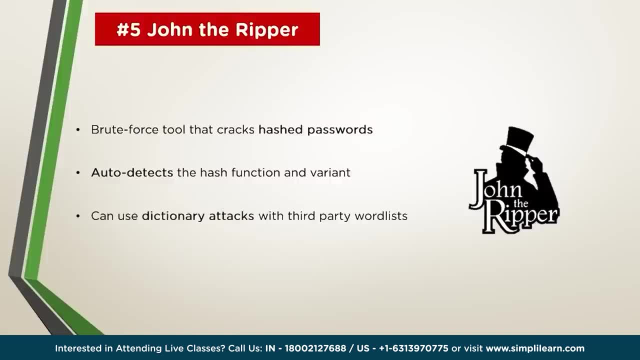 It can use dictionary attacks, along with regular brute forcing, to speed up the process of cracking the correct password without wasting additional resources. The word list being used in these dictionary attacks can be used by the user's end, allowing for a completely customizable process. We also have a few honorary mentions in our list that just missed the cut. 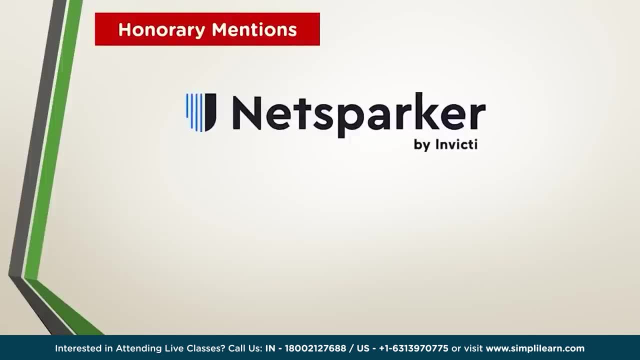 NetSparker, for instance, is an automated yet fully configurable web application security scanner that enables you to scan websites, web applications, websites, websites, websites, websites, websites, websites. The scanning technology is designed to help you secure web applications easily, without any fuss, so you can focus on fixing the reported vulnerabilities. 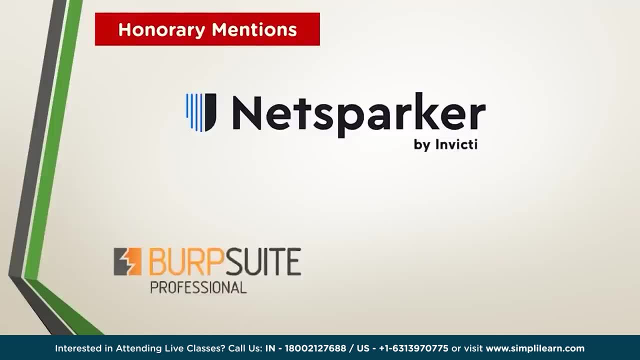 The Burp Suite Professional is one of the most popular penetration testing and vulnerability finder tools and is used for checking web application security. The term Burp, as it is commonly known, is a proxy based tool which is used to evaluate the security of a web based application and to do hands on testing. 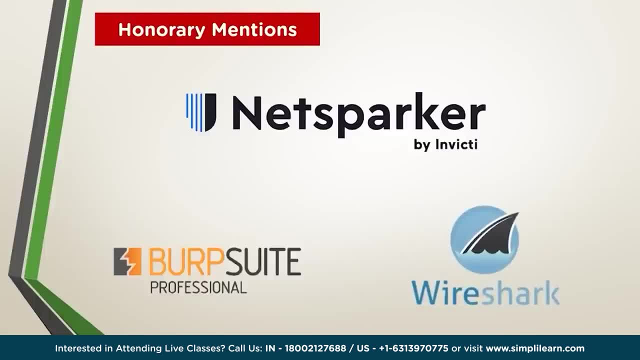 Moving away from websites and applications. Wireshark is a free and open source packet analyzer which was launched in 2006.. It is used for network troubleshooting, analysis, software and communications protocol development and education. It captures network traffic on the local network and stores data for offline analysis. 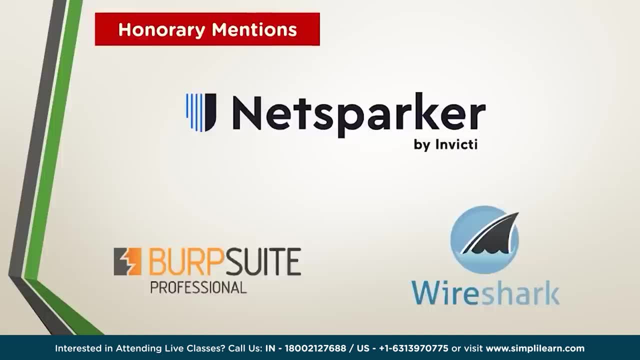 Wireshark captures network traffic from Ethernet, Bluetooth, wireless networks and frame relay connections. Now that we learned about the different features of Wireshark, let's move on to our next topic. Let's take a look at the different features of Wireshark. 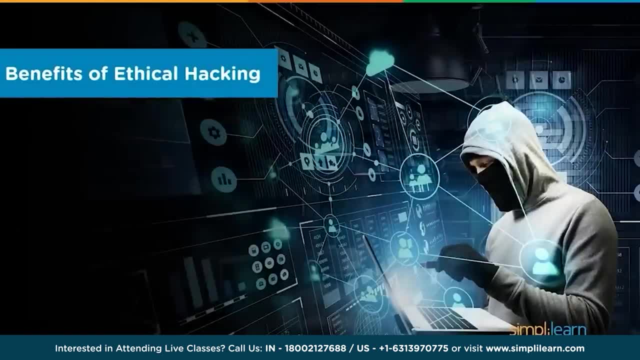 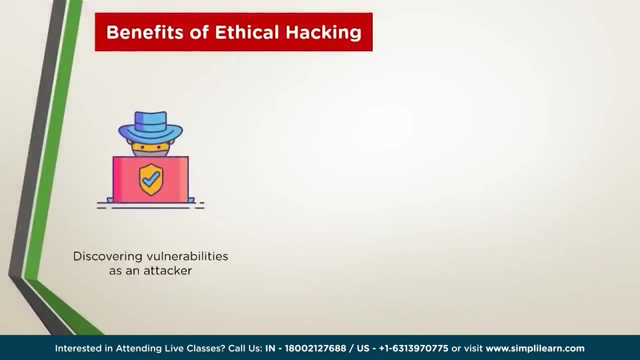 1. There are different types of tools that can be used when conducting an ethical hacking audit. Let's learn about some potential benefits of such campaigns and why organizations prefer to pay for such audits. Being able to identify defects from an attacker's perspective is game changing, since it displays 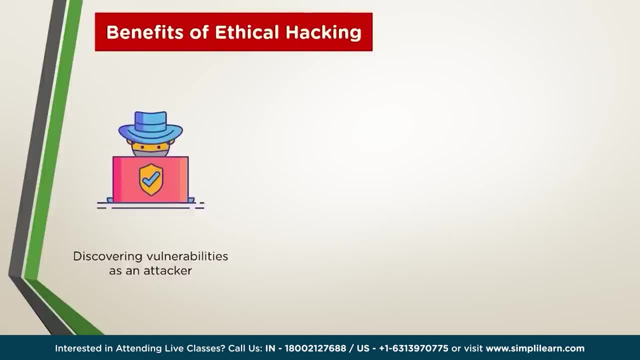 all the potential avenues of a possible hack. One can only prepare for the known vulnerabilities as a defensive specialist, but proactively trying to breach a network or device can be a challenge. 2. It can make hackers think of techniques that no defense contractors can account for. 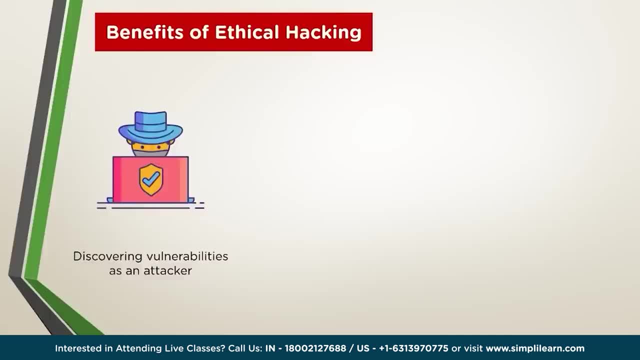 3. This kind of unpredictability goes a long way in securing a network against malicious actors. 4. Another advantage of hiring ethical hackers is the ability to preemptively fix possible weak points in a company's network infrastructure. As seen on many occasions, a real breach will cause loss of data and irreparable damage. 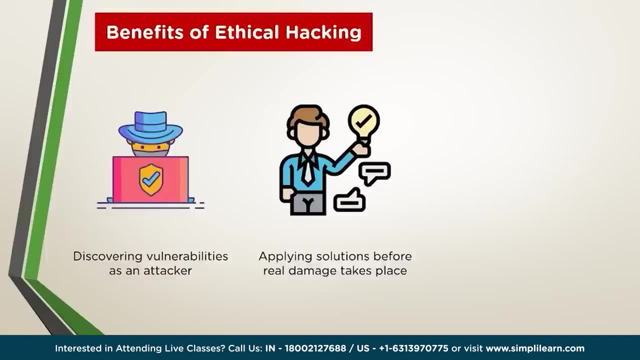 to the foundation of an organization. 5. Being able to gauge such shortcomings before they become public and can be used exploited is a benefit most organizations make use of. 6. This is not to imply that such security audits are only beneficial to the organization paying. 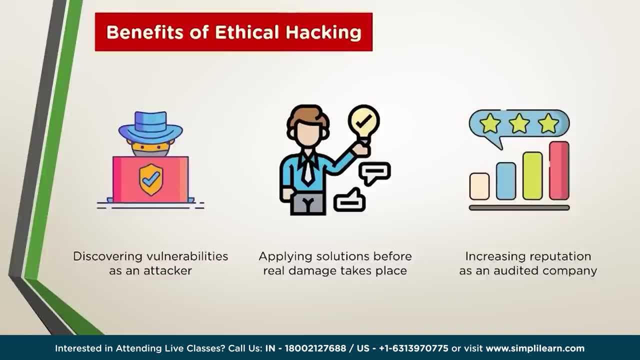 for it. When coming across companies that provide certain services, a reliable third-party security audit goes a long way in instilling trust and confidence over their craft. 7. If the ethical hackers cannot find any major vulnerabilities that can be leveraged by hackers, 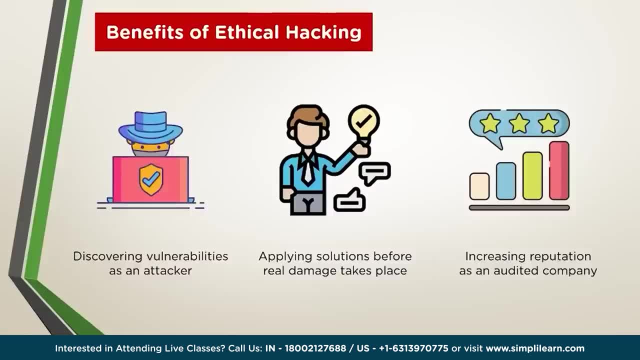 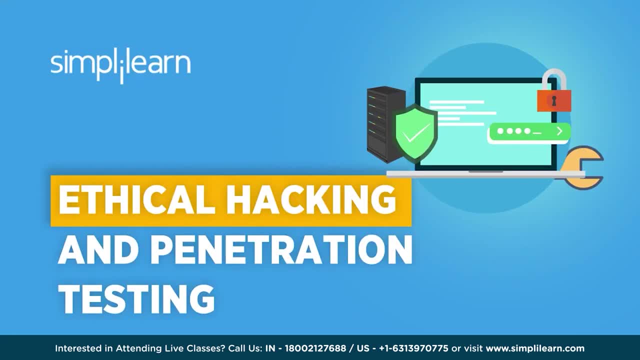 8. This is not to imply that such security audits are only beneficial to the organization. 9. This is a great opportunity to leverage the technical brilliance of the organization and its engineers, thereby increasing their clientele by a substantial amount. In this we are going to discuss Ethical Hacking and Penetration Testing. 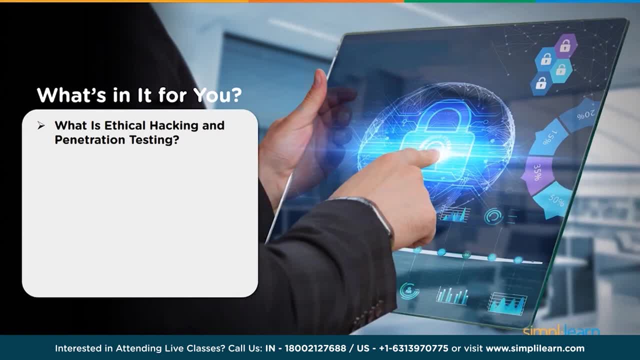 So we are going to talk about the concepts, about what constitutes an Ethical Hack and what is a Penetration Test. We are going to talk about the different types of Penetration Test and how they can be done. We are going to talk about an operating system called Kali Linux and we are going to talk 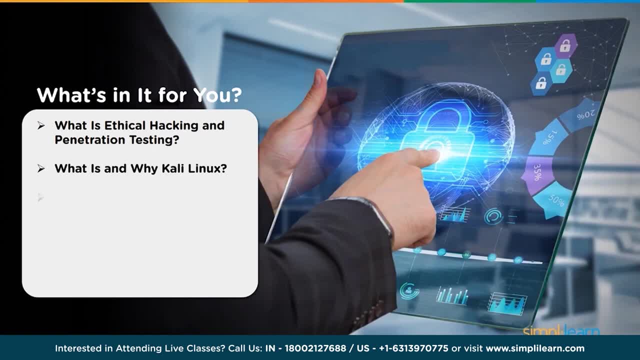 about its usage and its importance in cybersecurity. 10. We will also be discussing the different phases of Penetration Test and how people or hackers would utilize these phases to gain their objectives. 11. We will also be discussing what areas can we do a Penetration Test? how to do those. 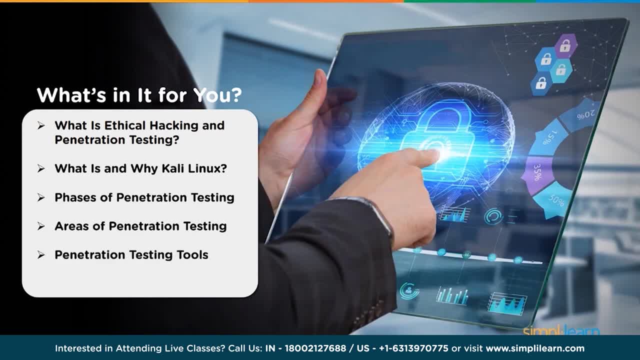 Penetration Tests: 12. We will be discussing quite a few bit of Penetration Testing tools that are available in the Kali Linux space. 13. And then we will be looking at a couple of demos at the end of the session to understand. 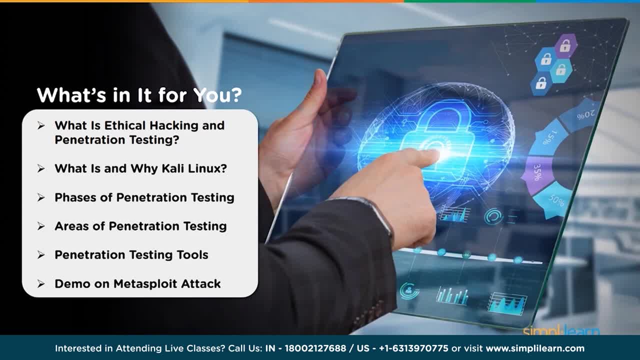 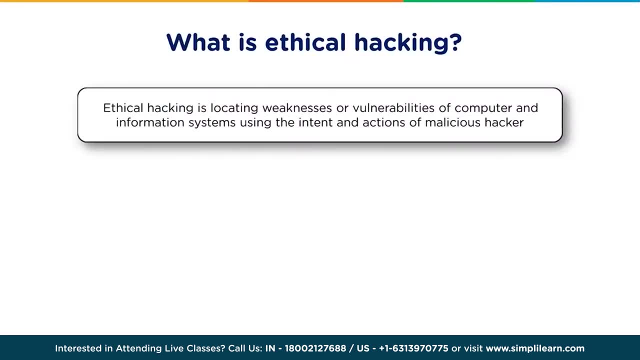 how these tools in the operating system can be utilized for various hacks 14.. So What is Ethical Hacking? Now, Plainly defined, Ethical Hacking is locating weaknesses or vulnerabilities of computers and information systems using the intent and actions of a malicious hacker. 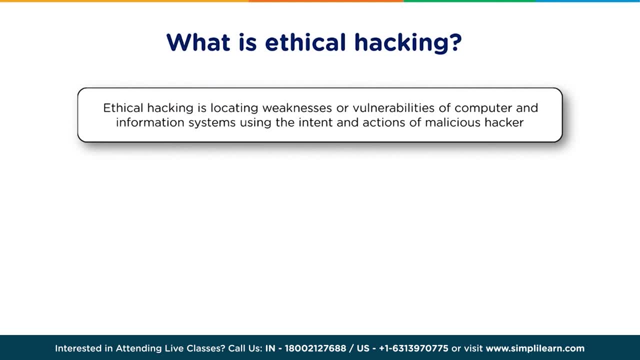 The major difference is here that we are hired to discover those weaknesses in a legal and ethical manner. That means, first and foremost, our intent should not be malicious, we do not wish any harm to the organization and whatever we discover is reported back and not misused. 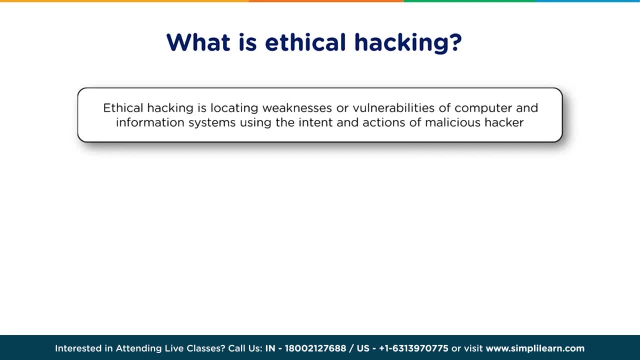 Once we report back, we would also be trying to help the user, to help them out, to mitigate or remove those weaknesses or vulnerabilities, to enhance the company's security posture. So essentially, we would have the same training or the same knowledge as that of a malicious hacker, except that the intent is going to be different. The intent is: 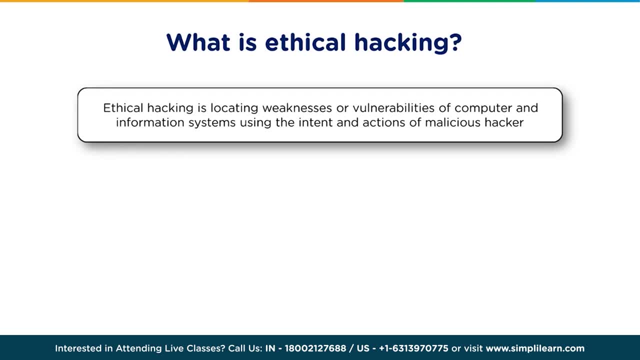 going to help the organization achieve security to protect themselves against malicious hackers. and the second most important thing about ethical hacking is that we are authorized to do that activity. I cannot, in good faith, hack somebody and then tell them: you know what? I just I just wanted to help you out and here are your vulnerabilities and this is the way you can. 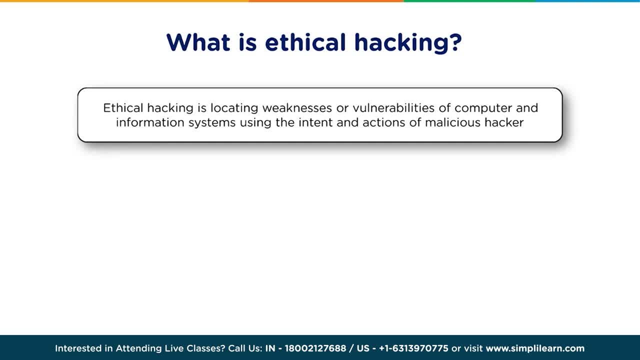 prevent them. I first need the authorization from the other party, and only then can I perform an ethical hack. So in this example, hacker attacks an individual with malicious intent and makes misuse of whatever information they have gotten. They steal the data, they maybe fry the operating. 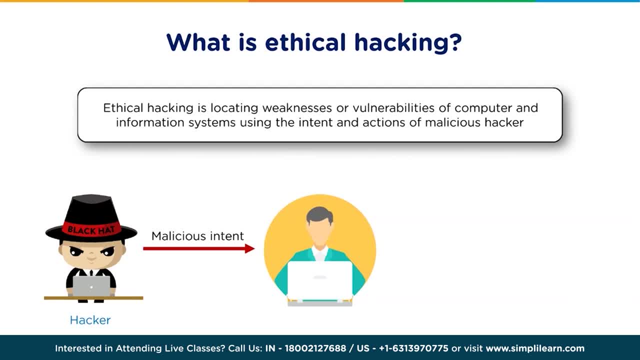 system hardware, destroy it, and then they can't do anything about it. So in this example, I can't do anything about it, and thus they leave the victim without a device. With authorization, an ethical hacker can also attack the same individual, minus the destruction, of course, and the 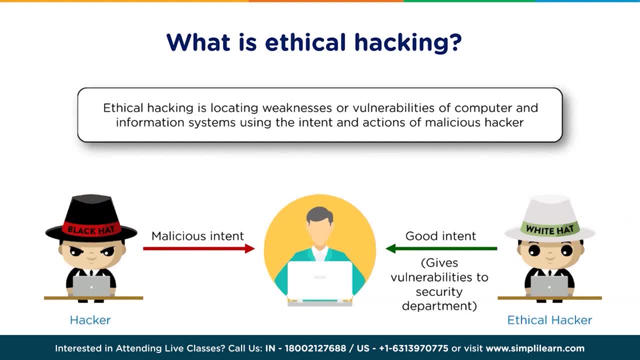 intent is good, So they are willingly finding out the vulnerabilities and helping the victim plug them out so that they wouldn't be a victim of a malicious attack. Now, here the first thing is authorization from the victim and the second thing is the good intent where we do not misuse those. 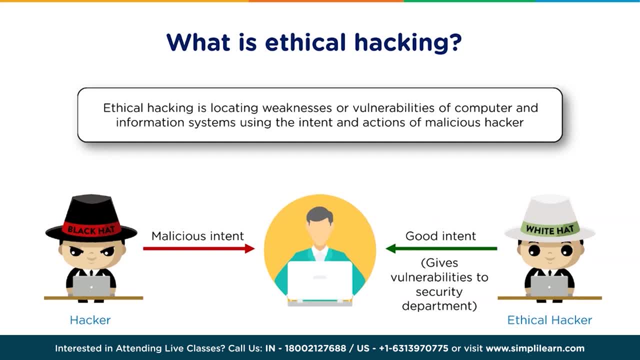 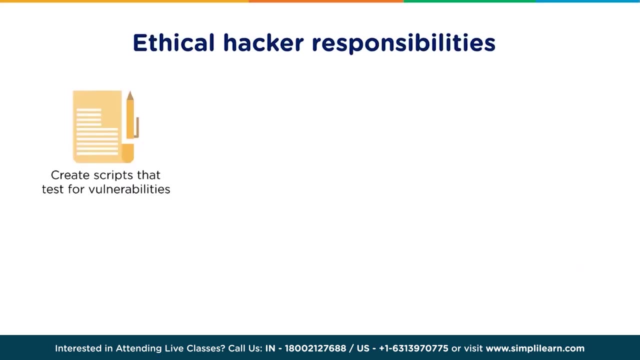 vulnerabilities and we report them back to the victim. So we report them back to the victim or to the client and help them patch those vulnerabilities. That's the main difference between a white hat and a black hat, So security experts are normally termed as white hat hackers. malicious hackers are termed as black hats. Now the responsibilities. 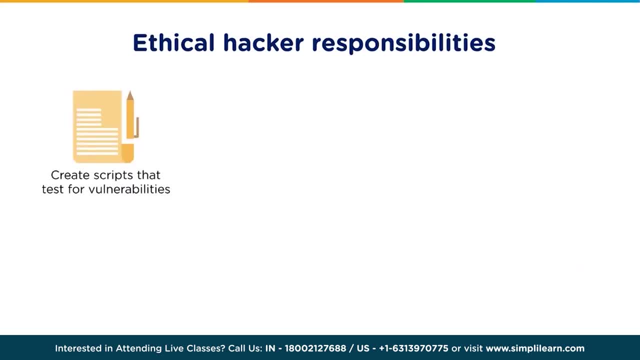 of an ethical hacker are multifold. First and foremost, you have to create scripts, test for vulnerabilities first, have to identify those in the first place. So there's a vulnerability assessment identifying those vulnerabilities, and then you're going to test them to see the 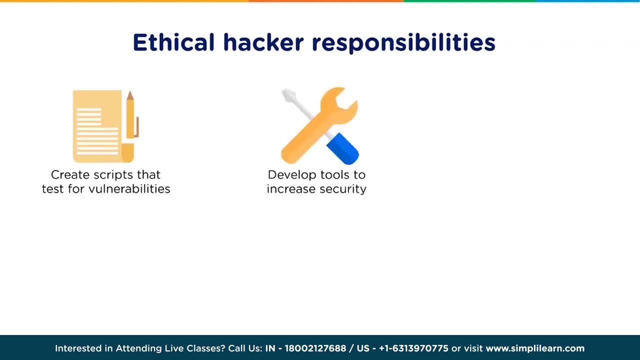 validity and the compliance. So that's the complexity of those vulnerabilities. So one of your responsibilities would be to develop tools to increase security as well, or to configure security in such a way that it would be difficult to breach. Performing risk assessment. Now, what is a risk? Risk is a threat that is posed to an organization. 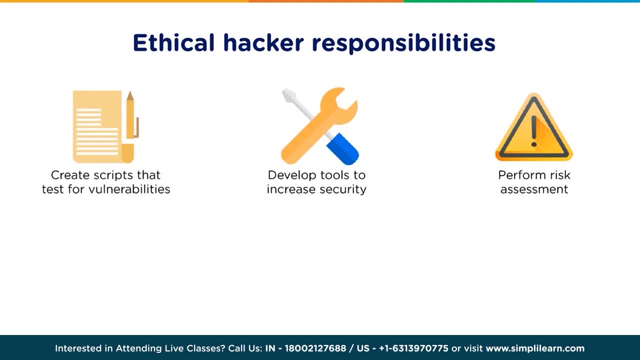 by a possibility of getting hacked. So let's say I, as an ethical hacker, run a vulnerability scanner on a particular client. I identify 10 different vulnerabilities. Within those 10 vulnerabilities, I do a risk assessment to identify which vulnerability is critical, would have the most impact on the client and what would be the repercussions if those 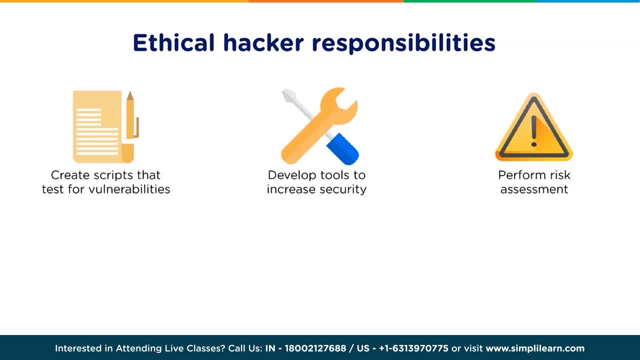 vulnerabilities actually get exploited. So I'm trying to find out in risk assessment that if the client gets hacked with the vulnerabilities identified, what is the loss they would be facing once they get hacked? And loss could not only be loss of data, it could be financial losses, it could be loss of reputation, penalties they have to pay to the client for breaches or penalties that they 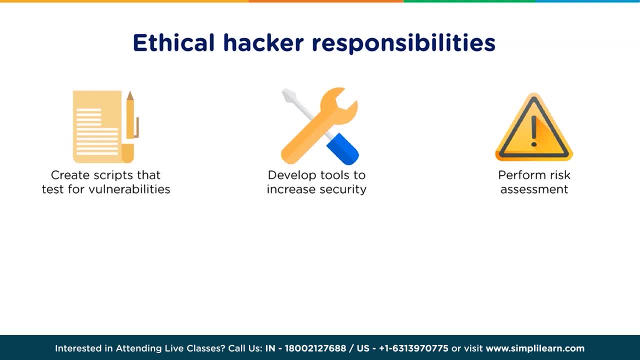 may have to pay for the governments in case of breaches that happened that couldn't be controlled. Another responsibility of the ethical hacker is to set up policies in such a way that it becomes difficult for hackers to get access to devices or to protected data, And finally, train the staff for 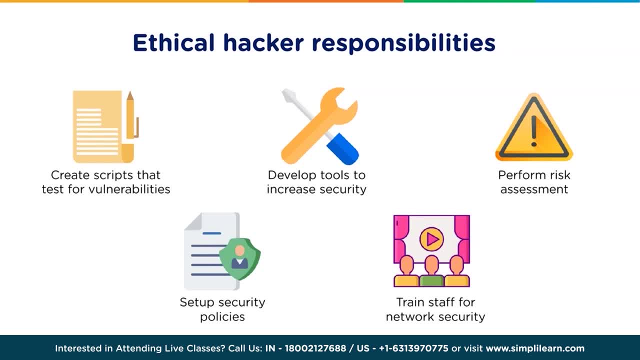 network security. So we've got a lot of employees in an organization. we need to train the staff of what is allowed and what is not allowed, how to keep themselves secure, so that they don't get compromised, thus becoming a vulnerability themselves to the organization. The policies that we have talked about are administrative policies to govern the employees of the organization, For example, 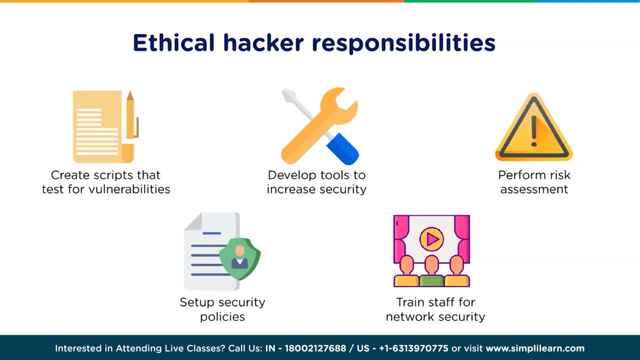 password policies. Most of the organizations will have a tough password policy where they say you have to create a password that meets a certain level of complexity before that can be accepted, And till you create that password you're not allowed to log in or you're not allowed to. 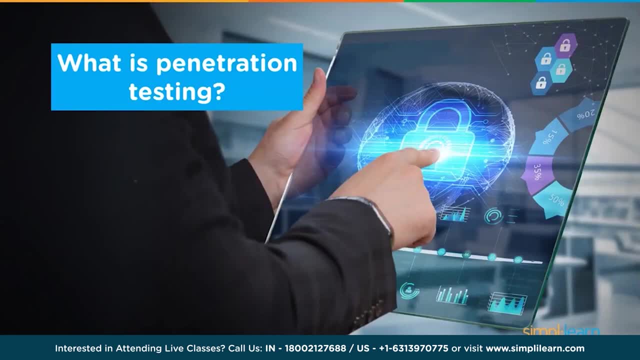 register. So let's move on to understand what is penetration testing. Now for penetration testing, there is a phase called vulnerability assessment that happens before this. Vulnerability assessment is nothing but running a scanning tool to identify a list of potential flaws or vulnerabilities within the. 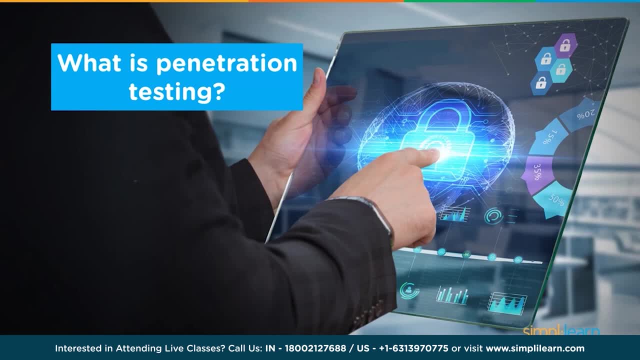 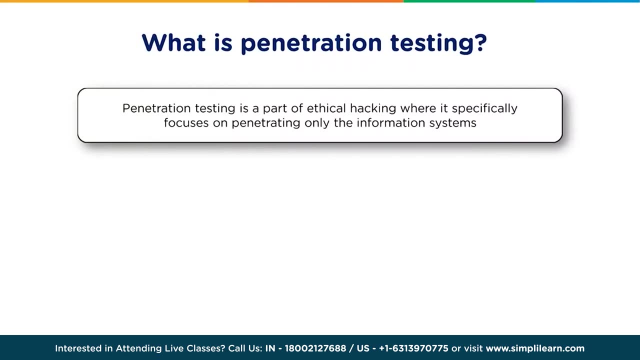 organization. Once you have identified the list of those vulnerabilities, you would then move on to penetration test. This is the part of ethical hacking where it specifically focuses on penetration only of the information systems. So you have identified that flaw. maybe it could be a. 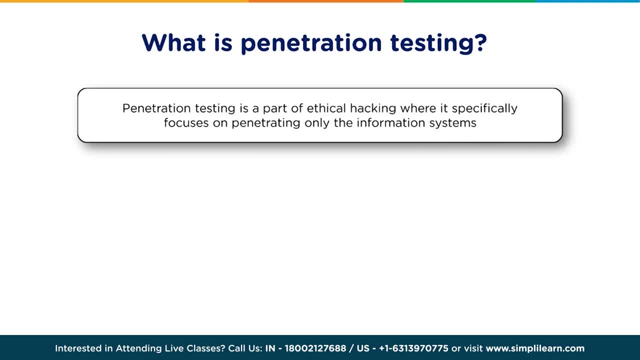 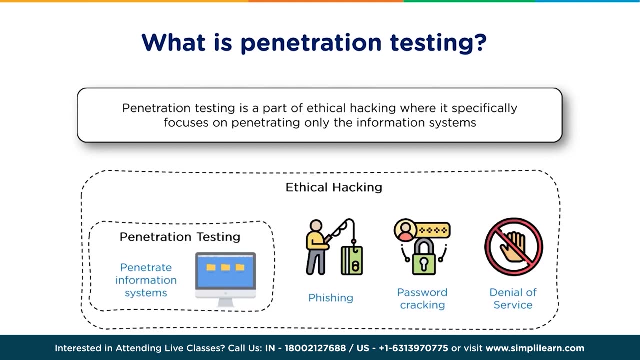 database with a SQL injection, or it could be a buffer overrun flaw, or it could be a simple password cracking attempt. Your idea is to create those tools, create those attacks and try to penetrate into those areas where security is weak. The essence of penetration testing is to 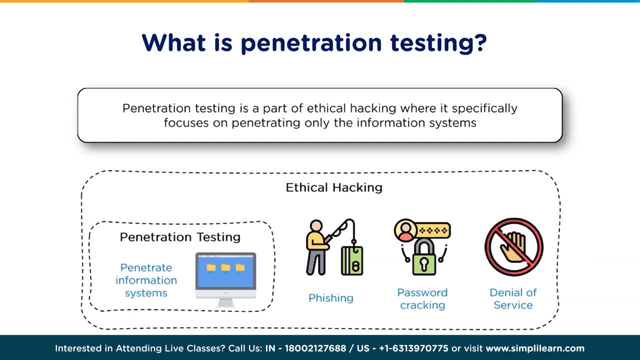 penetrate information systems using various attacks. The attacks could be anything like a phishing attack, a password cracking attack, a denial of service attack or any other vulnerabilities that you have identified during the vulnerability scan. So what is Kali Linux and why is it used? Kali Linux is an operating system. 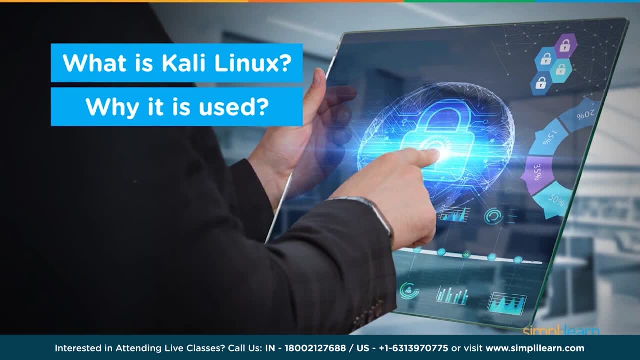 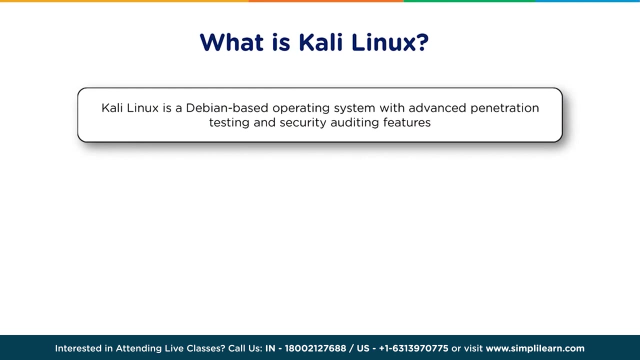 commonly used by hackers and ethical hackers do both because of the tool sets that the operating system contains. It is an operating system created by professionals with a lot of embedded tools. It is a Debian-based operating system with advanced penetration testing and security auditing features. There are more than 600 plus odd tools on that. 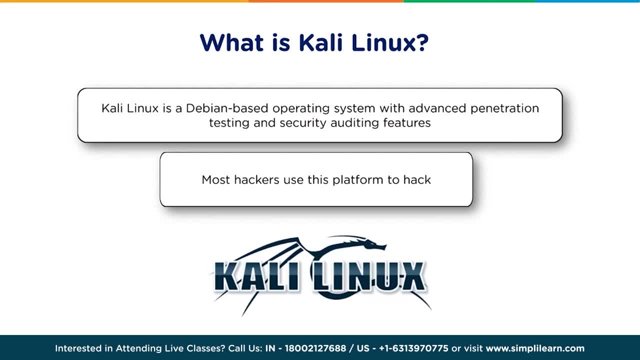 operating system that can help you leverage any of the attacks: man-in-the-middle attacks, sniffing, password cracking- any of these attacks would be possible with all the tools available. You just need to know how to utilize the operating system and its tools It contains. like I said, 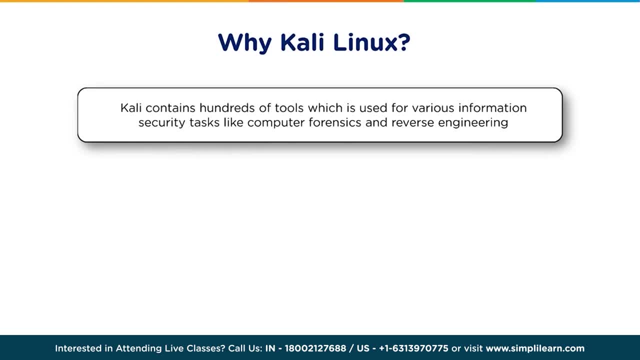 hundreds of tools that are used for various information security tasks, like computer forensics, reverse engineering, information finding, even getting access to different machines and then creating viruses, worms, trojans- anything that you will. 600 plus tools in the Kali Linux operating system. There are periodic updates that are given out to the 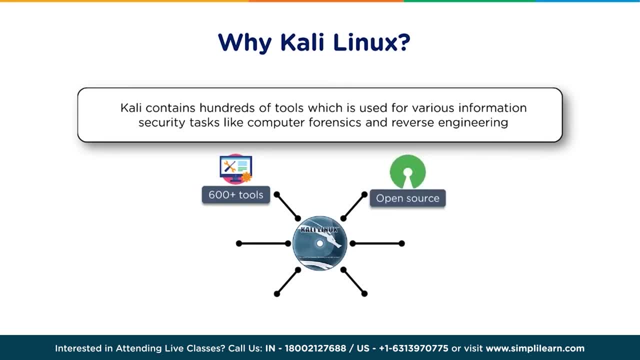 operating system as well. It is open source. That means it is free to use. You just need to know how to utilize the operating system and its tools. You can even have the source code. You can modify it if you want to. There's customizations. 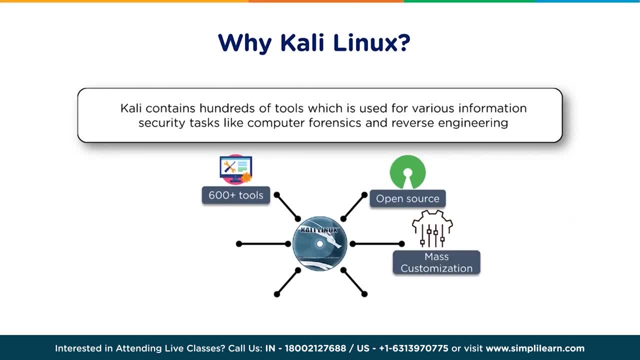 available for all the tools. You can download third-party tools and install them if you want. There's a wide support for wireless network cards. Multiple languages are being supported at the same time as well, And you can create a lot of attacking scripts You can create. 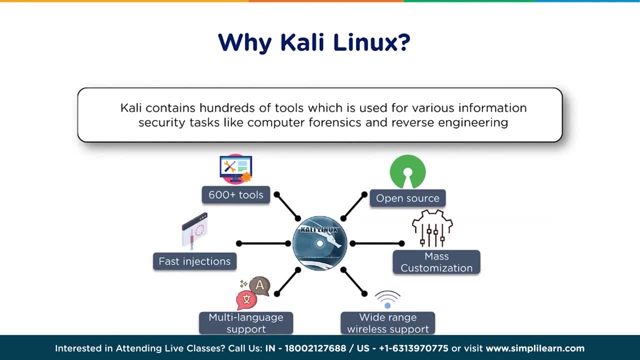 attacking tools, and you can write your own exploits as well on Kali Linux. So this all in all helps you create a very robust system where you can create your own attacks and then launch them against unsuspecting victims. Now, that is illegal, So as far as ethical, 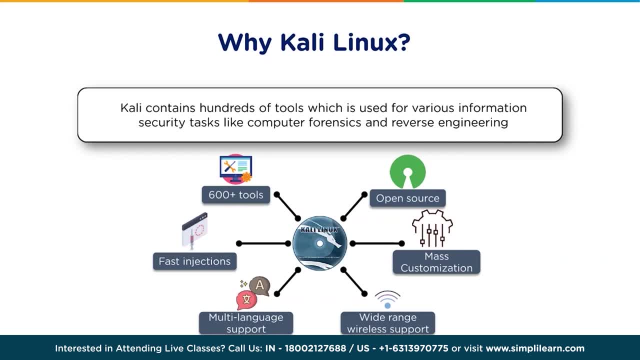 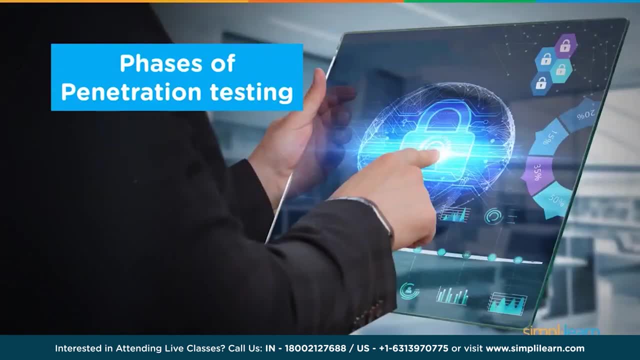 hacking is concerned. once you have authorization, you're going to identify which tools to be utilized, You're going to get the appropriate permissions and only then are you going to attempt those attacks. Let's talk about the phases of penetration testing Now there. 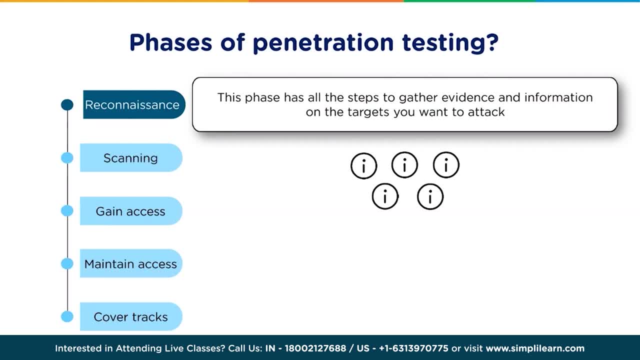 are five different phases. The first one is the reconnaissance phase, also known as the information gathering phase. This is the one where you're going to be able to identify the most important phase for any hacker. This is where the hacker, or the ethical hacker, 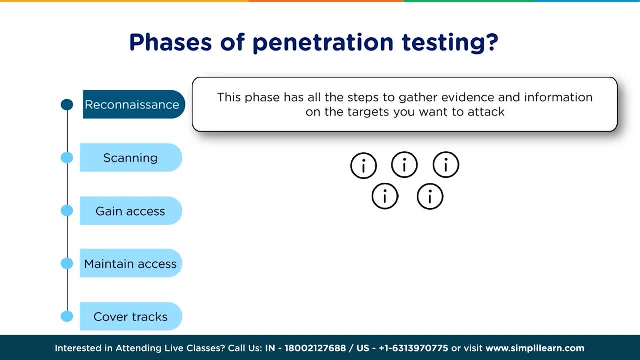 if you will, will gather as much information about the target's victim or vice versa, the victim right. So once you have that information, you would then be able to identify what tool sets to include and how to attack the victim. For example, you want to find out the IP addresses. 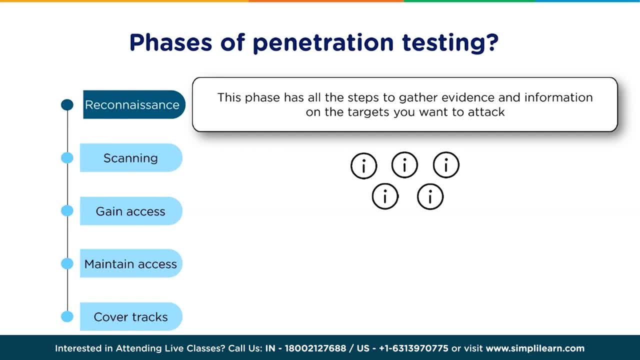 the domains, subdomains, the network architecture that is being utilized. You want to identify operating systems that are being utilized, the network IP ranges. You might want to identify employees within an organization for social engineering attacks in the future. email addresses, telephone numbers, anything and everything that will. 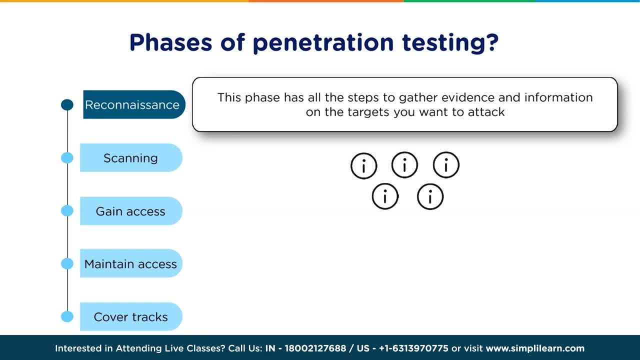 help you, validate and give you information about the target is something that you want to do in the reconnaissance phase. At this point in time, we are not going to question whether whatever information we are getting is useful or not. Only time will tell. depending on the various attacks that you will be building up later on, This becomes your baseline. 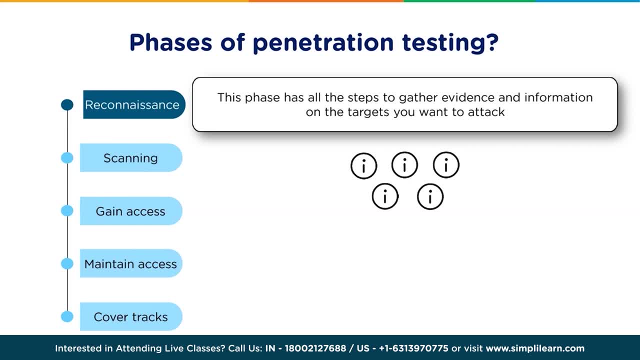 this becomes your database with all the information about the victim so that you can come back from later stages back to the reconnaissance phase to look at the information that you have gathered and then you can fine tune your attacks. Once you have done that, you are going to then start the scanning phase, Based on the 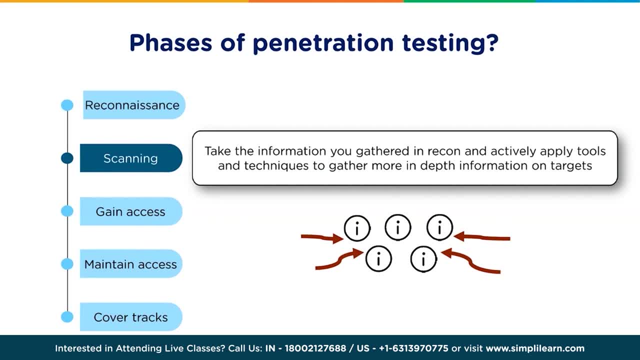 information that you have gathered, you are going to identify live machines within the network. Once you have identified the live machines, you will scan them for open ports, protocols and procedures, any processes that are running, and then we are going to identify vulnerabilities within these processes. 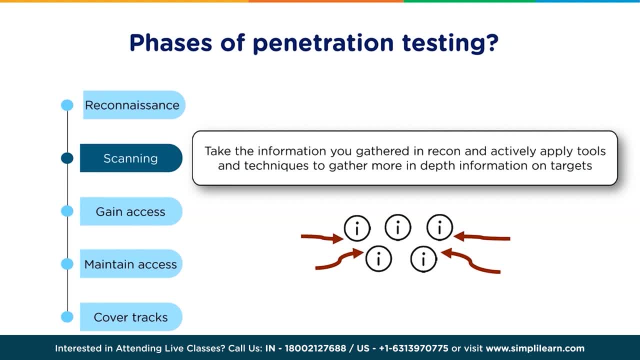 If airportmac request is changed, machine will not be opened. So in this kind of scan phase, why do we need to find live machines? Because we want to find out the machines that have booted up, have an operating system and are running on. 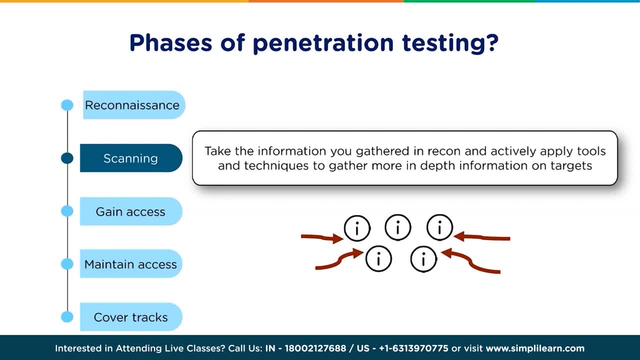 the network. If an machine is not available on the network or is in a shutdown mode, that machine cannot be hacked through a technical attack. Then it could be a physical attack, where you physically go to the machine and then do whatever you want to do with it. 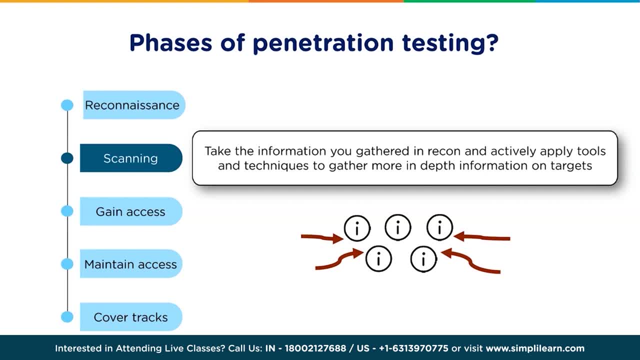 For a technical attack. you will have to identify the machines that are booted up. then you're open ports, because that's going to be our entry point and on the port would be a service that is running. so you scan the service as well, identify the version of the service and then do a vulnerability. 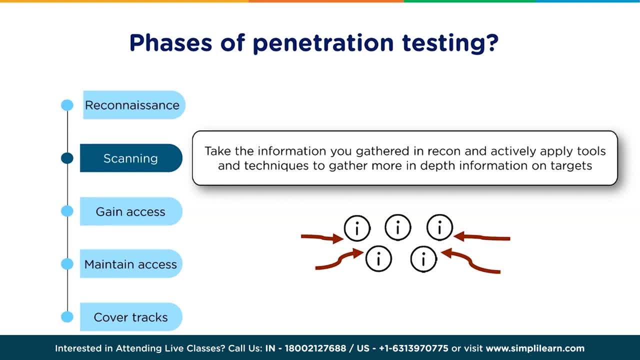 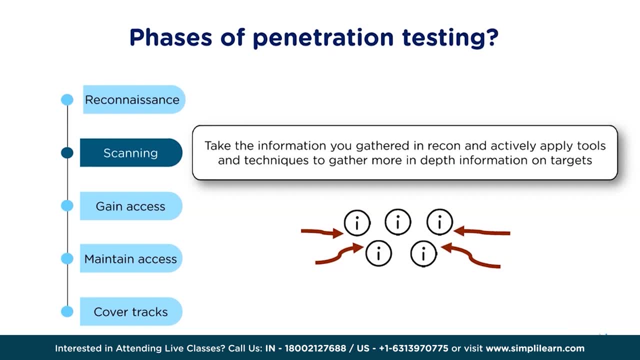 scan to identify if there are any vulnerabilities on those services that are running and then, based on all of this information, we are going to develop our attacks as we go on. So, once we have this, we go on to the gaining access phase, where we are going to attack and try to get access to our 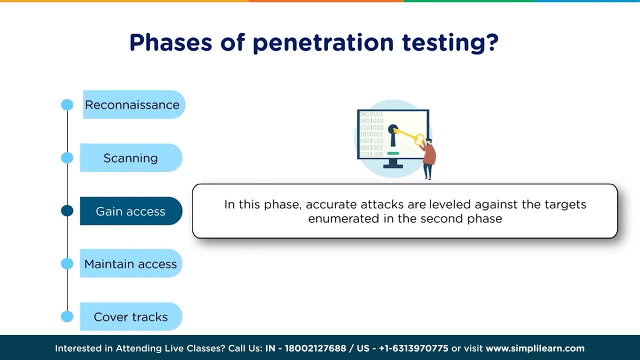 victim's machines Could be a social engineering attack based on the information gathering we have done in the technical assessment and scanning phase. if we have identified a vulnerability, you're going to identify a relevant exploit and then use that exploit to try to gain access. or we might just craft a trojan and try to execute that trojan on the victim's machine to check if 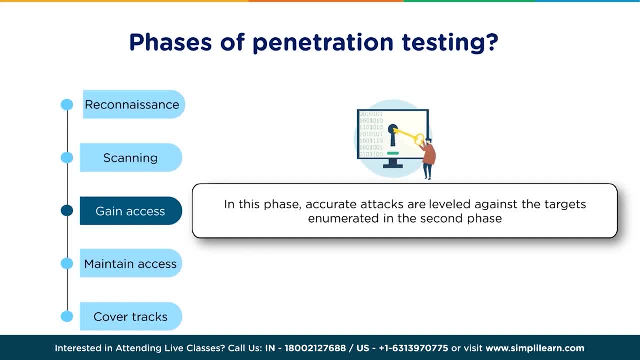 we can get access through that particular manner. Once we have the access could be even a simple password cracking attack, which we have been able to accomplish, and we have cracked the password of the person And now we have gained access to that person's computer. right, but these attacks would be temporary. 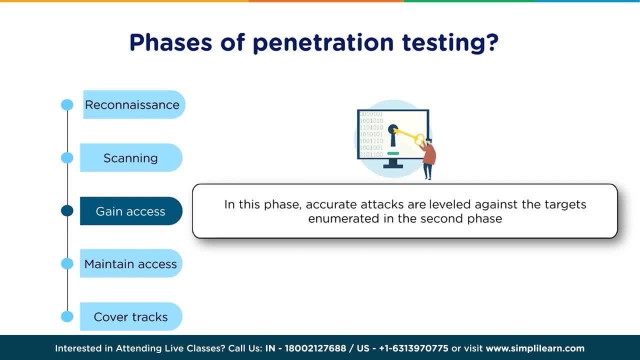 for example, we have cracked a password. somebody changes the password every 30 days after that period. our attack would be useless. If a trojan is executed, we get a connection to that machine for once, but then how do we get a repeated connection over and over again if we want to? 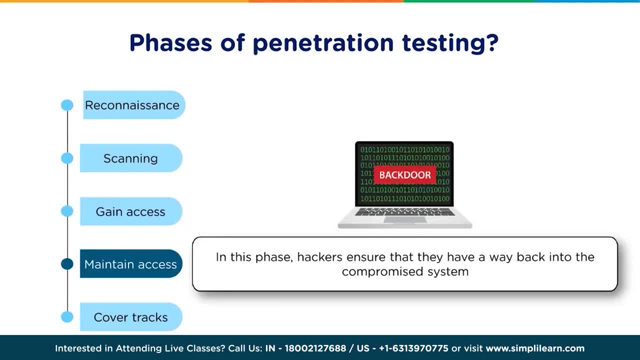 reconnect to that machine. So that's where we come into the maintaining access phase, where we install root kits, key loggers, sniffers and things like that. We have to have like that where we could get a back door entry to the victim's machine if we have. 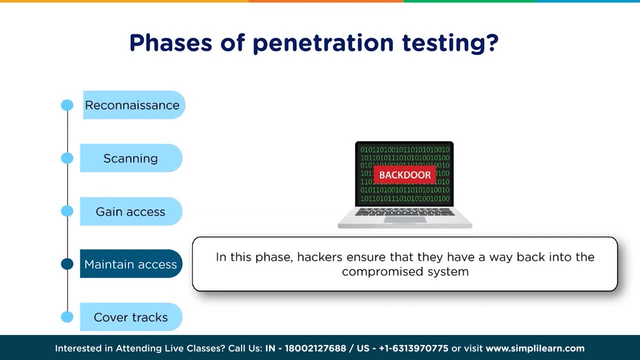 already been successfully installed a Trojan. we would want to add the Trojan to the start up menu so that every time the operating system starts, the Trojan gets automatically executed and does we maintain the back door entry to that victims machine Once we have done all of these. 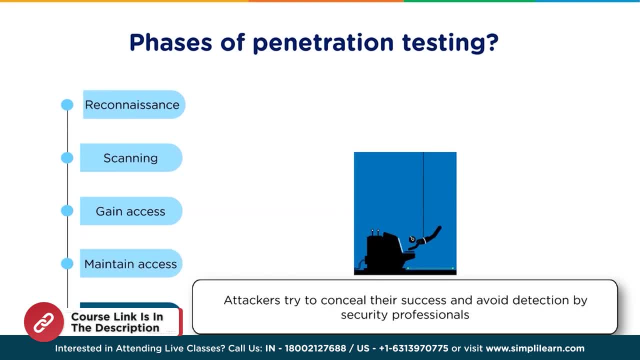 all these activities are going to leave a trace in the victims machine. So if we install a Trojan- a Trojan being an application would create directories and files- A virus be destructive in nature. if you are executing a script, it will leave some logs behind, if we even 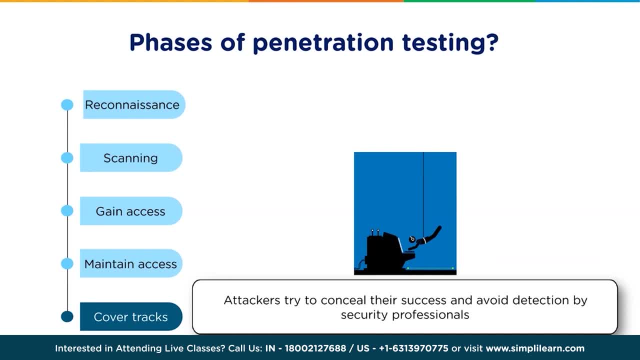 log in through the crack password that we have. it will create a login entry and for that particular timestamp, along with the ip address that we utilize in the covering tracks. we are essentially trying to avoid detection by deleting traces of our activity. that means that we need to identify: 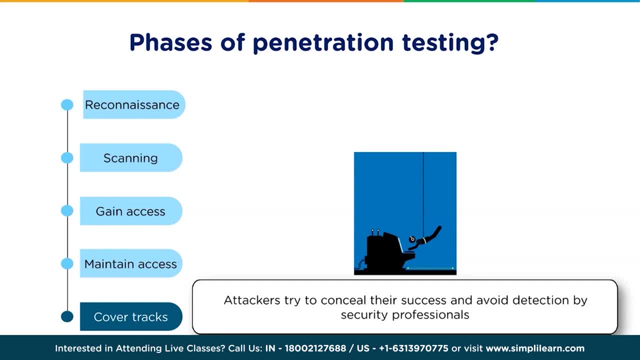 where logs have been stored. we need to address those logs and we need to delete them or modify them in such a way that our activity is not traceable. so these are the five main phases of a penetration test. gather as much information as you can scan for machines, ports, protocols and 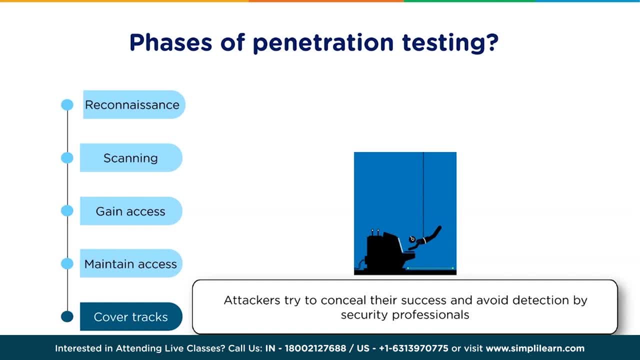 services running on the victim's device. try to gain access by password cracking, intrusions, exploits for the vulnerabilities, if any. maintain that access by installing further software which will allow you to get back door access to that particular system. and then try to cover your tracks by deleting all traces of your activity. once successful, the victim 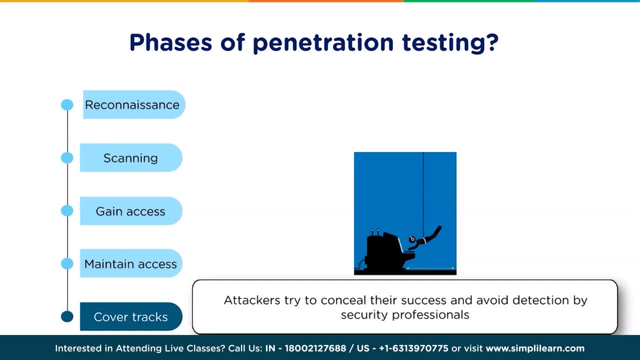 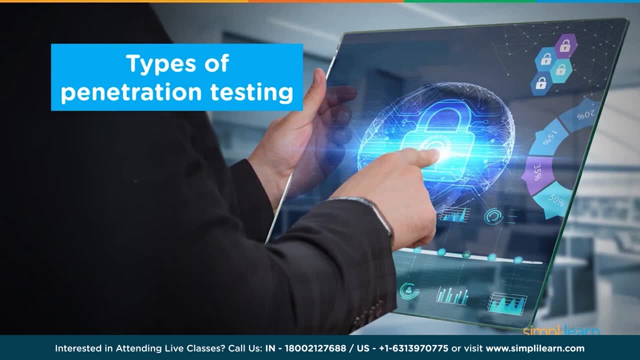 will have no idea and you have a backdoor entry and you can monitor the victim to the extent that you want. now, in an ethical hacker's perspective, this penetration test can be done in multiple aspects. so again, understand the fact that we are doing an authorized activity. we have identified. 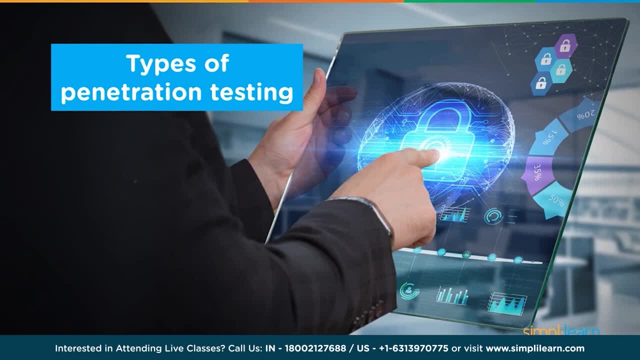 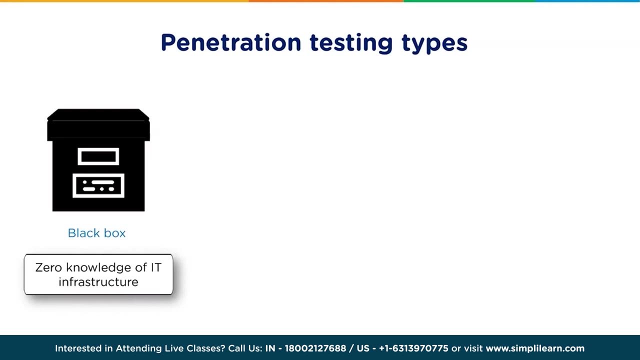 the tools that we have to use identified the attacks, we have got the appropriate authorization and based on that authorization, we are conducting a penetration test. the penetration test may be asked to be done in one of these manners. first is the black box test. the black box test is where no information is given to the ethical hacker about the it infrastructure. 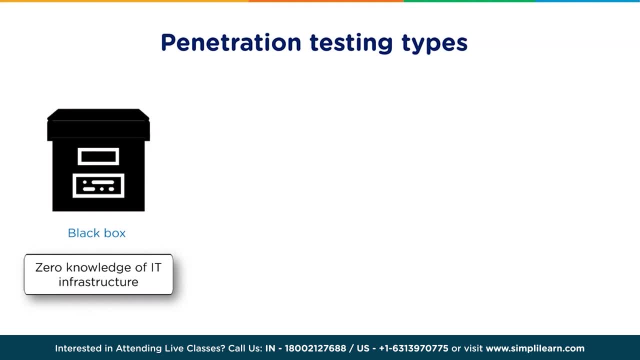 so they have no idea what it is. they start right from the first phase of the information gathering, gather as much information they can and, based on the gathered information, they try to create and launch attacks to see if they are going to be successful. now, not only does it test the knowledge, 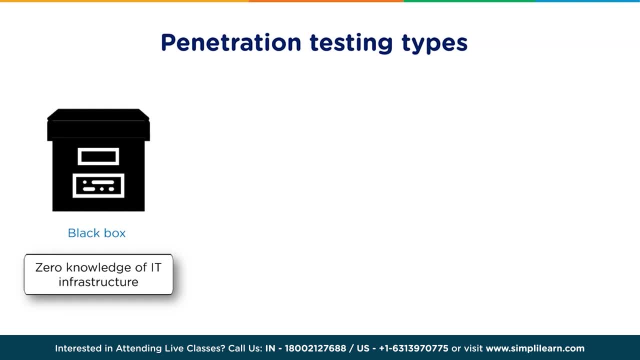 of the penetration tester. it would also test the security implementations that the organization has done to see whether they can identify the attack and prevent it in the first place. so this is the simulation of a malicious hacker's attack. so this is the simulation of a malicious hacker's attack. 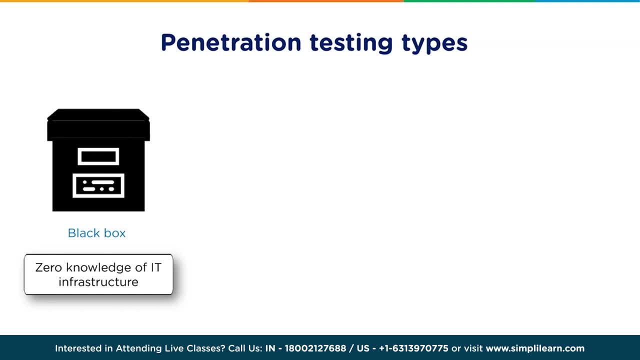 a scenario where a malicious hacker, having no idea about the organization, first tries to gather information and then tries to attack their organization. so no source code knowledge, no technological knowledge, nothing. they're just going to try to gather information, scan those devices and then try to gain access. the second test is a gray box test, where some information is given or 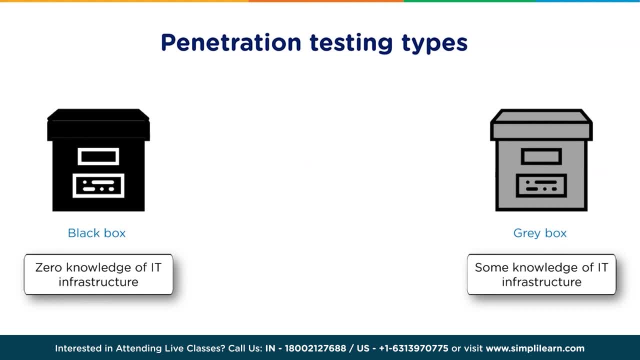 some knowledge of the id infrastructure is given. think of it from a employee's perspective: a regular employee in an organization who doesn't have extra privileges that are like an administrator, but it's just a regular employee. does that means that they got limited access within the organization based on which they get some knowledge of the id infrastructure? 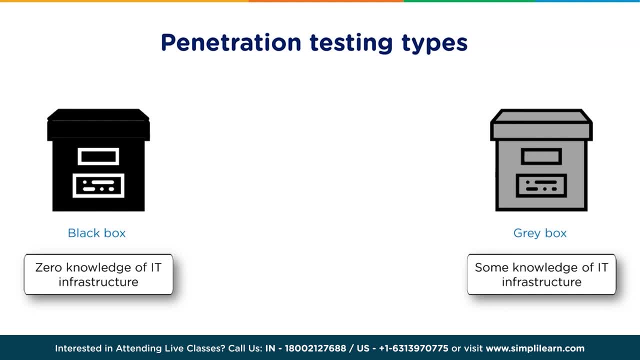 so this is an attempt of an insider simulation attack, where a regular user may want to try to misuse the access that they've been given and then try to gather information or try to gain access to other devices which they are not authorized to. the third test is white box. 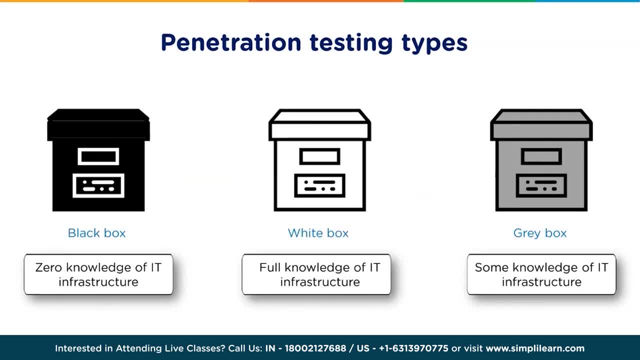 where there's full knowledge of the id infrastructure that has been given. so this is simulation of an insider attack, a malicious insider, if you will, but at this point in time the person has complete knowledge of the infrastructure, could be in an administrative position, and then they are trying to leverage their access to see if they can get information. 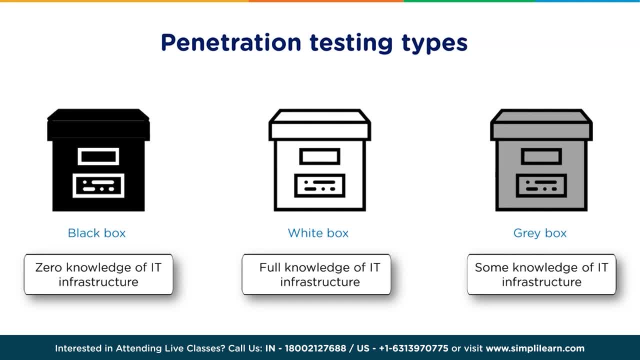 or they can compromise any stuff, any of the data. so the three attacks would be the first one, black box, where we are simulating a external threat, a hacker sitting outside the organization trying to gain access. the gray box is an insider threat, where there is a regular employee who is trying. 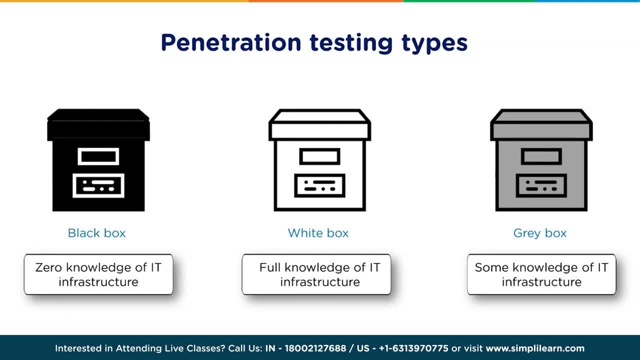 to gain access to infrastructure that they are not authorized for. and then the third audit is a white box audit, where there's an administrator who has all the leverage, all the access and the visibility within the infrastructure, and then they are trying to misuse their access to see what else. 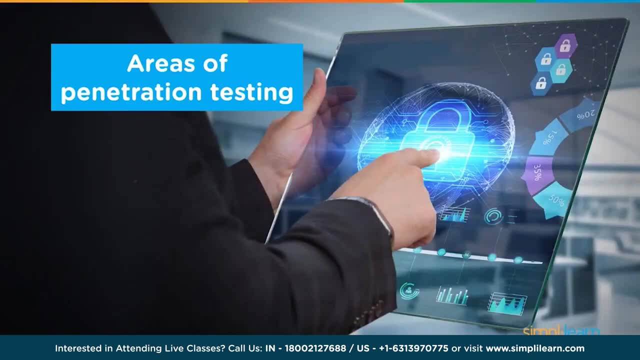 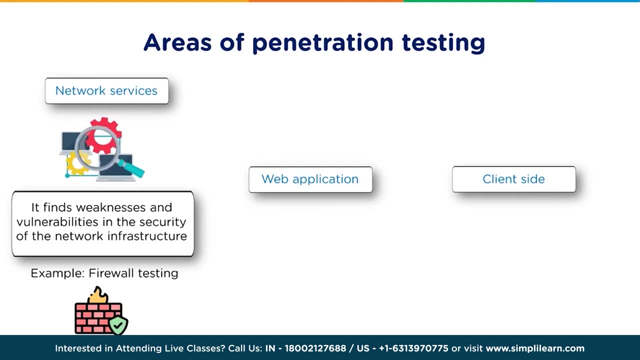 they can get from whatever access has been authorized to them. now let's look at the areas of penetration testing. where all could we do a penetration test, thus compromising the security of the application or of the server or of the user? so, first and foremost, network services. it finds vulnerabilities and weaknesses in the security of the network infrastructure. so for 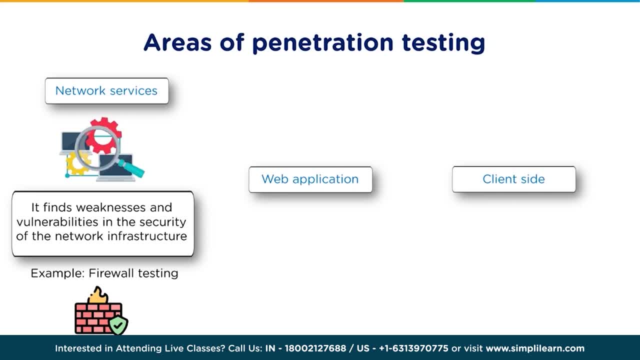 example, we have switches, routers, firewalls in the network. all of these are devices that need a configuration. if they have been not correctly configured or if they have not been correctly secured, they would leave some vulnerabilities behind. if we, as ethical hackers, are able to identify these flaws, these misconfigurations, these vulnerabilities, we could then try to. 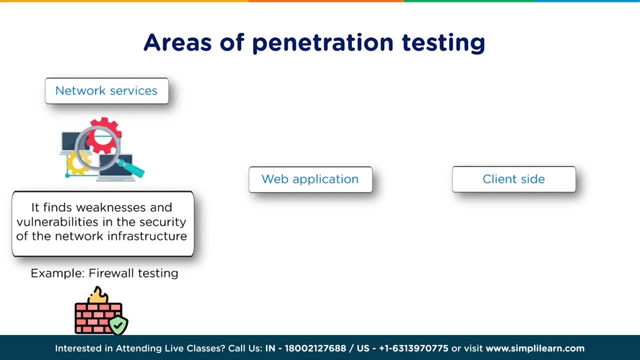 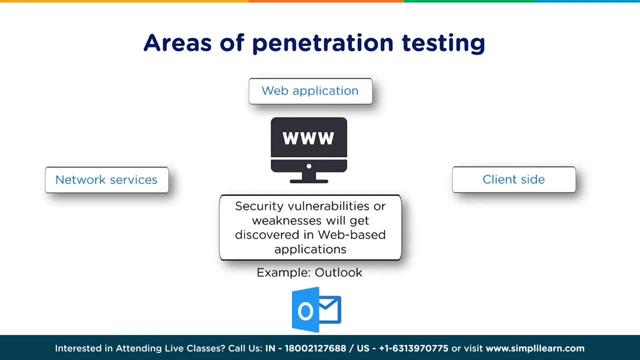 exploit them and try to gain access to the network and devices within that network by getting access to the network in the first place. then we have the web applications. web applications are nothing but softwares that are developed over or deployed over a web server and are made available over the intranet or the internet, for example, websites that we visit or 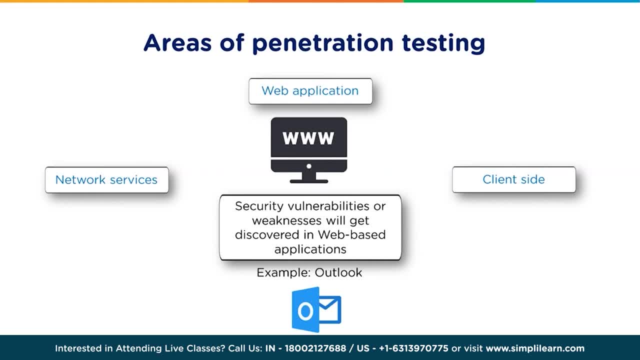 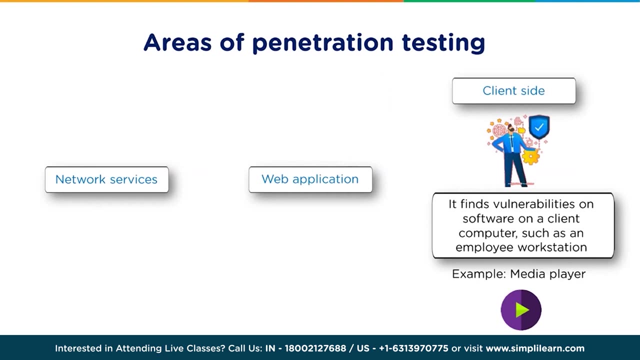 web applications like facebook, if you will right. so if these applications have vulnerabilities within them, we then try to attack the web-based applications and thus try to bypass authentication or get access to database or try to leak information through those applications. if not, then we try to attack the client side. now web application is at the server. 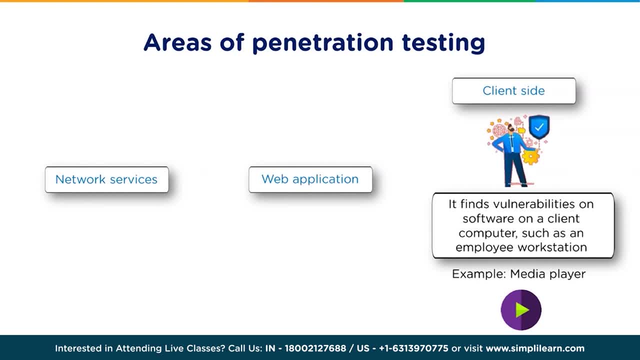 level and is hosted by the deployer, so that's at the server side. the client side is where we, as users, are using a computer with a browser and trying to interact with the web application. now the browser and the operating system that we are utilizing would have its own vulnerabilities. 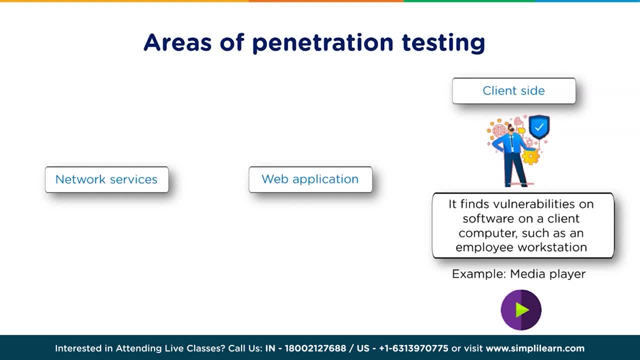 thus identifying a client-side vulnerability and then exploiting it to either either hack the client or then piggyback on the client's connection and try to get access to the server. you could attack the network, the web application or the client side itself, or you could attack. 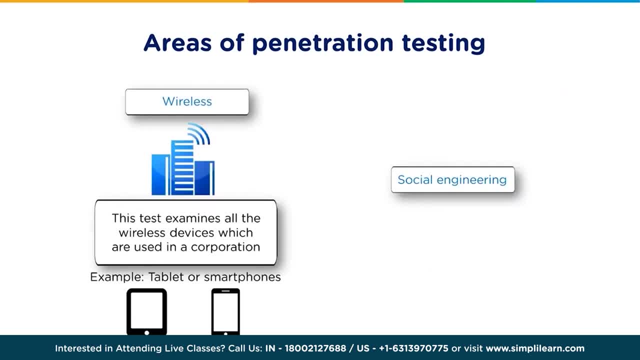 wireless networks. this test would examine all the wireless devices which are used in a corporation. most of the wireless would have laptops, smartphones, tablets, phablets- all of those connected to them. if you are able to access any of these devices through the wireless, it would help you gain access to other devices on the wireless as well. and then social engineering. 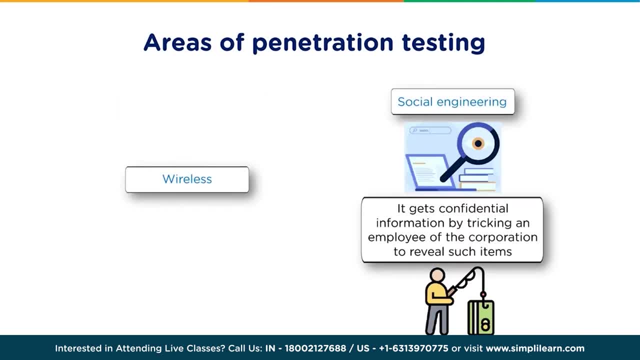 so this is where you are trying to attack humans. you are tracking an employee of a corporation to reveal some confidential information, knowingly or unknowingly, by tricking them with fake mails or fake websites or malicious emails that you have sent to them which they have failed to recognize as malicious and they click on it, thus getting victimized. social engineering. 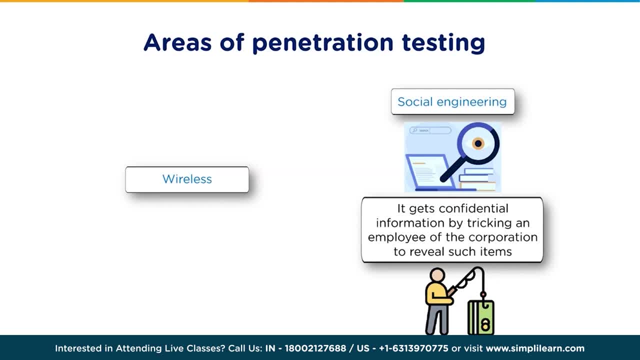 attacks are always successful because of the gullibility of humans: empathy, sympathy. humans basically have emotions. emotions can be toyed with and then taken advantage of if the person is not careful enough. for example, the most common social engineering attack that we see is the nigerian fraud, where we receive an email that someone somewhere has died and has left a huge 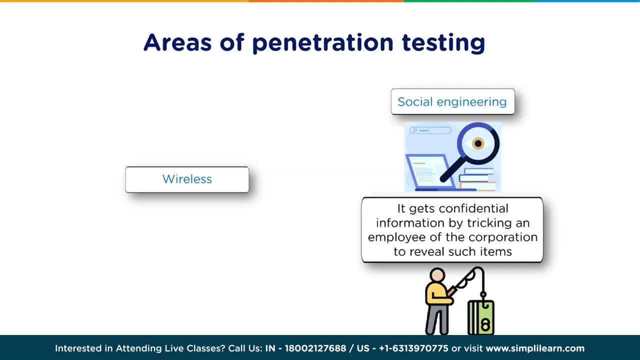 estate behind a few hundred million dollars, and we have been identified as the person through whom they want to transfer the money to a foreign land to save on taxes. what are the chances of that happening on a daily basis, right? how many princes are there? so that's something that we do not. 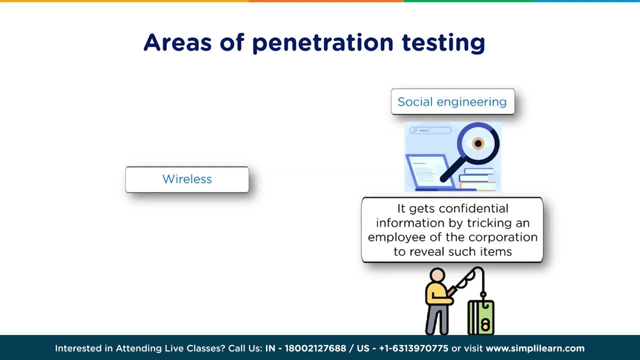 verify. it's just the- i guess the greed, if you will, of striking it rich quickly that makes us believe these kind of emails. we have also received emails of lottery tickets that we have won over a period of time without even having bought a lottery ticket. so if you 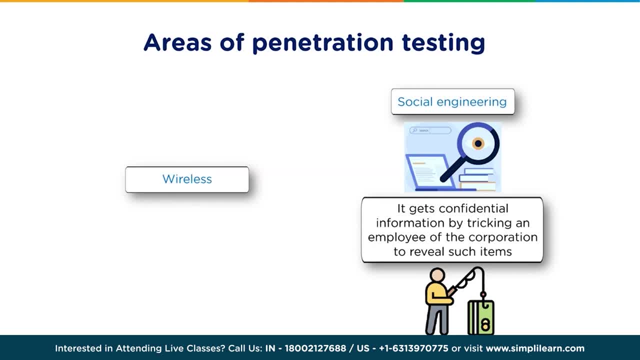 haven't bought one. what did you win? but we don't ask these questions. we just get excited about the amount of money that we have won and then we try to bet on our luck and try to see if that email is going to fructify or is it just under the scam? so social engineering attacks are dime a dozen these. 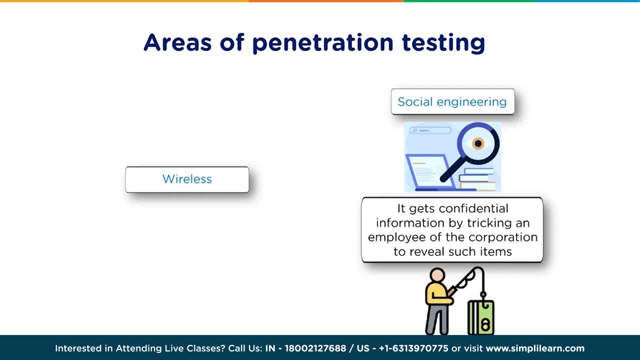 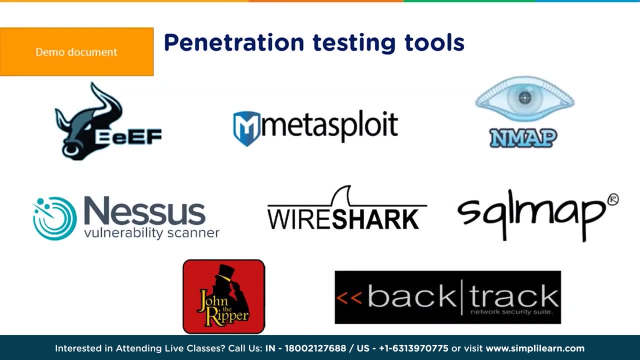 days and we need to be very careful on what we trust on the internet. let's look at the penetration tools. there are hundreds and thousands of tools out there. most of these have been concise and collected together and hosted on a operating system known as kali linux that we have talked about. 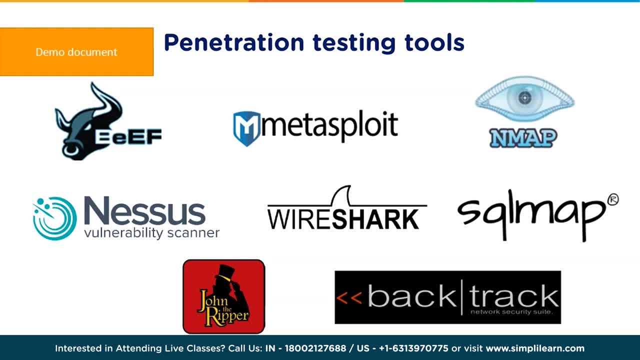 earlier now, the predecessor to kali linux was backtrack. backtrack is no longer continued. it has been discontinued and kali linux has taken the place of backtrack, within which are all the tools that you see on your screen. metasploit is one of the most favorite penetration testing tools. 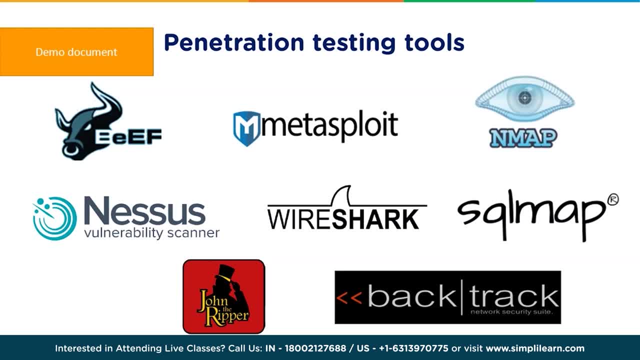 of hackers and ethical hackers. there are a lot of inbuilt exploits over there and we'll be doing a demo at the end of the session on this. nmap is the information gathering tool which will scan for live devices, scan for open ports, protocols and services. beef would be an application testing tool that would help us find exploits within. 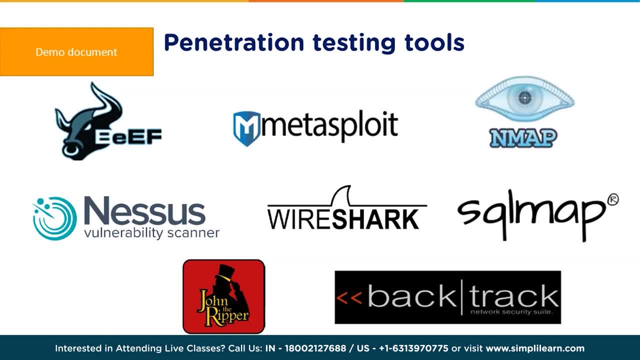 applications. nessus vulnerability scanner is a network and a host-based scanner that would help you identify vulnerabilities within such hosts. wireshark is a network sniffer which allows you to capture network packets and and analyze them to see if there are any. there is any information worth capturing within those. 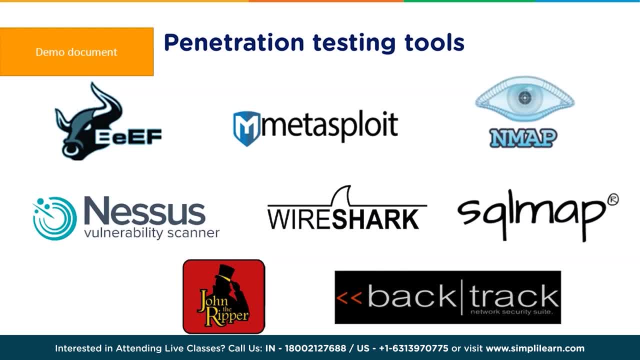 packets. sql map is a automated tool used for sql injection attacks. so you don't even have to craft your queries for sql injection. it will be done by the sql map tool. you just need to identify whatever is possible through the queries that the sql is going to create and then, based on the activity, 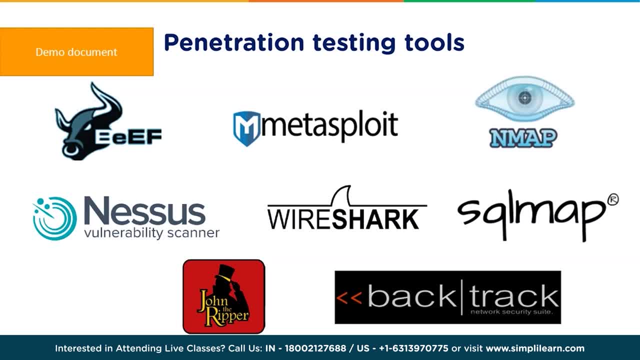 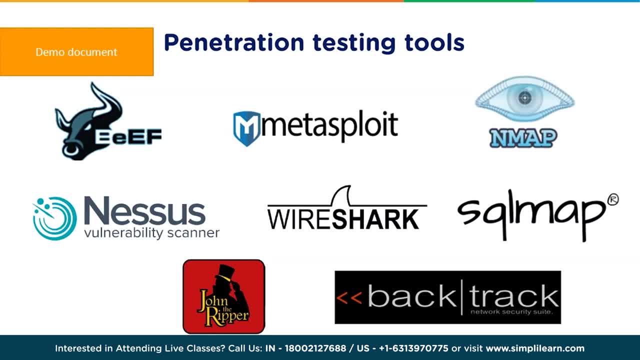 the sql map tool, and we'll be doing a demo on sql map or sql map as well. and then there is john the ripper. john the ripper is a tool that is used for password cracking, so dictionary attacks, brute force attacks, are done using john the ripper. what is a dictionary attack? a dictionary attack is an. 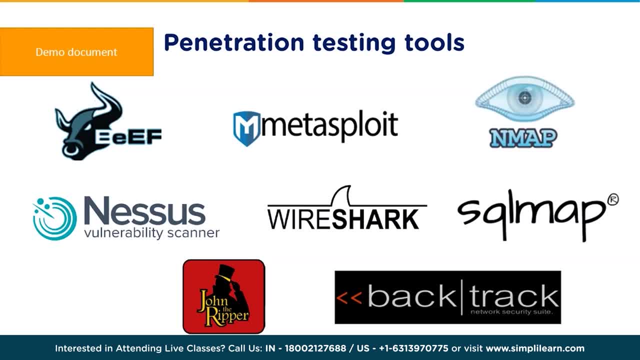 attack where we create list of all probable passwords, store them in a txt file and run that list against the password tool to see if any of those passwords are going to match a brute force attack is trying the same attack, but with every permutation and combination of the alphabet that. 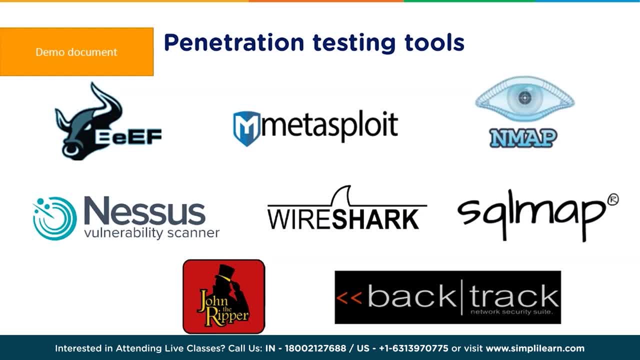 we have and we're going to try to figure out if we are able to crack the password at all. so these are just some of the tools. for every tool there are another supporting 100 tools, or more than that. uh, like for ness's vulnerability scanner, you'll have call this vulnerability scanner, you have. 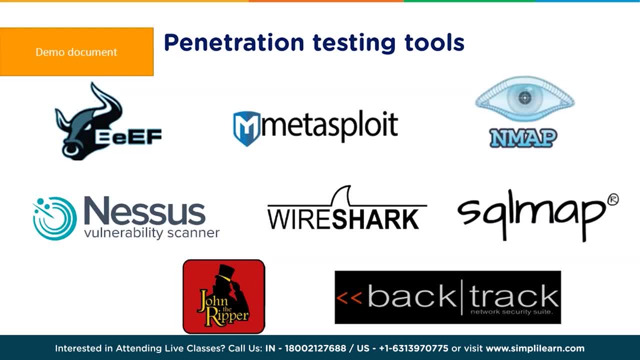 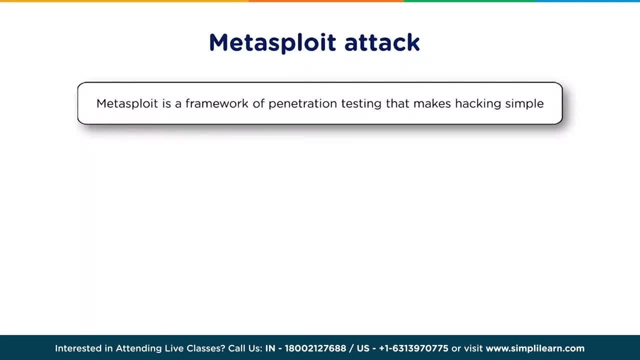 gfi, lan card, and there are other, lots of other softwares out there, but these are some of the most commonly utilized tools. let's look at the metasploit attack. metasploit is a framework of penetration testing that makes hacking very simple. you just need to know how to utilize the tool you 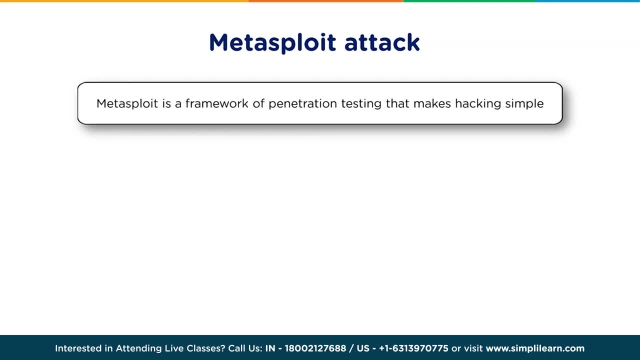 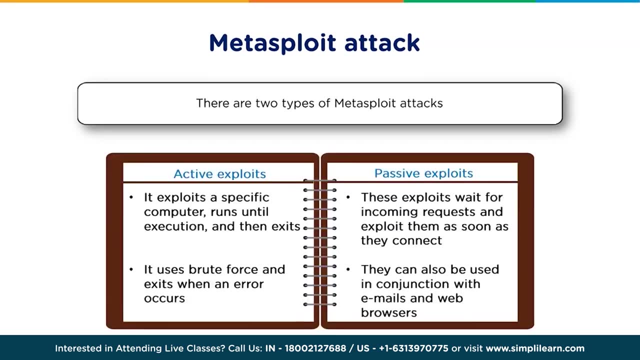 need to identify the vulnerability associated with a particular exploit and then run the exploit on metasploit. we'll be demoing this during the practical. so there are active exploits and passive exploits. inactive exploits exploits a specific computer runs until execution and then exits. uses brute force and exits when an error occurs in a passive exploit. these exploits wait. 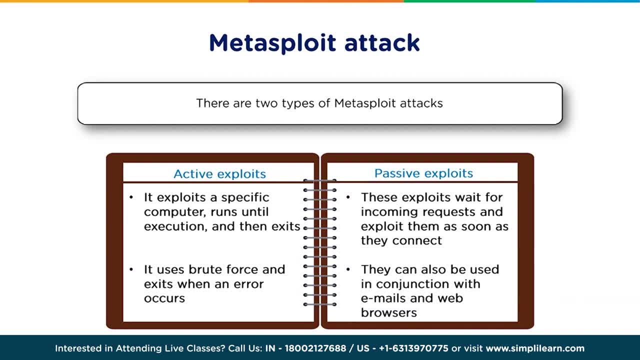 for incoming requests and exploit them as soon as they connect. they can also be used in conjunction with emails and web browsers. so in passive exploits we create a payload. we like a reverse connection payload. we send it to the victim. once the victim installs that software, the machine will then initiate a connection to us. our machine will be in a listen. 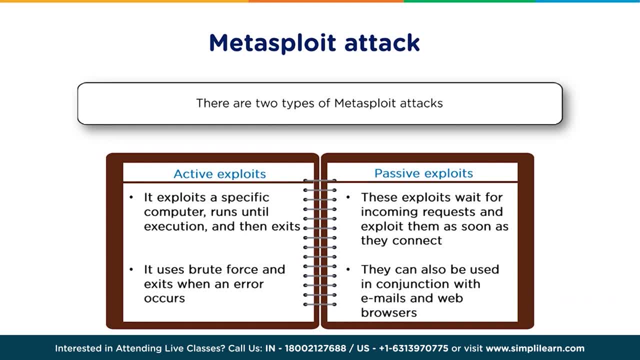 mode, and then we will, once the software is executed at their end, we would then try to connect and exploit that particular vulnerability. this is the uh practical that we'll be doing on metasploit. so let's move on with the demos and then we'll see, uh, what we can discuss amongst. 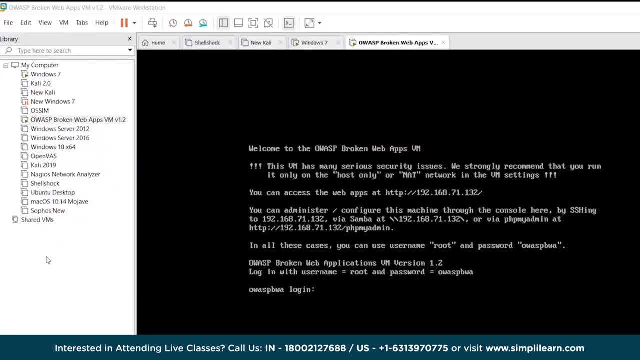 them. all right, let's have a look at some of the demos that we had, uh, talked about in the hacking and penetration testing module. we are going to look at three different demos. the first one is going to be a sql injection attack that we are going to perform on this tool that we 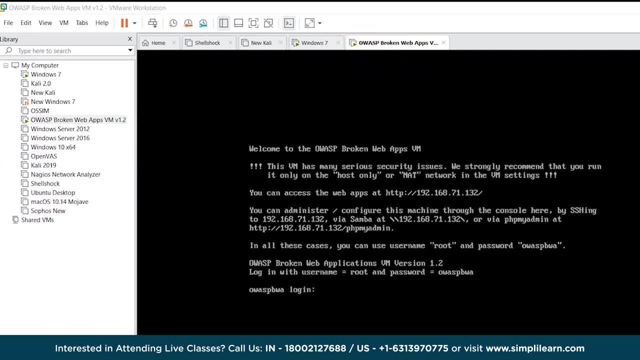 have. the second one is a password cracking attack on windows 7 and a third one is a meter breeder based or a metasploit based shell shock attack on a linux based web server. so let's get cracking. i've powered on this virtual machine, uh, which is the ovas broken web application. it is. 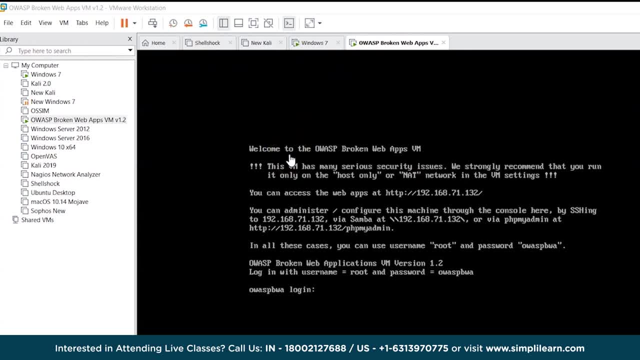 a tool that is provided for a people who want to enhance their skills, and they can practice, uh, how to do these attacks in a legal manner. so we are going to go to this site. i'm just going to open up my browser. the ip address is 71.132 and that's the ovas broken web application that. 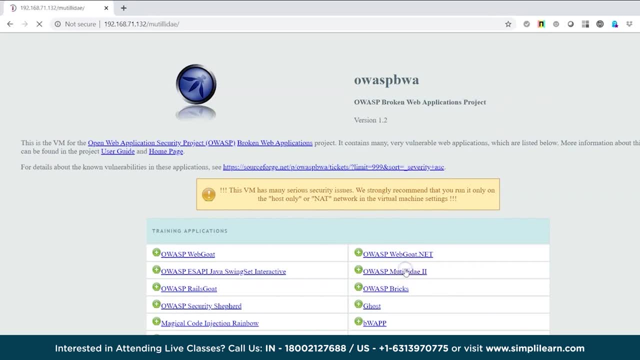 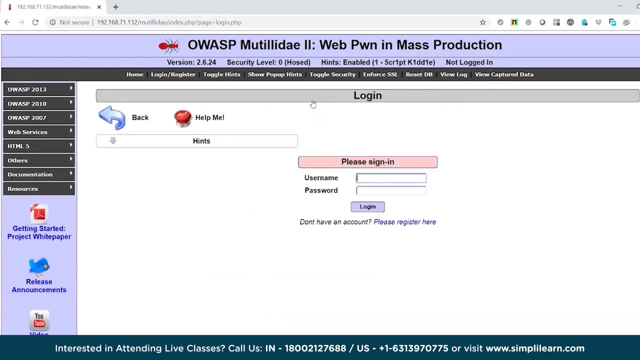 we want to utilize. we're going to head off to mutility 2 and we are going to look at a sql injection attack where we want to bypass authentication. now this takes us to the login screen, so we can just try our luck here and see that the authentication mechanism works. the 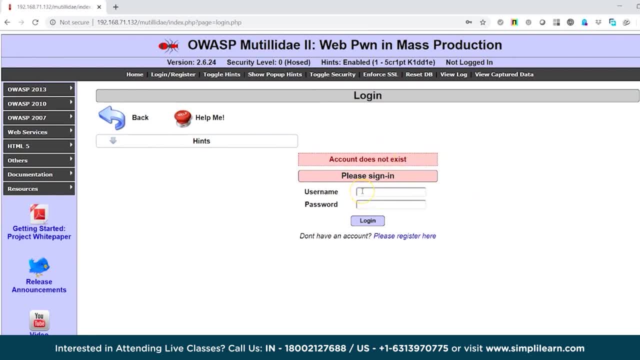 so the username and password that we have supplied is not the correct one. so we want to ensure that there's a sql database and we can try to attack it and see if we can bypass the authentication. now what we want to do is we want to create a sql based malform query that can give us a different 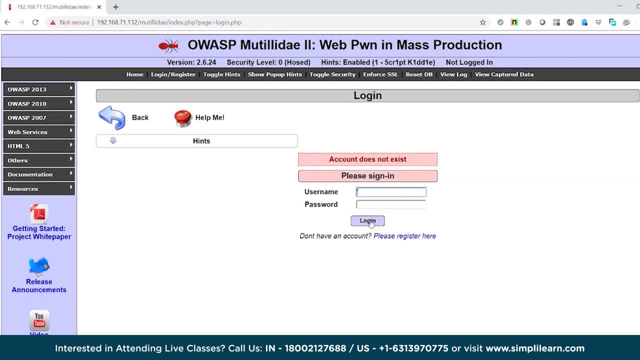 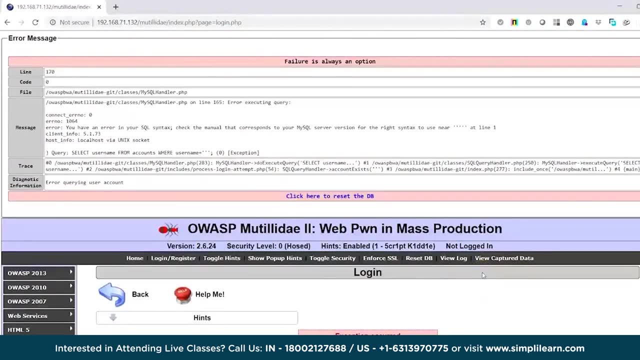 output. so i'm just going to type in a single quote over here and type login, and you can see that this is now suddenly recognized as a operator and there's an error that is given out. compared to the login that we tried earlier, when we used a proper text-based login mechanism, it gave us 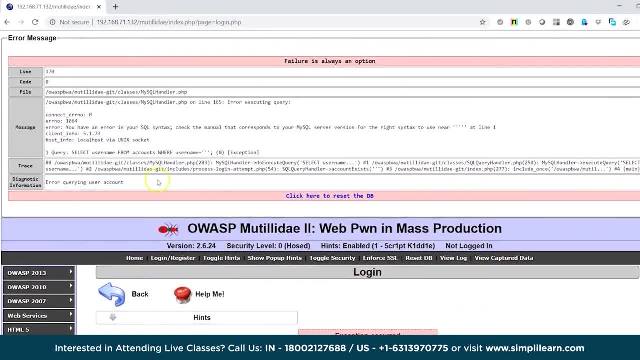 the account does not exist, but here the single quote gave us a error and it shows us how sql works. this is the query that we had created. now, in the trainings that you have for ethical hacking, there would be explanations of what these queries are all about, how this syntax works. here we're. 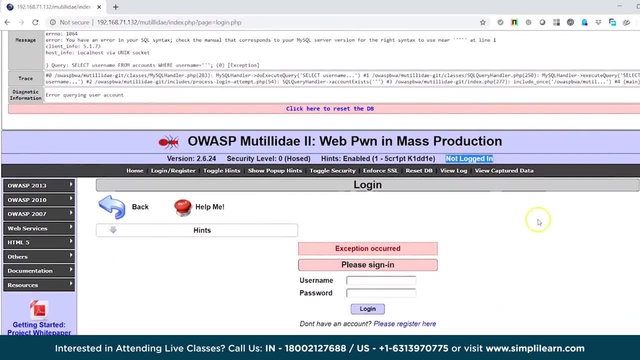 just going to see if we can create a malform query to log in as a user in this case. so what i'm going to do is create a query over here and we're going to give it a comparison. so we're going to give it a r. 1 equals 1 space, hyphen, hyphen space, and if you now click login, you should be able to bypass. 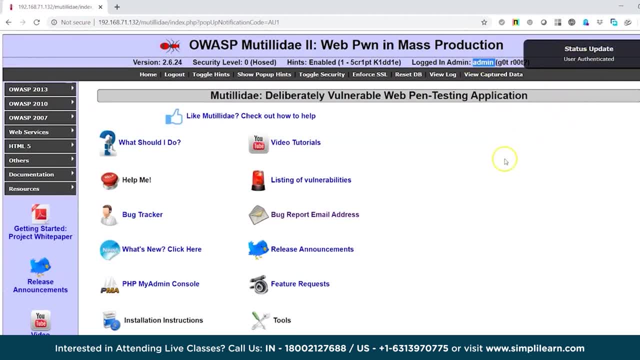 authentication and you can see user has been authenticated and we now have admin access to this application. now here the sql queries need to be crafted in such a perspective that they're going to work, so there would be a lot of exercise in identifying what the database is. there's a 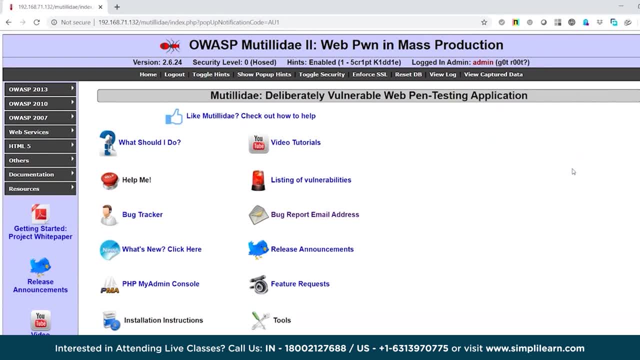 microsoft database and oracle database and so on, so forth, and then you have to choose those proper commands. but identifying that would come in the training. right now we're just looking at a demo. this is how a sql injection attack works. now let me log out here. similarly, now we are in 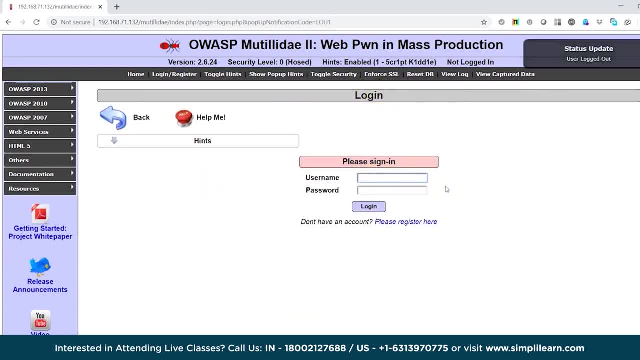 a login page, the same query work wonders where it allowed us to bypass authentication. so it also depends on what kind of a page i am and what query would be accepted at this point in time. so here application understanding would also come into the picture. where, uh, which function we are? 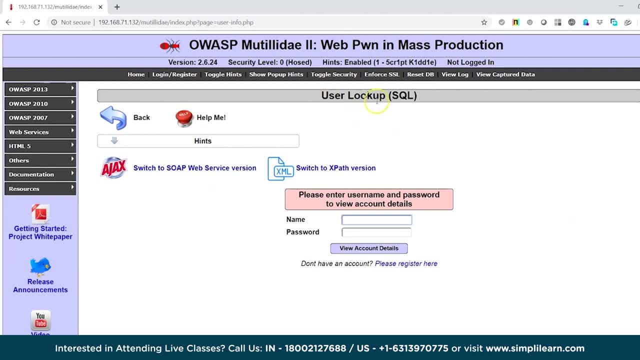 calling upon when we are connected to a particular page. now, this is a user lookup function. right, so again here we try the same method. test, test. that's not going to work. authentication error, bad user on password. and if we type in the same query over here, single quote. 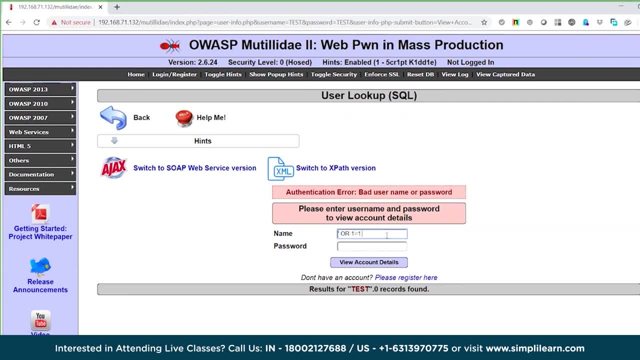 or, and give it a condition: single quote, or one equals one high space, hyphen, hyphen space. now here it is not going to log us in because this is not a login page. this is a user lookup form, so here it would instead give us a dump of all the databases that it has, so you can see all the 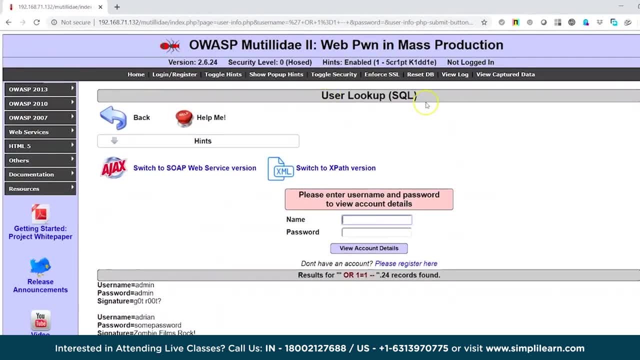 usernames and passwords coming in that are stored in the user lookup function. so let's go ahead and look at the user lookup field. so this is where the understanding comes in of which query to create, at what page we are, depending upon the function that has been called right? so that's the sql. 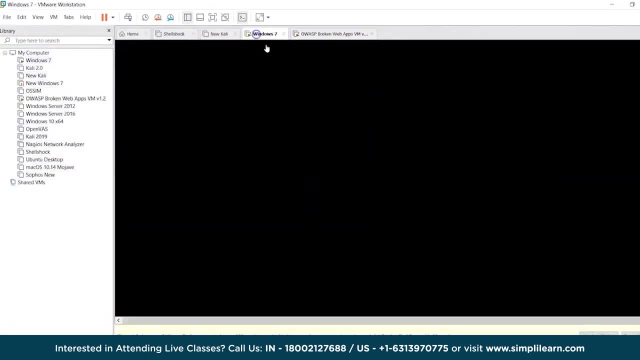 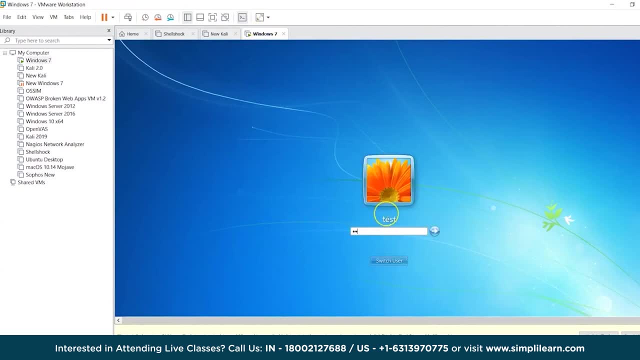 injection attack that we wanted to look at. let's move on to password cracking now. this is a windows 7 machine that we have. i'm just going to do a very basic password tracking example. we're just going to log in now. here, the assumption is that we are able to log in. we have access to a computer. 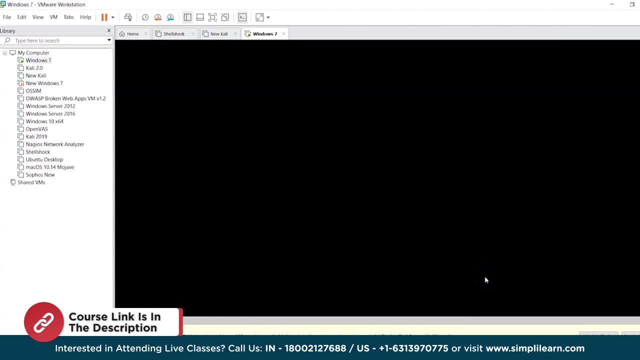 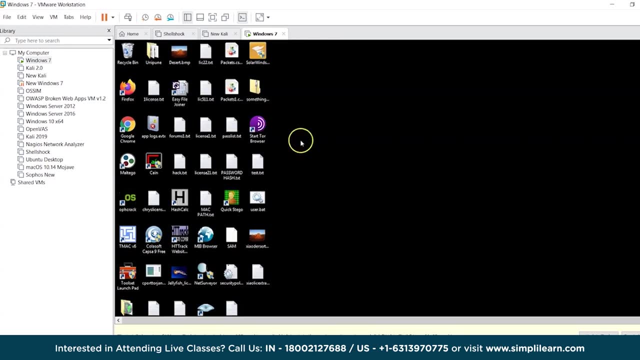 and we want to check out other users who are using this computer and see if we can find out their passwords so that we can log in as a different user, steal data if required, and we wouldn't be to blame if there are any logs that are created. so here we've got a tool called cain. 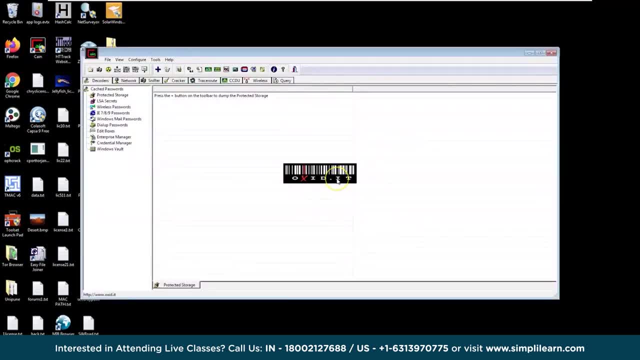 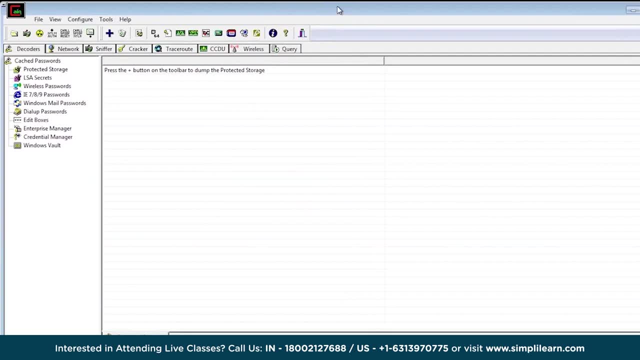 and able that is installed right here. now i'm already an administrator on this machine and checking out other administrators who share the same privileges or any other user who may be on this system whose password i can crack, and thus i would be able to get access through their account and then do any malicious activity right. so this allows me to do some kind of. 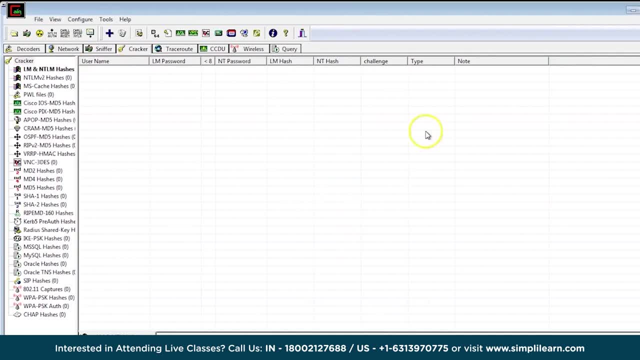 me to go into a cracker tool and it allows me to enumerate this machine and identify all the users and passwords that are there in this particular machine, right? So I'm just going to click on the plus sign and I'm going to import hashes. 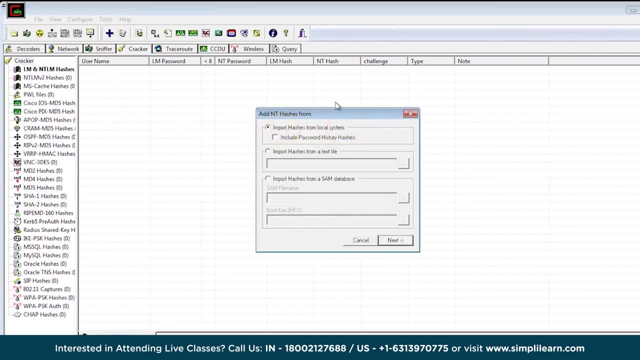 from a local system. So where are these files stored? Where does Windows store its passwords? In what format are they stored And what this tool does to retrieve those? That's something that we all need to know as ethical hacker. right? So import the hashes from the local system, click on next. 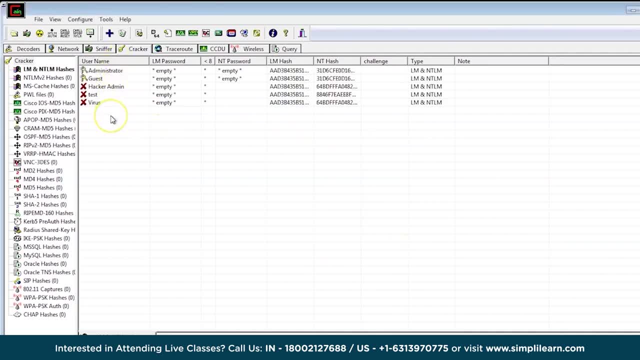 it's going to enumerate that file and it is going to give you a list of all the users that are there, So you can see the users are hacker, admin test, the one that we are logged in as, and then there's a user called virus as well, And you 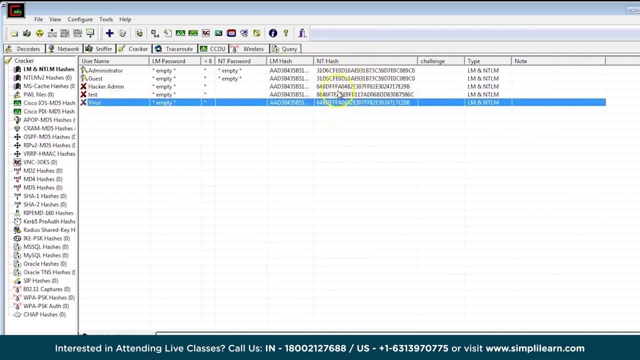 can see that this is the hash value of the password that is being utilized. Now there's a particular format for the hash value for Windows and how it stores. But once we have these hash values, let's say, if I want to crack this password there. 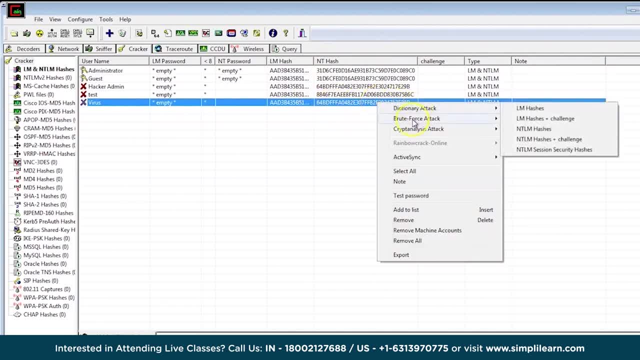 are various attacks that we can do, For example, a dictionary based attack or a brute force attack. Let's try a brute force attack right. NTLM is the hashing mechanism that is used by Windows, So we're going to try to create an NTLM hash attack, And here we are going to use a. 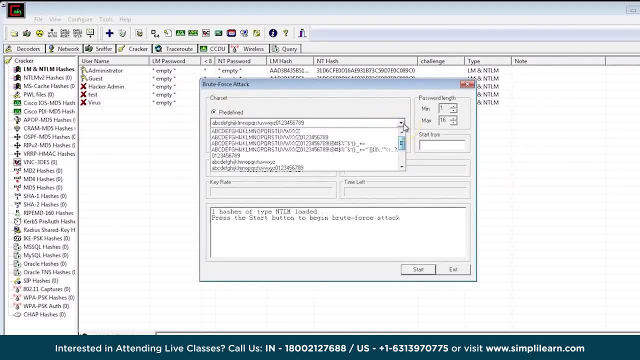 predetermined rule set. For example, we are not sure what characters are being utilized over here, So we just create an attack like this, using all characters and lowercase A through Z, uppercase A through Z, numeric 0 through 9 and all the special characters. 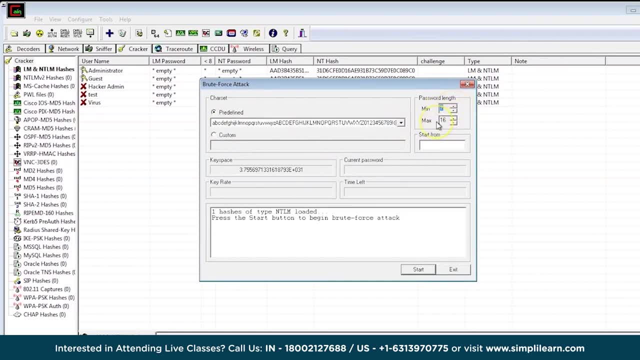 Let's say, the password is between 7 and 16 characters, And this is the character set that we want to try the brute force attack on. What is a brute force attack? It is an attack where the computer is going to try each and every permutation and 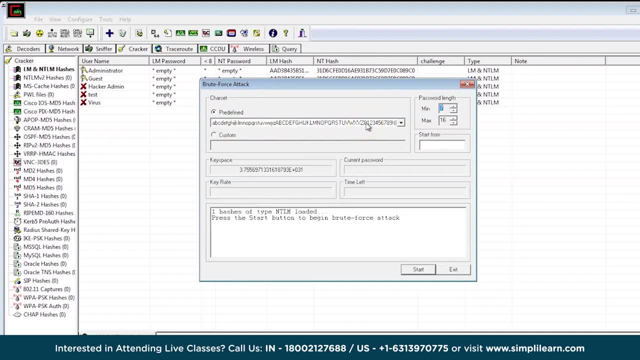 combination out of this character set and try to figure out if the password is going to be correct. So if we click start, it's going to start with a particular characters and then it is going to identify if that NTLM hash is going to work. 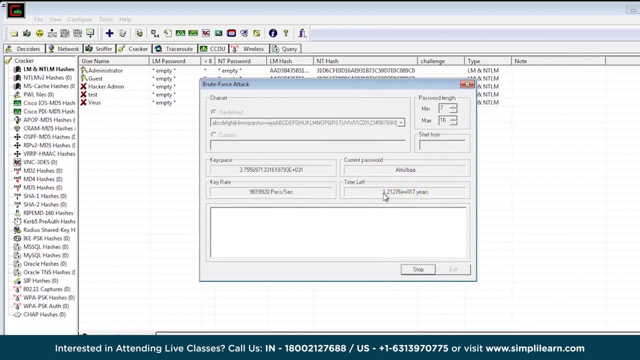 against this character, And you can see the time is going to be phenomenal over here. It's not necessarily that this attack would be viable. It will be 100% successful given the time frame. However, the time frame is huge enough for this attack to become a little bit. 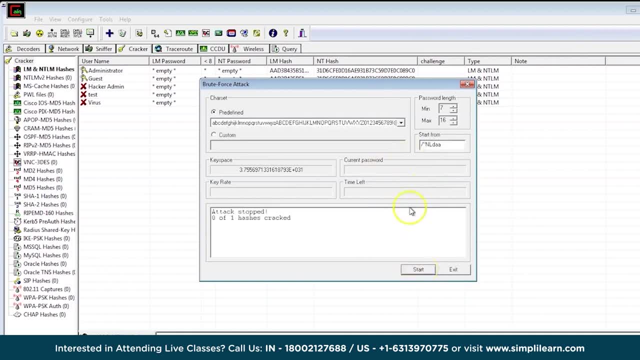 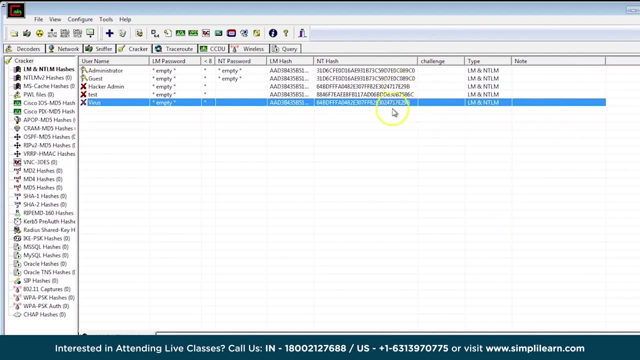 redundant. There are other attacks that we can do which can easily identify this data for us as well, But that is something that we will look on in future videos. So that's how we can get access to users and passwords. There are different mechanisms. 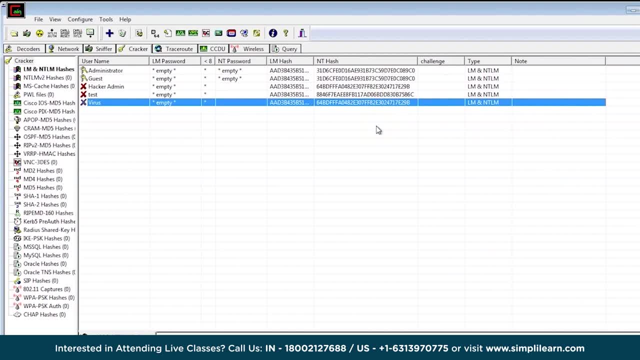 where, let's say, we don't have login access, then what are we going to do? how we can create a fake user login or how we can remotely access a machine and then try to get the same access. And that is what we are going to try to do in the next demo on a 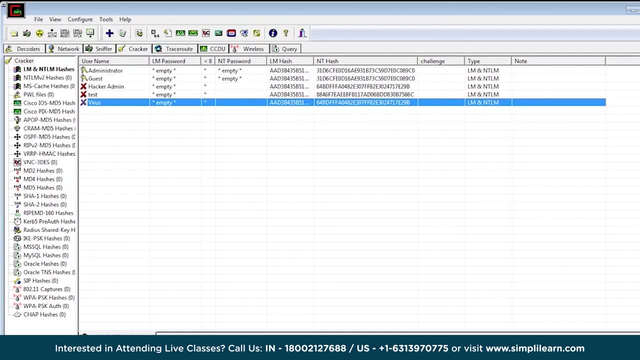 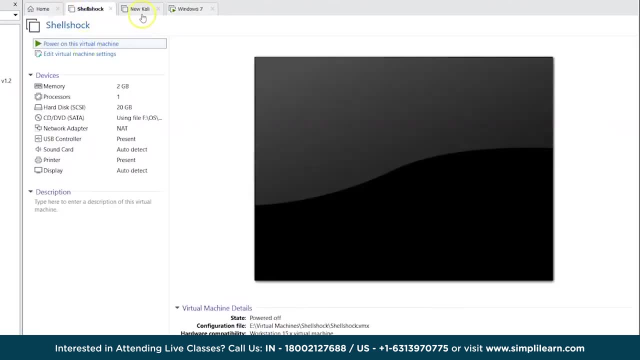 Linux machine. So what we are doing in a Linux machine could also be doable on the Windows machine with a different exploit. So what I'm going to do is this is the Linux web server that I have that I'm going to power on. I'm going to use a. 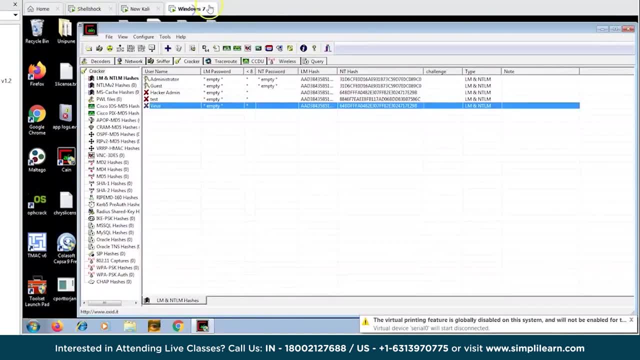 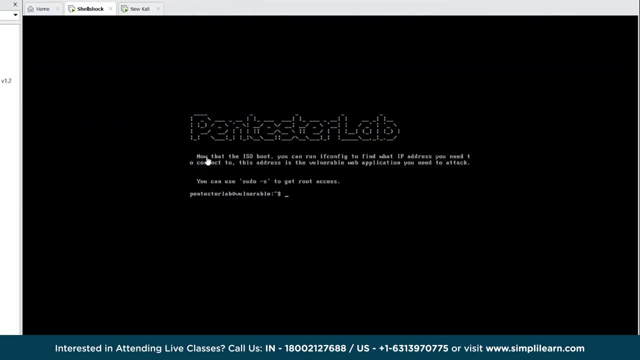 Kali Linux machine to hack that device, and I'm going to just power off my Windows 7 machine. Give it a minute till it boots up. Now, this is also a demo machine that we have, which has own pre-configured vulnerabilities. So here we've got something. 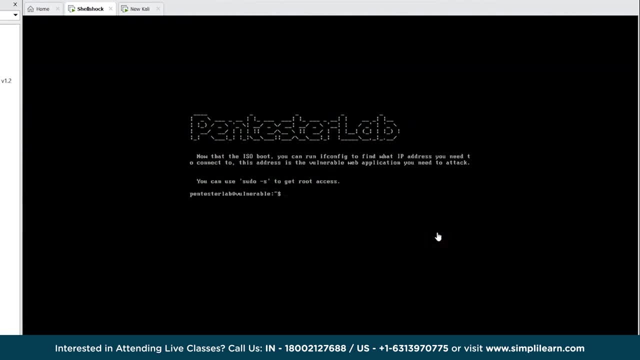 from the Pentester's lab and has a shell shock vulnerability implemented inside. Shell shock vulnerability affects Linux, Mac and Unix based operating systems for a particular version of the bash shell. Bash is the born again shell, which is the command line interface in these operating systems. So what we're trying? 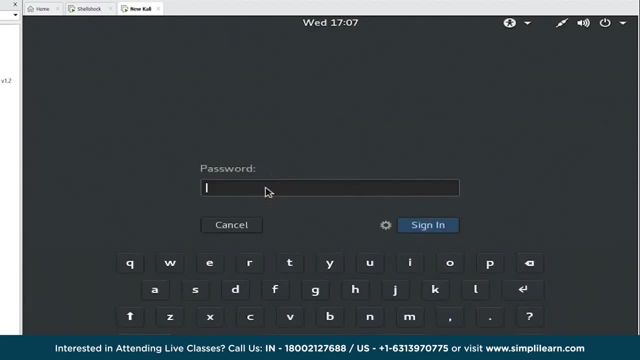 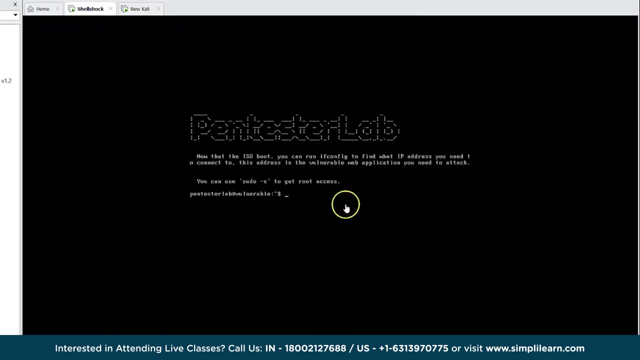 to do here is: we are going to use the Kali Linux machine, try to find out the vulnerability over here And, if it exists, we are going to use Metasploit To attack this machine. Now the first and foremost thing is we 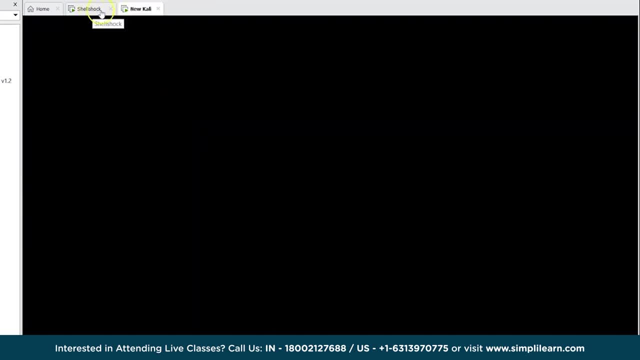 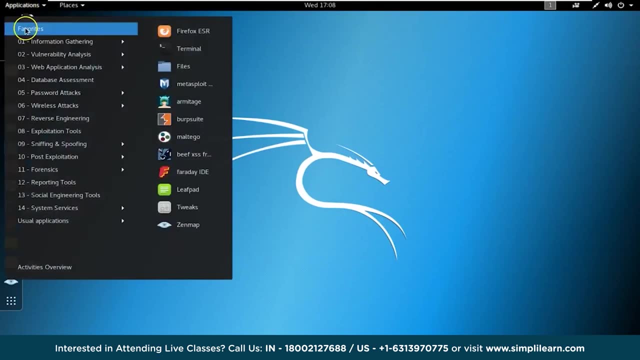 want to identify the IP address. We have no idea what the IP address is. We are in the same subnet, so we are assuming that we're able to connect to this machine. So what I'm going to do is I'm going to open up a tool called ZenMap. I'm going to open 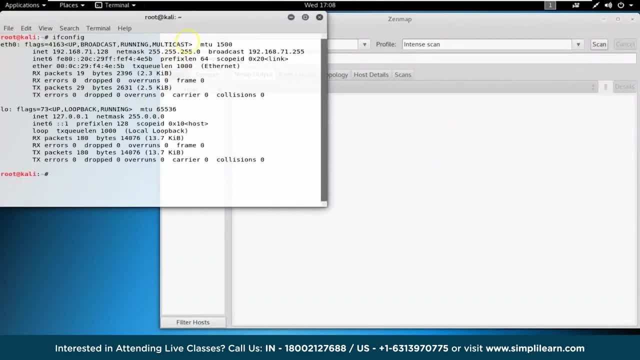 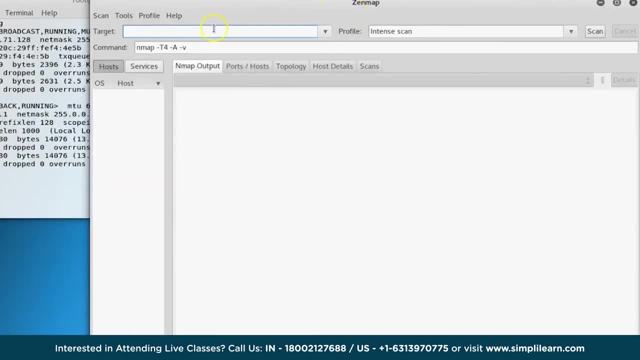 up a command line interface, find out what my IP address is. and my IP address is this, with a subnet mask of 255.255.255.0.. So I want to see if there are any other machines that are live in the same subnet. 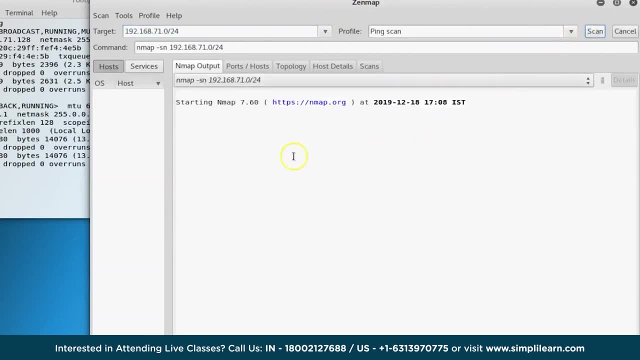 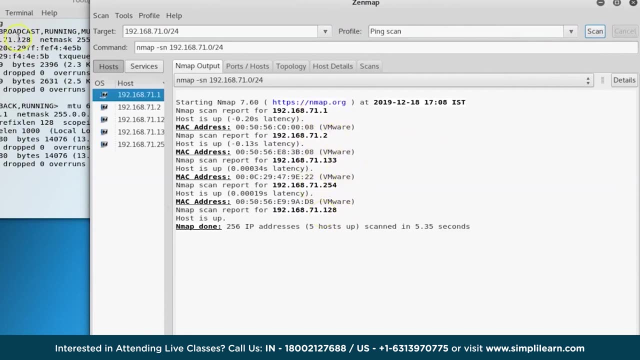 And we are doing a ping sweep over here to identify which machines are live. In a minute we'll get all the IP addresses: 71.1,, 2,, 133,, 254, and 128.. We know that we are 128 at this point in time. 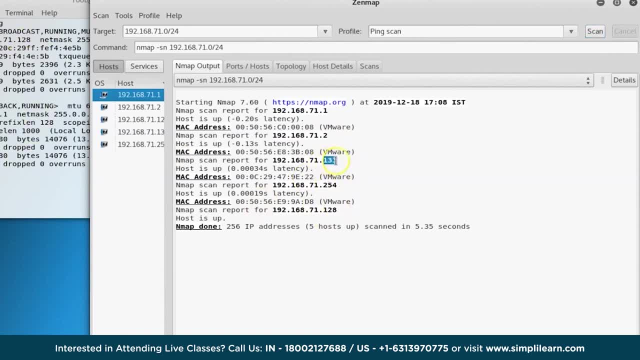 254 is the DHCP server. So we are assuming that 133 is the machine that we want to look at And let's then try to see if we can scan that machine 133.. And we're going to do an intense scan to find out which ports are open, what services are running over. 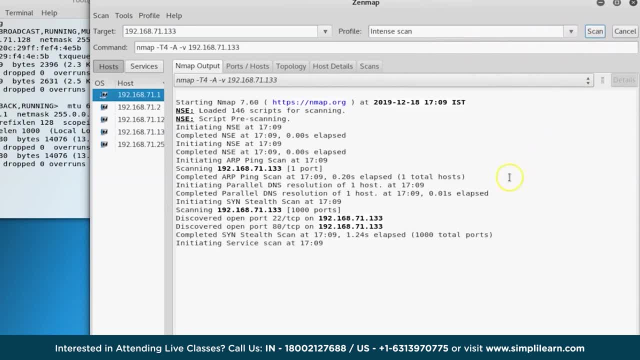 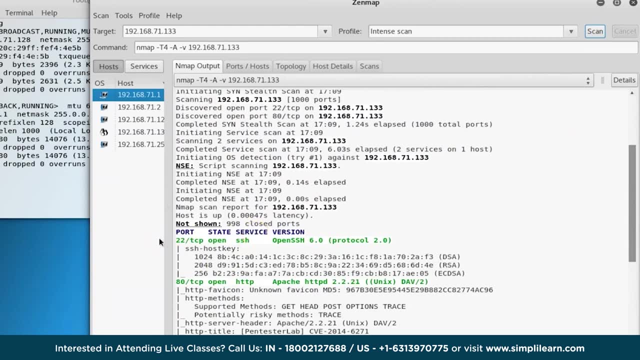 there And if it is open then we can see that we have a Pintest lab machine that we were looking for. You can see of the start, port 22 and port 80. And somewhere here it's going to give us the ports that are open. 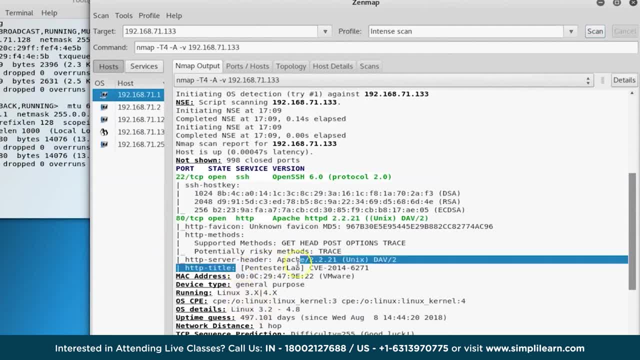 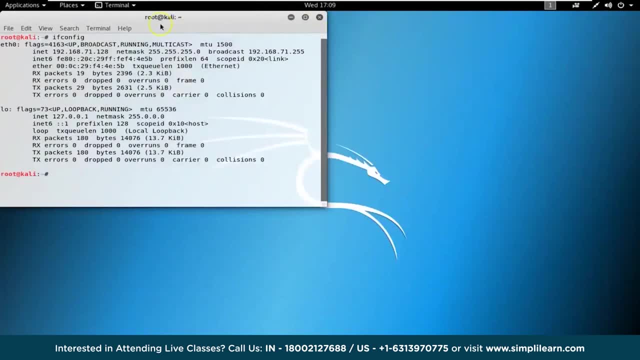 and the details about those ports, And somewhere here it will tell us that this is the Pintest lab machine that we wanted, which is correct. So now we want to do a vulnerability analysis on this. What we are going to do is: I'm going to use another GUI. 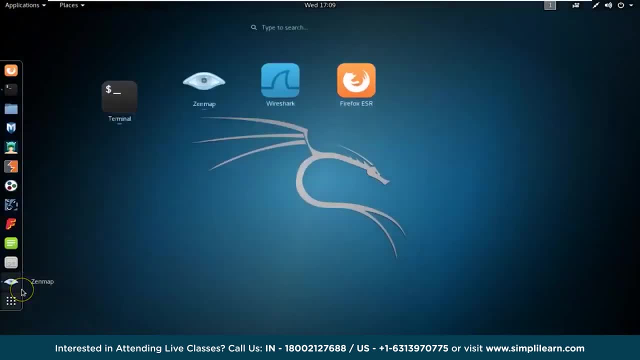 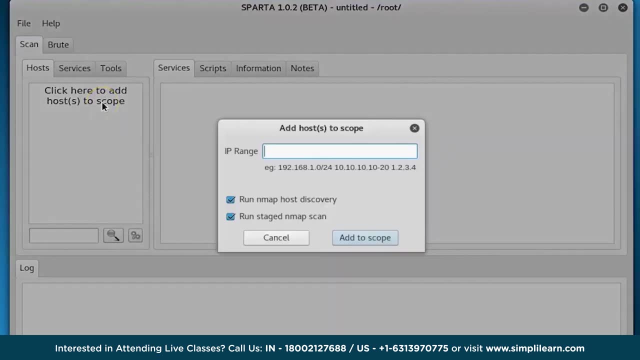 based tool called Sparta, which I can just find out from here. Sparta uses two tools in the background: a Nmap tool and a tool called Nicto. So we're just going to start scanning. 192.168.71.133. 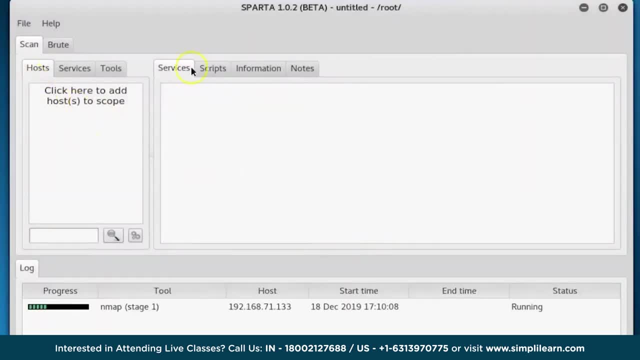 was the IP address, Add to scope And over a period of time you can see all of these will start populating with information. There we are. That's the Nicto tool coming in, scanning on port 80, which means 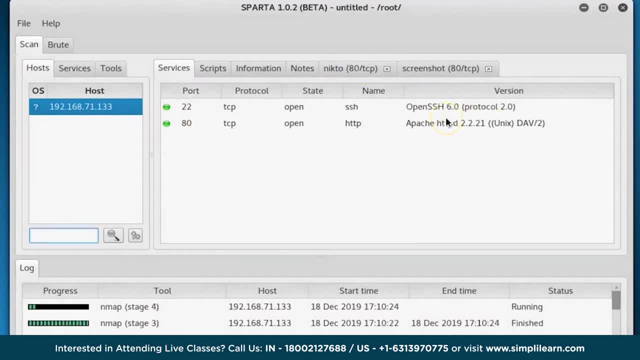 that it's a web server using HTTP. It tells us it's an Apache, HTTP 2.2.21.. And that gives us the 22 port number as well, If we head over to the tab of Nicto, or let's look at the screenshot. 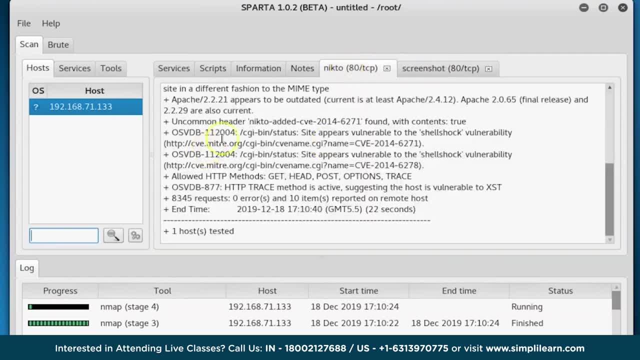 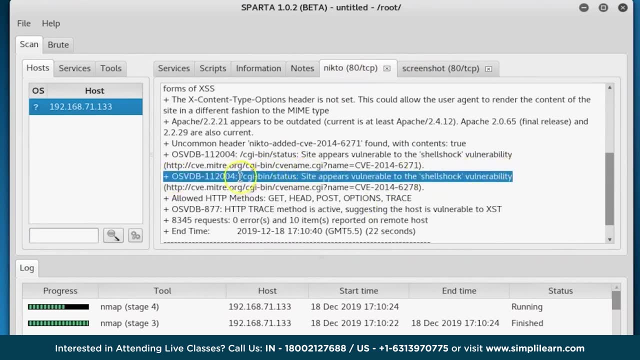 first, this is what the website would be looking like, And Nicto gives us the options over here. It tells us that there is a vulnerability over here for Shellshock And this is the path where the vulnerability is going to exist. So what we're? 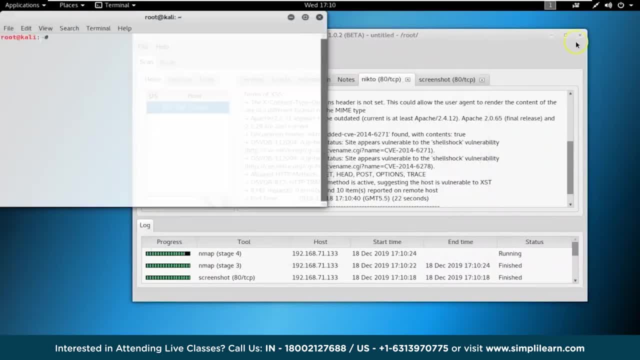 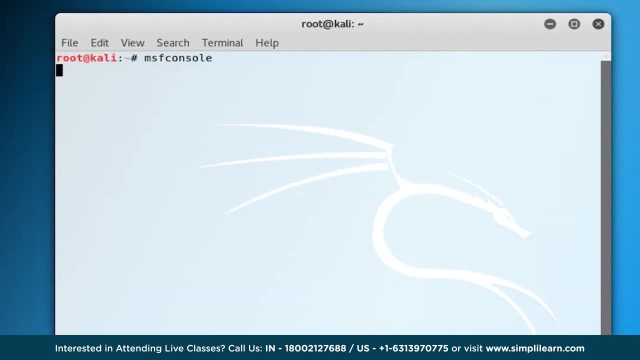 going to do? we go back to the command line so we open up a new one, minimize all these other windows and we're going to open up Metasploit. Metasploit is a penetration testing tool that is used by most hackers and ethical hackers to test applications and test. 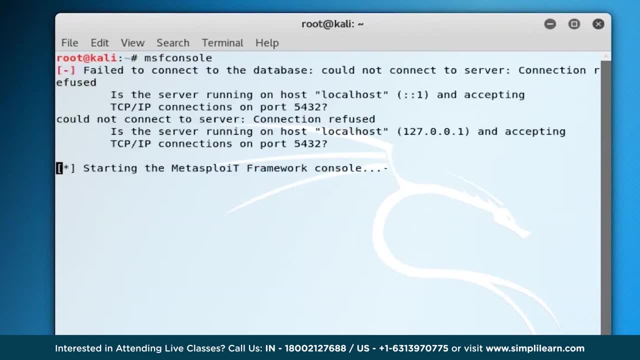 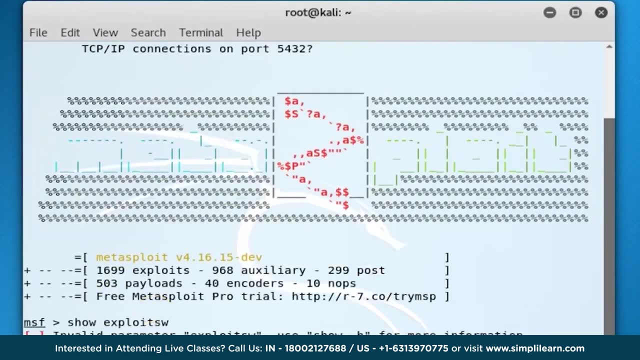 existing exploits and vulnerabilities. So just give it a minute till it starts. You can see there are already around 1700 exploits right here. We're going to see all those exploits with these commands There. we are sorry for the typo And it. 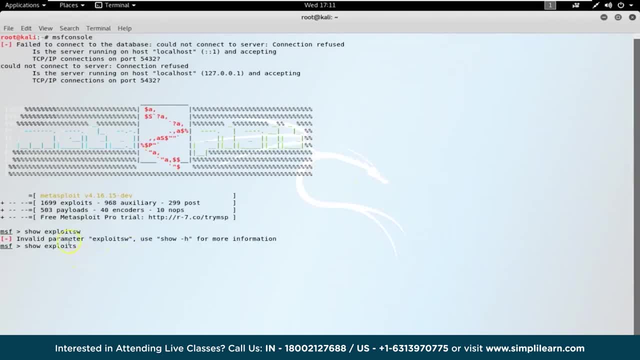 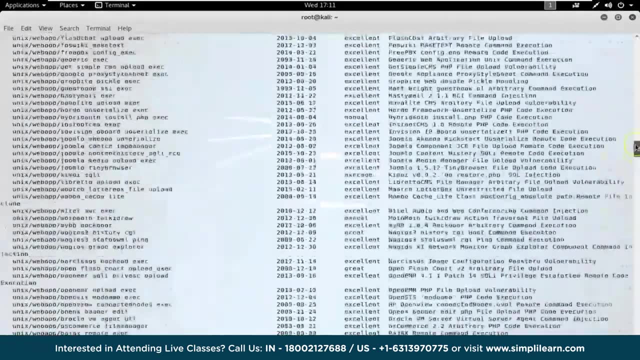 will just give us a list of all the exploits that are stored in Metasploit in this version. So all of these are Windows based. If we scroll up, we will be looking at other vulnerabilities as well, Or exploits, the Unix based exploits, Linux, OSX, multi. 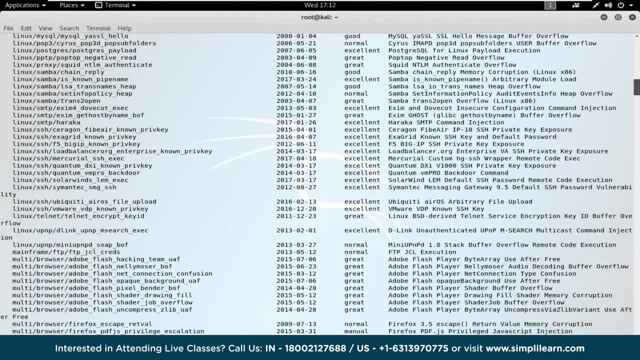 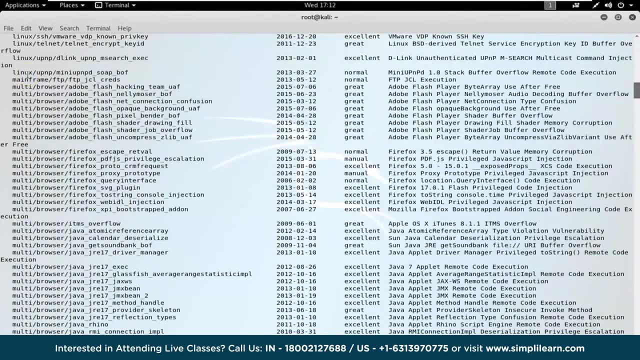 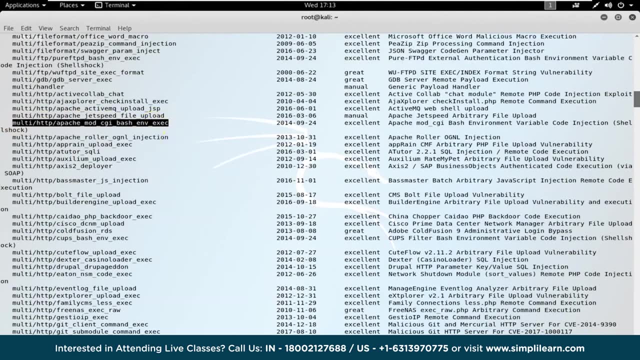 exploits And we're looking for a exploit for multi based Apache or HTTP. Let's go up, Let's look at. so this is the one that we're looking for: Apache mod, CGI, bash, environmental executable. So what we're going to do is we're just going to copy it go. 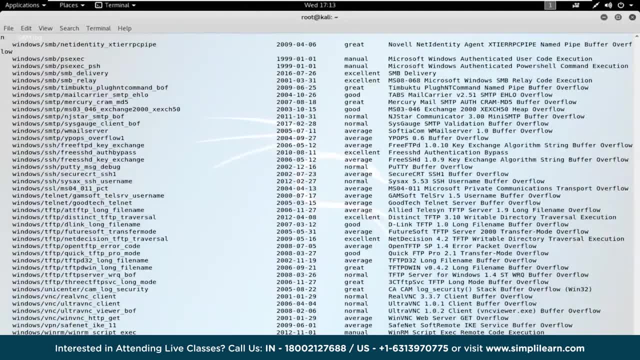 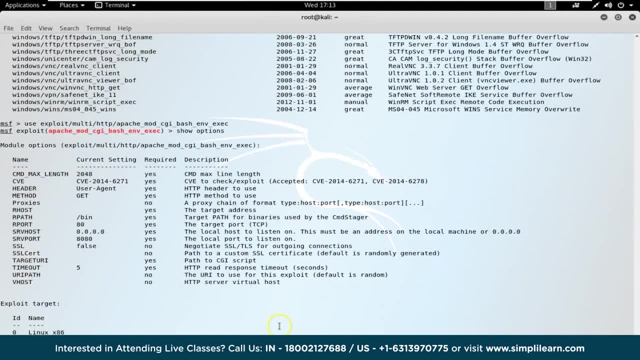 back to the bottom, say: use exploit and paste the one that we wanted. Press enter say show all Options. So it'll ask us to configure this. I'm just going to configure it based on the knowledge that we have Set our. 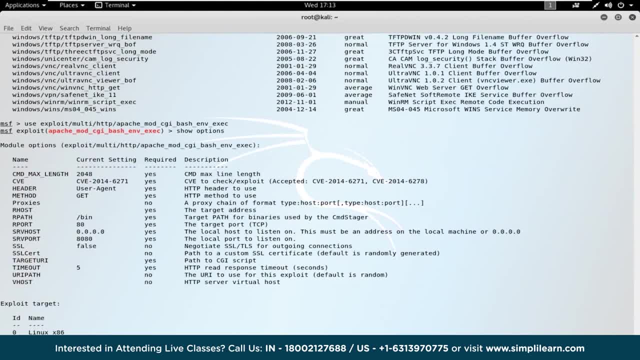 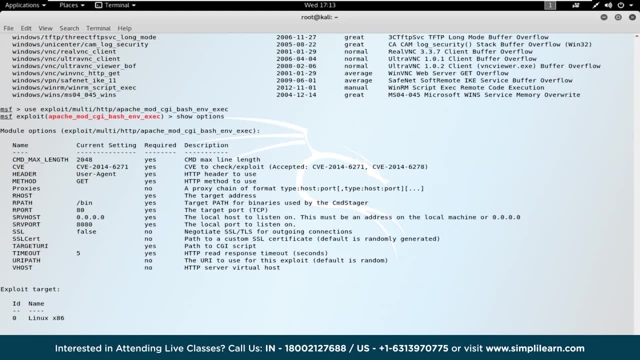 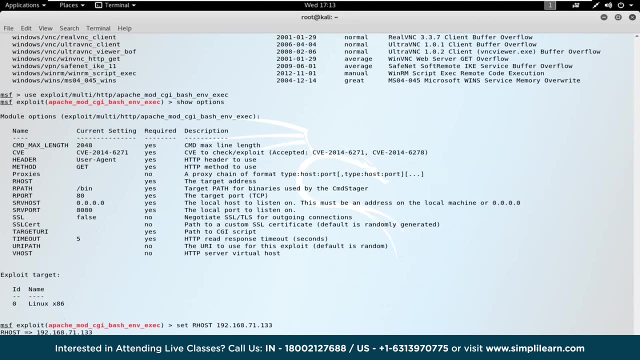 host, which is the remote host, the victims machine. So we put in the IP address. It asks us for the target URI. So that's the path that we saw: Set target URI to CGI hyphen bin, slash status, Enter. Now with the exploit, we need to find a. 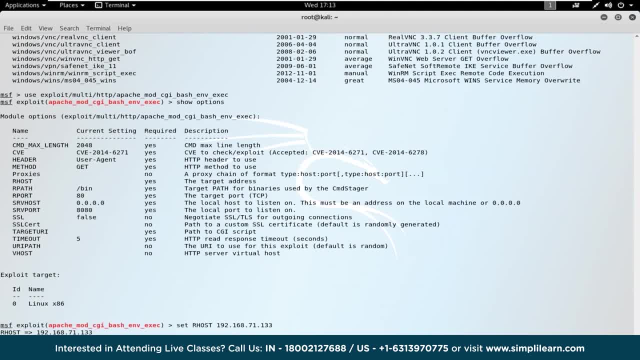 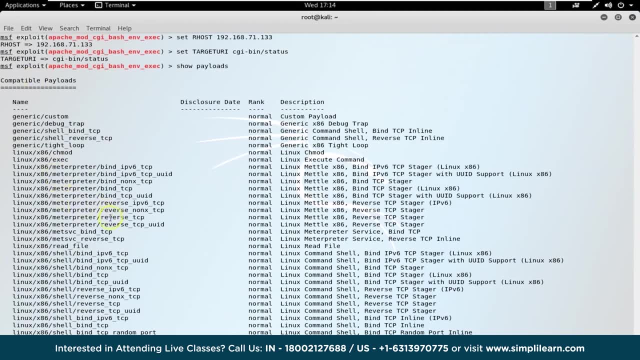 payload that is going to give us the output that we want. So we say show payloads And it will give us a list of all the compatible payloads with this exploit. And we want to create a reverse TCP connection, which is this: So we know it's a Linux operating system We want. 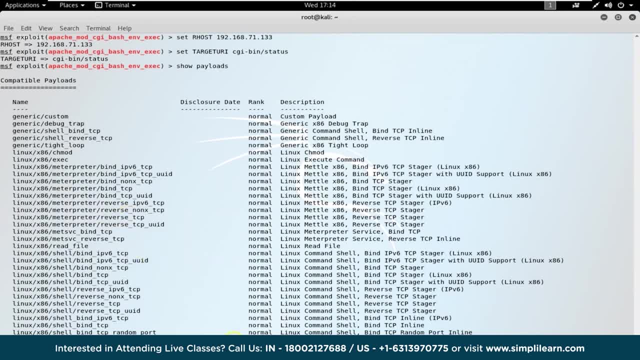 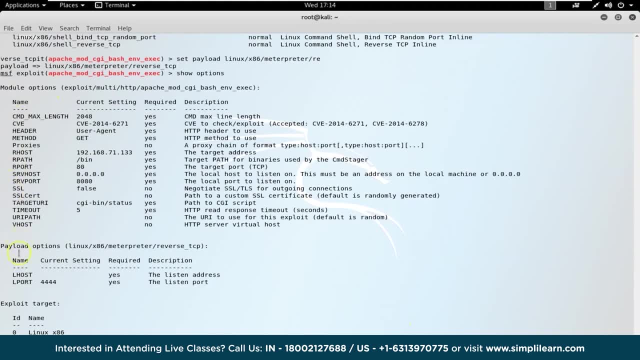 this payload to be set. So set payload. Press enter. That's the payload coming in. Show options: Now that we have set the payload, this is the options for the exploit, And now we want to set our options for the payloads as well. So we are. 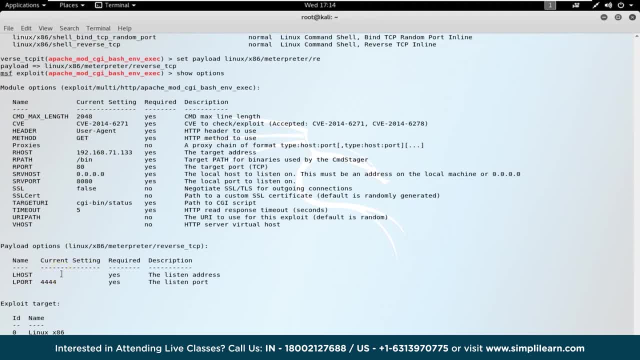 creating a reverse TCP connection, which means we are remotely executing code at the victim side and making the victim connect back to our machine, which means we need to set up a listener. So I need to put my IP address over here, Set localhost or lhost, 192.168.71,, not 128, which was our IP. 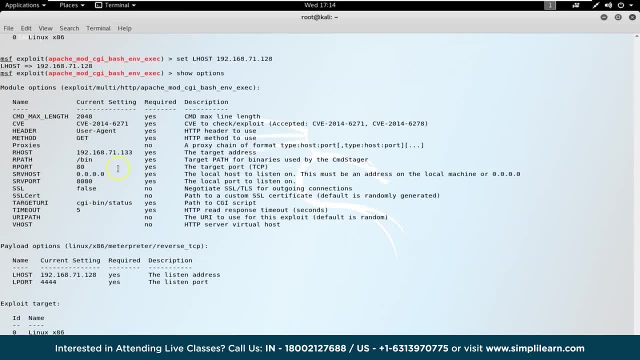 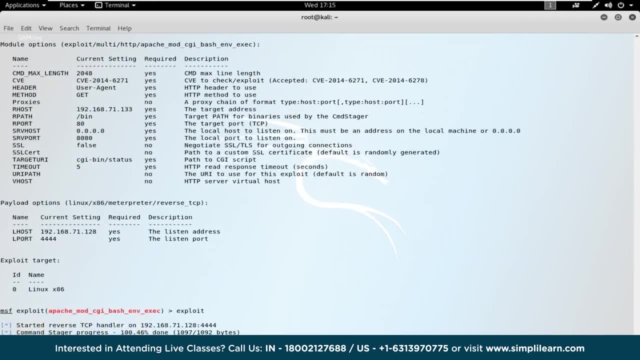 address, Show options again, just to ensure everything is fine, which looks like it is, And we then type in the word exploit so that it will start this attack. I can see that it has created a meter breeder session at the victim side and 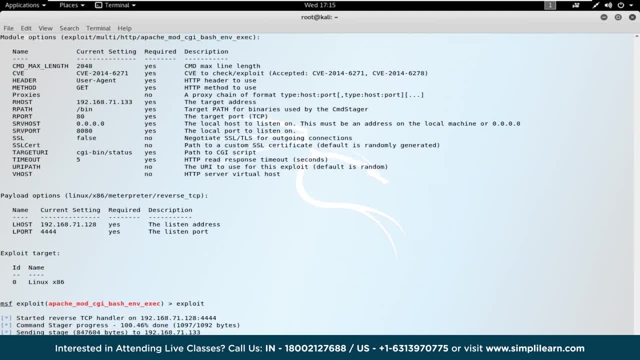 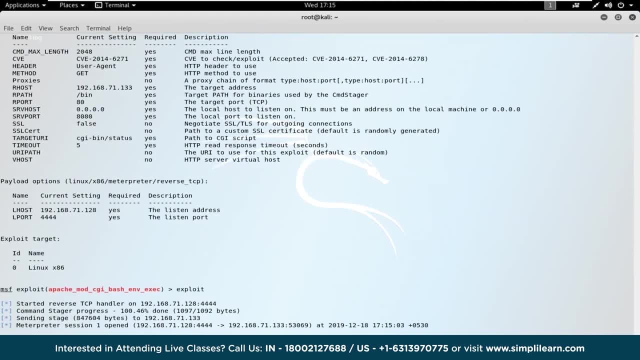 it has opened up a session. So if I do a PWD now, PWD is a Linux command for present working directory and it will show us that we'll connect it to var wwwcgi-bin. Do an ls, It will list all the files. That's the status file. 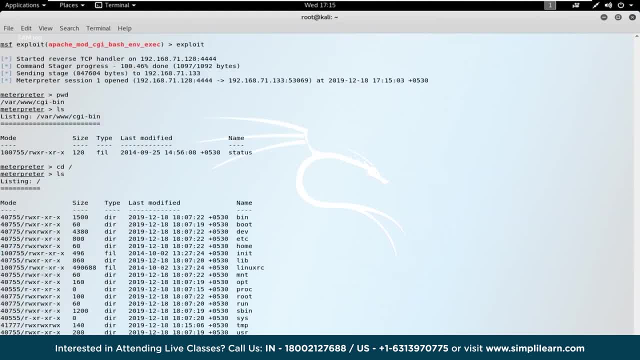 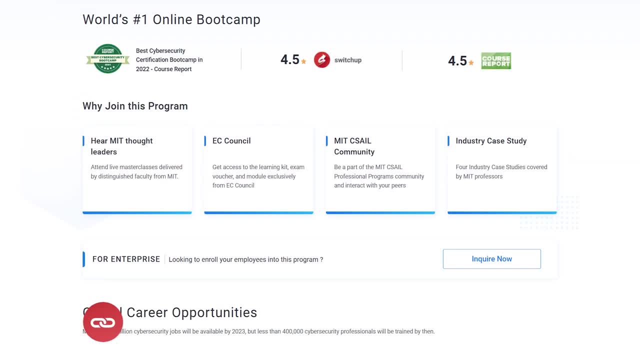 over there, Do a cd backslash. It will take us to the root of this machine And if you're someone who is interested in building a career in cybersecurity, that is, by graduating from the best universities, or a professional who elicits to switch careers with cybersecurity by learning. 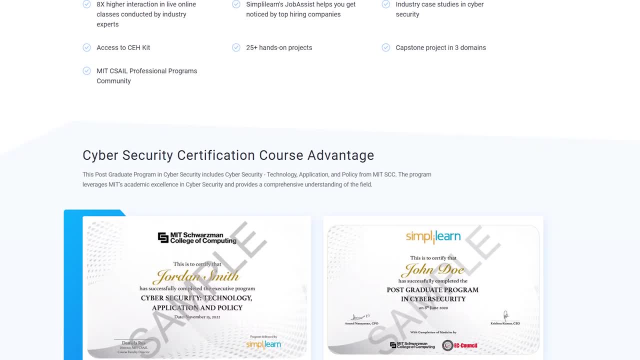 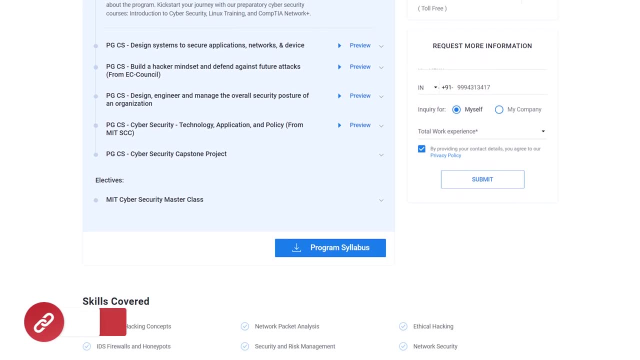 from the experts. then try giving a shot to Simply Learn's post-graduate program in cybersecurity With modules from the MIT Schwarzman College of Engineering, and the course link is mentioned in the description box. that will navigate you to the course page where you can find. 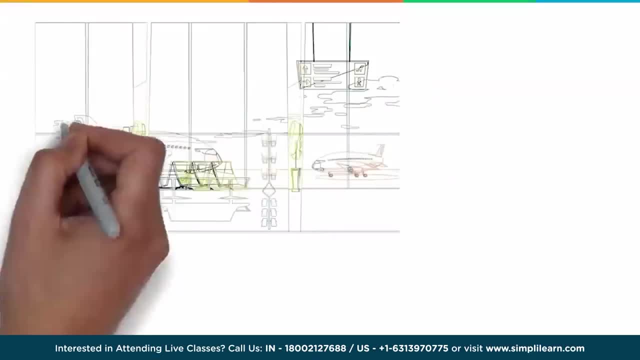 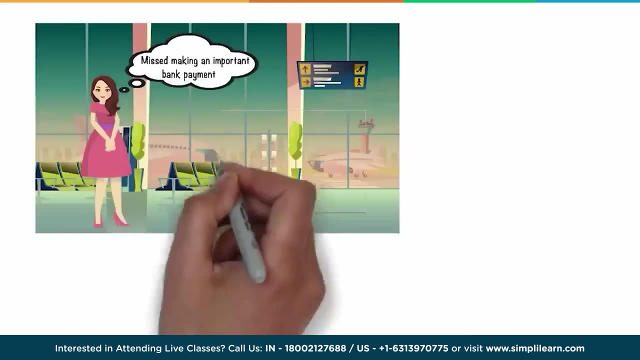 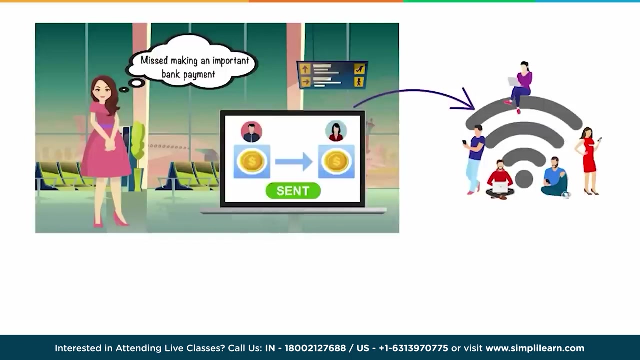 a complete overview of the program being offered. Jude is waiting at the airport to hop on her flight back home when she realizes that she missed making an important bank payment. She connects her laptop to the public Wi-Fi at the airport and goes ahead to carry out the bank transaction. Everything goes well. 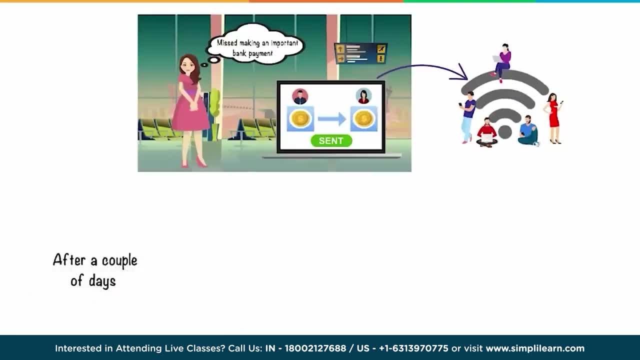 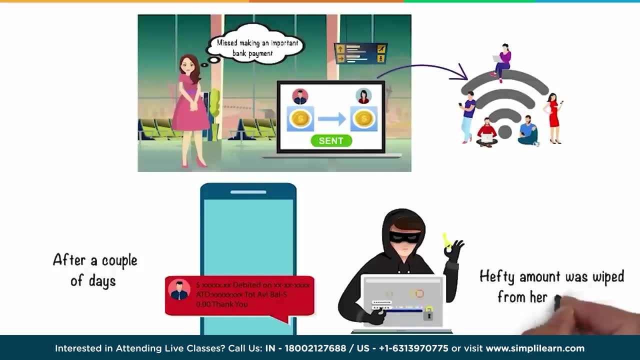 and Jude completes her transaction. After a couple of days, she was wiped off her feet when she learned that her bank account was subjected to a cyber attack and a hefty amount was wiped from her account. After getting in touch with the bank authority, she learned that her account was hacked at the airport. 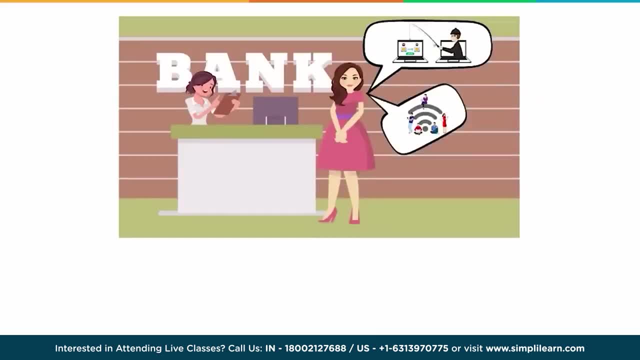 She then realized that the public Wi-Fi she used might have caused her this trouble. Jude wishes that had her bank transfer escaped the hacker's eyes, she would not have been a victim of a cyber attack. Bank officials advise her to use a VPN for future. 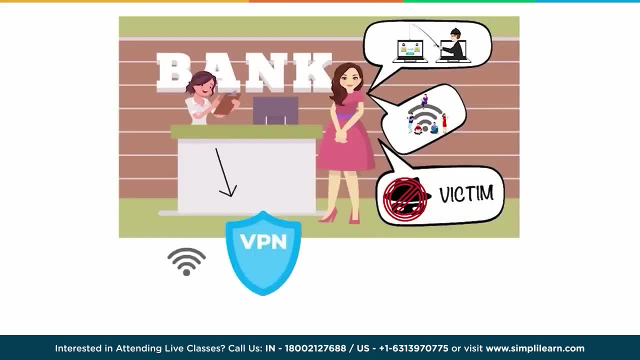 transactions, especially when connecting to an open or public network. Like most of us, Jude had come across the term VPN several times but didn't know much about it, and little did she think that the repercussions of not using a VPN would be this bad. 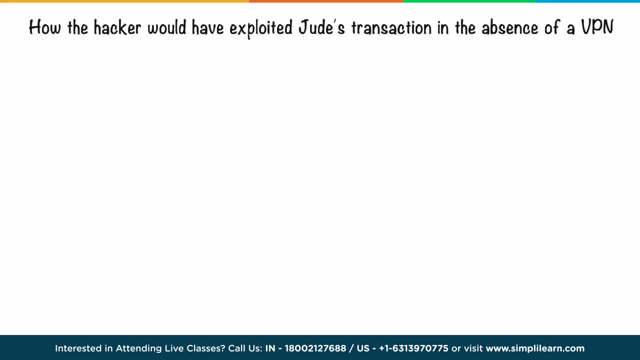 Let's understand how the hacker would have exploited Jude's transaction in the absence of a VPN. In this process, Jude's computer first connects to the Internet Service Provider which provides access to the Internet. She sends her details to the bank's server using her IP address. 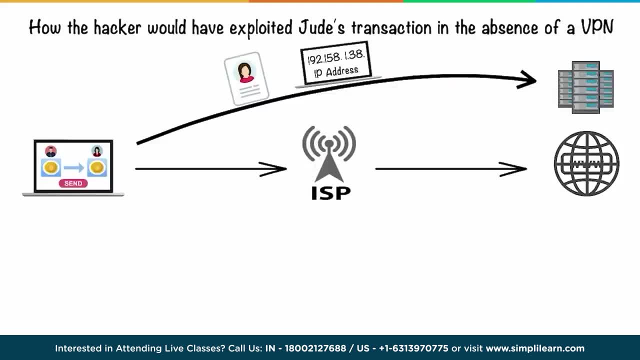 Internet Protocol Address, or IP address, is a unique address that recognizes a particular device, be it a laptop or a smartphone, on the Internet. When these details pass through the public network, the hacker, who passively watches the network traffic, intercepts it. 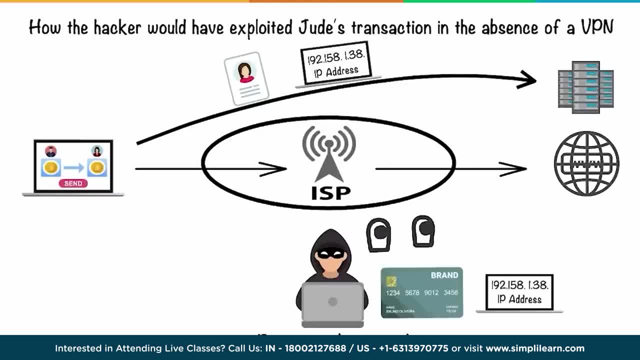 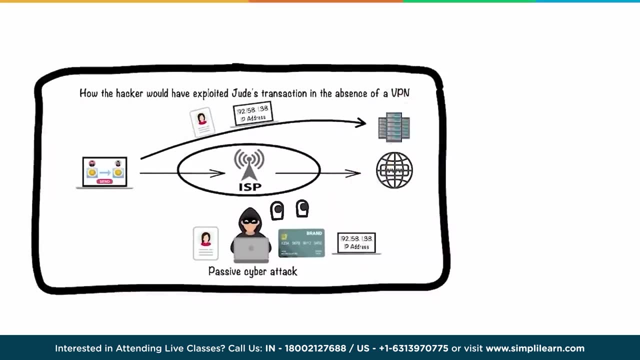 This is a passive cyber attack where the hacker collects Jude's bank details without being detected. More often or not, in such an attack, payment information is likely to be stolen. The targeted data here are the victim's username, passwords and other personal information. Such an unsecured connection exposed Jude's IP address and bank. 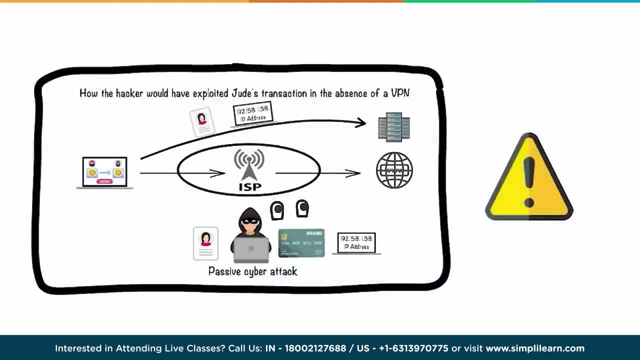 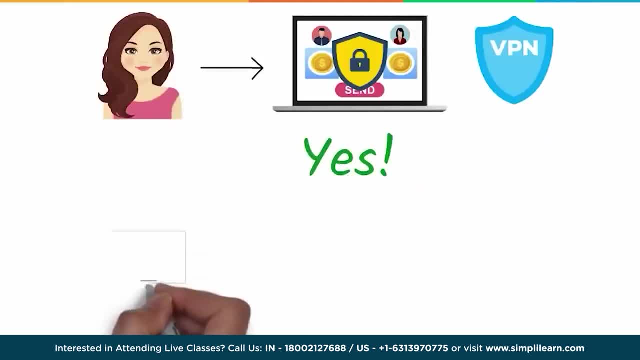 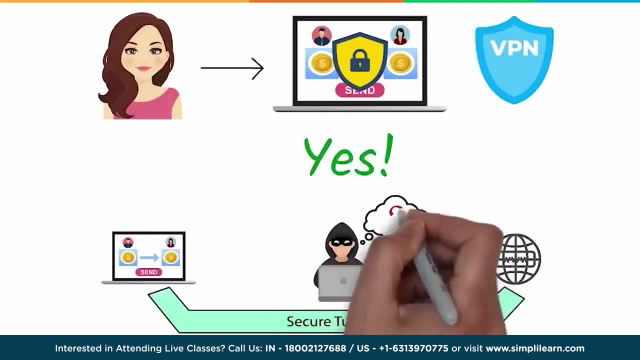 details to the hacker when it passed through the public network. So would Jude have been able to secure her transaction with the help of a VPN? Well, yes, Picture Jude's bank transaction to be happening in a tunnel that is invisible to the hacker. In such a case, the hacker will not be able. 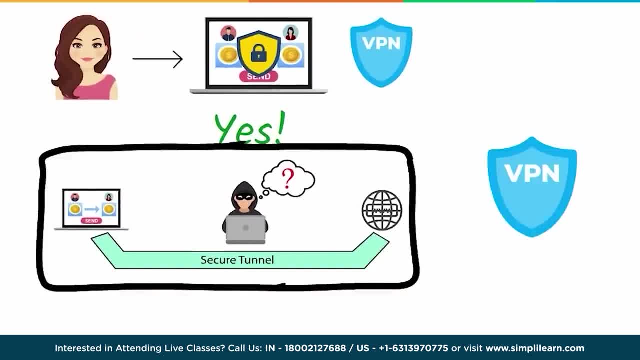 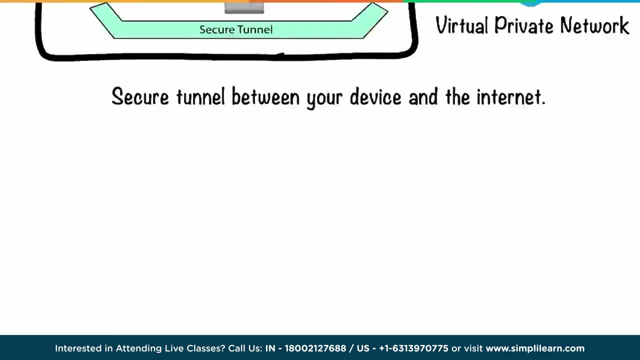 to access it, And that is precisely what a VPN does. A virtual private network, more often known as VPN, creates a secure tunnel between your device and the Internet. For using a VPN, Jude's first step would be to install software-based technology, known as the VPN client, on her. 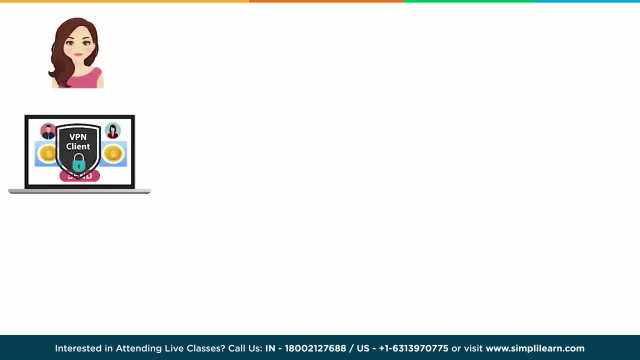 laptop or smartphone that would let her establish a secure connection. The VPN client connects to the Wi-Fi and then to the ISP. Here the VPN client encrypts Jude's information using the VPN protocols. Data is encrypted to make sure it is secure. Next, the VPN client establishes a VPN. 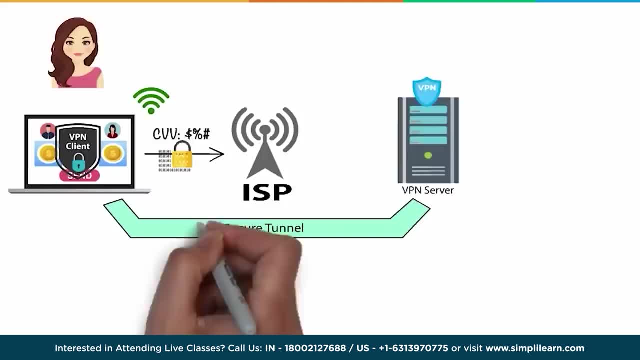 tunnel within the public network that connects to the VPN server. The VPN tunnel protects Jude's information from being intercepted by the hacker. Jude's IP address and actual location are changed at the VPN server to enable a private and secure connection. Finally, the VPN server connects to: 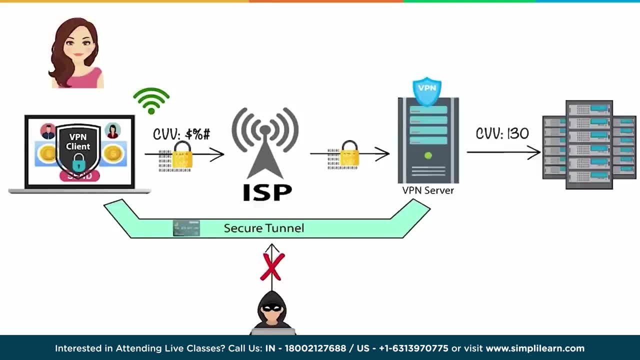 Jude's bank's server in the last step, where the encrypted message is declared. This way, Jude's original IP address is hidden by the VPN and the VPN tunnel protects her data from being hacked. This explains how VPN makes your data anonymous and secure when it passes. 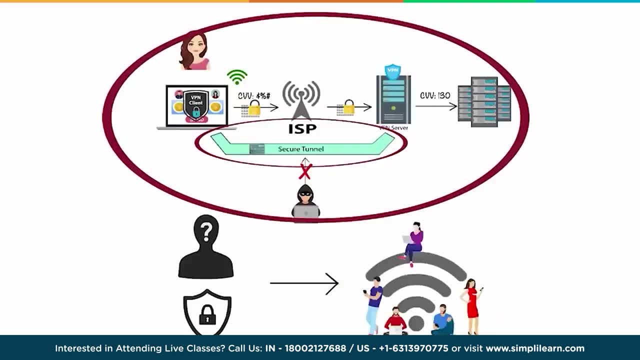 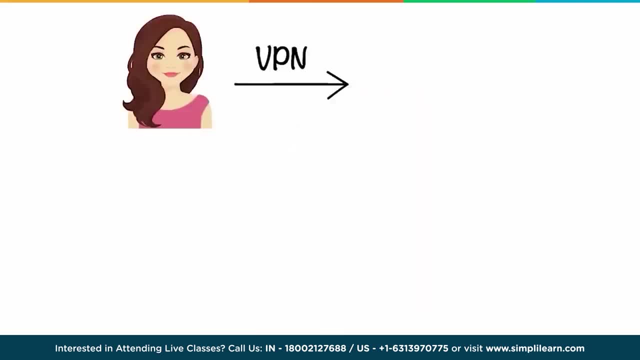 through the public network and the difference between a normal connection and a VPN connection. After learning about this, Jude was certain that she should start using a VPN to carry out her online transactions in the future. This is also applicable to each one of us, Even if you work. 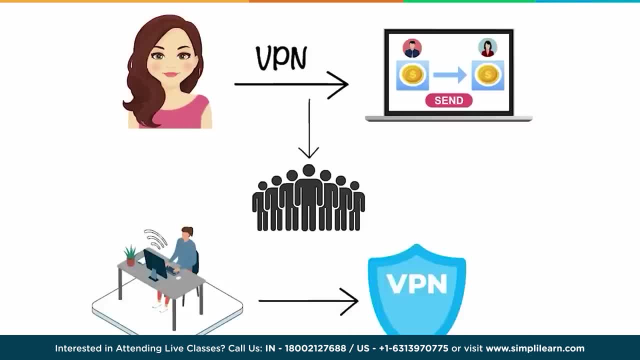 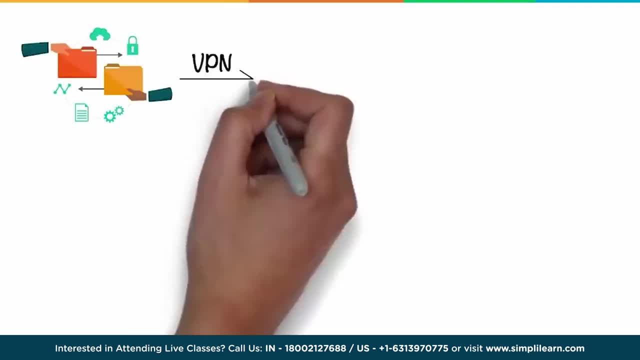 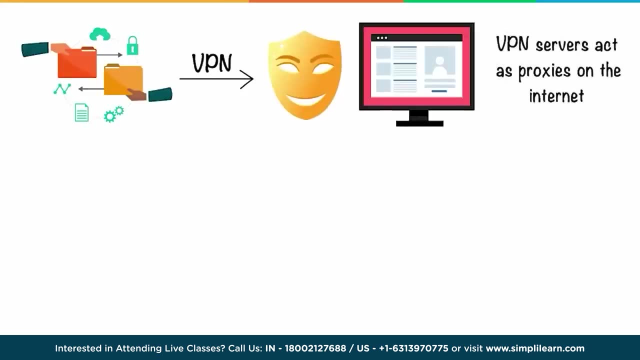 remotely or connect to public Wi-Fi using a VPN is the safest option. In addition to providing a secure, encrypted data transfer, VPNs are also used to disguise your whereabouts and give you access to regional web content. VPN servers act as proxies on the 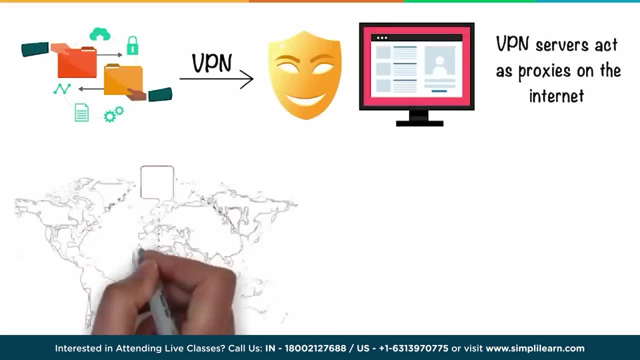 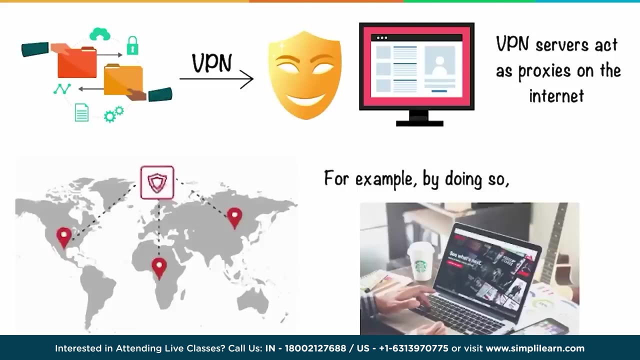 internet. This way, your actual location cannot be established. VPN enables you to spoof your location and switch to a server to another country and thereby change your location. For example, by doing so, you can watch any content on Netflix that might be unavailable for your region. Meet Jonathan. He is an investigative. 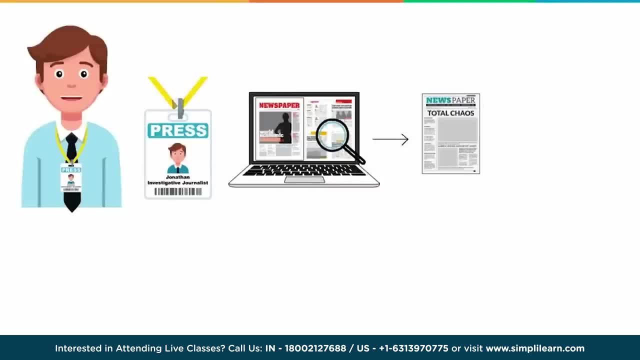 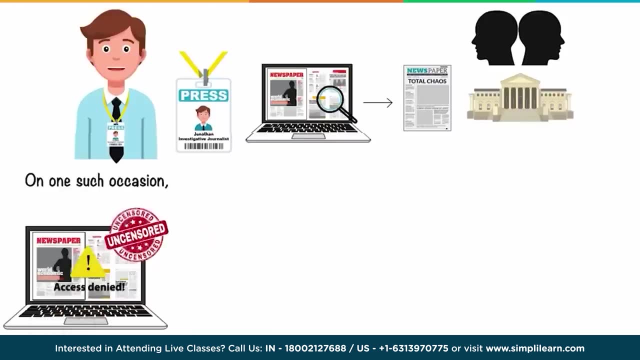 journalist who occasionally researches and publishes news articles contrary to the government's ideologies. On one such occasion, he could not access a global news website dealing with uncensored information. It seemed his IP was blocked from visiting the news website. With his IP blocked, Jonathan turned to a popular proxy service. 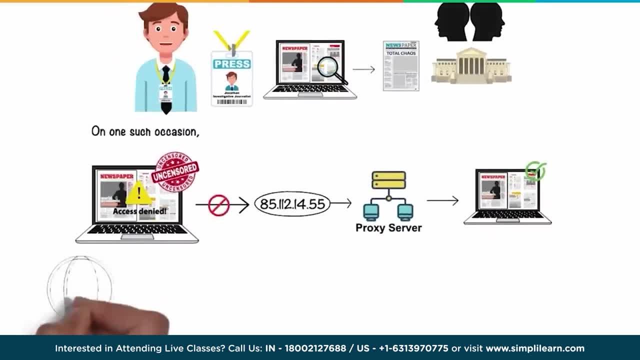 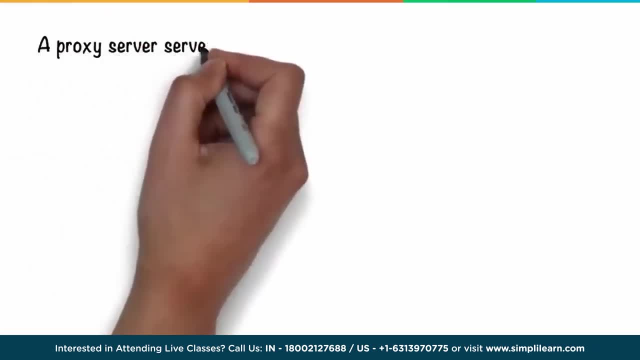 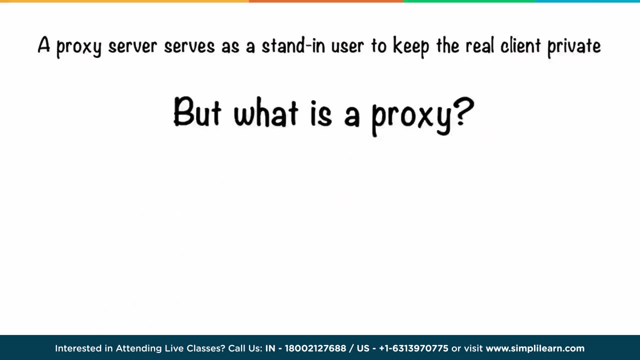 that was able to unblock the news website, thereby allowing an open internet to all users, Just like how your friend gives a proxy attendance for you. a proxy server serves as a stand-in user to keep the real client private. But what is a proxy? Let's understand. 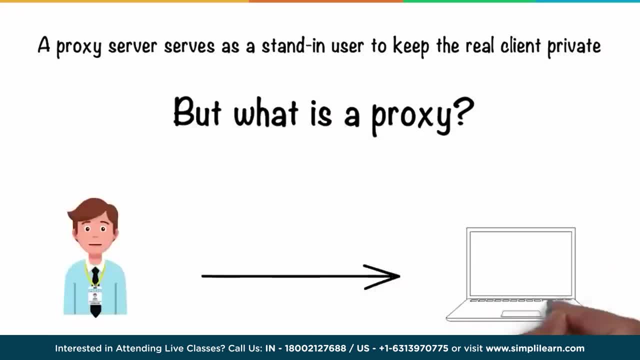 its working by taking a look at how Jonathan was able to access geo-blocked content without much hassle. A proxy server acts as a gateway or intermediary server between a user and its destination. This is a gateway or intermediary server between a user and its destination. 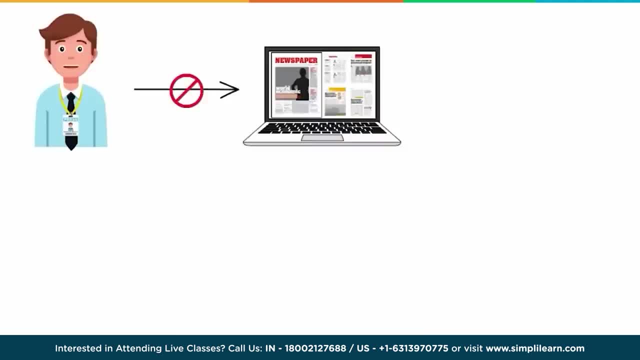 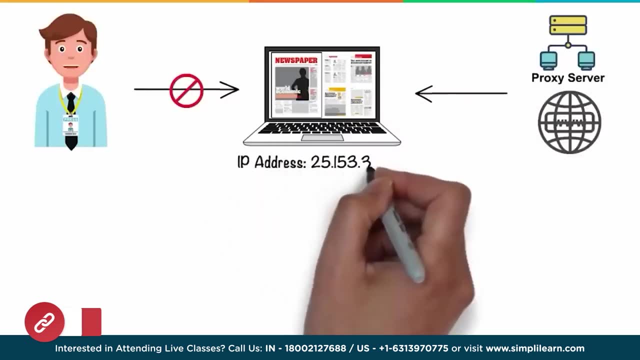 When Jonathan wasn't able to access the news website, he connected his system to a global proxy server. Once connected, the proxy server assigns a new IP address to Jonathan's system, an IP address of a different country where the website is not censored. Following this process, 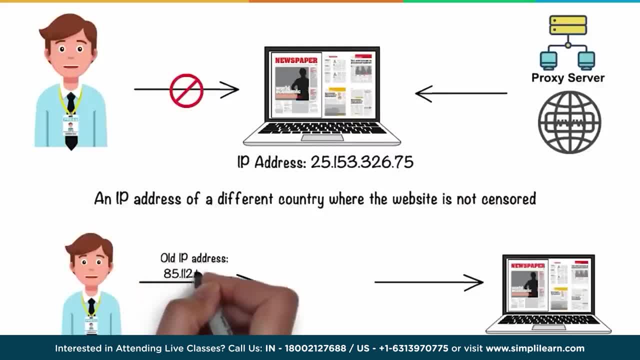 whenever Jonathan visits that website, the website administrators see the new IP address assigned via a proxy server and sees no reason to deny access to their account. Once the proxy server is able to access the website, it's passed on to Jonathan's system via the same channel. 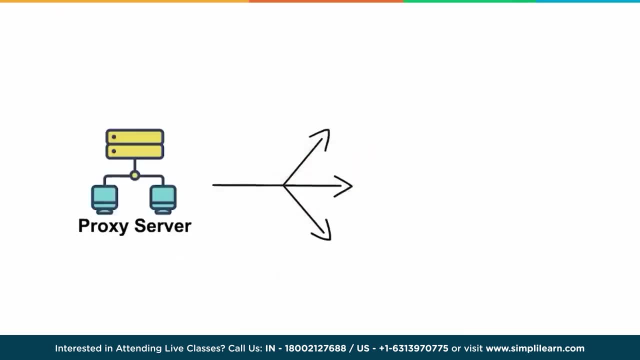 Regarding accessibility to proxy servers, you must first set it up on your computer device or network. Next check the steps required for your computer or network, as each operating system has its setup procedures. In most cases, however, setup entails using an automated configuration. 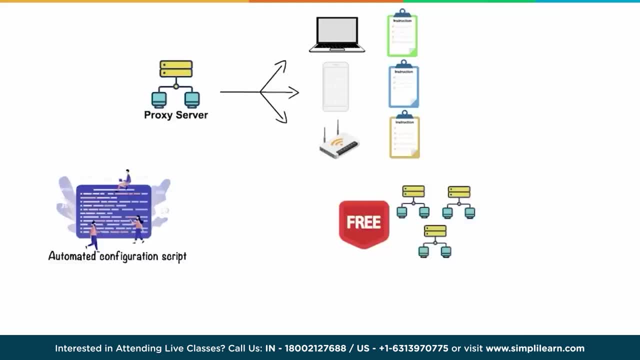 script. There are plenty of free proxy services available on the internet. However, the safety of proxies is rarely verified. Most free proxies will provide an IP address and a relevant port for connection purposes- Reputed proxy providers like Smartproxy and Brightdata that run on 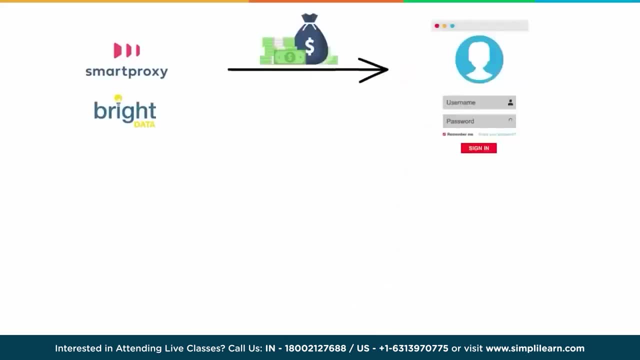 subscription models will most likely provide credentials to log into when establishing the connection. This extra step acts as authentication that verifies an existing subscription on the proxy provider's server. unlike free providers that are open to all, When it comes to hiding IP address, many people consider a VPN to be the primary solution. While that's true up to some extent, 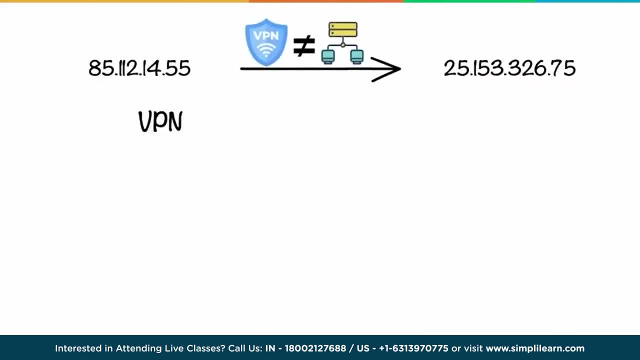 there are a few things proxies do differently. In the case of VPNs, extra encryption is also carried out to create a secure tunnel between the user's device and a VPN server. A VPN is usually much faster, more secure thanks to multiple layers of encryption, and has little to no downtime. 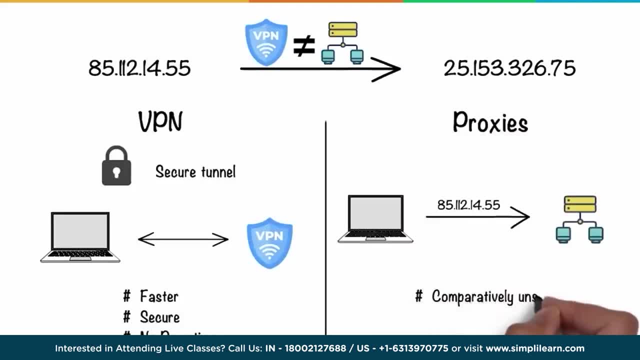 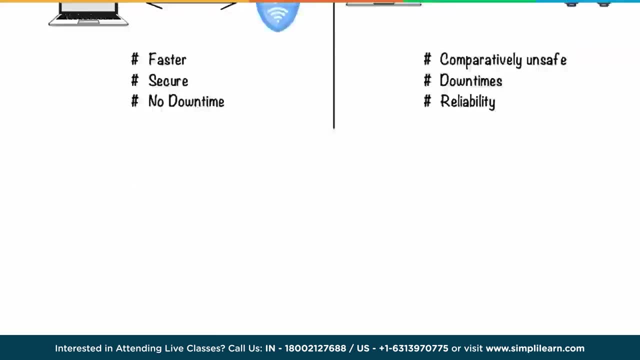 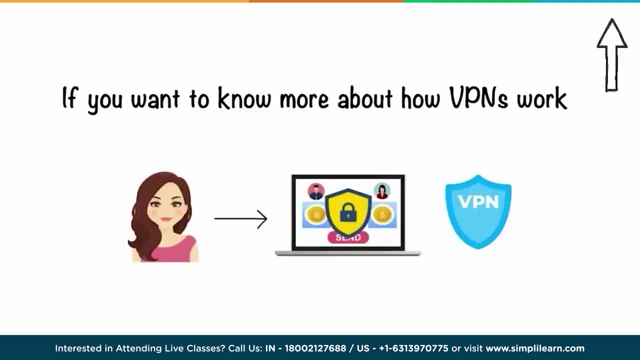 Proxies tend to be comparatively unsafe, with the service owners having the exact IP address of the end user and having no guarantees regarding downtimes and reliability. If you want to know more about how VPNs work, do watch how Jude could have protected her banking credentials using VPNs in our detailed video linked above. 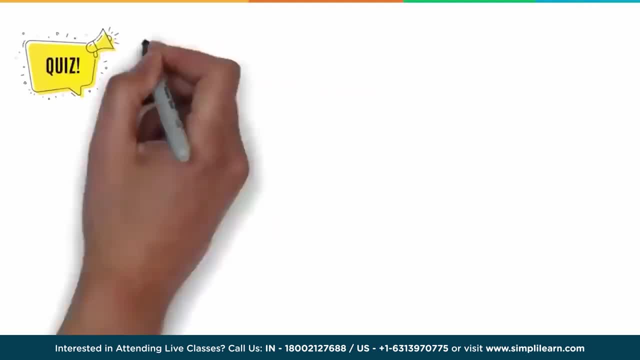 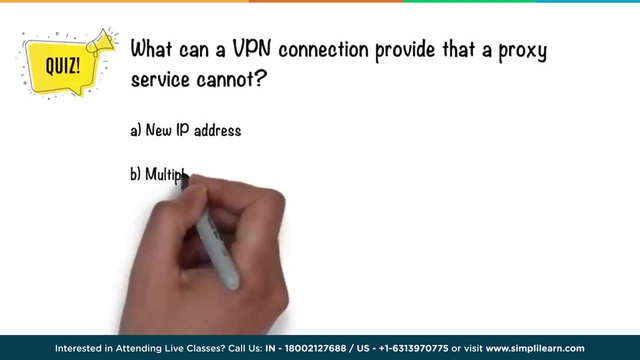 Now let's take a small quiz to check how much we have learned. What can a VPN connection provide that a proxy service cannot? A New IP address. B- Multiple layers of encryption. C- Access to geo-blocked content. D- Authentication credentials. 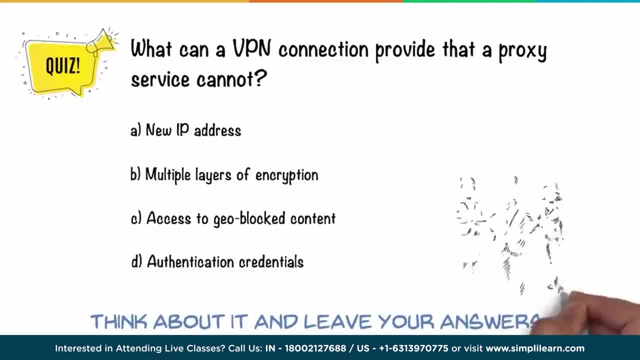 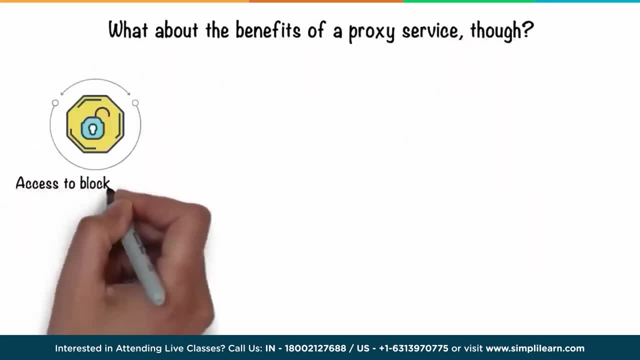 Think about it and leave your answers below in the comment section, and three lucky winners will receive Amazon gift vouchers. What about the benefits of a proxy service, though? Besides allowing access to blocked content, proxies can serve as an efficient firewall system. They can also filter content from third-party websites, allowing control over internet usage. 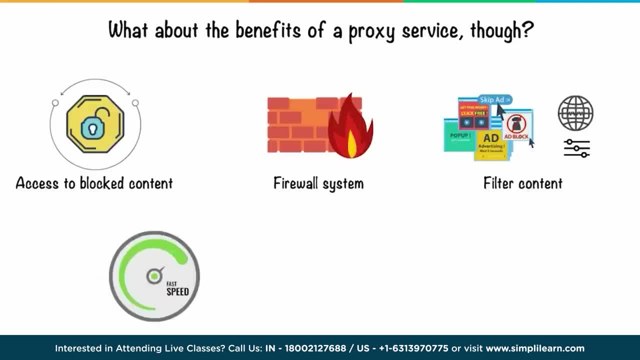 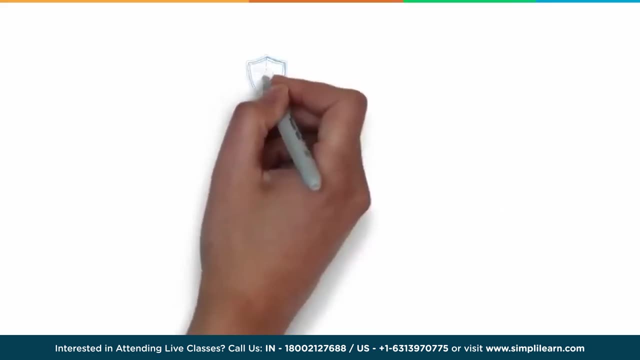 In many cases, browsing speeds are stabilized compared to vanilla internet, thanks to proper optimization on the base proxy server. The element of privacy proxies provide is highly lucrative to people looking to hide their actual IP address from as many crying eyes as possible. One can easily argue the benefits of using VPNs over proxies for added security measures. 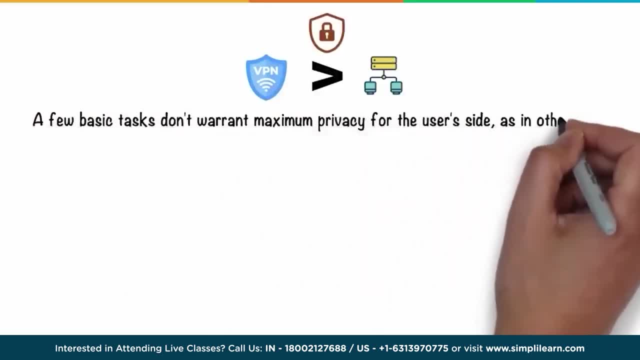 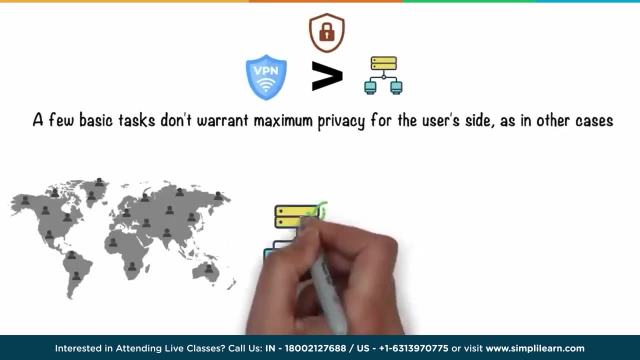 However, a few basic tasks don't warrant maximum privacy for the user's side, as in other cases. For example, many consumers worldwide find proxy services more convenient, since all major operating systems, starting from Windows to Android, allow proxy configuration without the hassle of installing new applications, as is in the case of a VPN. 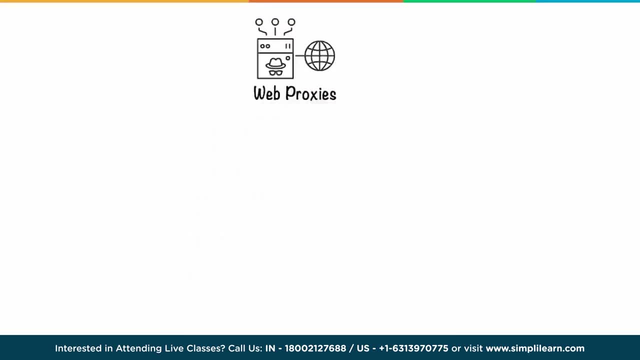 In addition, there are services online that function as web proxies, allowing users to access blocked content without any setup from their end. They can enter the target URL and the web proxy will route data from its physical server. This level of freedom is hard to come by in the case of a proxy service, but it's worth considering. 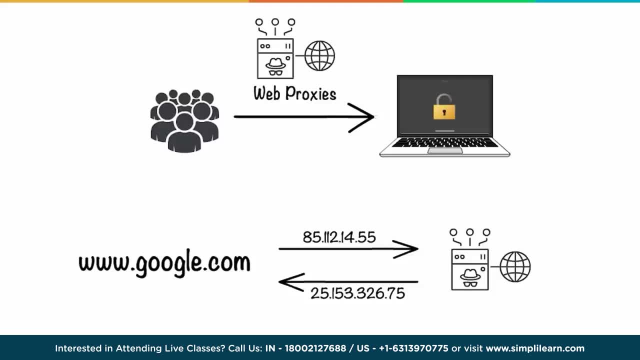 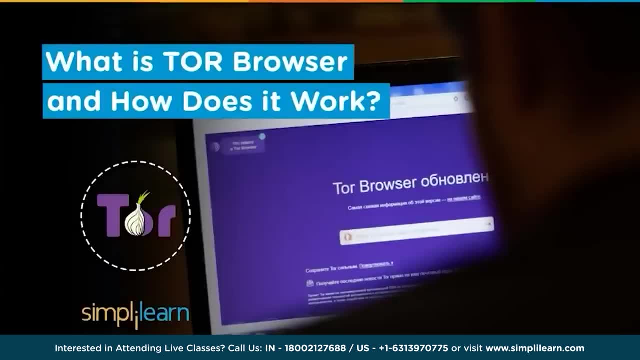 With the next generation of internet exchanges focused on maximum privacy and security, a variety of ways have been enforced to maintain them. as such, Censorship has been shifted from the streets to the digital domain. It forces the standard citizen to derive alternative ways to maintain anonymity- A major weapon in this battle for privacy and security. 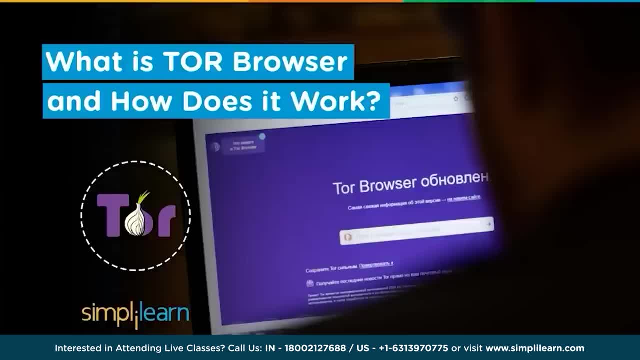 is the Tor Browser, An independent browser meant to browse the internet while reeling information through the Tor network. It serves as a meaningful alternative to the standard internet browsing habits. To better understand the purpose of this browser and such, you must learn about the work of the Tor Network, Featuring its own routing protocol. 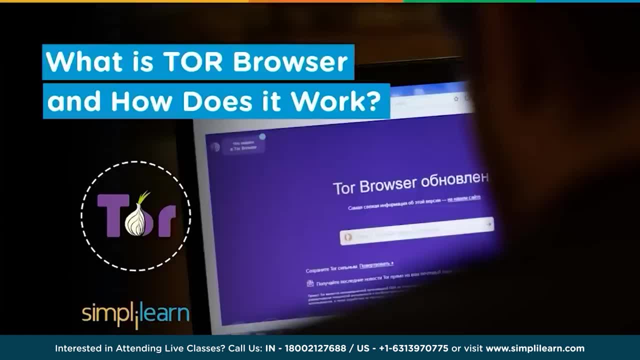 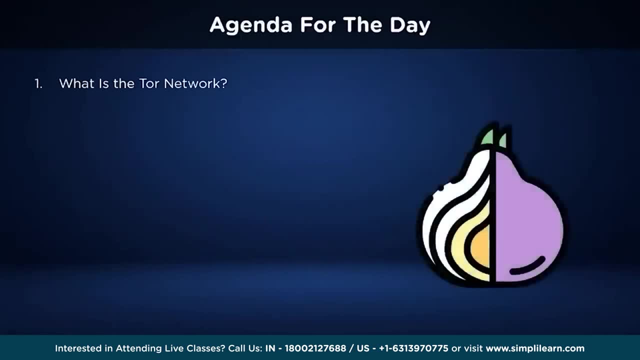 the Tor Browser is an easy way to maintain anonymity while browsing without emptying one's wallet. Let's take a look at the topics to be covered today. We start at the explanation of what is the Tor Network and its significance in the working of the Tor Browser. We take a take a look at what are the replied notifications with the program. Let's first take a look at the interpretation and the URL to the Tor Network. • The Tor Browser is an electronic payment network with zeroorphic lessons taught to still be available to people and accounts. You will receive instant access to it. • Every Berries have stocked or use Tor Net versus teach. 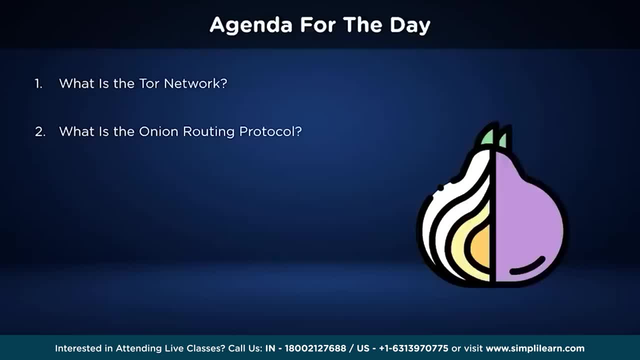 Take a look at the onion routing protocol and how it transmits the data from the client devices to the Tor directories in order to circumvent government censorship. Moving on, we learn a few features of the Tor browser and the distinct advantages the Tor network provides. 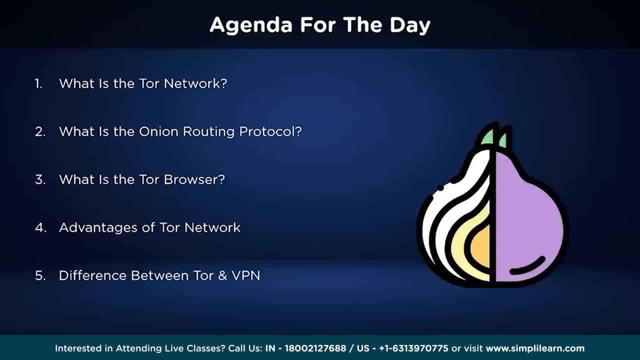 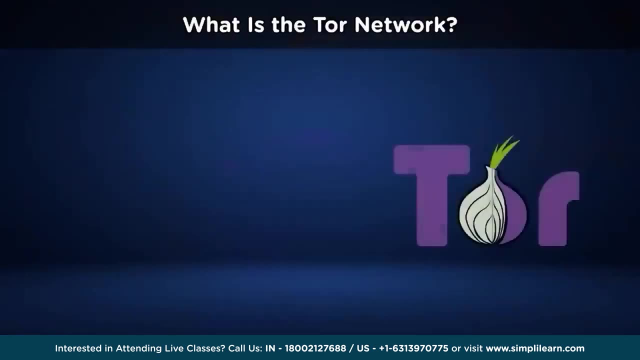 Next, we learn the difference between using a VPN and a Tor to anonymize internet usage And finally, we have a live demonstration of the Tor browser anonymization features in action. Let's move on to learning about the Tor network. Tor, short for the Onion Router, is an open-source privacy network that permits users to browse. 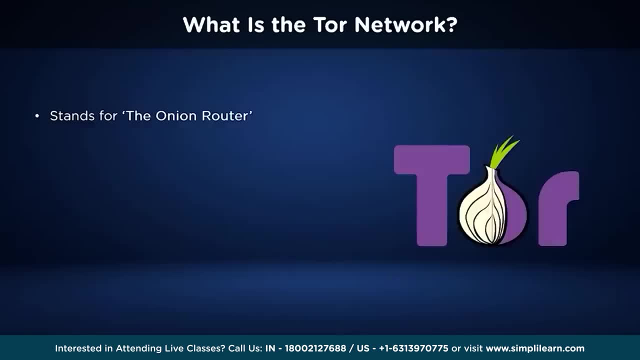 the web anonymously. The Tor was initially developed and solely used by the US Navy to protect sensitive government communications before the network was made publicly available. The digital era has disrupted the traditional way of doing things in every sector of the economy. The rapid rise in development and innovation of digital products has led to the rise in 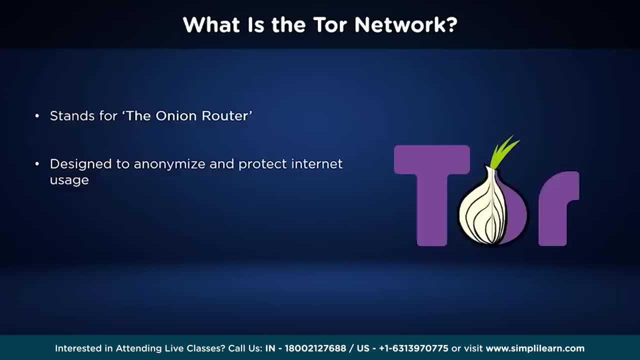 cyber-threats and data breaches. In response, consumers are increasingly opting for products that offer data privacy and cybersecurity. Tor is one such underground network that was implemented for the purpose of protecting users' identities. The Tor network is one example of the many emerging technologies that attempt to fill 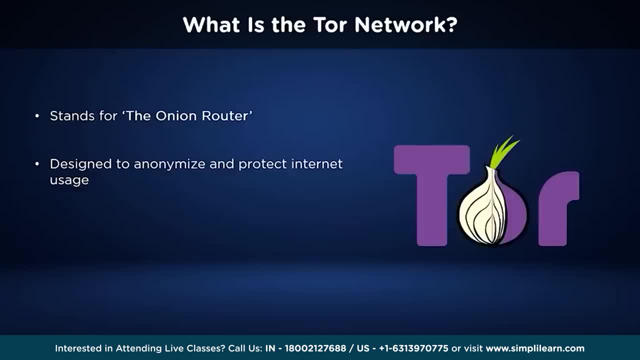 a data privacy void in a digital space plagued by cybersecurity concerns. The Tor network intercepts the traffic from your browser and bounces a user's request. then the data is passed to the user's requested final destination. These random users are volunteer devices which are called nodes or relays. 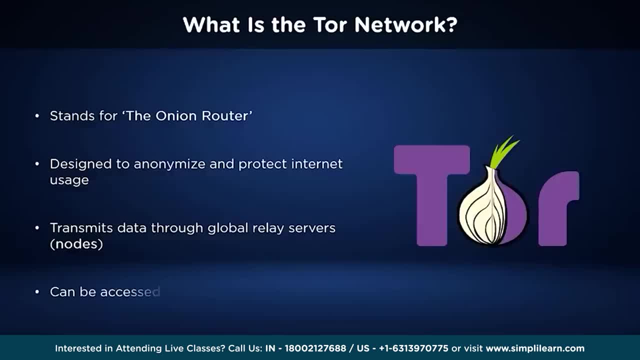 The Tor network disguises your identity by encrypting the traffic and moving it across different Tor relays within the network. The Tor network uses an Onion Routing technique for transmitting data, hence the original name of Onion Router. To operate within the Tor network, a user has to install the Tor network. 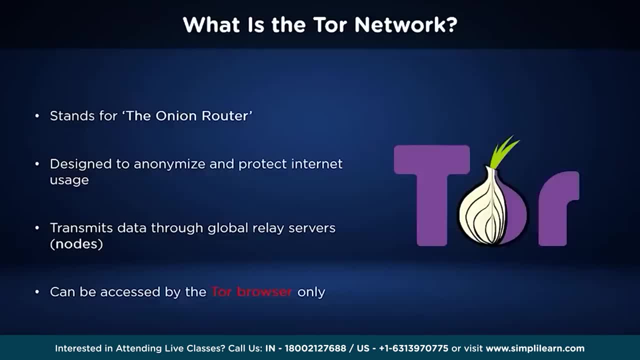 The Tor network uses an Onion Routing technique for transmitting data, hence the original name of Onion Router. The Tor network uses an Onion Routing technique for transmitting data, hence the original name of Onion Router. The Tor network uses an Onion Routing technique for transmitting data, hence the original. 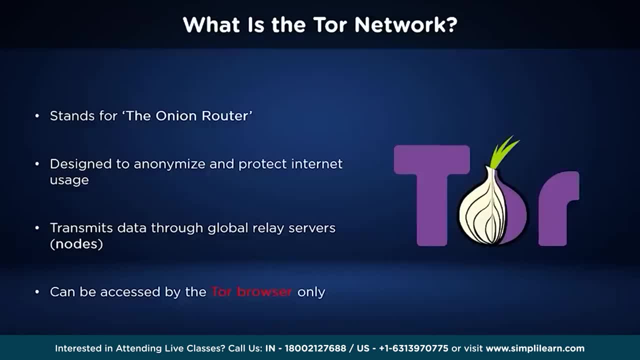 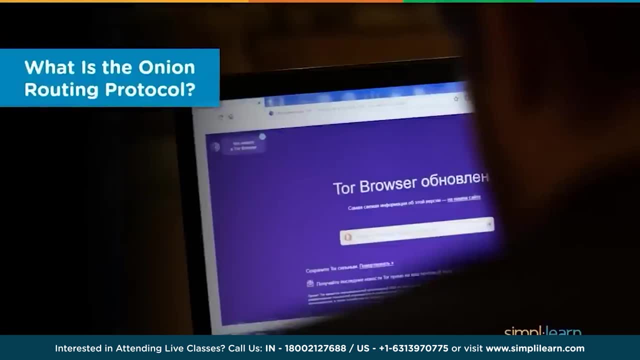 name of Onion Router. Any address or information requested using the Tor network is transmitted through the Tor network. It has its own feature set which we will be covering over later in this video. As we discussed already, the data passing through the Tor network must follow a unique 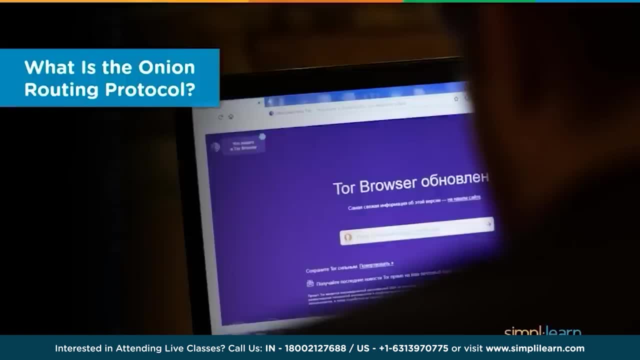 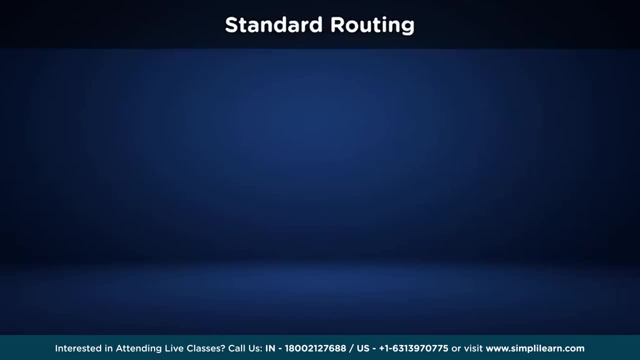 protocol, known as the Onion Routing Protocol. Let us learn more about its unique characteristics. In our normal network usage, the data is transmitted directly. The sender has data packets to transmit. This is done directly over a line of communication with either a receiving party or a server. 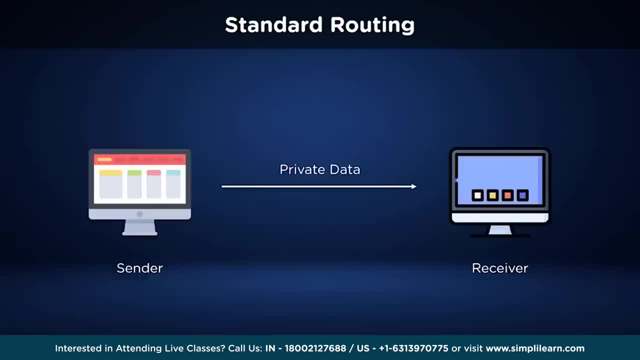 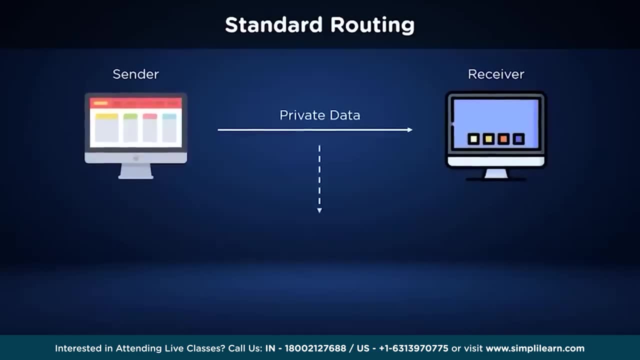 of some kind. However, since the data can easily be captured while being transmitted, the security of this exchange is not very reliable. Moreover, it becomes very easy to trace the origin of such requests. On many occasions, websites with questionable and controversial content are blocked from. 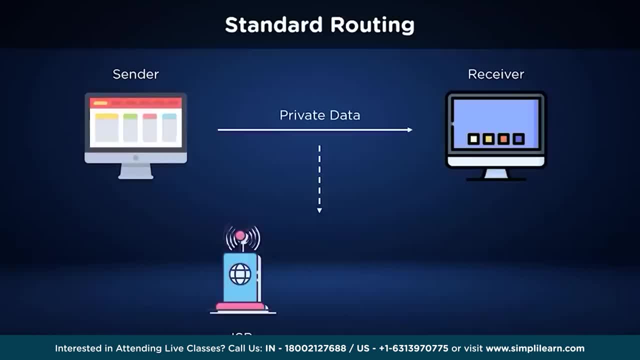 the ISP. This is possible since the ISP is able to detect and spy on user information passing through the network. Apart from ISPs, there is a steady chance of your private information being intercepted by hackers. Unfortunately, easy detection of the source and contents of a web request make the entire. 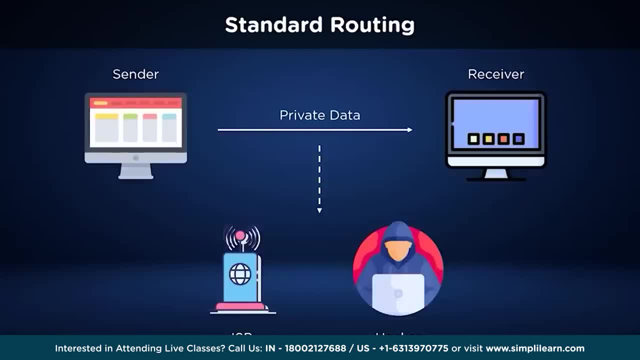 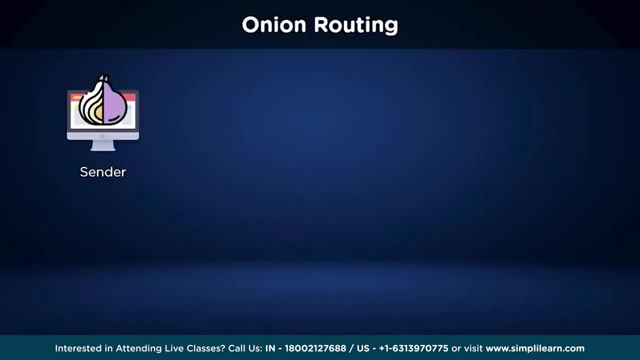 network extremely vulnerable for people who seek anonymity over the internet. However, in the Onion Routing Protocol, things take a longer route. We have a sender with the Tor browser installed on the client's system. The network sends the information to node 1's IP address, which encrypts the information. 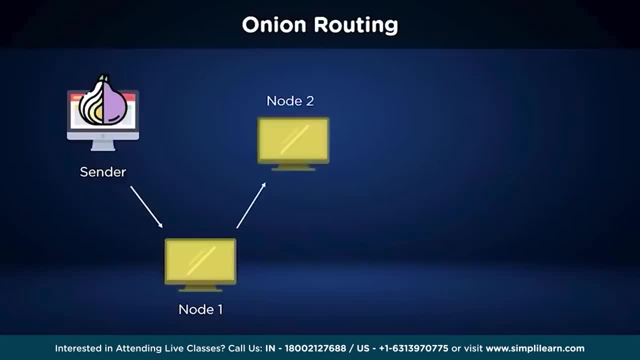 and passes it on to node 2's IP address. The Tor browser sends the information to node 3's IP address, which performs another encryption, and passes it on to node 3's IP address. This is the last address, which is also known as the exit node. 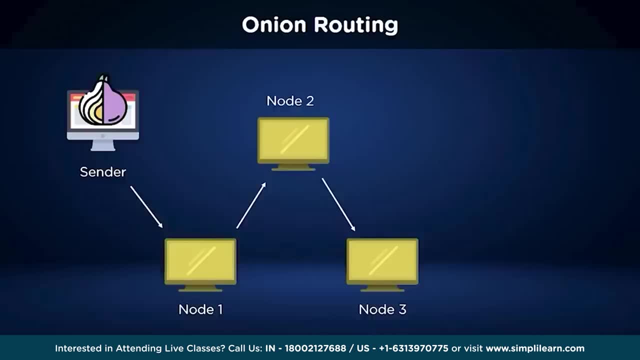 This last node decrypts the encrypted data and finally relays the request to the final destination, which can be another device or a server end. This final address thinks the request came from the exit node and grants access to it. The encryption process across multiple computers repeats itself from the exit node to the original. 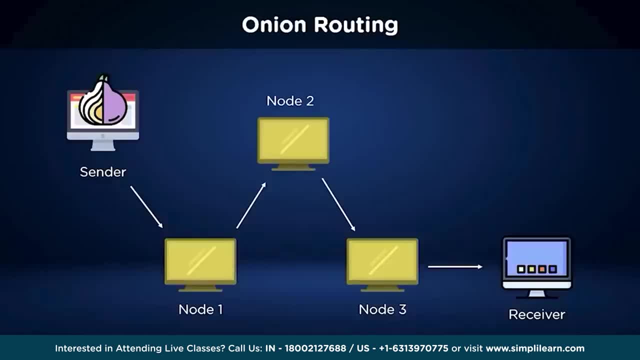 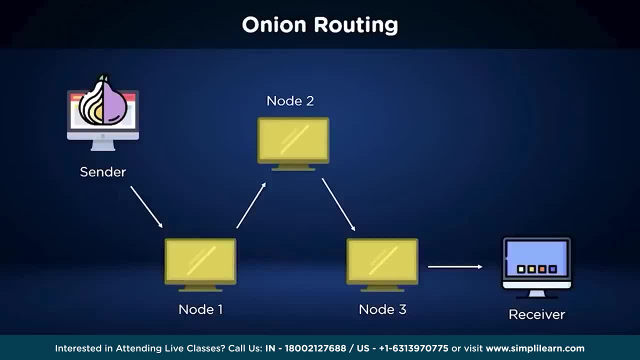 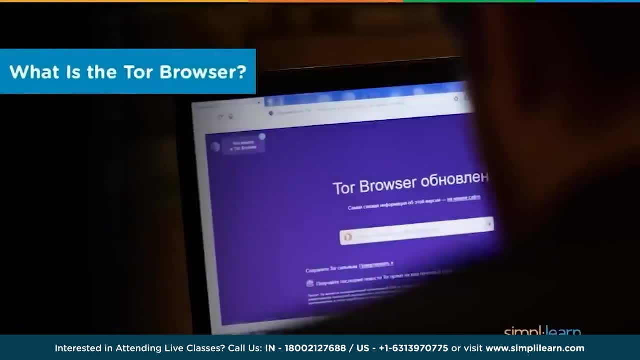 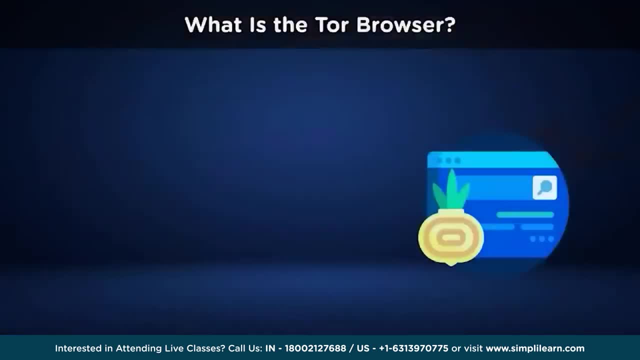 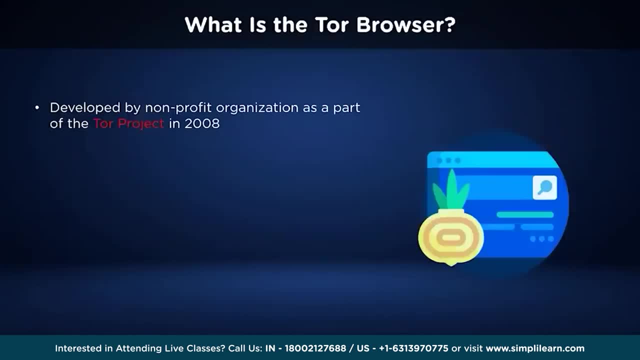 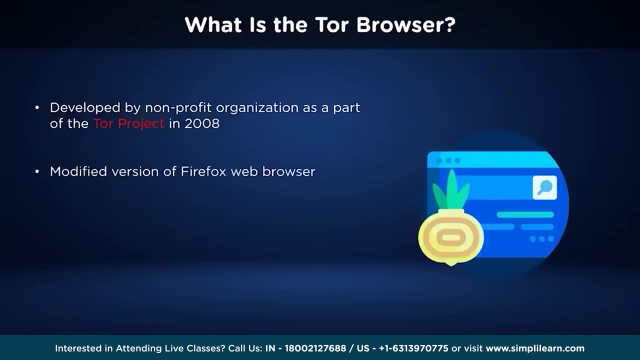 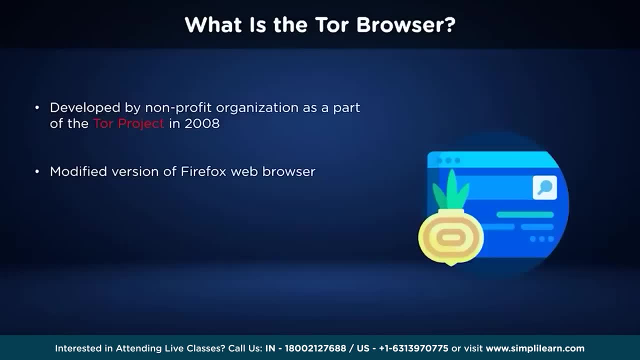 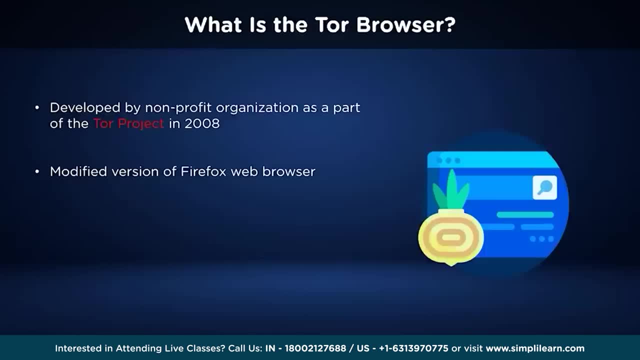 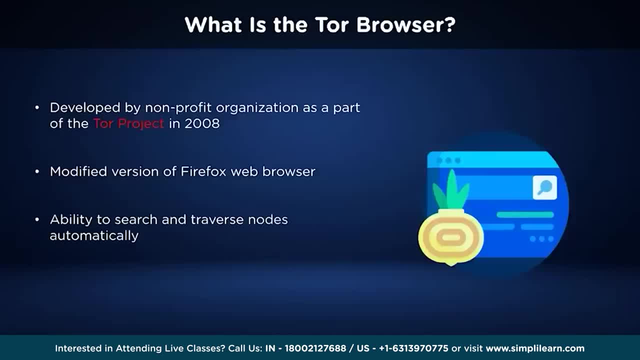 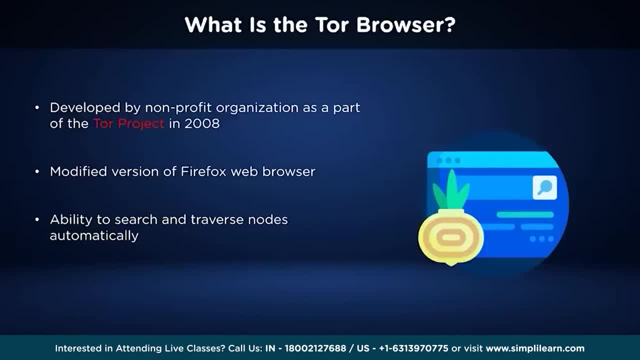 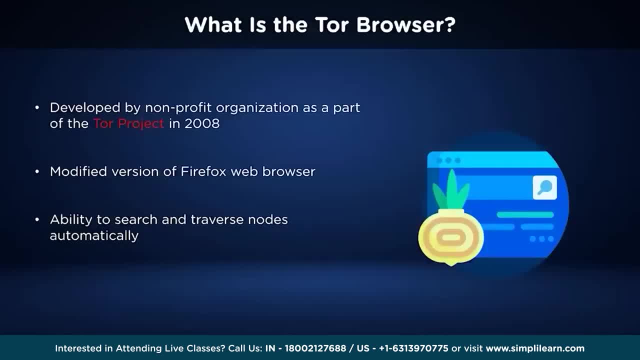 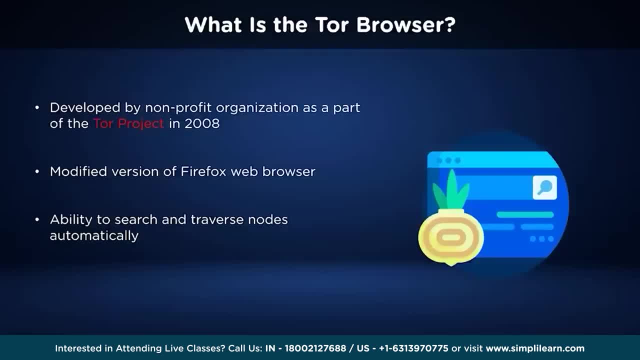 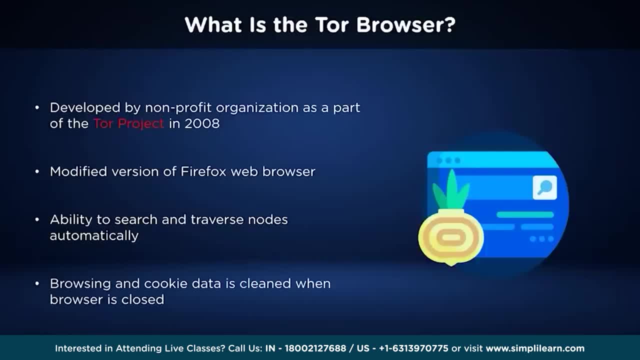 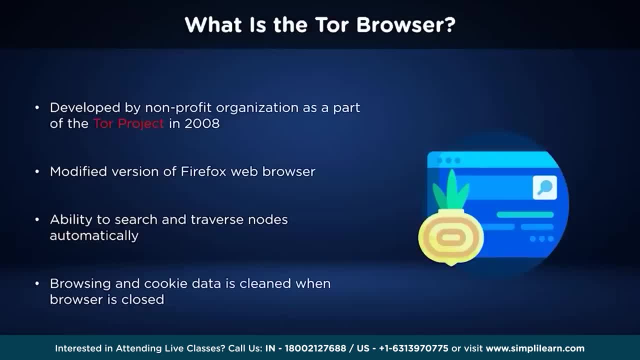 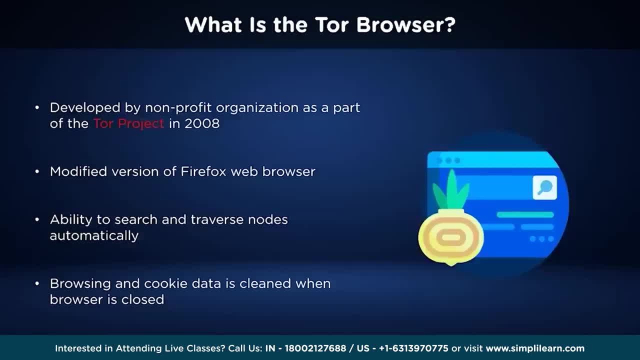 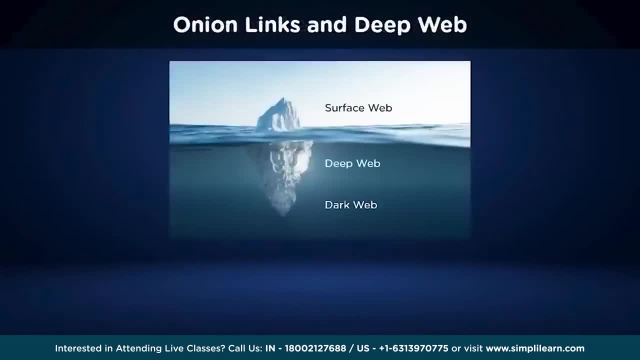 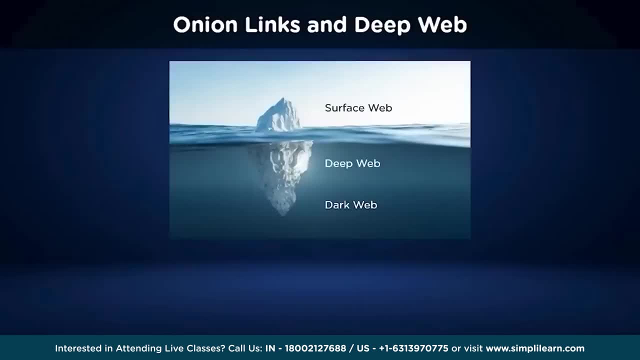 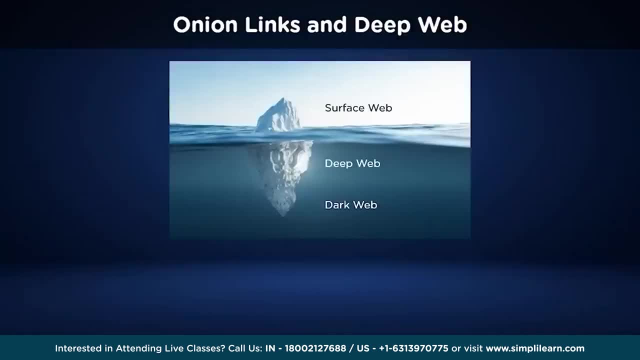 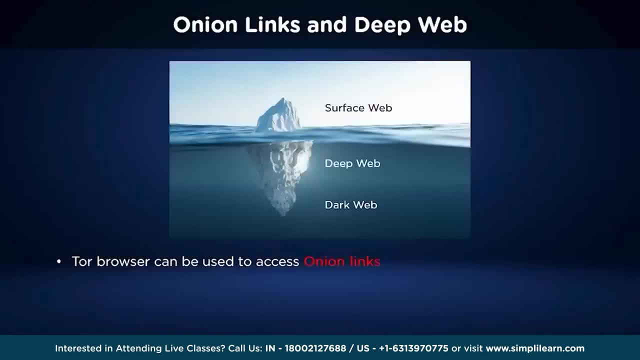 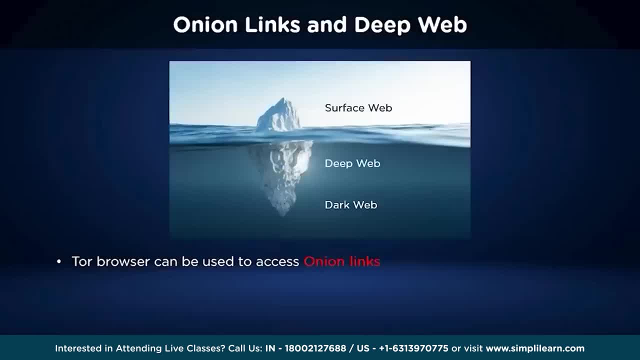 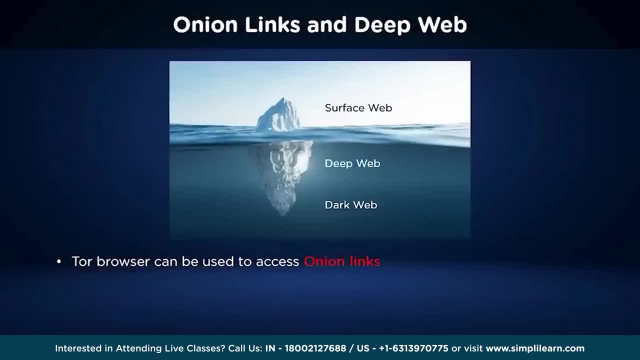 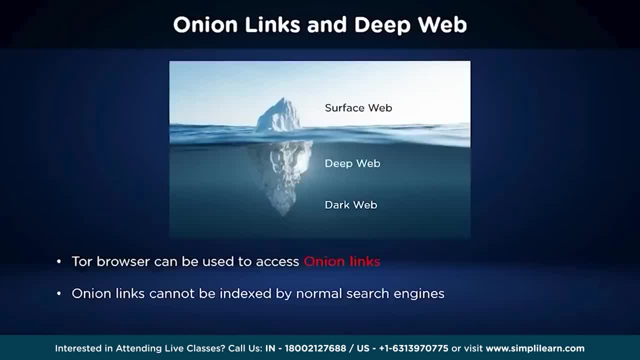 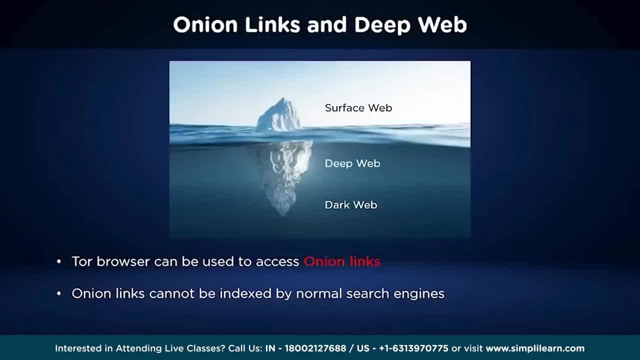 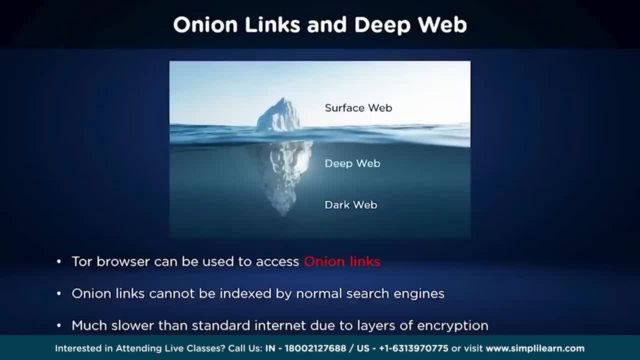 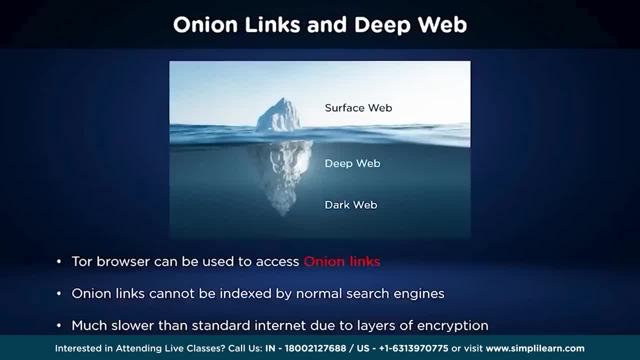 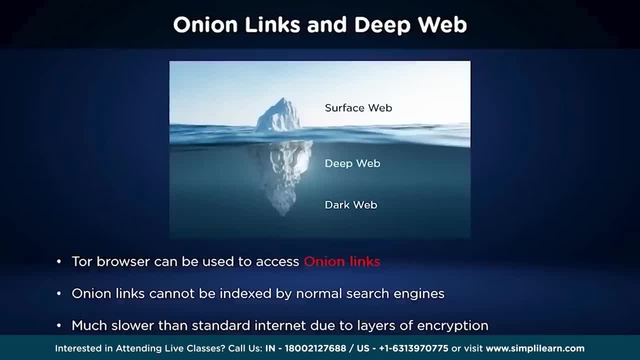 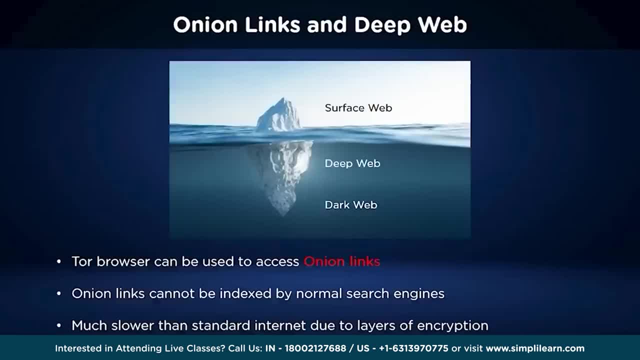 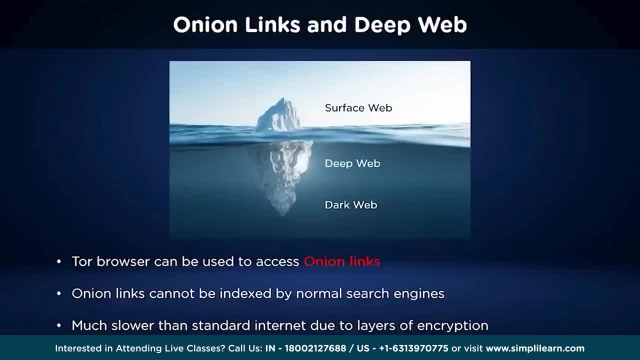 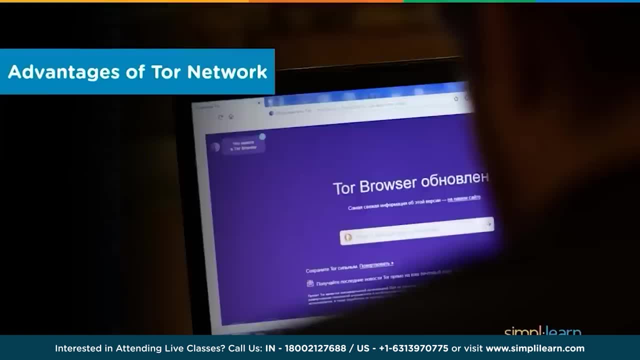 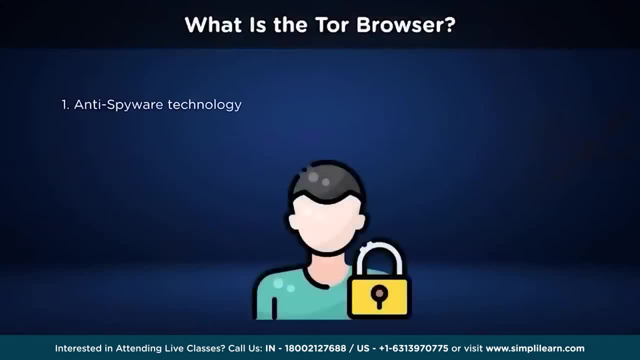 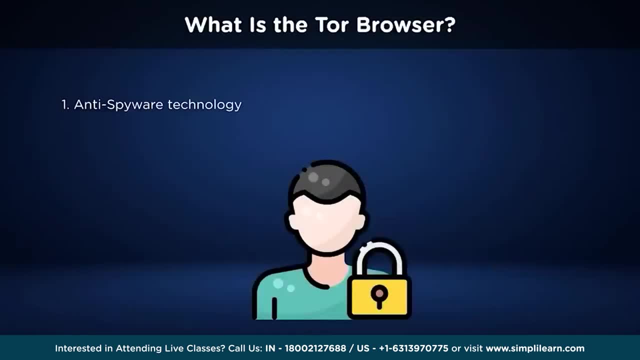 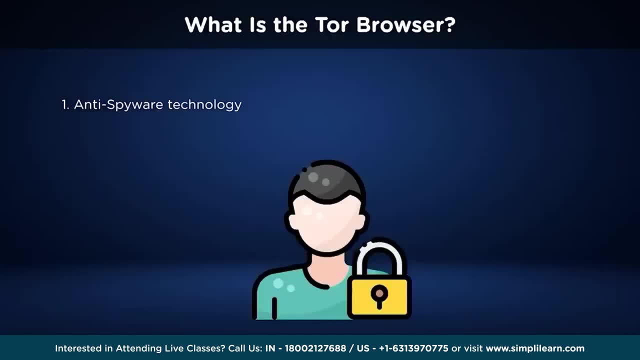 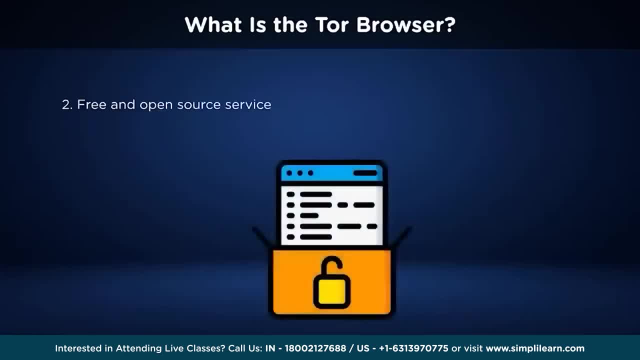 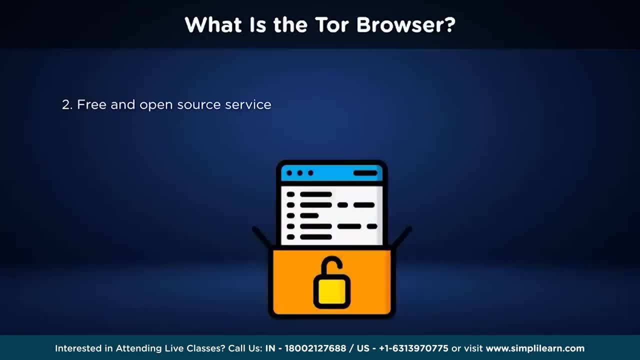 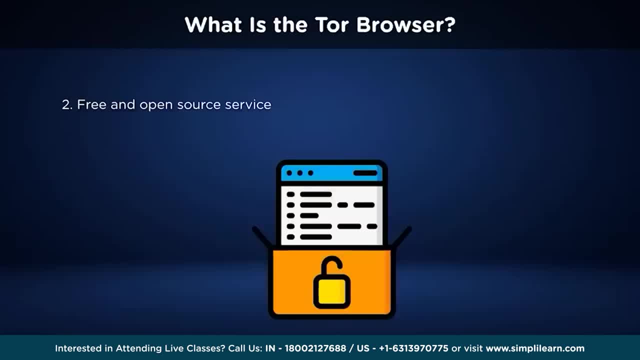 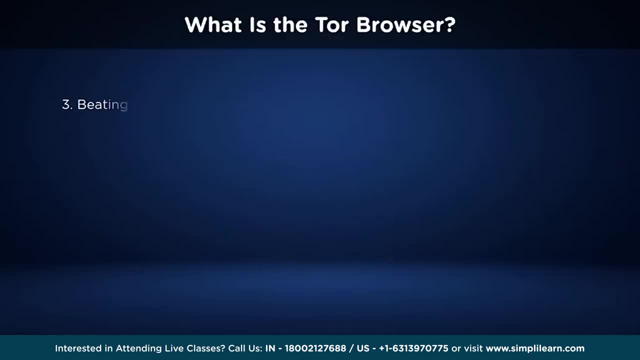 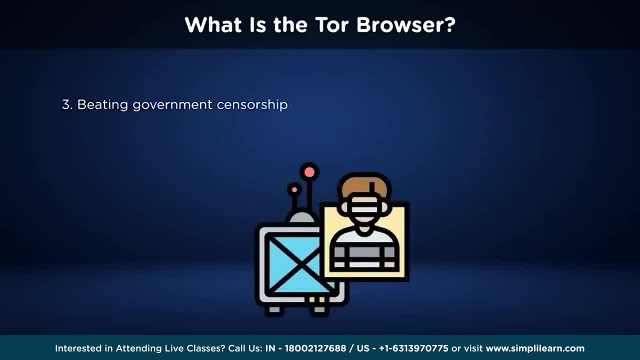 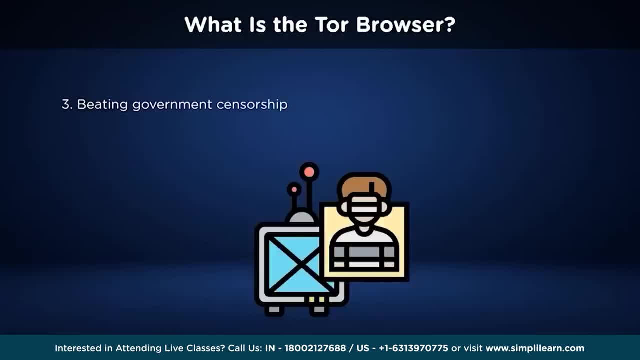 The Tor network obfuscates user IP addresses. The Tor network obfuscates user IP addresses, transfers data between multiple servers of random countries. the domains being blocked become available when used via Tor. Usage of these encryption messaging platforms is easily enforced using the Tor browser. 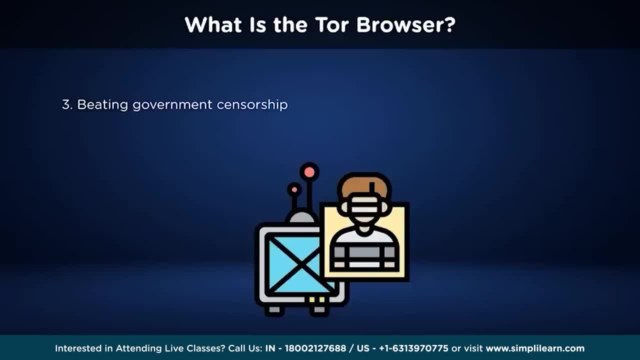 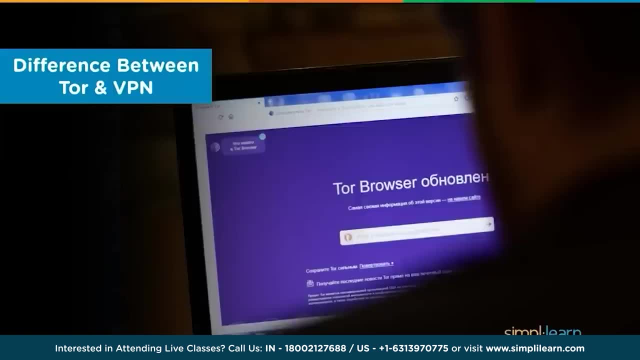 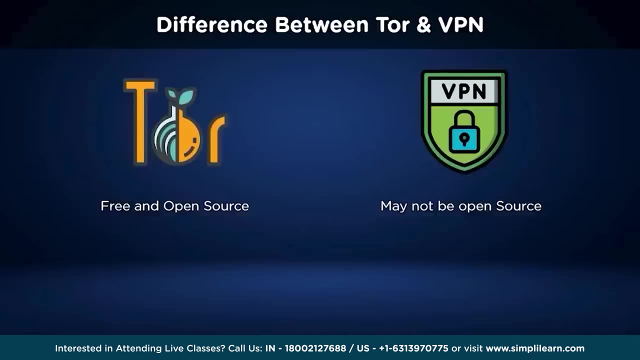 which otherwise would have been a difficult task under oppressive circumstances. Many people believe that a VPN offers the same benefits as the Tor browser. Let's put both of them to the test and see the differences between them. Coming to the first point of difference, Tor is completely free and open source. 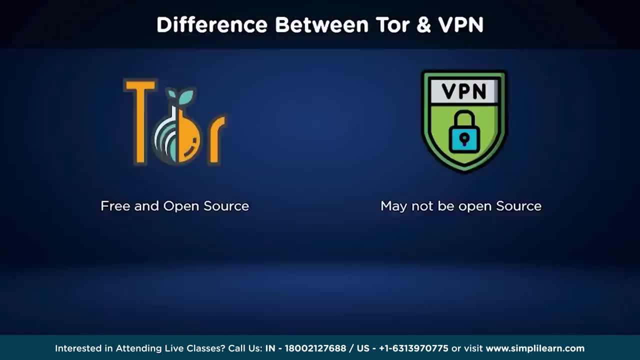 All of the code for the browser and the network can be audited and has been cleared for security concerns. When it comes to VPN, there are many different brands which have open source clients, but the same cannot be said for their counterparts. Some have partly open source, while some have completely locked up their code so that they 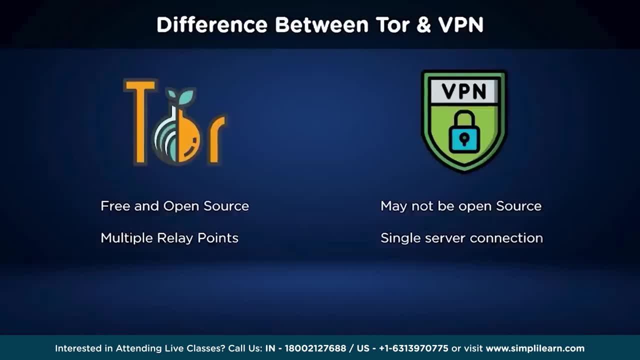 cannot be stolen further. Moving on, Tor has multiple relay points in its data transfer protocol. Between the server and the receiver there are three different IP nodes. That number can increase, but it will always be more than two. Once the data is passed from the sender, it goes through all of those relay points. 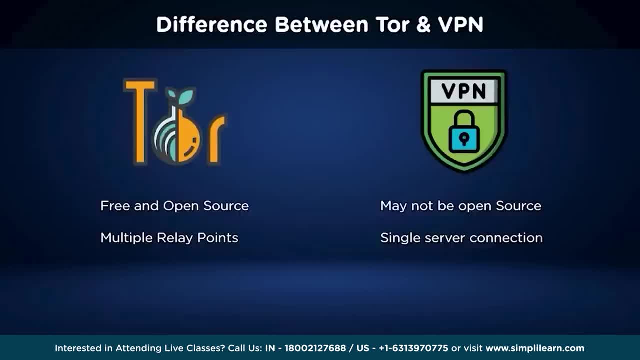 While in the case of a VPN, the connection is made from the client device to the VPN server and then to the requested destination, There is no other IP node that comes into work here, thereby making the connection a one-to-one between the client and a VPN. 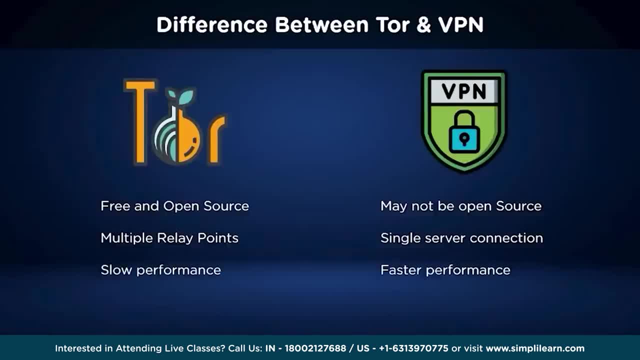 As a next point, since Tor handles multiple layers of encryption, it is very easy to understand the connection between the client and the VPN. When the data passes through multiple systems along the way, the performance is slow compared to a VPN, where the performance is relatively fast due to the less number of nodes. the data 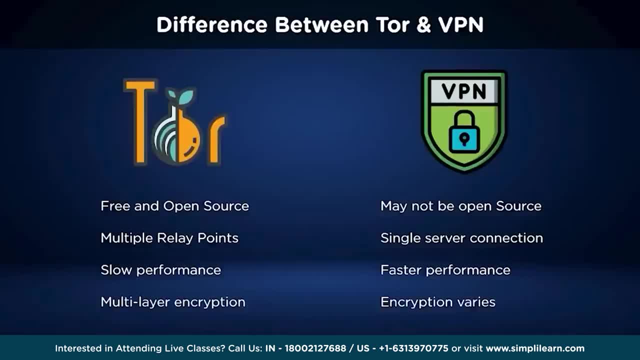 passes through. Similarly, the multi-layer encryption of Tor is consistent. If you use Tor browser, every single request passes through the same layer of encryption and follows the same routing protocol. In the case of a VPN, different companies offer different levels of encryption. 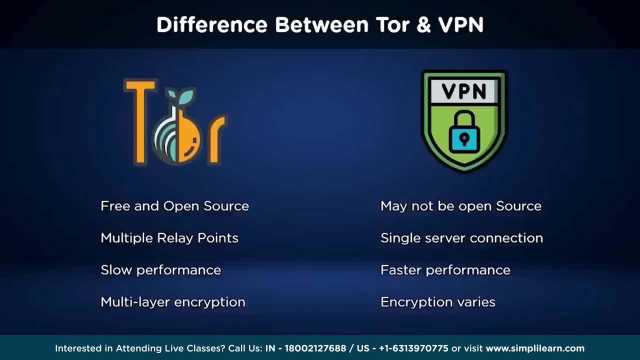 Some have multi-hop, some prefer a single one-to-one connection, and these kind of differences make the choice much more variable. Finally, the nodes and relays being used in the Tor network are volunteer. There is no company holding over them, so jurisdiction becomes relatively straightforward. 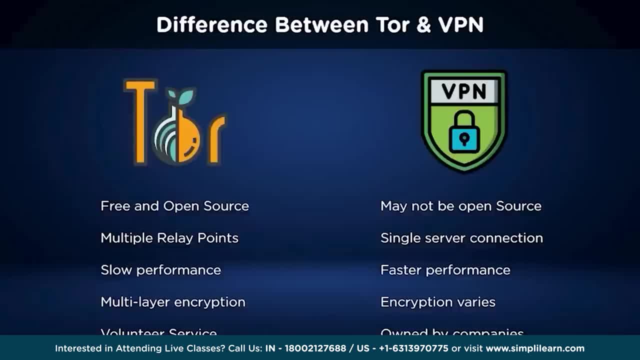 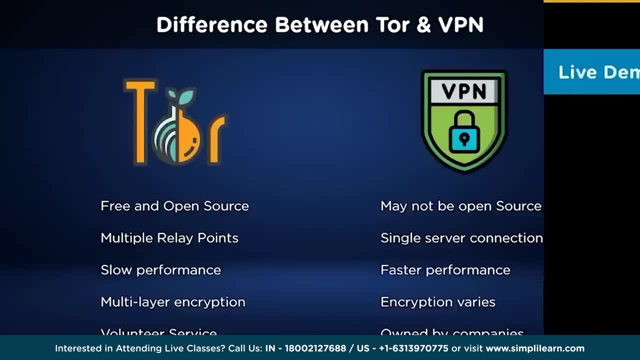 Whereas in the case of VPNs, many such VPNs are hosted by adware companies or are being monitored by central governments. to note the usage information. Now that we have seen the different types of VPNs, let's move on to the next topic. 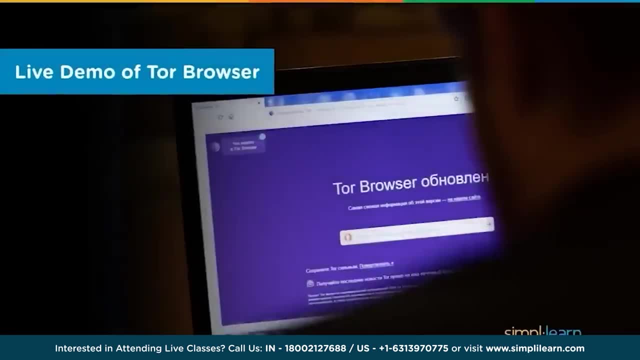 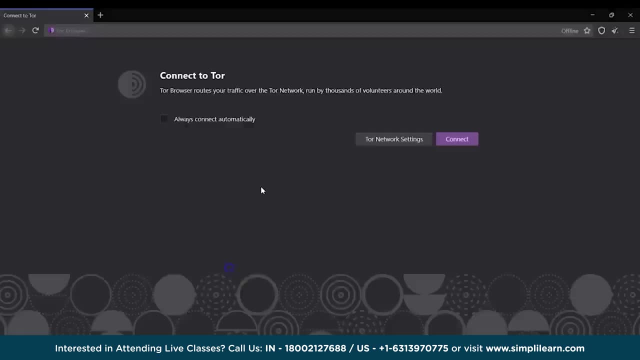 Let's talk about the usage of VPNs. Let's talk about the usage of VPNs. Now that we have a better understanding of the Tor browser and its routing, let us take a look at how the Tor browser can anonymize and protect our internet usage. 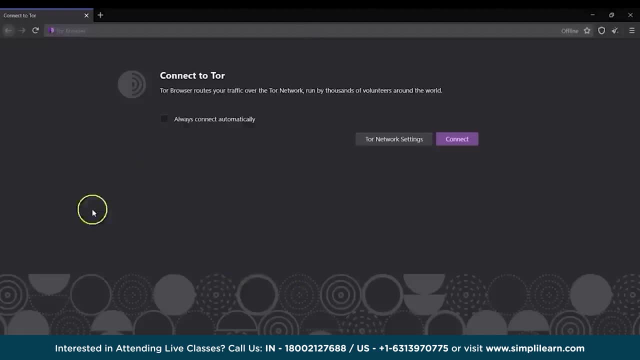 On opening up the Tor browser for the first time. this is the page that you are going to be welcomed with. You have the option of connecting to the Tor network before we start our browsing, So let's press connect and we can see that it is connected. 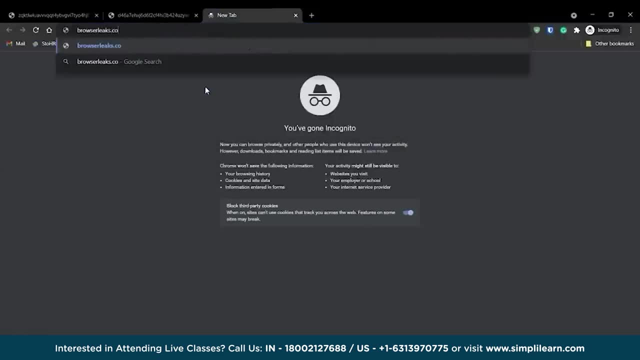 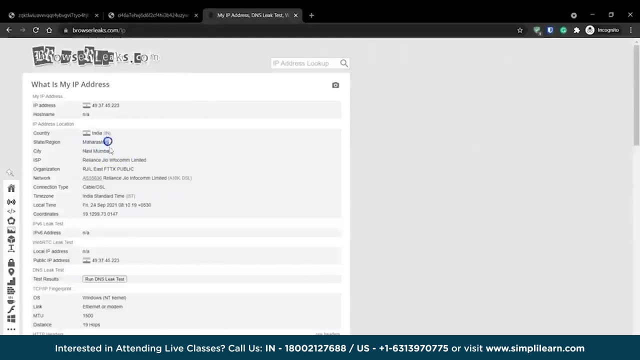 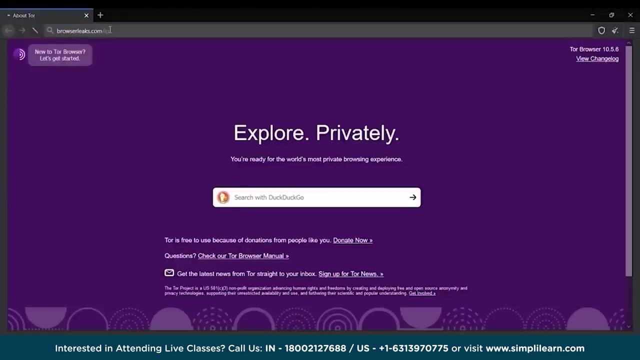 Coming to the anonymization, let's check my current location on Google Chrome. Currently it is showing as Navi Mumbai, in Maharashtra. If we check the same link on the Tor browser, we should get a different address. Now, every link that we open in the Tor browser will be a little delayed and the speed will 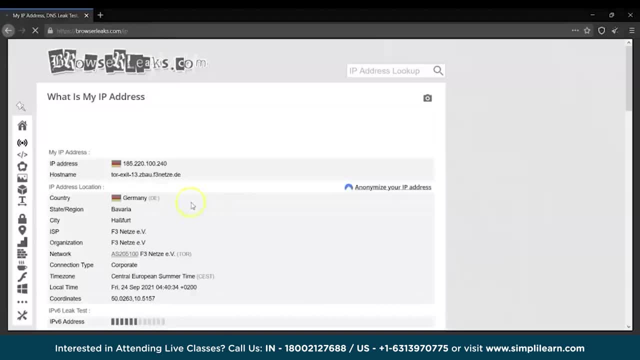 be hampered because of the multiple layers of encryption, like we discussed. Now, as you can see, it's showing a German IP and the state of Bavaria. This is how the anonymization works. There is no VPN configured. there is no proxy attached. it's straight up the out-of-the-box. 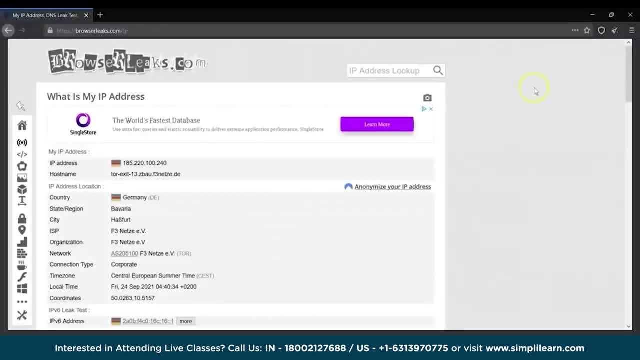 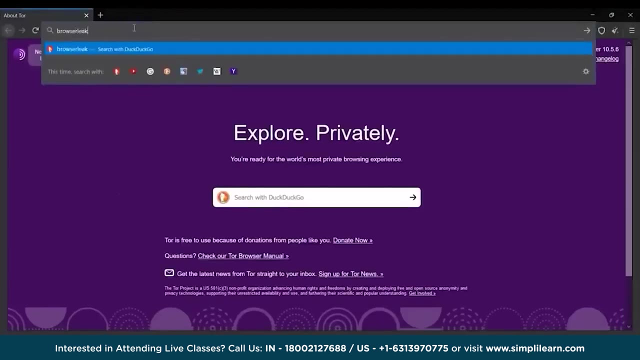 settings that come inbuilt with the Tor browser. Similarly, we have an option of cleaning up the data. Let's say, if you want to refresh your location and you want to use a different ID for the next browsing session, If you just restart it once and you can have to check it again, we should be seeing a different. 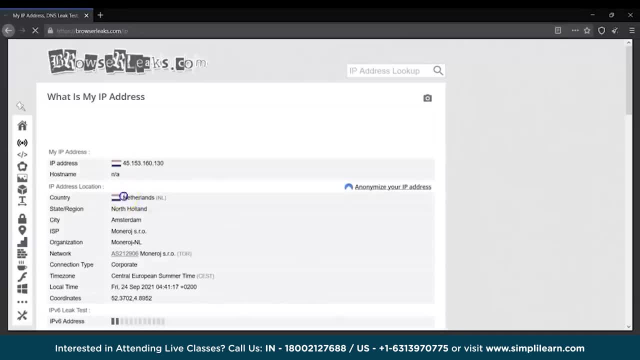 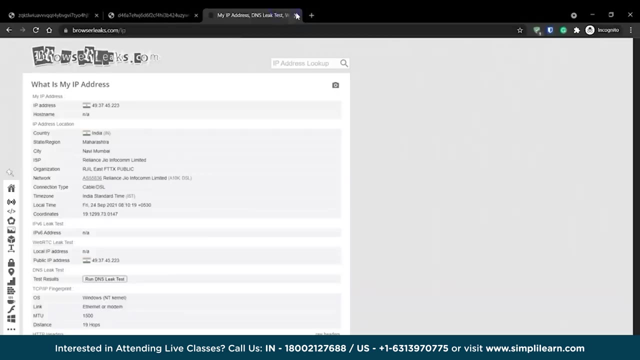 country. As you can see, we have Netherlands right now, So this is how you can keep refreshing your address. you can keep refreshing your host location so that you cannot be tracked when browsing the internet. Like we discussed, we have some onion links that can only be used on the Tor network. 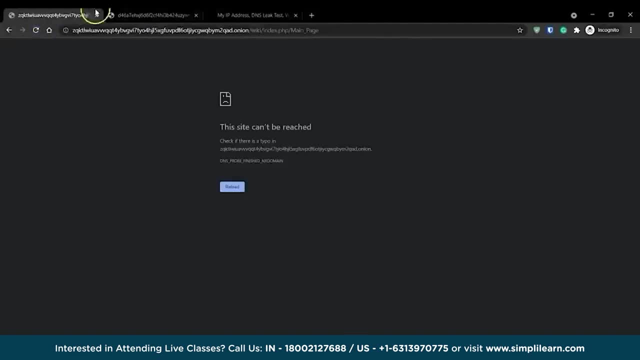 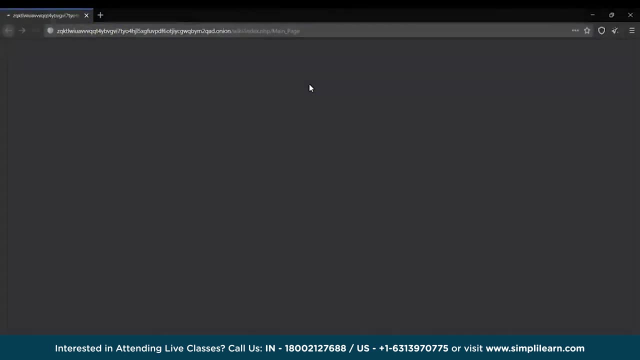 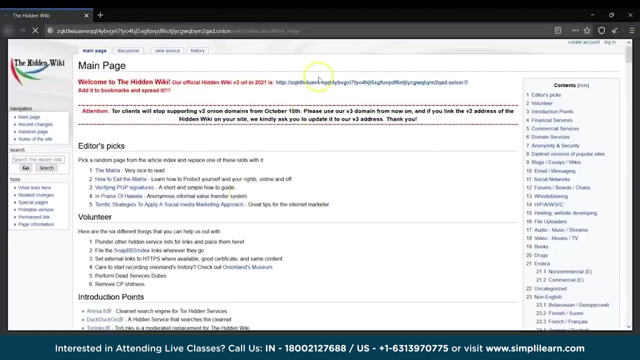 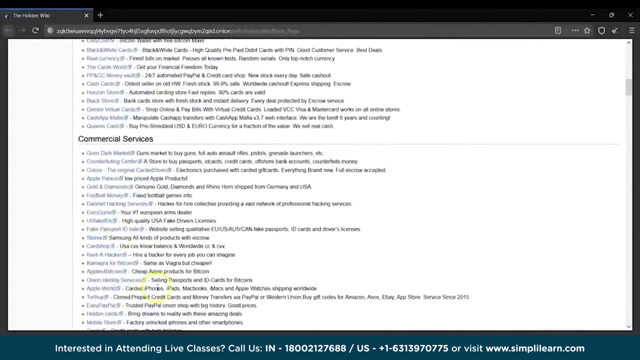 As you can see, these kind of links do not open in the Google Chrome browser, But once we copy these over to the Tor browser. As you can see, we have opened the hidden wiki, which is available only on the Tor network. This is kind of an alternative Wikipedia website where we can find articles to read and more. 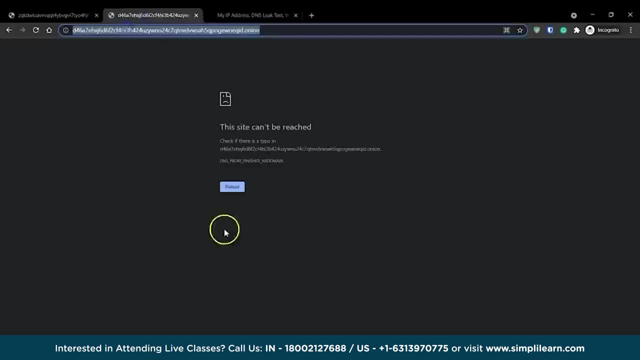 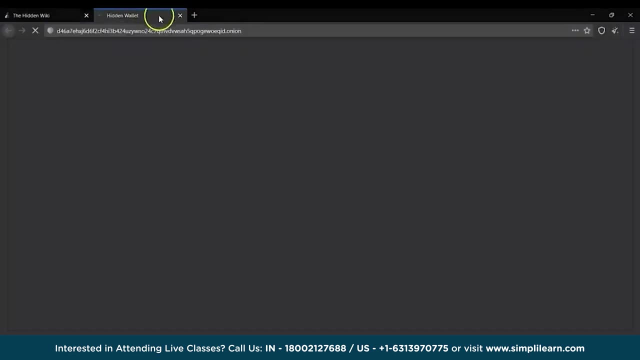 information to learn. Similarly, we have another onion link over here which is once again available only for the Tor browser, So let's go ahead and open it Now. these kind of delays are expected, but they are a valid compromise because they maintain. 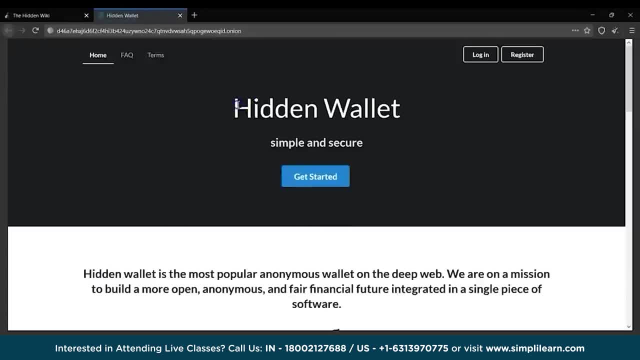 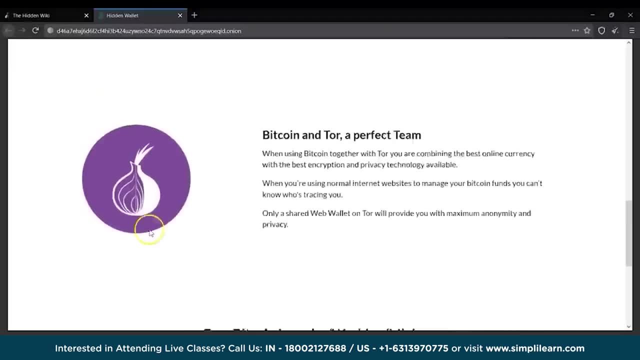 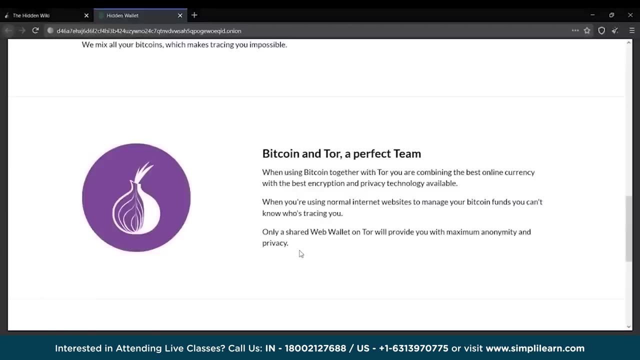 the anonymity that many people desire. Similarly, we have found a hidden wallet, which is a cryptocurrency wallet, which is specifically for dark web members. This operates over the Tor network and this is used by mostly journalists and people who want to anonymize their internet transactions when it comes to dealing money. 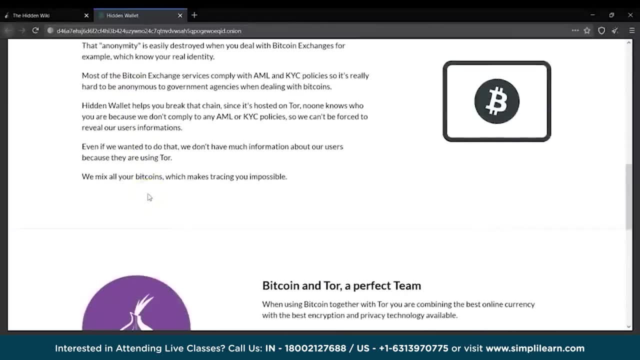 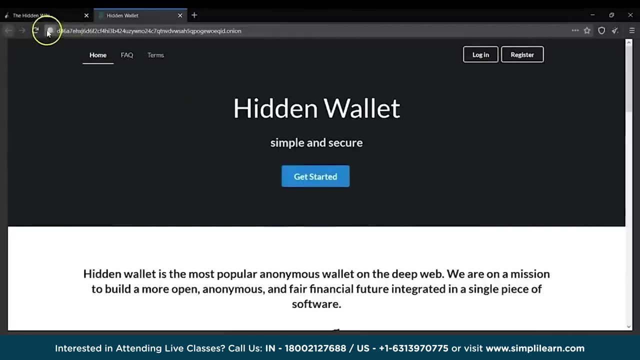 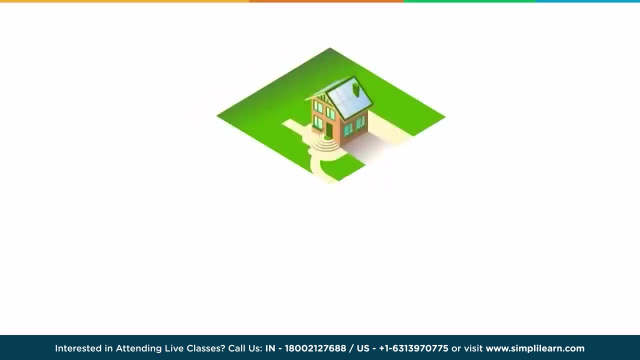 All of the transactions that occur over the Tor network Are almost impossible to track. Therefore, these kind of cryptocurrency wallets are very big on the deep web. This is just one example. while having multiple different wallets for every single cryptocurrency available, Imagine our houses without a fence or boundary wall. 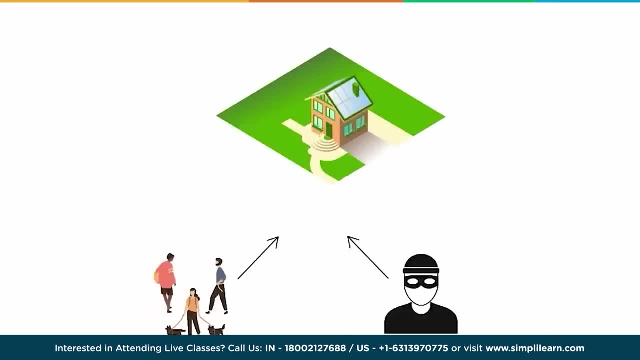 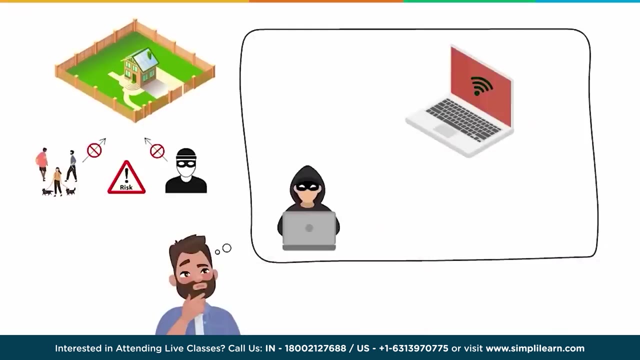 This would make our property easy accessible to trespassers and robbers and place our homes at great risk. right Hence, fencing our property helps safeguard it and keeps trespassers at bay. Similarly, Imagine our computers and networks without protection. This would increase the probability of hackers infiltrating our networks. 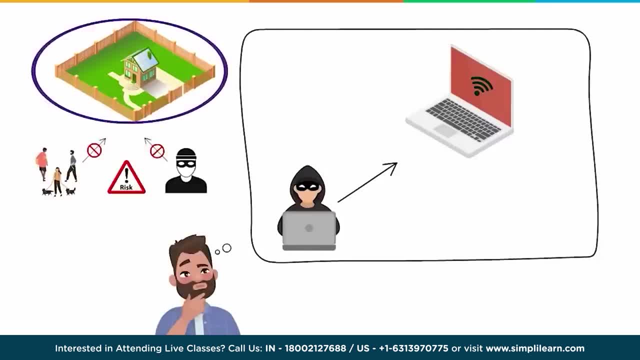 To overcome this challenge. just like how boundary walls protect our houses, a virtual wall helps safeguard and secure our devices from intruders, and such a wall is known as a firewall. Firewalls are security devices that filter the incoming and outgoing traffic within a 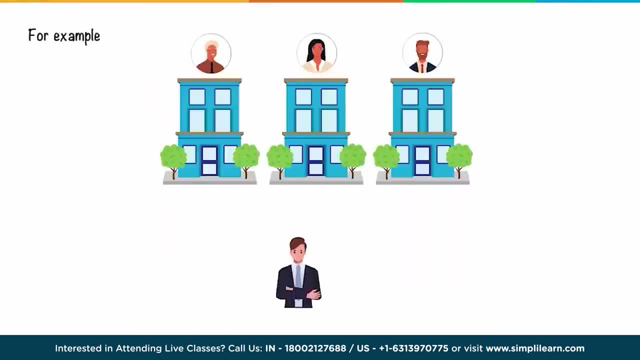 private network. For example, If you were to visit your friend who lives in a gated community- This is a security device that filters the incoming and outgoing traffic within a private community- You would first take permission from the security guard. The security guard would check with your friend if you should be allowed entry or not. 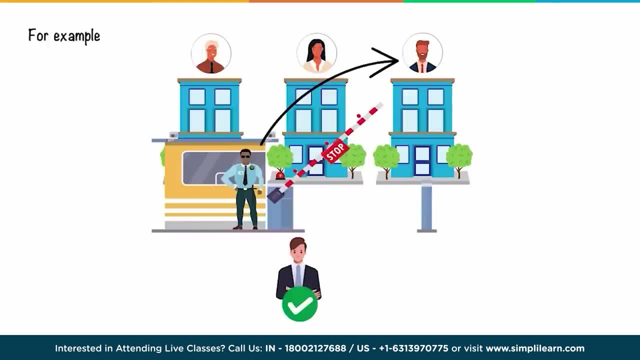 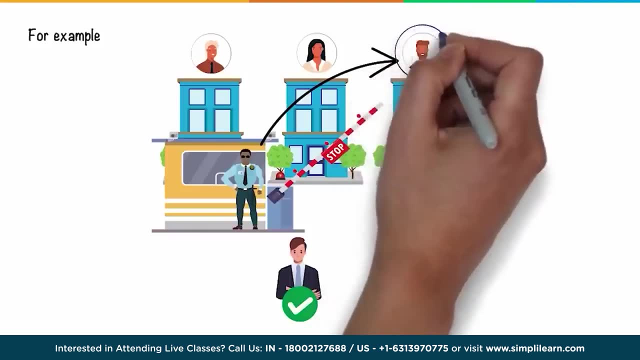 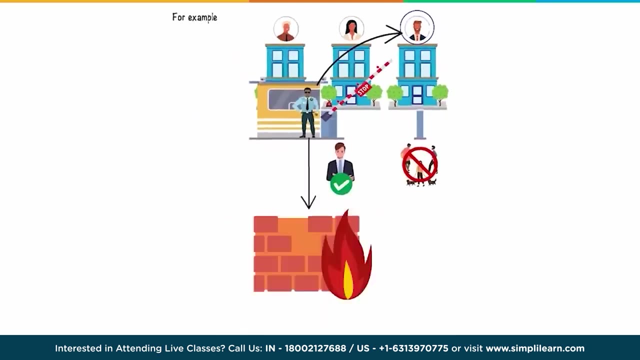 If all goes well, your access is granted. On the other hand, the security guard would not grant permission to a trespasser looking to enter the same premises. Here, the entry access depends solely on your friend, the resident's discretion. The role of the security guard in this case is similar to that of a firewall. 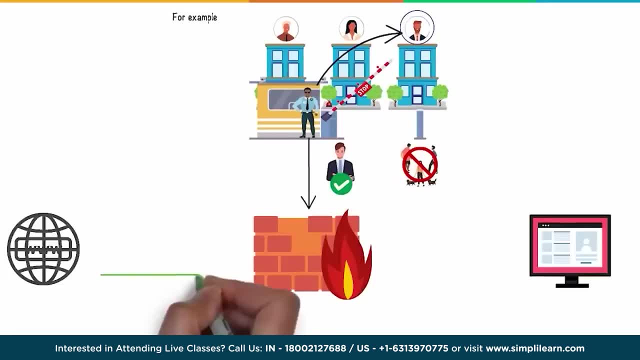 The firewall works like a gatekeeper at your computer's entry point. Just like the gatekeeper approached a building on your screen, a security guard passes by toş at a butler. If the security guard wants to talk to you, Quando chega penul. shown by security detainee. 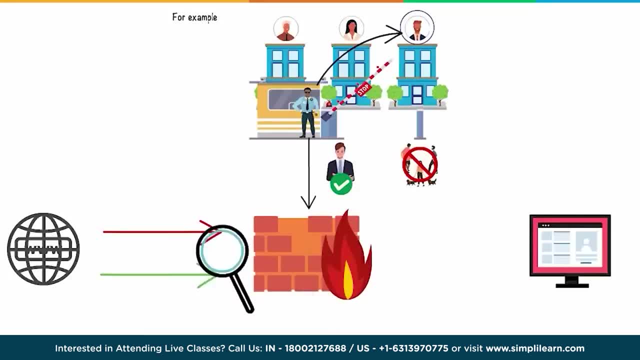 just turn your screen and watch the security guard as an Send Gold statoof weekday. It is useless to be a security guard when he gets logged out of a budget. The security guard tries its payday by purchasing one or two points that will be thick subtracting. 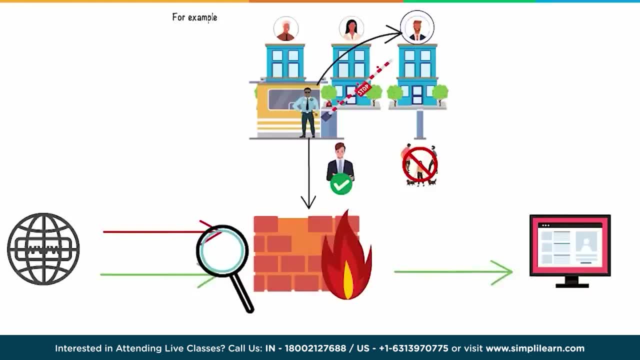 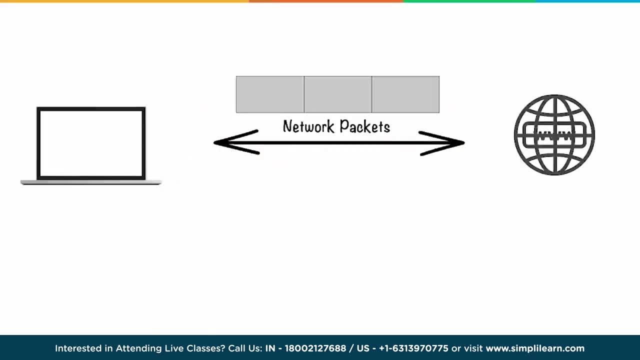 money throwing away- well worth $600,000 away- with women. The security guard will go to that website and then do a briefено with Bitcoin on salary. when she listens to the security guard, Your computer communicates with the internet in the form of network packets that hold details like the source address. 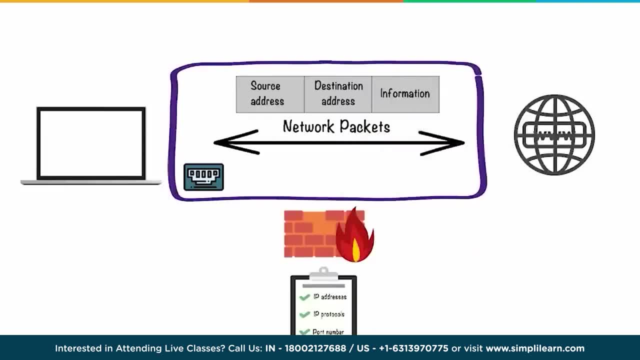 destination address and information Drink through photos. but on the internet may be the only one that matches these details of these network packets, like their source address, a destination address, content and port numbers. Only trusted traffic sources or IP addresses are allowed to enter your network. 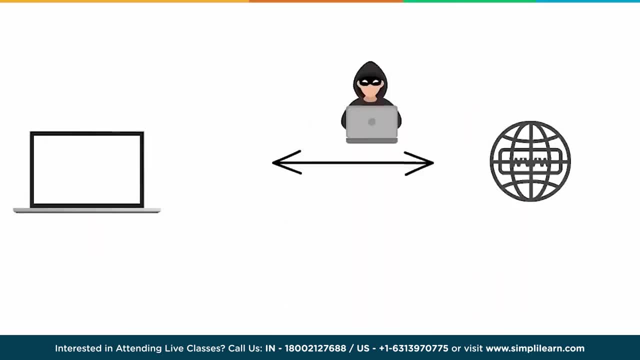 When you connect your computer to the internet, there is a high chance of hackers infiltrating your network. This is when a firewall comes to your rescue. by acting as a barrier between your computer and the internet, The firewall rejects the malicious data packet and thus protects your. 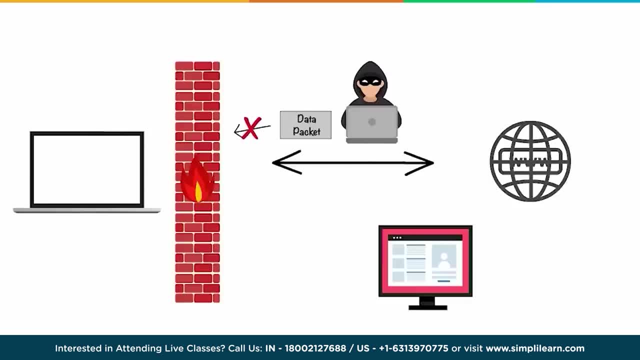 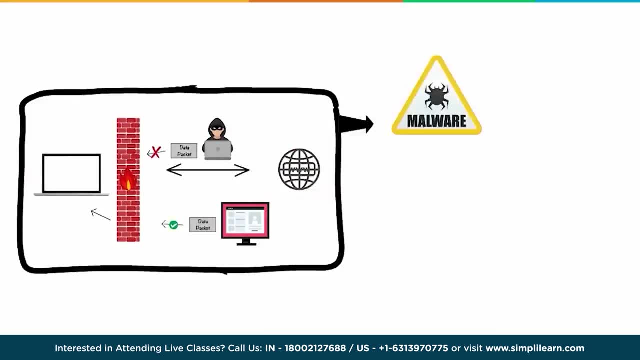 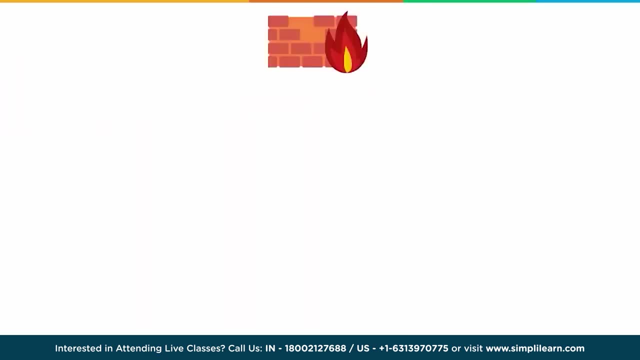 network from hackers. On the other hand, traffic from trusted websites is allowed access to your network. This way, the firewall carries out quick assessments to detect malware and other suspicious activities, thereby protecting your network from being susceptible to a cyber attack. Firewalls can either be hardware or software. Software firewalls are programs installed on 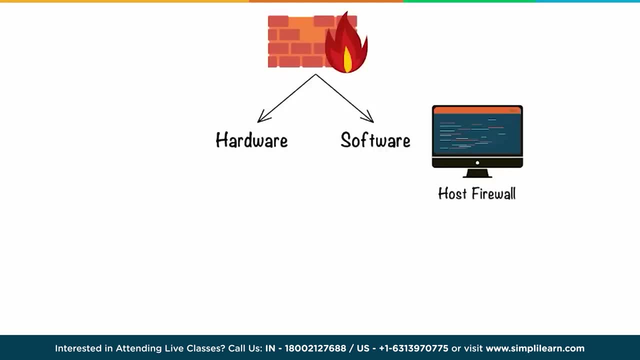 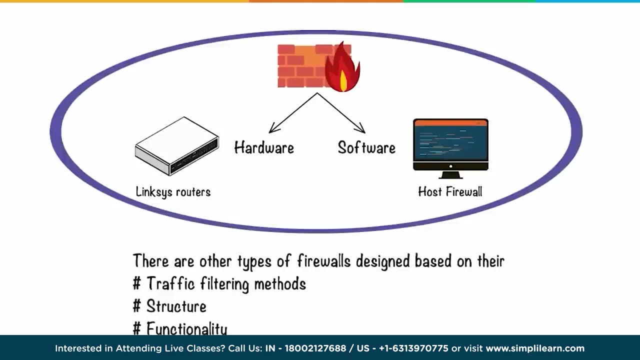 each computer. This is also called a host firewall. Meanwhile, hardware firewalls are equipments that are established between the gate of a computer and the network. In addition, there are other types of firewalls designed based on their traffic filtering methods, structure and functionality: The firewall that compares each outgoing and incoming network packet. 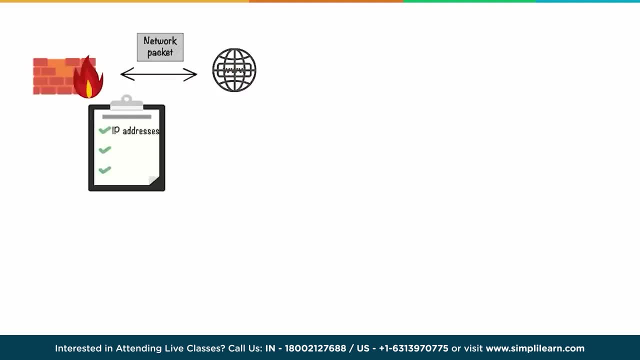 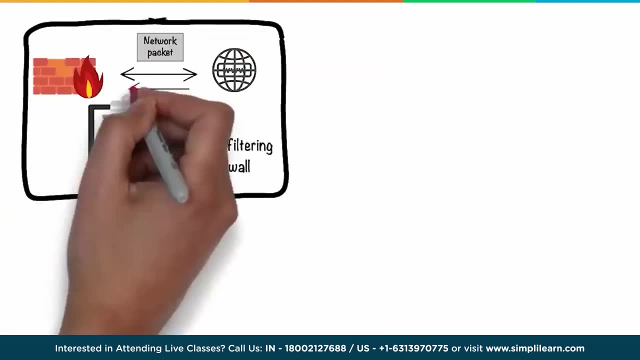 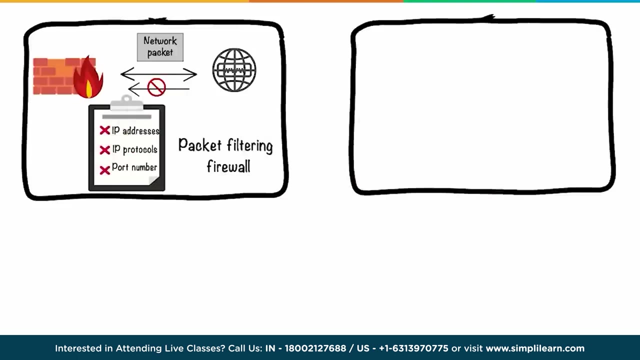 to a set of established rules such as the allowed IP addresses, IP protocols, port number and other aspects of the packet, is known as a packet filtering firewall. If the incoming network traffic is not per the predefined rules, that traffic is blocked. A variant of the packet filtering firewall is the stateful inspection. 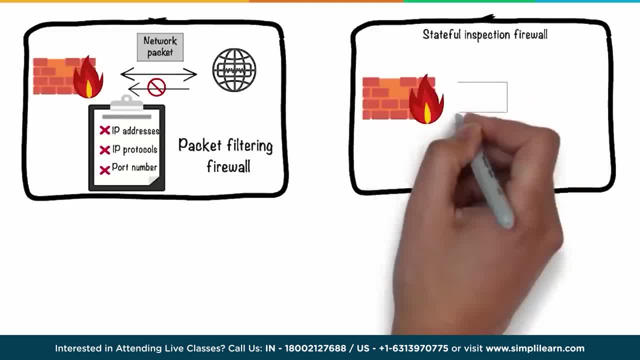 firewall. These types of firewalls not only examine each network packet, but also checks whether or not that network packet is part of an established network connection. Such firewalls are also referred to as dynamic packet filtering firewalls. Our next type of firewall is called: 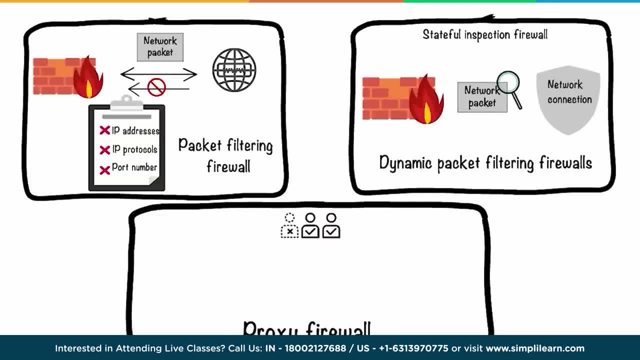 a proxy firewall. This draws close comparison to how you give proxy attendance for a friend, like how you take the authority to present your friend. The proxy firewall pretends to be you and interacts with the internet. They come between you and the internet and thereby prevents direct connections. 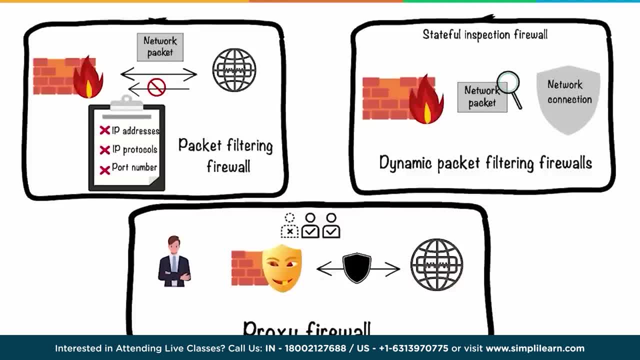 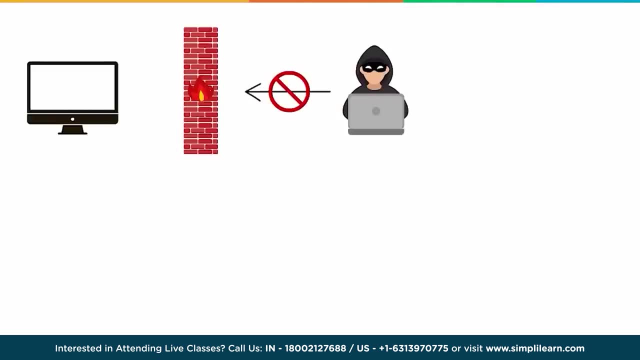 This protects your device's identity and keeps the network safe from potential attacks. Only if the incoming data packet contents are protected, the proxy firewall transfers it to you. They are also known as application-level gateway. A firewall can spot malicious actions and block your computer from receiving data packets from harmful sources. 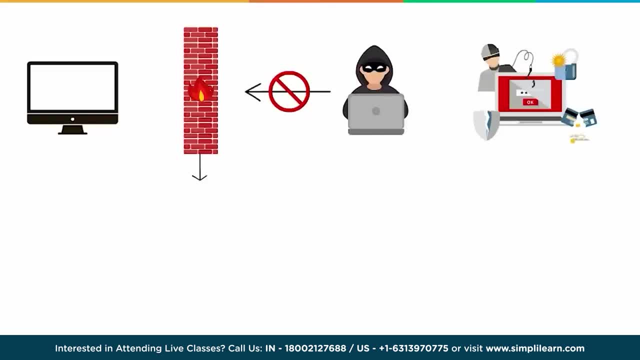 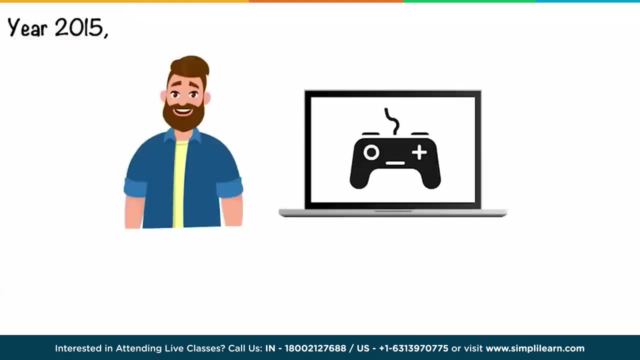 In addition to preventing cyber attacks, firewalls are also used in educational institutions and offices to restrict users' access to certain websites or applications. It is used to avoid access to unauthorized content. It's the year 2015, and Richard has just finished playing games on his computer. 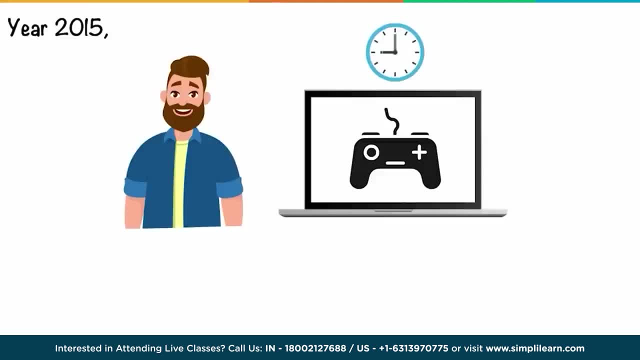 After a long gaming session, Richard tries to shut it down, but finds some random text file on the desktop that says Ransom Note. The text file mentioned how a hacking group had increased the number of hackers on the desktop and how the hacking group 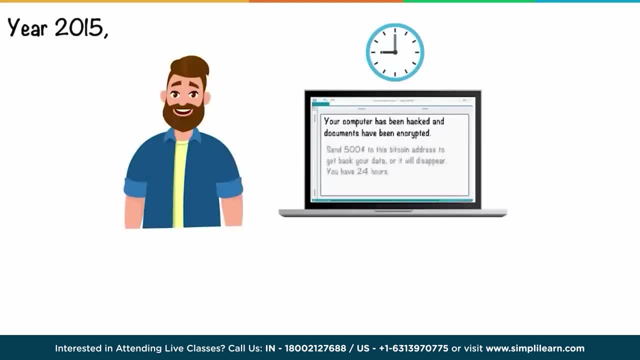 encrypted Richard's game files and private documents and he had to pay a ransom of $500 worth of Bitcoin in a specified Bitcoin address. Richard quickly checked his files only to see them being encrypted and unreadable. This is the story of how the Tesla Crypt ransomware 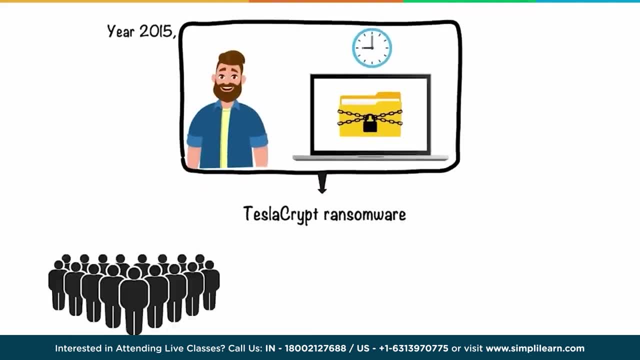 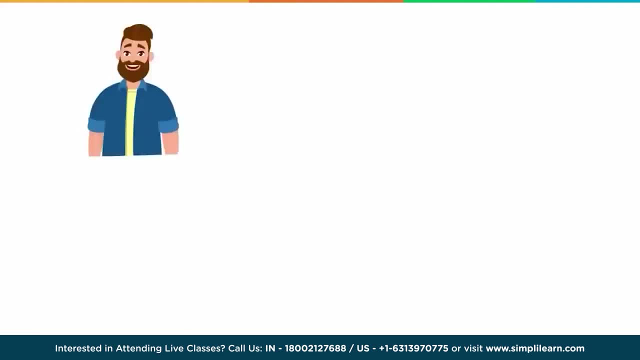 spread in 2015,, which affected thousands of gamers, before releasing the master key used for encrypting the files. So what is ransomware For Richard to be targeted by such an attack? he installed applications from untrusted sources or clicked an unverified link. Both of them can. 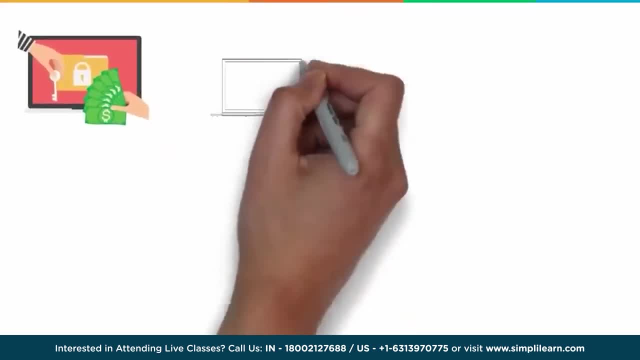 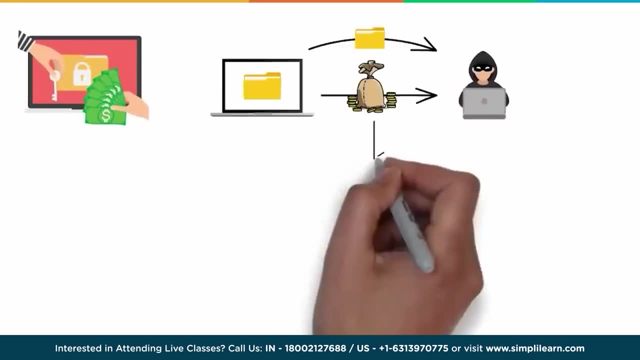 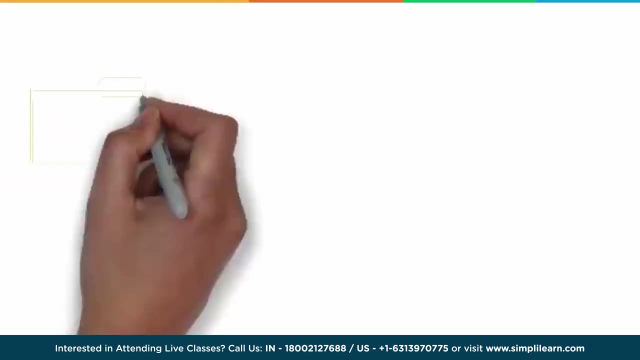 function as gateways for a ransomware breach. Ransomware is a type of malware that encrypts personal information and documents while demanding a ransom amount to decrypt them. This ransom payment is mainly done using cryptocurrency to ensure anonymity, but can also employ other routes Once the files are encrypted or locked behind a password. 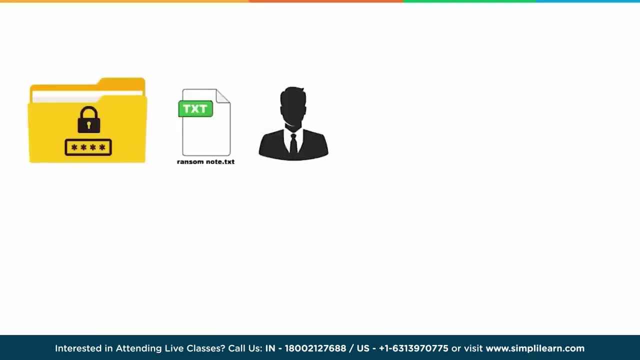 a text file is available to the victim explaining how to make a ransom payment and unlock the files for it, Just like Richard found the ransom note text file on his desktop Even after the money has been paid. there is no guarantee that the hackers will send the decryption key or unlock the files, But in certain sensitive situations. 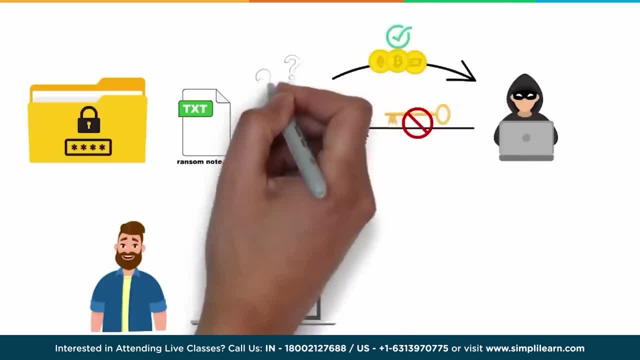 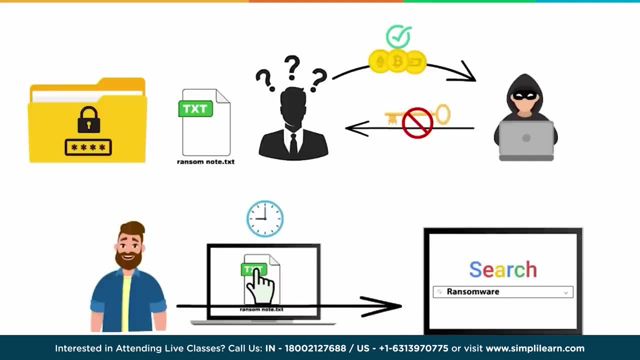 victims make the payment, hoping for the best. Having never been introduced to ransomware attacks before, this gave Richard an opportunity to learn more about this and he began his research on the topic. The spread of ransomware mostly starts with phishing attacks. To know more about phishing attacks: 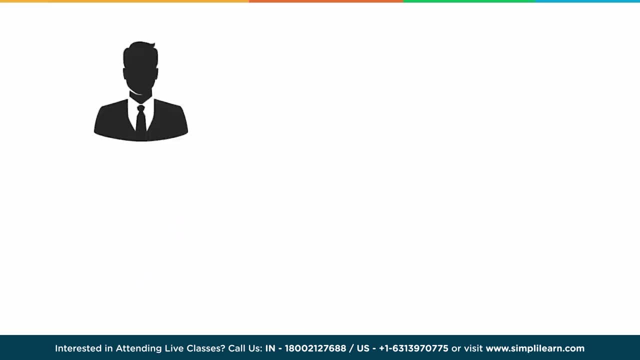 click the link in the button above. Users tend to click on unknown links received via emails and chat applications, promising rewards of some nature. Once clicked, a ransomware file is installed on the system that encrypts all the files or blocks access to computer functions. They can also be spread via malware. 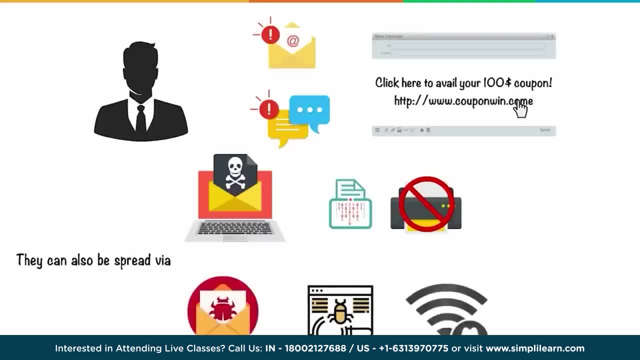 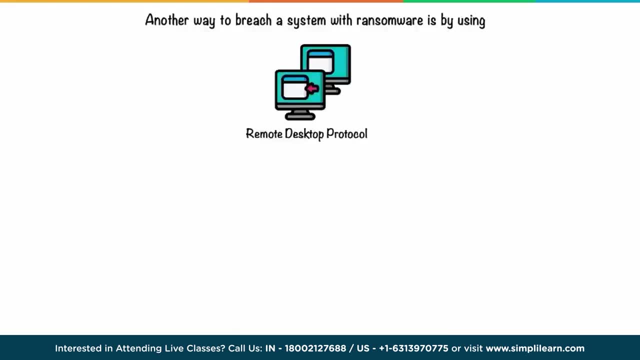 transmitted via untrusted application installation or even a compromised wireless network. Another way to breach a system with ransomware is by using the Remote Desktop Protocol or RDP access. A computer can be accessed remotely using this protocol, allowing a hacker to install malicious software on the system. 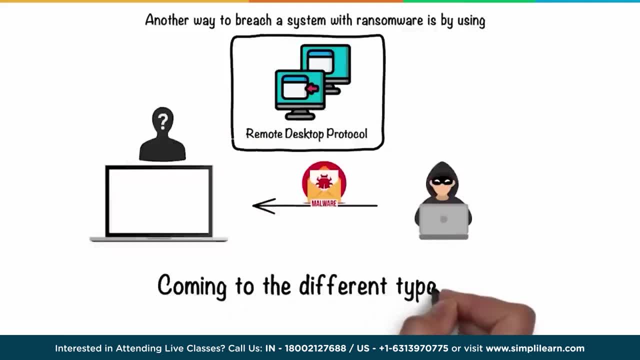 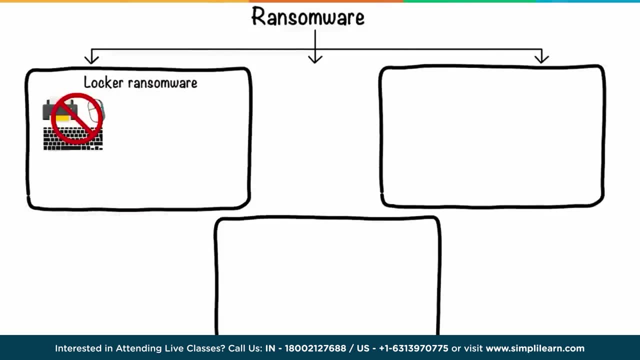 with the owner unaware of these developments. Coming to the different types of ransomware, First we have Locker Ransomware, which is a type of malware that blocks standard computer functions from being accessed until the payment to the hackers is complete. It shows a lock screen that doesn't allow the victim to use the computer. 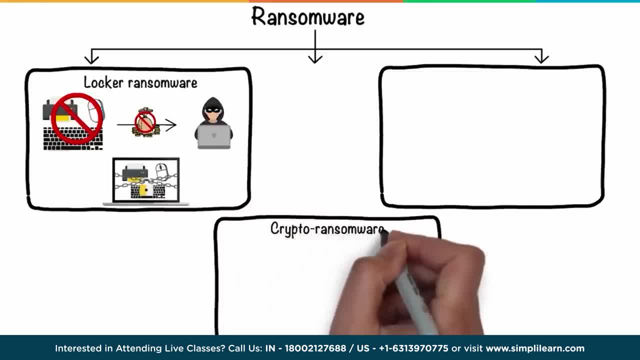 for even basic purposes. Another type is Crypto Ransomware, which encrypts the local files and documents in the computers. Once the files are encrypted, finding the decryption key is impossible, unless the ransomware variant is old and the keys are already available on the internet. 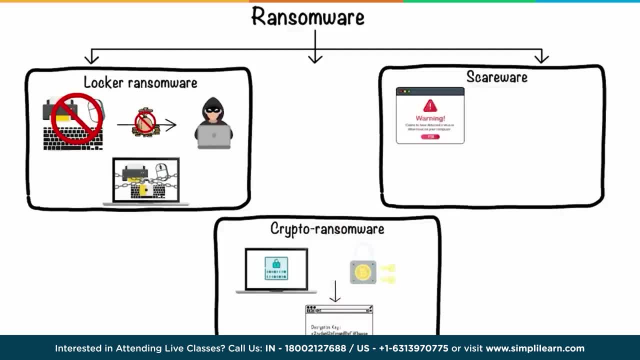 ScareWare is fake software that claims to have detected a virus or other issue on your computer and directs you to pay to resolve the problem. Some types of ScareWare lock the computer, while others simply flood the screen with pop-up alerts without actually damaging files. 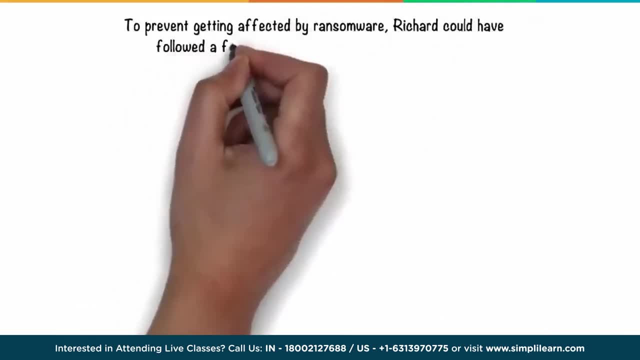 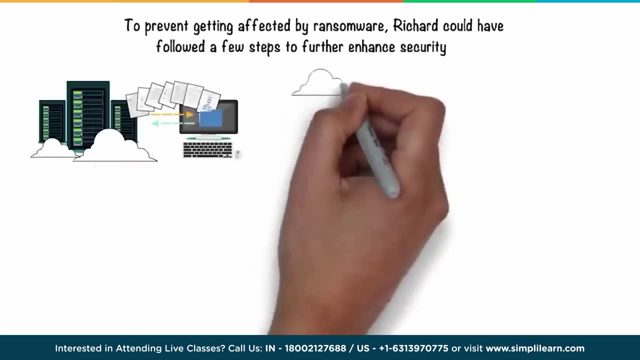 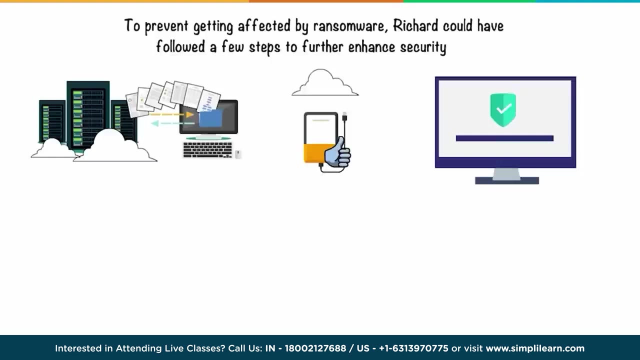 To prevent getting affected by ransomware. Richard could have followed a few steps to further enhance his security. One must always have backups of their data. Cloud storage for backup is easy, but a physical backup in a hard drive is always recommended, Keeping the system updated with the latest security patches. 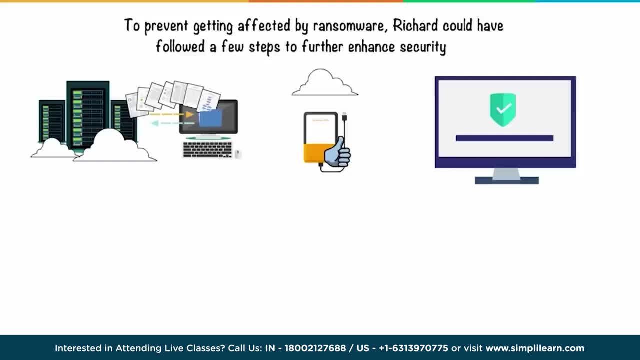 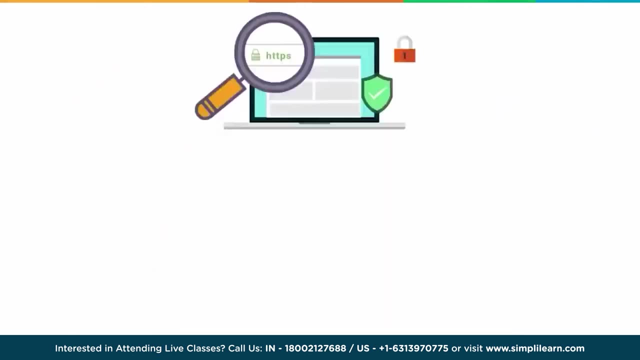 is always a good idea. Apart from system updates, one must always have reputed antivirus software installed. Many antivirus software like Kaspersky and Bitdefender have anti-ransomware features that periodically check for encryption of private documents. When browsing the internet, a user must always check for the lock symbol on the address bar. 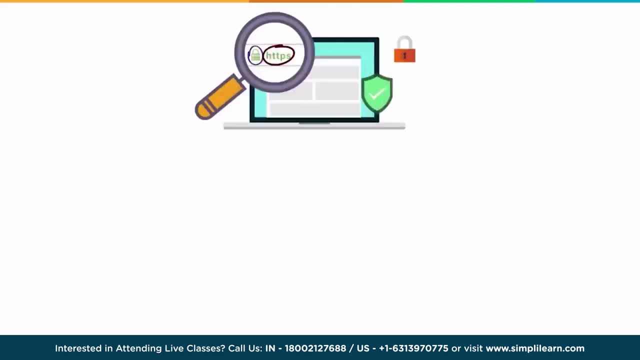 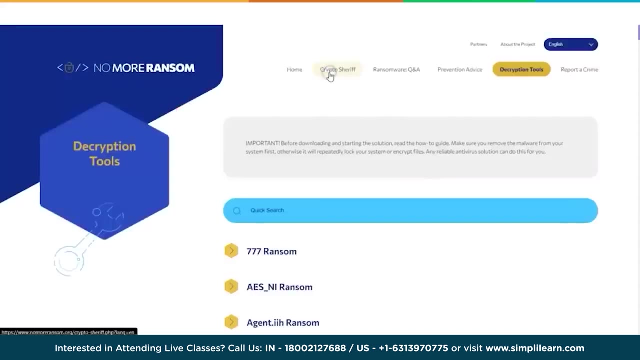 which signifies the presence of HTTPS protocol for additional security If the system is infected with ransomware. already there is a website, nomoreransomorg. It has a collection of decryption tools for most well-known ransomware packages. it can also help decrypt specific encrypted files, if the list of anti-ransomware tools didn't help the victim. 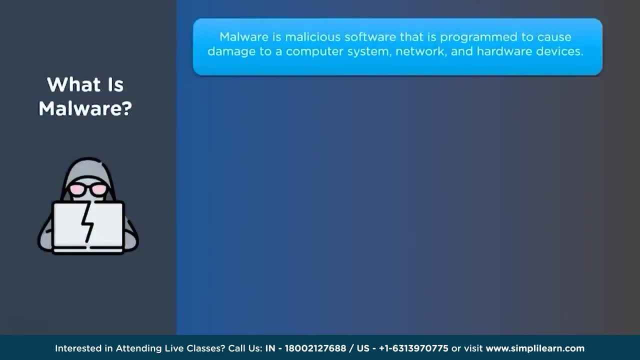 Malware is a malicious software that is programmed to cause damage to a computer system, network and hardware devices. Many malicious programs, like Trojan viruses, bombs and bots, which cause damage to the system, are known as malware. Most of the malware programs are designed to steal information from the targeted user or 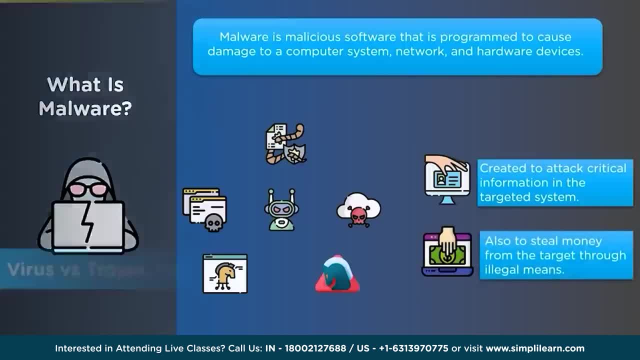 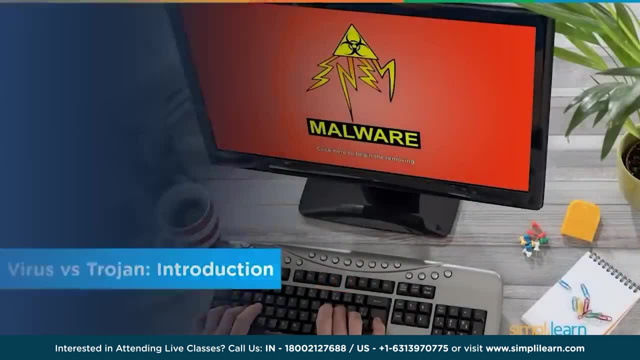 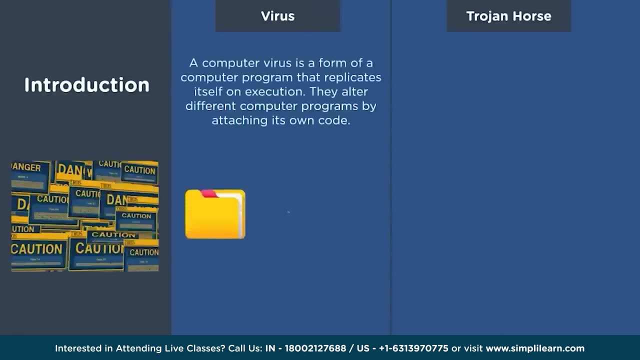 steal money from the target and by stealing sensitive data. Let's look at the introduction for two different types of malware – virus and Trojan. Firstly, let's take a look: what exactly is a virus program? A computer virus is a type of malicious program that, on execution, replicates itself. 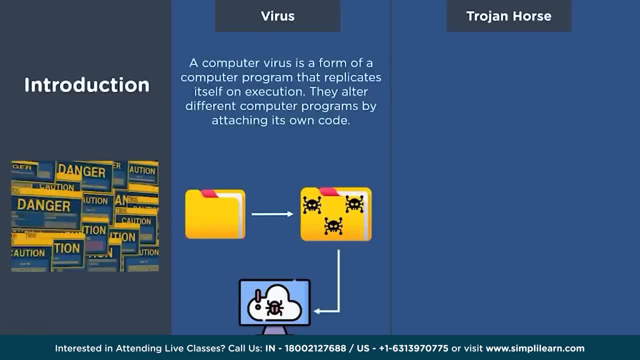 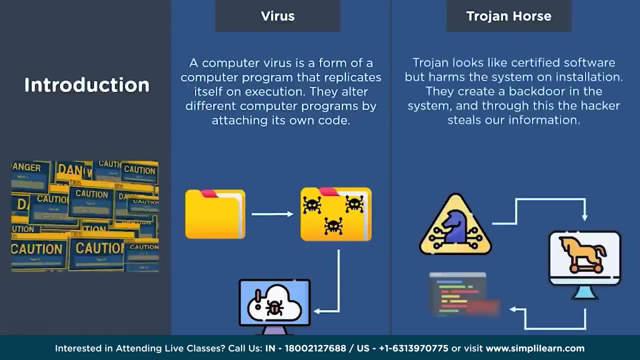 They get attached to different files and programs, which are termed as host programs. by inserting their code In the attachment succeeds, the targeted program is termed as infected with a computer virus. Now let's take a look at the Trojan horse. Trojan horse program is a 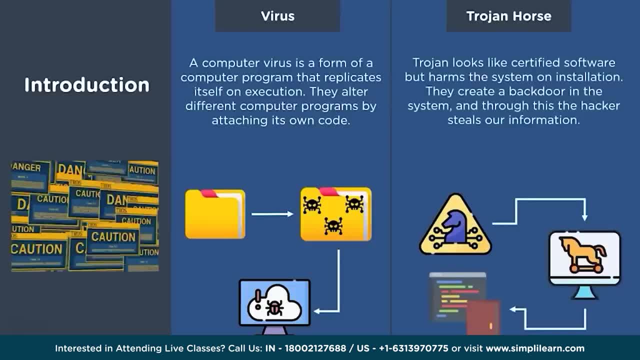 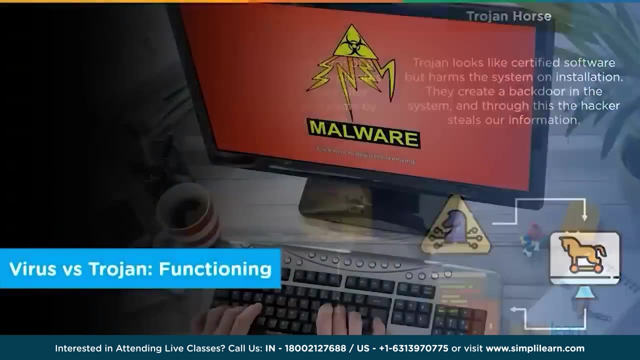 program that disguises itself as a legitimate program but harms the system on installation. They hide within the attachments and emails, then transfer from one system to another. They create bad doors into a system to allow the cyber criminal to steal our information. Let's take a look how they function. 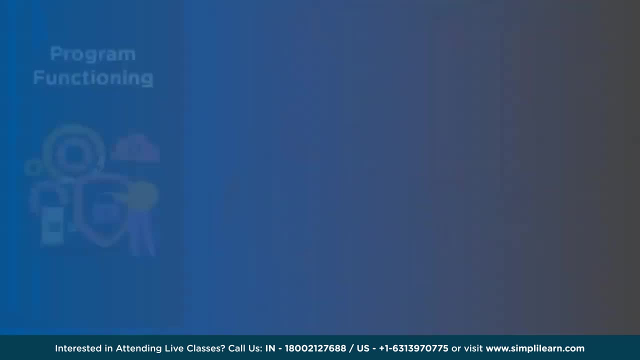 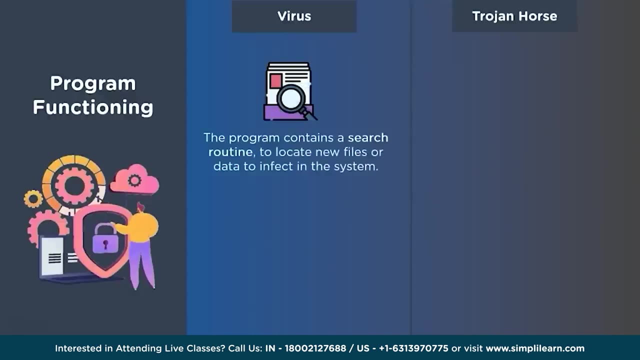 after getting installed into a system. Firstly, we have virus programs. The computer virus must contain two parts to infect the system. First is a search routine which locates new files and data that is to be infected by the virus program, and the second part is known as the copy routine, which is necessary for 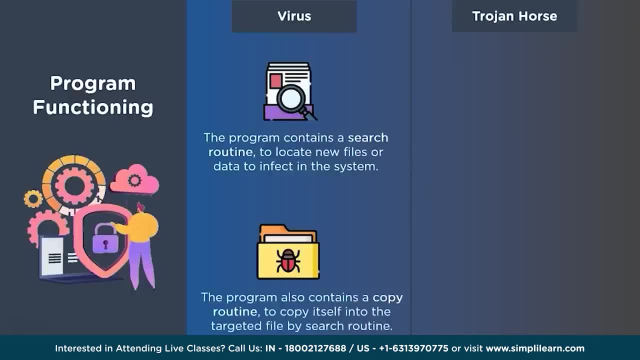 the program to copy itself into the system. This is the targeted file, which is located by the search routine. Now let's take a look at the Trojan horse functioning. For Trojan horses, entry way into our system is through emails that may look legitimate but may have unknown attachments and 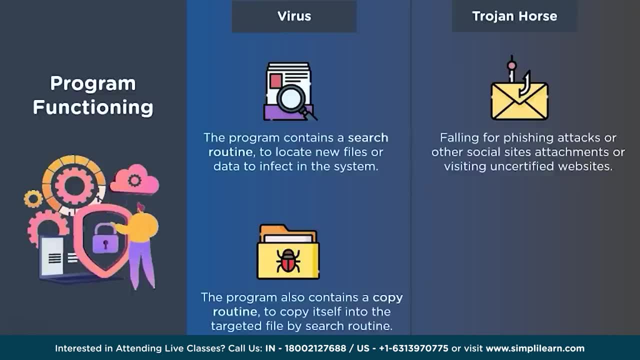 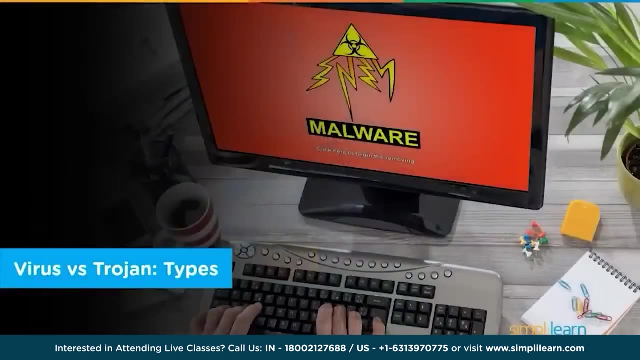 when such files are downloaded into the device, the Trojan program gets installed and infects the system. They also infect the system on the execution of infected application or the executable file and attacks the system. Now that we understand what virus and Trojans are, let's understand different. 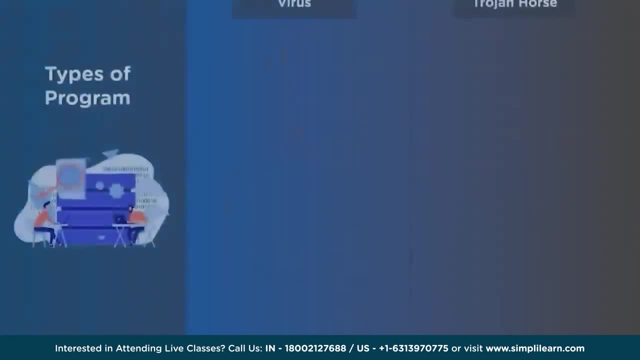 types of virus and Trojans. Let's take a look at different types of viruses. The first one is known as the boot sector virus. This type of virus damages the booting section of the system by infecting the master board record, which is also known as MBR. This damages the boot sector section by targeting the 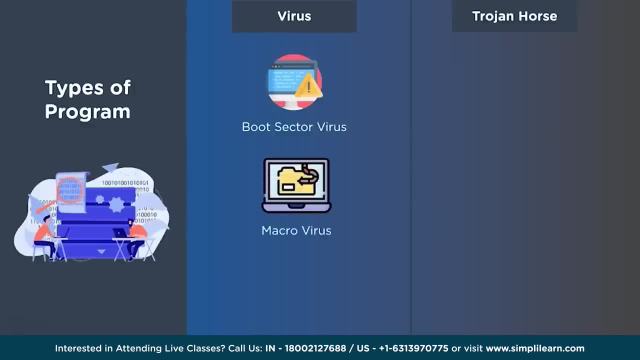 hard disk of the system. Then we have the macro virus. Macro virus is a type of virus that gets embedded into the document related data and is executed when the file is open. They also are designed to replicate themselves and infect the system on a larger scale. And lastly, we have the 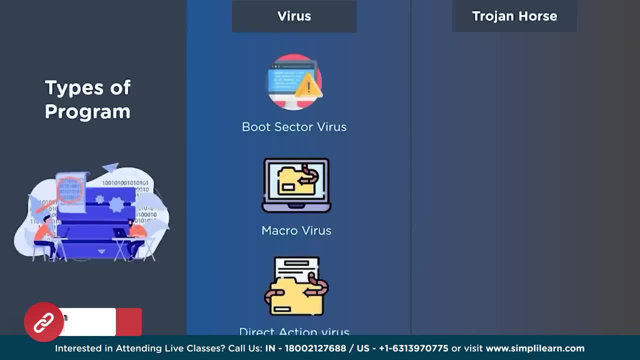 direct action virus. This type of virus gets attached to executable files which, on execution, activates the virus program and infects the system. Once the infection of the file is completed, they exit the system, which is also the reason it is known as a non-resident. 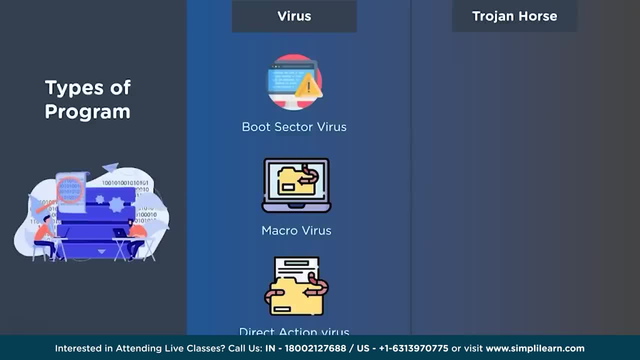 virus. Let's take a look at different types of Trojans. The first type of Trojan is the backdoor Trojan. They are designed to create a backdoor in the system on execution of an infected program. They provide remote access of a system to the hacker. This way, the cyber criminal can steal our 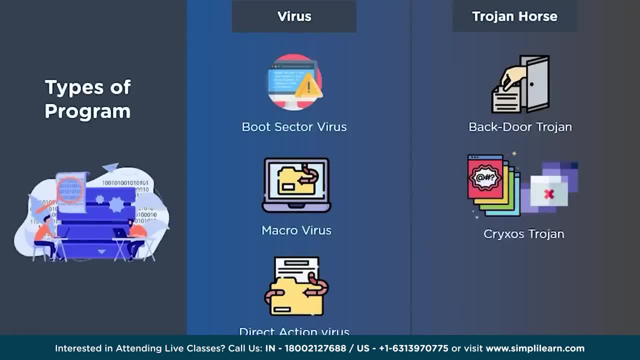 system data and may use it for illegal activities. Next we have a crick sauce Trojan. They enter the system by clicking the random pop-ups which we come across on the Internet. They attempt the user to give their personal details for different transactions or schemes Which may. 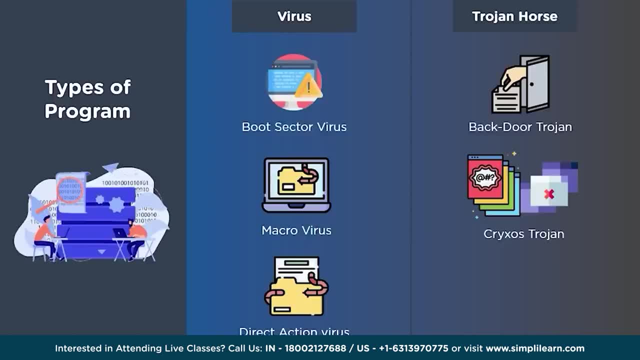 provide remote access of a system to the cyber criminal, And the last Trojan type is a ransom Trojan. This type of Trojan program, after entering the system, blocks the user from accessing its own system and and also affects the system function. The cybercriminal demands a ransom from the targeted user for the removal of the Trojan. 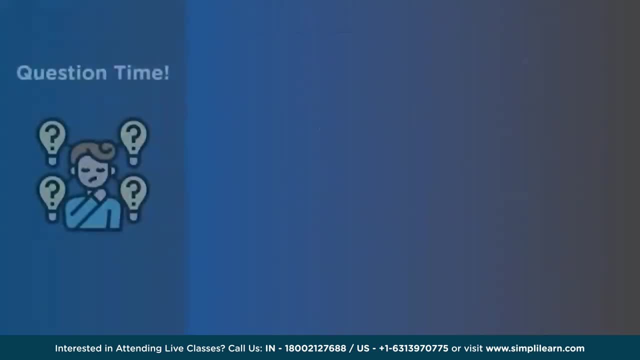 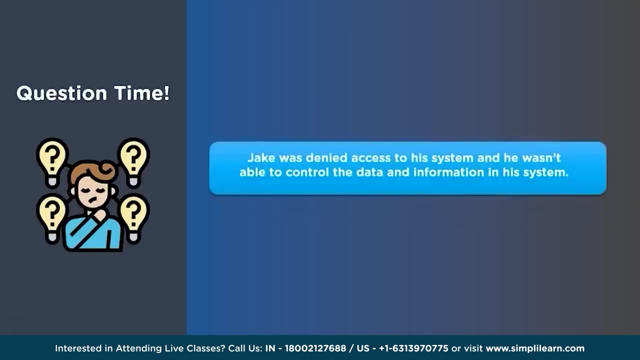 program from the device. Now that we understand some details regarding viruses and Trojan, let's solve a question. The question is: Jake was denied access to his system and he wasn't able to control the data and information in his system. Now the actual question is: what could be the reason behind his system's problem? 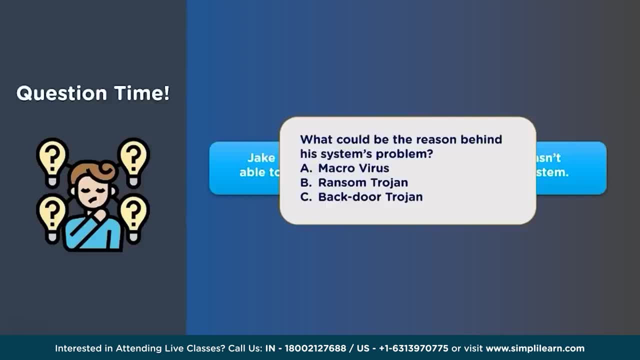 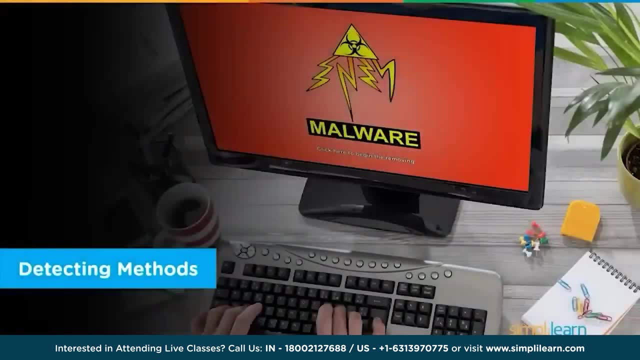 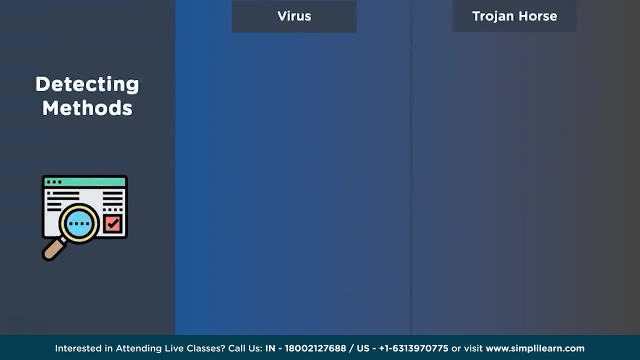 Option A: Macro virus. Option B: Ransom Trojan. Option C: Bagdor Trojan. Give your answers in the comment section. Now let's understand how to detect the activity of viruses and Trojan in a system. To detect virus or Trojan activity in a system, we can refer to the following points. 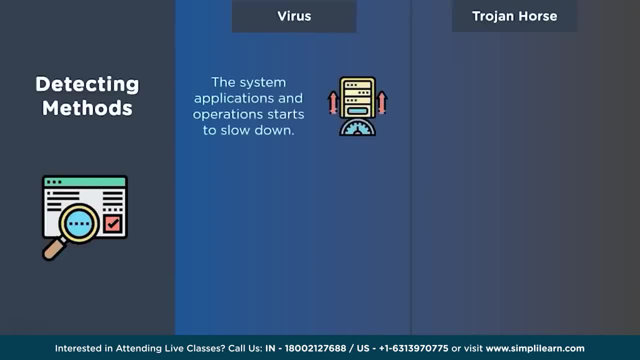 For viruses, we have slowing down of the system And frequent application freeze shows that the infection of the virus is present in the system. Then we have the viruses can also steal sensitive data, including passwords, account details, which may lead to unexpected logout from the accounts or corruption of the sensitive data. 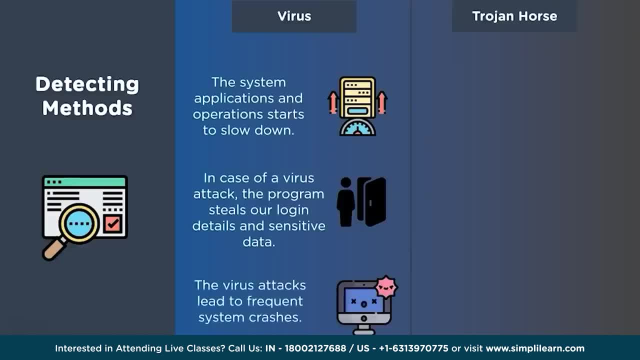 And lastly, we have frequent system crashes due to virus infection which damages the operating system For Trojan. we have frequent system crashes And system also faces slow reaction time. Then we have more random pop ups from the system which may indicate Trojan activity. 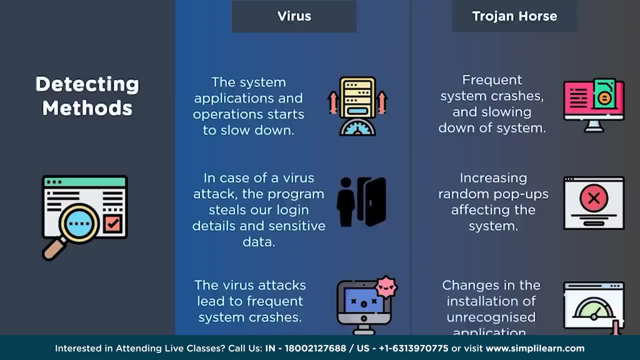 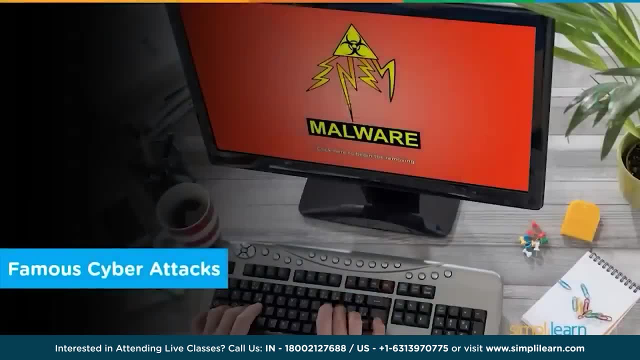 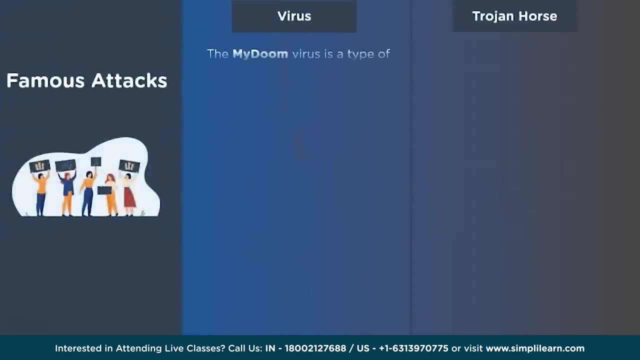 And lastly, we have modification in the system application and change of the desktop appearance can be also due to the infection of the Trojan program. Next, let's take a look at a famous cyber attack for virus and Trojan horse For virus. we have the MyDoom virus. 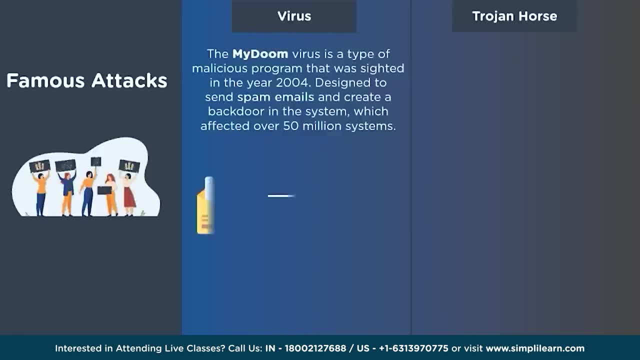 which was identified in the year 2004, which affected over 50 million systems, by creating a network of sending spam emails which was to gain backdoor access into our systems. Next, for the Trojan horse, we have the Emotat Trojan program, which is specifically designed for financial theft and for stealing bank. 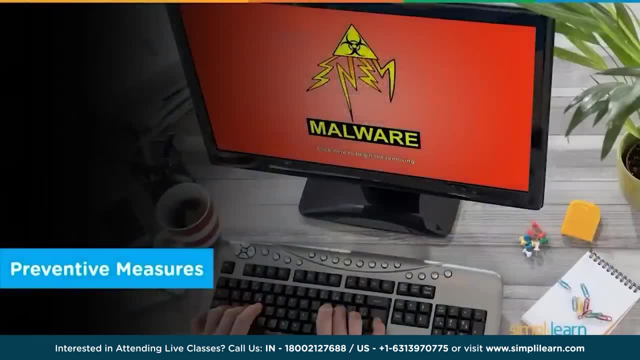 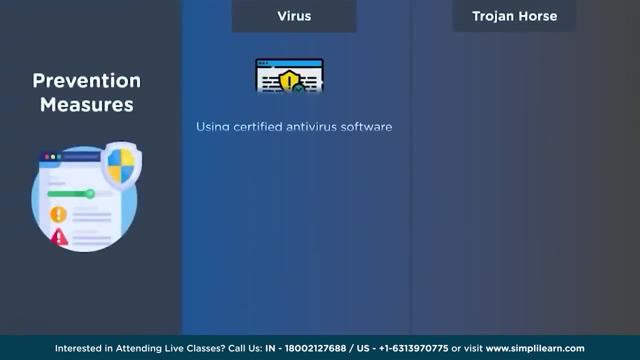 related information. Next, we have few points for how to prevent virus entry or Trojan attack for a system. The most basic way of virus protection is to using antivirus and do regular virus scan. This will prevent virus entry in the system and also, having more than one antivirus provides a much better. 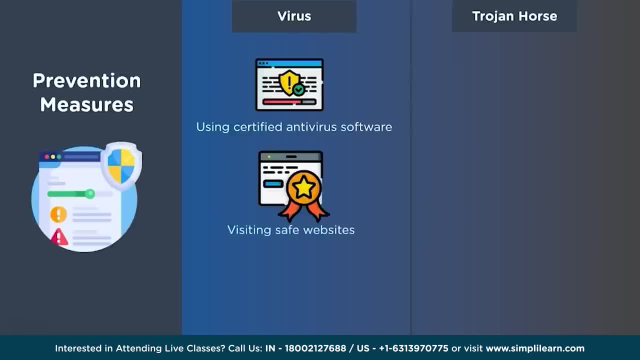 protection. Then avoid visiting uncertified websites can also prevent virus entry into our system. Then we have using regular driver updates and systems- Some updates- to prevent virus entry For Trojan. we have using certified softwares from legal sites to prevent any Trojan activity in our system and also avoid. 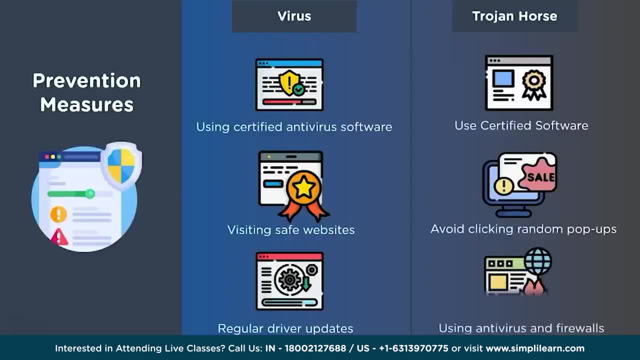 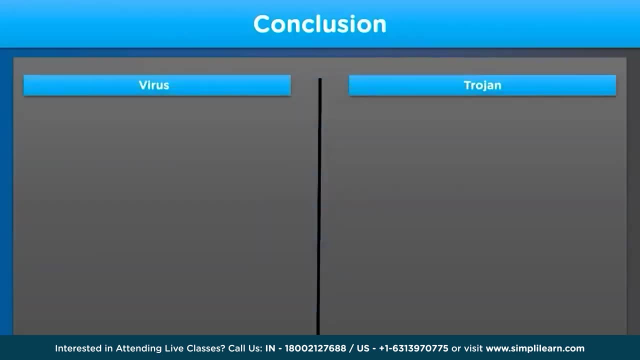 clicking random pop-ups that we often see on the Internet And, lastly, using antivirus and firewalls for protection against Trojan horses is a good habit. Now that we have reached the end of the video, let's take a look what we learned. For the first part, we will be talking about how to prevent virus entry into our system. 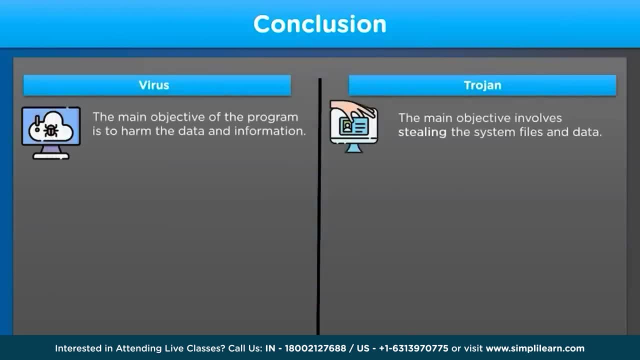 For the first part we saw the main objective of the virus is to harm the data and information in a system, whereas for the Trojan we have stealing of the data files and information. Effect of viruses is more drastic in comparison to the Trojan horses. Then we have viruses which are non remote programs, whereas Trojan 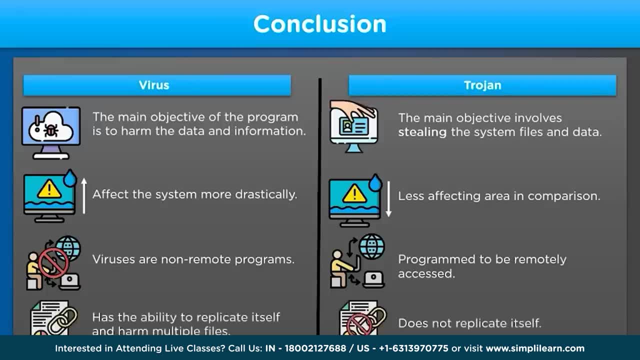 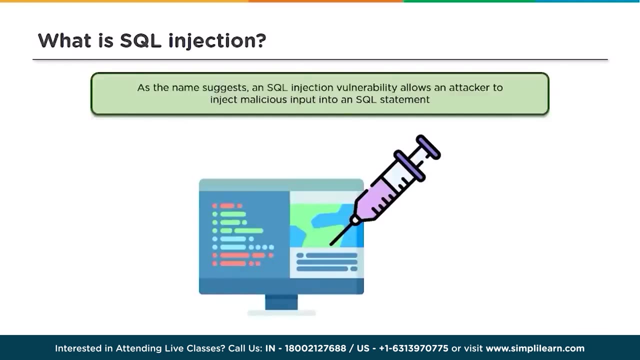 horses are remote accessed. And, lastly, viruses have the ability to replicate itself to harm multiple viruses. And, lastly, viruses have the ability to replicate itself to harm multiple files, whereas Trojan does not have the replication ability. So let's begin with. what is SQL injection? As the name suggests, SQL injection vulnerability. 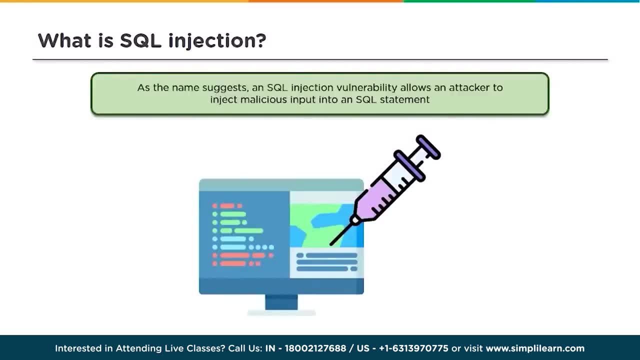 allows an attacker to inject malicious input into a SQL statement. So SQL stands for structured query language, which is a language used by an application to interact with a database. Now, normally this attack is targeted towards a database to extract the data that is stored within. However, the 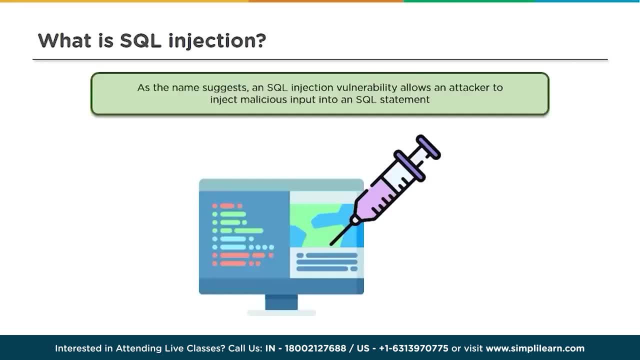 vulnerability does not lie in the database itself. The vulnerability will always lie in the application. It is the developer's prerogative of how to develop the application, how to configure it to prevent SQL injection queries from happening. A database is created to answer questions, and if a question is, 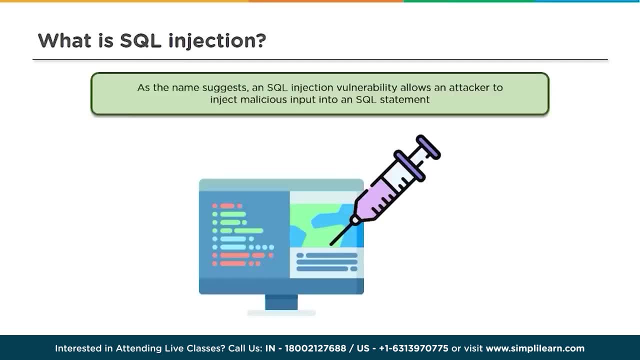 asked, it is supposed to answer it. Database needs to be configured for some amount of security, but the vulnerability, the flaw here for SQL injection will always lie in the application itself. That is how the application interacts with the database. that needs to be modified, that needs to be maintained by the developer rather than just configuring. 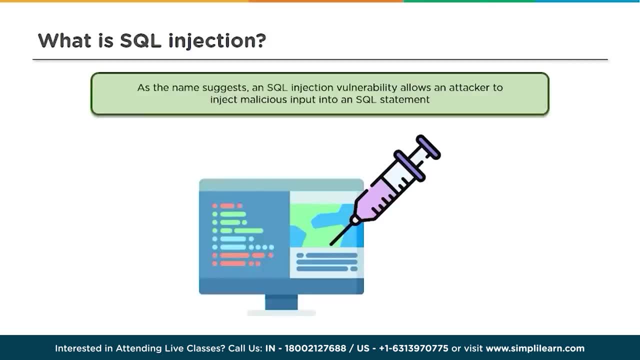 the database itself. So the attacker, at this point in time when they send a query to the application, will form a malformed query by injecting a particular command or an operator that is recognized by the SQL language, and if that operator is passed through the application to the database, then the database basically gets. 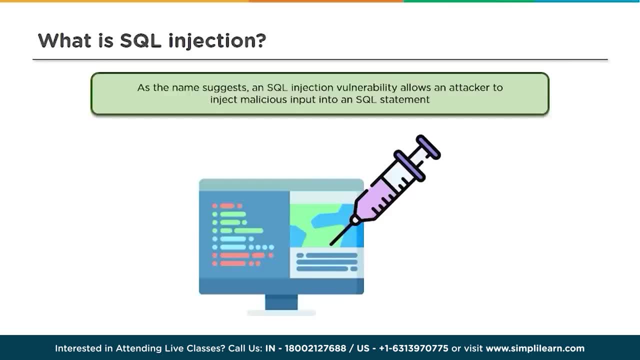 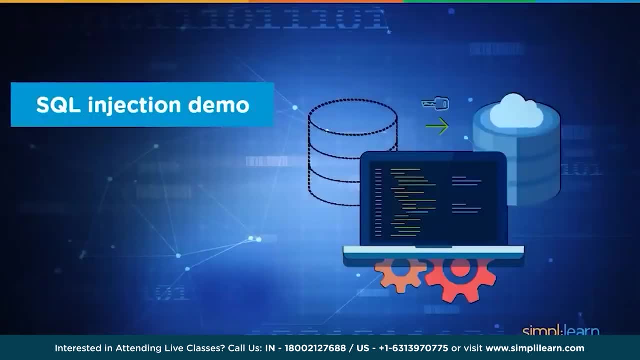 out does a data dump because of that unwanted character coming in, So this character needs to be filtered at the application level itself. Now let's look at a quick demo. So what we have done here is I have this virtual machine called OWASP- broken web applications virtual machine, version 1.2.. I'm going to 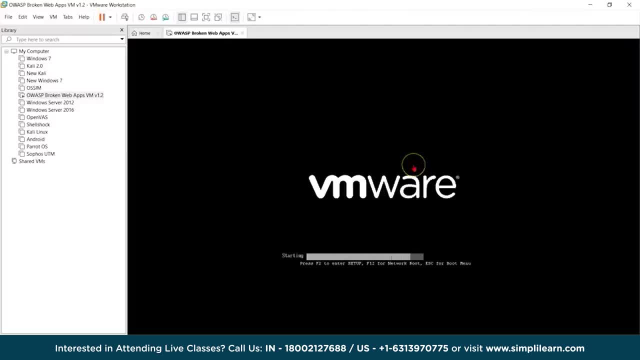 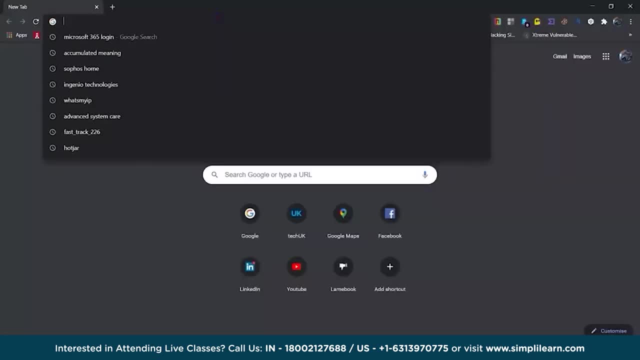 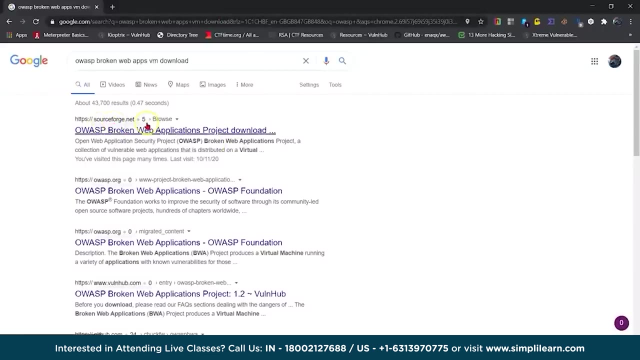 power this on Till this power is on. I'm going to show you where you can download this YouTube video. So you can just look for OWASP broken web application project download. You'll find it on sourceforcenet. Click on the link. You can download the broken web. 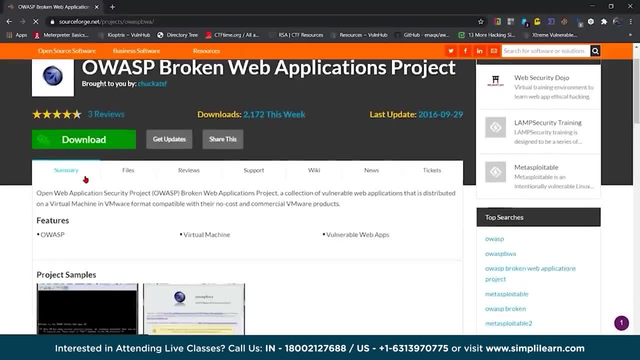 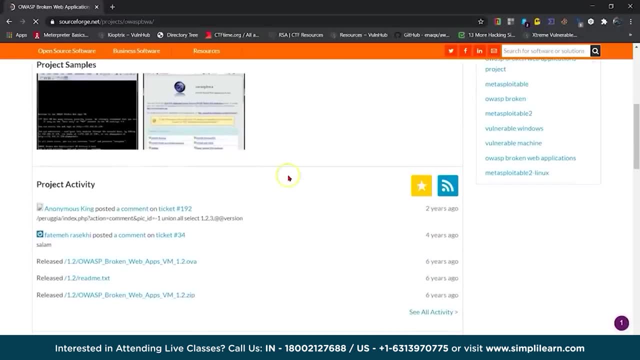 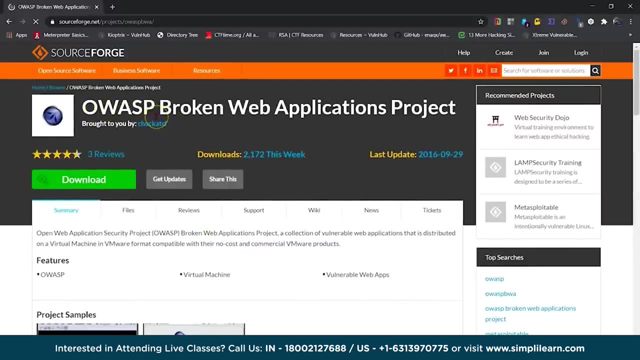 application project from here. This is a 1.9 GB download and you can have a zip machine directly for VMware or Oracle VirtualBox. Now, this is an application that has been developed by OWASP, which stands for open web application security. This is a non-profit organization and periodically releases the most top 10. 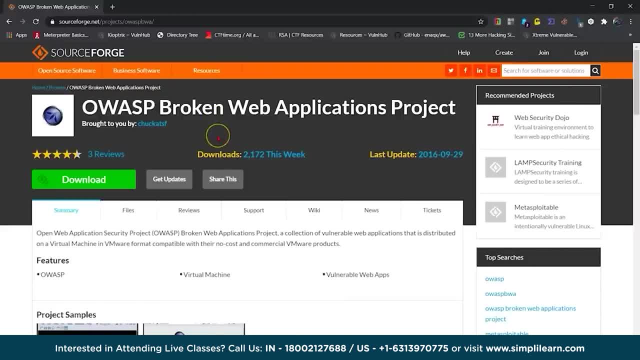 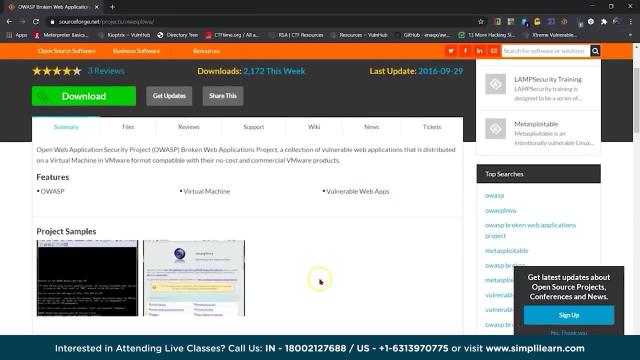 risks that an application will face for that particular year. So they have given a web application with inbuilt vulnerabilities for professionals like us to practice upon, to develop our skills upon, because doing this in the real world is illegal. I cannot go onto a website to demonstrate how a SQL engine is working. 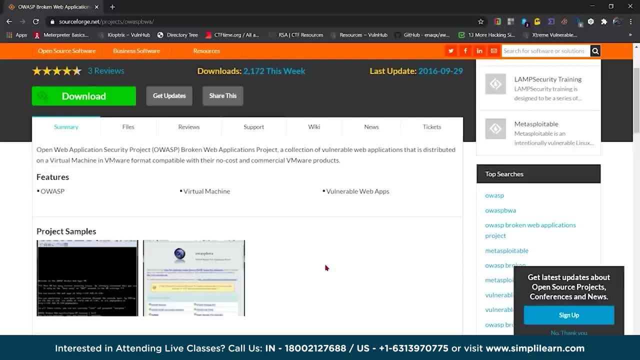 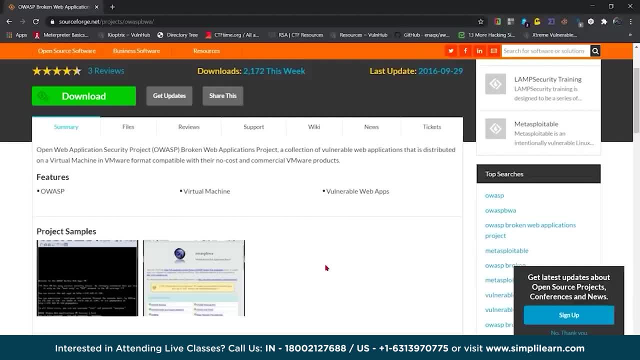 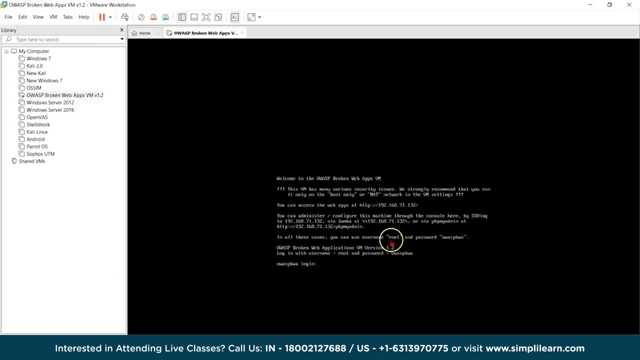 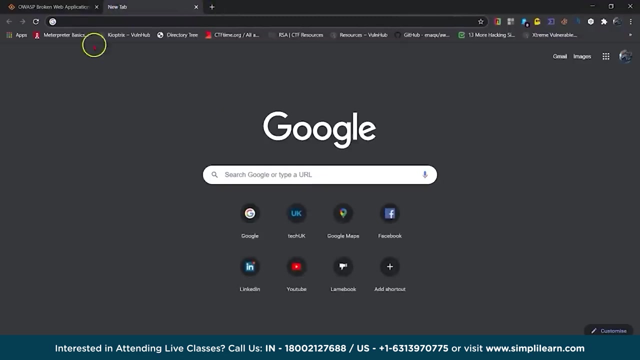 Neither should you try your hands on it till you become very well rehearsed with it. To upgrade your skill and upskill yourself, please download this machine information box and then try your skills on it. So just going back to the browser here, if I open up a new tab, you will see. 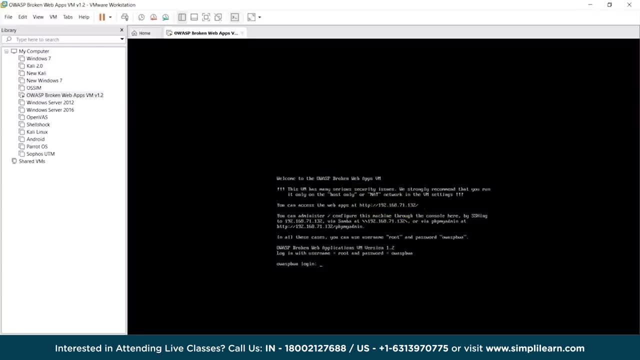 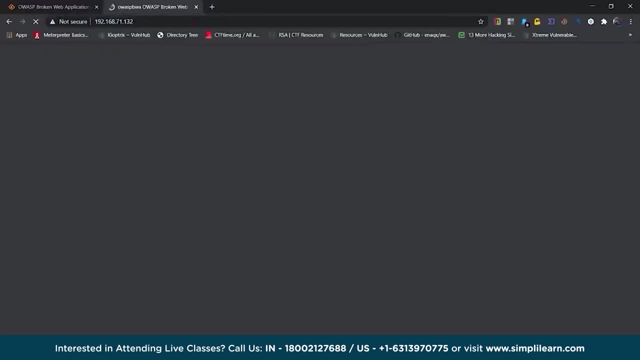 that this machine has booted up and has an IP address called 71.132. so if I just go on to that IP address and then I type in 192.168.71.132 and you'll see the OWASP broken web application project and there are a lot of training. 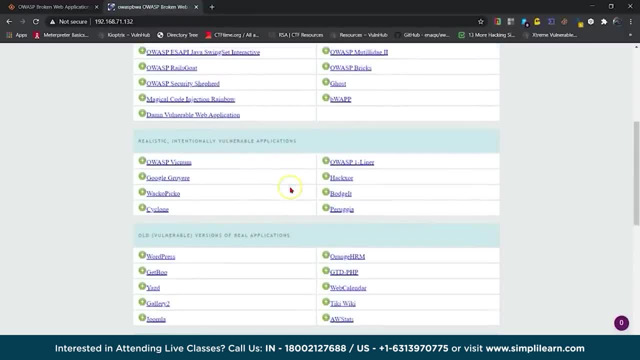 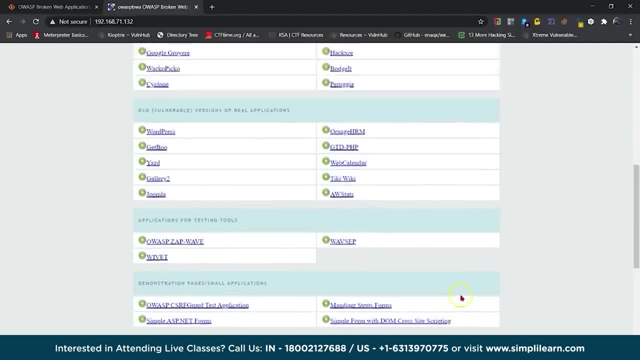 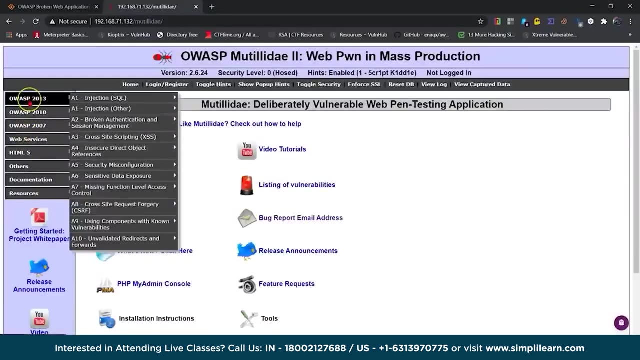 applications, realistic, intentionally vulnerable applications, old versions of real applications, and so on, so forth. so there is a lot of applications inbuilt over here that you can try your skills upon. we are going to try to use the OWASP mutility over here. this gives you the 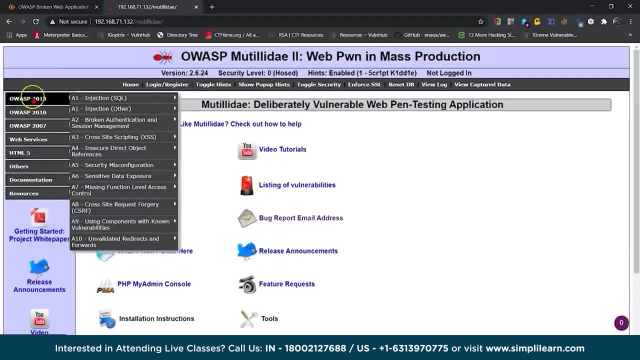 OWASP top 10 risks for 2010, 2013, 2017 is the latest one so far, but the difference between 2013 and 2017 is that some of these have changed, but not all of them. the order has changed a little. 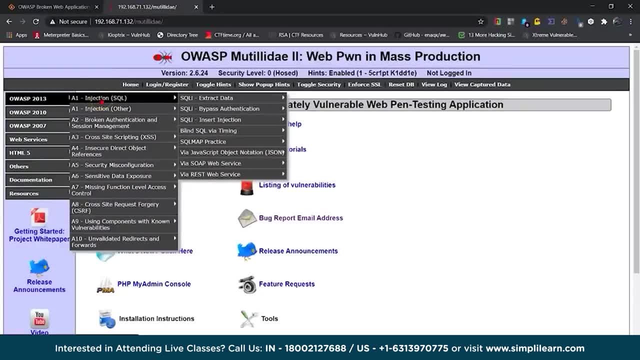 bit, but you can see that SQL injection is on the top A1 amongst the injection attacks, right? and you can see that SQL injection is on the top A1 amongst the injection attacks, right? and you can see that there are multiple types that have been given here: the SQL injection for extracting data. 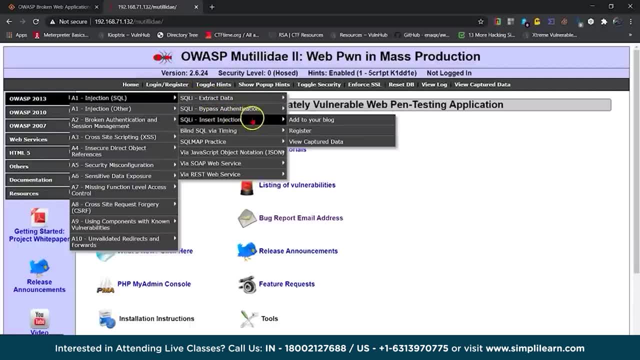 or SQL injection for bypass authentication or insert your injection attacks, blind SQL injection. and then there is a tool called SQL map which is available freely on your Linux machines- Kali Linux or Parrot Linux, whichever you want to use for your practice targets, and so on, so forth. so 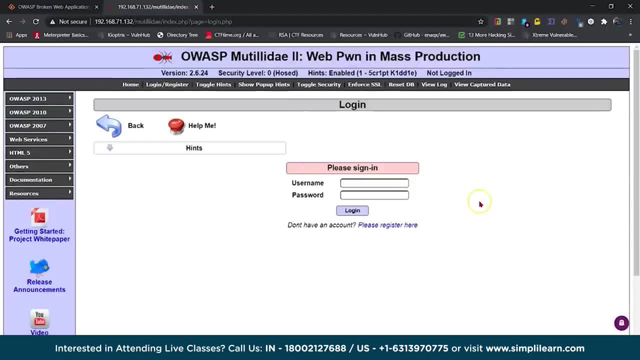 if I just take you here for bypass authentication- and this is a regular login page that an application may have, right, you look at a username, you look at password, you type that in and you log in. so let's say, I don't know a password here, I'm just going to type in a username, test password is passwd. 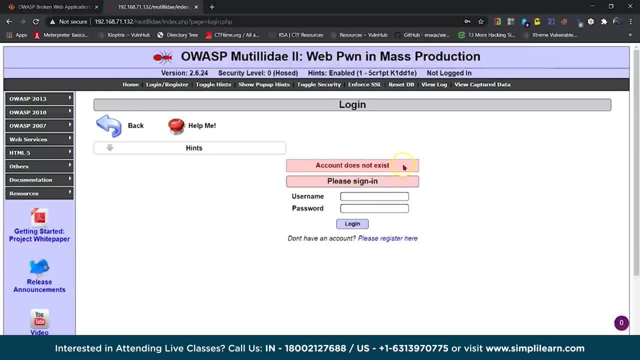 I'll try to log in and it shows me that the account does not exist, so the authentication mechanism does work. the I did try type in a username and password. it wasn't recognized, so the account does not exist. now let's try to type in a SQL query here. I'm going to just 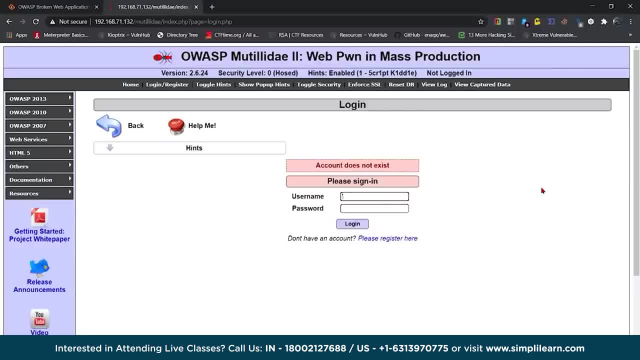 give it a single quote, which is an operator that is recognized by the SQL language which, when the database tries to execute, will cause the database to dump some data or to bypass authentication in this case, and I'm going to give it a condition: single quote or one equals one space, hyphen, hyphen. 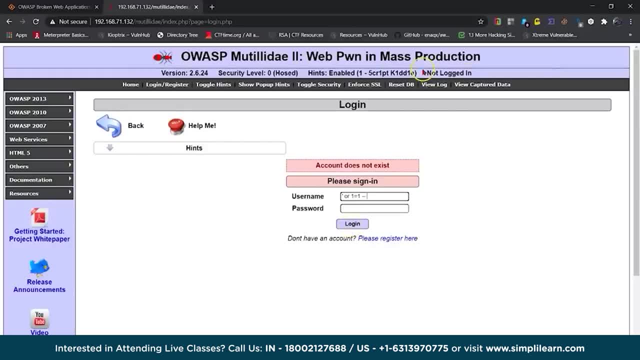 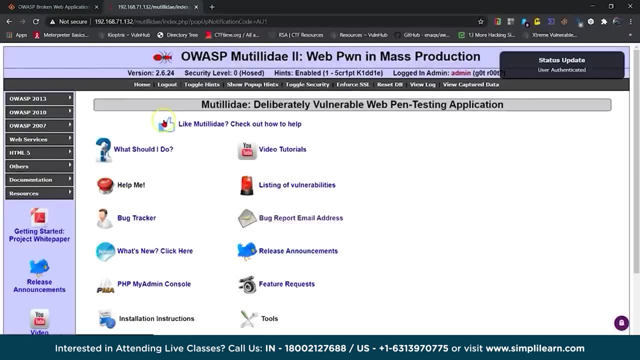 space and I'm going to click on login now. right now I'm not logged in at all and we tried our username and password and we weren't able to log in. so now if I log in, you will see that it gives me a status update saying the user has been authenticated and I'm logged in as admin got root. 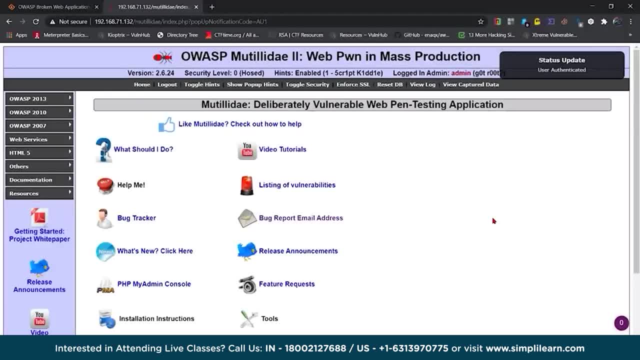 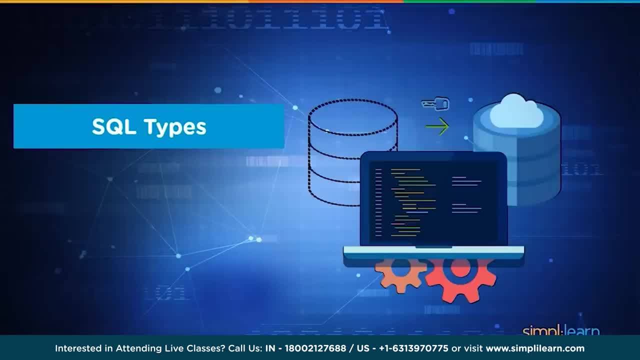 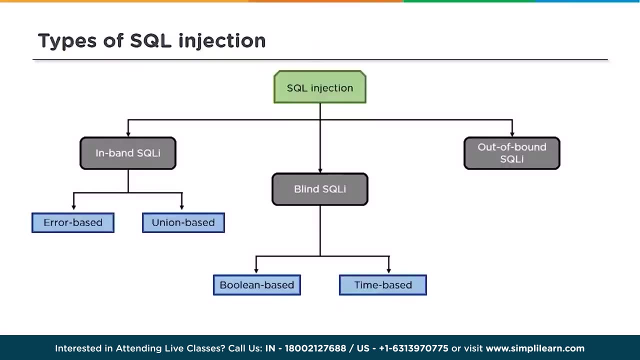 so that is what these SQL queries can achieve. I'm going to log out right now and we're going to look at the basics of SQL injection. so, looking at that small demo, looking now, let's look at what types of SQL injections are available. so the first is in-band SQL injection. 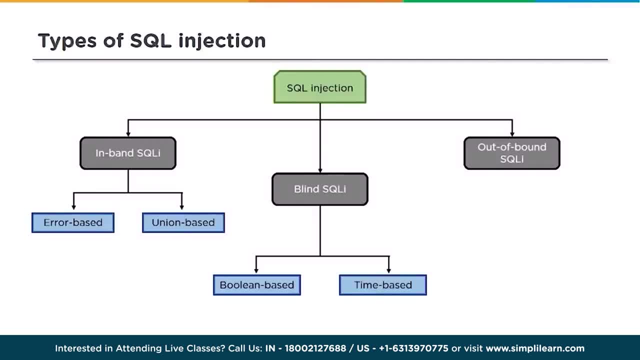 there are two subtypes within in-band: error based injection attack and a union based injection attack. the second type is blind SQL injection attack, where there's a boolean based and a time based attack, and the third one is out of bound SQL injection attack. now, what is in-band SQL injection? 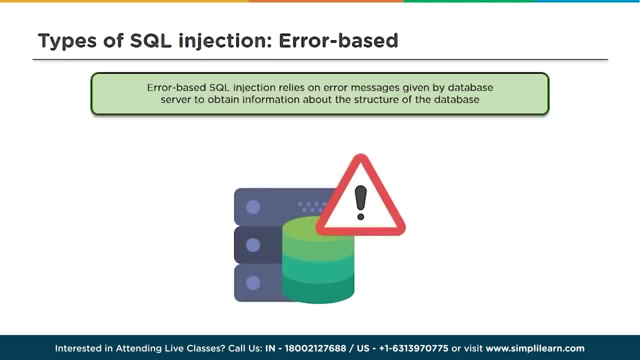 attack. in-band is where we are either attempting the error based or the union based. what is error based? we send a query to the database, we craft a query to the database and it generates an error message and it dumps the error message right in front of us on the screen. 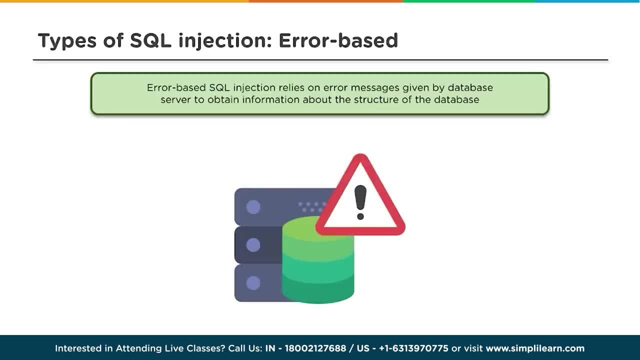 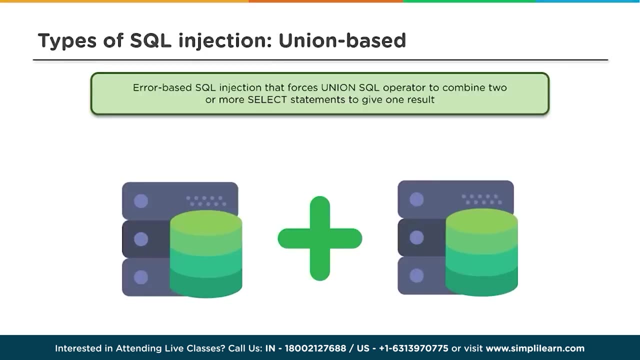 that makes us realize that there is a flaw, and there is some information that is dumped on the screen which we can then further utilize to craft our further queries as we go ahead. whereas union based is the, it is where we combine multiple statements at the same time. so if you look at 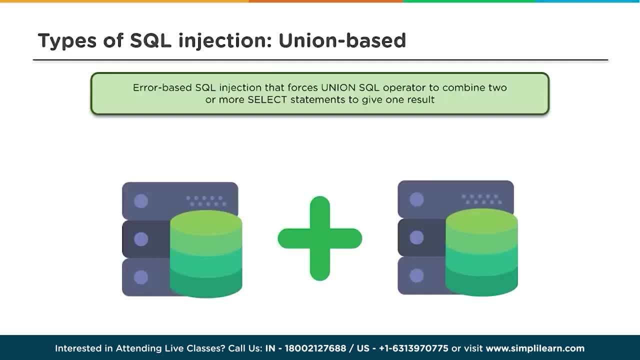 the URL. earlier in the URL you would see a large structure. in that URL. we can try to add more, two or more statements within the URL itself, to combine them and then confuse the database into executing both the statements together and giving a data dump at the same time. right, so what would a error based SQL injection look like? if I go back to the same, 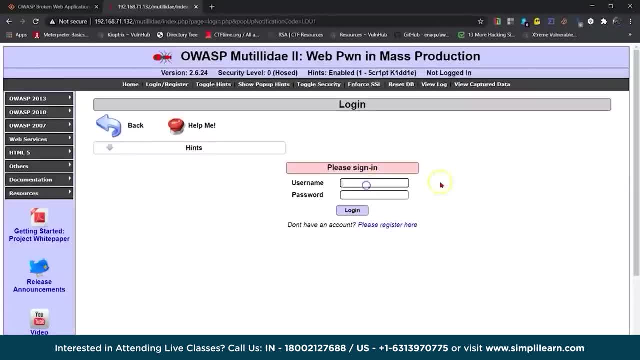 database, which is here right, and if you remember the username, we gave it a single quote, or one equals one space, hyphen, hyphen, space. we gave it the condition right. so basically what it did was a single quote is an operator that goes to the database, selects the default table in the user tables in this. 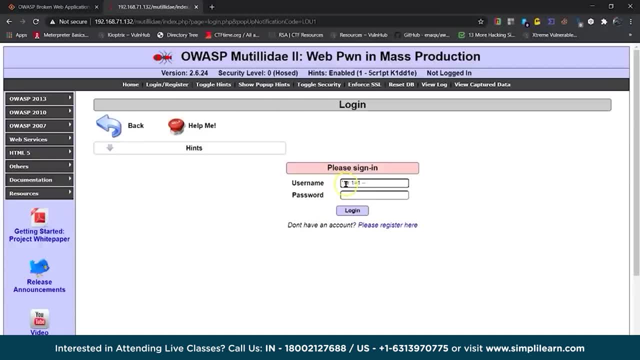 database column and then compares it to the condition that is given. so the condition that we gave was one equals one, which is always true. so what it did was it selected the default user table that was available in the database and, instead of comparing it to a password, it compared it to the condition. so if I give it one equals two, where the condition 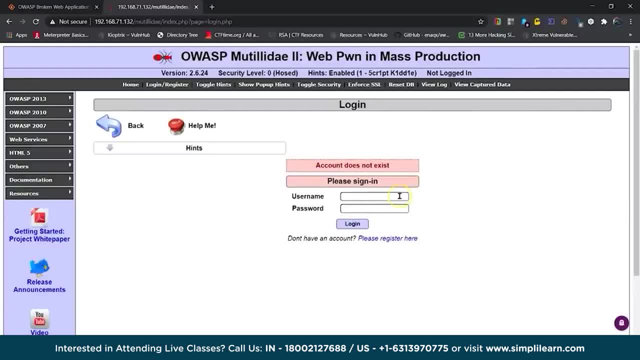 is false and if I log in, you will see that the account doesn't exist- comes back again because the condition was false and instead of comparing the user account to the password, it basically compared the user account to the condition. so if I give it a single quote- or one equals one- 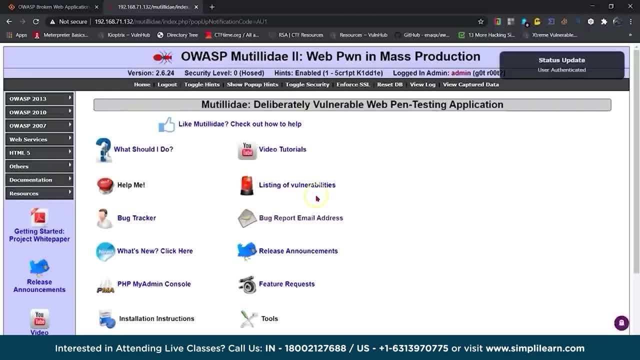 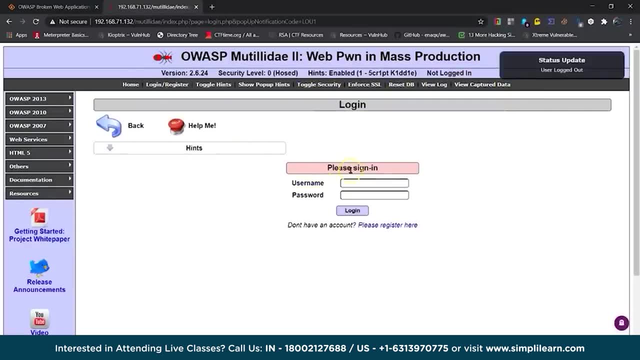 hyphen, hyphen space and log in. you can see that this is a correct condition and thus we are able to log in now. before we even go to that extent, if I just forget the condition over here and I just give it a single quote: the operator and I send this operator to the database. 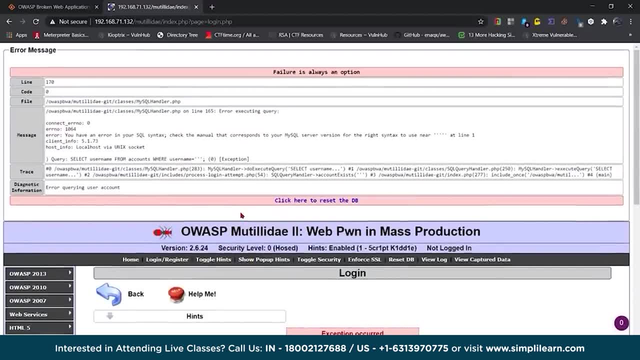 and I click on login, you will see that it generates an error, which is right on top, and it tells us the line, the file where the error happened- and you can see it happened in the mysql handlerphp file, right. and then it gives us the message: you have an error in your sql syntax. 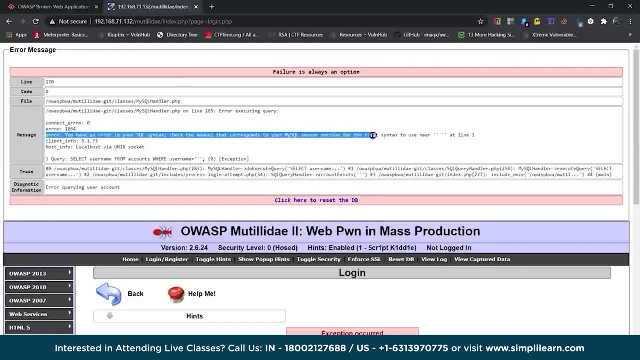 check the manual that corresponds to your code mysql server version for the right syntax to use. now why would a hacker want to do this in the first place? because there are different types of databases. so there is a mysql, msql or microsoft sql, oracle, sql, ibm, db2. all of these are variations of the sql database. uh, they use the sql language. 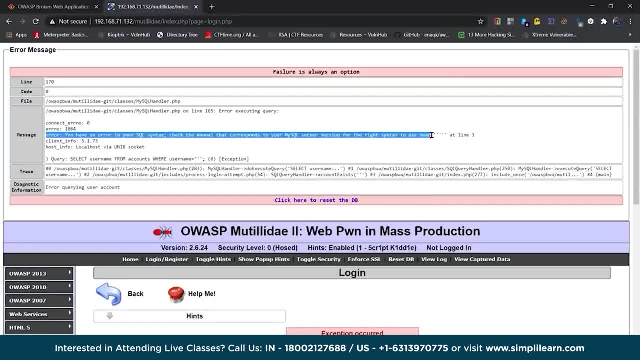 however, every database has its own command right there. they have their own syntax, they have their own uh, specific commands that are utilized for the sql server, and they use the sql language for the database. so in this scenario, the hacker wants to identify what database is being currently utilized so they can craft those particular queries. so now, with this injection, 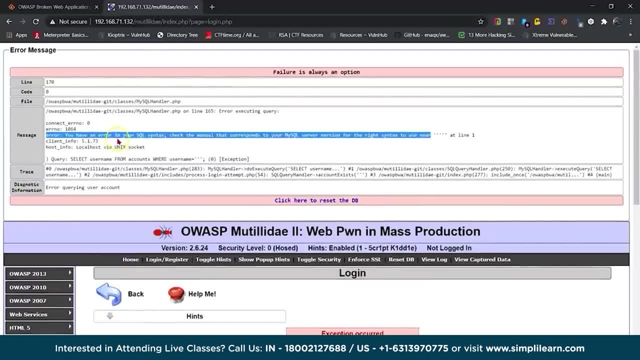 with just me sending the quote and the error getting generated. I now come to know that we are using a mysql server and the version of that server is 5.1.73, and the rest of the information about where the handlers are located, and so on, so forth. 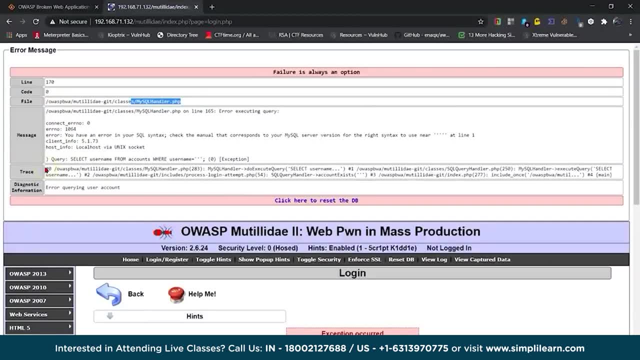 right. this gives the information to the hacker of how they want to proceed next, what kind of queries they want to create, what kind of syntax they want to utilize. so error based attack is where you generate these kind of errors, uh, and you get this information. the union base is where you craft. 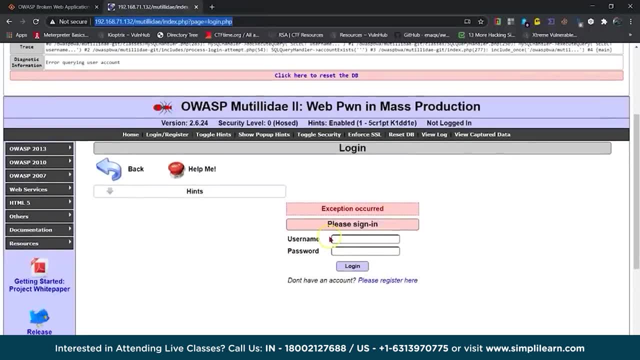 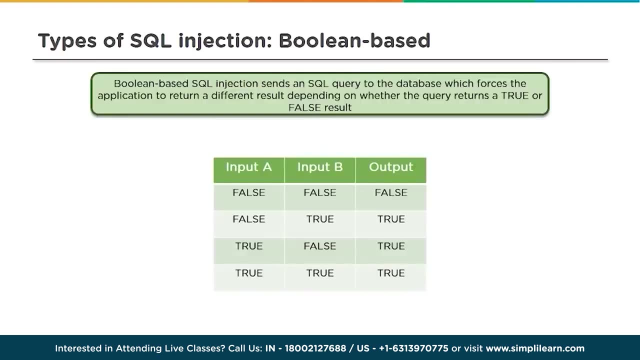 your queries within the url uh. you can try to combine multiple statements within the input fields and try to generate a response from that. then we come to boolean based sql injection. uh sends a sql query to the database which forces the application to return a different result depending on whether the query returns a true or a false result. so basically, if the input is false, 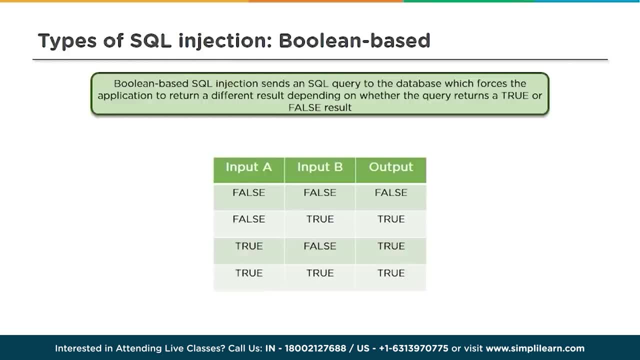 the input. both the inputs are false, the output would be false. uh, there's one input that is false, the other input that is true, input b, the output would be true, and so on, so forth. right, so depending on the result from the inputs, the attacker will come to know which input is true. 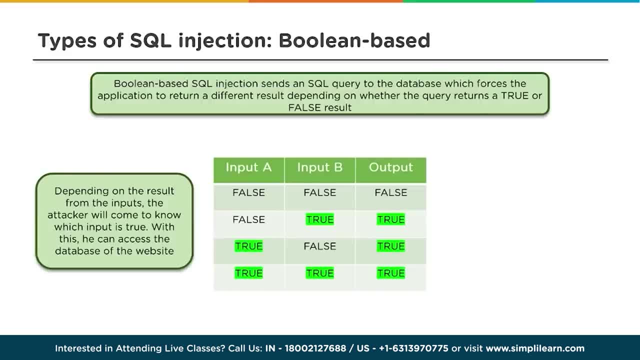 with this, he can then access the database of the website. so you are trying to figure out by sending out multiple inputs and then analyzing the output to see what exactly, which command exactly worked. what was the resultant output of that command? thus, from this kind of an information the hacker can infer their next step forward. then you have 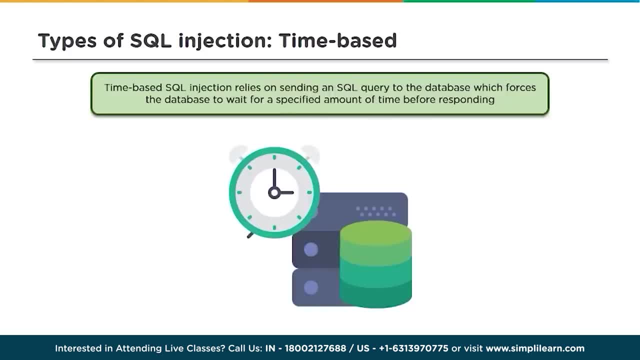 time-based sql injections. uh, now there are times when a database administrator or an application administrator has done some security configuration and thus have disabled verbose error messages. now, what is a verbose error message? the error message that we saw right here is a verbose error message. that means that the message gives out details. 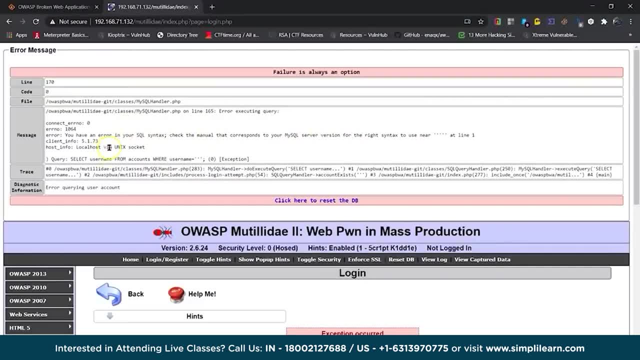 the message gives out details about what the database is, the version and whatnot. so if they have sanitized these errors and you no longer can generate these errors and thus you cannot figure out what database is, then what do you do right, for example, if i just take you to simply learn? 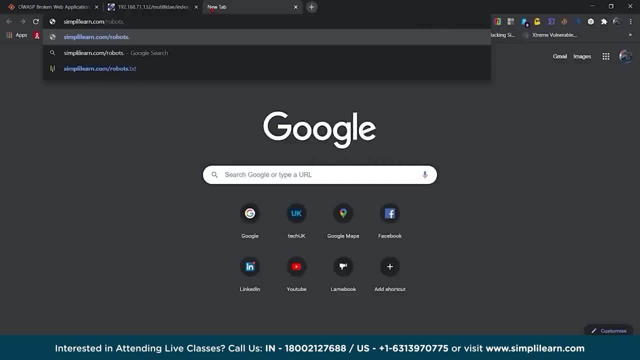 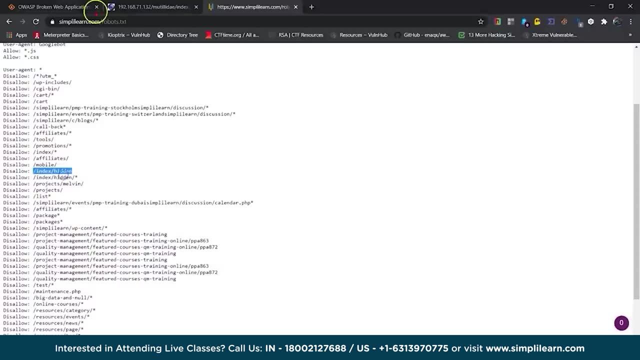 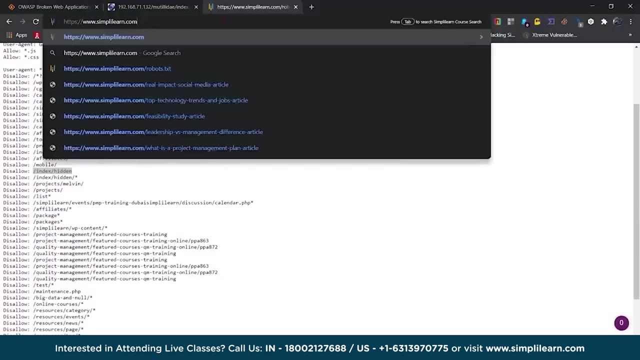 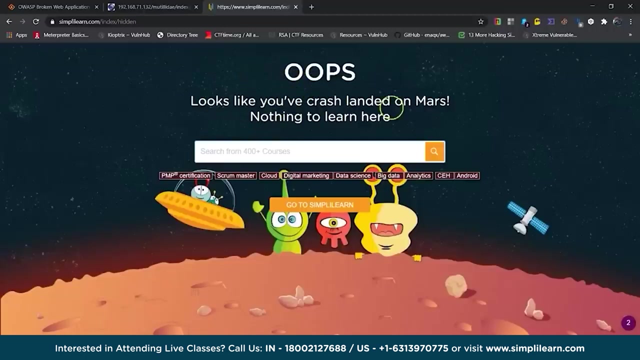 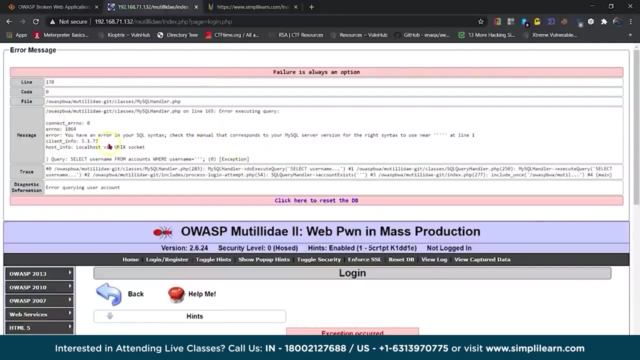 and take you to a url that is supposedly not accessible. you can see that that gives a generic error. oops, like it looks like you have crash landed on march. it doesn't give you a verbose error that we saw here. so this gives us a detail error of what went wrong, where it gives us the 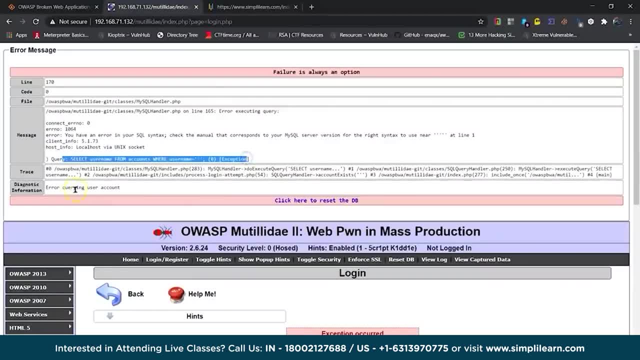 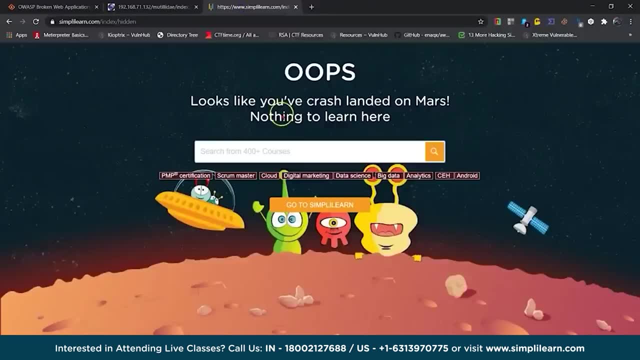 database, the version of the database and where the query went wrong, and etc. etc. etc. whereas on this site, where there's some, there's a lot of security that goes in here so you can see that it doesn't generate a error. you just get a generic page in front of you. so in that case, what does a 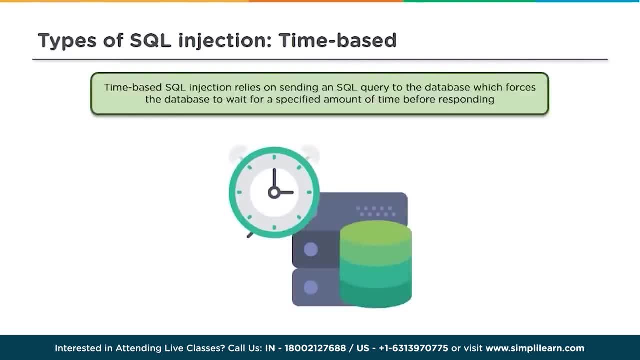 hacker do so. the hacker then injects a time-based query in the url which allows us to verify whether the command is being executed or not. so we put in a time weight, let's say 10 seconds of time weight. so if we the moment we inject the query, if the query times for 10 seconds and then gets, 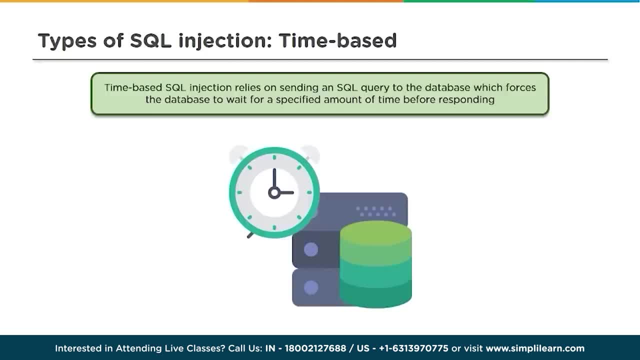 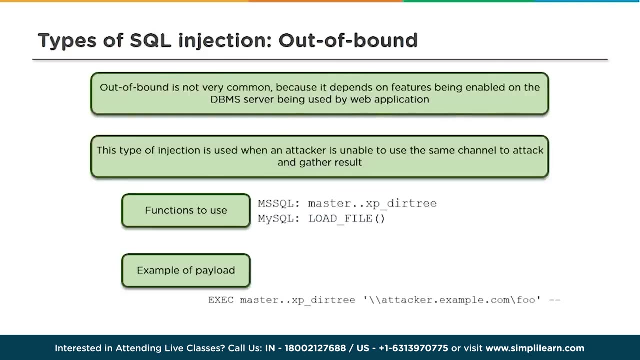 executed, that means that the sql injection is possible. however, if we inject the query and it just gets executed without the delay, that means that the time injection attack would not be possible on that particular site. out of bound is not a very common attack. it depends on the 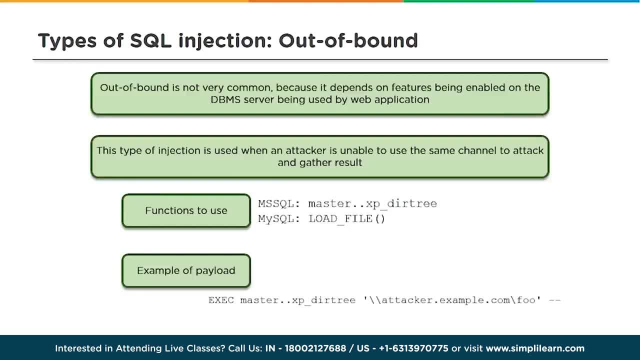 features being enabled on the database management system that is being used by the web application. so this can be a somewhat of a misconfiguration error by the database administrator where you have enabled functions and not sanitized them. so you have not done in access controls properly. you have given account control, so queries should never be executed at an administrative level. 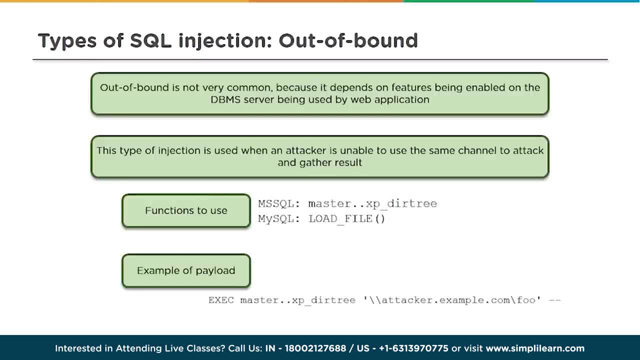 they should always be executed at a user level with minimum privileges that are required for that query to be executed. now, if you're allowing these kind of functions to be- uh, to be enabled at the dbms and there is an administrative account that can have access to them at that, 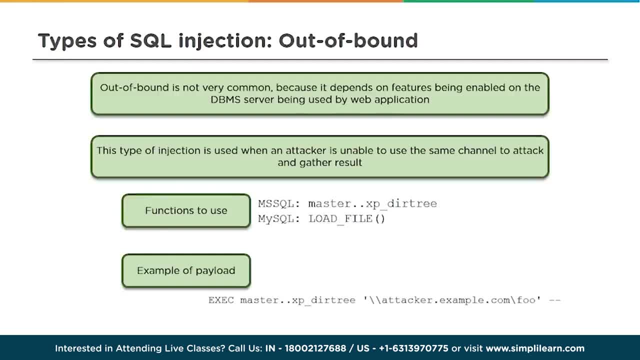 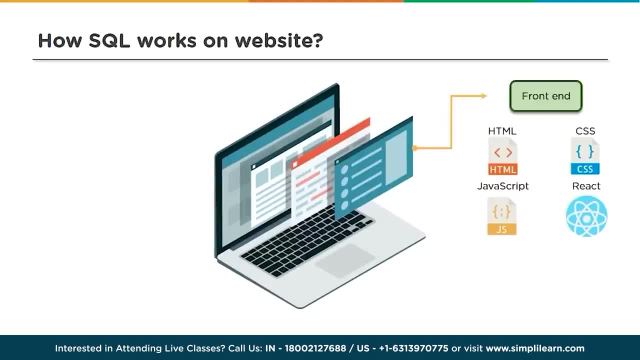 point in time, an out of bound injection attack is possible. so let's look at how our website works, right, uh, how sql works on a website. now. the website is constructed of html, hypertext markup language, which would include javascripting for functionality, cascading style sheets for the mapping of the website, right, and then react, js and whatnot for further functionality. 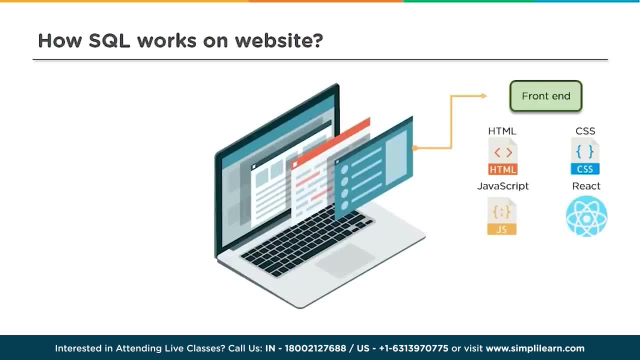 now, when we send a query to the website, it is normally using the http protocol or https protocol. when the query reaches the application, the application would then go ahead and generate the secret sql query. uh, at the client side, you'll have uh, all these scripting languages coming in. uh on the 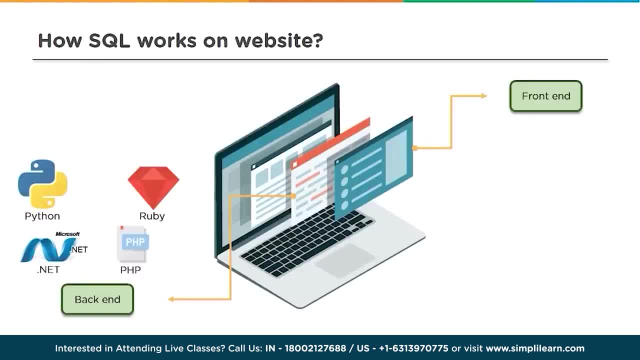 front end uh that we can utilize to craft queries and then send them across. at the server side you will have uh databases like oracle, mysql, msql and so on, so forth that will then execute those queries, right. so just to give you an example, if i use a tool called postman- what we generally do- 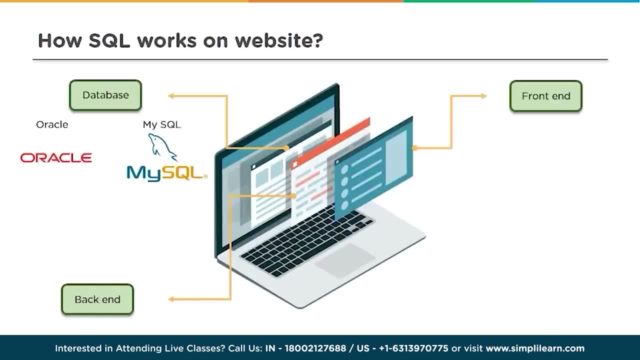 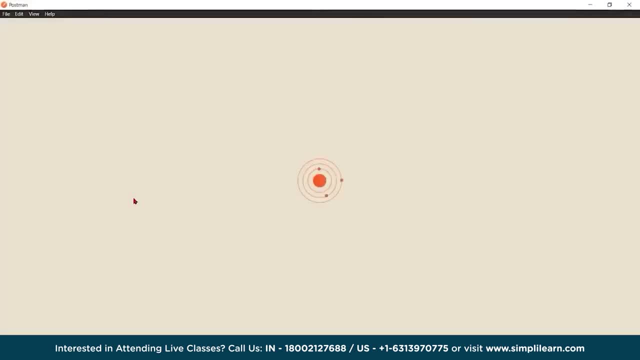 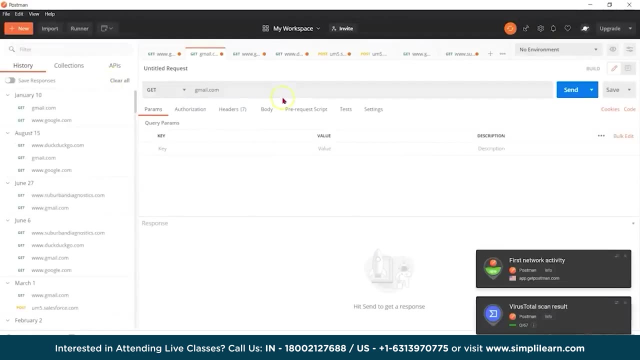 uh, when we craft a query is we send out a get request to the website and then we receive a response from the site with the html code and everything. so this is a tool that is utilized by software testers to test the responses that you're going to get from various websites. so 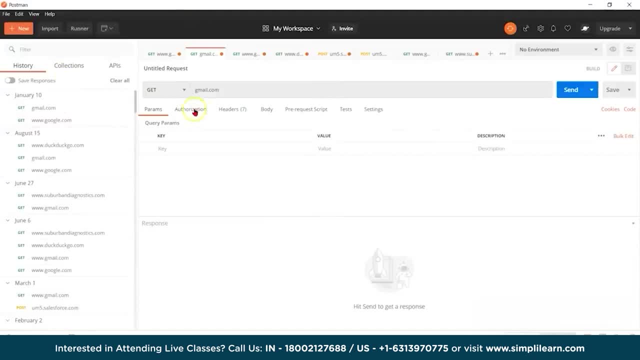 yes, on the left hand side you can see i've used it on quite a bit. here we have an example for gmailcom, so let's continue with that. so this is a get request being sent to gmail. the moment i send it, it's going to create an http request and send it across. the response that i get is this: this is: 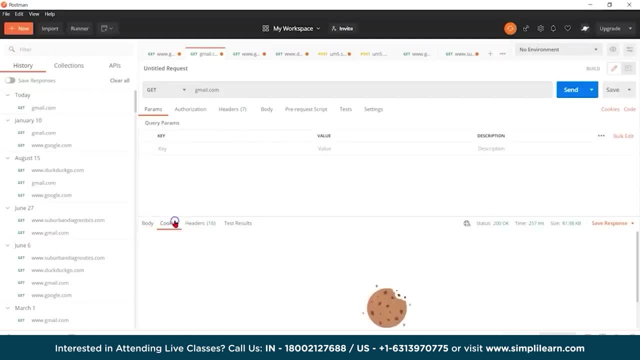 the html code for gmailcom: right, these are the cookies: uh, these are the headers: uh, that include information. so you can see, this is a text html, character set utilized is utf-8 and the configuration: uh, that has been done with the application, right? so this is where, uh, everything. 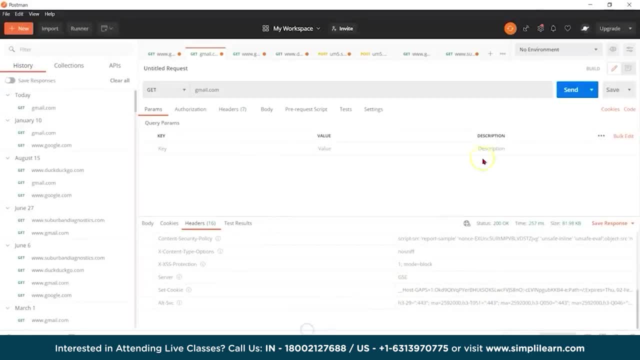 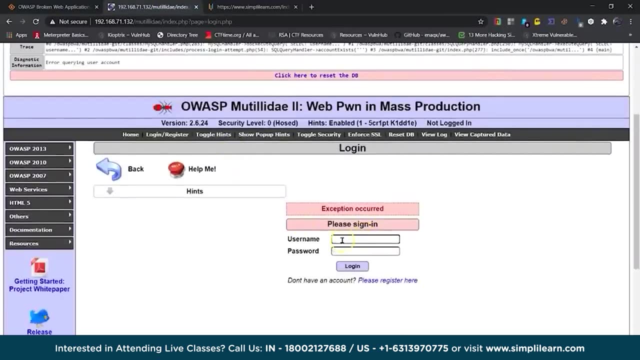 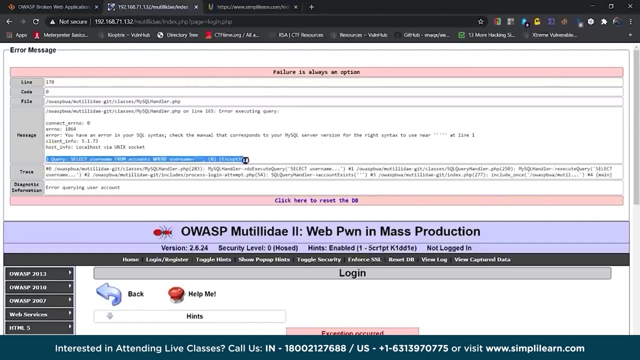 comes in. this is the cookie that has been sent with that particular uh request that i had sent out. now, if you analyze this query right, so, when we went on to this application and i typed in that single quote and we generated this error, right, uh, you can see that the application converted this. 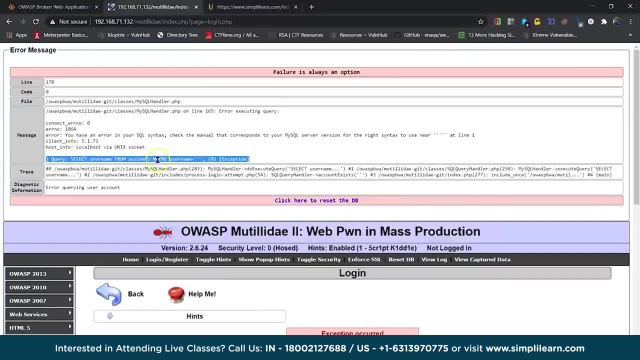 into a sql query. so the query was select username from accounts where the username in quotes single quotes, and we use this quote right, the single quote right there. so, uh, that's where we use that operator and that's where the exception error occurred. so these are the kind of queries that are structured by the application. 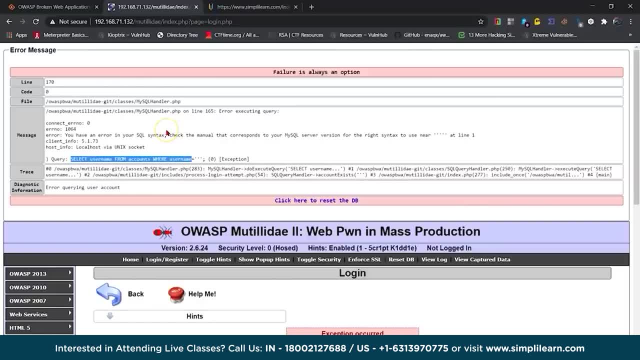 and then taken on to the database for execution. when we type in: uh, it is a http get request with the username and password within that query, that is sent to the application, the application converts it into a sql query, sends it to the database and the database responds. 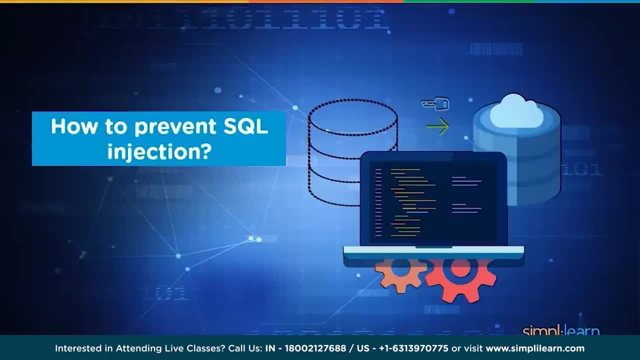 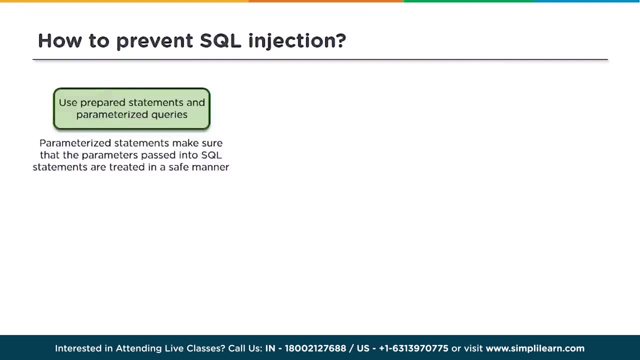 with the appropriate response. so how do we prevent sql injection in the first place? use prepared statement and parameterized queries. these statements make sure that the parameters passed into sql statements are treated in a safe manner. so, for example, we saw that the single code was an operator. this shouldn't be allowed to be. 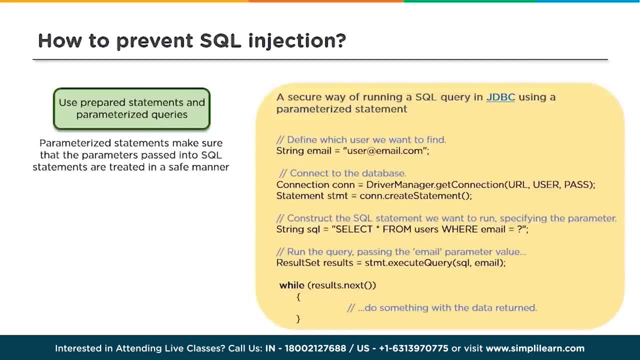 utilized in the first place, right, so here? what we are doing here is a secure way of running a sql query in the jdbs using a parameterized statement. define which user we want to find. so there's a string. the email comes in connection to the database we are going to: cloud server. 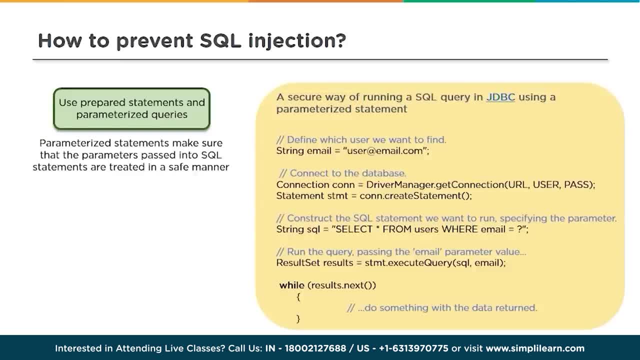 Figure out how the connection is going to be passed, how it is going to be created, Construct the SQL statement we want to run, specifying the parameter right. So we define how is it going to be created, what is going to be created, what can be passed. 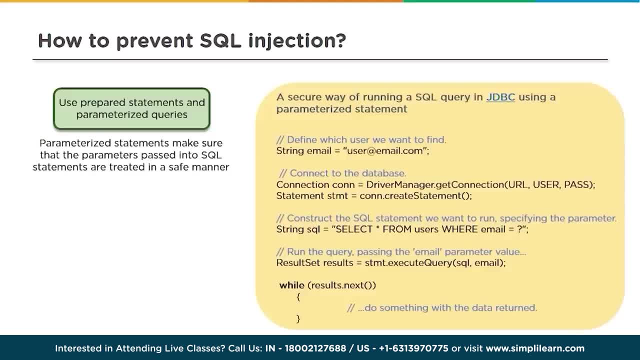 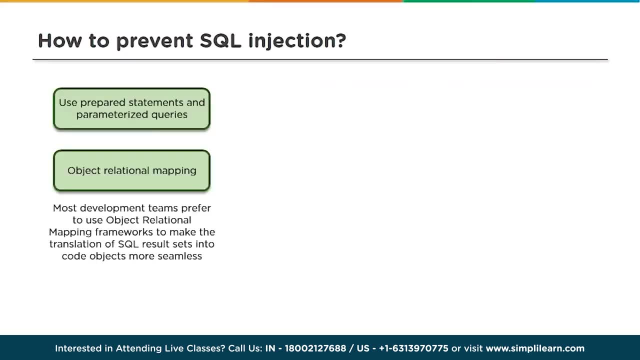 to the database and what should not be passed to the database. So that is one way of utilizing prepared statements and parameterized queries. Then we have object relational mapping. Most development teams prefer to use object relational mapping frameworks to evade the translation of SQL results set into code objects more seamless. 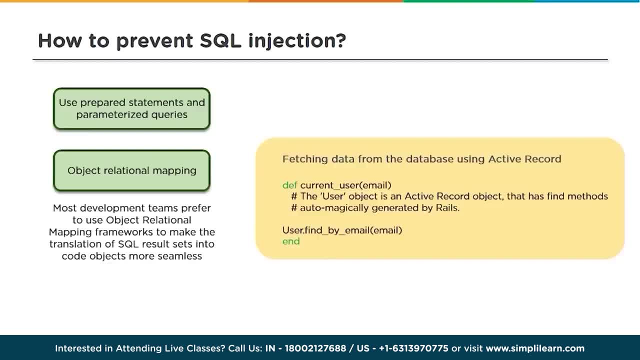 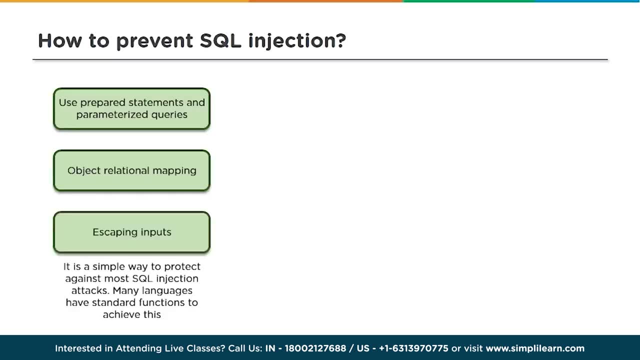 So this is an example of object relational mapping, where we map certain objects and allow that to be executed, And then escaping inputs. It is a simple way to protect against most SQL injection attacks. Many languages have standard functions to achieve this right, So you need to be very careful. 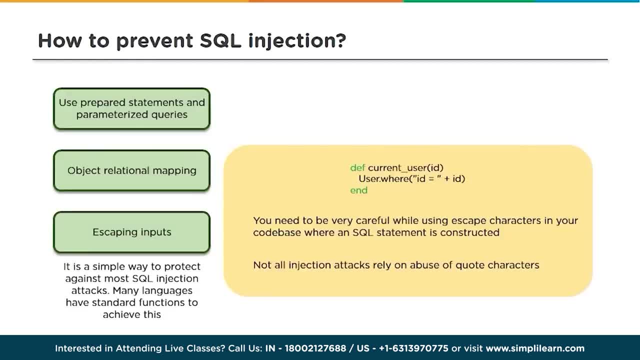 Using escape characters in your code base when a SQL statement is constructed. not all injection attacks rely on abuse of code characters, So you need to know what characters are being utilized in the configuration that you have created, in the structure that you have created, in the code that you have created, which characters. 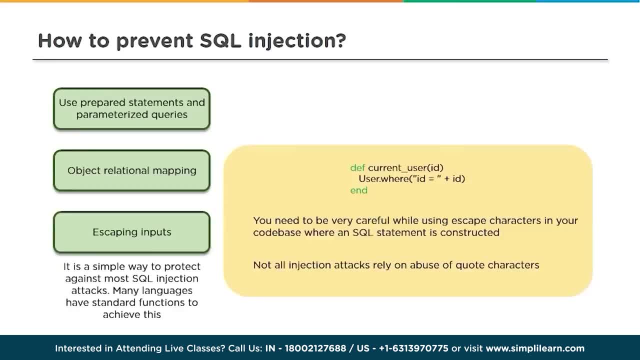 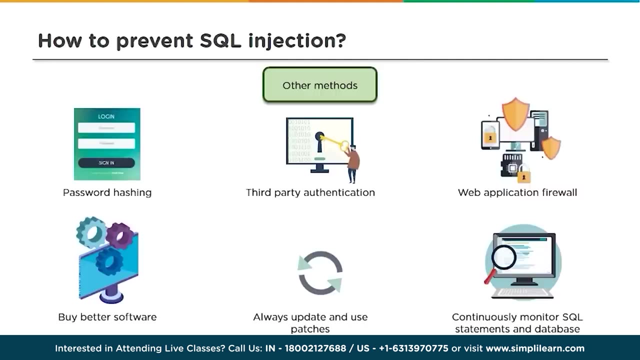 are being recognized as operators. You need to sanitize those operators and you need to basically ensure that these operators cannot be accepted as user input. If they are, they are peered out by the application and they never reach the database. Other methods of preventing SQL injection are password hashing, so that passwords cannot be 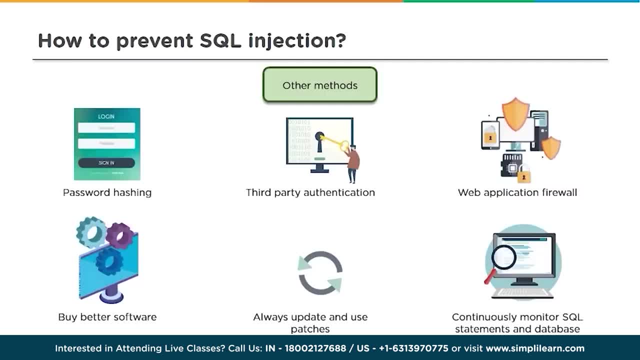 bypassed. The passwords cannot be recovered. Passwords cannot be cracked. Third party authentication: You use OAuth or some other service for a single sign on mechanism. Thus, you rely on a third party to maintain the security of authentication. And what? 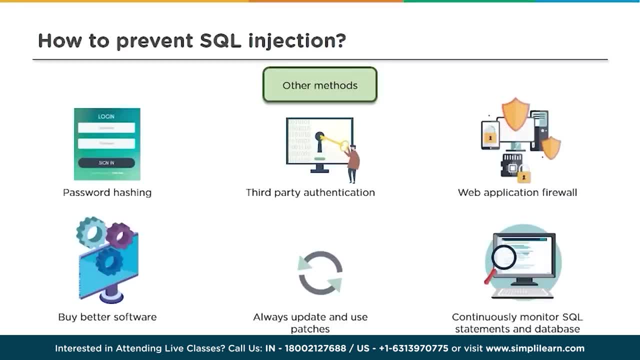 What kind of parameters are passed? For example, using LinkedIn logins or Facebook logins? right, For the layman: you normally go on to Facebook and you allow if you're using a game. right, If you start playing a game, you're allowed to log into the game using your Facebook credentials. 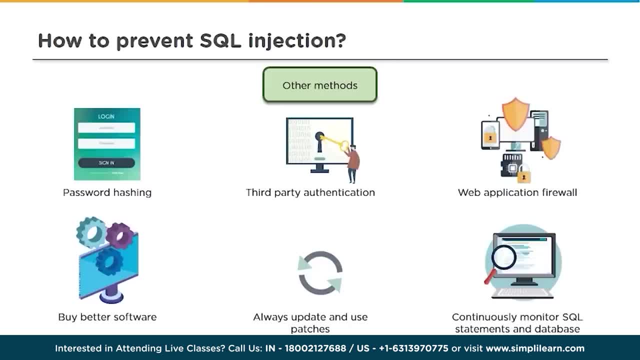 or your Google credentials. Now, that is not just for ease of use, but the game user, the developer, has outsourced the authentication mechanisms to third parties such as Facebook or Google, Because they understand that that authentication mechanism is as safe as can be. 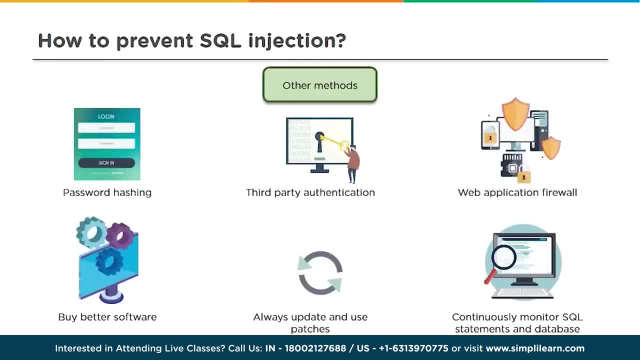 Facebook and Google are wealthy organizations, hire a lot of security experts, and the development for their authentication mechanisms is top notch. Small organization cannot spend that kind of money on security itself, right? So you use a third party authentication mechanism to ensure that these kind of attacks may not. 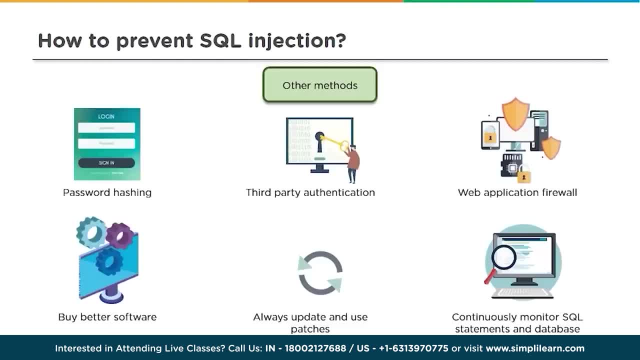 happen, Then web application firewalls. Having a web application firewall and configuring it- And configuring it properly- for SQL injection attacks is one of the sure shot method of mitigating or minimizing the threat in the first place. So at this point in time, you have realized that the application has some vulnerabilities. 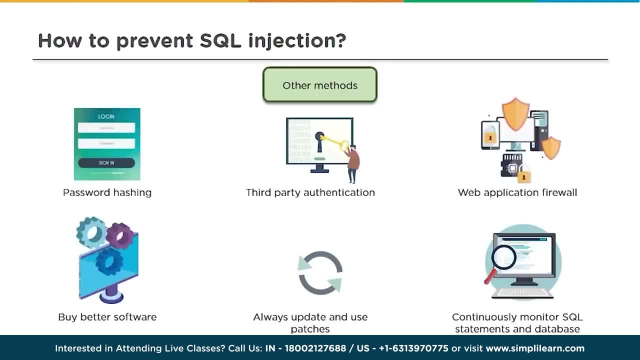 for SQL injection and instead of recoding or restructuring the application, you want to take the easier way out or the cheaper way out. So what you do is you install a web application firewall and you configure the web application firewall to identify malicious queries. 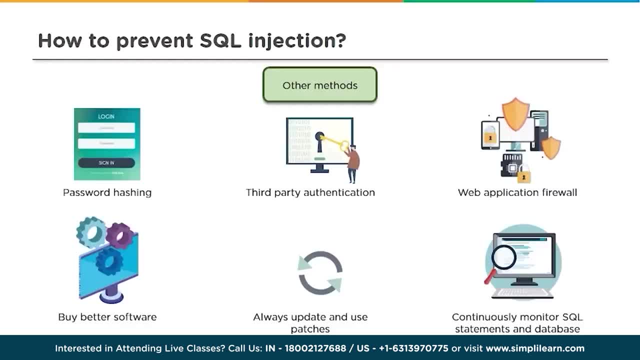 And stop them at the firewall level itself, So they never reach the application and thus the vulnerabilities on the application don't get executed. Buy better software and keep on updating the software. So it's not necessary that once you have a software you install it. it's going to be. 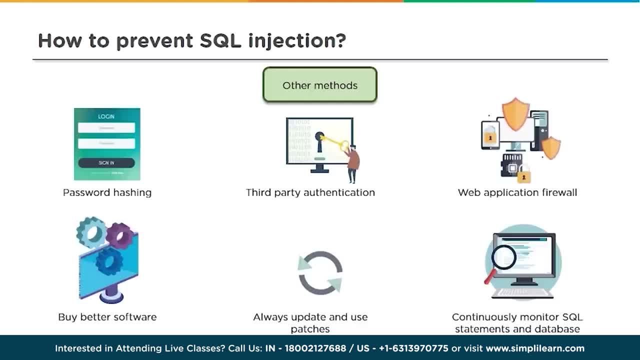 safe for life. New vulnerabilities are discovered every day, every hour, and it may so happen. what is secure today may be completely insecure tomorrow or the day after, Right? So you need to keep on upgrading the software. If there are no upgrades available and the vulnerability still exists, you might want. 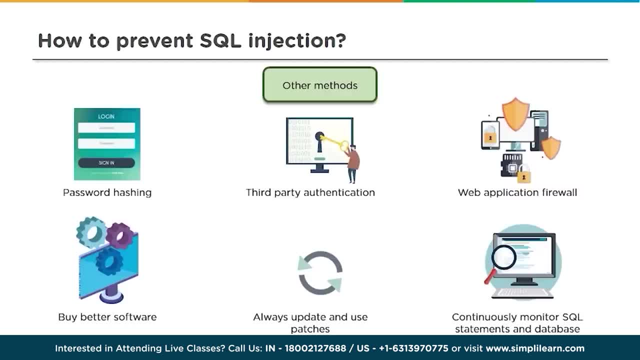 to migrate to a better software and thus ensure that you don't get hacked Right. Always update and use patches. Organizations keep on sending out updates and patches as and when they are released. You need to install them to enhance your security portions And then continuously monitor SQL statements and databases. 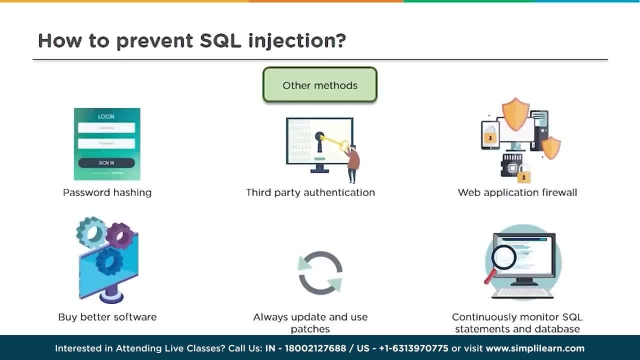 Use protocol monitors, Use different softwares, Use the firewalls To keep on monitoring what kind of queries you are getting and, based on those queries, you want to ensure the inputs and the queries that are creating are not detrimental to the health of the software that you have. 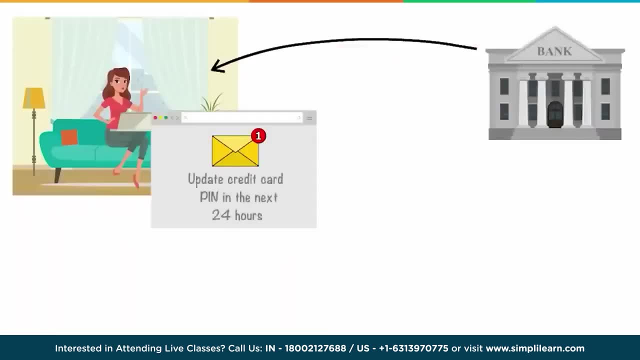 Jane is relaxing at home when she receives an email from a bank that asks her to update her credit card PIN in the next 24 hours as a security measure. Judging the severity of the message, Jane follows the link provided in the email On delivering her current credit card PIN. she will receive a message from the bank. 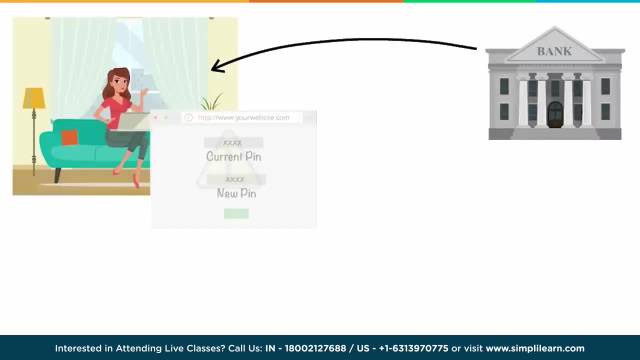 The bank will send her a message that it changed the credit card PIN and the supposedly updated one. The website became unresponsive, which prompted her to try sometime later. However, after a couple of hours she noticed a significant purchase from a random website. 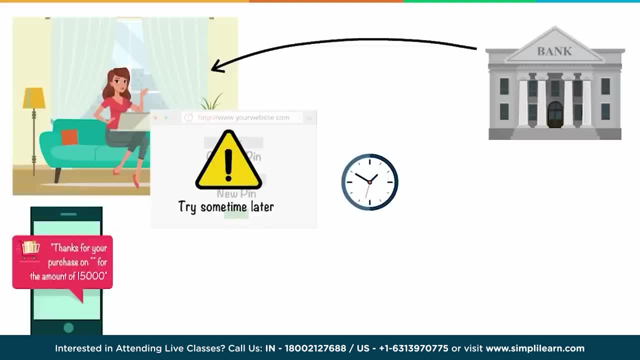 on that same credit card, which she never authorized. Frantically contacting the bank, Jane realized the original email was a counterfeit or a fake message with the malicious link that entailed credit card fraud. This is a classic example of a phishing attack. How to detect a phishing attack. 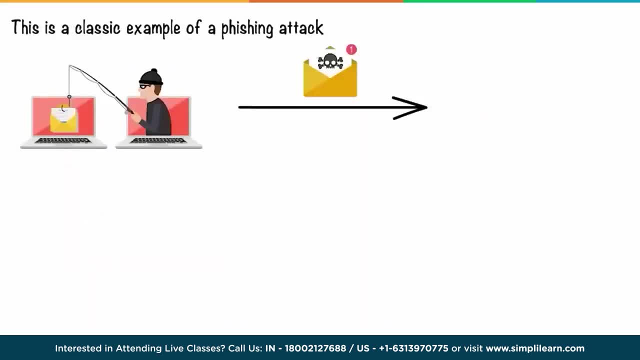 Bait attacks are a type of social engineering where a fraudulent message is sent to a target on the premise of arriving from a trusted source. Its basic purpose is to trick the victim into revealing sensitive information like passwords and payment information. It's based on the word phishing, which works on the concept of baits. 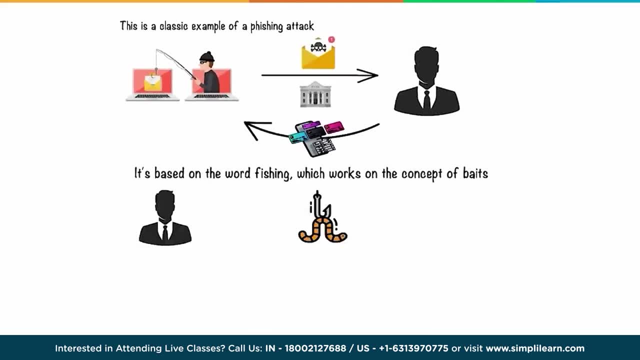 If a supposed victim catches the bait, the attack can go ahead, which, in our case, makes Jane the fish and the phishing emails the bait. If Jane never opened the malicious link or was cautious about the email authenticity, an attack of this nature would have been relatively ineffective. 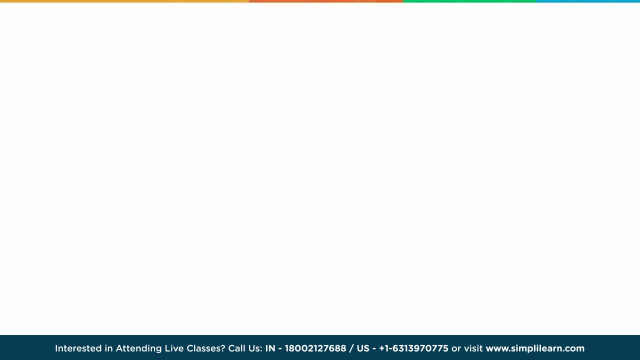 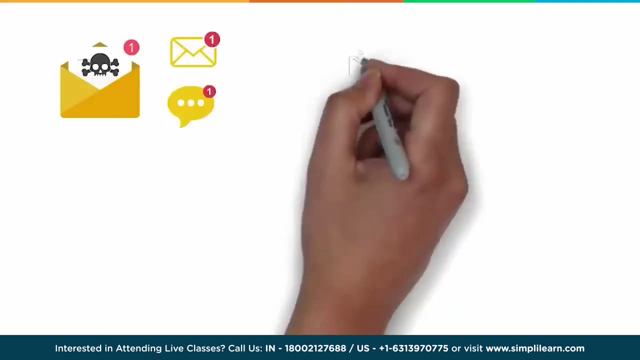 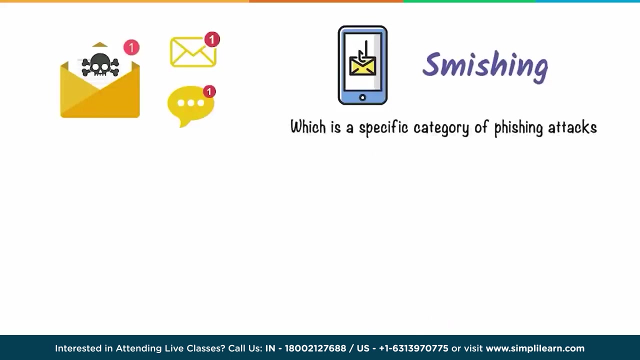 But how does the hacker gain access to these credentials? A phishing attack starts with a fraudulent message, which can be transmitted via email or chat applications, Even using SMS conversations. to impersonate legitimate sources is known as smishing, which is a specific category of phishing attacks. 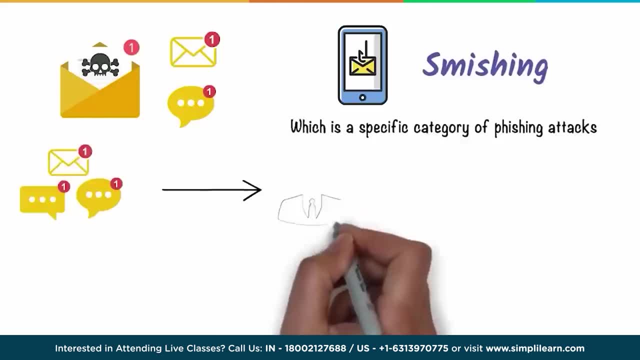 Irrespective of the manner of transmission, the message targets the victim in a way that coaxes them to open a malicious link and provide critical information on the requisite website. More often than not, the websites are designed to look as authentic as possible. 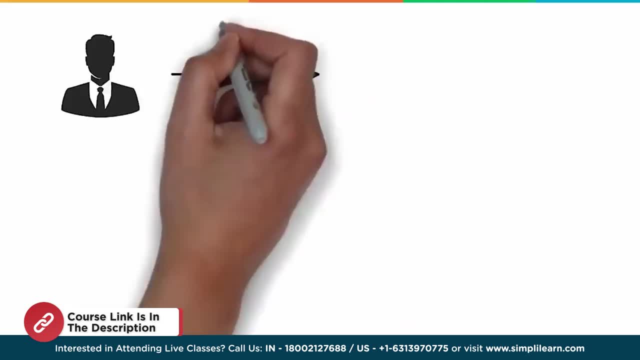 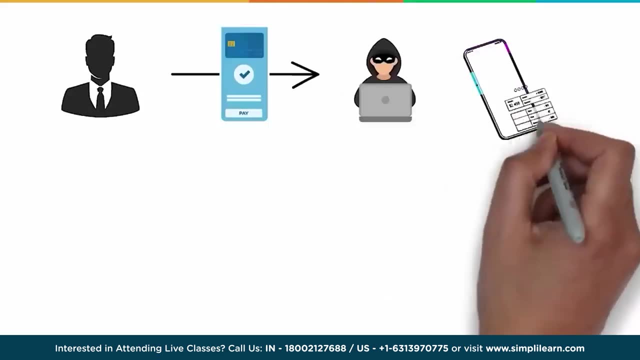 Once the victims submit information using the link, be it a password or credit card details, the data is sent to the hacker who designed the email and the fake website, giving him complete control over the account whose password was just provided, Often carried out in campaigns where an identical phishing mail is sent to thousands of users. the rate of success is relatively low, but never zero. Between 2013 and 2015,, corporate giants like Facebook and Google were tricked off of $100 million due to an extensive phishing campaign where a known common associate was impersonated by the hackers. 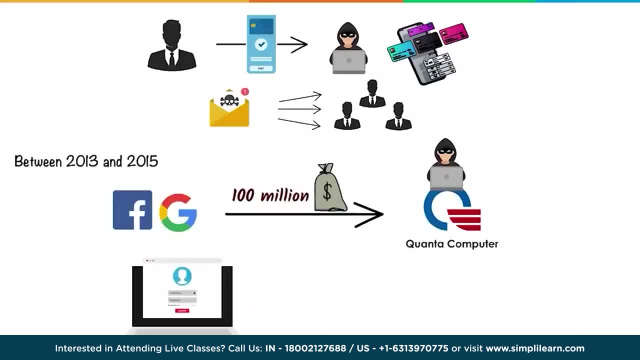 Apart from credit access, some of these campaigns target the victim device and install malware when clicked on the malicious links, Which can later function as a botnet or a target for ransomware attacks. There is no single formula, for there are multiple categories of phishing attacks. 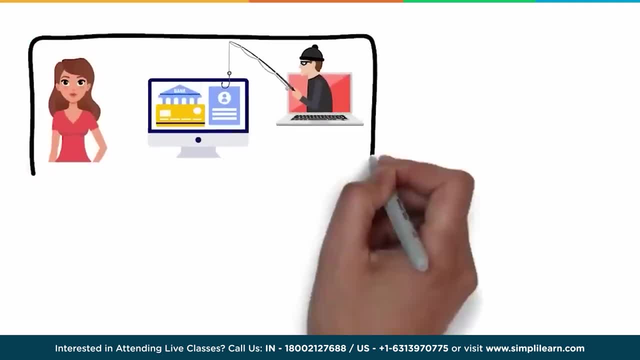 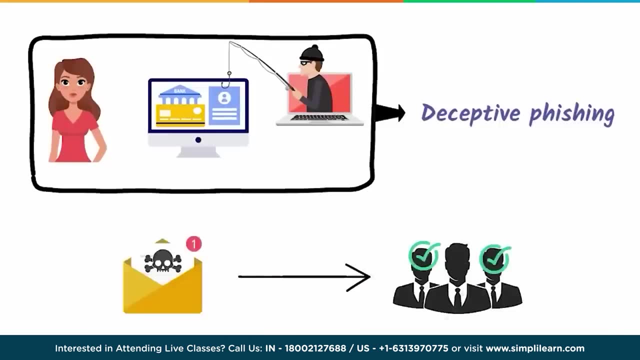 The issue with Jane, where the hacker stole her bank credentials, falls under the umbrella of deceptive phishing. A general email is sent out to thousands of users in this category, hoping some of them fall prey to this scam. Spear phishing, on the other hand, is a bit customized version. 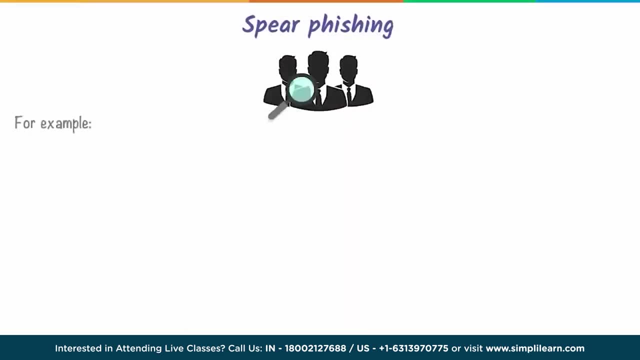 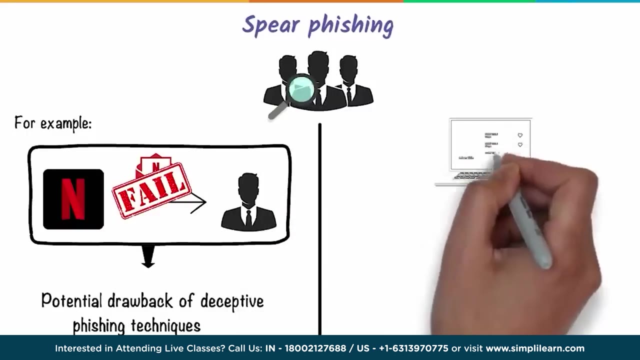 The targets are researched before being sent an email. For example, if you never had a Netflix subscription, sending you an email that seems like the Netflix team sends it becomes pointless. This is a potential drawback of deceptive phishing techniques. On the other hand, a simple screenshot of a Spotify playlist being shared on social media indicates a probable point of entry. 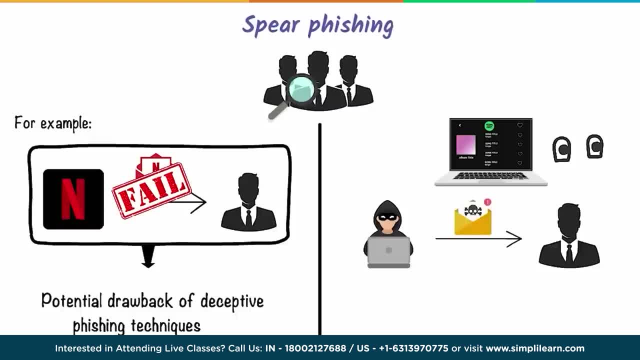 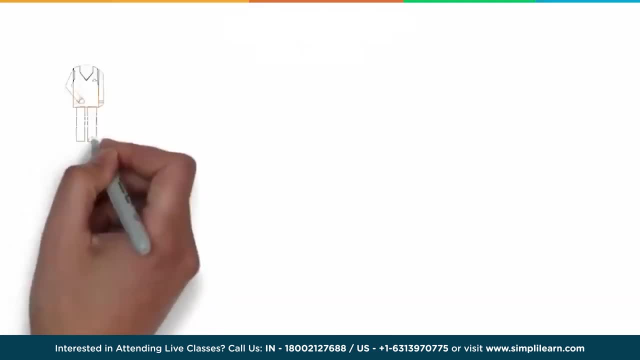 The hacker can send counterfeit messages to the target user while implying the source of such messages being Spotify, tricking them into sharing private information. Since the hacker already knows the target uses Spotify, the chances of victims taking the bait increase substantially. For more important targets, like CEOs and people with a fortune on their back, the research done is tenfold. 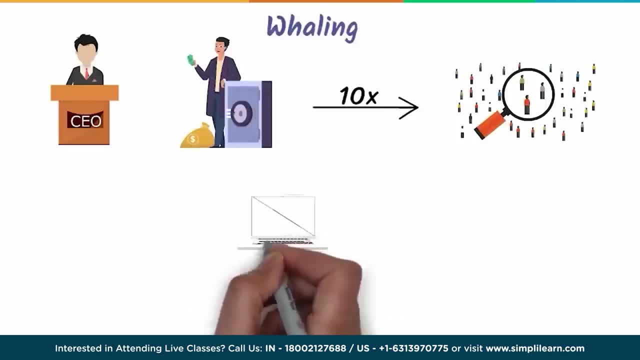 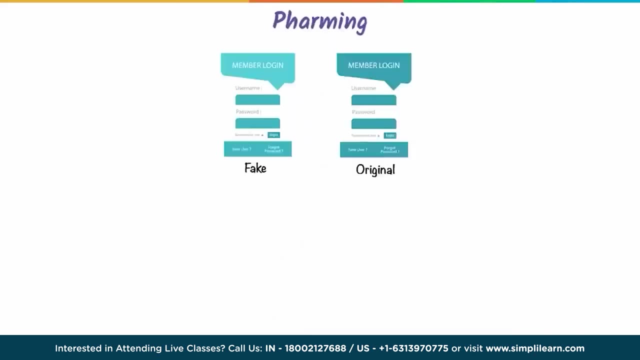 Which can be called a case of whaling. The hackers prepare and wait for the right moment to launch their phishing attack, often to steal industry secrets for rival companies or sell them off at a higher price. Apart from just emails, pharming focuses on fake websites that resemble their original counterparts as much as possible. 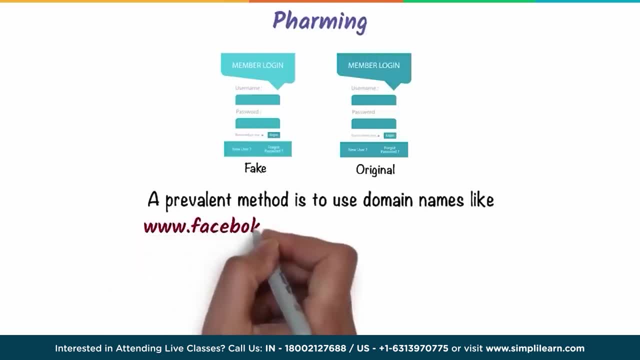 A prevalent method is to use domain names like Facebook with a single O or YouTube with no E. These are mistakes that people make when typing the full URL in the browser, leading them straight to a counterfeit webpage which can fool them into submitting private data. 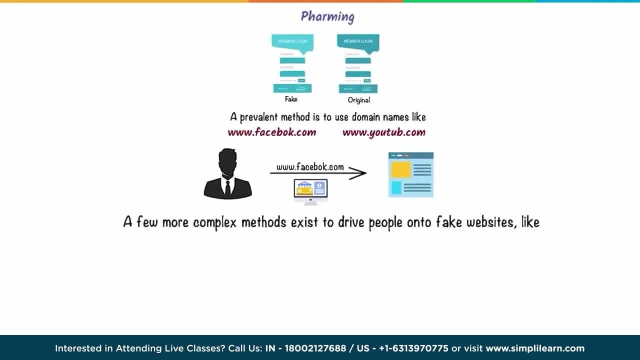 A few more complex methods exist to drive people onto fake websites, like ARP spoofing and DNS cache poisoning, but they are rarely carried out due to time and resource constraints. Now that we know how phishing attacks work, let's look at ways to prevent ourselves from becoming victims. 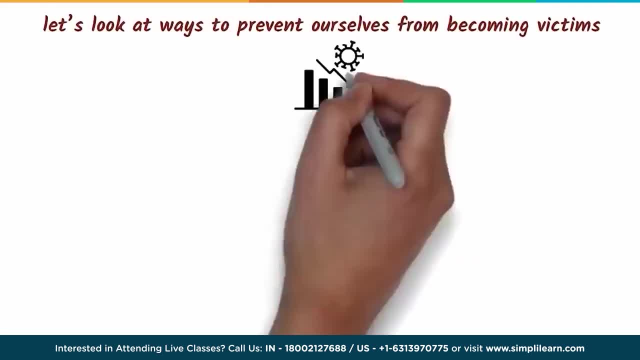 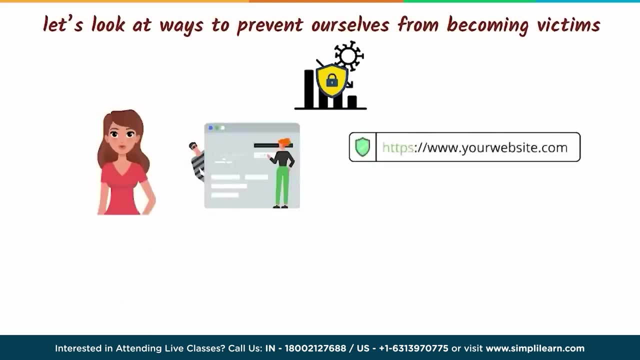 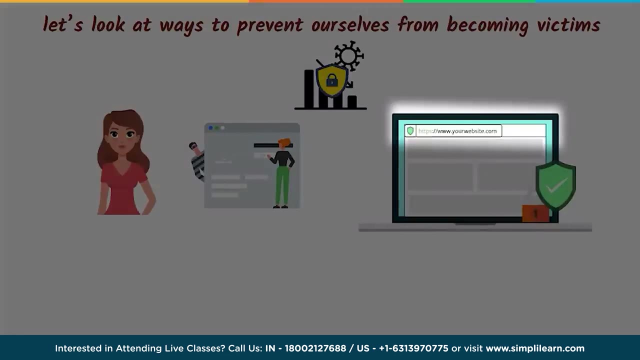 While the implications of a phishing attack can be extreme, protecting yourself against these is relatively straightforward. Jane could have saved herself from credit card fraud had she checked the link in the email for authenticity and that it redirected to a secure website that runs on the HTTPS protocol. 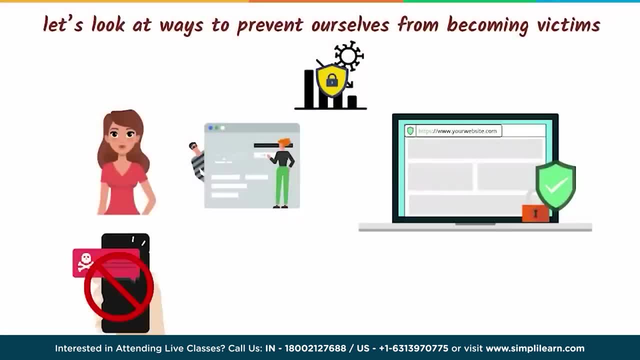 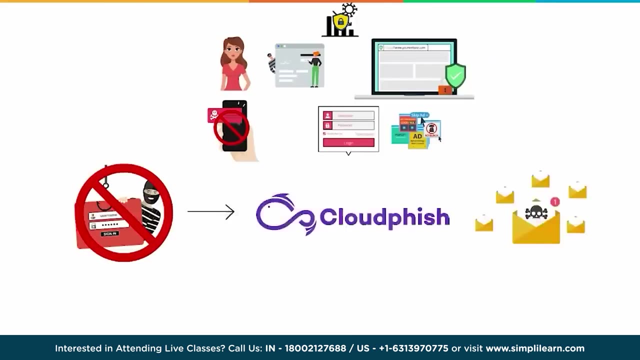 Even suspicious messages shouldn't be entertained. One must also refrain from entering private information on random websites or pop-up windows, irrespective of how legitimate they seem. It is also recommended to use secure anti-phishing browser extensions like Cloudfish to sniff out malicious emails from legitimate ones. 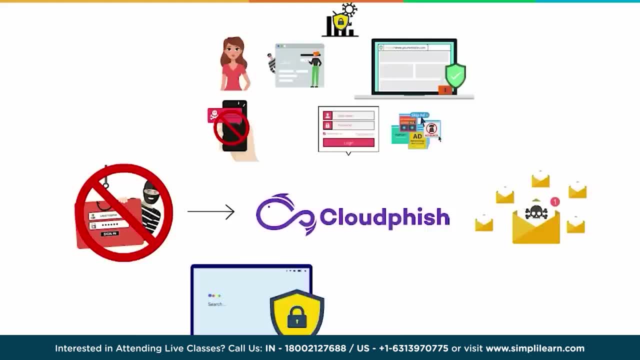 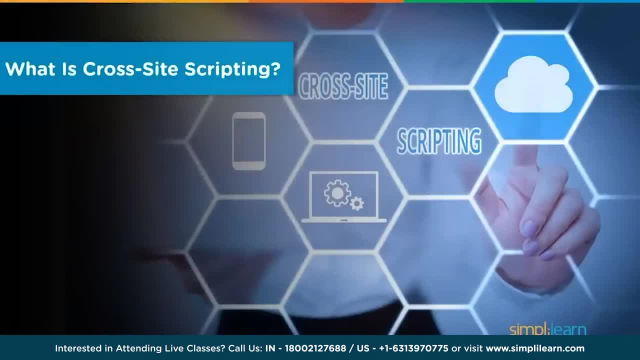 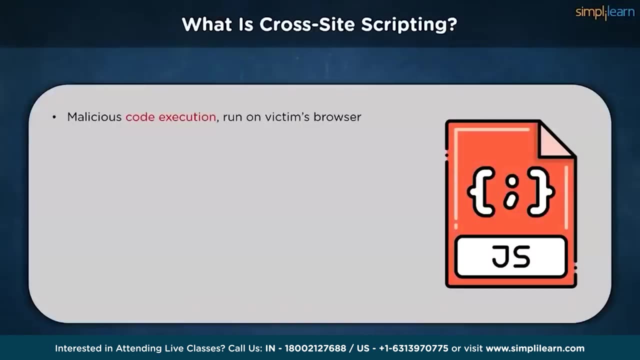 The best way to prevent phishing is browsing the internet with care and being on alert for malicious attempts at all times. Let's start by learning about cross-site scripting from a layman's perspective. Cross-site scripting, also known as XSS, is a type of code injection attack that occurs on the client's side. 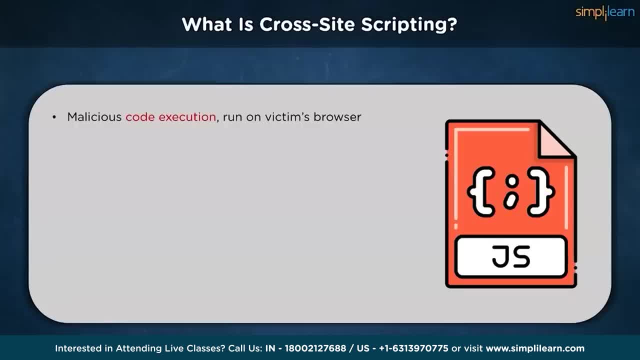 The attacker intends to run harmful scripts in the victim's web browser by embedding malicious code in a genuine web page or online application. The real attack takes place when the victim hits the malicious, code-infected web page or online application. The web page or application serves as a vehicle for the malicious script to be sent to the user's browser. 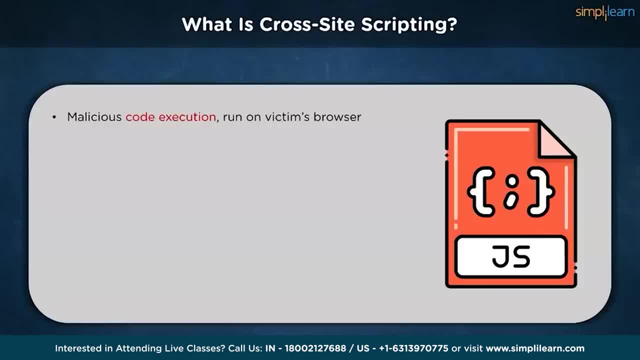 Forums, message boards and online pages that enable comments are vulnerable vehicles that are frequently utilized for cross-scripting assaults. A web page or web application is vulnerable to XSS if the output it creates contains unsanitized user input. The victim's browser must then parse this user input. 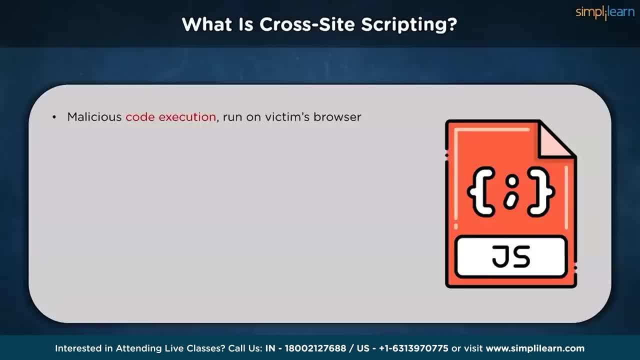 In VBScript, ActiveX, Flash and even CSS. cross-site scripting attacks are conceivable. They are nevertheless most ubiquitous. They are ubiquitous in JavaScript owing to the fact that JavaScript is most important to most browser experiences nowadays. The main purpose of this attack is to steal the other user's identity, be it via cookies, session tokens and other information. 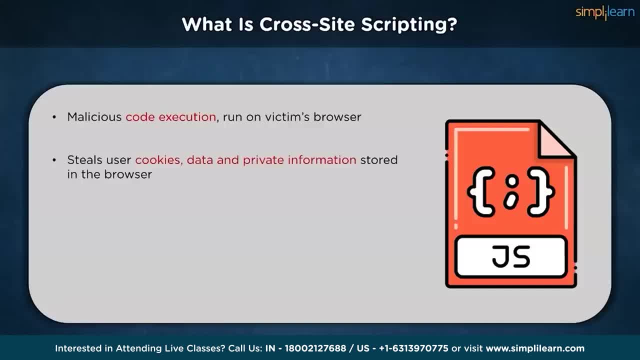 In most of the cases, this attack is being used to steal the other person's cookies. As we know, cookies help us to log in automatically. Therefore, with the stolen cookies, we can log in with other identities, And this is one of the reasons why this attack is so important. 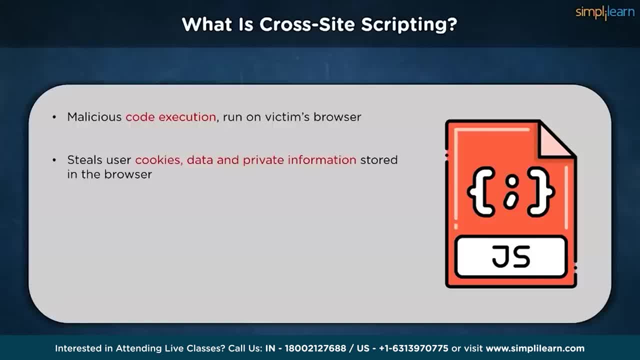 This attack is considered as one of the riskiest attacks. It can be performed with different client-side programming languages as well. Cross-site scripting is often compared with similar client-side attacks, as client-side languages are mostly being used during this. However, an XSS attack is considered riskier because of its ability to damage even less vulnerable technologies. 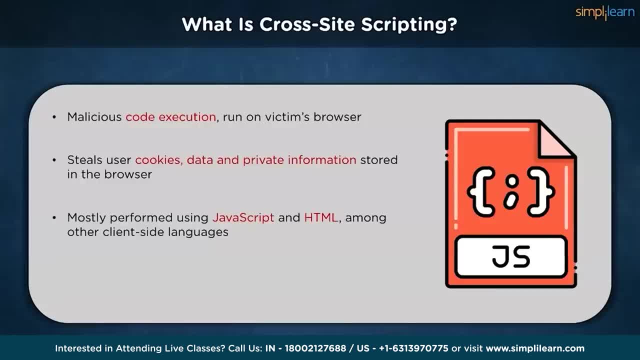 Most often, this attack is performed with JavaScript and HTML. JavaScript is a programming language that runs on web pages inside your browser. The client-side code adds functionality and interactivity to the web page and is used extensively on all major applications and CMS platforms. 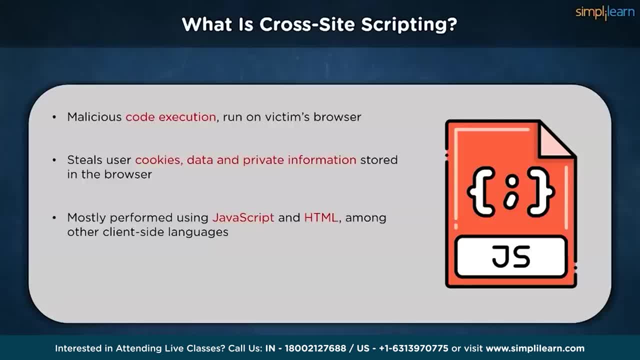 Unlike server-side languages such as PHP, JavaScript code runs inside your browser and cannot impact the website for other visitors. It is sandboxed to your own navigator and can only perform actions within your own browser window. While JavaScript is client-side and does not attack other users, it is also a programming language that runs on web pages inside your browser. 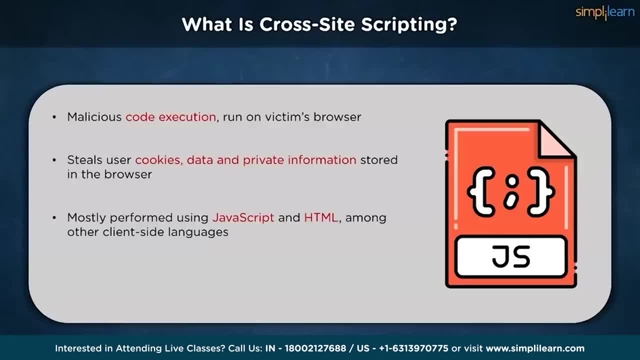 JavaScript is a programming language that runs on web pages inside your browser. While JavaScript is client-side and does not run on the server, it can be used to interact with the server by performing background requests. Attackers can then use these background requests to add unwanted spam content to a web page without refreshing it. 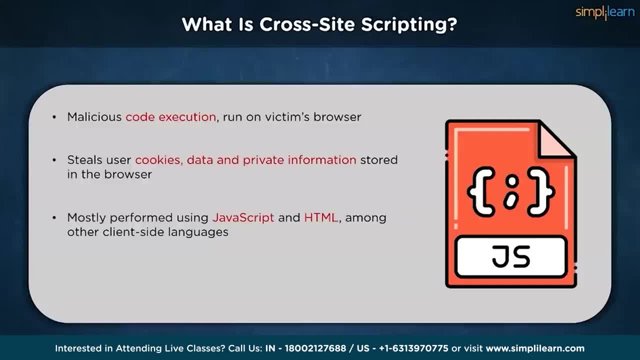 They can then gather analytics about the client's browser or perform actions asynchronously. The manner of attack can range in a variety of ways. It can be a single link which the user must click on to initiate a JavaScript piece of code. It can be used to show any piece of images. 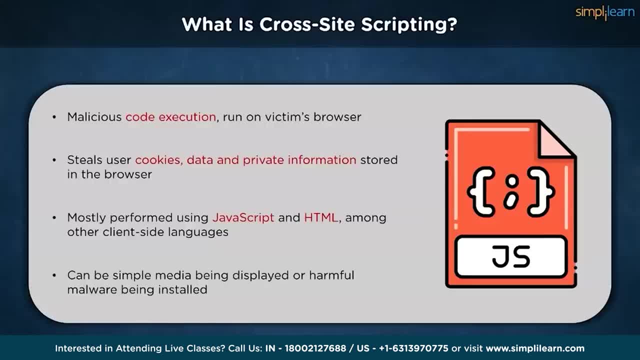 It can be used to show any piece of text that can be later used as a front-end for malicious code being installed as malware. With the majority of Internet users unaware of how metadata works or the ways in which web requests are called, the chances of victims clicking on and redirecting links is far too high. 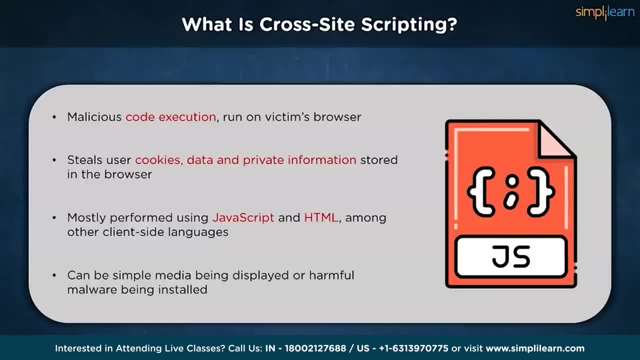 Cross-site scripting can occur on the malicious script executed at the client-side using a fake page or even a form that is displayed to the user. On websites with displayed advertisements, malicious emails can also be sent to the victim. On websites with displayed advertisements, malicious emails can also be sent to the victim. 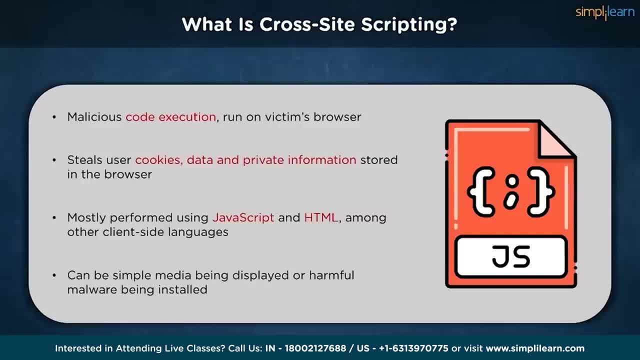 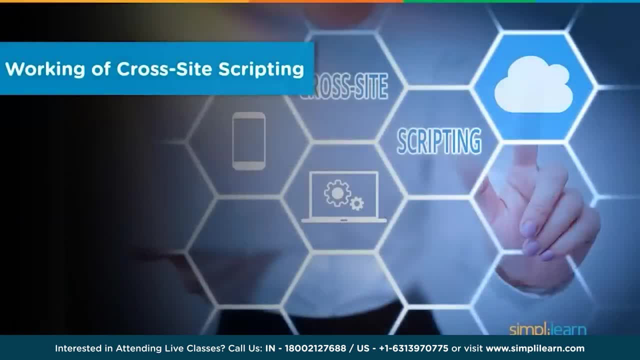 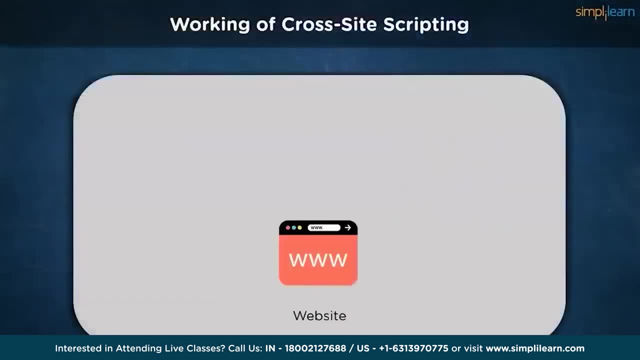 These attacks occur when the malicious user finds the vulnerable parts of the website and sends it as appropriate malicious input. Now that we understand the basics of cross-site scripting, let's learn more about how this kind of attack works Now, first place, we have the website or the web browser which is used to show content to the victim, or which is the user in our case. 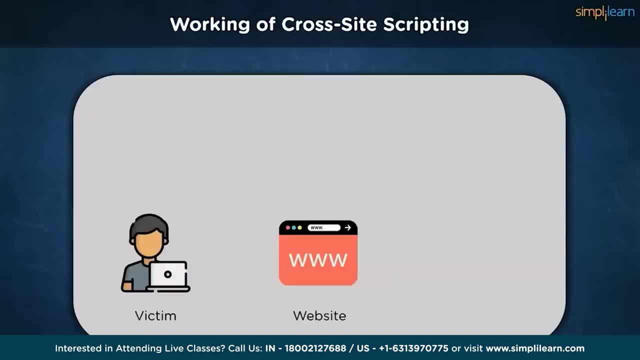 Whenever the user wants to grab some content from the website, the website asks the data from the server. Whenever the user wants to grab some content from the website, the website asks the data from the server, the data from the server. The server provides this information to the website. 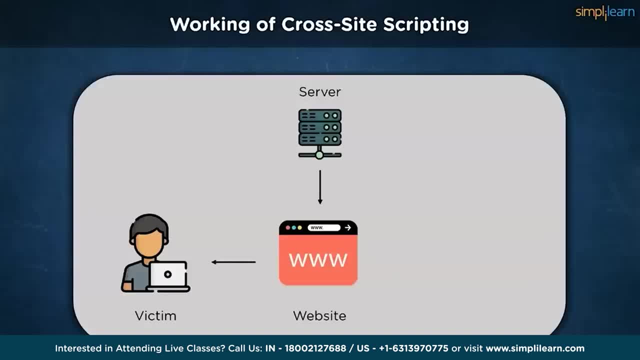 and the web browser, which ultimately resists the victim. How the hacker comes into play here: it passes on certain arguments to the web browser, which is can be then forwarded back to the server or to the user at hand. The entire cross-site scripting attack vector means sending and injecting malicious code or 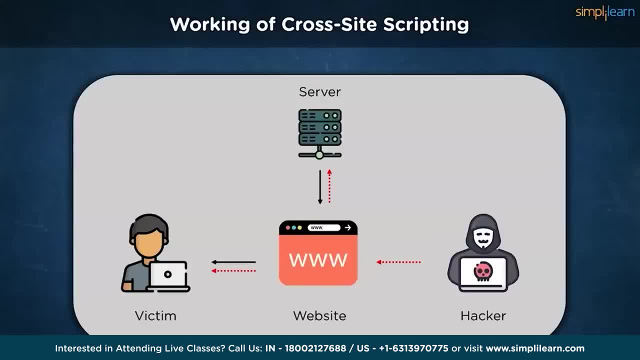 script. This attack can be performed in different ways Depending on the type of attack. the malicious script may be reflected on the victim's browser, but stored in the database and executed every time when the user calls the appropriate function. The main reason for this attack is inappropriate users. 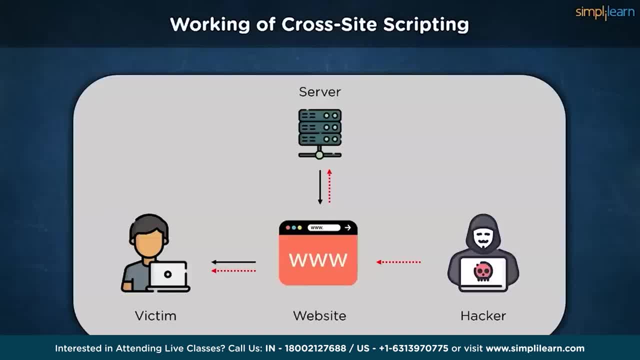 input validation, where the malicious input can get into the output. A malicious user can enter a script which will be injected on to the website's code. then the browser is not able to know if the executed code is malicious or not. Therefore, this malicious script is being 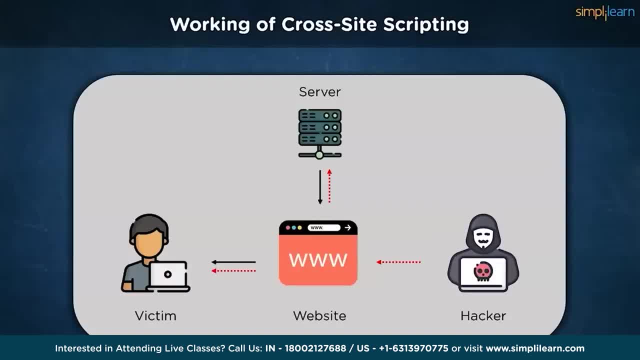 executed on the web victim's browser or any faked form if that is being displayed for the users. There are many ways to trigger an XSS attack. For example, the execution could be triggered automatically when the page loads or when a user hovers over specific elements of the page, like hyperlinks. 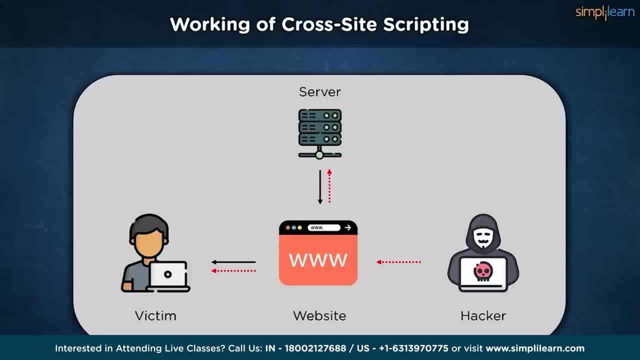 Potential consequences of cross-site scripting attacks include capturing keystrokes of a user, redirecting a user to malicious websites, running web browser based exploits, obtaining cookie information of a user who is logged into a website, and many more. In some cases, XSS attack leads to complete compromise of the victim's account. 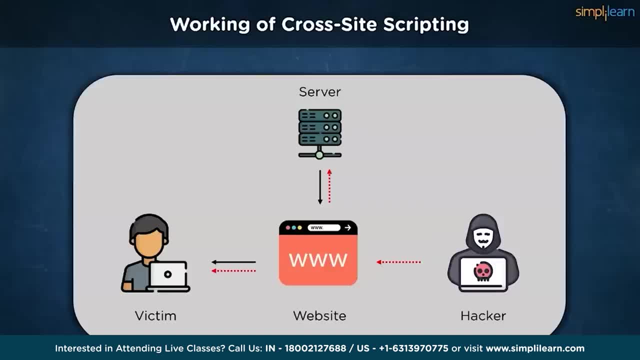 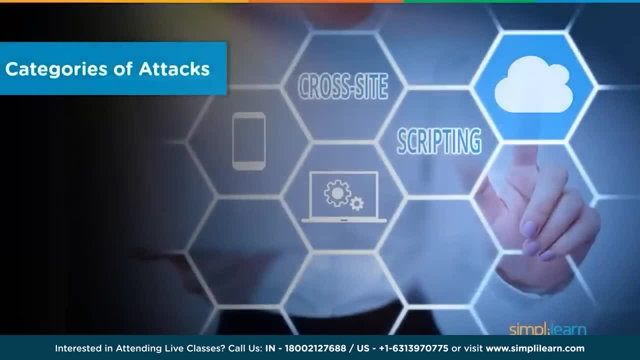 Attackers can trick users into entering credentials on a fake form, which can then provide all information to the attacker. With the basic working of a XSS attack out of the way, let us go over the different ways hackers can leverage vulnerable web applications to gather information and eventually breach. 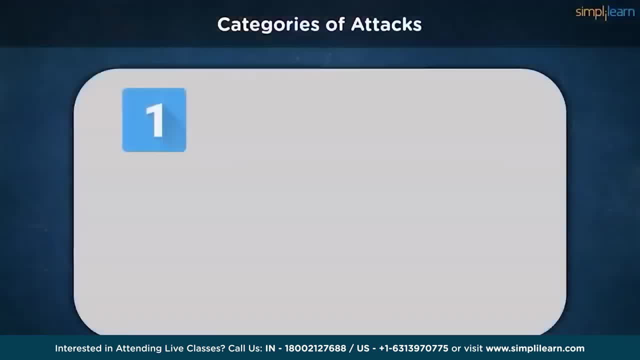 those systems. 1. The prime purpose of performing XSS attack is to steal the other person's identity. As mentioned, it may be cookies, session tokens, etc. XSS may also be used to display faked pages or forms for the victim. 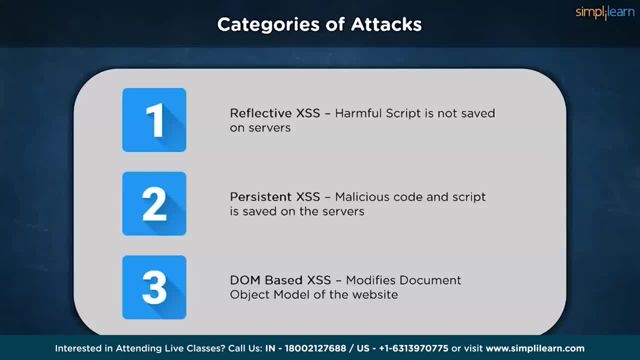 However, this can be performed in several ways. We have a Reflected attack. This attack occurs when a malicious script is not being saved on the web server but is reflected in the website results. Reflected XSS code is not being saved. It is not being saved permanently. 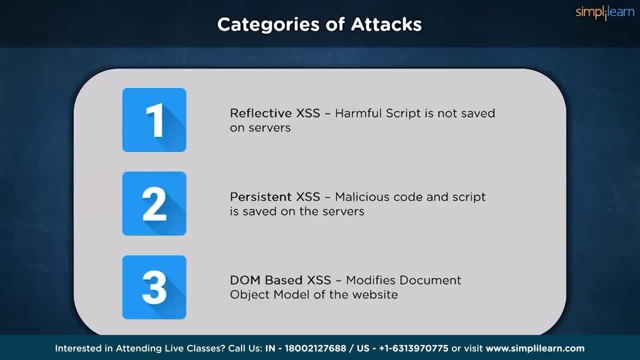 In this case, the malicious code is being reflected in any website. result: The attack code can be included in the faked URL or in the HTTP parameters. It can affect the victim in different ways, by displaying a faked malicious page or by sending a malicious email. 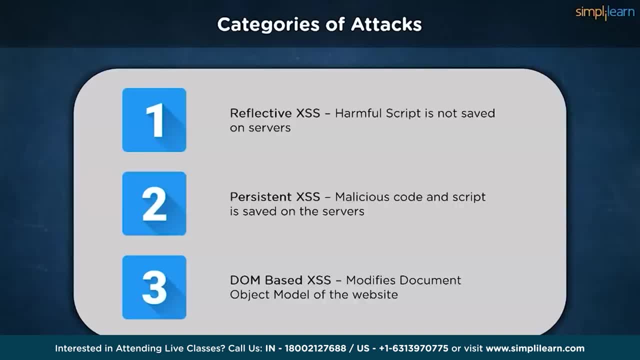 In a Reflected XSS scripting example, the input of a search form is reflected on the page to show what the search key was. An attacker may craft a URL that contains malicious code and then spread the same URL. The user can then use the search key to search the page. 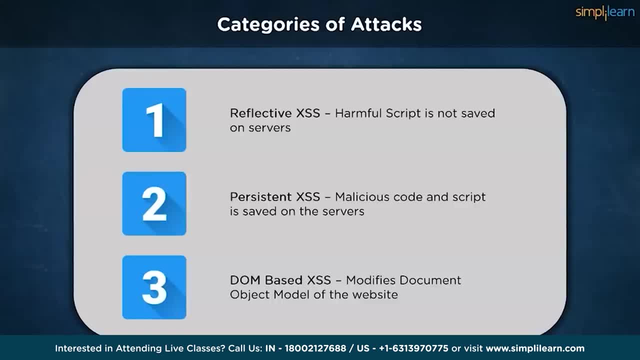 In this case, the attacker may craft a URL that contains malicious code and then spread the same URL. A user who clicks on this link opens the valid web application, which then runs the malicious code in the browser. This script is not stored in the web application and malicious code is shown only to one user. 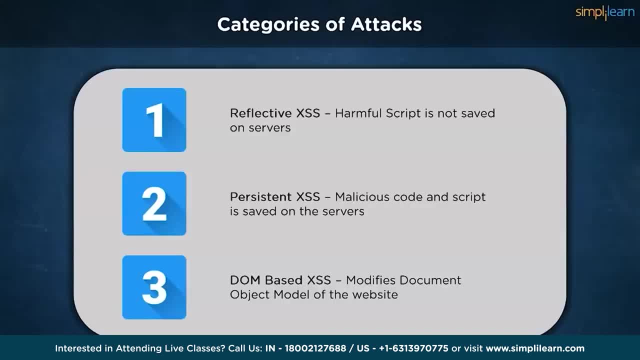 The user that opens the link executes this script, and the attack is not necessarily visible on the server side or to the app owner itself. The next variant is the Stored Cross-Site Scripting attacks. This occurs when a malicious script is not being saved on the web server or to the app owner itself. 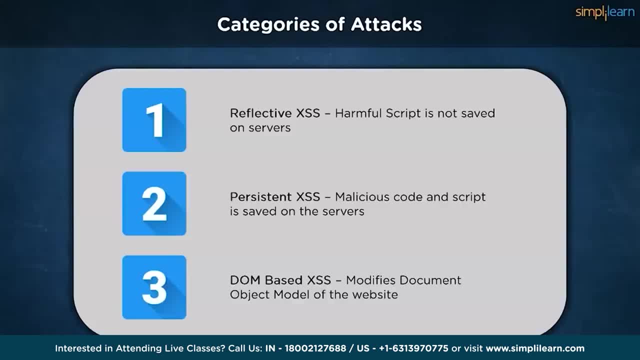 The next variant is the Stored Cross-Site Scripting attacks. This occurs when a malicious script is not being saved on the web server or to the app Server permanently. The first threat can be a riskier attack, since this rate has leverage for more damage. 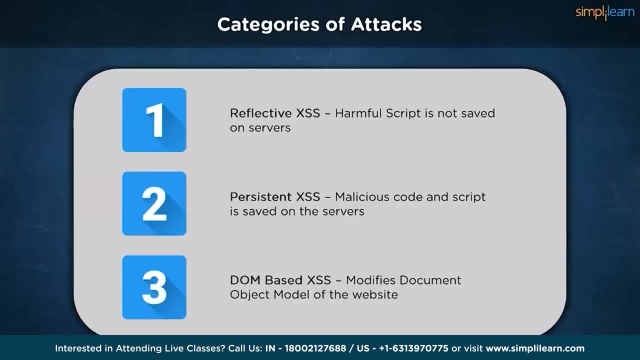 In this type of manner, the malicious code or script is being saved on the server, for example in the database. It is executed every time the user calls the appropriate functionality. This way Stored XSS attack can affect many users. Also, as the script is being stored on the web server, it will affect the web server for a longer time. 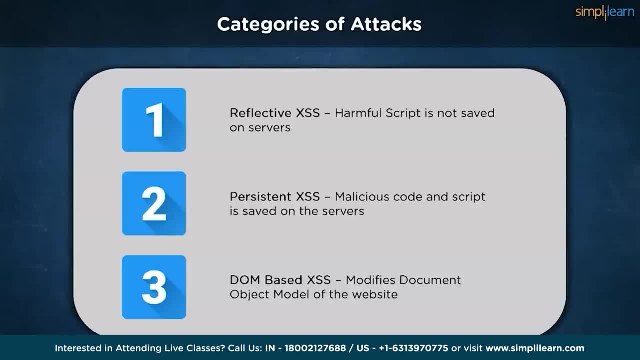 In order to perform stored XSS attack, the malicious scripts should be sent through the vulnerable input form. for example can be a comment field or a review field. This way, the appropriate script will be saved in the database and evaluated on the page load or appropriate function calling. 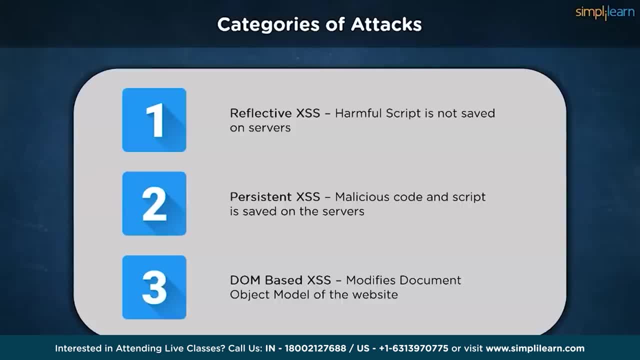 In a stored XSS example, the script might have been submitted via an input field to the web server, which did not perform a sufficient validation and stores the script permanently in the database. The consequence of this might be that this script is now being delivered to all users. 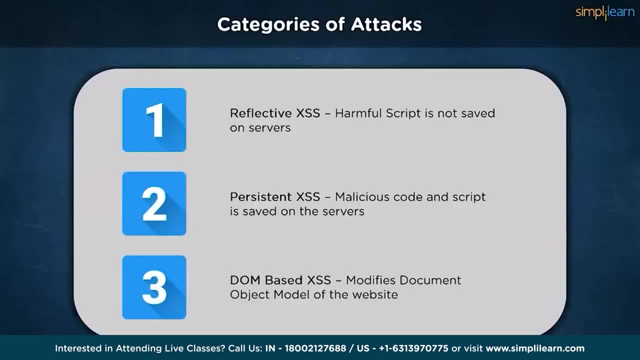 visiting the web application and are, for example, able to gain access to the user session cookies. In this attack, the script is permanently stored in the web app. The users visiting the app after the information retrieve the script. The malicious code then exploits the flaws in the web application and the script and 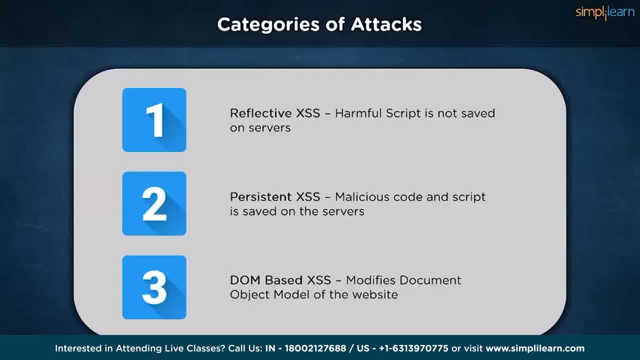 the attack is visible on the server side or to the app owner as well. The third variant is the user session cookies. The third variant is DOM based cross-site scripting attacks. This type of attack occurs when the DOM environment is being changed, but the client-side code. 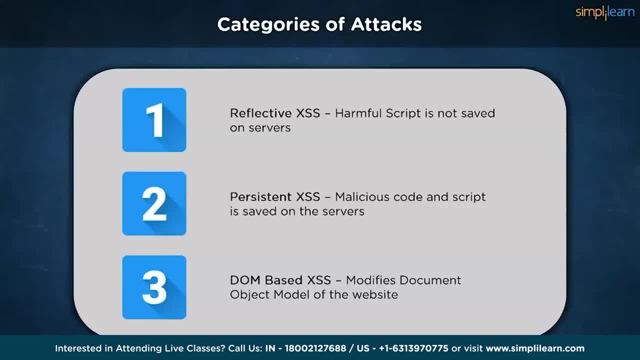 does not change When the DOM environment is being modified in the victim's browser. the client-side code executes differently. In order to get a better understanding of how XSS DOM attack is being performed, let us analyze the following example. If there is a website called textincom, we know default is a parameter. 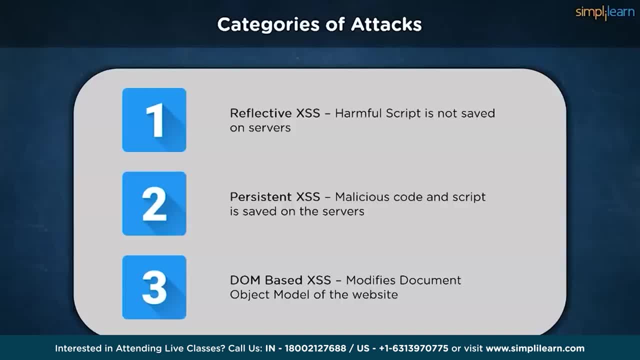 Therefore, if we want to use default, we need to use default. Therefore, in order to perform XSS DOM attack, we should send a script as parameters. A DOM based XSS attack may be successfully executed even when the server does not embed any malicious code into the web page by using a flaw in the JavaScript executed in the browser. 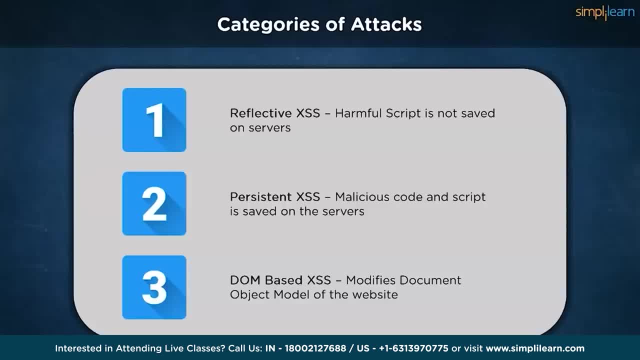 For example, if the client-side JavaScript modifies the DOM tree of the web page, it can be based on an input field or the GET parameter, without validating the input. This allows the malicious code to be executed- The malicious code that exploits flaws in the browser on the user side and the script. 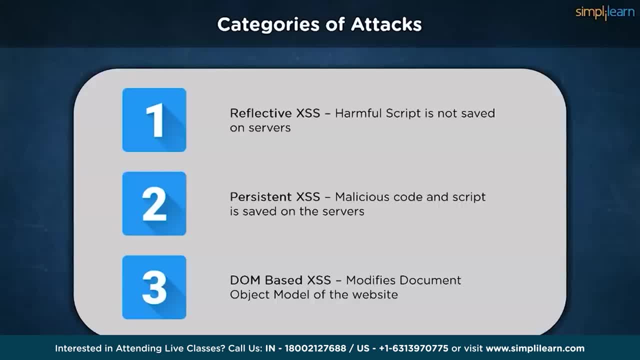 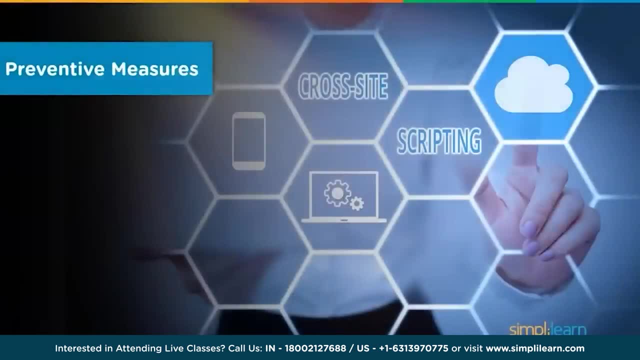 and the attack is not necessarily visible on the server side or to the app owner. By now, it is clear that cross-site scripting attacks are difficult to detect and even tougher to fight against. There are, however, plenty of ways one can safeguard against such attacks. 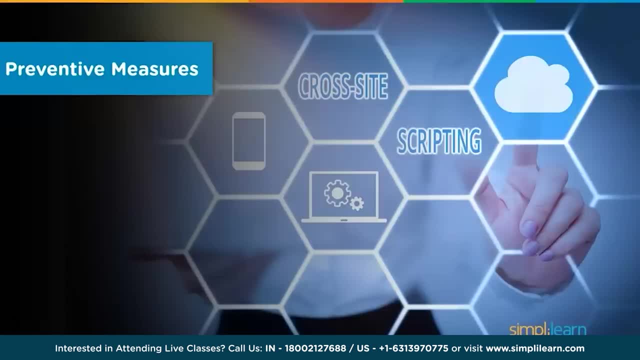 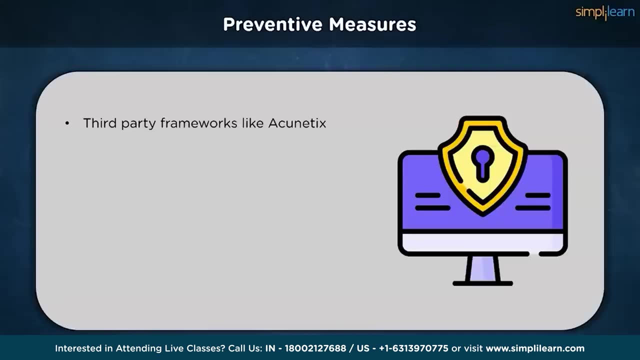 Let's go through some of these preventive measures. 1. Like mentioned earlier, XSS attacks are sometimes difficult to detect. However, this can be changed if you get some external help. A way to prevent XSS attacks is using automated testing tools like Crashtest Security Suite. 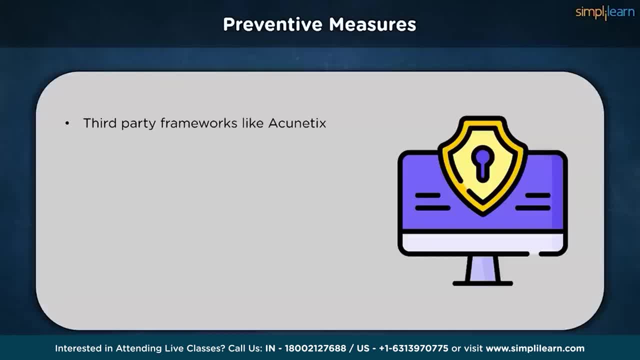 or Acunetix Security Suite. Still, manual testing is highly time-consuming and costly, and therefore not possible to be done for every iteration of your web application. Consequently, your code shouldn't be untested before any release. 2. Using automated security, you can scan your web application for cross-site scripting and. 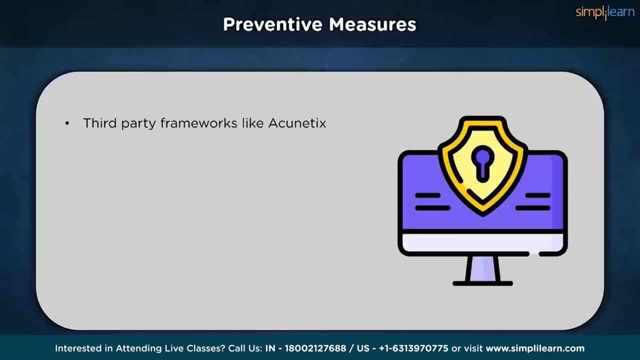 other critical vulnerabilities before every release. This way, you can ensure that your web application's live version is still secured whenever you alter or add a feature. Input fields are the most common point of entry for XSS attack scripts. Therefore, you should always screen and validate any information input into data fields. 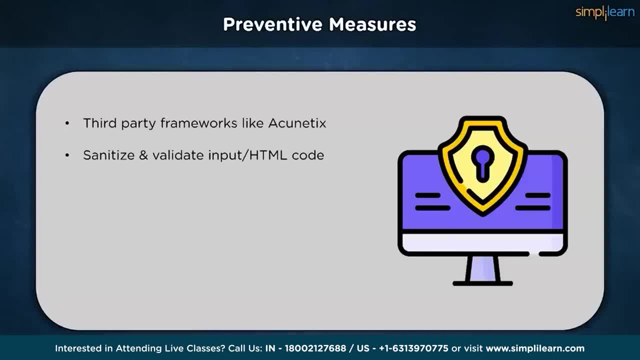 This is particularly important if the data will be included as HTML output. This can be used to protect against reflected XSS attacks. Validation should occur on both the client side and server side. as an added precaution, This helps validating the data before it's being sent to the servers and can also protect 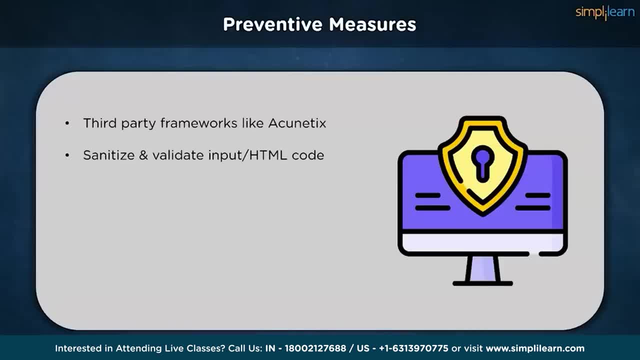 against persistent XSS scripts. This can be accomplished using JavaScript. XSS attacks only appear if any user input is being displayed on the web page. Therefore, try to avoid displaying any untrusted user input if possible. 3. If you need to display user data, restrict the places where the user input might appear. 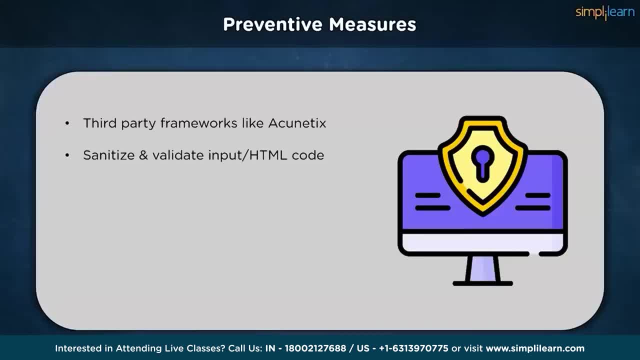 Any input displayed inside a JavaScript tag or a URL shown on the site is much more likely to be exploited than the input that appears inside a division or a span element inside the HTML body. Protecting against XSS vulnerabilities typically requires properly escaping user-provided data. 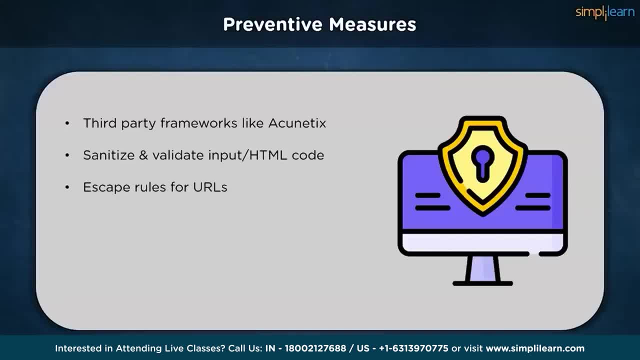 that is placed on the page, rather than trying to determine if the data is user-provided and could be compromised. We should always play it safe and escape data, whether it is user-provided or not. Unfortunately, because there are many different rules for escaping, you still must choose. 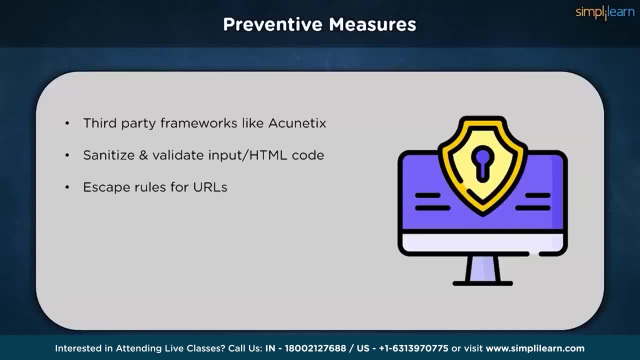 the proper type of escaping before settling on a final code. Encoding should be applied directly before user-controllable data is written to a page, because the context you're writing into determines what kind of encoding you need to use. For example, values inside a JavaScript string require a different type of encoding than a. 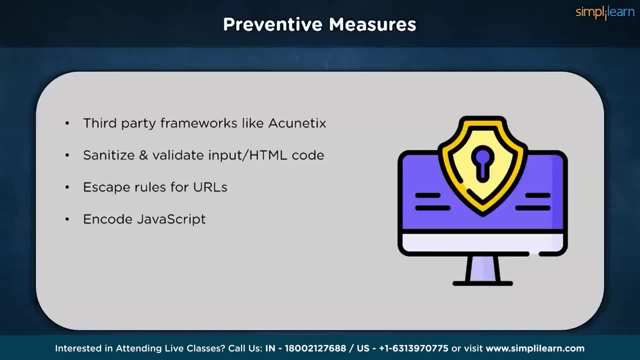 JavaScript string. Sometimes you'll need to apply multiple layers of encoding in the correct order. For example, to safely embed user input inside an event handler, you need to deal with both JavaScript context and the HTML context, So you need to first Unicode escape the input and then HTML encode it. 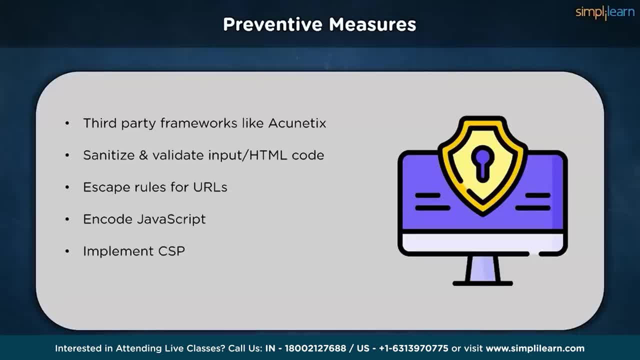 Content Security Policy is a computer security standard introduced to prevent cross-site scripting, click-checking and other code-injection attacks resulting from the execution of malicious content in the trusted web page context. It is a candidate recommendation of the W3C Working Group on web application security. 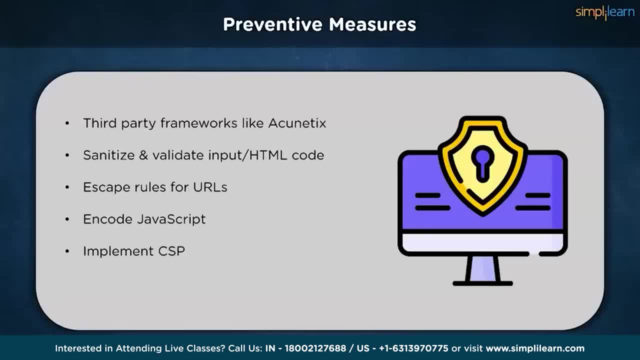 It's widely supported by modern web browsers and provides a standard method for website owners to declare approved origins of content that browsers should be allowed to load on that website. HTTP-only is an additional flag included in a set-cookie HTTP response. It's a standard method for website owners to declare approved origins of content that. 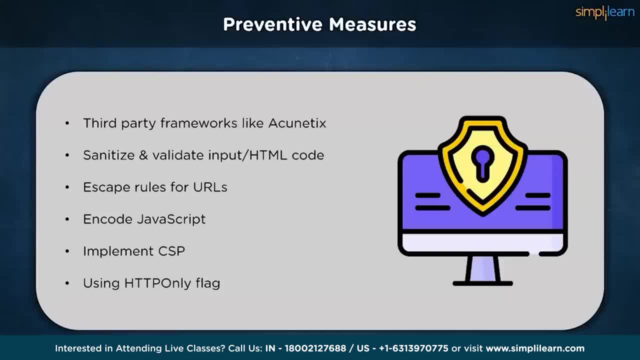 browsers should be allowed to load on that website. Using the HTTP-only flag when generating a cookie helps mitigate the risk of client-side script accessing the protected cookie, that is, if the browser supports it. If the HTTP-only flag is included in the HTTP response header, the cookie cannot be accessed. 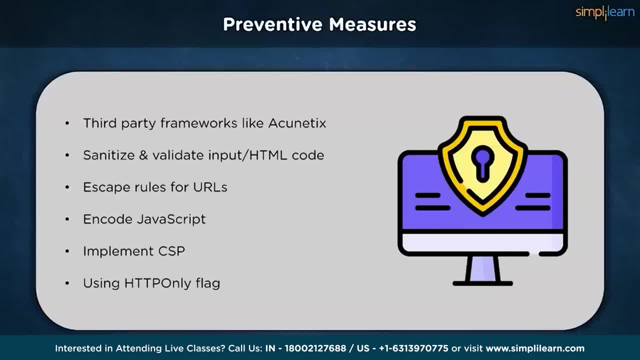 through a client-side script. again, this is if the browser supports this flag. As a result, even if a cross-site scripting flaw exists and a user accidentally accesses a link that exploits this flaw, The browser will not review it. It will deal the cookie to a third party. 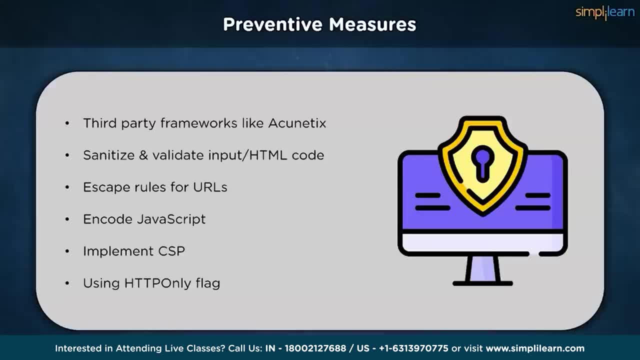 If a browser does not support HTTP-only and a website attempts to set an HTTP-only cookie, the HTTP-only flag will be ignored by the browser, thus creating a traditional script-accessible cookie. As a result, the cookie becomes vulnerable to theft of modification by any malicious. 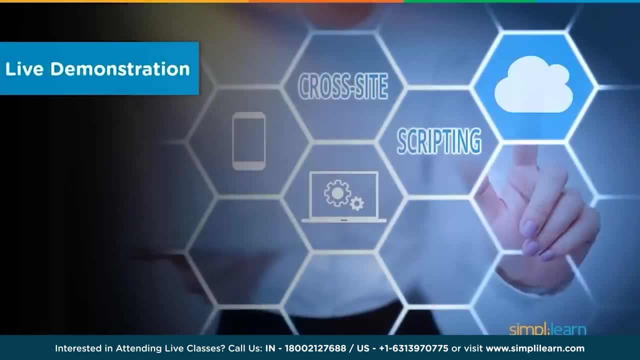 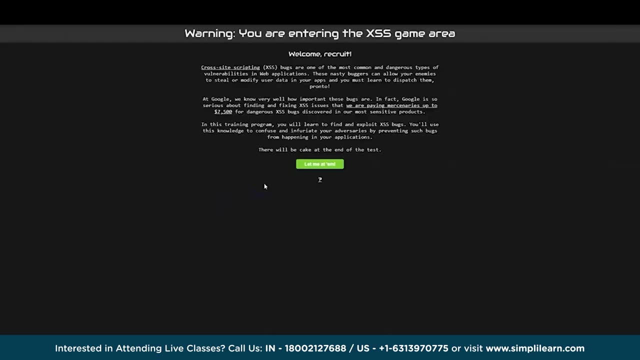 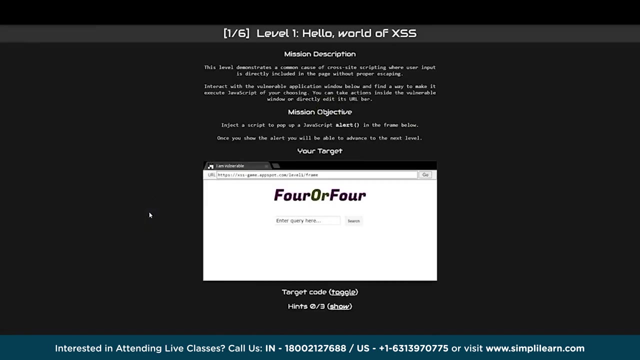 script. Next on our docket is a live demonstration where we solve a set of cross-site scripting problems, starting from the basic level to the top-most level. Let's begin In this verb application. it demonstrates the common cause of cross-site scripting where 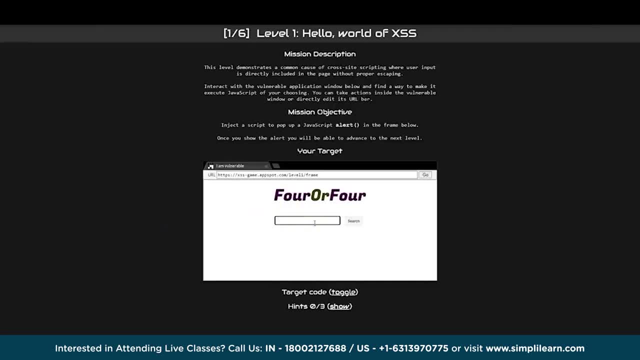 user input is directly included in the page without proper escaping. If we interact with the Vulnerable application window here and find a way to make it execute JavaScript of our choosing, we can take actions inside the Vulnerable window or directly edit its URL bar. 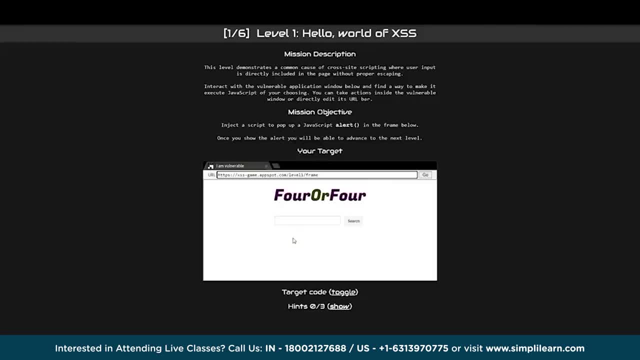 This doesn't mean that we can't execute JavaScript of our choosing. This task needs only basic knowledge. Let's see why the most primitive injections work here right away. Let's do a simple query and inspect the resulting HTML page. I'm going to use this phrase with a single quote as a special character. 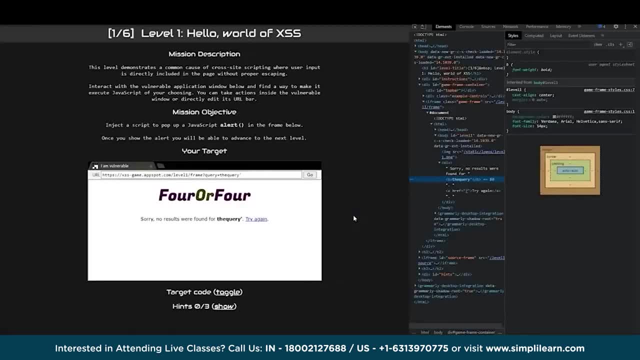 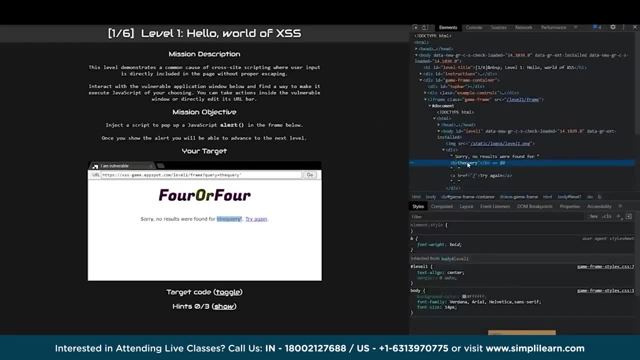 We can now inspect the HTML page. We can see here in this line, the special character single quote appears in the result over here. The provided query text is placed directly in a tag as in a body element. We need to perform a reflected XSS into the web application because they are non-persistent. 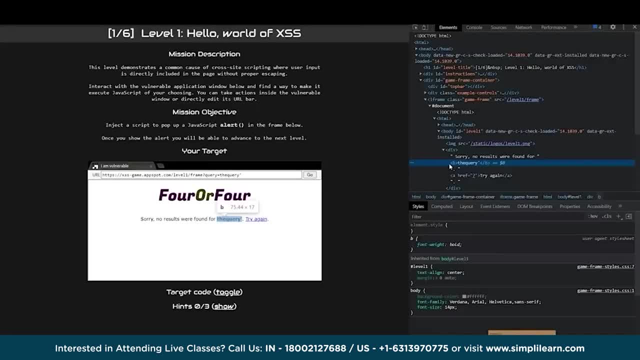 XSS attacks and the payload should be included in the URL to perform successful exploitation. We can use any of these. We can use any payload, but we're going to use the simple one to perform an alert in this web application. It's simple and can be shown easily. 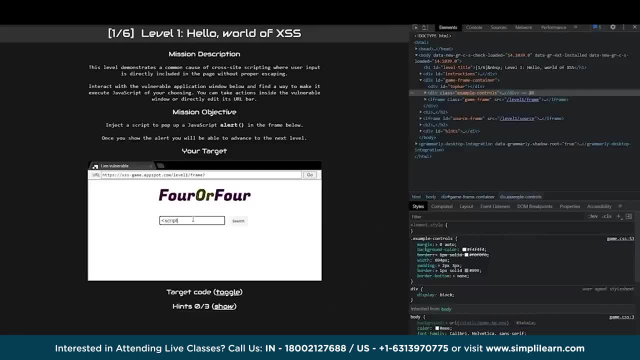 We're just going to write the script over here, Great, And we're going to press search. As you can see, we have successfully launched our first cross-site scripting attack. We can see an alert box pop up with the necessary message, and a similar process can be used. 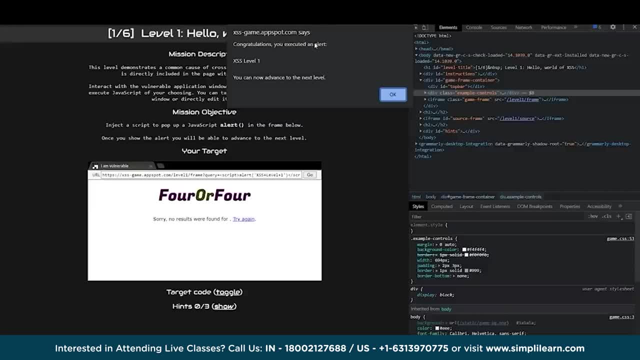 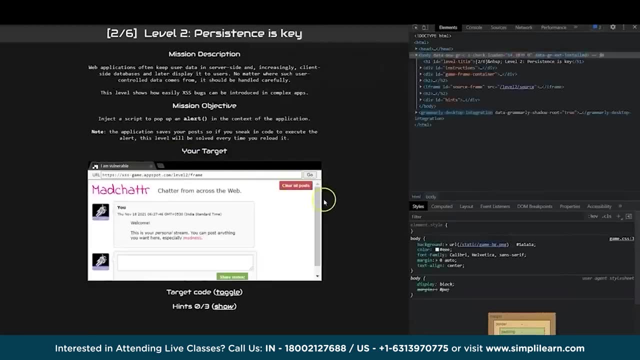 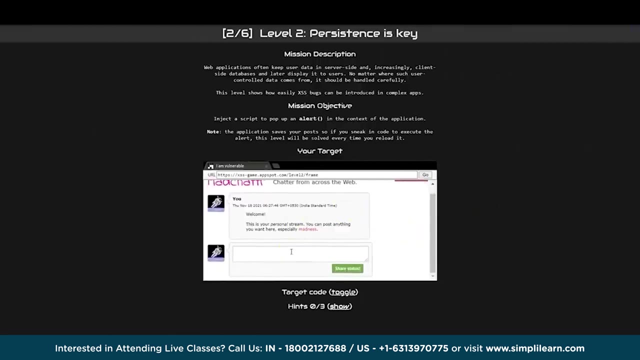 to steal browser cookies and passwords, albeit with different commands. Now we have the option to move to level two In this web application. it shows that how easily XSS bugs can be introduced in complex chat applications. Chat app conversations are stored in a database and retrieved when a user wants to see the 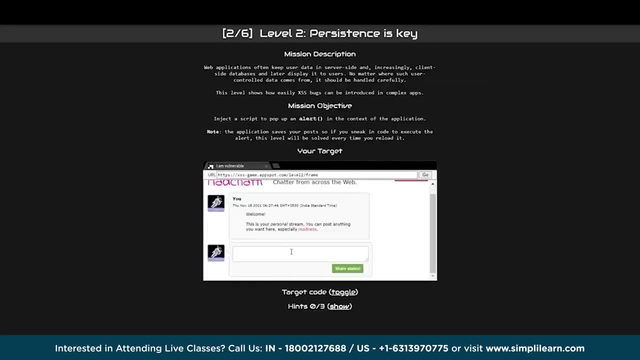 conversation. Therefore, if a malicious user injects some JavaScript code, all visitors will be infected. This kind of cross-site scripting attack is more powerful and it is more riskier than reflected crosses scripting attacks, And that's why is known as stored XSS. 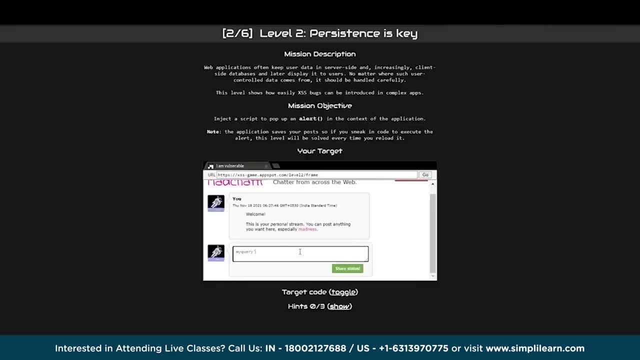 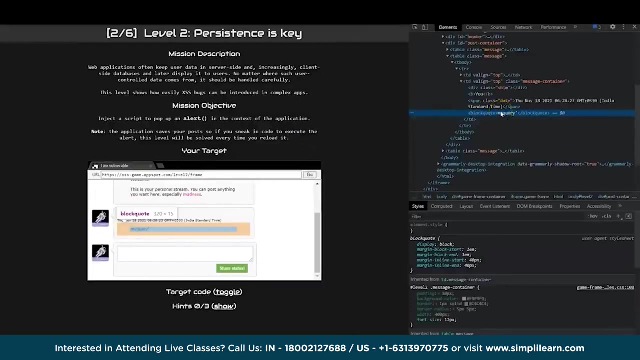 I posted my query with a special character of a single quote And this is what I get. Whatever I type in simply appeared on the page right after I click on Here status. Let's see the source You can see here. Yeah, posted seems directly put inside a block code tag. 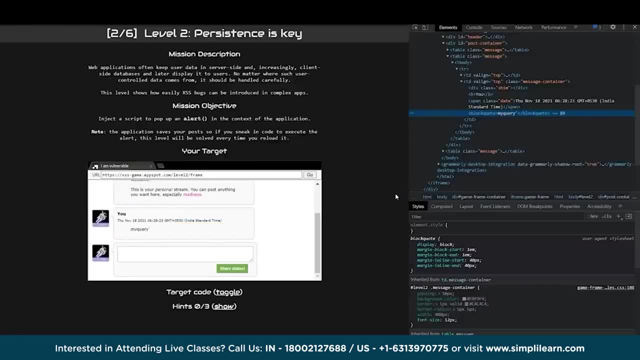 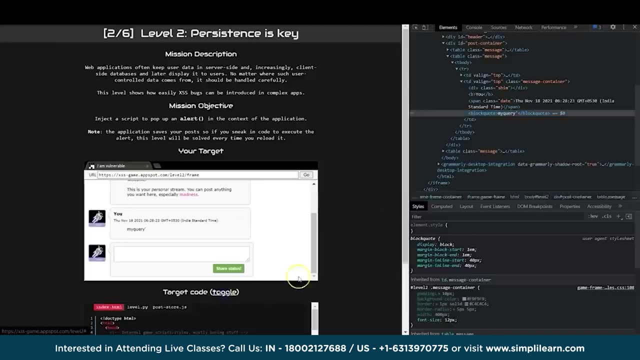 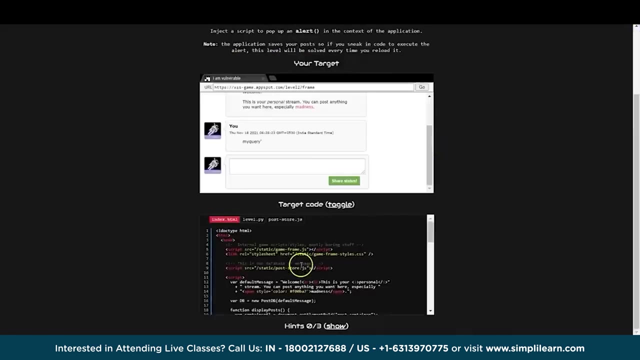 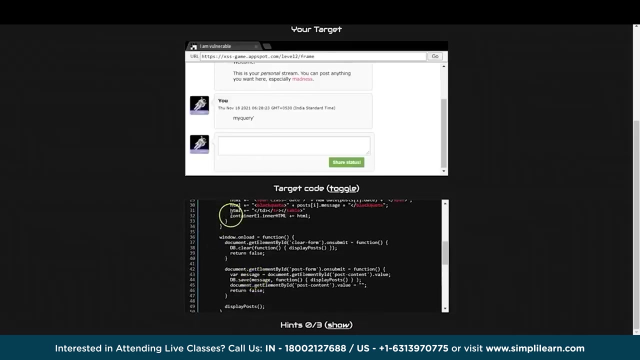 So even a simple script tag we used in level one should work here, but it will not. Let us examine the code to understand why. We're going to toggle the code over here and check the indexhtml file. Second part is line 32.. 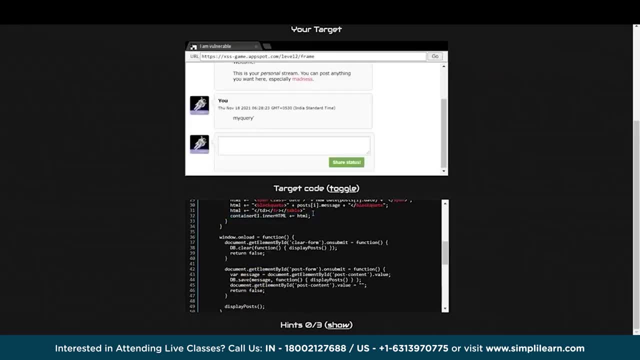 The generated HTML fragment, which is the HTML variable in the code, is added to the mail HTML using the inner HTML method. So when the browser parsing this HTML fragment, it will not execute any script tag defined within that HTML fragment. HTML parser will not execute a script tag when it parses HTMLs via this method. 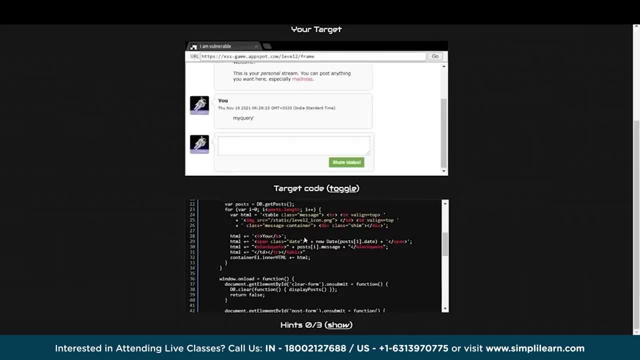 This is why the script tag, like we used in level one, It's not going to work here. Our solution is to use events. Events will execute the defined JavaScript. We're going to use an image over here. Okay, Okay, Okay. 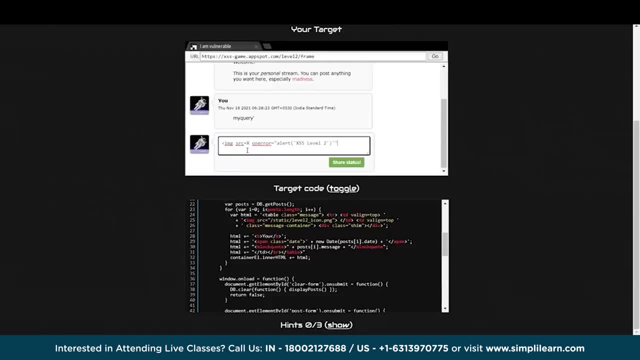 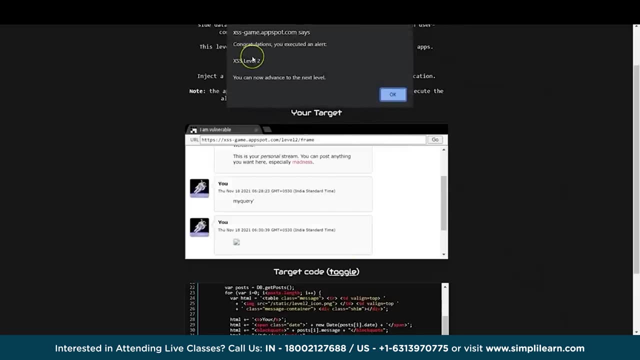 Okay, Okay. When we add an image over here and when we press on share status in the above injection, we're loading an image that doesn't exist, which causes to trigger an on error event. In on error event, it will execute our alert method. 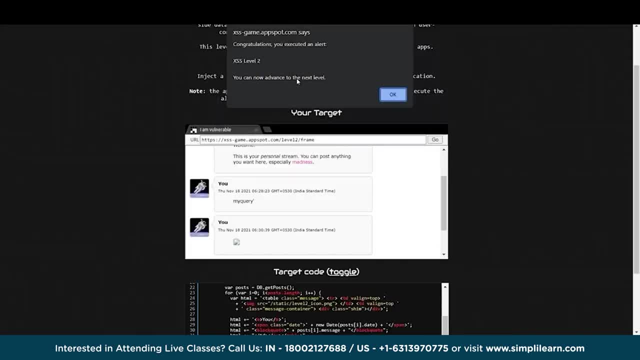 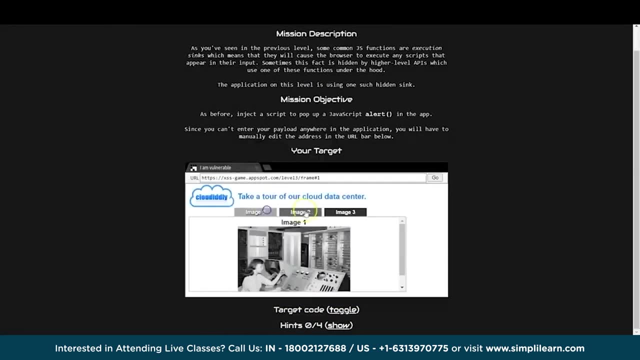 With that, we are able to beat level two and we can now move up to the next level in our challenge. As you can see, clicking on any tab causes the tab number to be displayed in the URL fragment. This hints that the value after the hashtag controls the behavior of the page, that is. 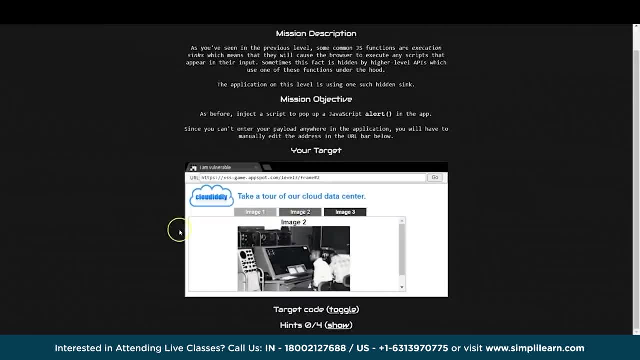 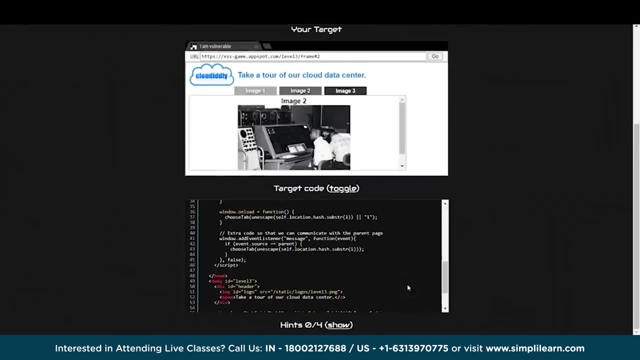 it is an input variable. To confirm. let's analyze the code. As you can see in line 43, inside the event handling, the value provided after the hash in the URL is directly passed onto the true tab method. No input validation is being performed. 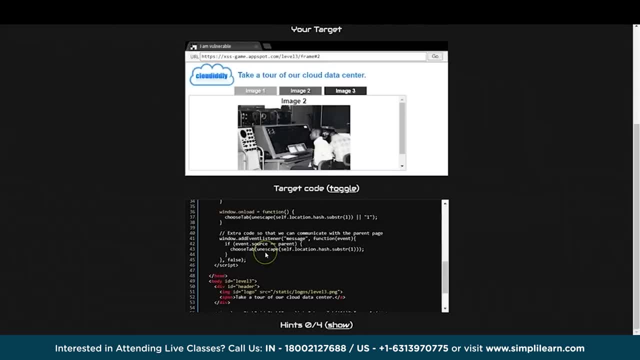 The value passed to the choose tab method is directly injected into the IMG tag in line 17.. This is an unsafe assignment and it is the vulnerable part of the code Now. all we have to do now is to craft a payload that would adjust the IMG tag to execute our 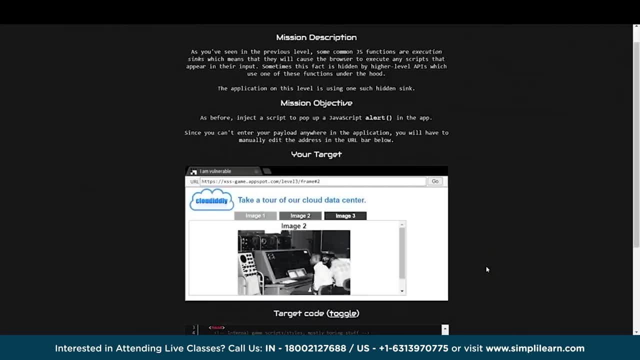 JavaScript, Remember, the script tag from level 1 would not work here, since the variable HTML is used to add the DOM dynamically. hence the events are our aces here. once again, I will choose to use the existing IMG tag and change the source to something that doesn't. 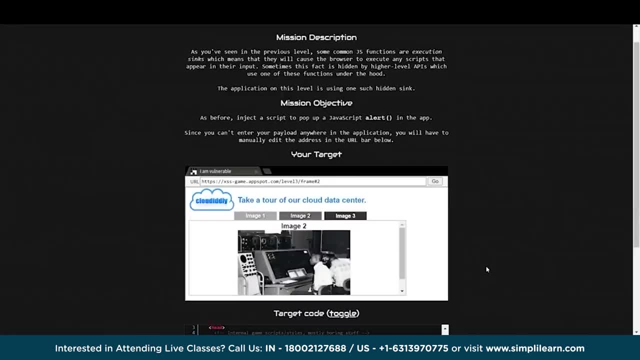 exist, hence forcing it to fall in to execute an on error, even which. I will pass the URL. Let's see how this works. Once we visit that URL, we can see that our Java popup has opened up here with the same message of XSS: level 3 has been completed. 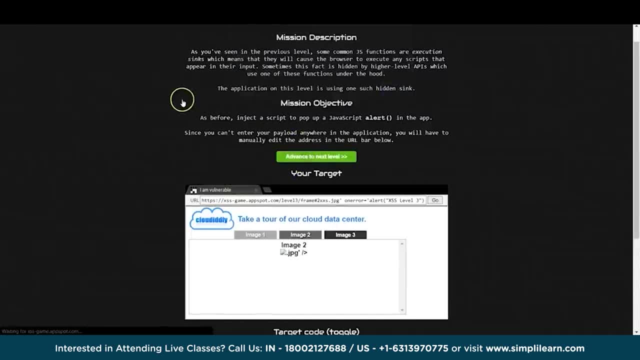 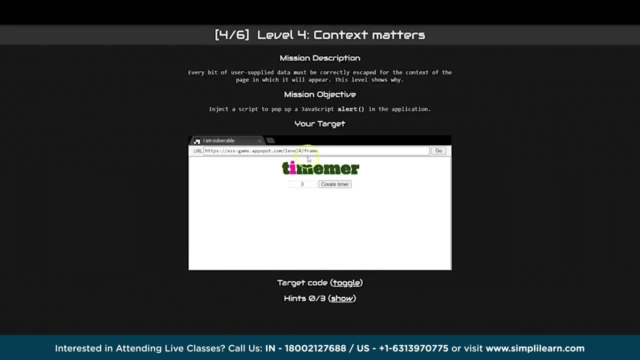 With this we can now move on to level 4, which is going to present a different kind of attack. In this server application there is a timer on the page. that means whatever numbers we put in the box, a countdown starts. This will ensure a lot of time on the page. 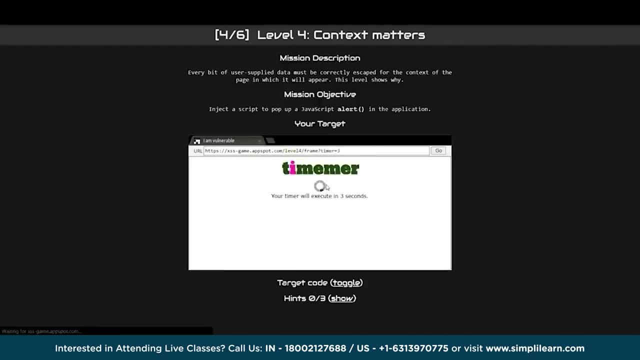 And when it finishes, the application alerts that the countdown is finished And we can see the time is a pop-up appearing over here and this resets the timer again. Now it is obvious that the value entered in the text box is transferred to the server. 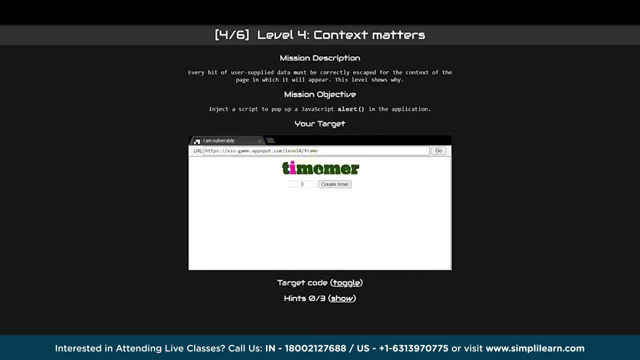 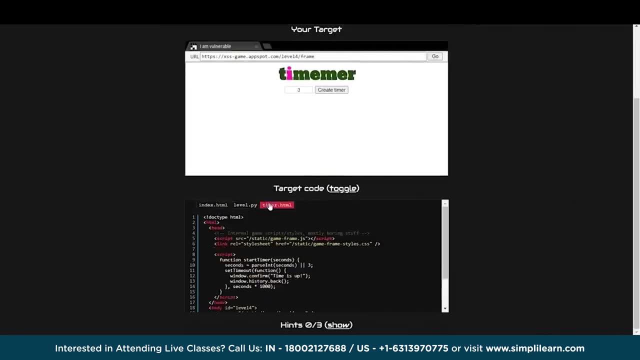 over the timer parameter in the URL. Let us examine the code to see how the timer parameter is being handled. We're going to visit timerhtml over here And we're going to check over here In line 21,. the start timer method is being called in the onLoad event. 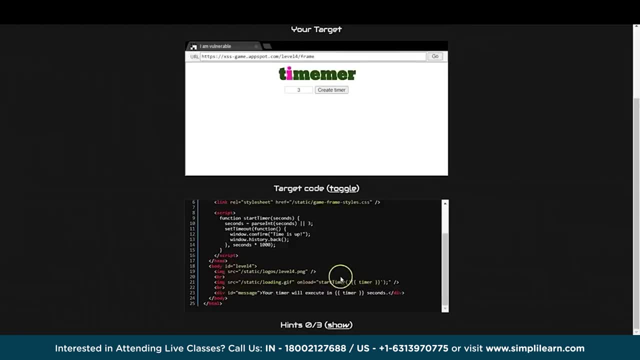 However, the timer parameter is being directly passed to the start timer method. We need to perform a pop-up alert in the web application which escapes the content of the function start timer without breaking the JavaScript code. The parameter value is directly added to the start timer method without any filtering. 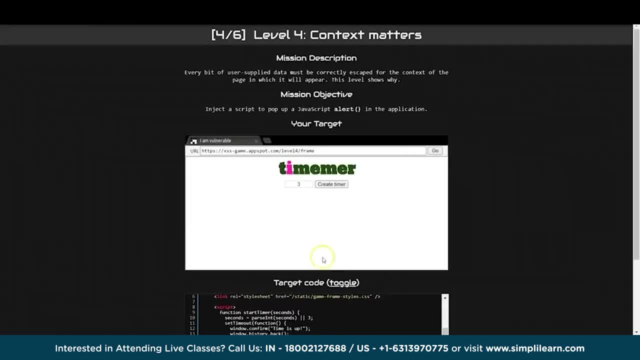 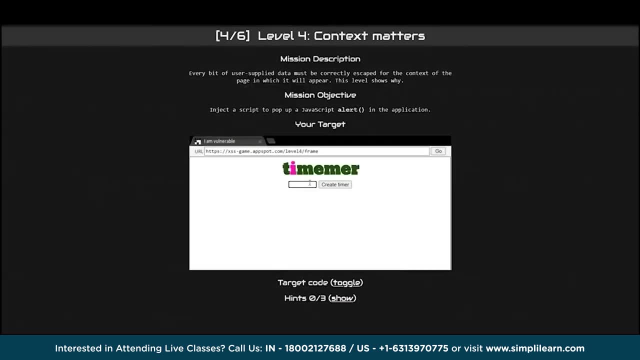 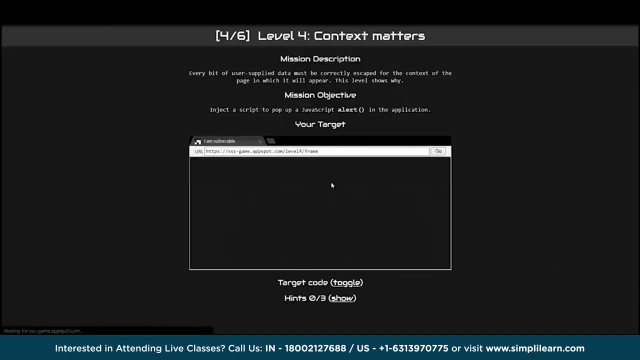 But we can run it. So what I have to do here is to inject an alert function to be executed inside the onLoad event along with the start timer method. We're going to remove this argument and put our script over here. Now I may press on create timer. 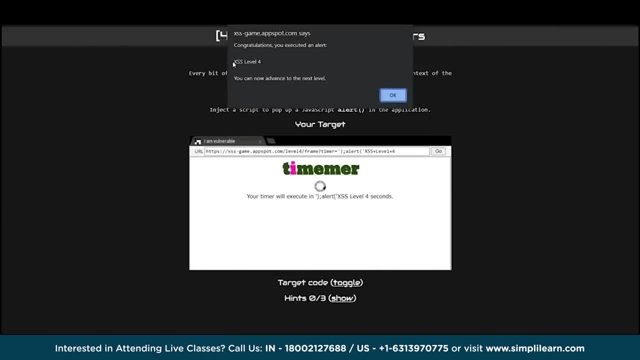 And we have a pop-up with the XSS. level 4 completed. Okay, We can now move on to level 5.. In this web application, this application XSS, is different because this challenge description says: cross-site scripting isn't just about correctly escaping data. 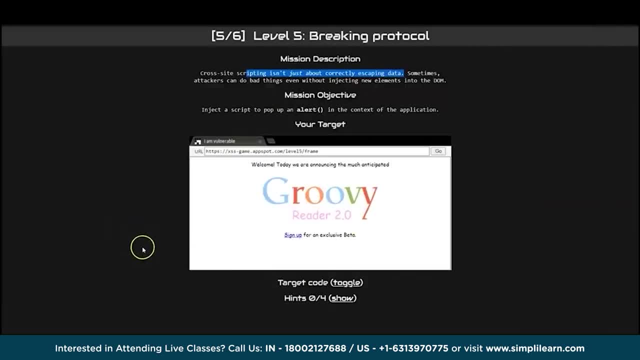 Sometimes attackers can do bad things even without injecting new elements into the DOM. It's kind of open redirect, because the attack payload is executed as a result of modifying the DOM environment In the victim's browser. this environment is used by the original client-side script. 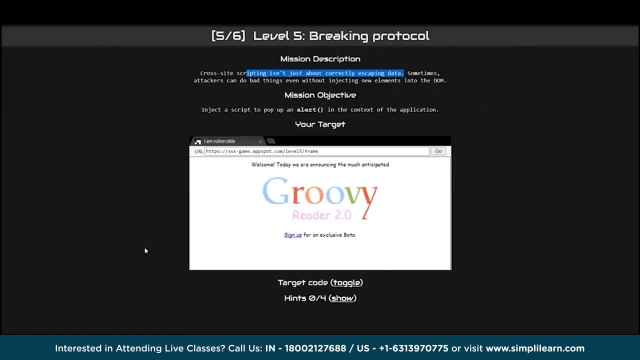 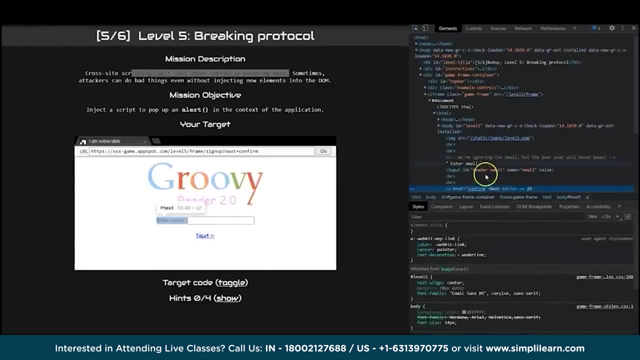 so that the client-side code runs in an unexpected manner. The vulnerability can be easily detected if the next link in the signup page is inspected. The HREF attribute value of next link is confirm, Which is the default value of the HREF attribute. 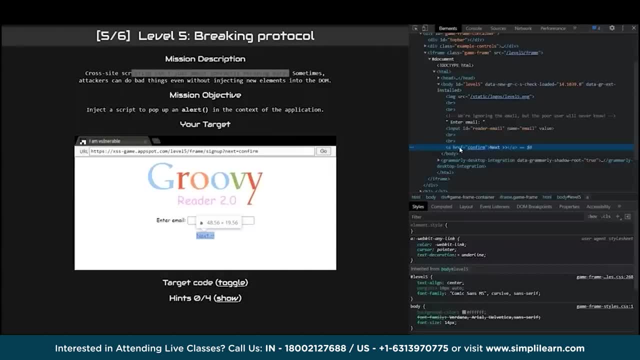 Next, This is exactly the value of the next URL query parameter. as you can see over here, This means using the next query parameter can be used to inject a JavaScript code to the HREF attribute of the next link. The following is the best way to do it: 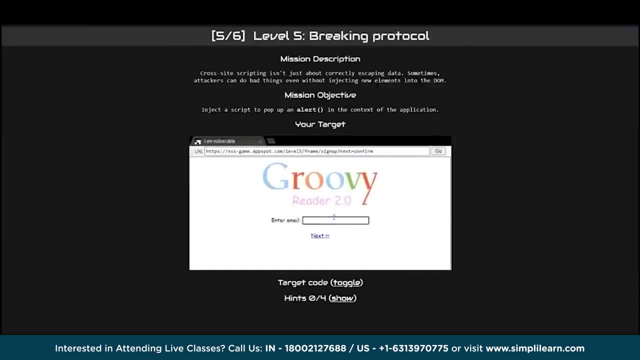 As soon as the user clicks on the link, the script will be triggered. We are then going to press anything random, And now that we click next, we can see the XSS level 5 that we had provided in the URL as a parameter to the next variable. 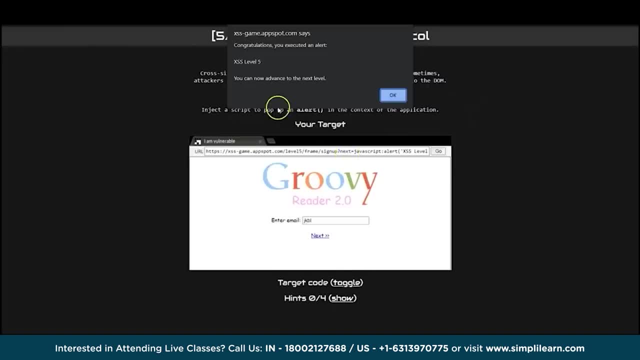 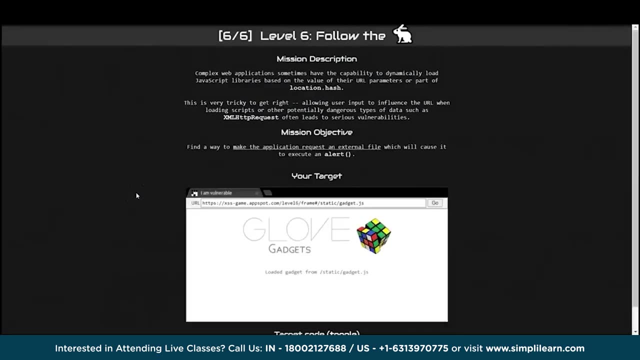 We can see it's a valid variable. Since the value of next provided appears on a pop-up, we can consider the attack a success and move on to the final level 6.. In this server application it shows some of the external JavaScript is retrieved. 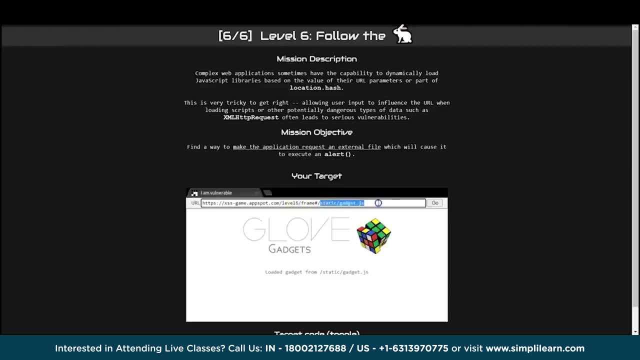 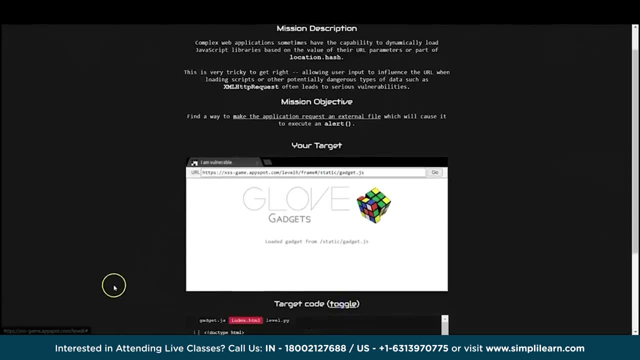 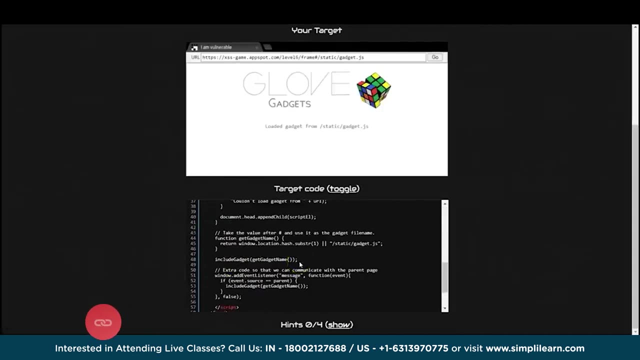 If you analyze the URL, you can see that the script is loaded already. The vulnerability lies within how the code handles the value after the hashtag. If you check on line 45, the value right after the hashtag is taken as the gadget name. 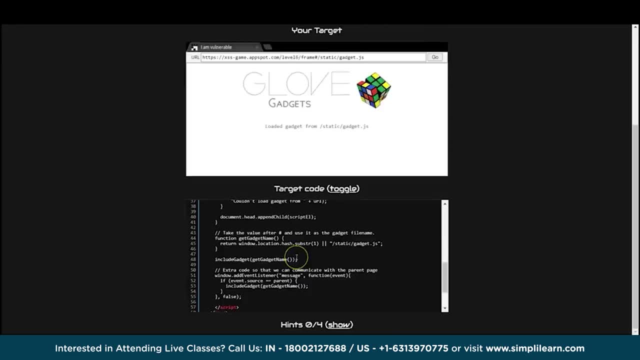 And then in line 48, the value is directly passed on to the includeGadget method And in the includeGadget method that we can see over here- you can see in line 18, a script tag is created and the URL gadget name parameter value is directly used as the source attribute. 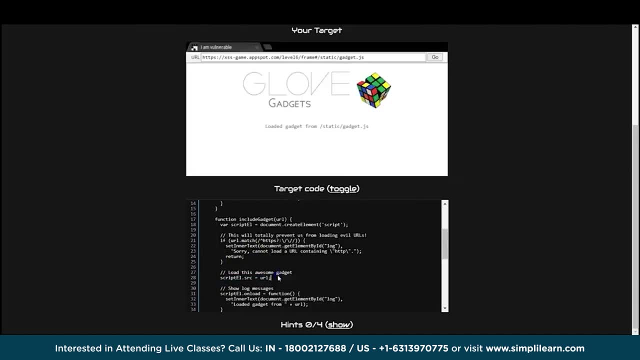 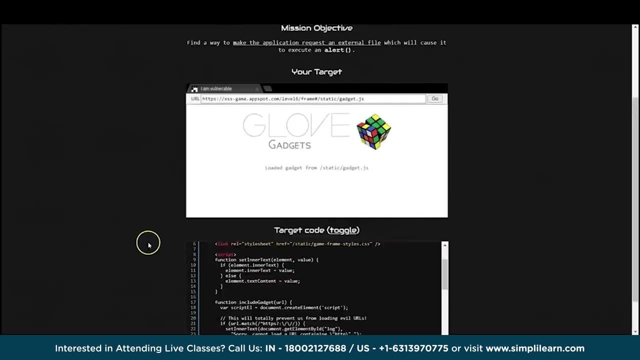 of the script tag in line 48.. This means we can completely control the source attribute of the script tag that is being created. That is, with this vulnerability, we can inject our own JavaScript file into the code. We can inject a URL of our own hosted JavaScript into the web applications URL after the hashtag. 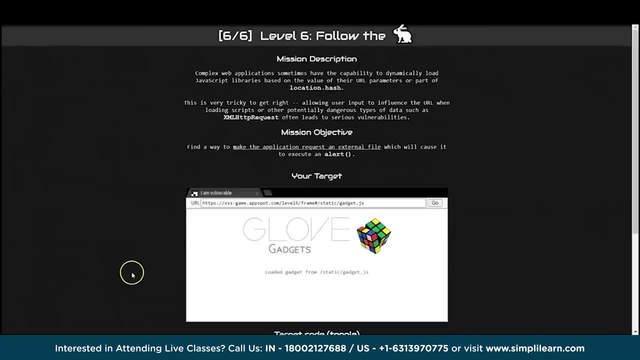 and the URL should not be using HTTPS but anything like that to bypass the regular expression for security checking. Going to remove the pre-stored URL, And we are going to load our own JavaScript file. Finally, we have reached the end of our challenge, completed six different varieties of cross-scripting. 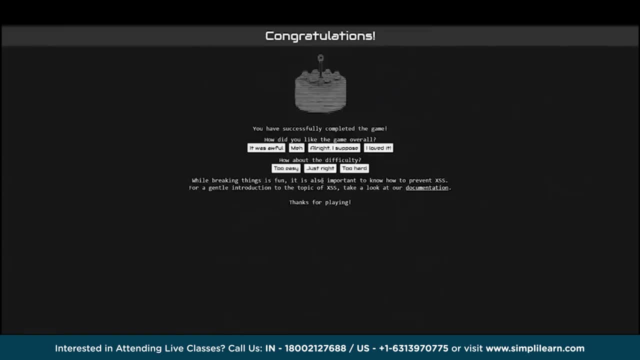 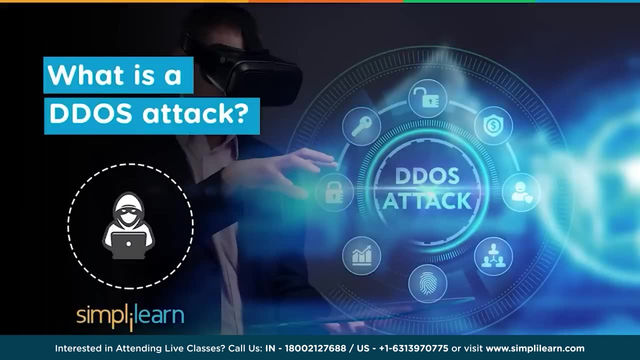 attacks and use different solutions for all of the six questions. With work from home being the norm in today's era, people spend considerable amount of time on the internet, often without specific measures to ensure a secure session. Apart from individuals, organizations worldwide that host data and conduct business over the. 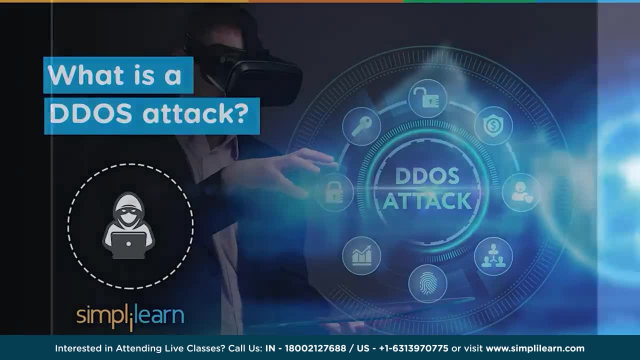 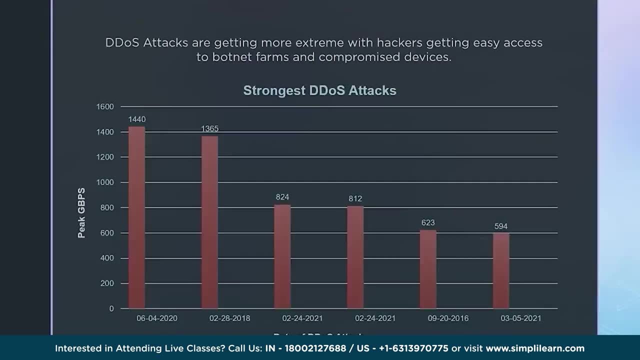 internet, They are always at the risk of a DDoS attack. These DDoS attacks are getting more extreme, with hackers getting easy access to botnet farms and compromised devices. As can be seen in the graph, three of the six strongest DDoS attacks were launched in. 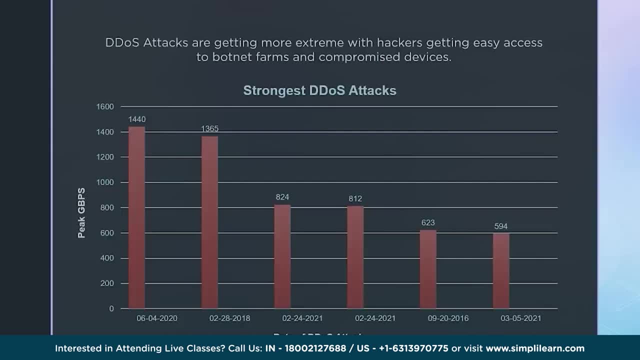 2021, with the most extreme attack occurring just last year in 2020.. Lately, cybercriminals have been actively seeking out new services and protocols for amplifying these DDoS attacks. Active involvement with hacked machines and botnets Allowing further penetration into the consumer space. 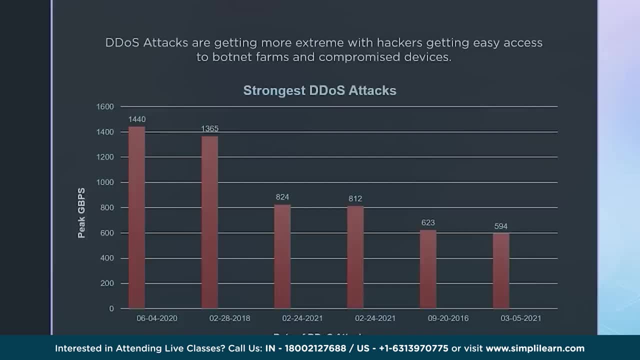 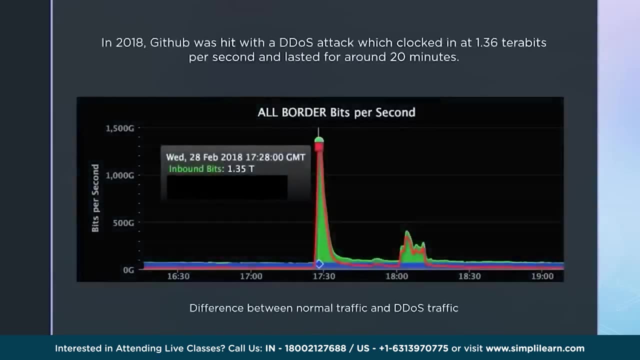 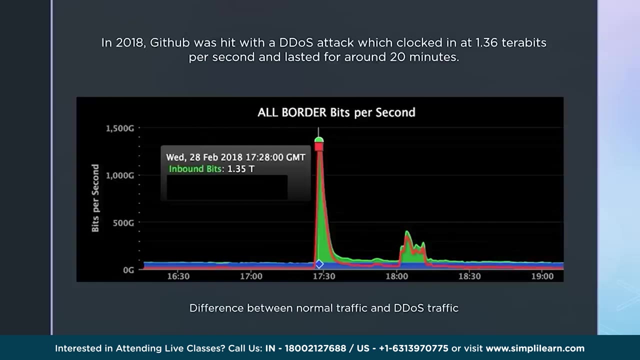 Allowing much more elaborate attack campaigns. Apart from general users, multinational corporations have also had their fair share of problems. GitHub, a platform for software developers, was the target of a DDoS attack in 2018.. Widely suspected to be conducted by Chinese authorities, this attack went on for about 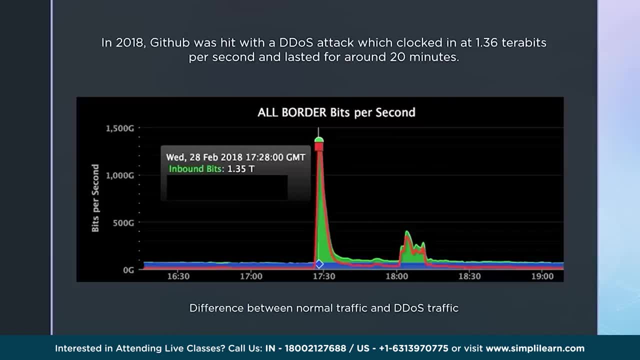 20 minutes, after which the systems were brought into a stable condition. It was the strongest DDoS attack to date at the record And made a lot of companies reconsider the security practices to combat such attacks. Even after years of experimentation, DDoS attacks are still at large and can affect 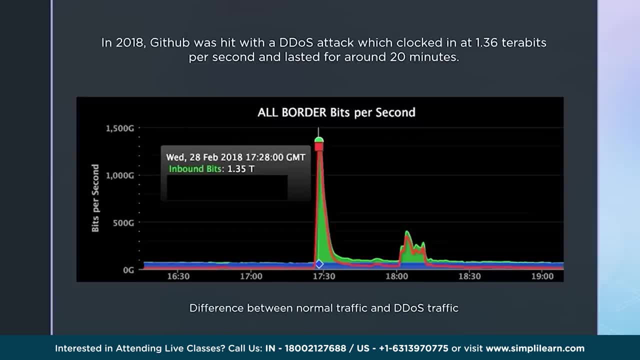 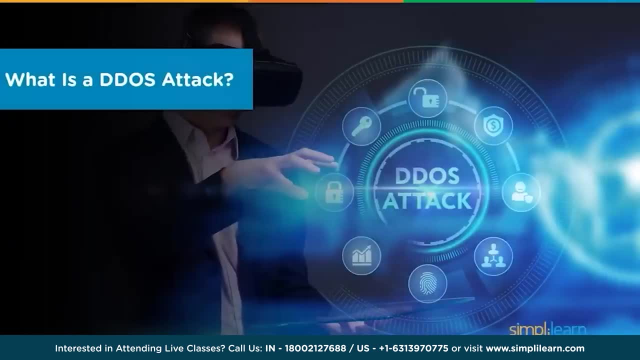 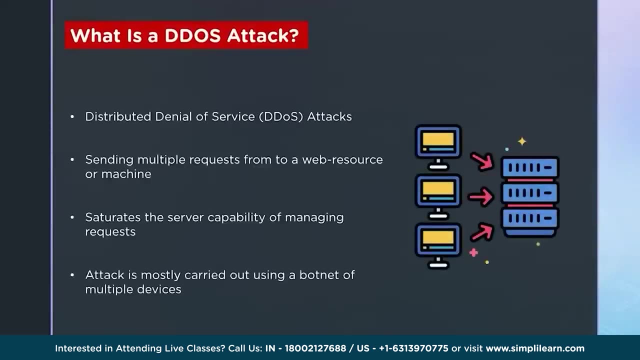 anyone in the consumer and corporate space. Hey everyone, this is Bhavab from Simply Learn, and welcome to this video on what is a DDoS attack. Let's learn more about what is a DDoS attack. A Distributed Denial of Service attack, or DDoS, is when an attacker or attacker who's 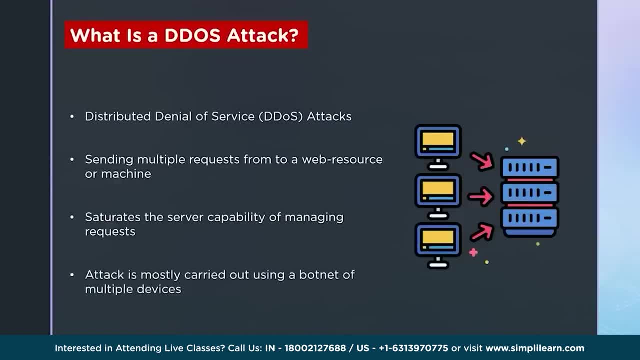 in the system is trying to make it impossible for a service to be delivered. This can be achieved by thwarting access to virtually anything: Servers, devices, services, networks, applications and even specific transactions within applications. In a DDoS attack, it's one system that is sending the malicious data or requests. 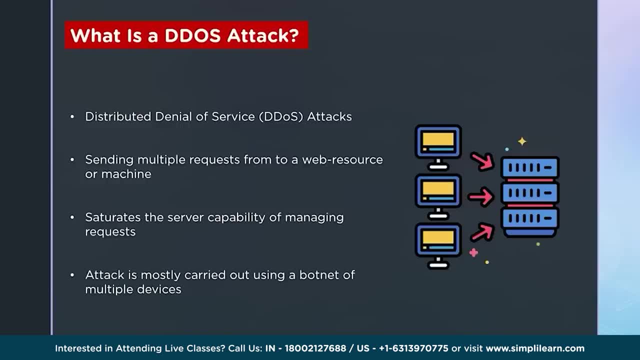 A DDoS attack comes from multiple systems. Generally, these attacks work by drowning a system with requests for data. A server sends so many requests to a server page that it crashes under the demand, or it could be a database being hit with a high volume of queries. 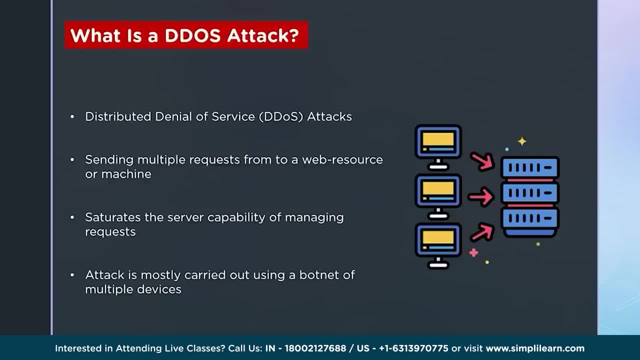 The result is available: internet bandwidth, CPU and RAM capacity become overwhelmed. The impact could range from a minor annoyance from disrupted services to experiencing entire websites, applications or even entire businesses taking offline. More often than not, these attacks are launched using machines in a botnet. 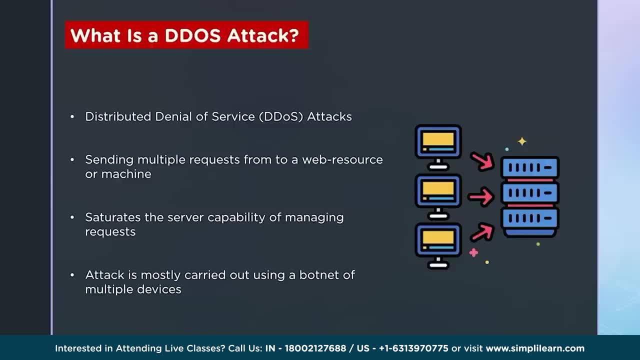 A botnet is a network of devices that can be triggered to send requests from a remote source, often known as the command and control center. The bots in the network attack a particular target, thereby hiding the original perpetrator of the DDoS campaign. 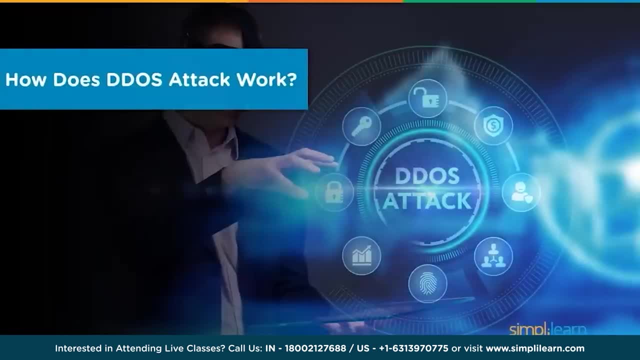 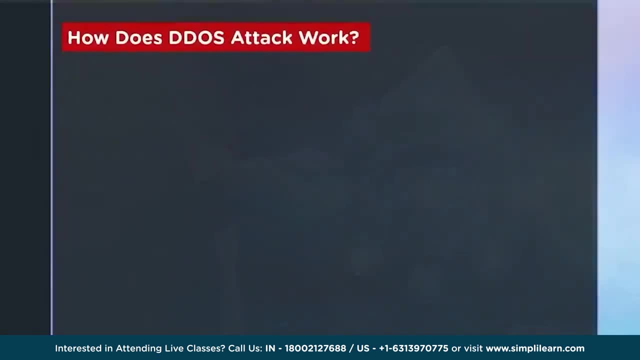 But how do these devices come under a botnet And what are the requests being made to the web servers? Let's learn more about these and how DDoS attack work. A DDoS attack is a two-phase process. In the first phase, a hacker will send a request to the web server. 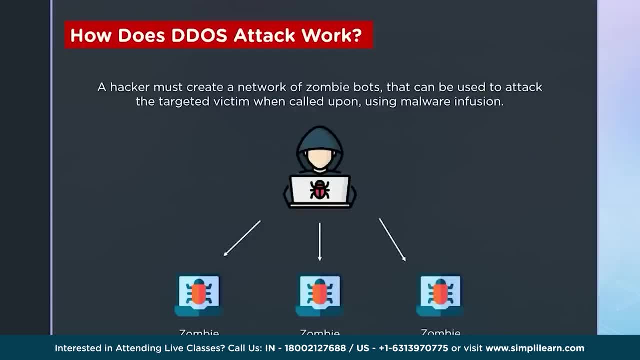 In the second phase, a hacker will send a request to the web server. In the third phase, a hacker will send a request to the web server. In the fourth phase, a hacker will send a request to the web server. The hacker creates a botnet of devices. 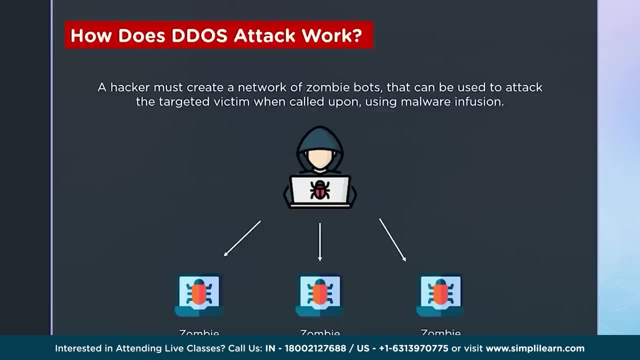 Simply put, a vast network of computers are hacked via malware, ransomware or just simple social engineering. These devices become a part of the botnet, which can be triggered anytime to start bombarding a system or a server on the instruction of the hacker that created the botnet. 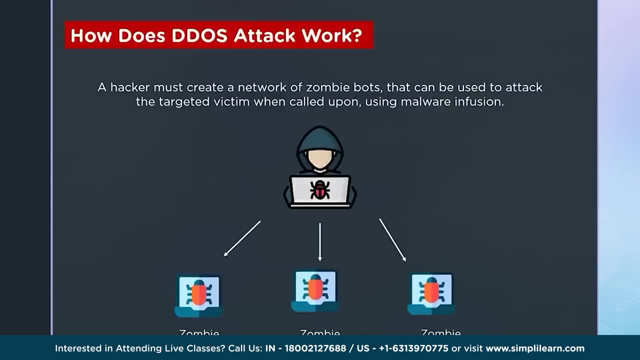 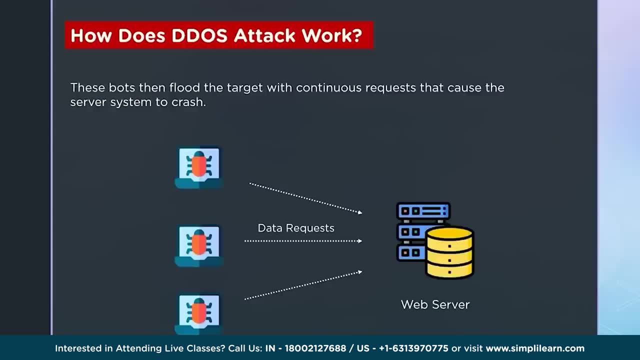 The devices in these networks are called bots or zombies. In the second phase, a particular target is selected for the attack. When the hacker finds the right time to attack, all the zombies in the botnet network, send these requests to the target, thereby taking up all the server's available bandwidth. 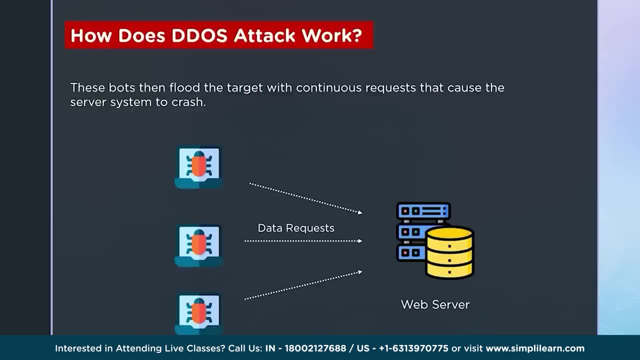 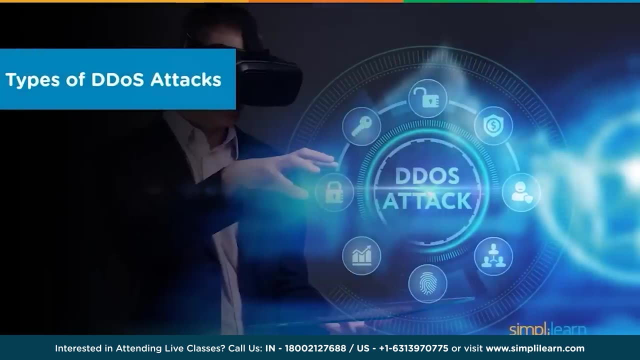 These can be simple ping requests or complex attacks like SYN flooding and UDP flooding. The aim is to overwhelm them with more traffic than the server or the network can accommodate. The goal is to render the website or service inoperable. There is a lot of wiggle room when it comes to the type of DDoS attack. a hacker can go. 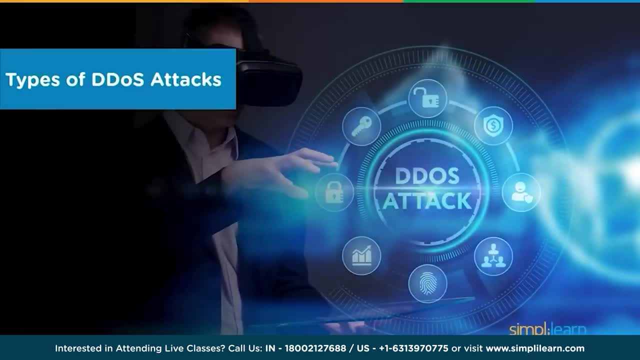 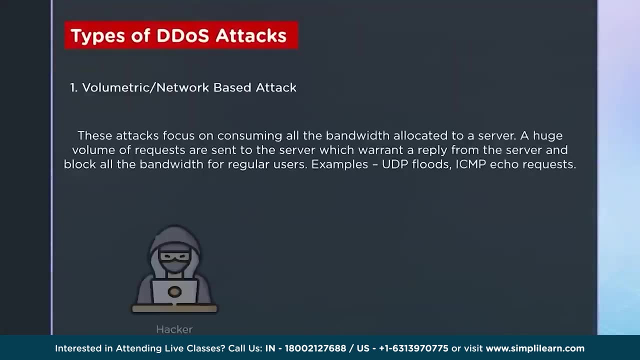 with. Depending on the target's vulnerability, we can choose one of the three broad categories of DDoS attacks. Volume-based attacks use massive amounts of bogus traffic to overwhelm a resource. It can be a website or a server. They include ICMP, UDAP and spoofed packet flood attacks. 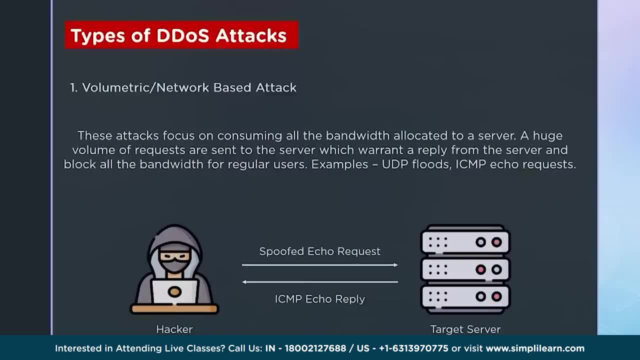 The size of the volume-based attack is measured in bits per second. These attacks focus on clogging all the available bandwidth for the server, thereby cutting the supply short. Several requests are sent to the server, all of which warrant a reply, thereby not. 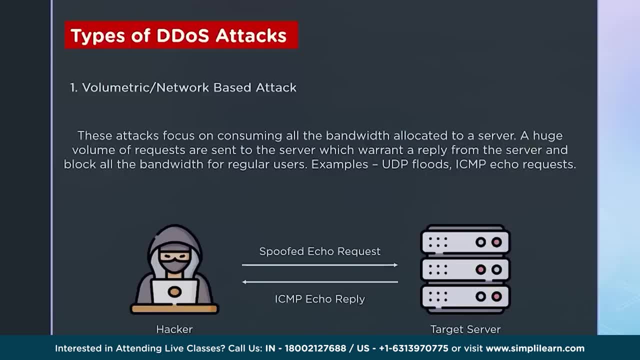 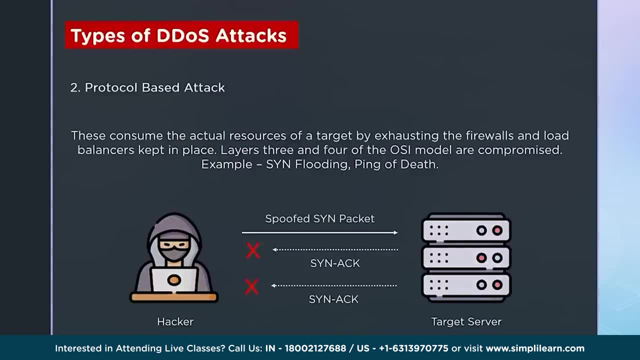 allowing the target to cater to the general legitimate users. Next, we have the protocol-level attacks. These attacks are meant to consume essential resources of the target's server. They exhaust the load balances and firewalls which are meant to protect the system against. 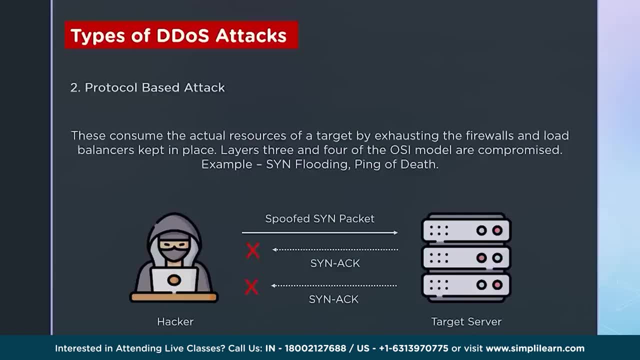 the DDoS attack. These protocol attacks include SYN floods and smurf DDOS, among others, and the size is measured in packets per second. The use of this attack takes about 15 minutes to deal with one of the most important issues in the system. 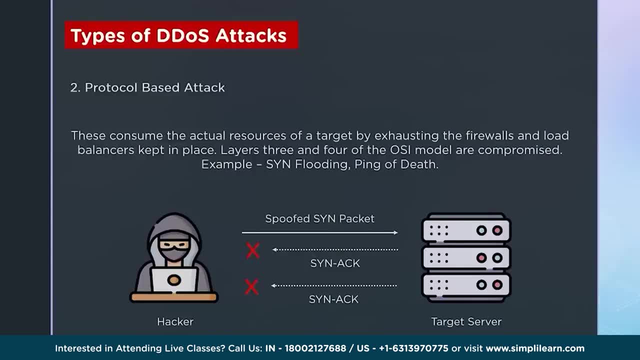 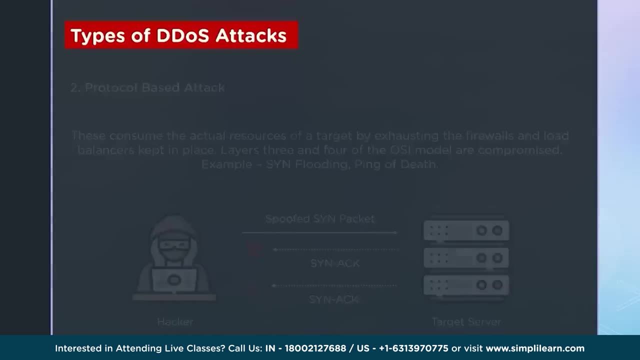 For example, in an SSL handshake server replies to the hello message sent by the hacker, which will be the client in this case, But since the IP is spoofed and leads nowhere, the server gets stuck in an endless loop of sending the acknowledgement without any end in sight. 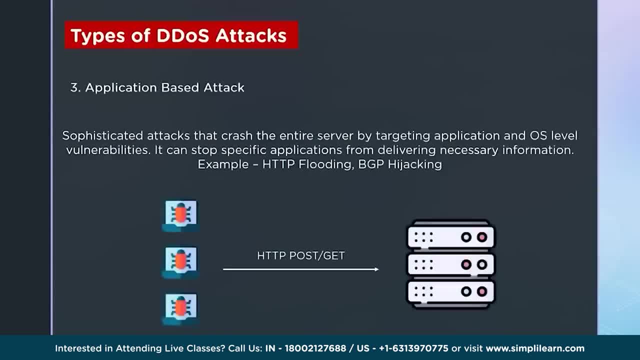 Finally, we have the application level attacks. Application layer attacks are conducted by flooding applications with maliciously crafted requests. The size of application layer attacks is measured in requests per second. These are relatively sophisticated attacks that target the application and operating system level vulnerabilities. 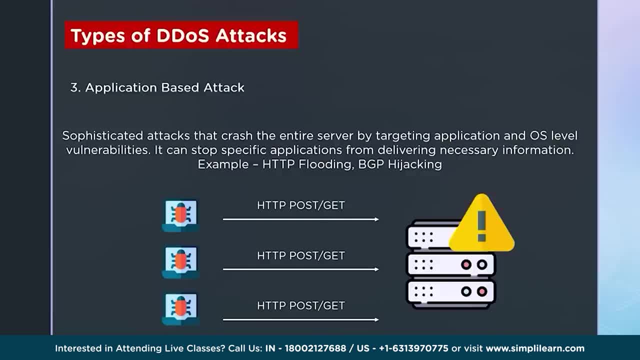 They prevent the specific applications from delivering necessary information to users and hog the network bandwidth up to the point of a system crash. Examples of such an attack are HTTP flooding and BGP hijacking. A single device can request data from a server using HTTP POST or GET without any need for 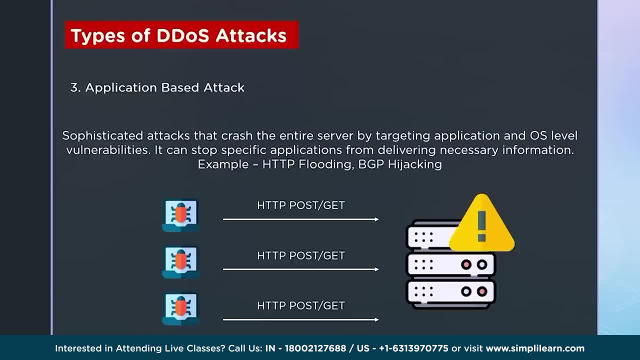 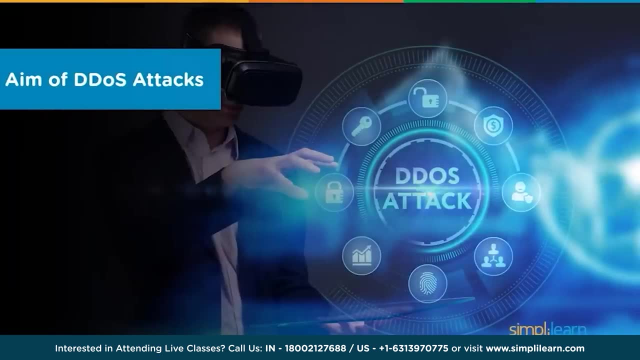 any issues. However, when the requisite botnet is instructed to bombard the server with thousands of requests, the database bandwidth gets jammed and it eventually becomes unresponsive and unusable. But what about the reasons for such an attack? There are multiple lines of thought as to why a hacker decides to launch a DDoS attack. 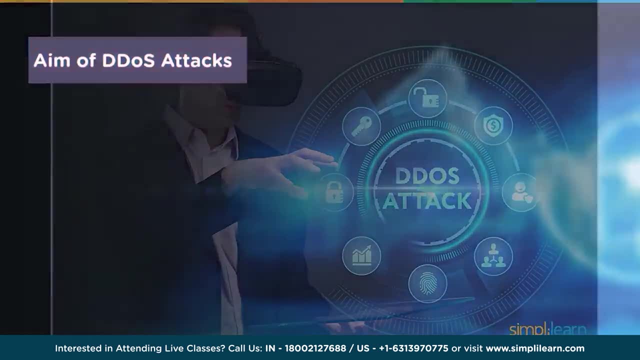 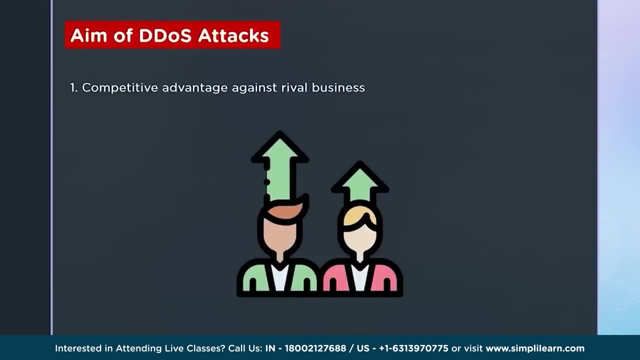 on unsuspecting targets. Let's take a look at a few of them. The first option is to gain a competitive advantage. Many DDoS attacks are competitive. They are conducted by hacking communities against rival groups. Some organizations hire such communities to stagger their rival's resources at a network. 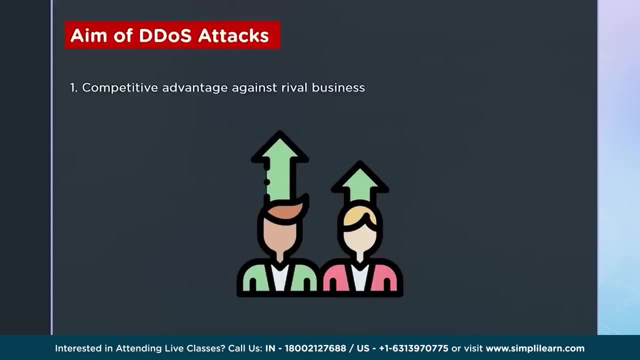 level to gain an advantage in the playing field. Since being a victim of a DDoS attack indicates a lack of security, the reputation of such a company takes a significant hit, allowing their rivals to cover up some ground. Secondly, some hackers launch these DDoS attacks to hold multinational corporations at ransom. 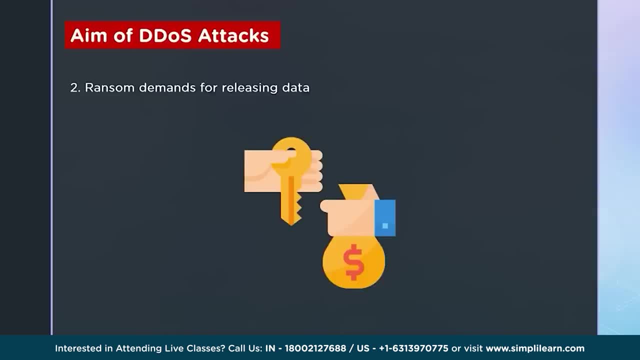 The resources are jammed, And the only way to clear the way is if the target company agrees to pay a designated amount of money to the hackers. Even a few minutes of inactivity is detrimental to a company's reputation in the global market, and it can cause a spiral effect both in terms of market value and product security. 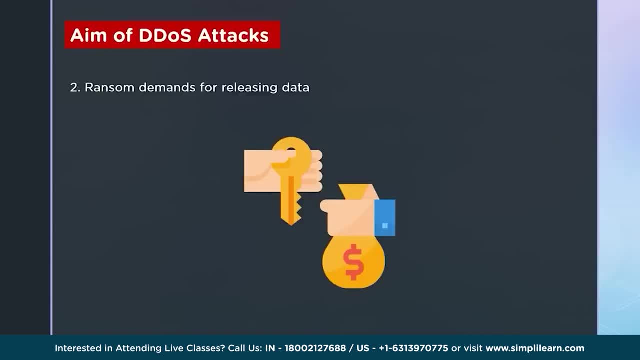 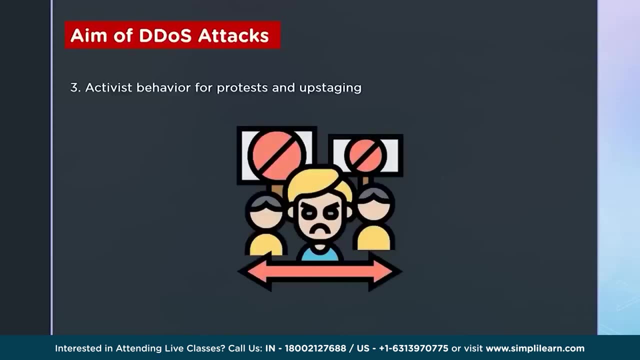 index. Most of the time, a compromise is reached and the resources are freed after a while. DDoS attacks have also found use in the political segment. Certain activists tend to use DDoS attacks to vandalize the market. Some of these attacks have been used in the political segment. 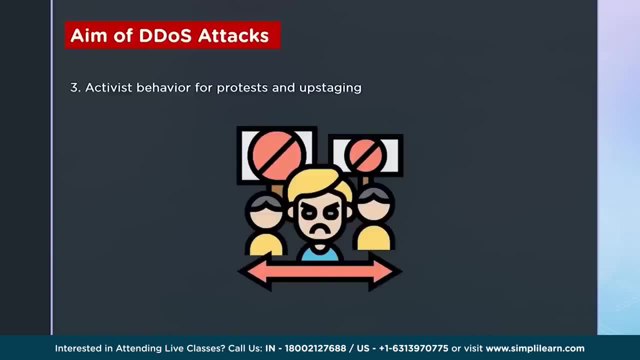 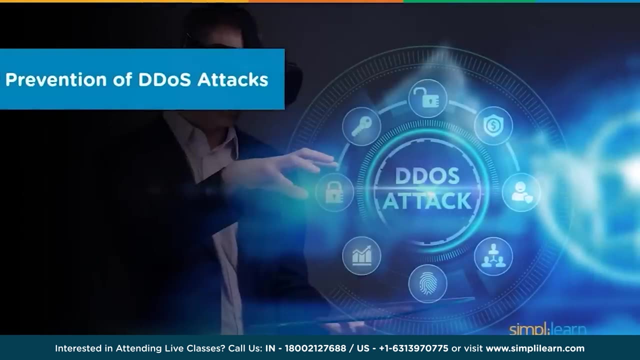 Some of these attacks have been used to voice their opinion. Spreading the word online is much faster than any local rally or forum. Primarily political, these attacks also focus on online communities, ethical dilemmas or even protests against corporations. Let's take a look at a few ways that companies and individuals can protect themselves against. 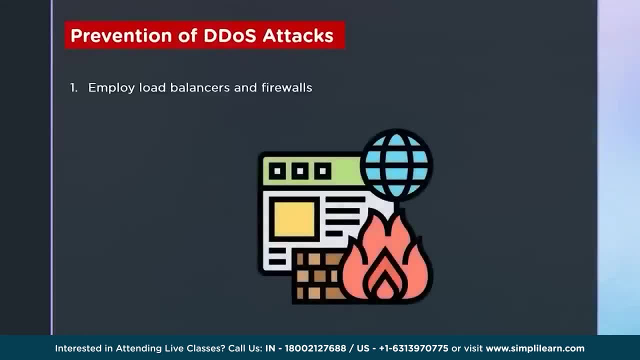 DDoS attacks, The company can employ load balancers and firewalls to help protect the data from such attacks. Load balancers reroute the traffic from one server to another in a DDoS attack. This reduces the single pointer failure and adds resiliency to the server data. 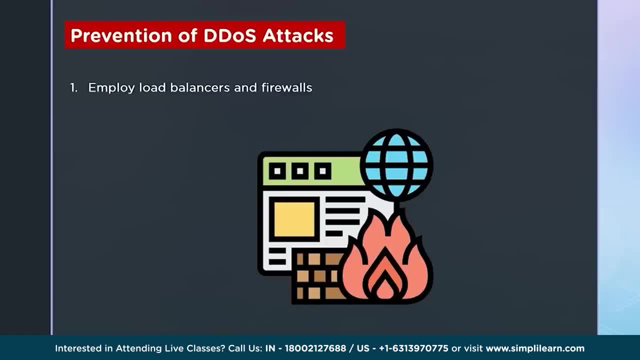 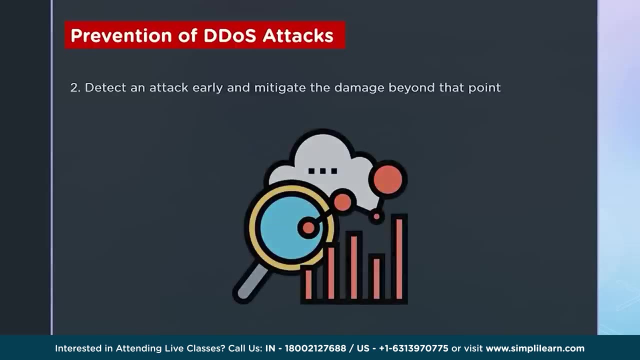 A firewall blocks unwanted traffic into a system and manages the number of requests made at a definite rate. It checks for multiple attacks from a single IP and occasional slowdowns to detect a DDoS attack in action. Early detection of a DDoS attack goes a long way in recovering the data lost in such an 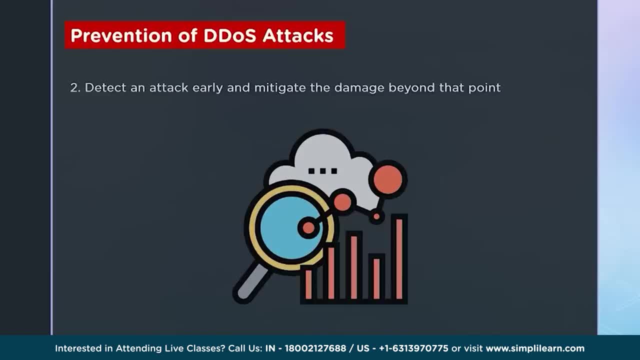 event. Once you've detected the attack, you will have to find a way to respond. For example, you will have to work on dropping the malicious DDoS traffic before it reaches your server, so that it doesn't throttle and exhaust your bandwidth. 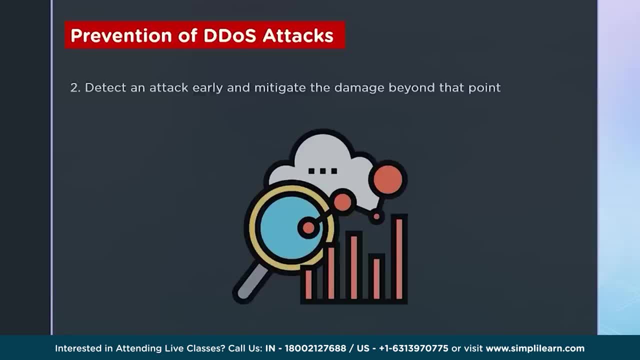 Here's where you will filter the traffic so that only legitimate traffic reaches the server. By intelligent routing, you can break the remaining traffic into manageable chunks that can be handled by your cluster resources. The most important stage in DDoS mitigation is where you will look for patterns of risk. 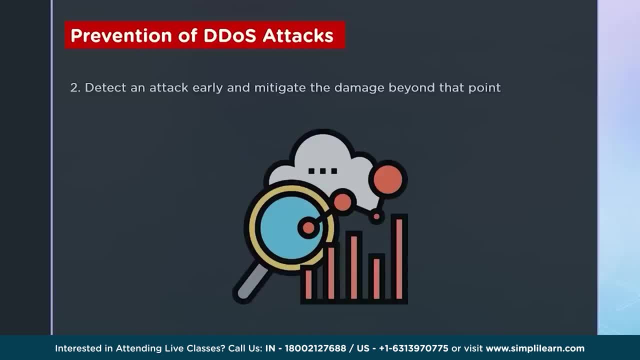 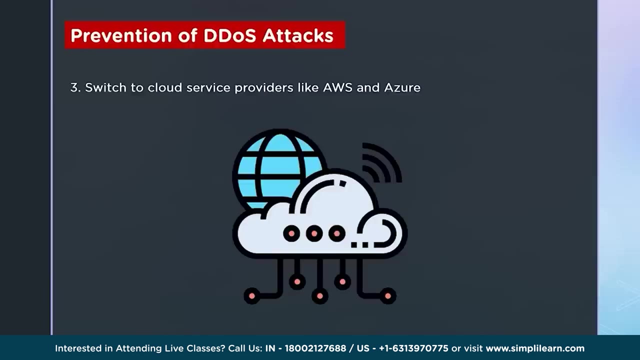 for DDoS attacks and use those to analyze and strengthen your mitigation techniques. For example, blocking an IP that's repeatedly found to be offending is a first step. Cloud providers like Amazon Web Services and Microsoft Azure, who offer high levels of cybersecurity, including firewalls and threat monitoring software, can help protect your. 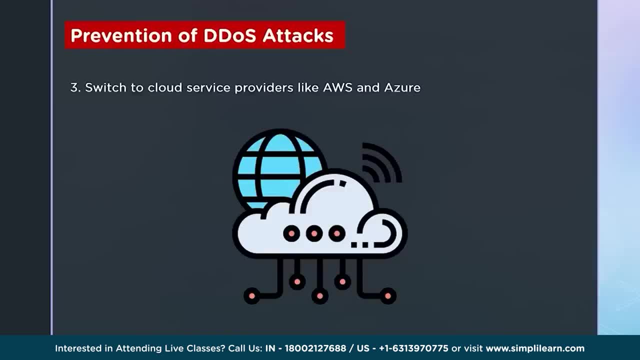 assets and network from DDoS criminals. The cloud also has greater bandwidth than most private networks, so it is likely to fail if under the pressure of a DDoS attack. Additionally, reputable cloud providers offer network redundancy: duplicating copies of your data systems and equipment so that, if your service becomes corrupted or unavailable. 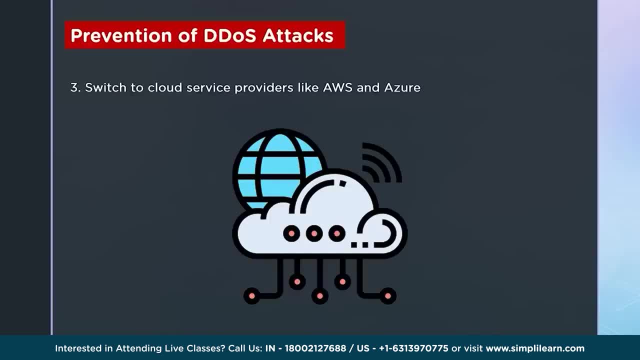 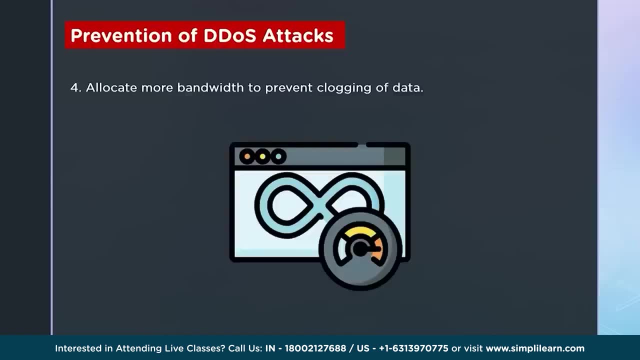 due to a DDoS attack. you can switch to a secure access on backed-up versions without missing a beat. One can also increase the amount of bandwidth available to a host server being targeted, Since DDoS attacks fundamentally operate on the principle of overwhelming systems with 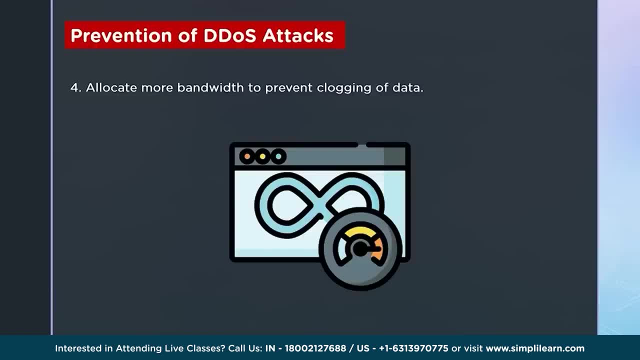 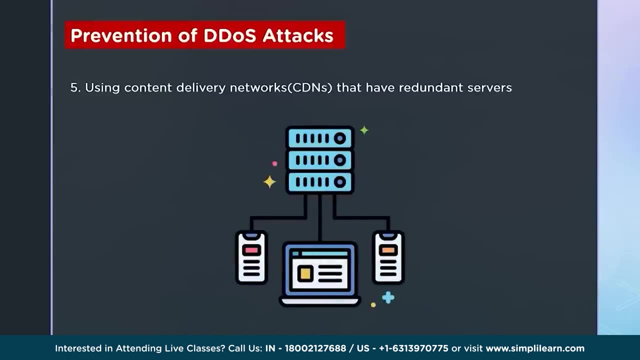 heavy traffic. simply provisioning extra bandwidth to handle unexpected traffic spikes can provide a measure of protection. This solution can prove expensive, as a lot of that bandwidth is going to go unused most of the time. A Content Delivery Network, or a CDN, distributes your content and boosts performance by minimizing 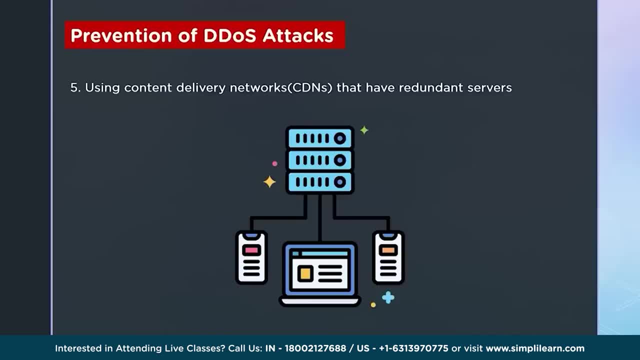 the distance between your resources and end users. It stores the cached version of your content in multiple locations and this eventually reduces the risk of DDoS attacks by avoiding a single point of failure when the attacker is trying to focus on a single target. 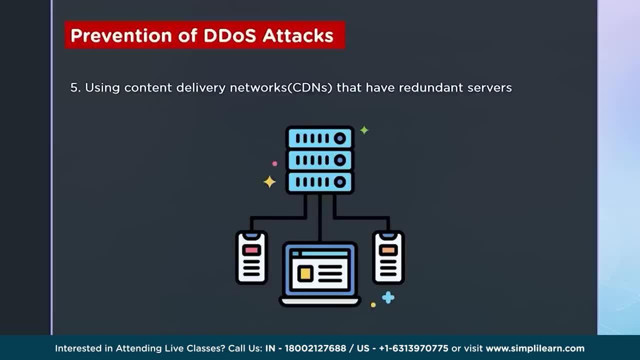 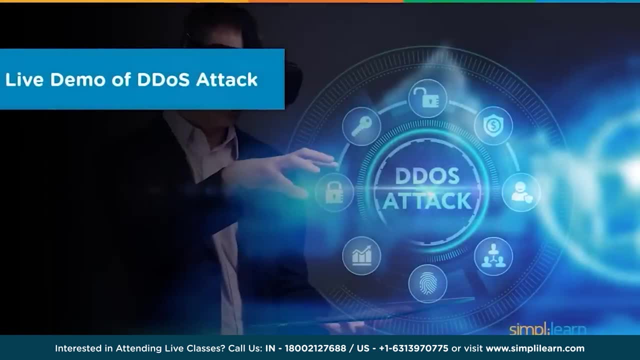 Popular CDNs include Akamai, CDN, Cloudflare, AWS, CloudFront, etc. Let's start with our demo regarding the effects of DDoS attacks on a system. For our demo, we have a single device that will attack a target, making it a DDoS attack. 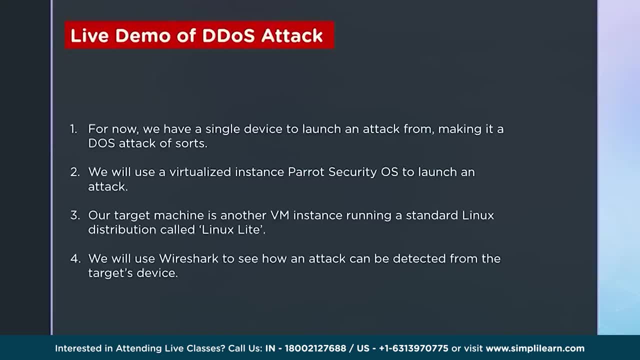 of sorts. Once a botnet is ready, multiple devices can do the same and eventually emulate a DDoS attack. To do so we will use the virtualization software called VMware. with an instance of Parag Security operating system running For a target machine, we will be running another VMware instance of a standard Linux distribution. 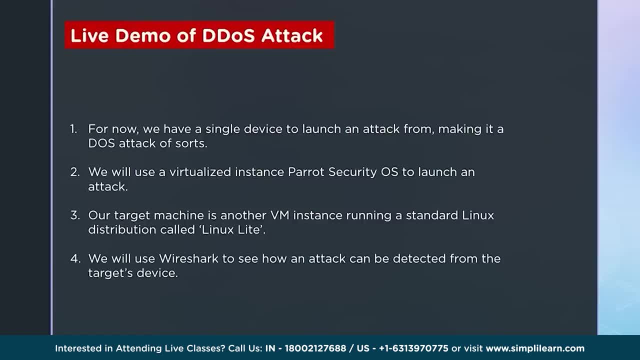 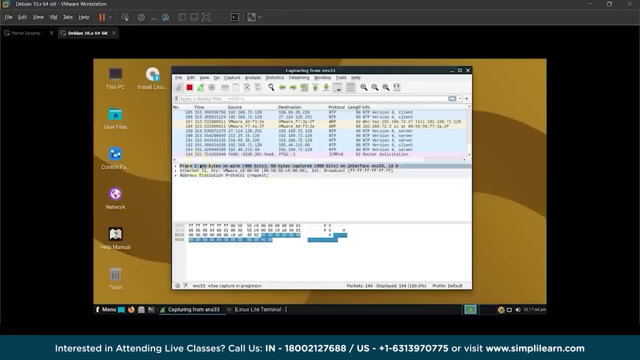 known as Linux Lite. In a target device, we can use Wireshark to determine when the attack begins and see the effects of the attack accordingly. This is Linux Lite, which is our target machine, And this is Parag Security, which is our target machine. 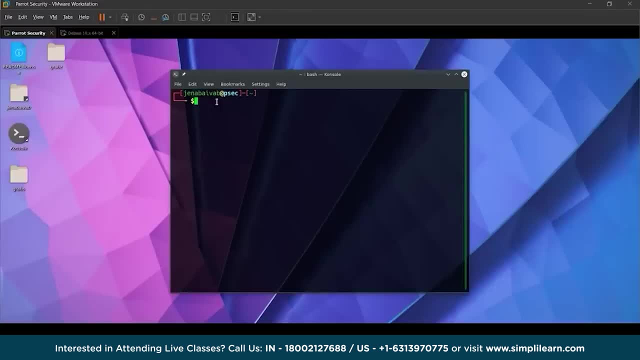 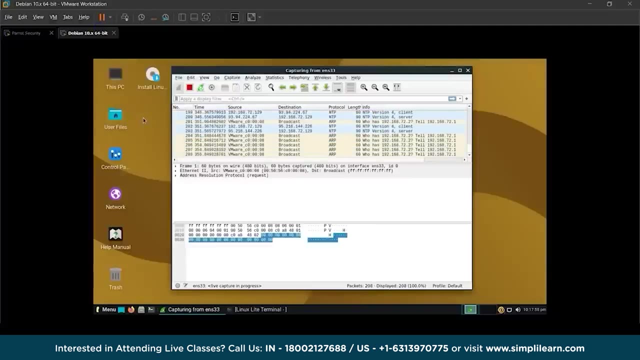 And this is Parag Security, which is used by the hacker when trying to launch a DDoS attack. This is just one of the distros that can be used To launch the attack. we must first find the IP address of our target. 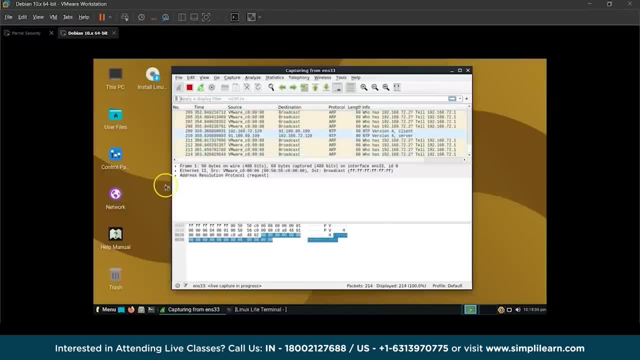 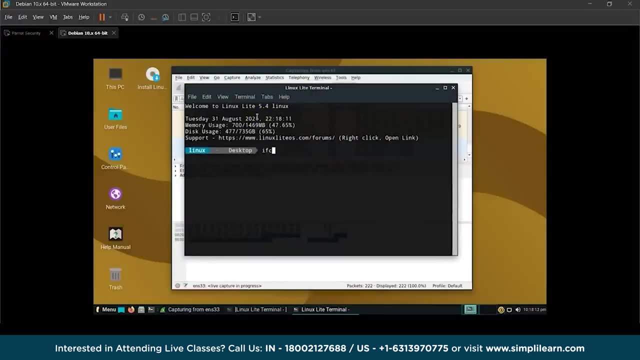 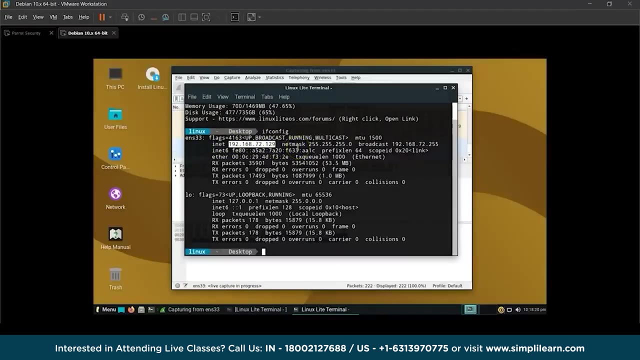 So to find the IP address, we open the terminal, we use the command ifconfig and here we can find the IP address. Now, remember, we are launching this attack in VMware. Now both the instances of Parag Security and Linux Lite are being run on my local network. 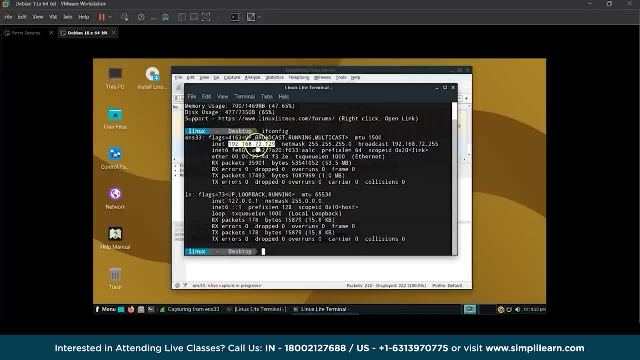 So the address that you can see here is 192.168.72.129,, which is a private address. This IP cannot be accessed from outside the network- basically anyone who is not connected to my Wi-Fi. When launching attacks with public servers or public addresses, 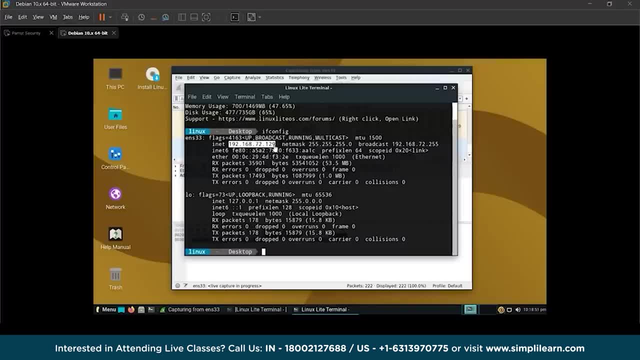 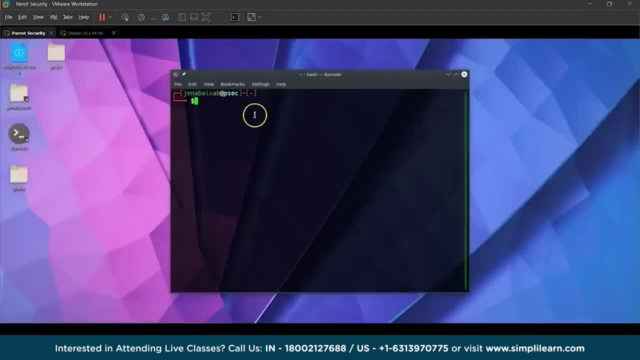 It will have a public IP address that does not belong to the 192.168 subnet. Once we have the IP address, we can use a tool called HPING3.. HPING3 is an open source packet generator and analyzer for the TCP IP protocol. 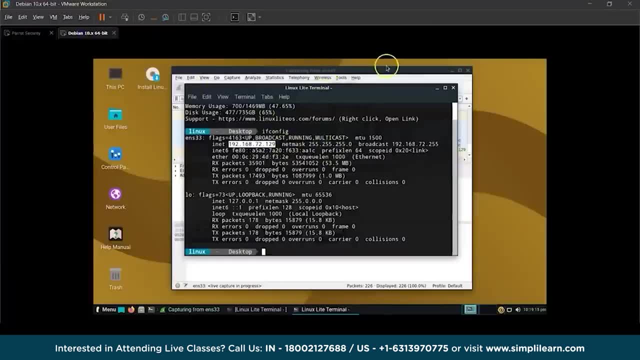 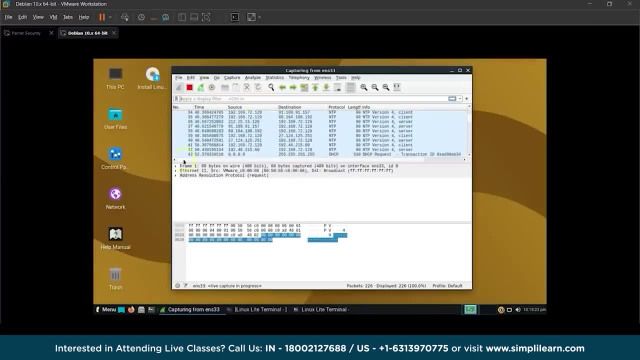 To check what are the effects of an attack, we will be using Wireshark. We can see whatever traffic that is passing through. the Linux Lite distro is being displayed over here with the IP address, the source IP and the destination IP as to where the 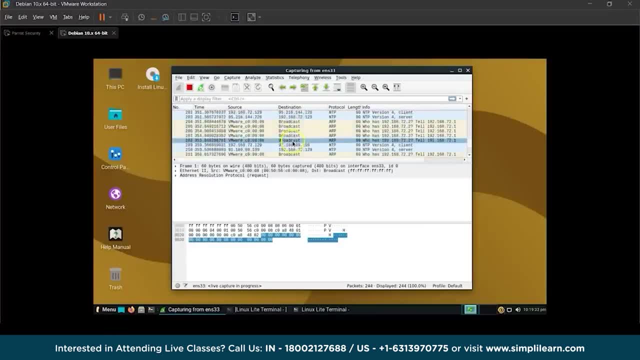 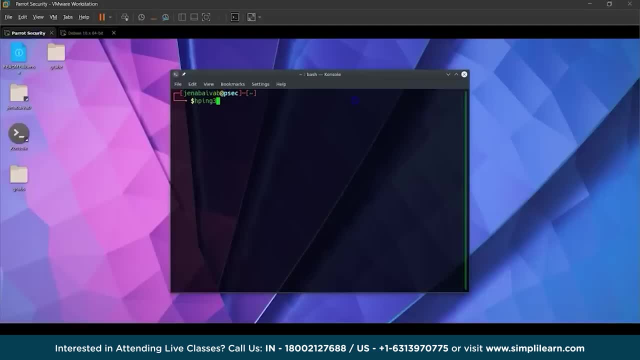 request is being transferred to. Once we have the DOS attack launched, you can see the results coming over here from the source IP, which will be Parag Security. Now, to launch the HPING3 command, we need to give sudo access to the console, which 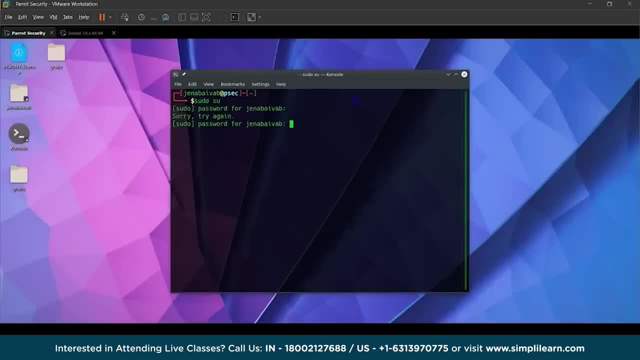 is the root access. Now we have the root access for the console, The HPING3 command will have a few arguments to go with it, which are, as you can see on the screen, minus s and a flood, a hyphen v, hyphen p18 and the IP address of the target. 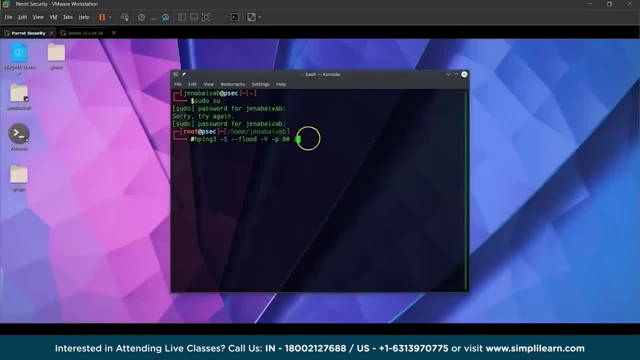 which is 192.168.72.129.. In this command we have a few arguments, such as the minus s, which specifies syn packets. Like in an SSL handshake, we have the syn request that the client sends to the server to initiate a connection. 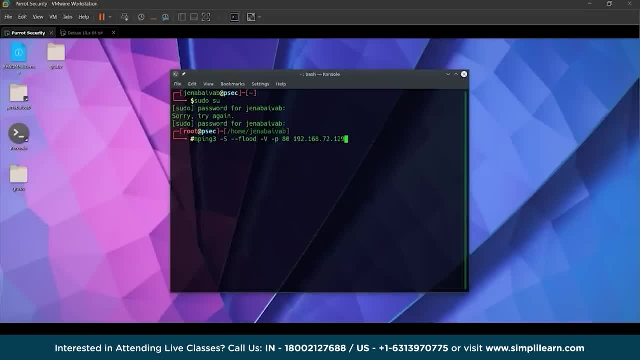 The hyphen flood aims to ignore the replies that the server will send back to the client in response to the syn packets. Here the Parag Security OS is the client and Linux Lite being the server. Minus v stands for verbosity, as in where we will see some output when the requests. 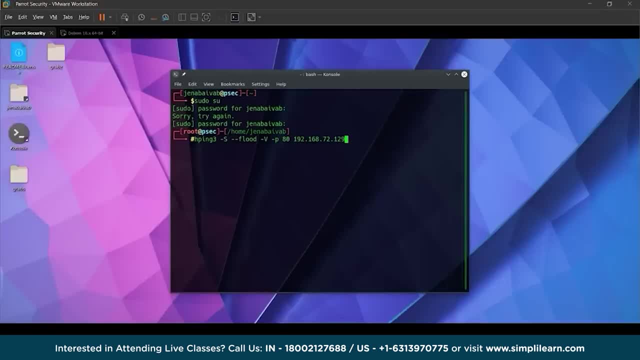 are being sent. The hyphen p80 stands for port 80, which we can replace the port number if we want to attack a different port. And finally, we have the IP address of our target. As of right now. if we check wireshark, we can see that the IP address of our target. 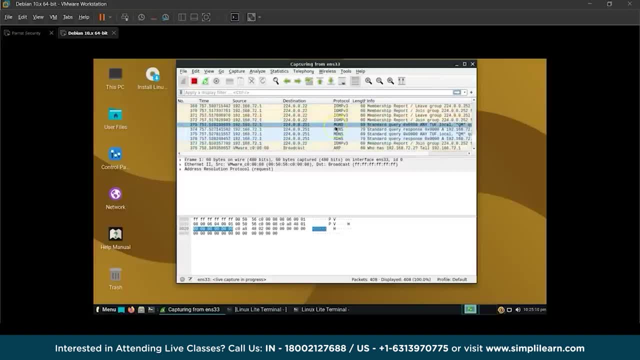 is 192.168.72.129.72.. It is relatively clear and there is no indication of a DDoS attack incoming Now. once we launch the attack over here, we can see the requests coming in from this IP, which is 192.168.72.128.. 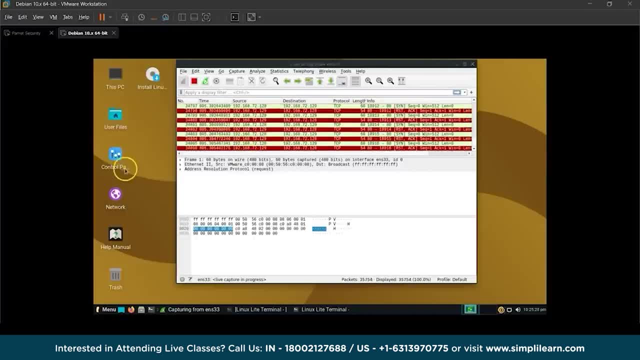 Till now, even if the network is responsive, and so is Linux Lite, the requests keep on coming. For example, we can see the HTTP flooding has started in flood mode. After a few seconds of this attack continuing, the server will start shutting down. 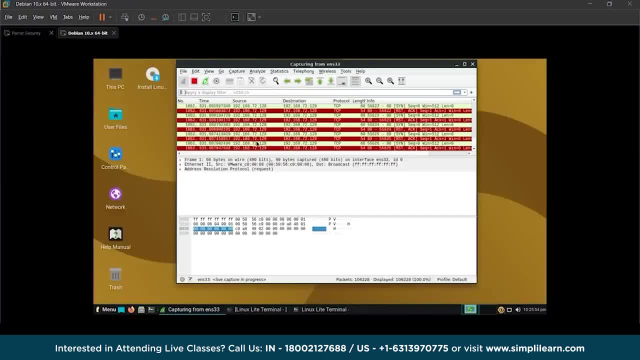 Now remember, Linux Lite is a distro that can focus on. that serves as a backend. Now remember, Linux Lite is a distro and such Linux distros are served as backend to many servers across the world, For example. a few seconds have passed. 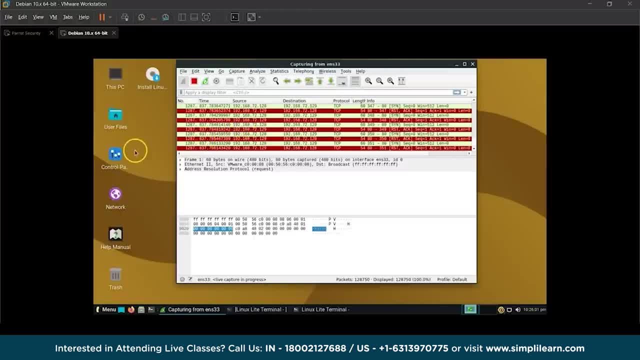 Now the system has become completely responsive. This has happened due to the huge number of requests that came from the security. You can see: whatever I press, nothing is responded. Even the wireshark has stopped capturing new requests because the CPU usage right now. 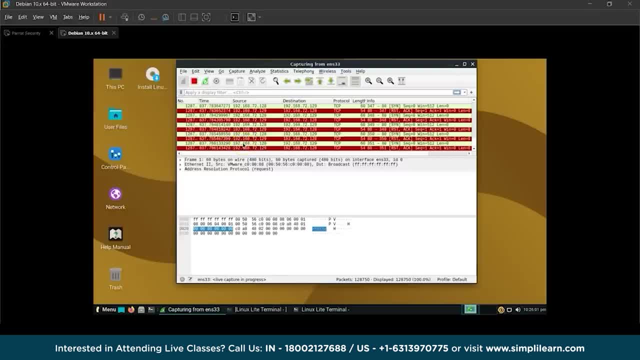 is completely 100% and at this point of time, anyone who is trying to request some information from this Linux distro or where this Linux distro is being used as a backend for a server or a database, cannot access anything else. 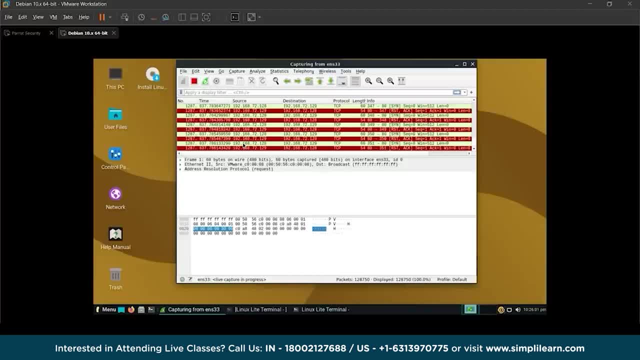 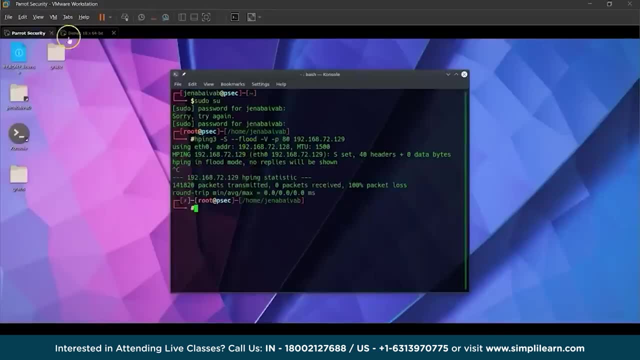 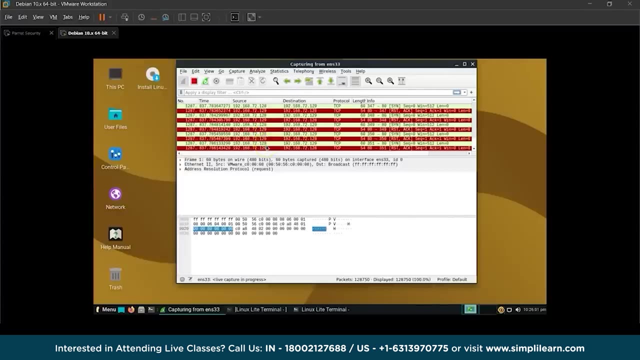 The system has completely stopped responding and any request, any legitimate request from legitimate users, will be dropped Once you stop the attack over here. it takes a bit of time to settle down Now. remember it's still out of control, but eventually the traffic dies down and the system regains its strength. It is relatively easy to gauge right now the effect of a DOS attack. Now remember This: Linux Lite is just a VM instance- Actual website servers and web databases. they have much more bandwidth and are very secure and it is tough to break into. 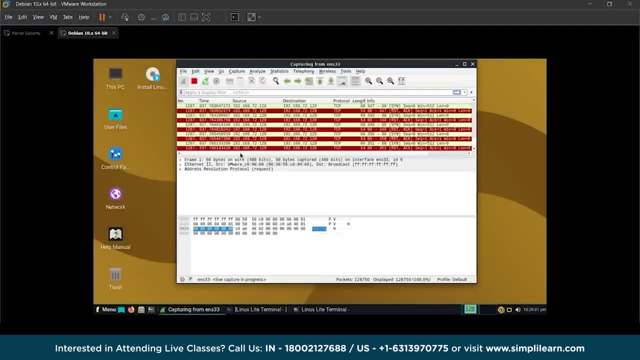 That is why we cannot use a single machine to break into them. That is where a DDoS attack comes into play. What we did right now is a DOS attack, as in a single system, is being used to penetrate a target server using a single request. 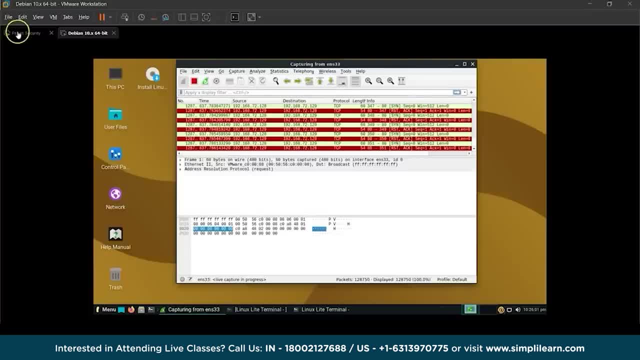 Now, When a DDoS attack, We need to be very careful. It is easy to lose our control over this system, And that's the reason why we use it. So remember multiple systems, such as multiple parallel security instances or multiple zombies. 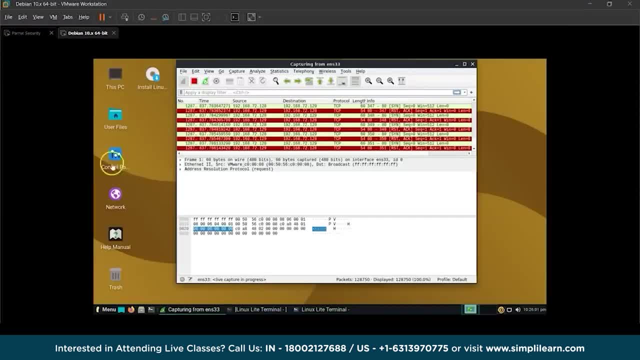 or bots in a botnet network can attack a target server to completely shut down the machine and drop any legitimate request, thereby rendering the service and the target completely unusable and inoperable. As a final note, we would like to remind that this is for educational purposes only, and 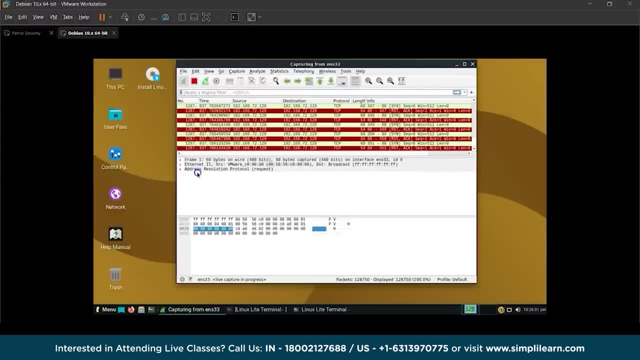 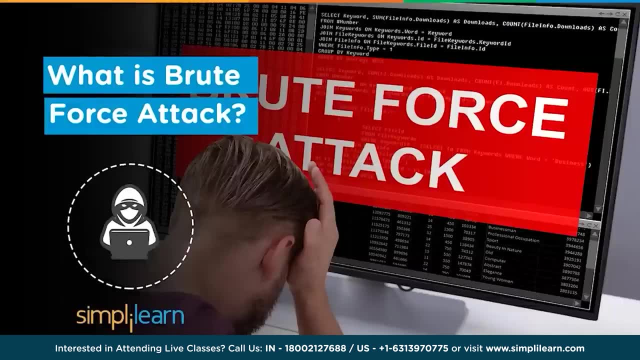 we do not endorse any attacks on any one domains. Only test this: servers and networks that you have permission to test on. Cybersecurity has become one of the most rigid industries in the last decade, while simultaneously being the most challenged With every aspect of corporate culture going online and embracing cloud computing there. 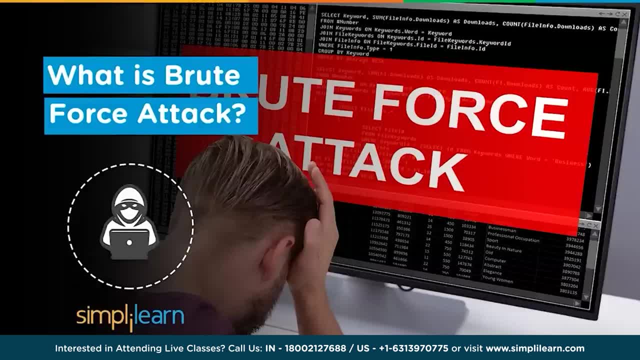 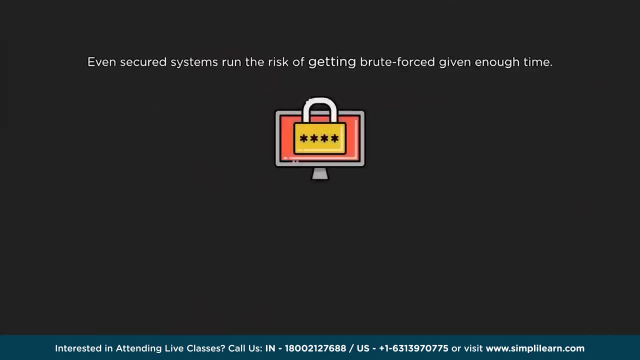 is a plethora of critical data circulating through the internet, all worth billions of dollars to the right person. Increasing benefits require more complex attacks, and one of these attacks is a brute force attack. A brute force, or known as brute force cracking, is the cyber attack equivalent of trying every 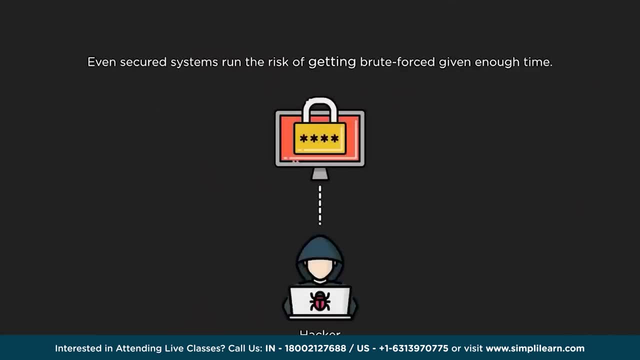 key on your keyring and eventually finding the right one. Brute force attacks are simple and reliable. There is no prior knowledge needed about the victim to start an attack. Most of the systems falling prey to brute force attacks are actually well secured Attackers. let a computer do the work, that is, trying different combinations of usernames. 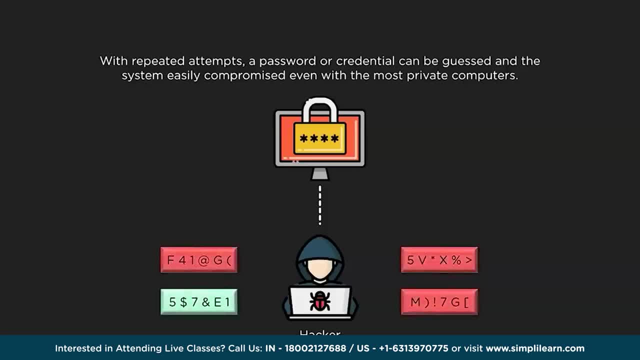 and passwords until they find the one that works. Due to this repeated trial and error for the system, the system is now able to execute all the tasks that it needs to do In the same format. the strength of password matters a great deal. 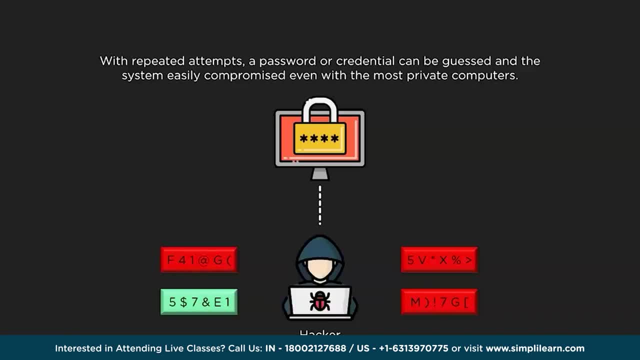 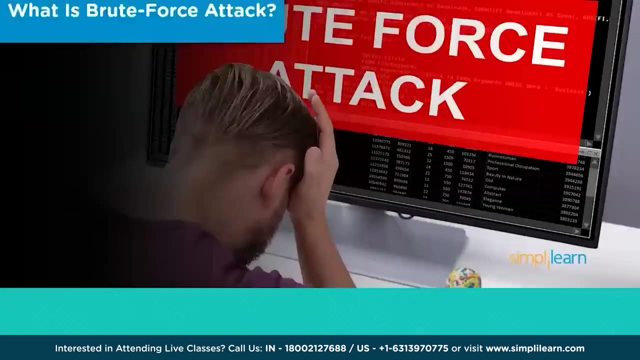 Although, with enough time and resources, brute force will break a system, since they run multiple combinations until they find the right passcode. Hey everyone, this is Bhavab from Simply Learn, and welcome to this video on what is a brute force attack. Let's begin with learning about brute force attacks in detail. 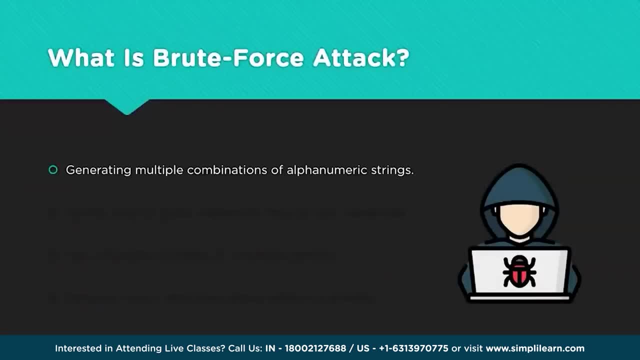 A brute force attack, also known as an exhaustive search, is a cryptographic hack that relies on guessing passable combinations of target attacks. It can be used to break into online accounts, encrypted documents or even network peripheral devices. The longer the password, the more combinations that will need to be tested. 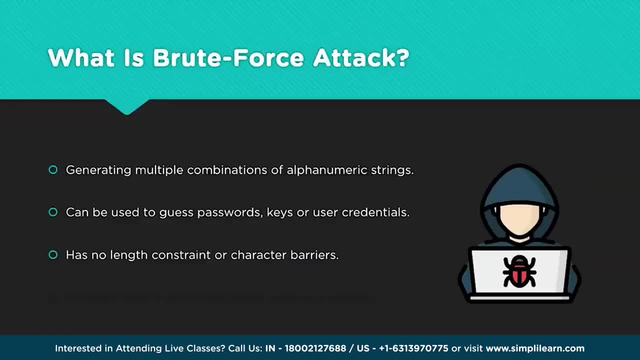 A brute force attack can be time consuming and difficult to perform if methods such as data obfuscation are used, and, at times, downright impossible. However, if the password is weak, it could merely take seconds with hardly any effort. Dictionary attacks are a very common method to use. 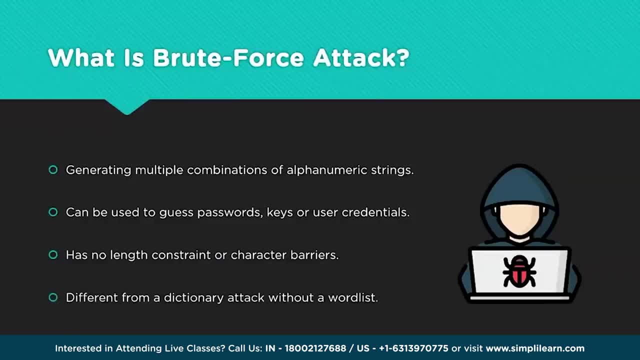 They can be used in multiple ways. They are an alternative to brute force attacks, where the attacker already has a list of usernames and passwords that need to be tested against the target. It doesn't need to create any other combinations on its own. Dictionary attacks are much more reliable than brute force in a real-world context. 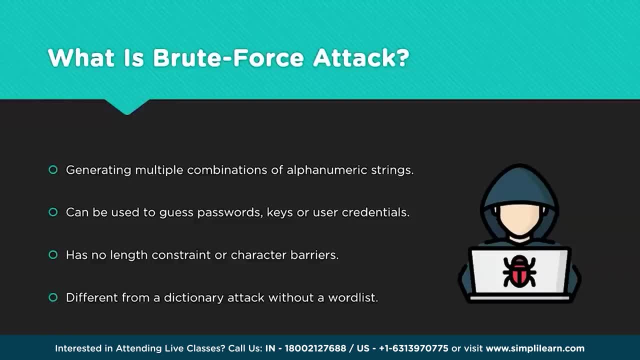 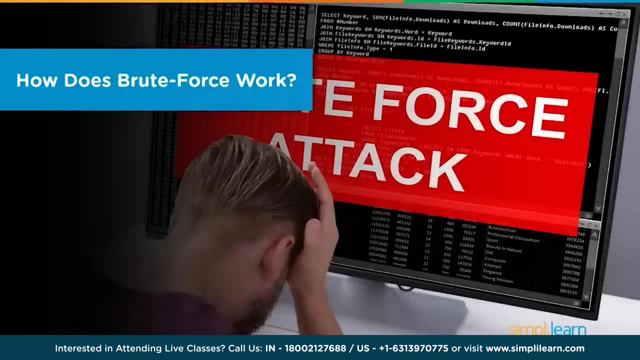 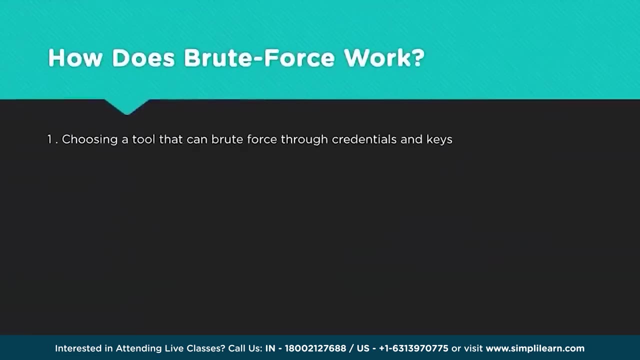 but the usefulness depends entirely on the strength of passwords being used by the general population. There is a three-step process when it comes to brute forcing a system. Let's learn about each of them in detail. Let's start with brute force. In step 1, we have to settle on a tool that we are going to use for brute forcing. 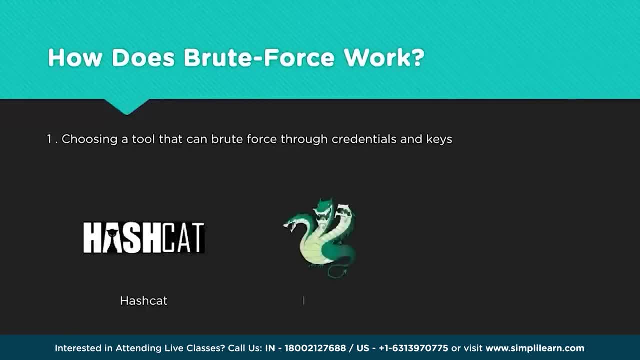 There are some popular names on the market, like Hashcat, Hydra and John the Ripper. While each of them has its own strengths and weaknesses, each of them perform well with the right configuration. All of these tools come pre-installed with certain Linux distributions that cater to. 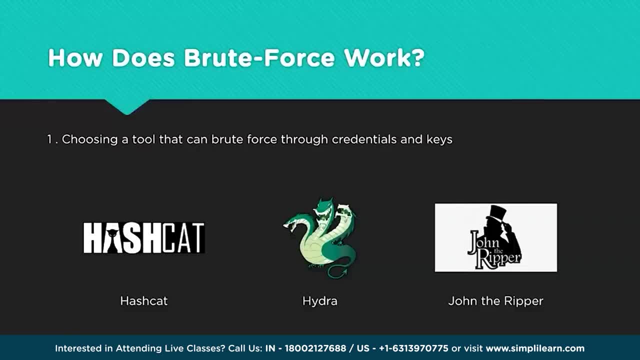 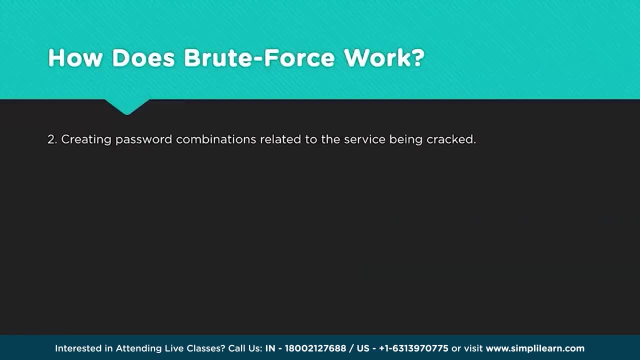 penetration testers and cybersecurity analysts like Kali Linux and Parrot Security. After deciding what tool to use, we can start generating combinations of alphanumeric variables whose only limitation is the number of characters. For example, while using Hydra, a single six-digit password will create 900,000 passwords with 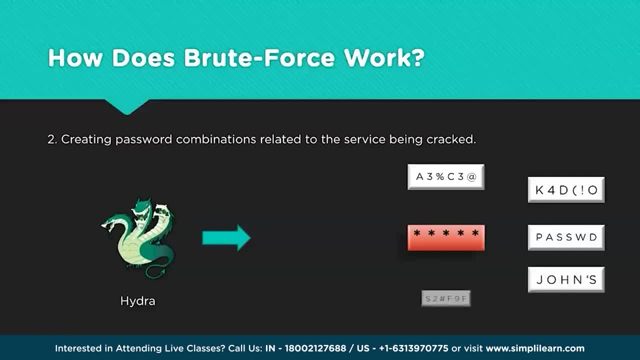 only digits involved. Add alphabets and symbols to that sample space and that number grows exponentially. The popular tools allow customizing this process. Let's say the hacker is aware of the password being a specific image. Let's say the hacker is aware of the password being a specific eight-digit word containing 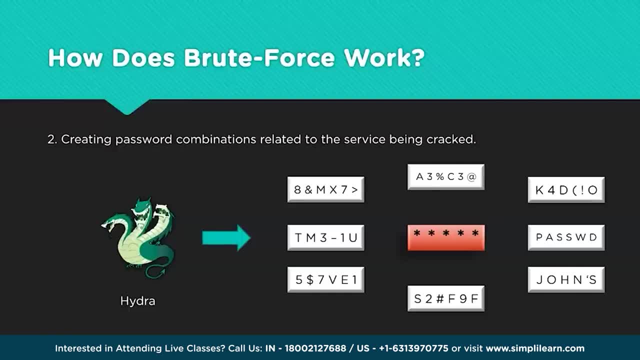 only letters and symbols. This will substantially increase the chances of being able to guess the right password. since we remove the time taken to generate the longer ones, We omit the need for including digits in such combinations. These small tweaks go a long way in organizing an efficient brute force attack, since running 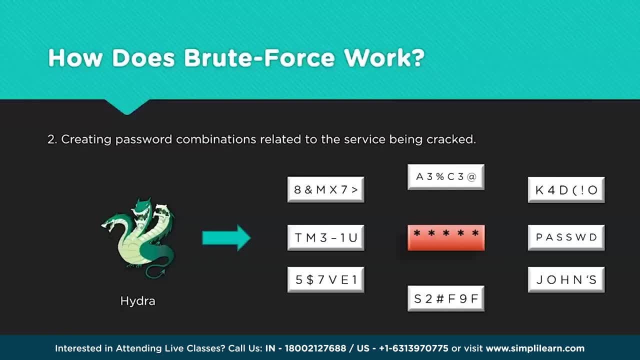 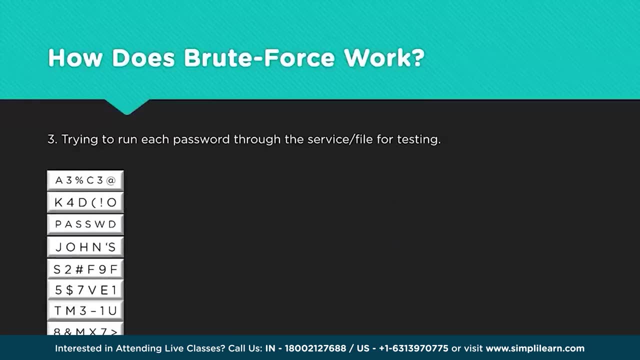 all the combinations with no filters will dramatically reduce the odds of finding the right credentials in time. In the final step, We can try and break into a specific encrypted document, a social media account or even devices at home that connect to the internet. 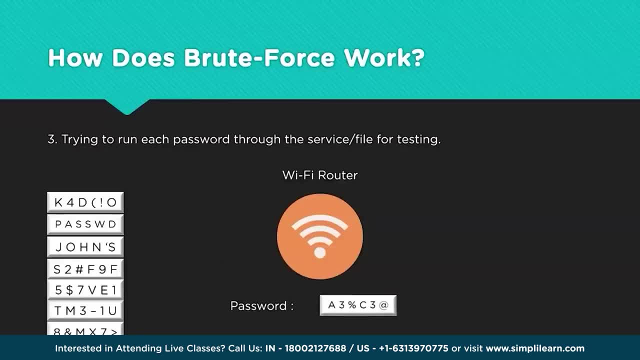 The generated passwords are then fed into the connection, one after the other. It is a long and arduous process, but the work is left to the computer, other than someone manually clicking and checking each of these passcodes. Any password that doesn't unlock the router is discarded and the brute force tool is. 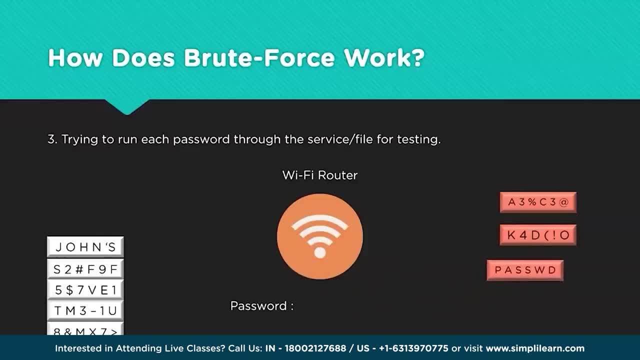 simply moved on to the next one. This keeps going on until we find the right combination which unlocks the router. Sometimes, reaching the success stage takes days and weeks, which makes it cumbersome for people with low computing power at their disposal. However, the ability to crack any system in the world purely due to bad password habits, 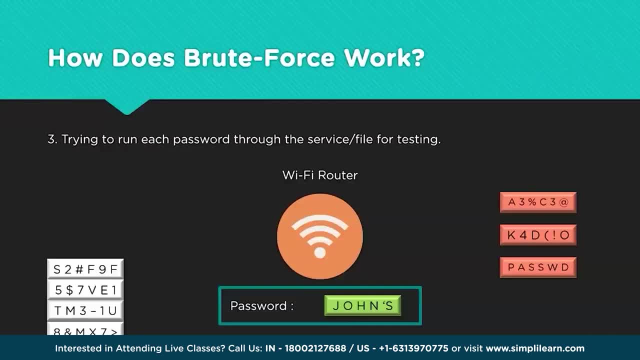 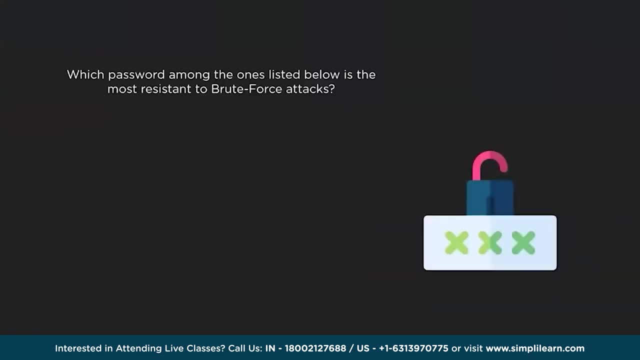 is very appealing, and the general public tends to stick with simple and easy to use passwords. Now let's look at the next step: 1.. Now that we have a fair idea about how brute force works, let's see if we can answer. 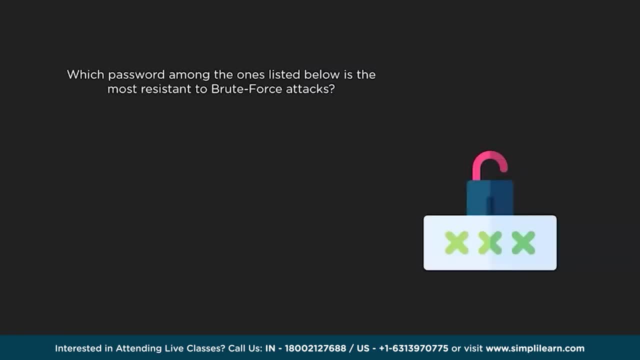 this question, We learnt about how complex passwords are tougher to crack by brute force. Among the ones listed on the screens, which one do you believe will take the longest to be broken when using brute force tools? Leave your answers in the comment section and we will get back to you with the correct. 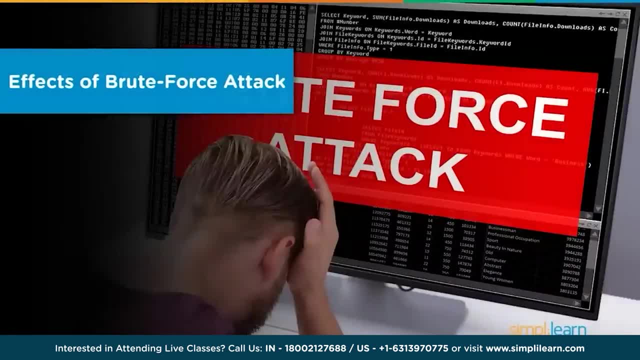 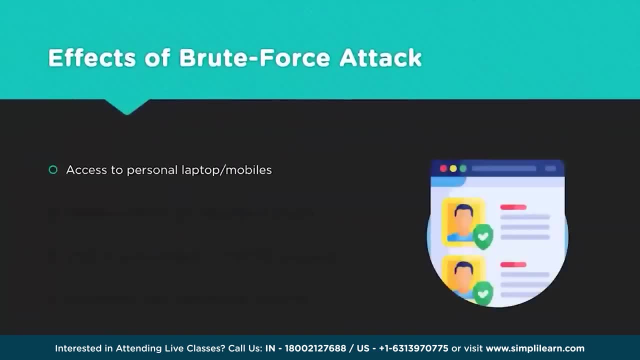 option next week. Let's move on to the harmful effects of getting a system compromised due to brute force attacks. A hacked laptop or mobile can have social media accounts logged in, giving the hackers free access to the victim's connections. It has been reported on multiple occasions where compromised Facebook accounts are sending 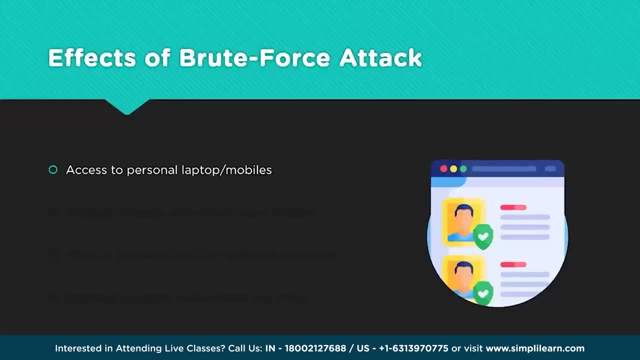 malicious links and attachments to people on their friends list. One of the significant reasons for hacking: malware infusion is best done when spread from multiple devices. similar to distributing spam, This reduces the chance of circling back the source to single devices. Once brute forced, a system can spread malware via email attachments, sharing links, file. 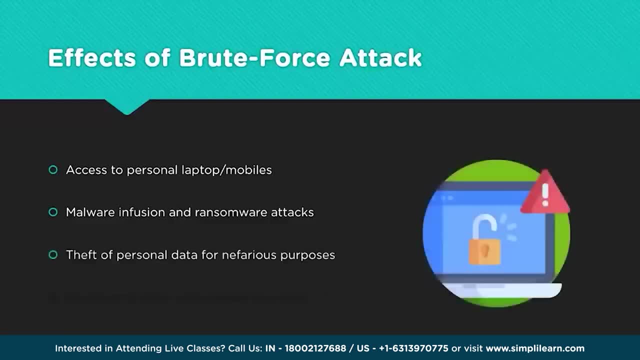 upload via FTP, etc. Personal information such as credit card data, usage habits, private images and videos are all stored in our systems, be it in plain format or root folders. A compromised laptop means easy access to these information that can be further used. 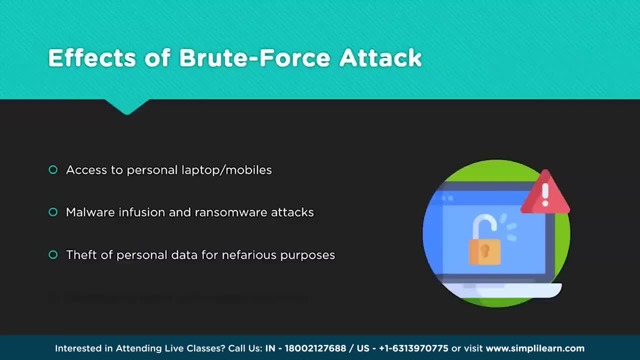 to impersonate the victim regarding bank verification, among other things. Once a system is hacked, it can also be used as a mail server that distributes spam across lists of victims. Since the hacked machines all have different IP addresses and MAC addresses, it becomes 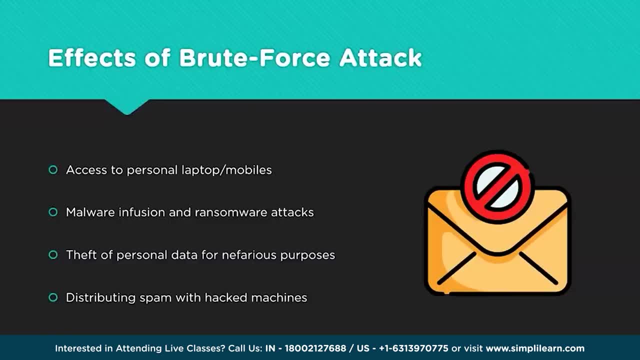 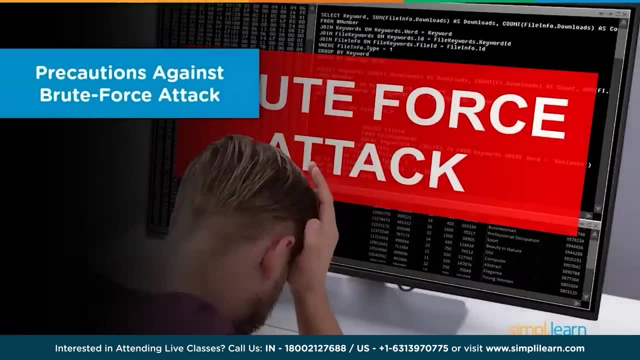 challenging to trace the spam back to the original hacker. With so many harmful implications arising from a brute force attack, it's imperative that the general public must be protected against such. Let's learn about some of the ways we can prevent ourselves from becoming a victim of. 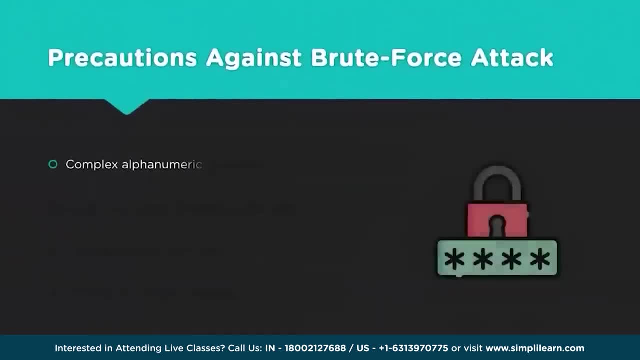 brute force attacks. Using passwords consisting of alphabets, letters and numbers have a much higher chance of extending brute force attacks thanks to the sheer number of combinations they can produce. The longer the password, the less likely it is that a hacker will devote the time and 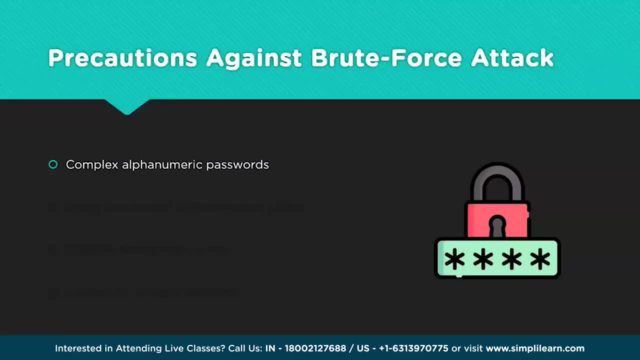 resources to brute force them. Having alphanumeric passwords also allows the user to keep different passwords for different websites. This is to ensure that if a single account or a password is compromised, the user will be able to keep different passwords for different websites. This is to ensure that if a single account or a password is compromised, the user will 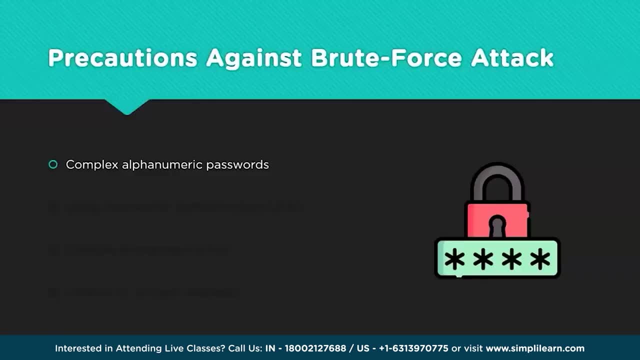 receive the same amount of password as if we had compromised a breach or a hack. the rest of the accounts are isolated from the incident. Two-Factor Identification involves receiving a one-time password on a trusted device before a new login is allowed. This OTP can be obtained either via email, SMS or specific 2FA applications like Authy. 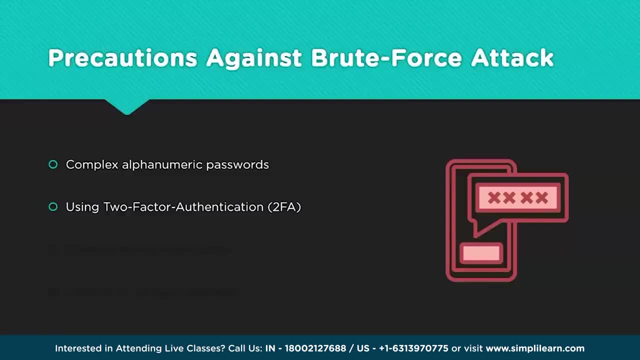 and Ages. Email and SMS based OTPs are considered relatively less secure nowadays due to the ease with which SIM cards can be duplicated and misplaced every time. Two-factor authentication involves receiving a one-time password on a trusted device before and mailboxes can be hacked. 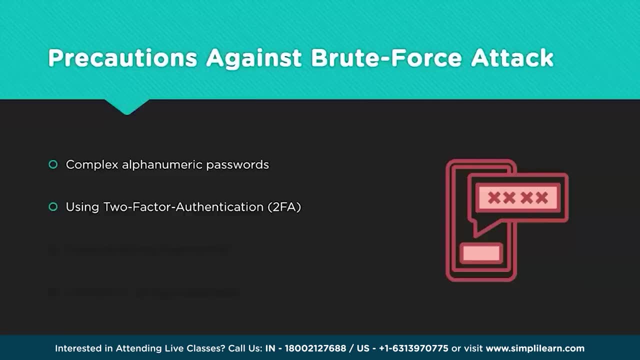 Applications that are specifically made for 2FA cores are much more reliable and secure. CAPTCHAs are used to stop bots from running through web pages precisely to prevent brute forcing through their website, Since brute force tools are automated, forcing the hacker to solve CAPTCHA for every iteration. 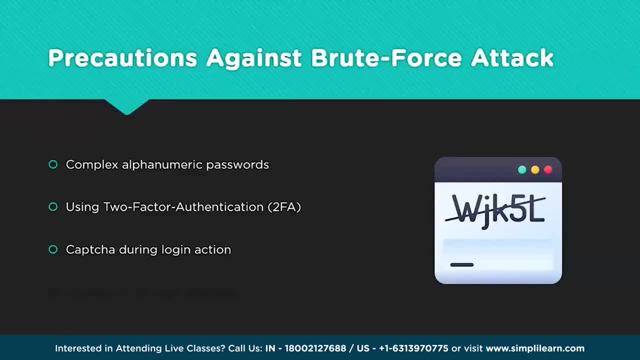 of a password manually is very challenging. The CAPTCHA system can filter out these automated bots that keep refreshing the page with different credentials, thereby reducing the chances of brute force considerably. A definite rule that locks the account being hacked for 30 minutes after a specified number. 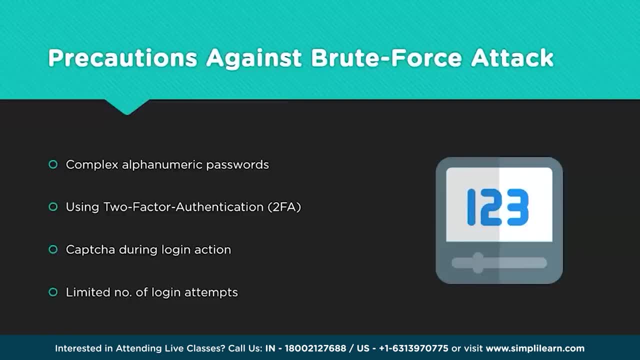 of attempts is a good way to prevent brute force attempts. Many websites lock accounts for 30 minutes after 3 failed password attempts to secure the account against any such attack. On an additional note, some websites also send an email instructing the user that there 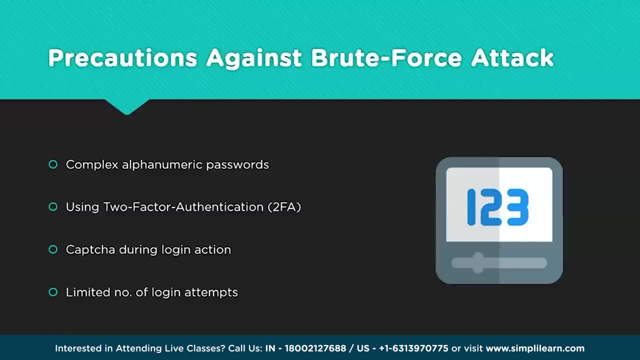 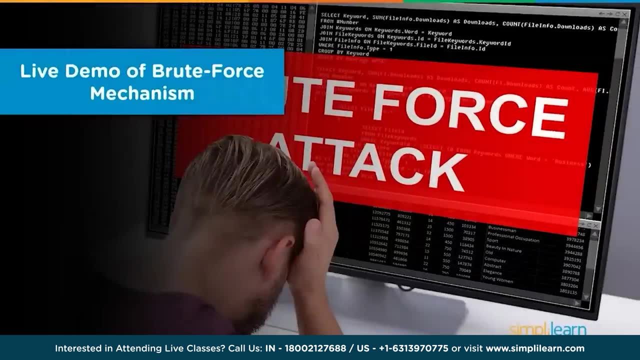 have been 3 insecure attempts to log into the website. Let's look at a demonstration of how brute force attacks work in a real-world situation. The world has gone wireless. With Wi-Fi taking the reins in every household, it's natural that their security will always. 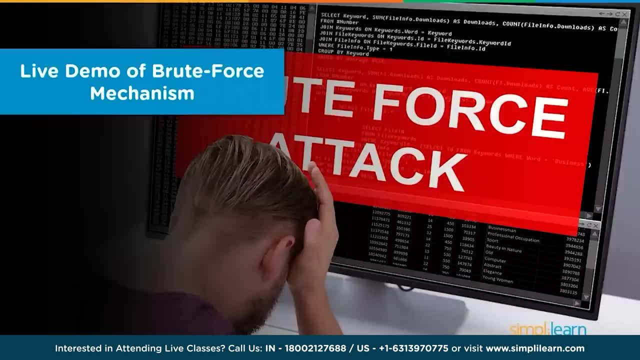 be up for debate, To further test their security index and understand brute force attacks. you will attempt to break into the password of a Wi-Fi router. For that to happen, you first need to capture a handshake file, which is a connection file from the Wi-Fi router to a connecting device. 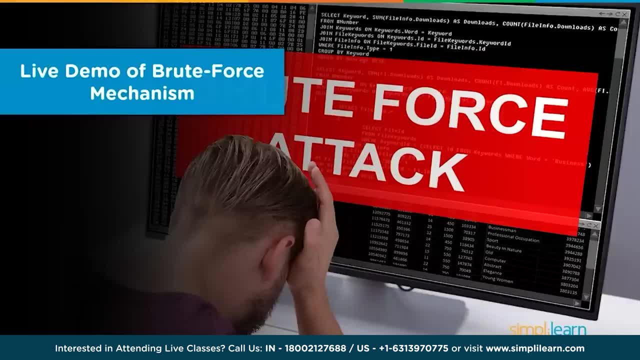 Like this, Like a mobile or a laptop. The operating system used for this process is Pallet Security, a Linux distribution that is catered to penetration testers. All the tools being used in this demo can easily be found pre-installed in this operating. 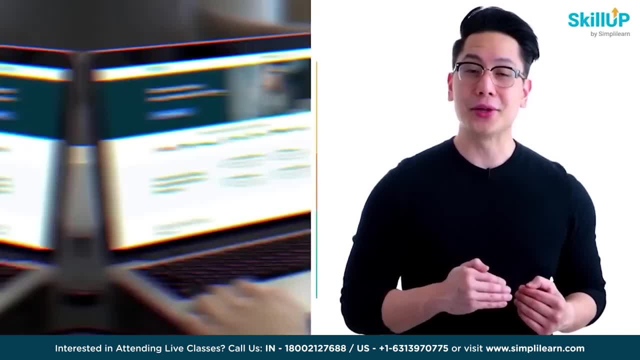 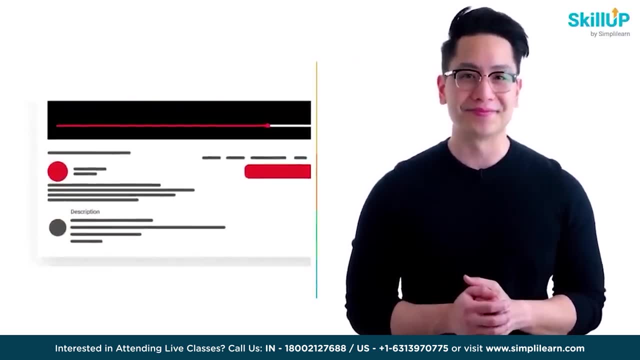 system. If getting your learning started is half the battle, what if you could do that for free? Visit SkillUp by SimplyLearn. Click on the link in the description to know more. To start our demo, we're going to use a tool called Airgeddon. 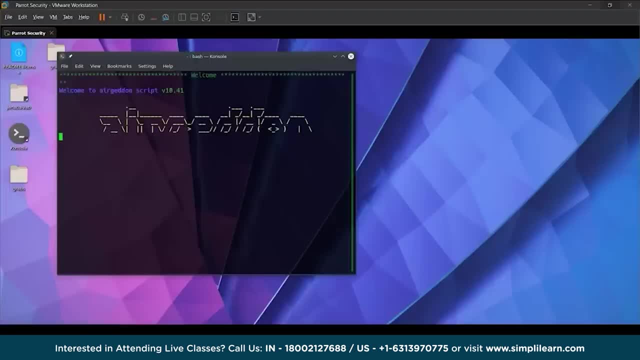 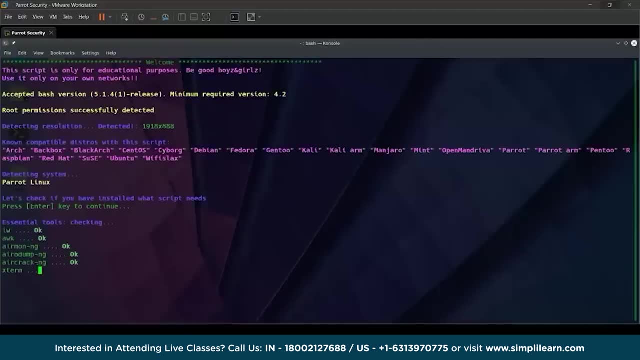 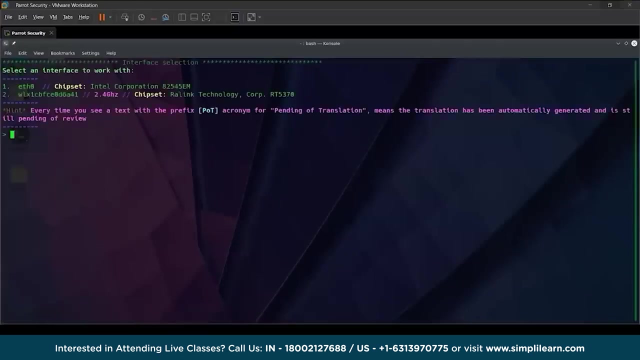 Which is made to hack into wireless networks. specifically, At this point it's going to check for all the necessary scripts that are installed in the system To crack into a Wi-Fi and to capture the handshake file. you're going to need an external network. 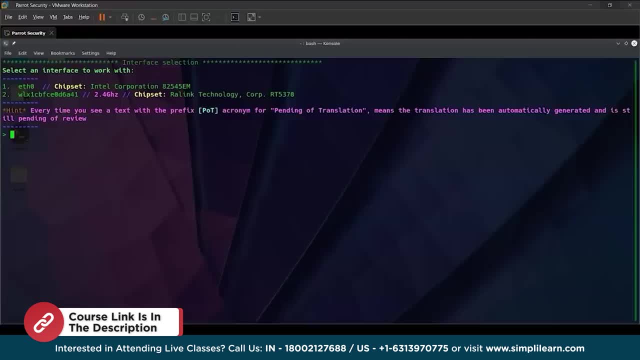 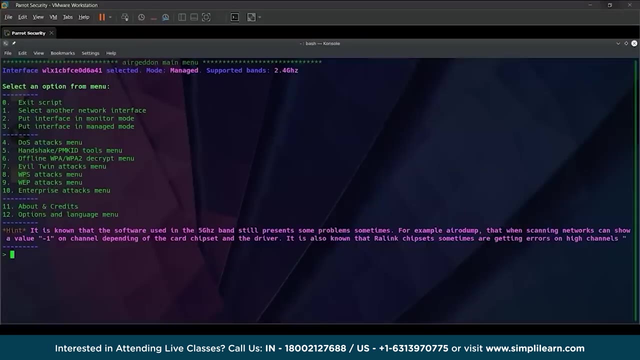 card. The significance of the external network card is a managed mode and a monitor mode. For now, the WLX1 named card is my external network adapter, which I'm going to select To be able to capture data over the air. we're going to need to put it in monitor mode. 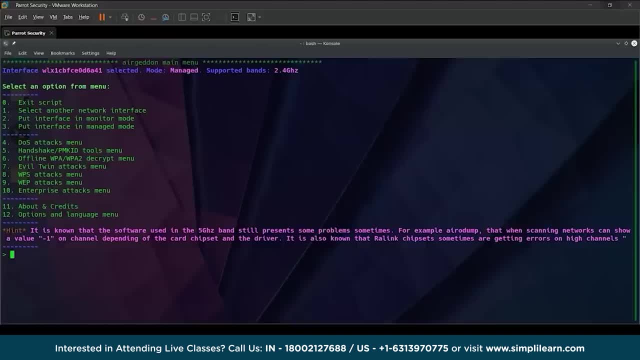 As you can see above, it's written: it is in managed mode right now, So we're going to select option two, which is to put the interface in monitor mode, And its name is now WLAN0 monitor. The monitor mode is necessary to capture data over the air. 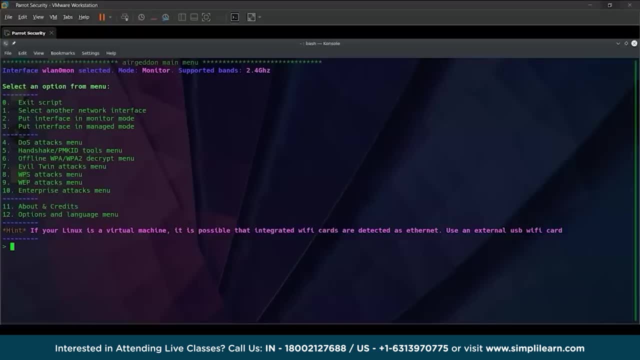 Data is stored. This is the necessary reason why we need an external card, since a lot of inbuilt cards that come with the laptops and the systems they cannot have a monitor mode installed. Once we select the mode, we can go into the fifth, which is the handshake tools menu. 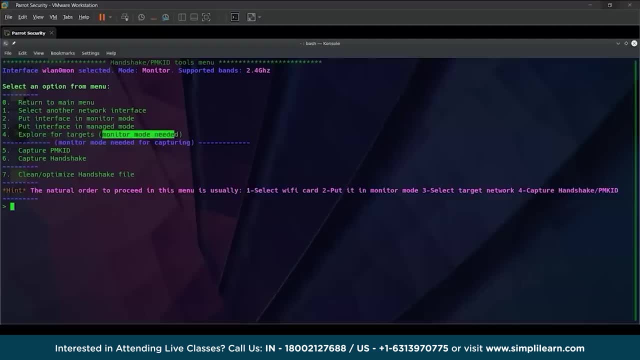 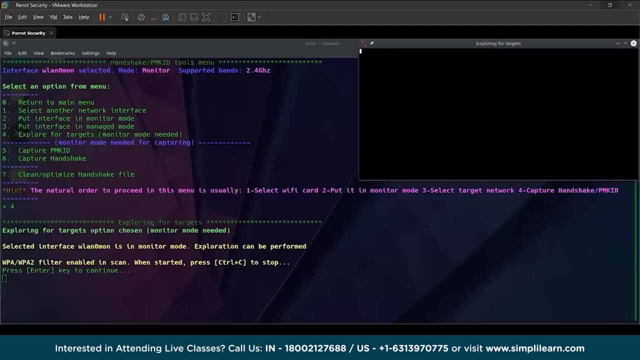 In the first step we have to explore for targets and it is written that monitor mode is necessary to select a target. So let's explore for targets and press enter. We have to let this run for about 60 seconds to get a fair idea about the networks that. 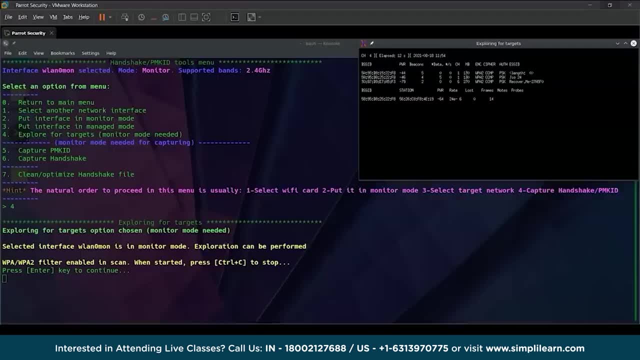 are currently working in this locality. For example, this ESS ID is supposed to be the Wi-Fi name that we see when connecting to a network. Geo24, RecoverMe- these are all the names that we see on our mobile when trying to search. 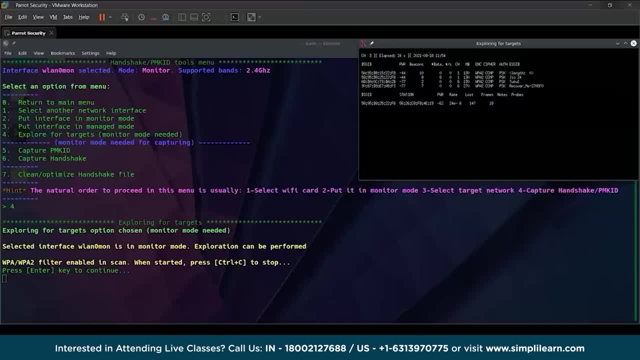 for the Wi-Fi. This BSS ID is supposed to be an identifier, Somewhat like a MAC address. Okay, This is a MAC address that identifies this network from other devices. The channels features on one or two, or there are some many channels that the networks can. 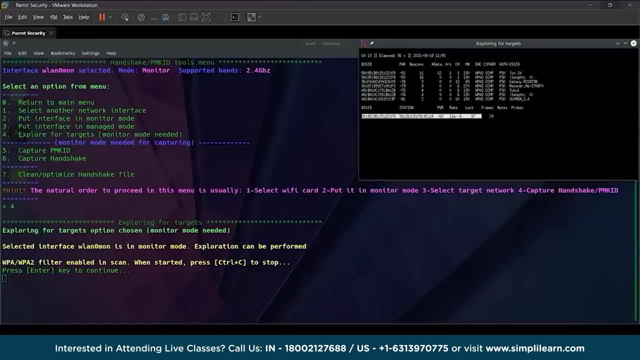 focus on This. here is supposed to be a client that is connected to one such network, For example, the station that you can see, 5626,. this is supposed to be the MAC address of the device that is connected to a router. This BSS ID is supposed to be which Wi-Fi it is connected to. 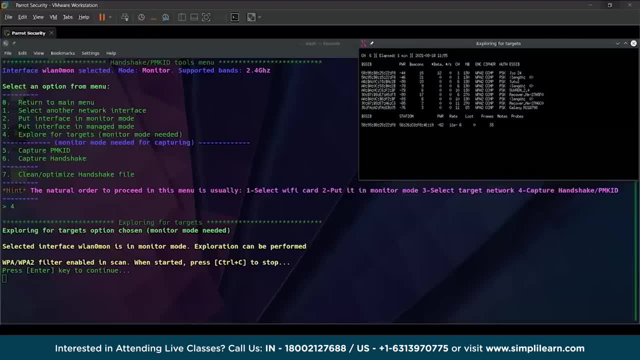 For example, 5895D8 is this one, which is the Geo24 router. So we already know which router has a device connected to it and we can use our attack to capture this handshake Now that we it has already run for one minute. 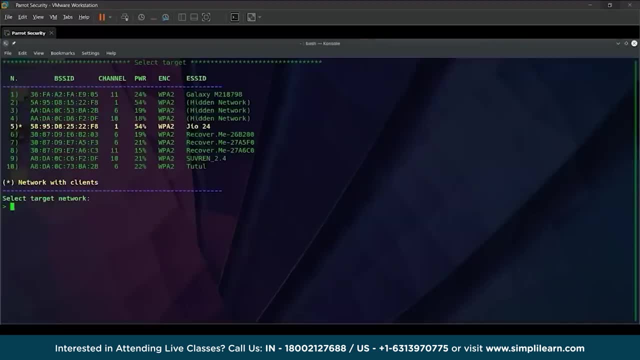 Now that we press control C, it will be asked to select a target. See, it has already selected the number five, which is the Geo24 router, as the one with clients. So it is easy to run an attack on And it is easy to capture a handshake for. 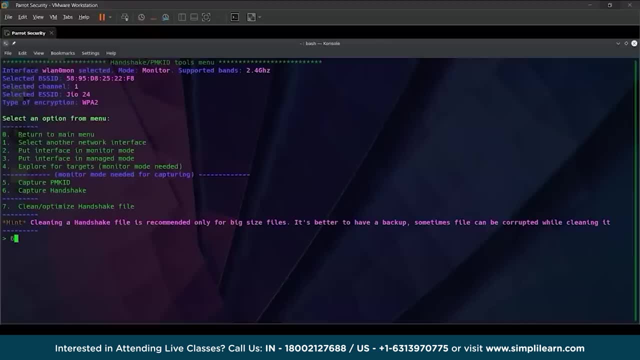 Select network five and we run a capture handshake. It says we have a valid WPA WPA2 network target selected and that the script can continue Now to capture the handshake. we have a couple of attacks: a deauth or a deauth air replay. 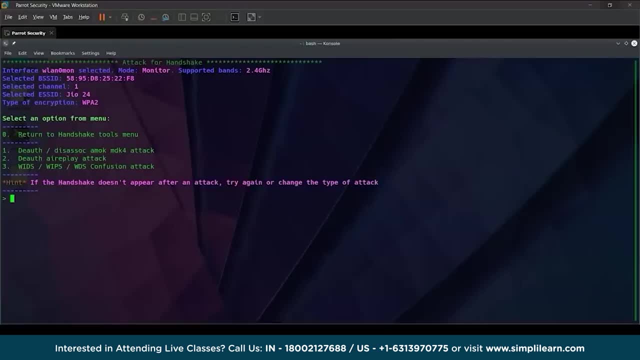 attack. What this attack does is kick the clients out of the network in return when they try to reconnect to the Wi-Fi, As they are configured that way that when a client is disconnected, it tries to reconnect it immediately. It tries to capture a handshake file which, in turn, contains the security key, which is: 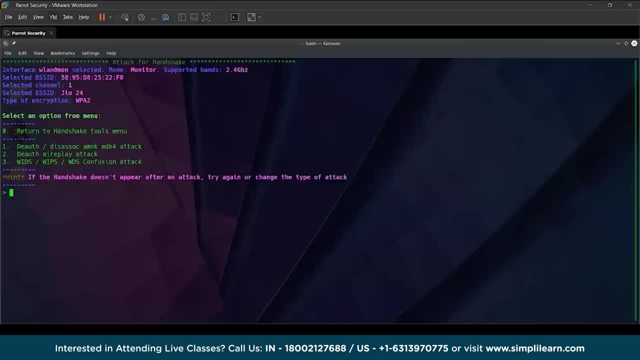 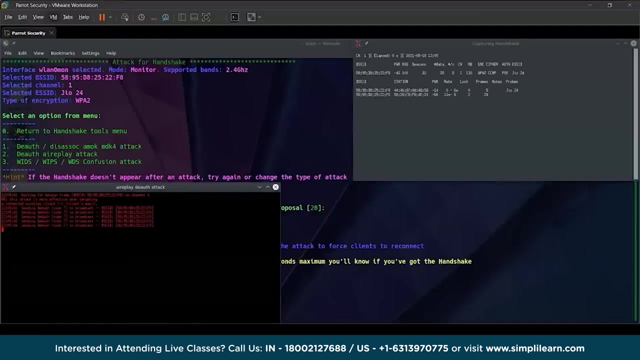 necessary to initiate the handshake For our demo. let's go with the second option, That is, the deauth air replay attack. Select a timeout value. Let's say we give it 60 seconds and we start the script. We can see it capturing data. 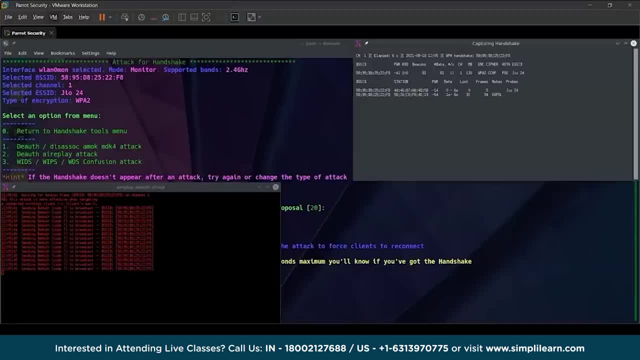 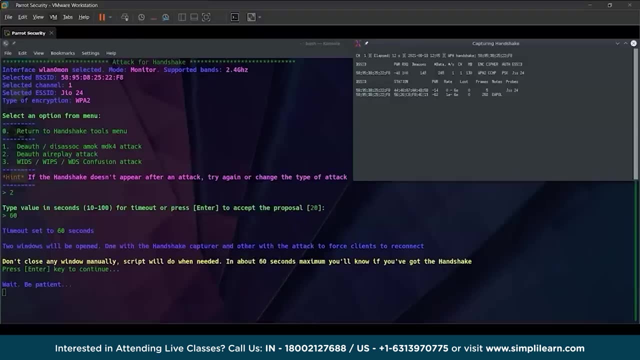 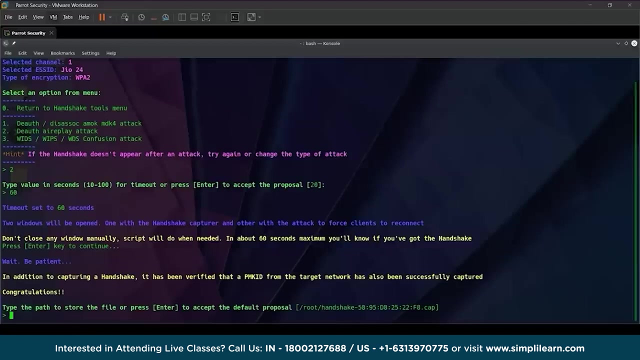 We can see the data from the Geo24 network. and here we go. We have the WPA handshake file. Once the handshake file is captured, we can actually close this. and here we go. congratulations In order to capturing a handshake. it has verified that a PMK ID from the target network. 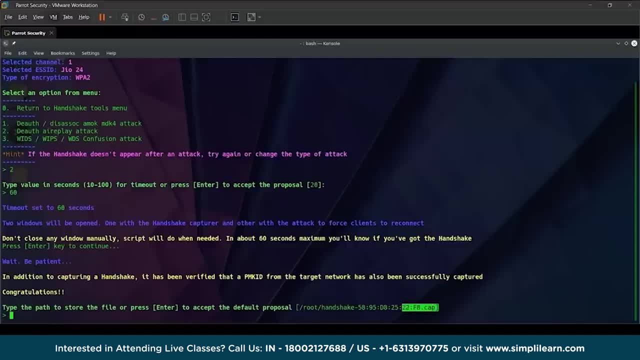 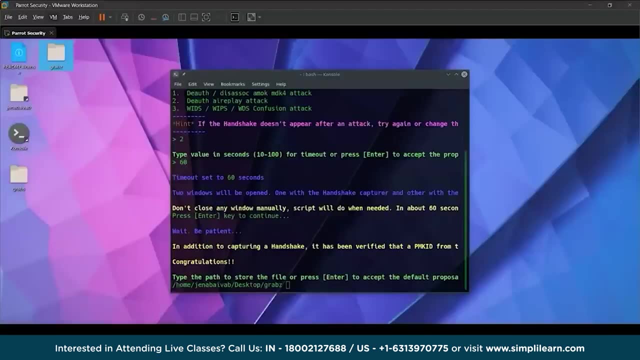 has successfully been captured. This is the file that is already stored, the cap file For the path. we can, let's say, we can keep it, We can keep it in a desktop, okay, we give the path and the handshake file is generated. 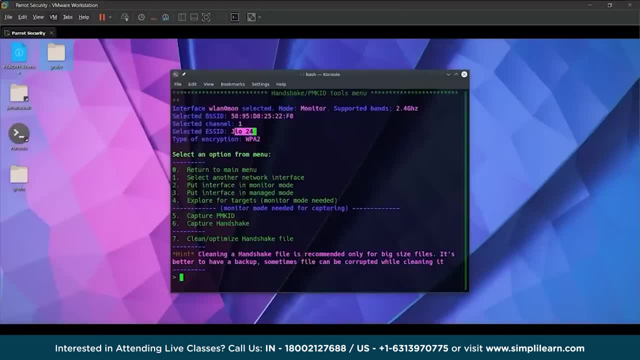 We can already see a target over here: same Geo24 router with the BSS ID. Now, if we return to its main menu, we already have the handshake file captured with us. Now our job is to brute force into that handshake capture file. 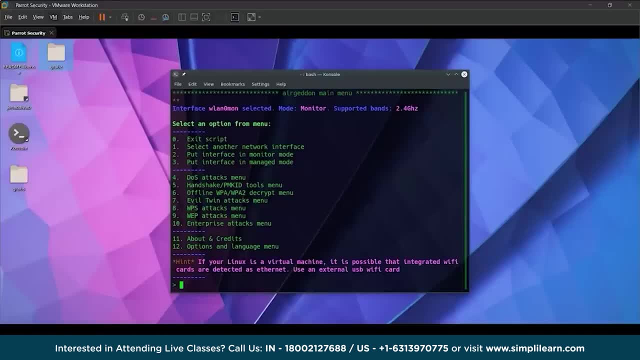 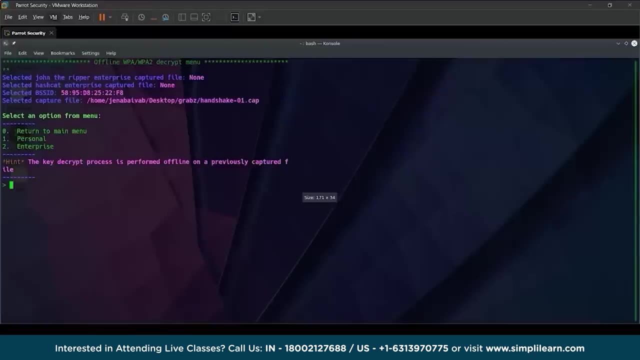 The capture file is often encrypted with the security key of the Wi-Fi network. If we know how to decrypt it, we will automatically get the security key. So let's go to the offline WPA WPA2 decrypt menu. Since we'll be cracking personal networks, we can go with option one. 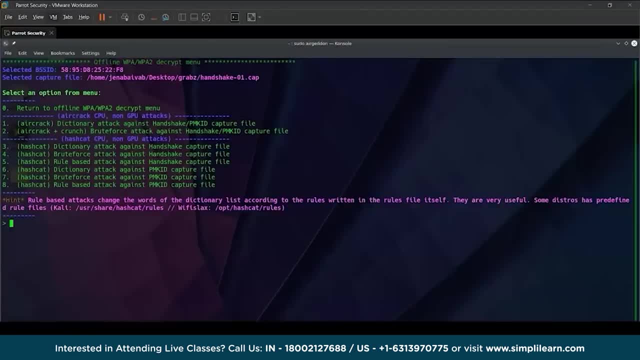 Now to run the brute force tool, we have two options: Either we can go with the Aircrack or we can go with the Hashcat. Let's go with Aircrack plus crunch, which is a brute force attack against a hashcat. 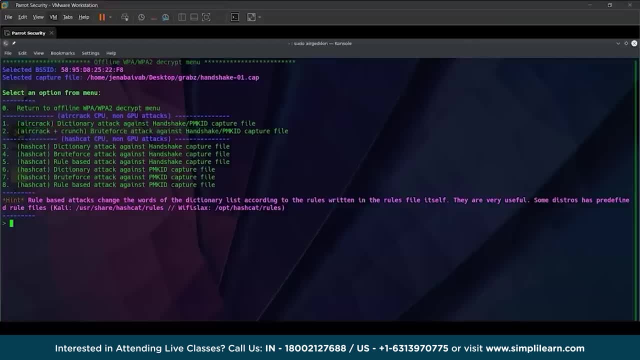 Let's go with Aircrack plus crunch, which is a brute force attack against a hashcat. Let's go with Aircrack plus crunch, which is a brute force attack against a hashcat. We can go with option two. We can go with option two. 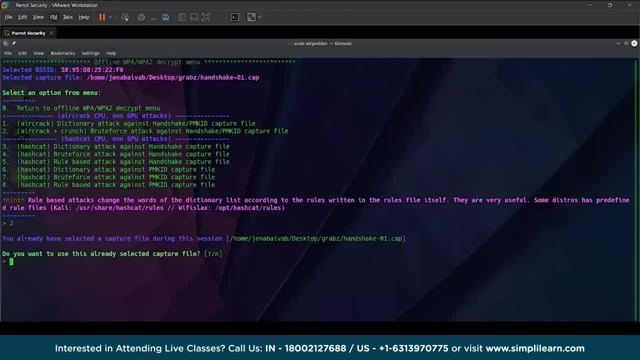 It can already detect the capture file that we have generated. so we select yes. The BSSID is the one which denotes the Jio 24 router, so we're going to select yes as well. The minimum length of the key, for example. it has already checked that the minimum length. 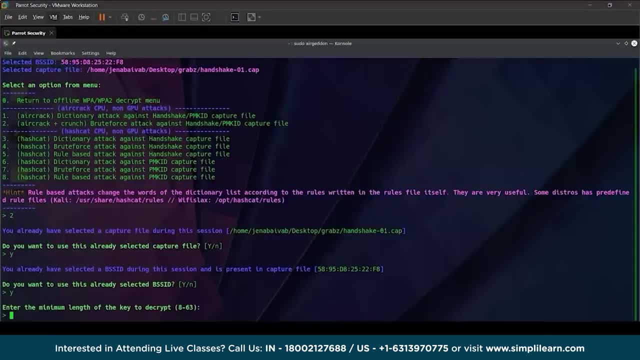 of a WiFi security key, which is a WPA2 Psk key, will always be more than eight digits and below 64 digits, So we have to select something in between this range. So if we already know, let's say, that the password is at least 10 digits, we can go. 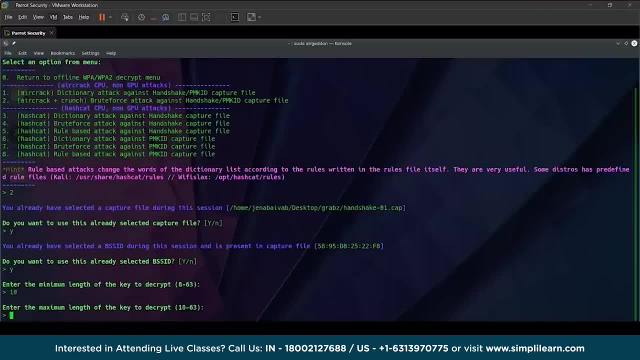 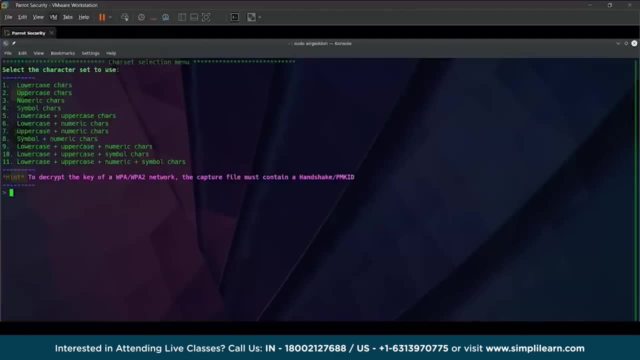 with the minimum length as 10.. And as a rough guess, let's say we put the maximum length as 20.. The character set that we're going to use for checking the password will affect the time taken to brute force, For example, if we already know that we have seen a user use a password while connecting. 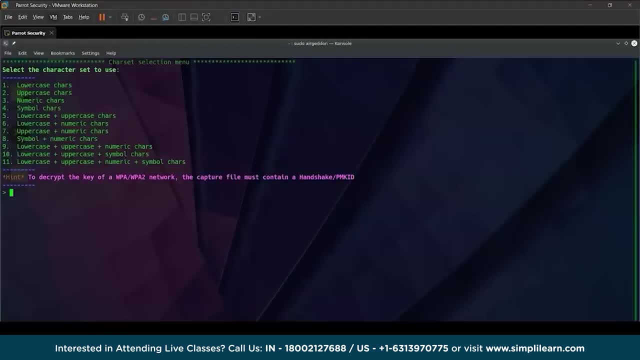 to the router as something that has only numbers and symbols, then we can choose accordingly. Let's say, if you go with only uppercase characters and numeric characters, go with option seven, and it's going to start decrypting. So how Aircrack is working right here. you can see this passphrase over here: 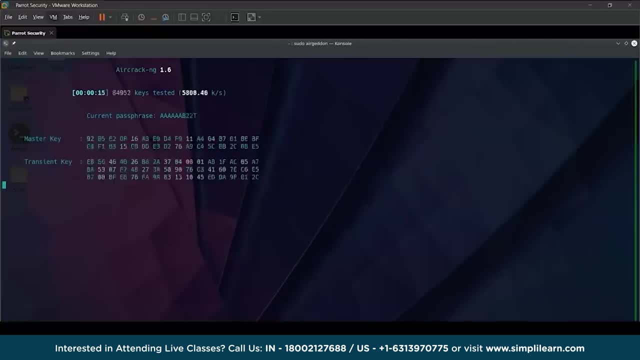 The first five or six digits are A, It starts working. It's working its way from the end, from the last character. It keeps trying every single combination. You can see the last, the fourth character from the right side, the D. It will eventually. 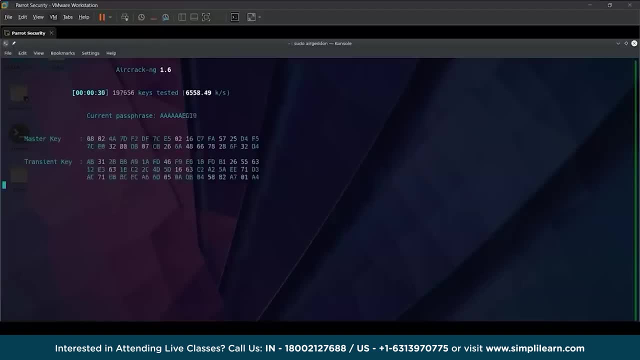 turn to E, because it keeps checking up every single character from the end. This will keep going on until all the single characters are tested and every single combination is tried out, Since the handshake file is encrypted using the security key, that is, the WPA2 key of. 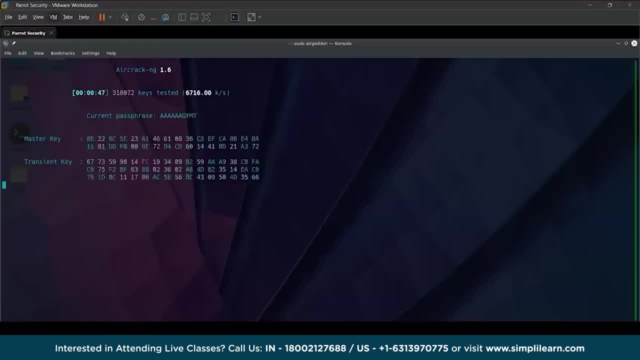 the router. Whichever passphrase is used, it will be checked. The passphrase is able to decrypt the handshake key completely will be the key of the Wi-Fi router. This is the way we can brute force into Wi-Fi routers anywhere in the world. 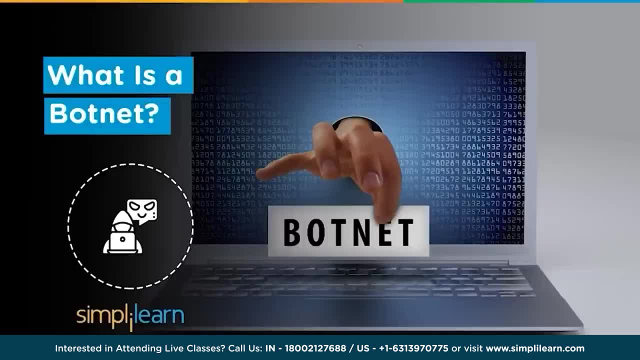 Cyber attacks are frequently making headlines in today's digital environment. At any time, everyone who uses a computer could become a victim of a cyber attack. There are various sorts of cyber attacks, ranging from phishing to password attacks. In this video, we'll look into one such attack. 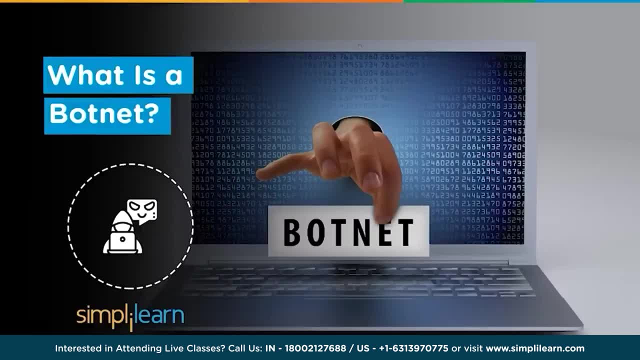 That is known as Botnet. But before we begin, if you love watching tech videos, subscribe to our channel and hit the bell icon never to miss an update. To begin with, let's take a look at some of the famous botnet attacks. 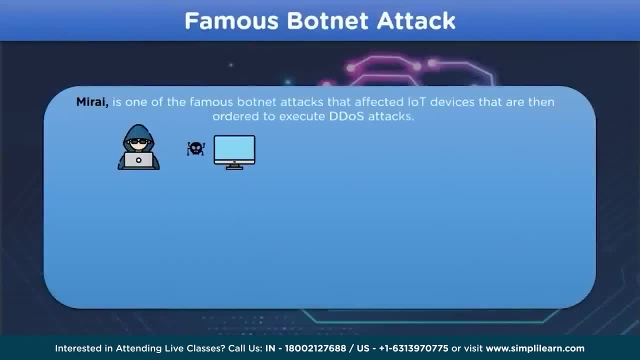 The first one is Mirai Botnet, which is a malicious program designed to attack vulnerable IoT devices and infect them to form a network of bots That, on command, perform basic and medium-level denial of service attacks. Then we have the ZooBotnet. 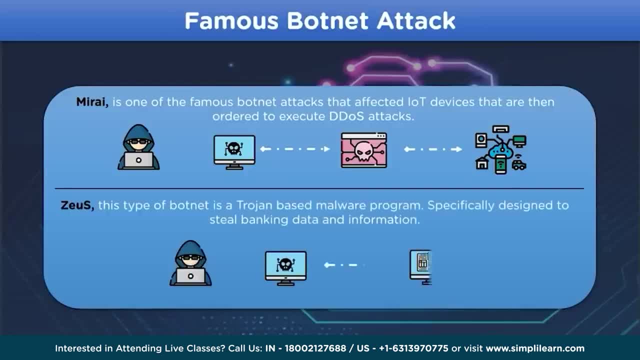 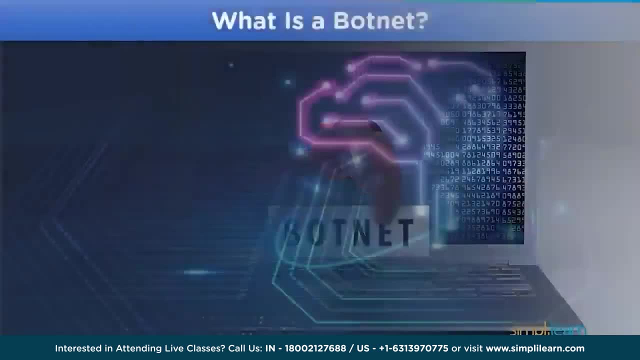 This is a botnet-based botnet. This is a botnet-based botnet. It is specifically designed for attacking the system for bank-related information and data. Now let's see what exactly a botnet is. Botnet refers to a network of hijacked interconnected devices that are installed with malicious 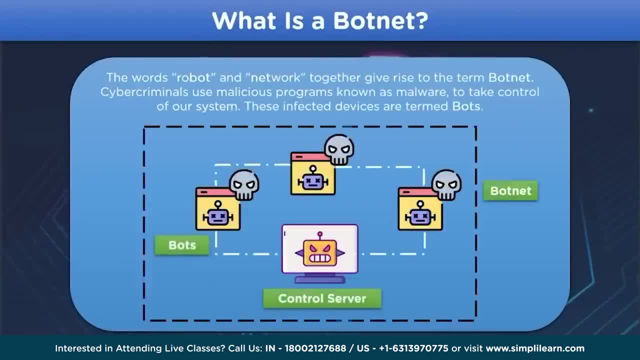 codes known as malware. Each of these infected devices are known as bots, and a hijacked criminal, known as a bot herder, remotely controls them. The bots are used to automate large-scale attacks, including data theft, piracy and server failure, malware propagation and denial of service attacks. 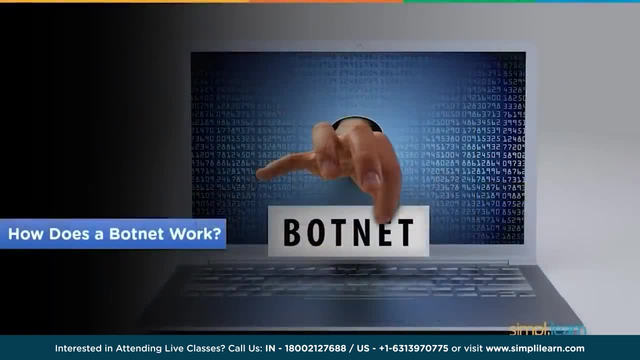 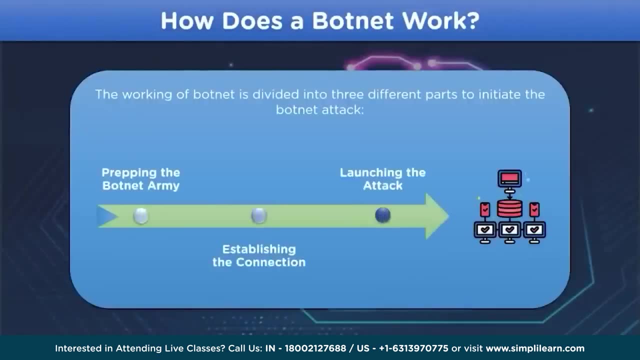 Now that we know what exactly a botnet is, let's dive deeper into learning how a botnet works. During the preparation of a botnet network, the first step involves preparing the botnet army. After that, the connection between the botnet army and the control server is established. 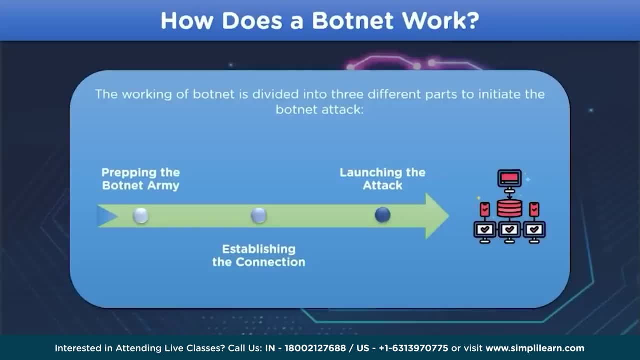 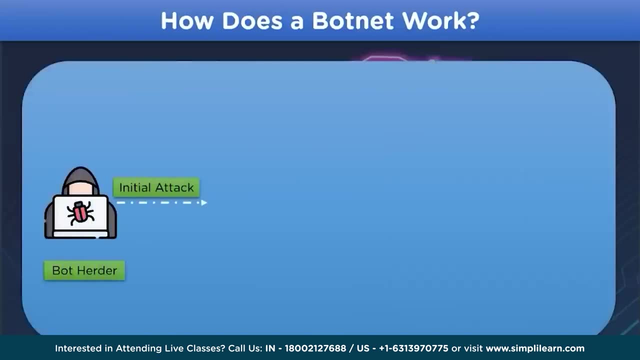 In the end, the launching of the attack is done by the bot herder. Let's understand through an illustration. Firstly, we have a bot herder that initiates the attack According to the control server commands the devices that are infected with the malware. 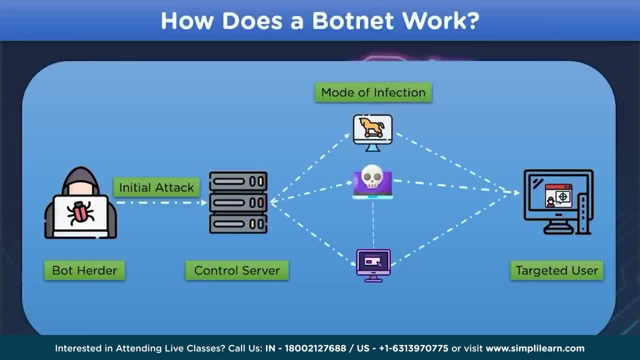 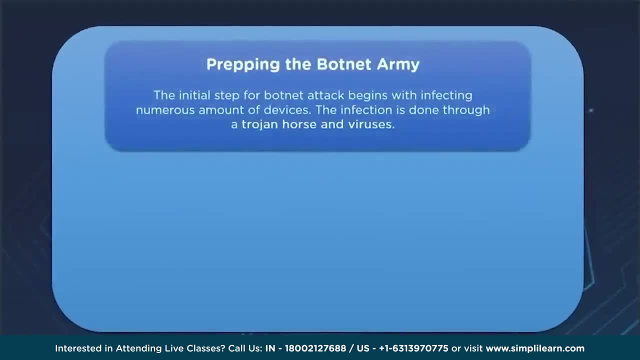 programs and begins to attack the infected system. Let's see some details regarding the preparation of the botnet army. The first step is known as the prepping the botnet army. The first step is creating a botnet is to infect as many as connected devices as possible. 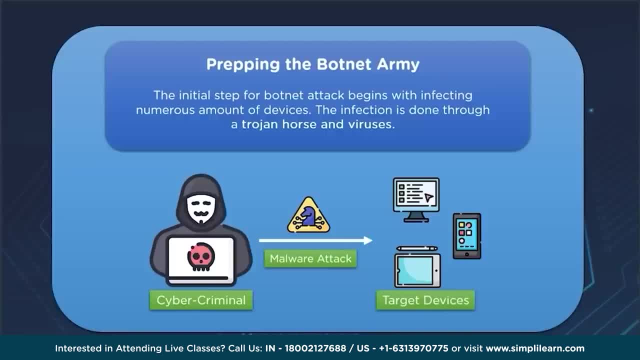 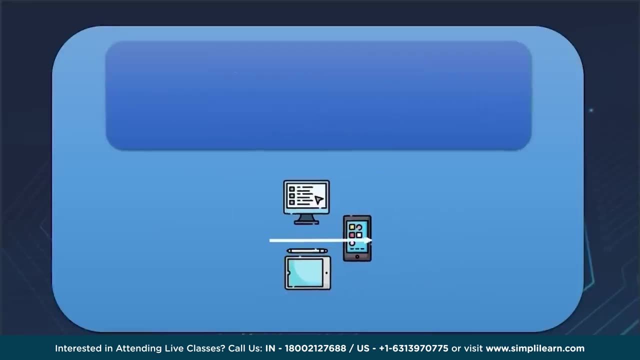 This ensures that there are enough bots to carry out the attack. This way, it creates bots either by exploiting the security gaps in the software or websites or using phishing attacks. They are often deployed through Trojan horses. For the next step, we have establishing the connection. 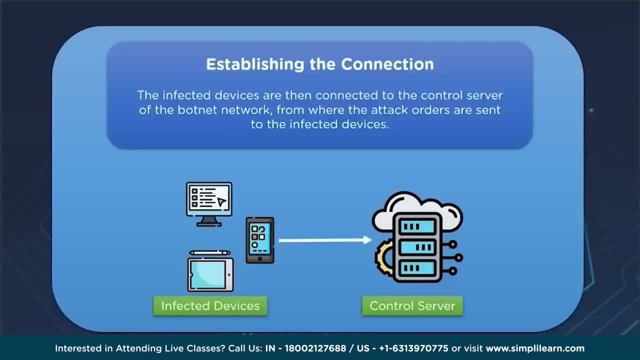 Once it hacks the device, as per previous step, it infects it with the specific botnet malware that connects the device back to the control bot server. A bot herder uses command programming to drive the bot's actions, And the last step is known as launching the attack. 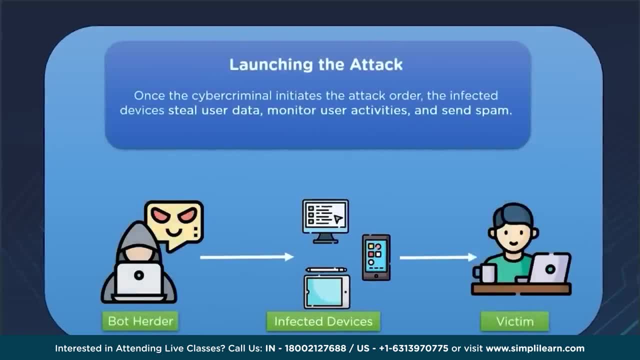 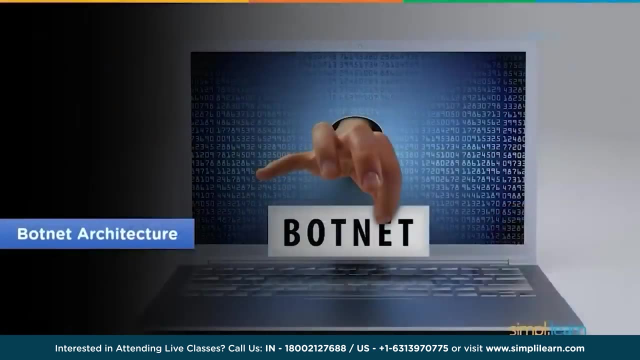 Once infected, a bot allows access to admin level operation like gathering and stealing of data, reading and rewriting the system, data monitoring user activities, performing denial of service attacks, including other cybercrimes. Now let's take a look at the botnet architecture. 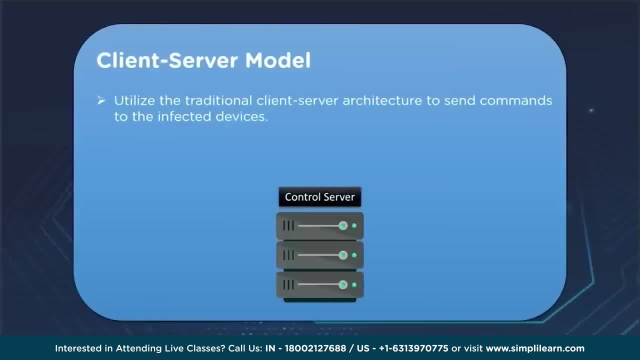 The first type is known as client-server model. The client-server model is a traditional model that operates with the help of a command and control center server and communication protocols like IRC. When the bot herder issues a command to the server, it is then relayed to the clients. 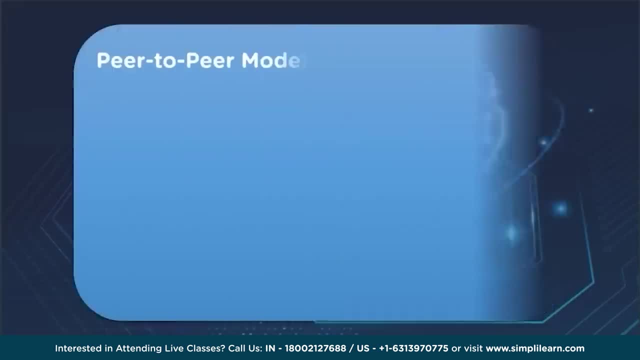 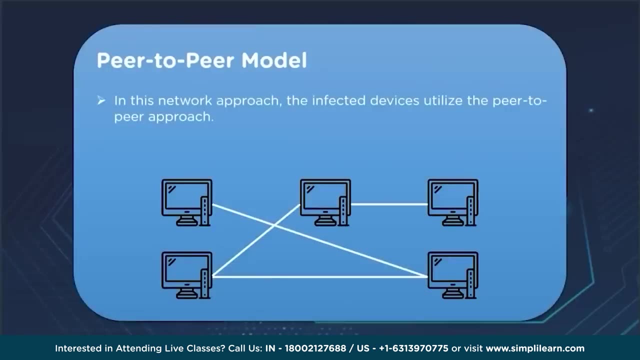 to perform malicious actions. Then we have peer-to-peer model Here. controlling the infected bots involves a peer-to-peer network That relies on a decentralized approach. that is, the bots are a topological interconnector and acts as both CNC servers, that is, the server and the client. 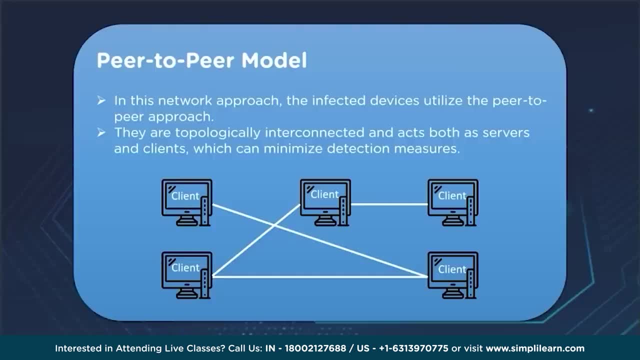 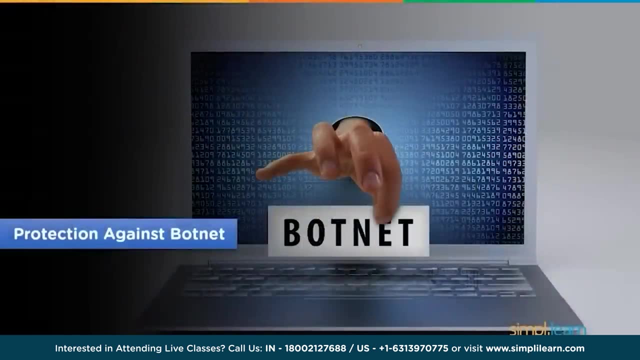 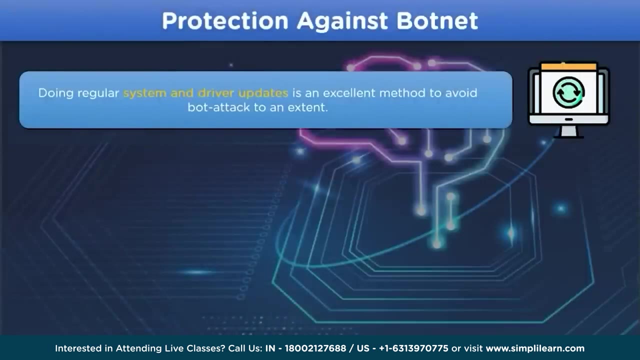 Today, hackers adopt this approach to avoid detection and single-point failure. In the end, we will see some points on some countermeasures against botnet attacks. The first step is to have updated drivers and system updates. After that, we should avoid clicking random pop-ups or links that we often see on the internet. 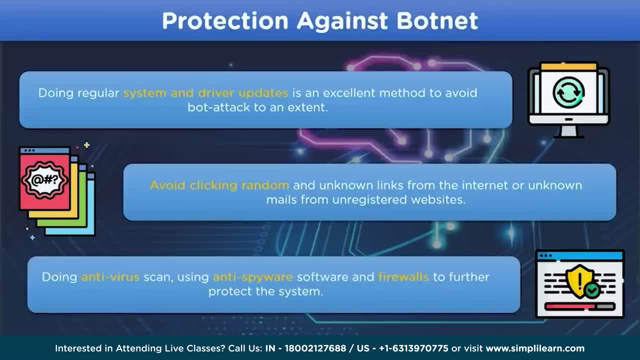 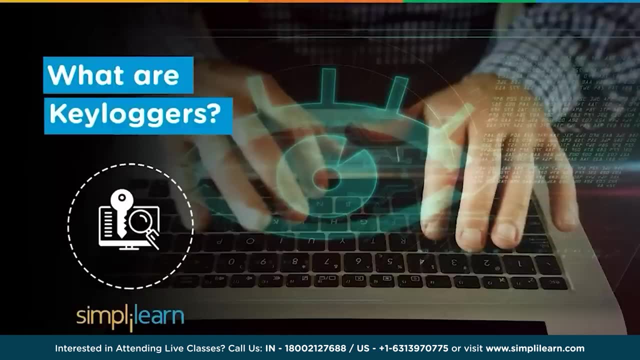 And lastly, having certified antivirus, anti-spyware softwares and firewall installed into a system will protect against malware attacks. The internet is an endless source of information and data. Still, in some cases, we come across some occurrences like cyberattacks, hacking, poor. 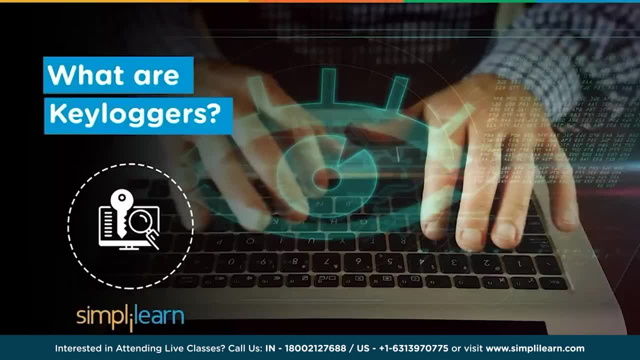 sentry which may affect our time on the web. Hi everyone and welcome to the Simply Lawn channel. Today we will look at some of the most common cyber-attacks. Let's get started. Today we will discuss a topic that secretly records our input data. that is known as. 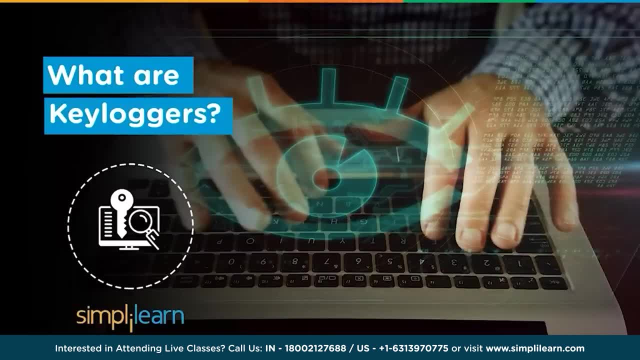 keyloggers. But before we begin, if you like watching tech videos, subscribe to our channel and hit the bell icon to never miss an update. To understand the keylogging problem better, let's take a look at an example. This is June. 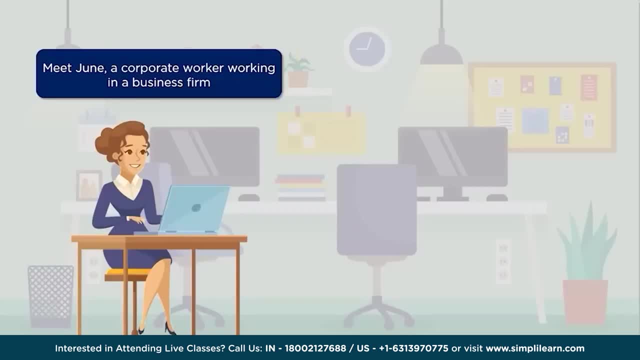 She works in a business firm where she manages the company's data regularly. This is Jacob from the information department, who is here to inform her about some of the security protocols. During the briefing, she informed him about some of the problems her system was facing. 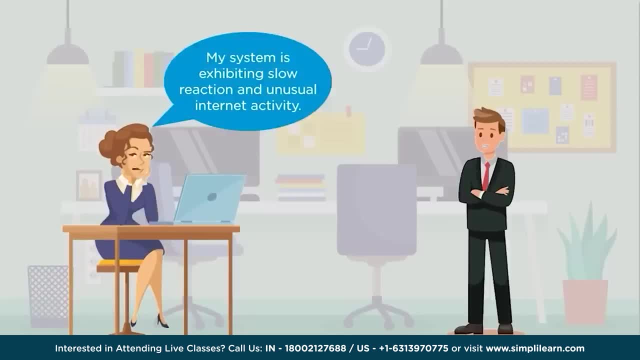 with, which included slow reaction speed and unusual internet activity. As Jacob heard about the problems with the system, he thinks of the possibility what could be the reason behind these problems her system was facing with. The conclusion that he came across was the keylogging issue. 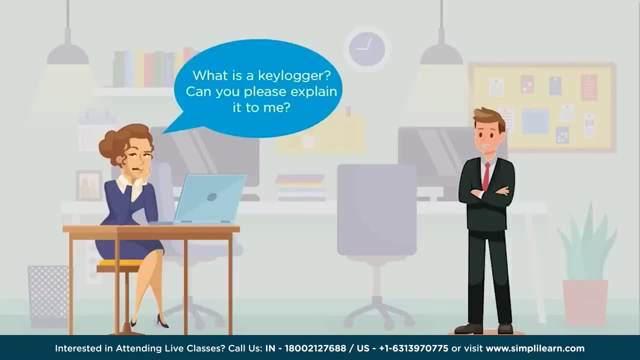 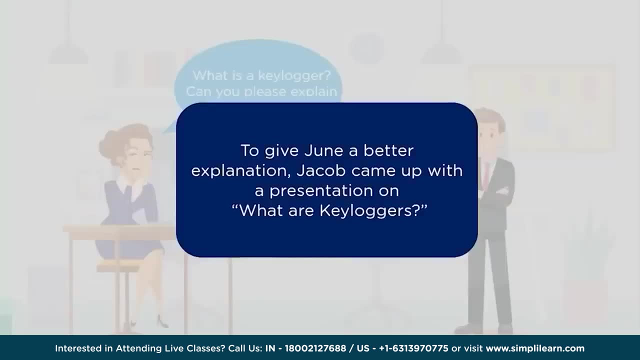 Unknown to the problem. She asked him about some of the details regarding it. For today's topic, we'll learn what exactly keyloggers are and how they affect our system. what are the harmful effects that keylogging can bring into the system? 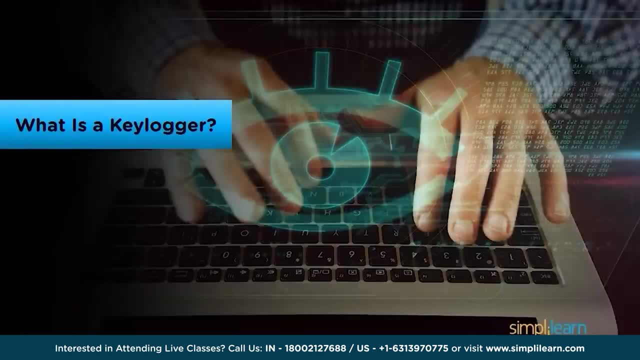 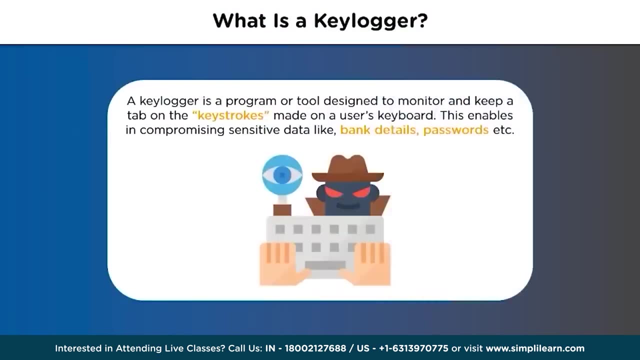 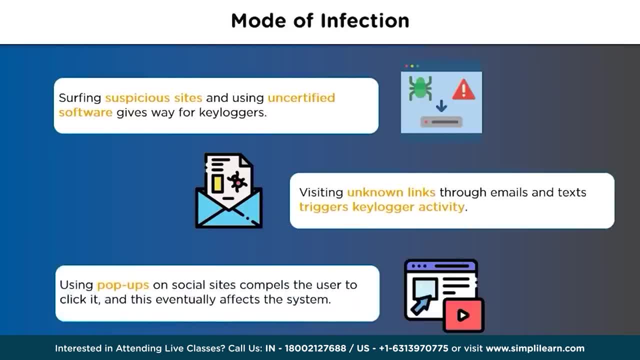 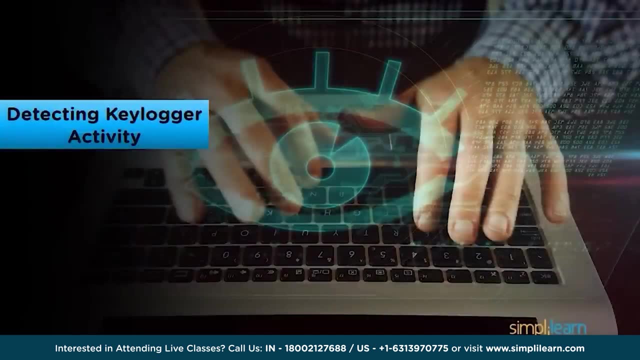 key logging issue entering into the system. and lastly, there are often cases where different pop-ups that we often see on social sites or different media sites can lead to the installation of key logging program into our system. now that we know how the problem gets into the system, let's take a look how to identify whether the system is infected by the key logging. 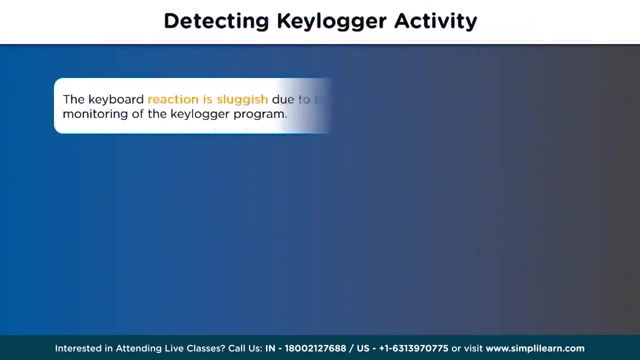 issue- the key logging issue- can be identified. if there are often cases when a keyboard lags behind the system, the data that we enter sometimes is stuck in between when we type through the input. then there are cases when the system freeze occurs unknowingly to what exactly could be the reason. 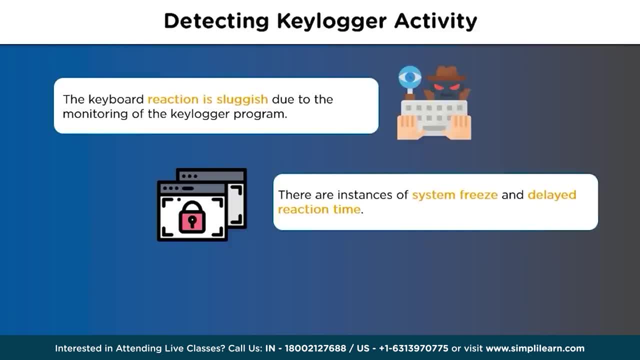 behind them, and also there are delayed reaction time for different applications that run on the system. and, lastly, there are different cases when we often see suspicious internet activity on the system that we don't know about. this could lead to the identification of a problem into the system. 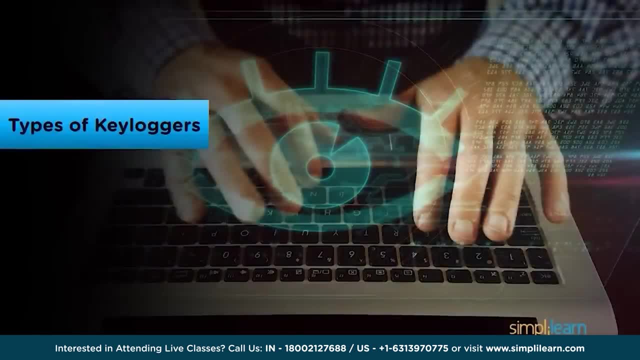 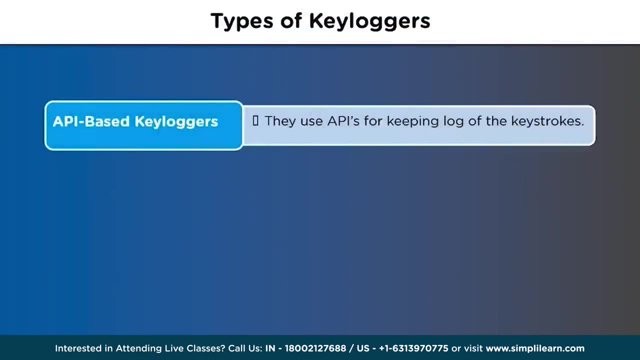 now we'll take a look at different types of key loggers that are present on the net which can harm our system differently. the first problem that key loggers arouse is api based, the most common key logging case, which uses apis to keep a log of the type data and share it to. 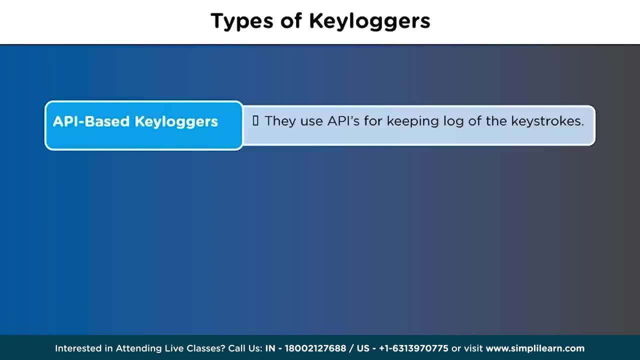 its origin for malicious purposes. each time we press a key, the key logger intercepts the signal and logs it. then we have form grabbing base key loggers. as the name suggest, they are a based key loggers that store the form data. that is, if we often use web forms for different kinds of forms. to enter different data, they can be recorded into the system. that may lead to anything likeviol. please remind to add this webinar's link in the description if you need your unique information after watching the video. the most common key logging case which uses api is to keep a log of the type data and share it to its origin我們 hari. 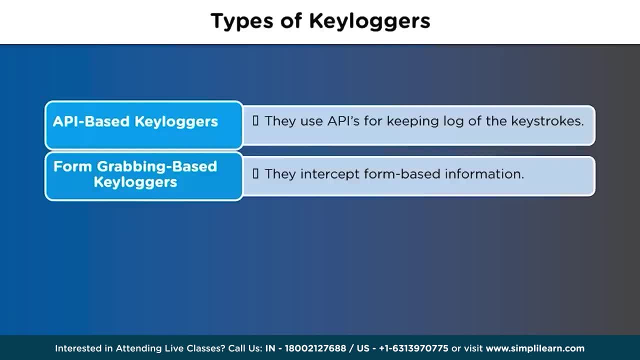 can be recorded into the system by the program and send it to its origin. then we have kernel based key loggers. these key loggers are installed deeply into the operating system where they can hide from different antivirus if not checked properly, and they record the data that we type on the keyboard and send it to. 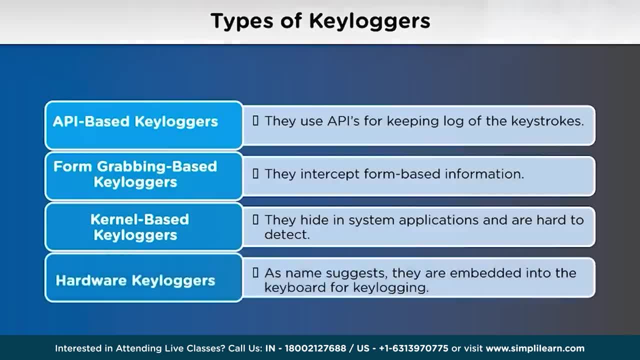 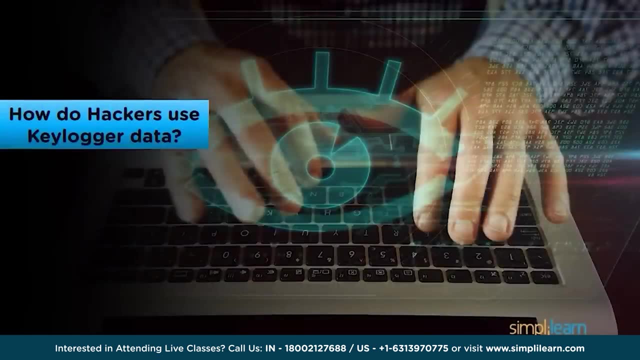 its origin. and lastly, we have hardware key loggers. these key loggers are present directly into the hardware, that is, they are embedded into system, where they record the data that we type on the keyboard. now let's take a look how hackers differentiate different type of recorded data and exploit them. 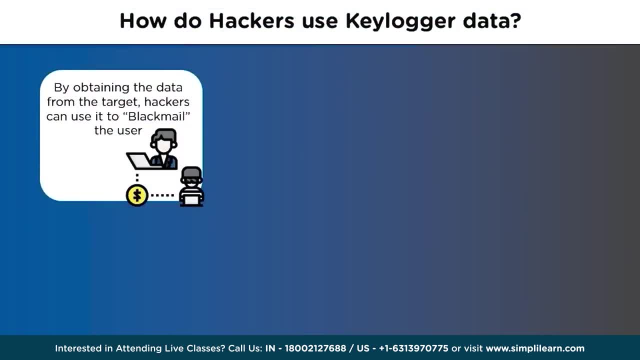 when hackers receive information about the target, they might use it to blackmail the target, which may affect the personal life of the target, and also blackmail them for different money related issues. then, in case of company data that is recorded by the key logging program, can also affect the economic value of the company in the market, which may lead to. 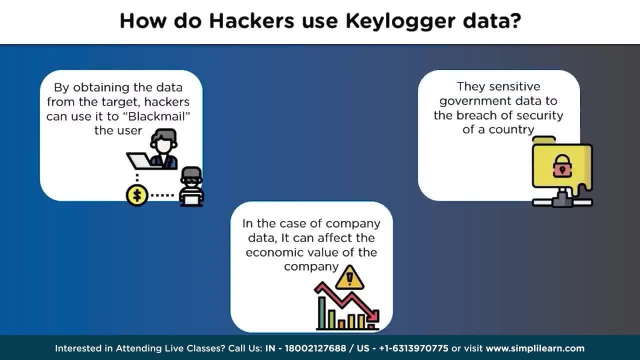 the downfall of the company. also, in some cases, the key logging program can also log data about military secrets, which may include nuclear codes or security protocols which are necessary to maintain the security of a country. now let's take a look where the mobile devices get infected with the key logging. 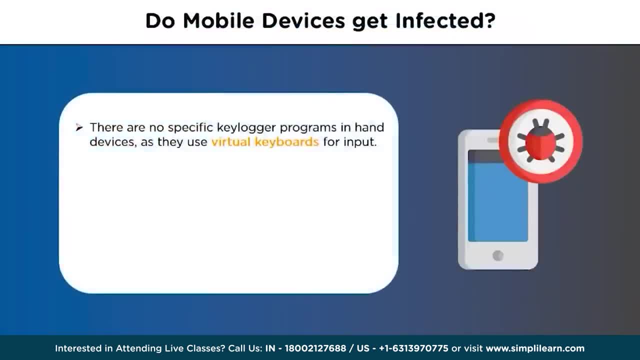 issue or not. in the case of hand devices, infection of key loggers are low in comparison to the computer systems as they use on-screen keyboard or virtual keyboard, but in some cases we often see different kinds of malicious programs getting installed into the hand device. if we often visit different uncertified 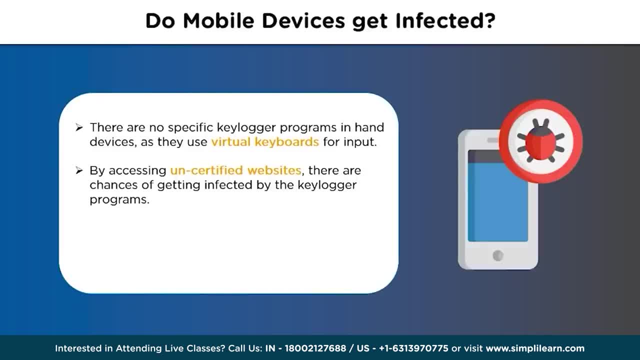 websites or illegal websites or torrent sites, and also the device that is infected with. the key logging issue or different kind of malicious program can often lead to the exploitation of data- that includes photos, emails or important files- by the hacker or the cyber criminal that installed a particular malicious program. 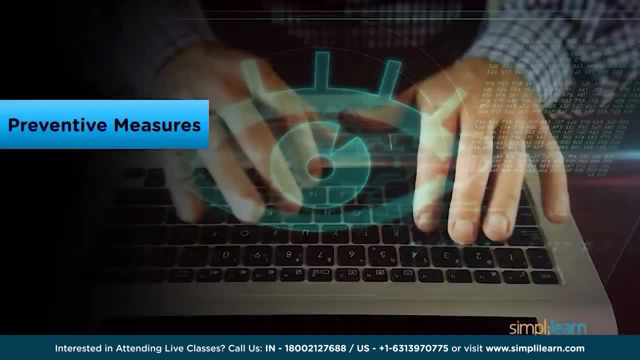 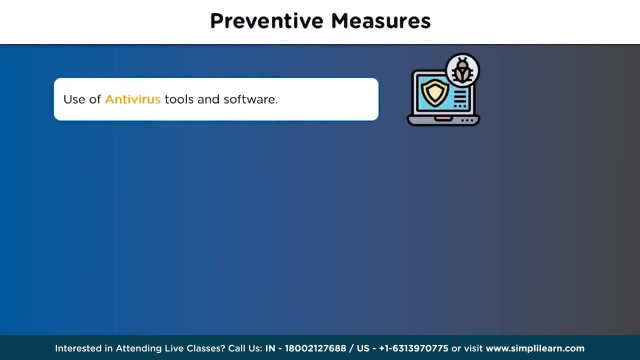 into the system. now to prevent a system from getting infected by the key logging program, let's take a look at different points. now to prevent a system from getting infected by the key logging program, let's take a look at different points. the first point includes using of different antivirus software or tools. 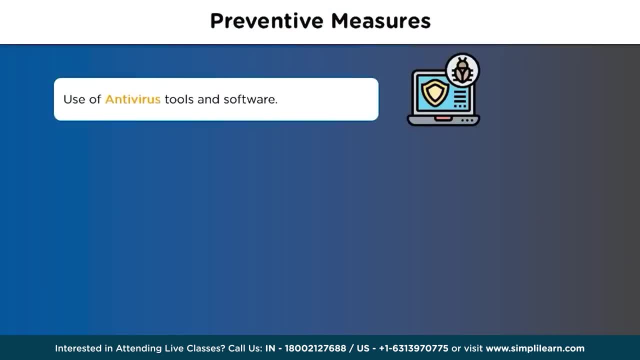 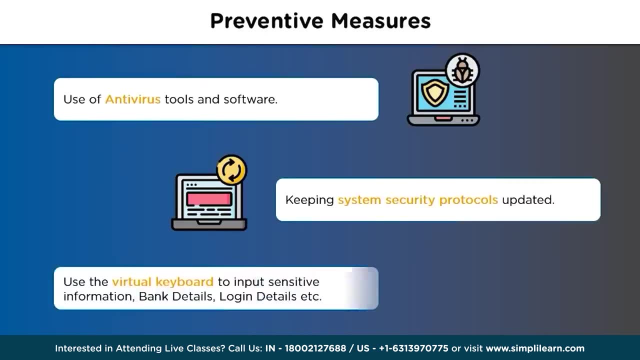 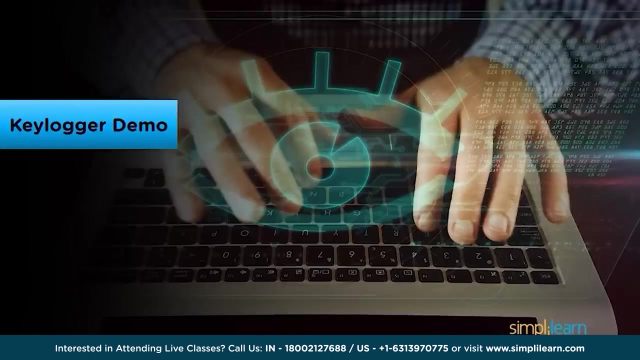 which can prevent the entering of malicious program into the system. then, keeping system security protocols regularly updated is also a good habit. and, lastly, using virtual keyboard to input our sensitive data, which may include bank details, login details or different passwords related to different websites. now that we have some understanding about the topic of key loggers, 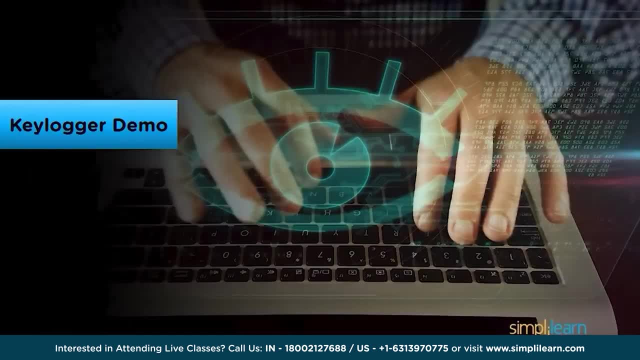 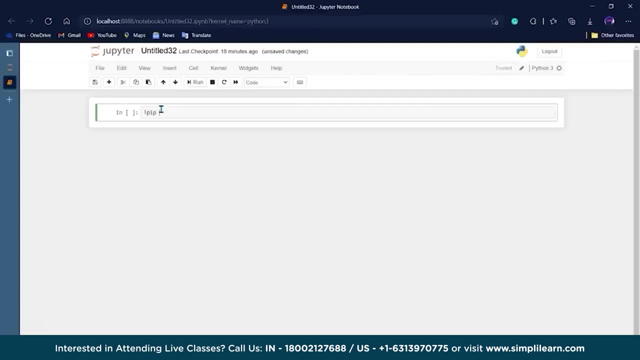 now that we have some understanding about the topic of key loggers. now that we have some understanding about the topic of key loggers, let's take a look at the demo to further increase the knowledge about the topic. for the first step, we have to download some of the important libraries that are: 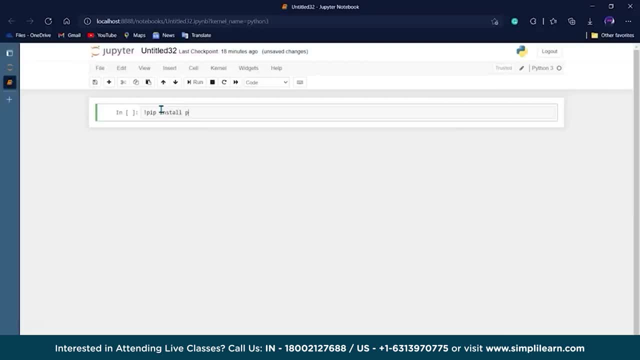 required into the system, which is this library. now we will run it. the system says the library is already installed into the system. now let's take a look what exists in the system. so let's run that, so that in the system we have a flo reduced keeper. 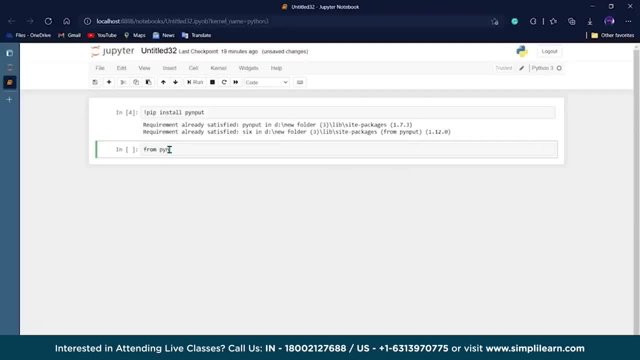 so let's run that so that in the system we'll see what exactly modules are required from the particular library. from this library will import tab. we will import the keyboard module, which will help us to record the data that we type on the keyboard. now, from the same we also import: key module and the listener module- key module and the listener module now from the same. we also import key module and the listener module and also access the new files into the cloud through the cloud enemies tricks and also access the new files into the cloud again from the data. and must remember. important is that this is a laptop application also and Promoting your Linux document is simple, even if you have an actual service and keep prompts while you are doing constructions. 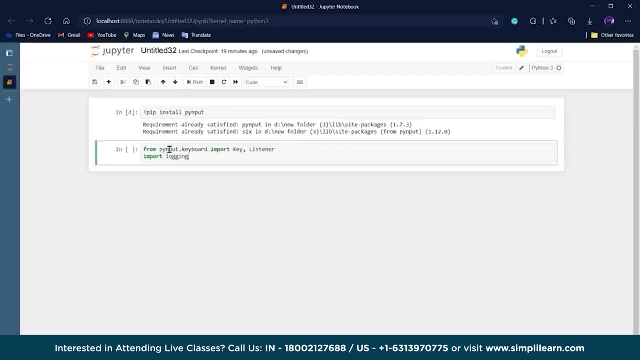 the logging module, which will help us to record the data into a log file. for the next part, we will write a piece of code that will allow us to save the data that is recorded by the program into our text file that will be named as key underscore. 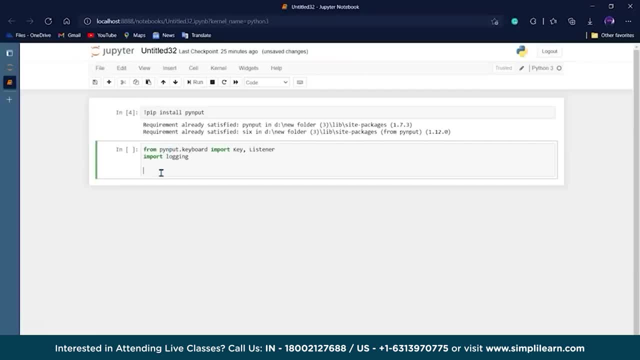 log text file along with the date and time stamp. let's take a look now. we'll provide it with the file name that will be given as key log dot txt file, and also so the part where the format of the data is recorded. put the brackets over here. 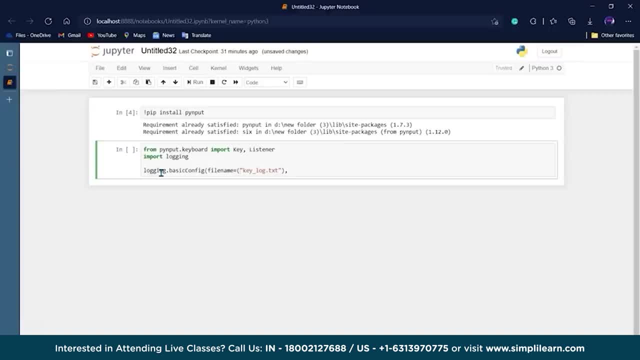 to contain the file name. now we'll write the format in which the data will be recorded into the log file, which will be given as the format would be the message and the time stamp which would be given as. the time stamp which will be given as. the time stamp which will be given as: 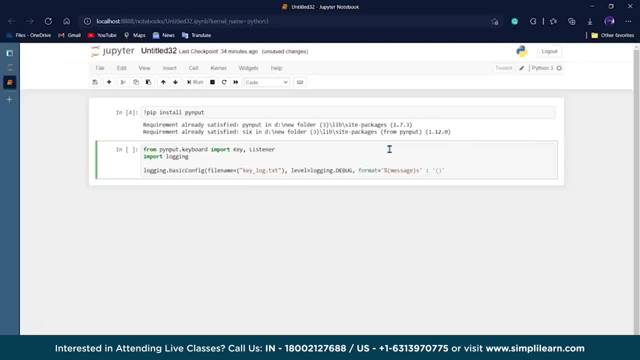 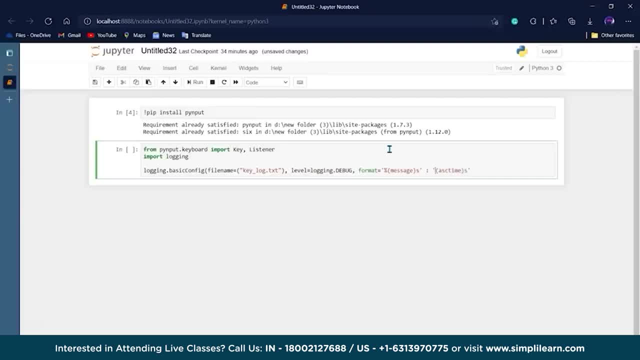 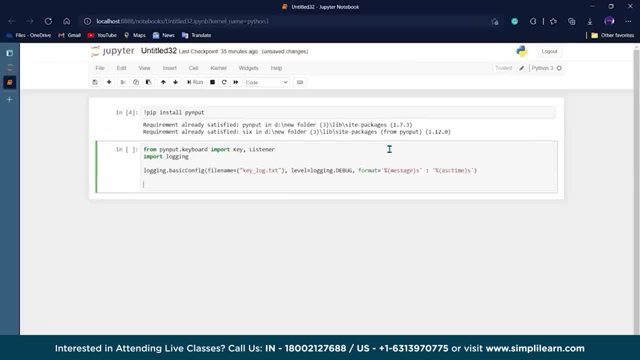 percentage and ending it with the bracket percentage, and ending it with the bracket percentage and ending it with the bracket. now for the next step. we will design two of the functions that will be used. now for the next step. we will design two of the functions that will be used. 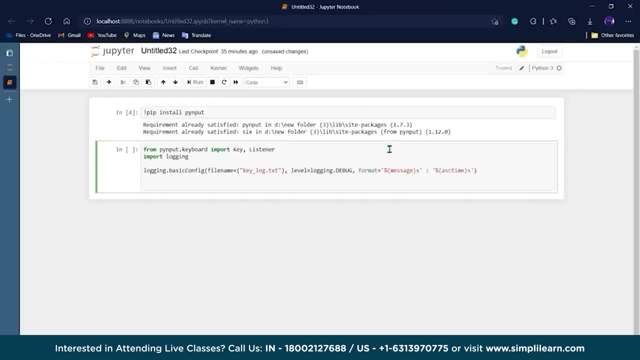 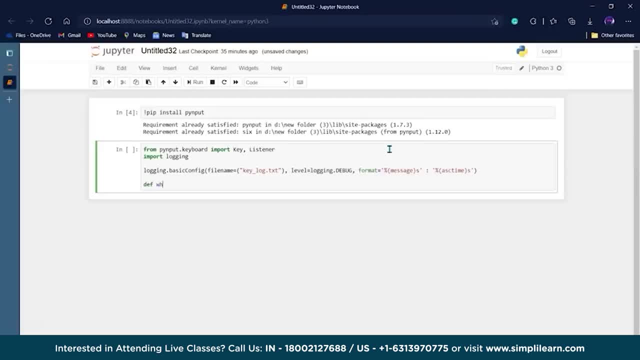 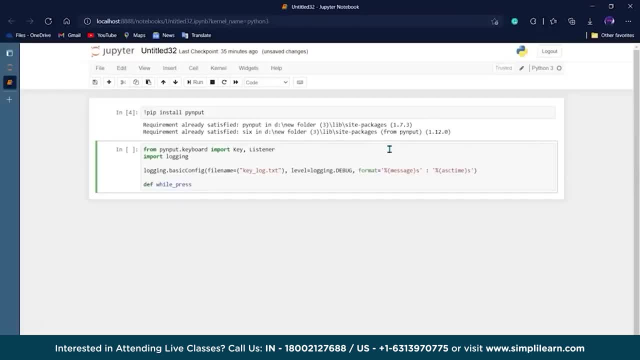 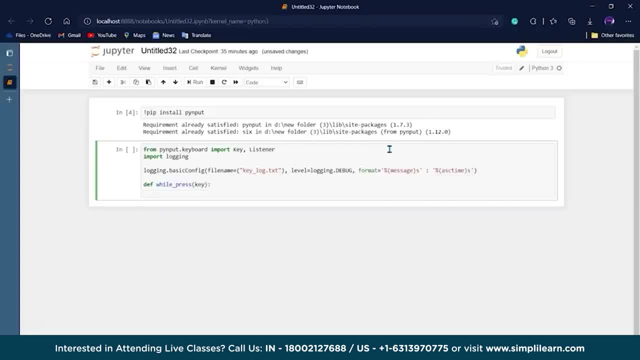 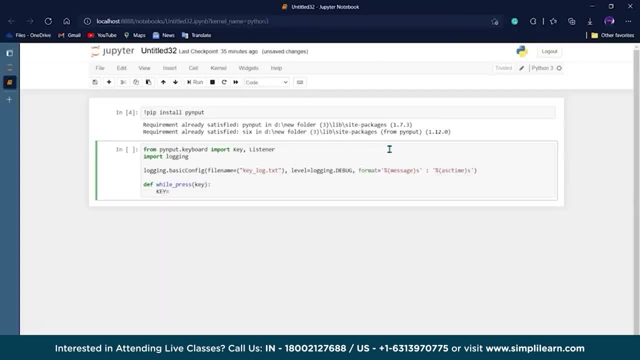 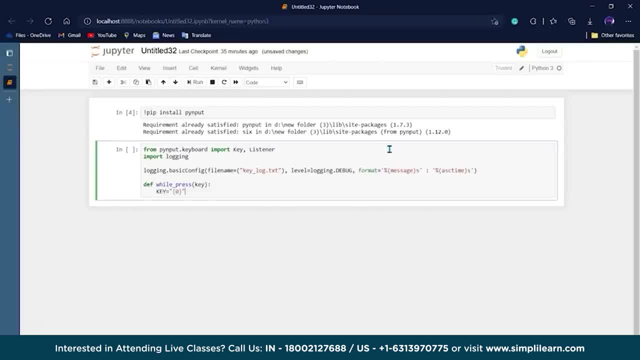 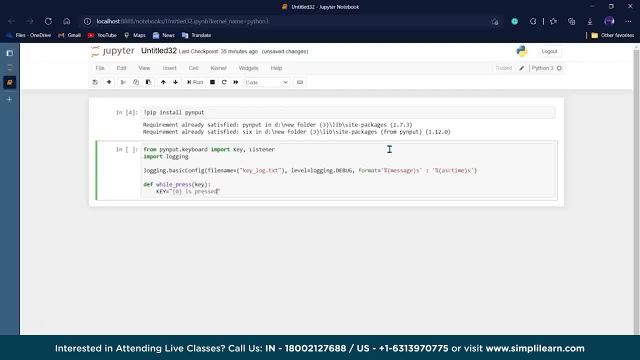 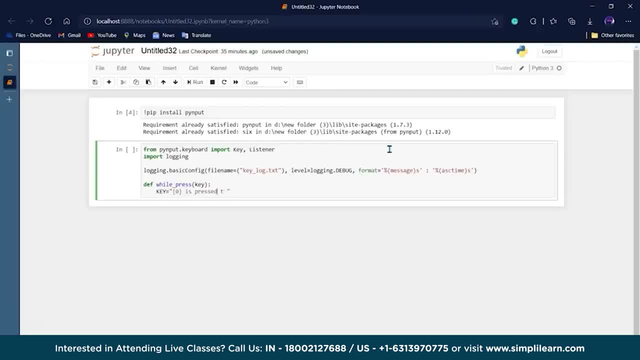 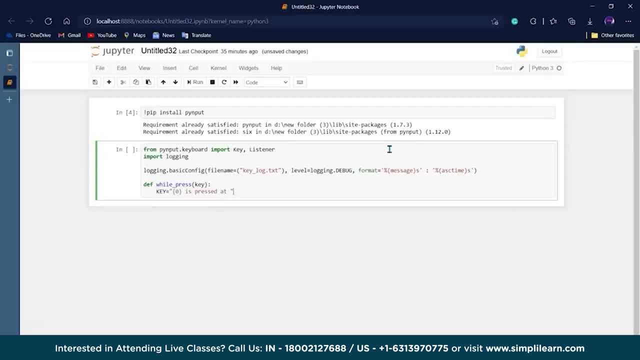 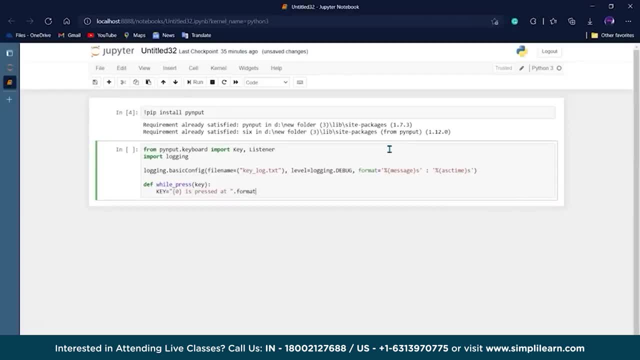 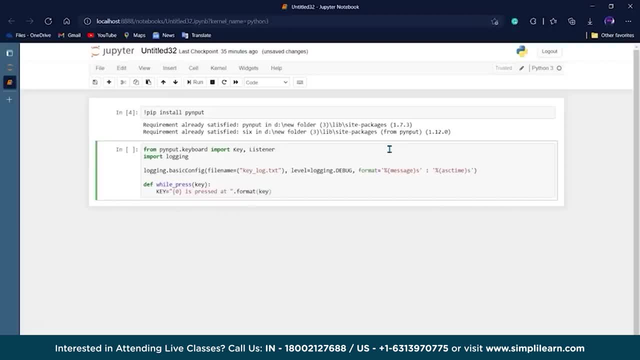 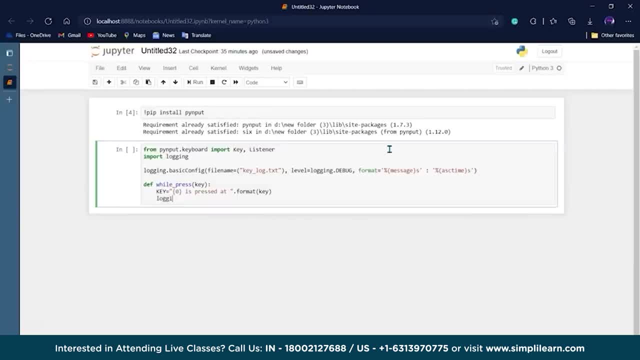 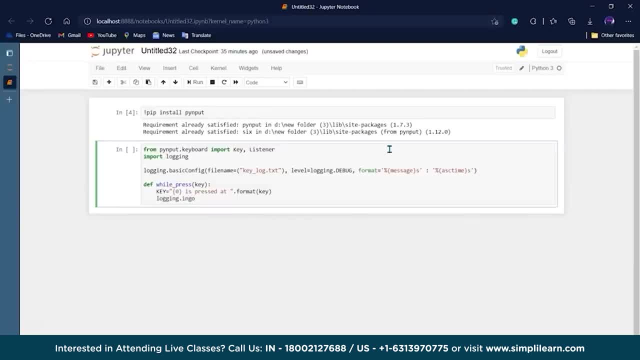 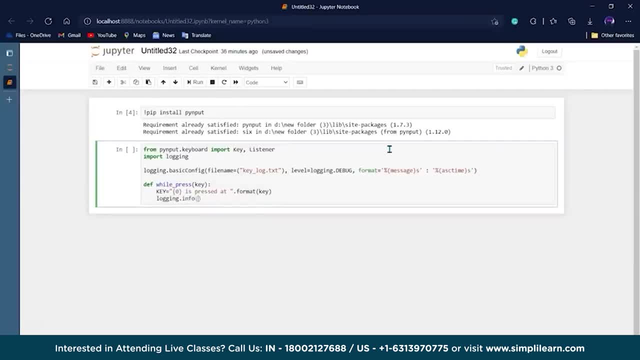 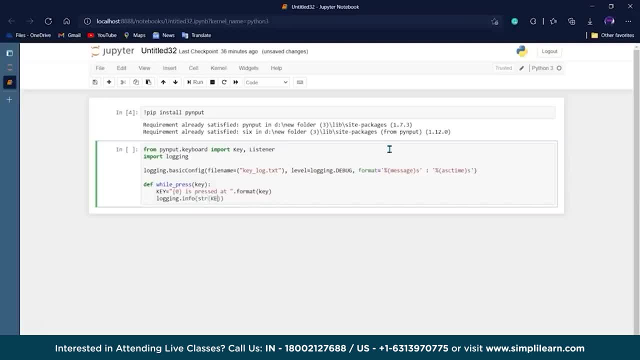 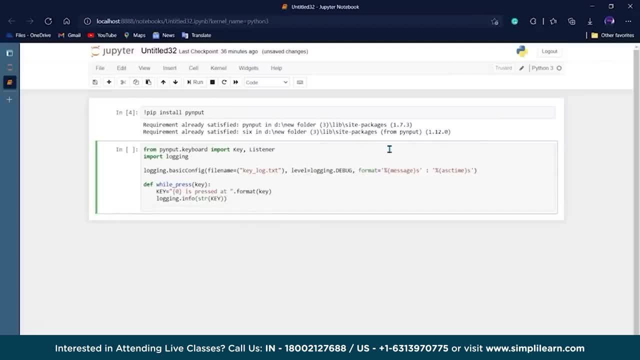 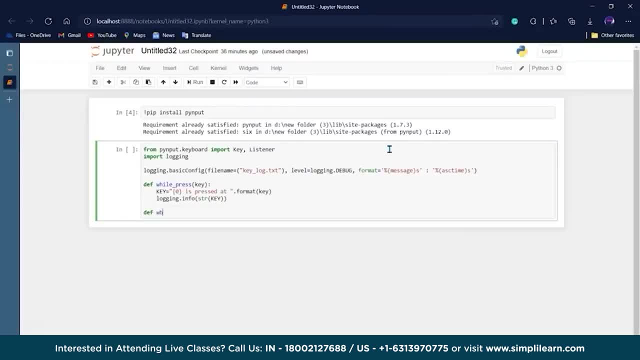 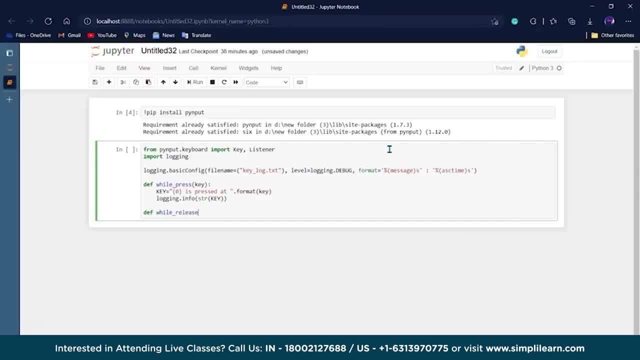 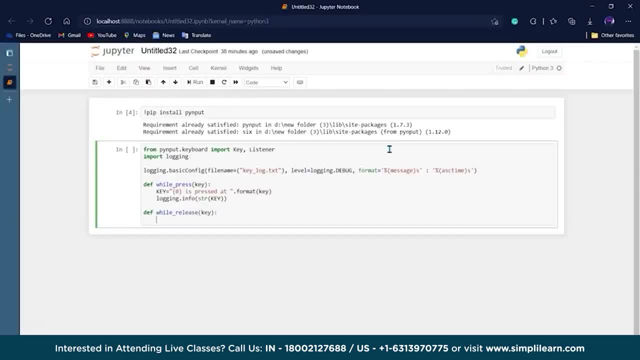 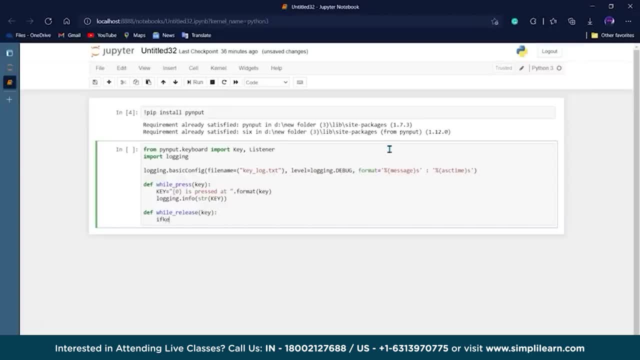 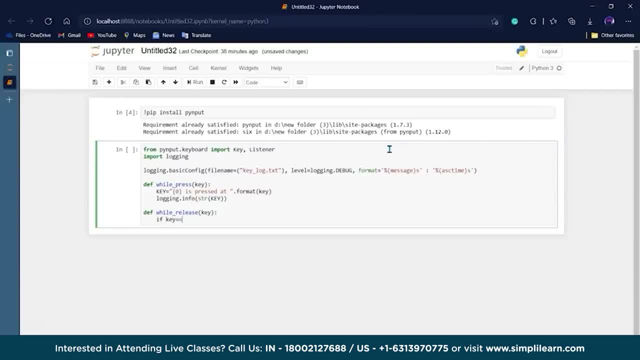 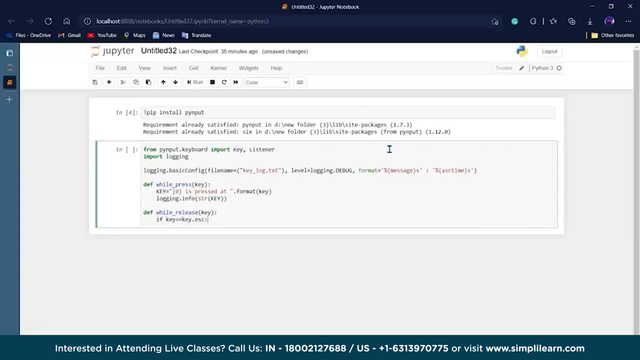 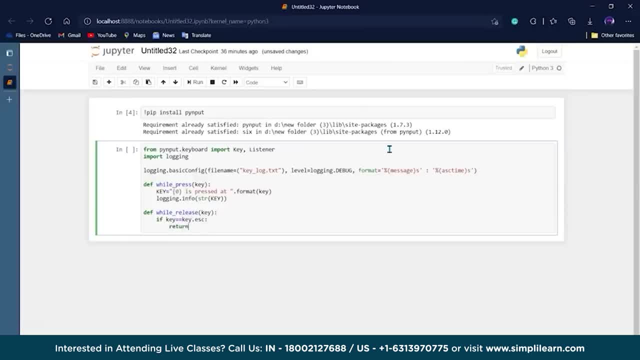 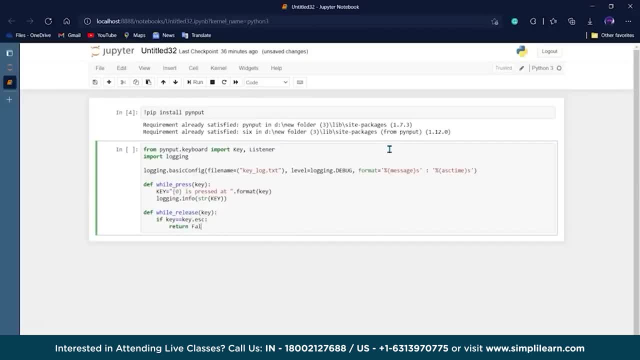 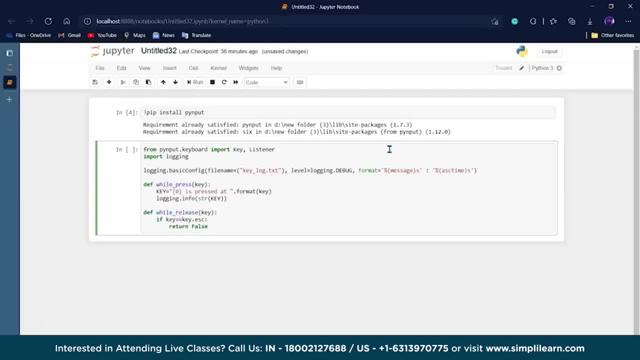 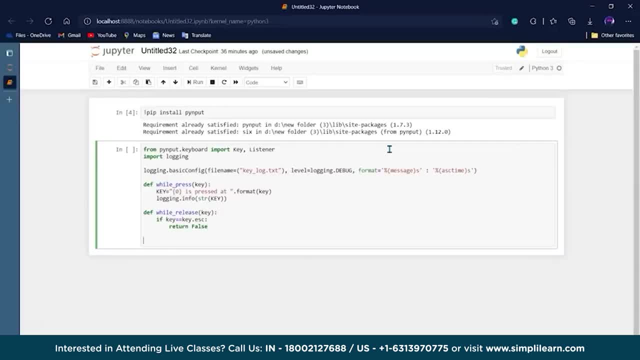 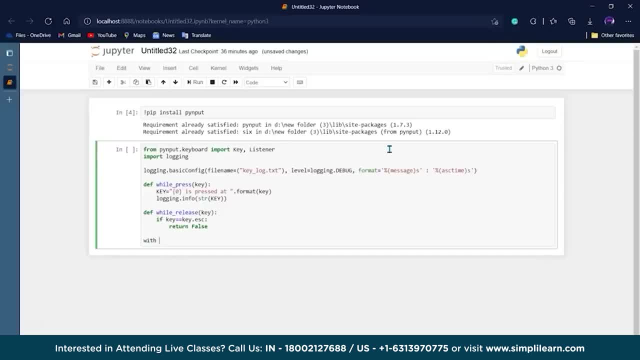 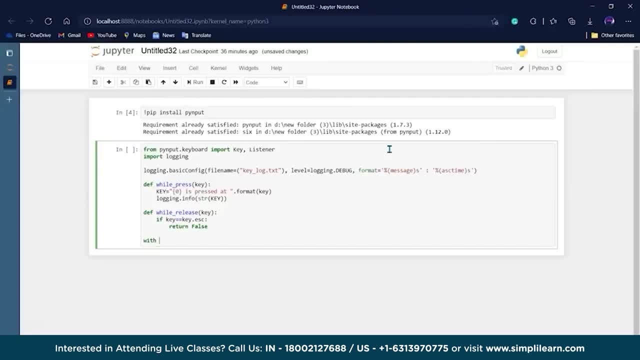 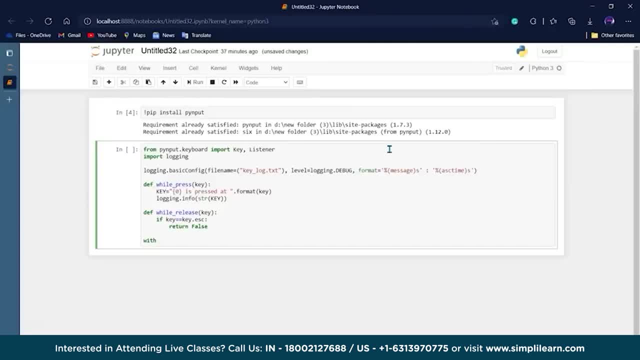 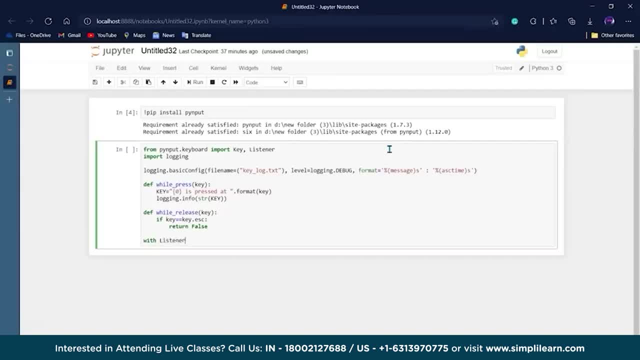 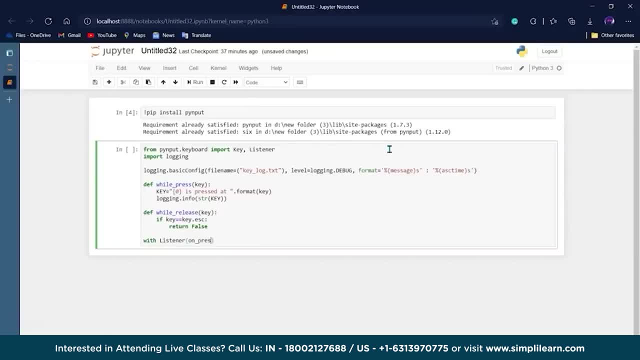 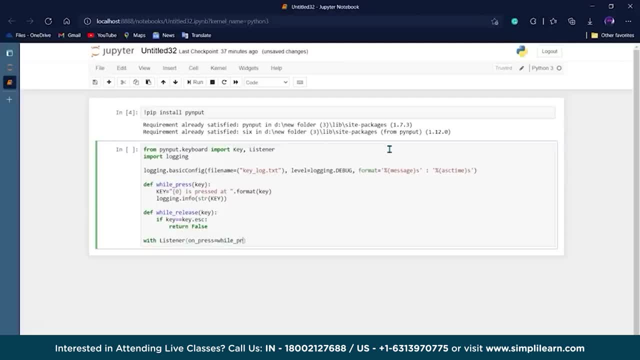 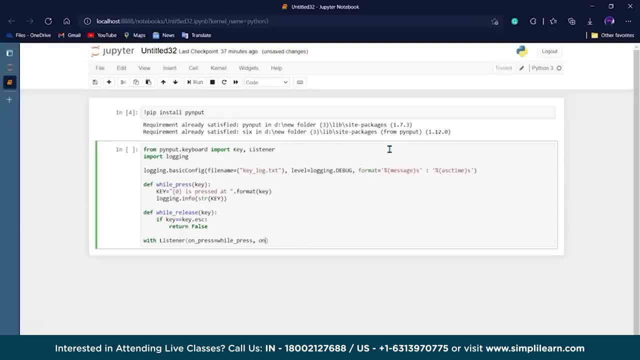 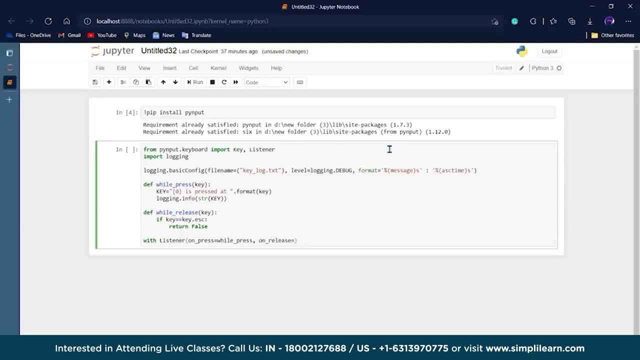 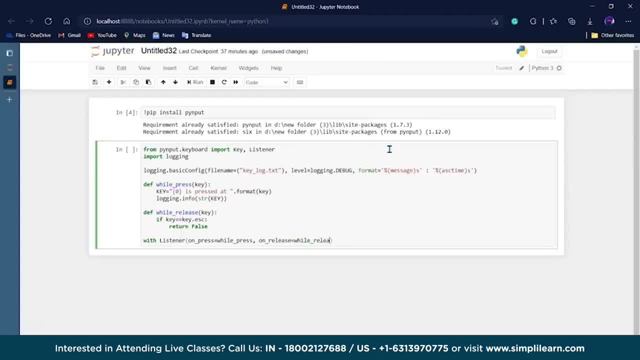 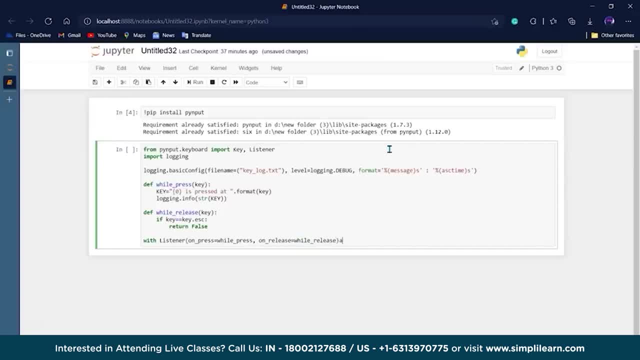 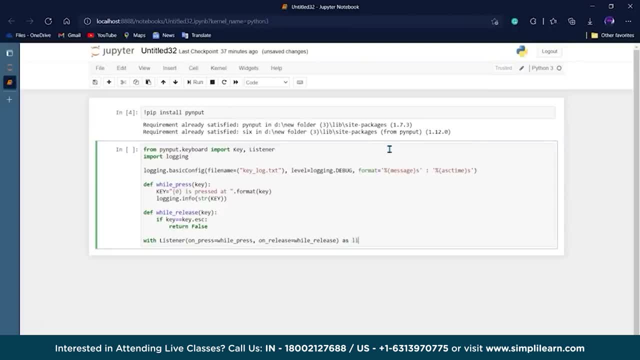 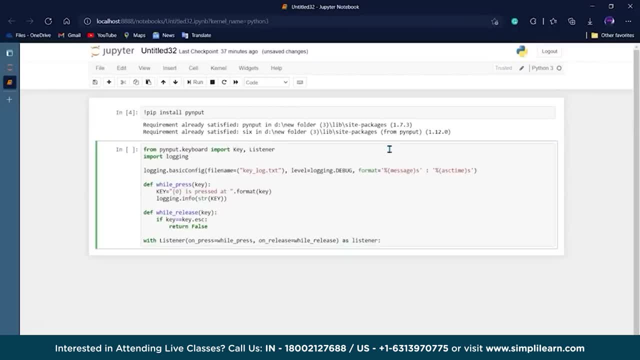 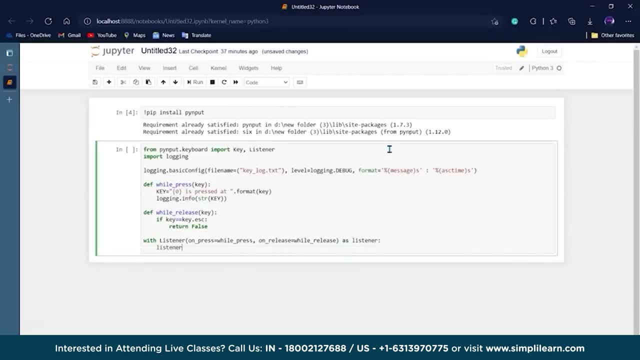 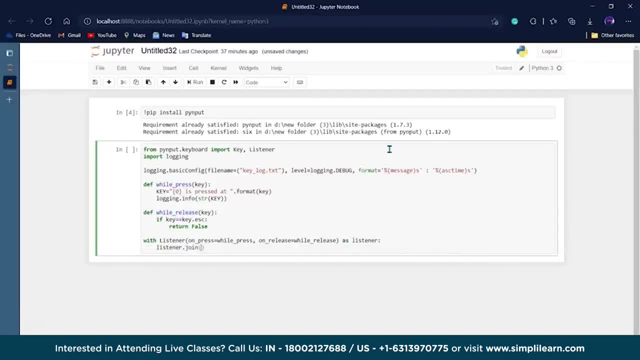 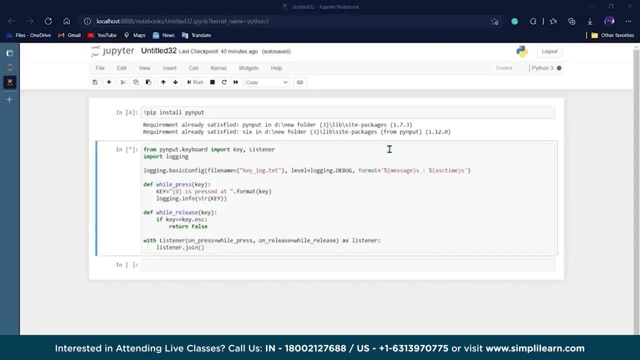 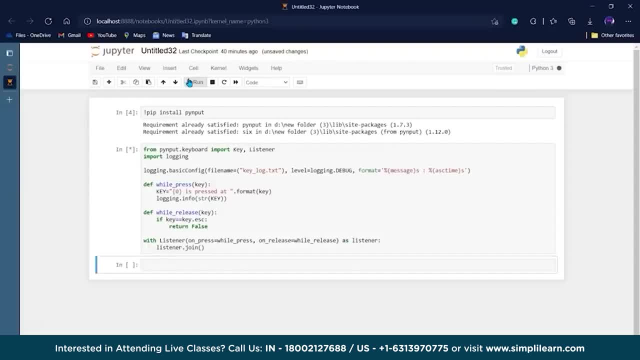 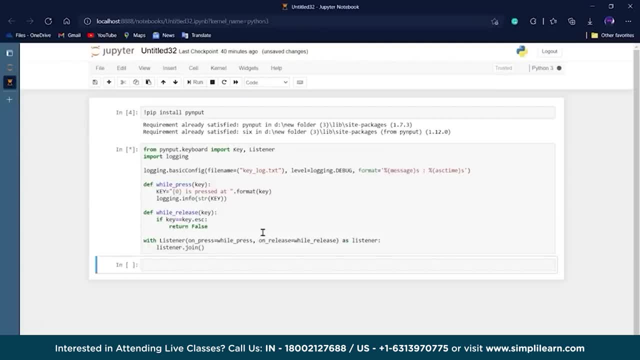 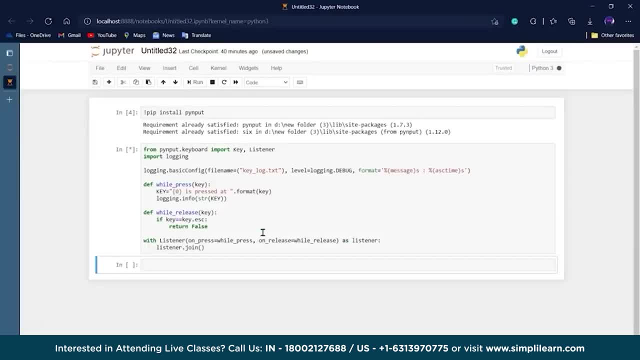 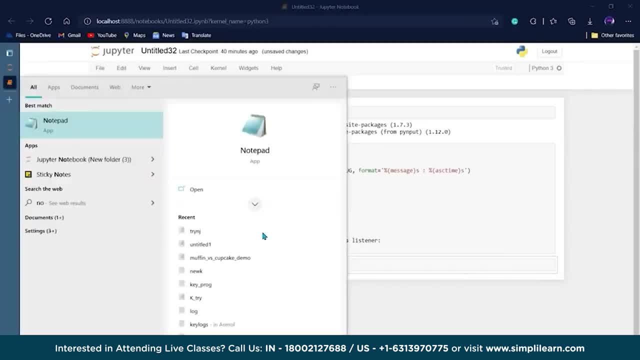 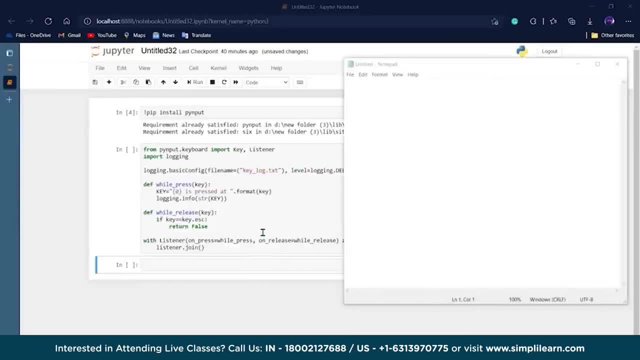 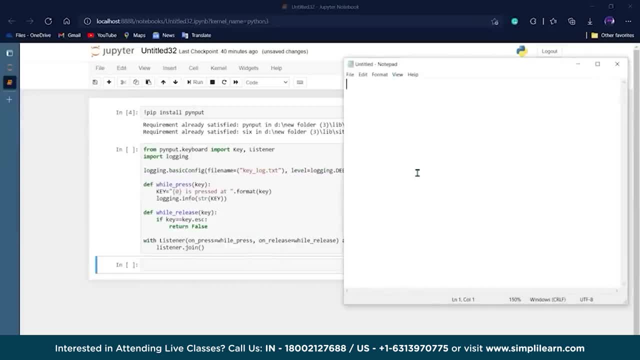 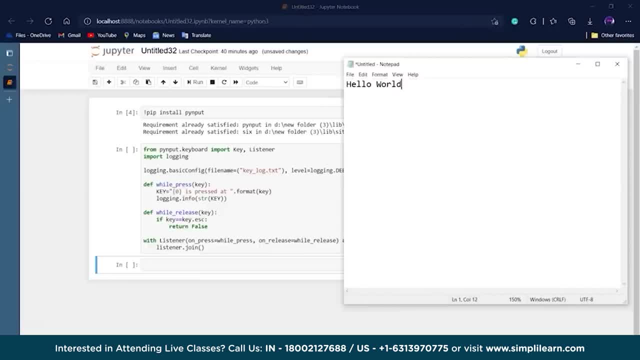 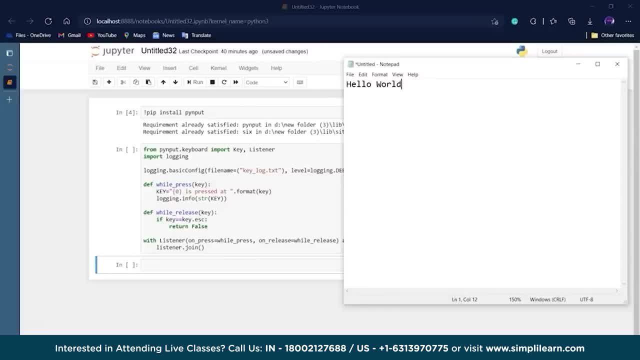 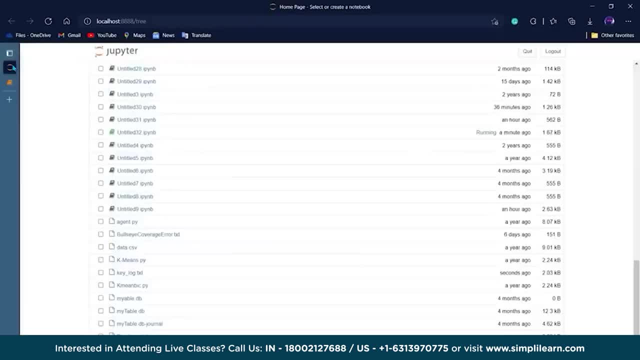 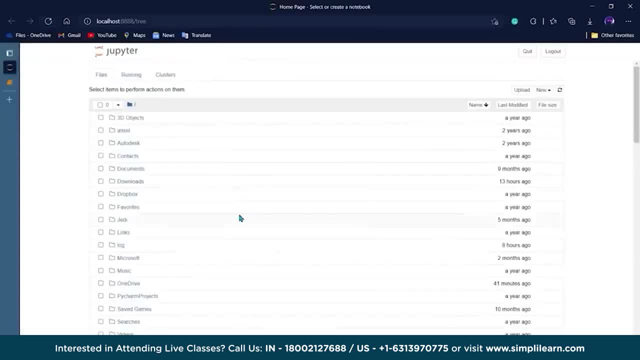 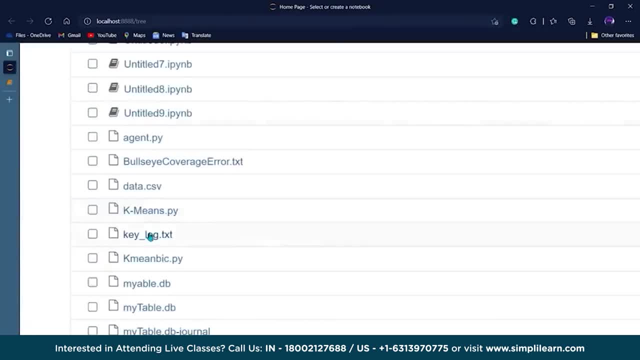 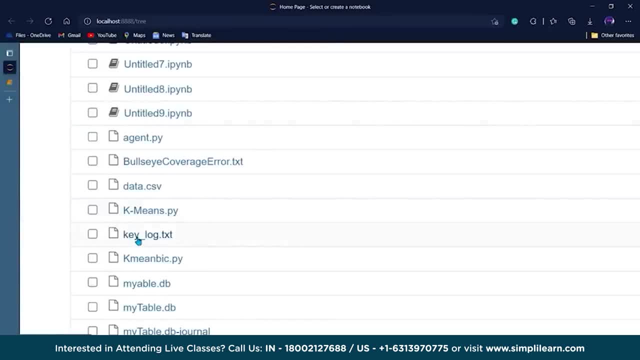 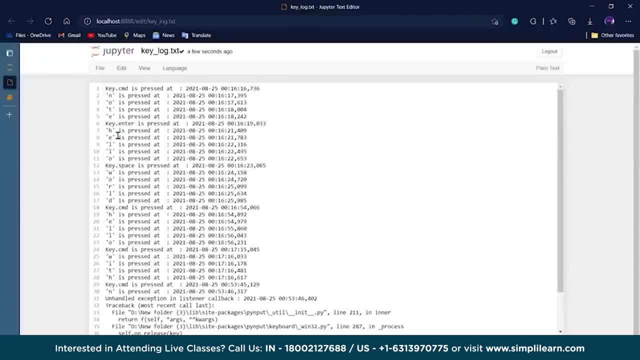 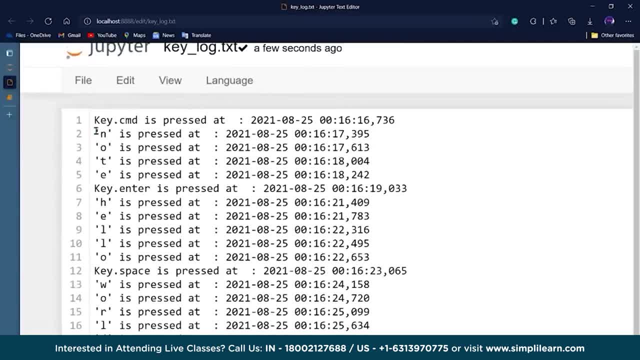 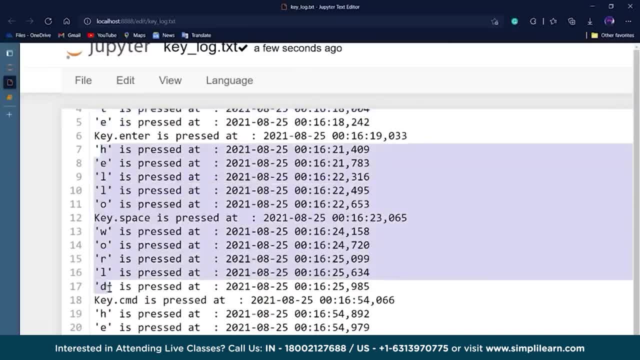 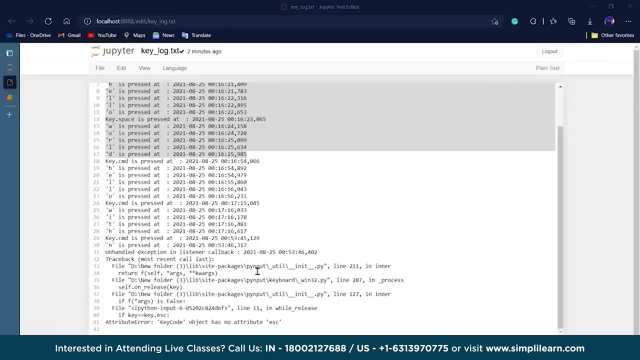 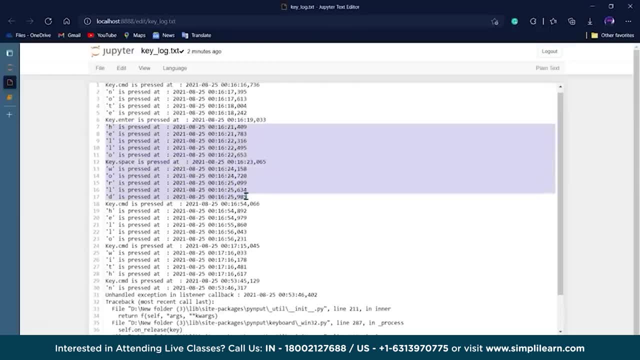 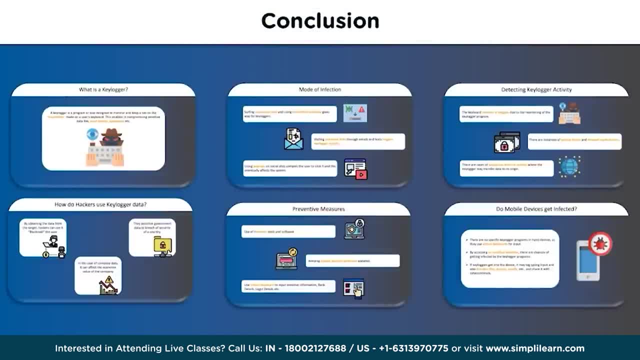 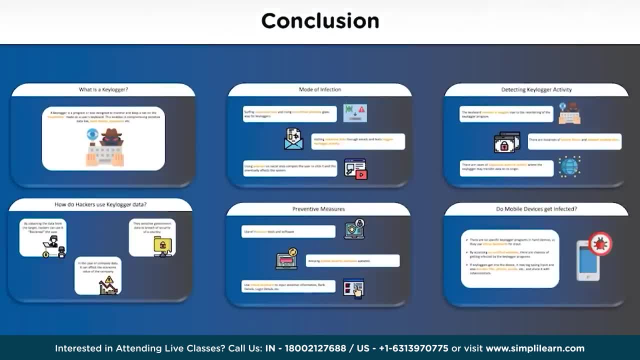 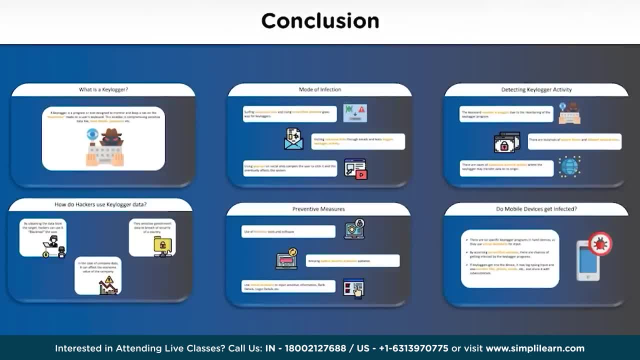 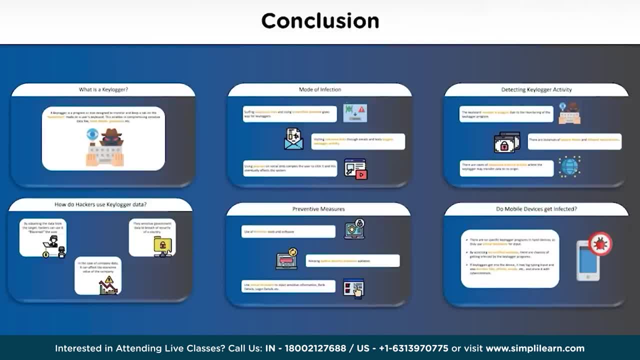 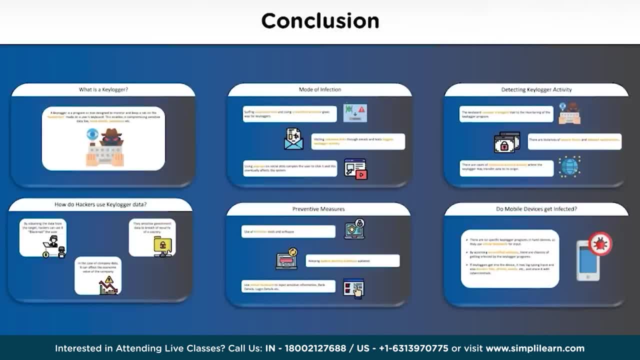 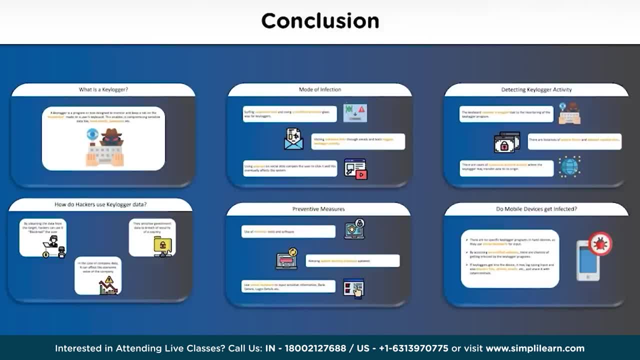 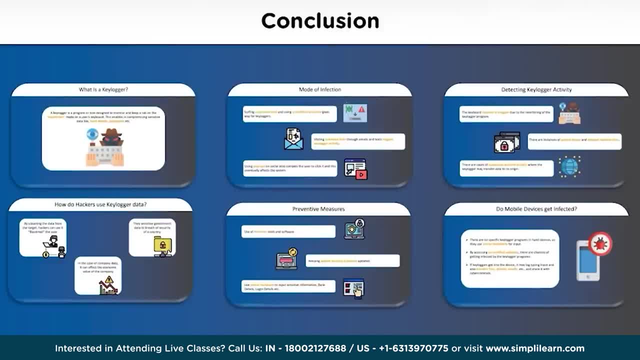 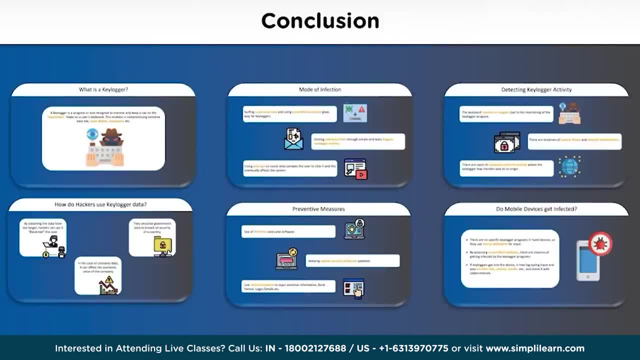 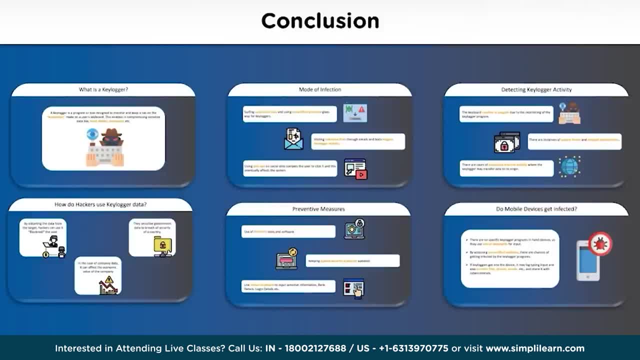 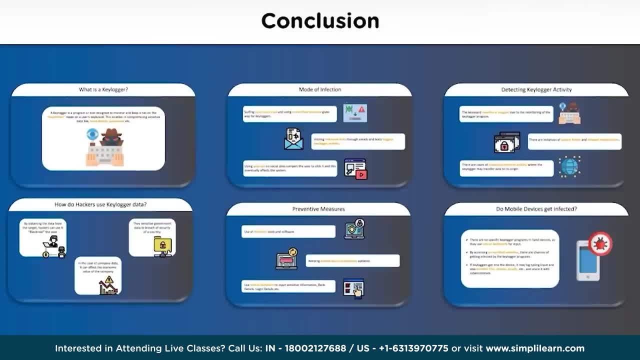 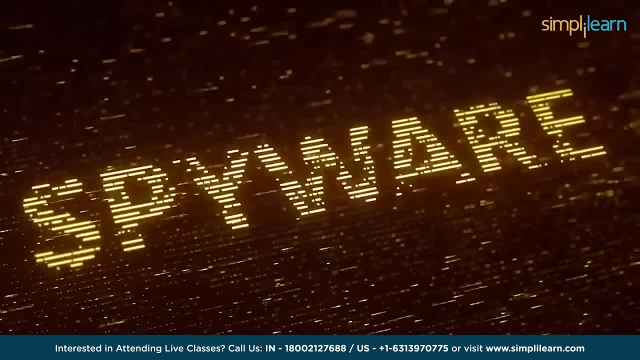 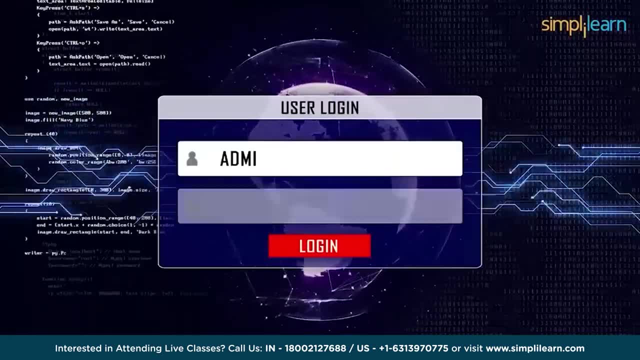 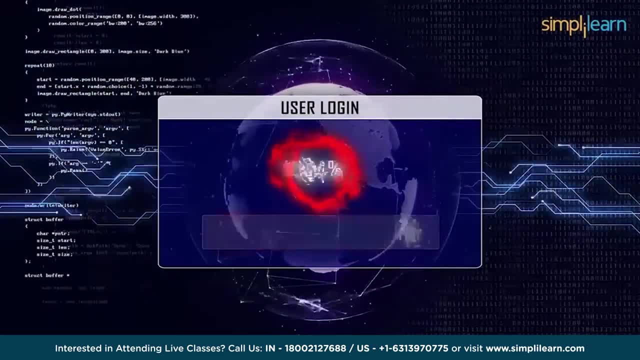 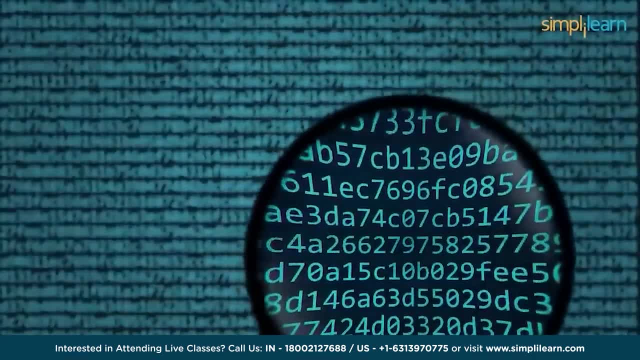 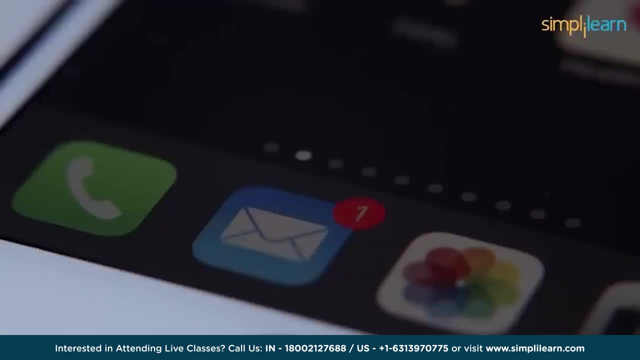 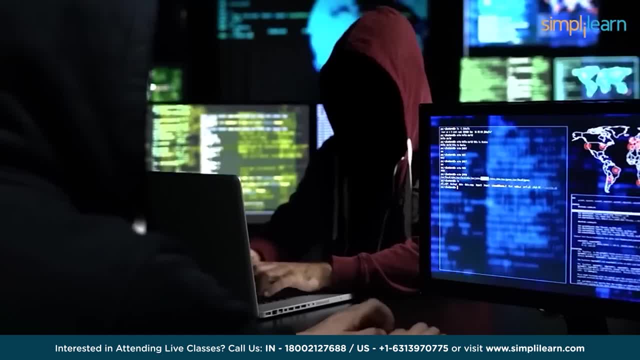 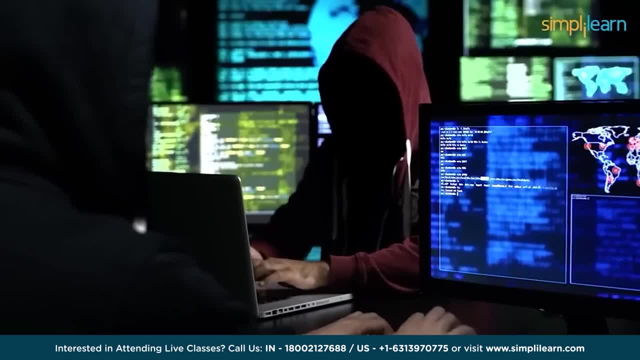 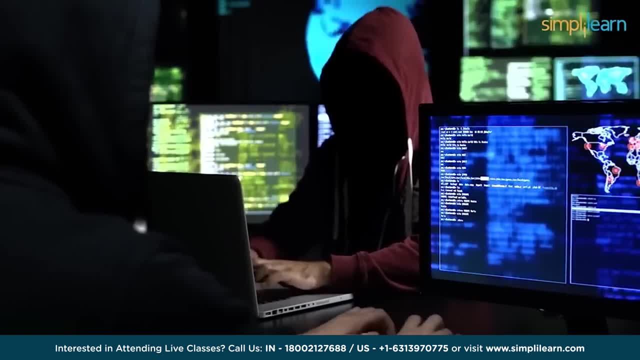 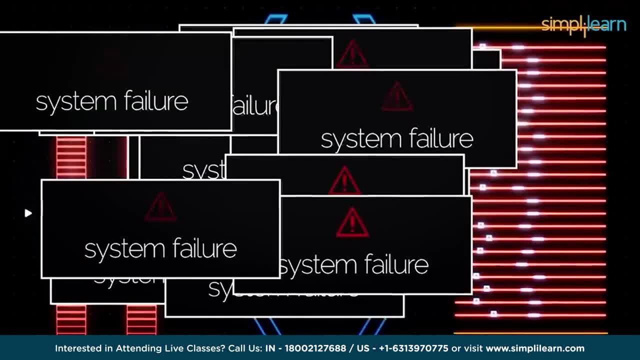 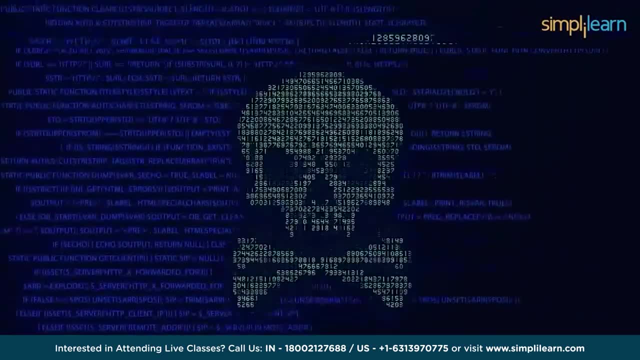 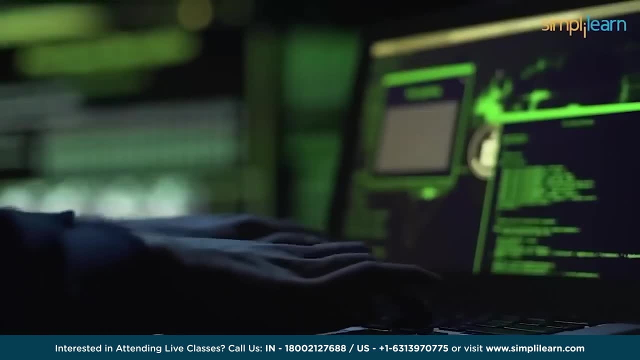 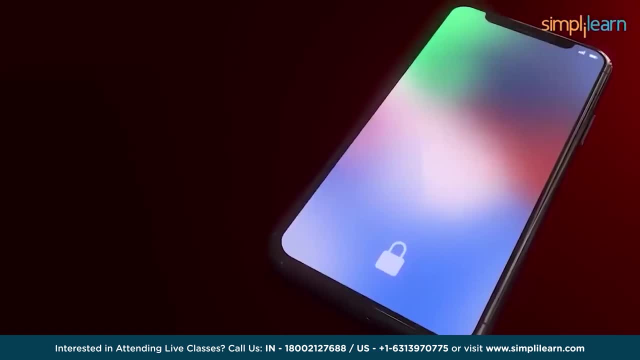 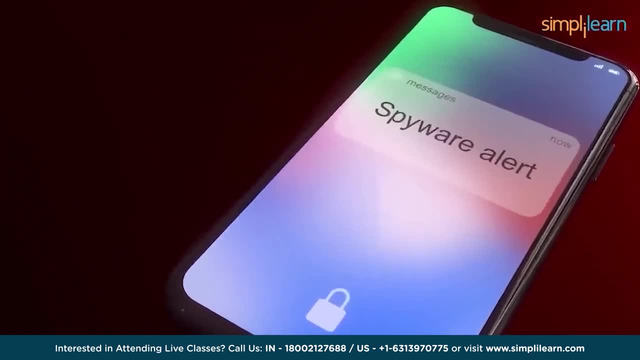 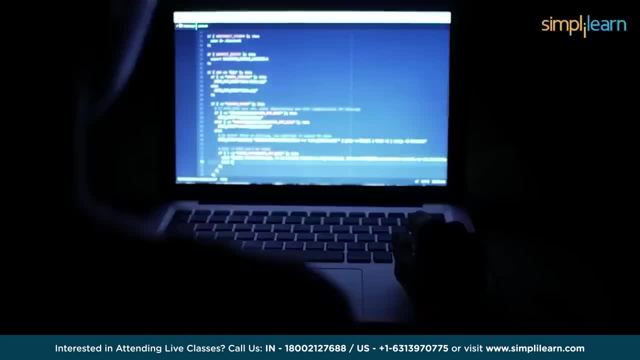 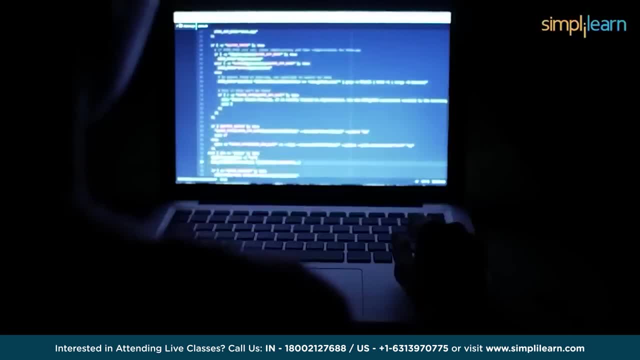 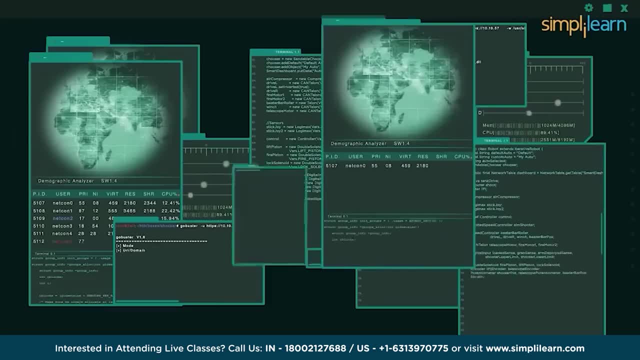 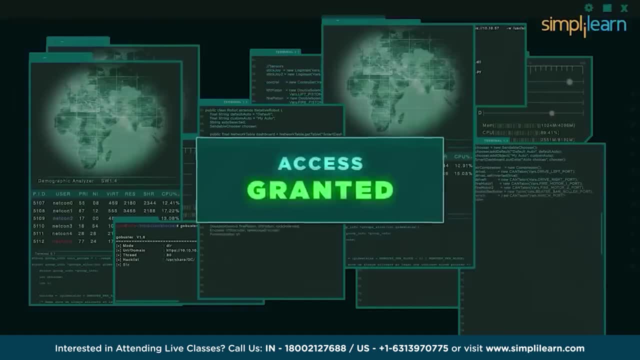 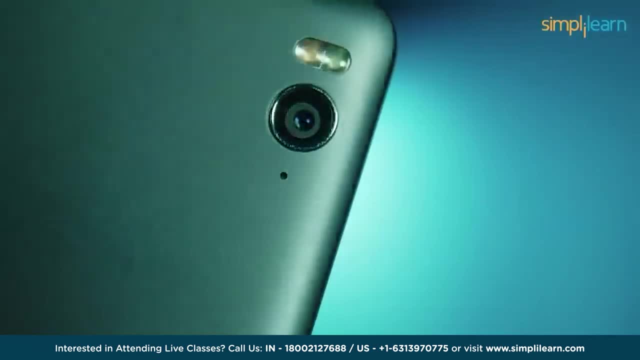 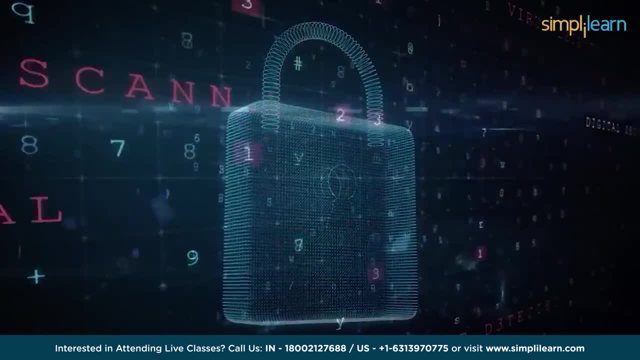 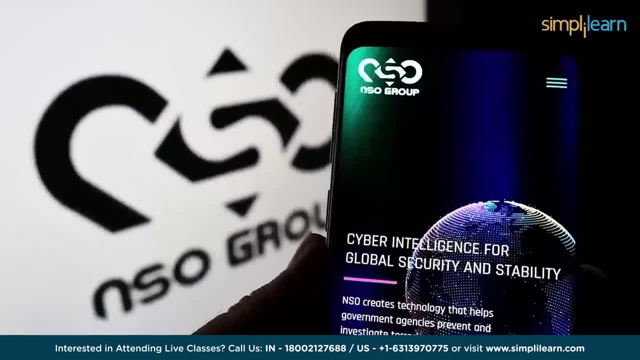 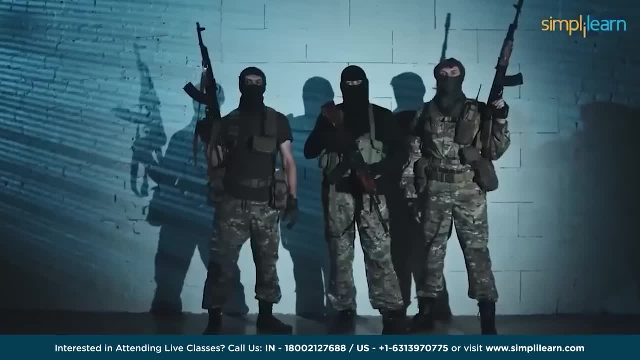 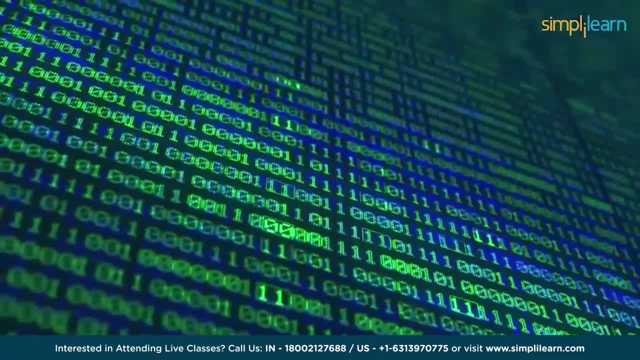 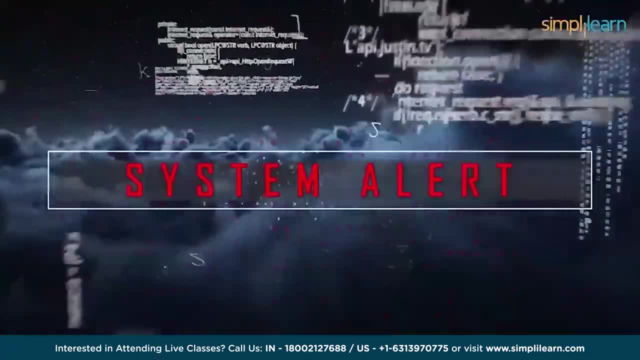 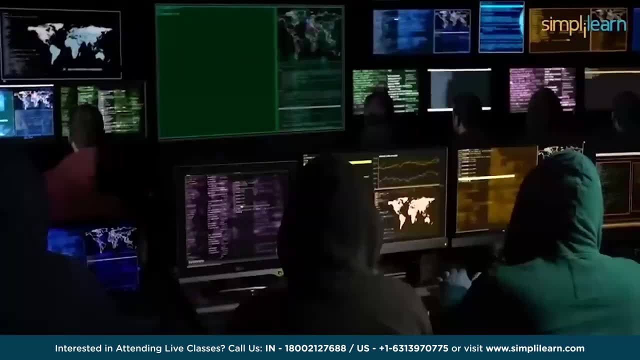 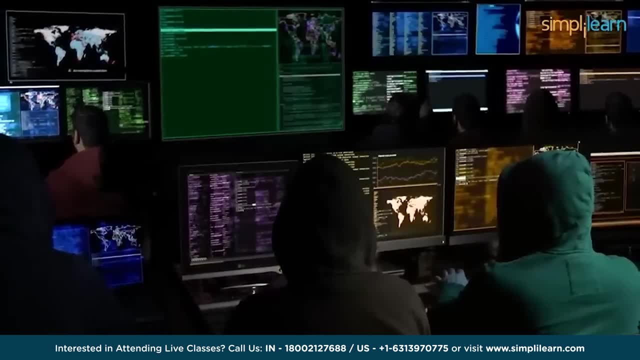 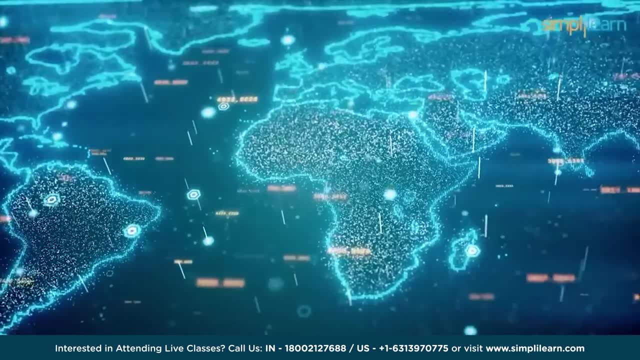 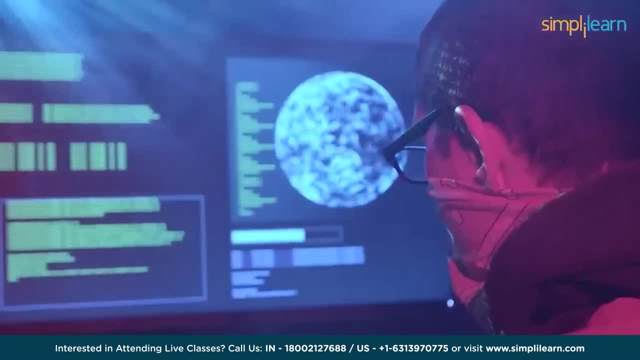 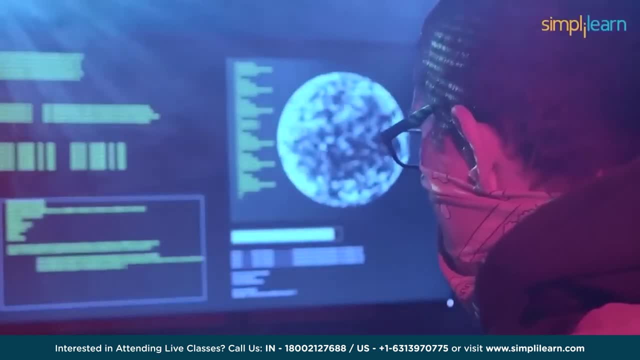 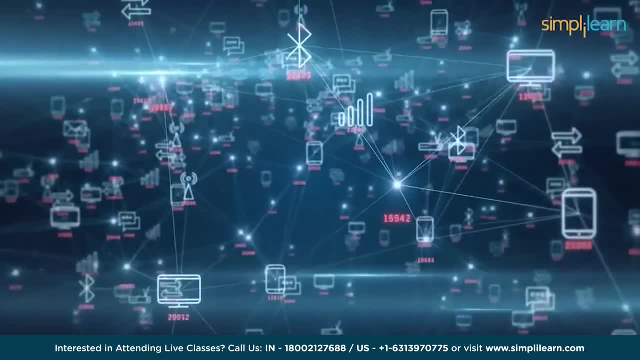 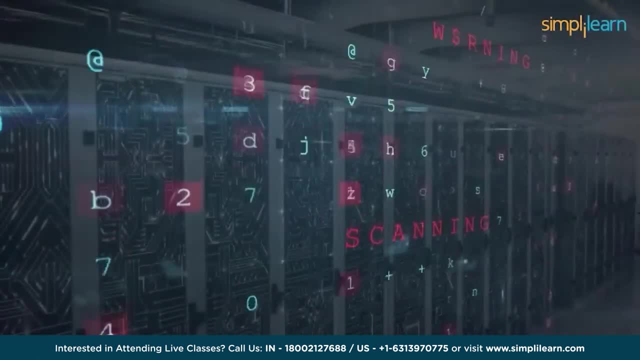 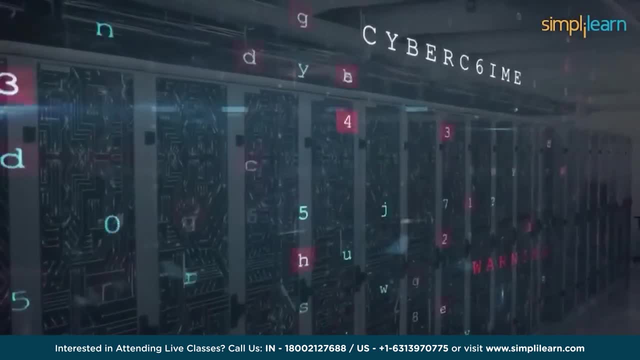 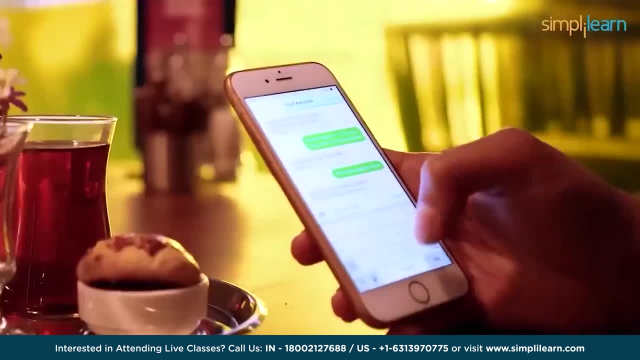 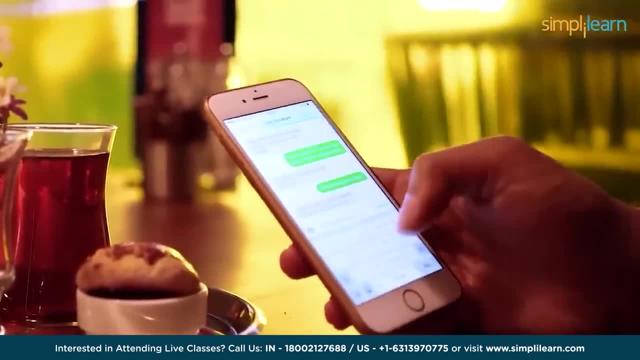 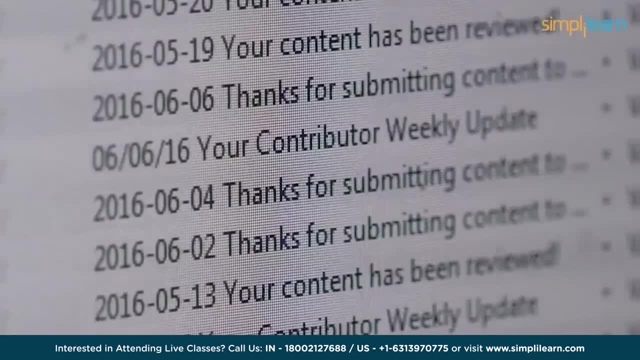 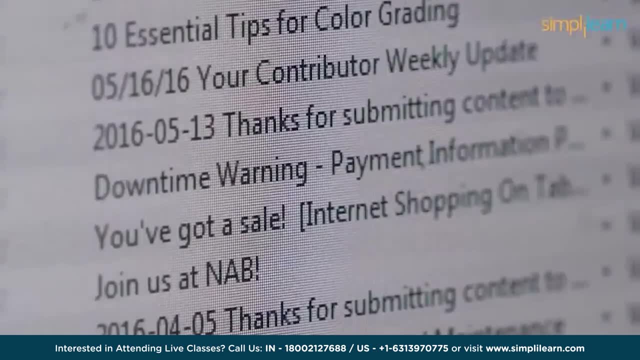 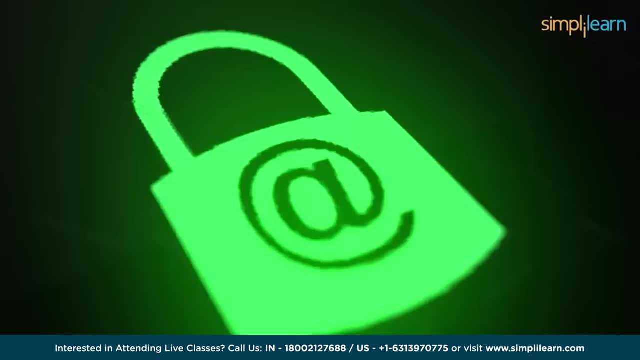 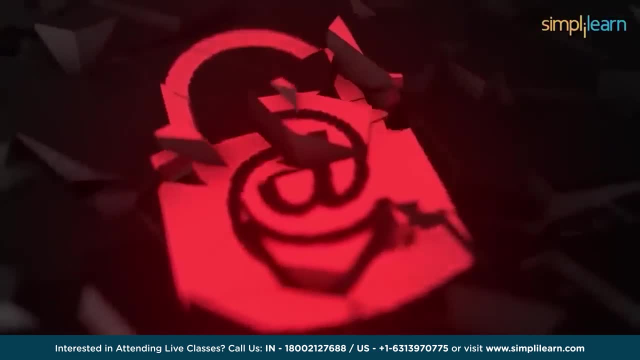 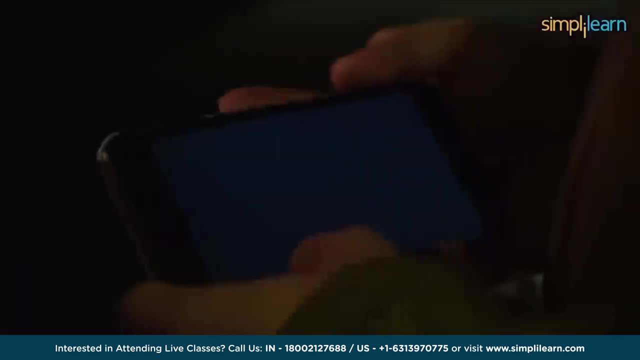 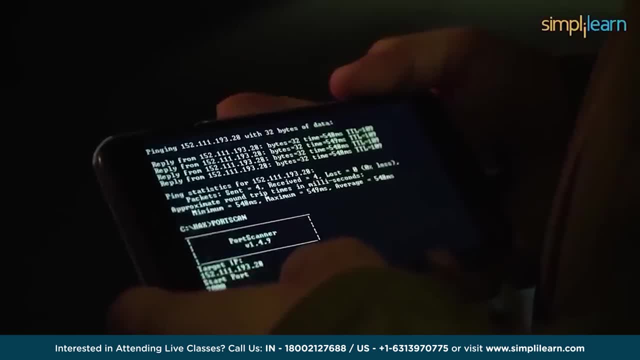 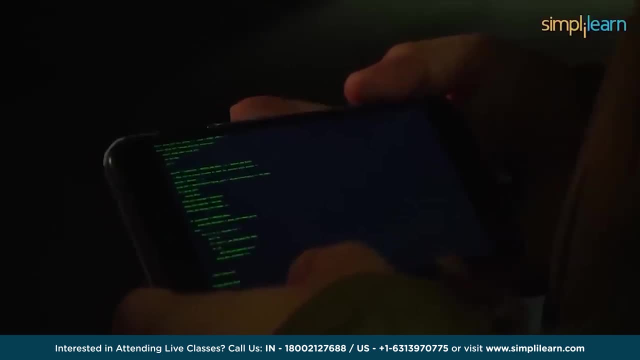 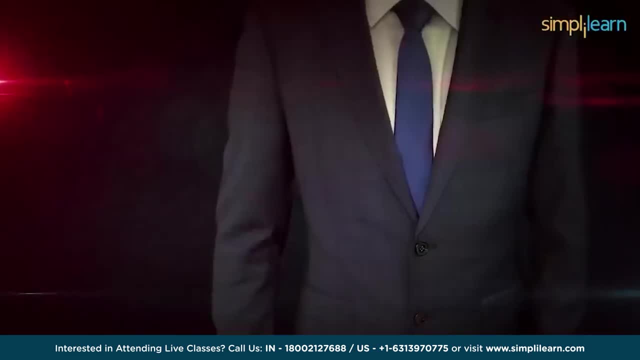 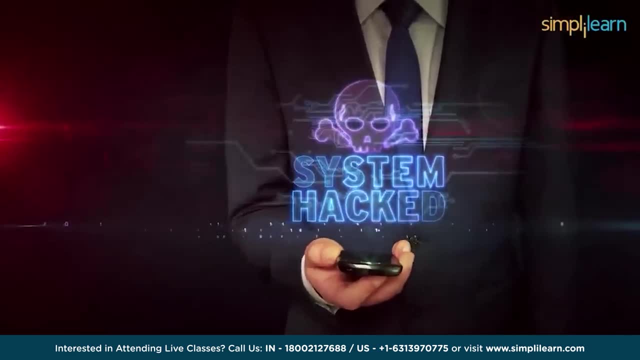 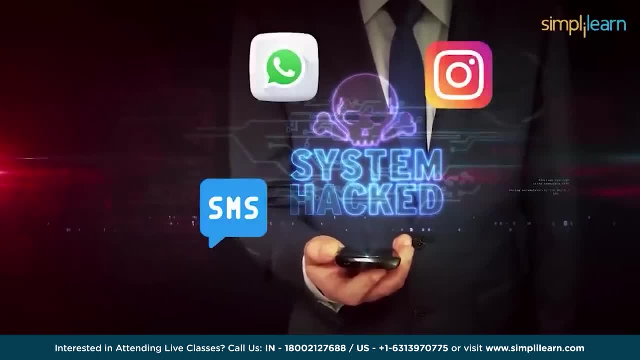 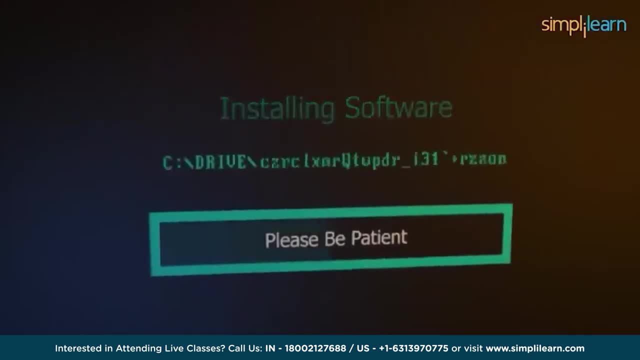 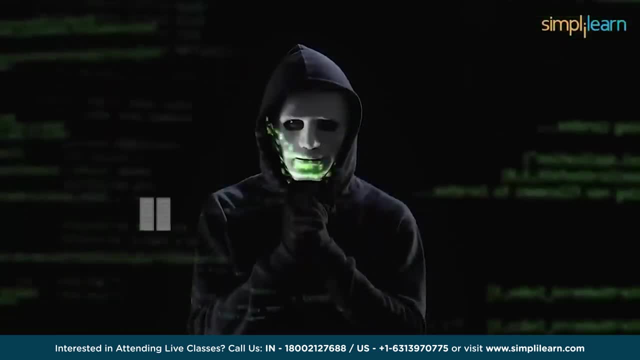 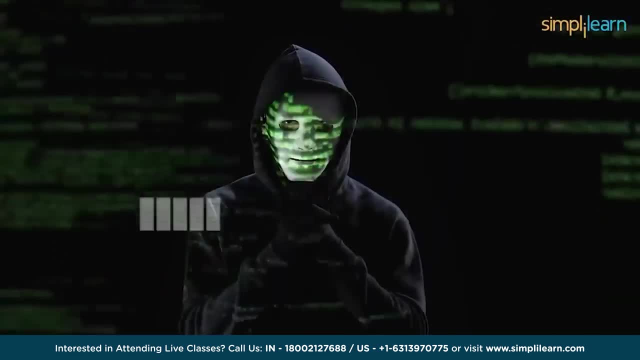 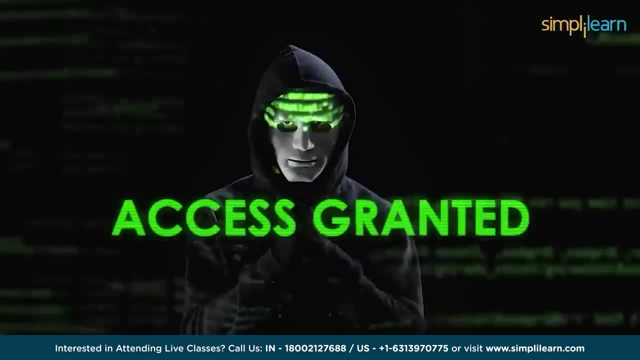 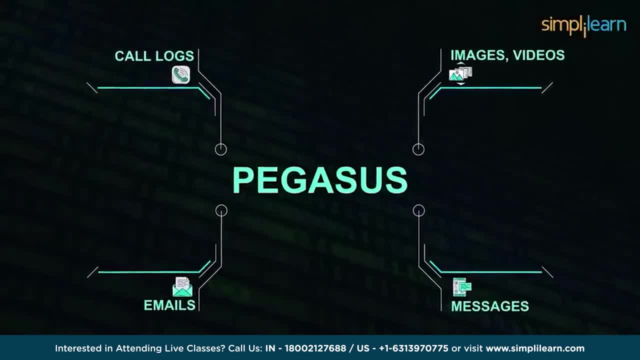 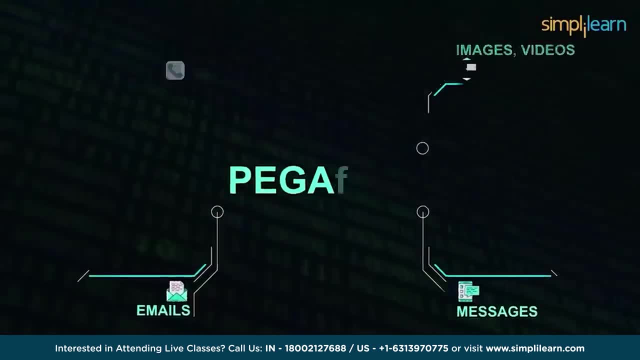 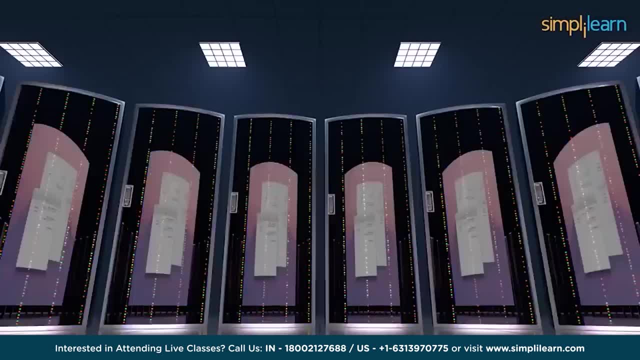 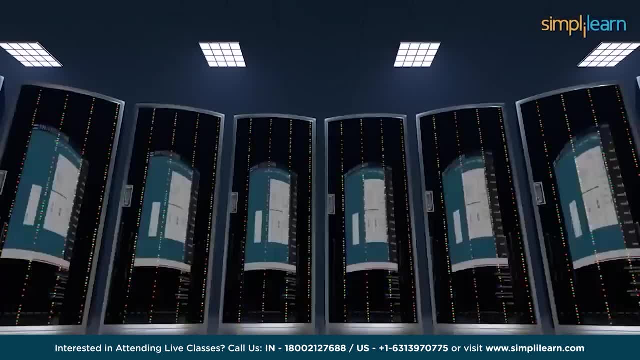 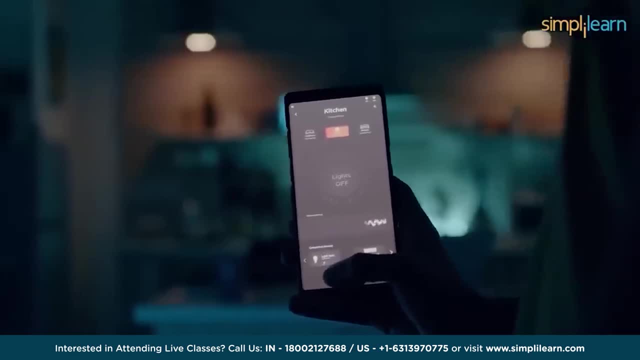 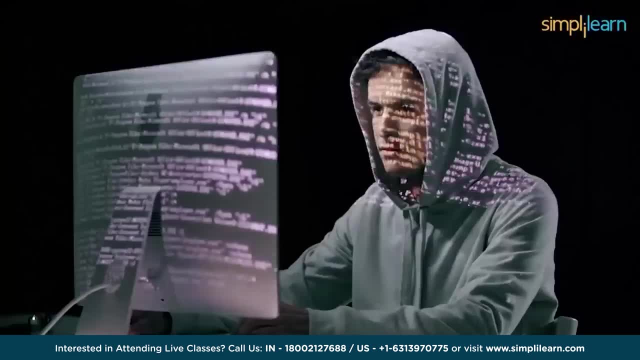 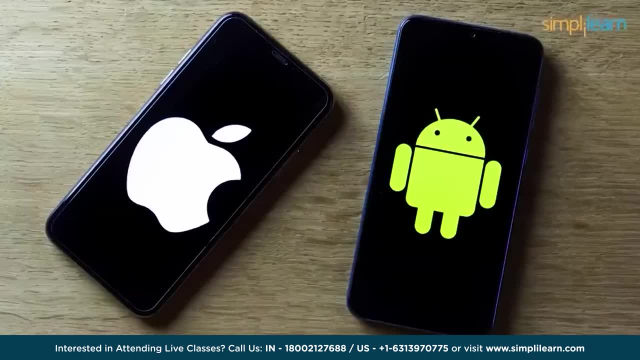 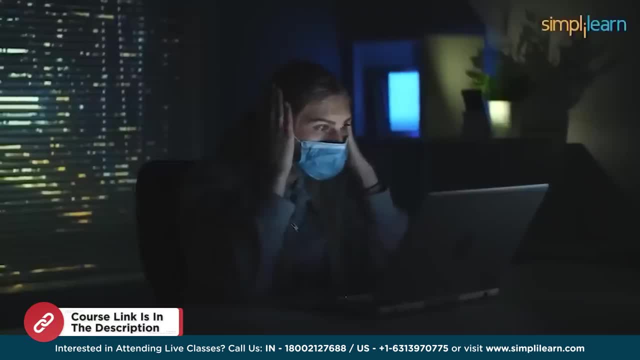 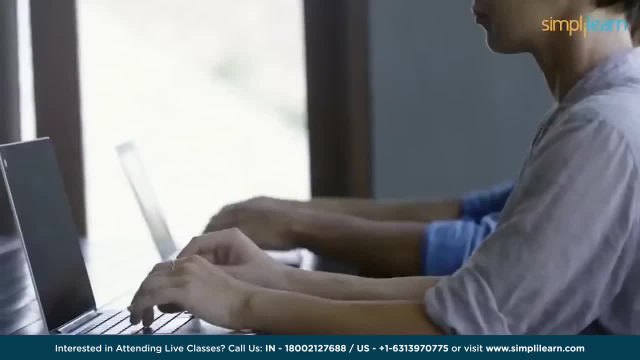 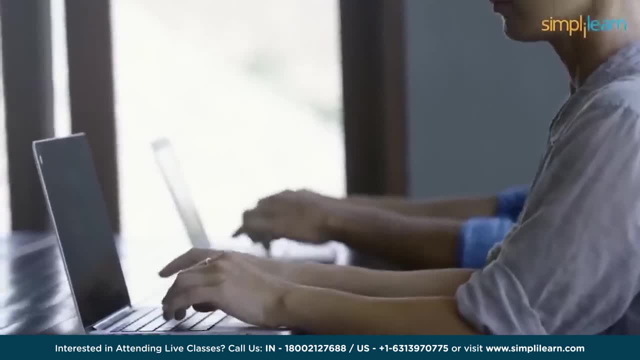 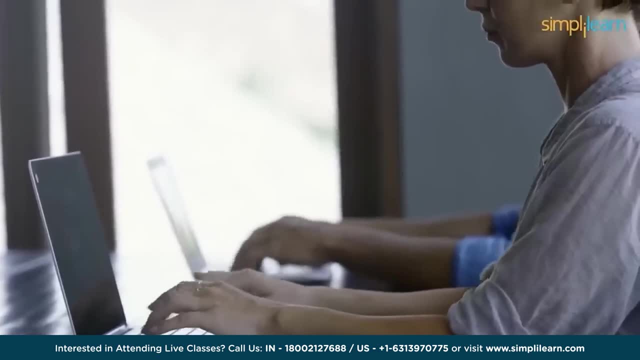 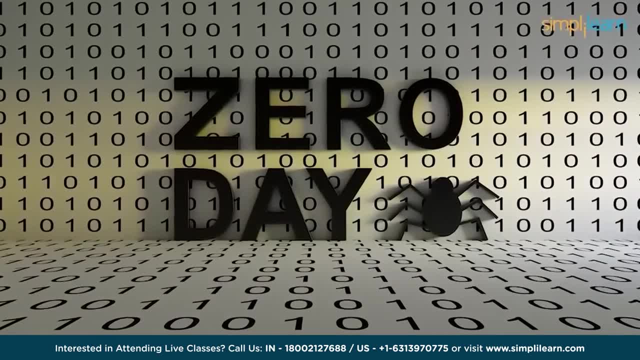 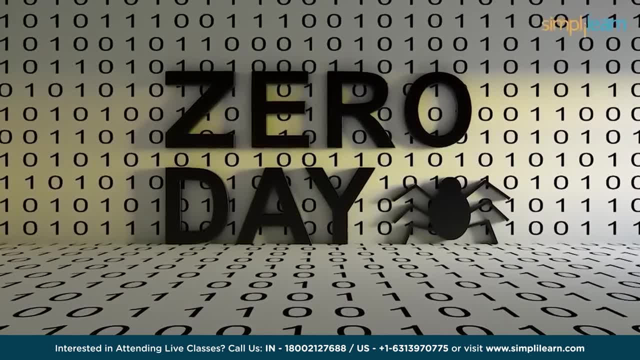 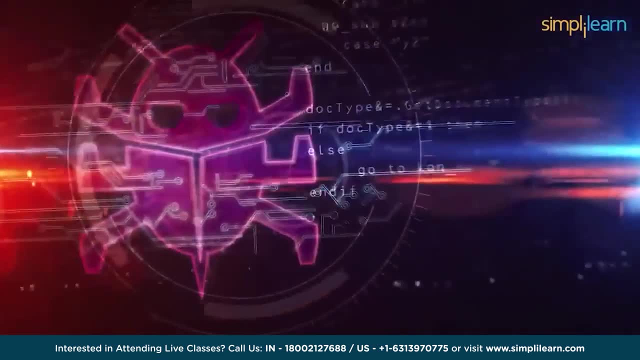 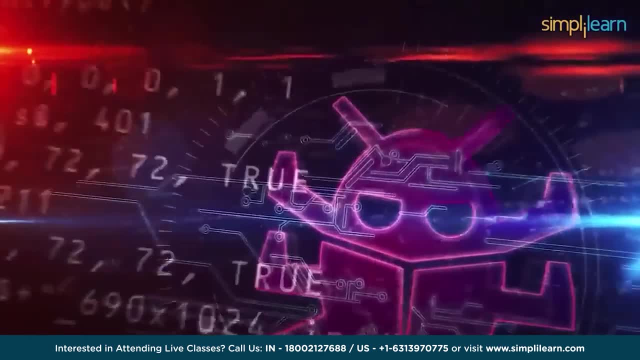 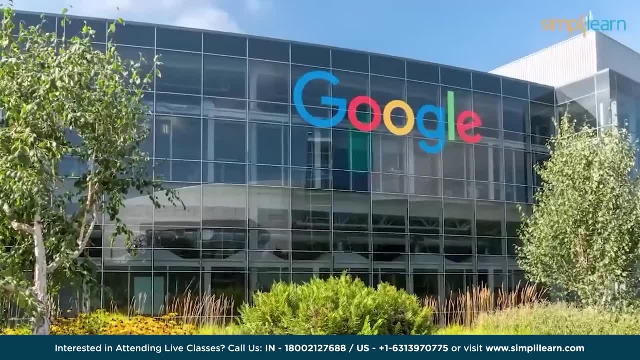 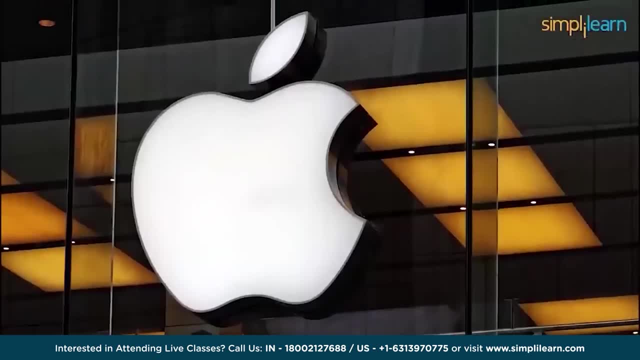 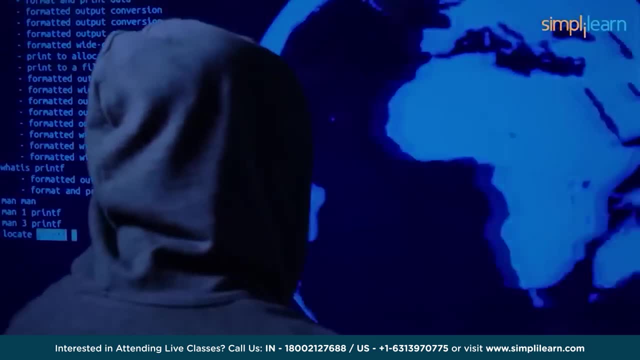 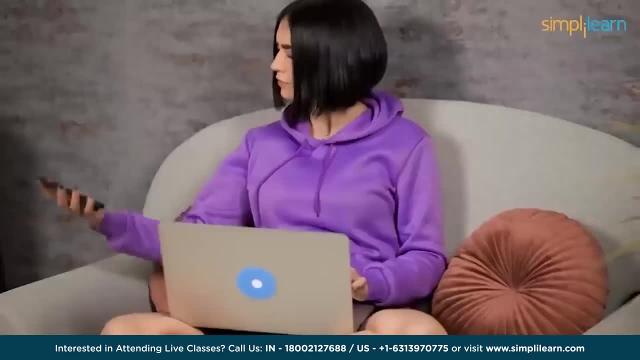 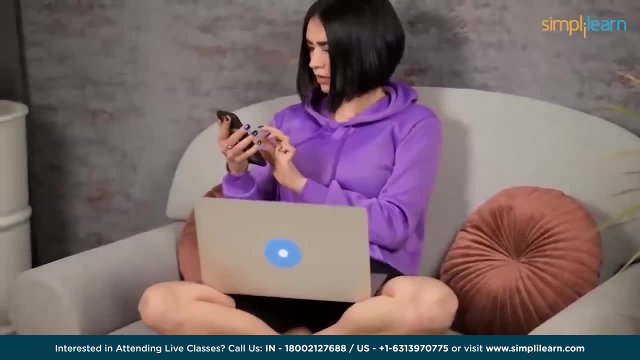 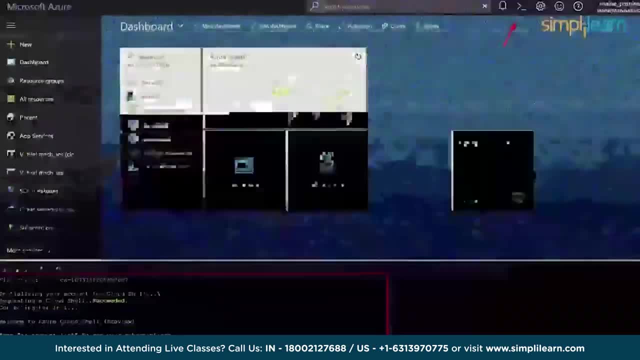 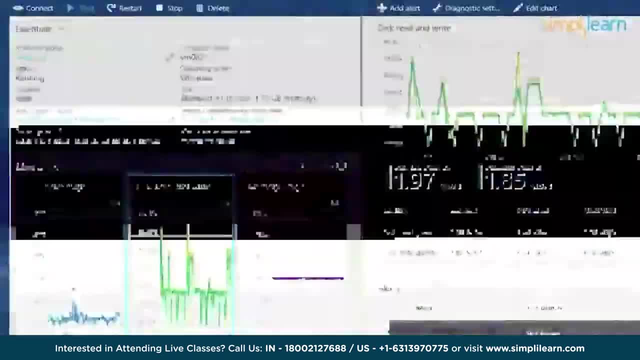 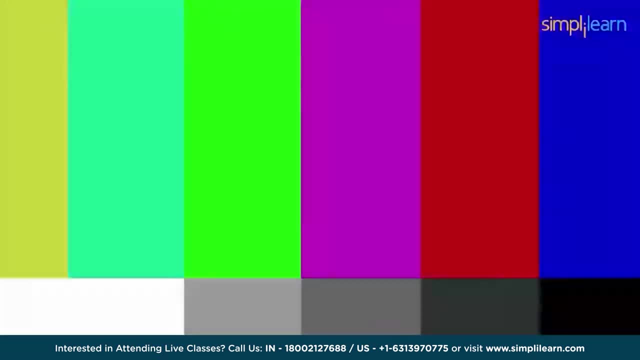 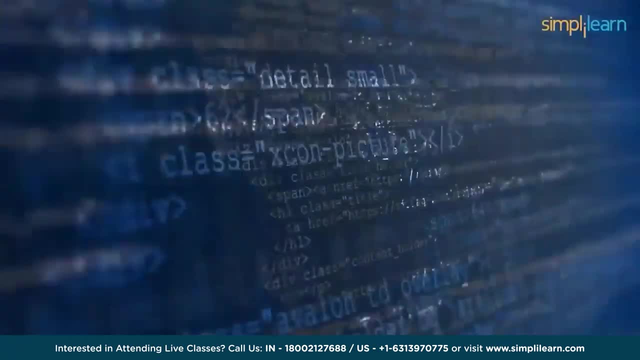 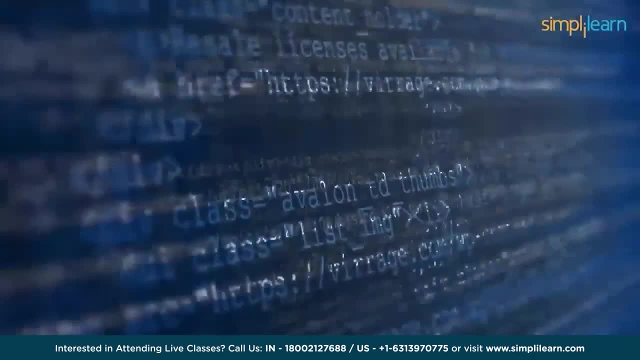 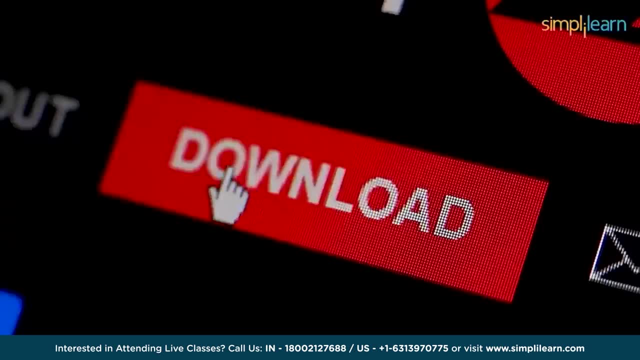 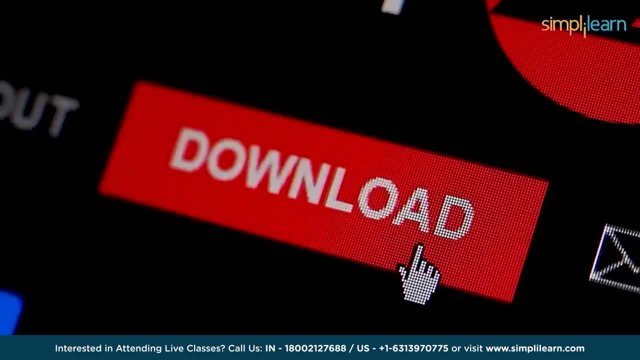 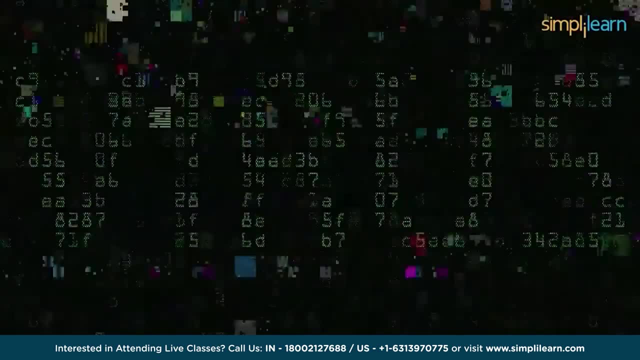 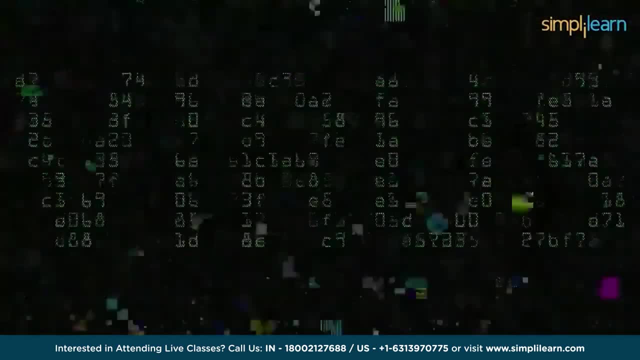 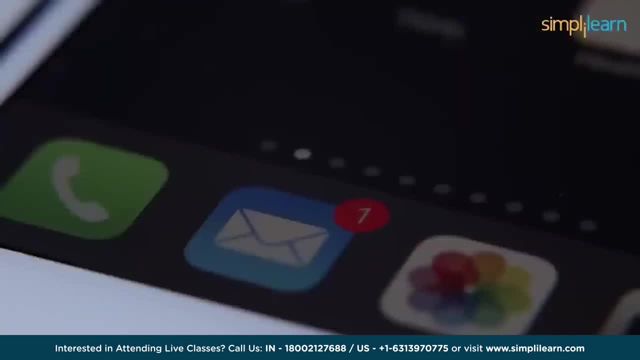 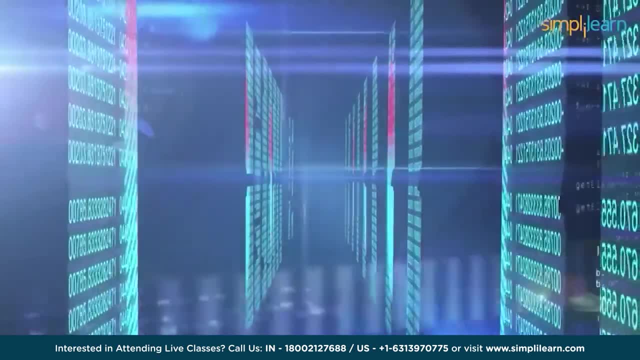 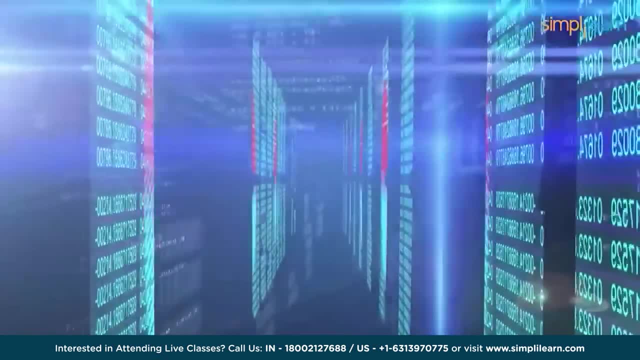 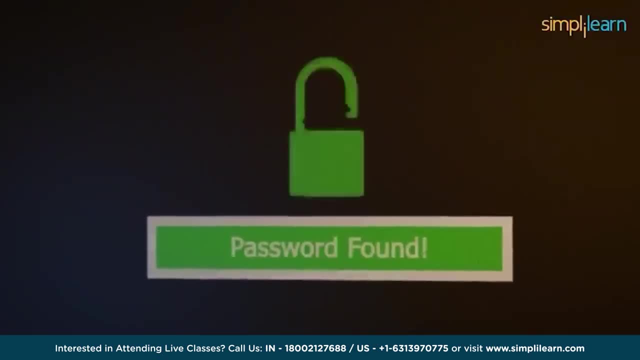 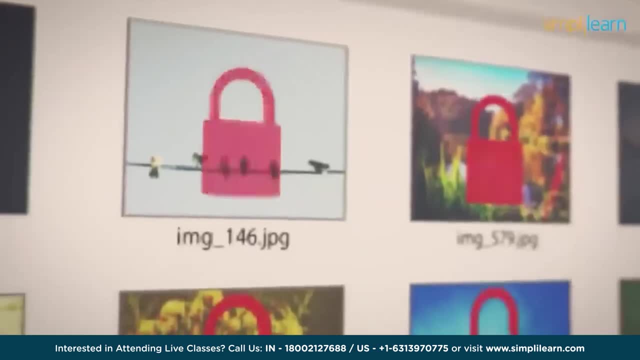 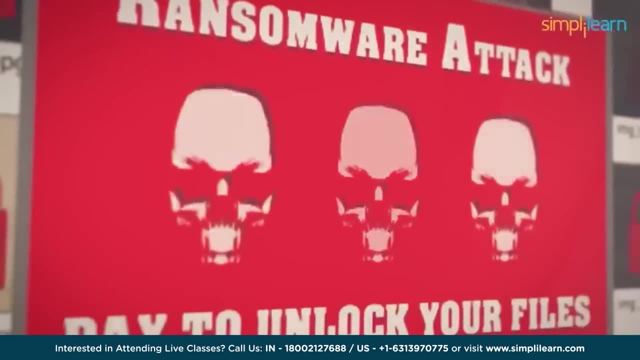 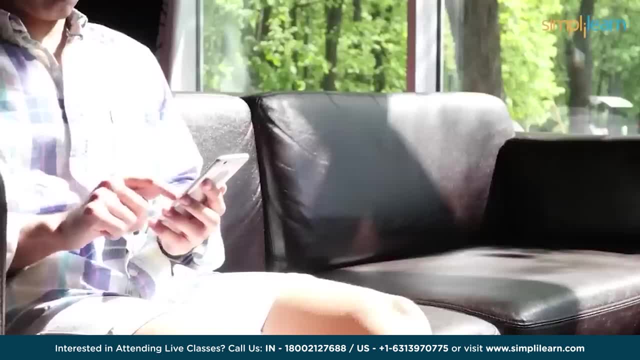 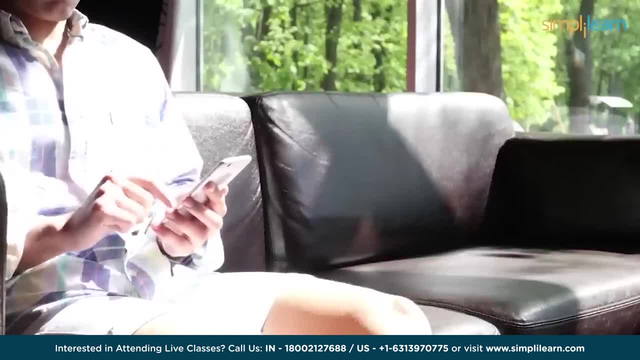 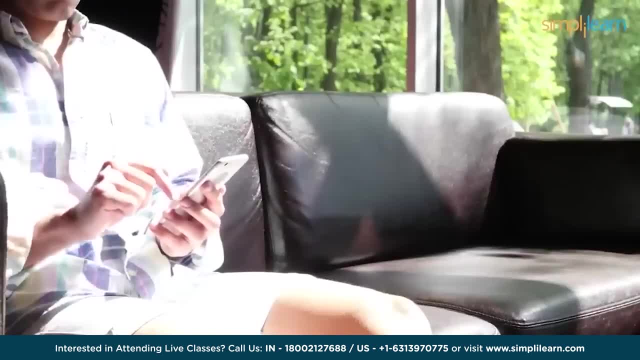 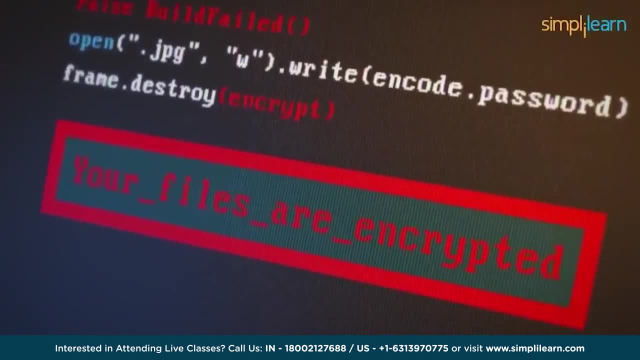 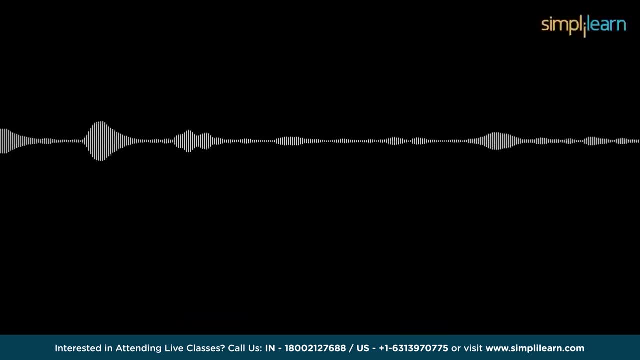 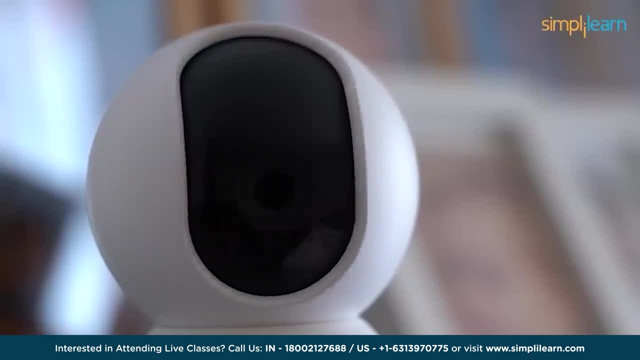 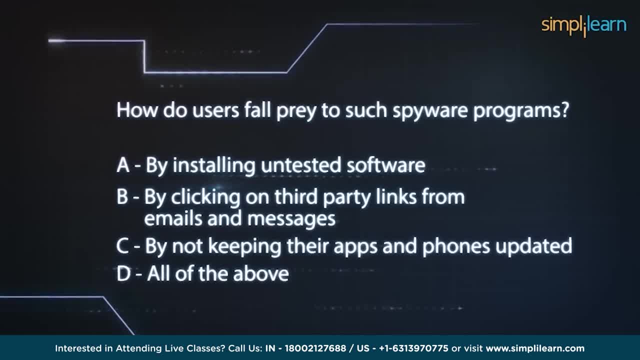 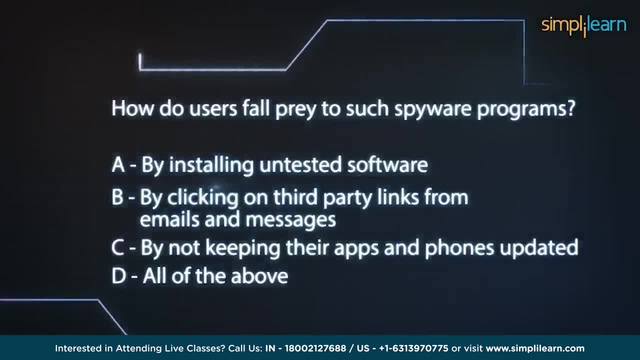 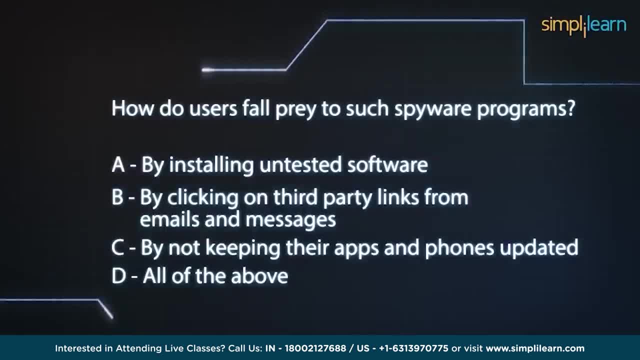 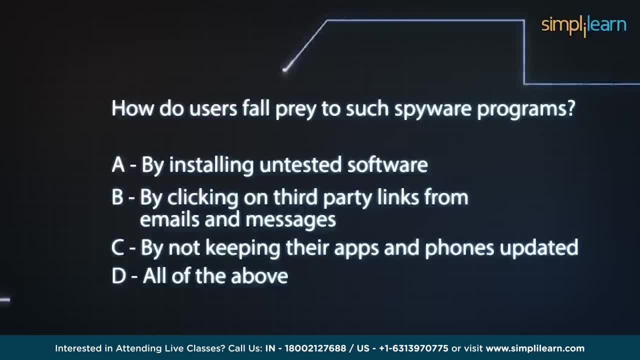 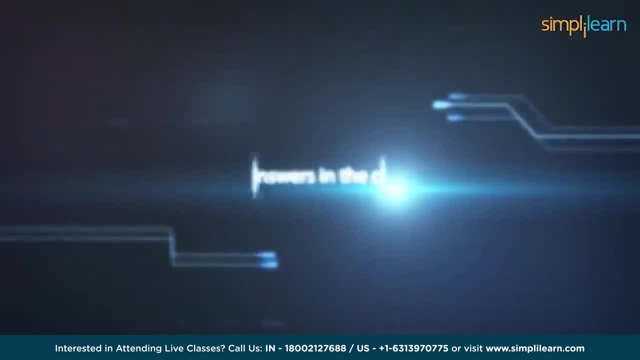 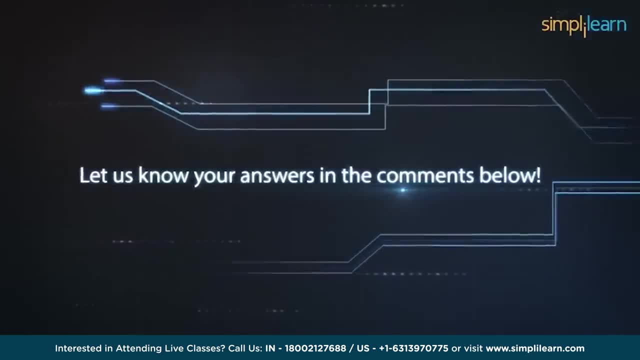 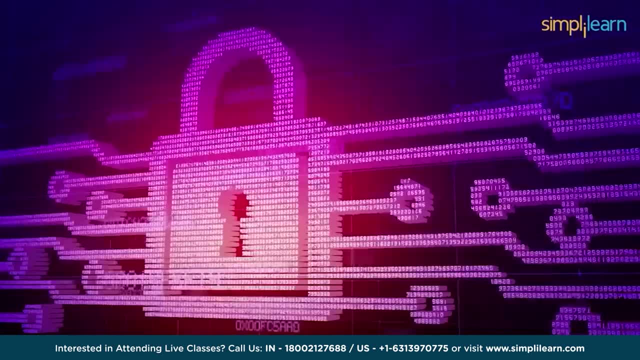 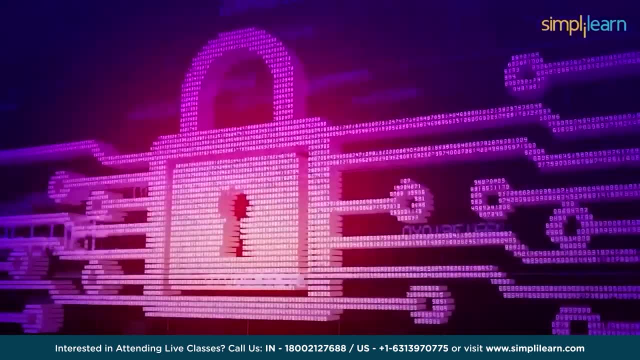 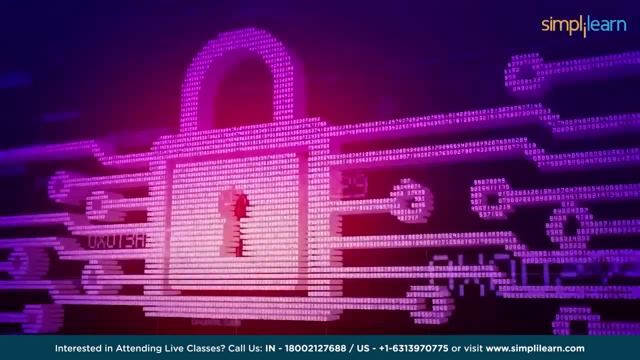 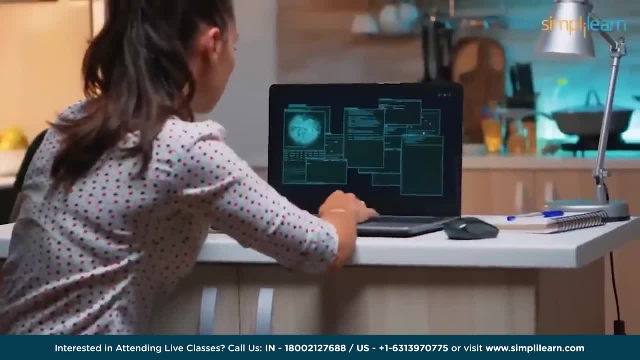 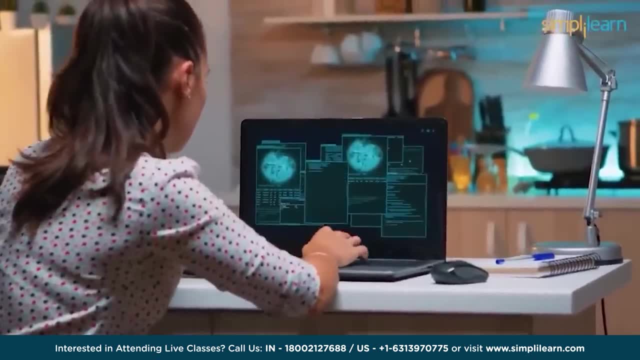 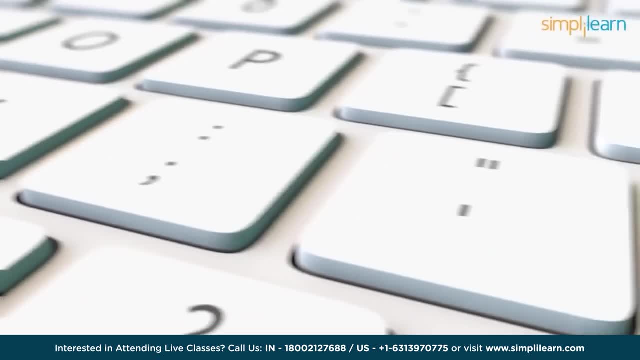 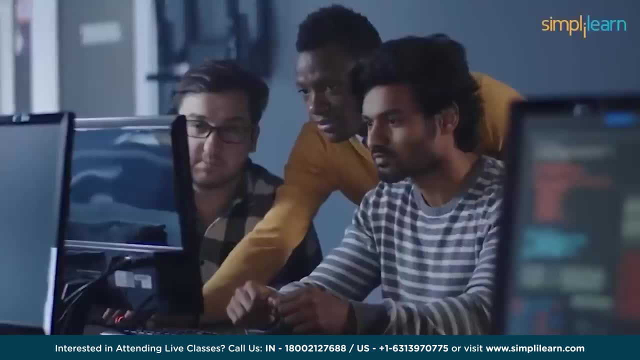 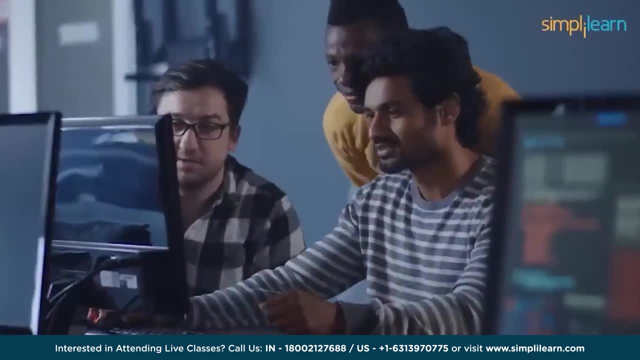 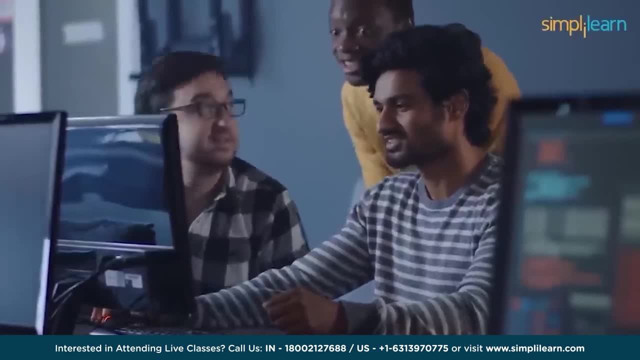 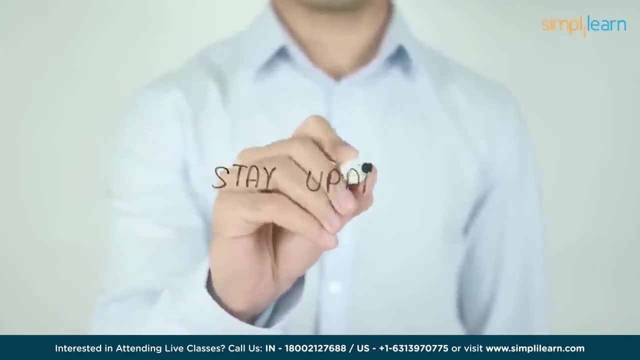 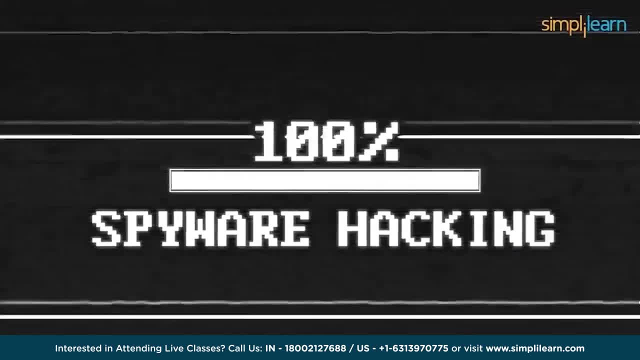 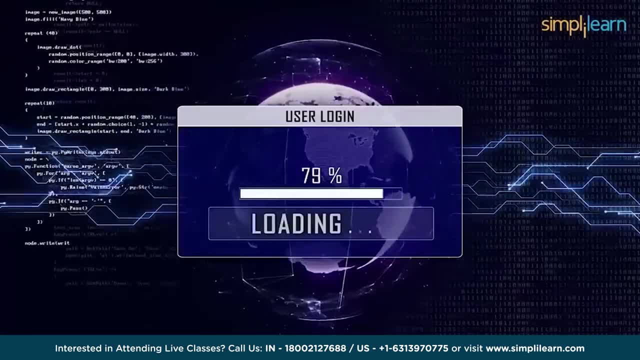 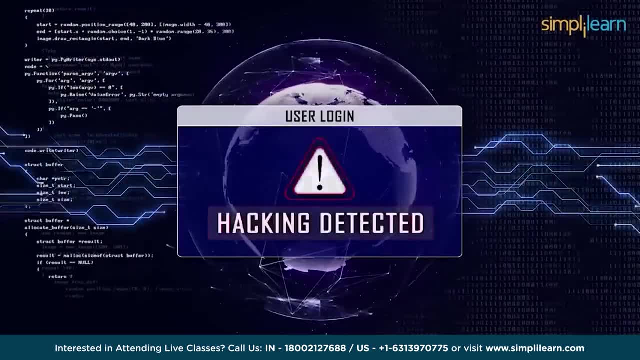 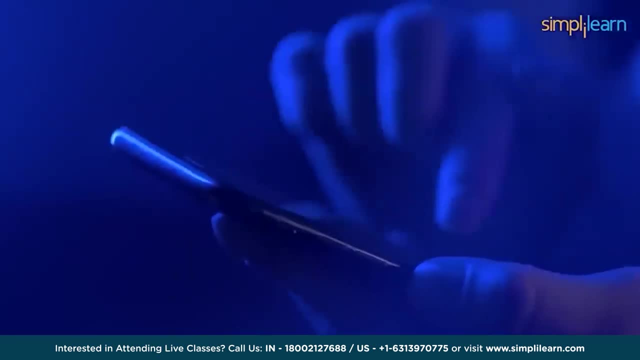 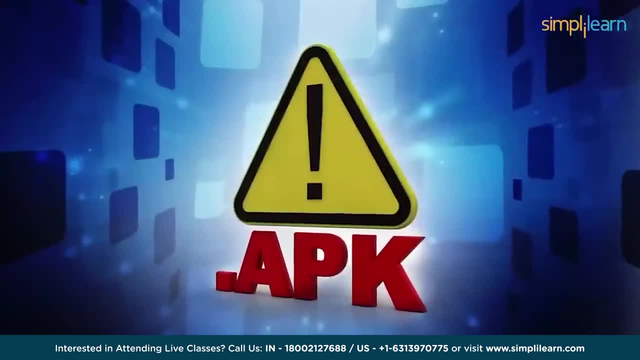 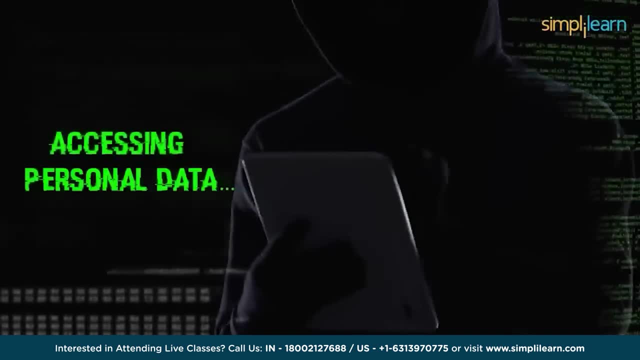 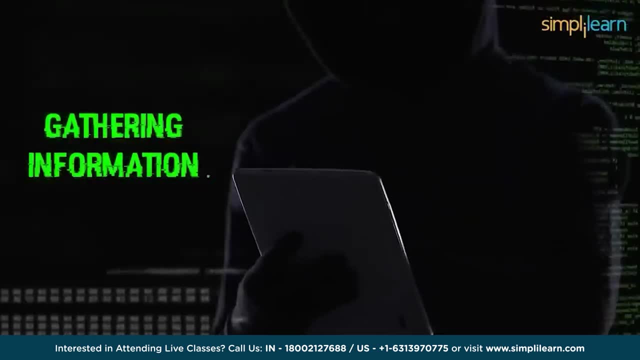 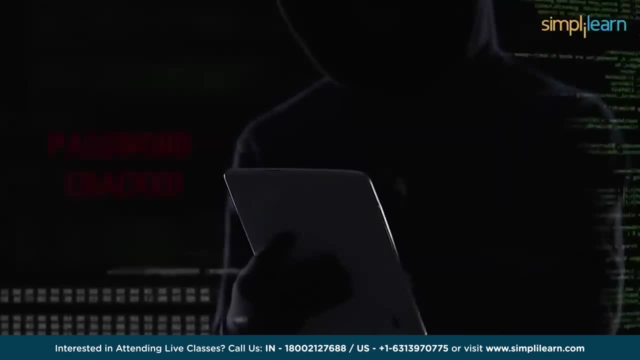 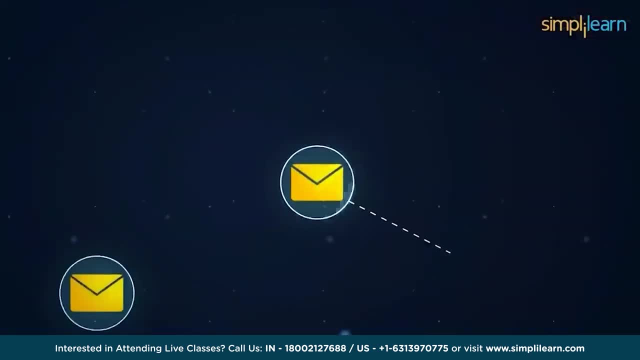 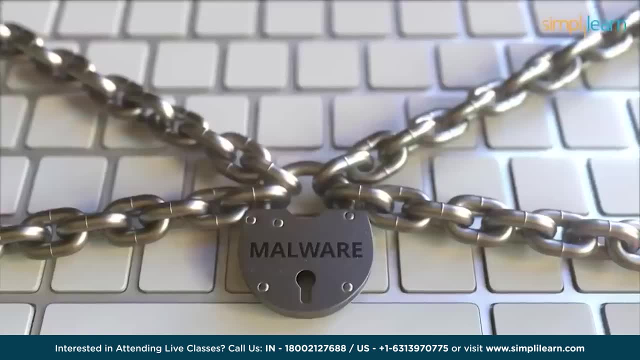 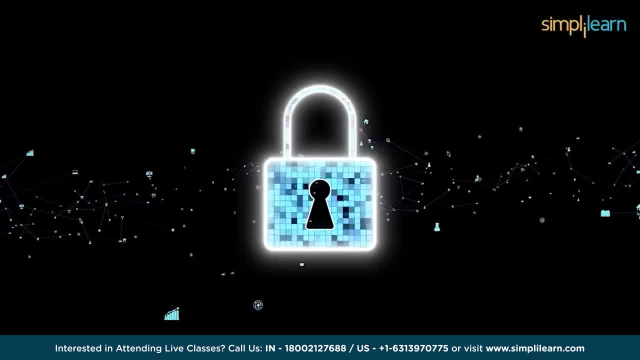 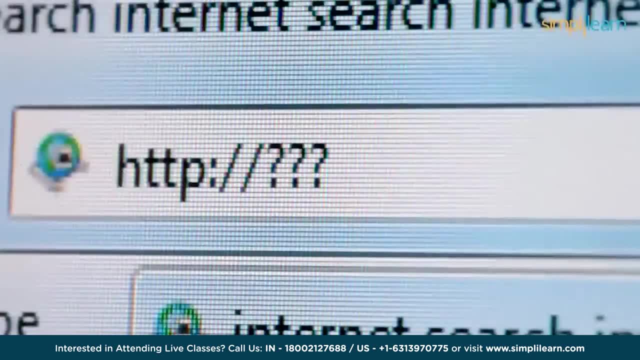 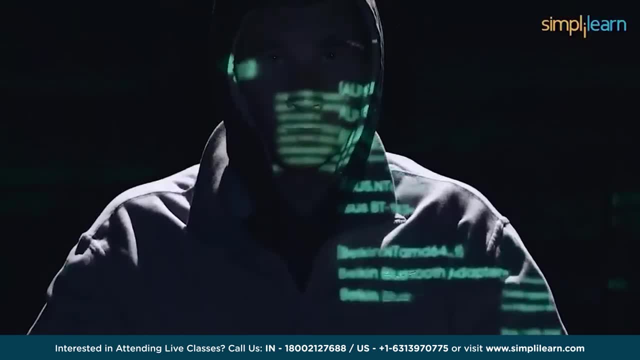 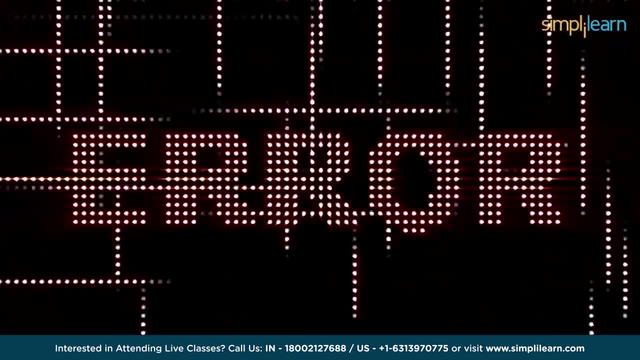 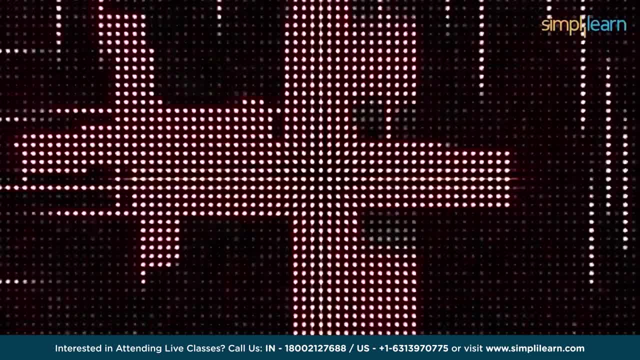 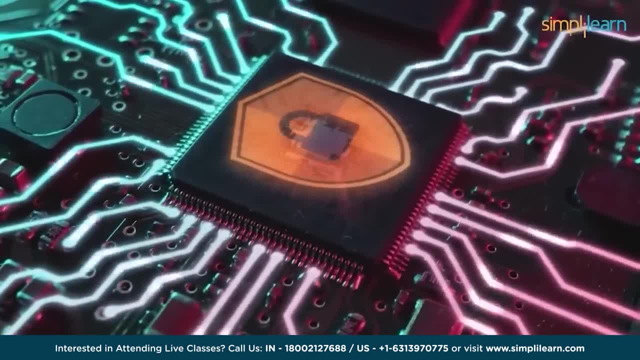 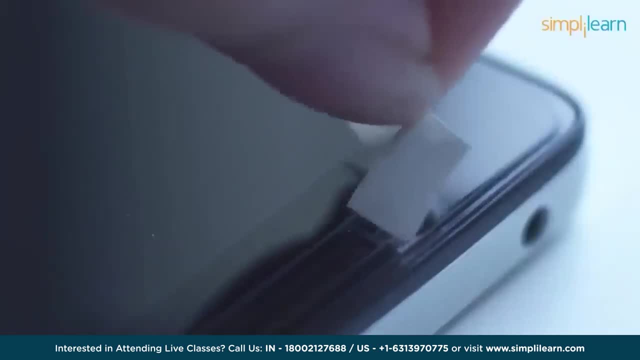 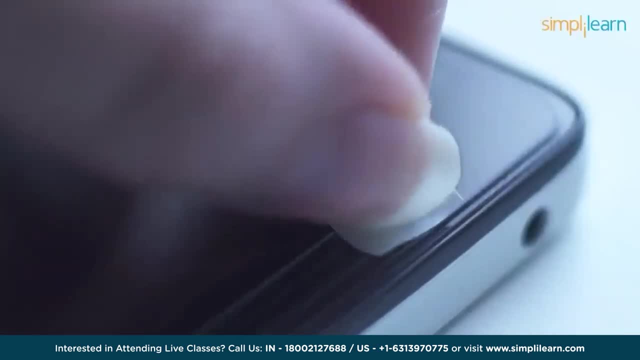 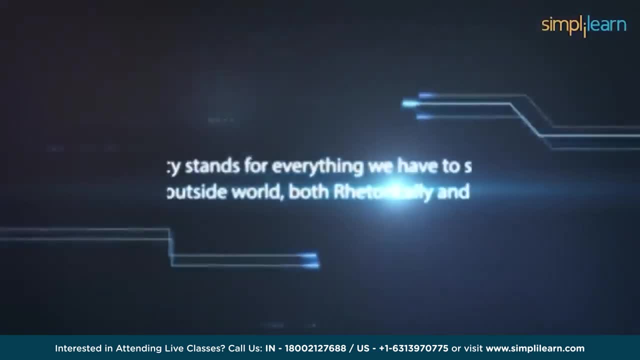 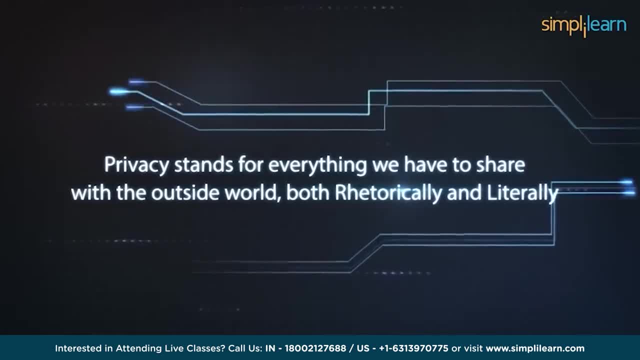 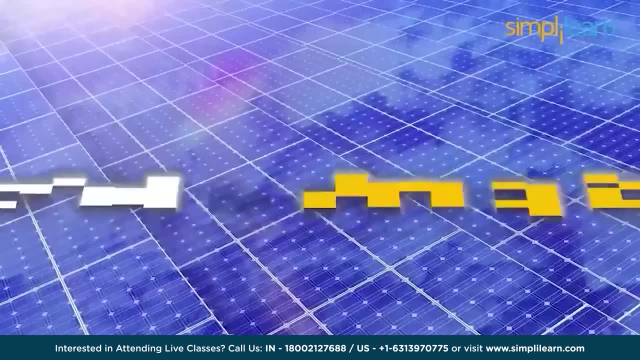 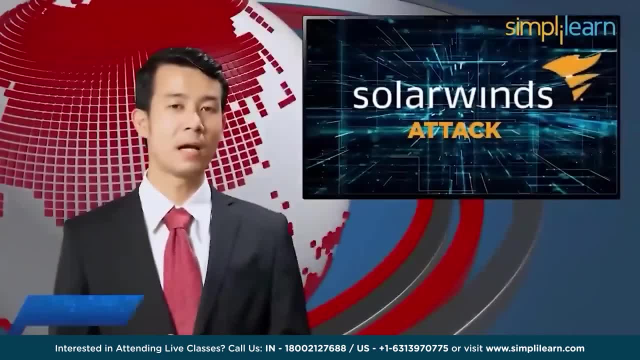 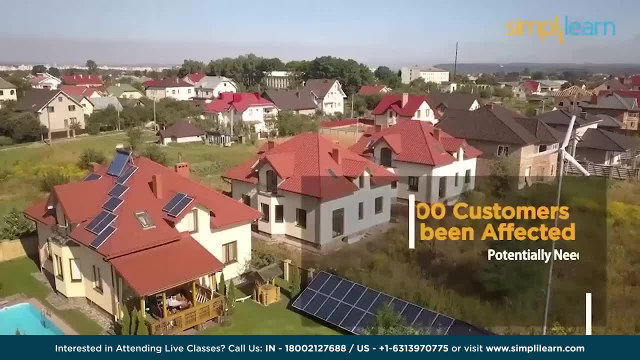 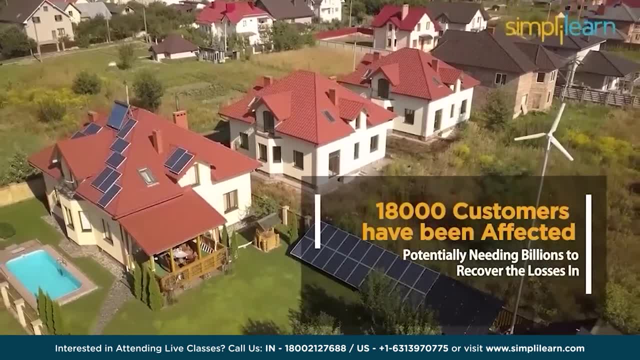 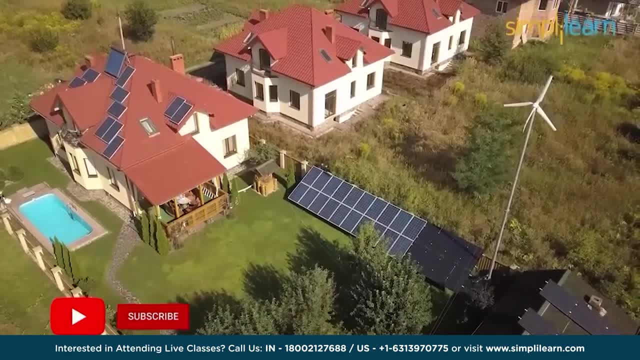 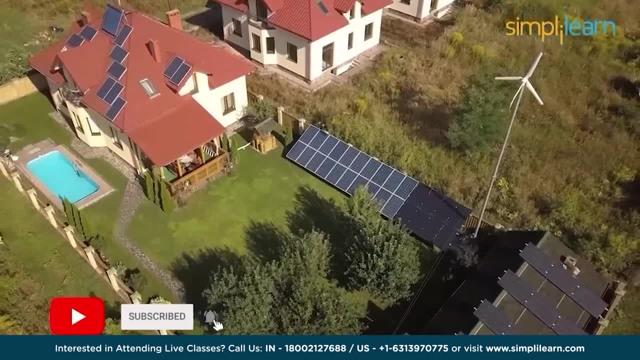 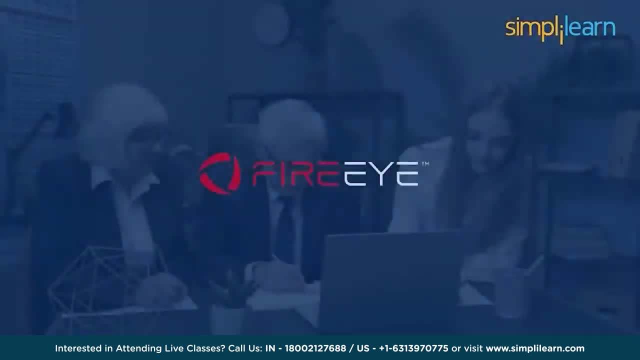 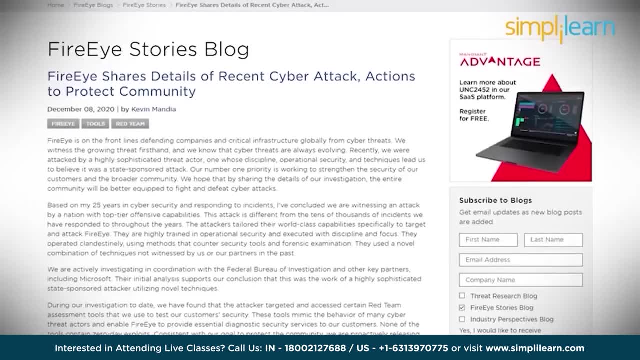 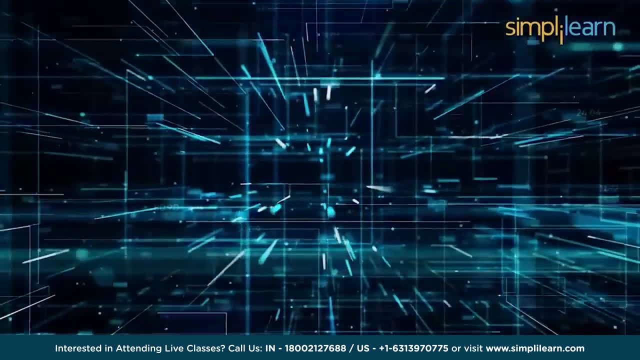 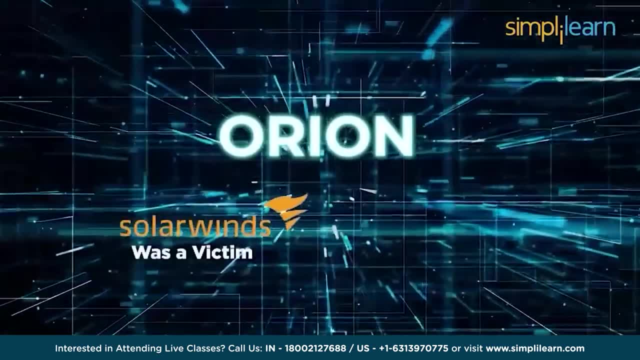 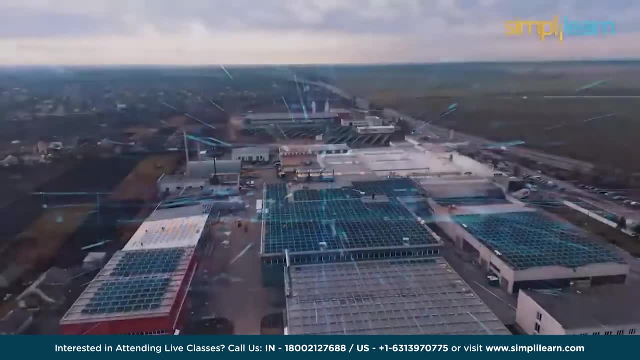 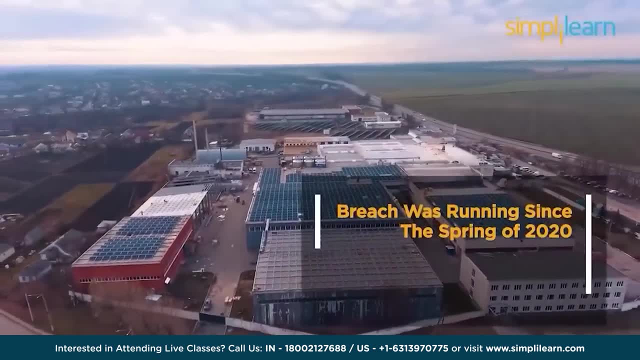 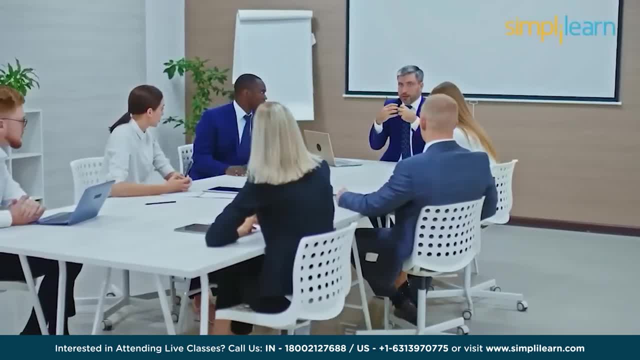 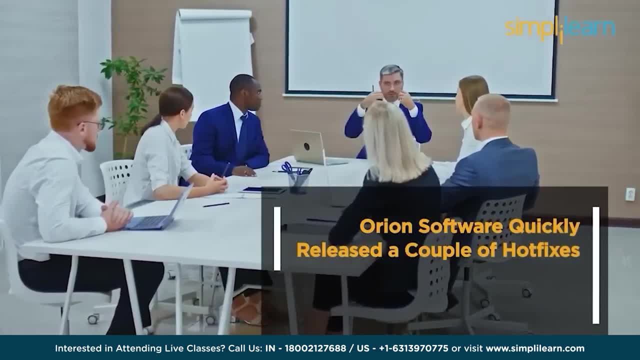 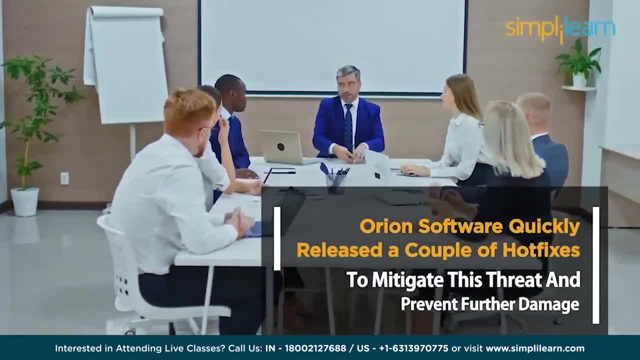 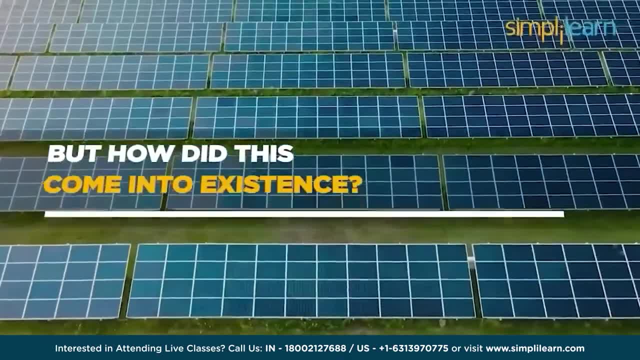 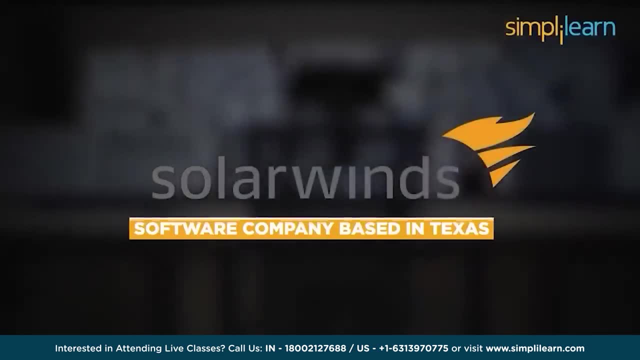 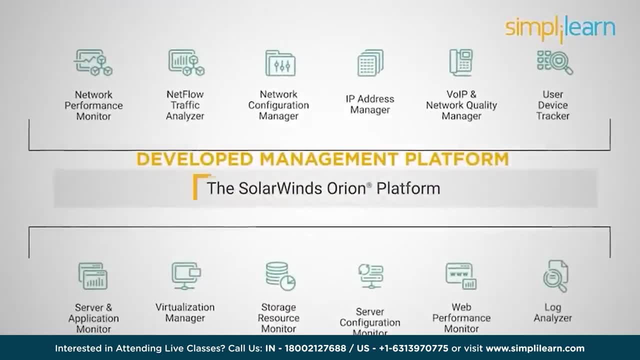 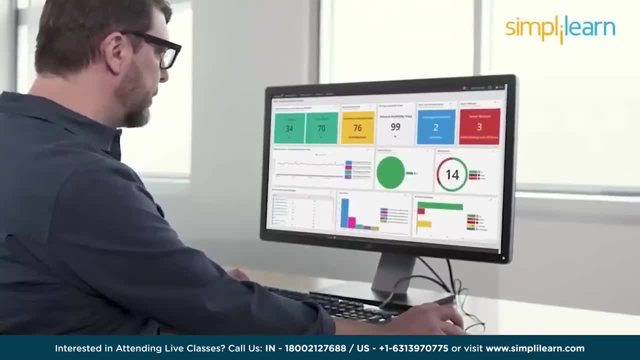 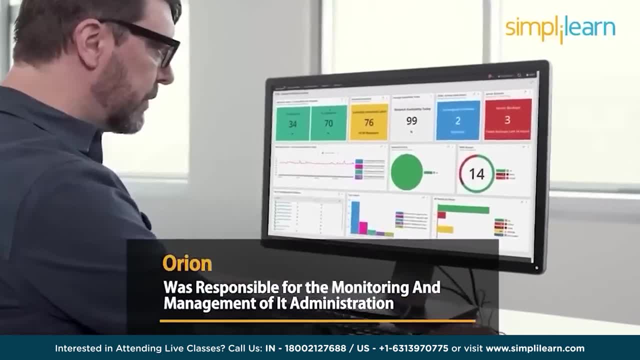 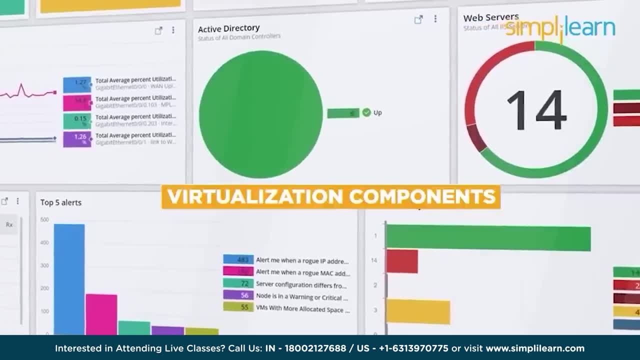 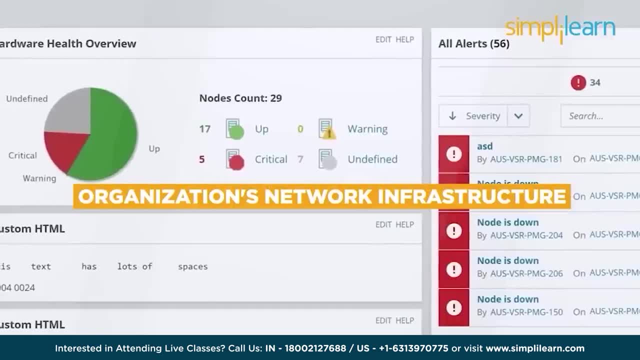 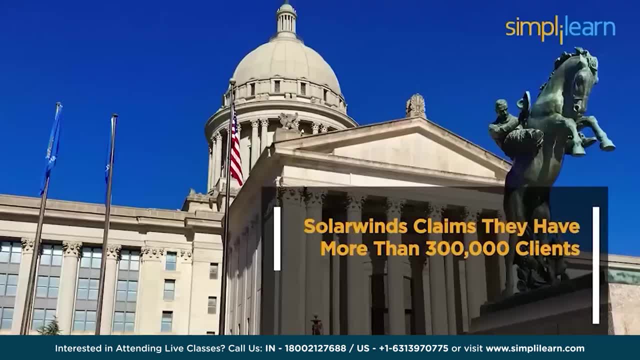 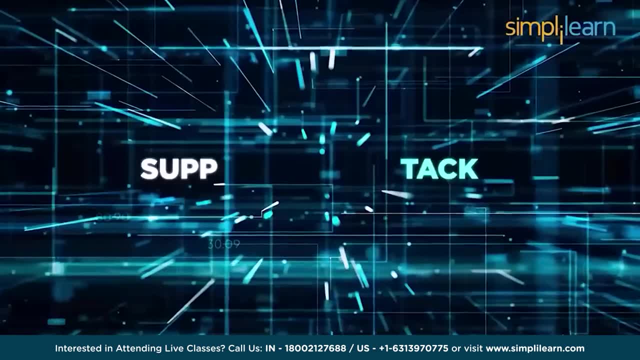 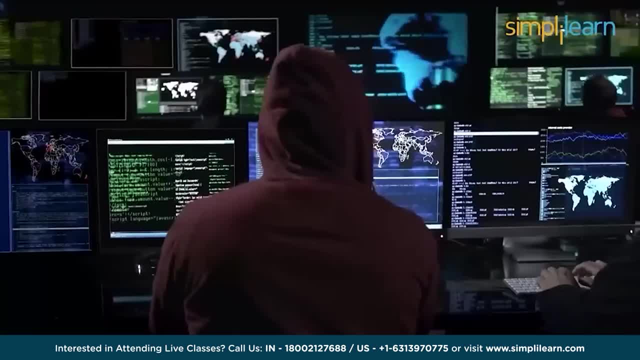 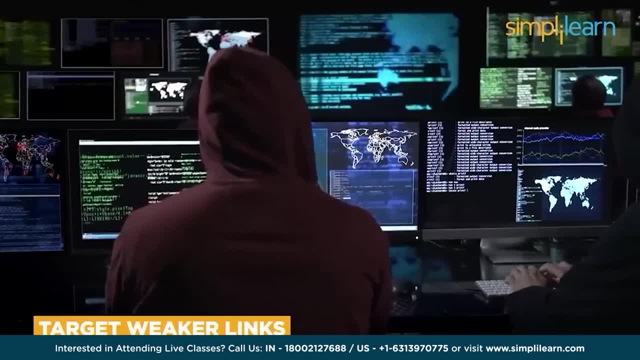 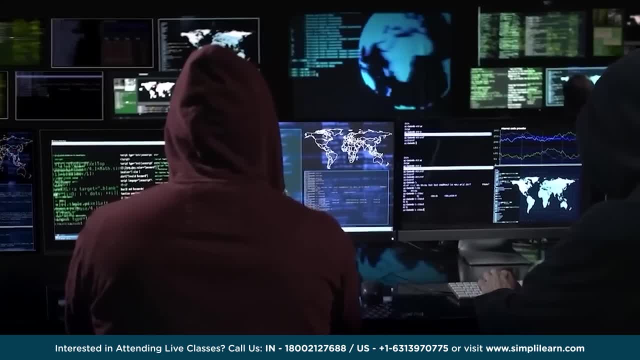 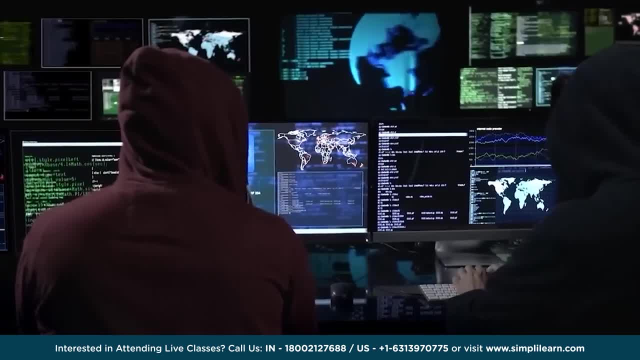 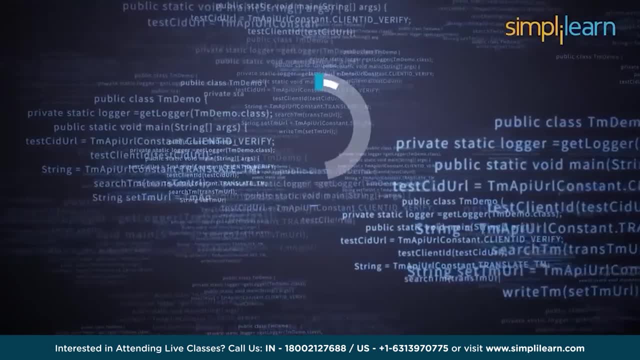 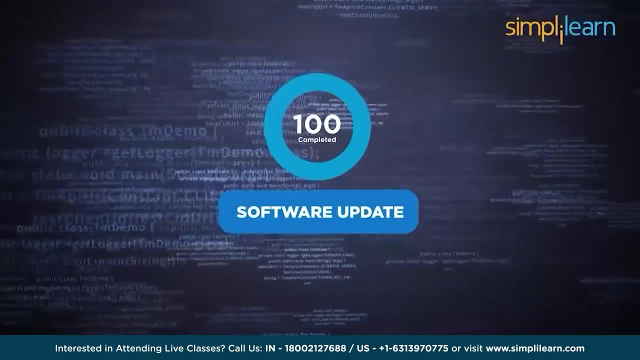 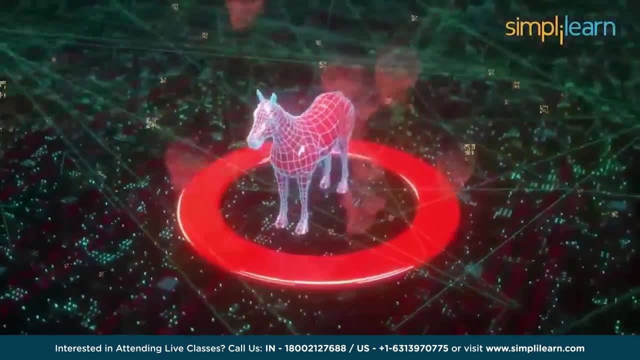 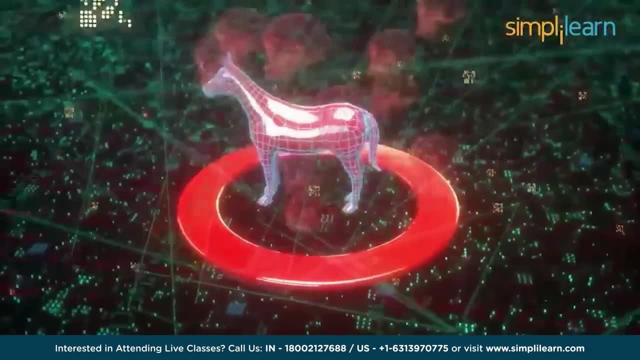 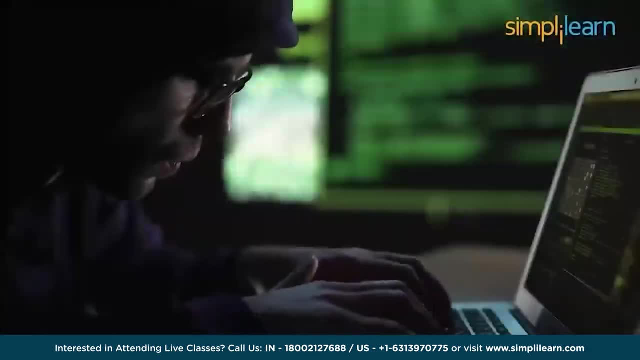 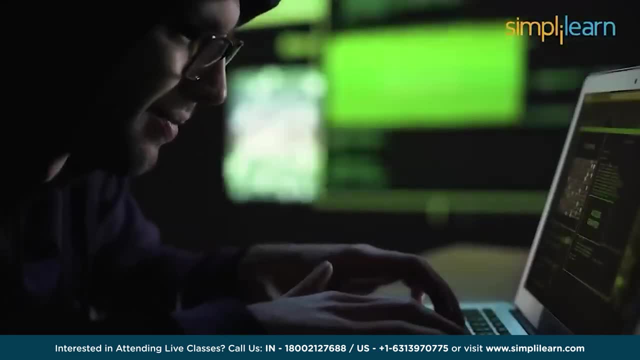 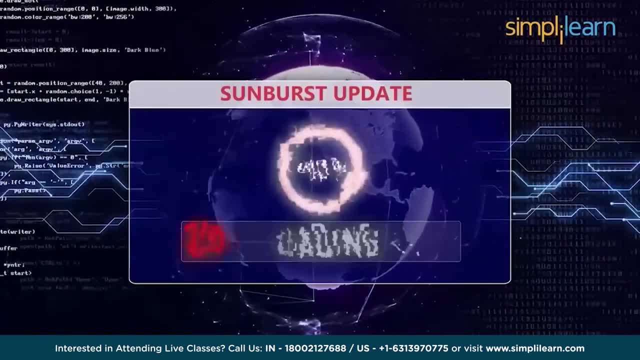 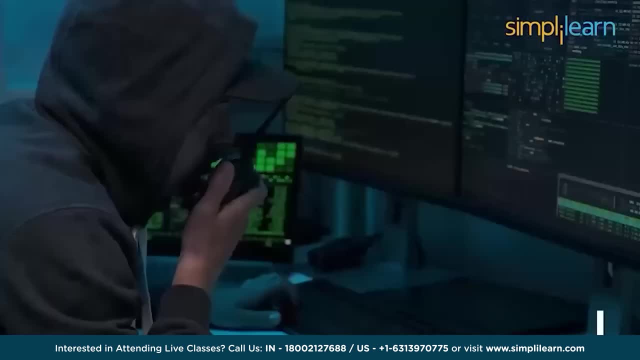 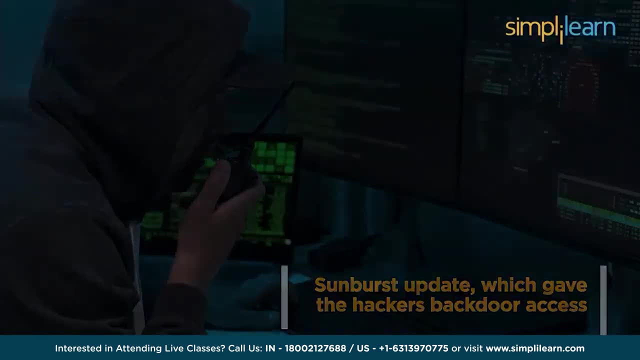 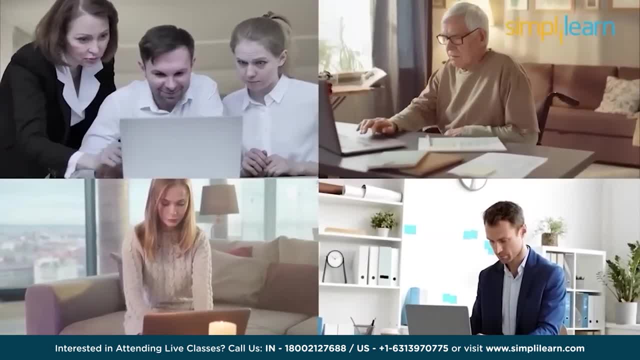 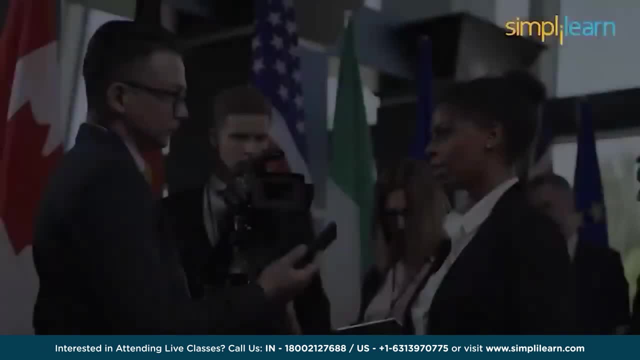 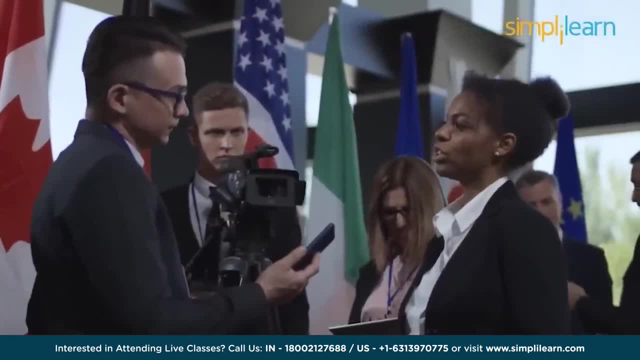 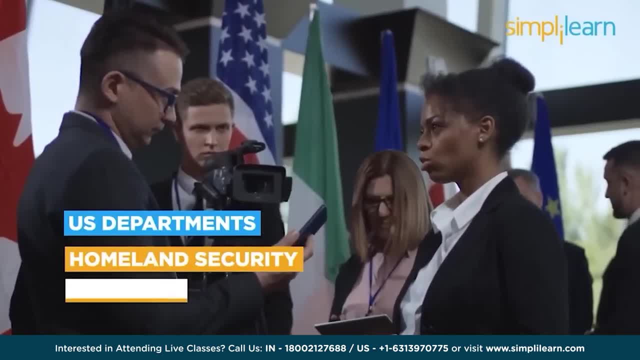 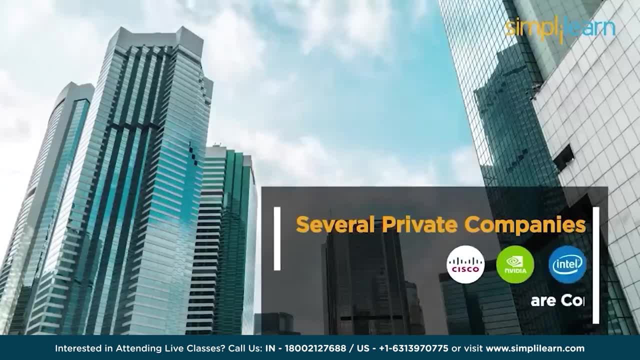 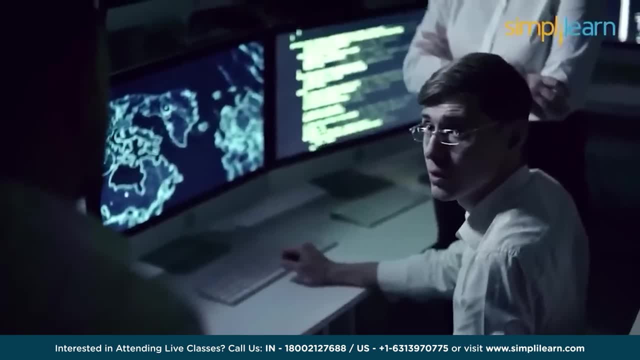 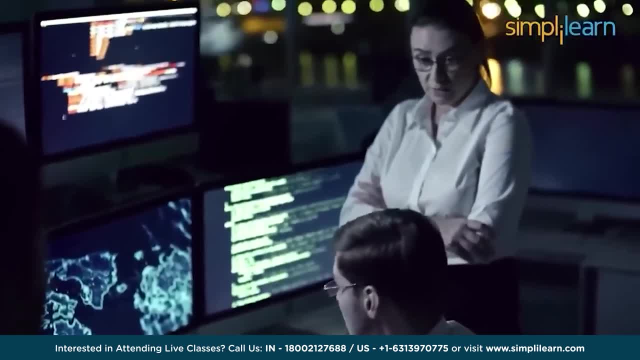 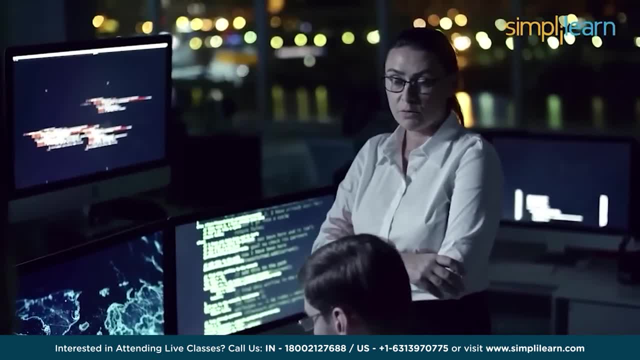 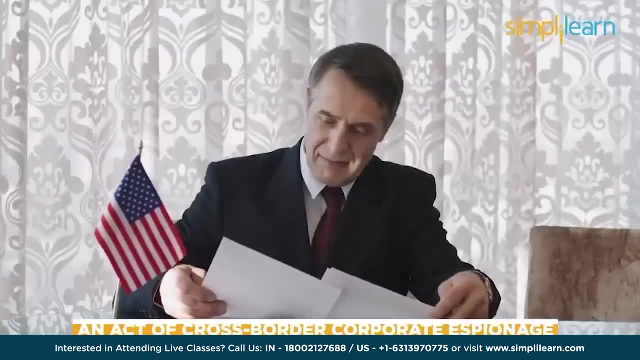 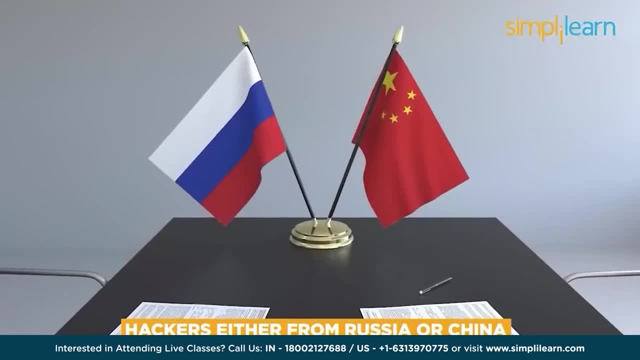 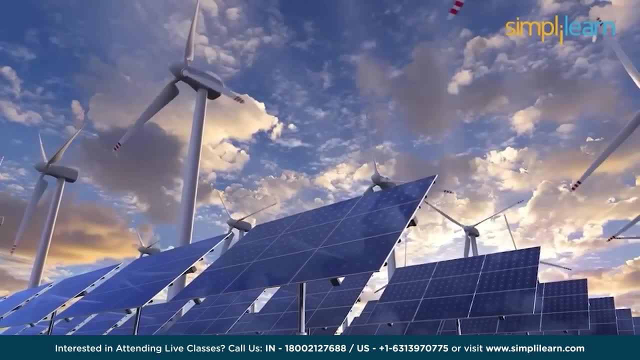 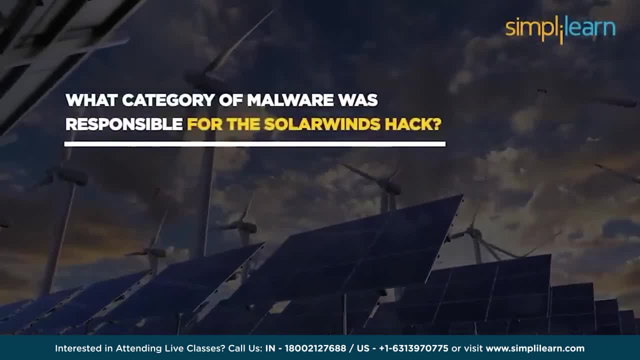 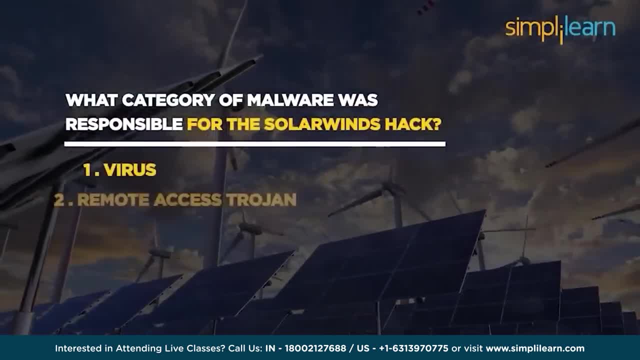 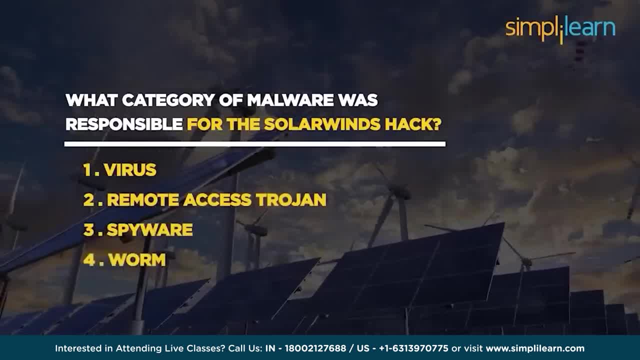 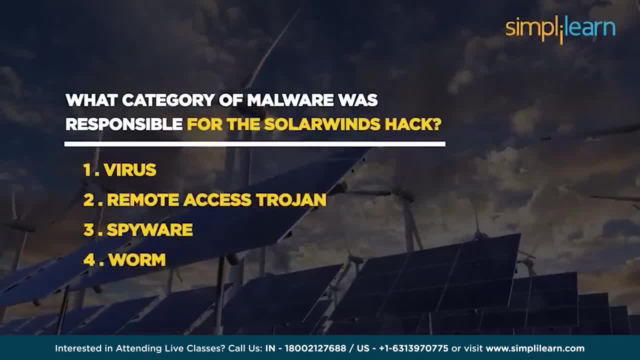 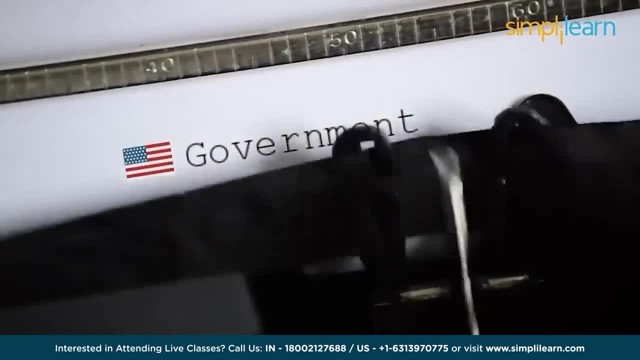 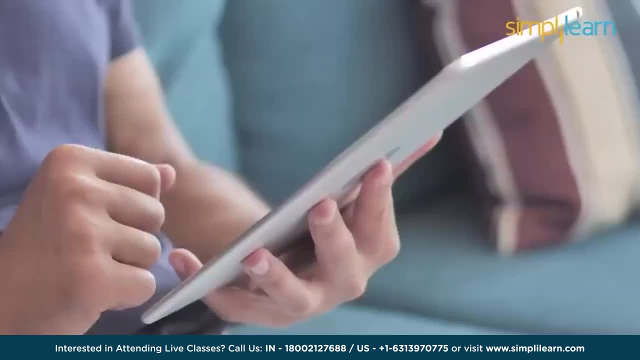 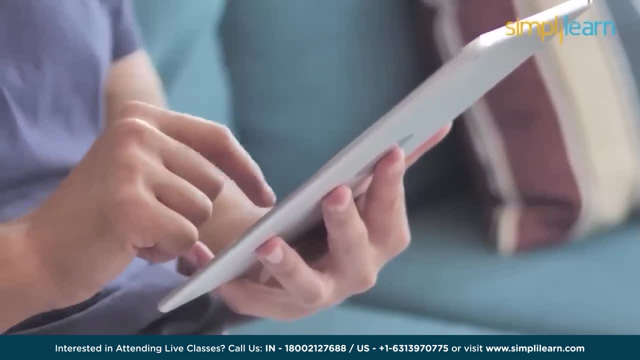 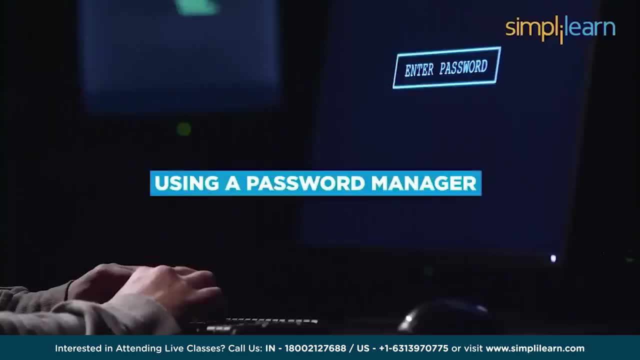 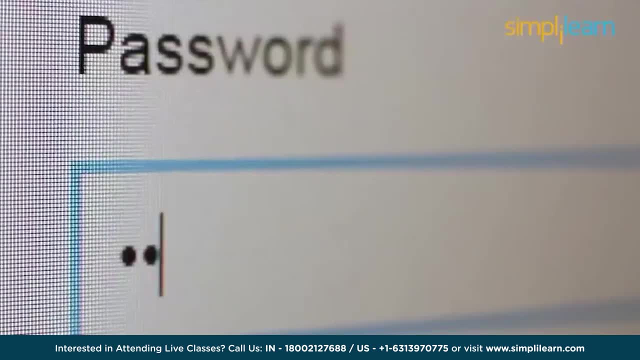 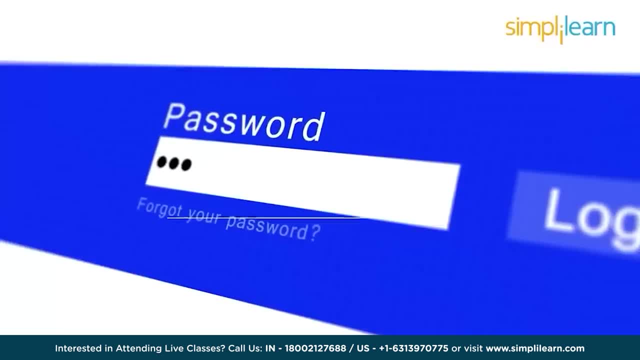 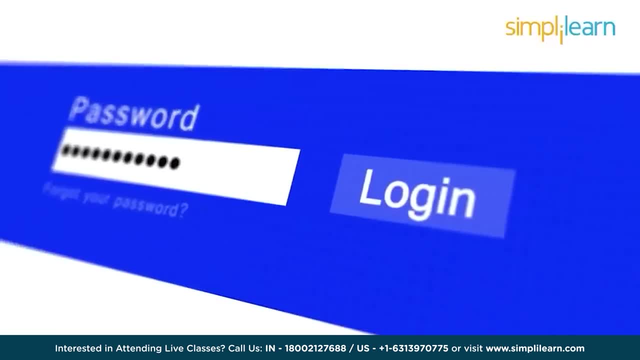 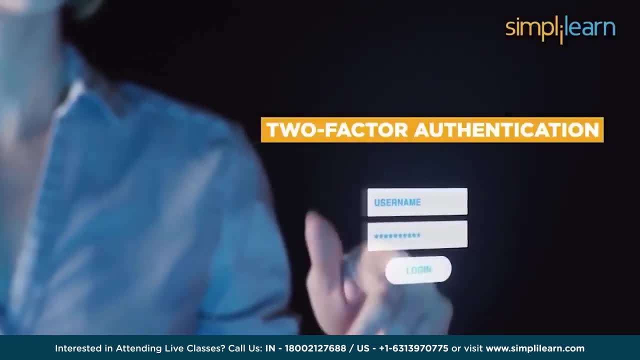 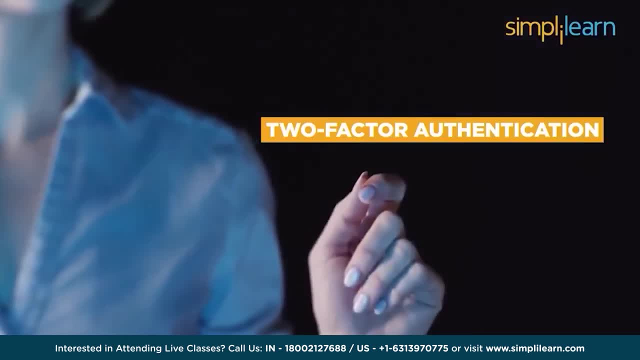 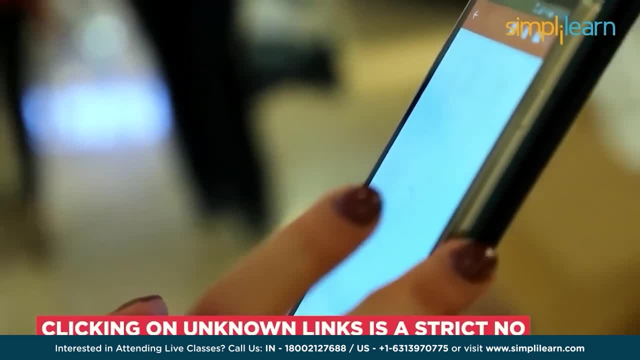 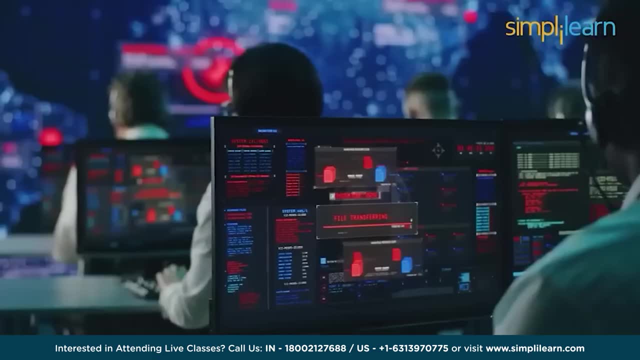 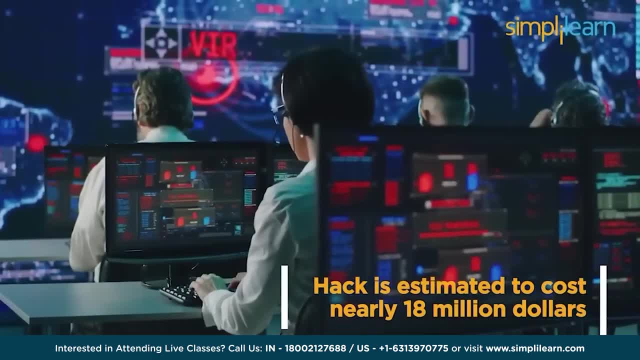 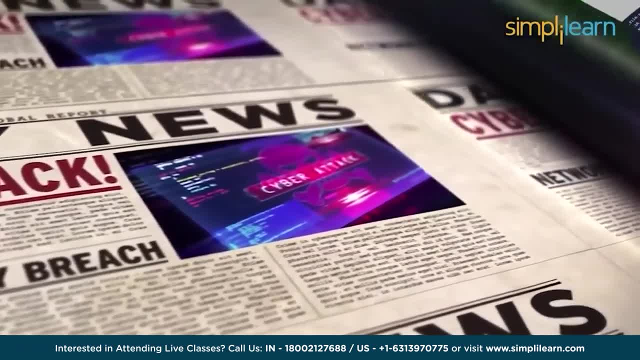 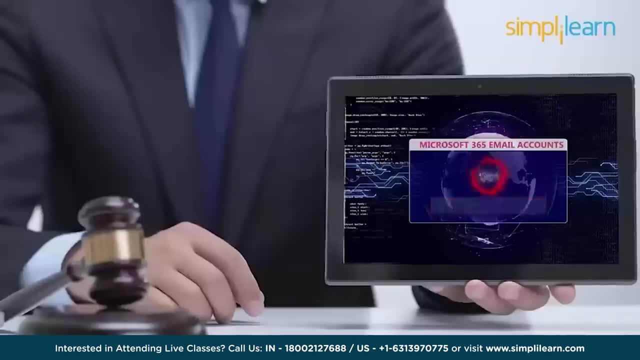 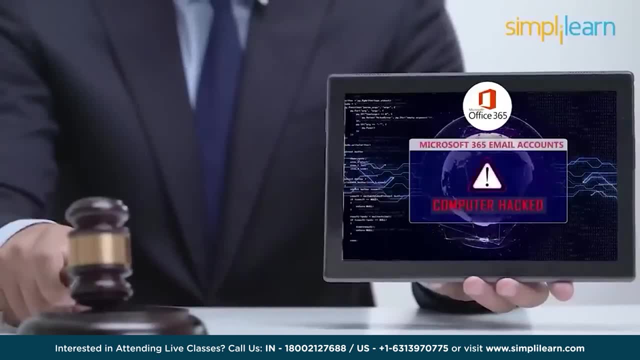 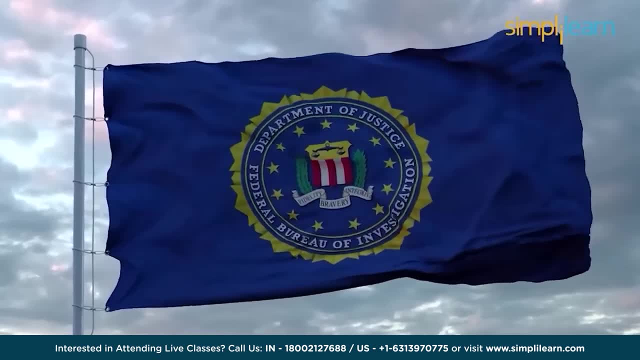 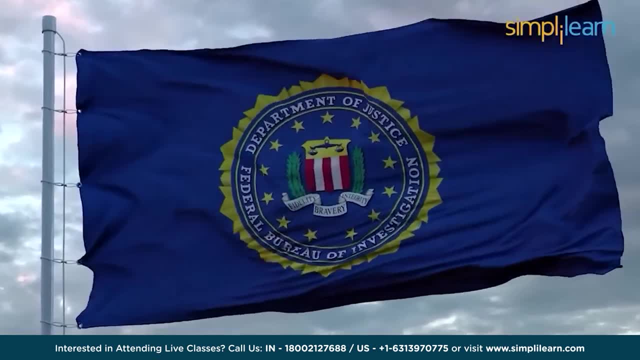 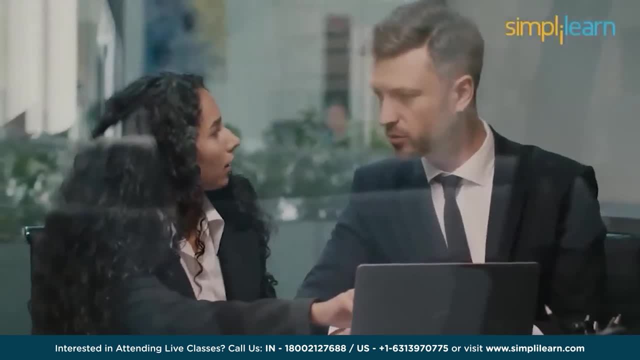 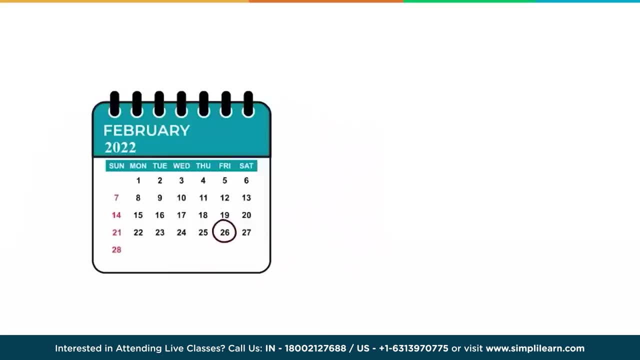 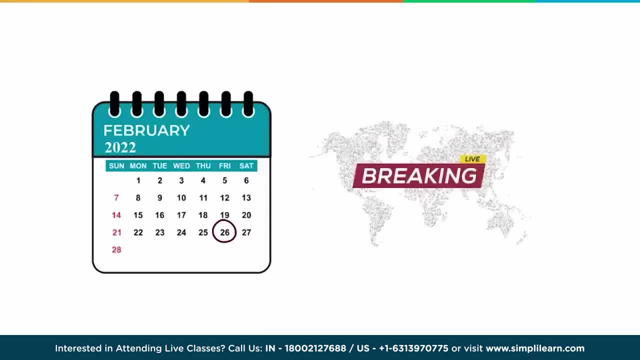 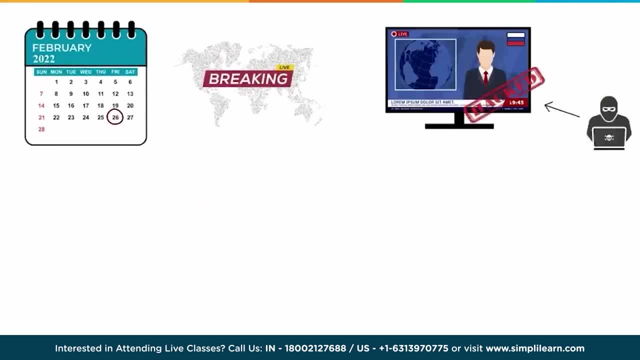 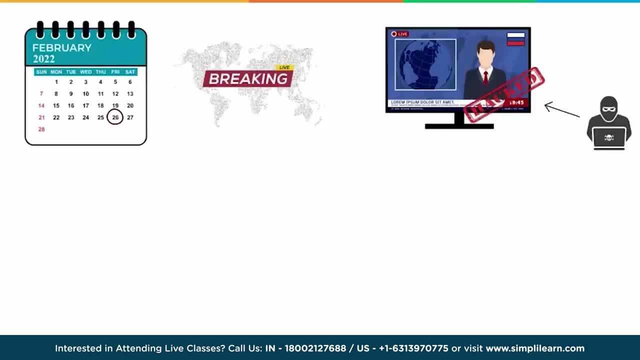 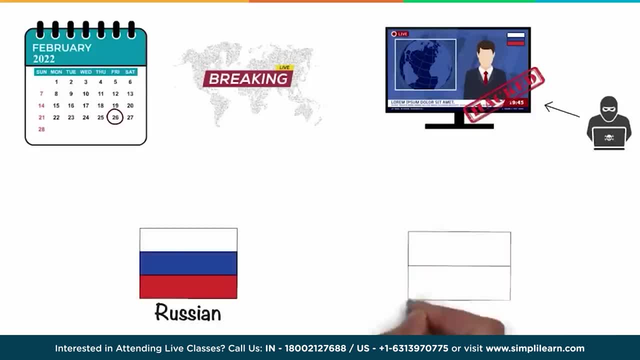 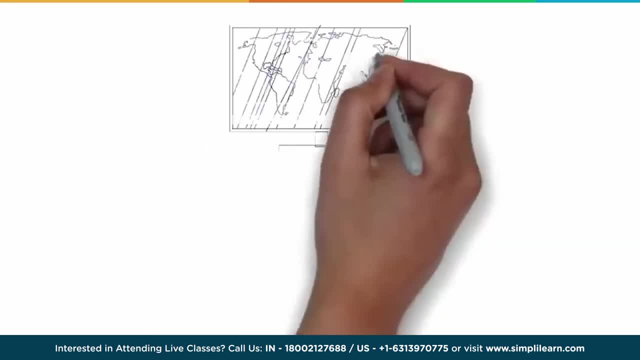 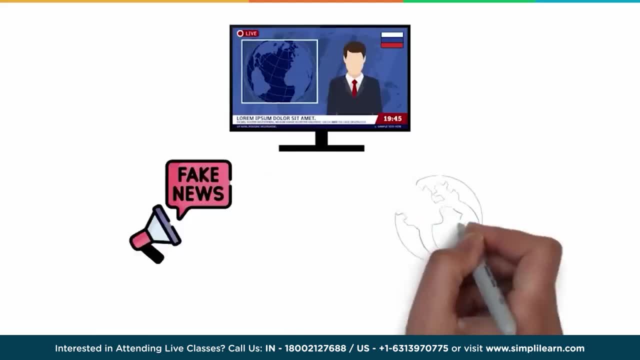 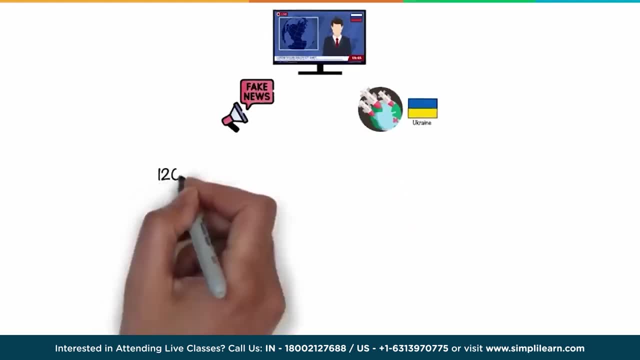 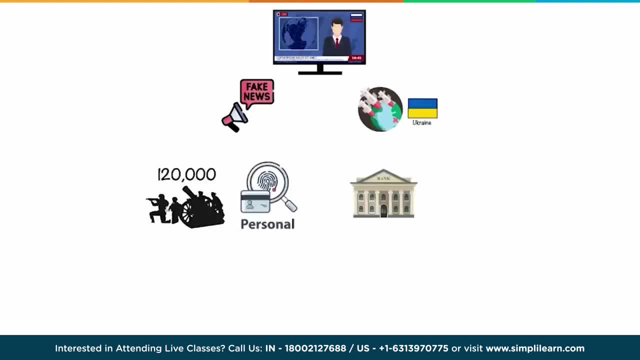 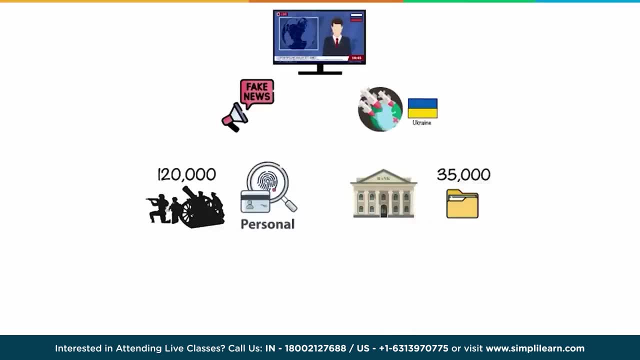 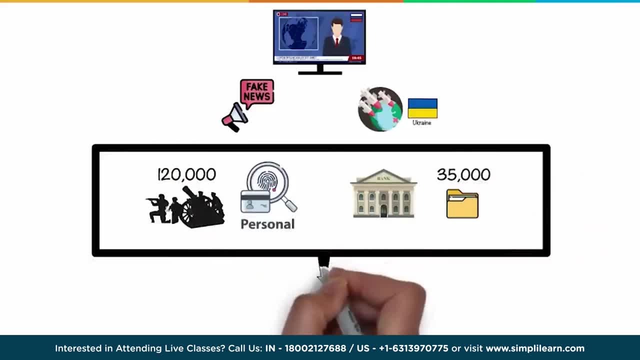 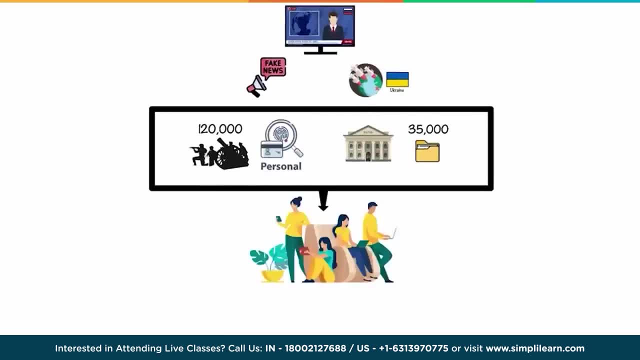 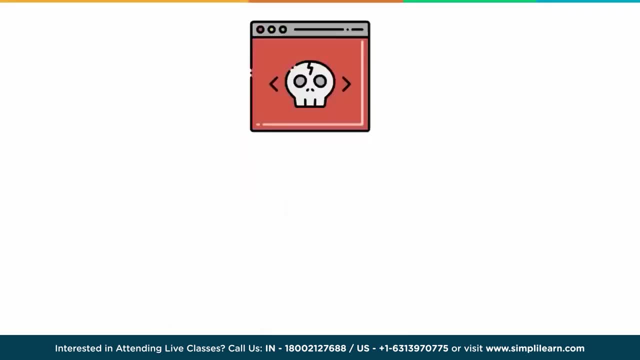 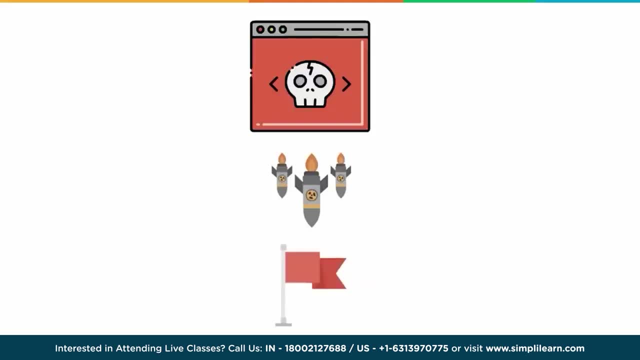 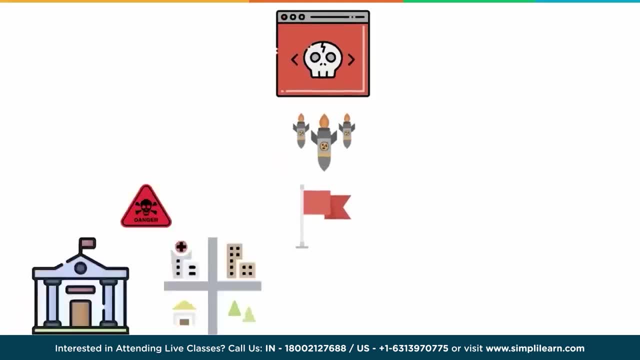 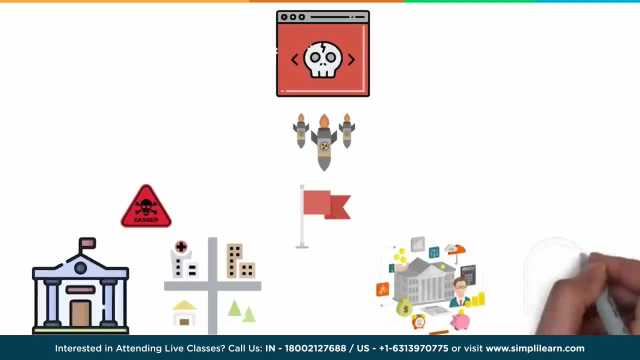 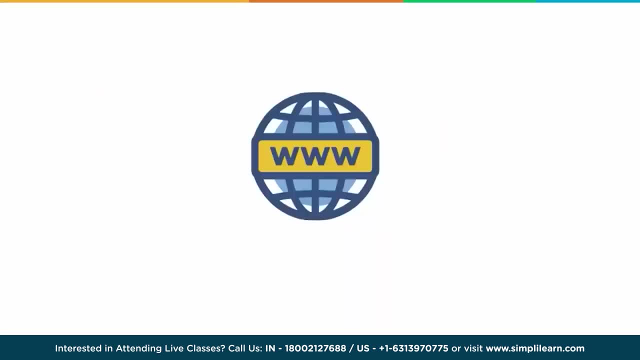 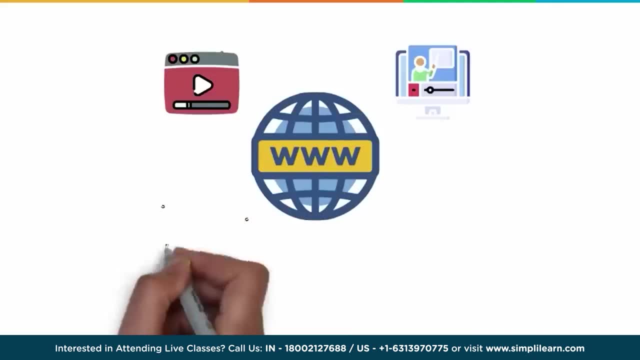 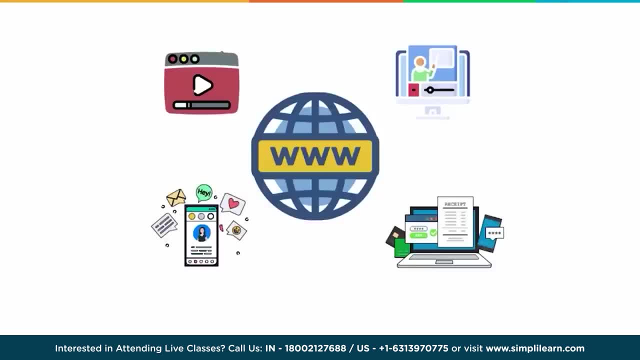 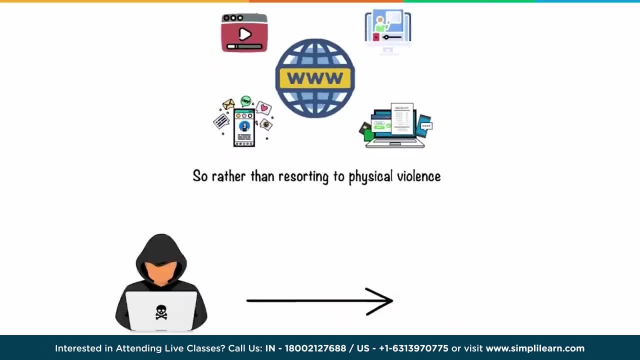 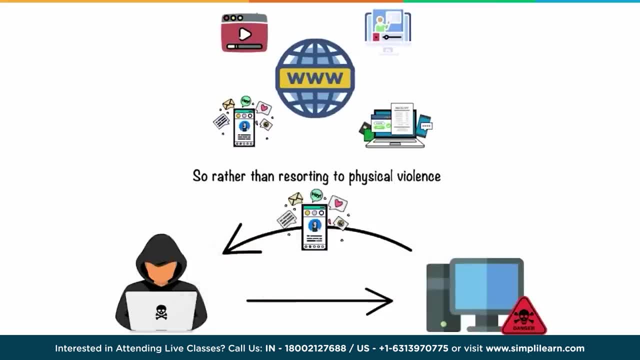 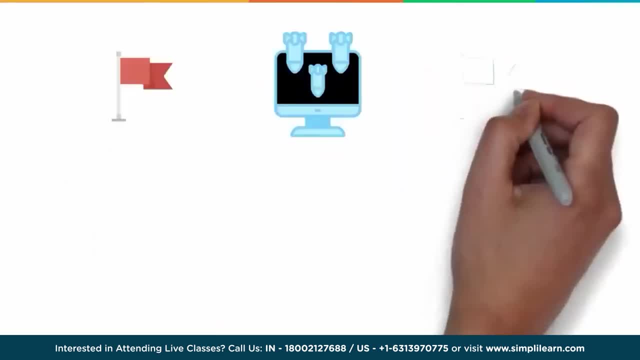 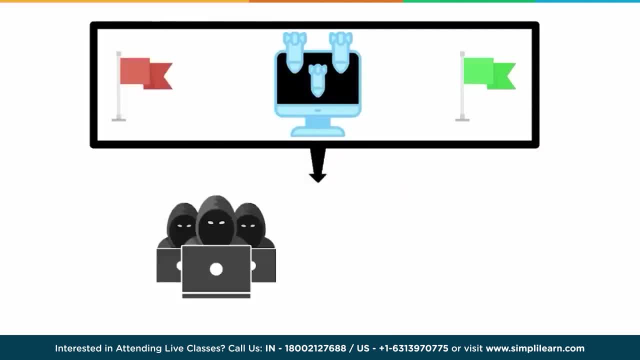 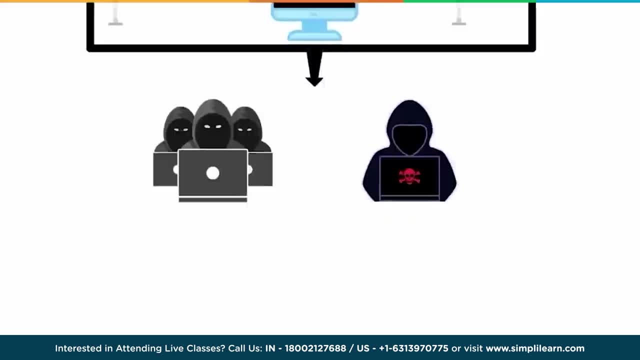 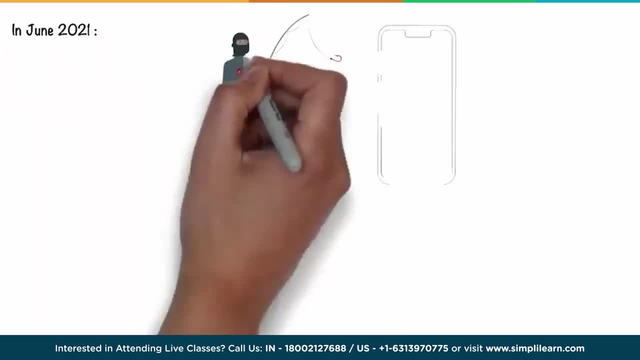 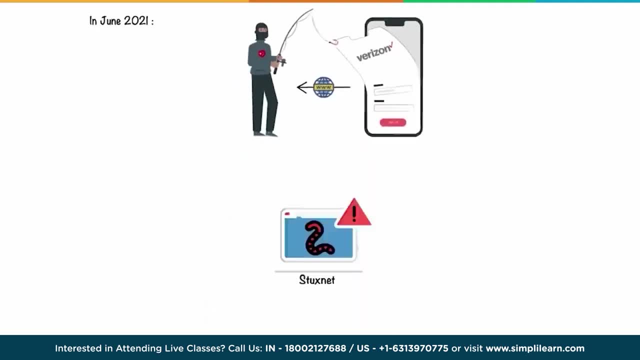 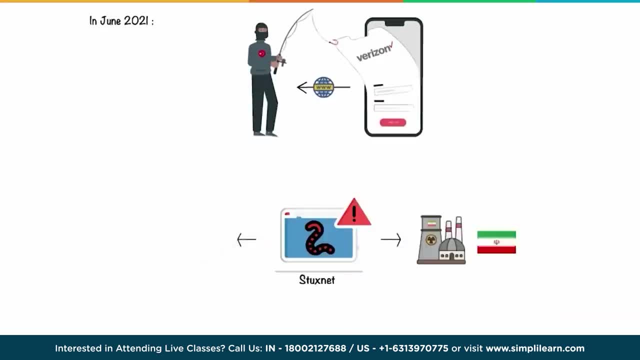 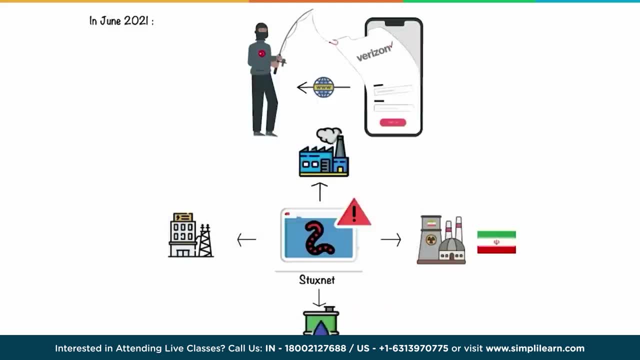 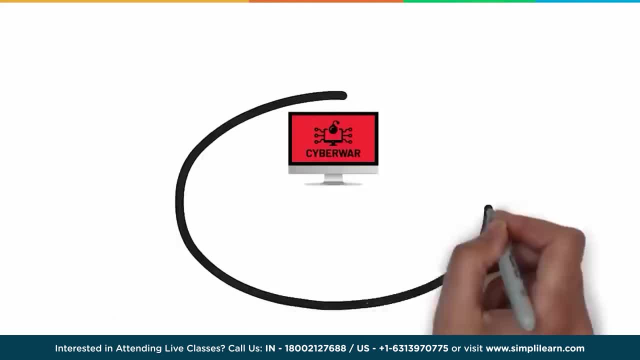 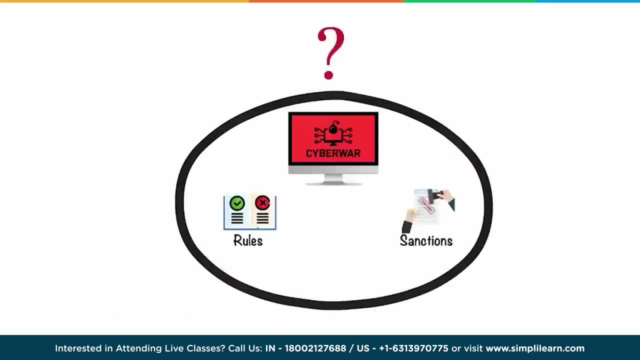 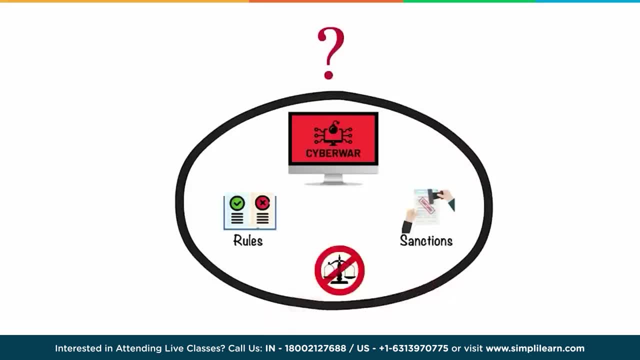 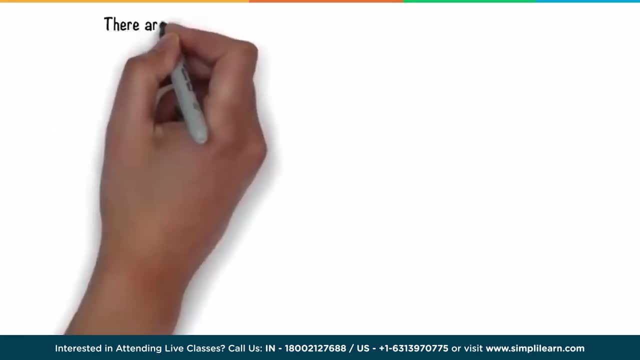 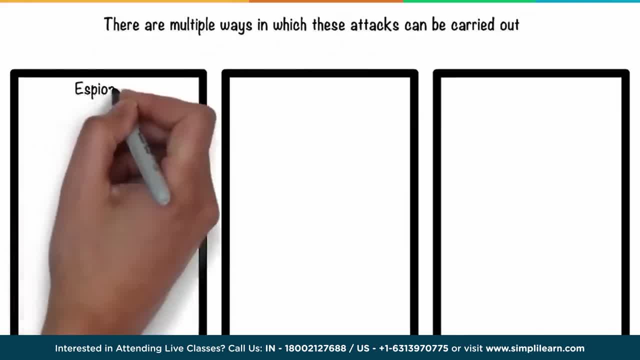 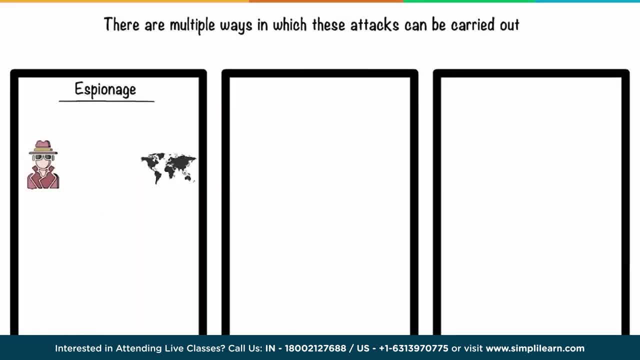 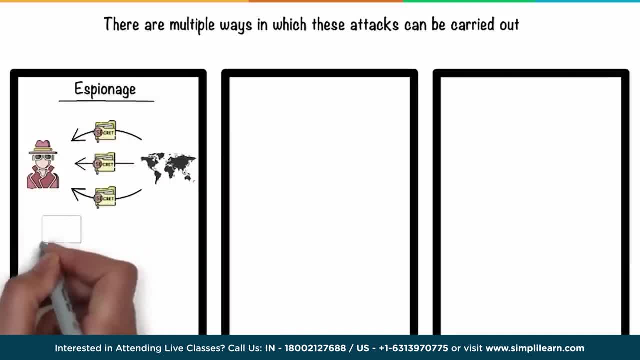 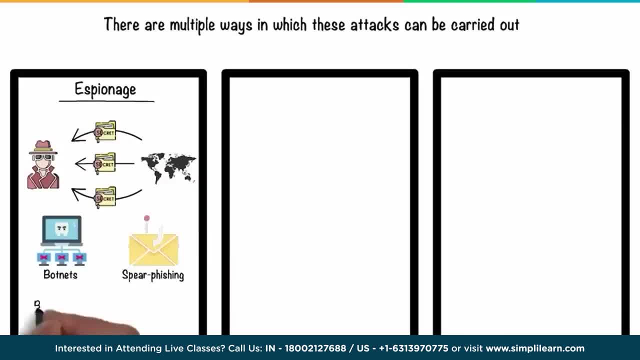 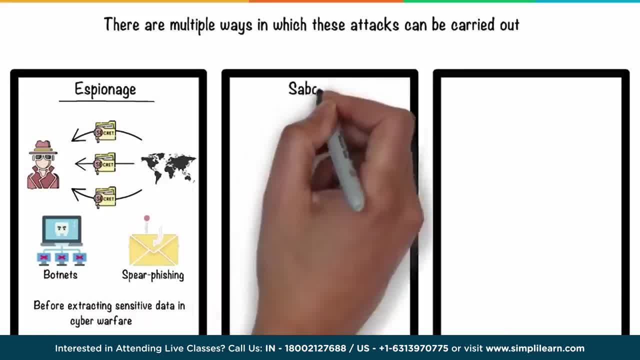 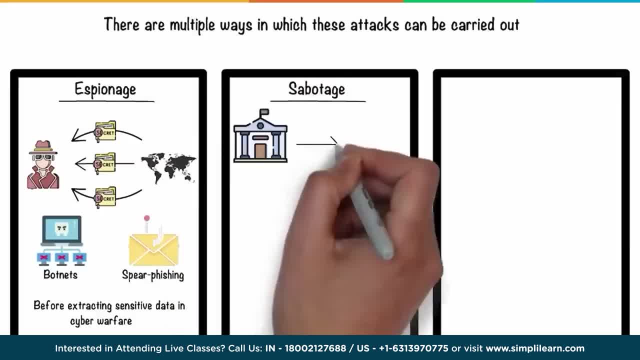 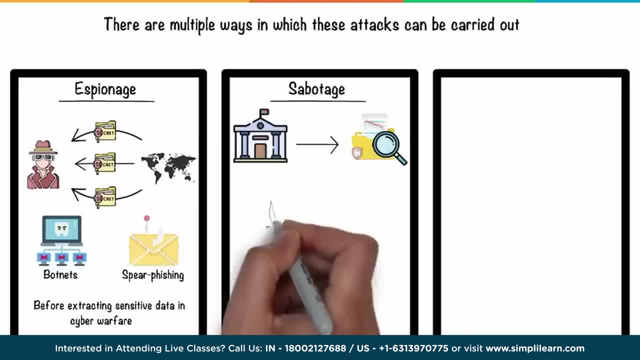 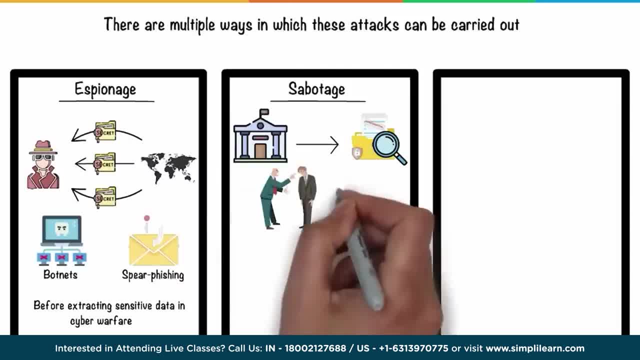 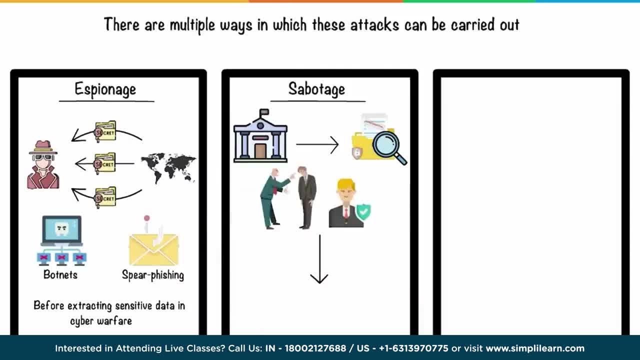 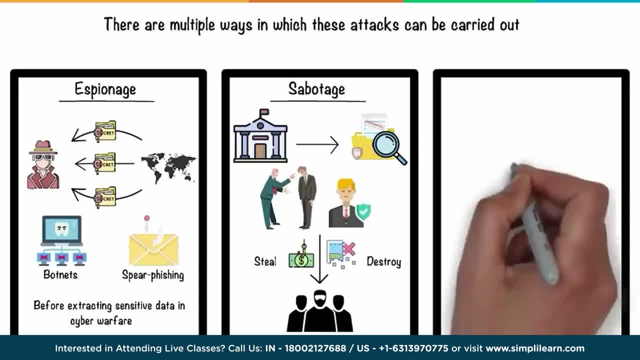 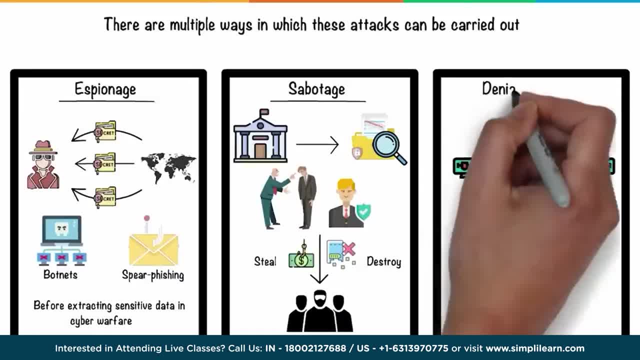 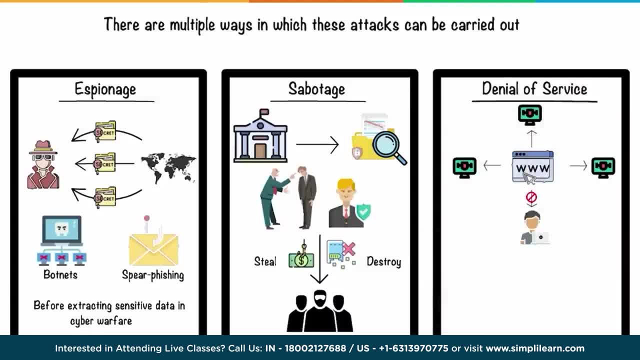 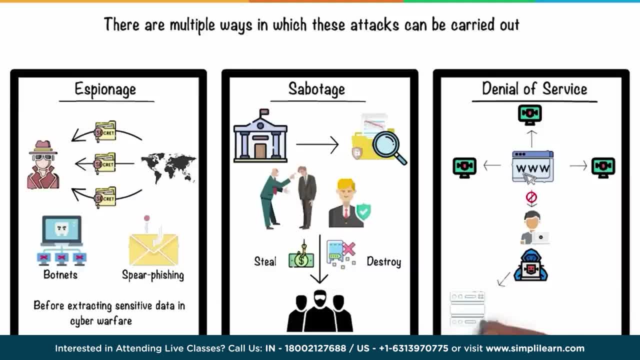 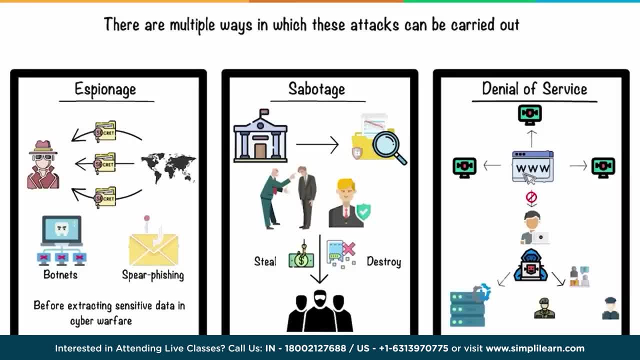 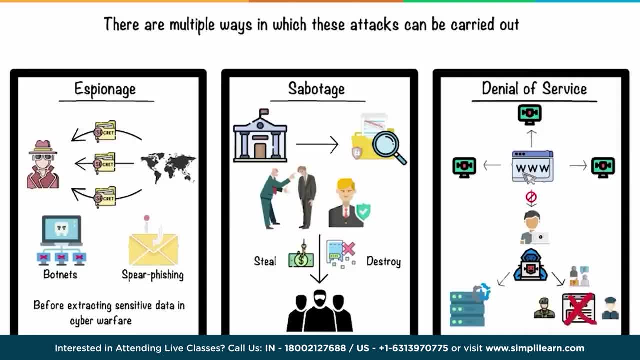 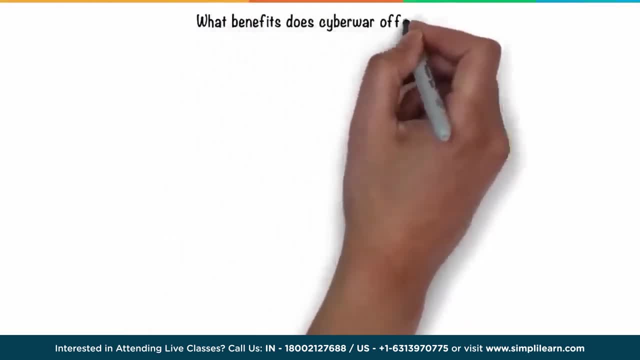 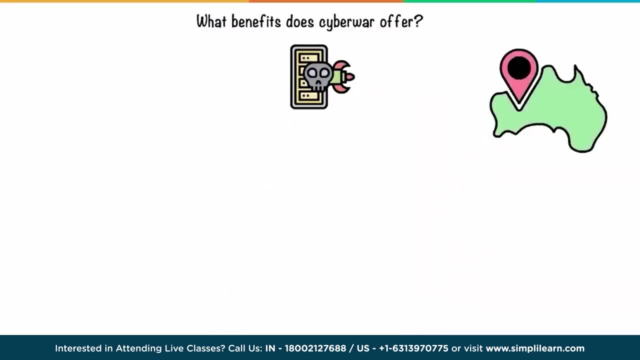 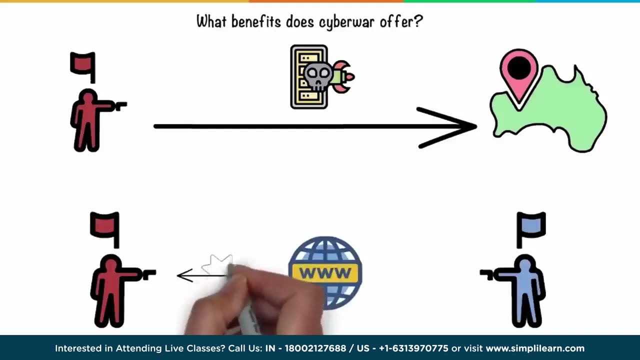 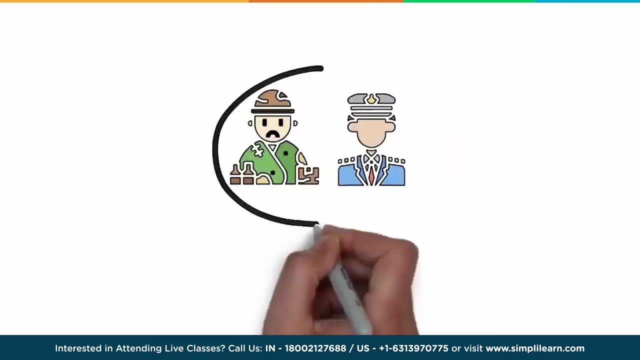 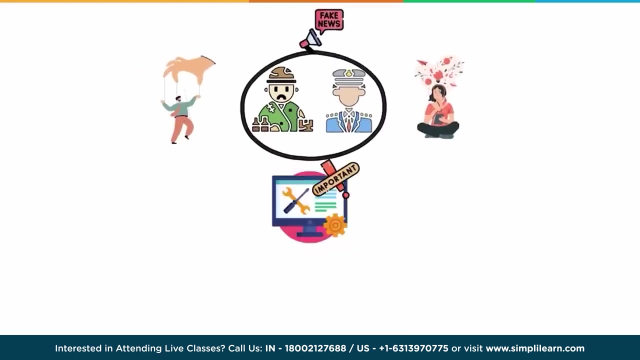 now for the next step. we will design two of the functions that will be used. Digital infrastructure is highly crucial in today's modern world, Starting from communication channels to secure storage servers. crippling a country's footprint and control on the internet is very damaging, But what are some of the ways we, as citizens, protect ourselves in the case of a cyber war? 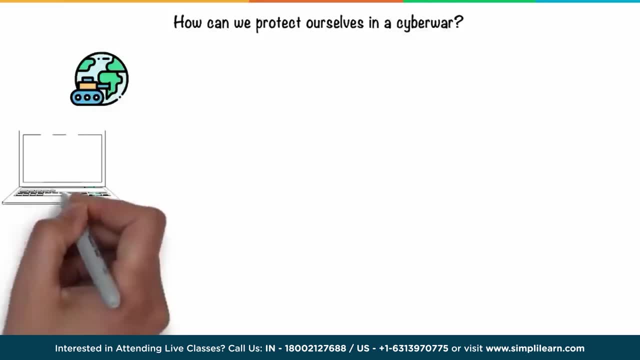 In the unfortunate event that your country is involved in warfare, be sure to fact-check every piece of information and follow only trusted sources. in that frame of time, Having conversations online should be limited to a need-to-know basis, considering propaganda campaigns have the power to influence the tide of war drastically. 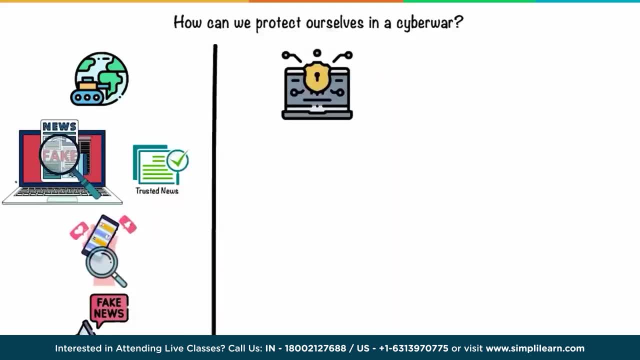 It is highly crucial to follow basic security guidelines to secure our devices, like regularly updating our operating systems, occasionally running full-system antivirus scans, etc. If your country or organization is being attacked. having devices segregated in a network goes a long way in bolstering security. 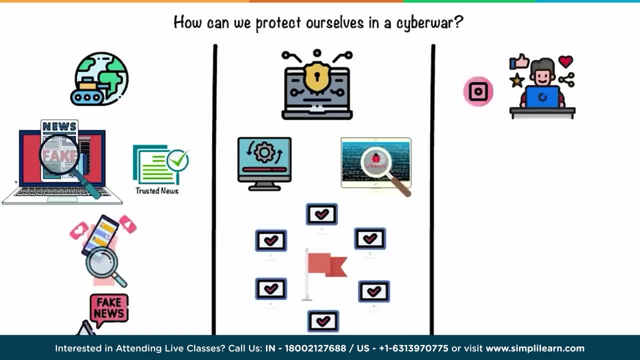 Try to avoid sharing information. In this era of Instagram and Facebook, divulging private information can be detrimental to keeping a secure firewall for your data. The more information an attacker has access to, the higher his chances of being able to devise a plan to infiltrate defenses. 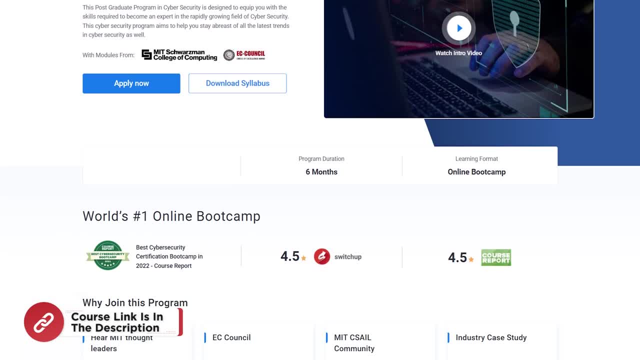 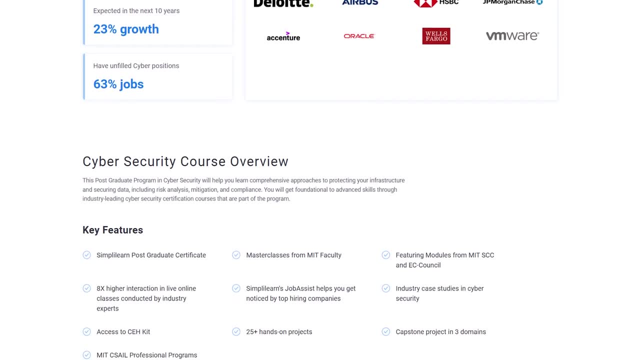 And if you are someone who is interested in building a career in cybersecurity- that is, by graduating from the best universities- or a professional who allocates to switch careers with cybersecurity by learning from the experts, Then try giving a shot to SimpliLearn's postgraduate program in cybersecurity with modules from: 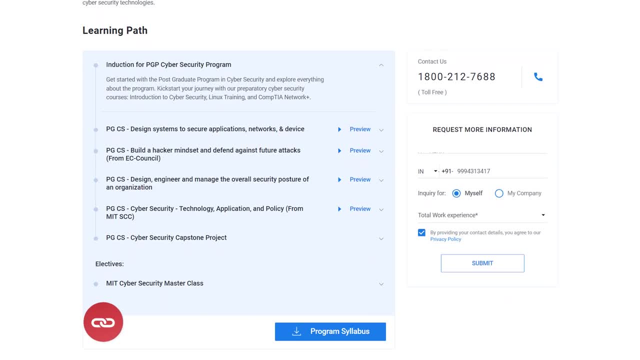 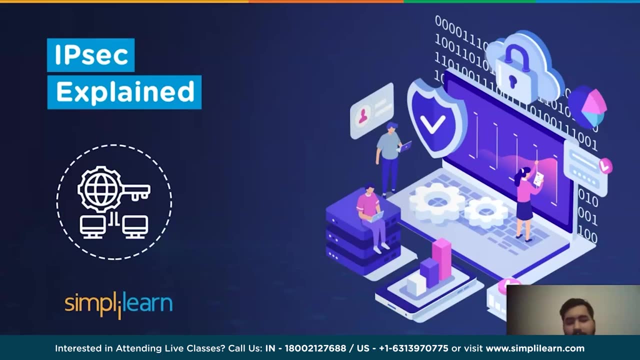 the MIT Schwarzman College of Engineering, And the course link is mentioned in the description box. that will navigate you to the course page where you can find a complete overview of the program being offered. During data transmission, there are various external factors which can affect the transmission. 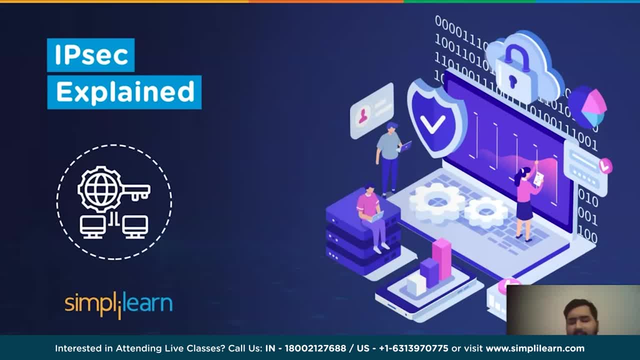 of data over a network channel. To prevent such cases from happening, we use Internet Protocol Security, which we will be discussing in this session on cybersecurity. Hi guys, and welcome to yet another interesting video by SimpliLearn. But before we begin, if you are watching tech videos, subscribe to our channel and hit the. 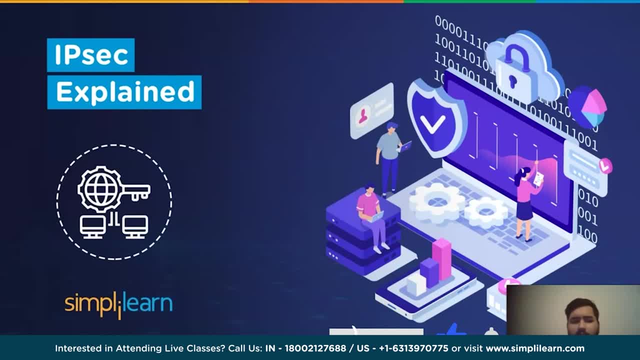 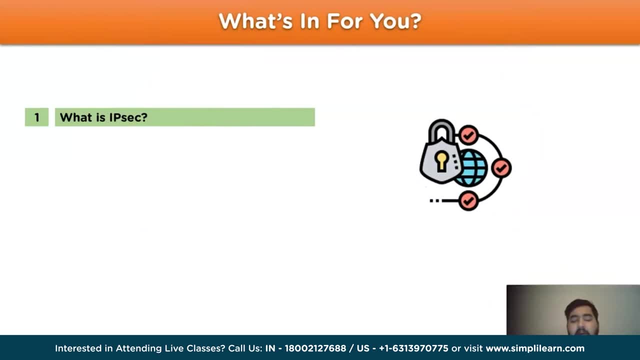 bell icon to never miss an update from us. Now, without further ado, let's take a look at the agenda for this session. To begin with, we will look into what is IPSec Continuing with. why do we use IPSec in our network, followed by components of IPSec. 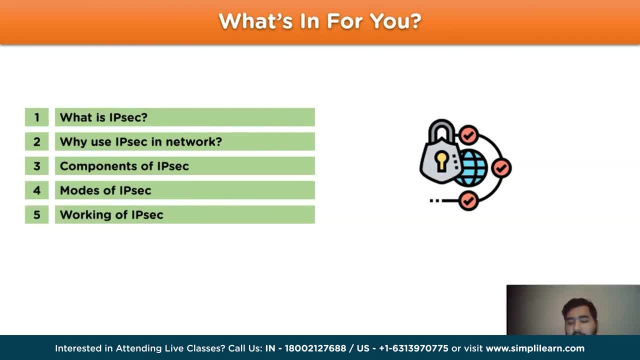 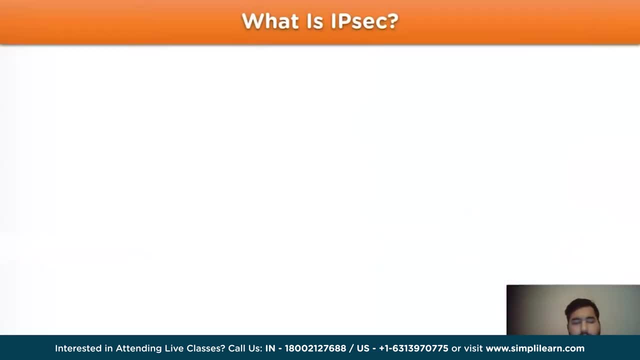 modes of IPSecure, and so on. As for the last topic, we will look into working steps involved in IPSecurity. Let's begin with the first heading, that is, what is IPSec? IPSec- Internet Protocol Security- is defined as a set of framework and protocol to ensure 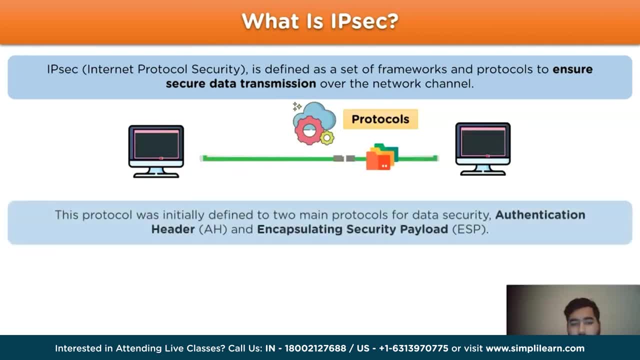 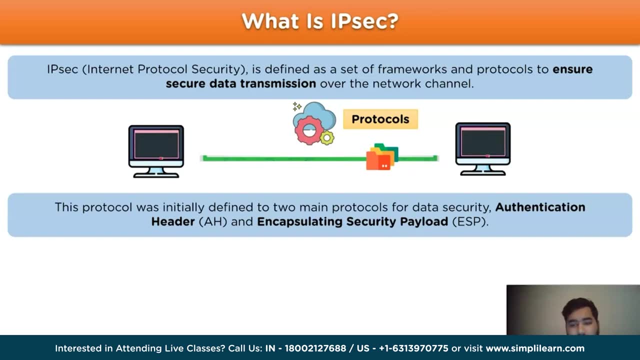 data transmission over a network channel. This protocol was initially defined of two main protocols for data security over a network channel. One is the Data Authentication Header, which is responsible for data integrity and anti-replay services, And the second protocol is Encapsulating Security Payload, in short ESP, which includes 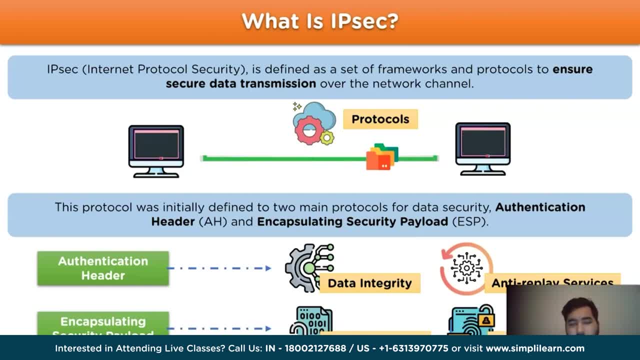 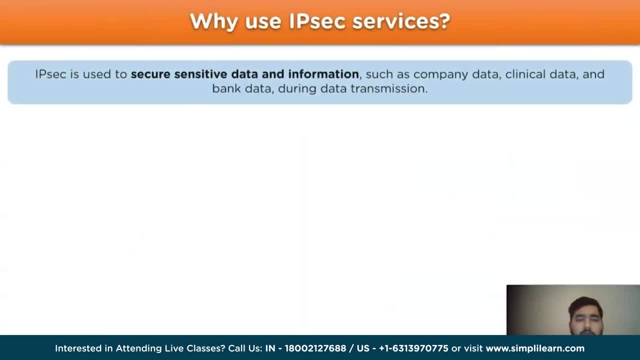 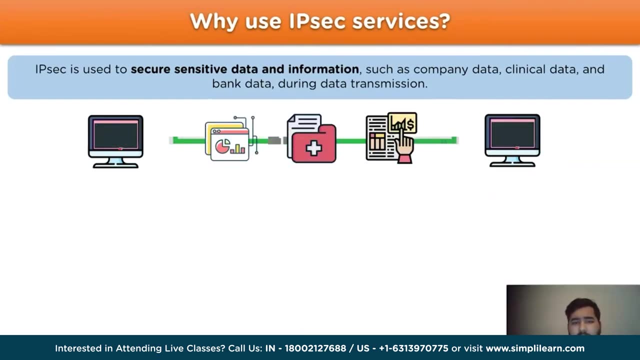 data encryption and data authentication. Now let's move on to the next heading. that is why do we use IPSec in our network. IPSec is used to secure sensitive data and information, Such as company data, Clinical data, Bank data. 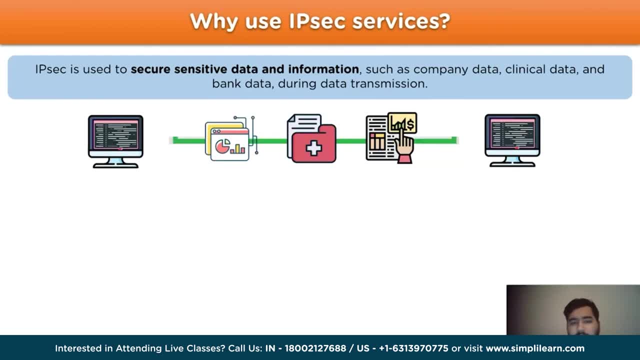 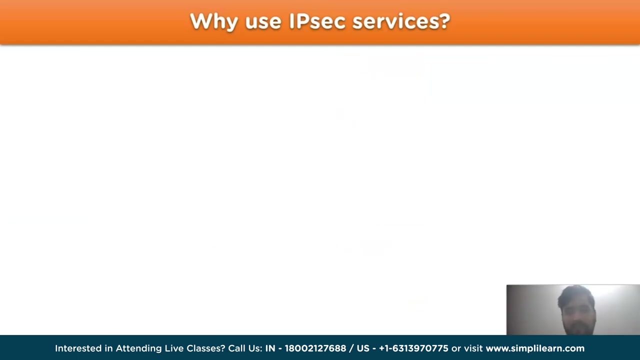 And various sensitive information regarding an institution which are used during data transmission over a network channel. The use of VPNs that are virtual private networks and apply IPSec protocols to encrypt the data for end-to-end transmission. Let's continue with why do we use IPSec services? 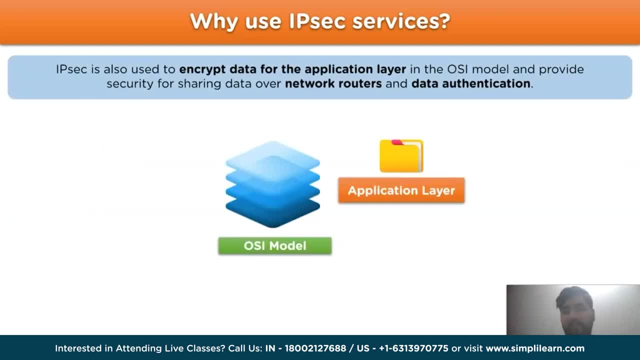 Those services also use to encrypt data for the application layer in the OSI model, and. 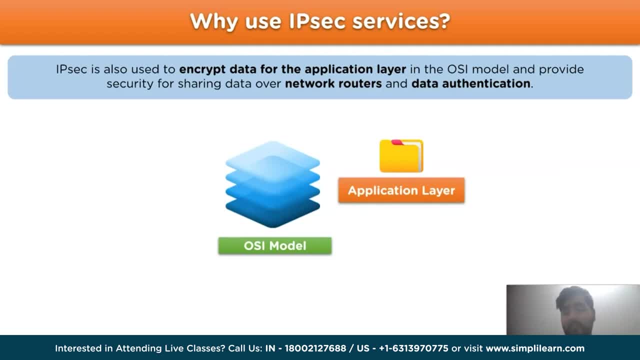 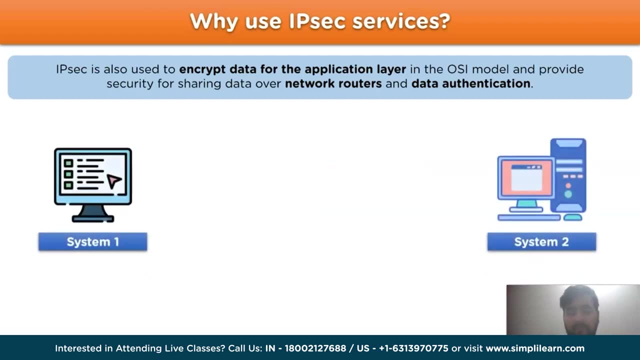 provide security for sharing data over network routers and data authentication. Let's take a look at the working of IPSec services. To begin with, we have two different systems- System 1 and System 2, which will establish a network channel and then the encryption of data will takes place when one host will. 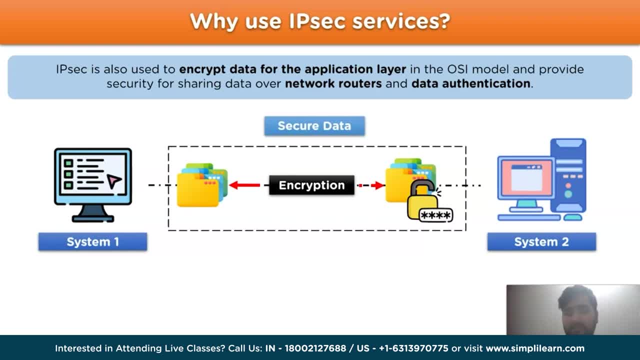 share the data to the second host. 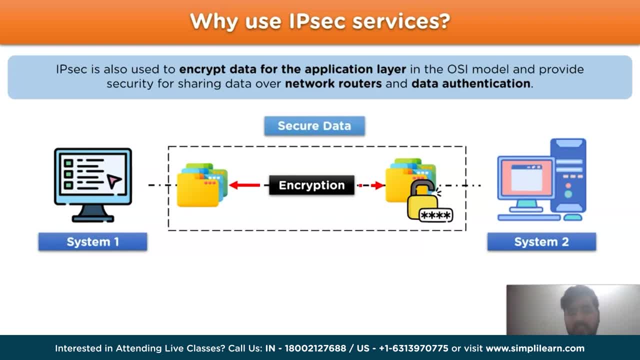 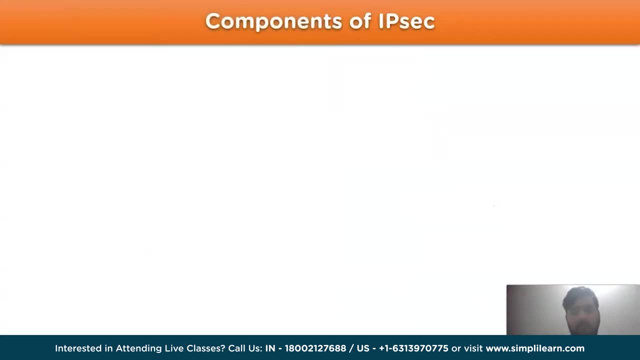 IPsec services will secure the data that is to be transferred over the network channel by applying router encryption and authentication. Now let's move on to the next topic, that is, components of IPsec. The IPsec services comprises of multiple protocols that ensure the data transmission over the 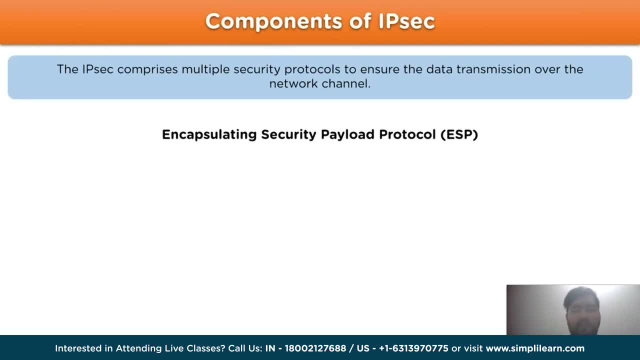 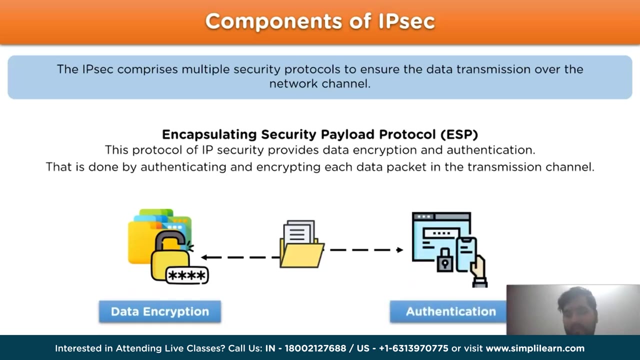 network channel. The first one is Encapsulating Security Payload Protocol, in short ESP. This protocol of IP security provides data encryption and authentication services, And it also authenticates and encrypts the data packet in the transmission channel. Moving on, we have Authentication Header, in short AH. 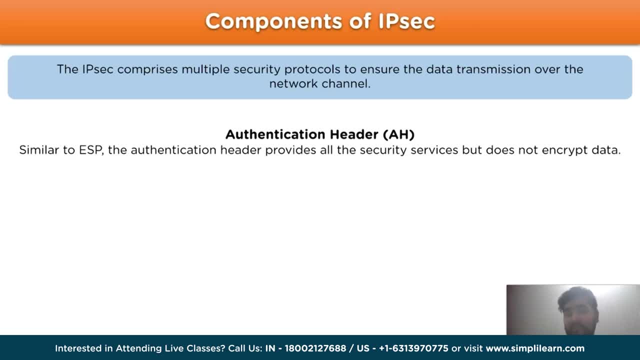 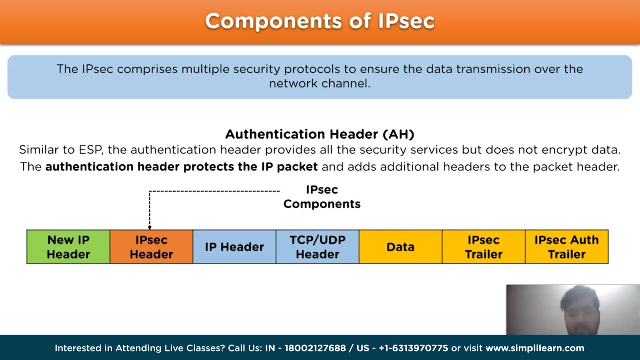 Similar to ESP, the authentication header also provides all the security services, but it does not encrypt the data. It also protects the IP packet and adds additional headers to the packet header. The modified IP datagram looks this way where the IP components are included at the second. 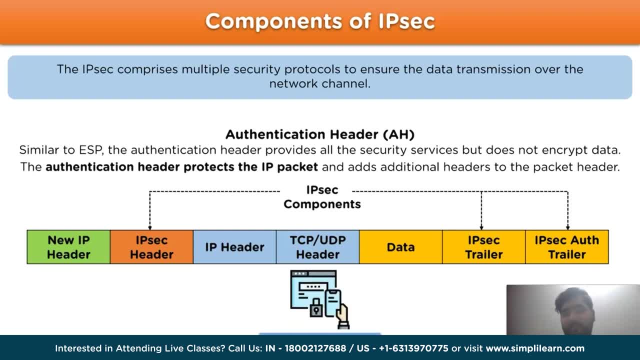 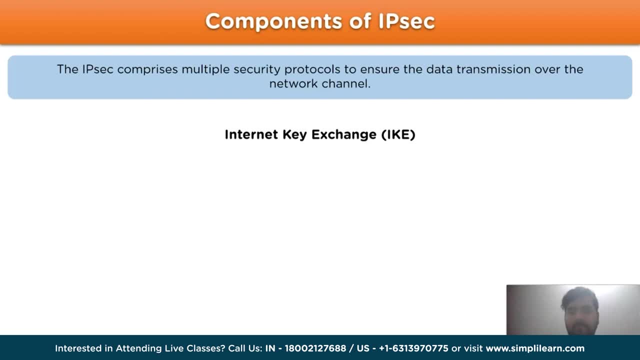 position, the seventh position and the sixth position, along with the authentication of data services over the network channel. Moving on, we have Internet Key Exchange. This protocol provides protection for content data And also changes the attribute of the original data to be shared by implementing SHA and. 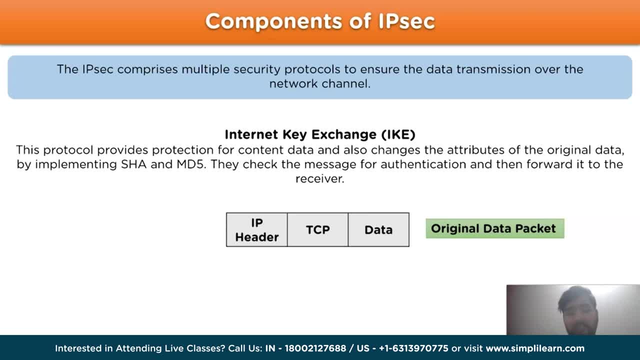 MD5 algorithms. They also check the message for authentication and then only is forwarded to the receiver side. For example, this is the original data packet we are used to with IP header, path, TCP, UDP and data, Whereas this is the modified IPsec data packet where ESP header is added between IP header. 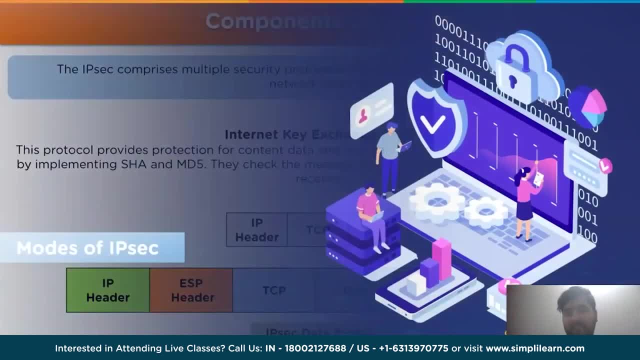 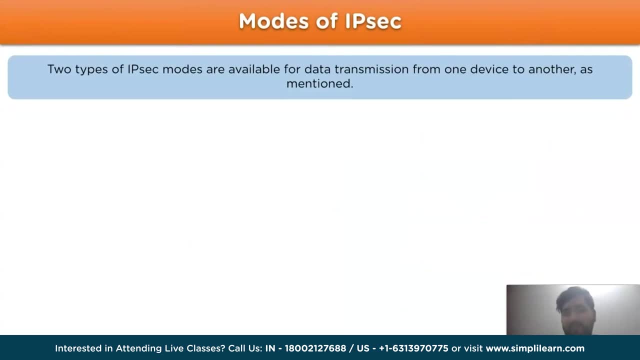 and the TCP protocol. Now let's move on to the next heading, that is, modes of IPsec. There are basically two types of IPsec modes available for data transmission over the network channel, Where the first one is Tunnel mode. This mode of transmission is used to secure gateway to gateway data. 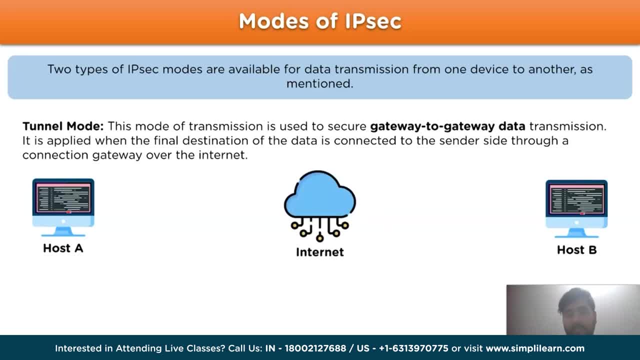 It is applied when the final destination of the data is to be connected to a sender site through a connection gateway or a network Over the internet. For example, we have two hosts, host A and host B. Through the host A, we are sending a message to host B, which will pass through a gateway. 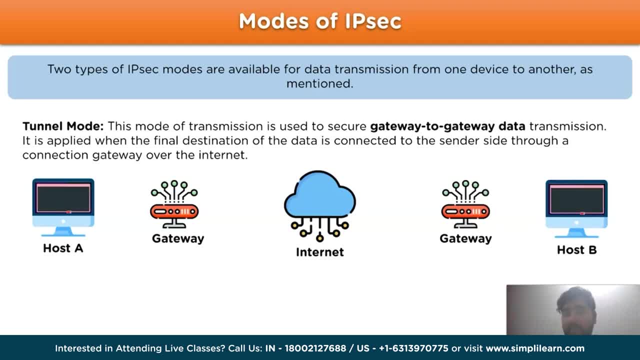 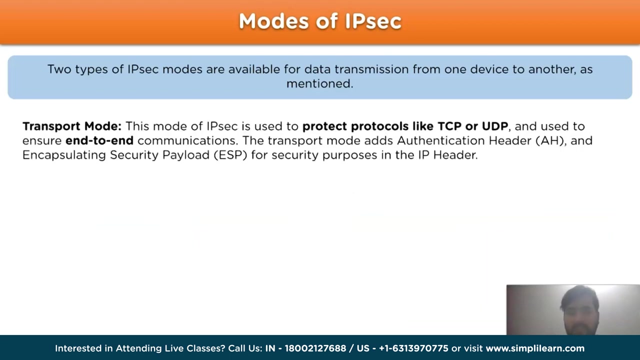 at host A point And it passes through a gateway to host B, then This is a basic format for gateway to gateway data transmission, And the given IP datagram format is used for Tunnel mode. Now let's move on to the second mode of IPsec, that is, Transport mode. 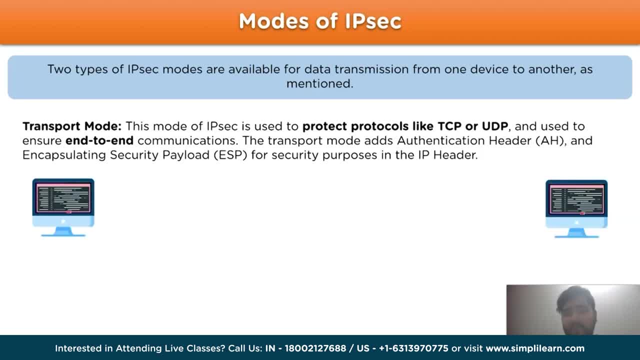 This mode of IPsec is used to protect protocols like TCP or UDP and is used to ensure end-to-end communication. unlike Tunnel mode, The transport mode data at authentication header and encapsulating security payload for security purpose in the IP header. The path: This is the modified IP datagram for transport mode. 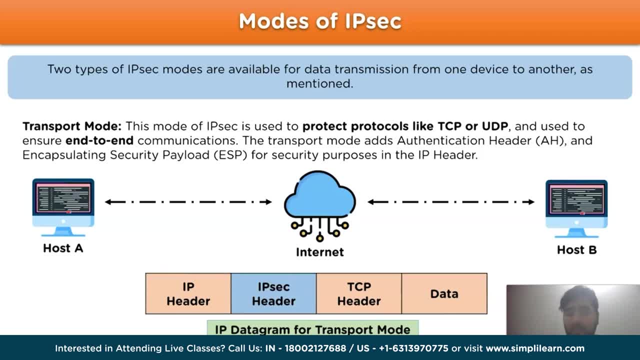 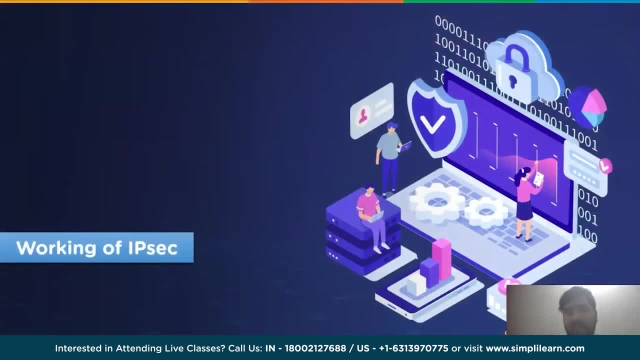 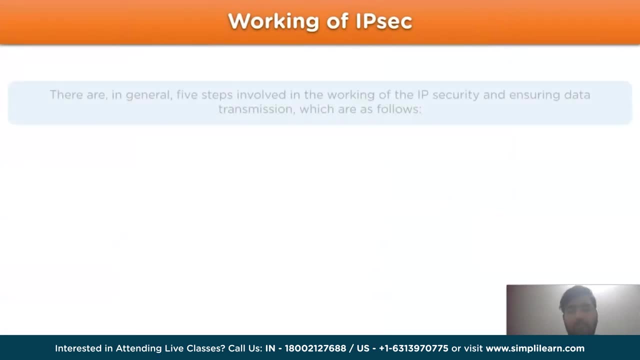 The point to be noted is the IPsec header is always added between IP header and TCP header. Now let's move on to the last setting for this session on IPsec, that is, the working steps involved in IP security In general. there are five steps involved in the working of IPsec to ensure data transmission over a network channel. 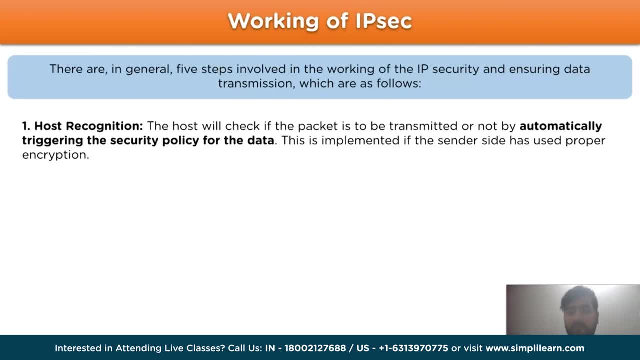 The first step is host recognition. In the first step the host system will check if the packet is to be transmitted or not by automatically triggering the security policy for the data which is implemented by the sender side for proper encryption. Then the second step is known as IKE phase one. 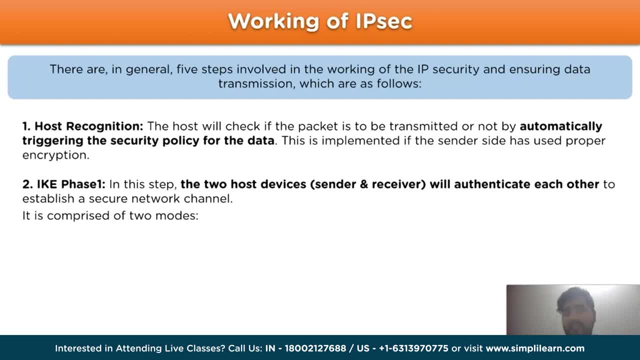 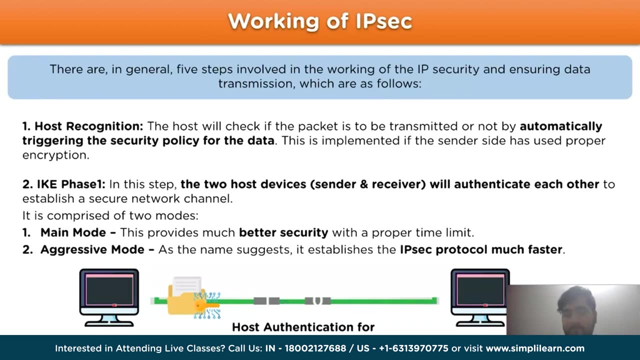 In this step, the two host devices, the sender and the receiver side, will authenticate each other to establish a secure network channel. It is comprised of two modes: the main mode. this provides much better security with a proper time limit, And the second mode, known as aggressive mode, as the name suggests. 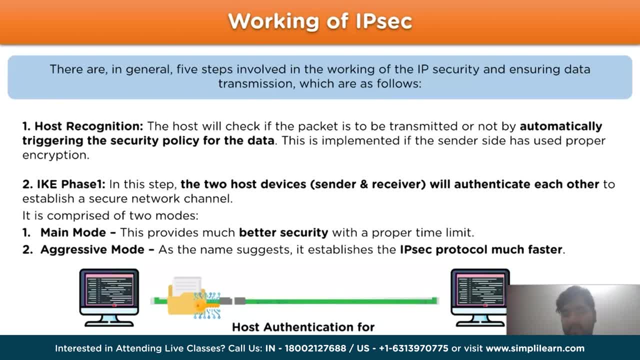 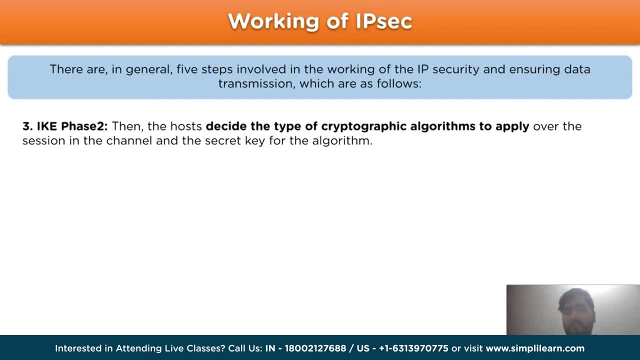 it establishes the IPsec protocol much faster in comparison to main mode. Let's move on to the third step, which is IKE phase two. After the second step, the host system will provide the type of cryptography algorithm to apply over the session in the network channel. 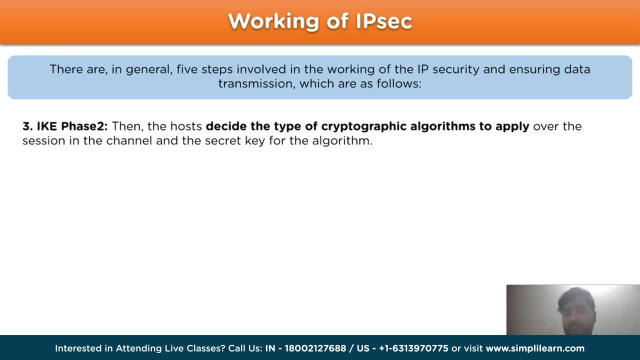 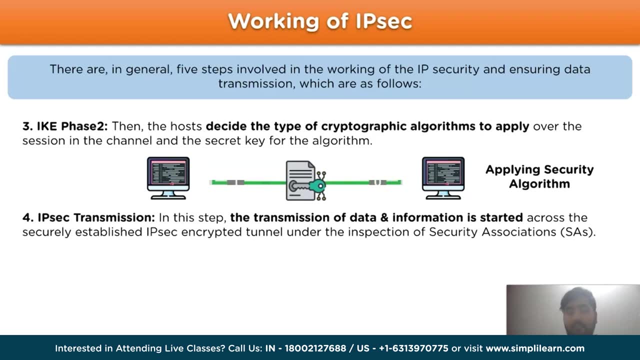 and the secret key for the algorithm to be used to encrypt the data for transmission. Then we have IPsec transmission. This step involves the actual transfer of data over the network channel using the various protocols used in IPsec security, which are implemented under the tunnel condition. 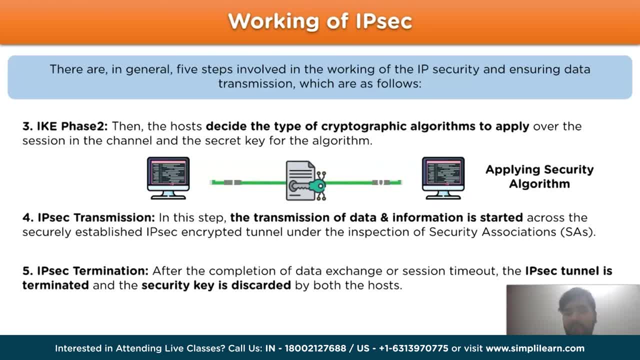 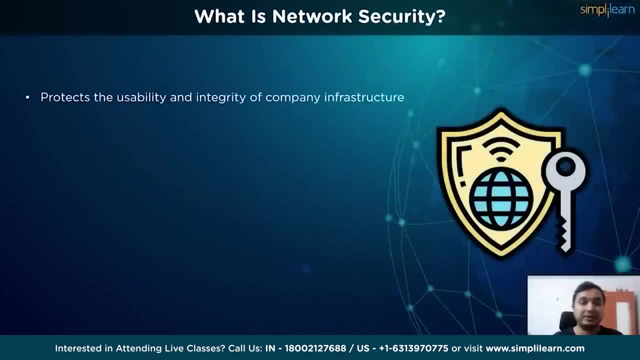 And the last step is IPsec termination. After the completion of data exchange or session timeout, the IPsec tunnel is terminated and the security key established is discarded by both the host system. Network security is a set of technologies that protects the usability and integrity of a company's infrastructure. 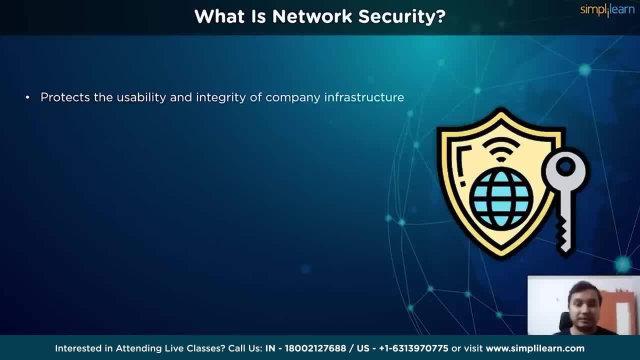 by preventing the entry or proliferation within a network. Its architecture comprises of tools that protect the network itself and the applications that run over it. Effective network security strategies are the following: Network security strategies employ multiple lines of defense that are scalable and automated. Each defensive layer here enforces a set of security policies, which are determined by the administrator beforehand. 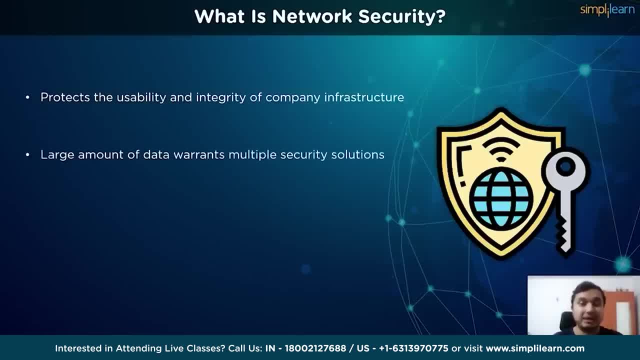 This aims at securing the confidentiality and accessibility of the data and the network. Every company or organization that handles a large amount of data has a degree of solutions against many cyber threats. The most basic example of network security is password protection. It has the network the user chooses. 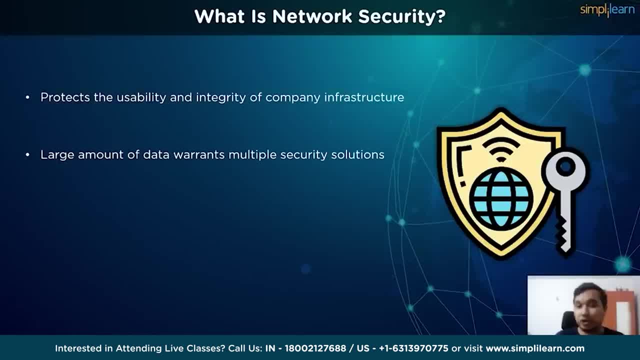 Recently, network security has become the central topic of cyber security, with many organizations involving applications from people with skills in this area. It is crucial for both personal and professional networks. Most houses with high-speed internet have one or more wireless routers, which can be vulnerable to attacks if they are not adequately secured. 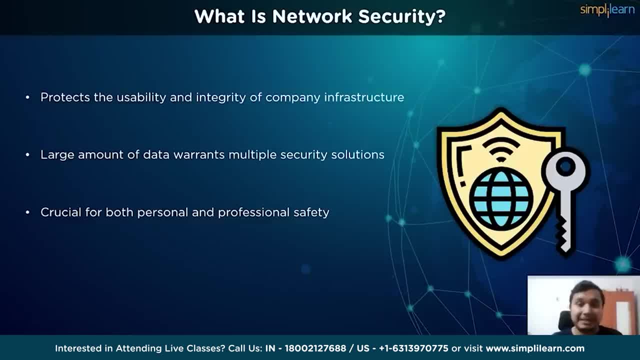 Data loss, theft and sabotage risk may be decreased with the usage of a strong network security system. The workstations are protected from hazardous firewalls. The network security system can be used to secure the data that is being shared over a network. Additionally, it guarantees the security of the data which is being shared over a network. 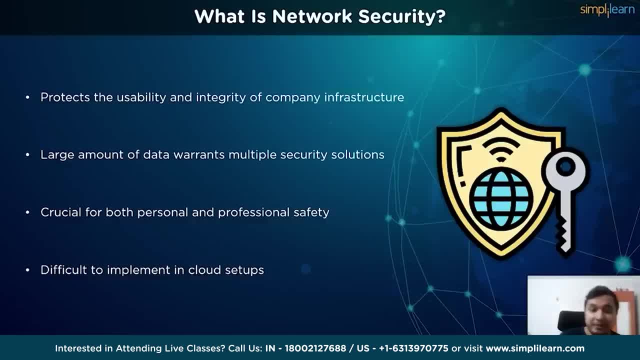 By dividing information into various sections, encrypting these portions and transferring them over separate pathways. network security infrastructure offers multiple levels of protection to thwart man-in-the-middle attacks, preventing situations like eavesdropping, among other harmful attacks. It is becoming increasingly difficult in today's hyper-connected environment, as more corporate 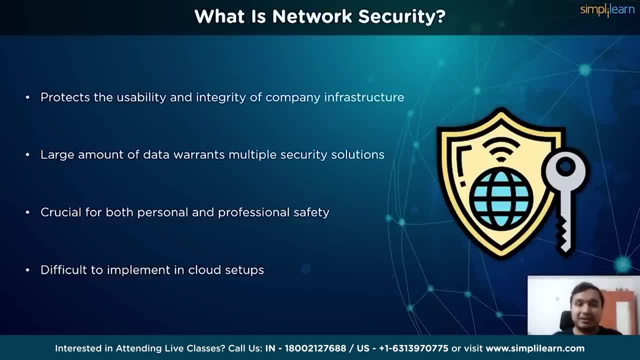 applications migrate to both public and private networks. This means that the network security infrastructure can be used to protect the data that is being shared over a network. Additionally, modern applications are also frequently virtualized and dispersed across several locations, some outside the physical control of the IT team. 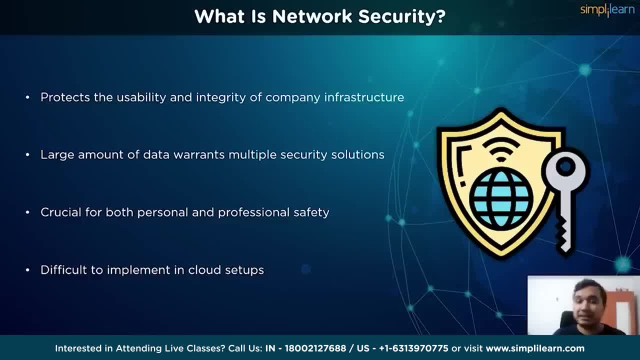 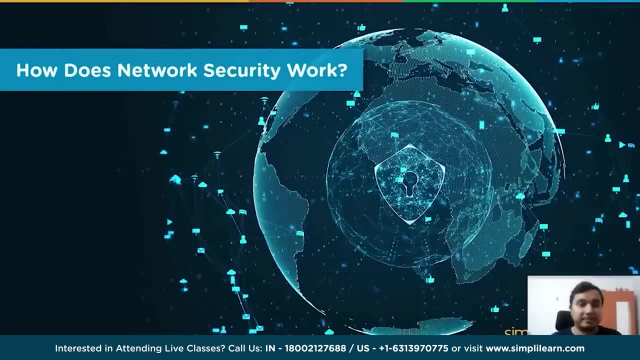 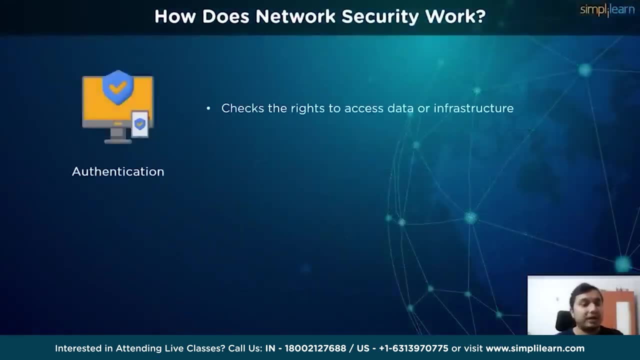 Network traffic and infrastructure must be protected in these cases, since assaults on businesses are increasing every single day. We have now understood the basics of network security, But we need to understand how network security works. in the next section in slightly more detail, Network security revolves around two points. 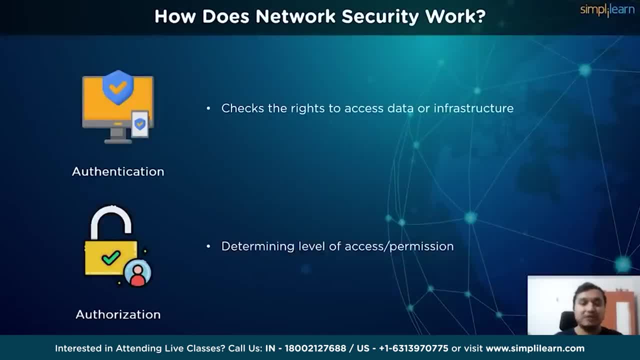 Authentication and authorization. The first process, which is authentication, is similar to access paths which ensure that only those who have the right to enter a building. In other words, authentication checks and verifies that it is indeed the user belonging to the network who is trying to access or enter it, thereby preventing unauthorized intruders. 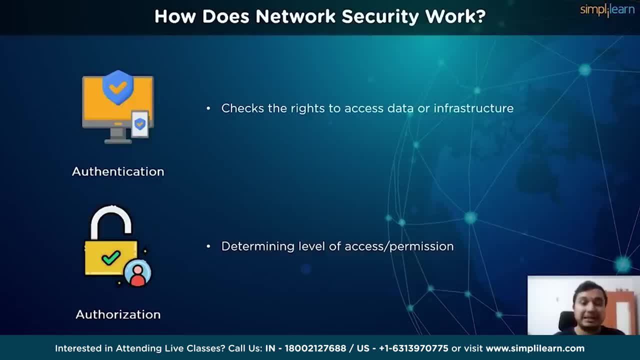 Next comes authorization. This process decides the level of access provided to the recently authenticated user. For example, the network admin needs access to the entire network, whereas those working within it probably need access to only certain areas within the network, Based on the network user's role. the process of determining the level of access. 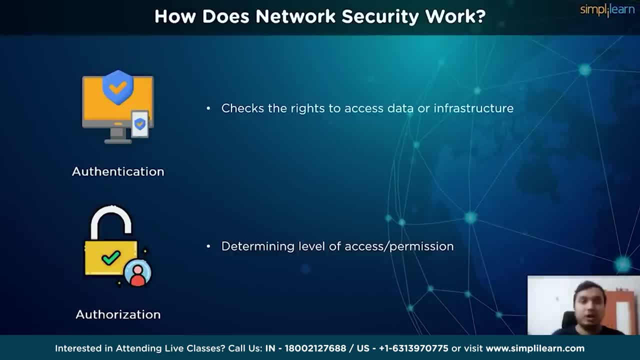 or permission level is known as authorization. Today's network architecture is complex and faces a threat environment that is always changing and attackers that are always trying to find and exploit vulnerabilities. These vulnerabilities can exist in many areas, including devices, devices and devices. 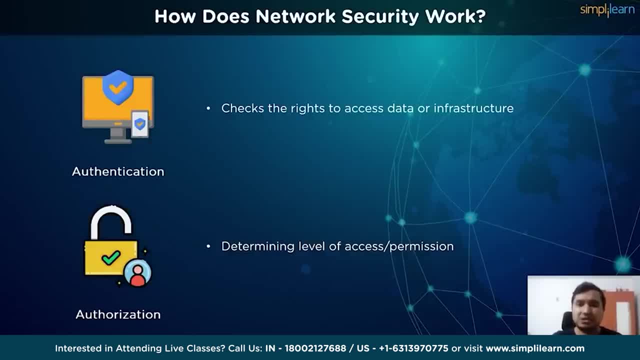 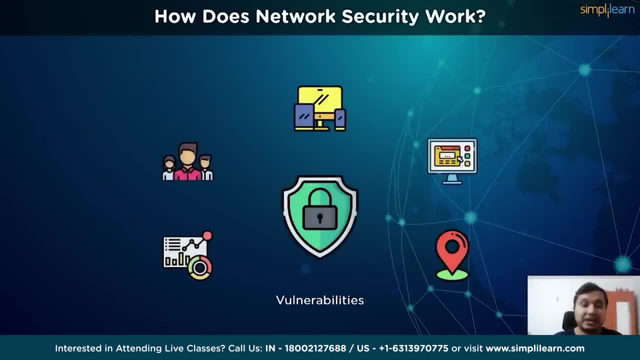 These vulnerabilities can exist in many areas, including devices, devices and devices. These vulnerabilities can exist in many areas, including devices, devices, data applications, users and locations. For this reason, many network security management tools and applications are in use today that 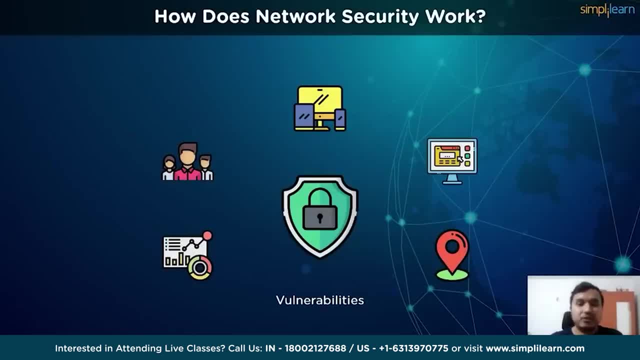 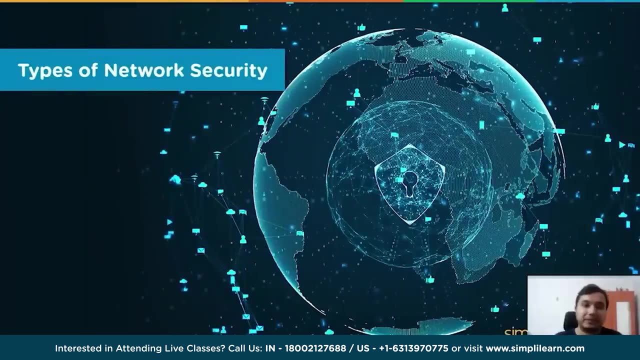 address individual threats. When just a few minutes of downtime can cause widespread disruption and massive damage to an organization's bottom line and reputation, it is essential that these protection measures are in place beforehand. Now that we know a little about network security and its working, let's cover the different. 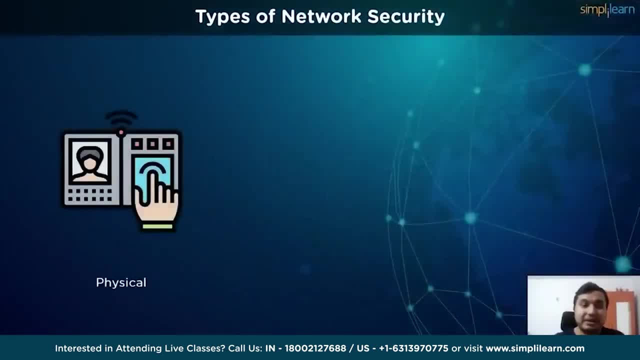 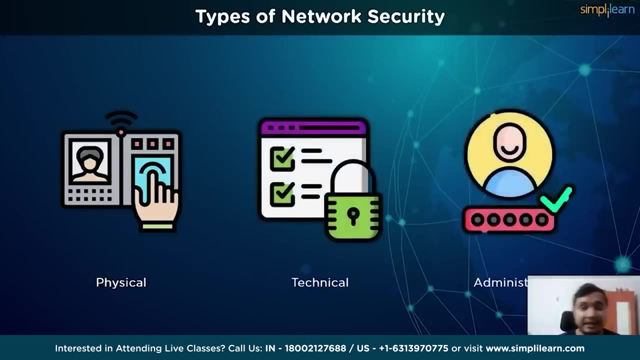 types of network security. The fundamental tenet of network security is the layering of protection for massive networks and stored data that ensure the acceptance of rules and regulations As a whole. there are three types, The first of which is physical security, the next being technical and the third being 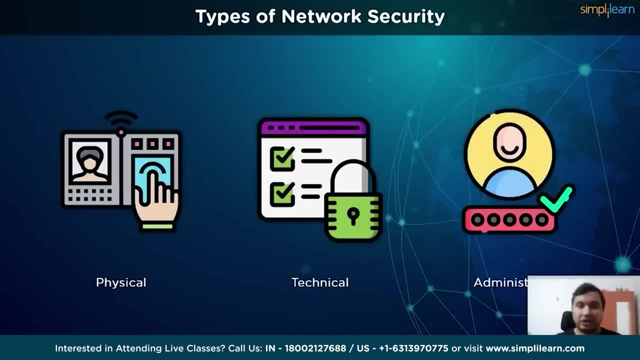 administrative. Let's look into physical security first. This is the most basic level. that includes protecting data and network to unauthorized personnel from acquiring control over the code. The second is confidentiality of the network. This includes external peripherals and routers that might be used for cable connections. 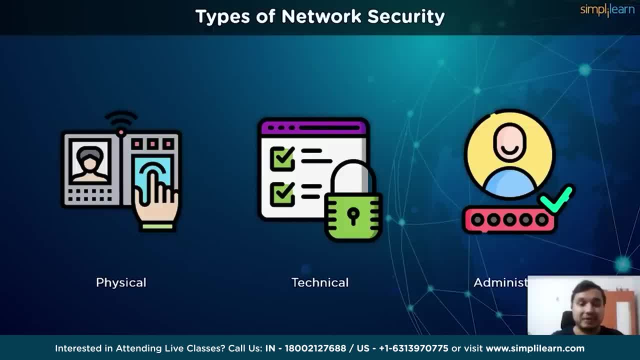 The same can be achieved by using devices like biometric systems. Physical security is critical, especially for small businesses that do not have many resources to devote to security personnel and the tools, as opposed to large firms. When it comes to technical network security, it focuses mostly on safeguarding data either. 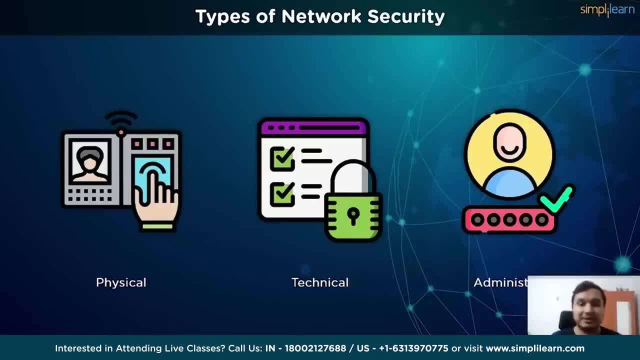 kept in the network or engaged in network transitions. This kind fulfils two functions. One is defense against unauthorized users, The other is a defense against malevolent actions. The last category is administrative. This level of network security protects user behavior, like how the permission has been. 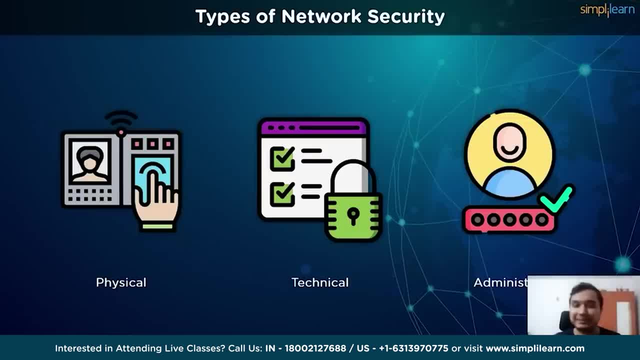 granted and how the authorization process takes place. This also ensures the level of sophistication the network might need to protect it through all the attacks. This level also suggests necessary amendments that have to be done to the infrastructure. I think that's all the basics that we need to cover on network security. 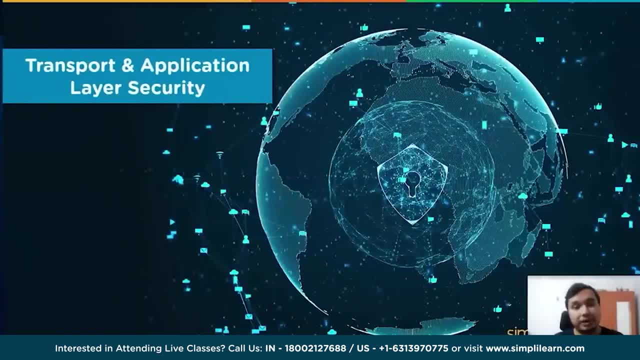 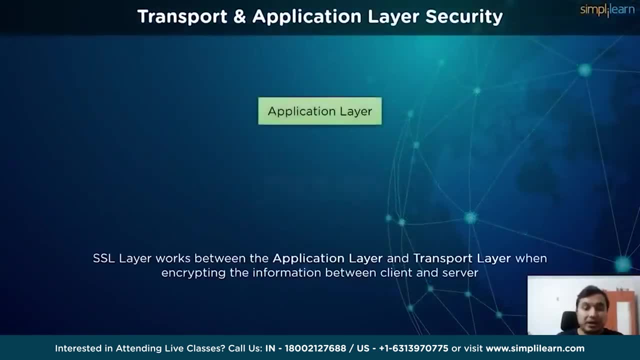 In which our next topic. we're going to go through two mediums of network security, which are the transport layer and the application layer. The transport layer is a way to secure information as it is carried over the internet, with users browsing websites, emails, instant messaging, etc. 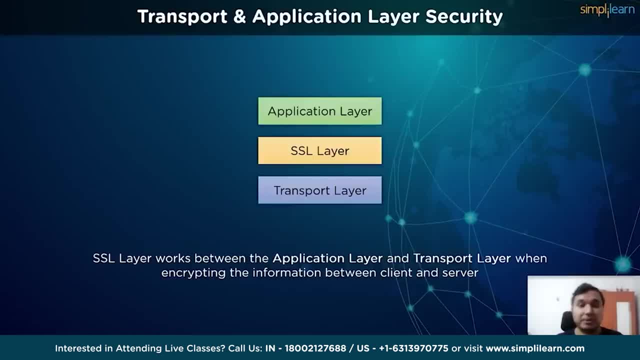 TLS aims to provide a private and secure connection between a web browser and a website server. It does this with a cryptographic handshake between two networks, The two systems, using public key cryptography. The two parties to the connection exchange a secret token and, once each machine validates, 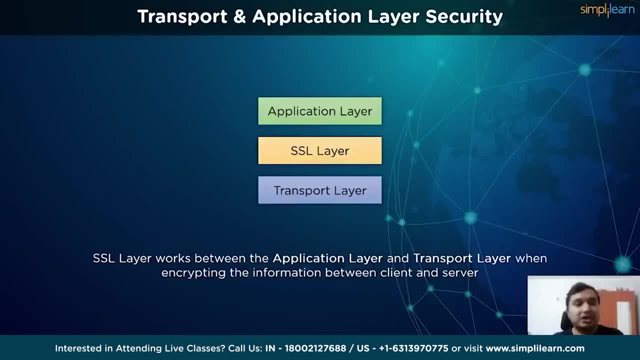 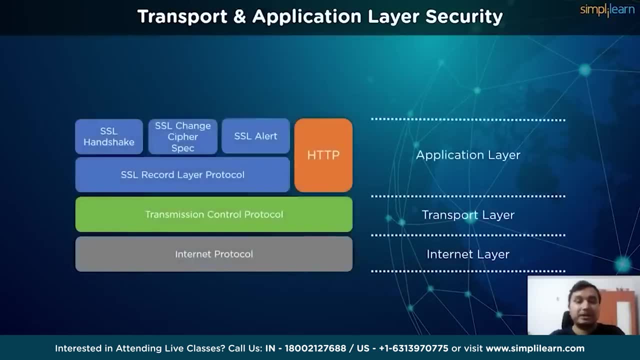 this token, it is used for all communications. The connection employs lighter symmetric cryptography to save bandwidth and processing power. Since the application layer is the closest layer to the end user, it provides hackers with the largest threat surface. Poor app layer security can lead to performance and stability issues, data theft and, in some 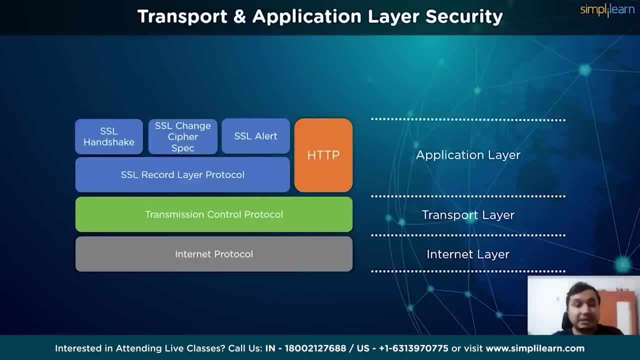 cases, the network being taken down. Examples of application layer attacks include distributed denial of service attacks or DDoS attacks, HTTP floods, SQL injections, cross-site scripting, etc. Most organizations have an arsenal of application layer security protections to combat these and more, such as web application firewalls, secure web gateway services, etc. 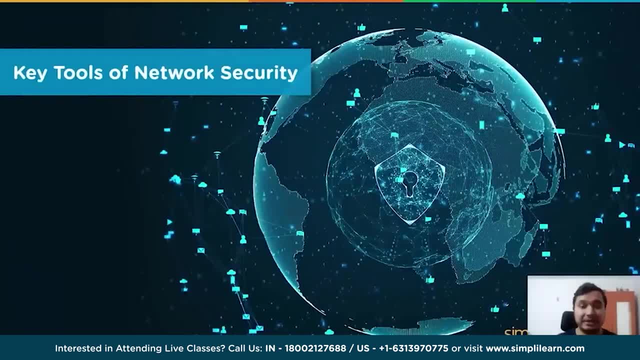 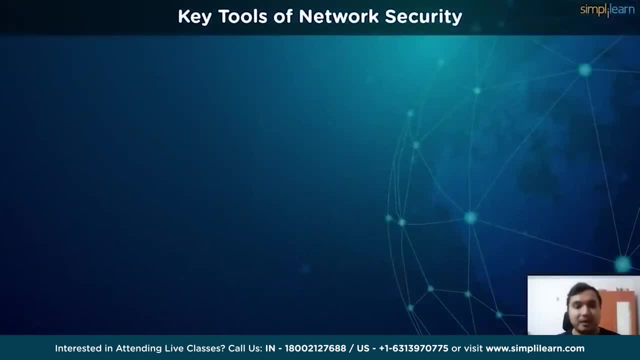 Now that we have the theory behind network security has been covered in detail, let us go through some of the tools that can be used to enforce these. The first tool to be covered in this section is a firewall. A firewall is a type of network security device that keeps track of incoming and outgoing 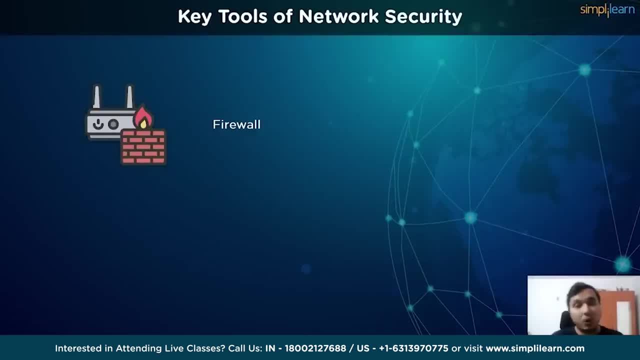 network traffic and it decides which traffic to allow or deny, in accordance to a set of security rules. For more than 25 years, firewalls have served as network security's first line of defense. They provide a barrier between trustworthy internal, protected and regulated networks from shady external threats. 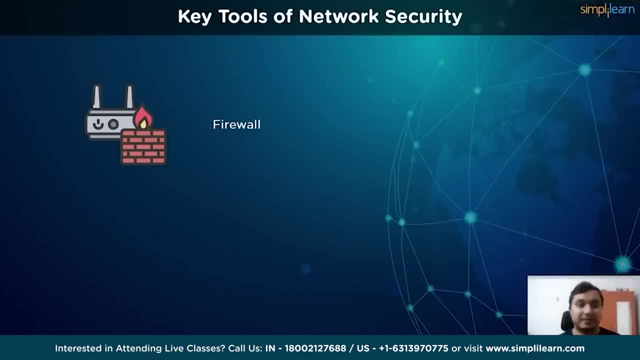 The next tool which can be used to bolster network security is a virtual private network, or VPN for short. It's an encrypted connection between a device and a network via the internet. The encrypted connection aids the secure transmission of sensitive data. It makes it impossible for unauthorized parties to eavesdrop on the traffic and enables remote 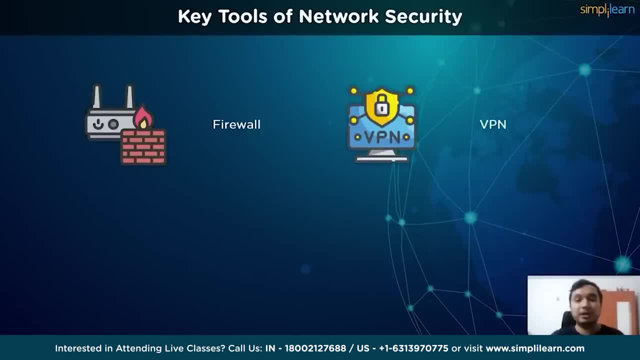 work for the user. The usage of VPN technology is common in both corporate and personal networks. Next, we cover the importance of Intuition Prevention Systems in Network Security or IPS frameworks. An Intuition Prevention System is a network security tool that continually scans the network. 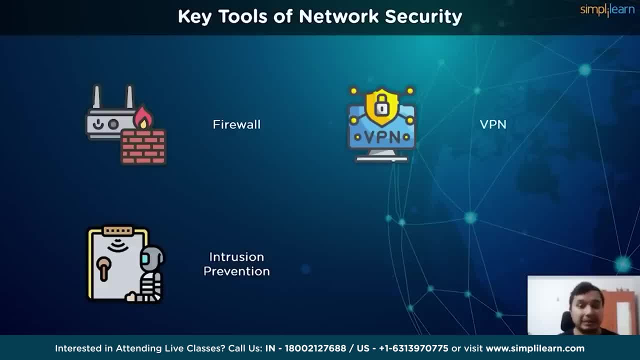 for harmful activity and responds to it when it does occur, by reporting, blocking or discarding it. It can be either hardware or software. It's more sophisticated than an Intuition Detection System or an IDS framework which can just warn an administrator and merely identify harmful activities. 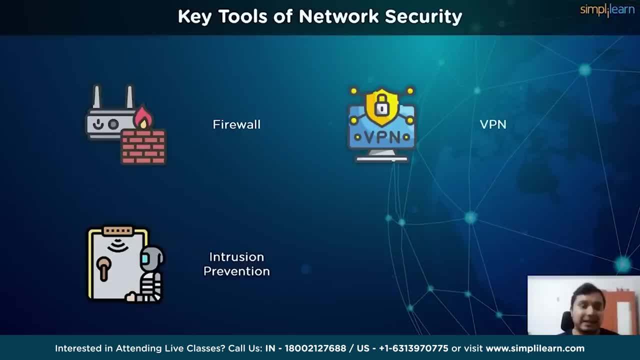 While a network security system can be used to identify and detect harmful activity, While in the case of an IPS, it actually takes against that activity. The next tool in this section, and the final one, are going to be Behavioral Analytics. Behavioral Analytics focus more on the statistics that are being carried over and stored through. 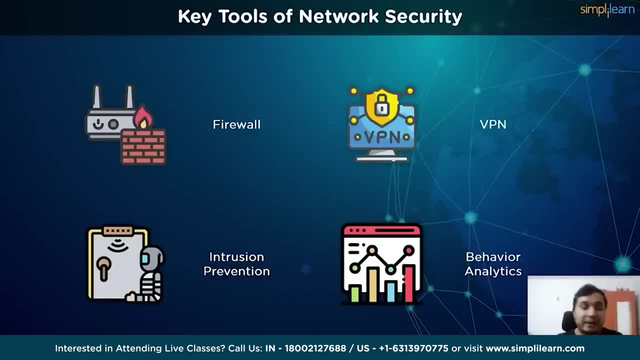 months and years of usage. Once some kind of similar pattern is noted, where the IT administrator can detect some kind of attack, the similar attacks can be stopped and the security can be further enhanced. Another: we have covered all that we need to know about network security, the necessary 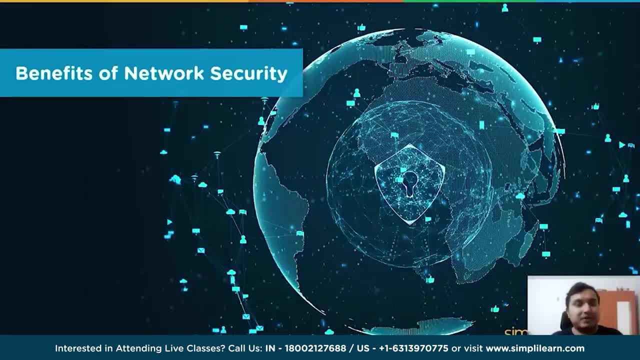 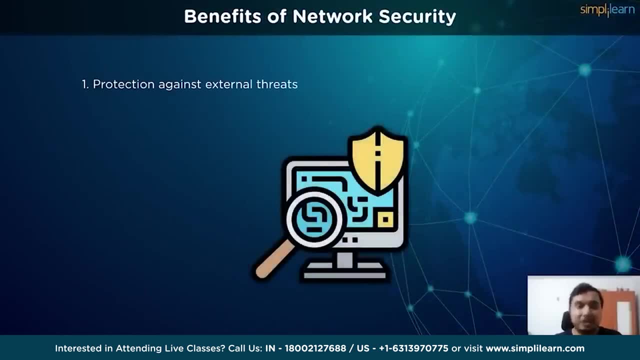 tools, its different types, etc. Let's go through the benefits of network security as a whole. The first, which is protection against external threats. The objective for cyber assaults can be as varied as the offenders themselves, Although they are typically initiated for financial gain, whether they are industrial. 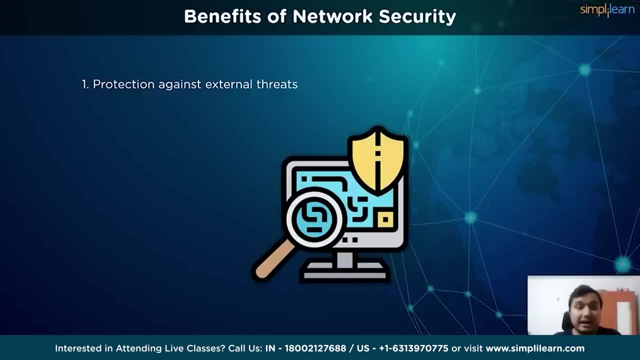 spies, hacktivists or cyber criminals- these bad actors all have one thing in common, which is how quick, clever and covert their attacks are. getting A strong cybersecurity posture that can save a lot of time and money can also be used to. 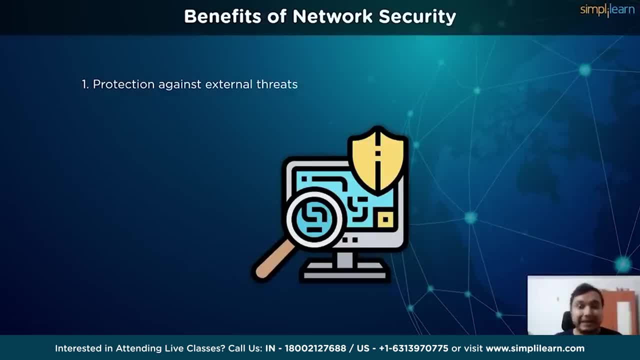 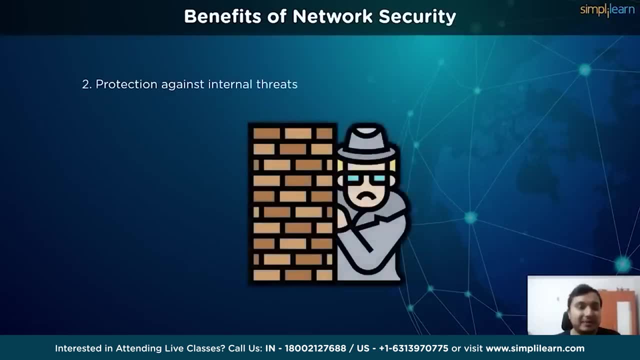 protect the environment. However, some of the risks involved in these attacks can be considered, as routine software updates may assist firms in identifying and responding to the abused techniques, tools and the common entry points. The next benefit is protection against internal threats. The human aspect continues to be the cybersecurity system's weakest link. 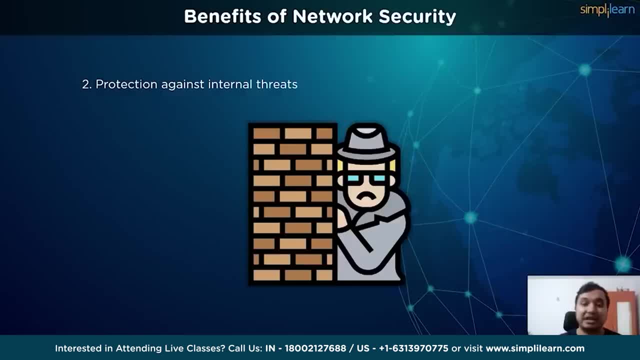 Insider risks can originate from current or former workers, third party vendors or even trusted partners, and they can be unintentional, careless or downright evil of remote work and the personal devices used for business purposes, while even IOT devices in remote locations can make it easier for these kind of threats to 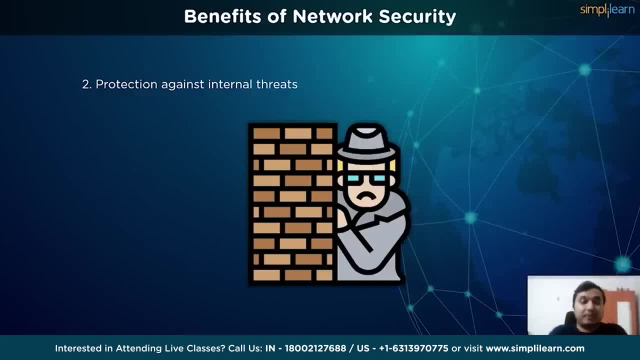 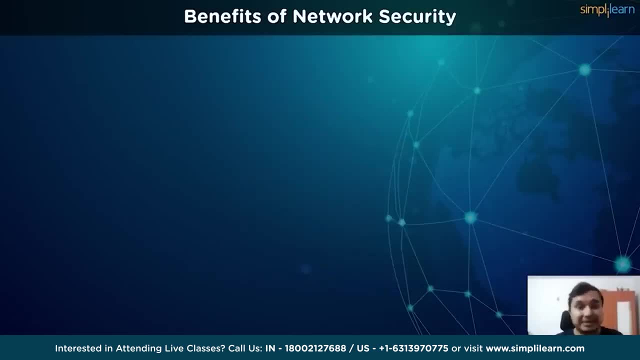 go undetected until it's too late. However, by proactively monitoring networks and managing access, these dangers may be identified and dealt with before they become expensive disasters. The third benefit is increased productivity. It is nearly impossible for employees to function when networks and personal 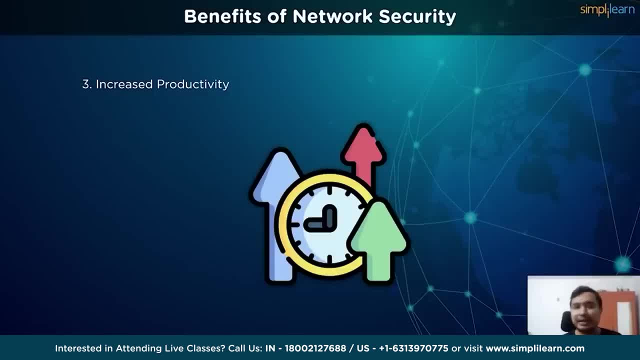 devices are slowed to a crawl by viruses and other cyber attacks during the operation of website and for the company to run. You may significantly minimize violations and the amount of downtime required to fix the breach by implementing various cybersecurity measures, such as enhanced firewalls, virus. 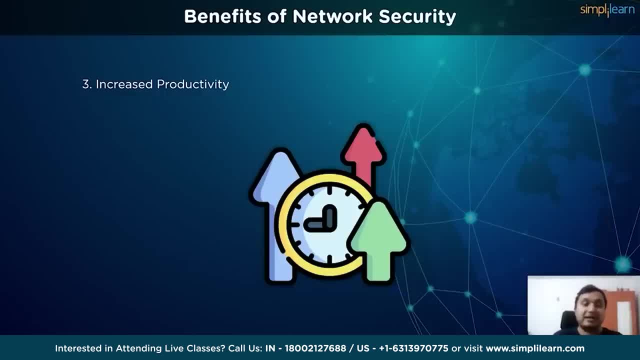 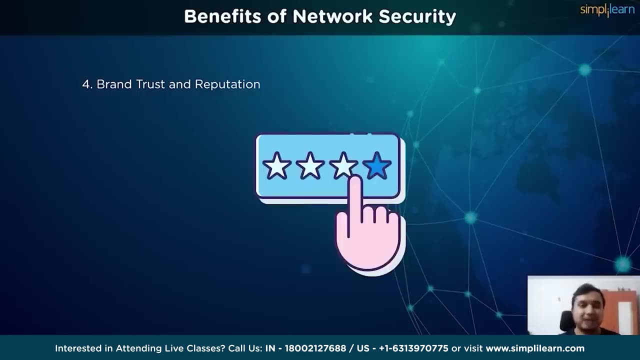 scanning and automatic backups. Employee identification of possible email phishing schemes, suspicious links and other malicious criminal activities can also be aided by education and training. Another benefit is increased productivity. This can be achieved by increasing the number of accounts that are used by the company's legal team. 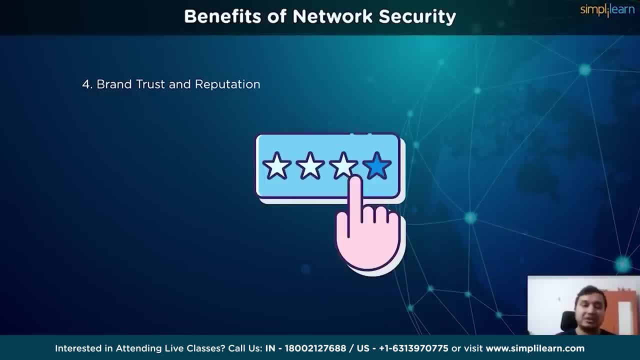 Another benefit is brand trust and reputation. Customer retention is one of the most crucial elements in business development. Customers today place a premium on maintaining brand loyalty through a strong cybersecurity stance, since this is the fastest way to get other businesses back, get referrals and sell more tickets overall. Additionally, it helps manufacturers get on the vendor list with bigger companies as a part of the supply chain which is only as strong as the Tweekest link. This opens possibilities for potential. 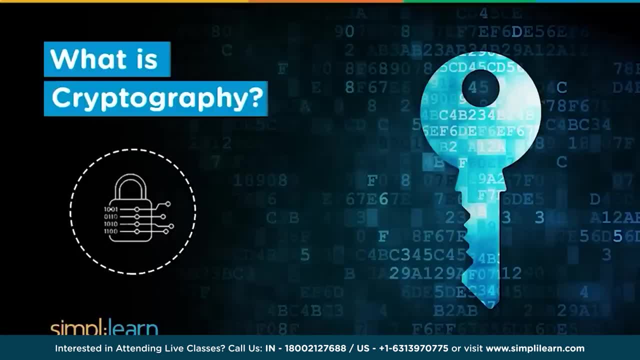 future endeavors and development. With the rise in censorship and general fear over privacy loss, consumer security is at an all-time high risk. Technology has made our life so much easier. while putting up a decent target on our personal information, It is necessary to understand how to simultaneously safeguard our data and be up to date with 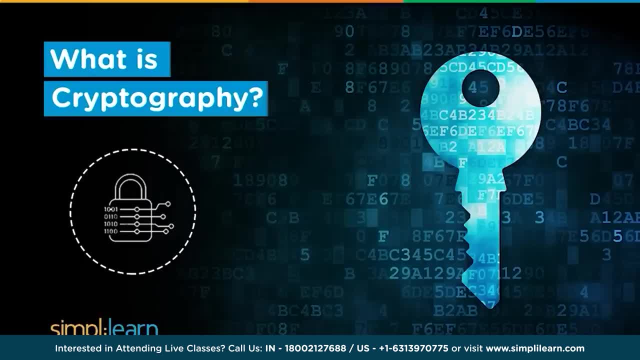 the latest technological developments. Maintaining this balance has become easier with cryptography taking its place in today's digital world. So, hey everyone, this is Bhavab from Simply Learn, and welcome to this video on cryptography. But before we begin, if you love watching tech videos, subscribe to our channel and 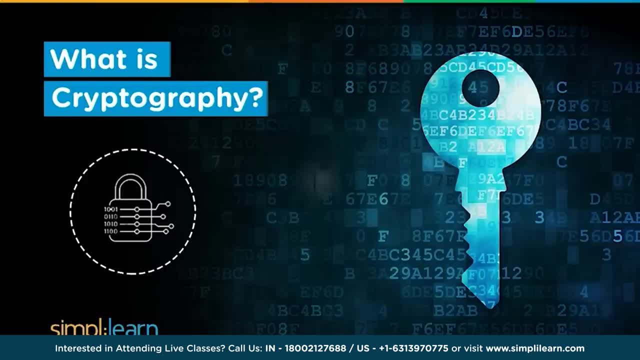 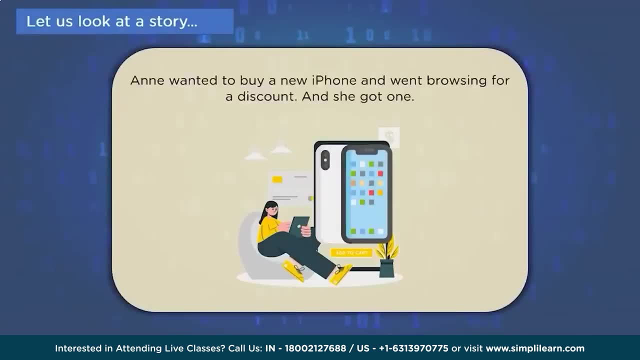 hit the bell icon to never miss an update from Simply Learn. So here's a story to help you understand cryptography. Meet Anne. Anne wanted to look for a decent discount on the latest iPhone. She started searching on the internet and found a rather shady website that offered. 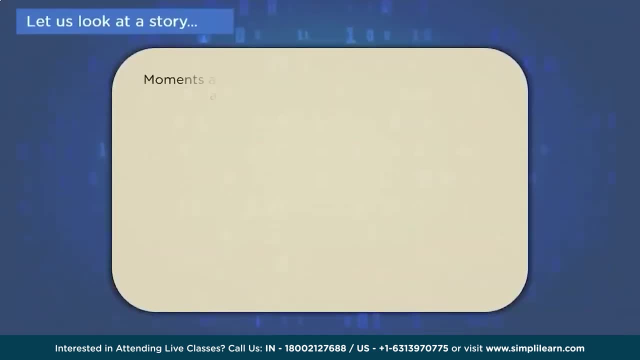 a 50% discount on the first purchase. Once Anne submitted her payment details, a huge chunk of money was withdrawn from her bank account. just moments after, Devastated, Anne quickly realized she had failed to notice that the website was a HTTP web page instead of an HTTPS one. 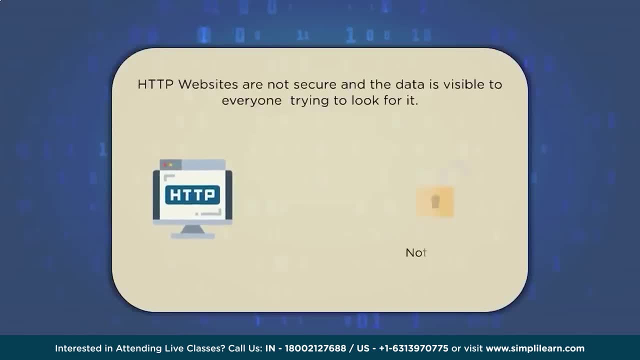 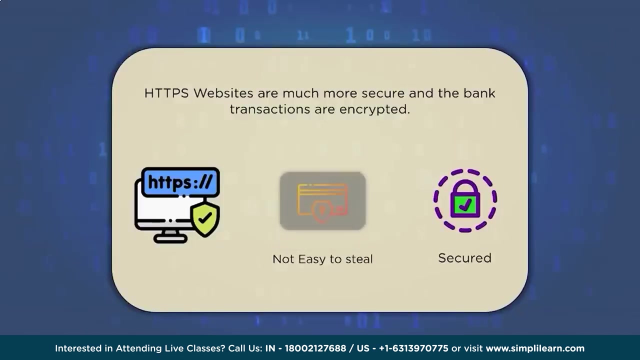 The payment information submitted was not encrypted and it was visible to anyone keeping an eye, including the website owner and hackers. Had she used a reputed website which has encrypted transactions and employs cryptography, her enthusiast could have avoided this particular incident. This is why it's never recommended to visit unknown websites or share any personal information. 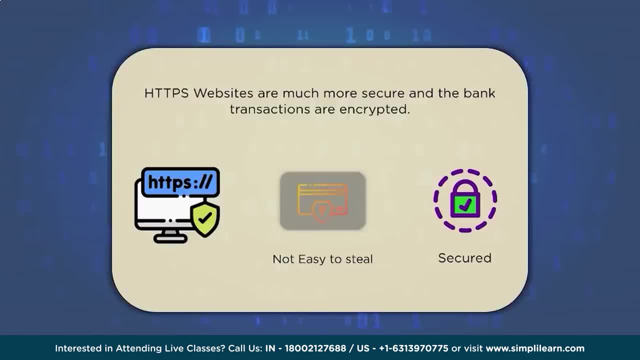 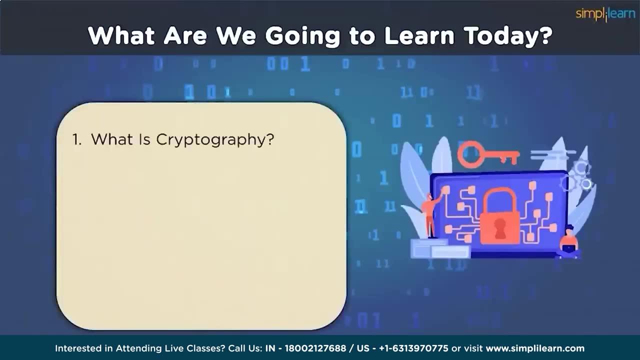 on them. Now that we understand why cryptography is so important, let's take a look at the topics to be covered today. We take a look into what cryptography is and how it works. We learn where cryptography is being used in our daily lives and how we are benefiting. 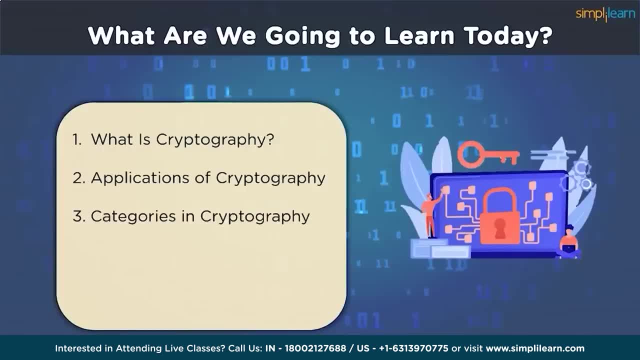 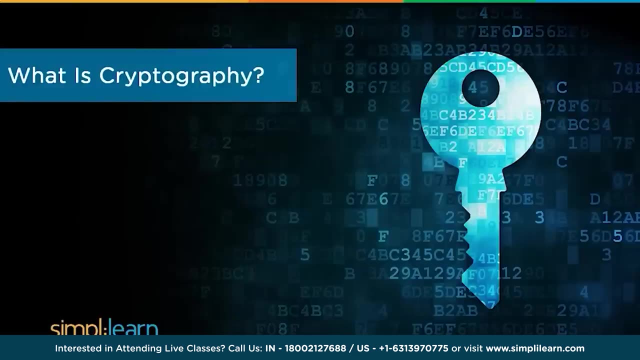 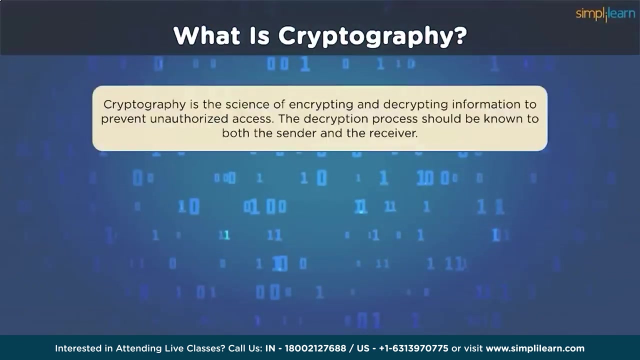 from it. Then we will understand the different types of cryptography and their history. Let's get started. 1. Cryptography is the science of encrypting or decrypting information to prevent unauthorized access. We transform our data and personal information so that only the correct recipient can understand. 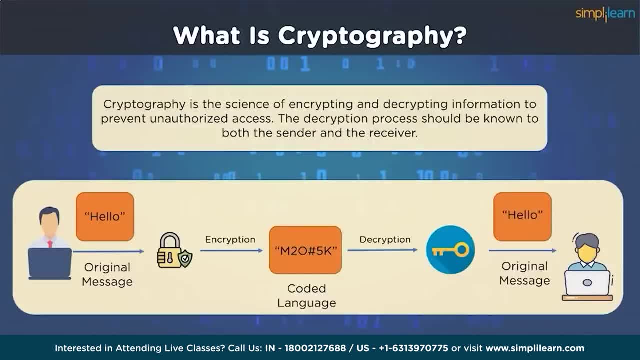 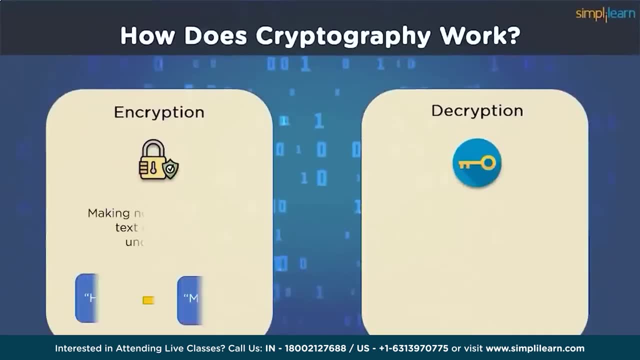 the message As an essential aspect of modern data security. Using cryptography allows the secure storage and transmission of data between willing parties. Encryption is the primary route for employing cryptography, by adding certain algorithms to jumble up the data. Decryption is the process of reversing the work done by encrypting information so that 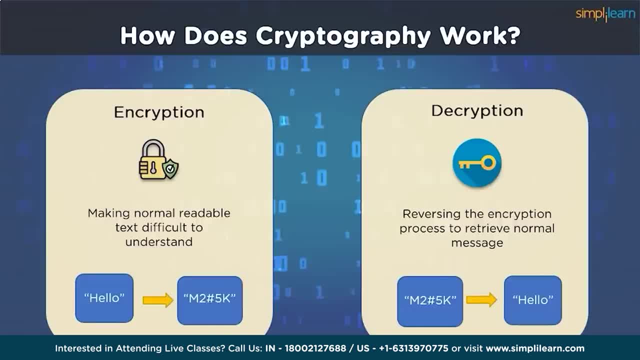 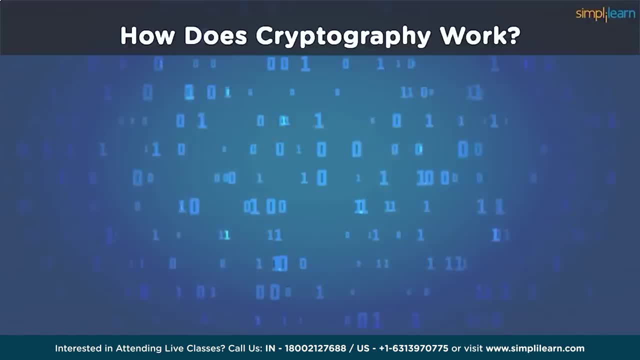 the data becomes readable again. Both of these methods form the basis of cryptography. For example, when Simply Learn is jumbled up or changed in any format, Not many people can guess the original word by looking at the encrypted text. The only ones who can are the people who know how to decrypt the coded word, thereby reversing. 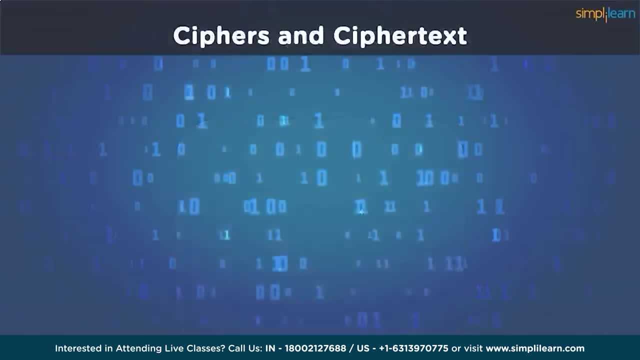 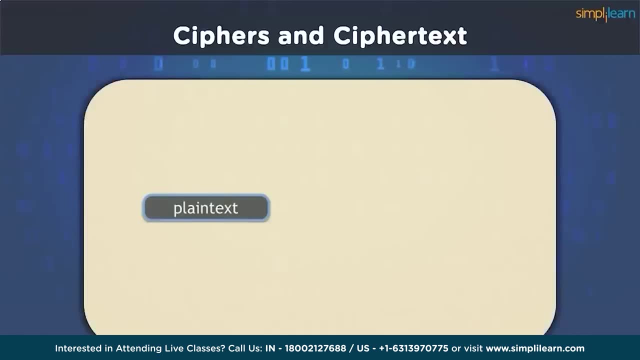 the process of encryption. Any data pre-encryption is called plain text or clear text. To encrypt the message, we use certain algorithms that serve a single purpose of scrambling the data to make them unreadable without the necessary tools. These algorithms are called ciphers. 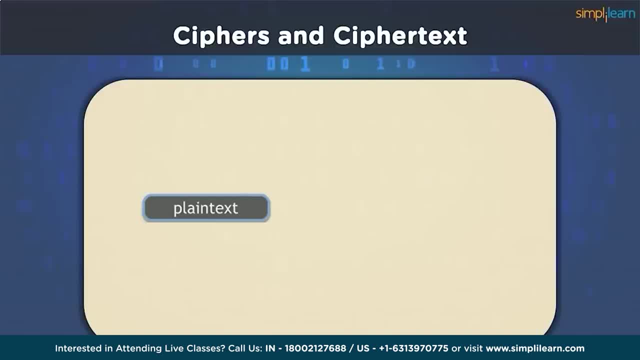 They are a set of detailed steps to be carried out, one after the other, to make sure the data becomes as unreadable as possible until it reaches the receiver. We take the plain text, pass it to the cipher algorithm and get the encrypted data. This encrypted text is called the ciphertext and this is the message that is transferred. 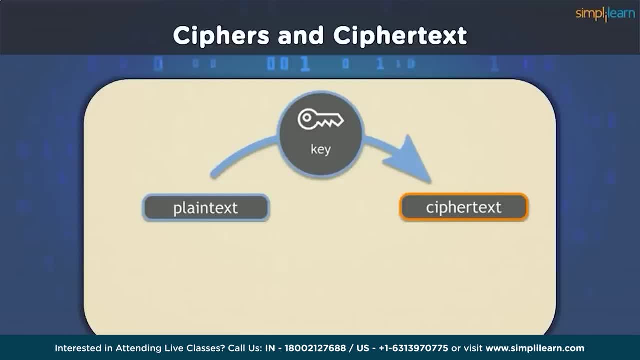 between the two parties. The key that is being used to scramble the data is known as the encryption key. These steps, ie the cipher and the encryption key, are made known to the receiver, who can then reverse the encryption on receiving the message. 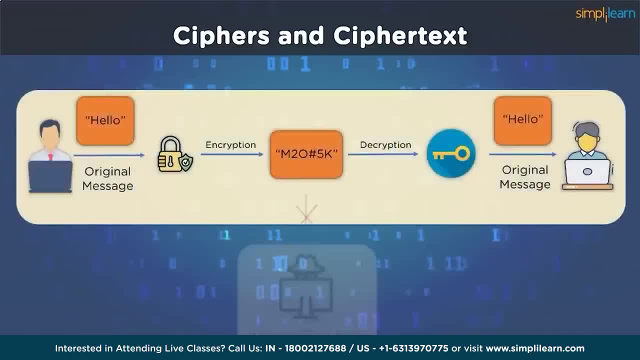 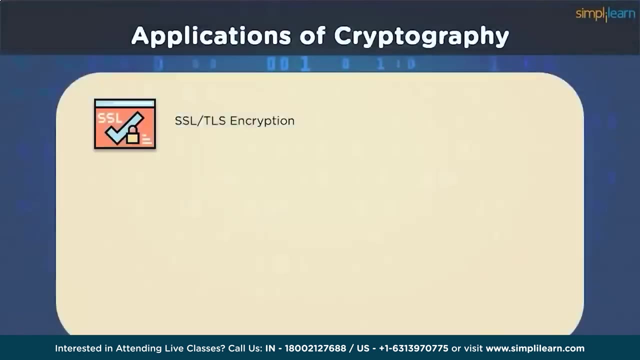 Unless any third party manages to find out both the algorithm and the secret key that is being used, they cannot decrypt the messages, since both of them are necessary to unlock the hidden content. Wonder what else we would lose if not for cryptography? Any website where you have an account can read your passwords. 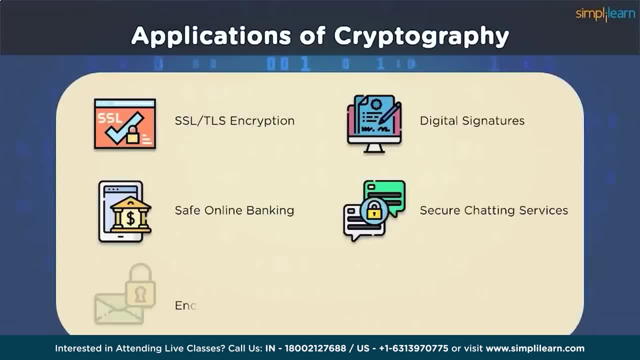 Important emails can be intercepted And their contents can be read without encryption during the transit. More than 65 billion messages are sent on WhatsApp every day, all of which are secured thanks to end-to-end encryption. There is a huge market opening up for cryptocurrency, which is possible due to blockchain technology. 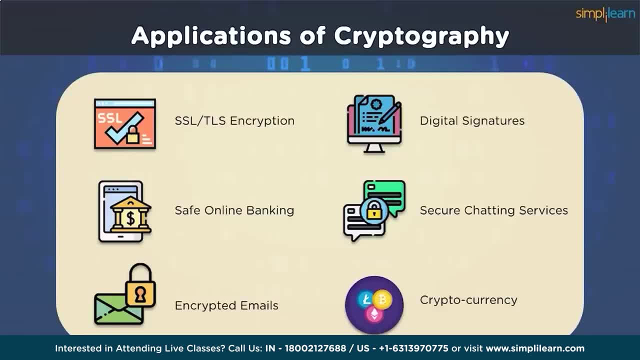 that uses encryption algorithms and hashing functions to ensure that the data is secure. If this is of particular interest to you, you can watch our video on blockchain, the link of which will be in the description. Of course, there is no single solution to a problem as diverse as explained. 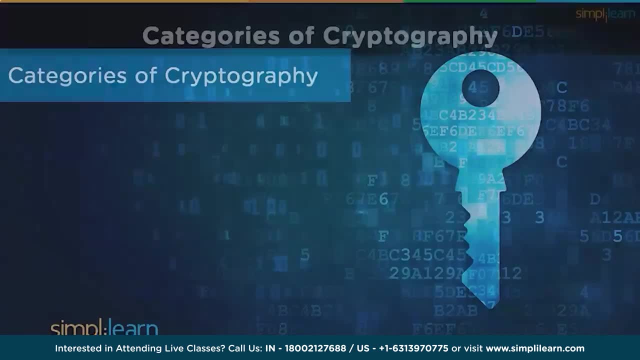 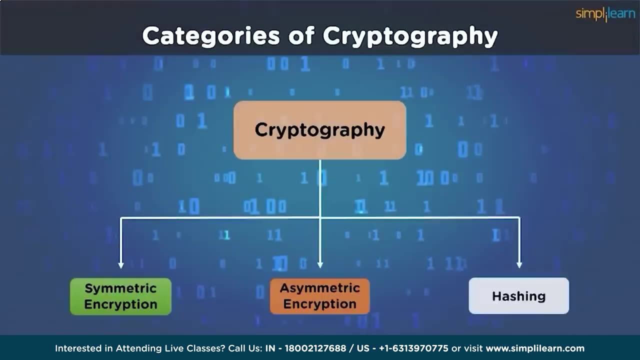 There are three variants of how cryptography works and is in practice. They are symmetric encryption, asymmetric encryption and hashing. Let's find out how much we have understood until now. Do you remember the difference between a cipher and ciphertext? Leave your answers in the comments. 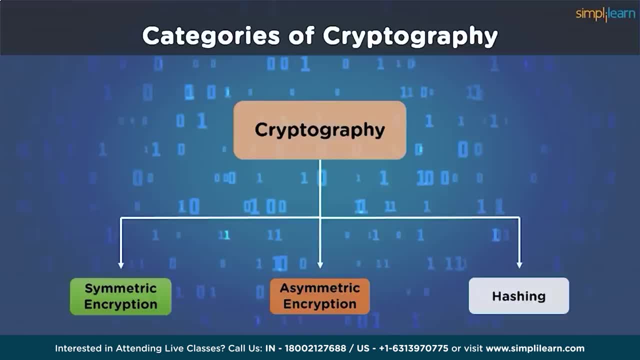 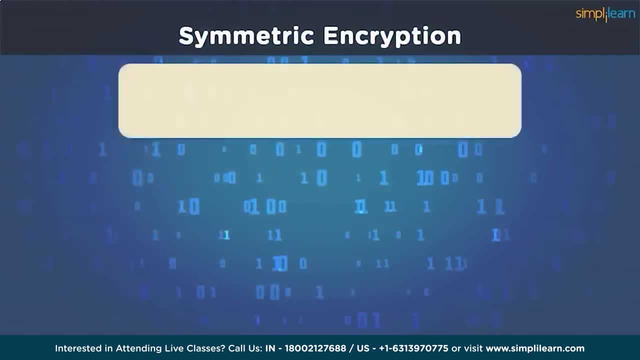 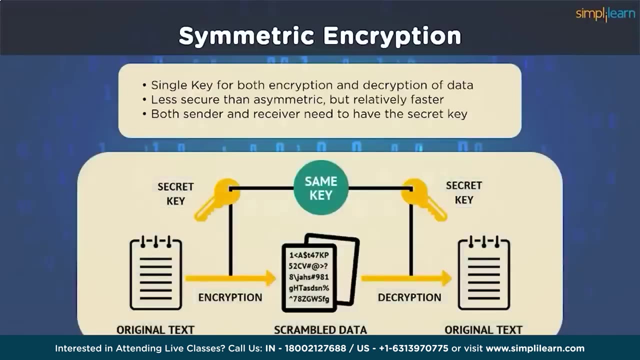 And before we proceed, if you find this video interesting, make sure to give it a thumbs up before moving ahead. Let's look at symmetric encryption first. Symmetric encryption uses a single key for both the encryption and decryption of data. It is comparatively less secure than asymmetric encryption, but much faster. 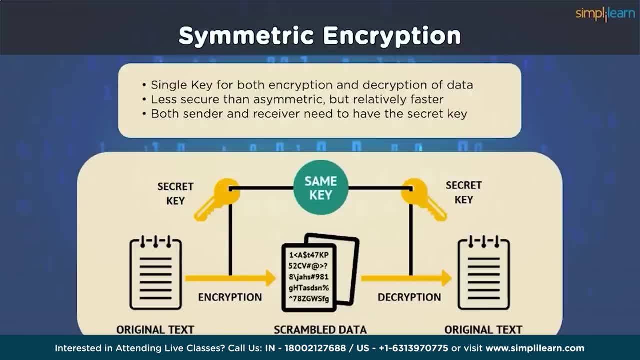 It is a compromise that has to be embraced in order to deliver data as fast as possible without leaving information completely vulnerable. This type of encryption is used when data rests on servers and identifies personnel for payment applications. The potential drawback with symmetric encryption is that both the sender and receiver need 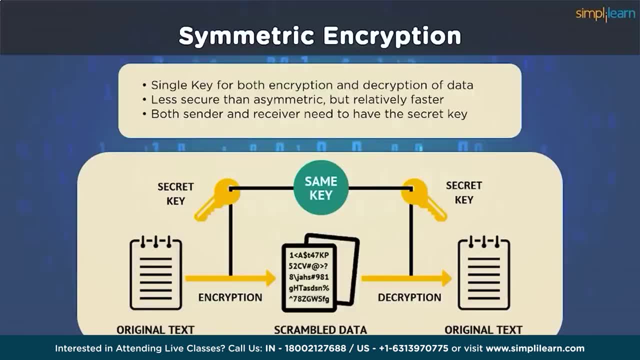 to have the same secret key, and it should be kept hidden at all times. Caesar cipher and enigma machine are both symmetric encryption examples that we will look into further. For example, if Alice wants to send a message to Bob, she can apply a substitution cipher. 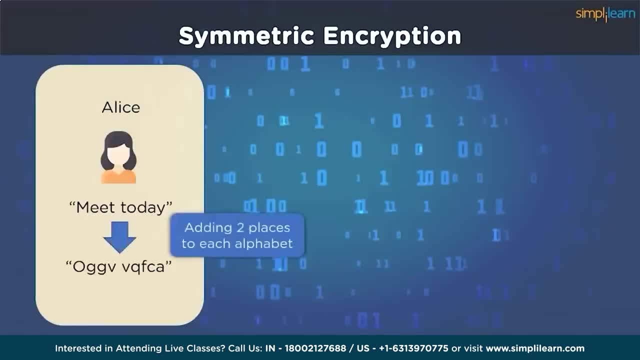 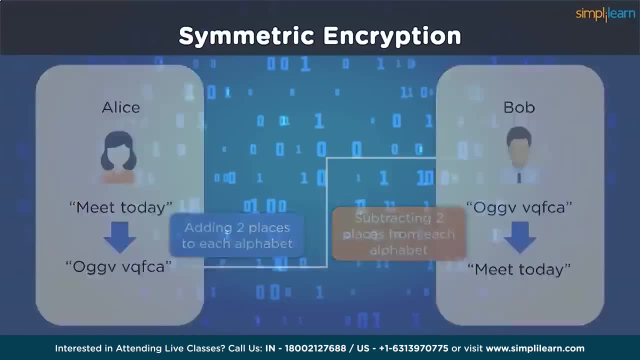 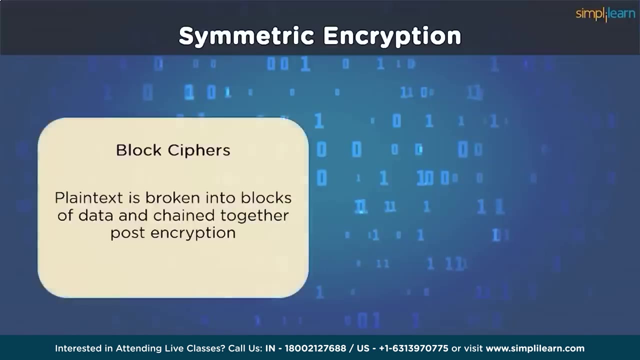 or a shift cipher to encrypt the message, But Bob must be aware of the same key itself So he can decrypt it. He can decrypt it when he finds it necessary to read the entire message. Symmetric encryption uses one of the two types of ciphers: stream ciphers and block ciphers. 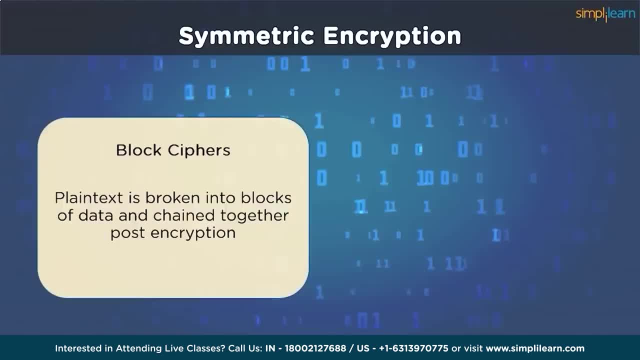 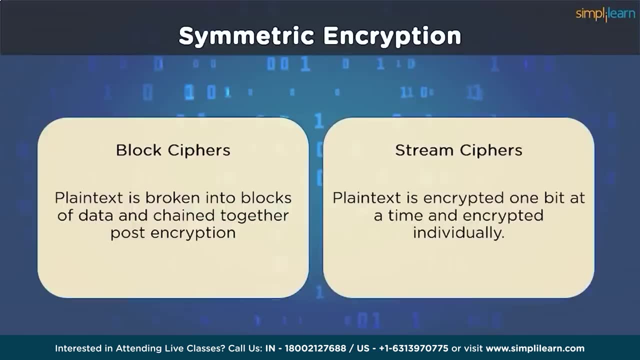 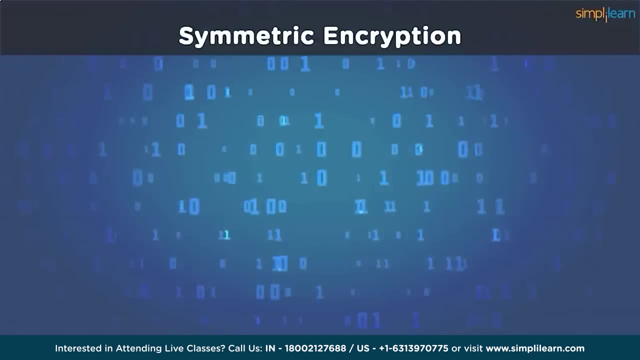 Block ciphers break the plaintext into blocks of fixed size and use the key to convert it into ciphertext. Stream ciphers convert the plaintext into ciphertext one bit at a time, instead of resorting to breaking them up into bigger chunks. In today's world, the most widely used symmetric encryption algorithm is enigma. 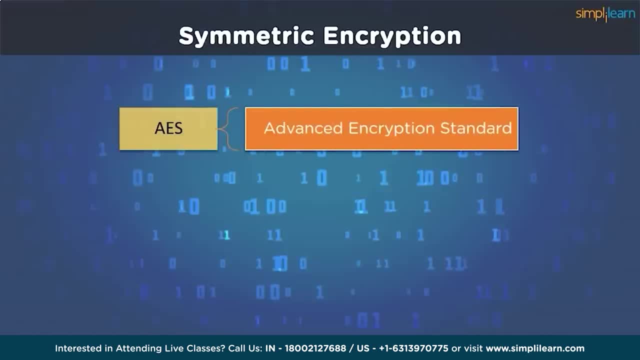 AES-256 stands for Advanced Encryption Standard, which has a key size of 256-bit, with 128-bit and 196-bit key sizes also being available. Other primitive algorithms like the Data Encryption Standard, the Triple Data Encryption Standard and Blowfish have all fallen out of favor due to the rise of AES. 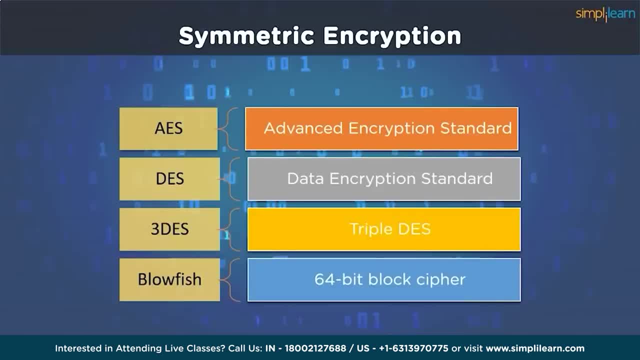 AES chops up the data into blocks and performs 10 plus rounds of obscuring and subtracting. AES-256 is the most popular encryption algorithm in the world. AES-256 is the most popular encryption algorithm in the world. AES-256 is the most popular encryption algorithm in the world. 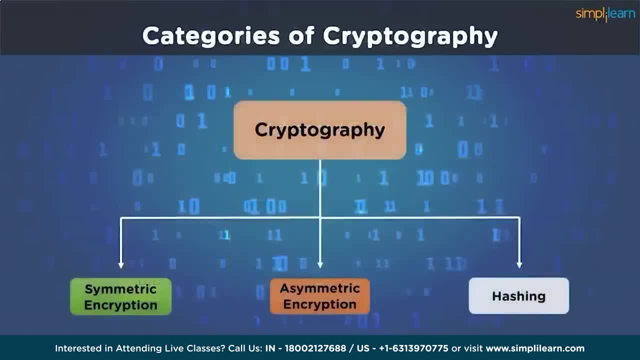 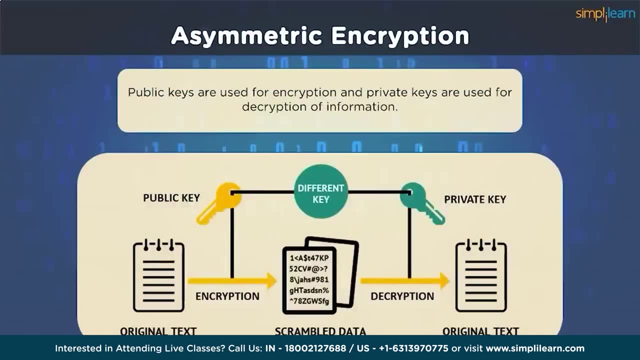 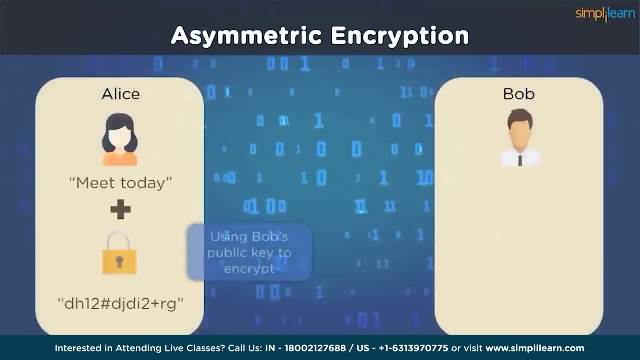 AES-256 is the most typical encryption algorithm in the world. AES will test a string of Kurdish Vegas languages for biblical entendents, Etc K. Korean English plays the Bob uses his own private key to decrypt the data. This way, nobody can intercept the message in between transmissions and there is no need. 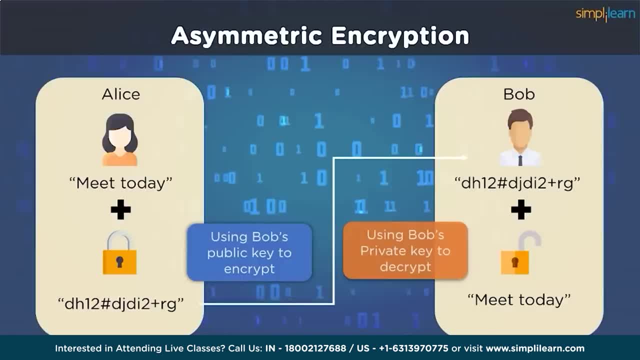 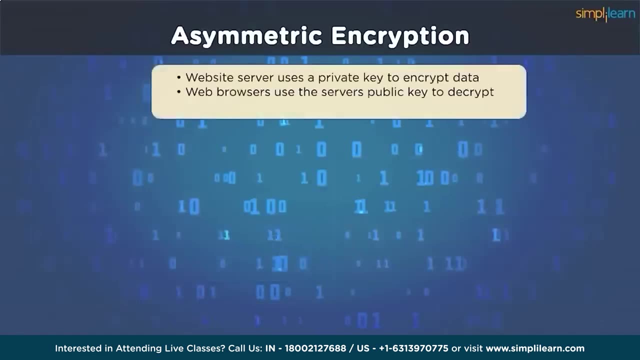 for any secure key exchange for this to work, since the encryption is done with the public key and the decryption is done with the private key that no one except Bob has access to, Both the keys are necessary to read the full message. There is also a reverse scenario, where we can use the private key for encryption and 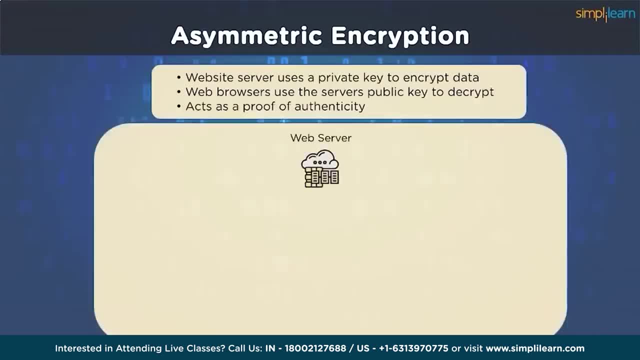 the public key for decryption. A server can sign non-confidential information using its private key, and anyone who has its public key can decrypt the message. This mechanism also proves that the sender is authenticated and there is no problem with the origin of the information. 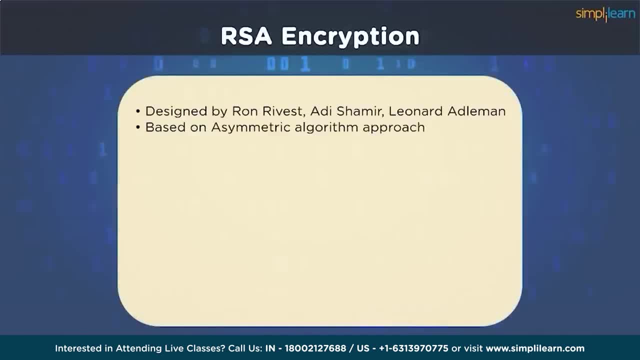 RSA encryption is the most widely used asymmetric encryption standard. It is named after its founders, Rivest, Shamir and Edelman, and it uses block ciphers that separate the data into blocks and obsequies Secure the information, Widely considered the most secure form of encryption, albeit relatively slower than. 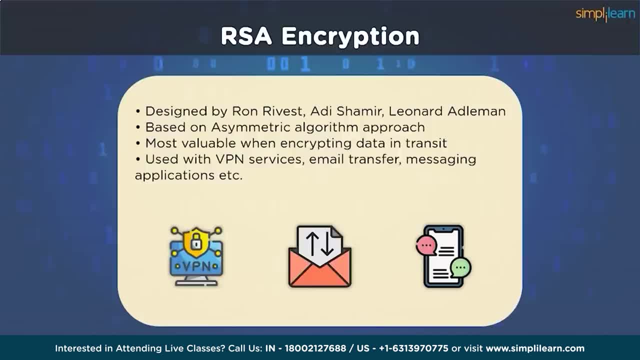 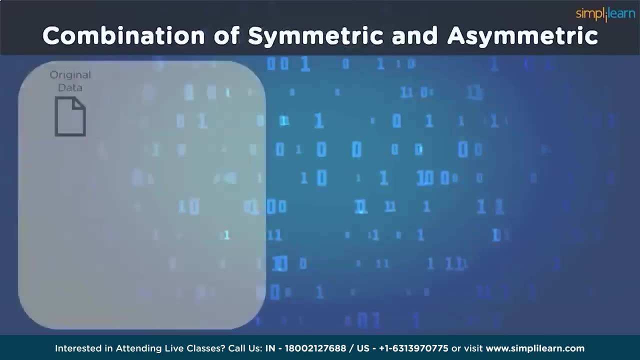 AES. it is widely used in web browsing, secure identification, VPNs, emails and chat applications. With so much hanging on the keys secrecy, there must be a way to transmit the keys without others reading our private data. Many systems use a combination of symmetric encryption and asymmetric encryption to bolster 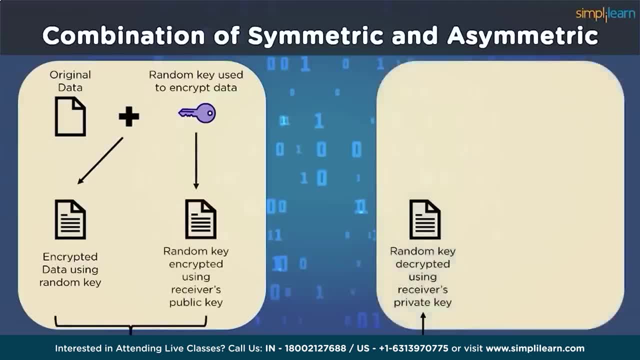 security and match speed. at the same time, Since asymmetric encryption takes longer to decrypt large amounts of data, the full information is encrypted using a single key, ie symmetric encryption. That single key is then transmitted to the receiver using asymmetric encryption, so you 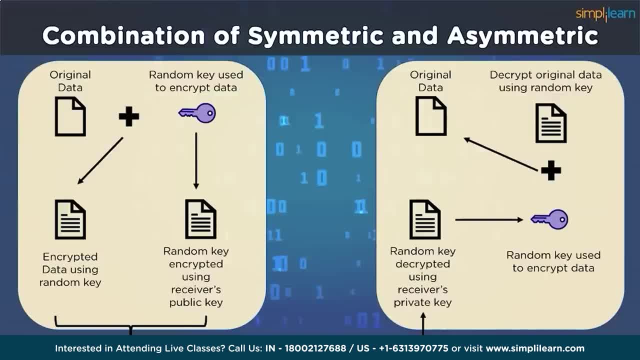 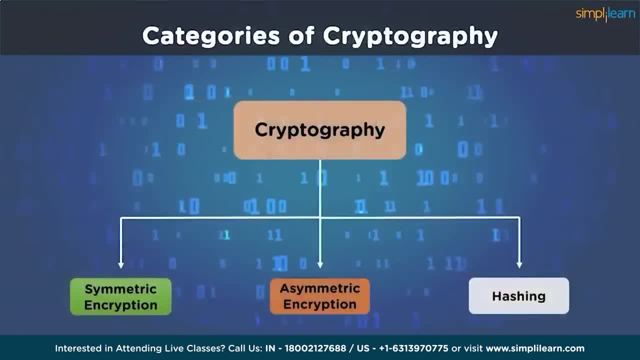 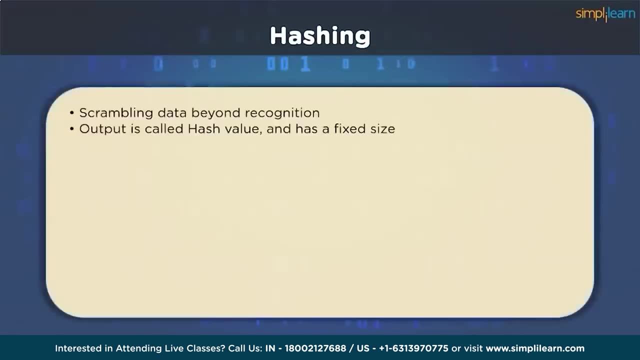 don't have to compromise either way. Another route is using the Diffie-Hellman key exchange, which relies on a one-way function and is much tougher to break into. The third variant of cryptography is termed as hashing. Hashing is the process of scrambling a piece of data beyond recognition. 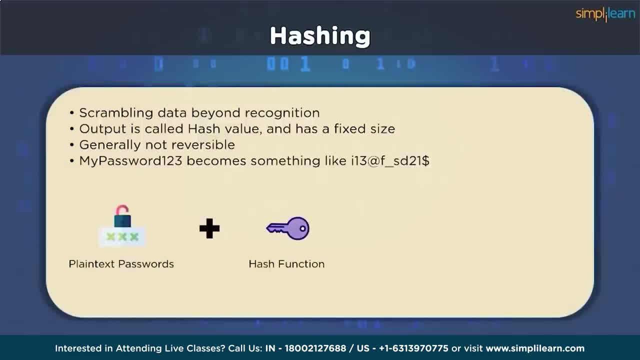 It gives an output of fixed size, which is known as the hash value of the original data or just hash in general. The calculations that do the job of messing up the data collection form the hash function. They are generally not reversible without resilient brute-force mechanisms and are very 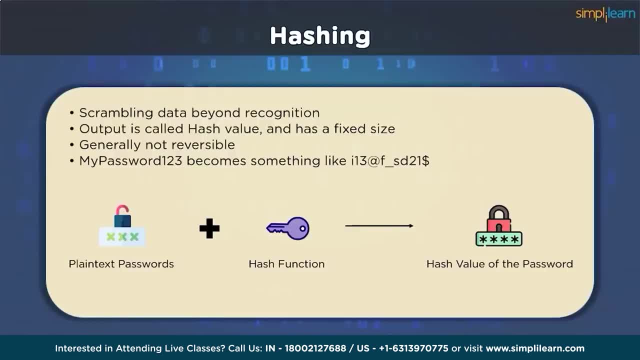 helpful when storing data on website servers that need not be stored in plain text. For example, many websites store your account partially. For example, you can store your password in a hashed format so that not even the administrator can read your credentials. When a user tries to log in, they can compare the entered password's hash value with the. 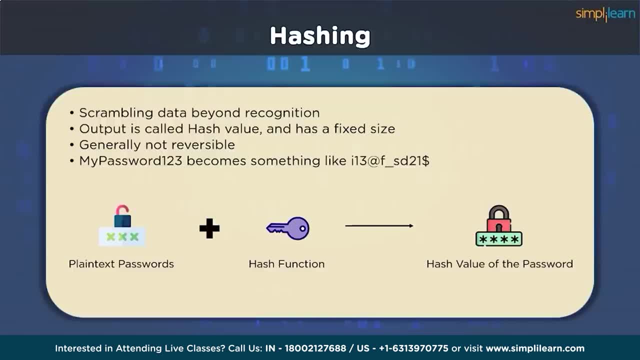 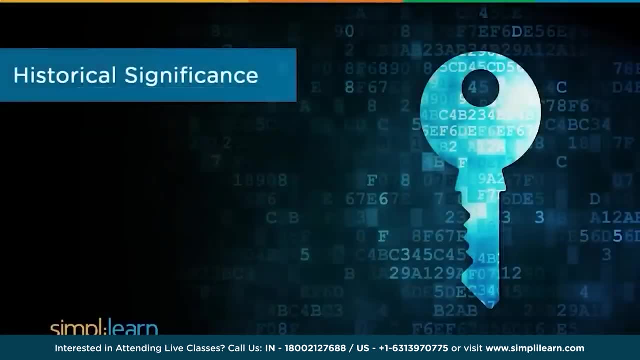 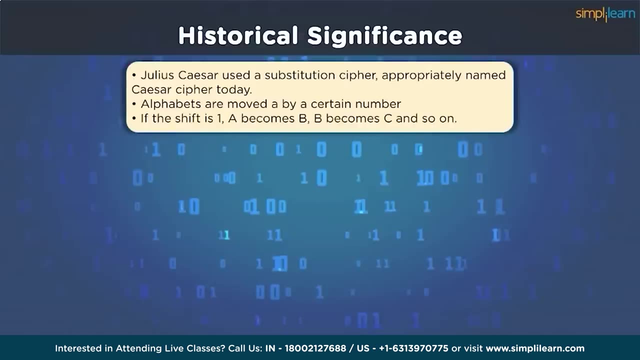 hash value that is already stored on the servers for authentication. since the function will always return the same value for the same input, Cryptography has been in practice for centuries. Julius Caesar used a substitution shift to move alphabets a certain number of spaces beyond their place in the alphabet table. 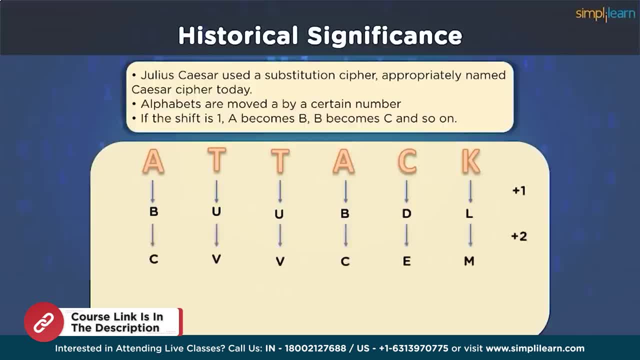 A spy can't decipher the original message at first glance. For example, if he wanted to pass confidential information to his armies and decides to use the substitution shift of plus 2, A becomes C, B becomes D, and so on. The word attack, when passed through a substitution shift of plus 3, becomes DWWDEFN. 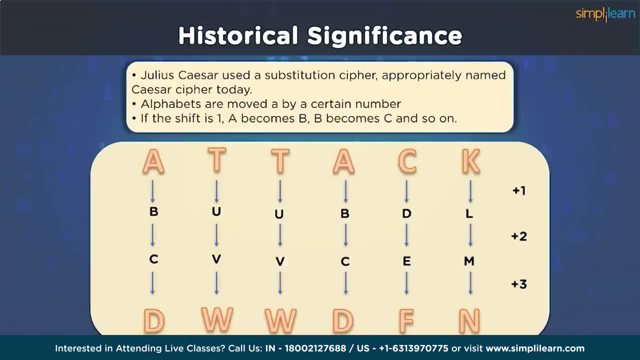 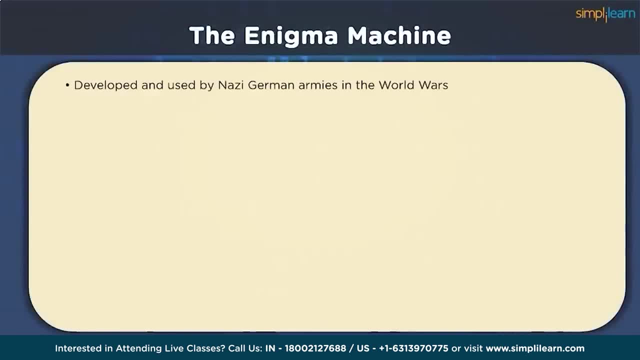 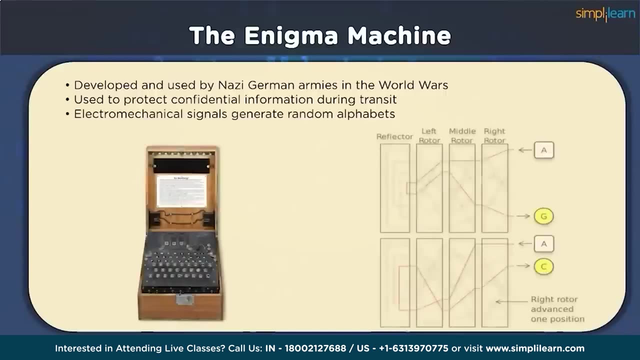 This cipher has been appropriately named the Caesar cipher, which is one of the most widely used algorithms. The Enigma is probably the most famous cryptographic cipher device used in ancient history. It was used by the Nazi German armies in the World Wars. They were used to protect confidential political, military and administrative information, and 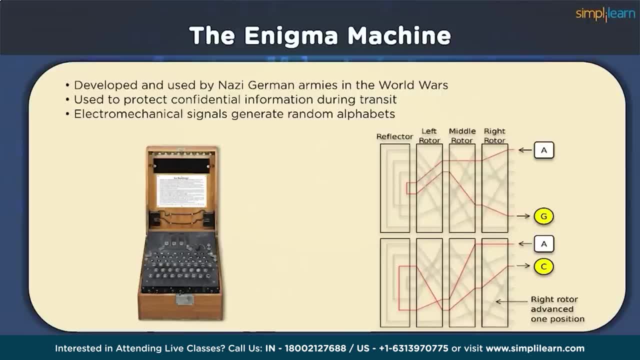 it consisted of three or more rotors that scrambled the original message, depending on the machine's state at that time. The decryption is similar, but it needs both machines to stay in the same state before passing the ciphertext So that we receive the same plain text message. 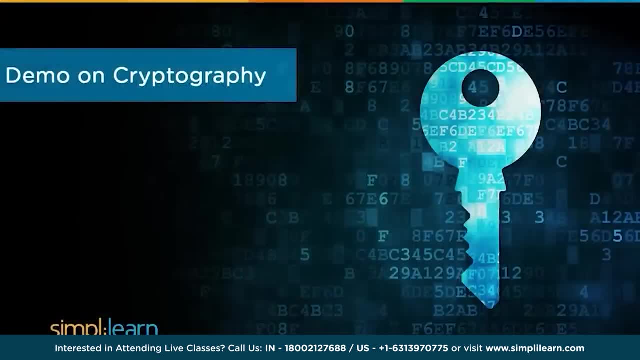 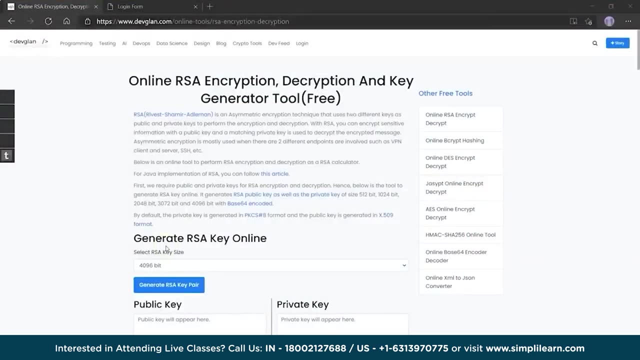 Let's take a look at how our data is protected while we browse the internet thanks to cryptography. Here we have a web-based tool that will help us understand the process of RSA encryption. We see the entire workflow, from selecting the key size to be used until the decryption. 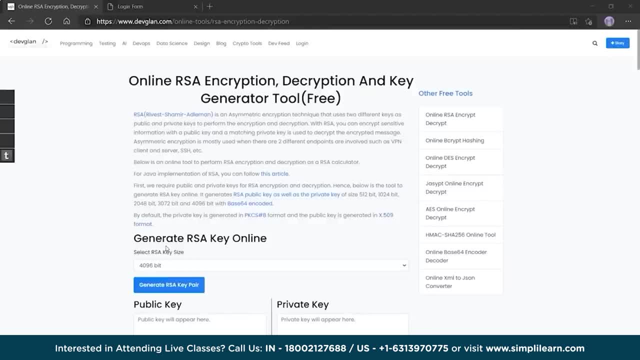 of the ciphertext in order to get the plain text back. As we already know, RSA encryption algorithm falls under the umbrella of asymmetric key cryptography. This basically implies that we have two keys at play here, a public key and a private key. Typically, the public key is used by the sender to encrypt the message, and the private key 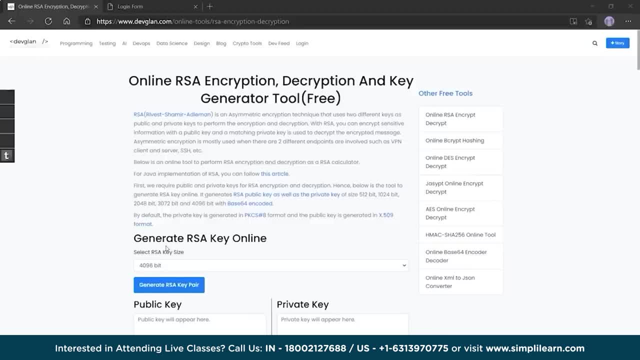 is used by the receiver to decrypt the message. There are some occasions when this allocation is reversed, and we will have a look at them as well. In RSA, we have the choice of key size. We can select any key from a 512-bit to 1024-bit, all the way up to a 4096-bit key. 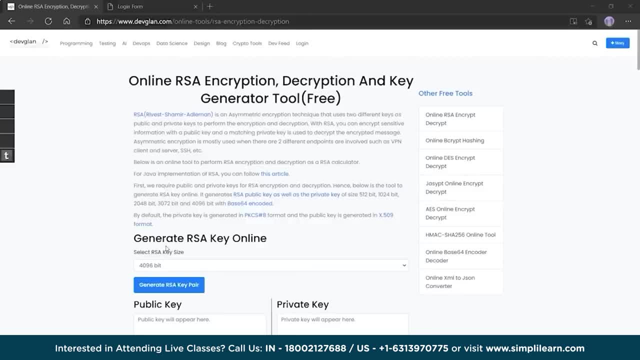 In RSA, we have the choice of key size. We can select any key from a 512-bit to 1024-bit, all the way up to a 4096-bit key. In RSA, we have the choice of key size. We can select any key from a 512-bit to 1024-bit key. 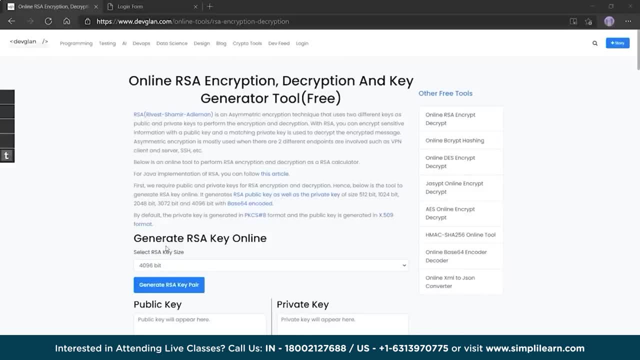 The longer the key length, the more complex the encryption process becomes and thereby strengthening the ciphertext. Although, with added security, more complex functions take longer to perform the same operations on similar size of data, We have to keep a balance between both speed and strength, because the strongest encryption 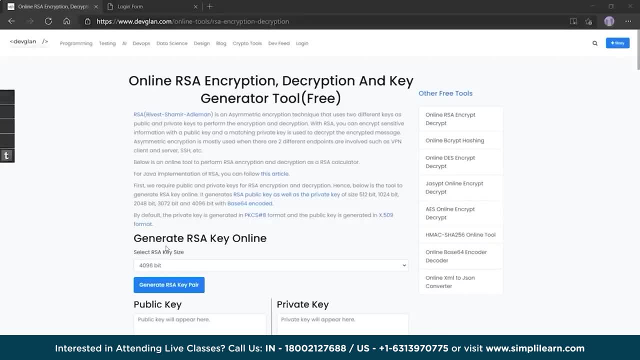 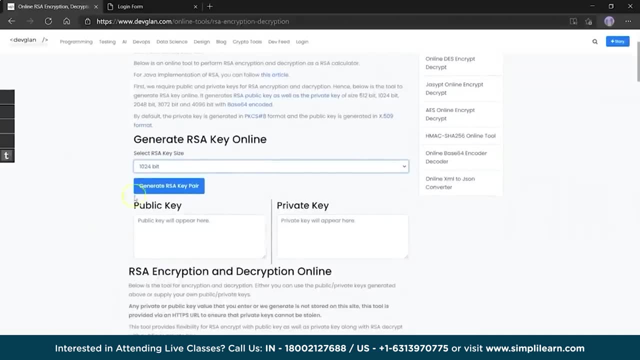 algorithms are of no use if they cannot be practically deployed in systems around the world. Let's take a 1024-bit key over here. Now we need to generate the keys. This generation is done by functions that operate on passphrases. The tool we are using right now generates the pseudorandom keys to be used in this explanation. 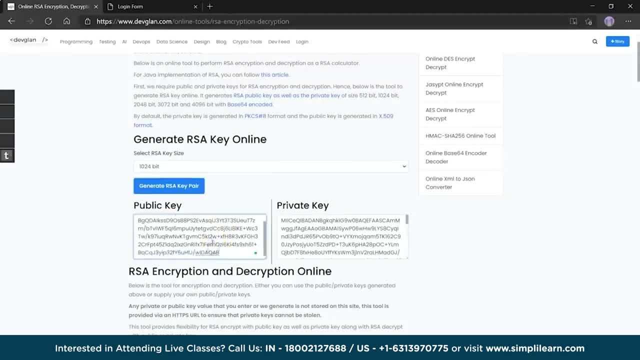 Once we generate the keys, you can see the public key is rather smaller than the private key, which is almost always the case. These two keys are mathematically linked with each other. They cannot be substituted with any other key and, in order to encrypt the original message, 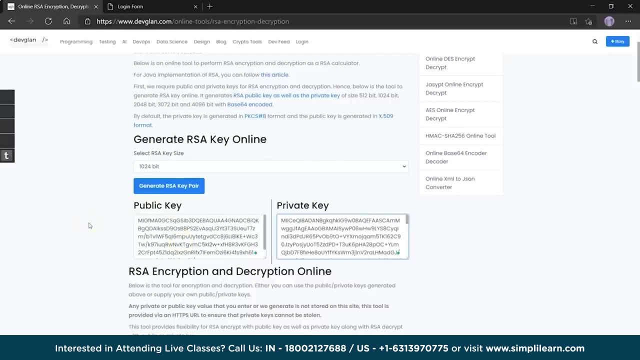 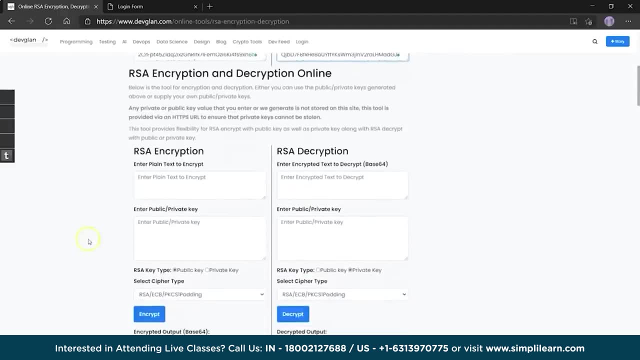 or decrypt the ciphertext. this pair must be kept together. The public key is then sent to the center. The receiver keeps the private key with himself. In this scenario, let's try and encrypt a word. simply learn. We have to select if the key being used for encryption is either private or public, since 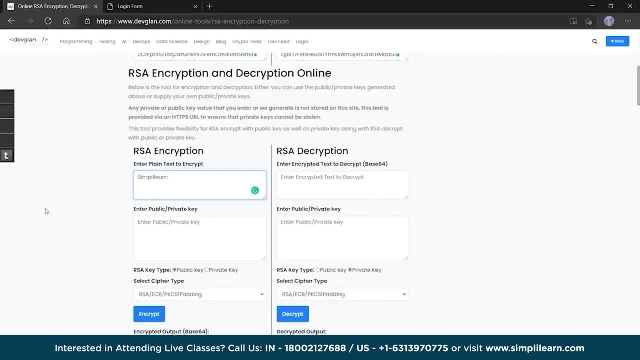 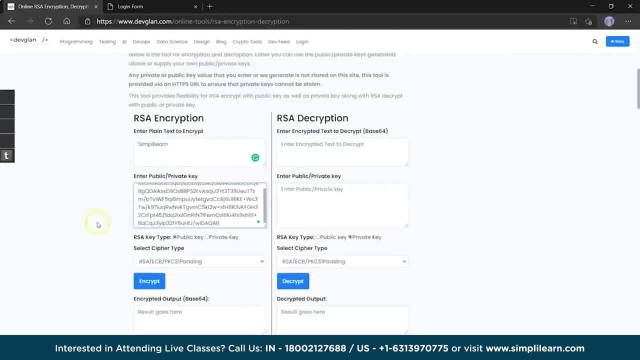 that affects the process of scrambling the information. Since we are using the public key over here, let's select the same and copy it and paste over here. The cipher we are using right now is plain-accessible. Let's copy it and paste over here. 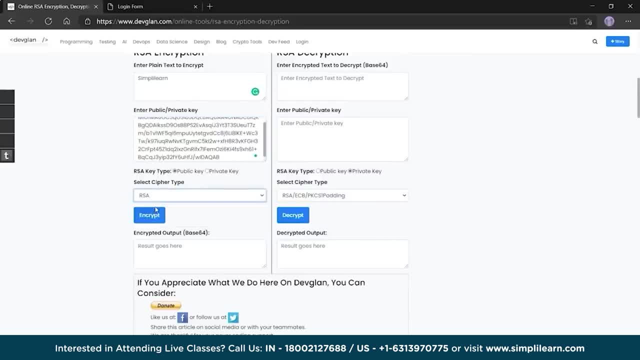 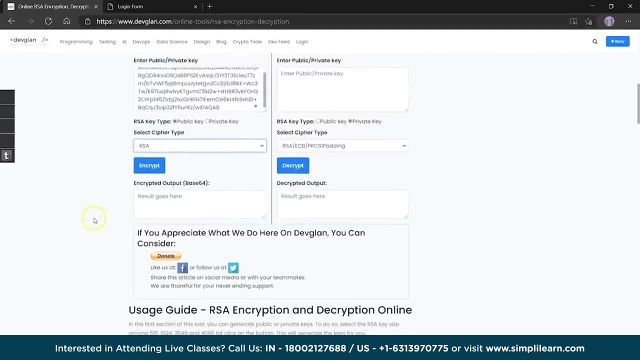 There are some modified ciphers, with their own pros and cons, that can also be used, provided we use it on a regular basis and depending on the use case as well. Once we click on encrypt, we can see the ciphertext being generated over here. The pseudorandom generating functions are created in such a way that a single character change. 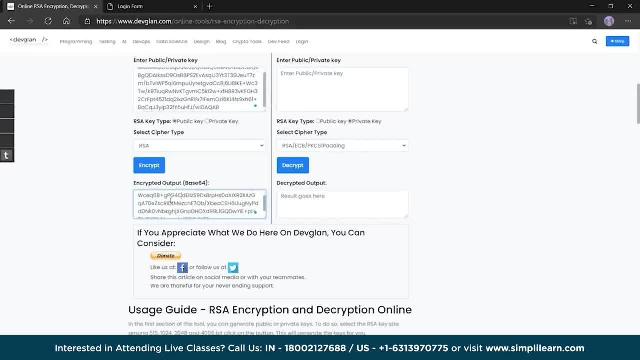 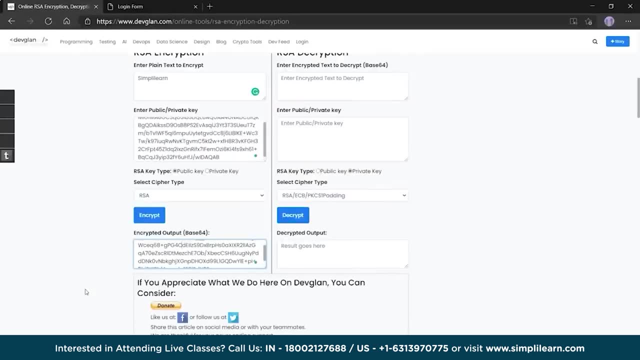 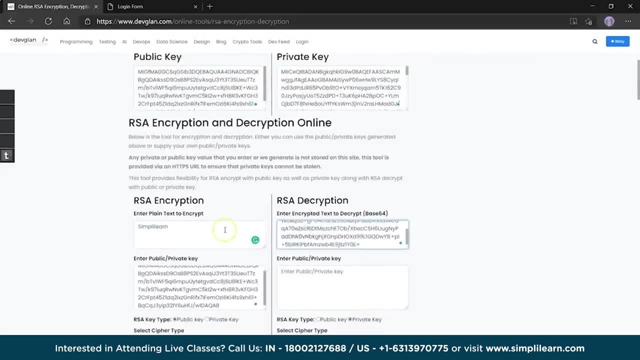 in the plaintext will trigger a completely different ciphertext. This is a security feature to strengthen the process from brute force methods. Now that we are done with the encryption process, let's take a look at the decryption part. The receiver gets this ciphertext from the sender with no other key or supplement. 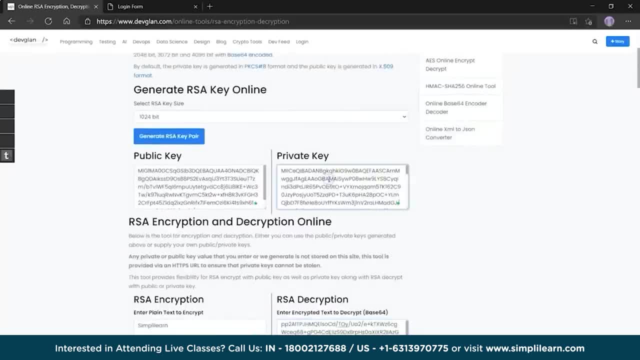 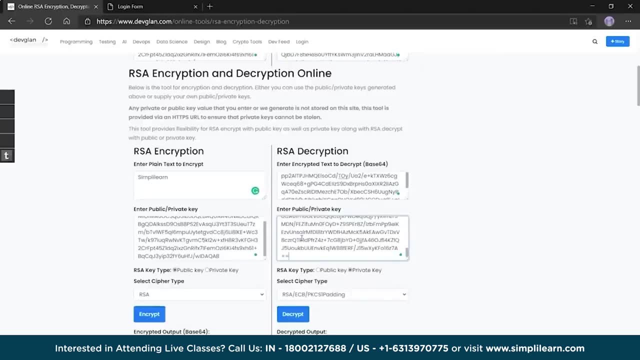 He or she must already possess the private key generated from the same pair. No other private key can be used to decrypt the message. since they are mathematically linked, We paste the private key here and select the same. The cipher must also always be the same used during the decryption. 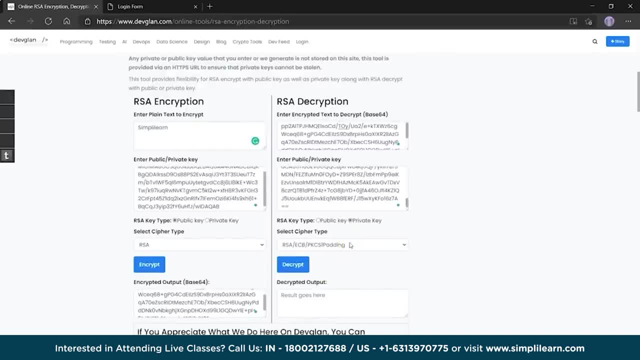 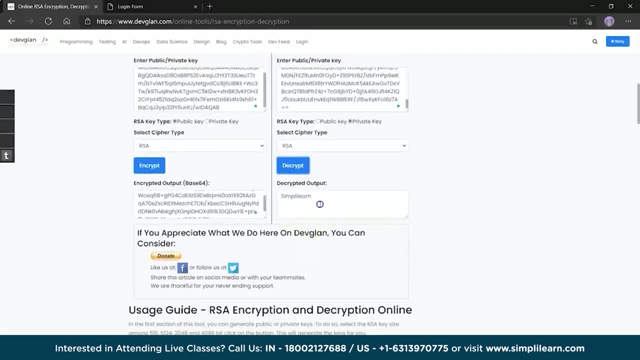 It is the same private key generated from the same pair. We paste the private key here and select the same. The cipher must always be the same used during the decryption, the encryption process. Once you click decrypt, you can see the original plain text we had decided to encrypt. 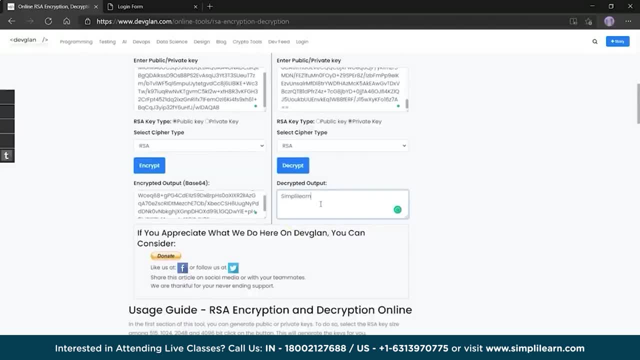 This sums up the entire process of RSA encryption and decryption. Now some people use it the other way around. We also have the option of using the private key to encrypt information and the public key to decrypt it. This is done mostly to validate the origin of the message. 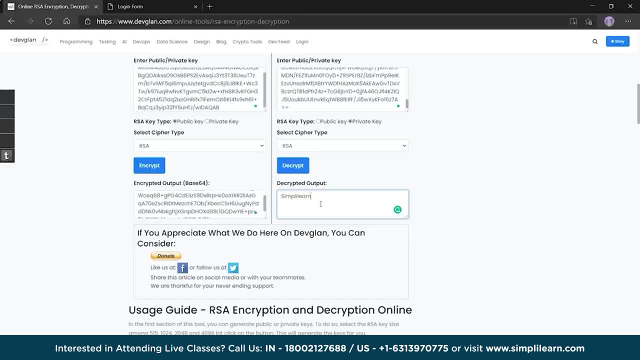 Since the keys only work in pairs, if a different private key is used to encrypt the message, the public key cannot decrypt it. Conversely, if the public key is able to decrypt the message, it must have been encrypted with the right private key and hence the rightful owner. 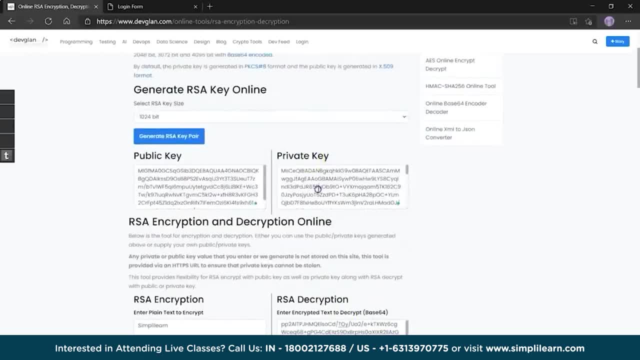 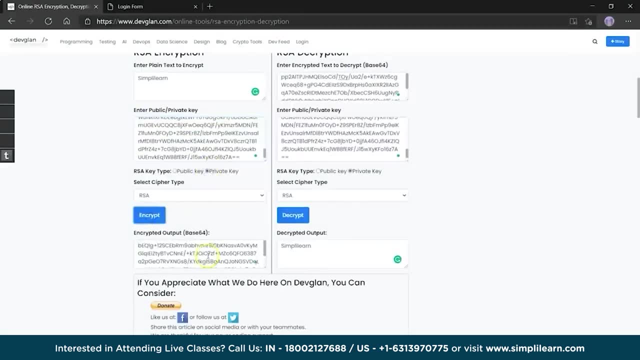 Here we just have to take the private key and use that to encrypt the plain text and select the same in this checkbox as well. You can see we have generated a completely new ciphertext. This ciphertext will be sent to the receiver, and this time we will use the public key for. 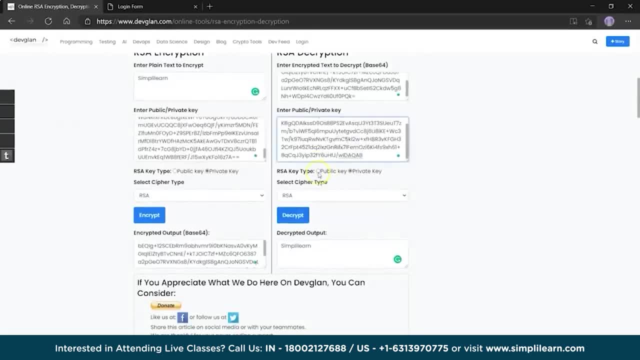 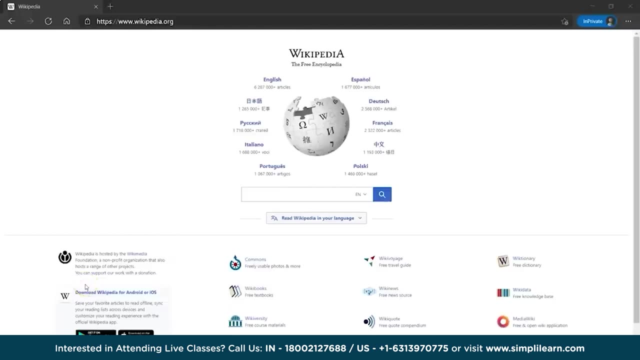 decryption. Let's select the correct checkbox And decrypt, and we still get the same output. Now let's take a look at practical example of encryption in the real world. We all use the internet on a daily basis and many are aware of the implications of using 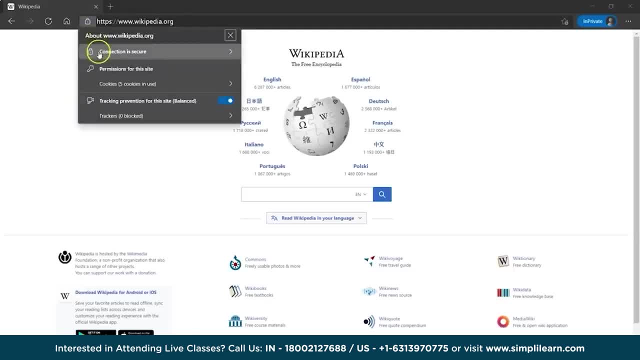 unsafe websites. Let's take a look at Wikipedia here. Pretty standard HTTPS website where the H stands for secured. Let's take a look at how it secures the data. Wireshark is the world's foremost and most widely used network protocol analyzer. 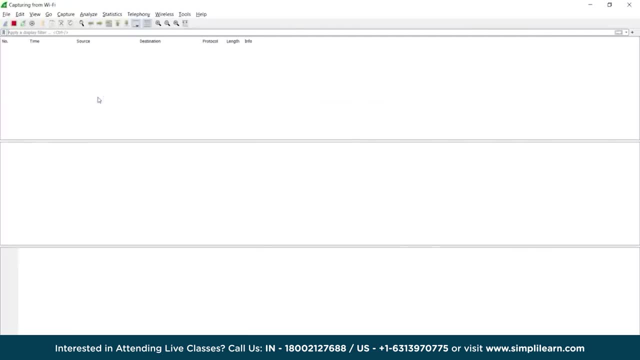 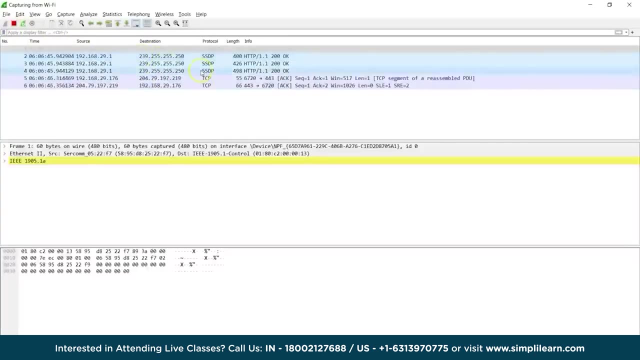 It lets you see what's happening on your network at a microscopic level, and we are going to use this software to see the traffic that is leaving our machine and to understand how vulnerable it is. Since there are many applications running in this machine, let's apply a filter that. 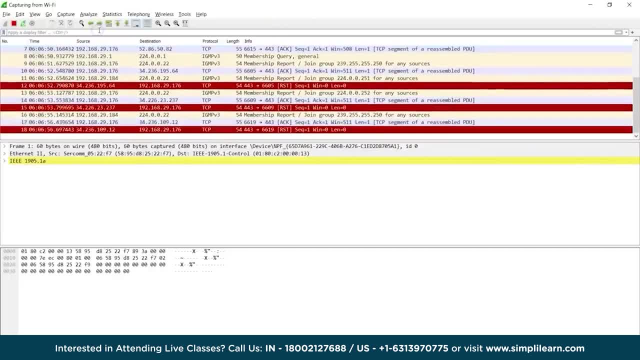 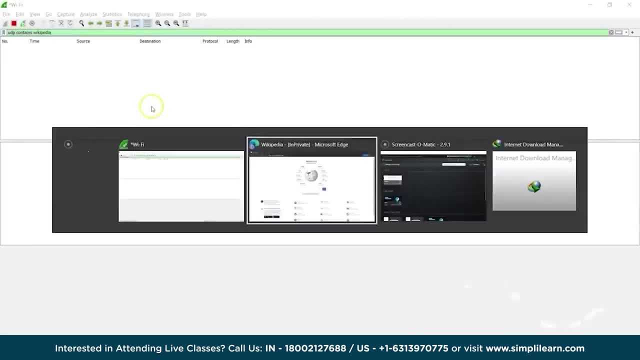 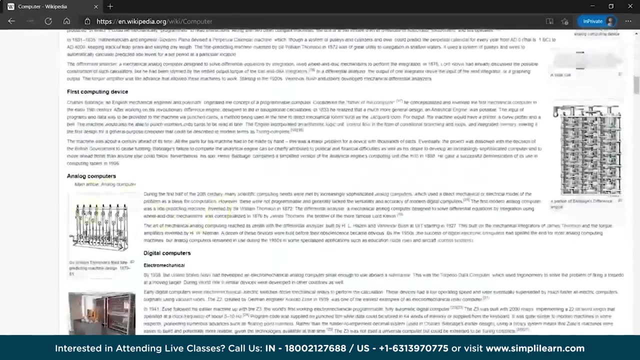 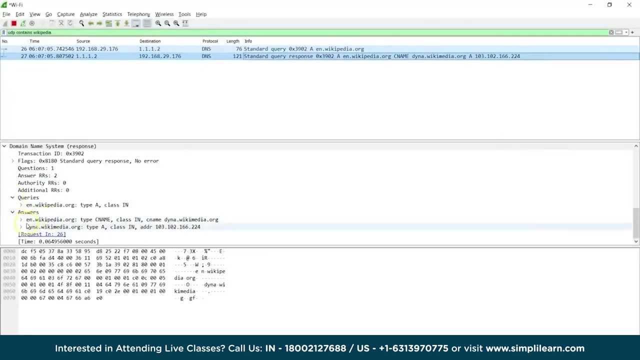 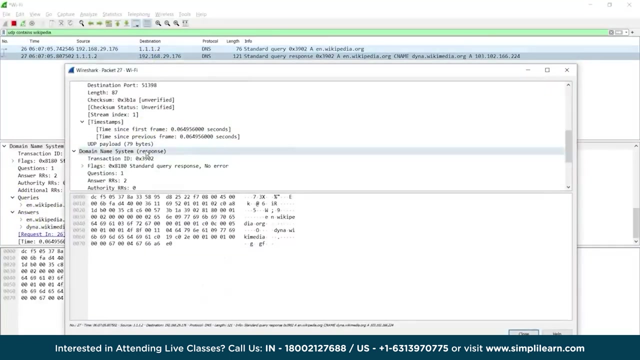 will only show us the results related to Wikipedia. Let's search for something that we can navigate the website with. Okay, once we get into it a little. you can see some of the requests being populated over here. Let's take a look at the specific request. 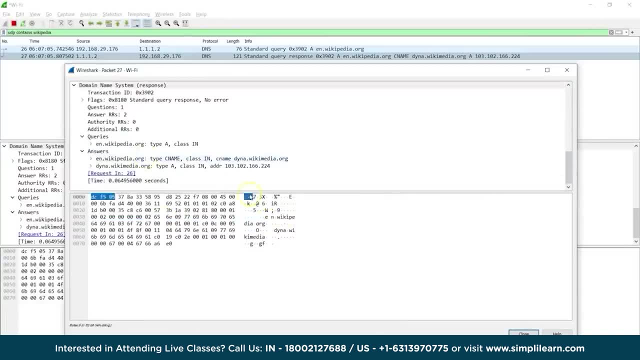 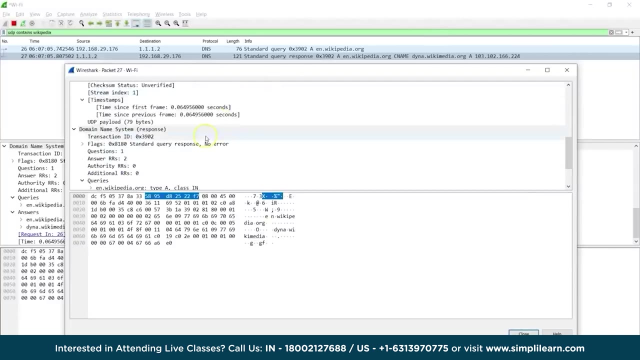 These are the data packets that basically transport the data from our machine to the internet and vice versa. As you can see, there's a bunch of gibberish data here that doesn't really reveal anything that we searched or watched. Similarly, other secured websites function the same way, and it is very difficult, if at 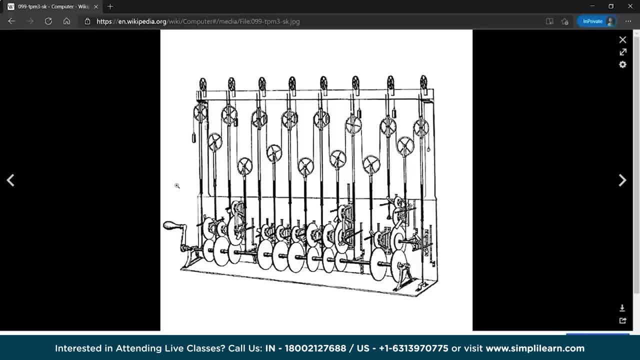 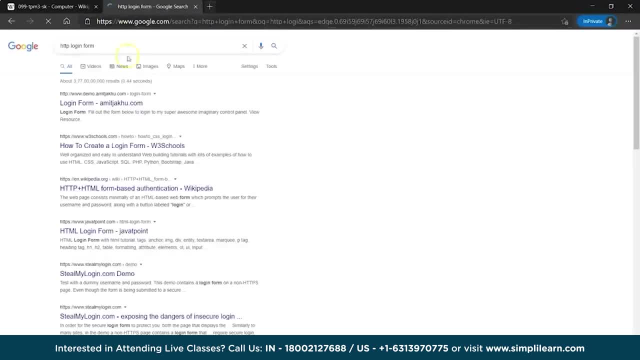 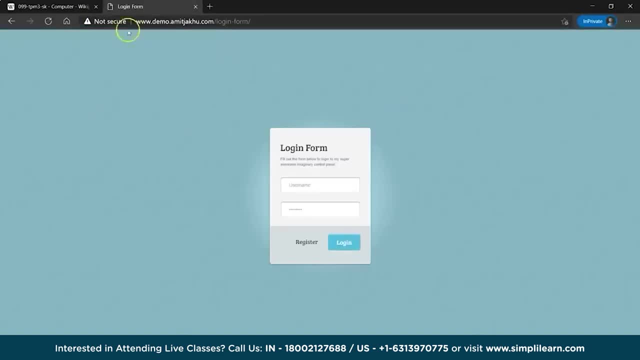 all possible to snoop on user data this way. To put this in perspective, let's take a look at another website, which is a HTTP web page. There's some verses here. Okay, This has no encryption enabled from the server end, which makes it vulnerable to attacks. 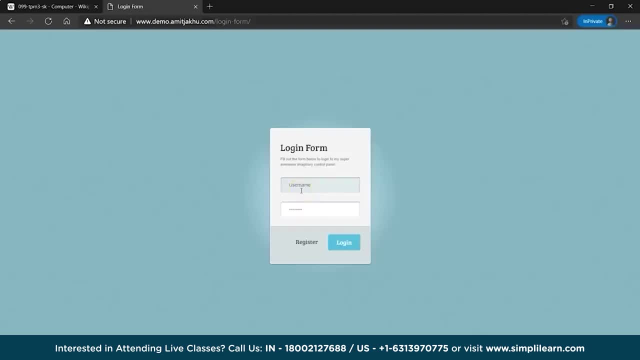 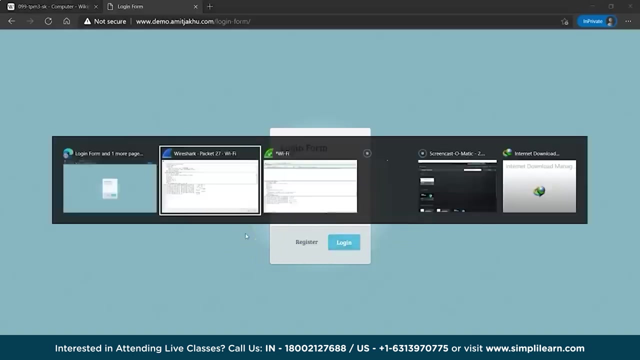 There is a login form here which needs legitimate user credentials in order to grant access. Let's enter a random pair of credentials. These obviously won't work, but we can see the manner of data's transfer. Unsurprisingly, we weren't able to get into the platform. 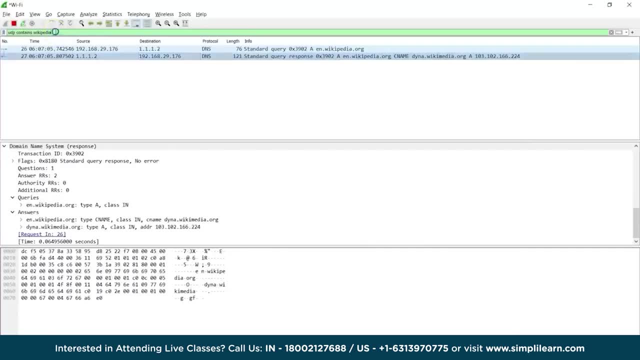 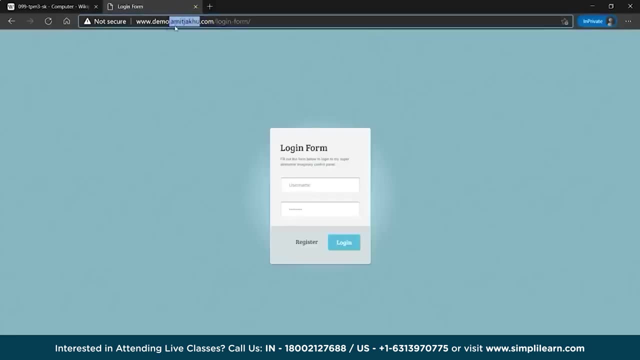 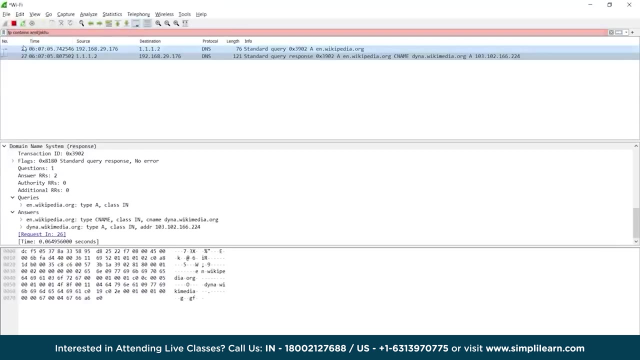 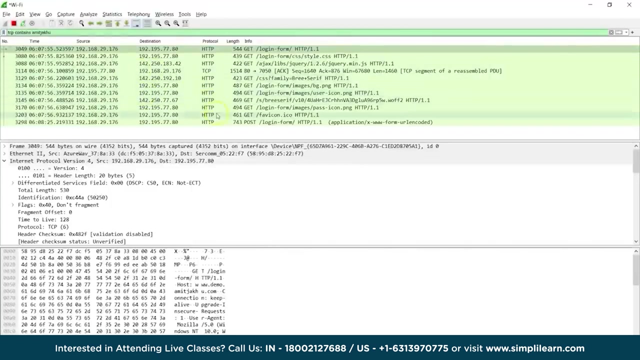 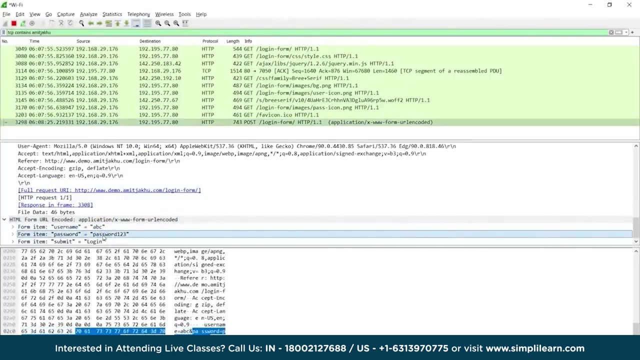 Instead, we can see the data packets. Let's apply a similar filter that will help us understand what request this website is sending. These are the requests being sent by the HTTP login form to the internet. If we check here, see whatever username and password that we are entering, we can easily 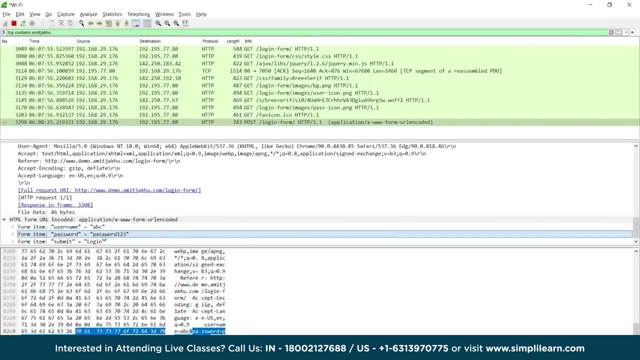 see it with the wireshark. Now, we used a dummy pair of credentials. If we select the right data packet, we can find our correct credentials. If any website had asked for our payment information or our legitimate credentials, it would have been really easy to get a hold of these. 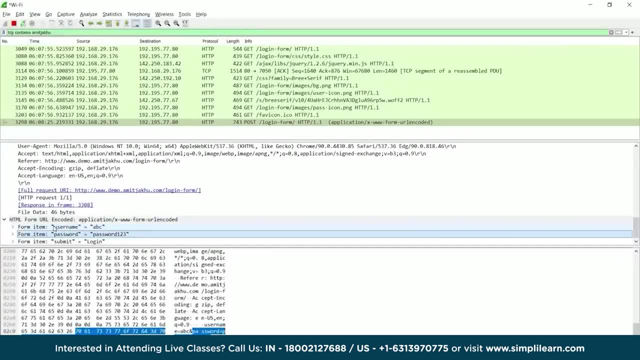 To reiterate what we have already learnt: we must always avoid HTTP websites and just unknown or not trustworthy websites, Because the problem we saw here is just the tip of the iceberg. Even though cryptography has managed to lessen the risk of cyber attacks, it is still prevalent. 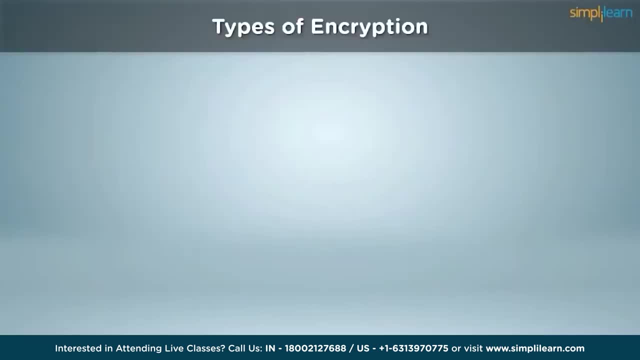 and we should always be alert to keep ourselves safe online. There are two types of encryption in cryptography: symmetric key cryptography and asymmetric key cryptography. Both of these categories have their pros and cons and differ only by their implementation. Today, we are going to focus exclusively on symmetric key cryptography. 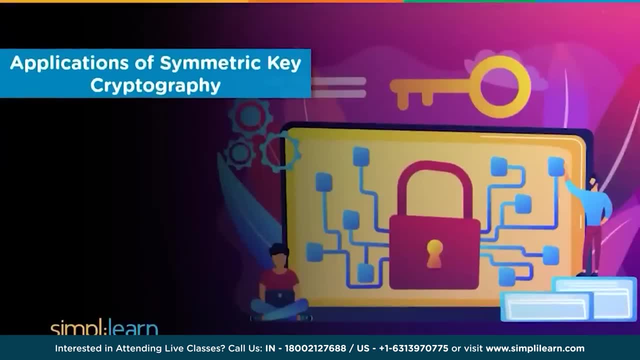 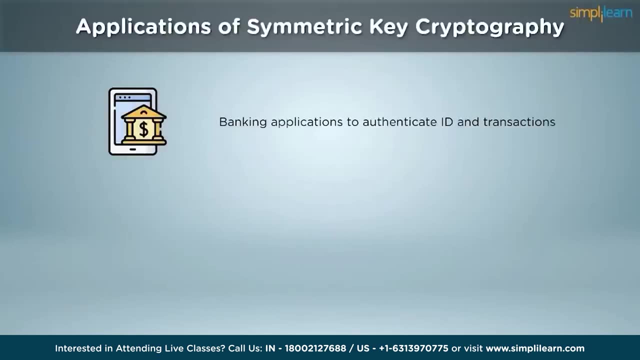 Let us have a look at its applications in order to understand its importance better. This variant of cryptography is primarily used in banking applications, where personally identifiable information needs to be encrypted. With so many aspects of banking, moving on to the internet, having a reliable safety. 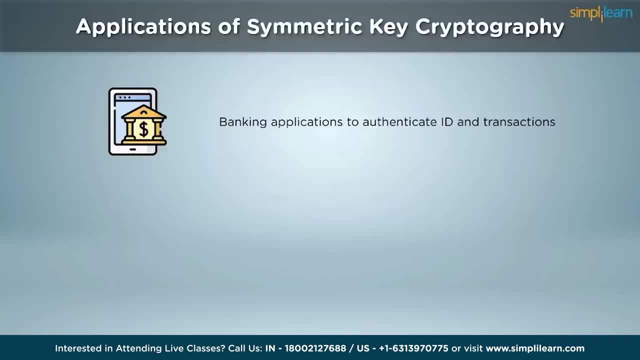 net is crucial. Symmetric cryptography helps in detecting bank fraud and boosts the security index of these payment gateways in general. Symmetric cryptography helps in detecting bank fraud and boosts the security index of these payment gateways in general. They are also helpful in protecting data that is not in transit and rests on servers and. 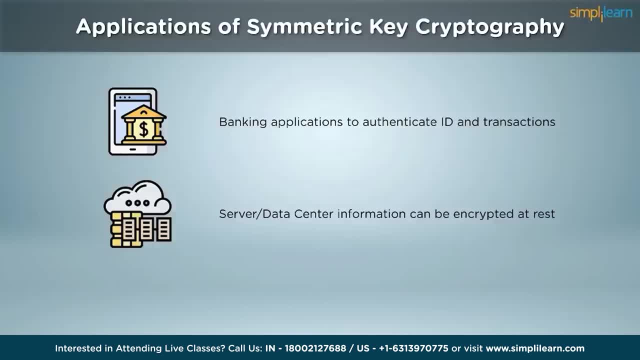 data centers. These centers house a massive amount of data that needs to be encrypted with a fast and efficient algorithm so that, when the data needs to be recalled by the respective service, there is the assurance of minor to no delay While browsing the internet. we need symmetric encryption to browse secure HTTPS websites. 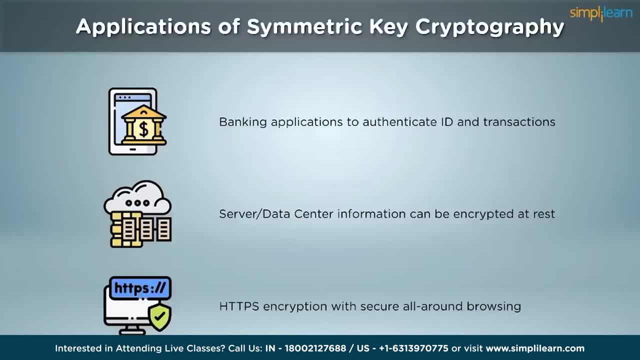 so that we get an all-around protection. It plays a significant role in verifying the security of data. It is also helpful in protecting data that is not in transit and rests on servers and data centers. It helps in identifying website server authenticity, exchanging the necessary encryption keys required. 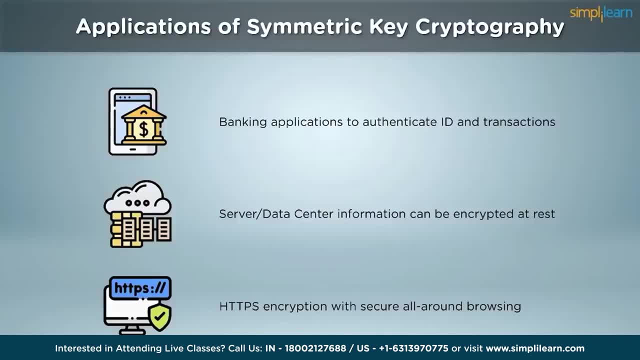 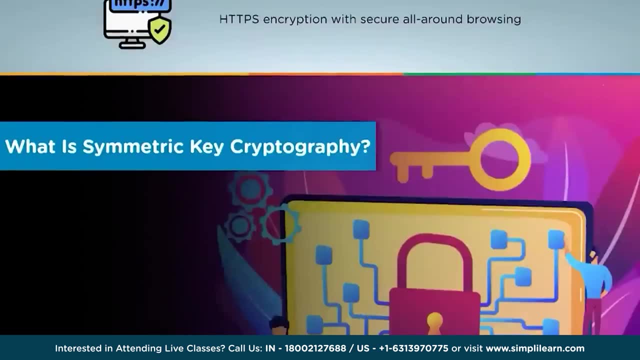 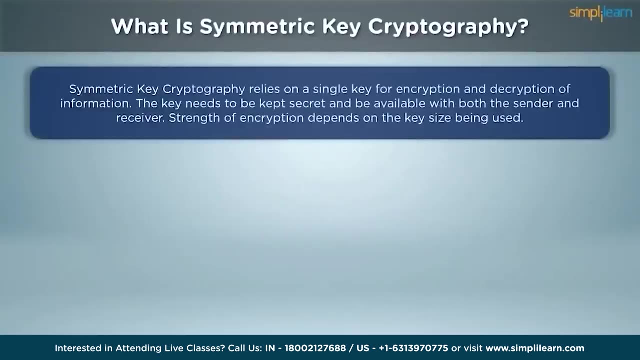 and generating a session using those keys to ensure maximum security. This helps us in preventing the rather insecure HTTP website format. So let us understand how symmetric key cryptography works first, before moving on to the specific algorithms. Symmetric key cryptography relies on a single key for the encryption and decryption of information. 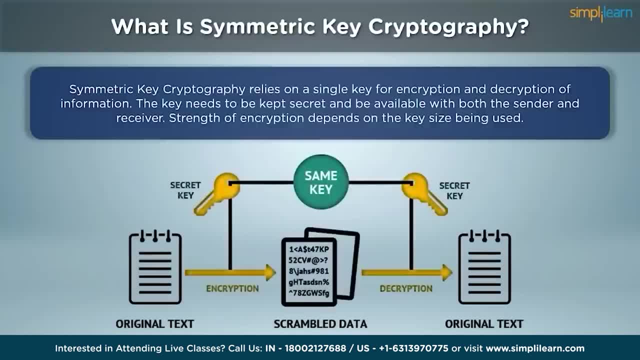 Both the sender and receiver need to be encrypted. We need to have a single key for the encryption and decryption of information, of the message, need to have a pre-shared secret key that they will use to convert the plaintext into ciphertext and vice versa. As you can see in the image, the key used for encryption is: 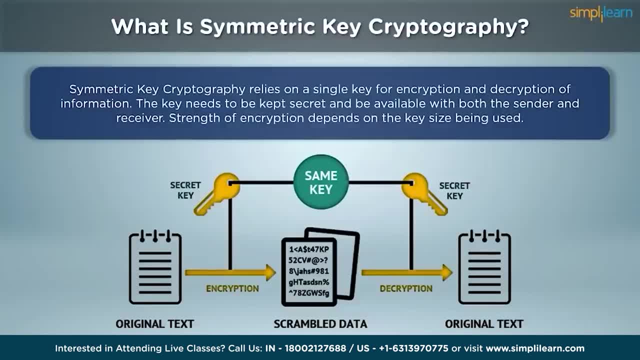 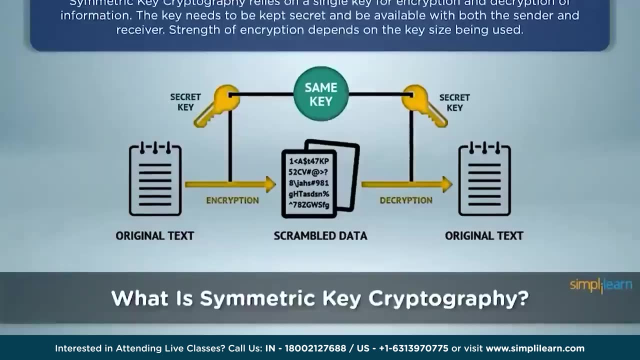 the same key needed for decrypting the message at the other end. The secret key shouldn't be sent along with the ciphertext to the receiver, because that would defeat the entire purpose of using cryptography. Key exchange can be done beforehand using other algorithms, like the Diffie-Hellman key exchange protocol, for example. For example, if Paul wants to send a simple 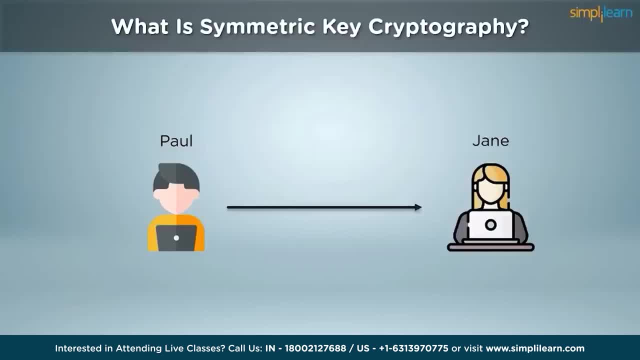 message to Jane. they need to have a single encryption key that both of them must keep secret to prevent snooping on by malicious actors. It can be generated by either one of them but must belong to both of them before the messages start flowing. Suppose the message I am ready is. 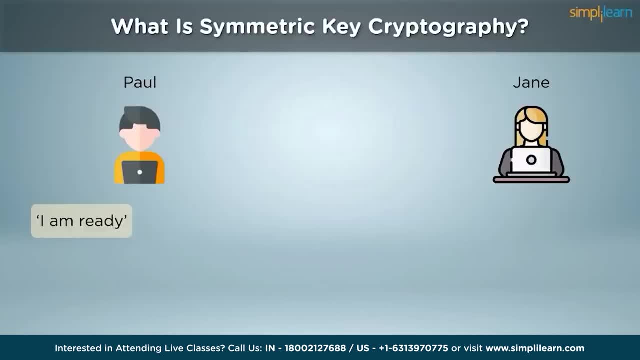 converted into ciphertext using a specific substitution cipher by Paul. In that case, the message will be sent to the receiver and the receiver will receive the message. Jane must also be aware of the substitution shift to decrypt this ciphertext once it reaches her, Irrespective of the scenario where someone manages to grab the ciphertext mid-transit to try and read. 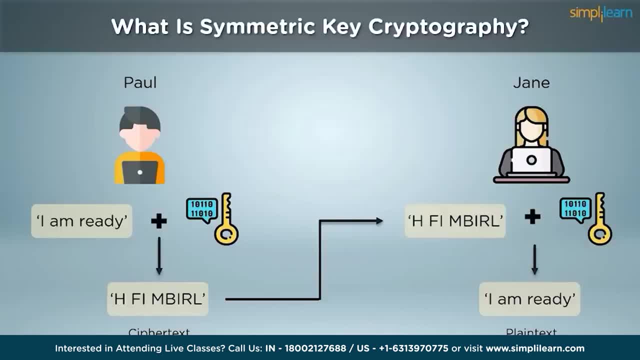 the message. not having the secret key renders everyone helpless looking to snoop in. The symmetric key algorithms like the data encryption standard have been in use since the 1970s, while the popular ones like the AES have become the industry standard today. 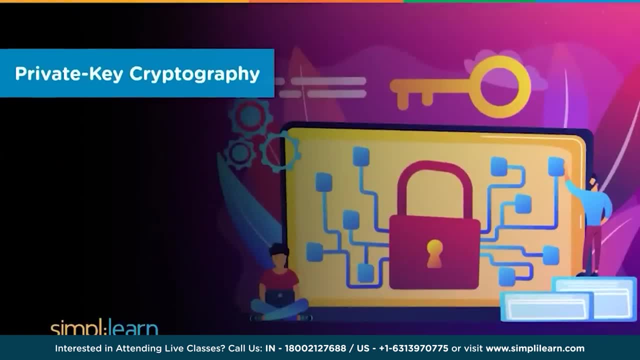 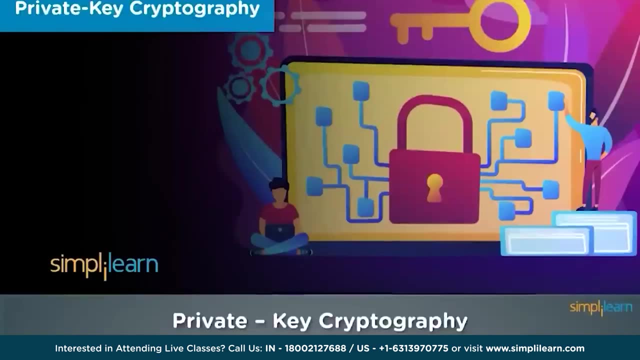 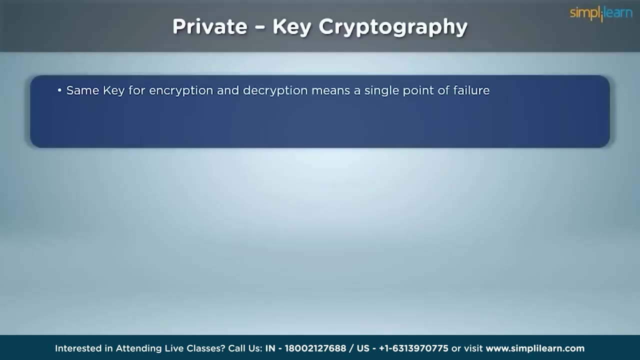 With the entire architecture of symmetric cryptography depending on the single key being used, you can understand why it is of paramount importance to keep it secret on all occasions. The side effect of having a single key for the encryption and decryption is it becomes a single point of failure. Anyone who gets their hand on it can read all the encrypted messages. 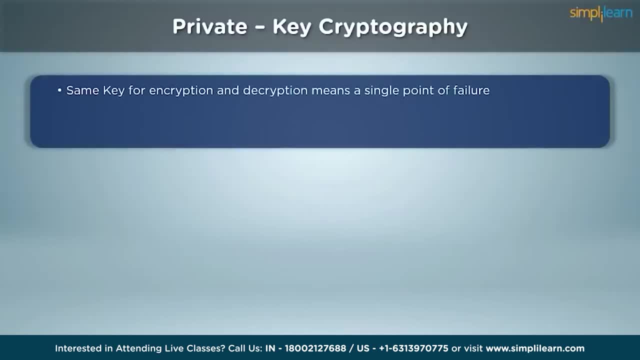 and do so mainly without the knowledge of the sender and the receiver. So it is the priority to keep the encryption and decryption key private at all times. Should it fall into the wrong hands, the third party can send messages to either the sender or the receiver using the same key to encrypt the message. 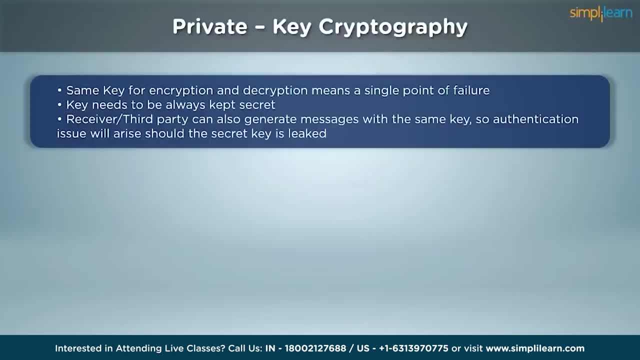 Upon receiving the message and decrypting it with the key, it is impossible to guess its origin. If the sender somehow transmits the secret key along with the ciphertext, anyone can intercept the package and access the information. Consequently, this encryption category is termed private key cryptography. 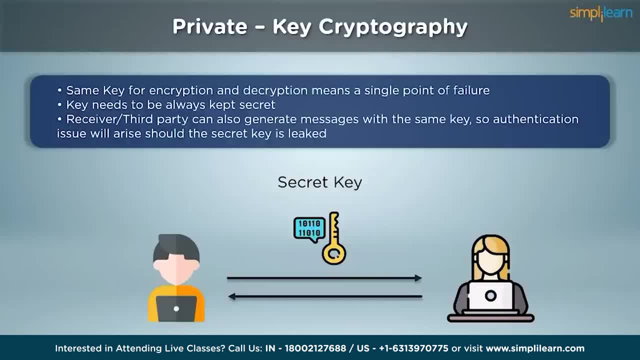 since a big part of the data's integrity is riding on the promise that the users can keep the keys secret. This terminology contrasts with asymmetric key cryptography, which is called public key cryptography because it has two different keys at play, one of which is public. 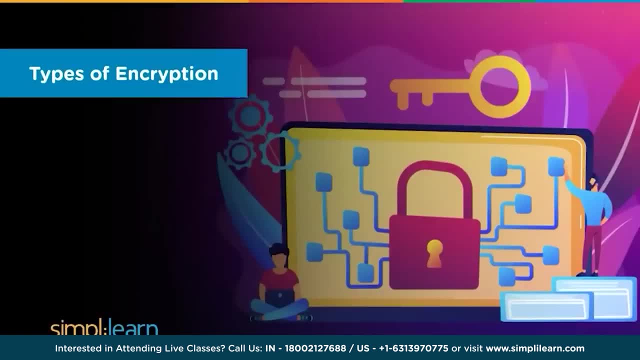 Provided we manage to keep the keys secret. we still have to choose what kind of ciphers we want to use to encrypt this information. In symmetric key cryptography, there are broadly two categories of ciphers that we can employ. Let us have a look. 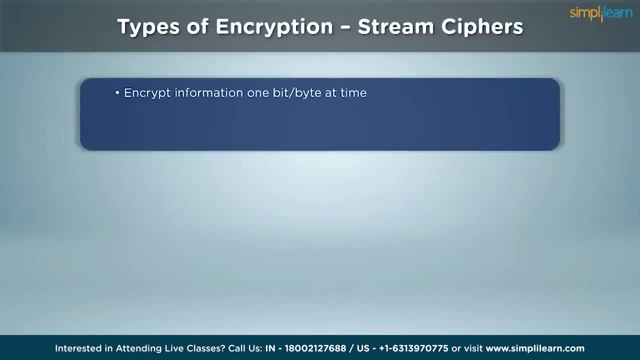 Stream ciphers are the algorithms that encrypt basic information, words and data one bit at a time. It can change depending on the algorithm being used, but usually it relies on a single bit or byte to do the encryption. This is the relatively quicker alternative. 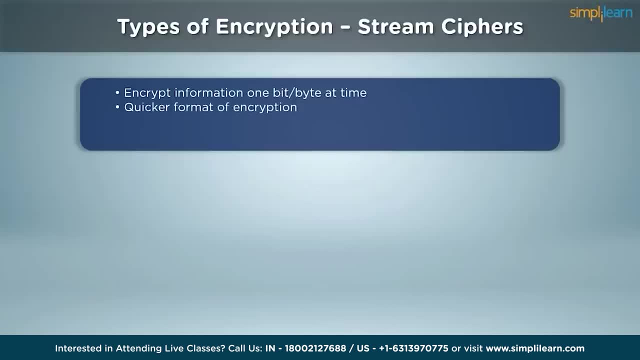 considering the algorithm doesn't have to deal with blocks of data at a single time. Every piece of data that goes into the encryption can and needs to be converted into binary format. In stream ciphers, each binary digit is encrypted, one after the other. 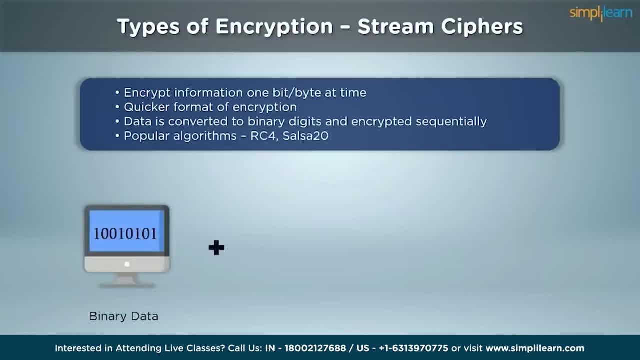 The most popular ones are the RC4, Salsa and Panama. The binary data is passed through an encryption key, which is a randomly generated bitstream. Upon passing it through, we receive the ciphertext that can be transferred to the receiver without fear of man-in-the-middle attacks. 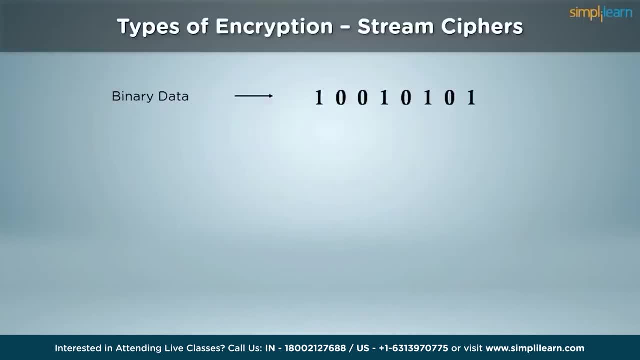 The binary data can be passed through an algorithmic function. It can have either XOR operations, as it is most of the time, or any other mathematical calculations that have the singular purpose of scrambling the data. The encryption key is generated using the random bitstream generator. 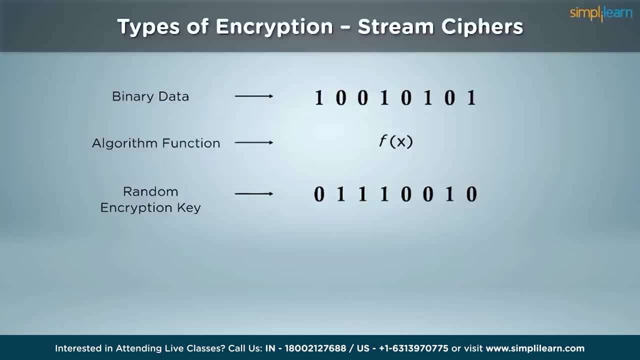 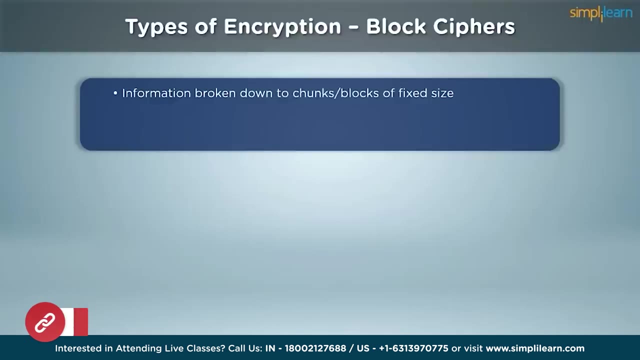 and it acts as a supplement in the algorithmic function. The output is in binary form, which is then converted into the decimal or hexadecimal format to give our final ciphertext. On the other hand, block ciphers dissect the raw information into chunks of data of fixed size. 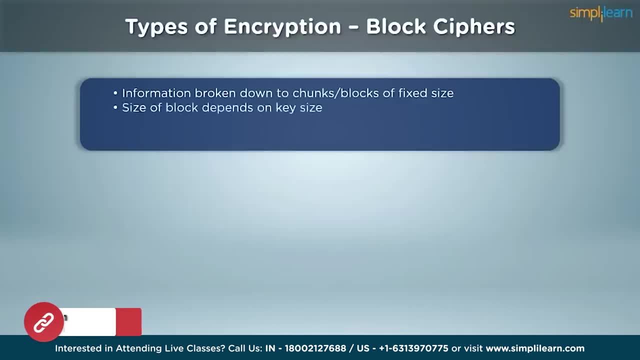 The size of these blocks depend on the exact cipher being used. A 128-bit block cipher will break the plaintext into blocks of 128-bit each and encrypt those blocks instead of a single digit. Once these blocks are encrypted individually, they are chained together to form our final ciphertext. 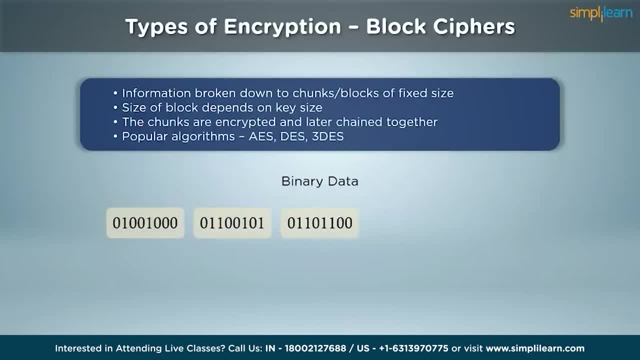 Block ciphers are much slower, but they are more tamper-proof and are used in some of the most widely used algorithms employed today. Just like stream ciphers, the original ciphertext is converted into binary format before beginning the process. Once the conversion is complete, 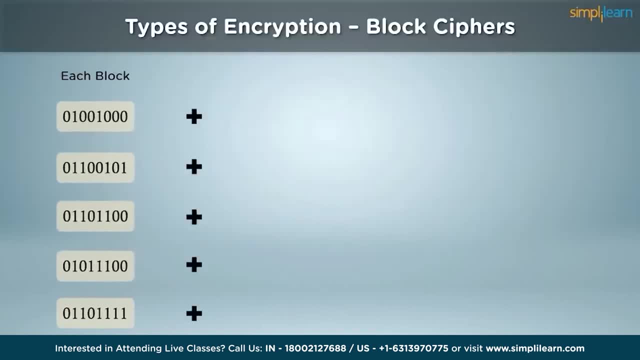 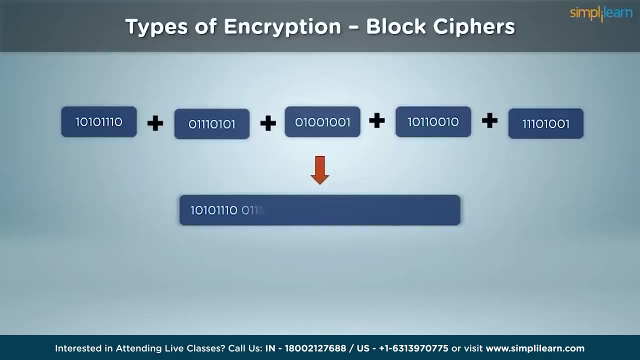 the blocks are passed through the encryption algorithm along with the encryption key. This would provide us with the encrypted blocks of binary data. Once these blocks are combined, we get a final binary string. This string is then converted into hexadecimal format to get our ciphertext. 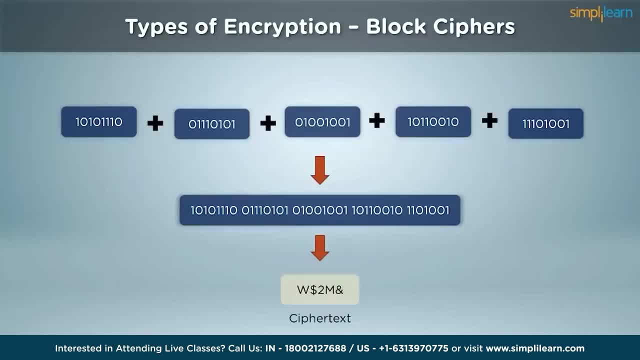 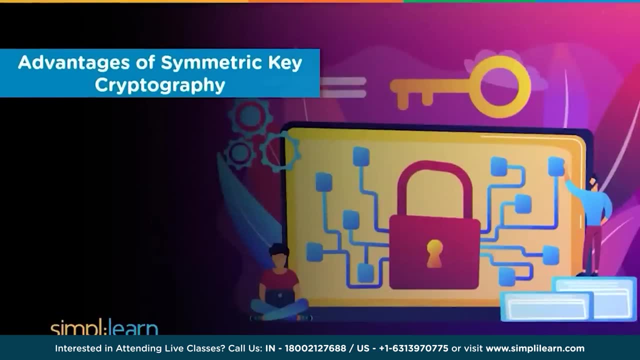 Today, the most popular symmetric key algorithms like AES, DES and 3DES are all block cipher methodology subsets. With so many factors coming into play, there are quite a few things symmetric key cryptography excels at, while falling short in some other. 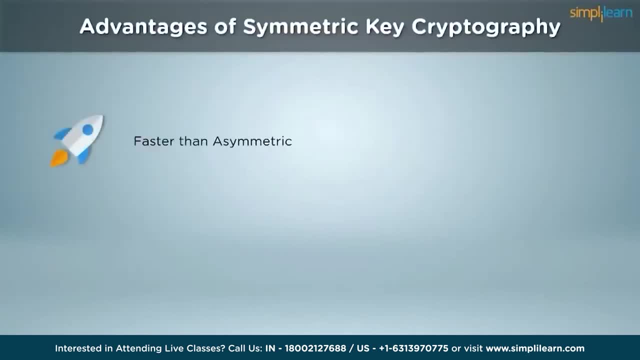 Symmetric key cryptography is a much faster variant when compared to asymmetric key cryptography. There is only one key in play, unlike asymmetric encryption, and this drastically improves calculation speed in the encryption and decryption. Similarly, the performance of symmetric encryption is much more efficient under similar computational limitations. 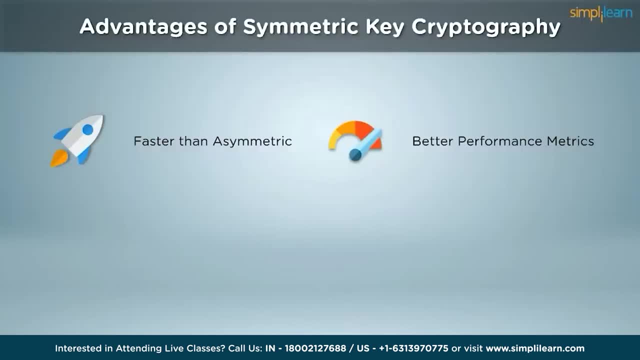 Fewer calculations help in better memory management for the whole system. Bulk amounts of data that need to be encrypted are very well suited for symmetric algorithms, Since they are much quicker. handling large amounts of data is simple and easy to use in servers and data farms. 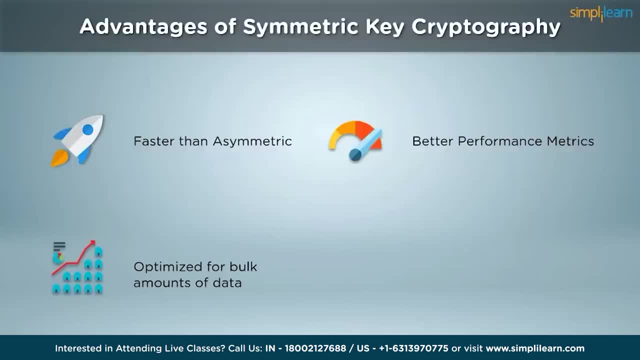 This helps in better latency during data recall and fewer mixed packets. Thanks to its simple single key structure, symmetric key cryptography algorithms are much easier to set up a communication channel with and offer a much more straightforward maintenance duties Once the secret key is transmitted to both the sender and receiver. 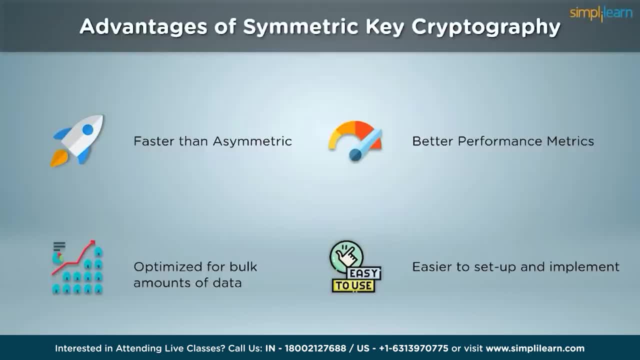 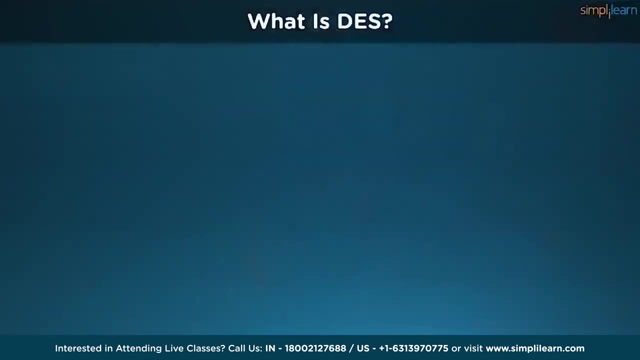 without any prior mishandling. the rest of the system aligns easily and everyday communications becomes easy and secure If the algorithm is applied as per the documentation. symmetric algorithms are very robust and can encrypt vast amounts of data with very less overhead. DES algorithm stands for Data Encryption Standard. 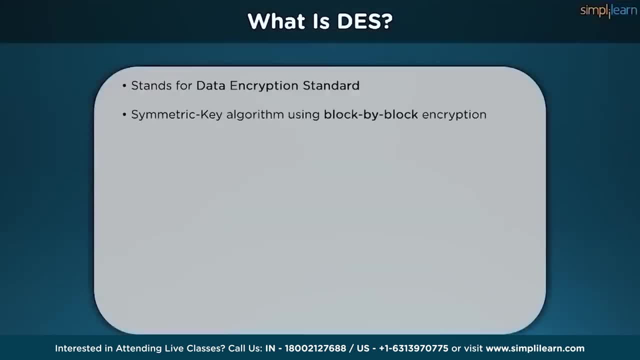 It is a symmetric key cipher that is used to encrypt and re-crypt information in a block-by-block manner. Each block is encrypted individually and they are later chained together to form our final ciphertext, which is then sent to a receiver. DES takes the original, unaltered piece of data. 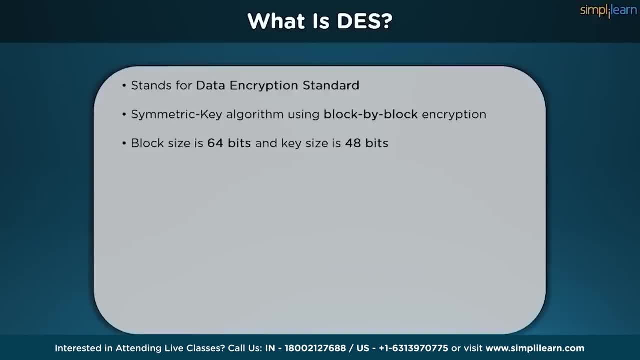 called the plain text in a 64-bit block and it is converted into an encrypted text that is called the ciphertext. It uses 48-bit keys during the encryption process and follows a specific structure called the Fistel cipher structure throughout the entire process. It is a symmetric key algorithm. 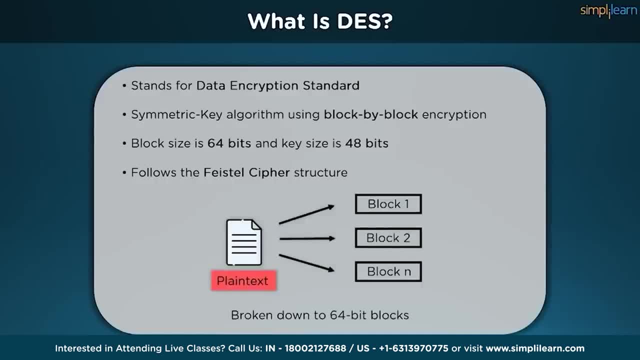 which means DES can reuse the keys used in the encryption format to decrypt the ciphertext back to the original plain text. Once the 64-bit blocks are encrypted, they can be combined together before being transmitted. Let's take a look at the origin and the reason DES was founded. 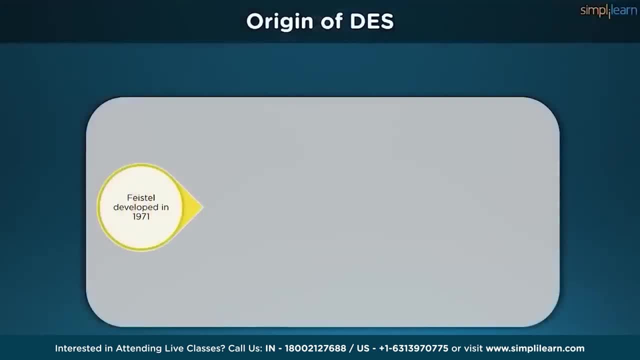 DES is based on a Fistel block cipher called Lucifer, developed in 1971 by IBM cryptography researcher Horst Fistel. DES uses 16 rounds of this Fistel structure, using a different key for each round. It also utilizes a random function with two inputs and provides a single output variable. 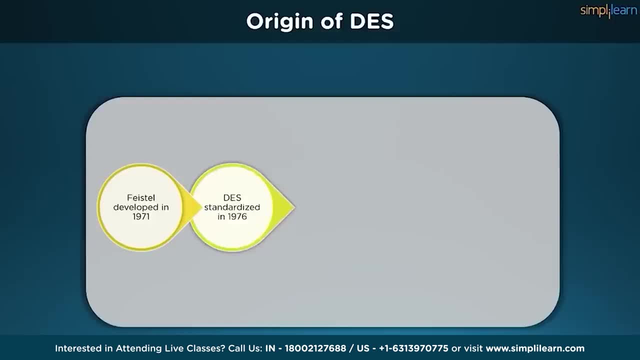 DES became the organization's approved encryption standard in November 1976 and was later reaffirmed as a standard in 1983, 1988 and finally in 1999.. But eventually DES was cracked and it was no longer considered a secure solution for all official routes of communication. 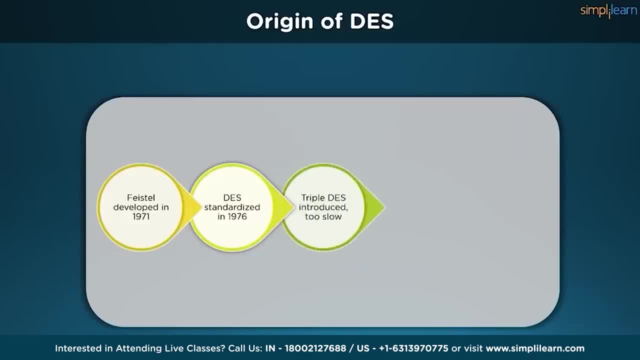 Consequently, Triple DES was developed. Triple DES is a symmetric key block cipher that uses a double DES cipher: Encrypt with the first key, delete encryption with the second key and encrypt again with the third key. There is also a variation of the two keys. 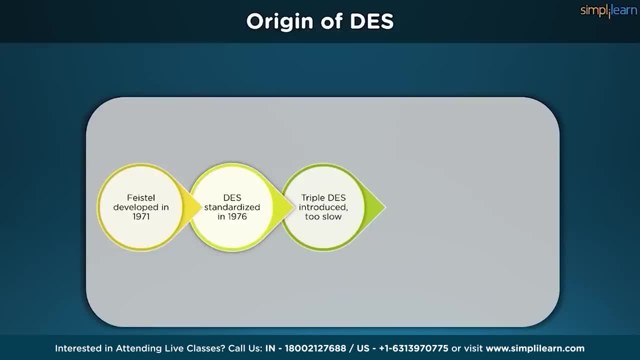 where the first and second key are duplicate of each other. But Triple DES was ultimately deemed too slow for the growing need for fast communication channels, and people eventually fell back to using DES for encrypting messages. In order to search for a better alternative, a public-wide competition was organized. 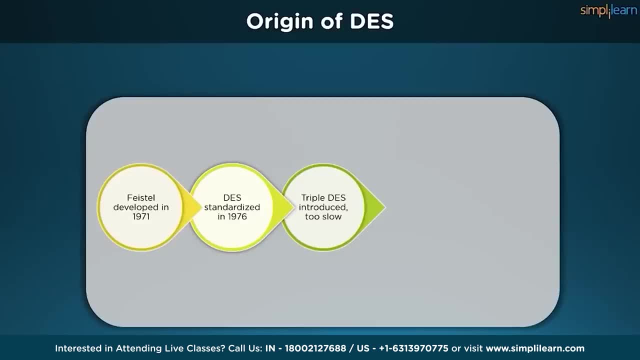 and helped cryptographers develop their own algorithm as a proposal for the next global standard. This is where the RingDial algorithm came into play and was later credited to be the next advanced encryption standard. For a long time, DES was the standard for data encryption for data security. 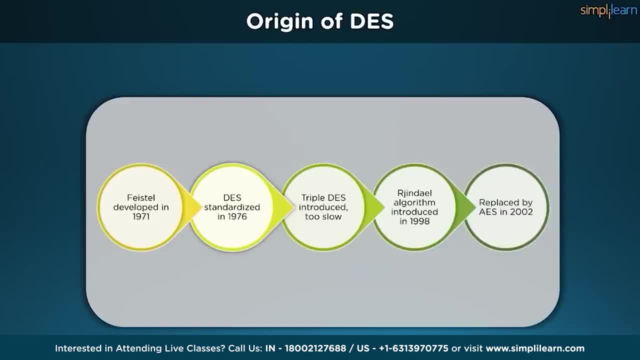 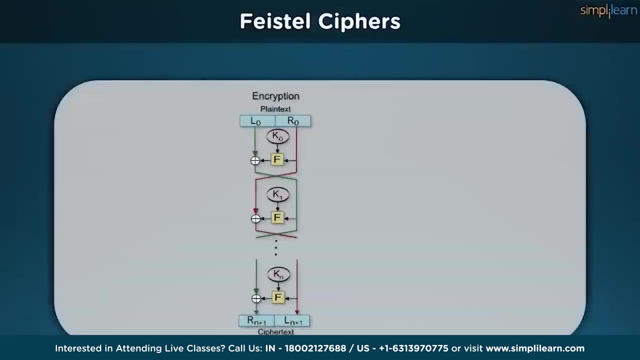 Its rule ended in 2002 when, finally, the advanced encryption standard replaced DES as an acceptable standard, following a public competition for a place To understand the structure of a Fistel cipher, we can use the following image as a reference: The block being encrypted is divided into two parts. 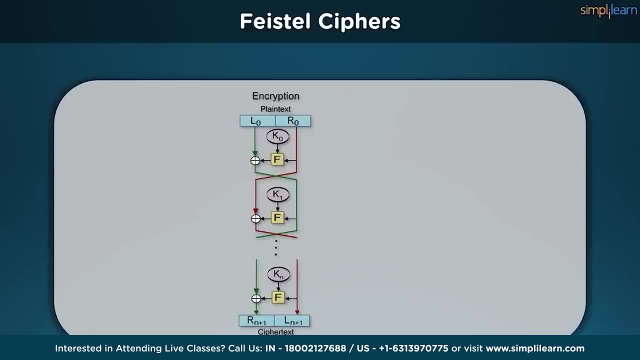 one of which is being passed on to the function, while the other part is XORed with the function's output. The function also uses the encryption key that differs for each individual norm. This keeps going on until the last step, until where the right-hand side 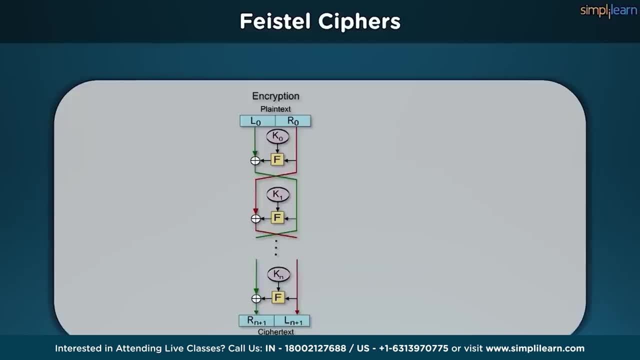 and the left-hand side are being swapped. Here we receive our final ciphertext For the decryption process. the entire procedure is reversed, starting from the order of the keys to the block sorting. If the entire process is repeated in a reverse order, we will eventually get back our plaintext. 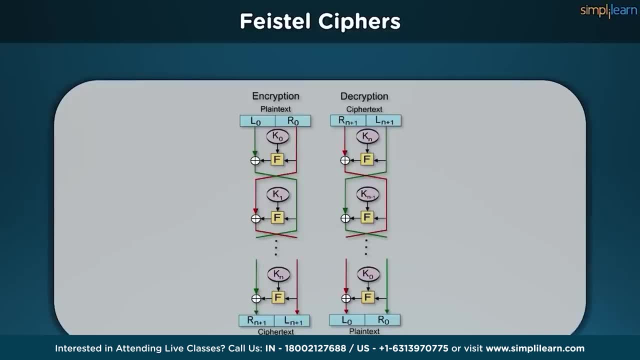 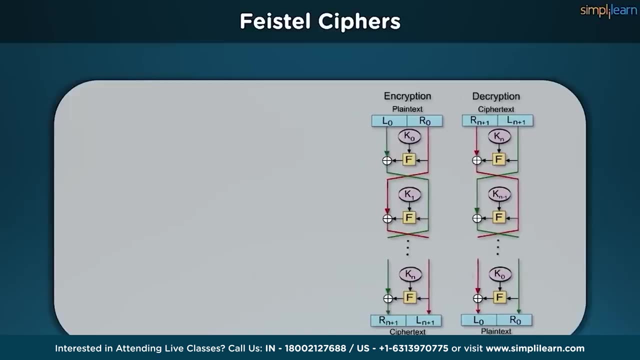 and this simplicity helps the speed Overall. this was later detrimental to the efficiency of the algorithm, hence the security was compromised. A Fistel block cipher is a structure used to derive many symmetric block ciphers, such as DES, which, as we have discussed, 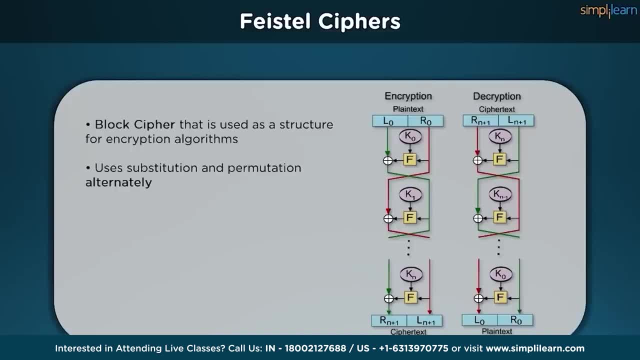 in our previous commentary. Fistel cipher proposed a structure that implements substitution and permutation alternately so that we can obtain ciphertext from the plaintext and vice versa. This helps in reducing the redundancy of the program and increases the complexity to combat brute force attacks. The Fistel cipher is actually based. 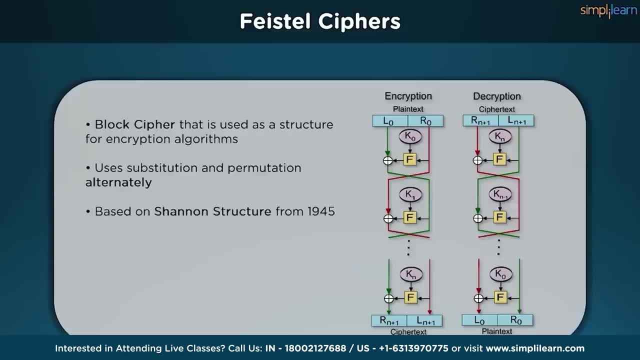 on the Shannon structure that was proposed in 1945.. The Fistel cipher is the structure suggested by Horst Feistel, which was considered to be a backbone while developing many symmetric block ciphers. The Shannon structure highlights the implementation of alternate confusion and diffusion. 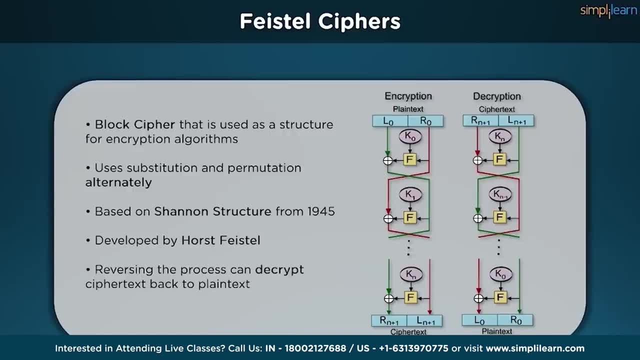 And, like we already discussed, the Fistel cipher structure can be completely reversed depending on the data. However, we must consider the fact that to decrypt the information by reversing the Feistel structure, we will need the exact polynomial functions and the key orders. 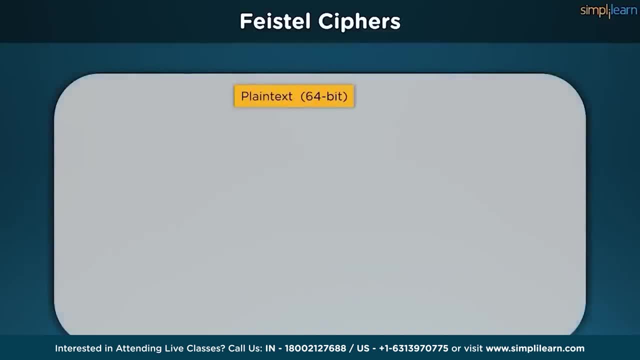 To understand how the blocks are being calculated, we take a plaintext which is of 64-bit and that is later divided into two equal halves of 32-bit each. In this, the right half is immediately transferred to the next round to become the new left half. 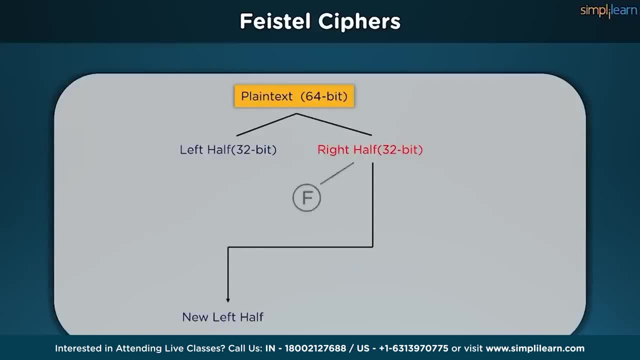 of the second round. The right hand is again passed off to a function which uses an encryption key that is unique to each round in the Fistel cipher. Whatever the function gives off as an output, it is passed on as an XOR input with the left half of the initial plaintext. 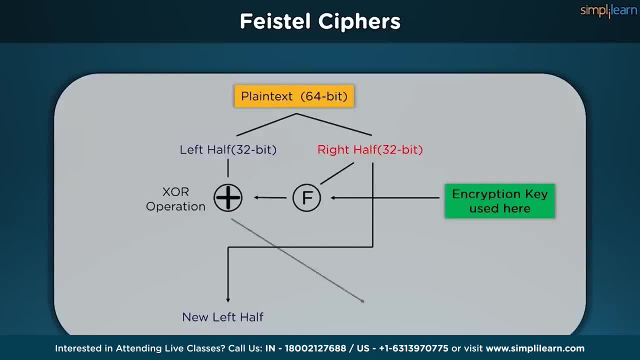 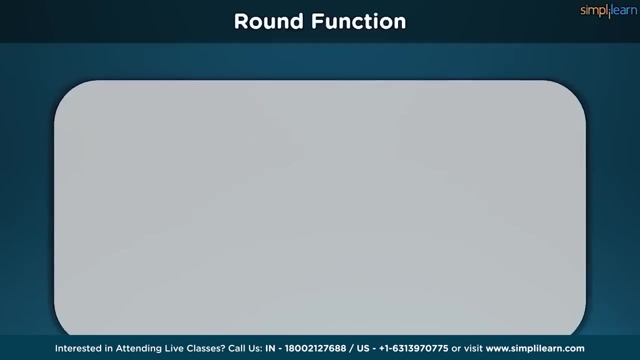 The next output will become the right half of the second round. for the plaintext, This entire process constitutes of a single round in the Fistel cipher. Taking into account what happens in a polynomial function, we take one half of the block and pass it through an expansion box. 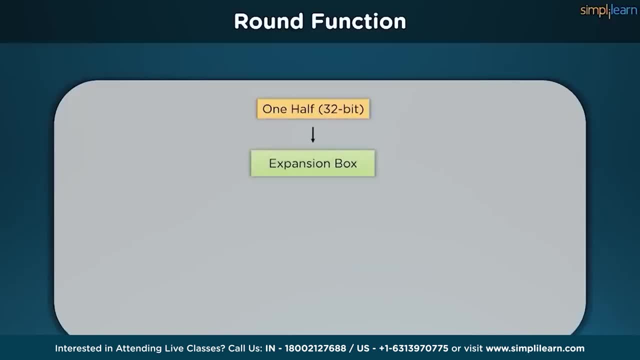 The work of the expansion box is to increase the size of the half from 32-bit to 48-bit text. This is done to make the text compatible to the 48-bit keys we have generated beforehand Once we pass it through the XOR function. 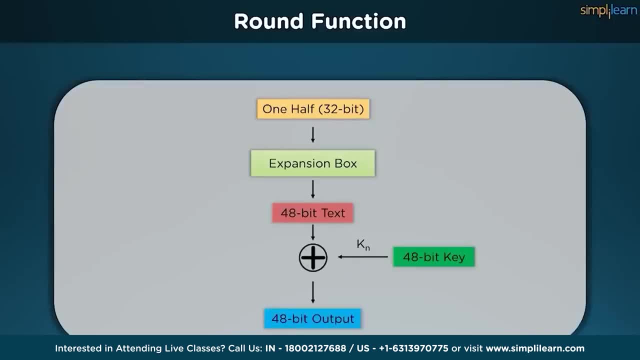 we get a 48-bit text as an output. Now, remember a half should be of 32-bit. So this 48-bit output is then later passed on to a substitution box. This substitution box reduces its size from 48-bit to 32-bit output. 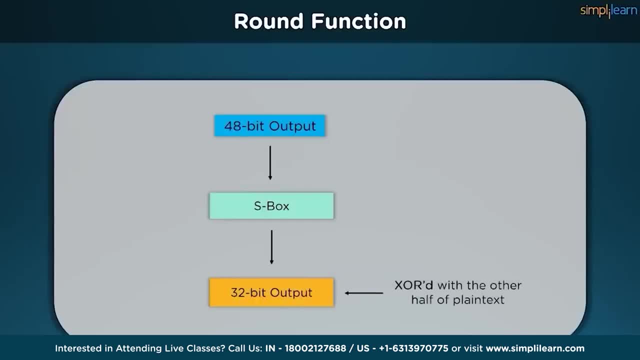 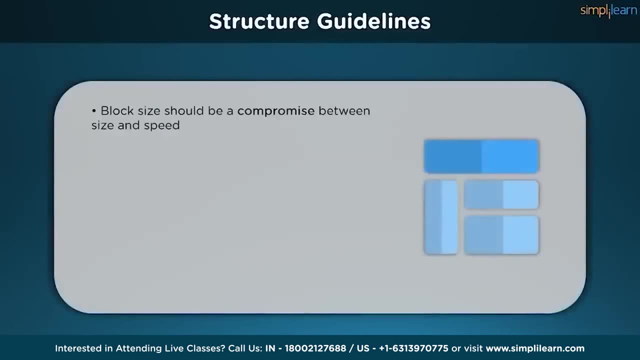 which is then later XORed with the first half of the plaintext. A block cipher is considered the safest if the size of the block is large. But large block sizes can also slow down encryption speed and the decryption speed. Generally the size is 64-bit. 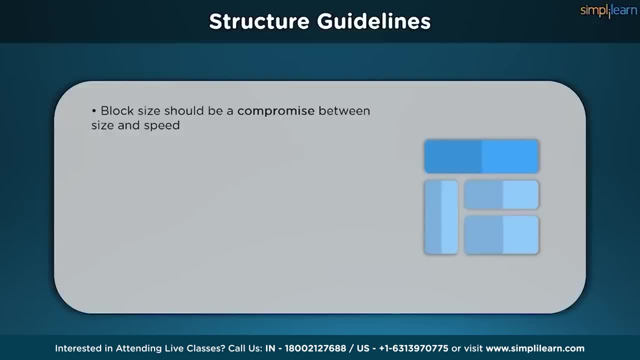 Sometimes modern block ciphers like AES have a 128-bit block size as well. The security of the block cipher increases with increasing key size. Larger key sizes may also reduce the speed of the process. Earlier 64-bit keys were considered sufficient. 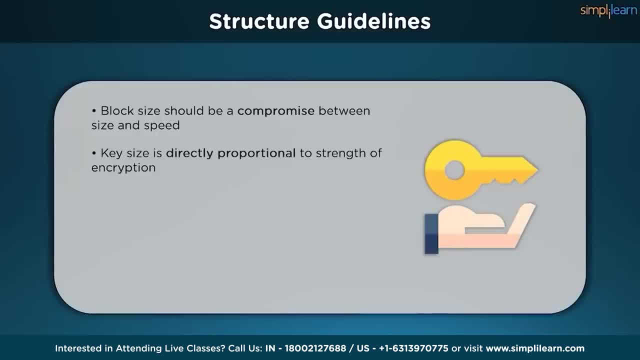 Modern ciphers need to use 128-bit keys due to the increasing complexity of today's computational standards. The increasing number of rounds also increases the security of the block cipher. Similarly, they are inversely proportional to the speed of encryption. A highly complex 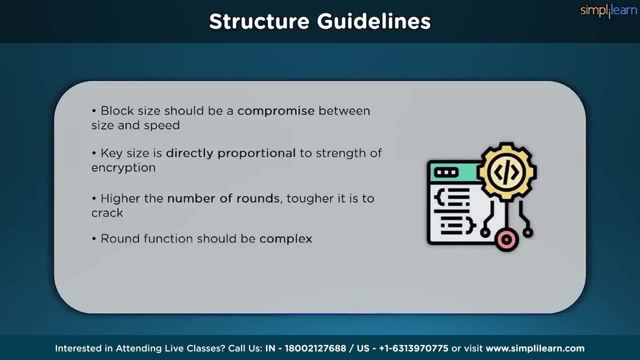 round function enhances the security of the block cipher. We must maintain a balance between the speed and security. The symmetric block cipher is implemented in a software application to achieve better execution speed. There is no use of an algorithm. It cannot be implemented in a real-life framework. 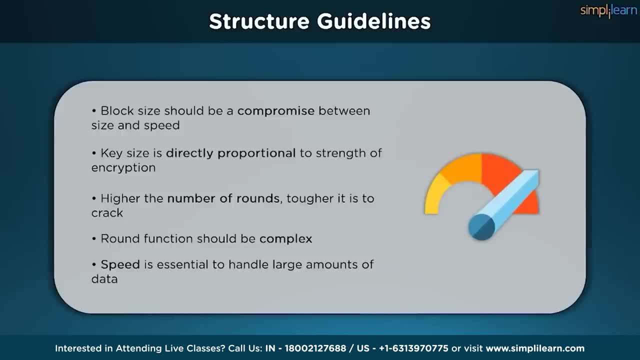 that can help organizations to encrypt or decrypt the data in a timely manner. Now that we understand the basics of Fistel ciphers, we can take a look at how DES manages to run through 16 rounds of this structure and provide the ciphertext. Now that we understand the basics, 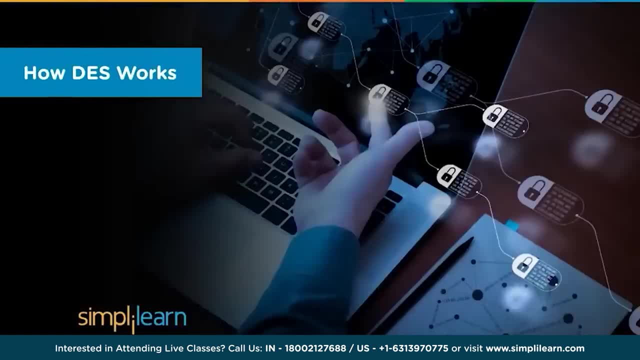 of Fistel ciphers. we can take a look at how DES manages to run through 16 rounds of this structure and provide the ciphertext. In simple terms, DES takes a 64-bit plaintext and converts it into a 64-bit ciphertext. And since we are talking about 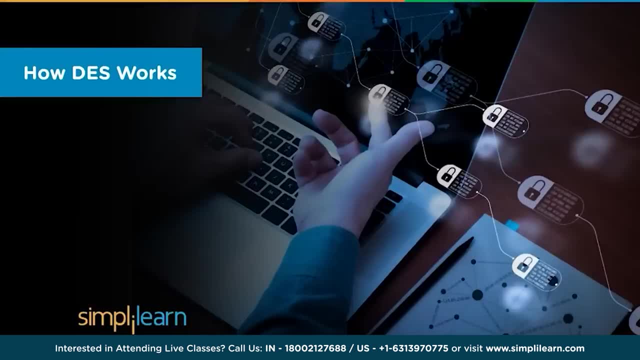 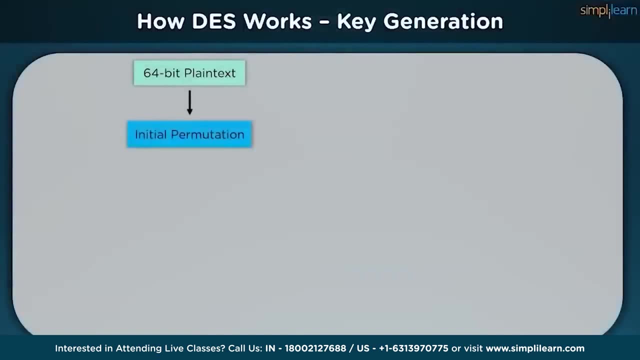 asymmetric algorithms. the same key is being used when it is decrypting the data as well. We first take a 64-bit plaintext and we pass it through an initial permutation function. The initial permutation function has the job of dividing the block into two different. 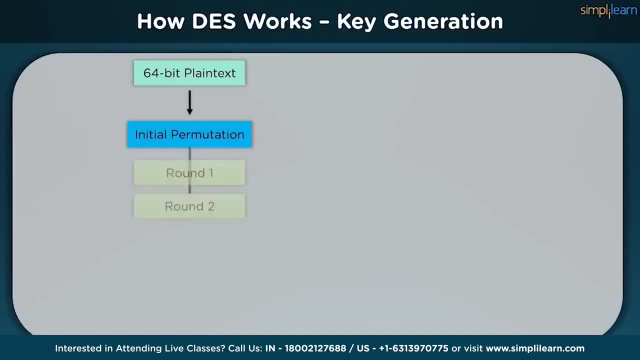 parts so that we can perform Fistel cipher structures on it. There are multiple rounds being procured in the DES algorithm, namely 16 rounds of Fistel cipher structure. Each of these rounds will need keys. Initially we take a 56-bit cipher key. 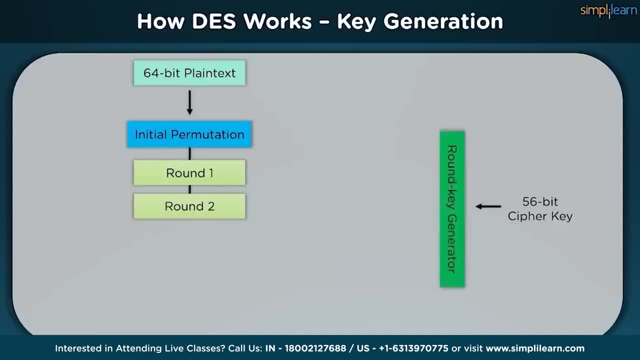 but it is a single key. We pass it onto a round key generator which generates 16 different keys for each single round. These keys are passed on to the rounds as 48-bits. The size of these 48-bits keys is the reason we use substitution. 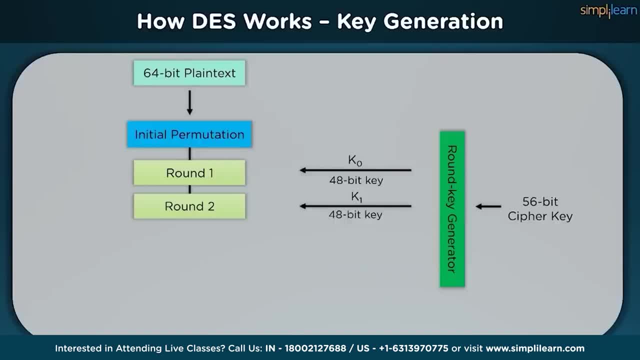 and permutation bounds in the polynomial functions of the Fistel ciphers. When passing through all these rounds, we reach round 16, where the final key is passed on from the round key generator and we get a final permutation. In the final permutation the rounds are swapped. 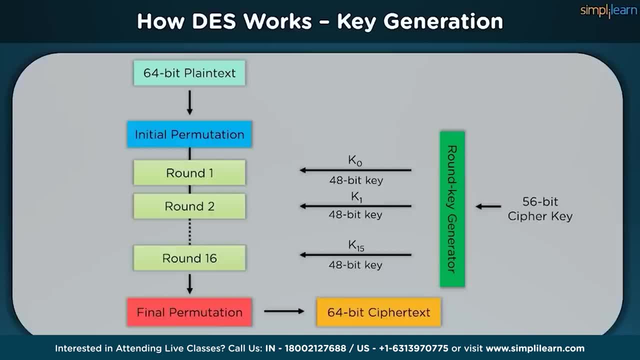 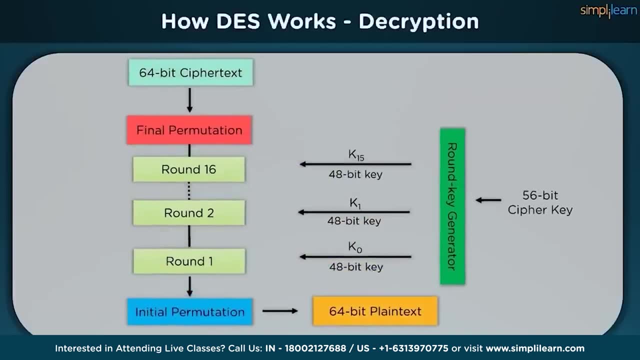 and we get a final ciphertext. This is called DES, with 16 rounds of Fistel ciphers encompassed in it. To decrypt a ciphertext back to the plaintext, we just have to reverse the process we did in the DES algorithm and reverse the key order. 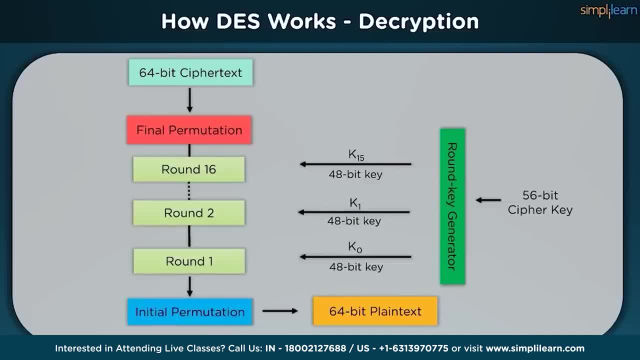 along with the functions. This kind of simplicity is what gave DES the bonus when it comes to speed, but eventually it was detrimental to the overall efficiency of the program. when it comes to security factors, DES have 5 different modes of operation to choose from. 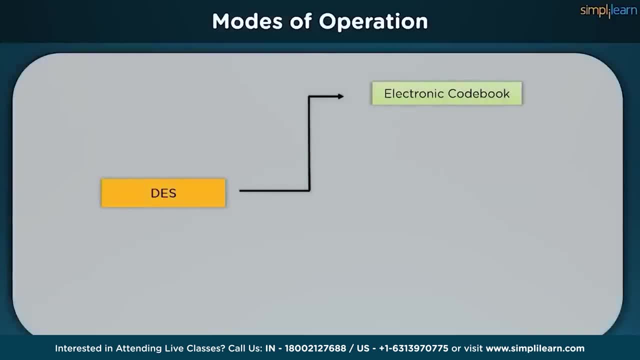 One of those is the electronic codebook. Each 64-bit block is encrypted and decrypted independently in the electronic codebook format. We also have cipherblock chaining or the CBC method. Here, each 64-bit block depends on the previous one and all of them. 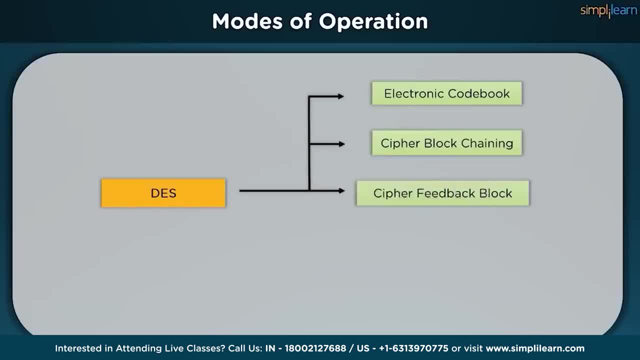 use an initialization vector. We have a cipherfeedback block mechanism where the preceding ciphertext becomes the input for the encryption algorithm. It produces a pseudo-random output which in turn, is XORed with the plaintext. There is an output feedback method as well, which is the same as cipherfeedback. 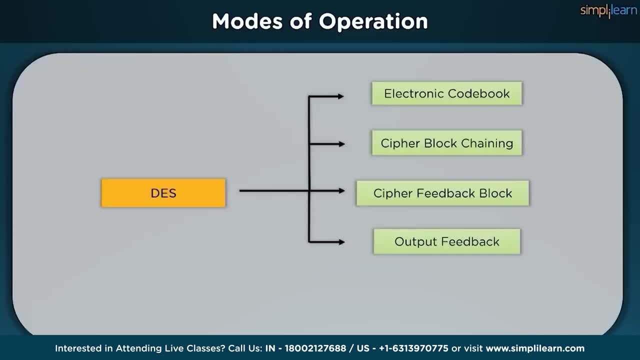 except that the encryption algorithm input is the output from the preceding DES. A counter method has a different way of approach, where each plaintext block is XORed with an encrypted counter, The counter is then incremented for each subsequent block. There are a few other alternatives. 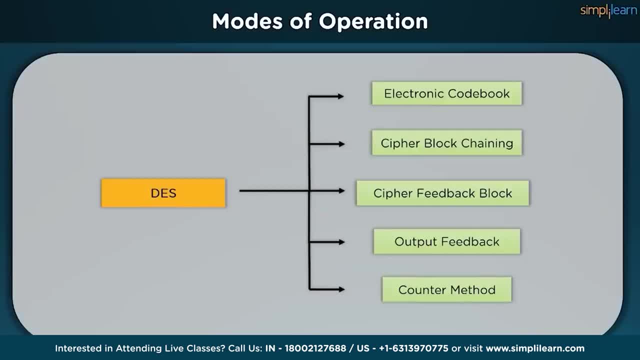 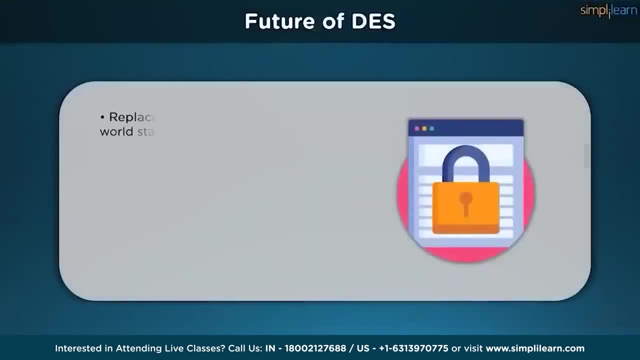 to these modes of operation, but the 5 mentioned above are the most widely used in the crypto industry and recommended by cryptographers worldwide. Let's take a look at the future of DES. The dominance of DES ended in 2002 when the Advanced Encryption Standard. 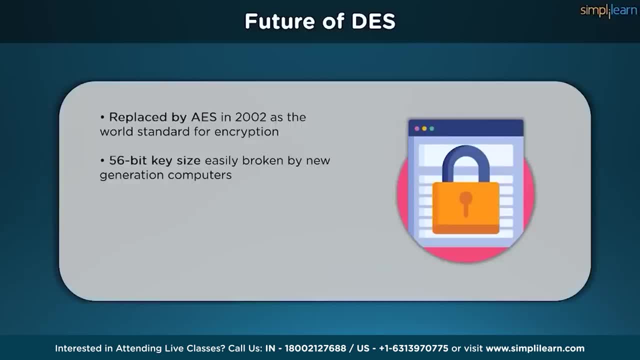 replaced the DES encryption algorithm as the accepted standard. It was done following a public competition to find a replacement. NIST officially withdrew the Global Acceptance Standard in May 2005,. although Triple DES has approved for some sensitive government information through 2030. 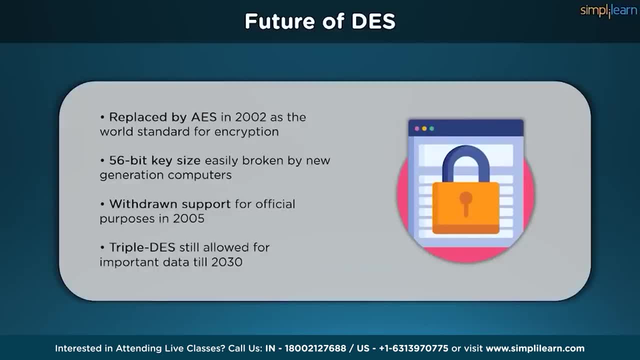 They decided to change the DES algorithm because its key length was too short, given the increased processing power of the new computers. Encryption power is related to the size of the key, and DES found itself a victim of ongoing technological advances in computing. We have received a point where 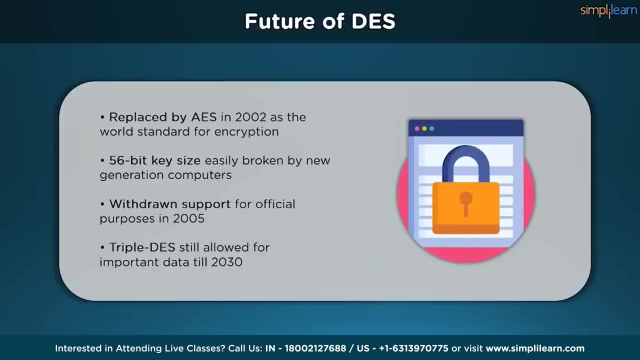 56-bit was no longer a challenge to the computers of cracking. Note that because DES is no longer the NIST federal standard, it does not mean that it is no longer in use. Triple DES is still used today and is still considered to be one of the most. 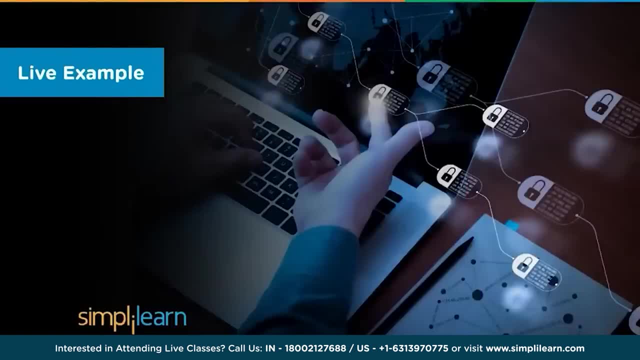 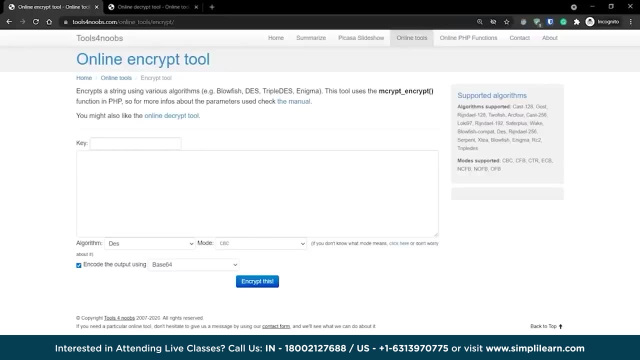 powerful NIST encryption algorithms. To get a better understanding of how these keys and ciphertext look like, we can use an online tool for our benefit. As we already know, to encrypt any kind of data, a key is mandatory. This key can be generated using mathematical functions. 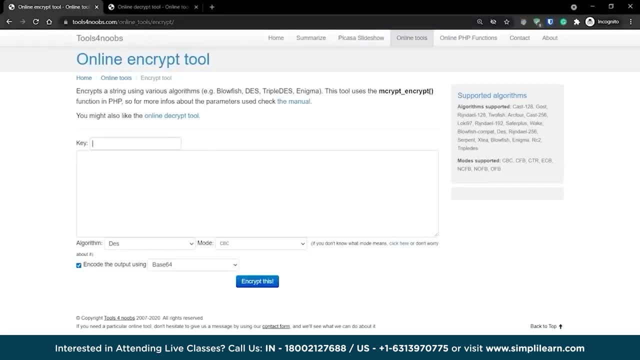 or a computerized key generation program such as this website offers. It can be based on any piece of text. Let's say the word is simply learn in our example. Once this is settled, we provide the plain text or the clear text that needs to be encrypted. 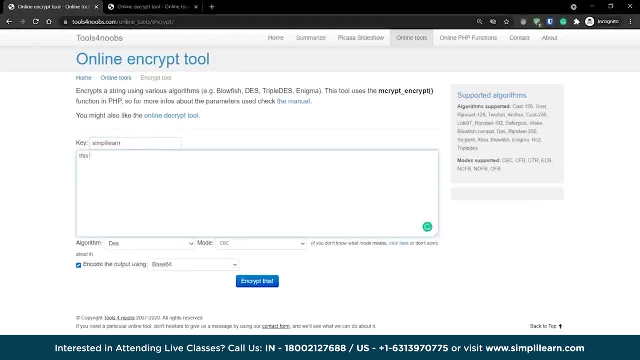 using the aforementioned key Suppose. our sentence for this example is: this is my first message. We have satisfied two prerequisites: the message and the key. Another variable that goes into play is the mode of operation. We have already learned about five different modes of operation. 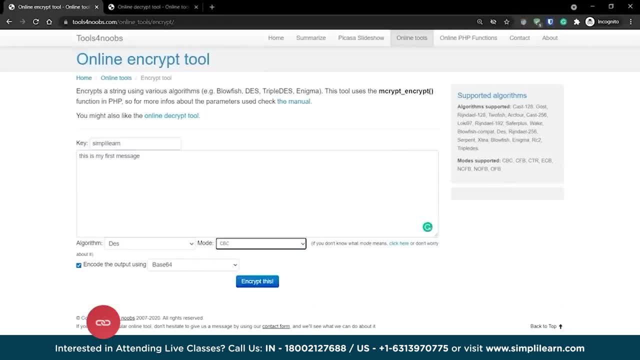 while we can see some other options here as well, Let's look at the CBC variant, which basically means the cipher block chaining method. One of CBC's key characteristics is that it uses a chaining process. It causes the decryption of our block of ciphertext to depend all on 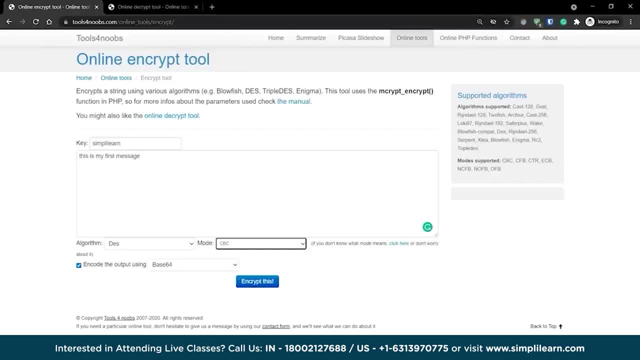 the preceding ciphertext blocks. As a result, the entire validity of all the blocks is contained in the previous adjacent blocks as well. A single bit error in a ciphertext block affects the decryption of all the subsequent blocks. Rearrangement of the order of these. 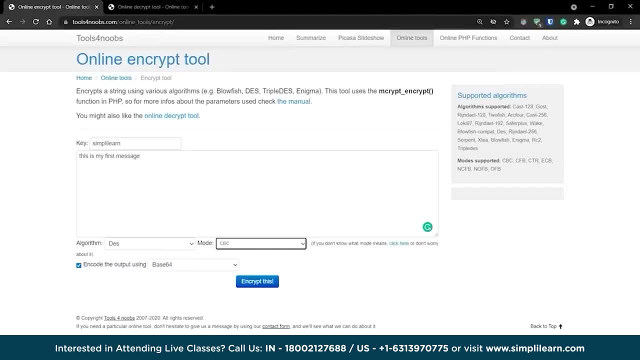 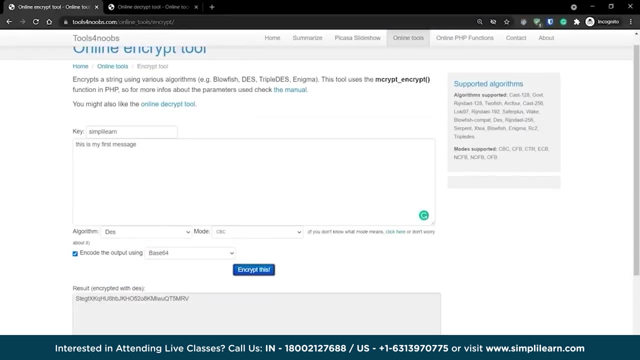 blocks, for example, can cause the decryption process to get corrupted. Regarding the manner of displaying binary information, we have two options here. We can either go with base64 or the hexadecimal format. Let's go with base64 right now, As you can see the ciphertext. 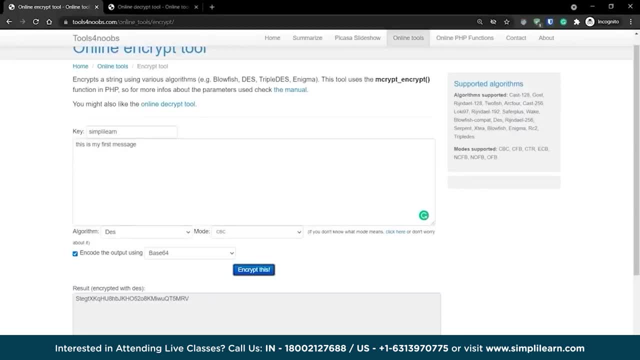 is readily available. Base64 is a little more efficient than hex, so we will be getting a smaller ciphertext when it comes to base64.. The size of both the formats will be the same. The hex has a longer ciphertext, since base64 takes 4 characters. 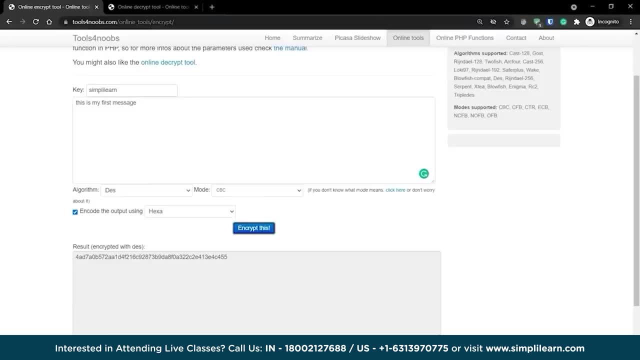 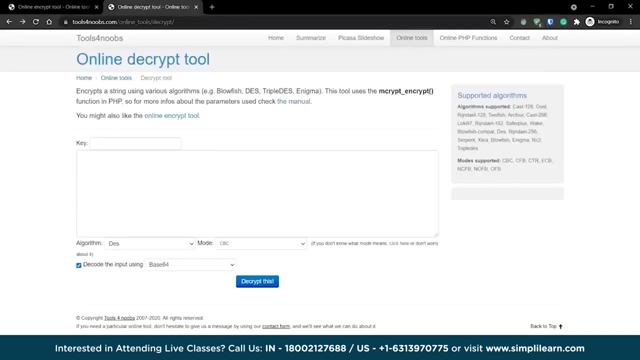 for every 3 bytes, while hex will take 2 characters for each byte. Hence base64 turns out to be more efficient. Now to decrypt the ciphertext, we go by the same format, Choose base64.. We copy the ciphertext onto our decryption tool and we have to. 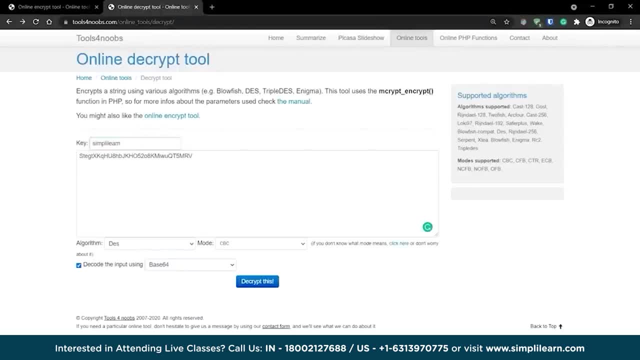 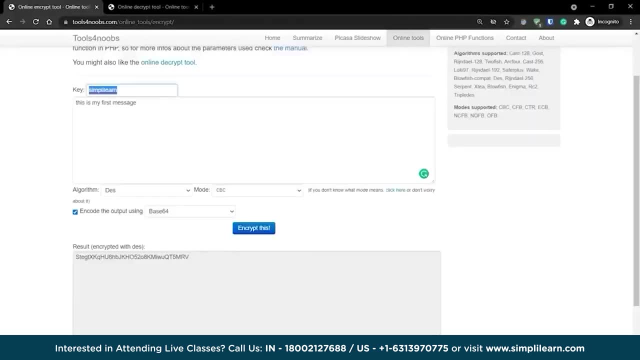 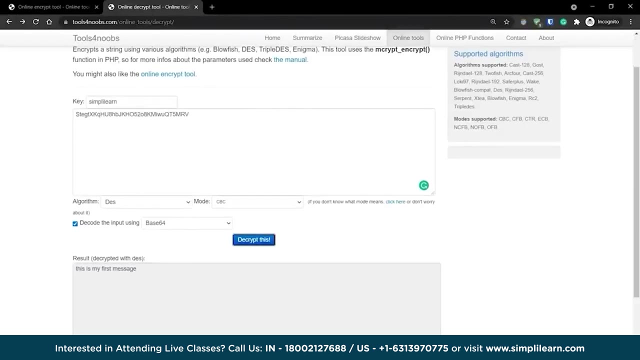 make sure that the key we are using is exactly the same. We choose similar mode of operation and we choose the correct encoding format as well, which is base64 in this case. As you can see, the decryption is complete and we get our plaintext back. 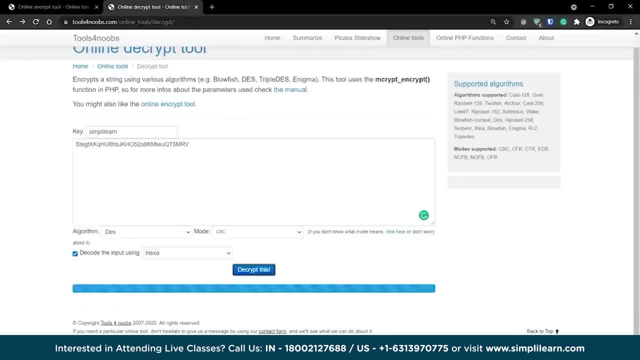 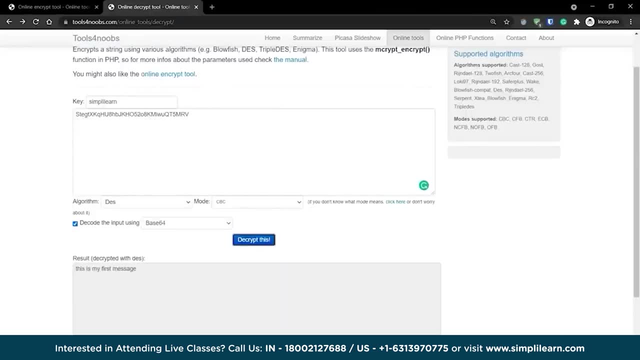 Even if we keep everything the same, but we just change the encoding format, it will not be able to decrypt anything. Unfortunately, DES has become rather easy to crack even without the help of a key. The advanced encryption standard is still on top when it comes to symmetric. 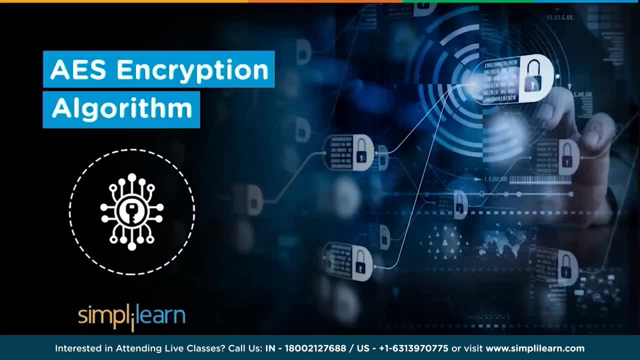 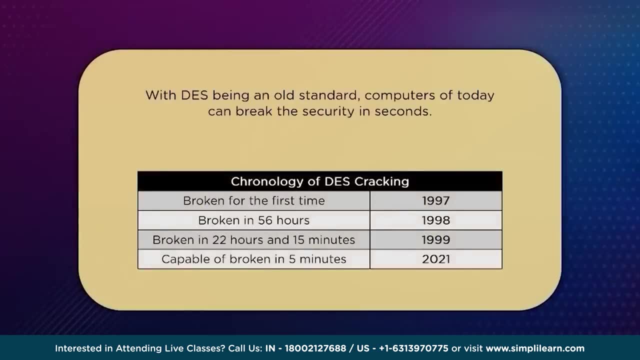 encryption security and will likely stay there for a while. Eventually, with so much computing power growth, the need for a stronger algorithm was necessary to safeguard our personal data. As solid as DES was, the computers of today could easily break the encryption with repeated attempts. 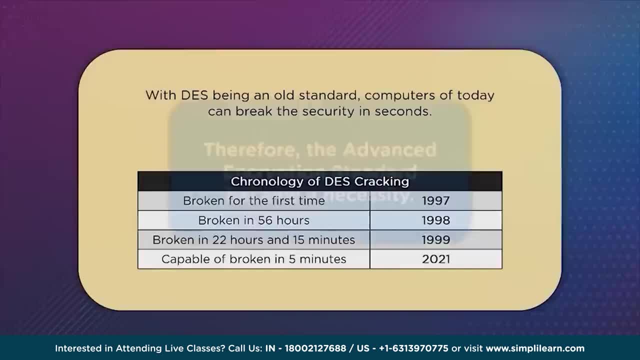 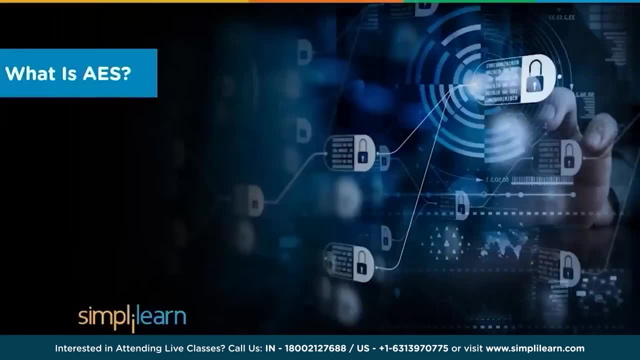 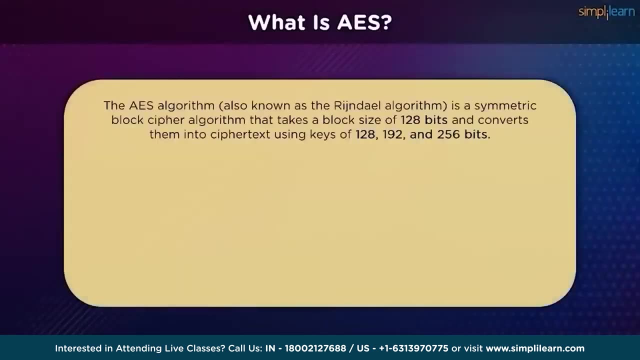 thereby rendering the data security helpless. To counter this dilemma, a new standard was introduced, which was termed as the Advanced Encryption Standard or the AES algorithm. Let's learn what is Advanced Encryption Standard, The AES algorithm, also known as the Rindahl algorithm. 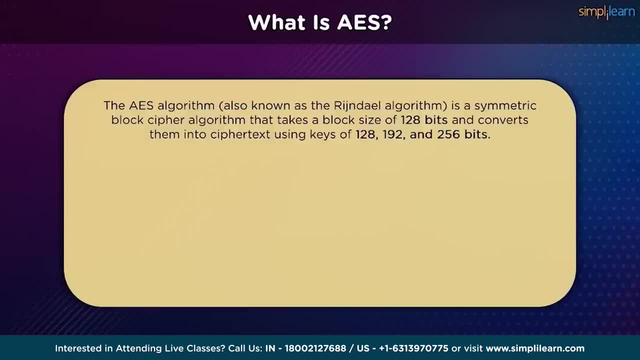 is a symmetric block cipher with a block size of 128 bits. It is converted into ciphertext using keys of 128,, 192, or 256 bits. It is implemented in software and hardware throughout the world to encrypt sensitive data. The National Institute of 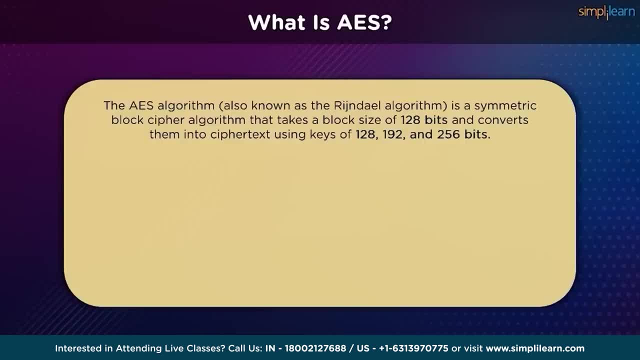 Standards and Technology, also known as NIST, started development on AES in 1997, when it was announced the need for an alternative to the data encryption standard. The new internet needed a replacement for DES because of its small key size With increasing computing power. 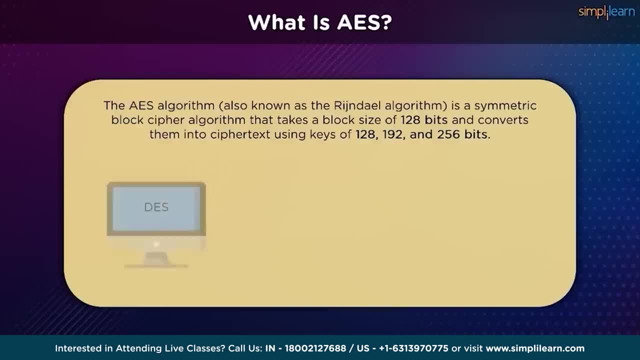 it was considered unsafe against entire key search attacks. The Triple DES was designed to overcome this problem. However, it was deemed to be too slow to be deployed in machines worldwide. Strong cases were present by the Mars, RC6, Serpent and the Two Fish algorithms, but 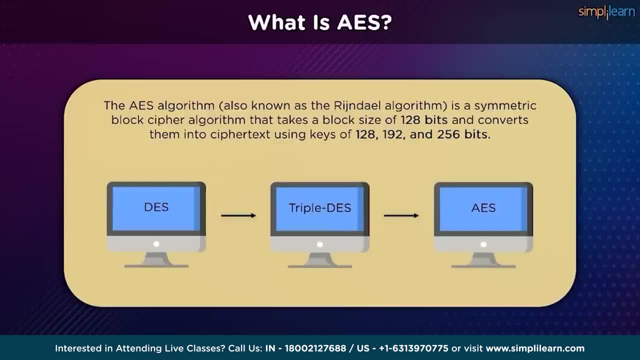 it was the Rindahl Encryption Algorithm, also known as AES, which was eventually chosen as the standard symmetric key encryption algorithm to be used. Its selection was formalized with the release of Federal Information Processing Standards publication 197 in the November of 2001.. 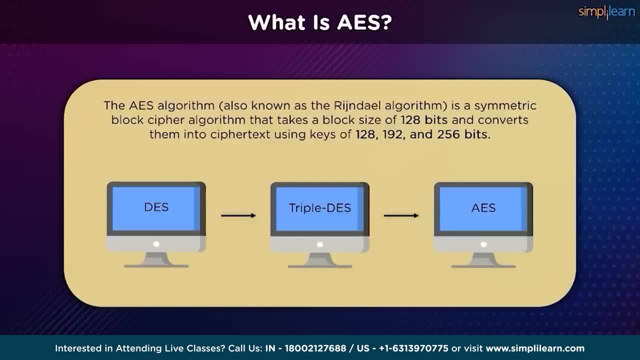 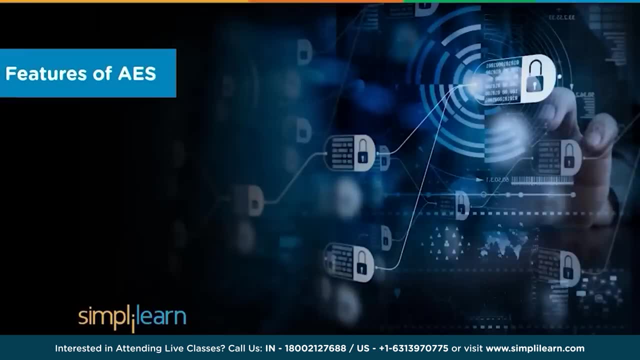 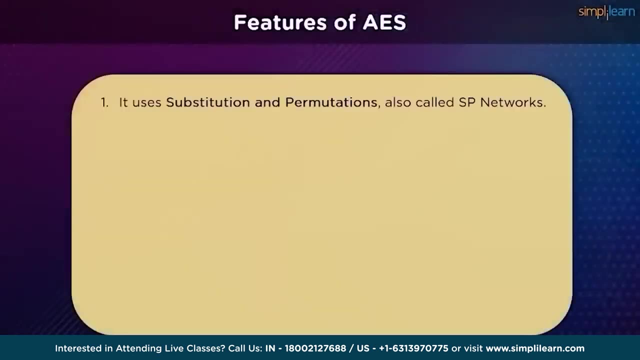 It was approved by the US Secretary of Commerce. Now that we understand the origin of AES, let us have a look at the features that make the AES encryption algorithm unique. The AES algorithm uses a substitution permutation or SP network. It consists of multiple rounds to produce a 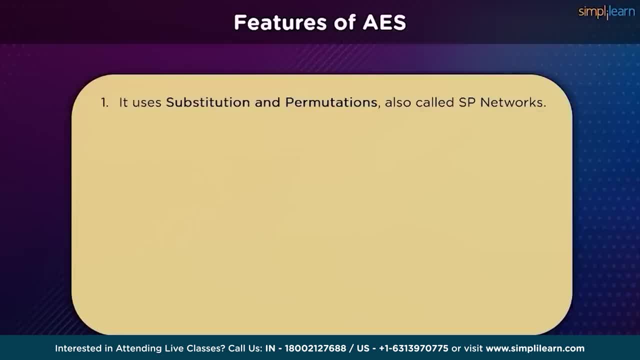 ciphertext. It has a series of linked operations, including replacing inputs with specific outputs, that is, substitutions, and others that involve bit shuffling, which is permutations. At the beginning of the encryption process, we only start out with a single key, which can be either: 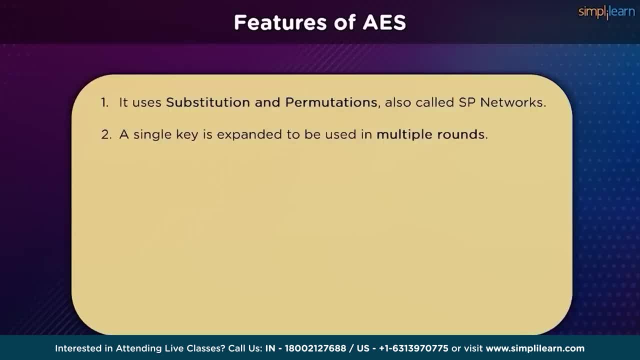 a 128-bit key, a 192-bit key or a 256-bit key. Eventually, this one key is expanded to be used in multiple rounds throughout the encryption and the decryption cycle. Interestingly, AES performs all its calculations on byte data instead of bit data. 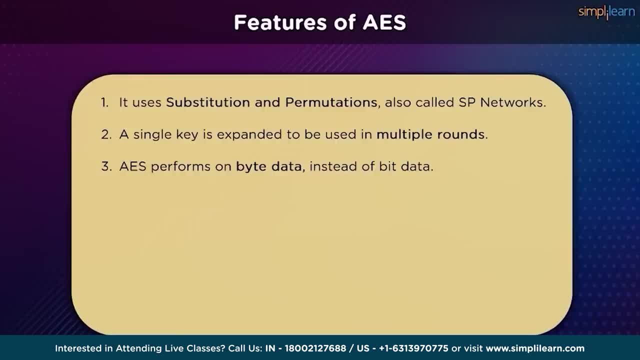 as seen in the case of the DES algorithm. Therefore, AES treats 128 bits of a clear text block as 16 bytes. The number of rounds during the encryption process depends on the key size that is being used, The 128-bit key size. 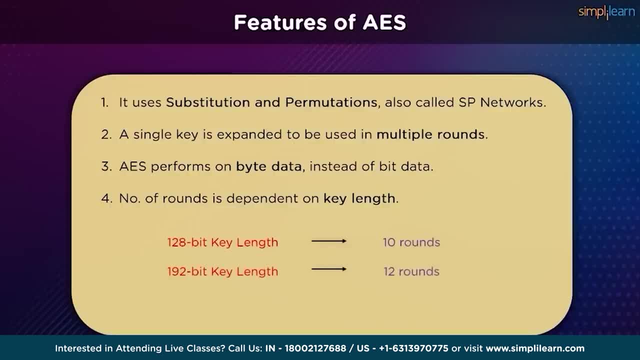 fixes 10 rounds. the 192-bit key size fixes 12 rounds and the 256-bit key holds 14 rounds. A round key is required for each of these rounds, but since only one key is input into the algorithm, the single. 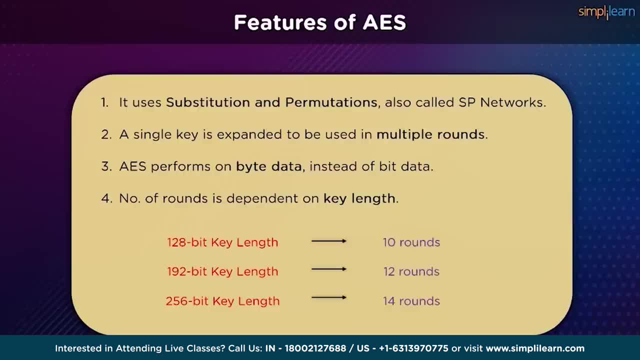 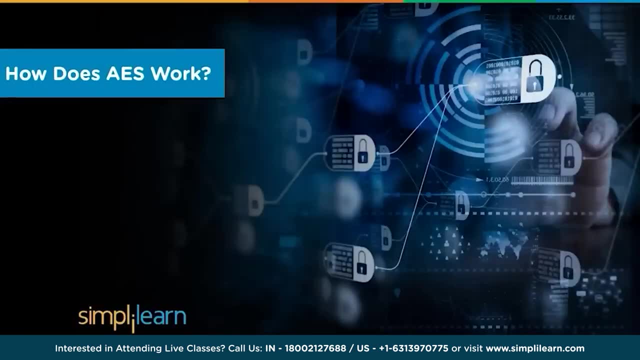 key needs to be expanded to get the key for each round, including the round 0.. With so many mathematical calculations going on in the background, there are bound to be a lot of steps throughout the procedure. Let's have a look at the steps followed in AES. 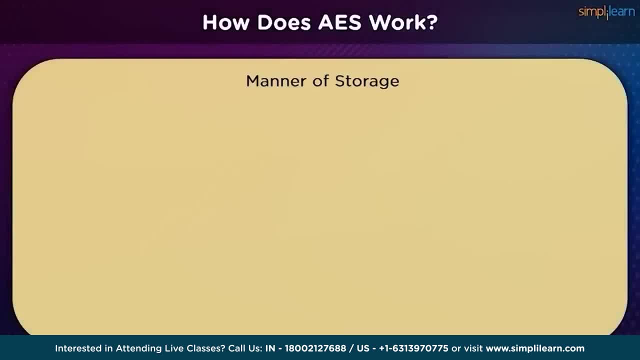 Before we move ahead, we need to understand how data is being stored during the process of AES encryption. Everything in the process is stored in a 4x4 matrix format. This matrix is also known as a state array, and we'll be using 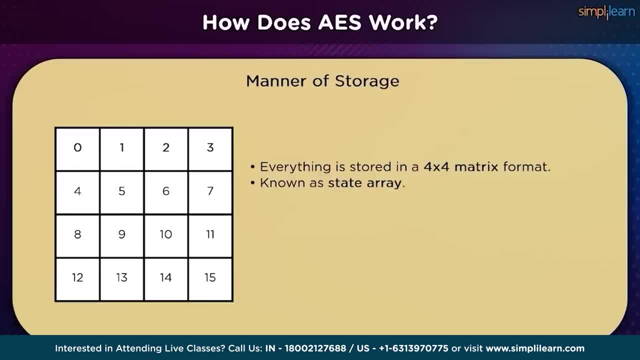 these state arrays to transmit data from one step to another and from one round to the next round. Each round takes state array as an input and gives a state array as output to be transferred to the next round. It is a 16 byte matrix with. 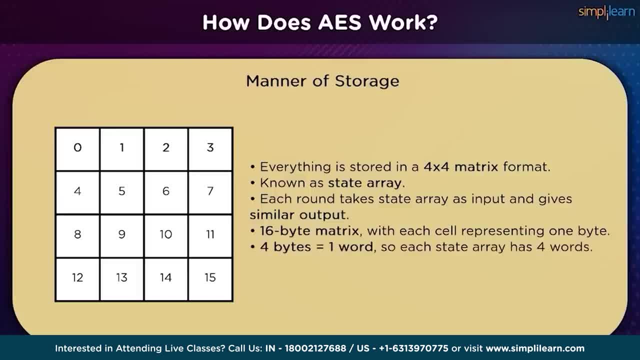 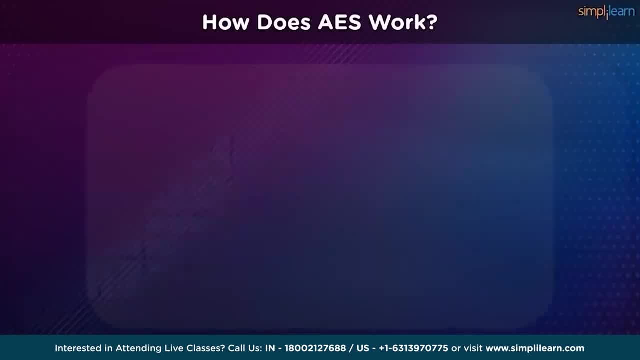 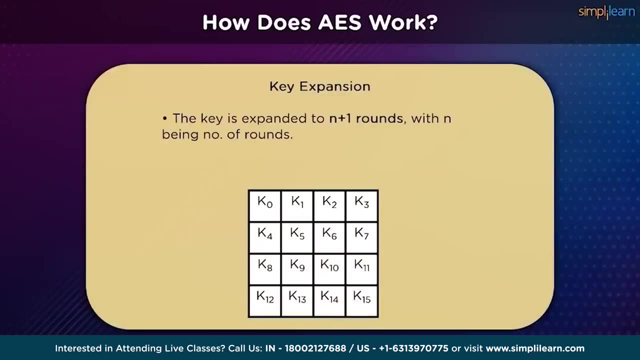 each cell representing 1 byte, with each 4 bytes representing a word. So every state array will have a total of 4 words representing it. As we previously discussed, we take a single key and expand it to the number of rounds that we need the key to be used in. 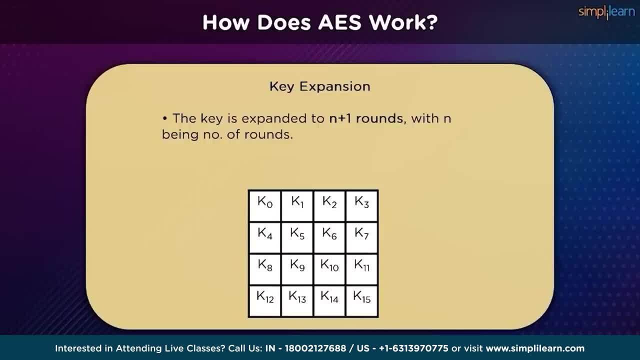 Let's say the number of rounds are n, then the key has to be expanded to be used with n plus 1 rounds, because the first round is the key 0 round. Let's say n is the number of rounds. The key is expanded to n plus. 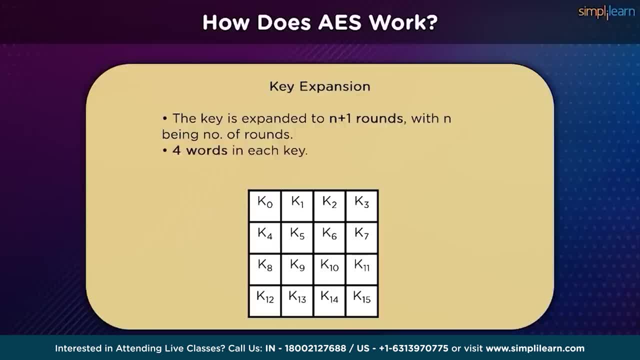 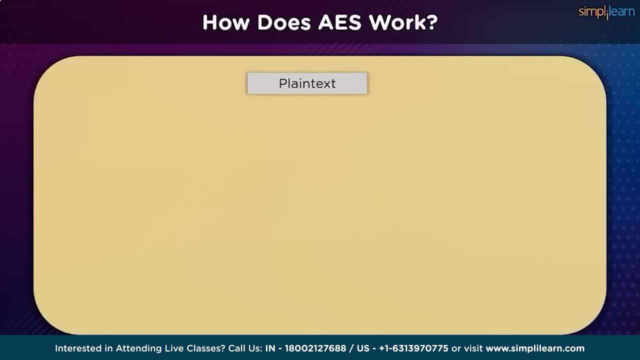 1 rounds. It is also a state array having 4 words in its vicinity. Every key is used for a single round and the first key is used as a round key. before any round begins, In the very beginning, the print text is captured and passed through an XOR function. 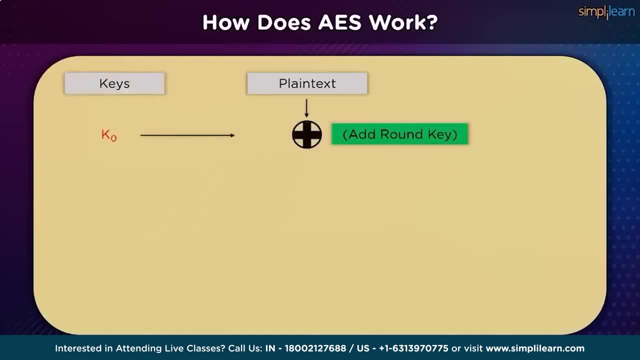 with the round key as a supplement. This key can be considered the first key from the n plus 1 expanded set. Moving on, the state array resulting from the above step is passed on to a byte substitution process. Beyond that there is a. 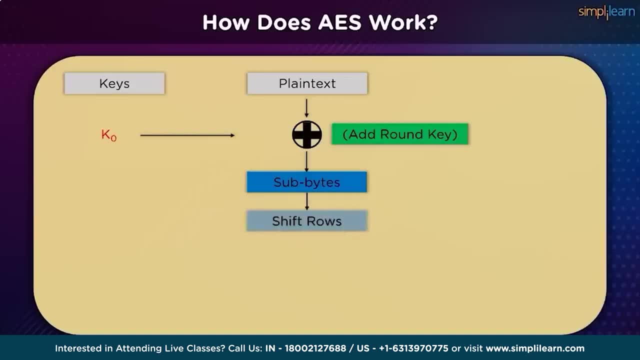 provision to shift rows in the state arrays. Later on, the state array is mixed with a constant matrix to shuffle its column in the mixed column segment, after which we add the round key for that particular round. The last four steps mentioned are part of. 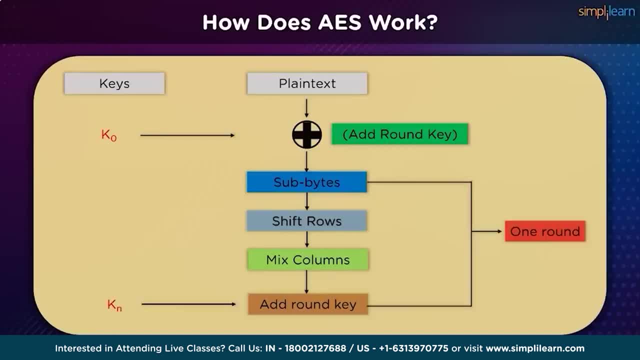 every single round that the encryption algorithm goes through. The state arrays are then passed from one round to the next as an input. In the last round, however, we skip the mixed columns portion, with the rest of the process remaining unchanged. But what are these byte? 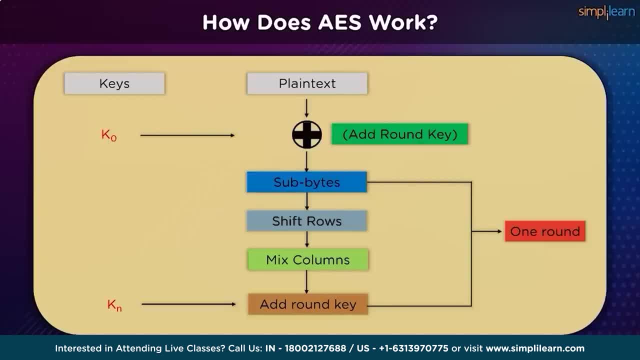 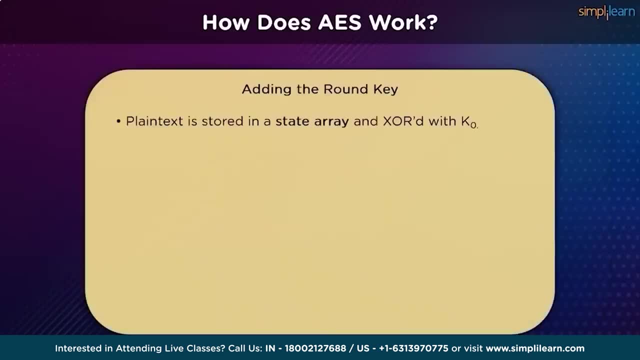 substitution and row shifting processes. Let's find out regarding each step in more detail. In the first step, the plaintext is stored in a state array and it is XORed with the K0,, which is the first key in the expanded key set. 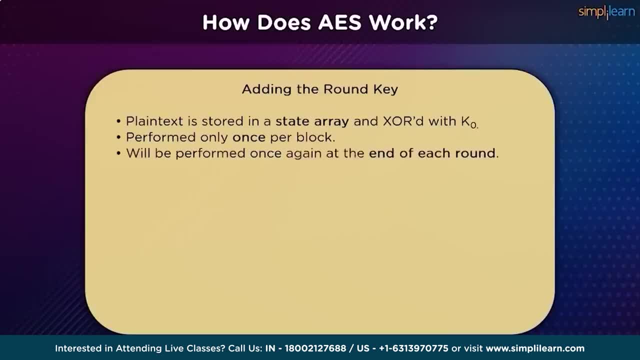 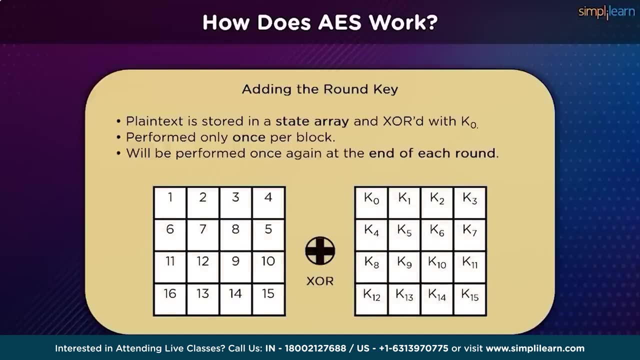 This step is performed only once on a block, while being repeated at the end of each round as per iteration demands. The state array is XORed with the key to get a new state array, which is then passed over as input to the sub bytes process. 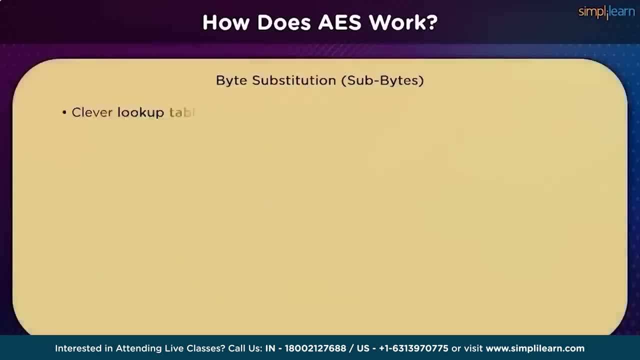 In the second stage we have byte substitution. We leverage an X box called as a substitution box to randomly switch data among each element. Every single byte is converted into a hexadecimal value having two parts. The first part denotes the row value and the second part denotes 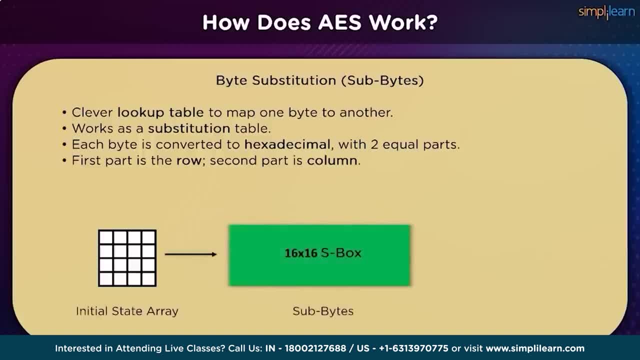 the column value, The entire state array is passed through the X box to create a brand new state array, which is then passed off as an input to the row shifting process. The 16 input bytes are replaced by looking at a fixed table given in the design. 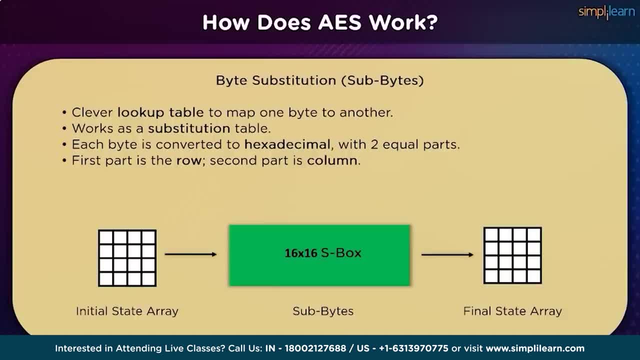 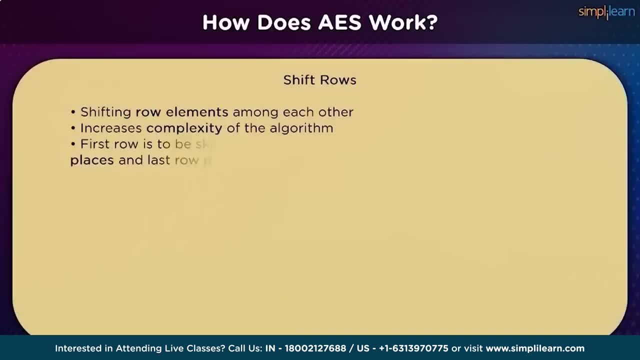 We finally get a matrix with 4 rows and 4 columns. When it comes to row shifting, each bit in the 4 rows of the matrix is shifted to the left. An entry that is a falloff is reinserted to the right of the line. The change 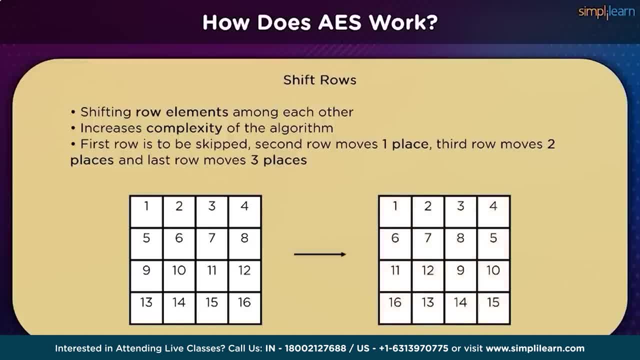 is done as follows: The first line is not moved in any way, The second line is shifted to a single position to the left, The third line is shifted 2 positions to the left and the fourth line is shifted 3 positions to the left. 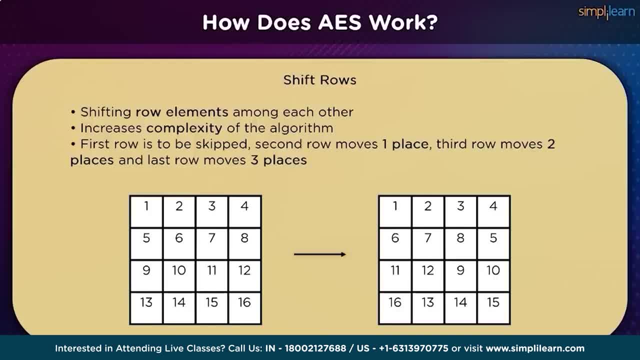 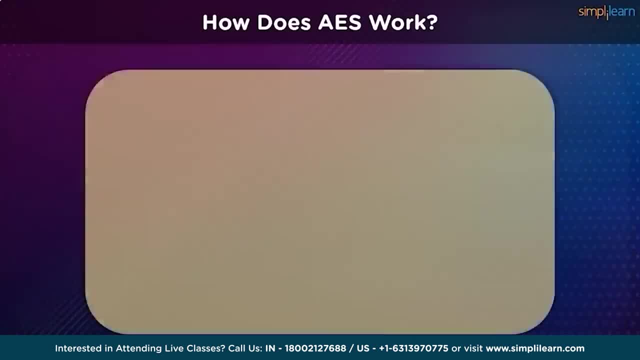 The result is a new matrix that contains the same 16 bytes but has been moved in relation to each other to boost the complexity of the program. In mixed columns, each column of 4 bytes is now replaced using a special mathematical function. The function takes: 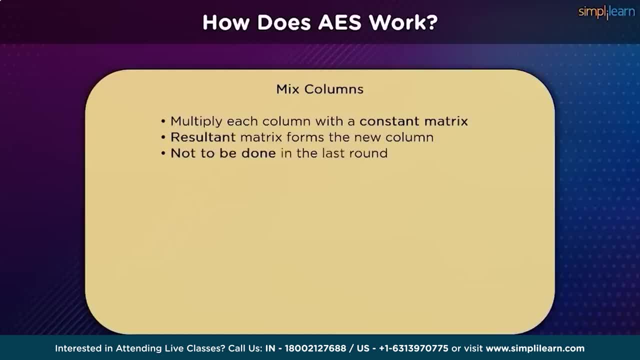 4 bytes of a column as input and outputs 4 completely new bytes. We will get a new matrix with the same size of 16 bytes, and it should be noted that this phase has not been done in the last round of the iteration. 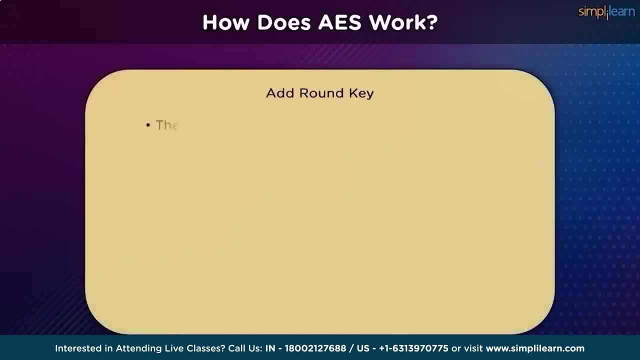 When it comes to adding a round key, the 16 bytes of the matrix are treated as 128 bits, and the 128 bits of the round key are XORed. If it is the last round, the output is the ciphertext. If we still have a few rounds, 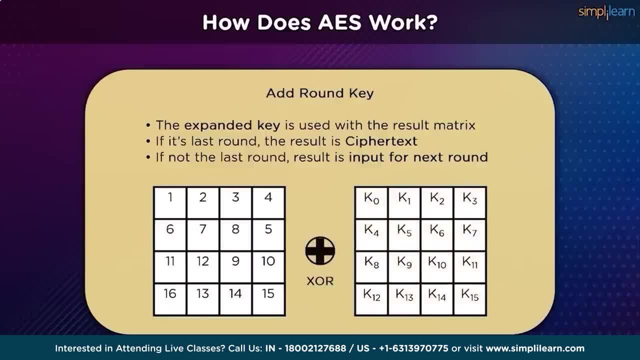 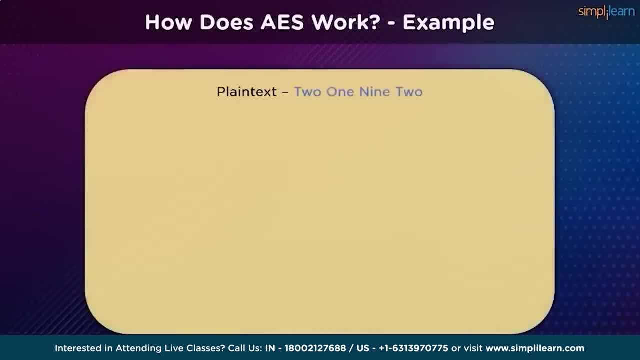 remaining. the resulting 128 bits are interpreted as 16 bytes and we start another similar round. Let's take an example to understand how all these processes work. If our plaintext is the string 2192,, we first convert it into a hexadecimal format. 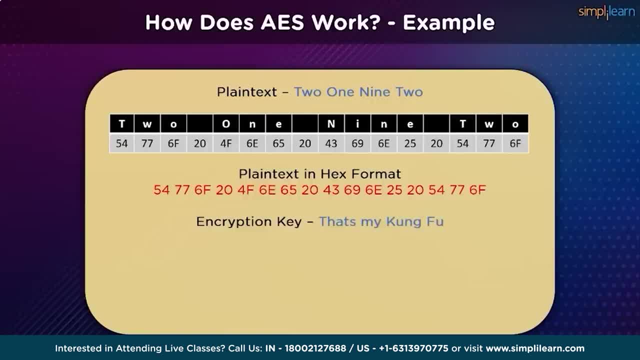 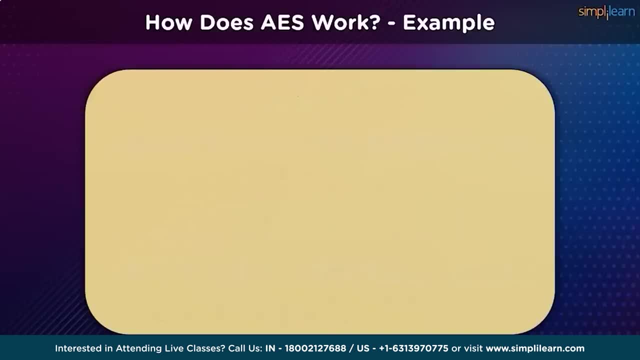 as follows: We use an encryption key, which is that's my kung fu, and it is converted into a hexadecimal format as well. As per the guidelines, we use a single key, which is then later expanded into n plus 1 number of keys. 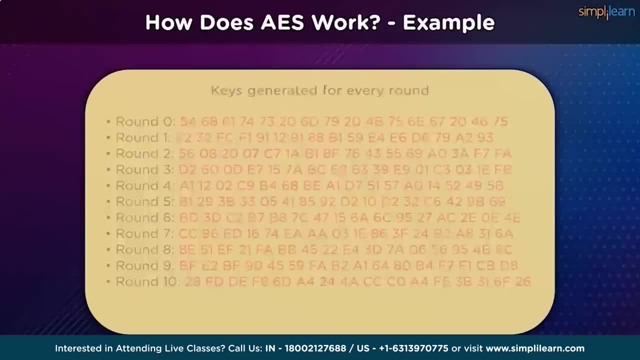 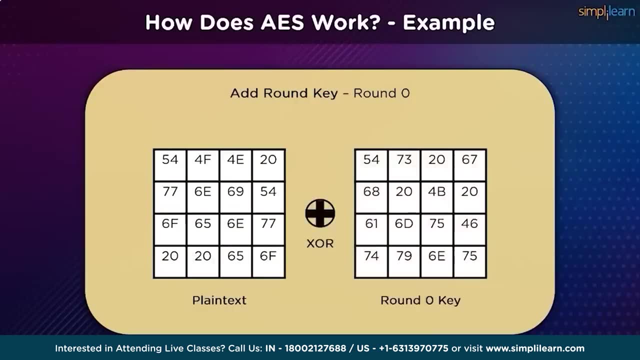 in which case it's supposed to be 11 keys for 10 different rounds. In round 0, we add the round key, the plaintext is XORed with the k0, and we get a state array that is passed off as an input. 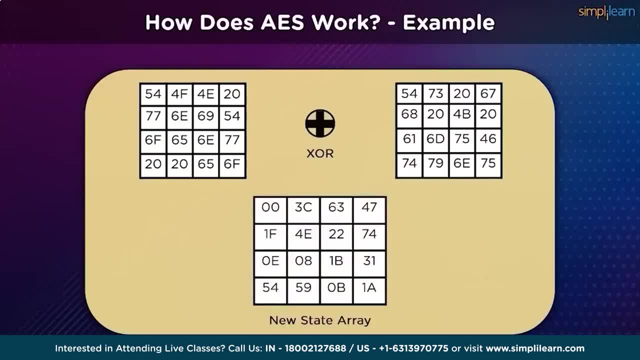 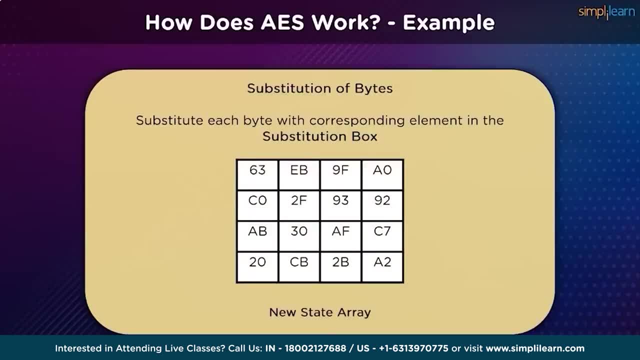 to the substitution bytes process. When it comes to the substitution bytes process, we leverage an S box to substitute the elements of each byte with a completely new byte. This way, the state array that we receive is passed off as an input to the row shifting process. 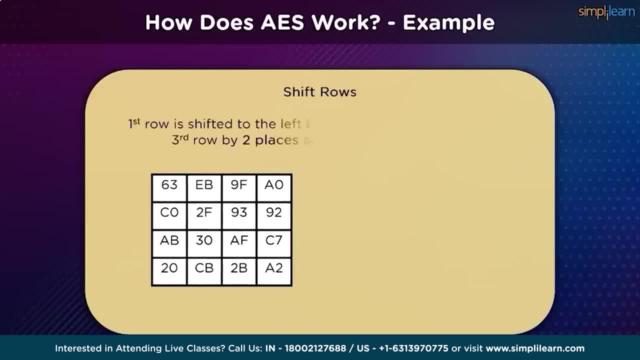 on the next step When it comes to row shifting, each element is shifted a few places to the left, with the first row being shifted by 0 places, second row by 1 place, third row by 2 places and the last by 3.. 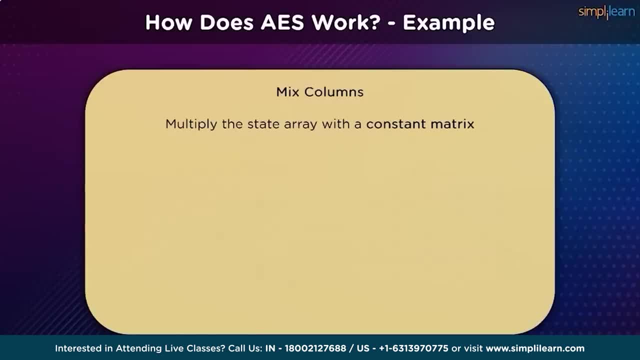 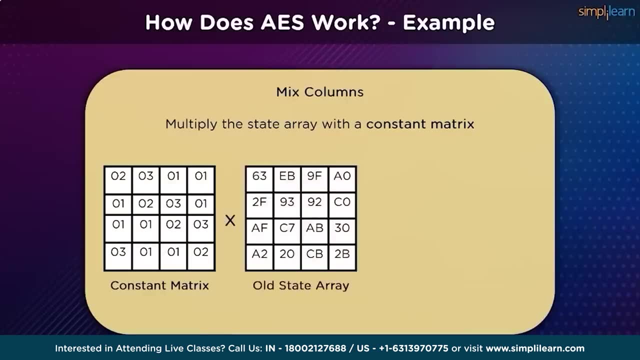 The state array that we received from the row shifting is passed off as an input to mixed columns. In mixed columns, we multiply the state array with a constant matrix, after which I receive a new state array to be passed on to the next step. 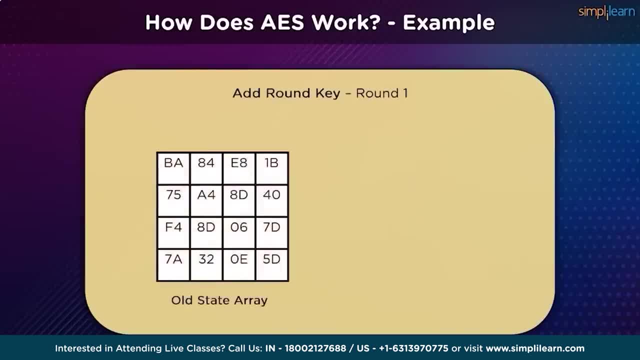 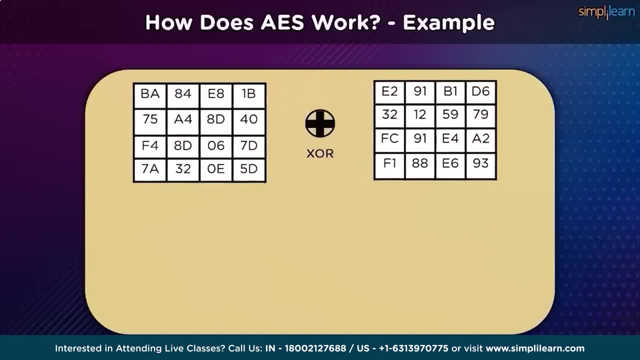 We add the new state array as an XOR with the round key of the particular iteration. Whatever state array we receive here, it becomes an output for this particular round. Now, since this is the first round of the entire encryption process, the state array that we receive: 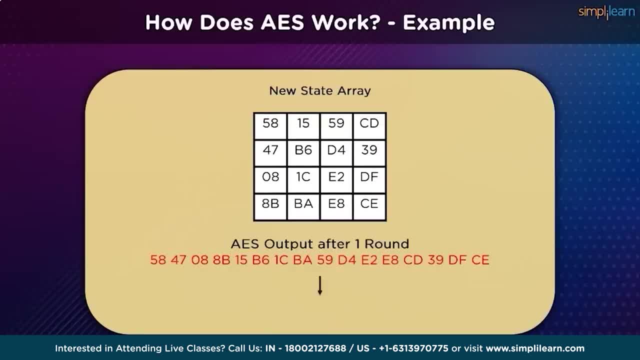 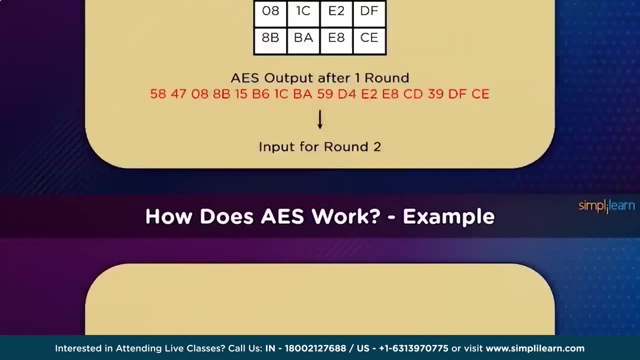 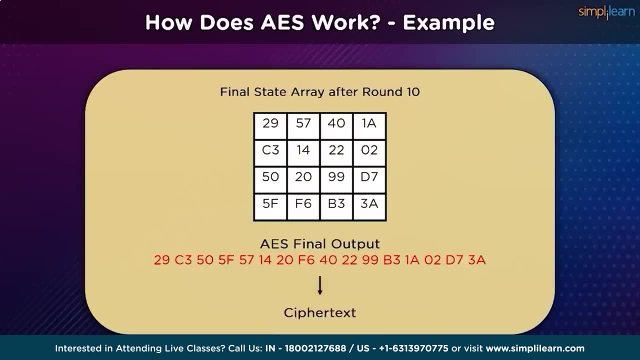 is passed off as an input to the new round. We repeat this process for 10 more rounds and we finally receive our final ciphertext. Once the final state array can be denoted in the hexadecimal format, this becomes our final ciphertext that we can use for transferring information. 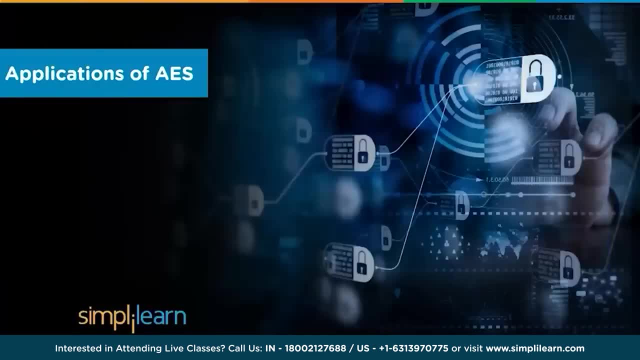 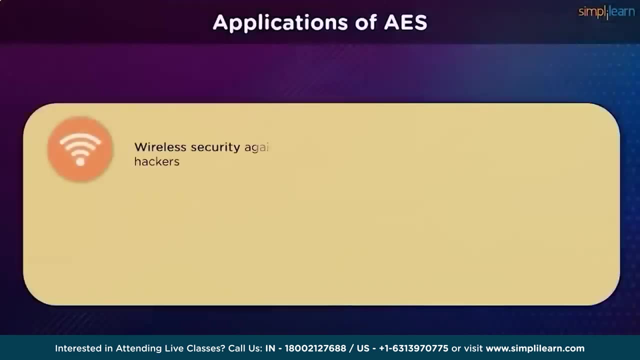 from the sender and receiver. Let's take a look at the applications of AES in this world. AES finds most use in the area of wireless security in order to establish a secure mode of authentication between routers and clients- Highly secure mechanisms like WPA and WPA2-PSK. 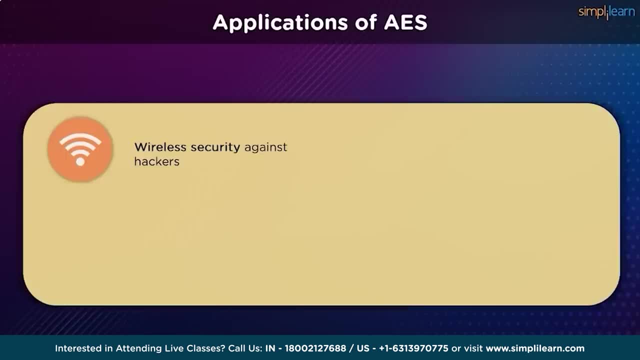 are extensively used in securing Wi-Fi endpoints. with the help of Rindahl's algorithm, It also helps in SSL TLS encryption that is instrumental in encrypting our internet browser sessions. AES works in tandem with other asymmetric encryption algorithms to make sure the web browser and 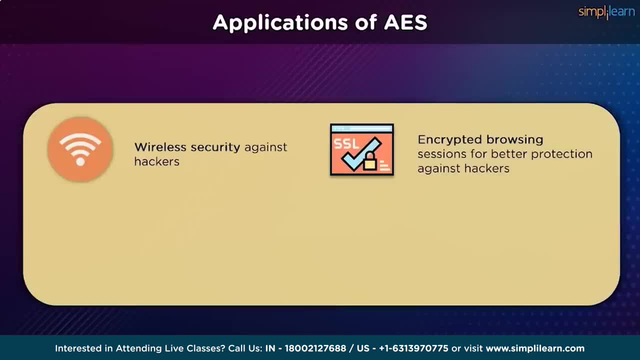 web server are properly configured and use encrypted channels for communication. AES works in tandem with other AES is also prevalent in general file encryption of various formats, ranging from critical documents to the media files. Having a large key allows people to encrypt media and decrypt data with maximum. 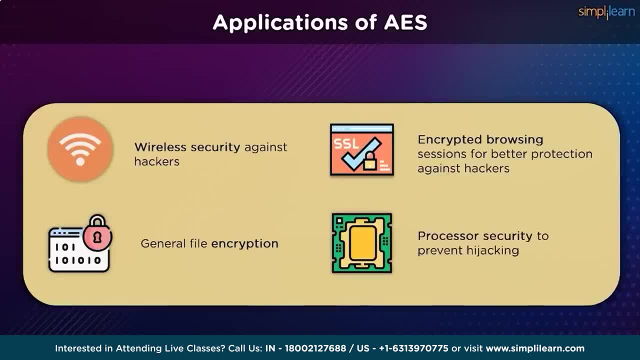 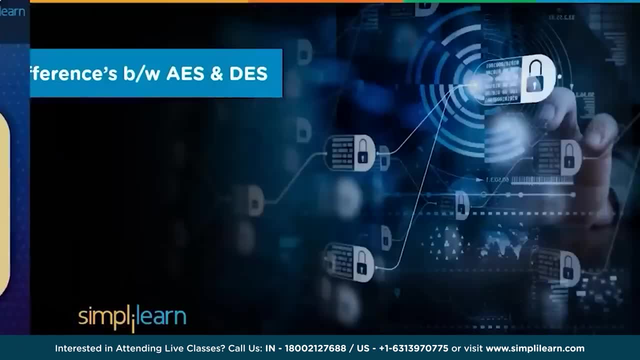 security possible. AES is also used for processor security in hardware appliances to prevent machine hijacking, among other things. As a direct successor to the DES algorithm. there are some aspects that AES provides an immediate advantage in. Let us take a look When it comes to key length. 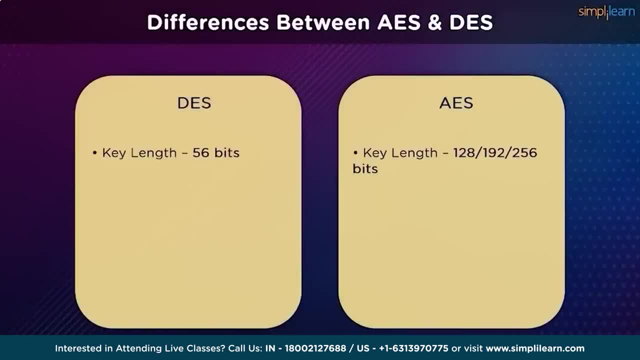 the biggest flaw in DES algorithm was its small length was easily vulnerable by today's standards. AES has managed to nab up 128,, 192 and 256 bit key lengths to bolster the security further. The block size is also larger in AES owing to more complexity of the algorithm. 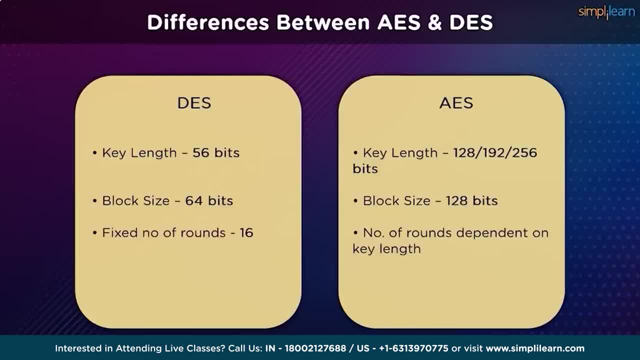 The number of rounds in DES is fixed irrespective of the plain text being used. In AES, the number of rounds depends on the key length that is being used for the particular iteration, thereby providing more randomness and complexity in the algorithm. The DES algorithm is considered to be simpler than AES. 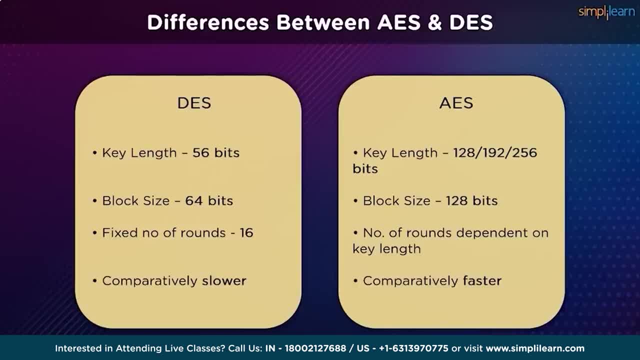 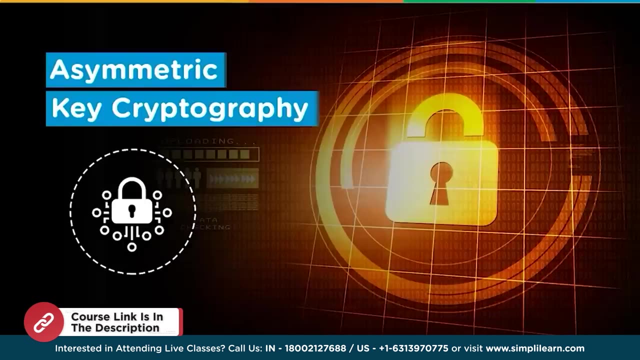 even though AES beats DES when it comes to relative speed of encryption and decryption. This makes advanced encryption standard much more streamlined to be deployed in frameworks and systems worldwide when it compares to the data encryption standard. Hello, in our last video on cryptography, we took a look at 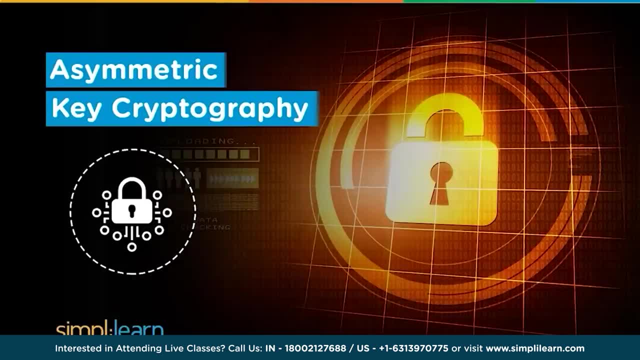 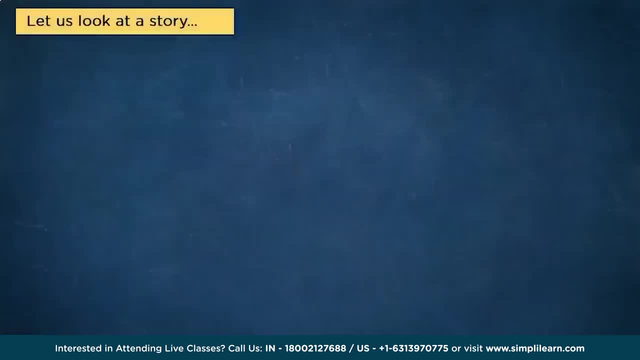 symmetric key cryptography. We used a single private key for both the encryption and decryption of data and it works very well in theory. Let's take a look at a more realistic scenario now. Let's meet Joe. Joe is a journalist who needs to communicate with Ryan. 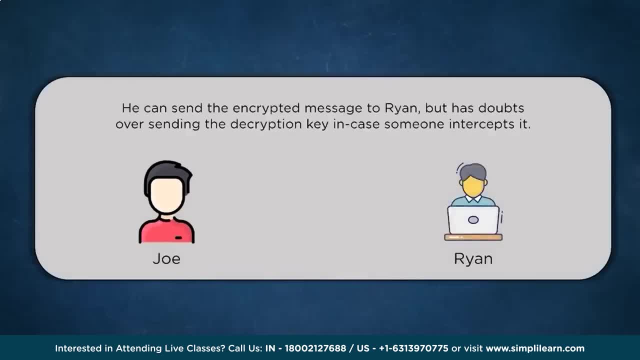 via long distance messaging Due to the critical nature of the information. people are waiting for any message to leave Joe's house so that they can intercept it. Now Joe can easily use symmetric key cryptography to send the encrypted data so that, even if someone intercepts the message, 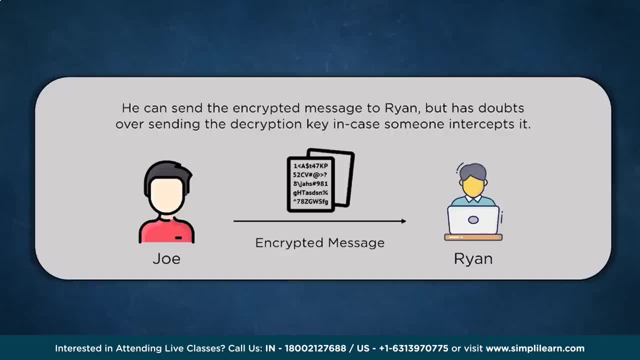 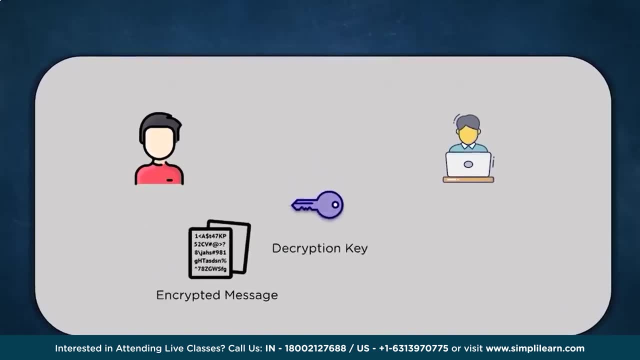 they cannot understand what it says. But here's the tricky part: How will Joe send the required decryption key to Ryan? The sender of the message as well as the receiver need to have the same decryption key so that they can exchange messages. Otherwise Ryan cannot decrypt. 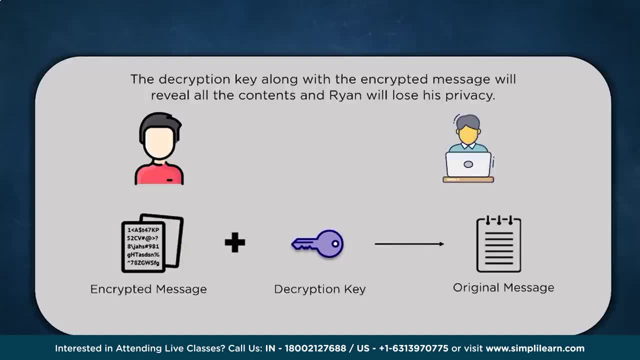 the information even when he receives the ciphertext. If someone intercepts the key while transmitting it, there is no use in employing cryptography, and so third party can now decode all the information easily. Key sharing is a risk that will always exist when symmetric key cryptography is being used. 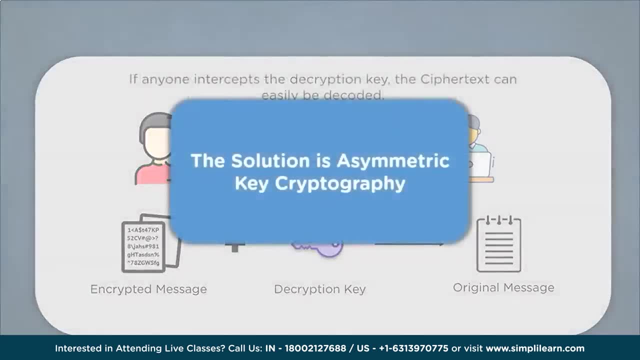 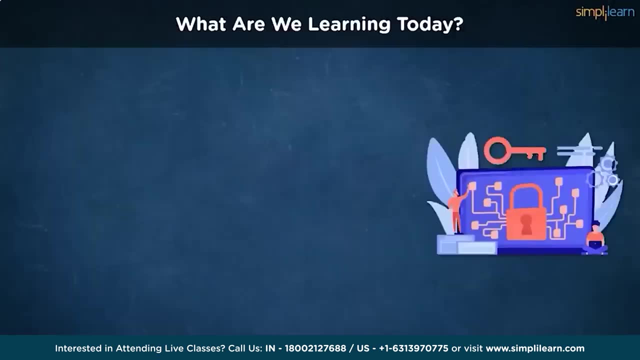 Thankfully, asymmetric key encryption has managed to fix this problem. This is Babab from SimplyLearn, and welcome to this video on asymmetric key cryptography. Let's take a look at what we are going to learn today. We begin by explaining what asymmetric key cryptography is. 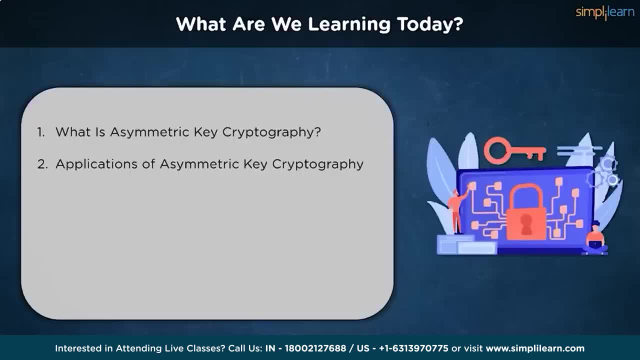 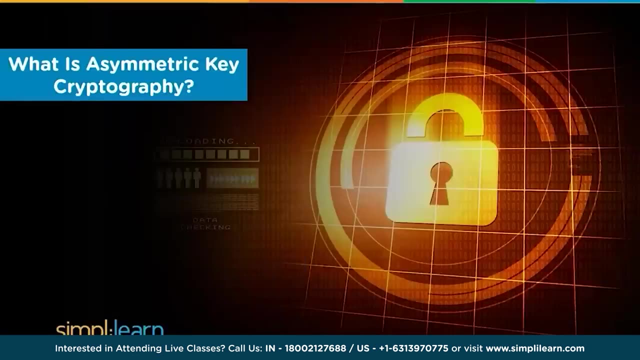 and how it works. We take a look at its application and uses. we understand why it's called public key cryptography, and then learn a little bit about RSA encryption. and then we learn about the advantages of asymmetric key cryptography over symmetric key cryptography. Let's understand. 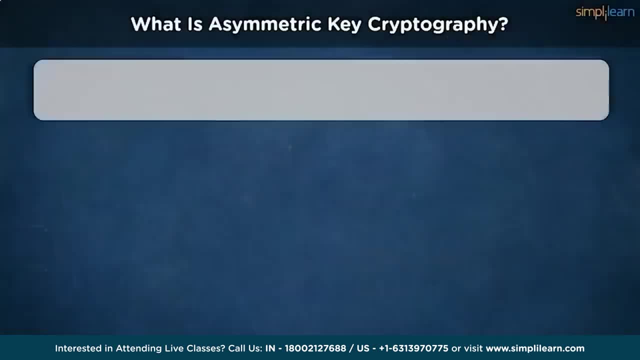 what asymmetric key cryptography is. Asymmetric encryption uses a double layer of protection. There are two different keys at play here: a private key and a public key. A public key is used to encrypt the information pre-transit and a private key is used to decrypt. 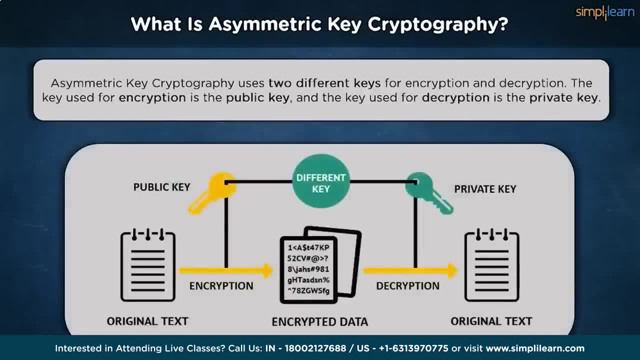 the data post-transit. These pair of keys must belong to the receiver of the message. The public keys can be shared via messaging, blog posts or key servers and there are no restrictions. As you can see in the image, the two keys are working in the system. 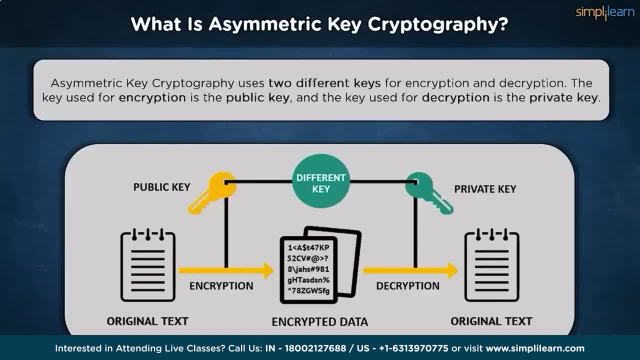 The sender first encrypts the message using the receiver's private key, after which we receive the ciphertext. The ciphertext is then transmitted to the receiver without any other key. On getting the ciphertext, the receiver uses the private key to decrypt it and get the plaintext back. There has been 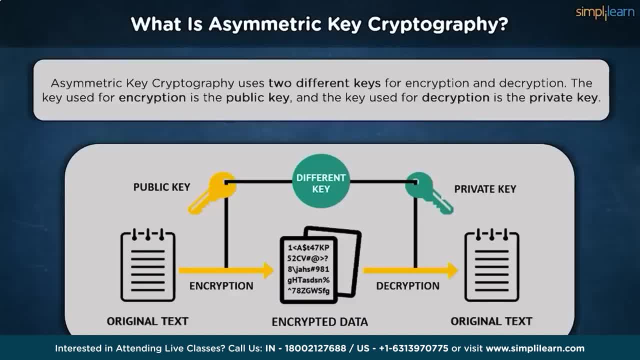 no requirement of any key exchange throughout this process, therefore solving the most glaring flaw faced in symmetric key cryptography: The public key, known to everyone, cannot be used to decrypt the message, and the private key, which can decrypt the message, need not be shared with anyone. 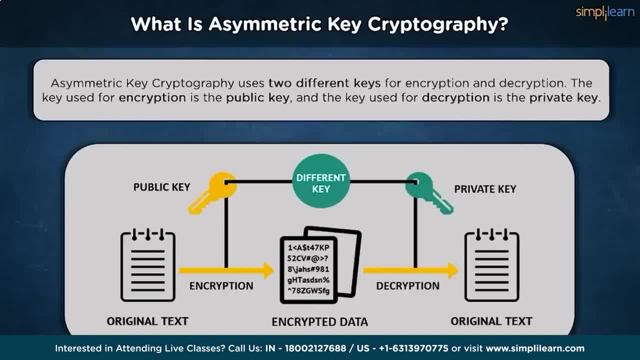 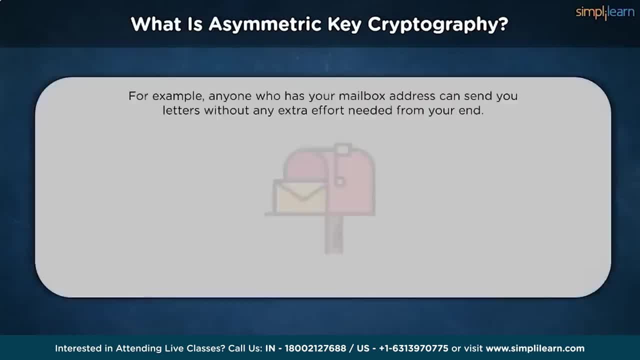 The sender and receiver can exchange personal data using the same set of keys as often as possible. To understand this better, take the analogy of your mailbox. Anyone who wants to send you a letter has access to the box and can easily share information with you In a way. 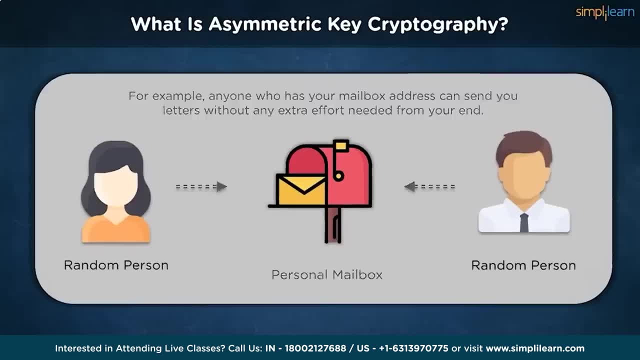 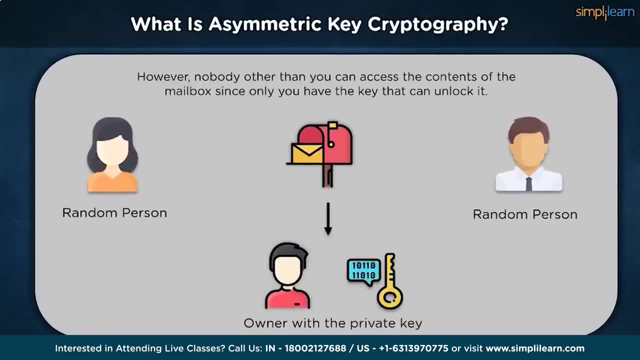 you can say: the mailbox is publicly available to all, but only you have access to the key that can open the mailbox and read the letters in it. This is how the private key comes to play. No one can intercept the message and read its contents. 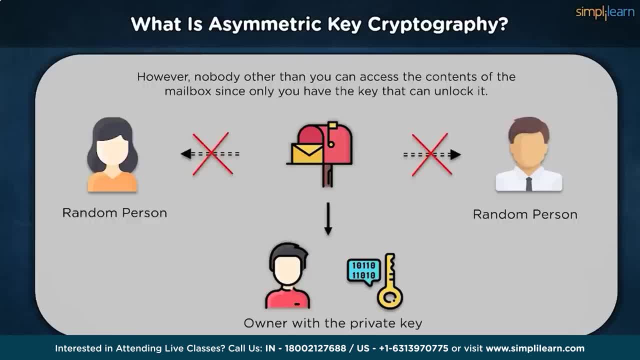 since it's encrypted, Once the receiver gets its contents, he can use his private key to decrypt the information. Both the public key and the private key are generated so they are interlinked and you cannot substitute other private keys to decrypt the data In another example. 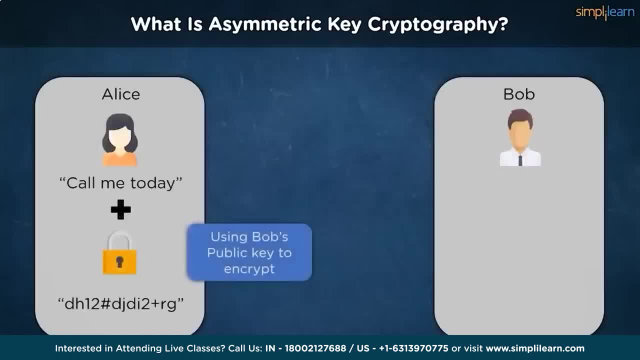 if Alice wants to send a message to Bob, let's say it reads: call me today- she must use Bob's public key while encrypting the message. Upon receiving the cipher message, Bob can proceed to use his private key in order to decrypt the message. 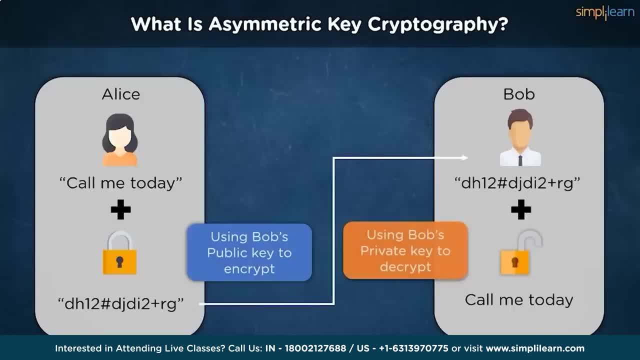 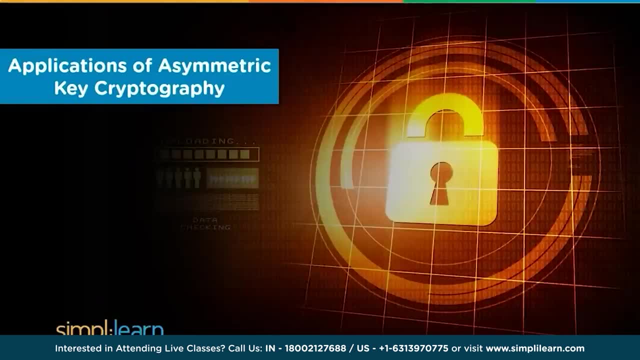 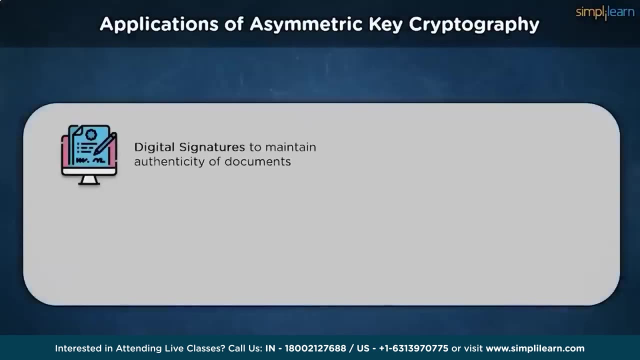 and hence complete security is attained during transmission without any need for sharing the key. Since this type of encryption is highly secure, it has many uses in areas that require high confidentiality. It is used to manage digital signatures, so there is valid proof of a document's authenticity. 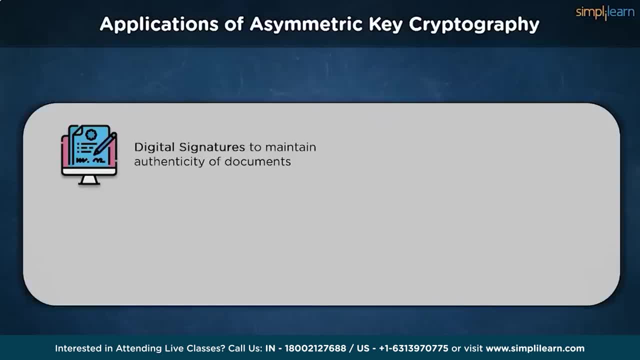 With so many aspects of business transitioning to the digital sphere, critical documents need to be verified before being considered authentic and acted upon. Thanks to asymmetric cryptography, senders can now sign documents with their private keys. Anyone who needs to verify the authenticity of such signatures can use the sender's 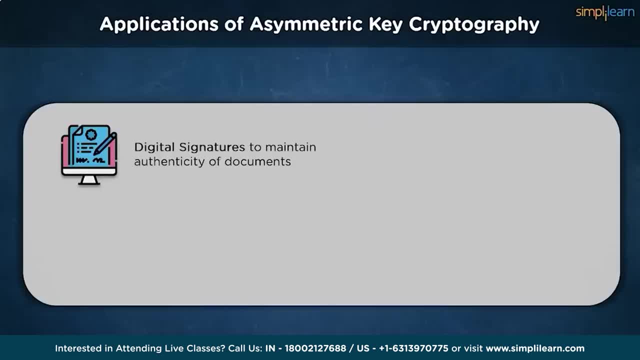 public key to decrypt the signature. Since the public and the private keys are linked to each other mathematically, it's impossible to repeat this verification with duplicate keys. Document encryption has been made very simple by today's standards, but the background implementation follows a similar approach. 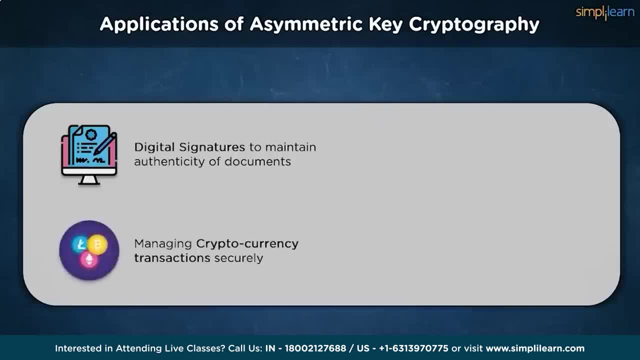 In blockchain architecture, asymmetric key cryptography is used to authorize transactions and maintain the system. Thanks to its two key structures. changes are reflected across the blockchain and its peer-to-peer network only if it is approved from both ends, Along with asymmetric key cryptography's. 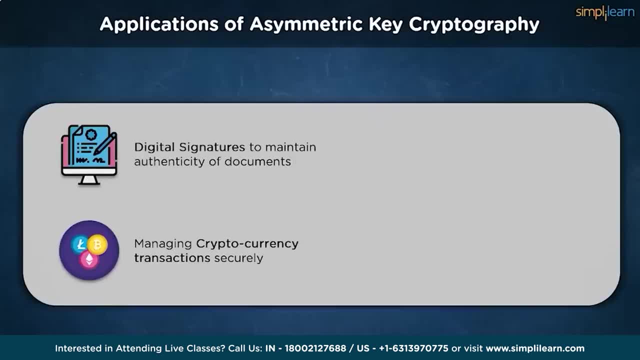 tamper-proof architecture. its non-repudiation characteristic also helps in keeping the network stable. We can also use asymmetric key cryptography combined with symmetric key cryptography to monitor SSL or TLS encrypted browsing sessions to make sure nobody can steal up personal information when accessing. 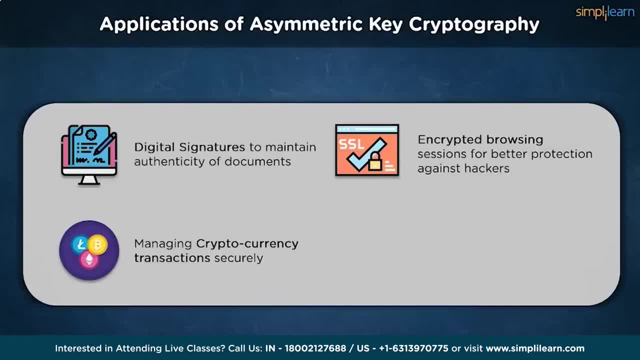 banking websites or the internet in general. It plays a significant role in verifying websites' authenticity, exchanging the necessary encryption keys required and generating a session using those keys to ensure maximum security, instead of the rather insecure HTTP website format. Security parameters differ on a session-by-session. 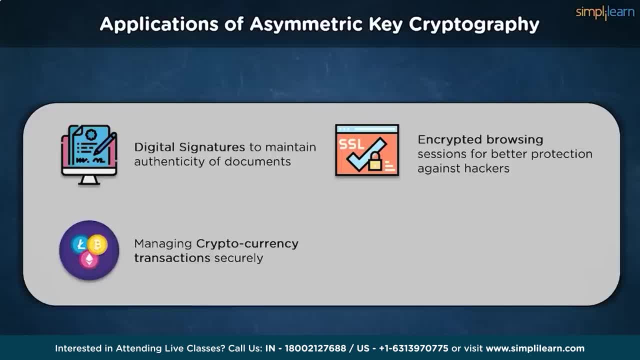 basis, so the verification process is consistent and utterly essential to modern data security. Another great use of the asymmetric key cryptography structure is transmitting keys for symmetric key cryptography, With the most significant difficulty in symmetric encryption being key exchange. asymmetric keys can help clear this shortcoming. 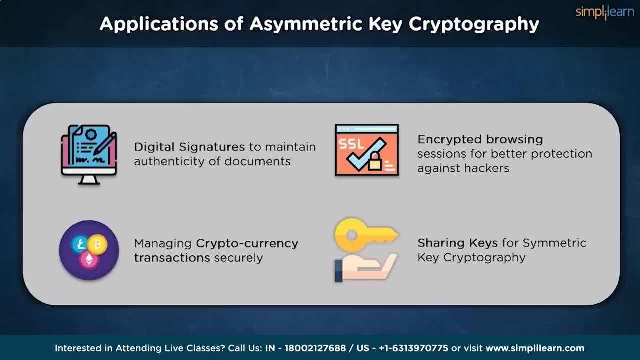 The original message is first encrypted using a symmetric key. The key used for encrypting the data is then converted into the ciphertext using the receiver's public key. Now we have two ciphertexts to transmit to the receiver. On receiving both of them, the receiver uses his private key. 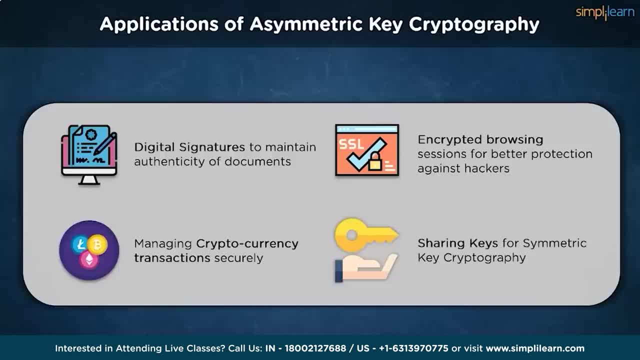 to decrypt the symmetric key. He can then use it to decrypt the original information on getting the key used to encrypt the data. While this may seem more complicated than just asymmetric key cryptography alone, symmetric encryption algorithms are much more optimized for vast amounts of data. on some occasions, 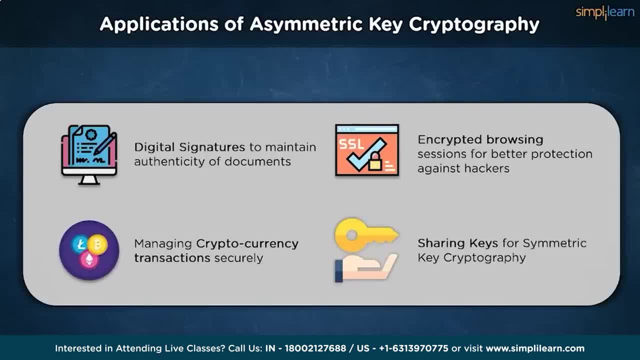 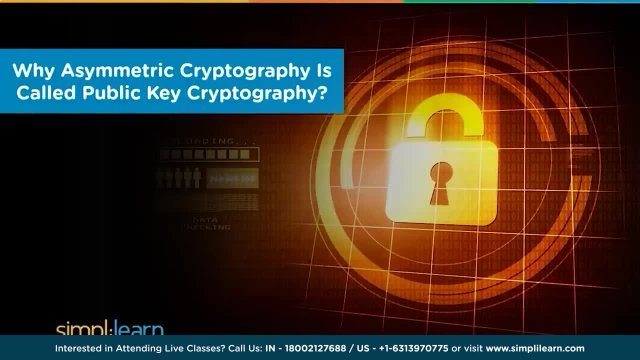 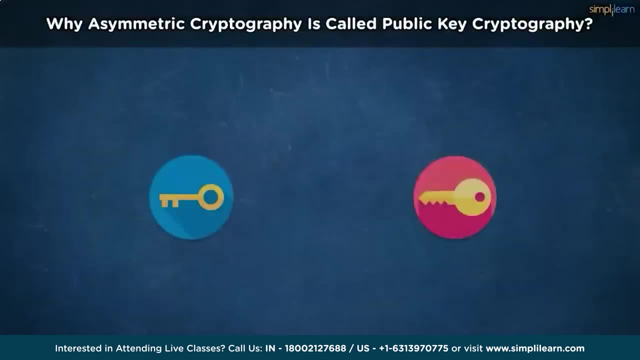 Encrypting the key using asymmetric algorithms will definitely be more memory efficient and secure. You might remember us discussing why symmetric encryption was called private key cryptography. Let us understand why asymmetric falls under the public key cryptography. We have two keys at our disposal: The encryption. 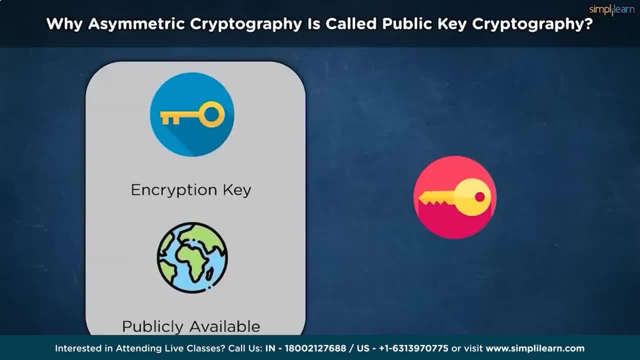 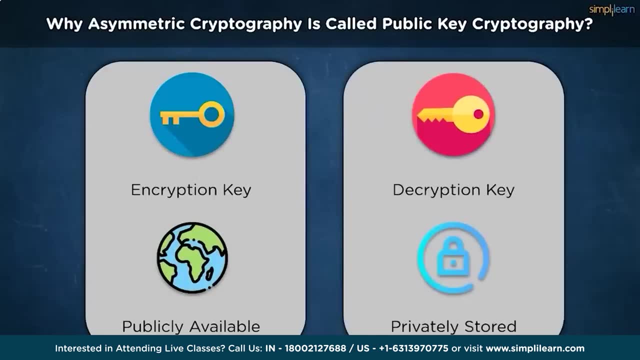 key is available to everyone. The decryption key is supposed to be private. Unlike symmetric key cryptography, there is no need to share anything privately to have an encrypted messaging system. To put that into perspective, we share our email address with anyone looking to communicate with us. 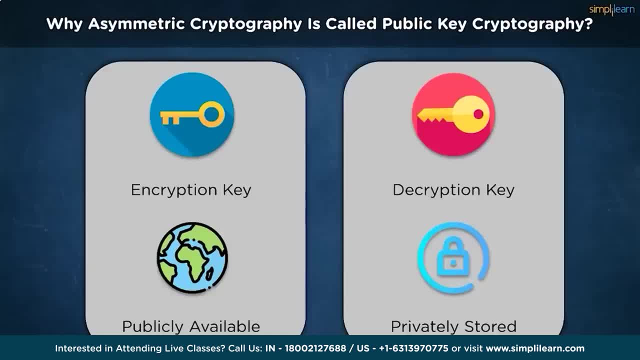 It is supposed to be public by design, so that our email login credentials are private and they help in preventing any data mishandling, Since there is nothing hidden from the world if they want to send us any encrypted information. this category is called the public key cryptography. 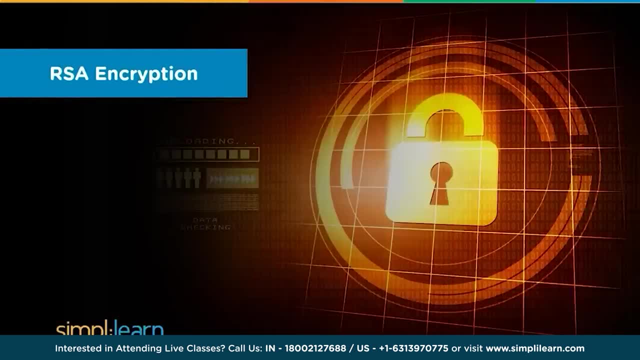 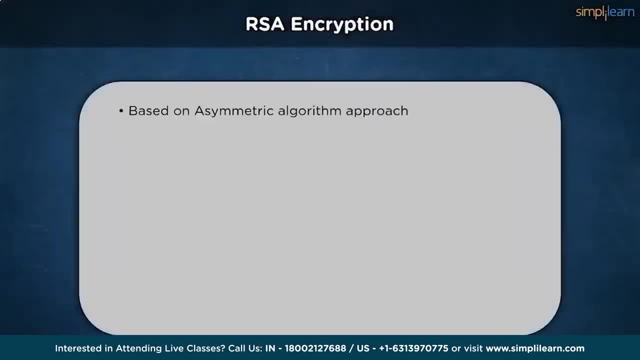 There are quite a few algorithms being used today that follow the architecture of asymmetric key cryptography, none more famous than the RSA encryption. RSA encryption is the most widely used encryption or public key encryption standard using asymmetric key approach Named after its founders Rivest. 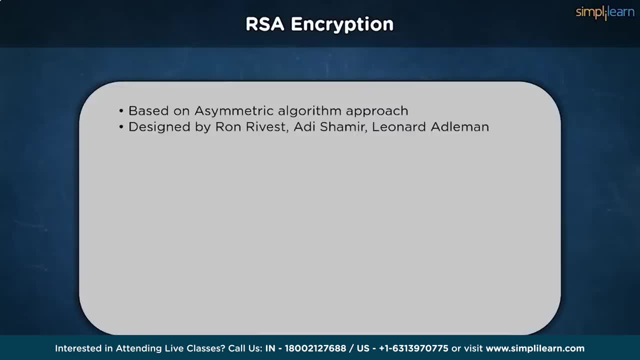 Shamir and Edelman. it uses block ciphers to obscure the information. If you are unfamiliar with how block ciphers work, they are encryption algorithms that divide the original data into blocks of equal size. The block size depends on the exact cipher being used. 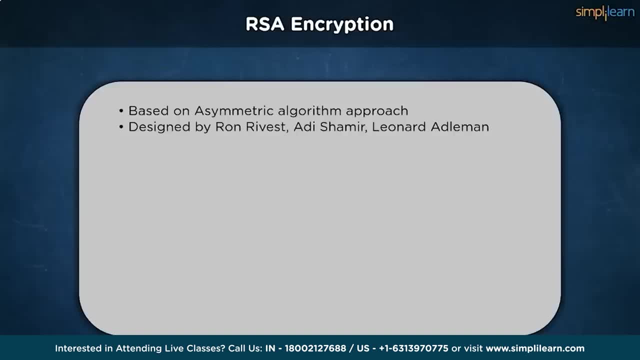 Once they are broken down, these blocks are encrypted individually and later chained together to form the final ciphertext, Widely considered to be the most secure form of encryption, albeit relatively slower than symmetric encryption algorithms. it is widely used in web browsing secure identification VPNs. 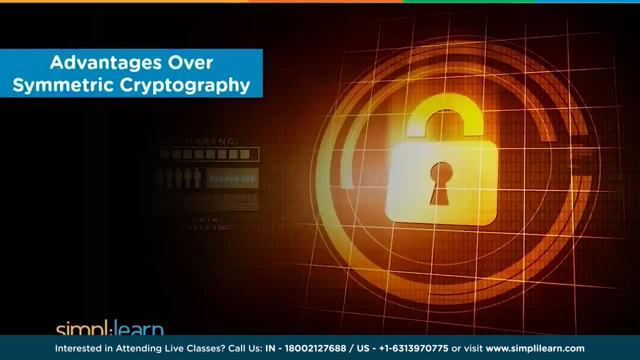 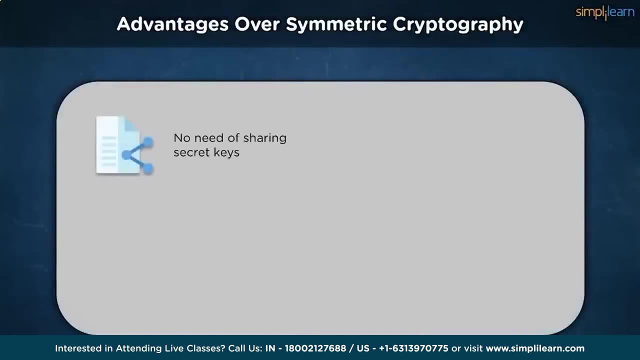 emails and other chat applications. With so many variables in play, there must be some advantages that give asymmetric key cryptography an edge over the traditional symmetric encryption methodologies. Let's go through some of them. There is no need for any reliable key sharing channel in asymmetric encryption. 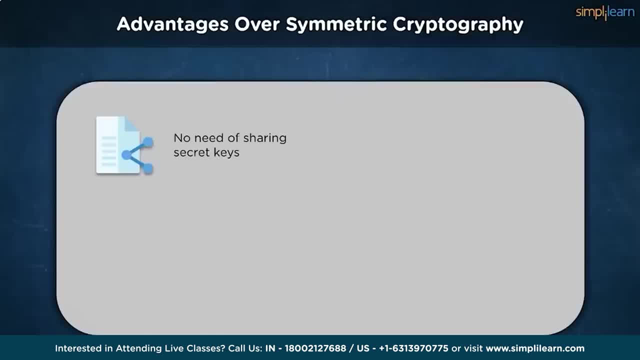 It was an added risk in private key cryptography. that has been completely eliminated in public key architecture. The key which is made public cannot encrypt any confidential information, and the only key that can decrypt doesn't need to be shared publicly under any circumstance. We have much more extensive 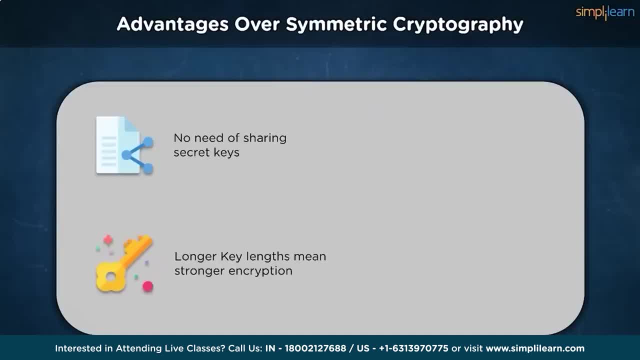 key lengths in RSA encryption and other asymmetric algorithms like 2048-bit key and 4096-bit keys. Larger keys are much harder to break into via brute force and are much more secure. Asymmetric key cryptography can be used as a proof of authenticity, since only the 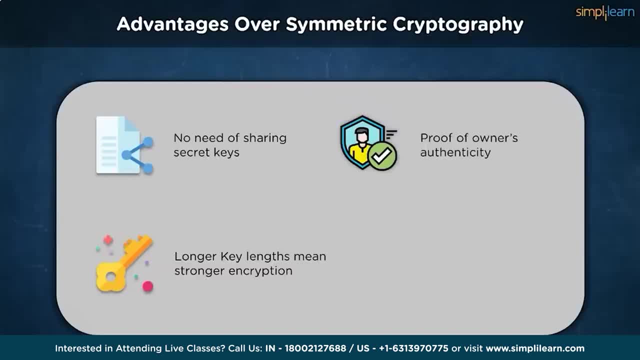 rightful owner of the keys can generate the messages to be decrypted by the private key. This situation can also be reversed: Encryption is done using a private key and decryption is done by the public key, which would not function if the correct private key is not used to. 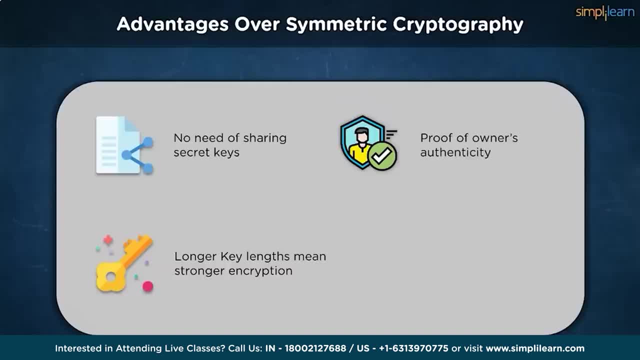 generate the message, hence proving the authenticity of the owner. It also has a tamper protection feature, where the message cannot be intercepted and changed without invalidating the private key used to encrypt the data. Consequently, the public key cannot decrypt the message and it is easy to realize the information. 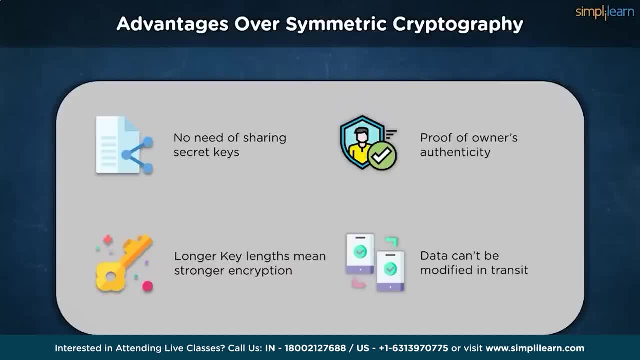 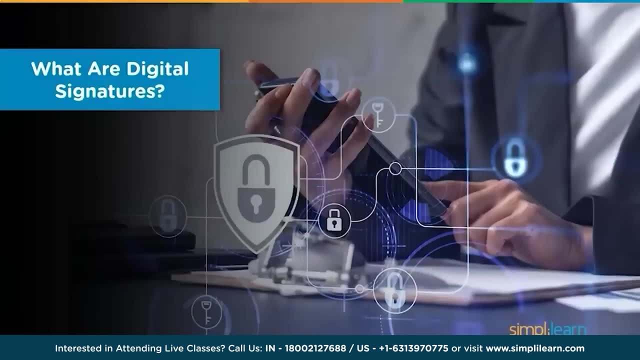 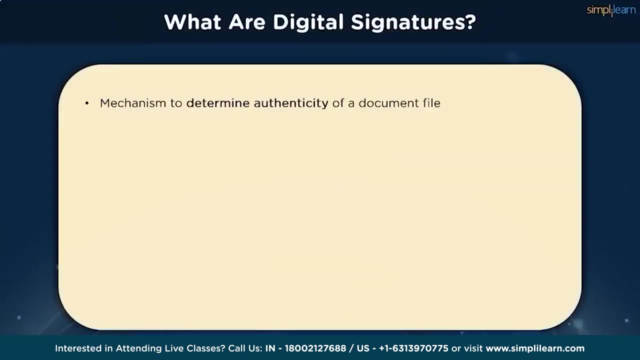 is not 100% legitimate when and where the case requires. Now that we have a proper revision, let's understand what digital signatures are before moving on to the algorithm. The objective of digital signatures is to authenticate and verify documents and data. This is necessary to avoid tampering. 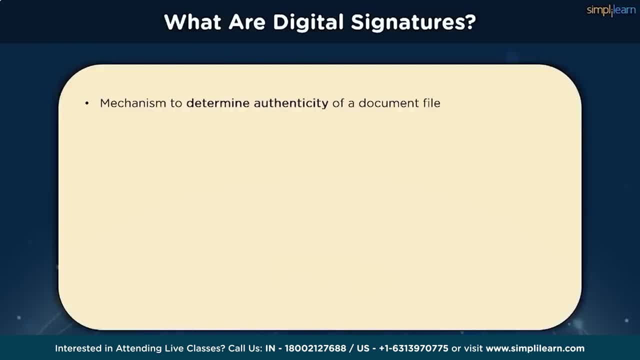 and digital modification or forgery of any kind during the transmission of official documents. They work on the public key cryptography architecture with one exception: Typically, an asymmetric key system encrypts using a public key and decrypts with a private key For digital signatures. 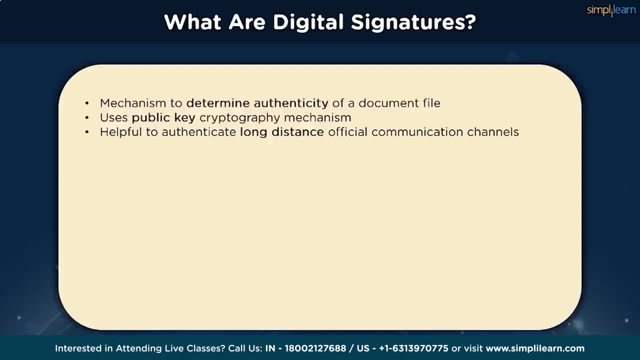 however, the reverse is true: The signature is encrypted using a private key and is decrypted with the public key, Because the keys are inked together. decoding it with a public key verifies that the proper private key was used to sign the document, thereby verifying the signature's provenance. 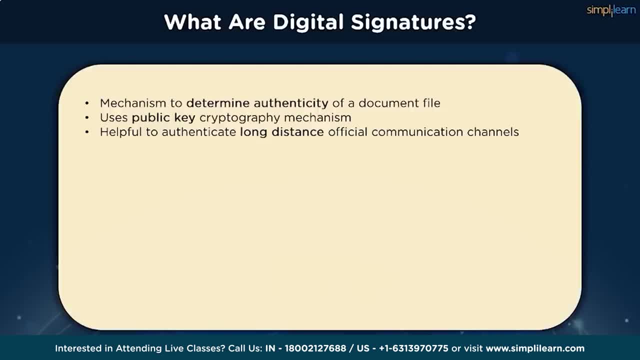 Let's go through each step to understand the procedure thoroughly. In step 1, we have m, which is the original plaintext message, and it is passed onto a hash function denoted by h to create a digest. Next, it bundles the message together with the hash digest. 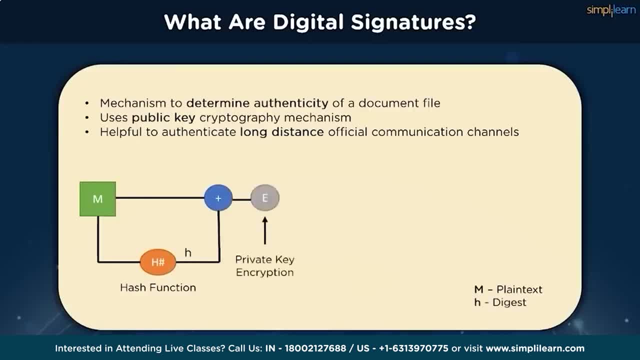 and encrypts it using the sender's private key. It sends the encrypted bundle to the receiver, who can decrypt it using the sender's public key. Once the message is decrypted, it is passed through the same hash function, hhash, to generate a similar. 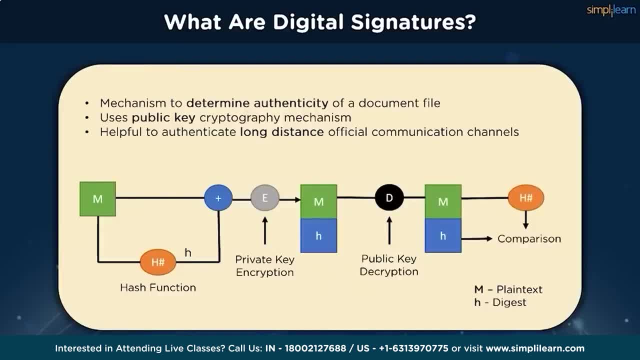 digest. It compares the newly generated hash with the bundled hash value received, along with the message. If they match, it verifies data integrity. In many instances they provide a layer of validation and security to messages through a non-secured channel Properly. 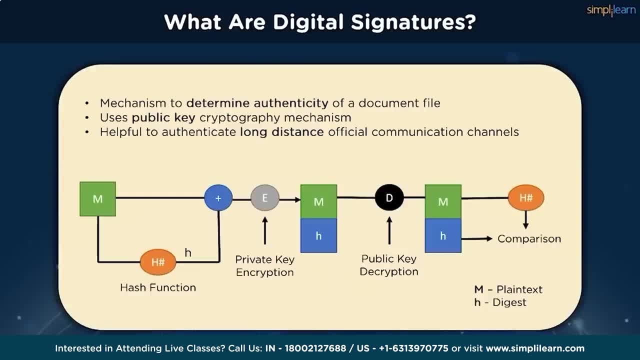 implemented, a digital signature gives the receiver reason to believe that the message was sent by the claimed sender. Digital signatures are equivalent to traditional handwritten signatures in many respects, but properly implemented digital signatures are more difficult to forge than the handwritten type Digital signature schemes in the sense used here. 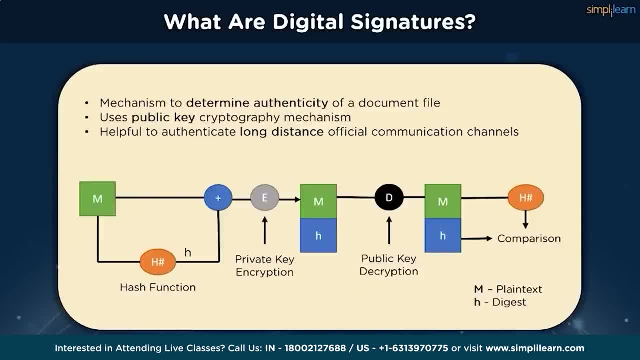 are cryptographically based and must be implemented properly to be effective. They can also provide non-repudiation, meaning that the signer cannot successfully claim that they did not sign a message while also claiming their private key remains secret. Further, some 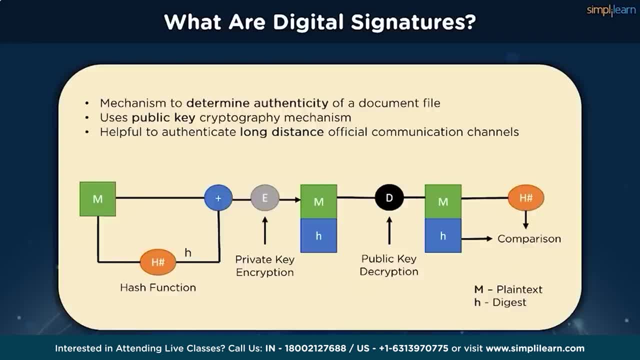 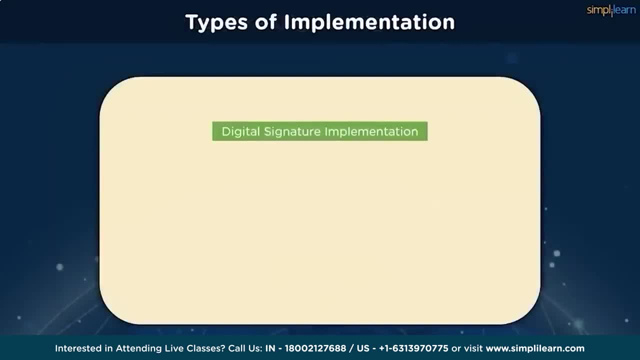 non-repudiation schemes offer a time stamp for the digital signature so that, even if the private key is exposed, the signature is valid. To implement the concept of digital signature in real world, we have two primary algorithms to follow: The RSA algorithm. 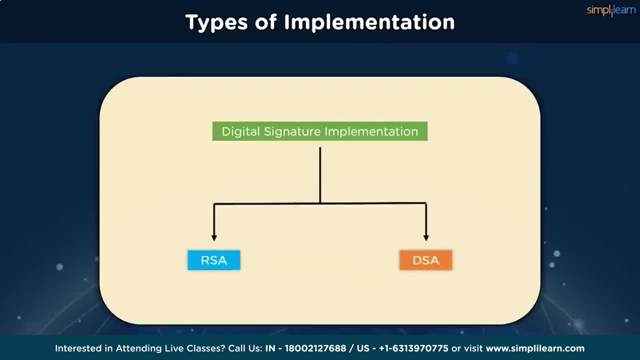 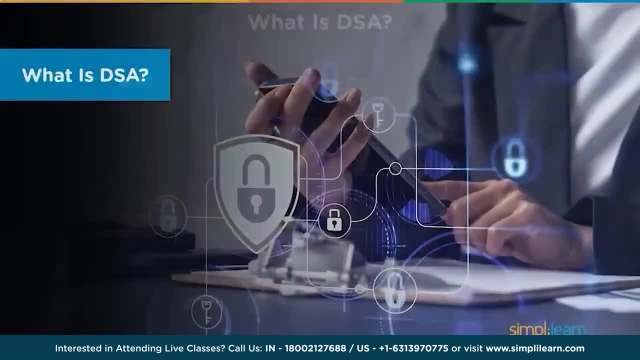 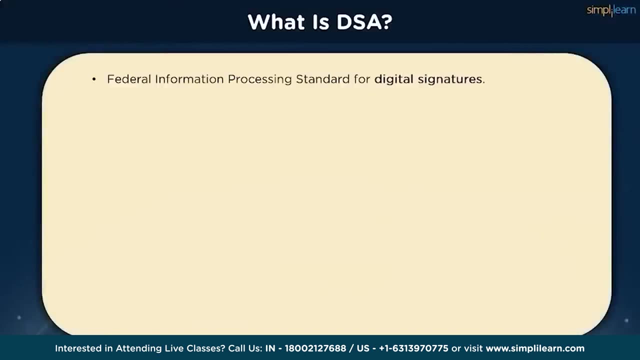 and the DSA algorithm, but the latter is a topic of learning today. So let's go ahead and see what the digital signature algorithm is supposed to do. Digital signature algorithm is a FIPS standard, which is the Federal Information Processing Standard for digital signatures. 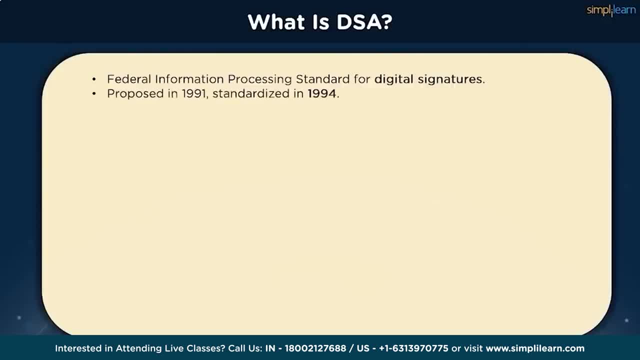 It was proposed in 1991, and globally standardized in 1994 by the National Institute of Standards and Technology, also known as the NIST. It functions on the framework of modular exponention and discrete logarithmic problems which are difficult to compute as a force-brute system. 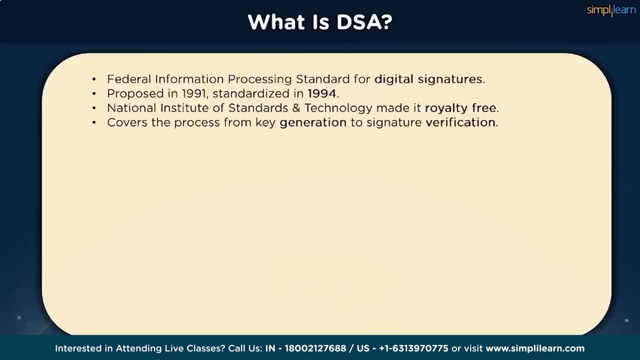 Unlike DSA, most signature types are generated by signing message digests with the private key of the originator. This creates a digital thumbprint of the data. Since just the message digest is signed, the signature is generally much smaller compared to the data that was signed. As a result, 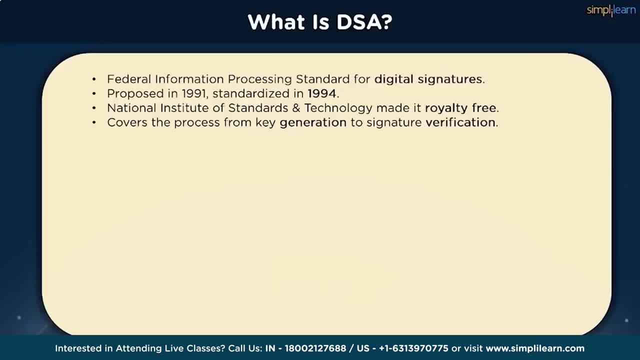 digital signatures impose less load on processors at the time of signing execution and they use small volumes of bandwidth. DSA, on the other hand, does not encrypt message digests using private key or decrypt message digests using public key. Instead, it uses mathematical. 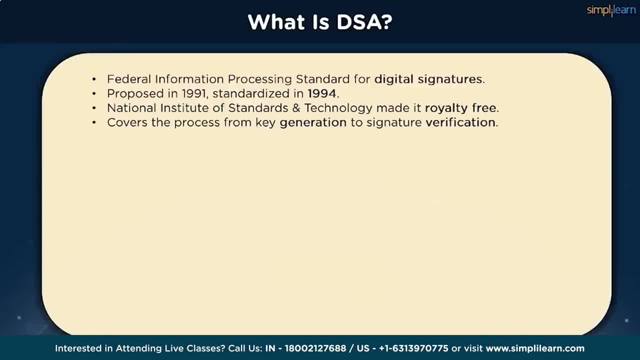 functions to create a digital signature consisting of two 160-bit numbers which are originated from the message digests and the private key. DSAs make use of the public key for authenticating the signature, but the authorization process is much more complicated when compared with RSA. 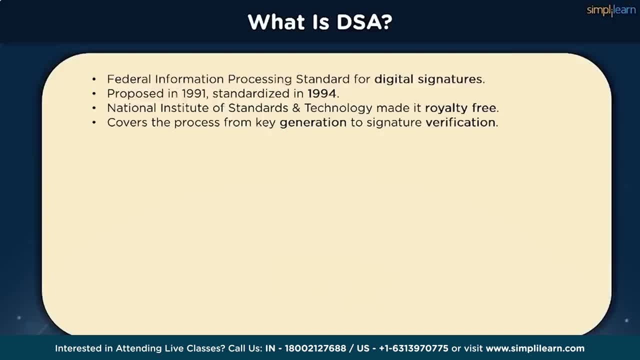 DSA also provides three benefits, which is the message authentication, integrity verification and non-repudiation. In the image we can see the entire process of DSA validation. A plain text message is passed onto a hash function where the digest is. 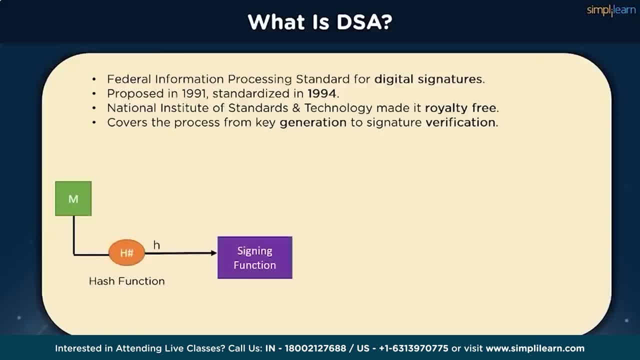 generated, which is passed onto a signing function. Signing function also has other parameters, like a global variable g, a random variable k and the private key of the sender. The outputs are then bundled onto a single pack with the plain text and sent to the receiver. 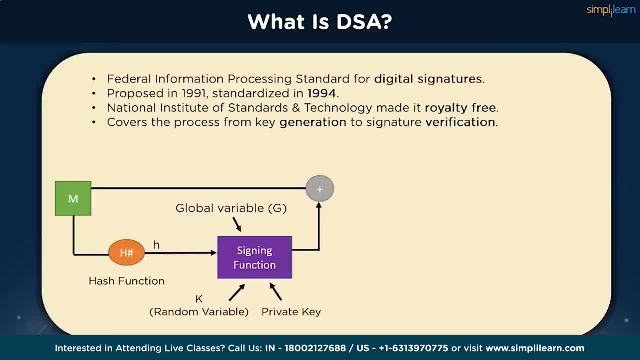 The two outputs we receive from the signing functions are the two 160-bit numbers denoted by s and r. On the receiver end we pass the plain text to the same hash function to regenerate the message digest. It is passed onto verification function, which has other requirements such as: 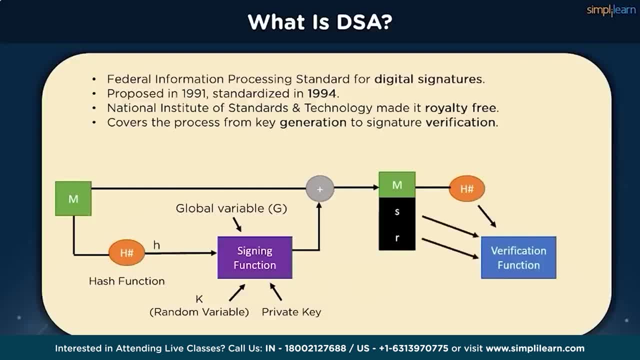 the public key of the sender, global variable g and s and r received from the sender. The value generated by the function is then compared to R. If they match, then the verification process is complete and data integrity is verified. This was an overview. 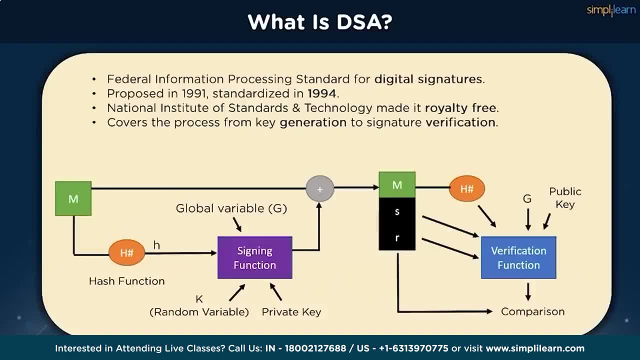 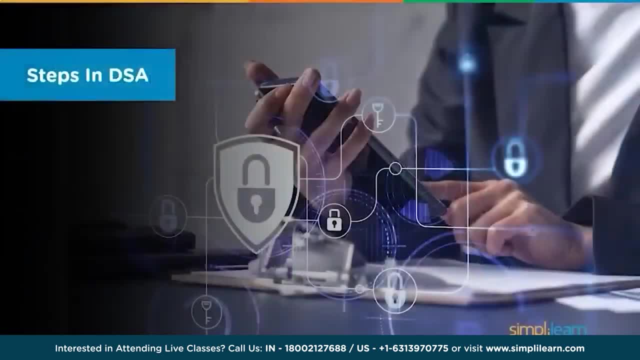 of the way the DSA algorithm works. You already know it depends on logarithmic functions to calculate the outputs, So let us see how we can do the same in our next section. We have three phases here, the first of which is key generation. 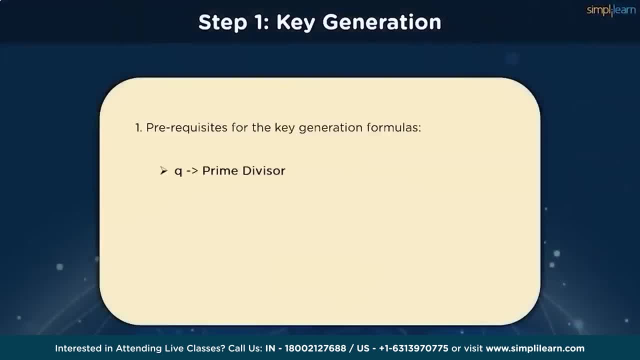 To generate the keys, we need some prerequisites. We select a q which becomes a prime divisor. We select a prime number, p, such that p-1 mod q equal to 0. We also select a random integer, g, which must satisfy the two formulas. 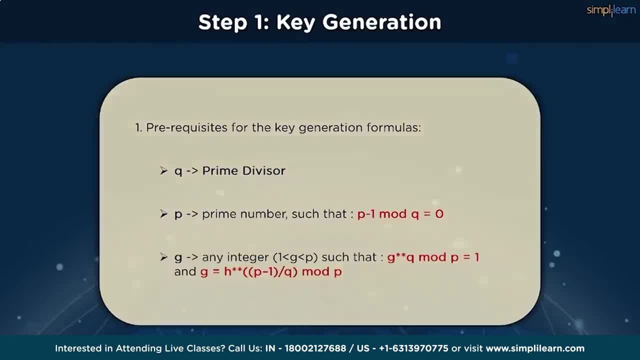 being mentioned on the screen right now. Once these values are selected, we can go ahead with generating the keys. The private key can be denoted by x and it is any random integer that falls between the bracket of 0 and the value of q. 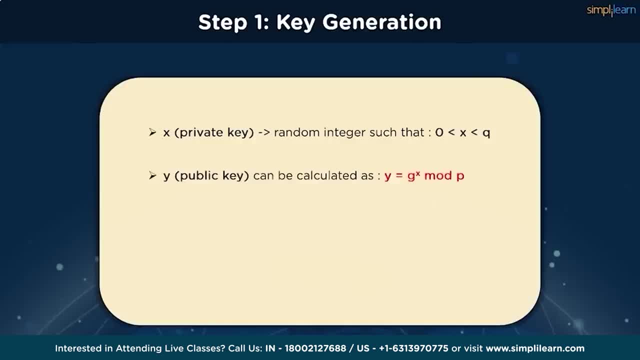 The public key can be calculated as y equal to g to the power x mod p, where y stands for the public key. The private key can then be packaged as a bundle which comprises of values of p, q, g and x. Similarly, the public key. 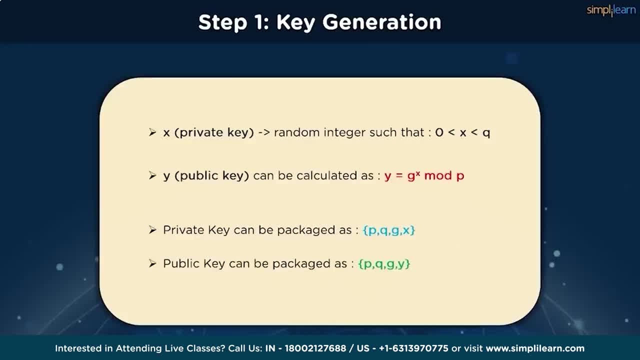 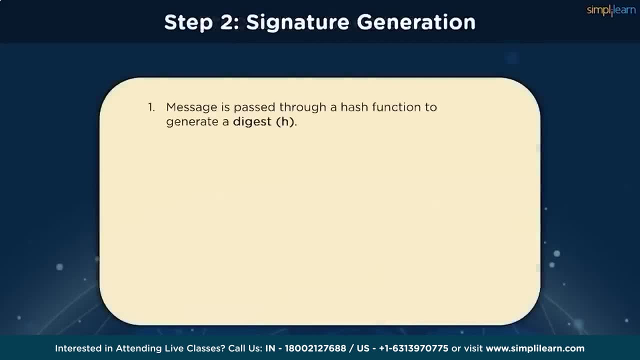 can also be packaged as a bundle, having the values of p, q, g and y. Once we are done with key generation, we can start verifying the signature and its generation Repeat. Once the keys are generated, we can start generating the signature. 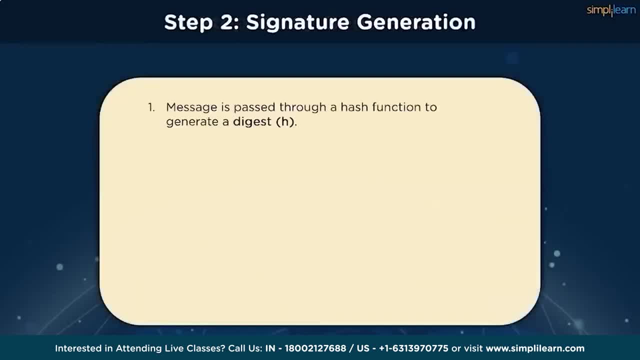 The message is passed through a hash function. to generate the digest edge first We can choose any random integer k which falls under the bracket of 0 and q. To calculate the first 160 bit number of assigning function of r we use the formula g to the power. 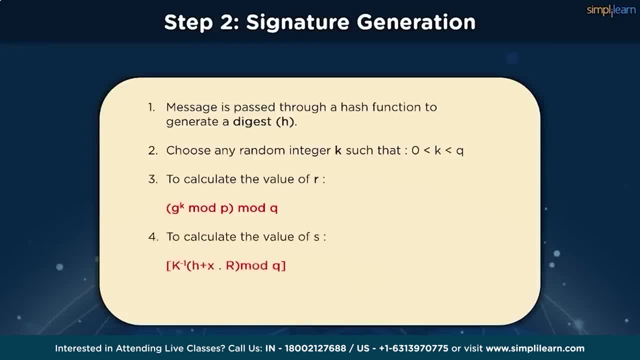 k mod p into mod q. Similarly, to calculate the value of the second output, that is, s, we use the following formula that is shown on the screen: The signature can then be packaged as a bundle having r and s. This bundle, along with the plain text message, 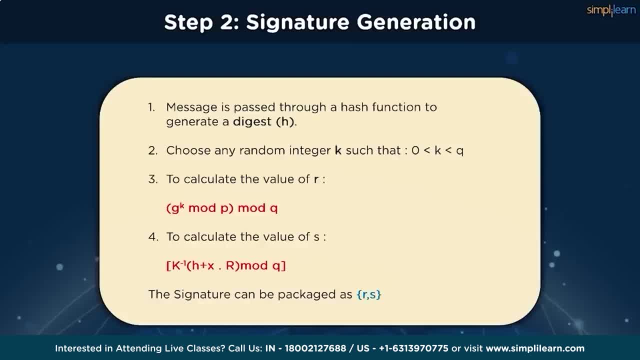 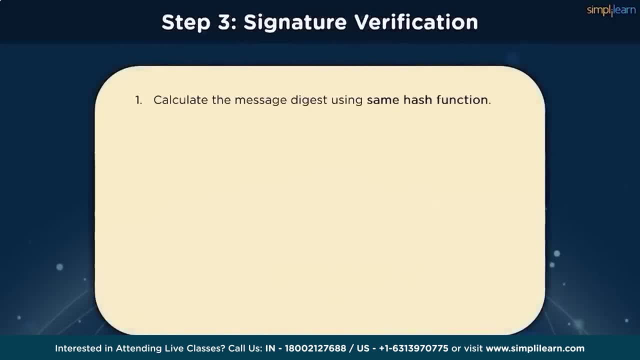 is then passed on to the receiver. Now, with the third phase, we have to verify the signature. We first calculate the message digest received in the bundle by passing it through the same hash function. We calculate the value of w, u1 and u2 using the formulas: 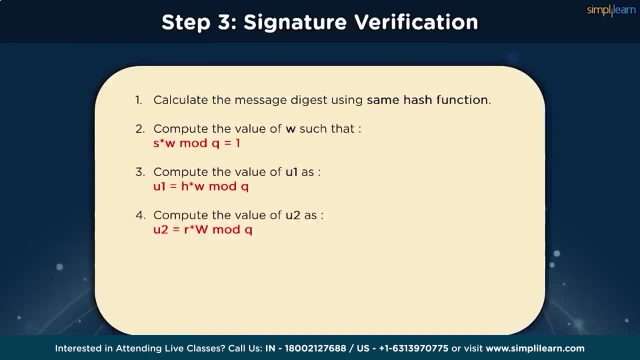 shown on the screen. We have to calculate a verification component, which is then to be compared with the value of r being sent by the sender. This verification component can be calculated using the following formula: Once calculated, this can be compared with the value of r. 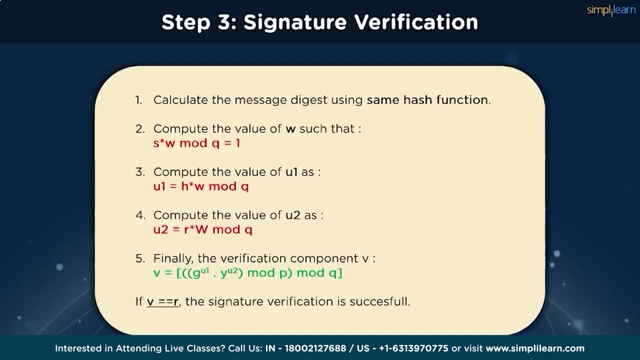 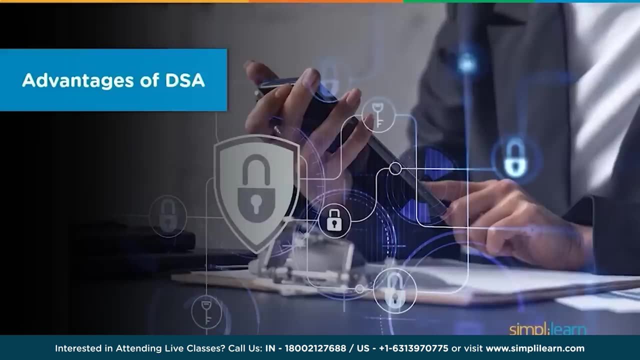 If the values match, then the signature verification is successful and our entire process is complete, starting from key generation to the signature generation, all the way up to the verification of the signature. With so many steps to follow, we are bound to have a few advantages. 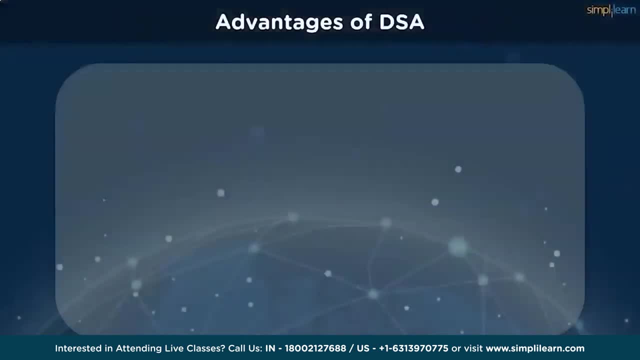 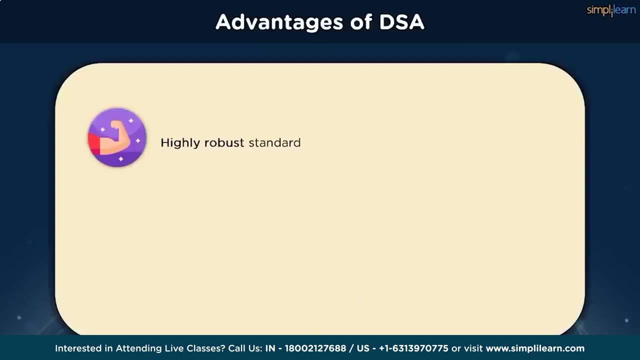 to boot this, and we would be right to think so. DSA is highly robust in the security and stability aspect when compared to alternative signature verification algorithms. We have a few other ciphers that aim to achieve the simplicity and the flexibility of DSA, but it has been. 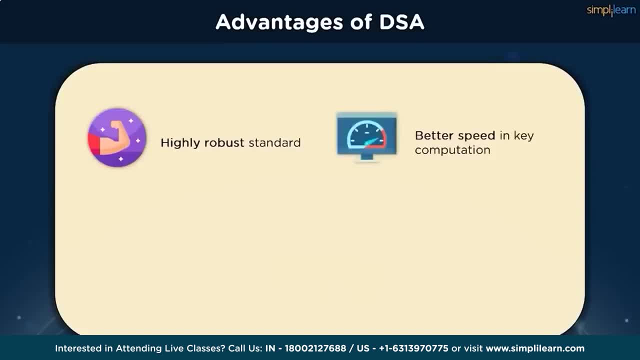 a tough ask. for all the other suits. The key generation is much faster when compared to the RSA algorithm and such, While the actual encryption and decryption process may falter a little in comparison. a quicker start in the beginning is well known to optimize a lot of frameworks. 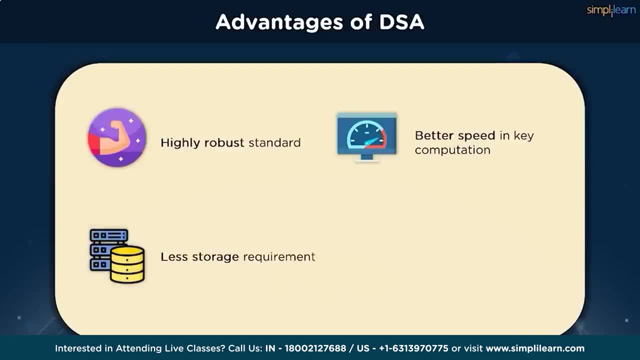 DSA requires less storage space to work its entire cycle. In contrast, its direct correspondent, that is, RSA algorithm, needs a certain amount of computational and storage space to function efficiently. This is not the case with DSA, which has been optimized to work with weaker hardware and lesser 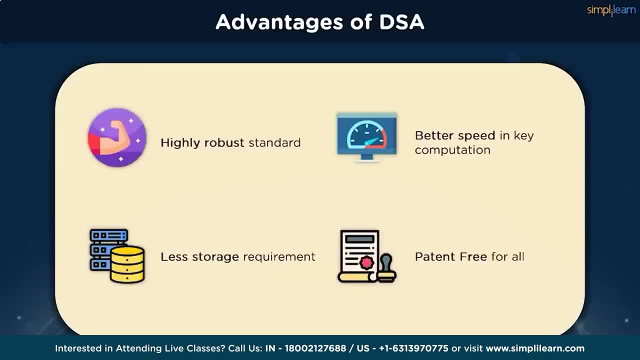 resources. The DSA is patented, but NIST has made this patent available worldwide royalty free. A draft version of the speculation FIPS 1865 indicates that DSA will no longer be approved for digital signature generation, but it may be used to verify signatures. 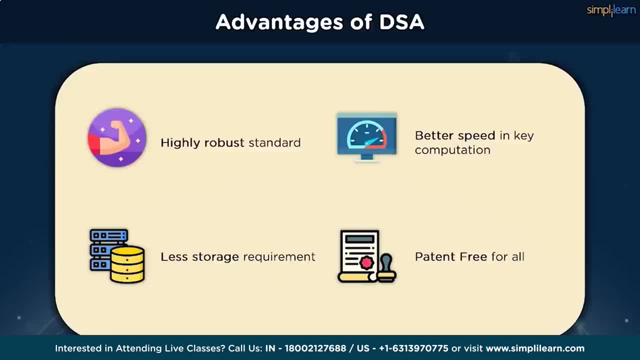 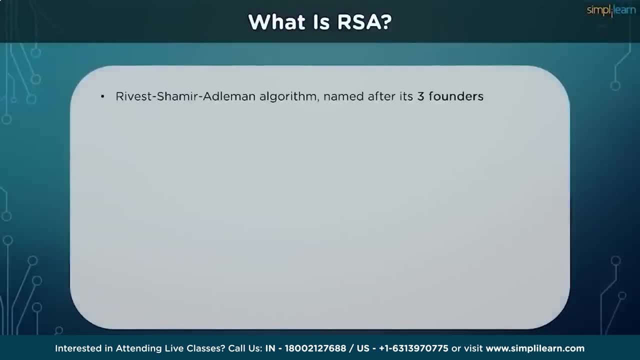 generated prior to the implementation date of that standard. The RSA algorithm is a public key signature algorithm developed by Ron Rivest, Adi Shamir and Leonard Edelman. The paper was first published in 1977 and the algorithm uses logarithmic functions to keep the working. 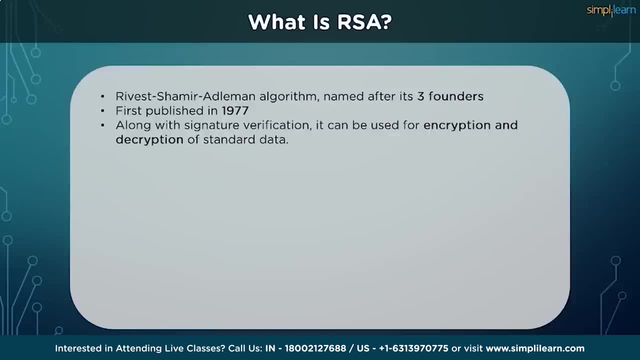 complex enough to withstand brute force and streamlined enough to be fast. post deployment. RSA can also encrypt and decrypt general information to securely exchange data, along with handling digital signature verification. Let us understand how it achieved this. We take our plain text message M. We pass it through a hash 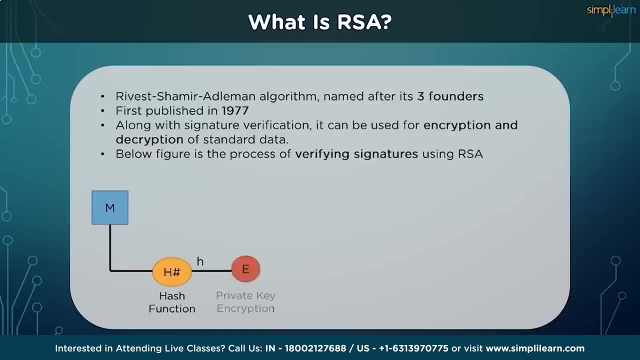 function to generate the digest H, which is then encrypted using the sender's private key. This is appended to the original plain text message and sent over to the receiver. Once the receiver receives the bundle, we can pass the plain text message through the same hash. 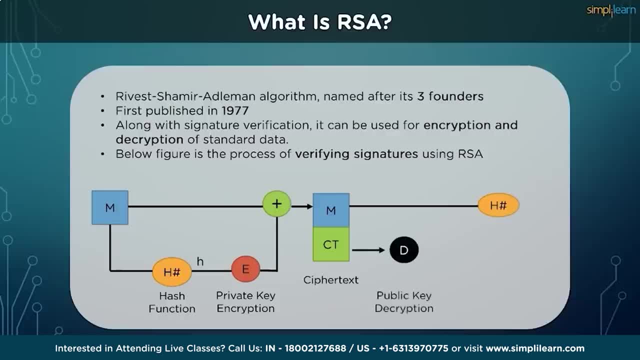 function to generate a digest, and the ciphertext can be decrypted using the public key of the sender. The remaining hashes are compared. If the values match, then the data integrity is verified and the sender is authenticated. Apart from digital signatures, the main case of 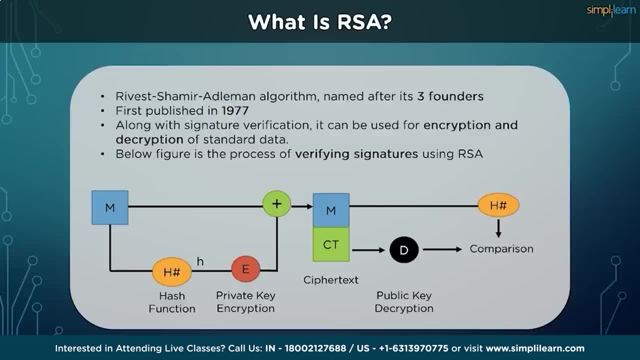 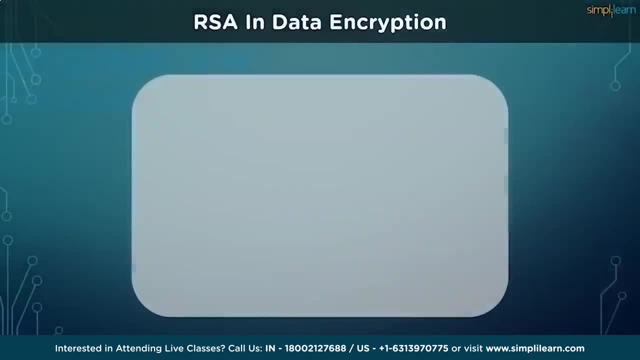 RSA is encryption and decryption of private information before being transmitted across communication challenge. This is where the data encryption comes into play. When using RSA for encryption and decryption of general data, it reverses the keyset usage. Unlike signature verification, it receives the receiver's 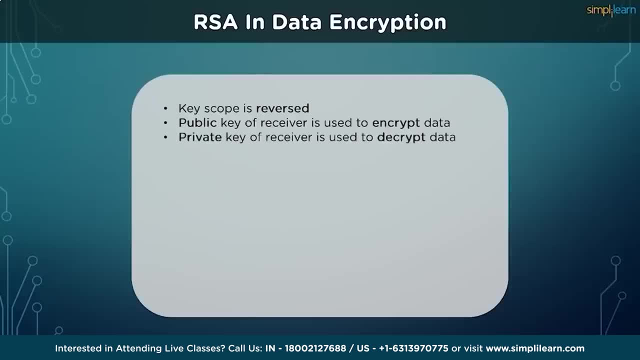 public key to encrypt the data and uses the receiver's private key in decrypting the data. Thus, there is no need to exchange any keys in this scenario, There are two broad components when it comes to RSA cryptography. One of them is key generation. 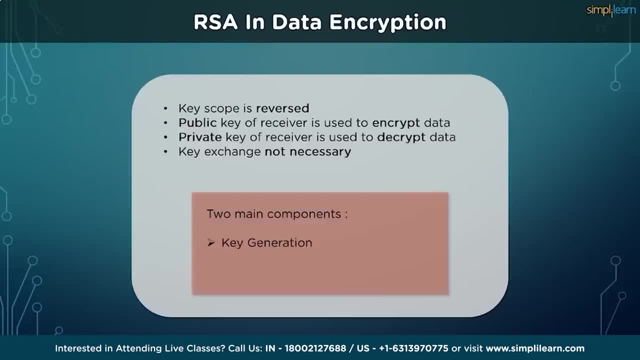 Key generation employs a step of generating the private and the public keys that are going to be used for encrypting and decrypting the data. The second part is the encryption and decryption functions. These are the ciphers and steps that need to be run when scrambling. 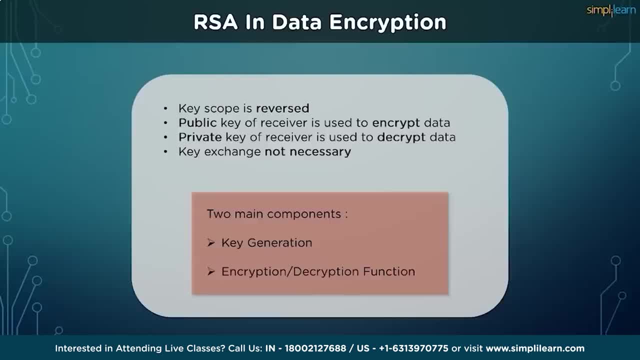 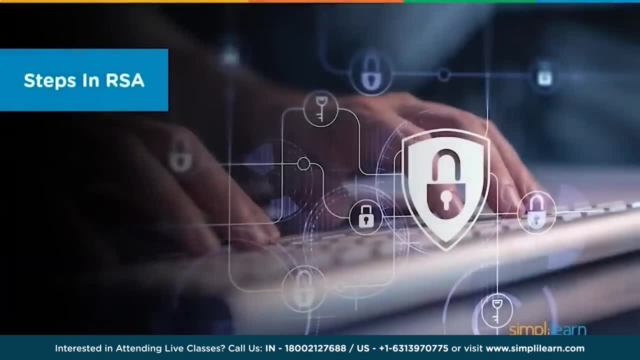 the data or recovering the data from the ciphertext. You will now understand each of these steps in our next subtopic. Keeping the previous two concepts in mind, let us go ahead and see how the entire process works, starting from creating the key pair to encrypting and. 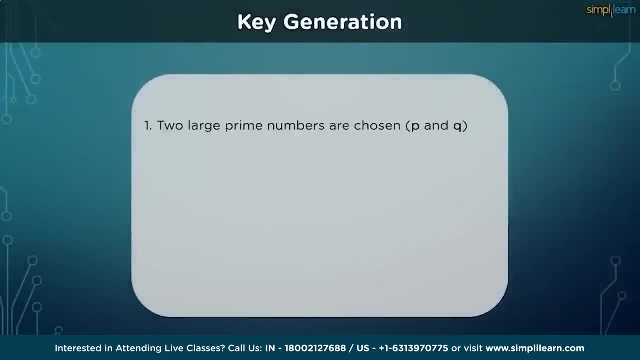 decrypting the information, You need to generate the public and private keys before running the functions. to generate ciphertext and plaintext, They use certain variables and parameters, all of which are explained. We first use two large prime numbers, which can be denoted by p and q. 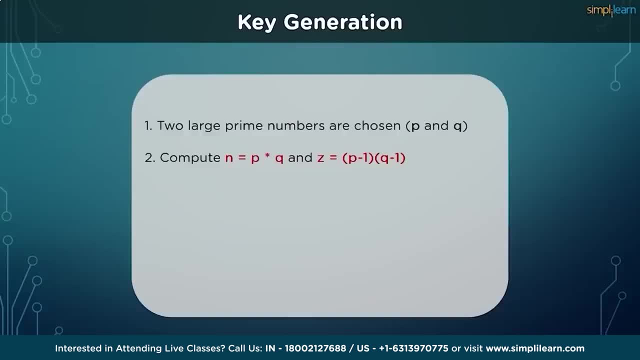 We can compute the value of n as n equal to p into q and compute the value of z as p minus 1 into q minus 1.. A number e is chosen at random, satisfying the following conditions, and a number d is also selected at random following the: 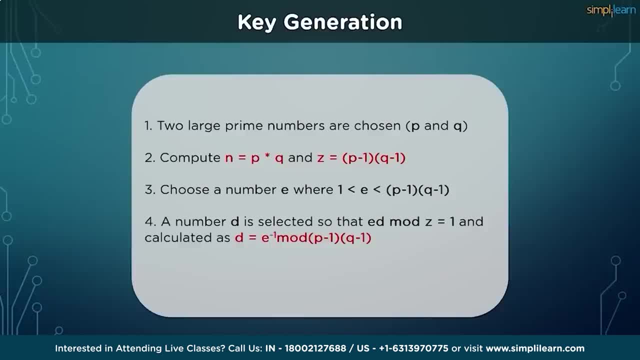 formula ed mod z equal to 1, and it can be calculated with the formula given below. The public key is then packaged as a bundle with n and e, and the private key is packaged as a bundle using n and d. This sums up the 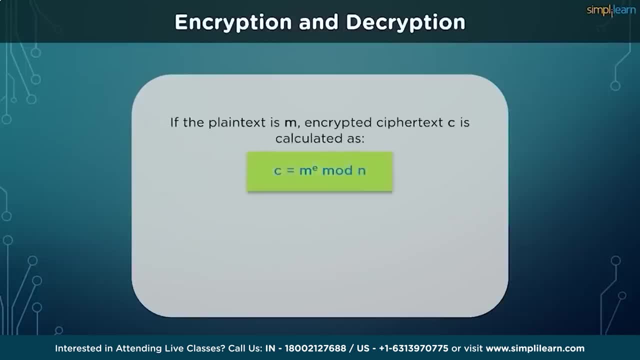 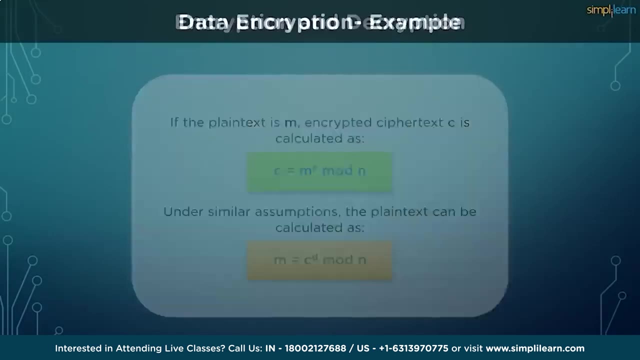 key generation process. For the encryption and decryption function we use the formula c and m. The ciphertext can be calculated as c equal to m to the power e mod n, and the plaintext can be calculated from the ciphertext as c power d mod n. 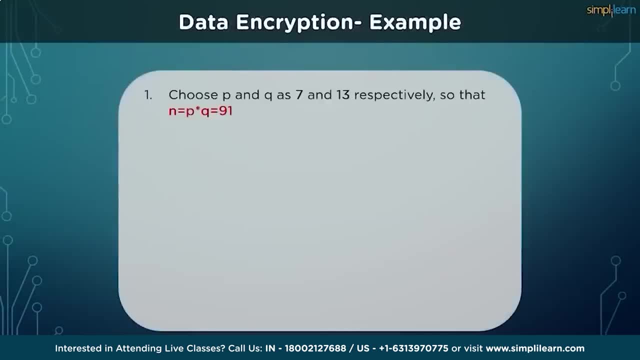 When it comes to a data encryption example, let's take p and q as 7 and 13.. The value of n can be calculated as 91. If we select the value of e to be 5,, it satisfies all the criteria that. 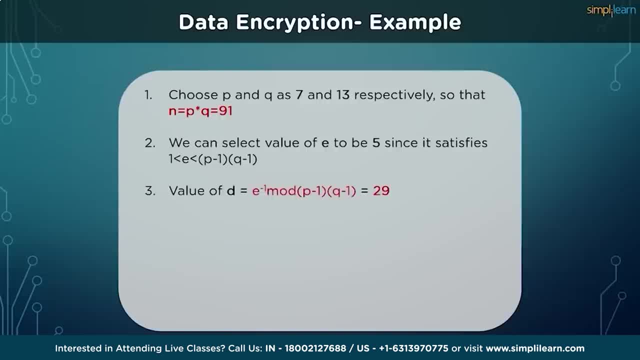 we need it to. The value of d can be calculated using the following function, which gives it as 29.. The public key can then be packaged as 91 comma 5,, and the private key can then be packaged as 91 comma 29.. 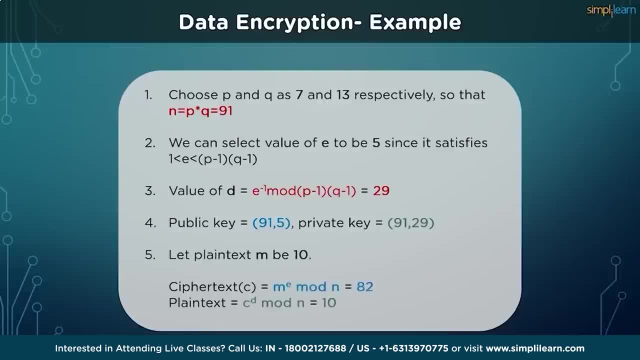 The plaintext, if it is 10, which is denoted by m, Ciphertext can be calculated with the formula c, equal to m to the power e mod n, which gives us 82. If somebody receives this ciphertext, they can calculate the plaintext using the formula c. 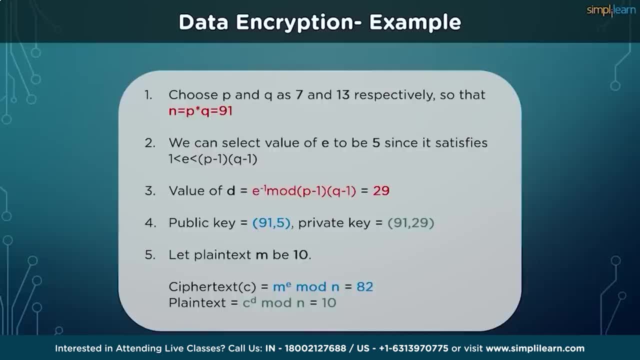 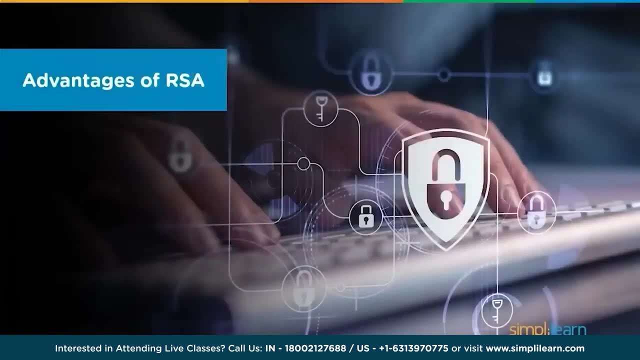 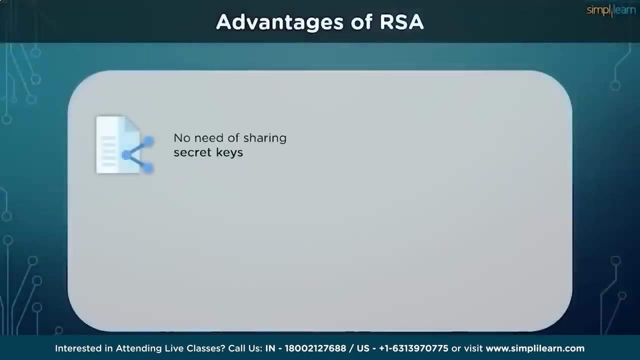 to the power d mod n, which gives us the value of 10, as selected as our plaintext. We can now look at the factors that make the RSA algorithm stand out versus its competitors in the advantageous topics of this lesson. RSA encryption depends on using the receiver's 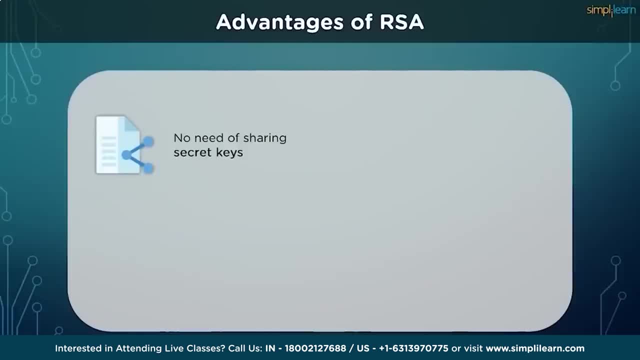 public key, so that you don't have to share any secret key to receive the messages from others. This was the most glaring flaw faced by symmetric algorithms, which were eventually fixed by asymmetric cryptography structure, Since the key pairs are related to each other. 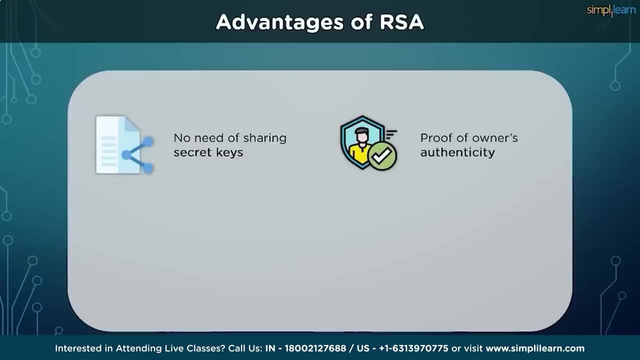 a receiver cannot intercept the message since they didn't have the correct private keys to decrypt the information. If a public key can decrypt the information, the sender cannot refuse signing it with his private key without admitting the private key is not, in fact, private anymore. 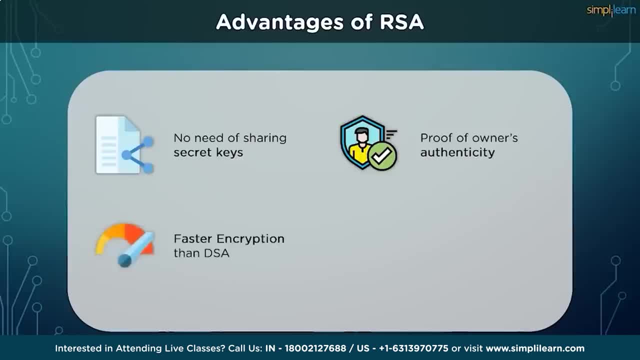 The encryption process is faster than that of the DSA algorithm, Even if the key generation is slower in RSA. many systems across the world tend to reuse the same keys so that they can spend less time in key generation and more time on actual ciphertext. 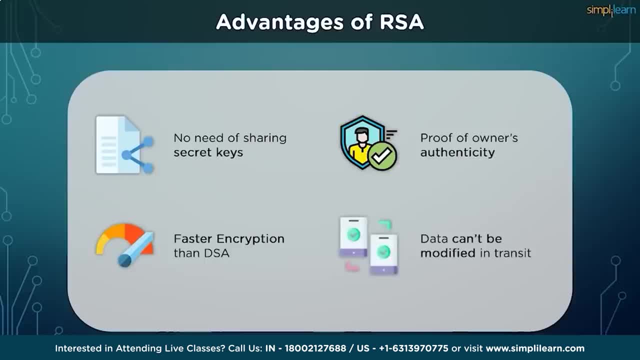 management Data will be tamper-proof in transit, since meddling with the data will alter the usage of the keys. The private key won't be able to decrypt the information, hence alerting the receiver of any kind of manipulation in between. The receiver must be aware of any. 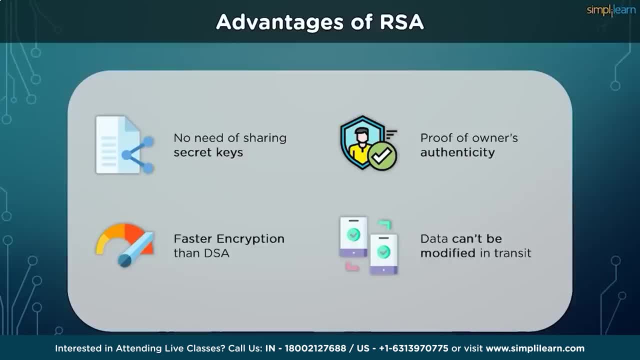 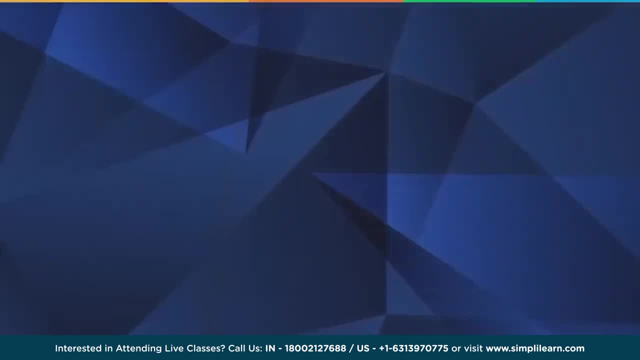 third party who possesses the private key, since they can alter the data mid-transit, the cases of which are rather low. Imagine creating an account on a new website. You provide your email address and set a password that you are confident and you would not forget. 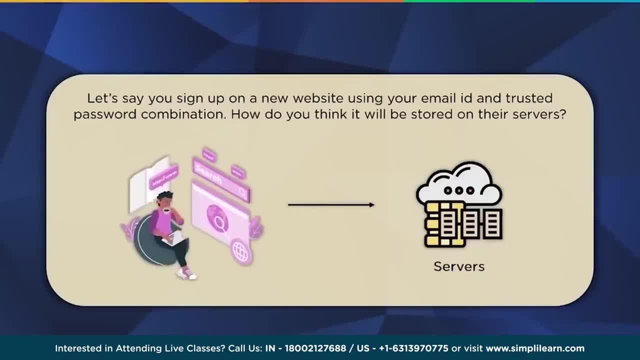 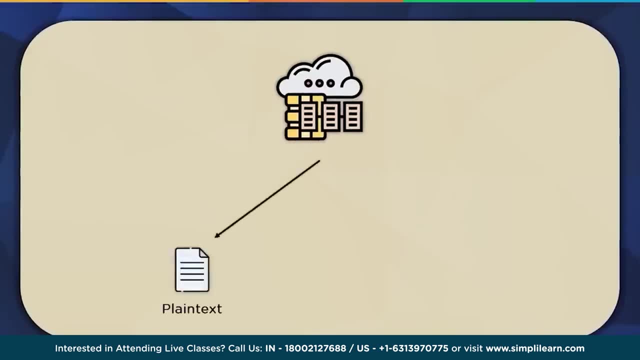 What about the website owner? How securely are they going to store your password? For website administrators they have three alternatives. They can either store the passwords in a plain text format, they can encrypt the passwords using an encryption and decryption key, or they can store. 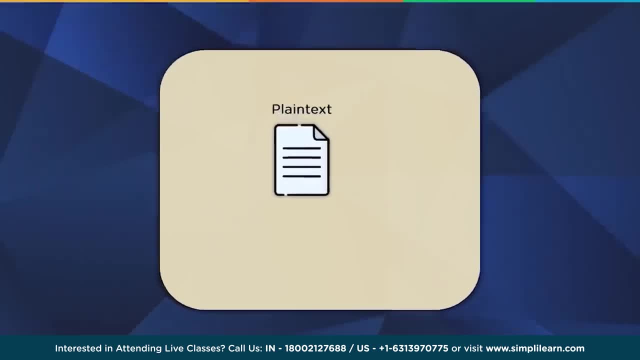 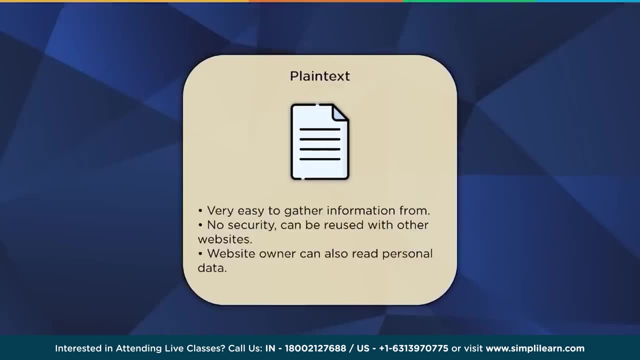 the passwords in a hash value. Let's have a look at each of these. When a password is stored in plain text format, it is considered to be the most unsafe option, since anyone in the company can read your passwords. A single hack and 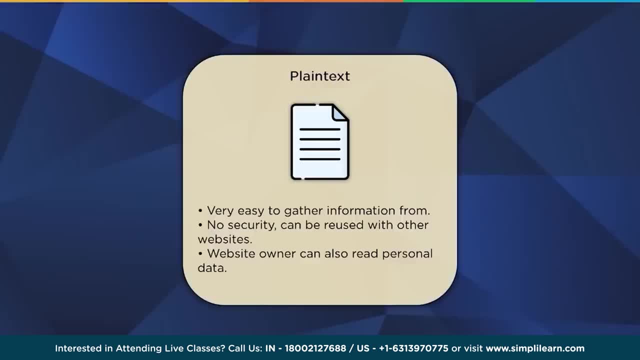 a data server breach will expose all the account's credentials without needing any extra effort To counter this. owners can encrypt the passwords and keep them in the servers as a second alternative, But that would mean they also have to store the decryption key somewhere on their 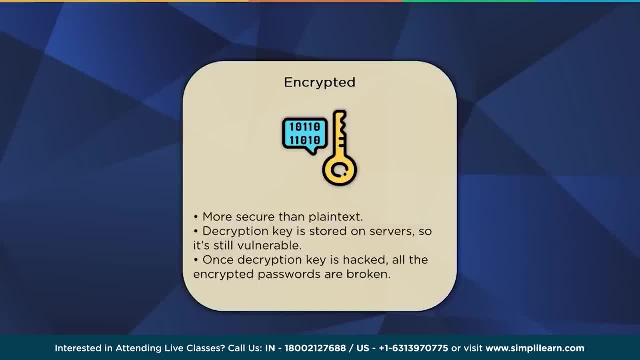 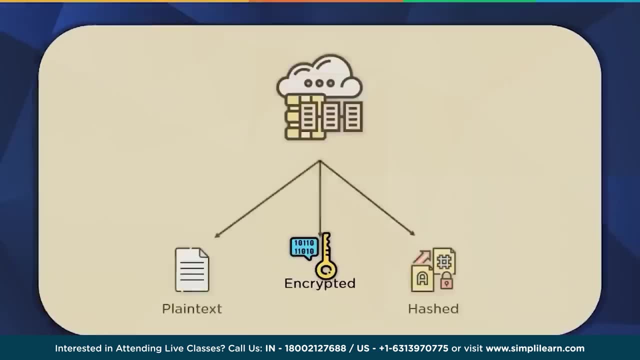 servers. In the event of a data breach or the server hack, both the decryption key and encrypted passwords will be leaked, thus making it a single point of failure. What if there was an option to store the passwords after scrambling them completely? This is where hashing comes to play. 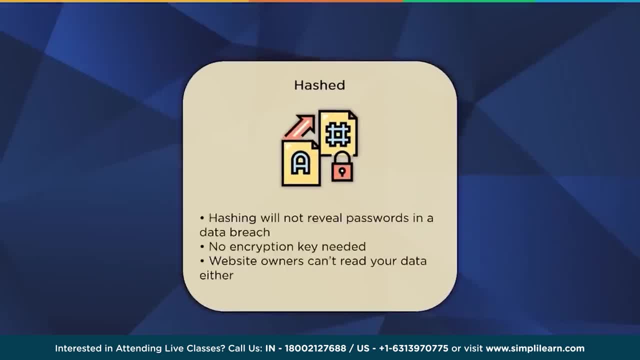 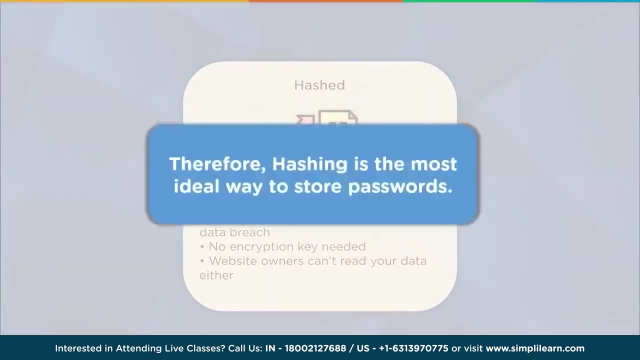 Since only the hashed values are stored in the server, no encryption is needed, With no plain text passwords to protect. your credentials are safe from the website administrators. Considering all the pros, hashed passwords are the industry standard when it comes to storing credentials nowadays. 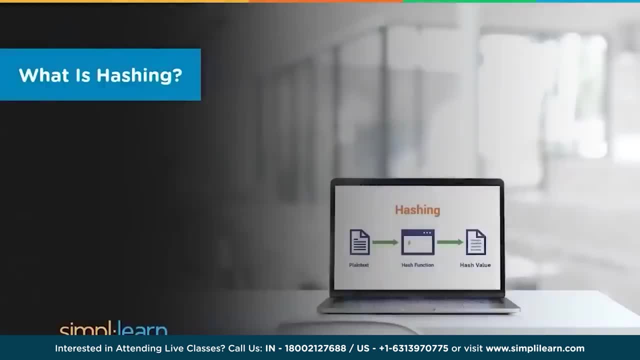 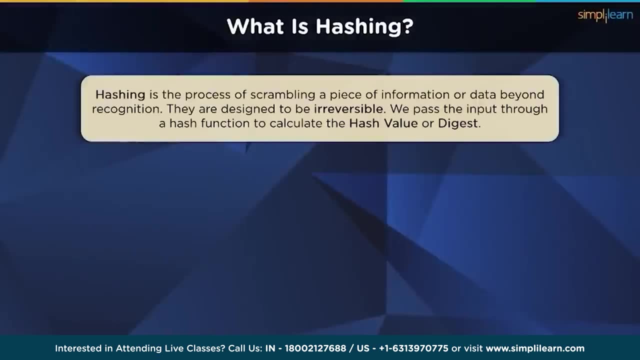 Before getting too deep into the topic, let's get a brief overview of how hashing works. Before getting too deep into the topic, let's get a brief overview of how hashing works. Hashing is the process of scrambling a piece of information or data beyond recognition. 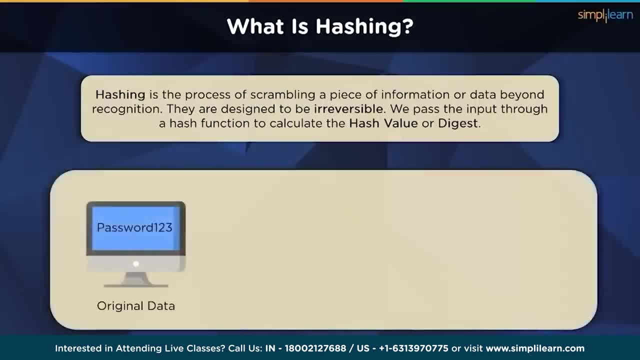 We can achieve this by using hash functions, which are essentially algorithms that perform mathematical operations on the main plain text. The value generated after passing the plain text information through the hash function is called the hash value digest or, in general, just the hash of the original data. 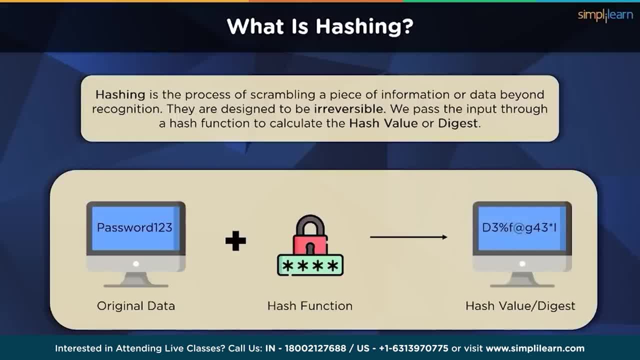 While this may sound similar to encryption, the major difference is hashes are made to be irrelevant and reversible. No decryption key can convert a digest back to its original value. However, a few hashing algorithms have been broken due to the increase in computational complexity of today's new generation. 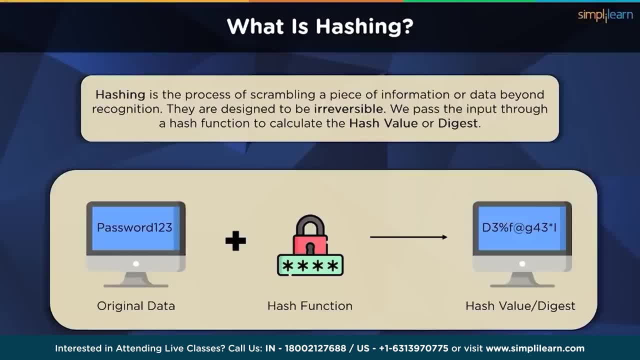 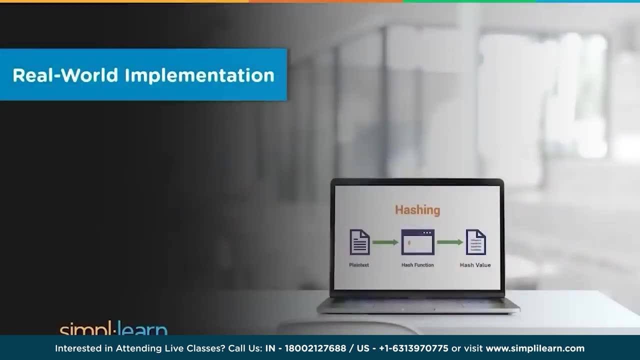 computers and processors. There are new algorithms that stand the test of time and are still in use among multiple areas for password storage, identity verification, etc. Like we discussed earlier, websites use hashing to store the user's passwords, So how do they make use of? 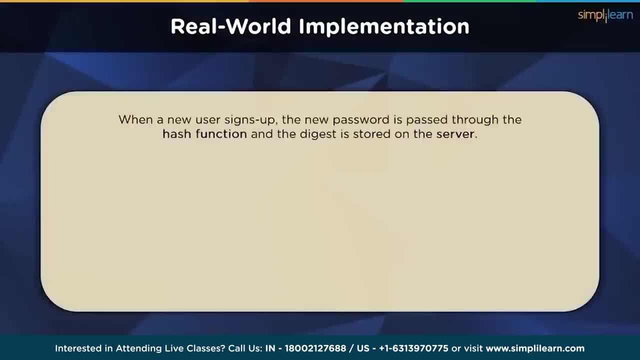 these hash passwords. When a user signs up to create a new account, the password is then run through the hash function and the resulting hash value is stored on the servers. So the next time a user comes to login to the account, the password he enters is passed through the same. 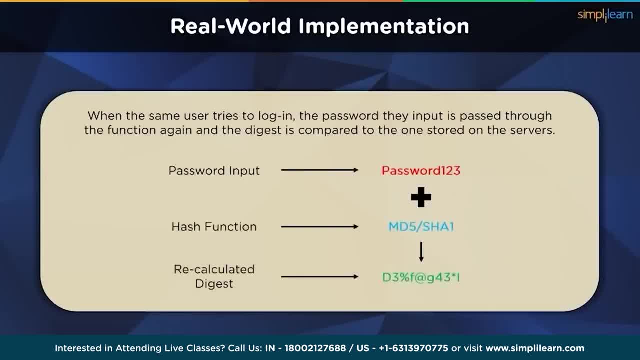 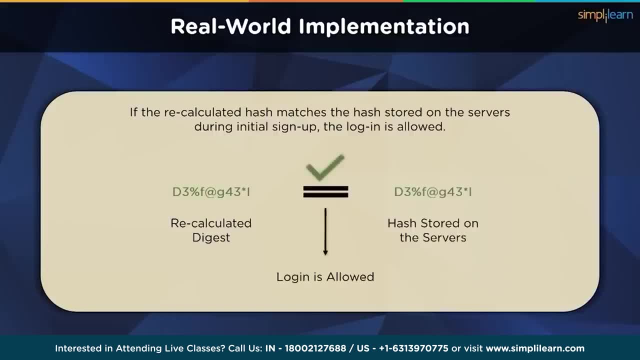 hash function and compared to the hash stored on the main server. If the newly calculated hash is the same as the one stored on the website server, the password must have been correct because, according to hash function's terminology, same inputs will always provide the same. 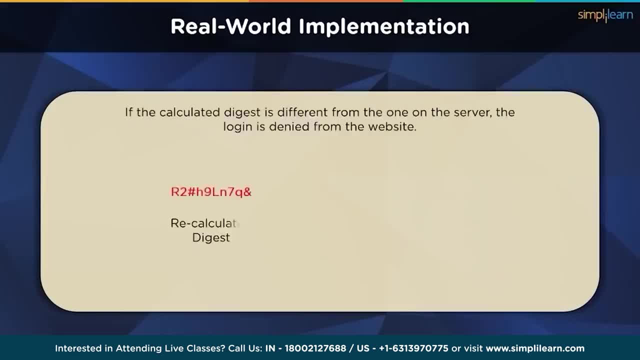 outputs. If the hashes do not match, then the password entered during login is not the same as the password entered during the signout. hence the login will be denied. This way, no plain text passwords get stored, preventing both the owner from snooping on user. 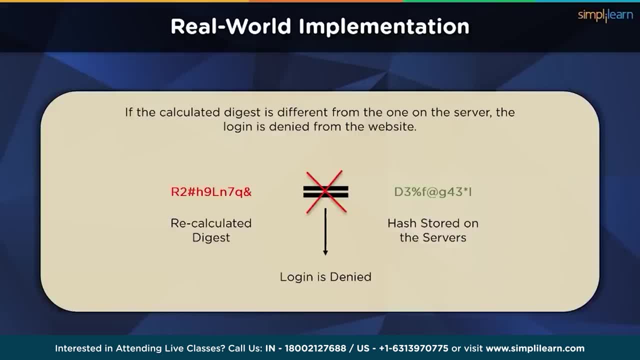 data and protecting user's privacy in the unfortunate event of a data breach or a hack. Apart from password storage, hashing can also be used to perform integrity checks. When a file is uploaded on the internet, the file's hash value is generated and it is uploaded. 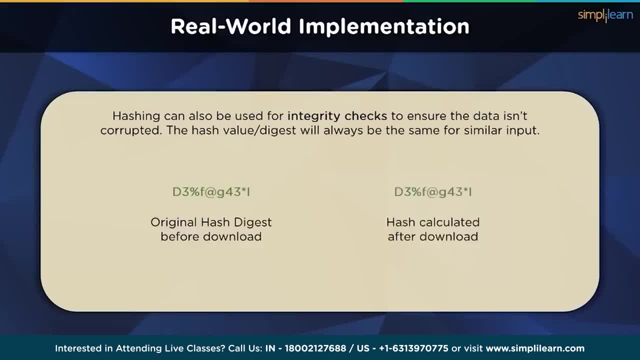 along with the original information. When a new user downloads the file, he can calculate the digest of the downloaded file using the same hash function When the hash values are compared, if they match, then file integrity has been maintained and there has been no data. 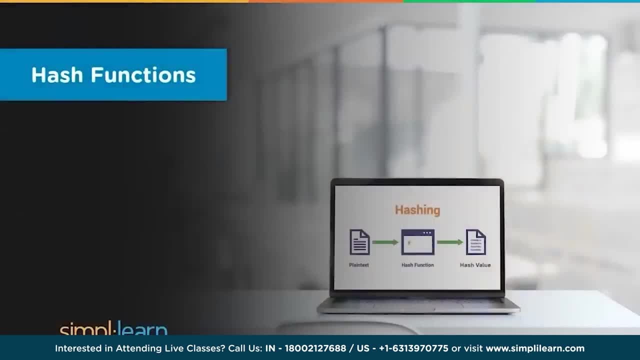 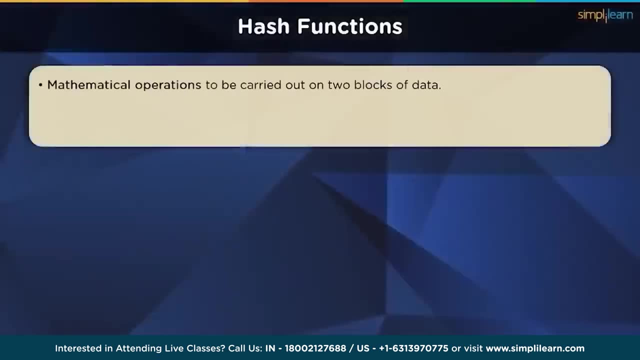 corruption. Since so much important information is being passed onto the hash function, we need to understand how they work. A hash function is a set of mathematical calculations operated on two blocks of data. The main input is broken down into two blocks of similar size. The block, 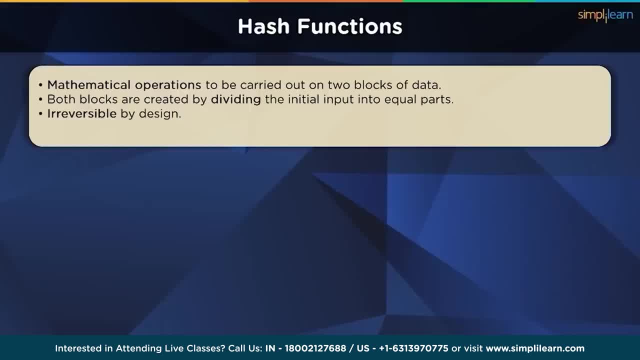 size is dependent on the algorithm that is being used. Hash functions are designed to be one way. They shouldn't be reversible, at least by design. Some algorithms, like the previously mentioned MD5, have been compromised, but more secure algorithms are being used today, like the SHA family of algorithms. 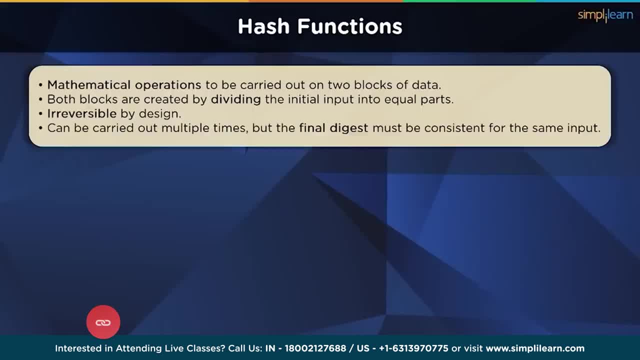 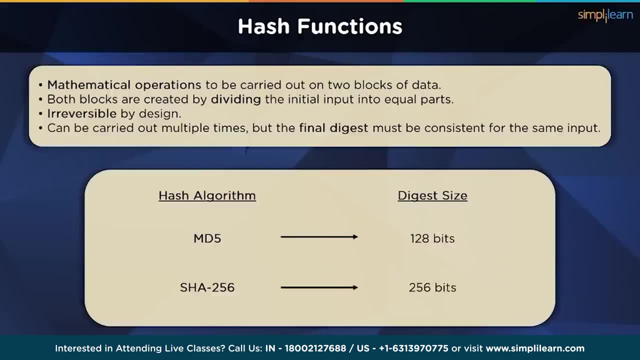 The digest size is also dependent on the respective algorithm being used. MD5 has a digest of 128 bits, while SHA-256 has a digest of 256 bits. This digest must always be the same for the same input, irrespective of how many times the 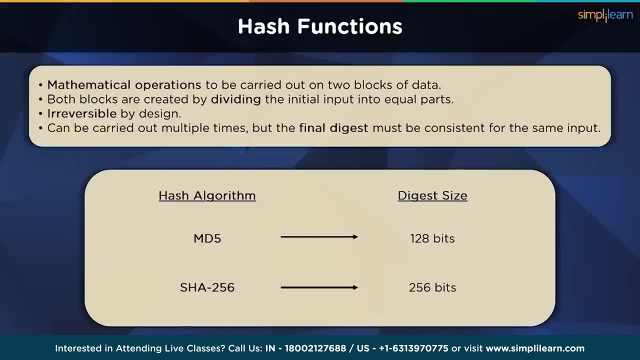 calculations are carried out. This is a very crucial feature, since comparing the hash value is the only way to check if the data is untouched, as the functions are not reversible. So there are certain requirements of a hash function that need to be met before they are. 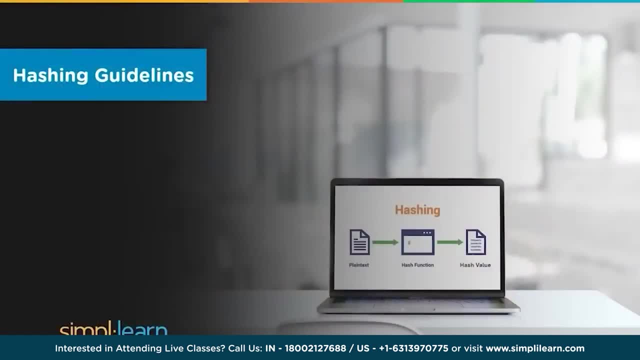 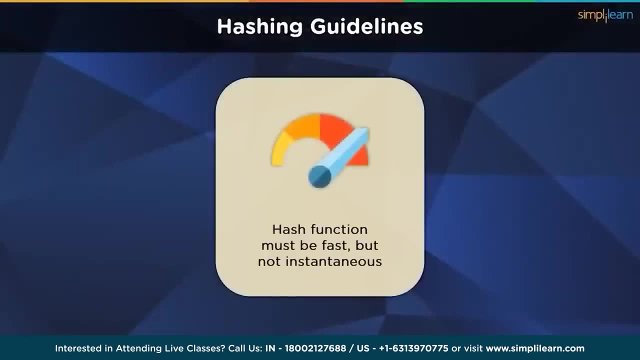 accepted. While some of them are easy to guess, others are placed in order to preserve security in the long run. The hash function must be quick enough to encrypt large amounts of data at a relatively fast pace, but it also shouldn't be very fast. 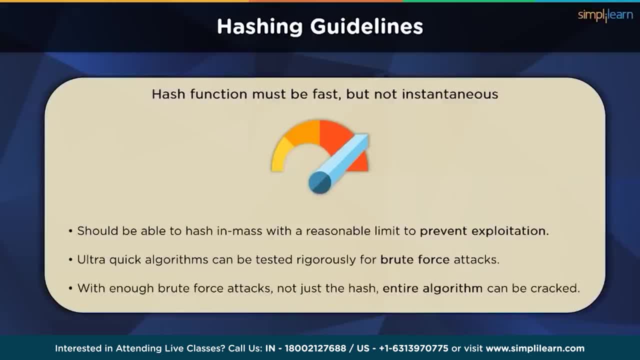 Running the algorithm on all cylinders makes the functions easy to goodforce and a security liability. There must be a balance to allow the hash function to handle large amounts of data and not make it ridiculously easy to bruteforce by running through all the possible combinations. 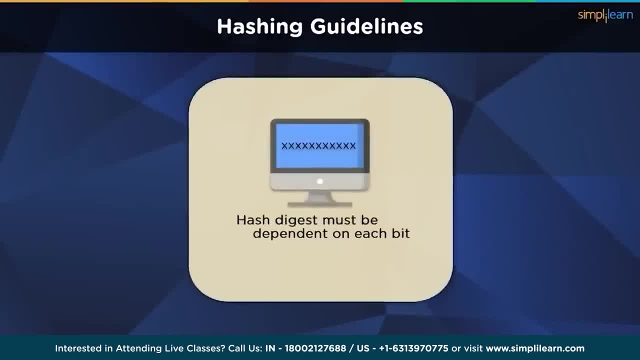 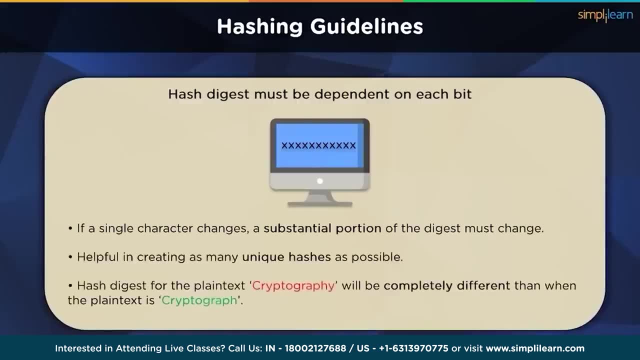 The hash function must be dependent on each bit of the input. The input can be text, audio video or any other file extension. If a single character is being changed, it doesn't matter how small that character may be. the entire digest must have a distinctly 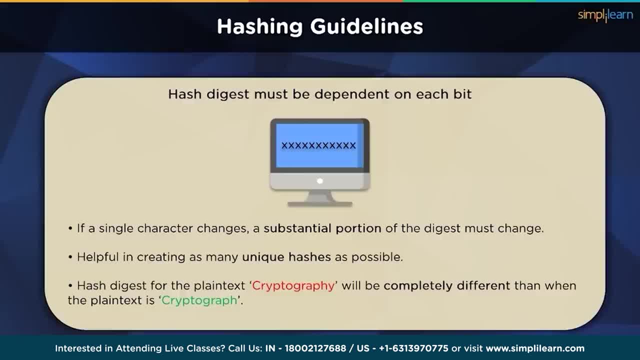 different hash value. This is essential to create unique digests for every password that is being shown. But what if two different users are using the same password? Since the hash function is the same for all users, both the digests will be the same. This is called. 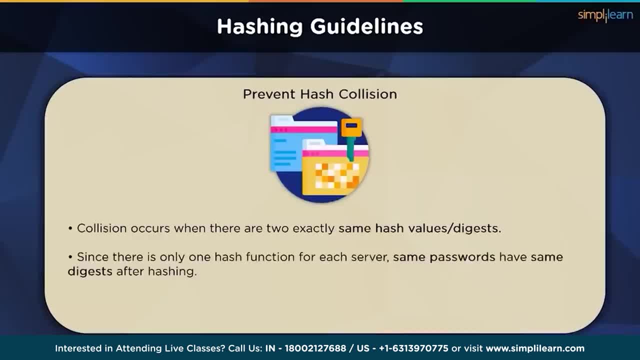 a hash collision. You may think this must be a rare occasion where two users have exactly the same password, but that is not the case. We have techniques like salting that can be used to reduce these hash collisions, as we will discuss later in this video. 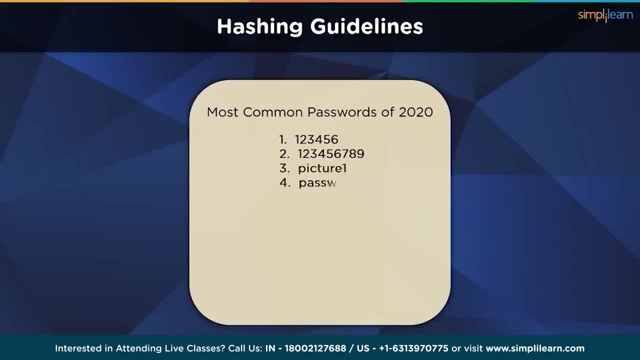 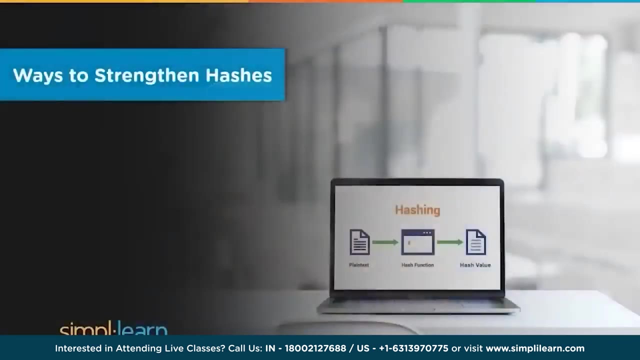 You would be shocked to see the most used passwords of 2020.. All of these passwords are laughably insecure and since many people use the same passwords repeatedly on different websites, hash collisions risks are more common than one would expect. Let's say the hash functions find. 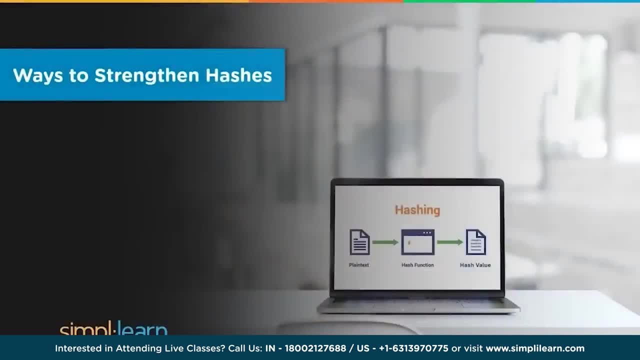 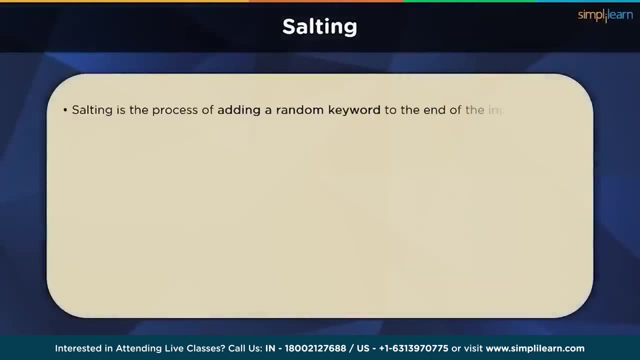 two users having the same password, How can they store both the hashes without messing up the original data? This is where salting and peppering come to play. Salting is the process of adding a random keyword to the end of the input before it is passed on to the hash. 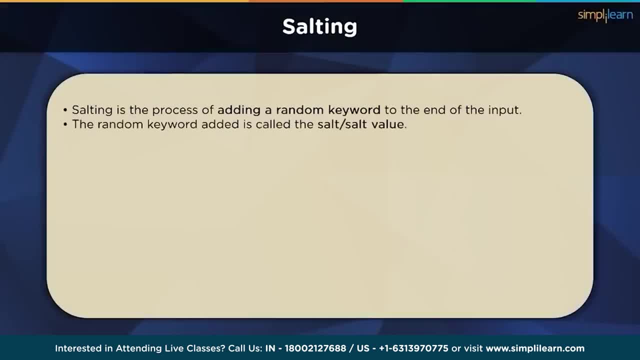 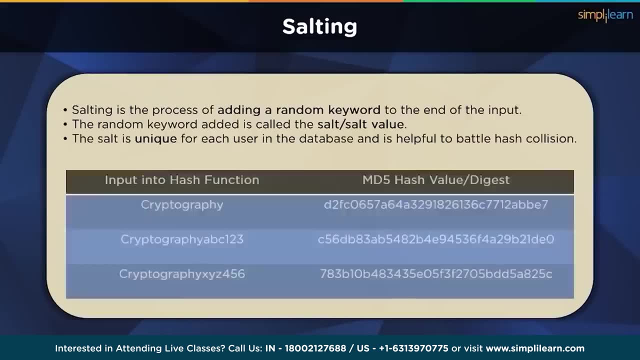 function. This random keyword is unique for each user on the system, and it is called the salt value or just the salt, So even if two passwords are exactly the same, their salt value will differ, and so will their digest. There is a small problem with this process, though. 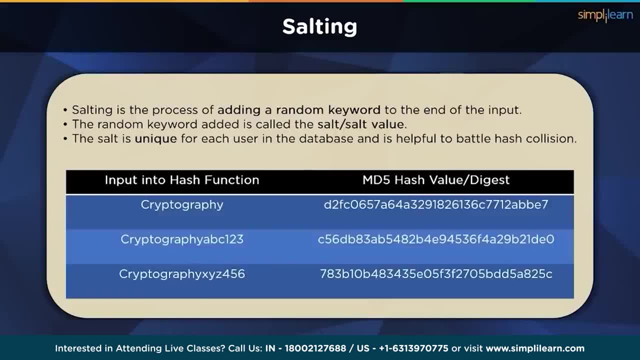 Since the salt is unique for each user, they need to be stored in the database, along with the passwords and sometimes even in plain text, to speed up the process of continuous verification. If the server is hacked, then the hashes will need to be brute-forced, which takes a lot of time. 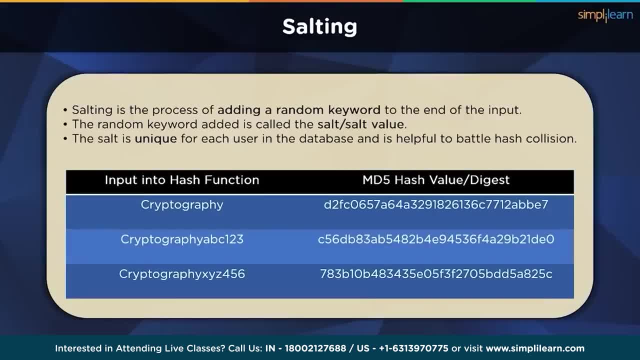 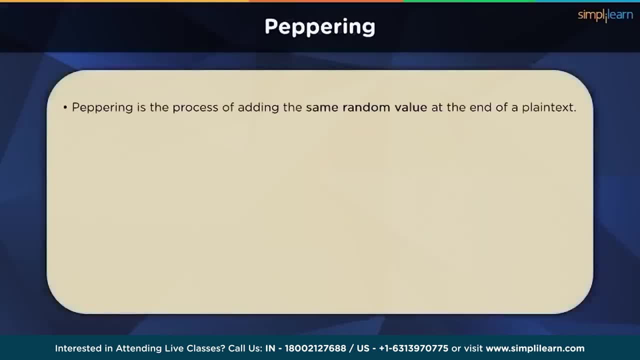 But if they receive the salts as well, the entire process becomes very fast. This is something that peppering aims to solve. Peppering is the process of adding a random string of data to the input before passing them to the hash function, But this time the random string is not. 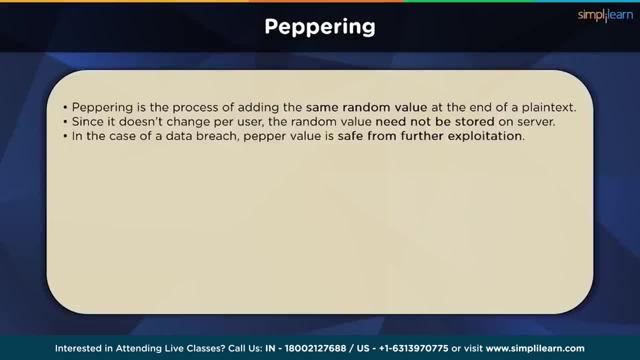 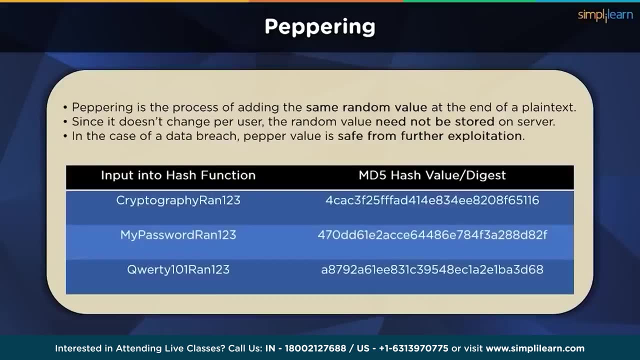 unique for each user. It is supposed to be common for all users in the database and the extra bit added is called the pepper. in this case, The pepper isn't stored on the server. it is mostly hard-coded onto the website's source code, since 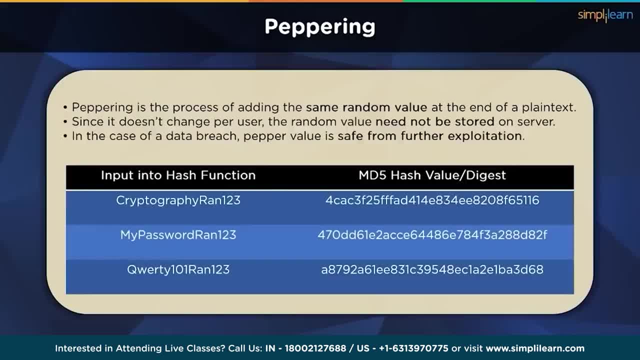 it's going to be the same for all credentials. This way, even if the servers get hacked, they will not have the right pepper needed to crack into all the passwords. Many websites use a combination of salting and peppering to solve the problem. 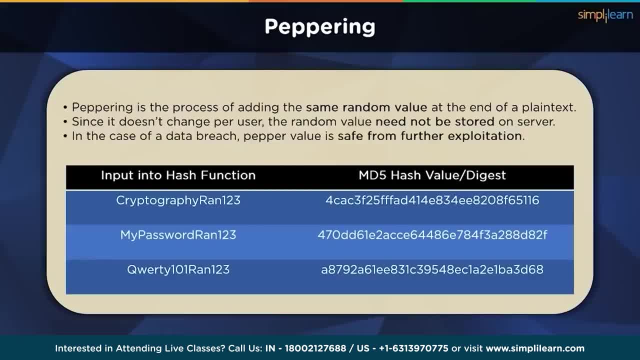 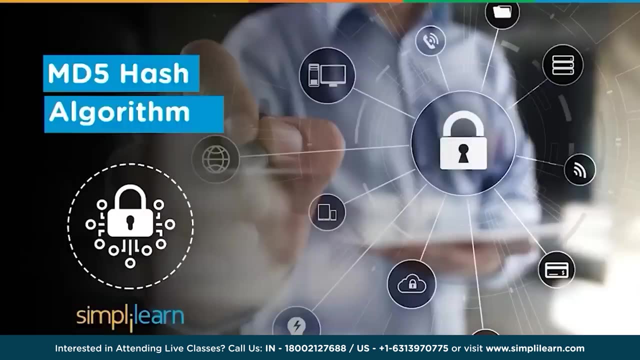 of hash collision and bolster security. Since brute-force takes such a long time, many hackers avoid taking the effort. The returns are mostly not worth it and the possible combinations of using both salting and peppering is humongous. With the consensus aiming towards an 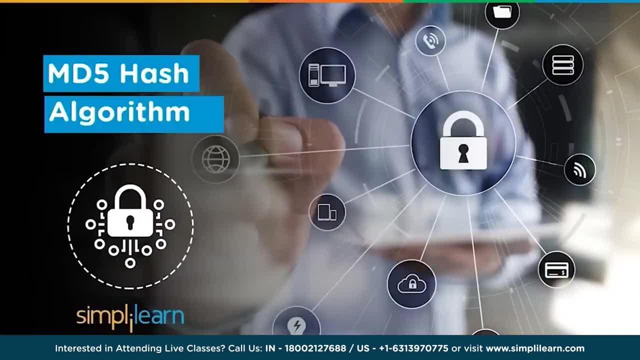 educated public on digital privacy. it's no surprise to see an increasing interest in encryption algorithms. We have already covered the major names like the DES and the AES algorithm. MD5 algorithm was one of the first hashing algorithms to take the global stage as a successor to the MD4. 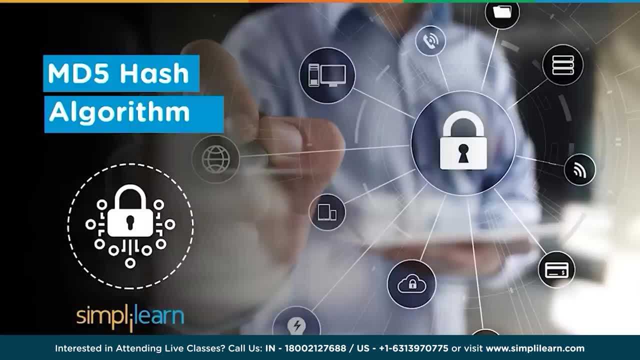 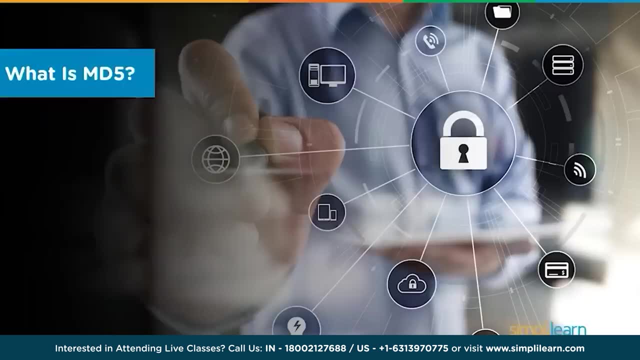 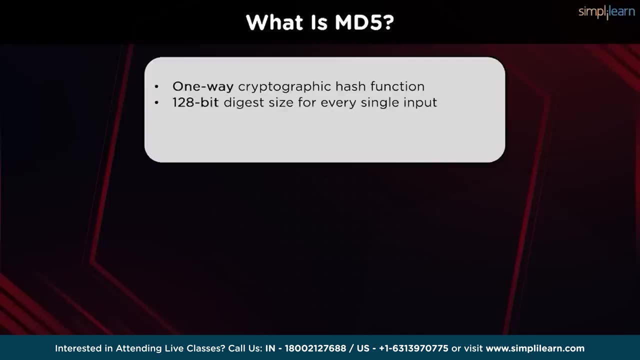 Despite the security vulnerabilities encountered in the future, MD5 still remains a crucial part of data infrastructure in a multitude of environments. The MD5 hashing algorithm is a one-way cryptographic function that accepts a message of any length as input and it returns as output a fixed length. 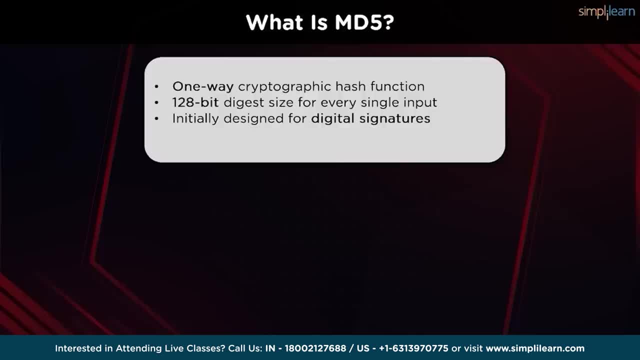 digest value to be used for authenticating the original messages. The digest size is always 128 bits, irrespective of the input. The MD5 hash function was originally designed for use as a secure cryptographic hash algorithm to authenticate digital signatures. MD5 has also. 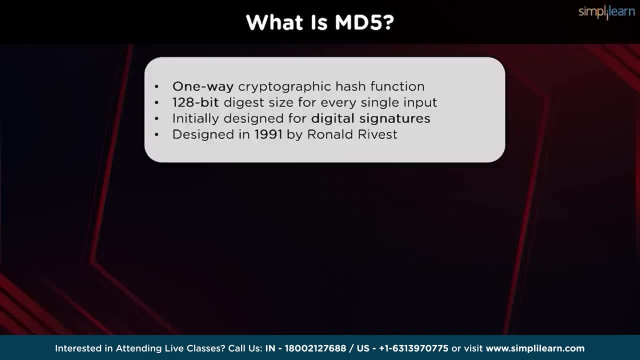 been depreciated for uses other than as a non-cryptographic checksum to verify data integrity and detect unintentional data corruption. Ronald Rivest, founder of RSA Data Security and Institute professor at MIT, designed MD5 as an improvement to a prior message digest algorithm. 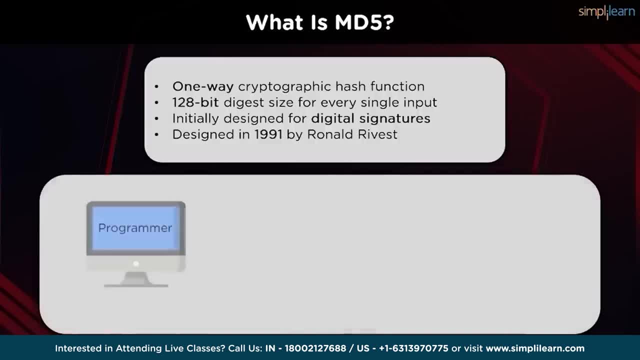 which was the MD4.. As already iterated before, the process is straightforward. We pass a plain text message to the MD5 hash function, which in turn performs certain mathematical operations on the clear text to scramble the data The 128-bit digest received from this. 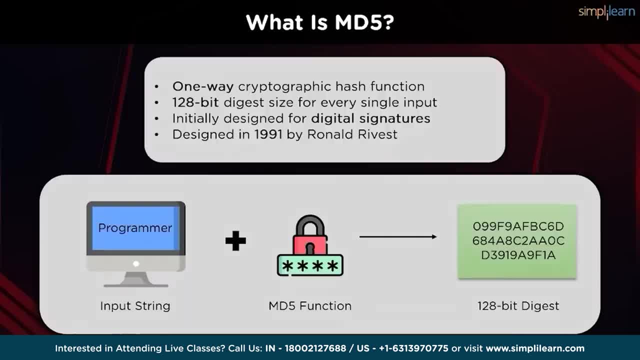 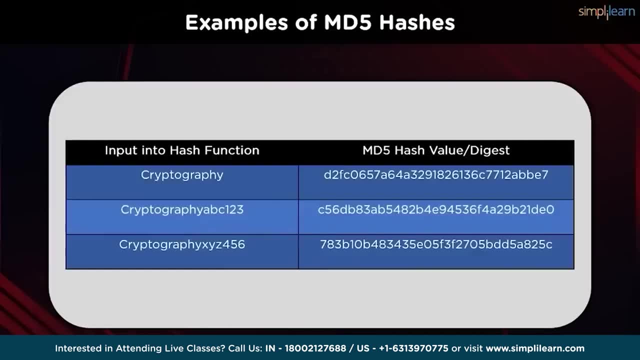 is going to be radically different from the plain text. The goal of any message digest function is to produce digests that appear to be random To be considered cryptographically secure. the hash function should meet two requirements. First, that it is impossible for an attacker 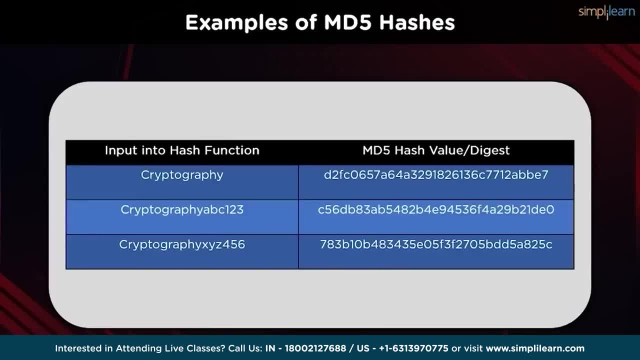 to create a message that matches a specific hash value and second, that it is impossible for an attacker to create two messages that produce the same hash value. Even a slight change in the plain text should trigger a drastic difference in the two digests. 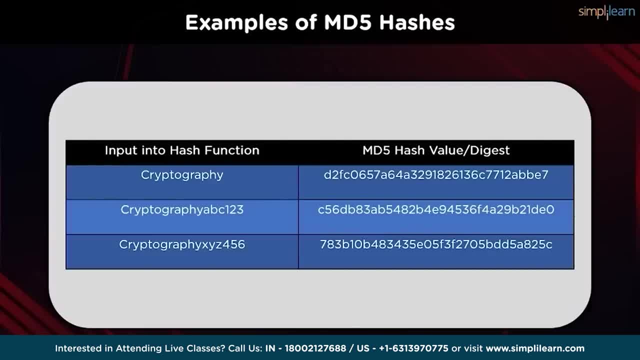 This goes a long way in preventing hash collisions which take place when two different plain texts have the same digest. To achieve this level of intricacy, there are a number of steps to be followed before we receive the digest. We will look at the detailed procedure. 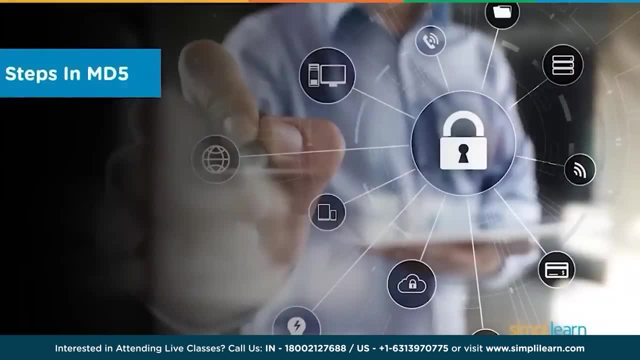 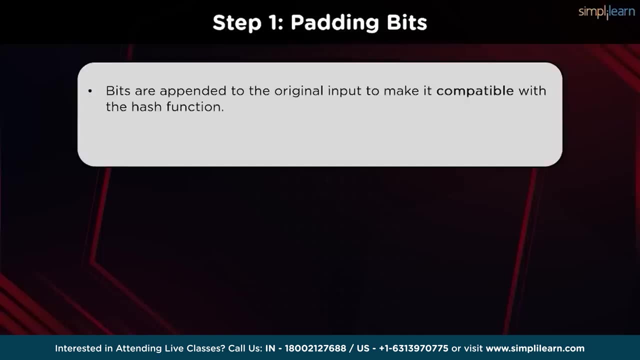 as to how the MD5 hash algorithm works. The first step is to make the plain text compatible with the hash function. To do this, we need to pad the bits in the message. When we receive the input string, we have to make sure the size is 64 bits. 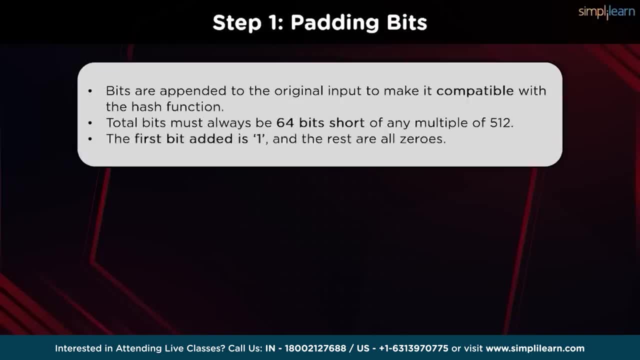 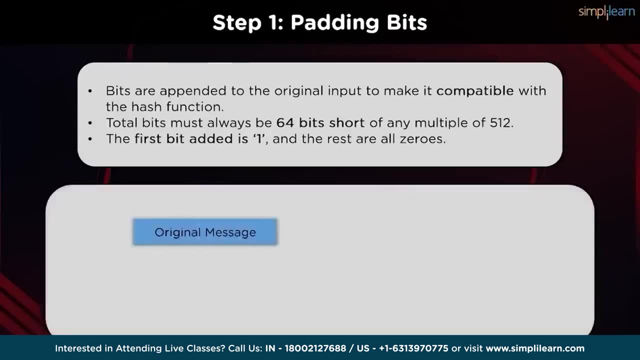 short of a multiple of 512.. When it comes to padding the bits, we must add one first, followed by zeros, to round out the extra characters. We need to have a length of just 64 bits, less than any multiple of 512. 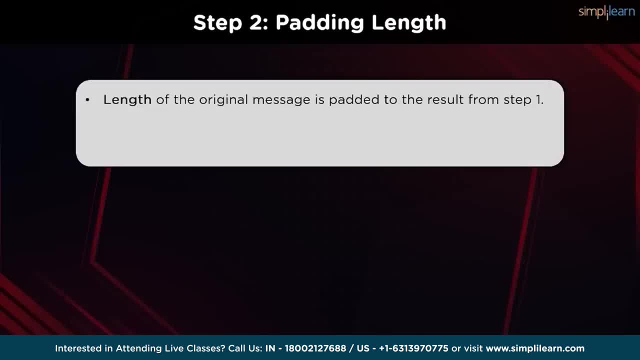 Here on out we can proceed on to the next step, where we have to pad the length bits. Initially in the first step we appended the message in such a way that the total length of the bits in the message was 64 bits short of any multiple of 512. 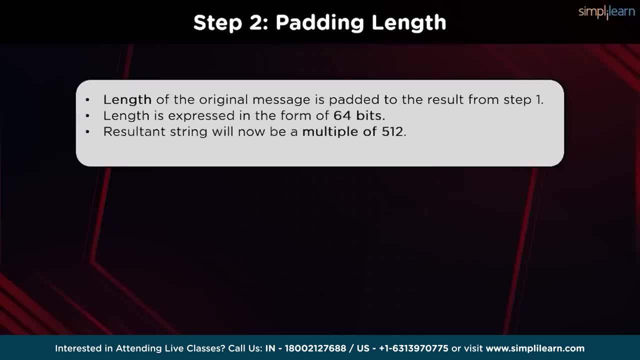 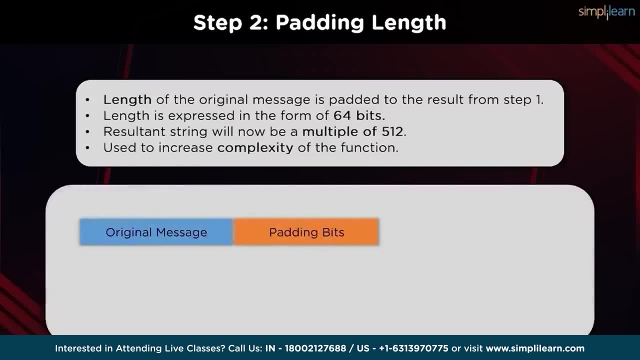 Now we add the length bits in such a way that the total number of bits in the message is perfectly a multiple of 512. That means 64 bits- lengths, to be precise, are added to the message. Our final string to be hashed is now a definite multiple of 512. 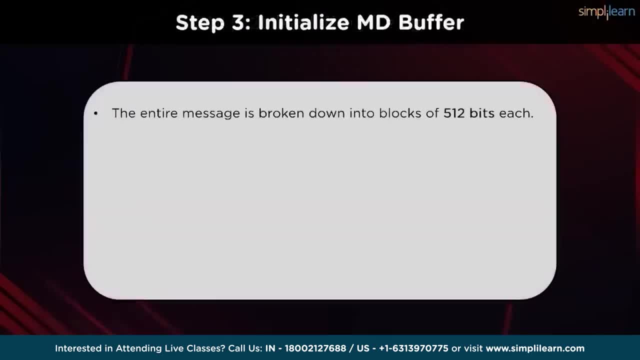 The next step would be to initialize the message digest buffer. The entire hashing plain text is now broken down into 512-bit blocks. There are four buffers or registers that are of 32 bits each, named A, B, C and D. There are four buffers or registers. 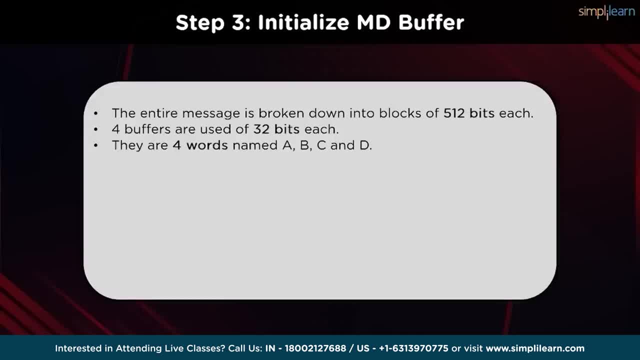 that are of 32 bits each, named A, B, C and D. These are the four words that are going to store the values of each of these sub-blocks. The first iteration to follow these registers will have fixed hexadecimal values, as shown on the screen below. 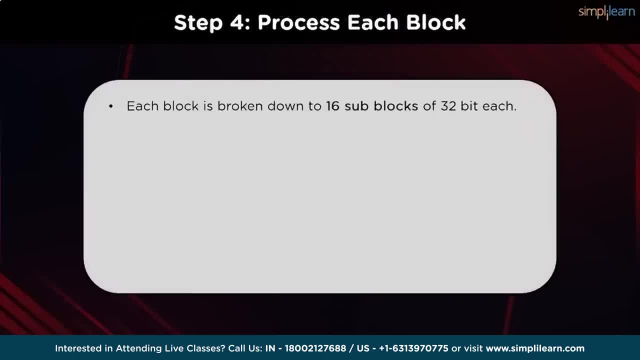 Of these 512 blocks, we can divide each of them into 16 further sub-blocks of 32 bits each. For each of these sub-blocks we need to have the four buffer variables A, B, C and D. These rounds require the other. 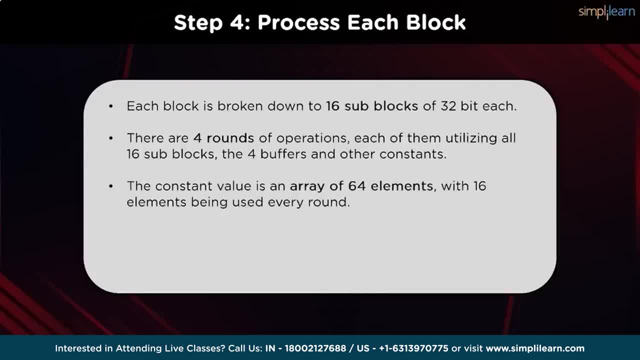 constant variables as well, which differ with each round of operation. The constant values are stored in a random array of 64 elements. Since each 32-bit sub-block is run 4 times 16 such sub-blocks equal 64 constant values needed. 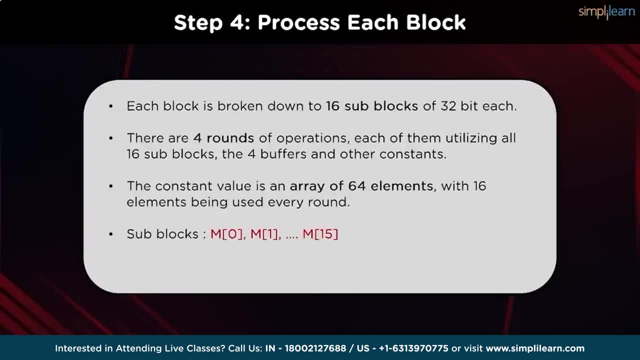 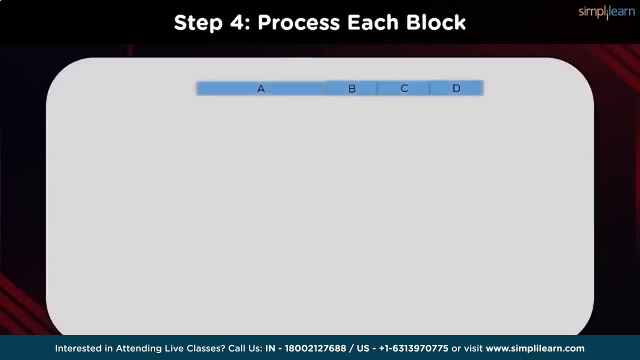 for a single block iteration, The sub-blocks can be denoted by the alphabet M and the constant values are denoted by C. Coming to the actual round of operation, we see our four buffers which already have pre-initialized values for the first iteration. 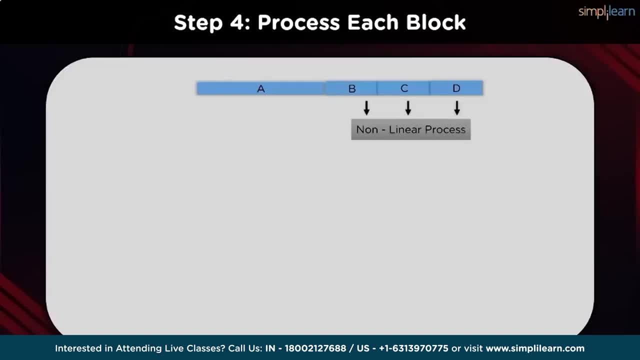 At the very beginning, the values of buffers B, C and D are passed on to a non-linear logarithmic function. The formula behind this function changes by the particular round being worked on, as we shall see later in this video, Once the output is calculated. 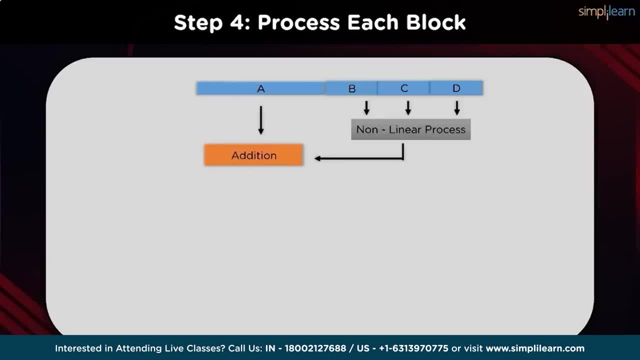 it is added to the raw values stored in buffer A. We now have a 32-bit sub-block using which we are running the four operations. The output of this requisite function then needs to be added to a constant value derived from the constant array K. 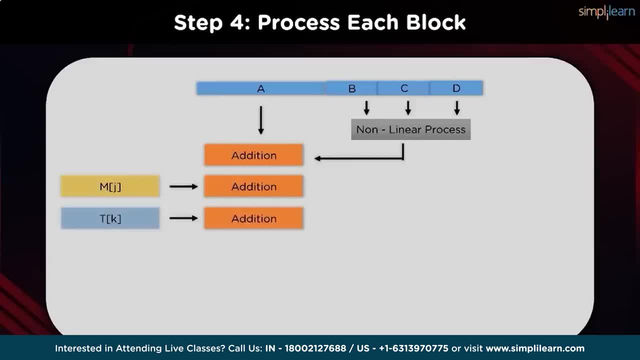 Since we have 64 different elements in the array, we can use a distinct element for each iteration of a particular block. The next step involves a circular shift that increases the complexity of the hash algorithm to create a unique digest for each individual input. The output generated is later added. 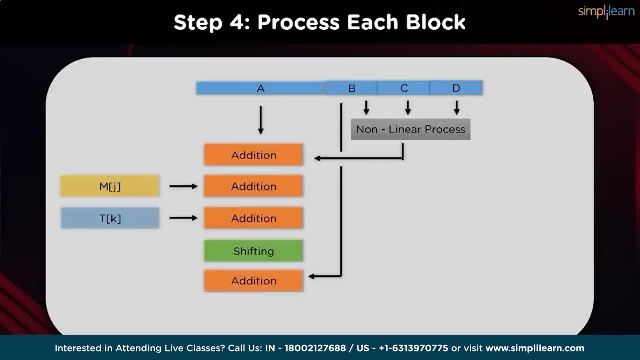 to the values stored in buffer B. The final output is now stored in the second buffer of B of the output register. Individual values of C, D and A are derived from the preceding element before the iteration started, meaning the value of B gets stored in C. 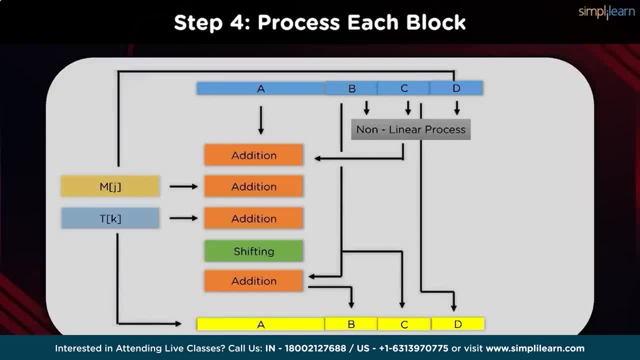 value of C gets stored in D and the value of D in A. Now that we have a full register ready for this sub-block, the values of A, B, C, D are moved on as input to the next sub-block Once all 16 sub-blocks are completed. 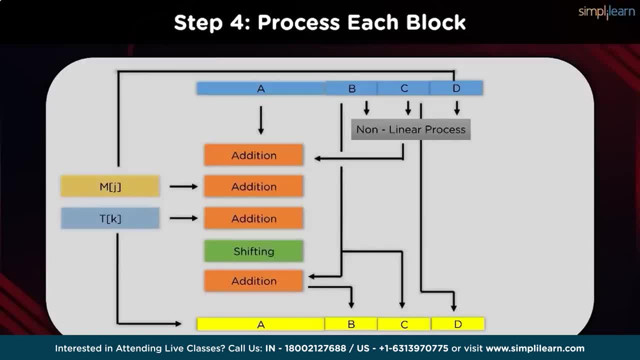 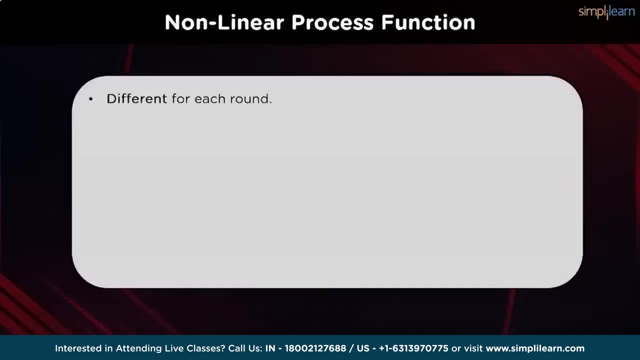 the final register value is saved and the next 512-bit block begins. At the end of all these blocks, we get a final digest of the MD5 algorithm. Regarding the non-linear process mentioned in the first step, the formula changes for each round it's being run on. 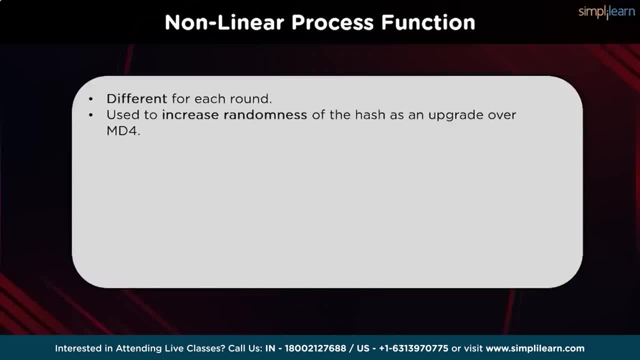 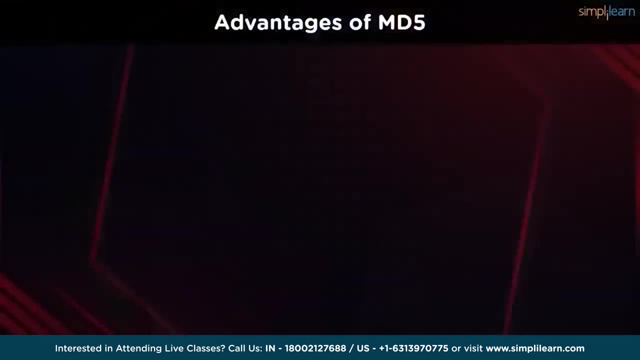 To increase the functional complexity of the algorithm and to increase randomness of the procedure, the formula for each of the four rounds uses the same parameters, that is, B, C and D, to generate a single output. The formulas being used are shown on the screen right now. 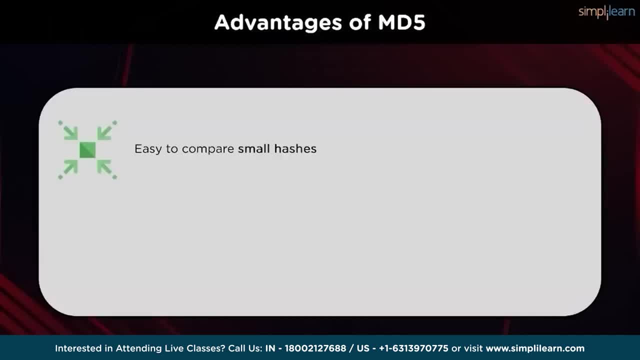 Unlike the latest hash algorithm families, a 32-bit digest is relatively easier to compare when verifying the digests. They don't consume a noticeable amount of disk storage, so it's important to remember and reiterate. Passwords need not be stored in plain text format. 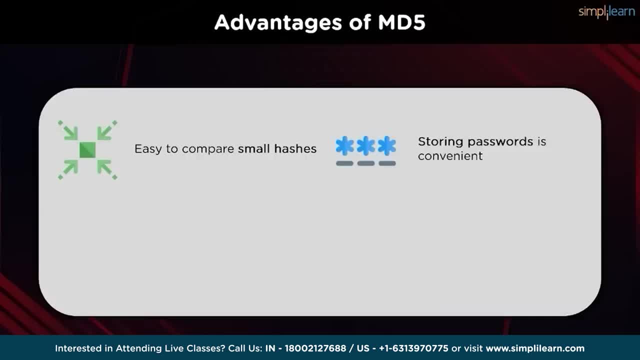 making them accessible for hackers and malicious actors. When using digest, the database security also gets a boost, since the size of all the hash values will be the same. In the event of a hack or a breach, the malicious actor will only receive the hashed values. so there is no way. 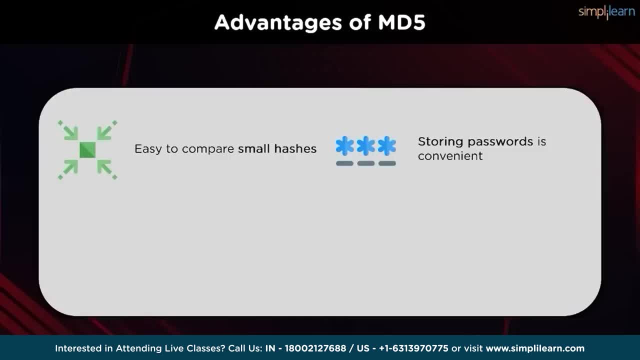 to regenerate the plain text, which would be the user passwords in this case. This is irreversible by design. Hashing has become a compulsion when storing user credentials on the server. nowadays, A relatively low memory footprint is necessary when it comes to integrating multiple services. 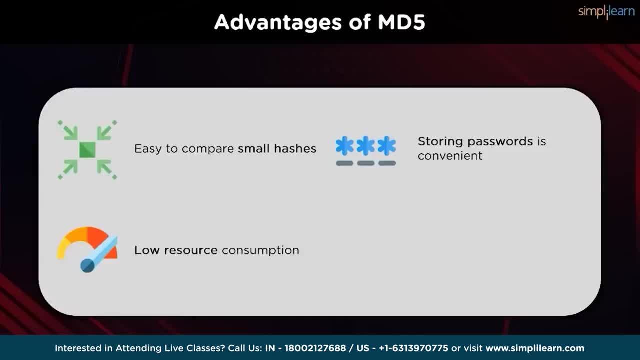 into the same framework without a CPU overhead. The digest size is the same and the same steps are run to get the hash value, irrespective of the size of the input string. This helps in creating a low requirement for computational power on older hardware, which is pretty common in server farms. 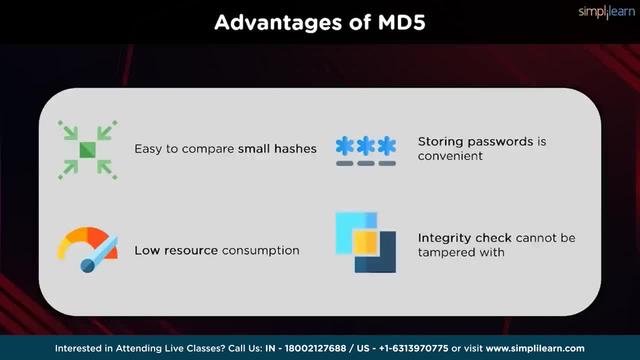 around the world. We can monitor file corruption by comparing hash values before and after transit. Once the hashes match, file integrity checks are valid and we can avoid data corruption. Hash functions will always give the same output for the similar input, irrespective of the iteration parameters. 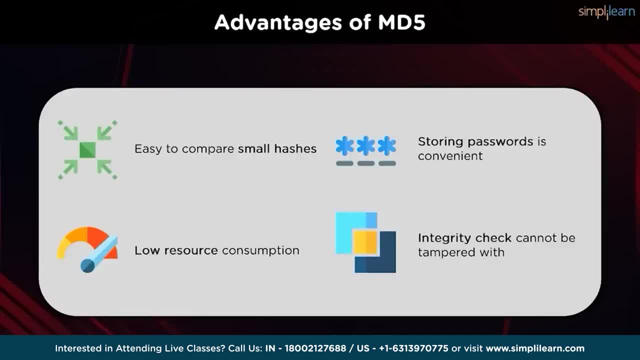 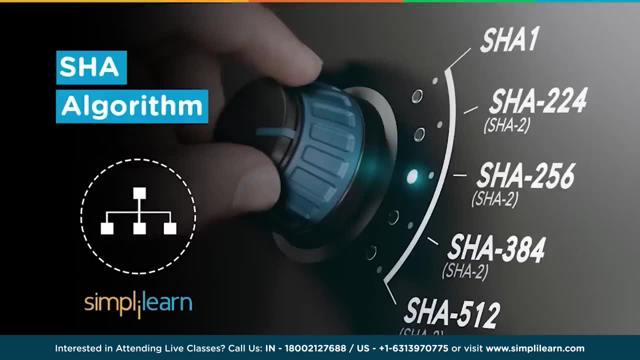 It also helps in ensuring that the data hasn't been tampered with and we don't root to the receiver of the message. We use our Wi-Fi every day for work and we use the Internet for entertainment and communication. The dependency on technology is at an all-time high. 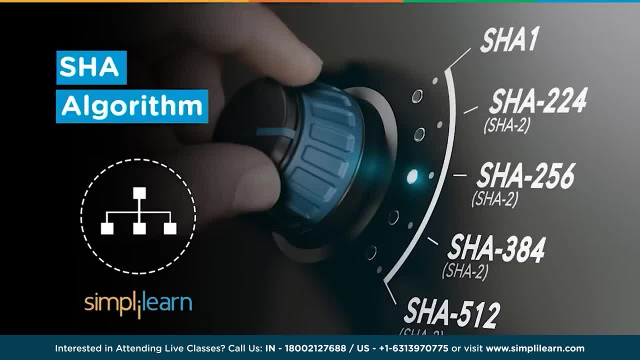 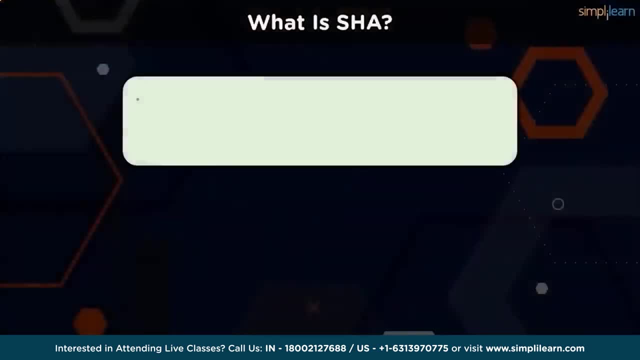 thanks to the radical developments and innovation in these last two decades. A big portion of this belongs to ensuring secure channels of communication and data transmission. The secure hash algorithms are a family of cryptographic hash functions that are published by the National Institute of Standards and Technology. 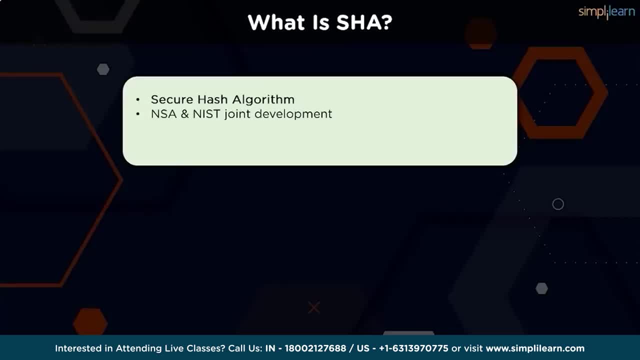 along with the NSA, It was passed as a Federal Information Processing Standard, also known as FIPS. It has four different families of hash functions. SHA0 is a 160-bit hash function published in 1993, and it was closed down later after an undisclosed. 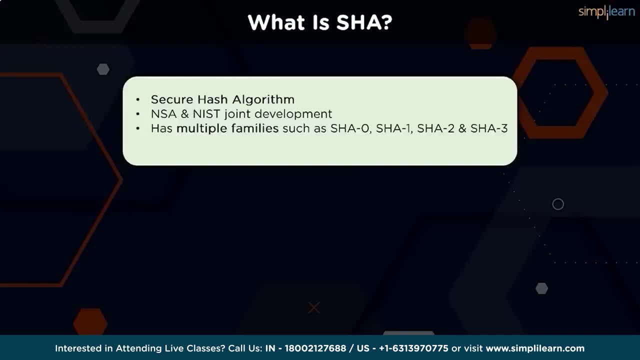 significant flaw. SHA1 is also a 160-bit hash function which resembles the earlier MD5 algorithm. This was designed by the NSA to be a part of the digital signature algorithm. SHA2 is a family of two similar hash functions with different block sizes. 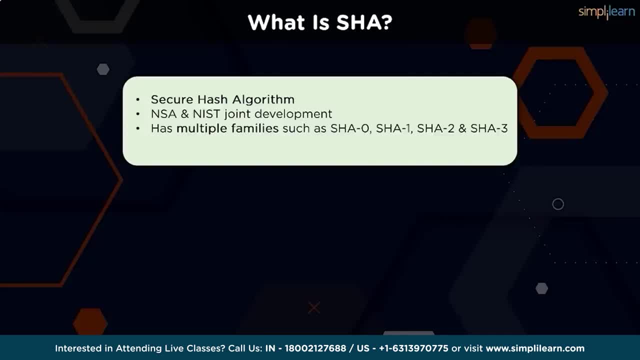 known as the SHA256 and the SHA512.. They differ in the word size. SHA256 uses 32-bit words, while SHA512 uses 64-bit words. SHA3 is a hash function, properly known as KCAC. It was chosen in 2018. 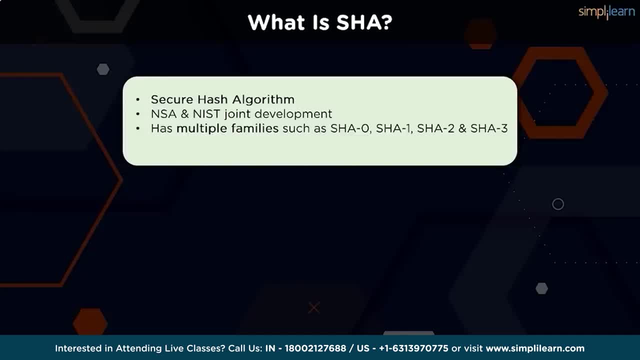 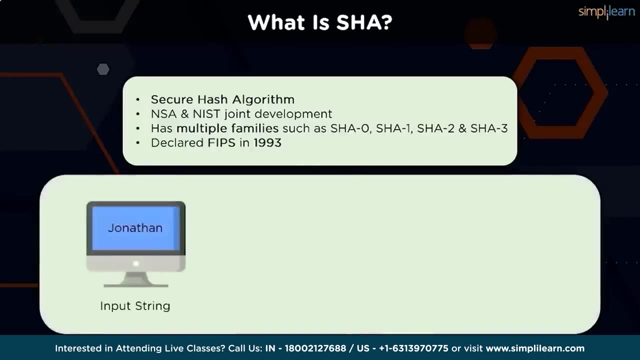 after a public competition among non-NSA designers. It supports the same hash lengths as SHA2 and its internal structure differs significantly from the rest of the SHA family. As we have already iterated, the process is straightforward: We pass a plain text message to the SHA. 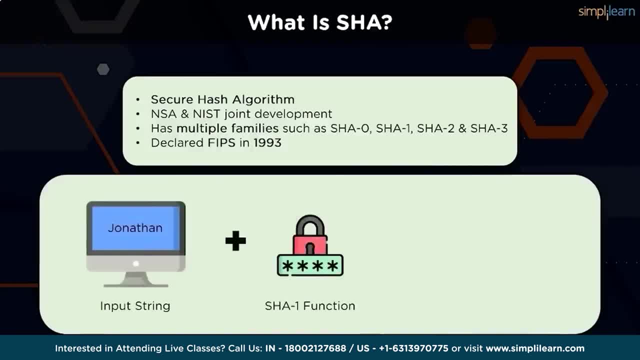 hash function which in turn performs certain mathematical operations on the clear text to scramble the data. The 160-bit digest received from this is going to be radically different from the plain text. The goal of any hash function is to produce digests that appear to be random. 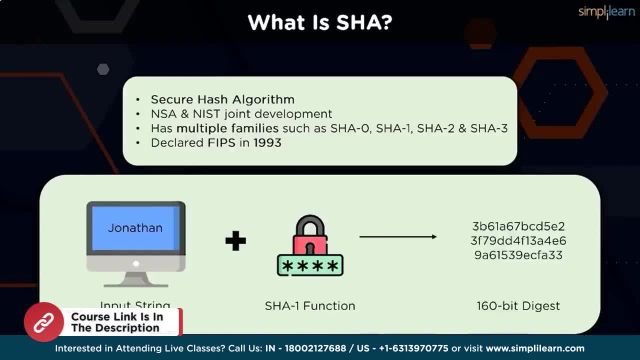 To be considered cryptographically secure, the hash function should meet two requirements: First, that it is impossible for an attacker to generate a message that matches a specific hash value. and, second, it should be impossible for an attacker to create two messages producing the exactly. 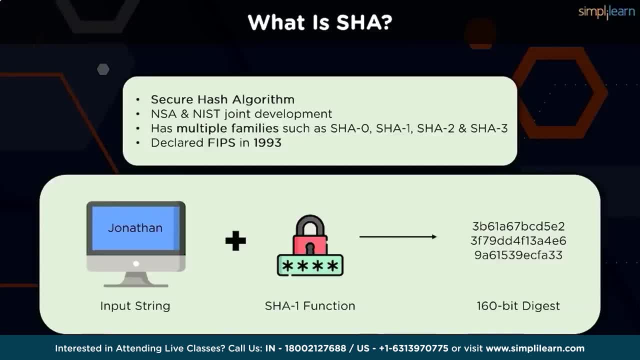 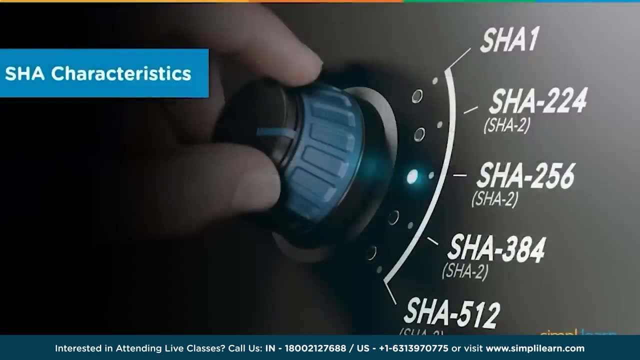 same hash value. Even a slight change in the plain text should trigger a drastic difference in the true digest. This goes a long way in preventing hash collisions which takes place when two different plain texts have the same digest. The SHA family functions have some characteristics that they need to follow. 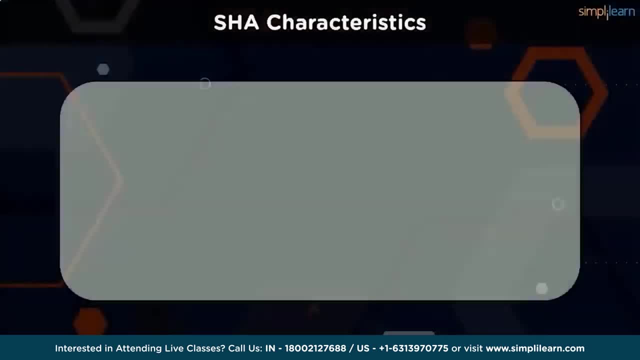 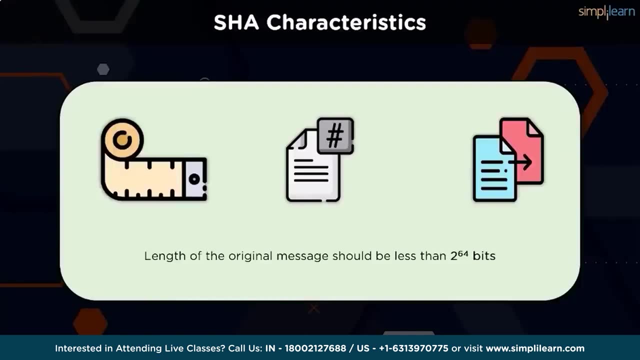 while generating the digests. Let's go through a few of them. The length of the clear text should be less than 2 to the power 64 bits in the case of SHA-1 and SHA-256.. This is essential to keep the plain text compatible. 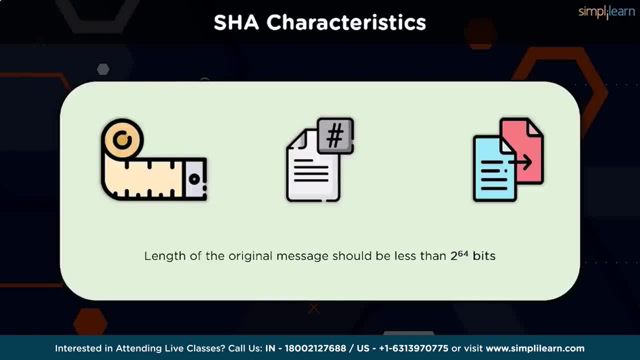 with the hash function and the size needs to be in comparison area. to keep the digest as random as possible, The length of the hash digest should be 256 bits in the SHA-256 algorithm, 512 bits in the SHA-512 algorithm, and so on. 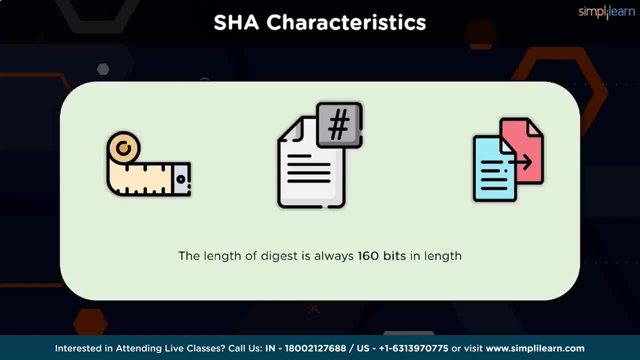 Bigger digest usually suggests significantly more calculations at the cost of speed and space. We typically go for the longest digest to bolster security, but there must be a definite balance between the speed and security of a hash function. By design, all hash functions of the SHA-512, SHA-256. 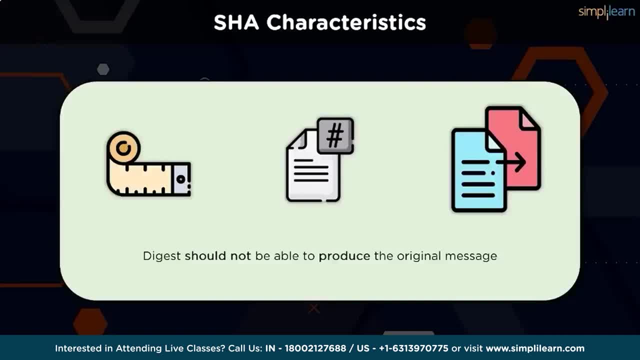 are irreversible. You should neither get a plain text when you have the digest beforehand, nor should the digest provide the original value when you pass it through the same hash function again. Another case of protection is that when the hash digest is passed into the SHA function, 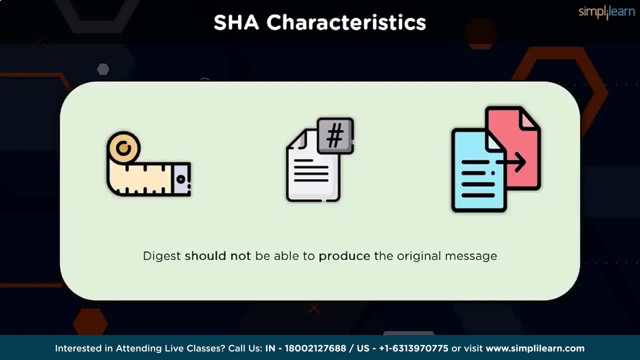 for a second time, we should get a completely different digest from the first instance. This is done to reduce the chance of brute force attacks. To achieve this level of intricacy, there are a number of steps to be followed before we receive the digest. Let us 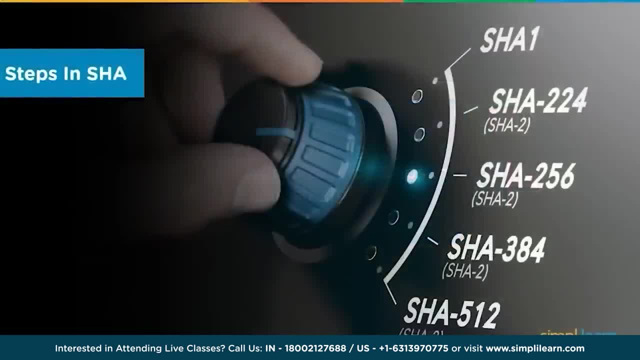 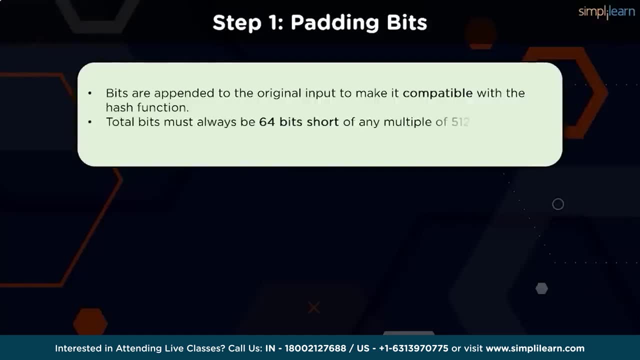 take a look at the detailed procedure as to how the SHA algorithm works. The first step is to make the plain text compatible with the hash function. To do this, we need to pad the bits in the message When you receive the input string. you have to make sure. 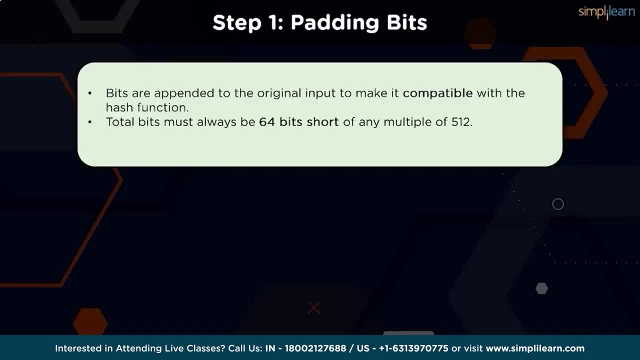 the size is 64 bits short of a multiple of 512.. When it comes to padding the bits, you must add one first, followed by the remaining zeros to round out the extra characters. This prepares our string to have a length just 64 bits, less than any. 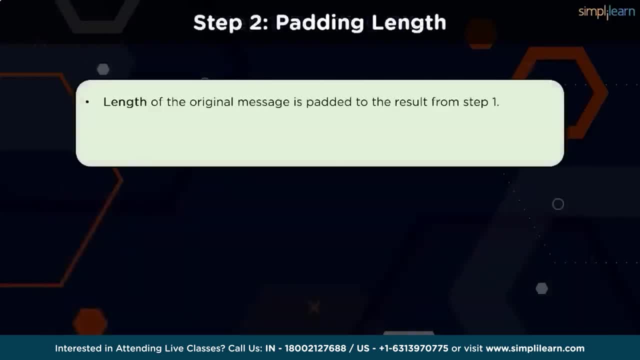 multiple of 512.. Here on out we can proceed to the next step, where we have to pad the length bits. Initially, in the first step, we appended the message in such a way that the total number of bits in the message was 64. 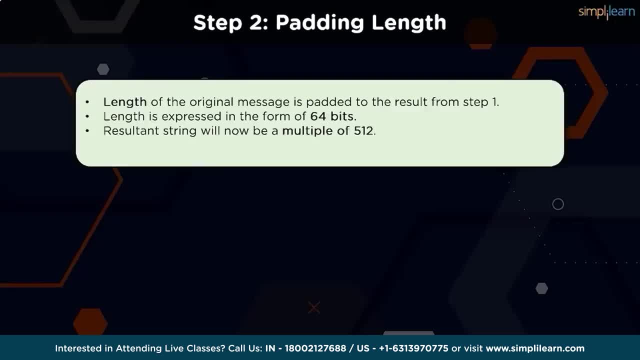 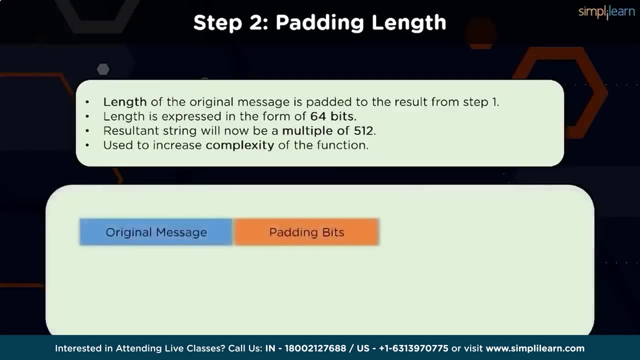 bits short from becoming a multiple of 512.. Now we add the length of bits in such a way that the total number of bits in the message is a perfect multiple of 512. That means 64 bits plus the length of the original message becomes a multiple. 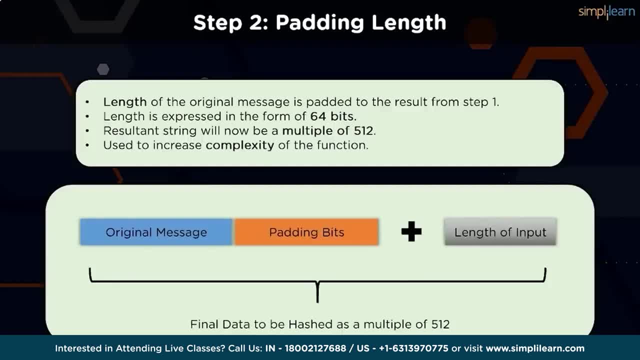 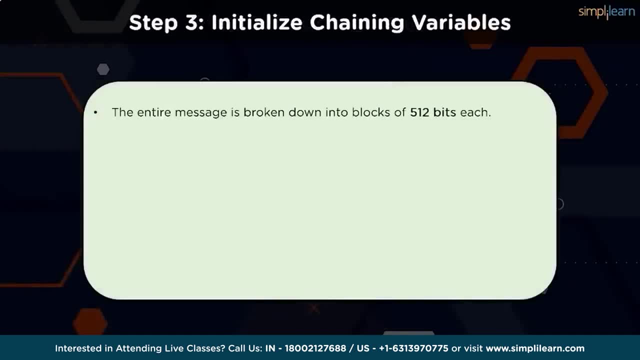 of 512.. This becomes a final string that needs to be hashed. In the next step, we have to initialize these chaining variables. The entire plain text message can now be broken down into blocks of 512 bits each, Unlike other hash algorithms like MD5. 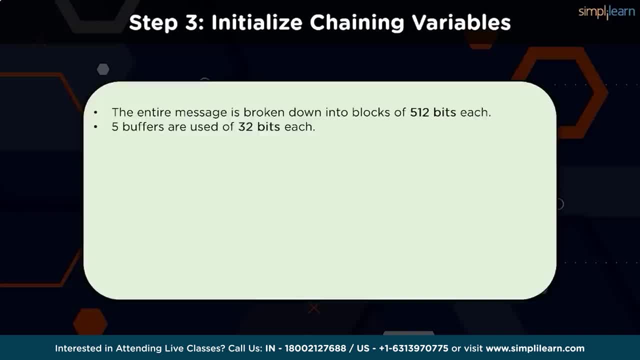 which use 4 registers or buffers. SHA family use 5 buffers of 32 bits each. They are named A, B, C, D and E. These registers go through multiple rounds of operation where the first iteration has fixed hexadecimal values, as can be seen in the screen. 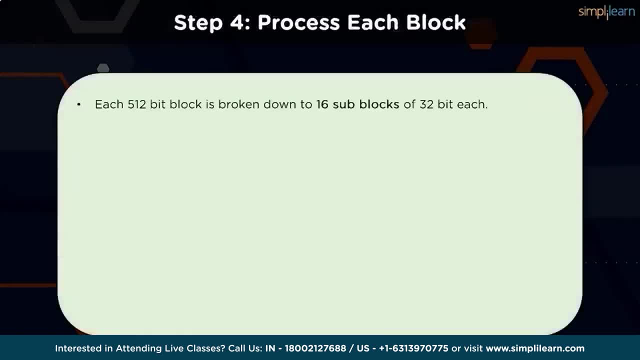 Moving on, we have to process each of the 512 bit blocks by breaking each of them into 16 sub-blocks of 32 bits each. Each of them goes through 4 rounds of operation that use the entire register and have the 512 bit block. 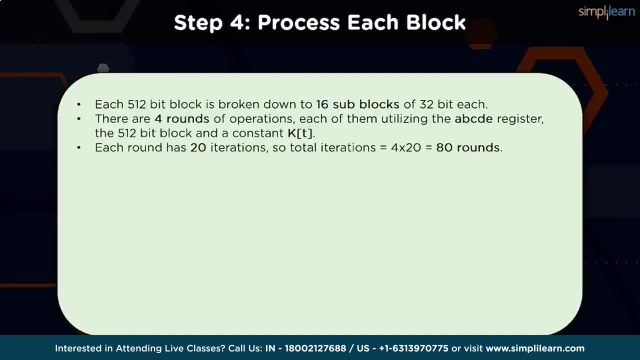 along with the constant array Out of those 4 rounds. each round has 20 iterations, So in general we have 80 rounds. sum total, The constant value of k is an array of 80 elements. Of those 80, 16 elements. 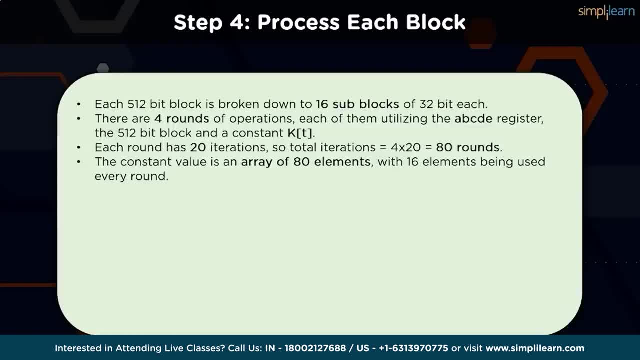 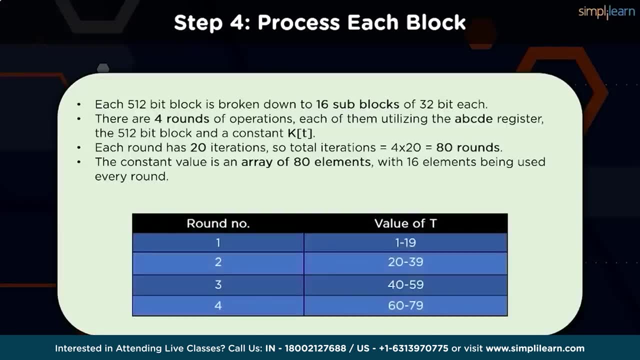 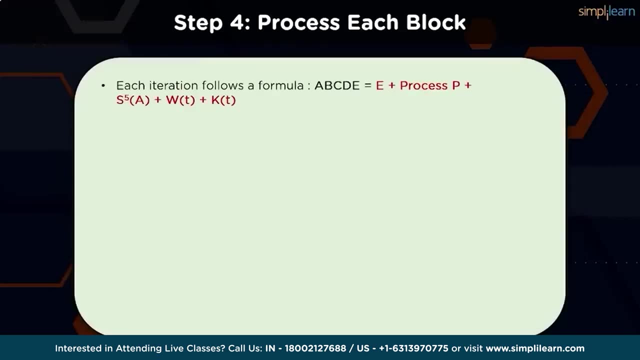 are being used each round, So that comes out to 80 rounds for each of those elements. The value of t differs by the number of rounds, as can be seen in the table below. A single formula is necessary to calculate the output of each round and iteration. 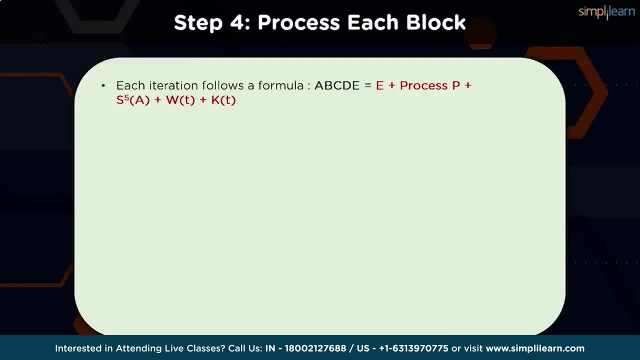 The formula can be A, B, C, D. E register is equal to E plus a non-linear process, P, along with a circular shift of A plus WT plus KT. In this formula, A, B, C, D is the register value of the chaining variables as 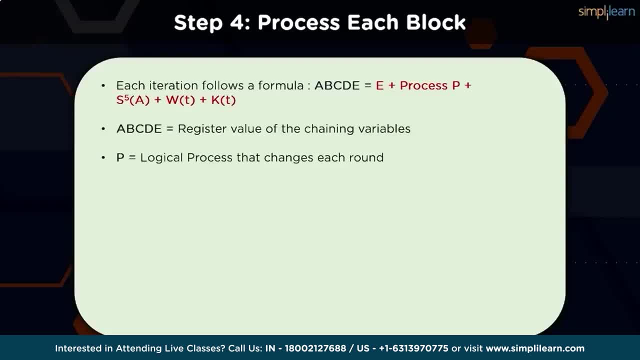 we discussed before. P is a logical process which has a different formula for each round. S5 is a circular shift by 5 bits. WT is a 32 bit string derived from the existing sub-block. This can be calculated depending on the iteration at hand. 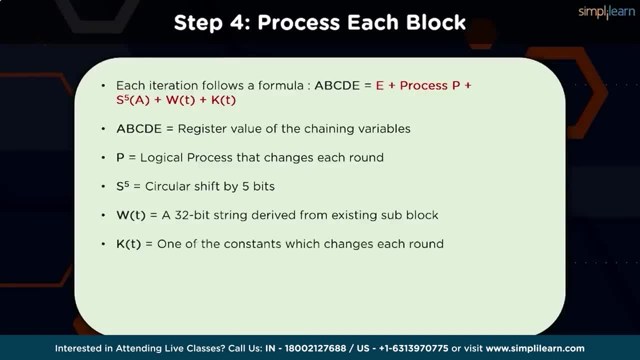 KT signifies a single element of the 80 character element array, which changes depending on the particular round at hand. For the values of WT, the first 16 values are the same as that of the sub-blocks, so there is no extra calculation needed For the 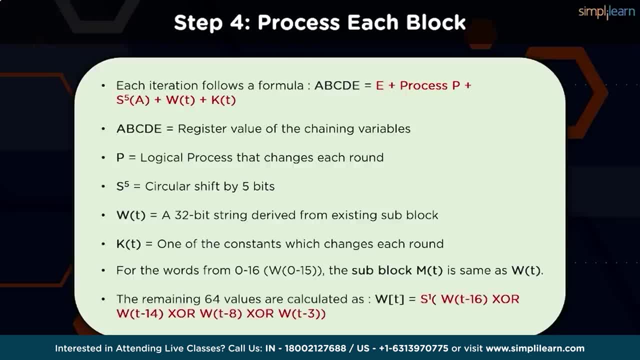 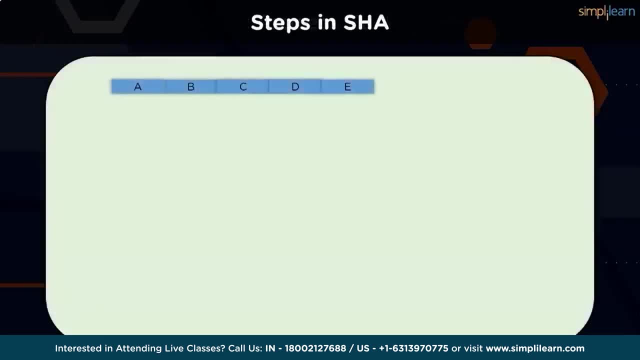 next 64 elements. the value of WT can be calculated as shown in the formula here. To better understand this, let's take a look at how each of this goes in a sequential process. We have our initial register using the 5 words of: 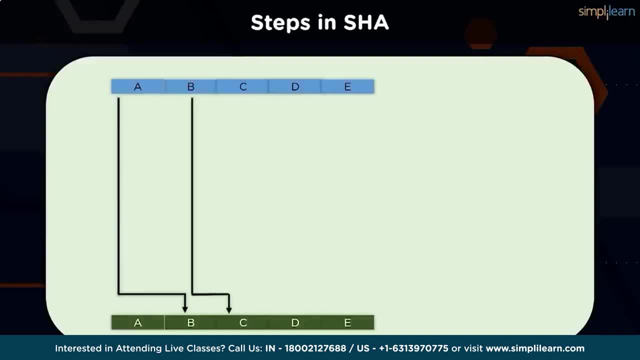 32 bits each. In the first step, we put the values of A, B, C and D to the subsequent register as the output. Next, we use a non-linear process B that changes depending on the round and uses the values of B. 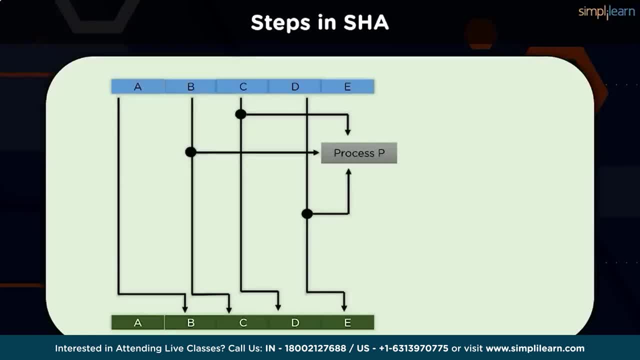 C and D as input. Whatever output is generated from the non-linear process, it is added with the value of the E register. Next, the value of A is circular, shifted by 5 bits and is added with the output generated in the previous step. 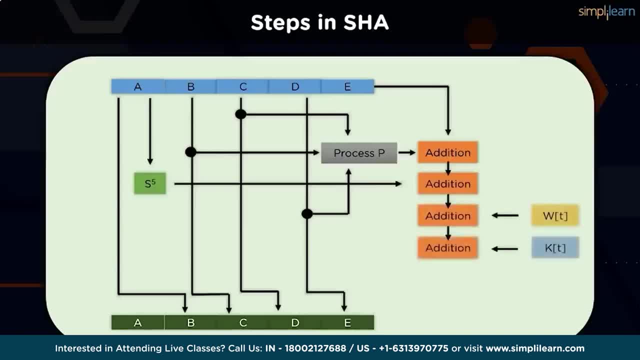 The next step is adding the value of WT and the constant element of KT. The current output is then stored in the register A. Similarly, this iteration is repeated every round and for each sub-block in the process, Once all the registers are complete and all the sub-blocks are joined together. 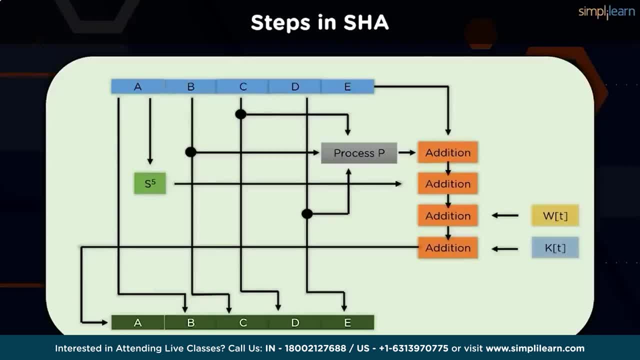 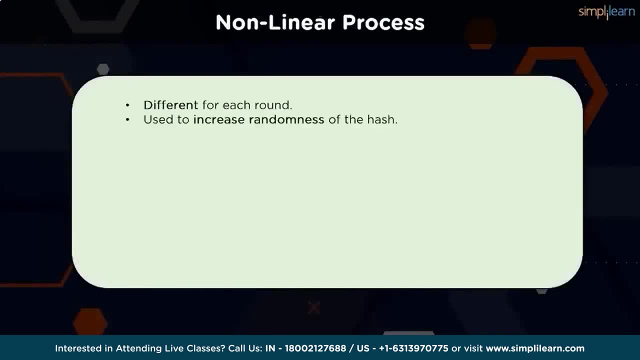 to form the single ciphertext message, we will have our hashed output. Regarding the non-linear process B that uses the values of B, C and D as input. the formula changes every round to maintain a complexity of the program that can withstand brute-force attacks Depending. 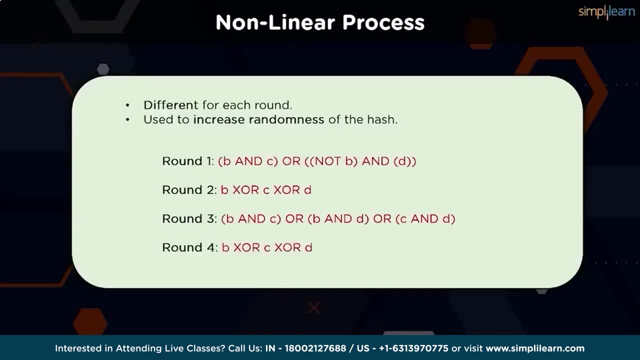 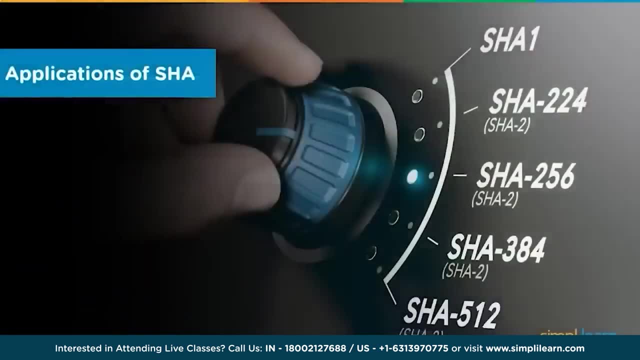 on the round. the values are passed through a logical operation, which is then added with the values of WT, KT and so on. Now that we understand how to get our hash digest from the plaintext, let us learn about the advantages we obtain when using the SHA hash. 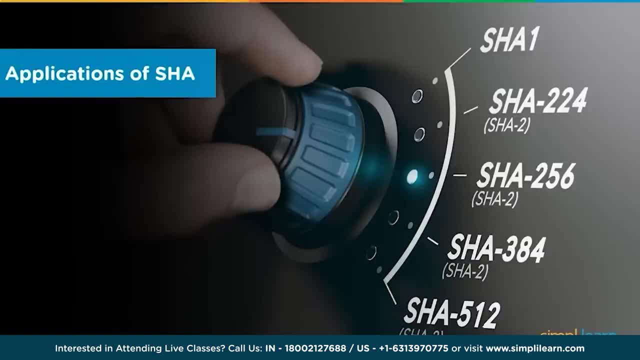 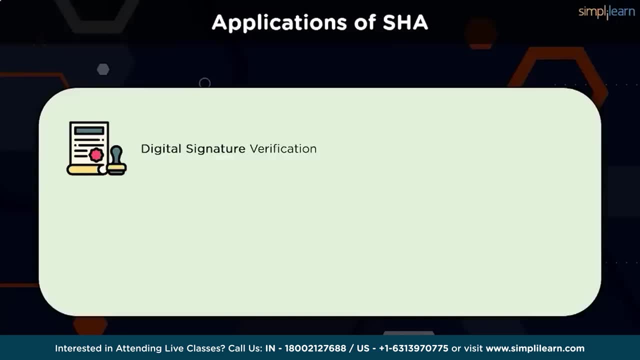 algorithm instead of relying on data in a plaintext format. Digital signatures follow asymmetric encryption methodology to verify the authenticity of a document or a file. Hash algorithms like SHA-250, SHA-556 and the industry standard SHA-512 go a long way in ensuring the verification. 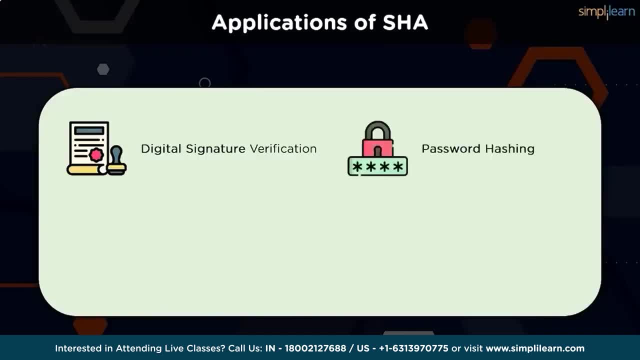 of signatures. Passwords need not be stored in a plaintext format, which makes them accessible to hackers and other malicious actors. When using digest, the database security also gets a boost, since the size of all hash values will be the same In the event of. 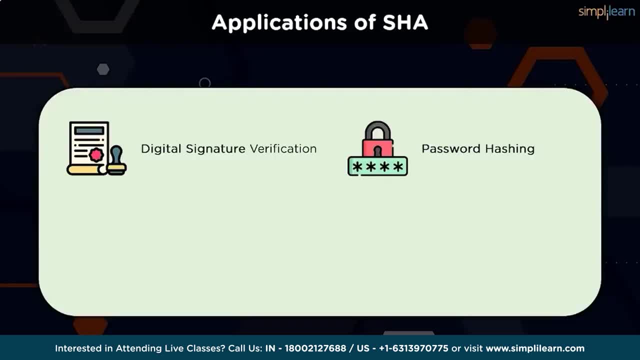 a hack or a breach, the malicious actor will only receive the hash values, with no way to regenerate the plaintext. In this case, the plaintext would be user credentials. Since the hash functions are irreversible by design, it has become a compulsion when storing. 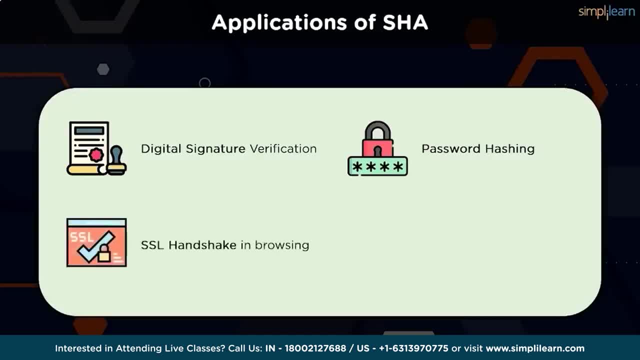 passwords on the servers. The SSL handshake is a crucial segment of the web browsing sessions and is done using SHA functions. It consists of your web browsers and the web servers agreeing on encryption keys and hashing authentication to prepare a secure connection. It relies on a combination of symmetric and 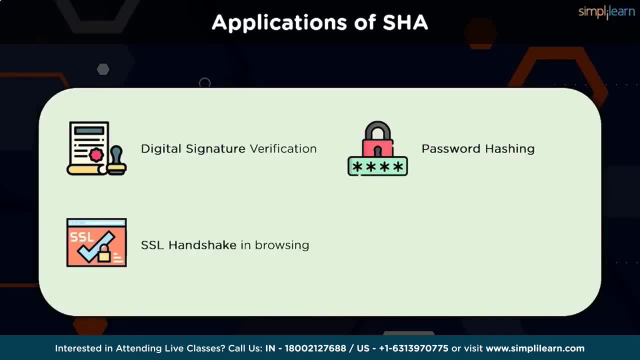 asymmetric algorithms which ensure the confidentiality of the data transmitted between a web server and a web client. like the browsers, You can monitor file corruption by comparing hash values before and after transit. Once the hashes match, file integrity checks are valid and data corruption is avoided. 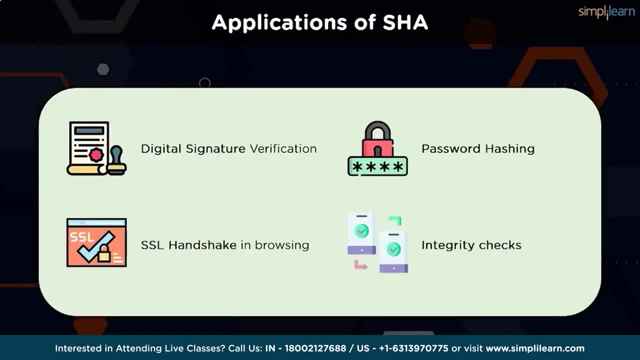 Hash functions will always give the same output for the same input, irrespective of the iteration parameters. It also helps in ensuring that the data hasn't been tampered with en route to the receiver of the message. Passwords are by far the most common type of 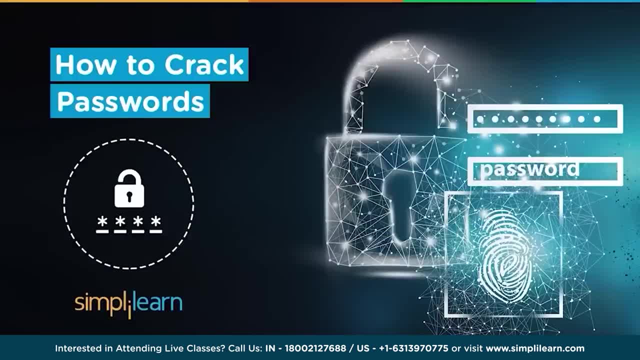 user authentication. They are popular because their theory makes perfect sense to individuals and is reasonably simple to implement for developers. On the other hand, poorly constructed passwords can pose security flaws. A well-designed password-based authentication process does not save the user's actual password. This would 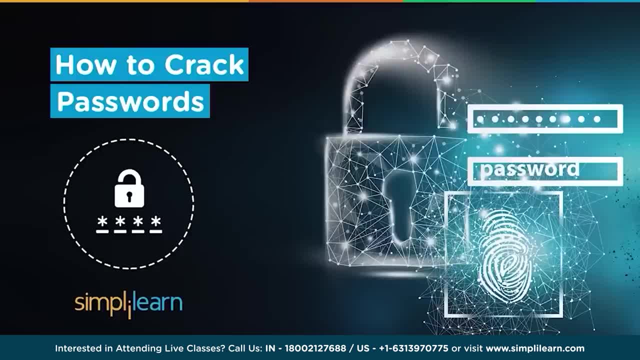 make it far too simple for a hacker or a malevolent insider to access all of the system's user accounts. In this video, you will learn how to crack passwords and simultaneously try to make your passwords as brute-force resistant as possible. Let's take a look at the topics to be covered today. 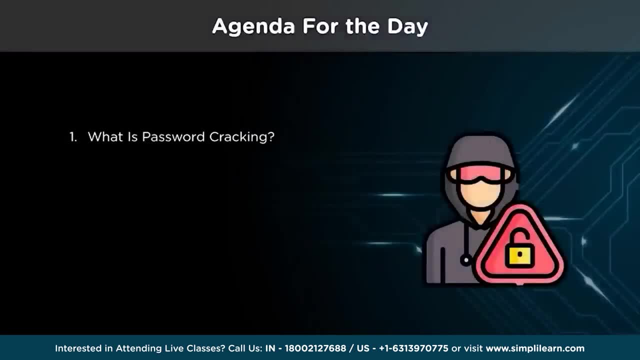 We start by learning about what is password cracking in general. Next, we take a look at the different techniques of password cracking that hackers use in order to generate user credentials for hacking. Moving on, we take a look at the multiple tools that hackers can use to generate these. 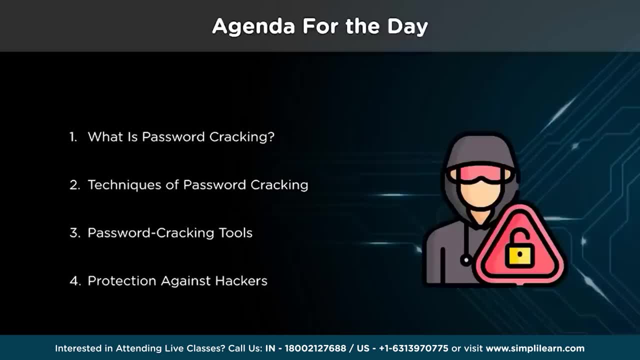 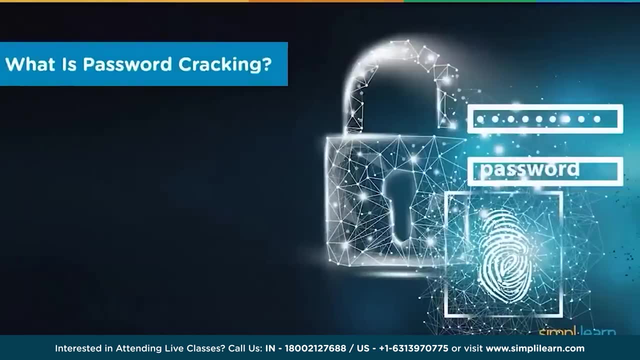 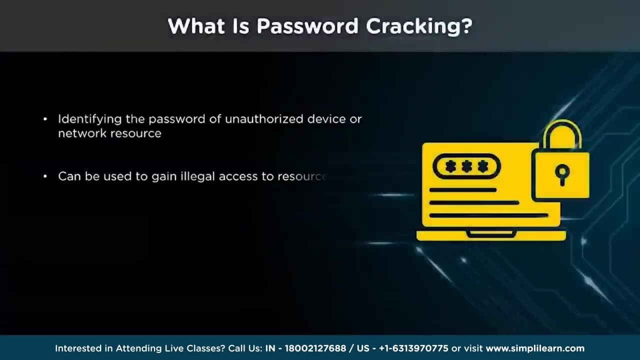 hashes and the passwords. Finally, we take a look at the steps and the guidelines that users can follow to prevent their passwords from being cracked. Let's start by giving a basic idea about password cracking. Password cracking is the process of identifying an unknown password. 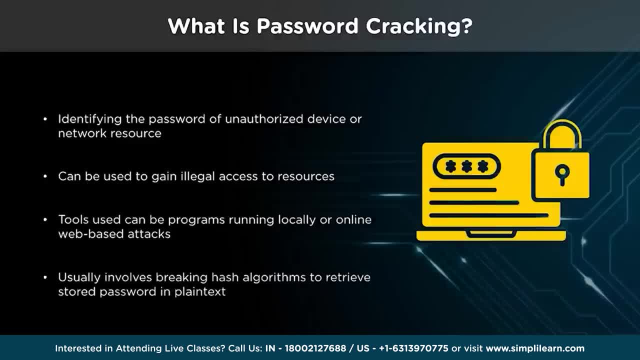 to a computer or a network resource using a program code. It can also assist a threat actor in gaining illegal access to resources. Malicious actors can engage in various criminal activities with the information obtained through password cracking. The procedure might entail comparing a set of words to guess credentials. 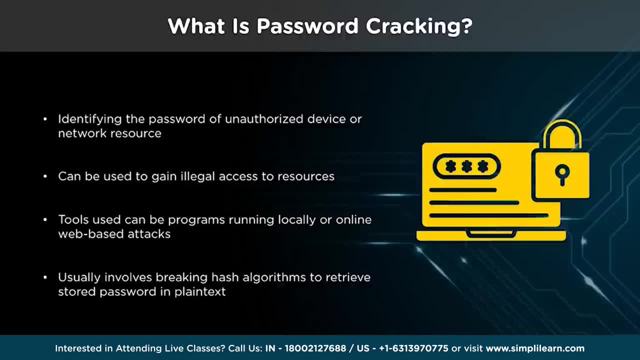 or using an algorithm to guess the password repeatedly. Password cracking can be done for several reasons, but the most malicious reason is in order to gain unauthorized access to a computer without the owner's awareness. This results in cybercrime, such as stealing passwords for the purpose of accessing banking information. 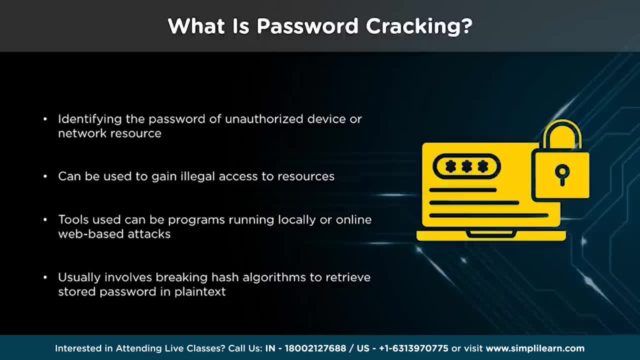 Other non-malicious reasons for password cracking occur when someone has misplaced or forgotten a password. Another example of non-malicious password cracking may take place if a system administrator is conducting tests on password strength as a form of security test. This enables so that the 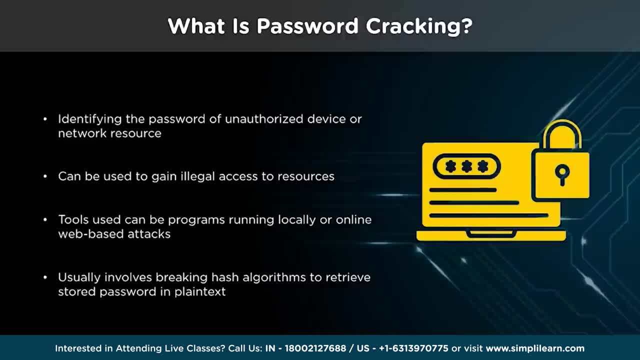 hacker cannot easily access protected systems. The best way that users can protect their passwords from cracking is to ensure that they choose strong passwords. Typically, passwords must contain a combination of mixed-case random letters, digits and symbols. Strong passwords should never be actual words. 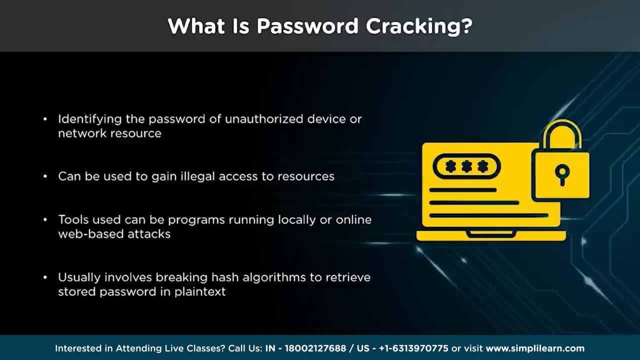 In addition, strong passwords are at least 8 characters long. In many password-protected applications, users are notified of the strength of the password they have chosen upon entering it. The user can then modify it and strengthen the password based on the indications of its strength. 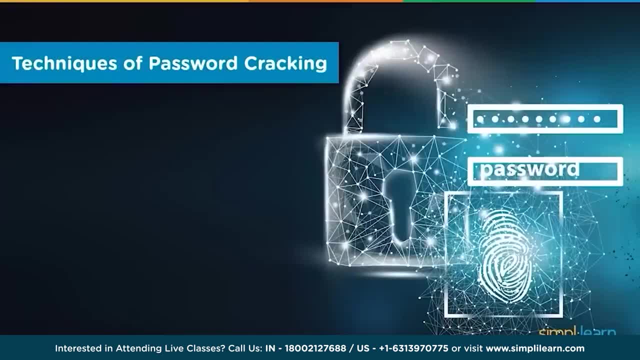 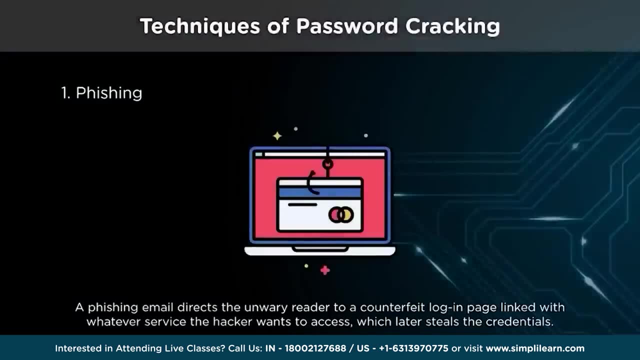 Now that we understand the basics of password cracking, let's go to the basic techniques hackers use to retrieve passwords from general victims. Asking the customer for their password is a simple approach to hacking. A phishing email directs the unwary reader to a counterfeit login page, linked with whatever. 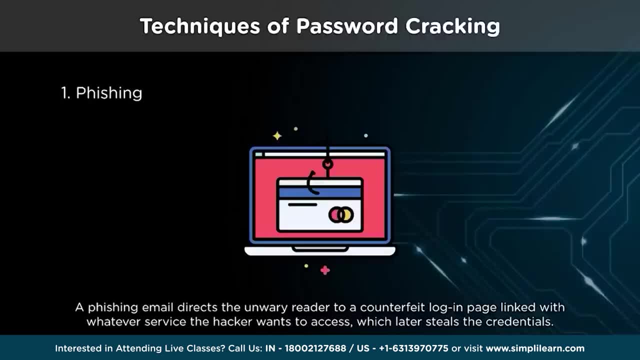 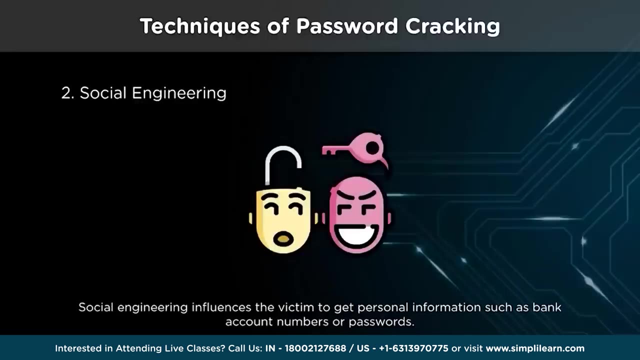 service the hacker wants to access, generally by demanding the user fix some critical security flaw or aid in a database reset. That page then captures their password, which the hacker can subsequently exploit for their own purpose. Social engineering influences the victim to get personal information such as. 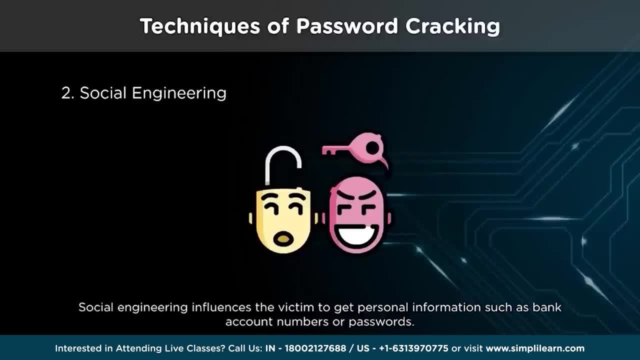 bank account numbers or passwords. This strategy is popular among hackers because they realize that humans are the gateway to vital credentials and information. Through social engineering, the employee tried and true tactics to exploit and influence age-old human tendencies rather than devising novel means to 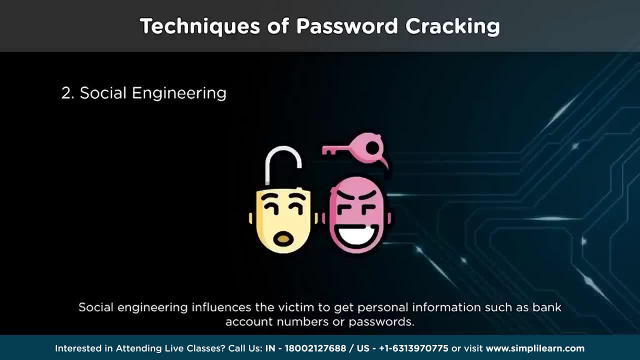 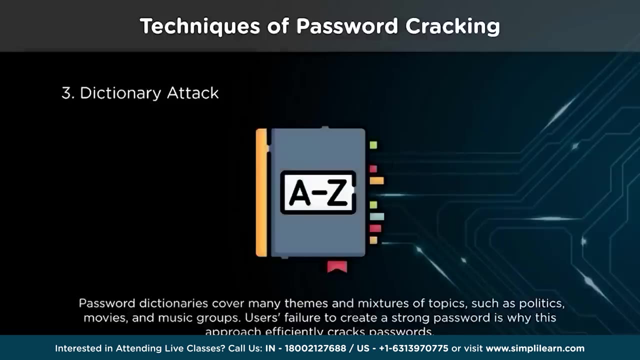 breach secure and advanced technologies. It has been demonstrated that many firms either lack adequate security or are overly friendly and trustworthy when they should not be. They allow granting access to critical facilities based on a uniform or a sob story. A hacker searches a password dictionary for the correct password. 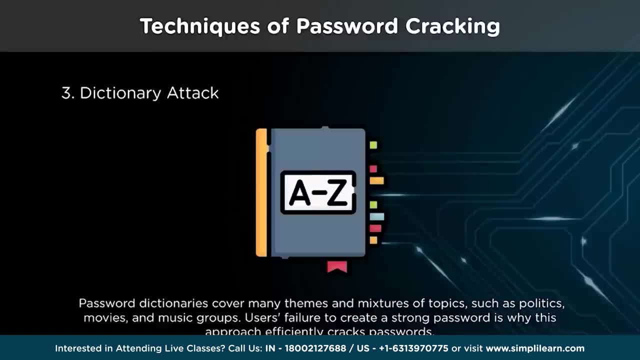 in the case of a dictionary attack Password. dictionaries cover many themes and a mixture of topics such as politics, movies and music groups. Users' failure to create a strong password is why this approach efficiently cracks passwords day to day. Simply said, 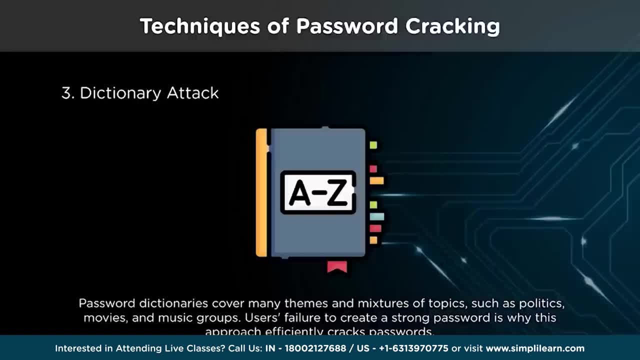 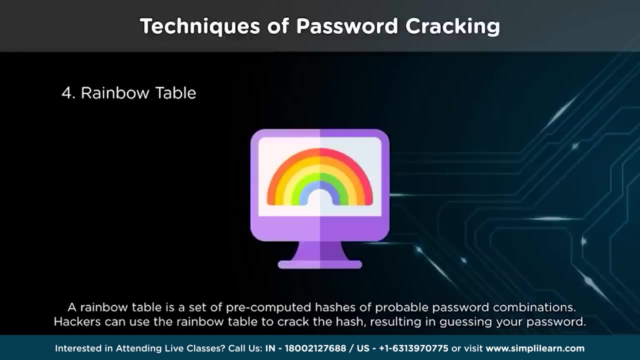 this assault employs the same terms that many individuals use as passwords. A hacker can compare the password hash obtained to hashes of the password dictionaries to find the correct plain text password. Now that the passwords have been hashed, the hackers attempt to achieve authentication by breaking the password. 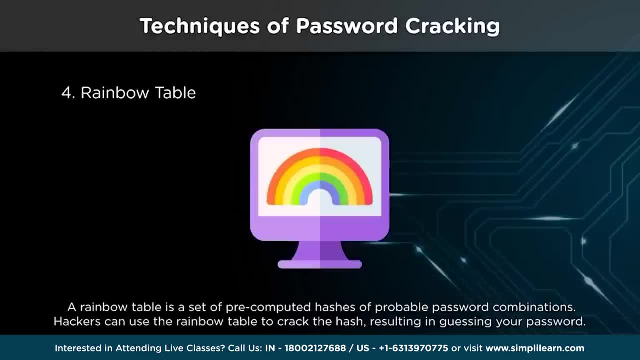 hash. They accomplish this by employing a rainbow table, which is a set of pre-computed hashes of portable password combinations. Hackers can use the rainbow table to crack the hash, resulting in guessing your password. As a result, it retrieves the password hash from the system. 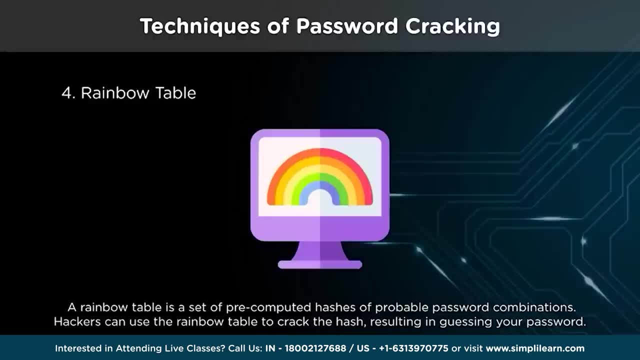 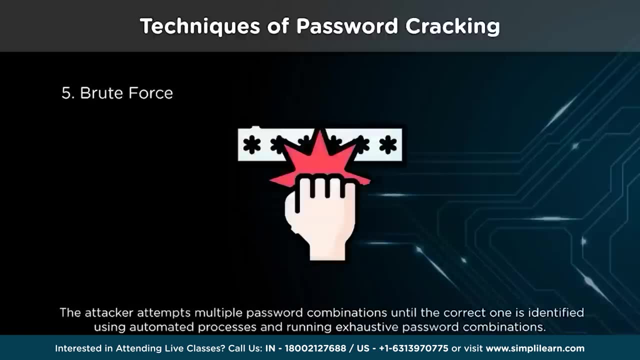 and eliminates any need to break it. Furthermore, it does not necessitate the discovery of the password itself. The breach is accomplished if the hash matches In a brute force assault. the attacker attempts multiple password combinations until the correct one is identified. The attacker uses software to automate. 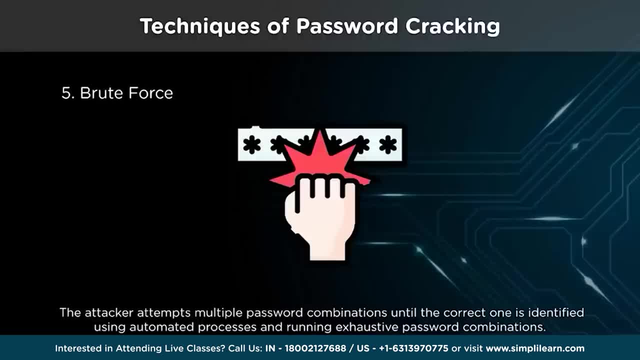 this process and run exhaustive password combinations in a substantially shorter length of time. With the growth of hardware and technology in recent years, such programs have been invigorated. It won't be quick if your password is more than a few characters lengthy, but it will eventually reveal. 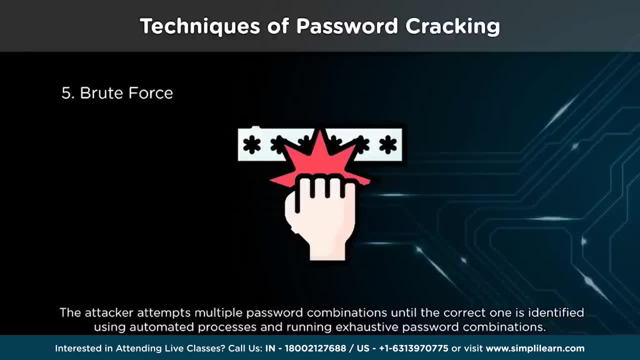 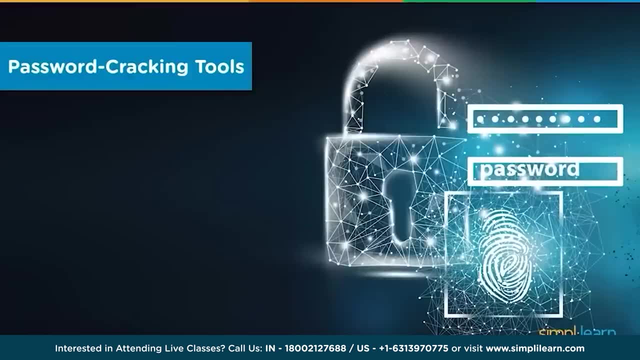 your password. Brute force assaults can be sped up by throwing more processing resources at them. With so many different techniques coming together to crack passwords, none of them are useful without the right tools. There are a plethora of scripts and snippets of code that can retrieve 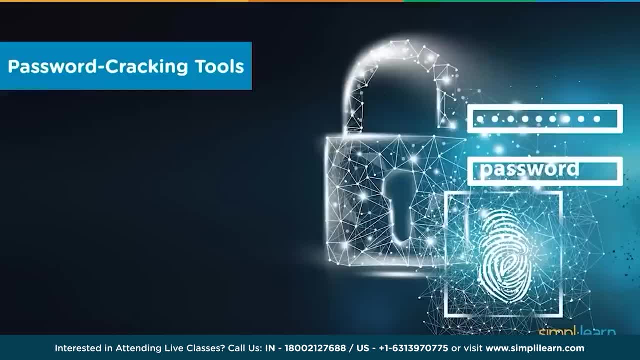 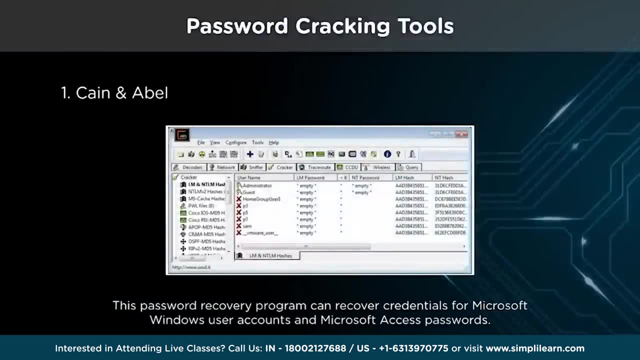 passwords from either encrypted storage or from the hash digest. Let's go through some of these tools. Cane and Able is a password recovery tool for Microsoft operating systems. It allows easy recovery of various kinds of passwords by sniffing the network, cracking encrypted passwords using dictionary. 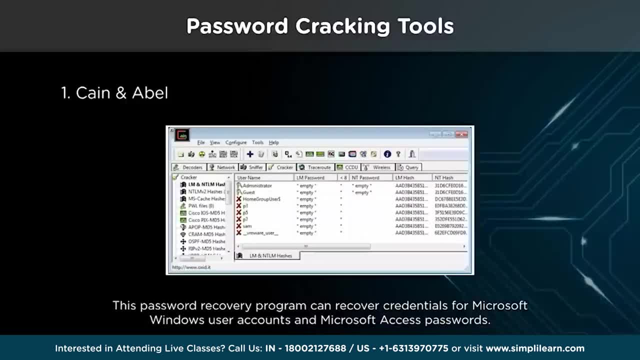 brute force and cryptanalysis. Recording VoIP conversations, decoding, scrambled passwords, recovering wireless network keys, etc. are some of the other features of Cane and Able. The latest version is faster and contains a lot of new features, like ARP Poison Routing, which enables 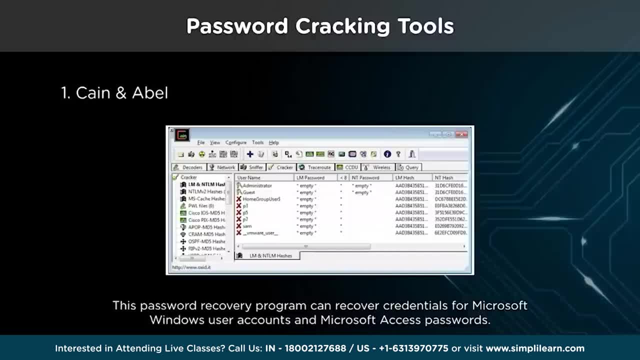 sniffing on switched LANs and man-in-the-middle attacks. The sniffer in this version can also analyze encrypted protocols such as SSH1 and HTTPS, while containing filters to capture credentials from a wide range of authentication mechanisms. It also ships routing protocol authentication monitors. 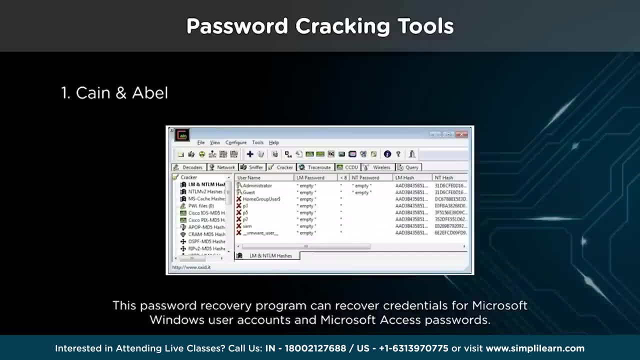 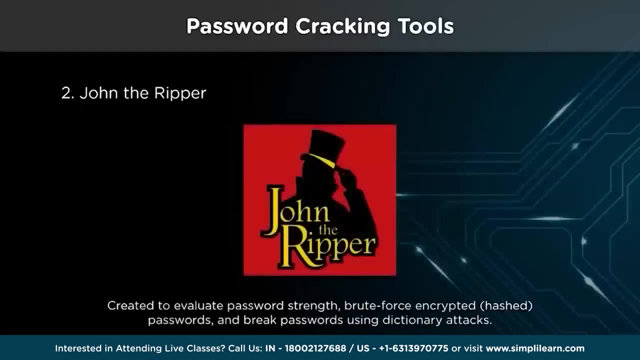 and route extractors. Dictionary and brute force crackers are also present, along with common hashing algorithms and several specific authentications, password hash calculators and other features. John the Ripper is a password cracking application that was first released in 1996. 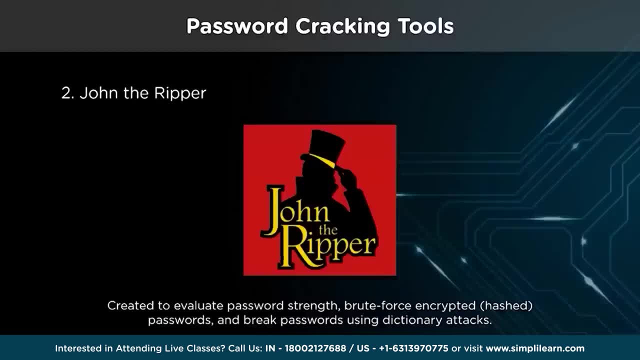 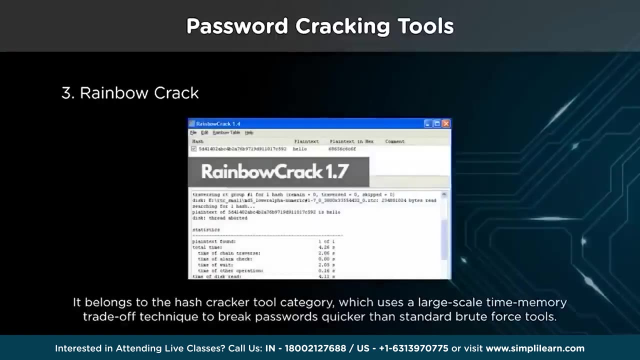 for Unix-based computers. It was created to evaluate password strength, brute force, encrypted hash passwords and break passwords using dictionary attacks. It can use dictionary attacks, rainbow tables and other attacks, depending on the target type. Rainbow crack is a password cracking application that uses time-memory trade-off. 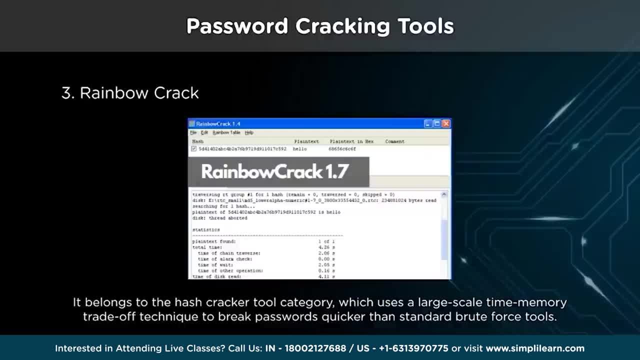 algorithm to crack password hashes with rainbow tables. Rainbow tables make password cracking more easier and faster than traditional brute force attacks. It is like a dictionary containing nearly every possible password and the pre-calculated hashes. Creating this kind of dictionary takes much more time than cracking. 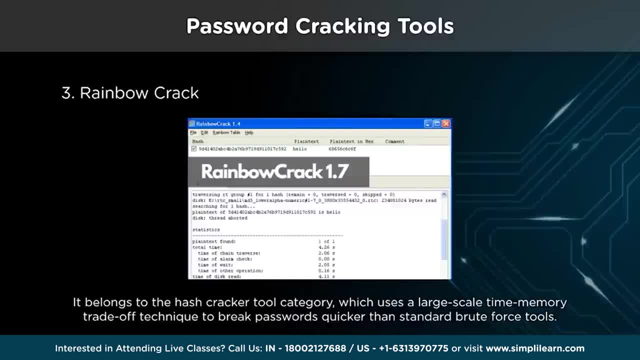 a single hash, but after that you can use the same dictionary over and over again. This procedure might take a long time. However, once the table is ready, it can break passwords far quicker than brute force methods, With so many tools ready to nab. 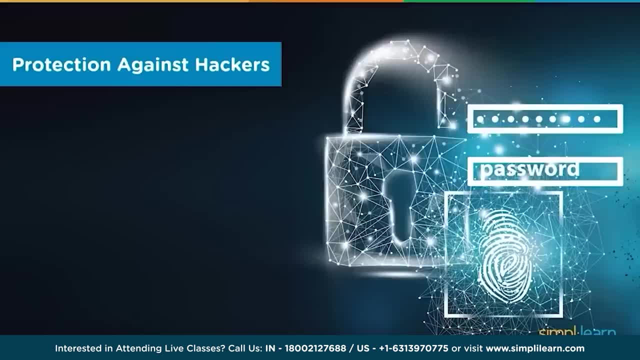 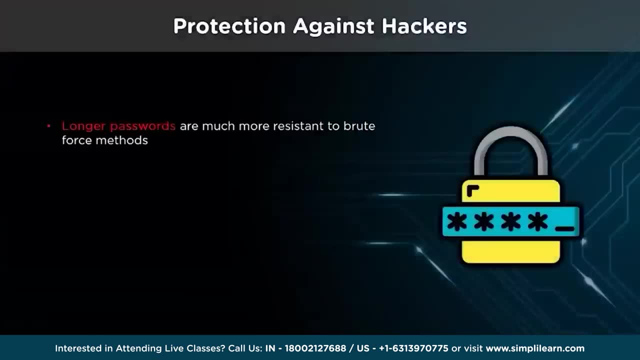 our passwords. there are certain set of rules users can follow to protect their credentials from being compromised. Let's cover some of these guidelines. Longer passwords are required, making the brute force mechanism tougher to implement. Longer passwords and passphrases have been demonstrated to boost security. 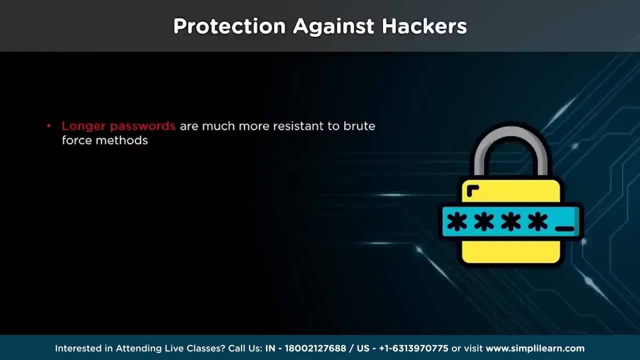 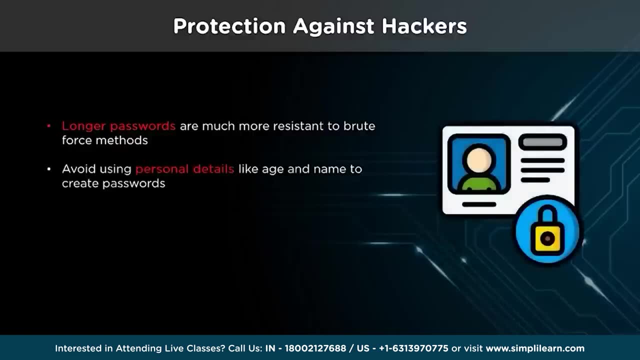 significantly. However, it is still critical to avoid lengthier passwords that have previously been hacked or that feature often in cracking dictionaries. This password policy encourages users to establish passwords that do not contain personal information. As previously said, most users create passwords utilizing personal 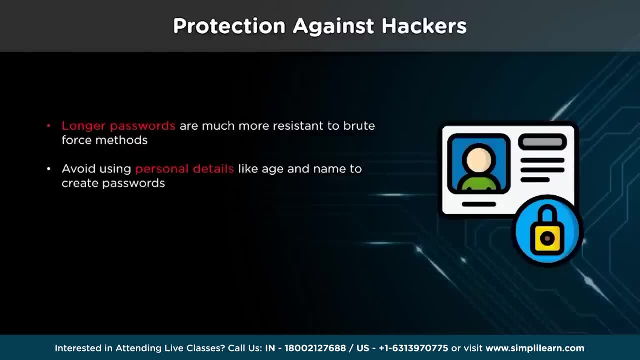 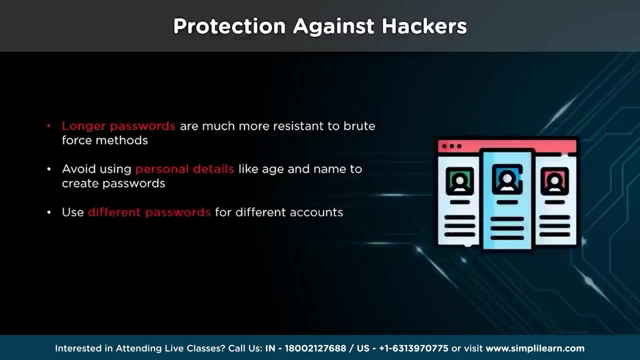 information such as hobbies, nicknames, pet or family members, phone number names, etc. If a hacker has access to personal information about a specific user, for example via social media, they will test password combinations based on that knowledge. Password regulations should. 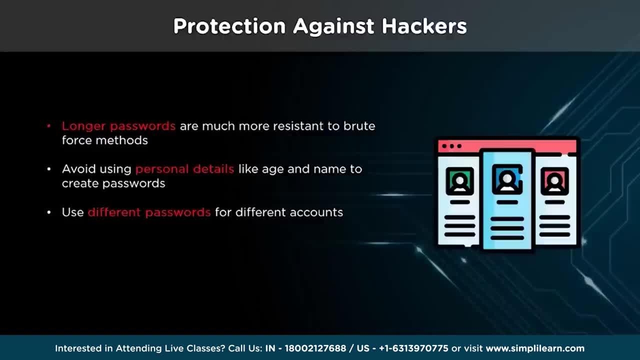 compel users to distinguish between security and convenience. Users should be prohibited from using the same password for all services. Password sharing between users, including those who work in the same department or use the same equipment, should be avoided. A single breach password doesn't affect your other. 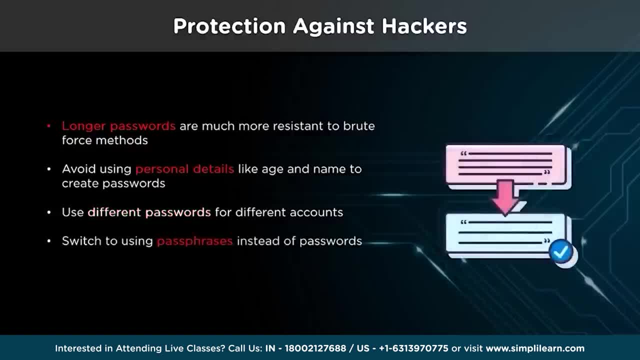 accounts with this policy. Some password regulations necessitate the creation of a passphrase rather than a password. While passphrases serve the same objective, their length makes them more difficult to break. In addition to letters, a good pass should include numbers and symbols. Passwords may be: 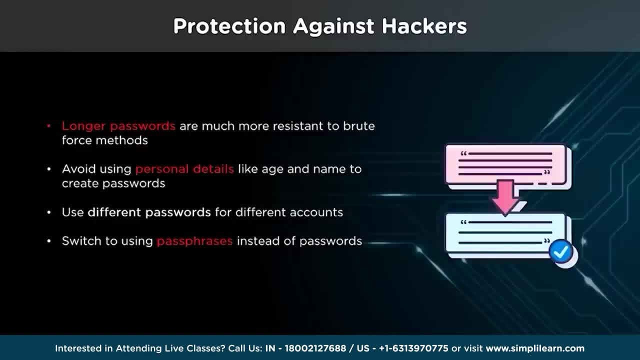 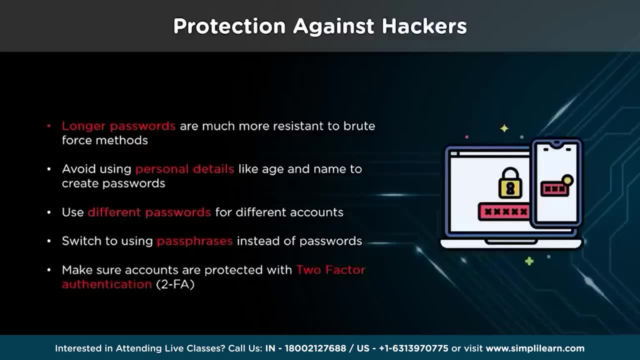 easier for users to remember than passphrases. However, the latter is much more breach-resistant. Two-factor authentication, or 2FA, can help secure an online account or even a smartphone. 2FA does this by asking the user to provide two forms of information: a password- 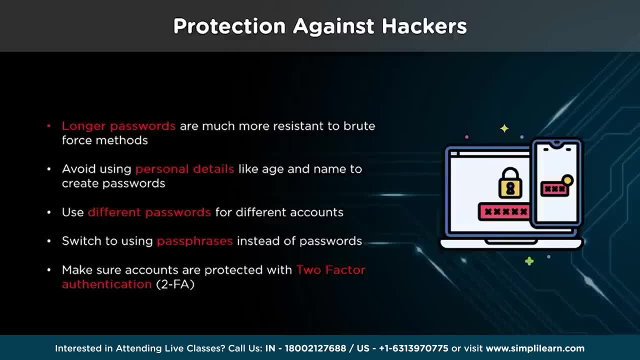 or a personal identification pin and a code texted to the user's smartphone, or a fingerprint, before accessing whatever is secured. This helps discourage unauthorized entries to an account without the original owner's permission. At this point, you may wonder why you need a strong. 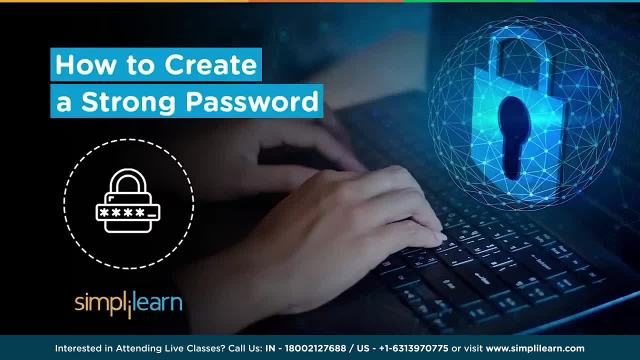 password in the first place. Even if most websites are safe, there is still a danger that someone will try to access or exploit your information. A strong password is among the most effective ways to protect your accounts and personal information from hackers. You should follow certain rules and guidelines. 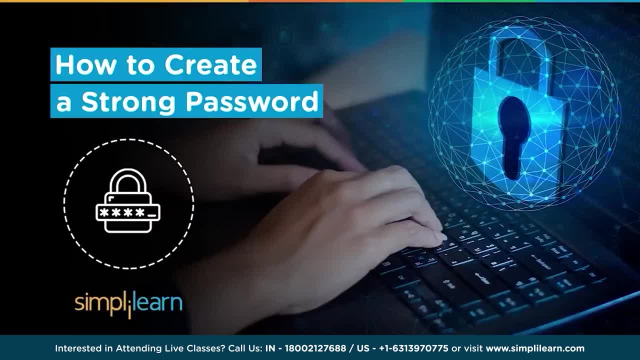 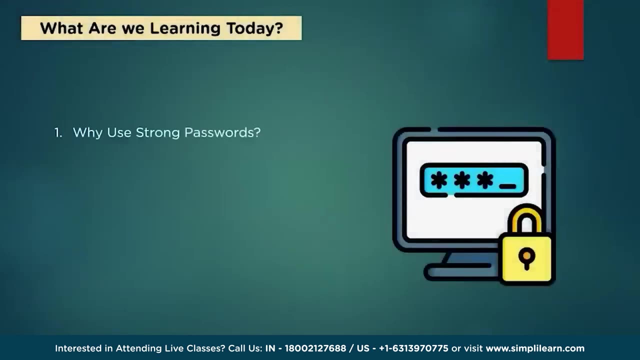 while creating a strong password. Password managers are also recommended to help remember the created passwords for convenience of usage. With that being said, let's take a look at the topics we are covering today. We start by learning about the state of password cracking in today's world, and 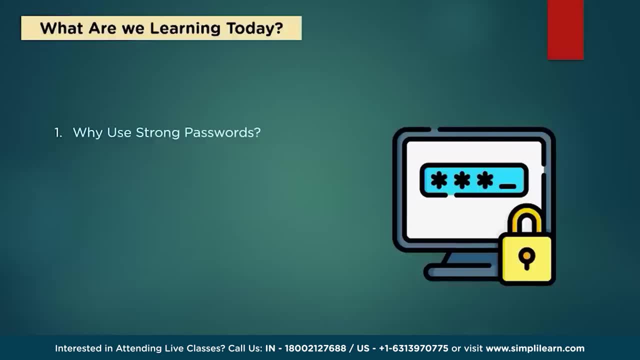 why creating strong passwords is an absolute must for every account. Next, we will look at some guidelines and rules that help strengthen passwords and make password cracking a daunting task for hackers. Moving on, we understand why past faces have gone in popularity and are being 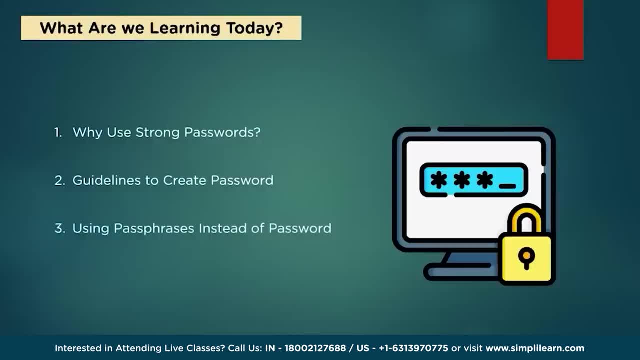 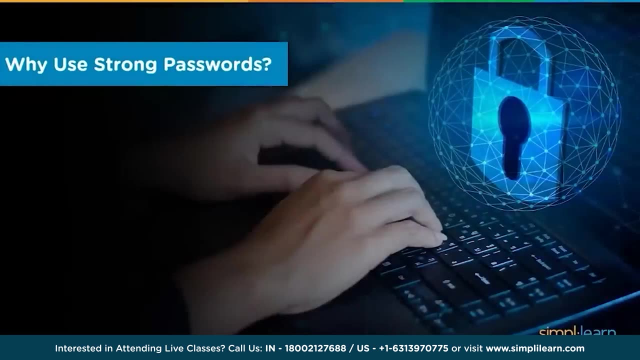 recommended for credential protection over traditional passwords. And finally, we take a look at how password managers help alleviate the problem of creating and remembering complex passwords, along with other critical personal information. Let's start by learning about what passwords are and why strong passwords have become an absolute necessity. 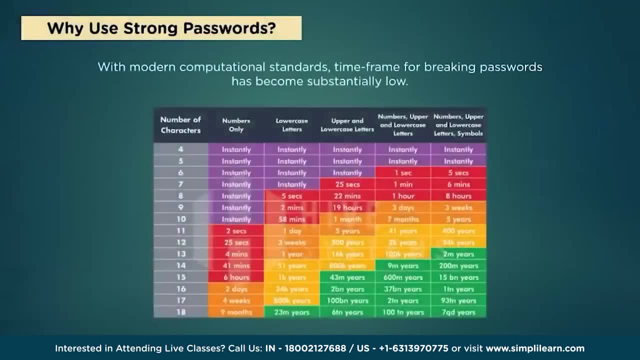 One of the most common ways that hackers break into computers is by guessing passwords. Simple and commonly used passwords enable intruders to easily gain access and control a computing device. Conversely, a password that is difficult to guess makes it prohibitively difficult for common hackers. 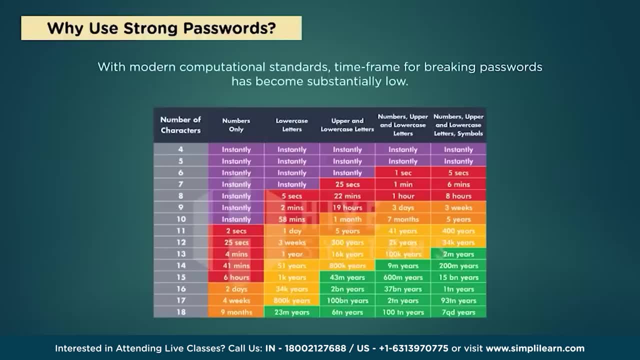 to break into a machine and will force them to look for another target. The more difficult the password, the lower the likelihood that one's computer will come to an unwanted intrusion. Many individuals opt to tie their websites to something they can readily recall, to generally easy, memorable combos. 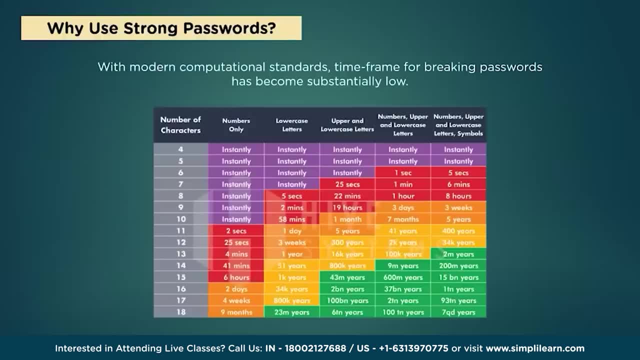 However, this does not make the password unique. In fact, it's the reverse. Passwords are handled by 53% of individuals using their recollections and memory. With modern computational standards, simple passwords take seconds and a couple of minutes at worst. 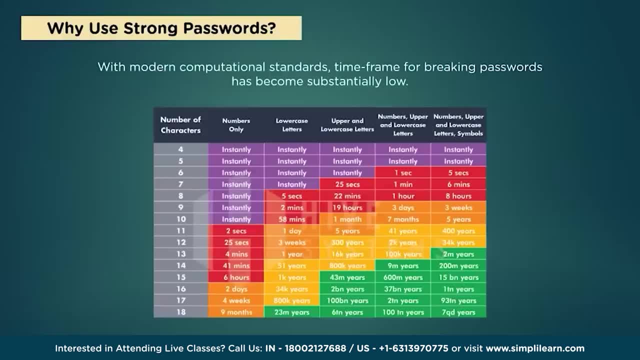 to be completely brute-forced. According to global surveys, more than 60% of people use the same passwords for their personal and job applications. While this may allow the user never to forget the password, it makes a single point of failure, the only pin to drop. 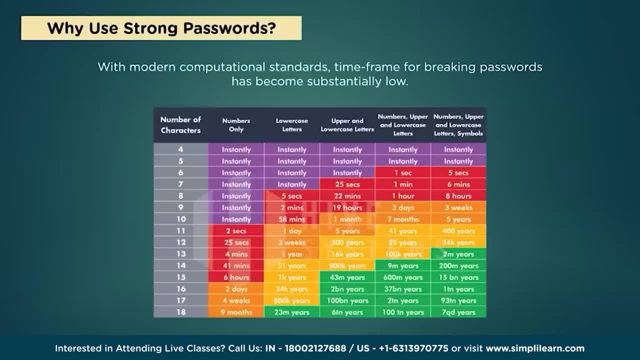 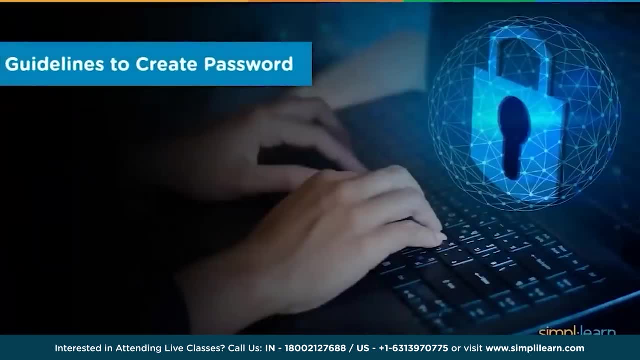 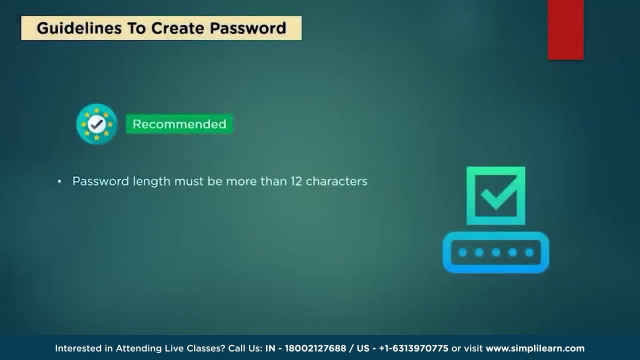 If one of the accounts gets breached, all subsequent accounts are as good as hacked. To further elaborate on how you can create strong passwords, let's go through some of the guidelines. Let's go through some do's and don'ts to understand how to create new. 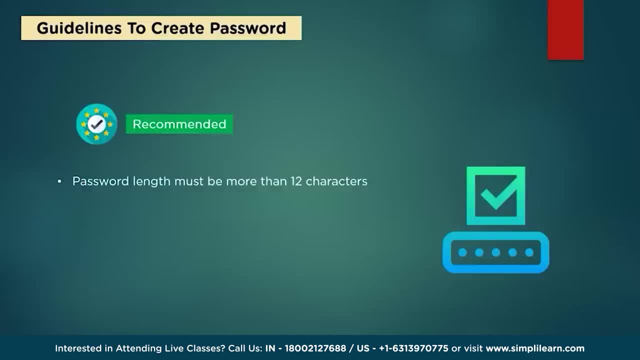 passwords for our accounts. It is recommended to keep the password length at least 12 characters. to ensure brute-forcing to be difficult, A combination of upper and lowercase alphabets is an absolute necessity when creating strong passwords. It is also recommended to use numerics. 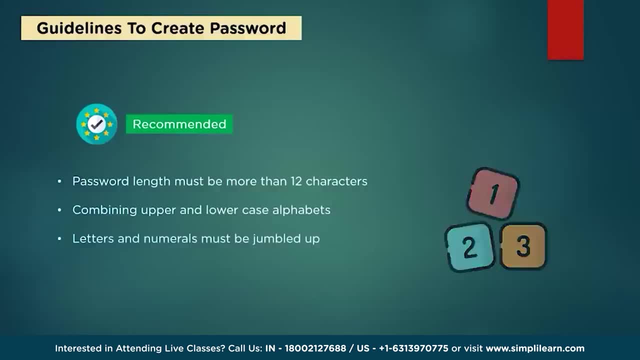 along with those alphabets to create a complicated password. Finally, special characters help in making a password much more brute-force resistant than any number of alphabets or letters can make. Moving over to the don'ts section, it is absolutely not recommended. 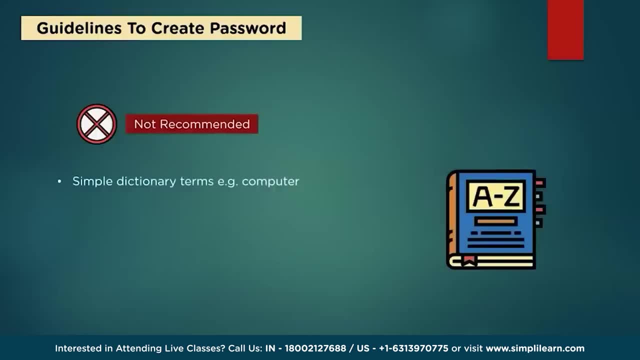 to keep simple dictionary terms such as computer or even the word password as your credential, because those are very easy to be brute-forced and are usually present in majority of the dictionary attack word list. Similarly, changing a single alphabet or a single character in a dictionary word does not make 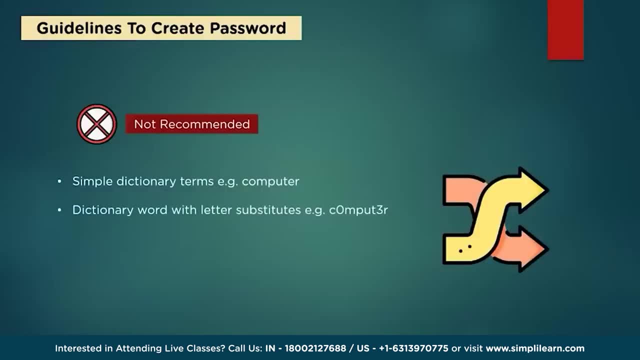 it brute-force resistant, considering there are already algorithms present that can counter this tactic. Using the same character multiple times in a password also reduces the strength and makes it easier to crack for hackers, Apart from using single characters multiple times, following patterns that are present. 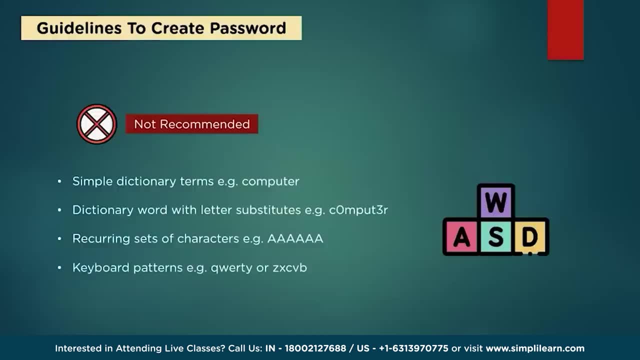 on the traditional English keyboard, such as E, W, E, R, T, Y, or the line below the main alphabet, such as Z, X, C, V, B, N, M, etc. make it easier to guess, since these are once again common combinations that are present in the dictionary word list already. 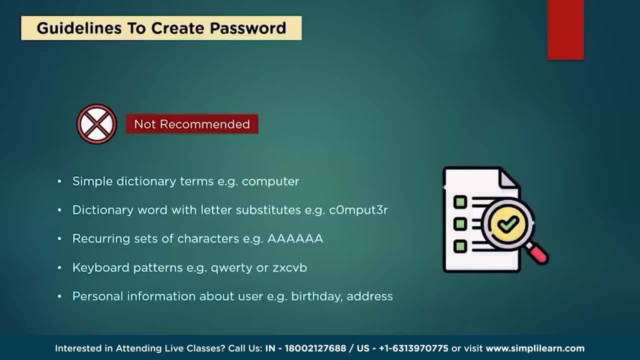 Finally, the most important part being not using personal information such as birthdays, addresses and other important information in the passwords. More often than not, if a hacker is trying to break into your account- there has been some amount of research done, be it via social media. 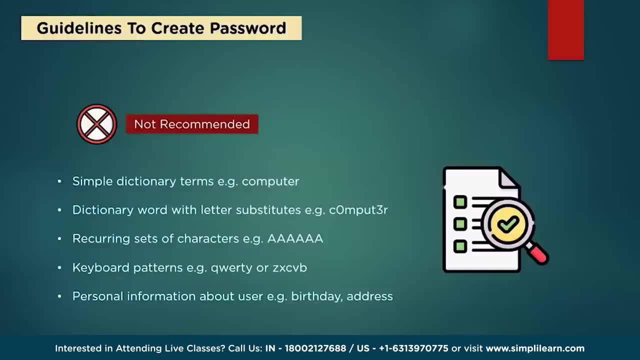 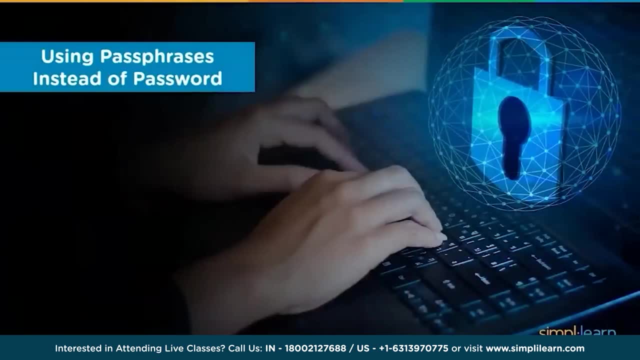 or any other medium, If they have already this information present with them. breaking into your account becomes all the more easier Now that you understand how to create a strong password. look at how passphrases have become prevalent as a replacement for plain text passwords. 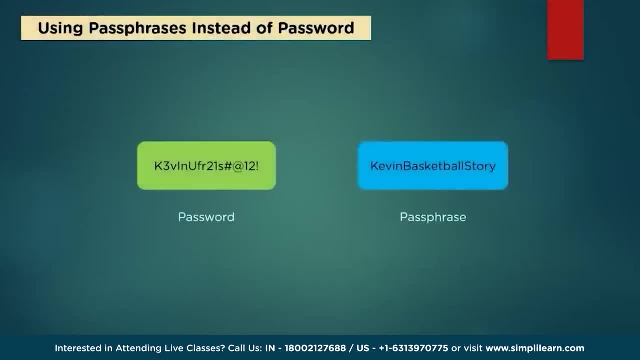 A passphrase is a sentence-like string of words used for authentication that is longer than a traditional password, easy to remember and difficult to crack. Typical passwords range, on an average, from 8 to 16 characters, while passphrases can reach up to 100 characters or more. 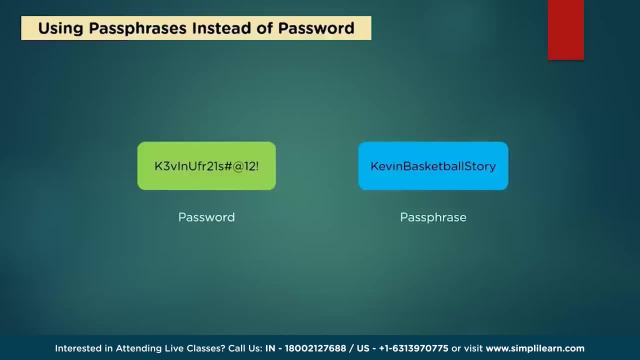 Using a long passphrase instead of a short password to create a digital signature is one of the many ways that users can strengthen the security of their data, devices and accounts. The longer a passphrase is, the more likely a user is to incorporate bits of entropy or factors. 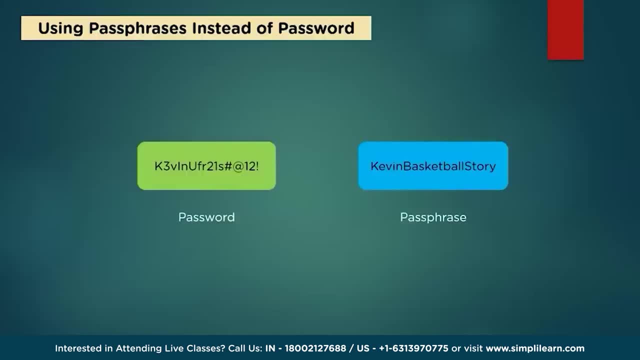 that make it less predictable to potential attackers. As more websites, applications and services increase their user security requirements, a passphrase is a fast and easy way to meet these criteria. Let's take a look at some of the advantages that passphrases have over common passwords. 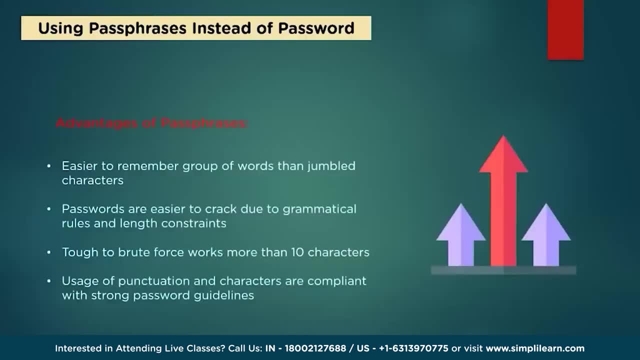 Passphrases are simpler to remember than just a random assortment of symbols and characters. It's easier to comprehend a line from your favorite song or a quotation than a short but difficult password. Passwords are reasonably easy for humans and robots to guess or crack. 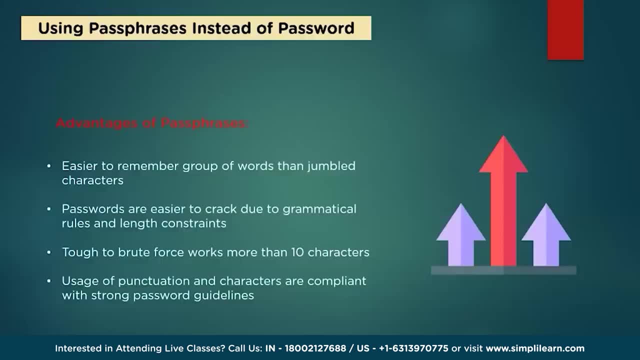 Online thieves have also advanced and created cutting-edge hacking tools to crack even the most complex passwords. Passphrases are nearly hard to crack, since most efficient password-cracking programs fail at approximately 10 characters. As a result, even the most sophisticated cracking tool. 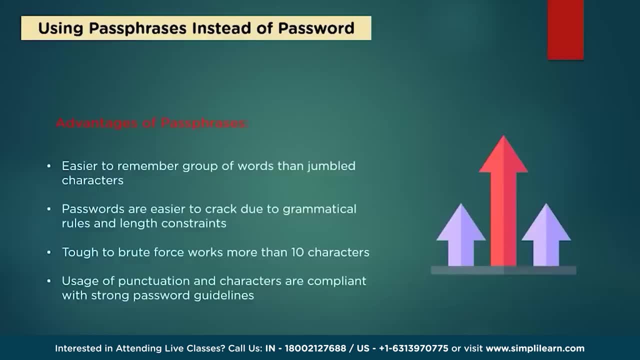 will be unable to guess, brute-force or pre-compute these passwords. Compliance with password-setting rules with ease are passphrases. The usage of punctuation and upper and lower-case passwords satisfy the password complexity criteria. Most operating systems and apps support passphrases. 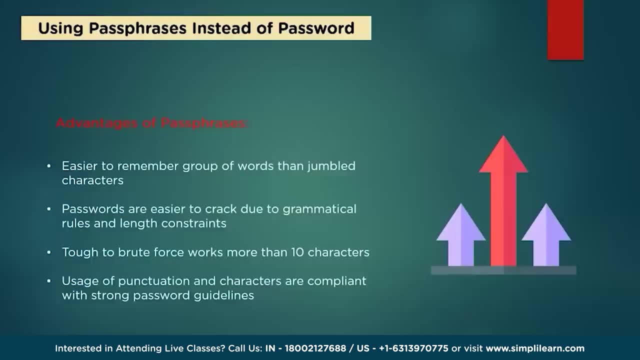 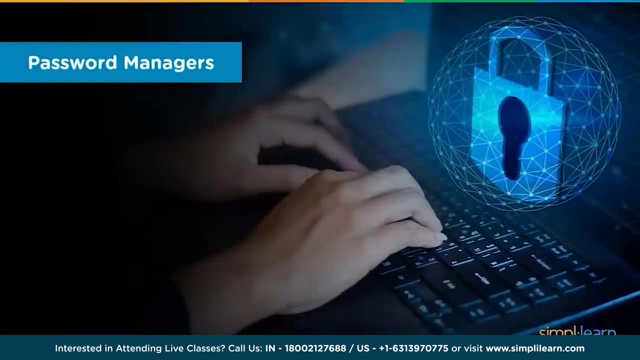 Phrases of up to 127 characters are permitted on all major operating systems, including Windows, Linux and Mac. As a result, for optimal protection, you can use lengthier passphrases, But when creating a strong password, the major problem people come across. 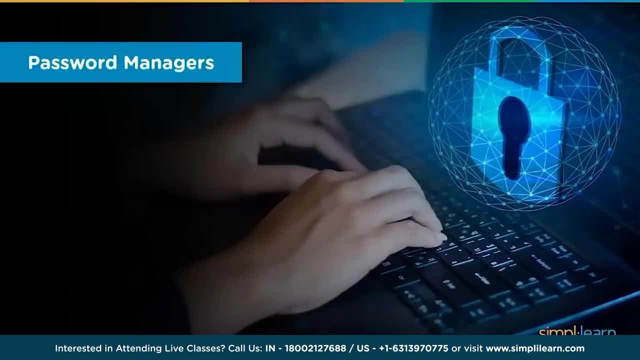 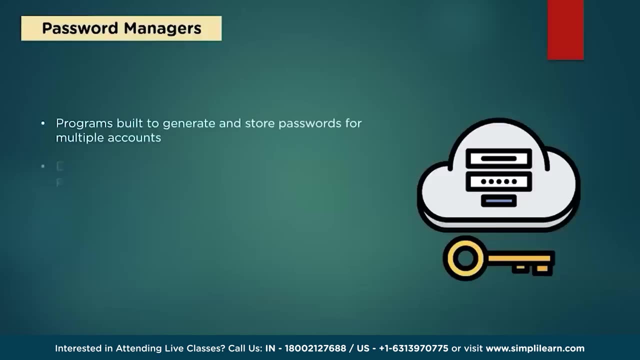 is remembering these passwords or the passphrases. This is where you can find a use for a password manager. When you establish accounts or change passwords, password managers generate new strong passwords and they keep all of them in one place, protected by a single strong 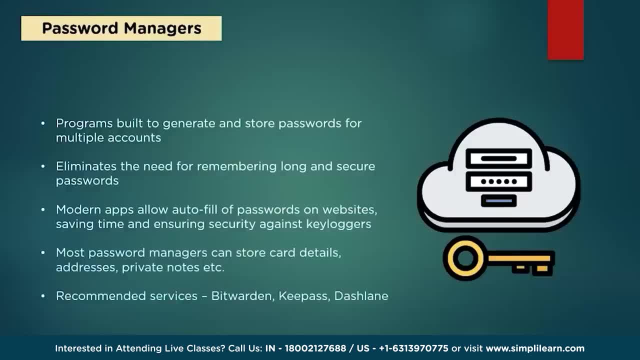 password. If you maintain your master password, the manager will retain everything else, including your username and passphrases, and fill them in for you whenever you sign on to a website or app on your computer or phone. There is no good memory needed for this. 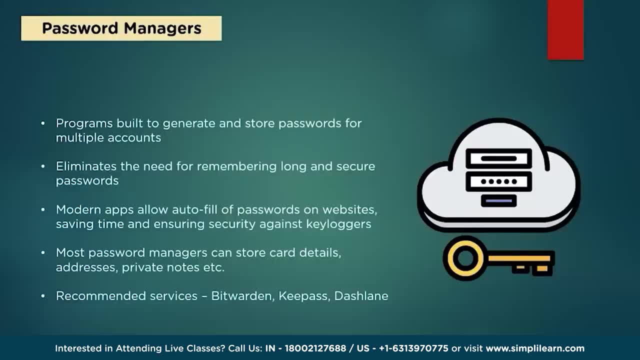 This implies that everyone may use the most recent suggestions for strong passwords, such as extended phrases, symbols, grammar and capitalization. Password managers enable consumers to write a single master password and automatically fill each website with their own unique set of credentials, And not just passwords. 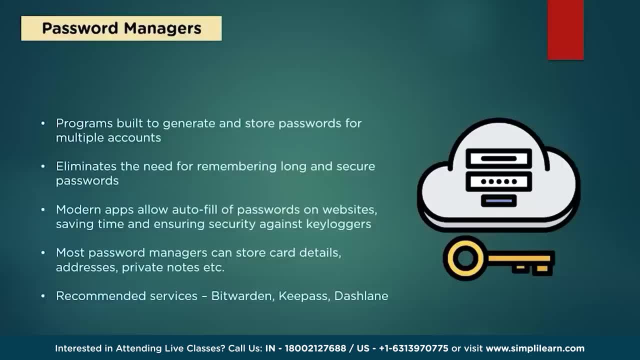 Credit card information may be stored securely with several password managers. Some others make multi-factor authentication or use a second test, such as answering a question once the correct password is input, which is a simple and effective solution to verify legitimate login inputs Among the global players in password. 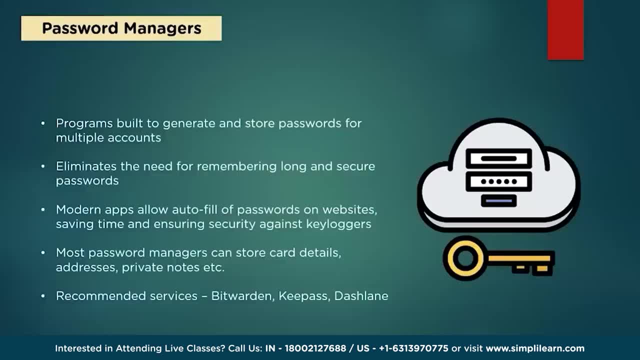 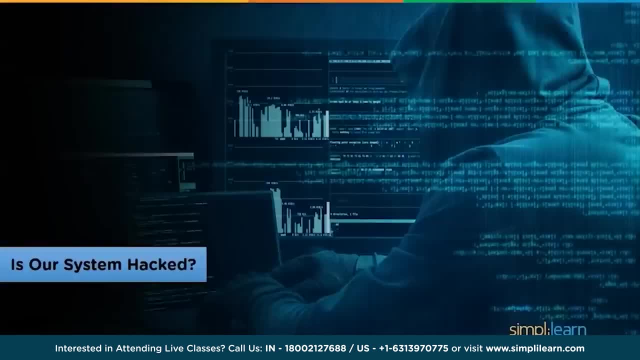 managers. services like Bitwarden, KeePass and Dashlane have been running for years now and are very worthy recommendations if you want to get started with password management. Now that we understand what is hacking, let's take a look at some points to know whether a system is already. 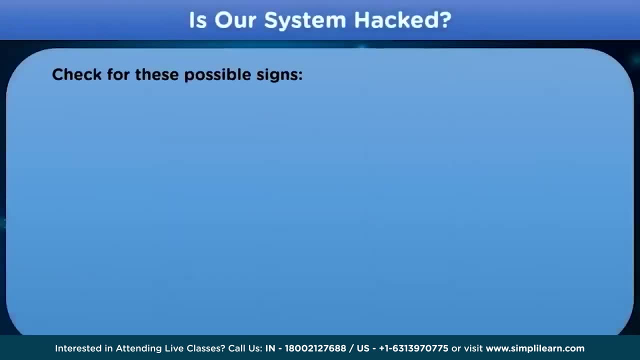 hacked or not. The first point regarding how to check whether a system is hacked or not can be cases where the system's security is switched off by unknown means and it is not visible to the user. This is one of the most primary checkpoints: to know if 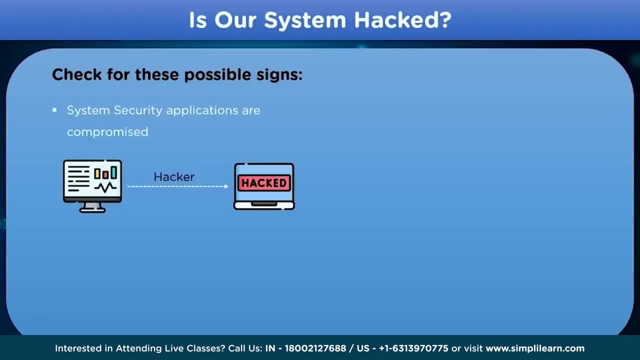 a system is hacked or not. Next point to check whether a system is hacked or not would be frequent antivirus software failures, which are due to the interference from hacking attempts performed by a professional hacker or a cybercriminal. Then we also face problems regarding system's reaction speed. 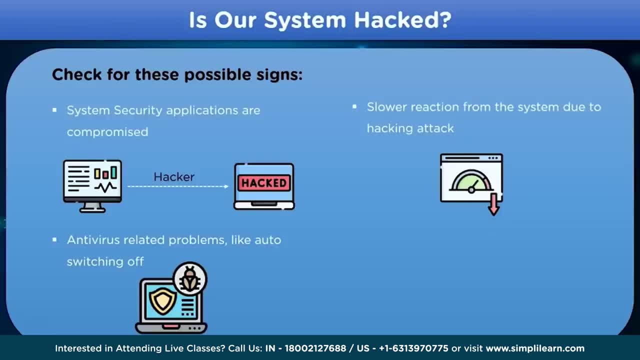 which is affected due to the execution of unknown applications in the background of the system, which also affects the hardware resources in the device. Next, we also face problems regarding passwords which are no longer working or are changed without a user's intervention, which might indicate that there was some. 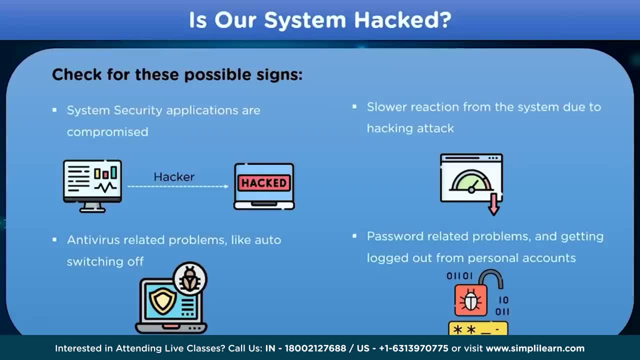 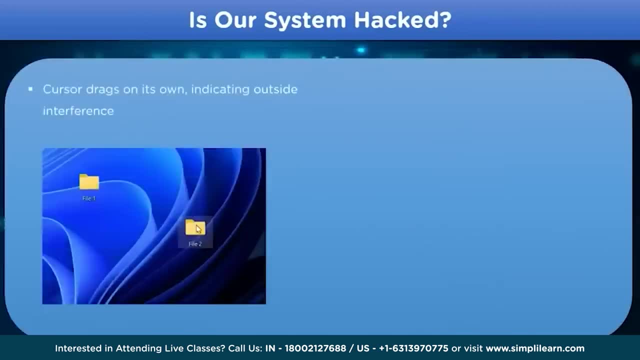 unknown hacking activity that took place in our account. Let's take a look at some more points regarding the topic. There are often cases when the system's cursor move on its own and perform tasks indicating that the system is being used by someone else using an illegal. 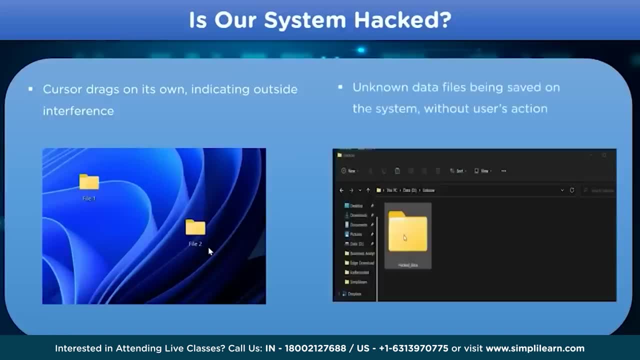 hacking method. There are also cases when we often see files and folders being created in the storage disk on the system which is unknown to us. To better understand the points regarding how to identify whether our system is hacked or not, let's take a look. 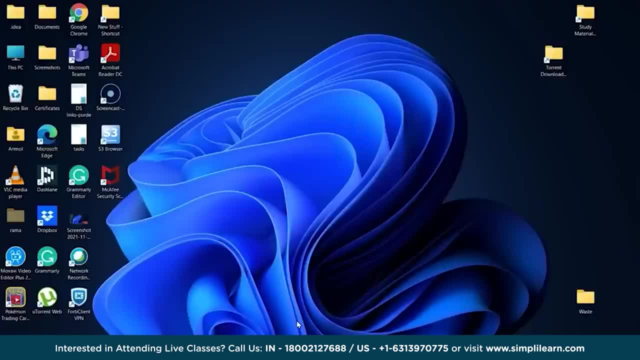 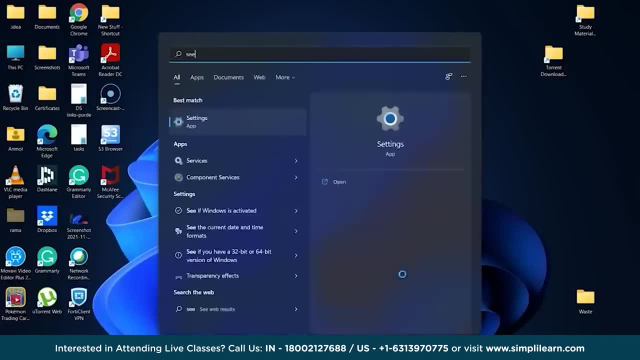 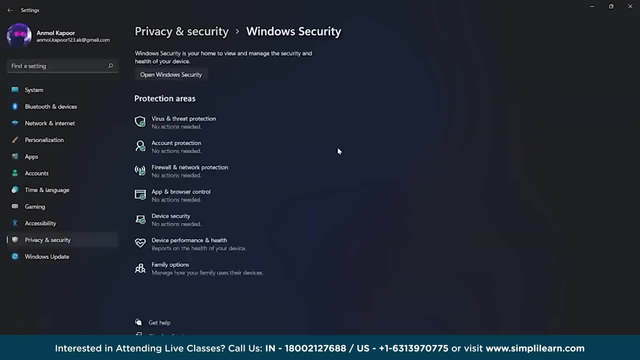 Then let's start with the first point. If we want to check whether our system is hacked or not, the first point would be to choose the settings option and using privacy and security and moving on to the windows security, This option that is available on our system. 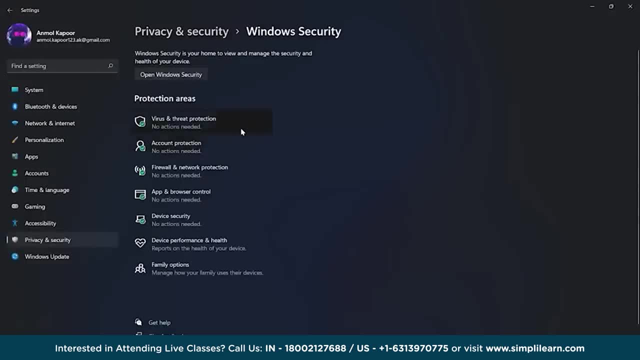 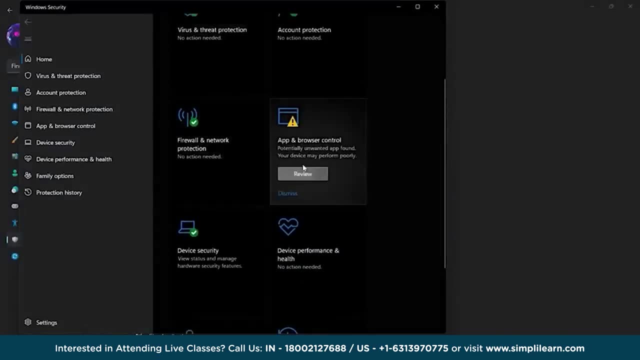 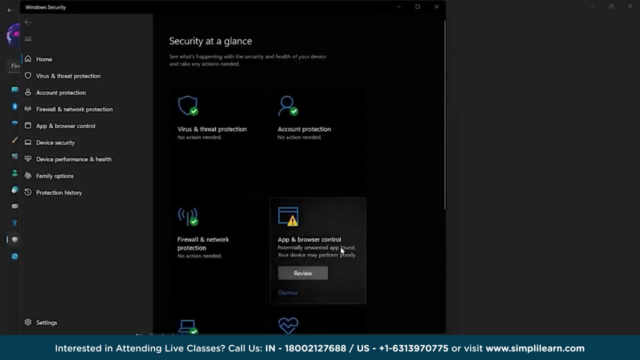 allows us to see various protection applications that are available on the system. If we see any problem regarding any one of them, for example, apps and browser control, in my system it says there is a problem with it, which might be due to hacking attempts that was done on my system. 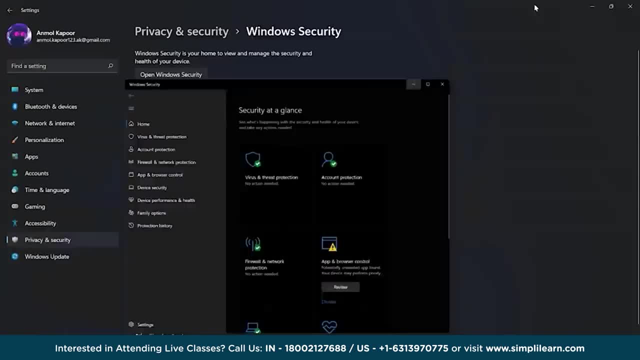 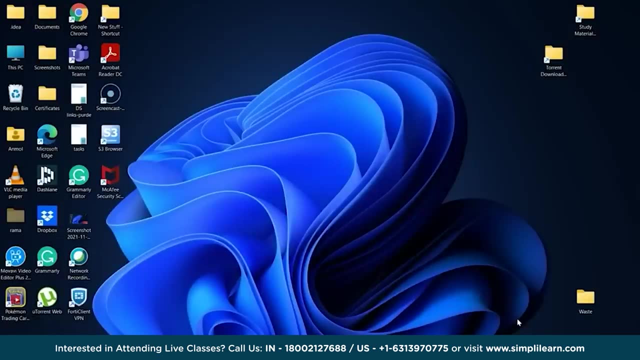 Now let's take a look at the other option: how we can check whether our system is hacked or not. That would be checking the antivirus software that is installed in our system. If you face problems regarding that, this might be the issue, According to my antivirus software. 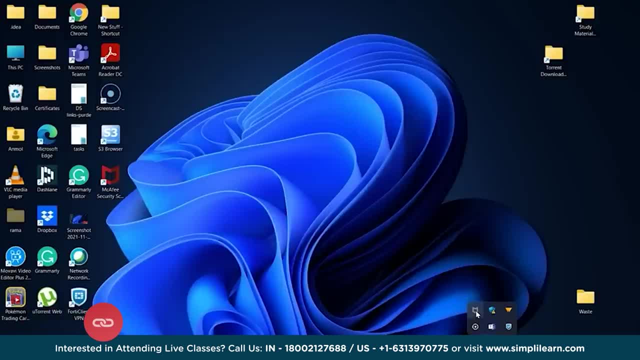 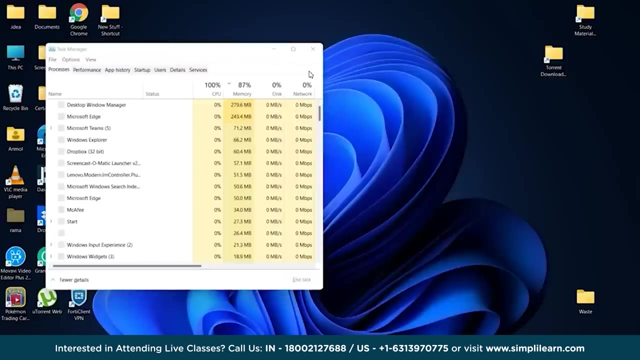 it says my computer is at risk. This might be due to the interference from a cyber criminal or a hacker while using different illegal software during its hacking attempt. Then there are also cases where we see there are unknown programs being executed in the background of our system. 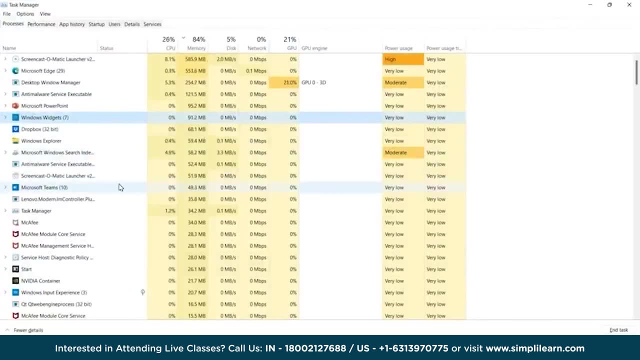 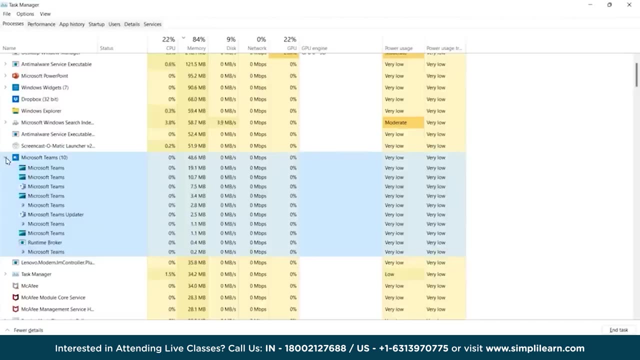 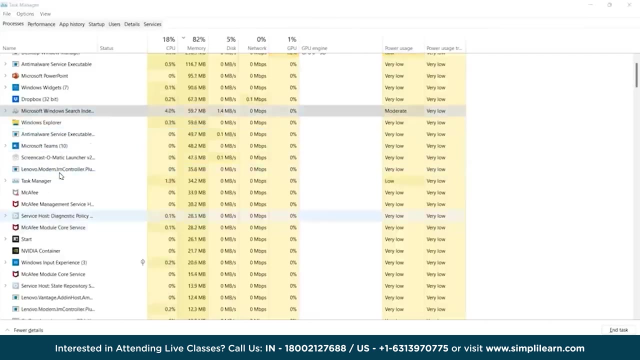 Which we can take a look using the task manager software. Using the task manager, we can take a look at each and every application that is being executed in the system and see the origin. If we find any unknown program or application, we can assume that it might be due to. 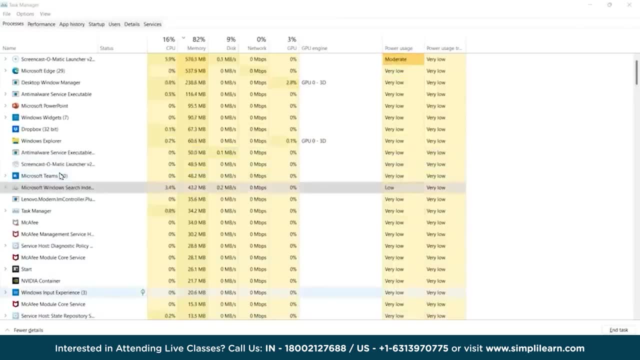 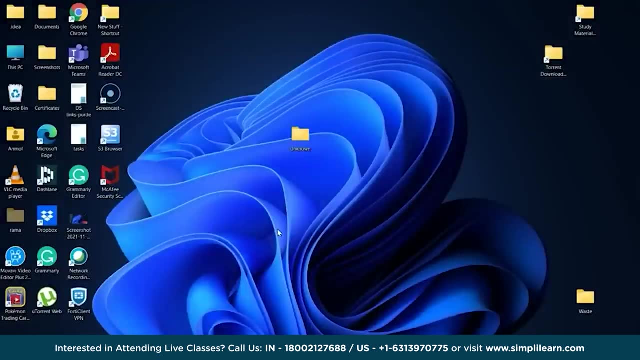 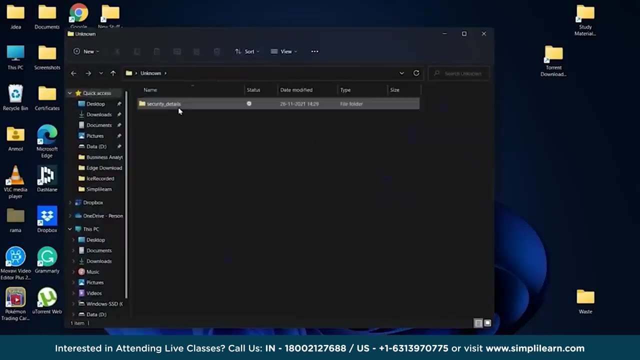 a hacking attempt. Moving on, if we want to check further whether our system is hacked or not, we can check for files that are being created unknown to us, For example, this unknown folder which contains some security details that are unknown to me. This might be also due to 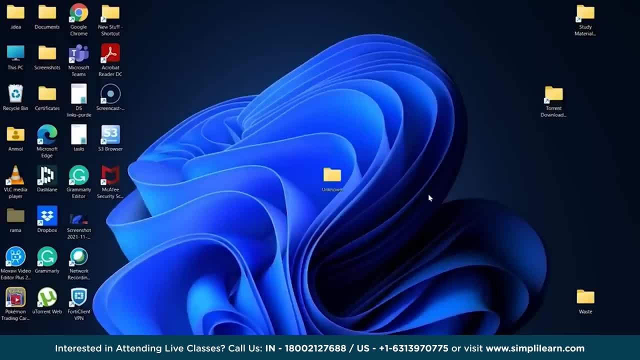 a hacking attempt by a hacker or a cyber criminal. Then there are also cases when the system's cursor moves on its own and performs tasks that are not initiated by us and performs copying of different people to other. This is due to a hacking attempt that was done on our system. 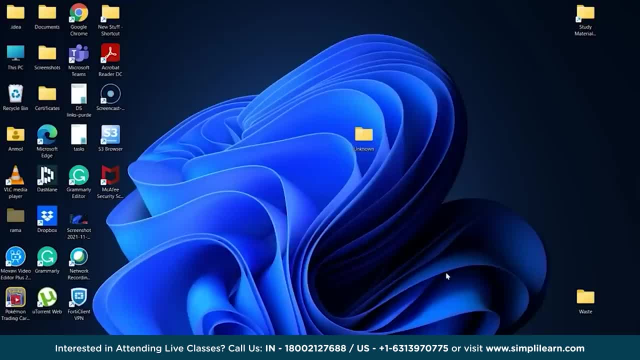 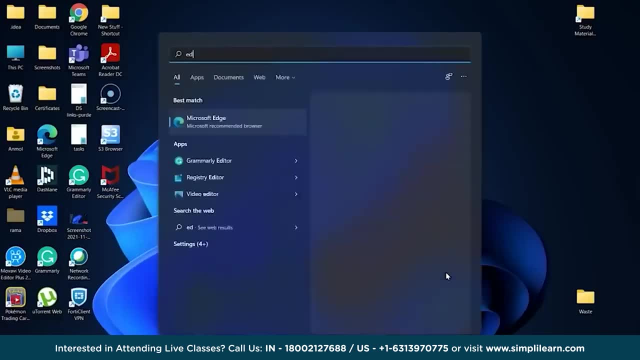 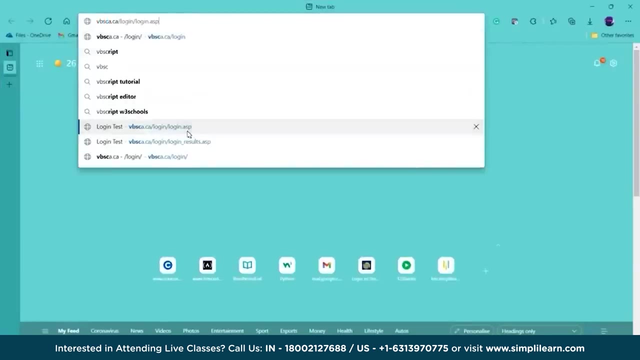 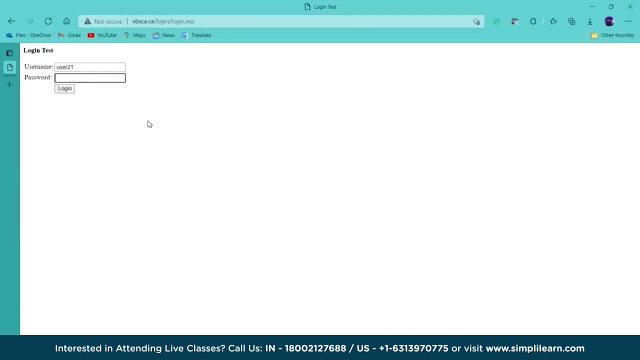 and the hacker has taken control of our system. Then there are also cases regarding login issues or password problem. For example, if I want to access into my account and there is a problem with the password, it might be due to the attempt of hacking into my account. 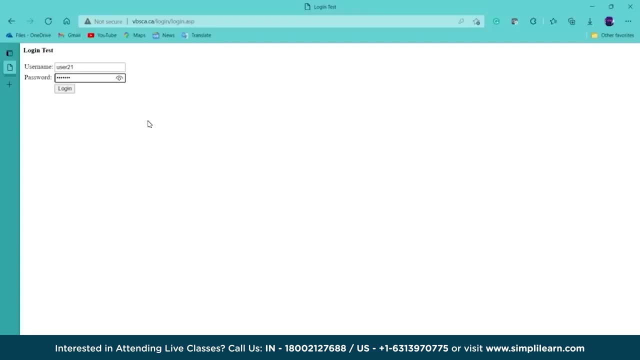 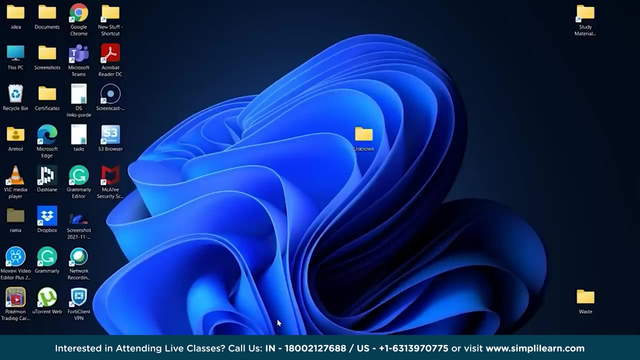 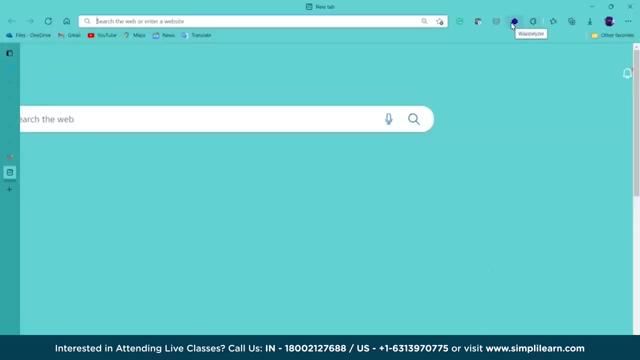 by a professional hacker. Seems like there is a problem with the username, which means there was a hacking attempt by a professional hacker. We can further check hacking attempts by accessing our web browser and checking whether there is some extra add-ons or unknown add-ons that wasn't installed. 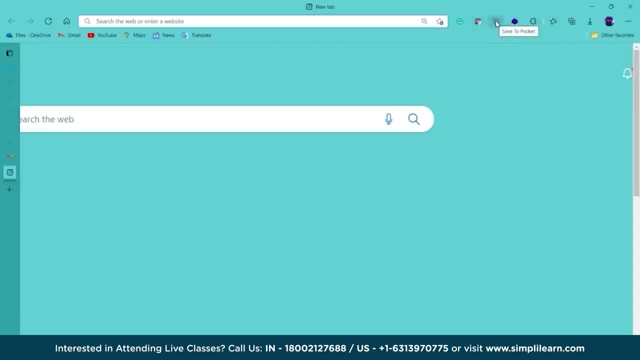 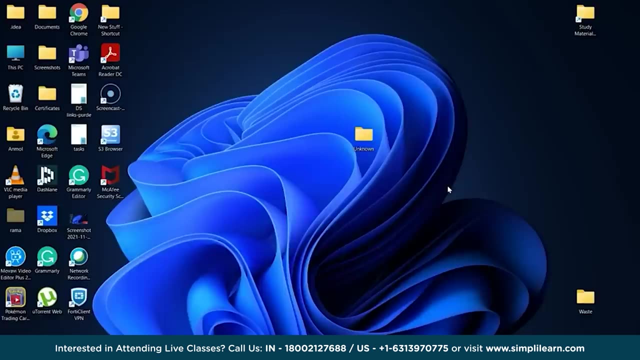 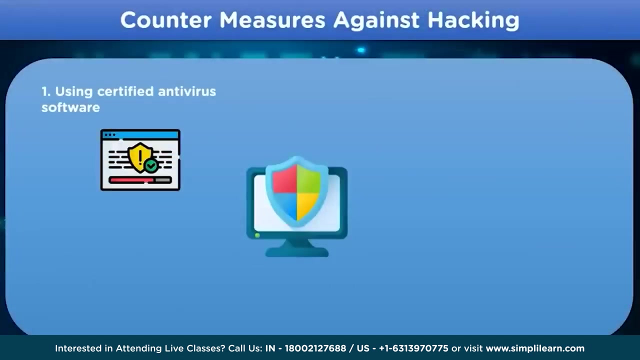 by us. This might also indicate a hacking attempt on the system. Now that we are clear about how to check whether a system is hacked or not, let's take a look at some of the countermeasures against hacking. Let's begin The first point regarding 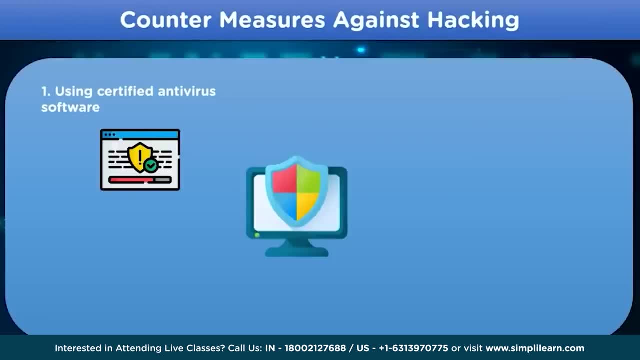 how to avoid hacking is: do regular manual security checks and keep the system security updated. Using certified antivirus software is a basic countermeasure against hacking attempts And, if possible, visit only secure websites for surfing on the internet, or use VPN or other internet security applications to mask your system's network. 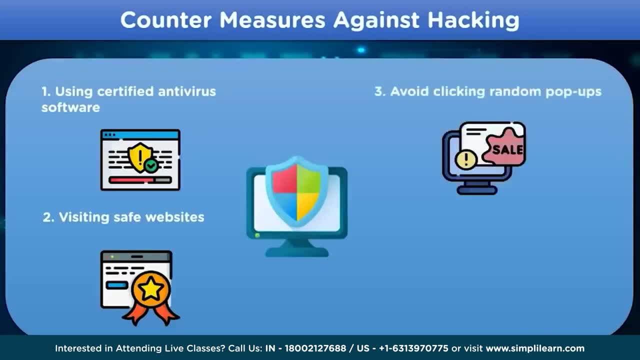 to avoid any hacking attempts for the device. Then we have avoid clicking on random web pop-ups and ads to avoid hackers from getting into a system and accessing a device data. And, lastly, use strong passwords and complex passwords for your login details. Applying these countermeasures, 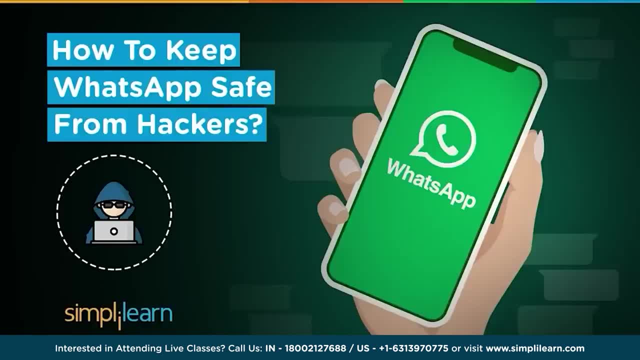 we can avoid hacking to a certain extent. The concept of instant messaging crossed into the mainstream in the 1990s, allowing friends, acquaintances, colleagues and like-minded thinkers from all over the world to connect in real time. Since then, instant messaging 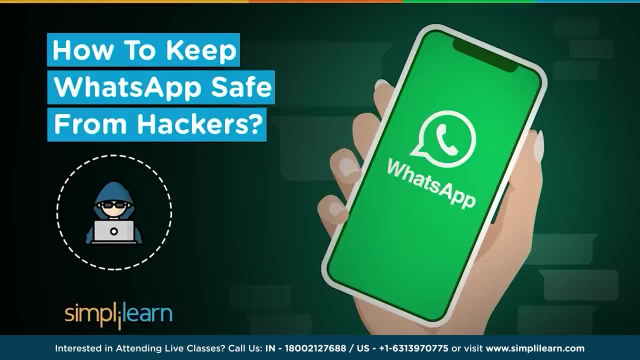 has revolutionized how we communicate, and today, over a billion people are signed up for at least one messaging app, And it intuitively integrates features like video, photos, voice, e-commerce and gaming with plain old messaging. Among these apps, WhatsApp has comfortably 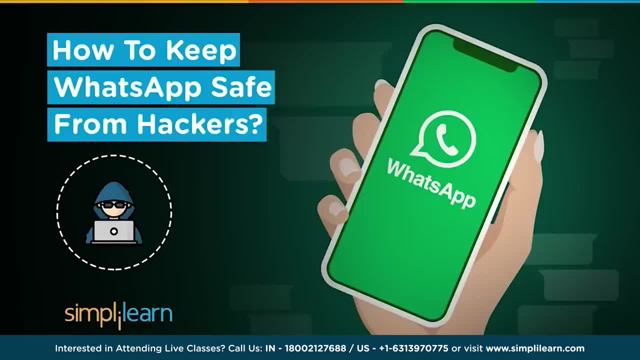 found its place among the most popular messaging platforms. Like everyone associated with the internet, a matter of security is never far away. Considering the huge user base of this messaging app, hackers are always on the lookout for compromised accounts to grab. Today, we are going to cover some of the ways. 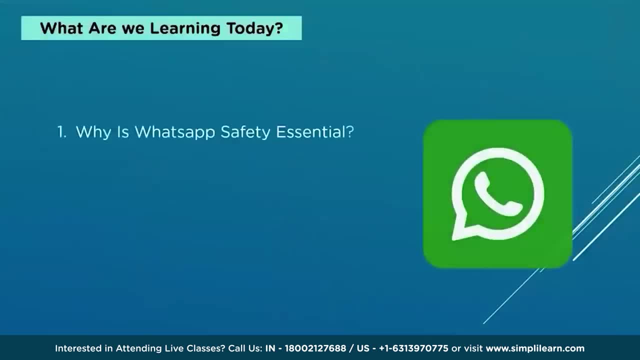 we can protect our WhatsApp account from hackers. We start by learning about the importance of security when it comes to WhatsApp and instant messaging apps in general. Next, we cover some of the most important steps that should be followed in order to protect our WhatsApp accounts. 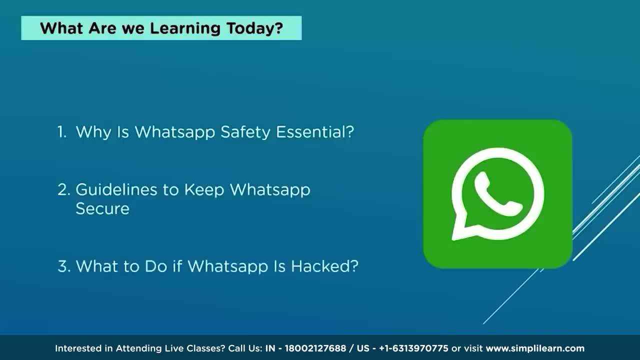 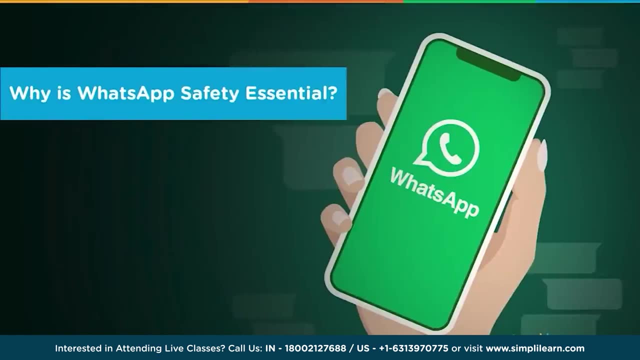 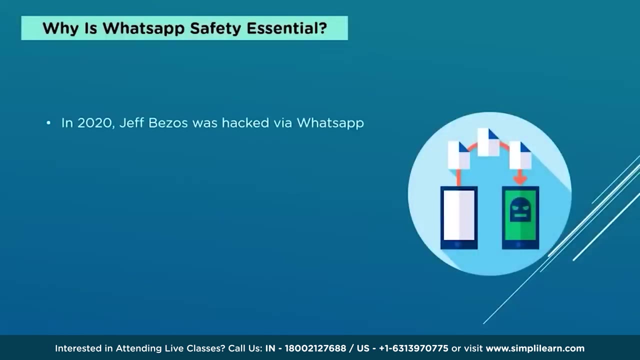 from hackers. Finally, we learn what we should do when a WhatsApp account gets compromised. Let's start by learning why we need to focus on the safety of WhatsApp In the year of 2020,. the big news was about Amazon CEO Jeff Bezos. 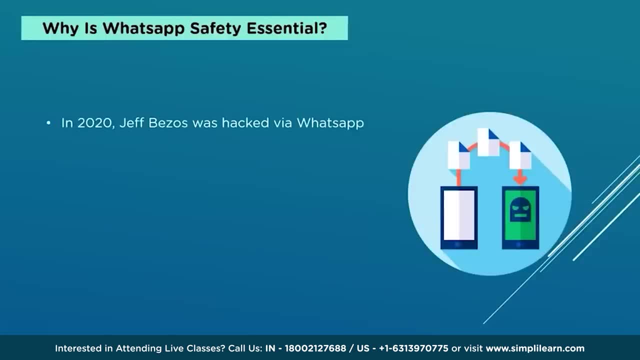 and his phone being hacked by Saudi Arabia. A report coming from The Guardian suggested that Bezos' phone was hacked via a video file sent on WhatsApp. The report said that Bezos' mobile phone was hacked by Saudi Arabian Prince in the year 2018. 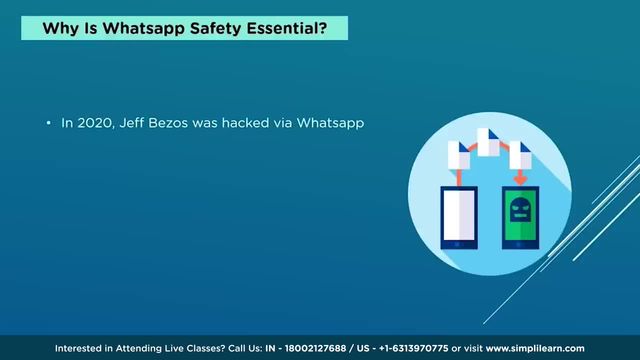 and gigabytes worth of data was stolen from the device, While there are some issues being raised about the report, which states with the medium to high confidence that Jeff Bezos' phone was hacked by a regular user- After all, if the phone of one of the world's 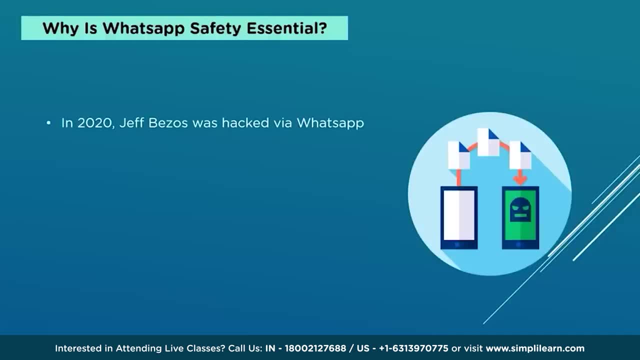 most powerful men can be hacked. the same can happen to any one of us as well. When it comes to regular users, we exchange messages with our loved ones regarding a paradigm of topics. The information which may seem trivial initially can later function as ammunition. 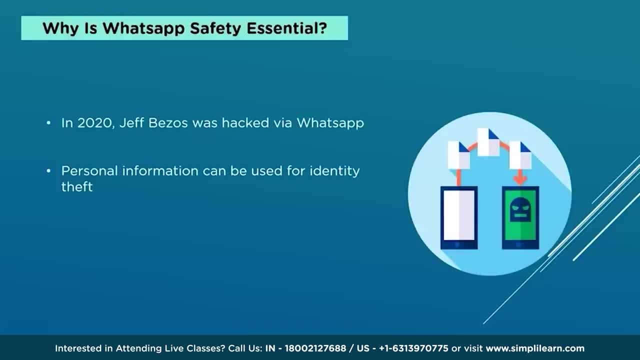 for a campaign regarding identity theft. Basic information like preferred banks, occasional dining places, can go a long way in social engineering attacks, further increasing the need for secure messaging habits. WhatsApp uses end-to-end encryption to protect all communication on its platform. These encryption keys not only make it. 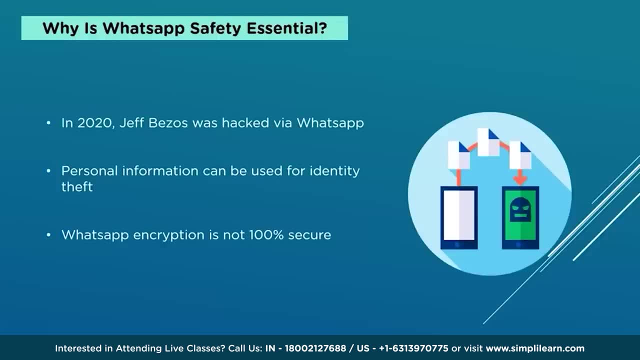 impossible to decrypt messages, but they also prevent third parties and even WhatsApp from accessing messages or calls, But not entirely. Although end-to-end encryption makes WhatsApp more secure than other communication apps, no app is 100% safe to use, Like any application or digital device. 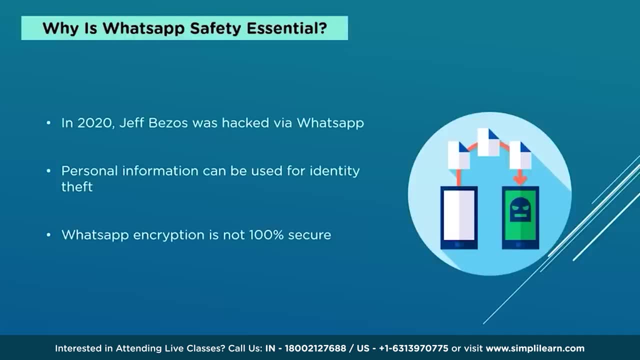 WhatsApp is often targeted by bad actors. It also has access to your contacts and tracks where and how long you use it, putting your privacy and personal information at risk. We all have access to our cell phones, so it's no surprise that SMS two-factor authentication. 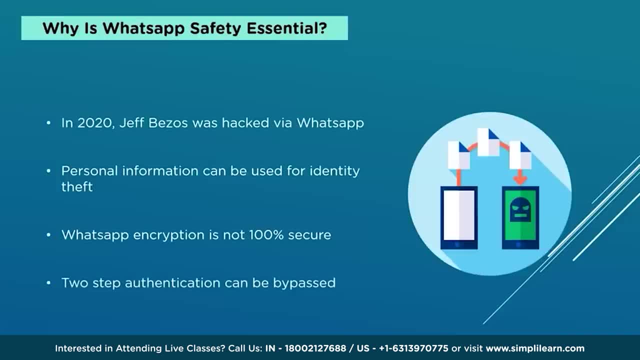 is one of the most widespread types of MFA available. You don't need any apps or digital keys and it's not tied to a specific ecosystem. Unfortunately, it's also not a secure multi-factor authentication method. The nature of SMS itself opens up your organization. 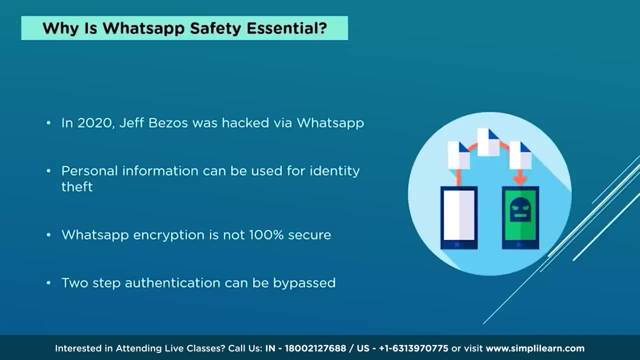 at risk. Hackers may have many ways to leverage SMS to find a way into your accounts and network, Be it via spoofed SIM cards or message hijacking WhatsApp. two-factor authentication using SMS isn't a foolproof solution. Now that we understand. 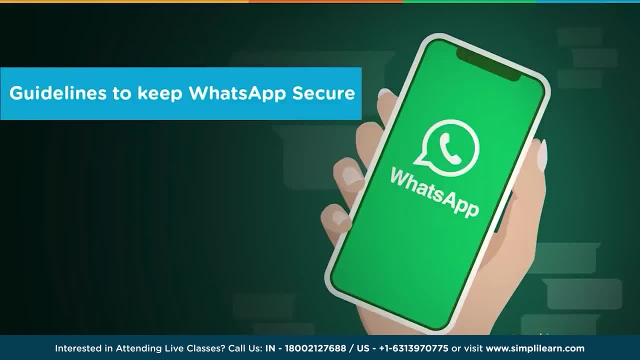 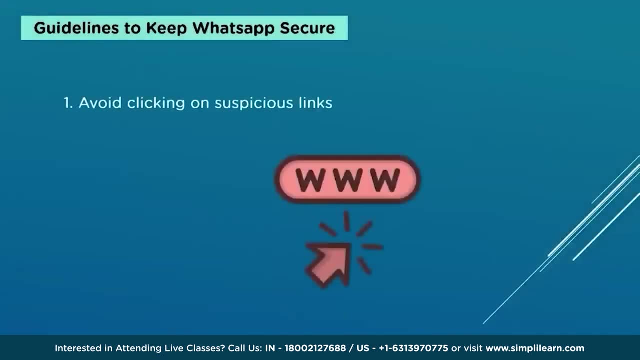 the variety of reasons why WhatsApp needs extra security. let's go through some of the ways we can achieve this. It is more than probable that one fine day you might receive a WhatsApp message or even an SMS that your order is delayed. please check its data here. 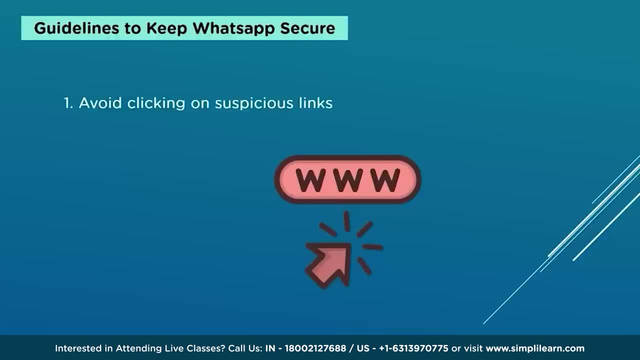 or your account is locked and please unlock it here. or even some tempting messages like win free 3G and movie tickets here. Some of them may sound intimidating and some of them may be lucrative, But they all have one purpose: to trick you into clicking that link. 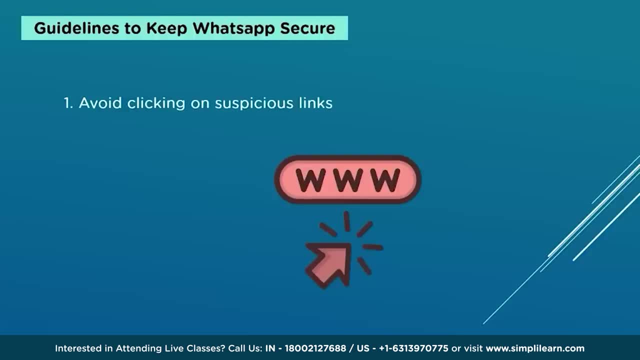 and once you do that, it's already over. It will install malware on your phone and you won't have a clue about it Only when you start noticing that your phone bills are abnormally high or your bank account has been used without your permission. 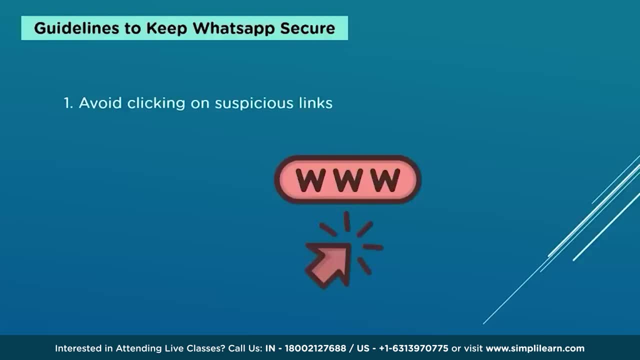 will. the authorization will dawn upon you that something is wrong with your phone, But by then it may be too late. WhatsApp in itself provides various privacy options to users. The messaging platform provides users with option to choose who they want to share their profile photo status. 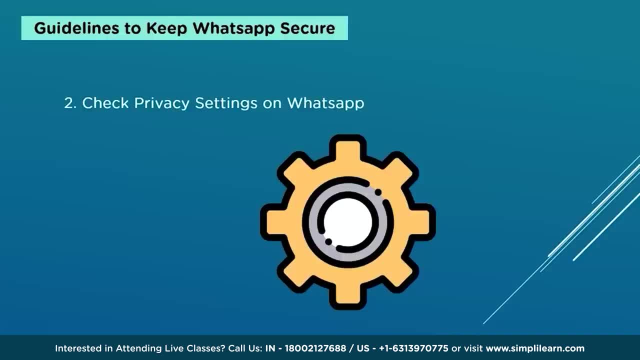 and other details with. It's a good idea to change the settings to contacts only. This means only phone numbers that are saved on your smartphone will be able to see your profile, photo, status and other details as well. Make sure you enable the option. 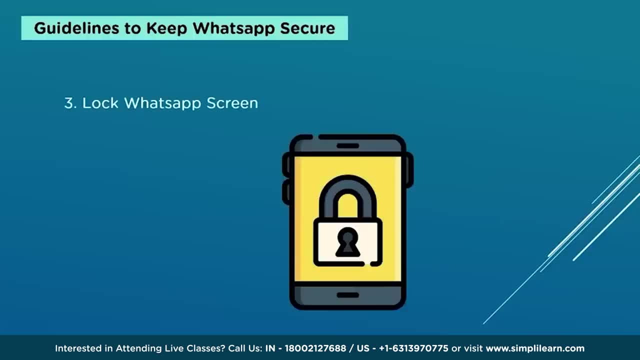 to lock the screen every time WhatsApp is closed. This will ensure no one else but you can open your WhatsApp account. Just head to the settings menu, privacy, and select the screen lock option. You will then need to register your fingerprint After the process is completed. 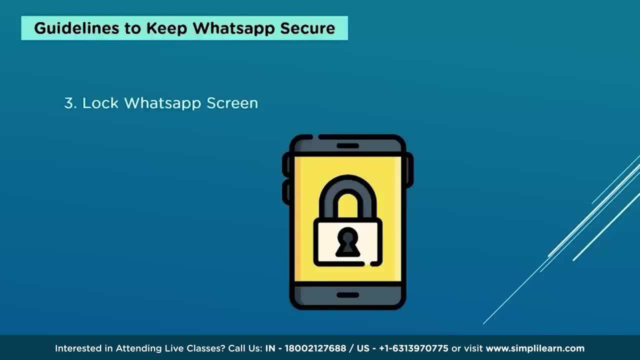 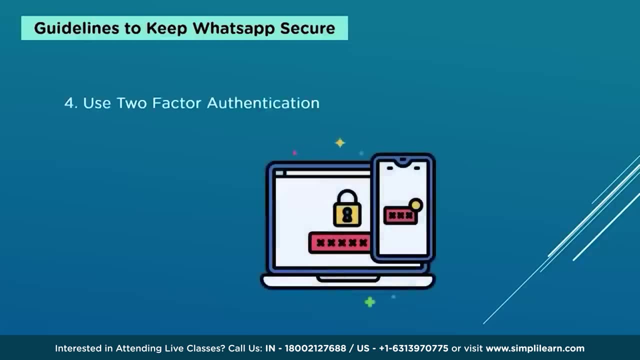 you will have to scan your fingerprint every time you open the WhatsApp app. This adds an extra layer of security. The two-step verification works as an extra layer of security and helps WhatsApp users to protect their OTPs and documents shared through WhatsApp. It's very easy to set up a PIN. 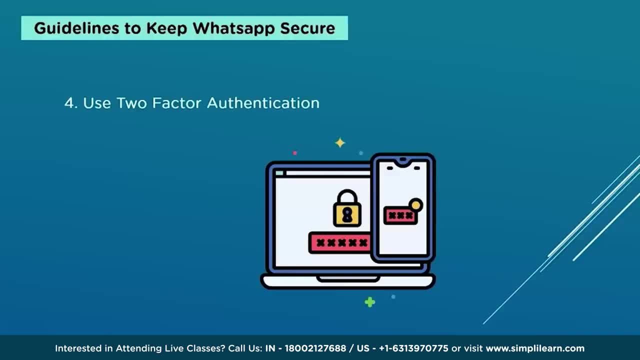 to activate a two-step verification, Users have to enter it periodically. once it is activated, WhatsApp will sometimes keep asking users to enter this six-digit passcode. Users cannot disable this without disabling the two-step verification feature altogether, In case users do not provide WhatsApp. 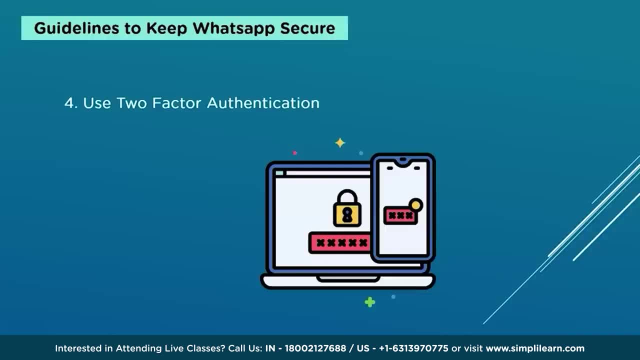 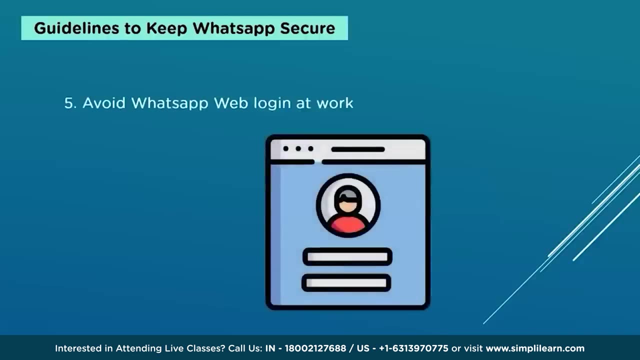 with an email ID and want to disable two-step verification, then the number will be permitted to re-verify on WhatsApp without the passcode after seven days, However, the users will lose all pending messages upon re-verifying. We often have the tendency to log into WhatsApp. 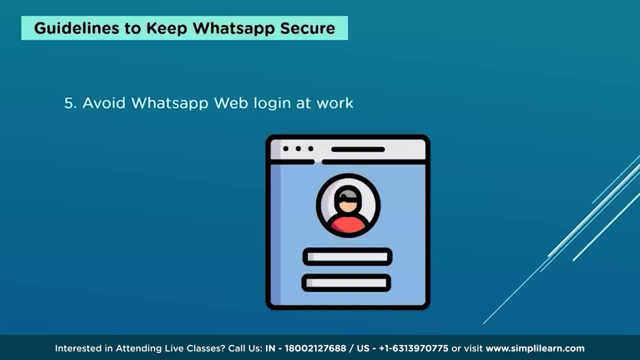 web at the office and then leave the account open on the desktop. This habit can actually create problems for you. Someone else sitting on the same PC can access all your chats without you even realizing it. It's a good practice to log out from WhatsApp before leaving. 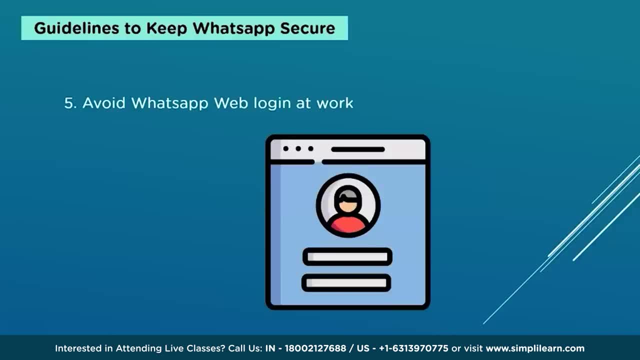 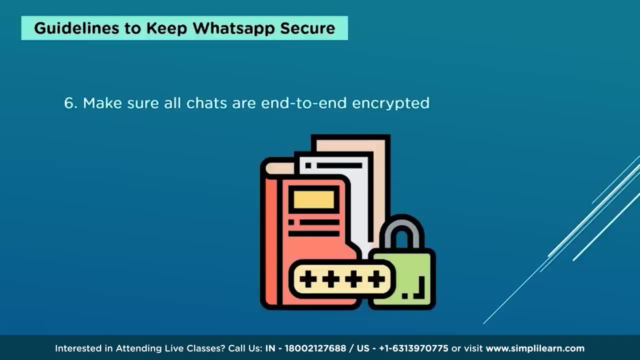 the office. It just takes a few seconds to log in again by just scanning the code and you're done. All WhatsApp users should ensure that the chats are end-to-end encrypted. To verify that a chat is end-to-end encrypted: open the chat. tap on the name of the 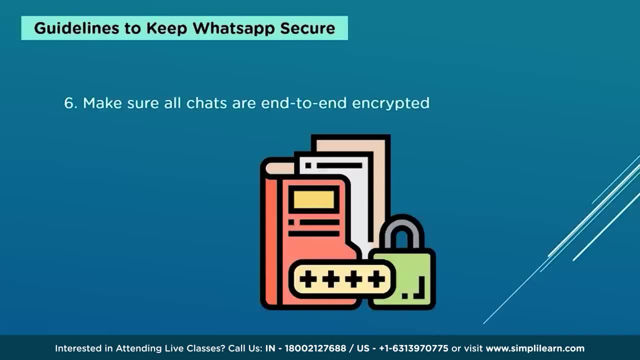 contact to open the contact info screen and then tap Encryption to view the QR code and a 60-digit number. WhatsApp end-to-end encryption ensures that only you and your contact can read the messages that are being exchanged, and nobody in between, not even. 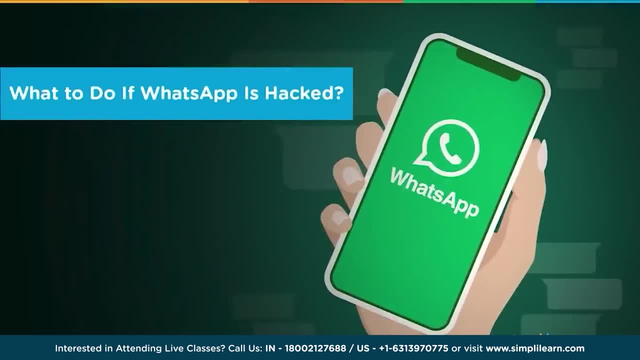 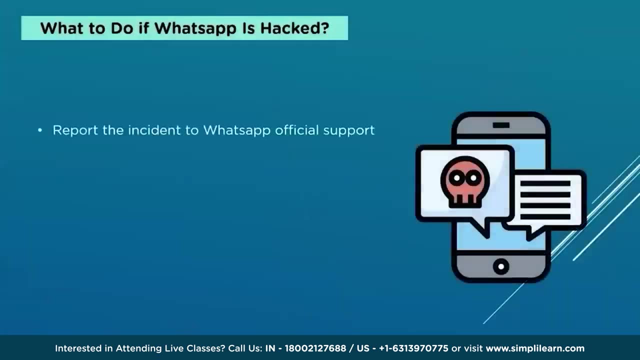 WhatsApp. With the necessary guidelines out of the way, let us go through the recommended course of action. should our WhatsApp accounts be compromised, The first and most important thing that you need to do is report the issue to the WhatsApp support team for assistance. Make sure. 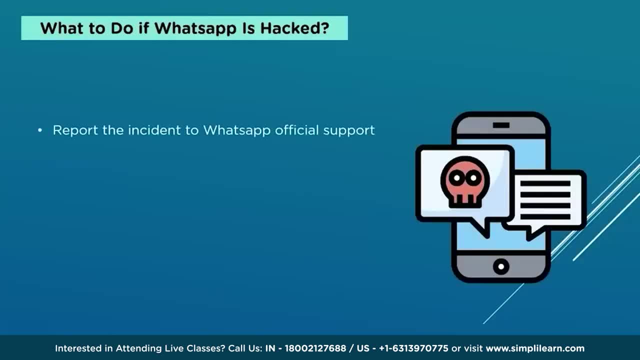 that you reach out to the support team through its help desk and report the hacking attempt. WhatsApp Help Center will take the shortest time to resolve your issue, via email or within the app itself. This will help you to take prompt legal action against the hackers. 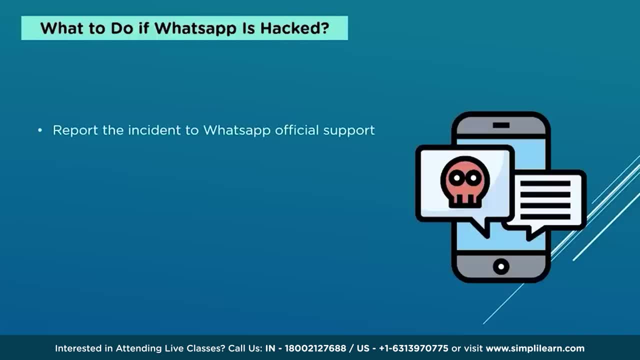 If you can't access your email, call the support team. In some cases, the support will deactivate your WhatsApp account and request you to reactivate it within 30 days if you don't want it to be deleted completely. When someone compromises your WhatsApp account, they can now. 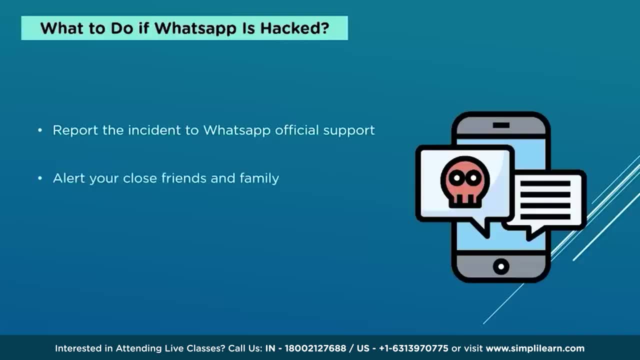 send messages to your contacts stating that the company sent your verification code and gain access to that account. That's why one of the first things you'll want to do is send a message to your friends and family letting them know that you've lost access to. 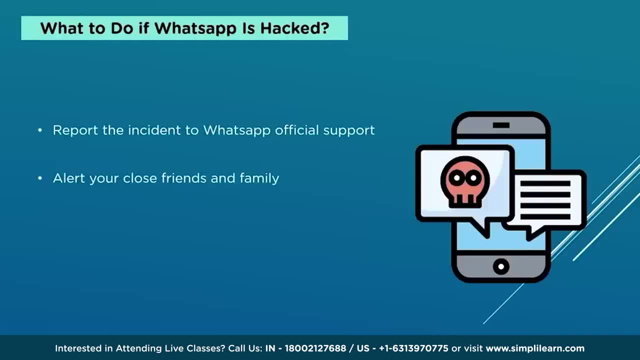 your account. This action prevents further exploitation of your account and others. Another reason you'll want to let your contacts know you have no access to your WhatsApp account is that they may fish for personal information, From your banking number to your email address. hackers will 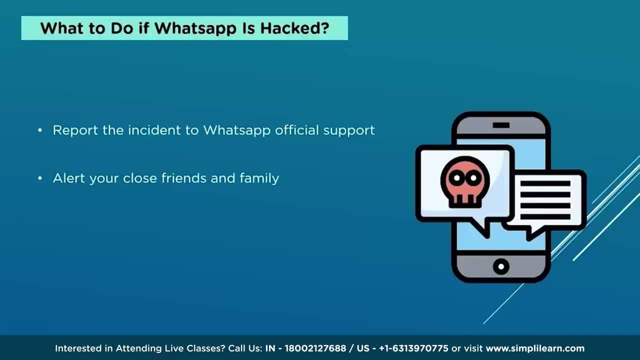 cleverly attempt to gain as much access to your personal information as possible. WhatsApp Web is an extension of WhatsApp Messenger over the web that facilitates easy synchronization of our smartphone and personal computer. This is the biggest security threat that hackers can easily exploit to get into your personal data. 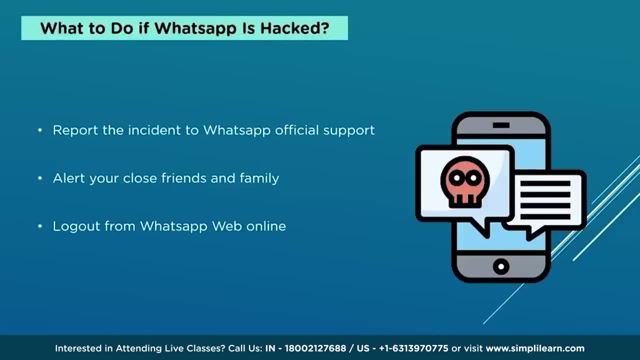 over WhatsApp. Therefore, it is highly recommended that you use this WhatsApp feature carefully. Once you notice that your WhatsApp Messenger has been hacked, go to your WhatsApp web and tap or click on the logout from all computers option. This will deactivate all the web extensions of your account. 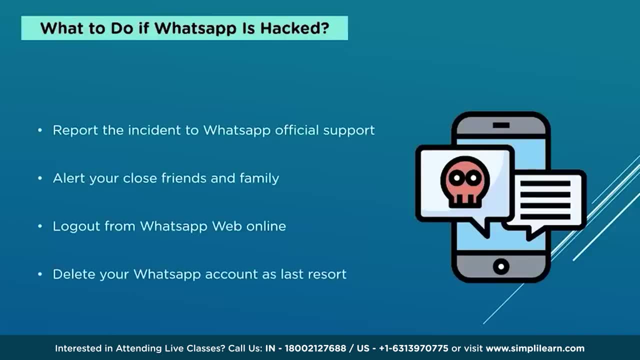 Under the unfortunate circumstances where the account recovery doesn't seem likely, you can always ask WhatsApp support to delete your account permanently. While far from the ideal solution, it can act as a fail-safe option. if you want to protect your personal data at any cost possible, You can always. 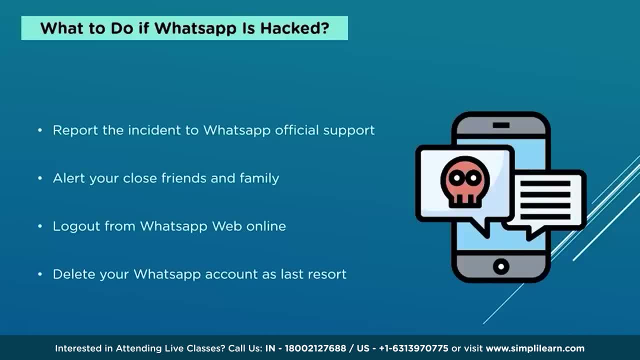 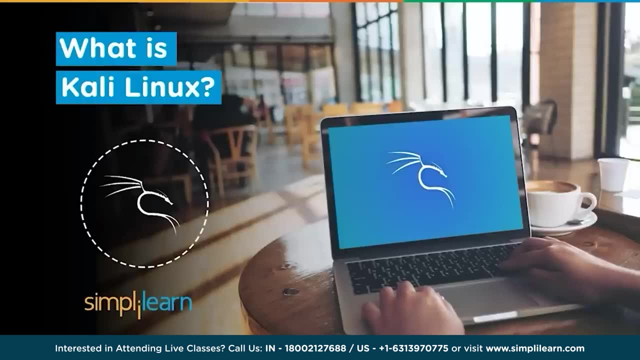 open a new account later with the security issues mitigated. It's no secret that the majority of our internet usage is at the risk of being hacked, be it via unsafe messaging applications or misconfigured operating systems To counteract this void of digital security. 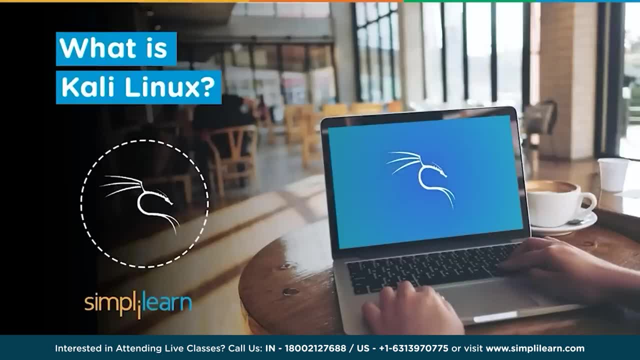 penetration testing has become the norm when it comes to vulnerability assessment. Kali Linux is an operating system that has become a well-known weapon in this fight against hackers. A Linux distribution that is made specifically for penetration testers, Kali Linux has layers of features that we will be covering in today's 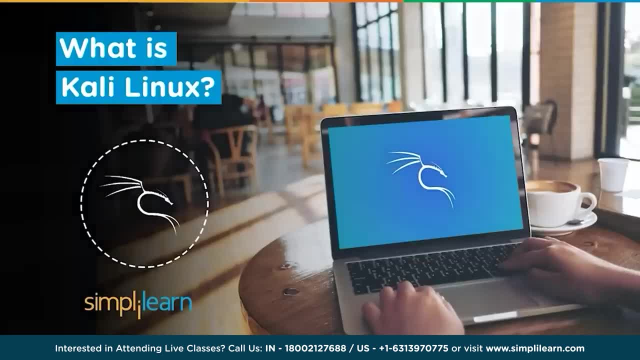 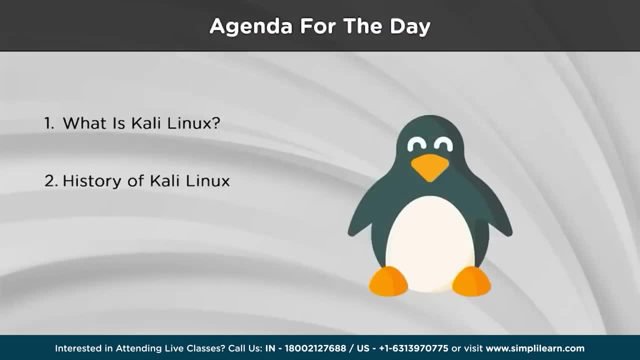 lesson. Let's take a look at the topics to be covered in this video. We start by learning about Kali Linux and a basic explanation of its purpose. We take a look at the history of Kali Linux, from the story of its origin to its current day exploits. 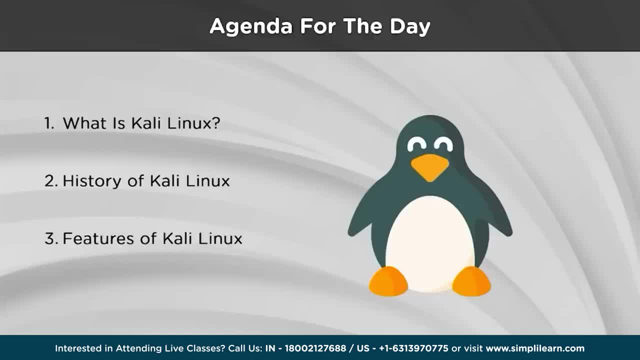 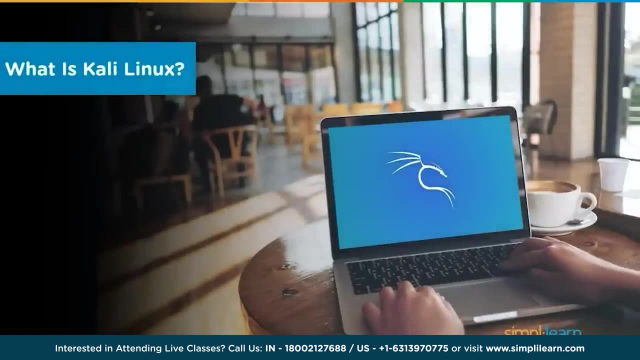 Next we learn a few distinct features of Kali that make it an attractive choice for penetration testers worldwide. Finally, we take a look at the multiple ways we can install Kali Linux to start our journey in the world of penetration testing, Let's start by learning about Kali. 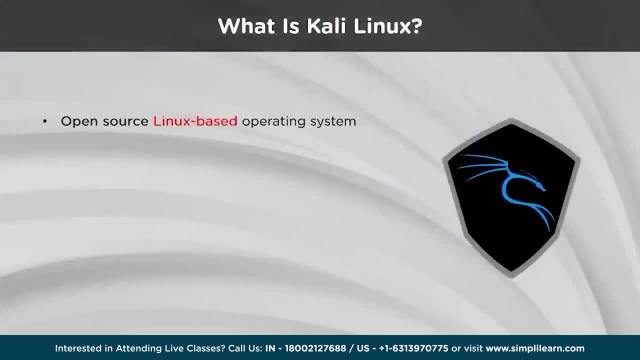 Linux in general. Kali Linux, which is formerly known as Backtrack Linux, is an open source Linux distribution aimed at advanced penetration testing and security computing. It contains several hundred tools that are targeted towards various information security tasks, such as penetration testing. 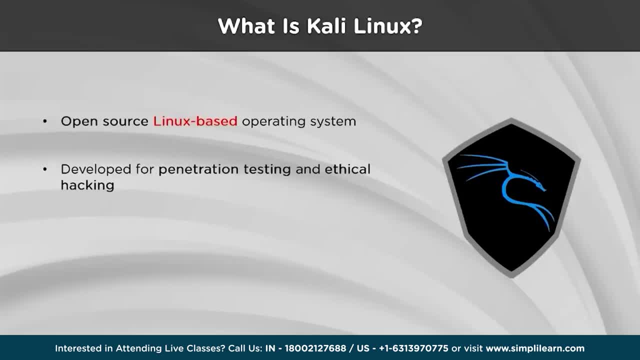 security, research, computer forensics and reverse engineering. Kali Linux is a multiple platform solution accessible and freely available to information security professionals and hobbyists. Among all the Linux distributions, Kali Linux takes its roots from the Debian operating system- Debian. 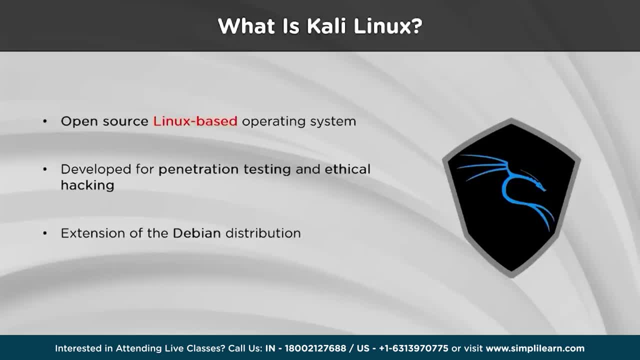 has been a highly dependable and stable distribution for many years, providing a similarly strong foundation to the Kali desktop. While the operating system is capable of practically modifying every single part of our installation, the networking components of Kali become disabled by default. This is done. 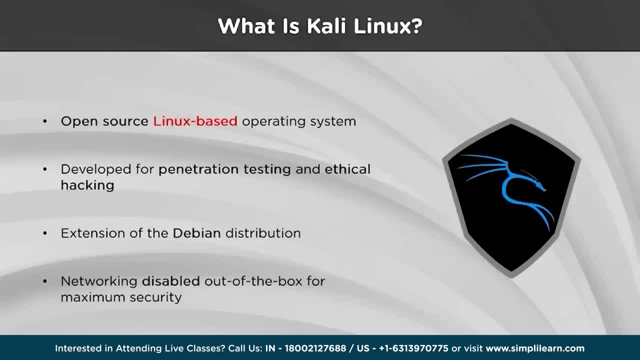 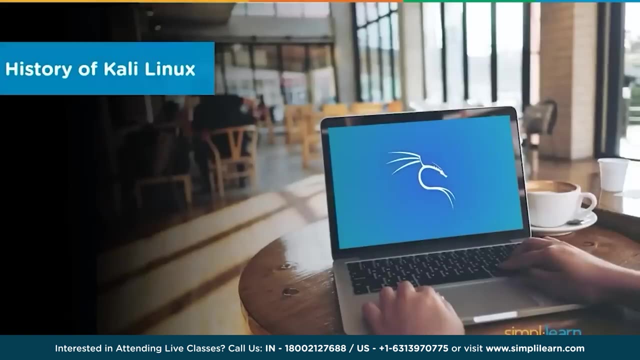 to prevent any external factors from affecting the installation procedure which may pose a risk in critical environments. Apart from boosting security, it allows a deeper element of control to the most enthusiastic of users. We did not get Kali Linux since the first day. How did it come into existence? 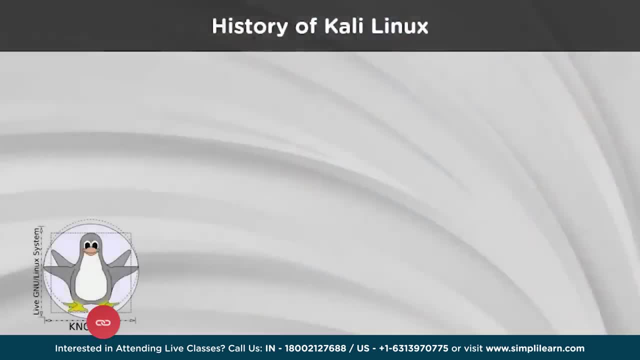 Let's take a look at some of its history. Kali Linux is based on years of knowledge and experience in building, penetration, testing and operating systems. During all these project lifelines there have been only a few different developers, as the team has always. 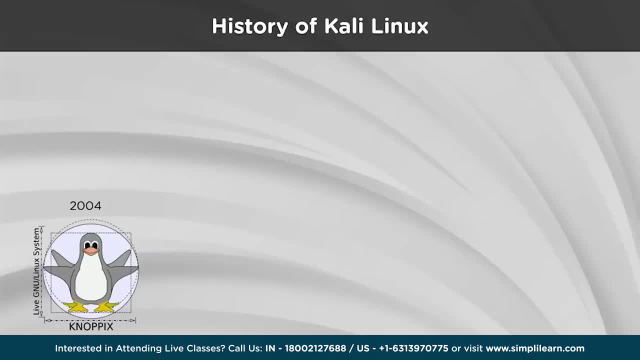 been small. The first project was called Wopex, which stands for White Hat Knopex. As can be inferred from the name, it was based on the Knopex operating system as its underlying OS. Wopex had releases ranging from version 2.0. 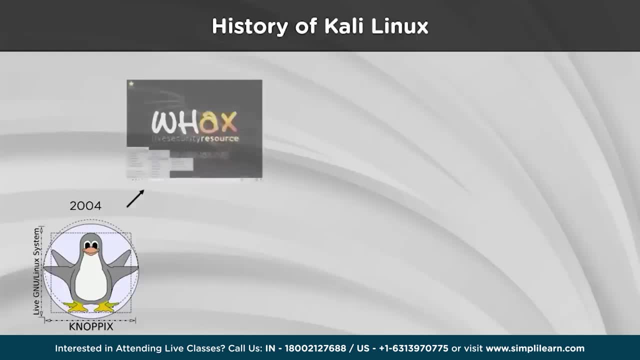 to 2.7.. This made way for the next project, which was known as Wax, or the long hand being White Hat Slacks. The name change was because the base OS was changed from Knopex to Slacks. Wax started at version 3 as a nod it carrying. 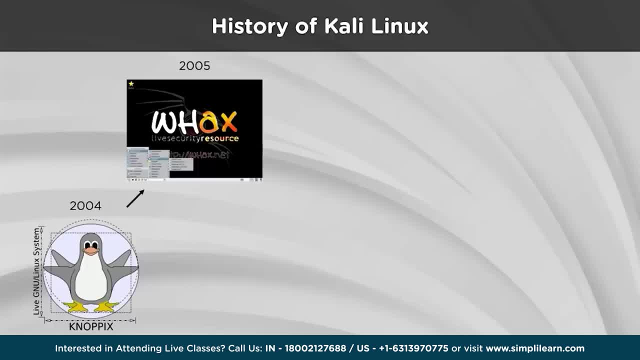 on from Wopex. There was a similar OS being produced at the same time: Auditor Security Collection, often being shorted to just Auditor, Which was once again using Knopex. Its efforts were combined with Wax to produce Backtrack. Backtrack was based on Slackware. 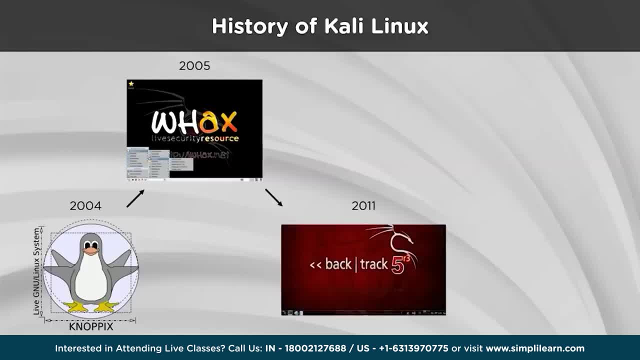 from version 1 to version 3, but switched to Ubuntu later on, with version 4 to version 5.. Using the experience gained from all of this, Kali Linux came after Backtrack in 2013.. Kali started off using Debian stable. 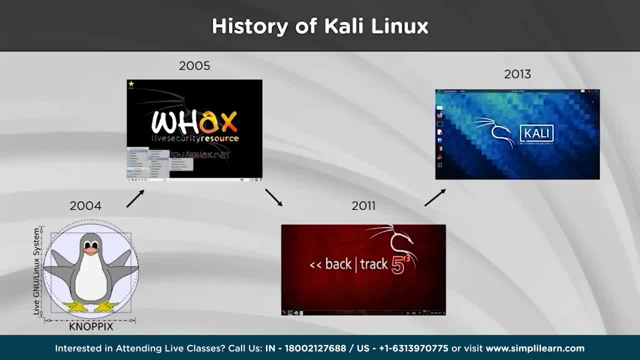 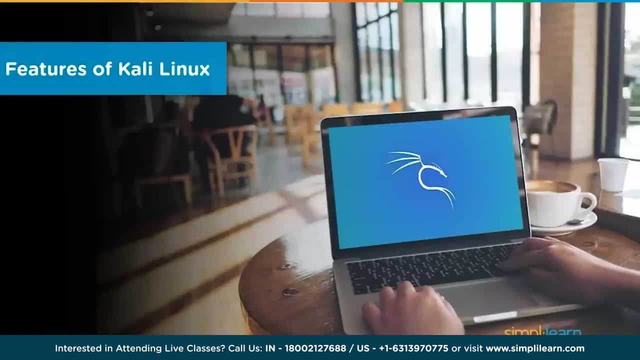 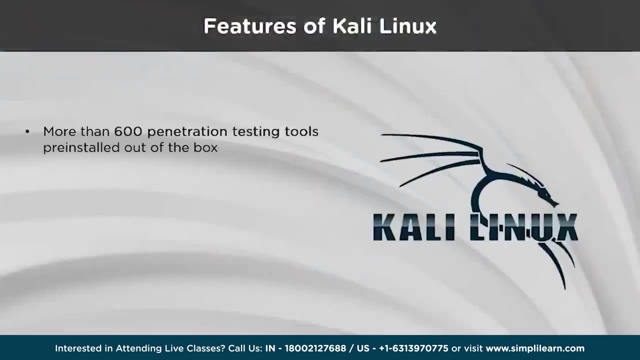 as the engine under the hood before moving to Debian testing, when Kali Linux became a rolling operating system. Now that we understand the history and the purpose of Kali Linux, let us learn a little more about its distinct features. The latest version of Kali comes with more than 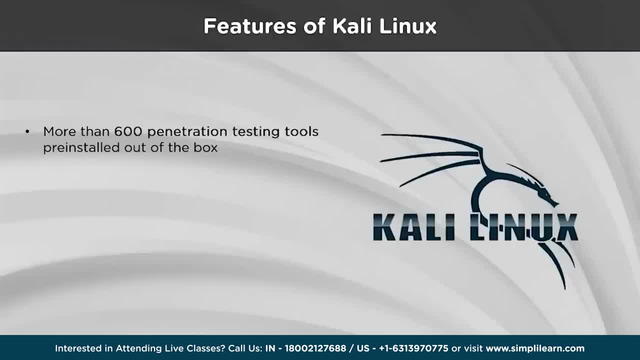 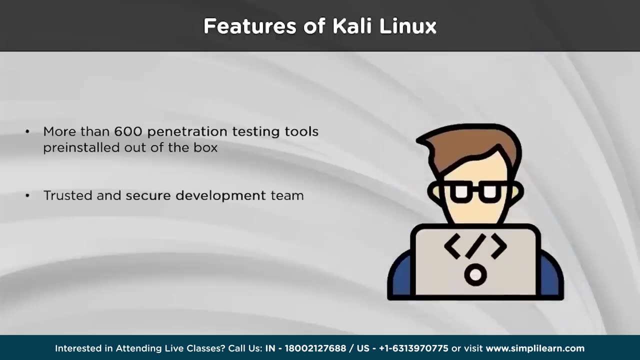 600 penetration tools pre-installed. After reviewing every tool that was included in Backtrack, developers have eliminated a great number of tools that either simply did not work or which duplicated other tools that provided the same or similar functionality. The Kali Linux. 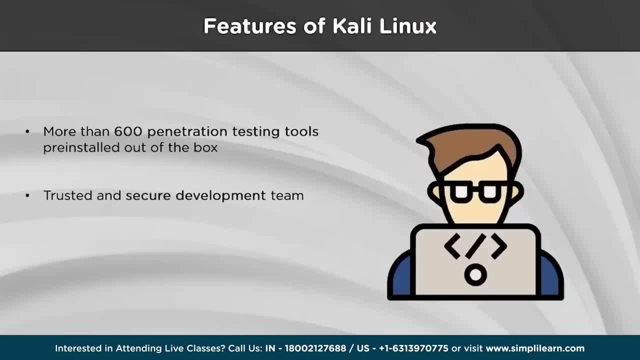 team is made up of a small group of individuals who are the only ones trusted to commit packages and interact with the repositories, all of which is done using multiple secure protocols. Restricting access of critical code bases to external assets greatly reduces the risk of 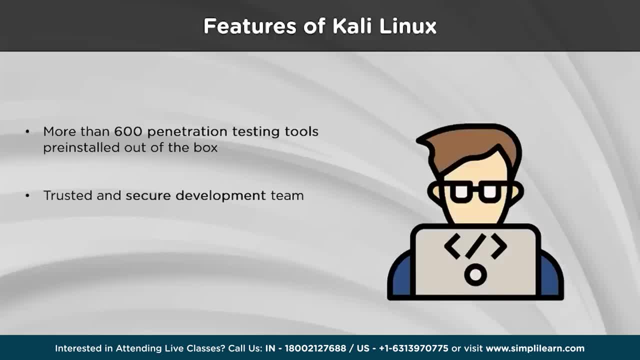 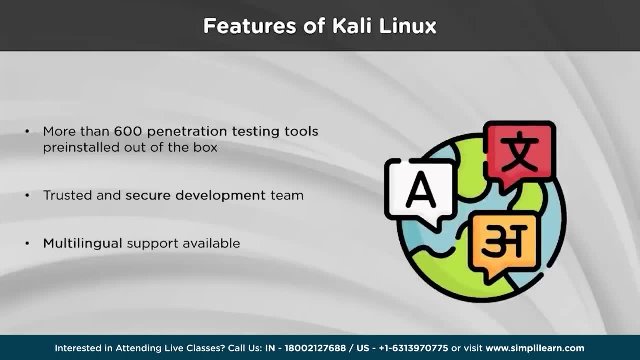 source contamination which can cause Kali Linux users worldwide a great deal of damage as a direct victim of cybercrime. Although penetration tools tend to be written in English, the developers have ensured that Kali includes true multilingual support, allowing more users to operate. 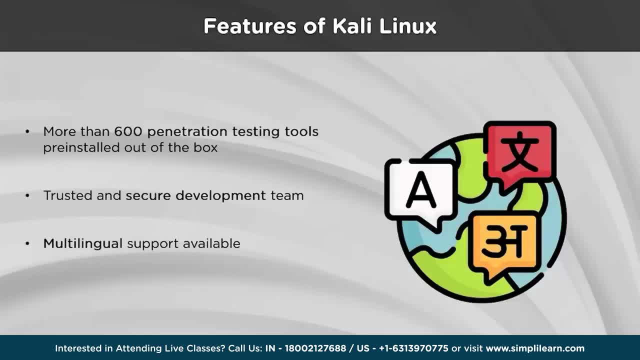 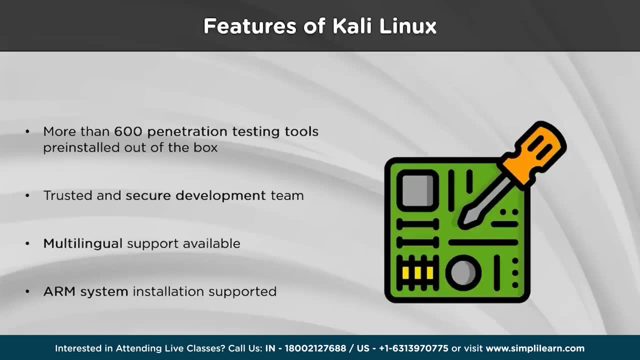 in their native language and locate the tools they need for the job. The more comfortable a user feels with the intricacies of their operating system, the easier it is to maintain a strong hold over the configuration and the device in general, Since ARM-based single board systems like the Raspberry, 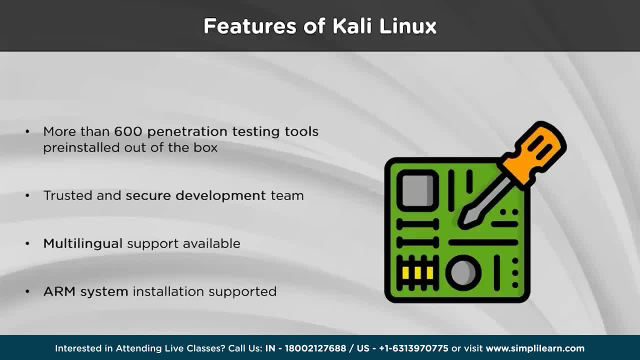 Pi are becoming more and more prevalent and inexpensive, the development team knew that Kali's ARM support would need to be as robust as they could manage with fully working installations. Kali Linux is available on a wide range of ARM devices and has ARM repositories. 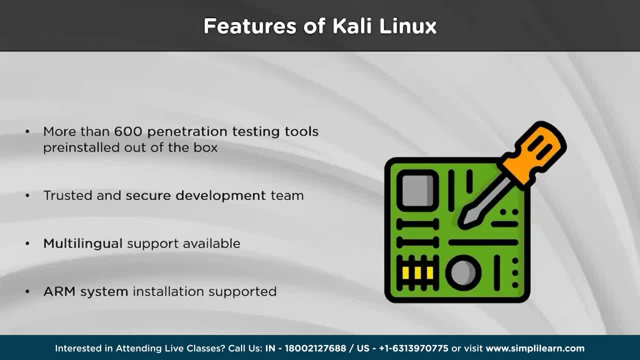 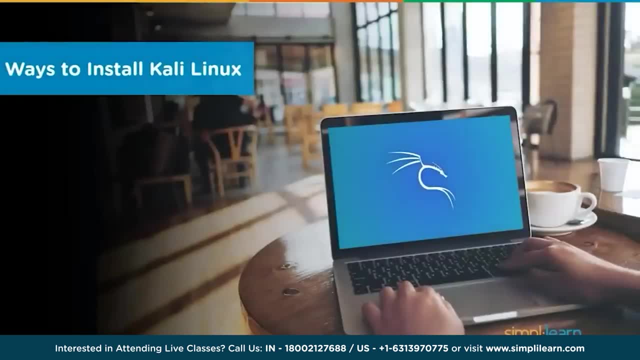 integrated with the mainline distributions, so the tools for ARM are updated in conjunction with the rest of the distribution. All this information is necessary for users to determine if Kali Linux is the correct choice for them. If it is, what are the ways that they can go? 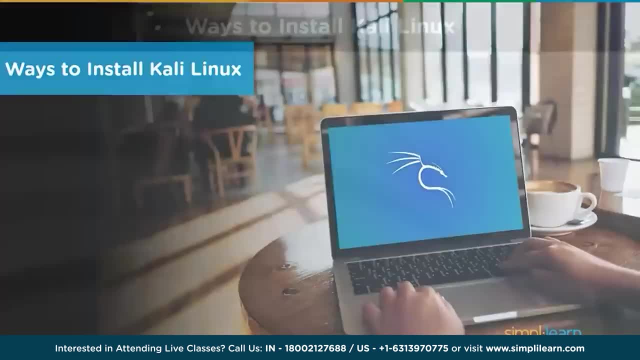 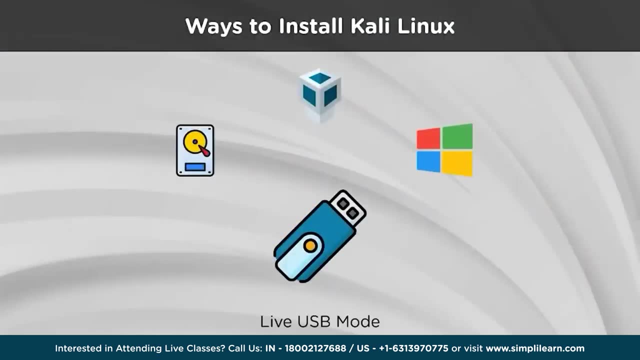 forward with this installation and start their penetration testing journey. The first way to use Kali Linux is by launching the distribution in the live USB mode. This can be achieved by downloading the installer image file or the ISO file from the Kali Linux website and flashing. 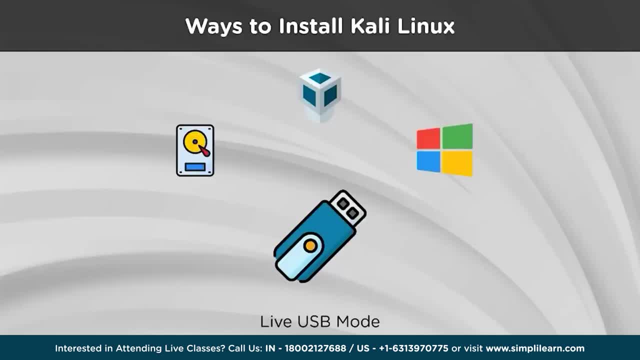 it to a USB drive with a capacity of at least 8 GB. Some people don't need to save their data permanently, and a live USB is the perfect solution for such cases. After the ISO image is flashed, the thumb drive can be used to boot a fully working installation of. 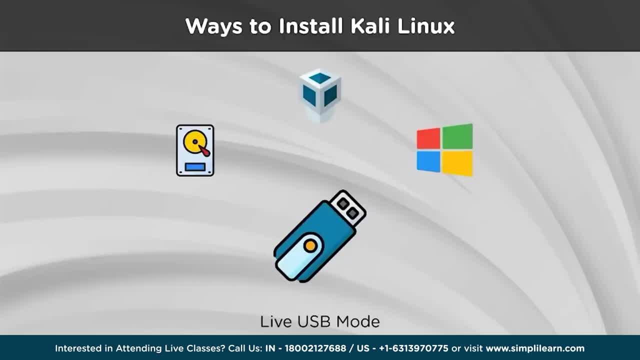 the operating system, with the caveat that any changes made to the OS in this mode are not returned permanently. Some cases allow persistent usage in live USBs, but those require further configuration than normal situations. But what if the user wants to store data permanently in the installed OS? 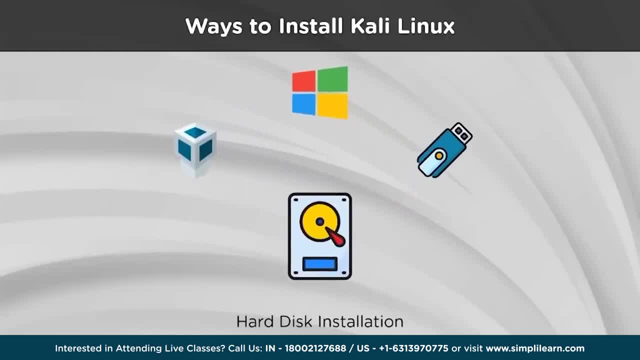 The best and the most reliable way to ensure this is the full fledged hard disk installation. This will ensure the complete usage of the system's hardware capabilities and will take into account the updates and the configurations being made to the OS. This method is supposed to override. 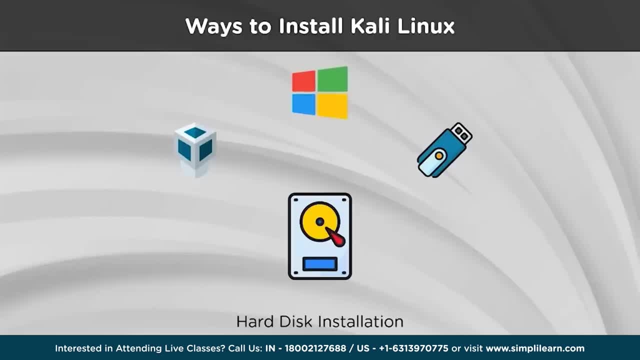 any pre-existing operating system installed on the computer, be it Windows or any other variant of Linux. The next alternative route for installing Kali Linux would be to use virtualization software such as VMware or VirtualBox. The software will be installed as a separate application on an. 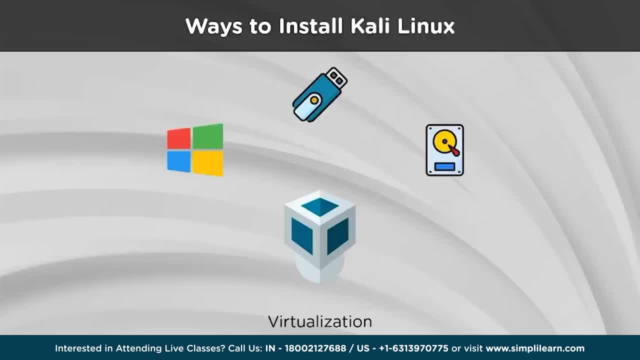 already existing OS and Kali Linux can be run as an operating system in the same computer as a Windows. The hardware requirements will be completely customizable, starting with the allotted RAM to the virtual hard disk capacity, The usage of both a host and guest operating system like Kali Linux. 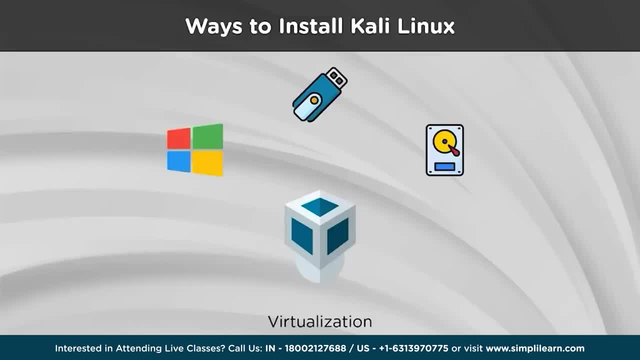 allows users a safe environment to learn while not putting their systems at risk. If you want to learn more about how one can go forward with this method, we have a dedicated video where Kali Linux is being installed on VMware while running on a Windows 10. 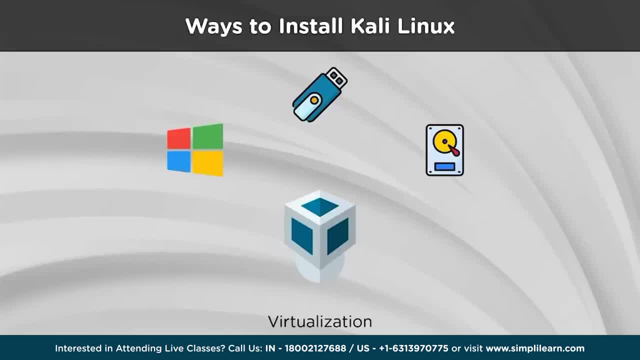 operating system. You can find the link in the description box to get started with your very own virtual machine. The final way to install Kali Linux is by using a dual boot system. To put it in simple words, the Kali Linux OS will not be overwriting any pre-installed 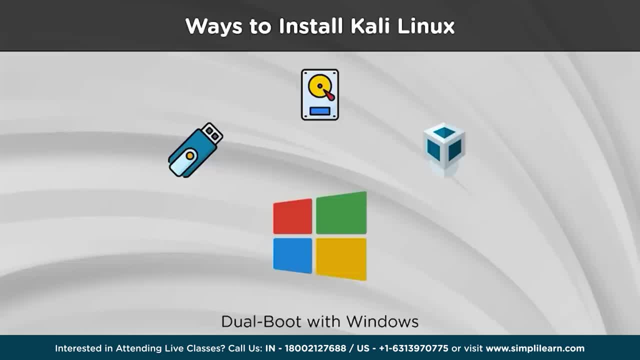 operating system on a machine but will be installed alongside it. When a computer boots up, the user will get a choice to boot into either of these operating systems. Many people prefer to keep both the Windows and Kali Linux installed. so the distribution of work and recreational 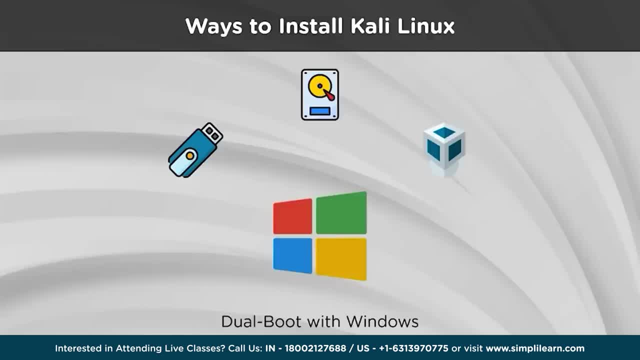 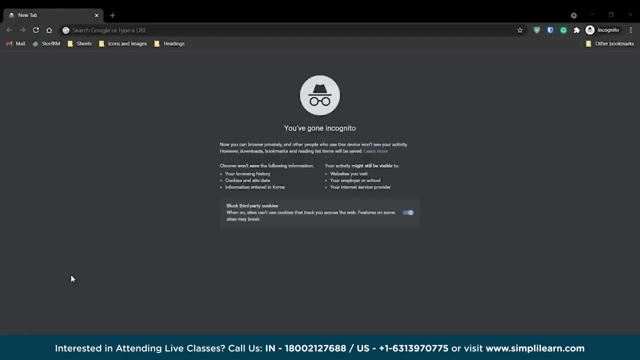 activities is also allotted effectively. It gives users a safety valve should their custom Linux installation run into any bugs that cannot be fixed from within the operating system. Now, for the convenience of explanation, we're going to install Kali Linux today on a virtual machine software. 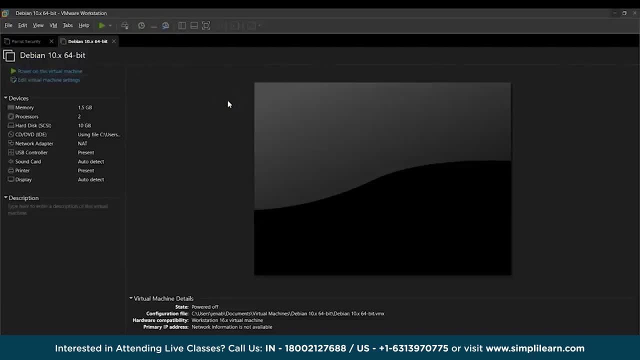 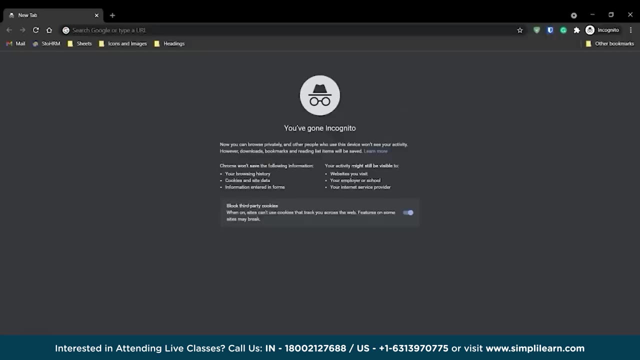 known as VMware. VMware is able to run multiple operating systems on a single host machine, which in our case is a Windows 10 system. To get started with Kali Linux installation, we have to go to the website to download an image file. We go to Get Kali. 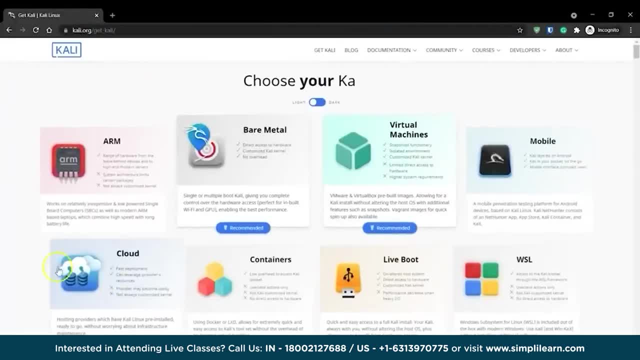 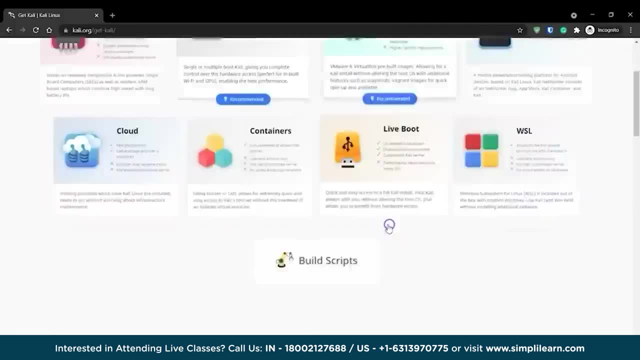 and, as you can see, there are multiple platforms on which this operating system can be inverted. As per our requirement, we're going to go with the virtual machine section. as you can see, it is already recommended by the developers. This is the download button, which will download a 64. 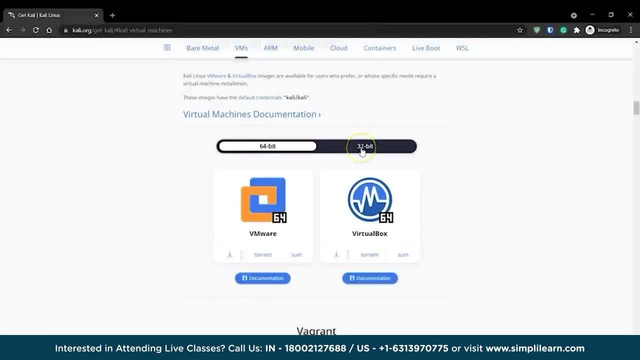 bit ISO file. We can download 32 bit, but that is more necessary for hard metal machines or if you're going to use it for older devices which do not support 64 bit operating systems yet. After clicking on the download button, we can see: 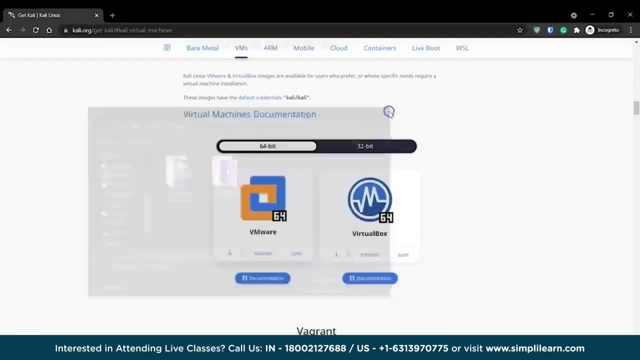 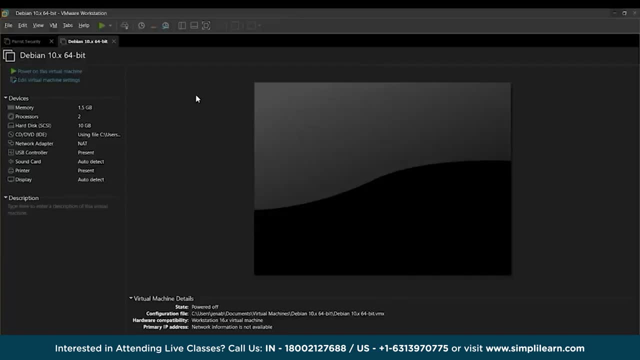 we have a WinRAR archive which will have the ISO files. For now, we have downloaded the ISO file and it is already present with me, So we can start working on the VMware side of things. Once the ISO file is downloaded, we open up VMware workstation. 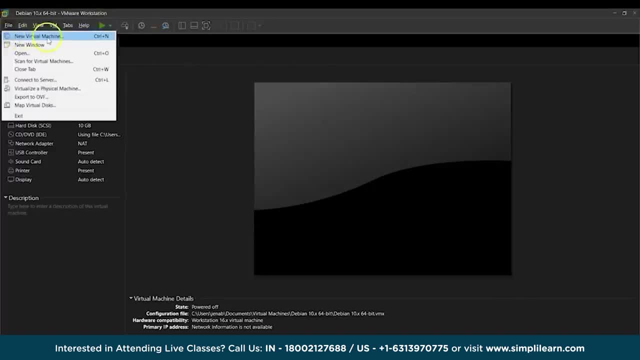 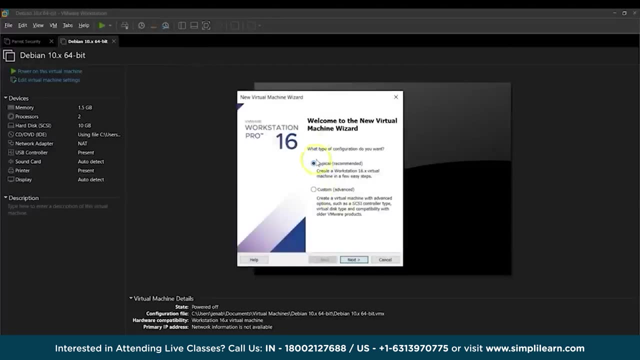 Go to File and we create a new virtual machine. In these two options, it is highly recommended to go with the typical setup rather than the custom one. The custom is much more advanced and requires much more information from the user, which is beneficial for developers. 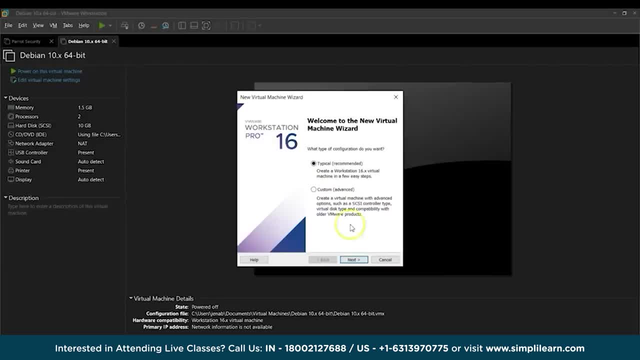 and people who are well versed with virtualization software. but for 90% of the cases typical setup will be enough. Here we can select the third option, which will be: I will install the operating system later In some operating systems we can use. 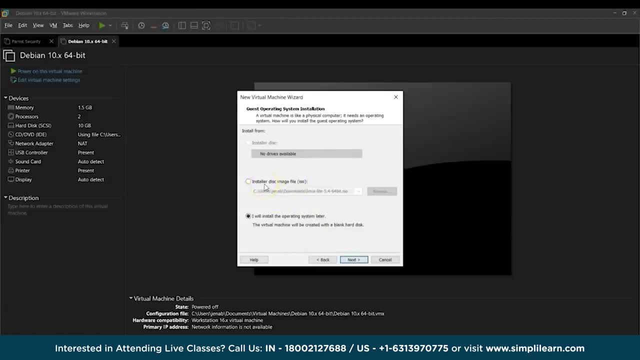 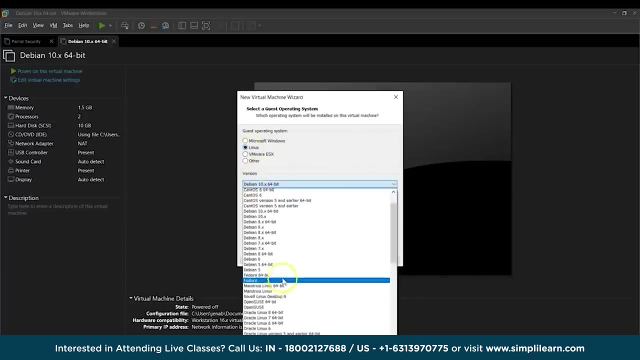 the ISO file here directly and VMware will install it for us. but right now, in the case of Kali Linux, the third option is always the safest. Kali Linux is a Linux distribution, so we can select Linux over here and the version as you can. see here have multiple versions, such as the multiple kernels. Every distribution has a parent distribution. For example, Kali Linux has Debian and there are other distributions which are based or forked from some parent distribution. Kali Linux is based off Debian, so we can go. 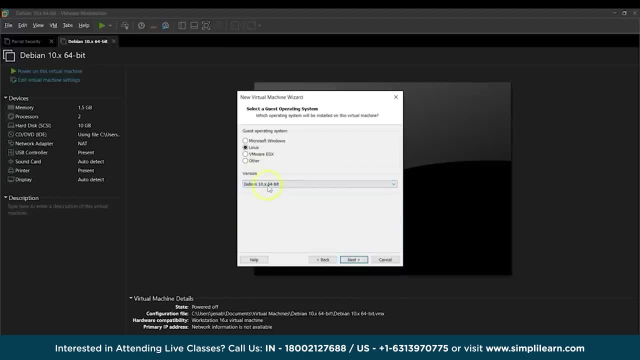 with the highest version of Debian, which is the Debian 10.x 64 bit. Go on. next, We can write any such name. We can write Kali Linux, so that it will be easier to recognize the virtual machine among this list of virtual machine instances. 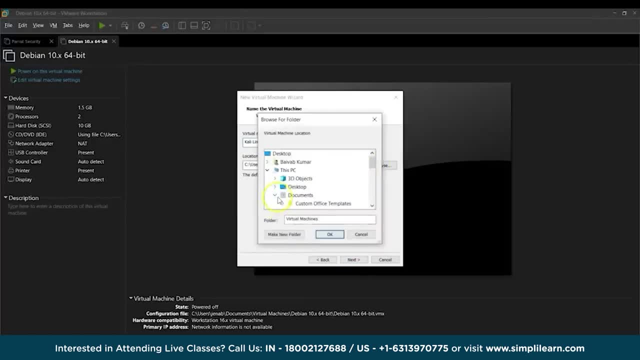 The location can be any location you decide to put. By default it should be the documents folder. but anywhere you put, it will hold up all the information of the operating system, All the files you download, all the configurations you store. everything will be stored in this particular location. 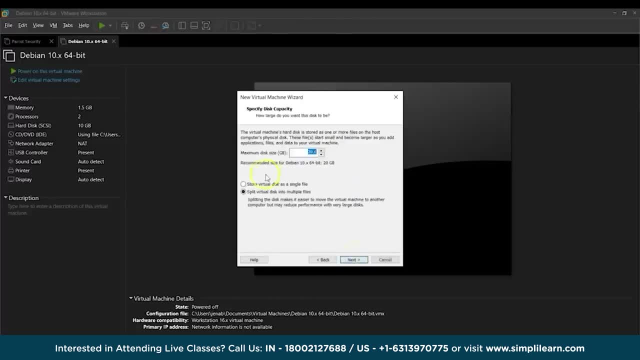 that you provide. When we go next, we are asked about the disk capacity. This disk capacity will be all the storage that will be provided to your virtual machine of Kali Linux. Think of your Windows device If you have a one terabyte. 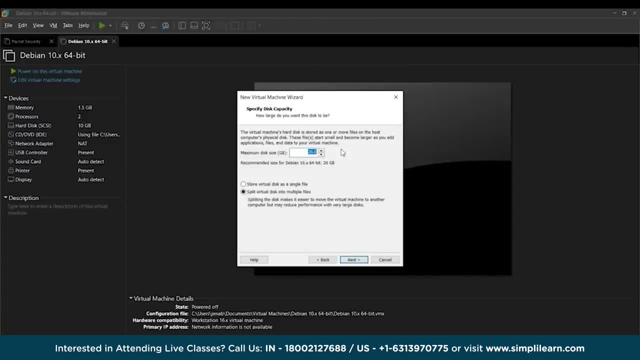 of hard drive. you have the entirety of the hard disk to store data on How much data you give here. you can only store up to that amount of data, Not to mention some amount of capacity will be taken up by the operating system itself to store its programs. 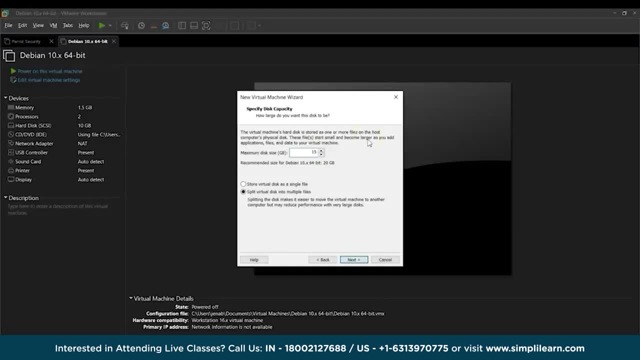 and applications. For now we can give around, let's say, 15 GB of information. or if a recommended size for Debian is 20, you can just go ahead at 20.. It depends all on the user case If you are going to. 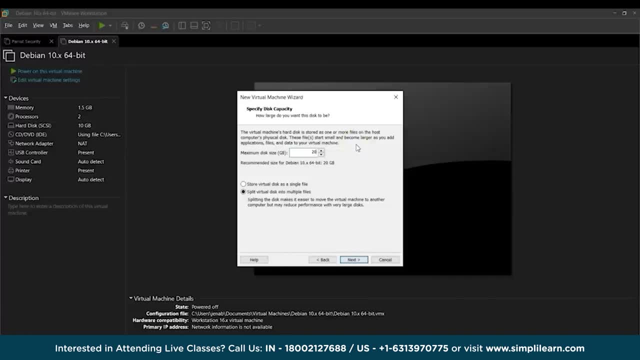 use it extensively. you can even go as high as 50 or 60 GB if you have plans to download many more applications and perform multiple different tests. Another option we get over here is storing virtual disk as a single file or storing them into multiple. 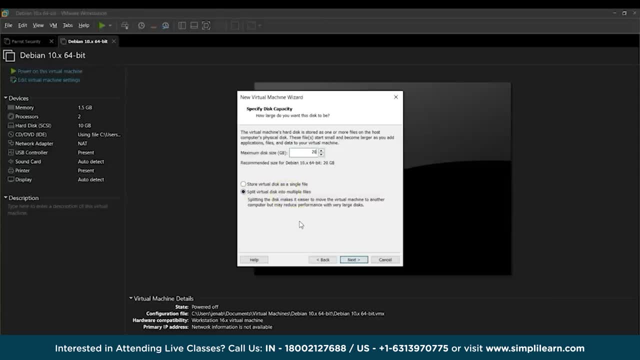 files. As you already know, this virtual machine runs entirely on VMware. Sometimes, when transferring these virtual machine instances, let's say from a personal computer to a work computer, you're going to need to copy up the entire folder that we had mentioned before over. 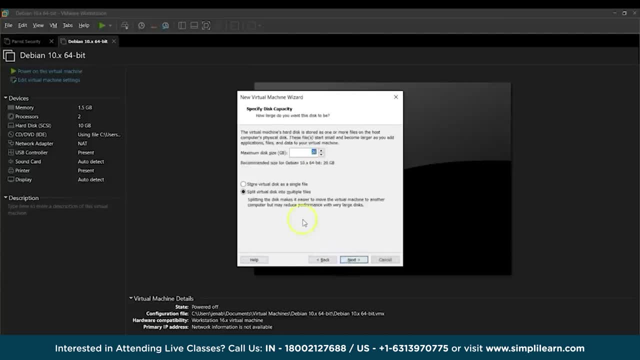 here. Instead, all virtual machines have a portability feature. Now, this portability feature is possible for all scenarios, except it is much easier if they split the virtual disk into multiple files. Now, even if this makes porting virtual machines easier from either system to system, 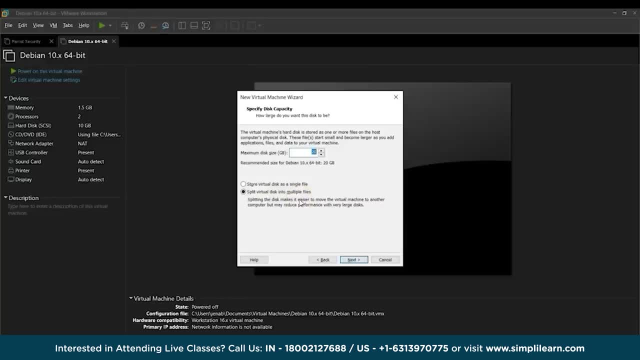 or software to software. let's say, if you want to switch from VMware to VirtualBox or vice versa, the performance takes a small hit, It's not huge, but it's recommended to go with storing the virtual disk as a single file if you have no purposes of. 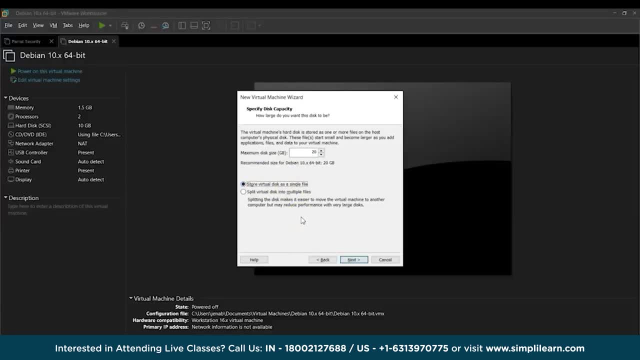 ever moving the virtual machine. Even if you do, it's not a complete stop that it cannot be ported. it's just easier when using multiple files. But in order to get the best performance out of the virtual machine, we can store it. 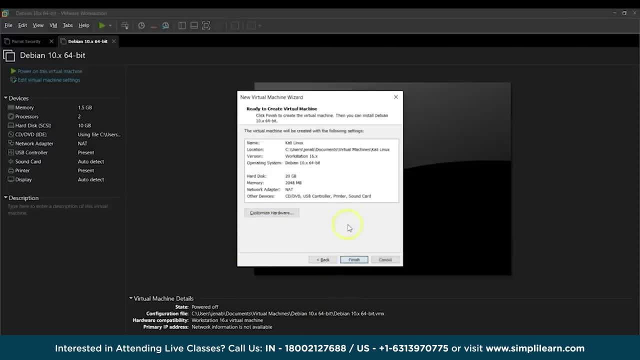 as a single file over here. This is a summary of all the changes that we made and all the configurations that have been settled until now. Now, at this point of time, we have not provided the iso file yet, which is the installation file for the. 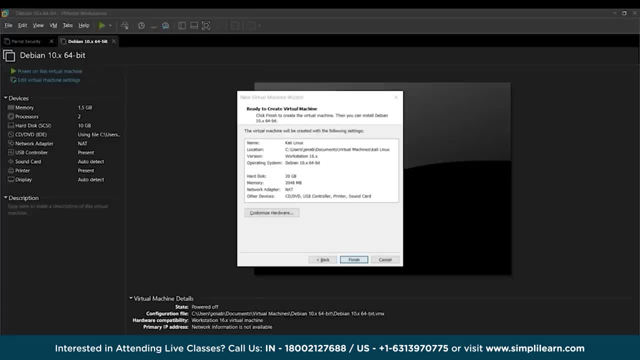 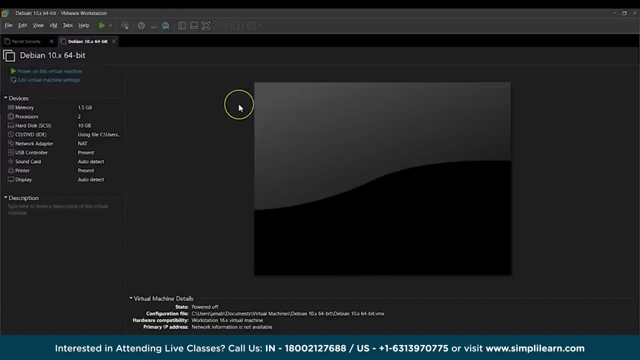 Kali Linux that we downloaded from this website. As of right now, we have only configured the settings of the virtual machine, So we can press on finish And we have Kali Linux in the list. Now, to make the changes further, we press on edit. 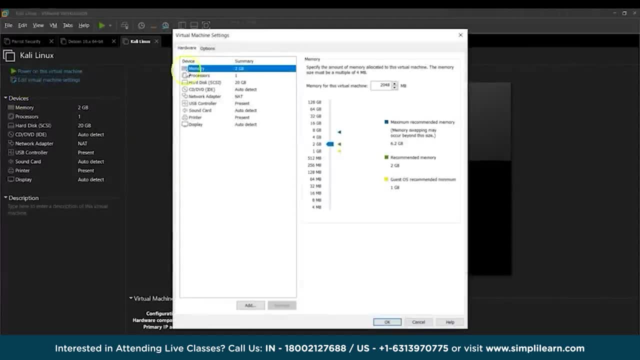 virtual machine settings. The memory is supposed to give the RAM of the virtual machine. The devices with RAM of 8GB or below that. giving high amount of RAM will cause performance issues and the host system If the memory has some amount of free storage. 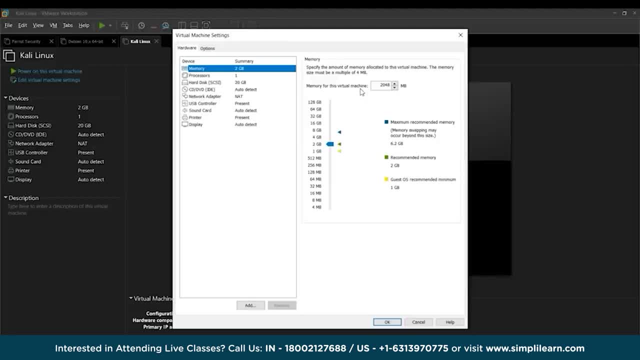 left, let's say on idle storage. my Windows machine takes about 2GB, So I have 6GB of memory to provide, Although if you provide all of the 6GB, it will be much more difficult for the host system to 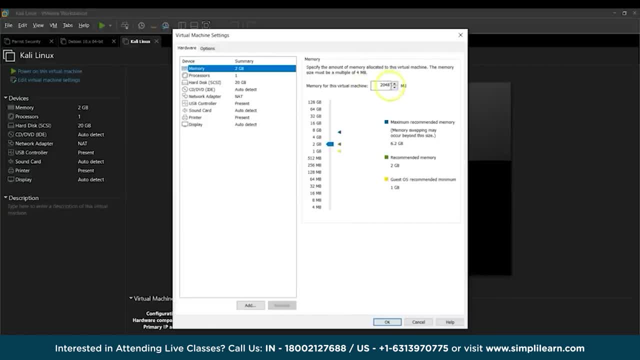 run everything properly. So for this instance we can keep it as 2GB of memory for the virtual machine instance. Similarly, we can use the number of processors and we can customize it according to our liking, Let's say if we want to use one processor. 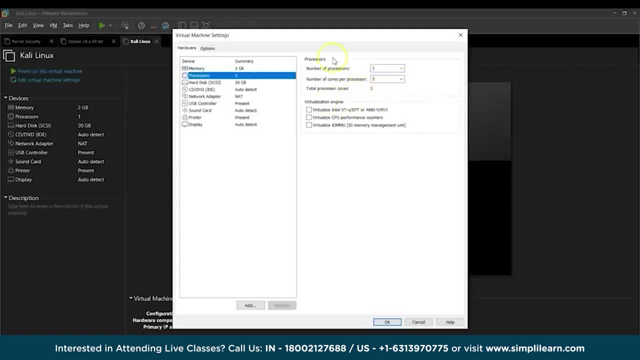 but we want to use two different cores. we can select them as well. Hard disk is pre-set up as the SCSI hard disk and it does not need to be changed for the installation of this operating system at all. CD, ID, DVD: This is where. 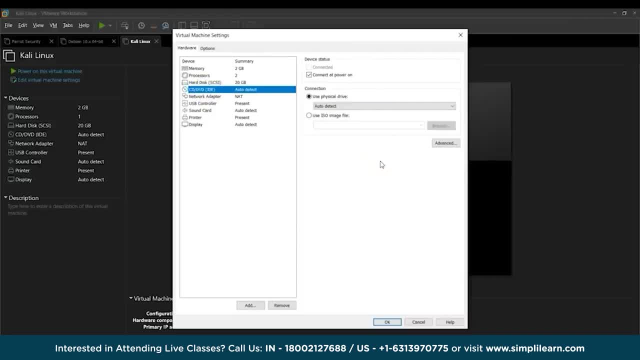 the installation file comes. You can think of the ISO file that we downloaded as a pen drive or a USB thumb drive, which is necessary to install an operating system. To provide this, we're going to select use ISO image file. We're going to click on browse. 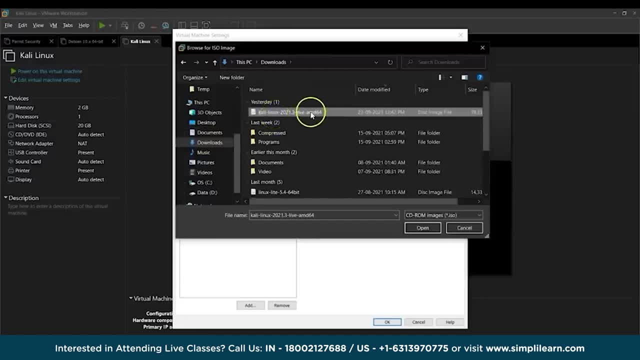 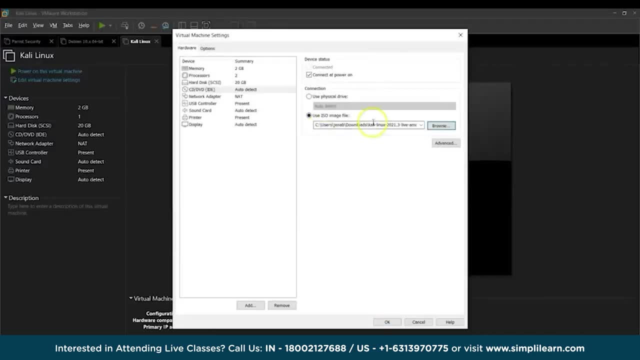 Go to downloads and select the ISO file over here. Select open And we can see it is already loaded up. Next, in the network adapter it is recommended to use NAT. This helps the virtual machine to draw the internet from the host machine settings, If your. 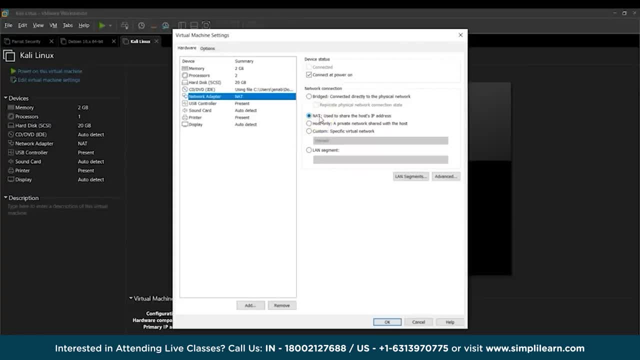 host machine is connected to the internet, then the virtual machine is connected as well. There are some other options, such as host only or custom segments or LAN segments, but those are not necessary for installation. Rest of them are pretty standard, which do not need any extra configuration and can be. 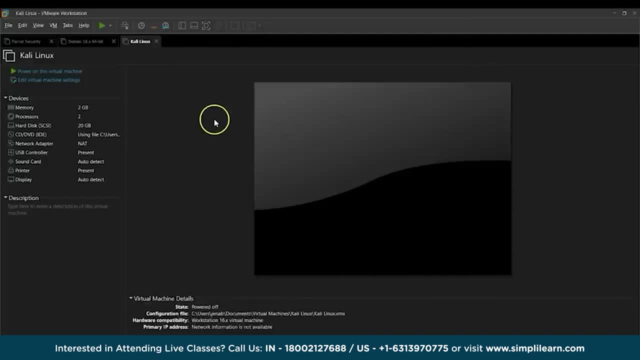 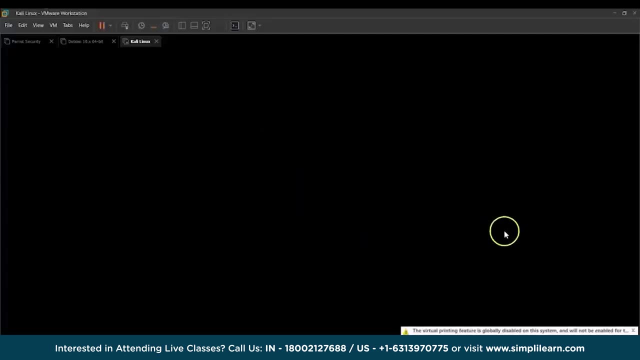 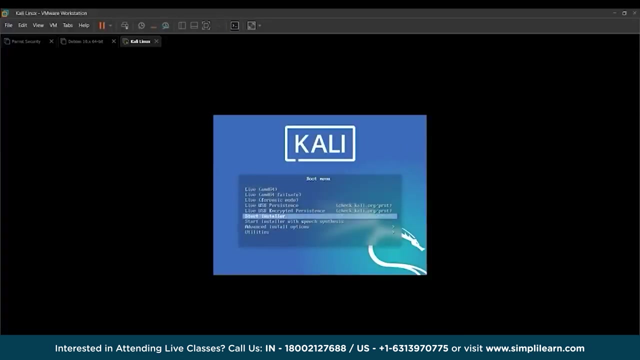 left as it is, Press ok And now we can power on this virtual machine. In this screen we can choose how we want to proceed with the installation. We have a start installer option over here, So we're going to press enter on that. 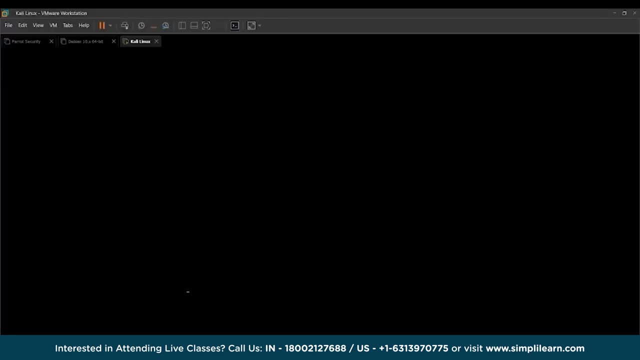 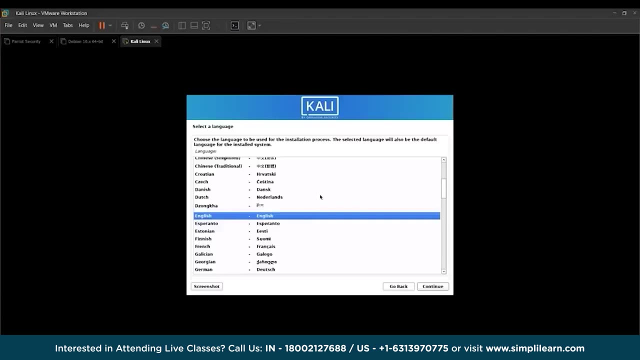 We're going to wait for the things to load from the ISO file. The first step in the installation is choosing the language of the operating system. For this, we can go with English as standard. This is the location. This will be used for setting up the time and some of the 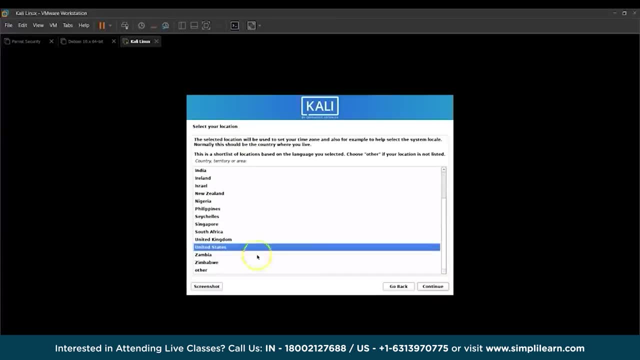 internal settings which depend entirely on the location of the user. So for this we're going to go with India. Configuring the keyboard: it's always recommended to go with the American English first. Many people make a mistake of going with the Indian keyboard. 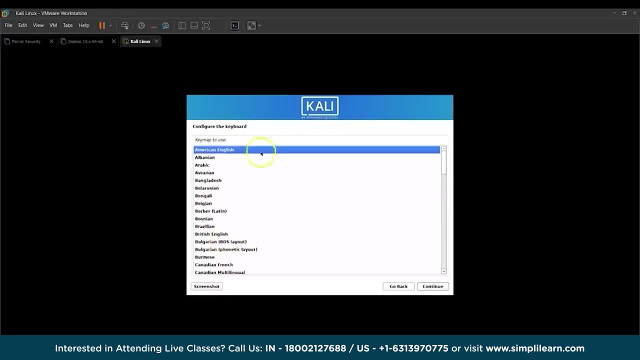 if it is possible and it provides a lot of issues later on. So it's always preferred to go with the American English, and if later we see some necessity of another keyboard dialect that is required, we can install it later, But for now we should always stick with. 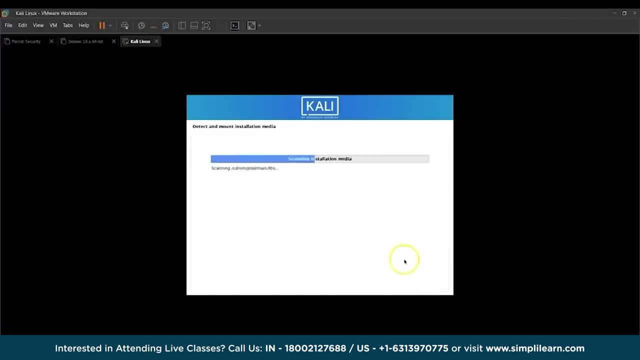 American English as a basic. At this point it's going to load the installation components from the iso file. It is a big file of 3.6 GB, so it has a lot of components that need to be put into the virtual machine. 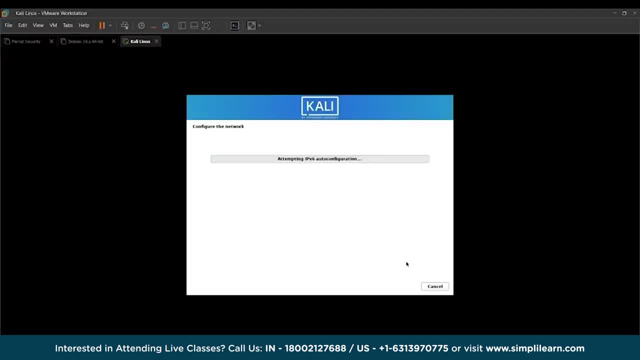 which can also be used to detect hardware. Once the hardware and the network configuration is done by the iso file, we want to write a host name for the system. This host name can be anything which is used to recognize this device on a local. 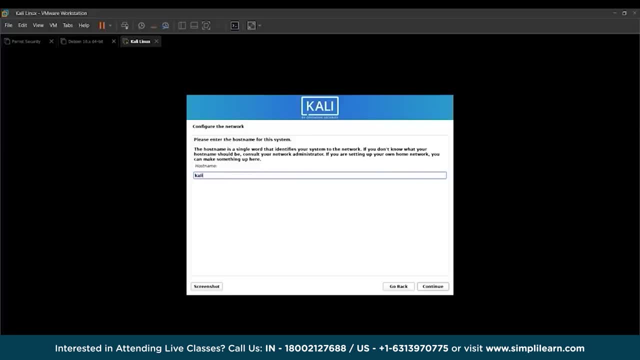 network or a LAN cable. Let's say, if we use the name Kali Domain name, we can skip it for now It's not necessary as such for the installation. This is the full name for the user. Let's say we can. 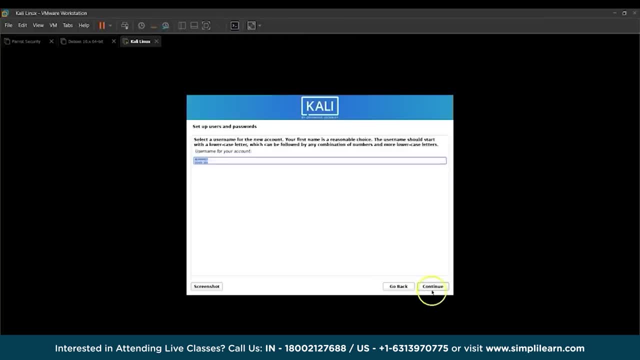 provide the name as simply learn as a full name. Next, we're going to set up a username. This username is going to be necessary to identify the user from its root accounts and the subsequent below accounts. For now, we can give it as something. 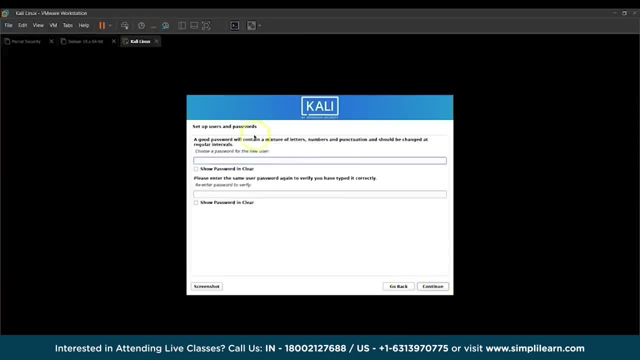 as simply123.. Now we have to choose a password for the user. Now, remember, since this is the first user that is being added onto this newly installed operating system, it needs to be a password for the administrator. We can use whichever password we like over here. 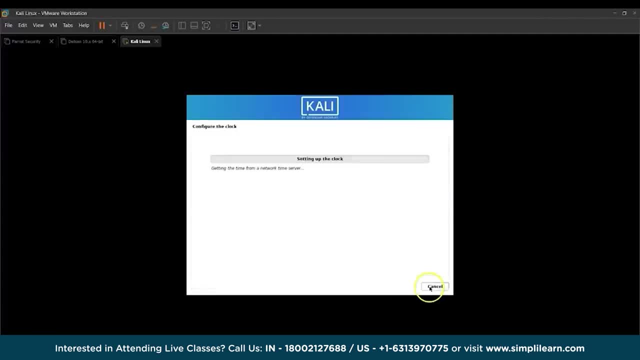 and use the same password below and press on continue. At this point it's going to detect on the components on which the operating system can be installed. Like here, there are multiple options, like the use entire disk, use entire disk and setup LVM. 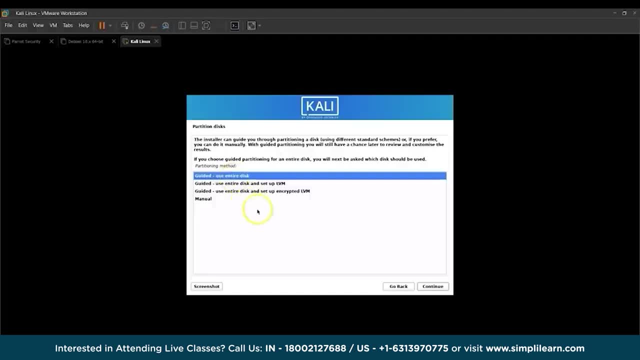 use entire disk and setup encrypted LVM. For newcomers, it is recommended to just use the first one, since LVM encryption is something that you can learn afterwards, when you're much more hands-on with the Linux operating system. For now, we're going to use the 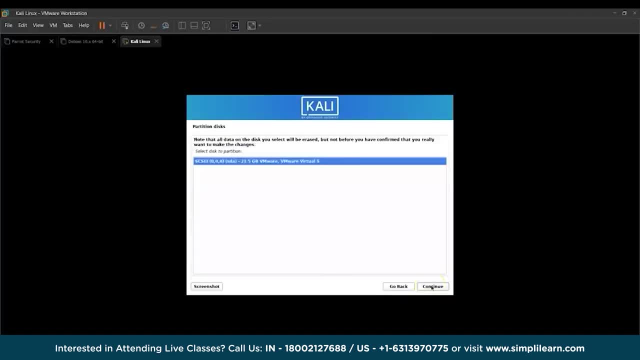 use entire disk guided installation and press on continue. When we set up the virtual machine on VMware, we had set up a disk capacity that we gave a purpose: 20 GB. That is the hard disk which is being discovered here, Even though it is a virtual disk. 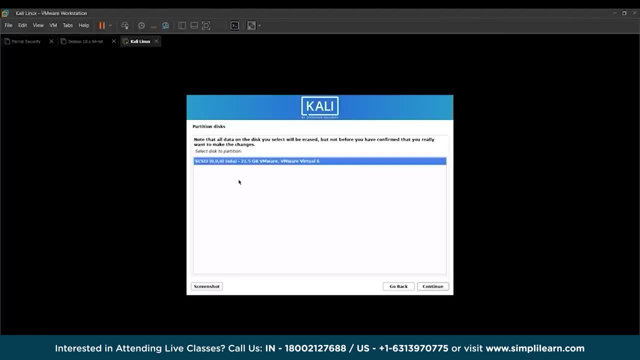 on VMware. it acts as a normal hard disk on which an operating system can be installed, So we select this one and press on continue. Here there is a multiple partition system. All the operating systems that are installed have different components. One is used for the 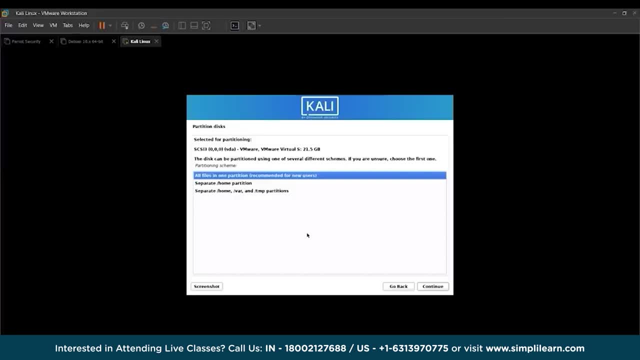 keeping of the applications, one for the files, other for the RAM management and other things. For newcomers, it is always recommended to keep it in one partition, and we're going to select that and press on continue. This is just an overview of the partition it's going to make. 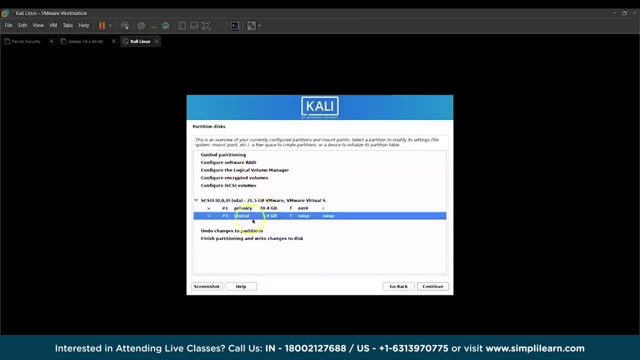 As you can see, it has a primary partition of 20.4 GB and a logical partition of 1 GB used for swap memory. Now, these kind of naming can be confusing for people who are not well versed with Linux operating systems or in general. 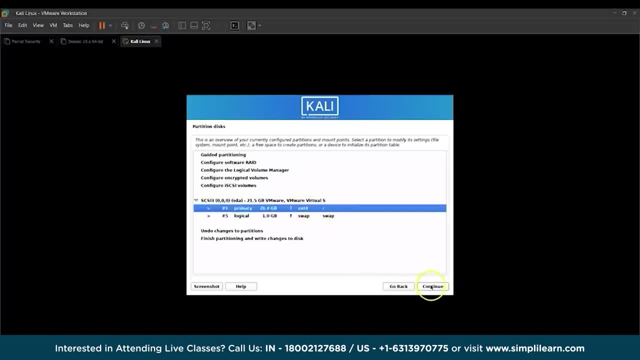 virtualization, But for now you can go ahead and press on continue, as this will be fine. We can press on finish partitioning and write changes to disk and continue. It's just a confirmation page. As you can see, SCSI3 is our. 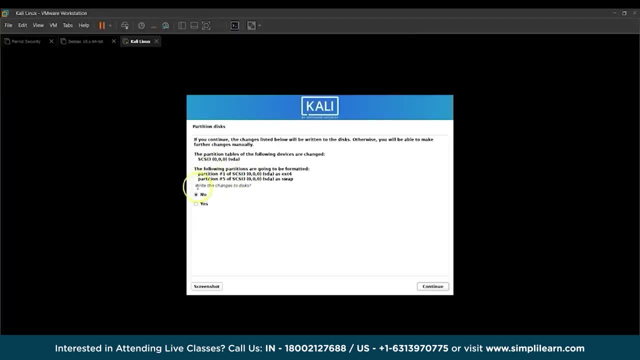 virtual hard disk of 20 GB disk capacity. Write the changes to the disk. We press yes and click on continue. At this point the installation has started. This installation will take a while, depending on the amount of RAM provided the processors provided. 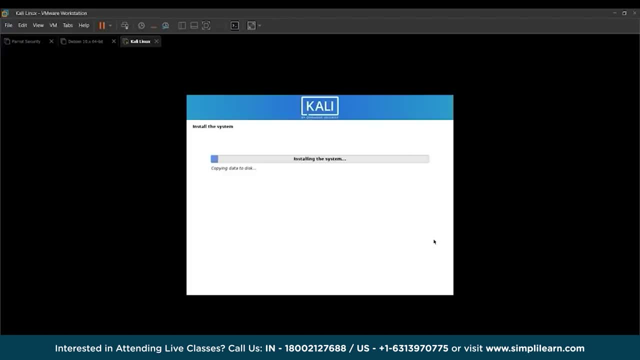 and how quickly the performance of the system is being hampered by the host machine. On quicker systems, this will be rather quick, while on the smaller ones, this will take a while, Since this is going to take some time to install as it is being run on a virtual machine. 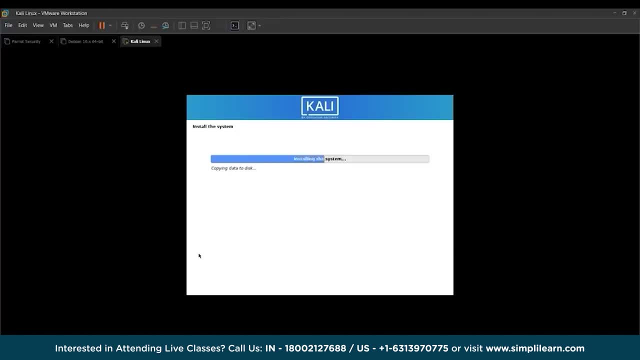 with only 2 GB of RAM. we are going to speed up this part of the video so we don't have to waste any more time just watching the progress bar. Now that our core installation is completed, it's asking us to configure a package manager. 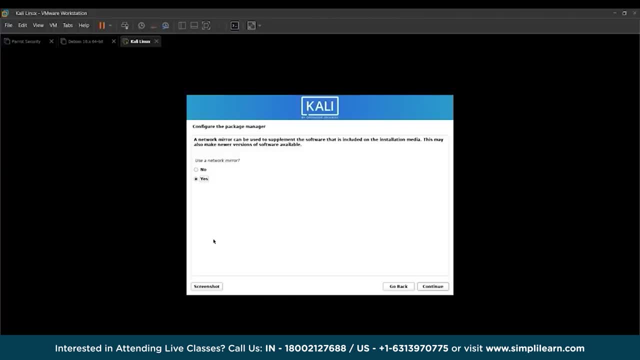 The work of a package manager on Linux operating system is similar to the Google Play Store on Android mobile devices and on the App Store for the Apple devices. It's an interface to install external applications which are not installed by default, Let's say for Google Chrome or any other. 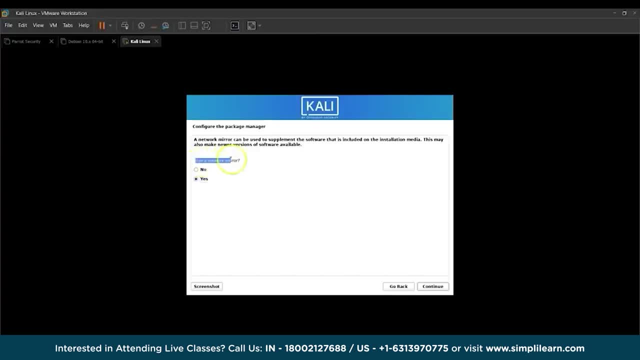 browser which can be used to browse the internet At this point of time. it's asking us to select a network mirror. We are going to select as yes and move forward with this. Next, it's going to ask us for a HTTP proxy. 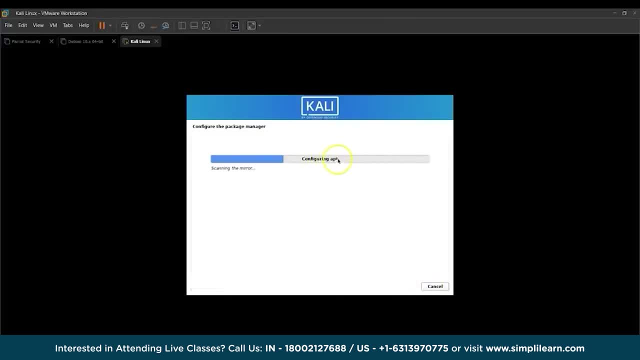 which we can leave it as blank and press it as continue forward. At this point of time it's looking for updates to the Kali Linux installation. This will fetch the new builds from the Kali server, so the installation is always updated to the latest. 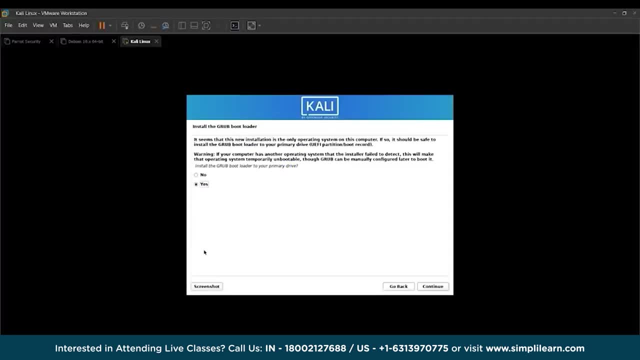 version. Now that the package manager is configured, we have the grub bootloader. The grub is used for selecting the operating system while booting up. Its core functionality is to allow the operating system to be loaded correctly without any faults At this point of time. if it asks, install the 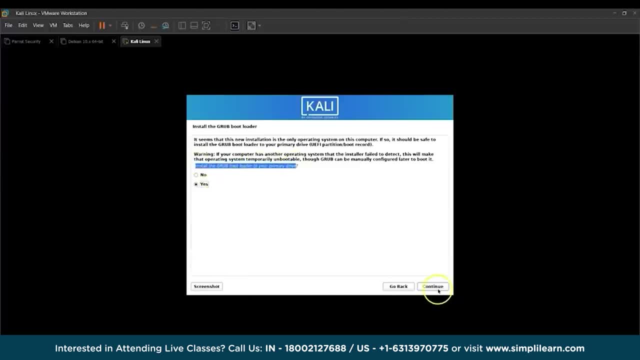 grub bootloader to your primary dive. we can select it as yes and press continue. Remember the installation was conducted on Dev SDA. We are going to select installation of the grub bootloader on the same hard disk that we have configured. Press this one and press continue. 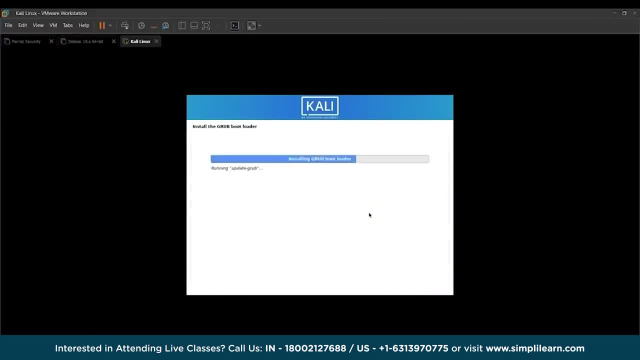 So now the grub bootloader is being installed. The grub is highly essential because it shows the motherboard where to start the operating system from. Even if the operating system is installed correctly and all the files are in correct order, the absence of a bootloader will not. 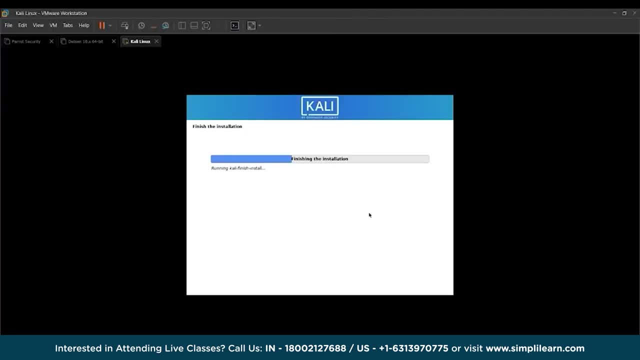 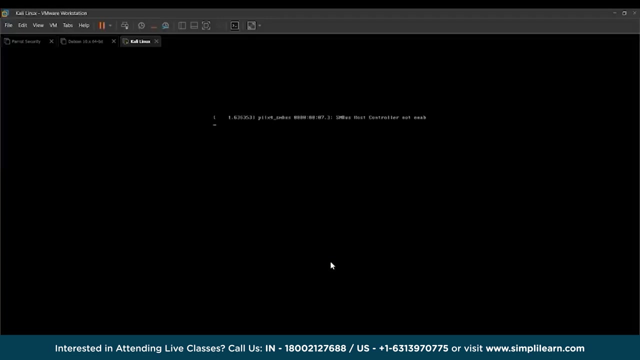 be able to launch the OS properly. As you can see, the installation is finally complete, So now we can press on, continue, and it's going to finalize the changes. Now you can see Kali Linux being booted up straight away. It doesn't check for the ISO. 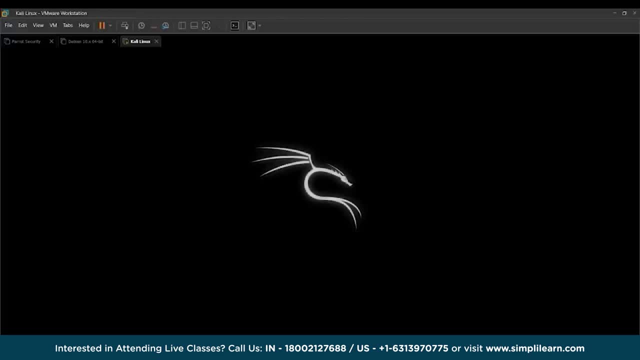 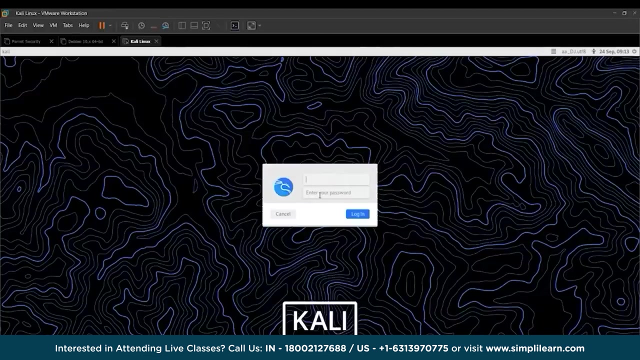 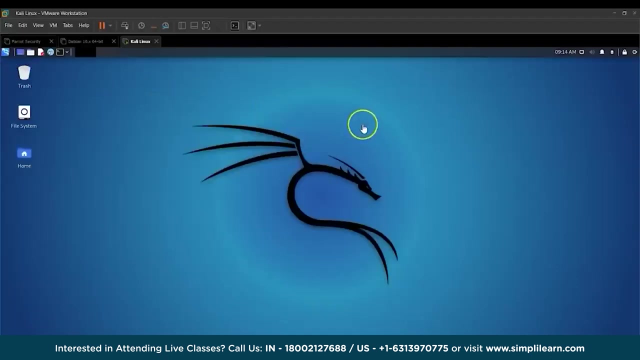 file anymore, since the operating system is now installed onto the virtual hard disk storage that we had configured before. Here we are going to enter our username and password that we had set up before, And we have the Kali Linux system booted up. And this is your home page. 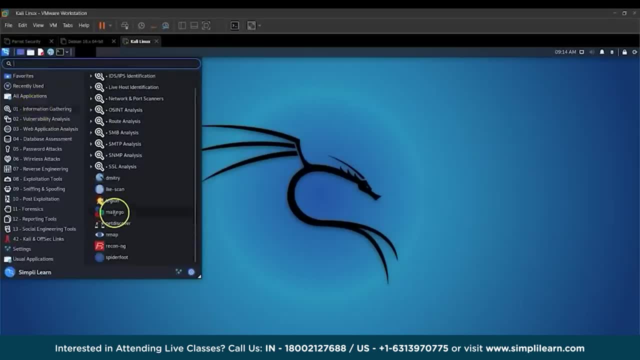 We can see the installed applications over here which are being used for penetration testing by multiple security analysts worldwide. All of these come pre-installed with Kali Linux, and others can be installed using the APT package manager that we had configured. We can see our full name over here. 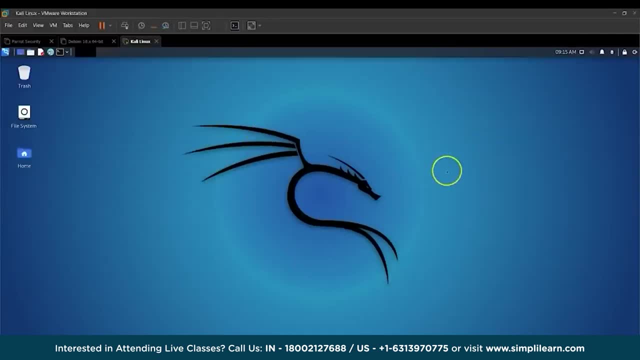 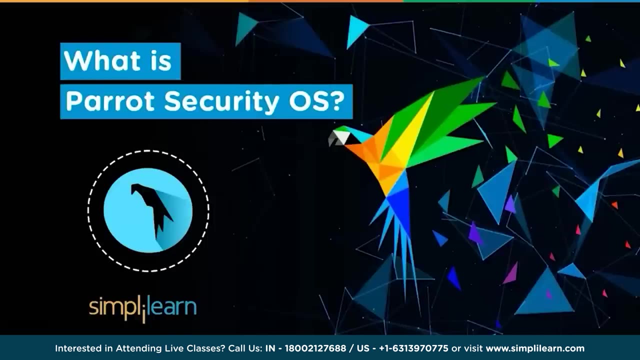 And with this, our installation of the Kali Linux is complete. Hey everyone, It's no secret that the majority of our internet usage is at the risk of getting hacked, Be it via unsafe messaging applications or misconfigured operating systems. To counteract this void of digital security, 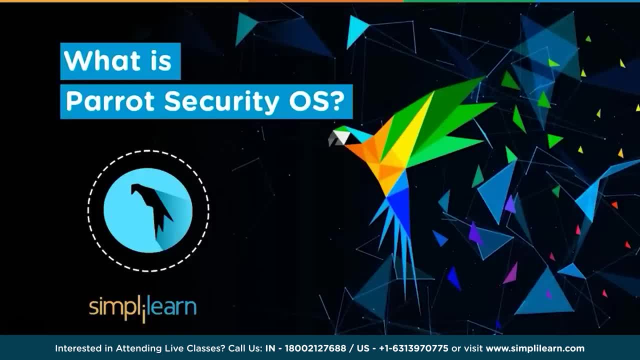 penetration testing has become the norm when it comes to vulnerability assessment. Parag Security OS is an operating system that has become a well-known weapon in this fight against hackers. While enough distribution more cater towards penetration testers specifically, Parag Security has layers of features. 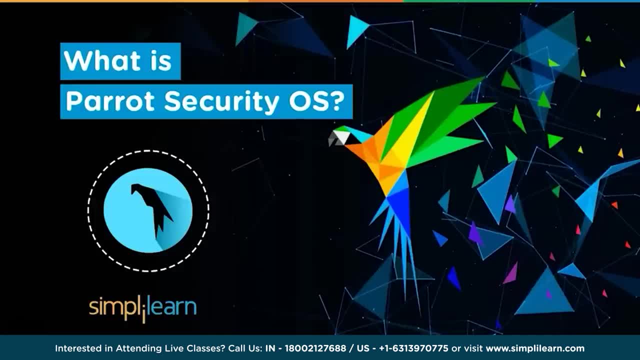 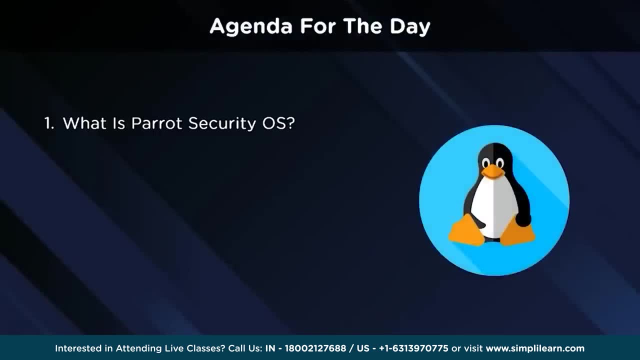 that we will be covering in today's lesson. Let's take a look at the top topics for this video. We start by learning about what Parag Security is and why it should be considered as a viable alternative, next to Kali Linux, for penetration testers. 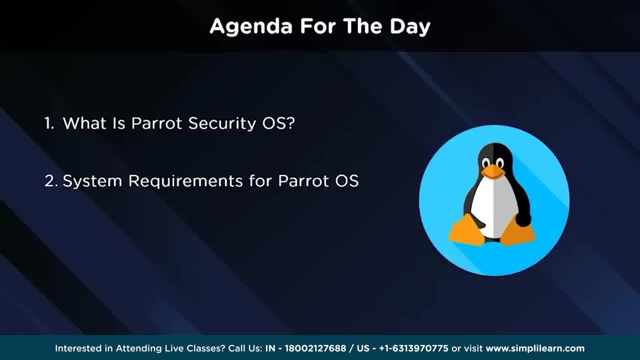 Next, we take a look at the minimum system requirements necessary to obtain optimum performance from an installation of Parag Security. Moving on, we learn about some unique features that make Parag stand out among the multiple ethical hacking operating systems available on the market. 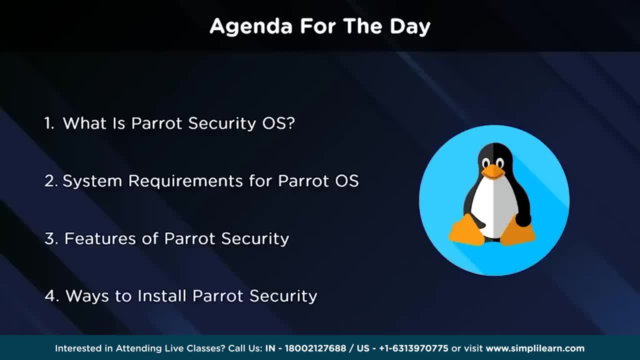 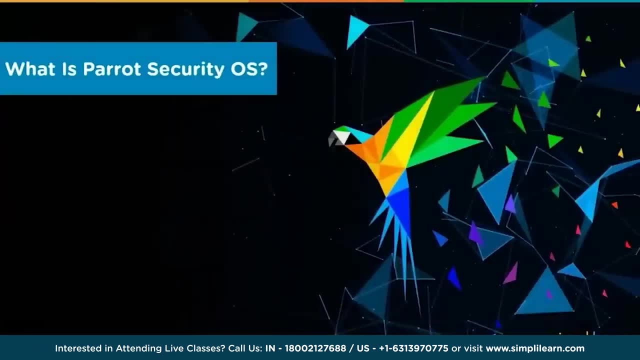 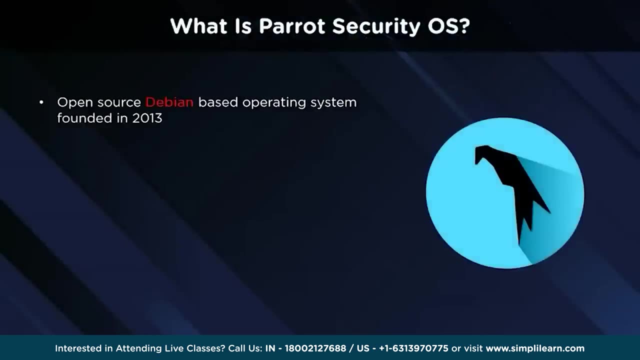 And finally, we look at the multiple ways that Parag Security OS can be installed, be it on a single system or for portable media. So let's start out by learning what Parag Security is. Parag Security is a Debian-based Linux distribution. 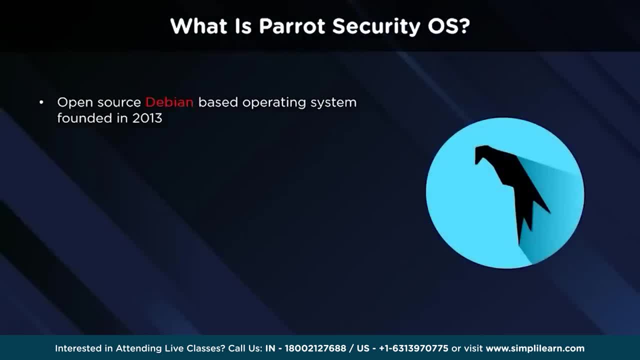 with an emphasis on security, privacy and development. It is built on Debian's testing branch and uses a custom hard Linux kernel, while being founded in 2013.. Parag Security contains several hundred tools targeted towards various information security tasks, such as penetration testing, security research. 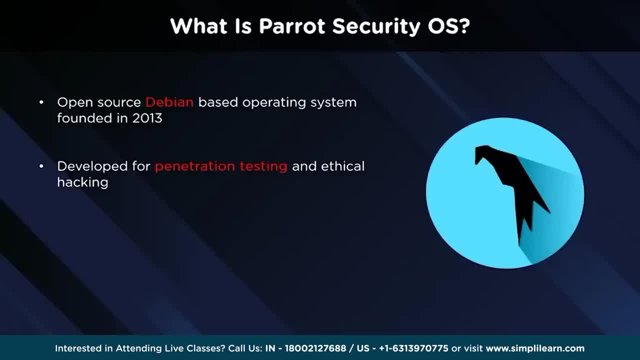 computer forensics and reverse engineering, It has become a multi-platform solution, accessible and freely available to information security professionals and hobbyists. It features a distinct forensics mode that does not mount any of the system hard disks or partitions and has no influence on the host system. 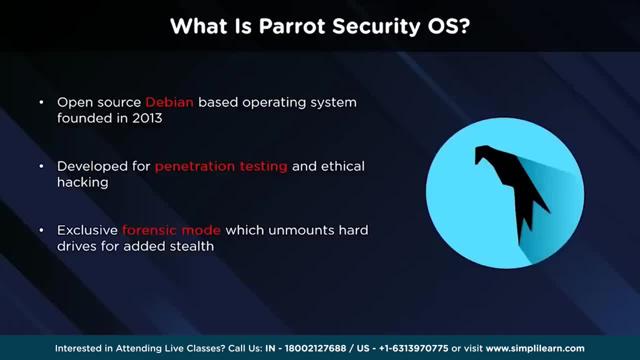 making it more stealthy than regular mode. This mode is used on the host system when there is a need for executing forensic procedures In software development. a rolling release is a paradigm in which software upgrades are rolled out constantly rather than in batches of versions. 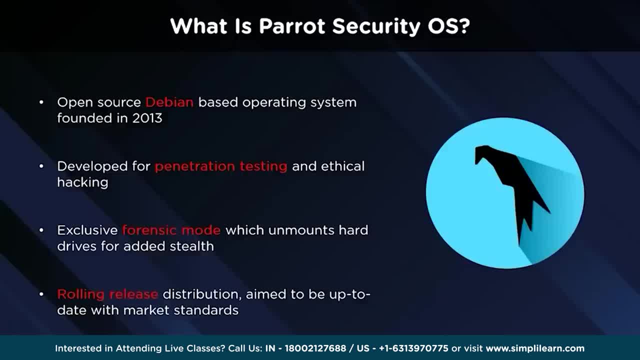 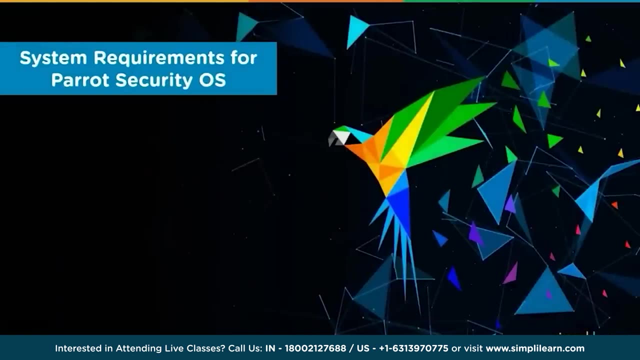 This ensures that the software is constantly up to date. A rolling release distribution such as Parag Security OS follows the same concept, providing the most recent Linux kernel and software versions as they become available on the market. The basic introduction to the operating system out of the way, Let us 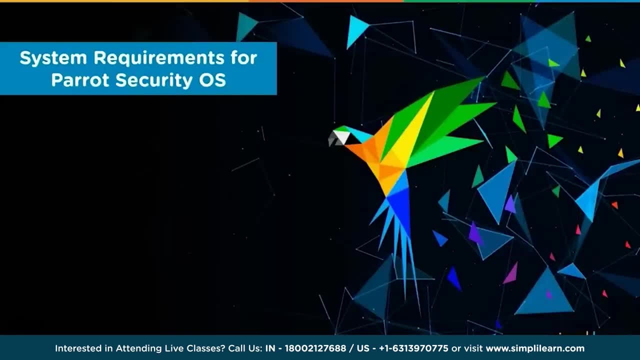 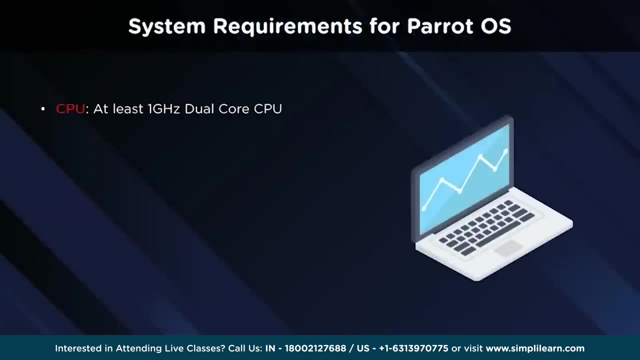 have a look at the bare minimum system requirements necessary to be able to run this operating system. First up, we got a CPU requirement which states that a 1 GHz dual-core CPU is the absolute minimum in order to use Barrett OS, While multiple-core systems 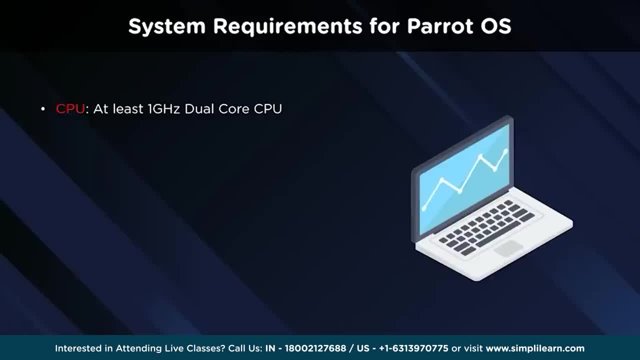 will provide more optimum performance. a small beginner has been included. A very distinct thing to be noted is that the operating system can be installed on all variants of chipsets, be it 32-bit, 64-bit and the newly popular ARM portfolio of devices. 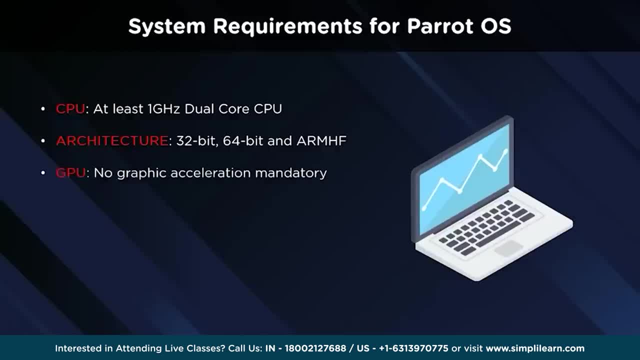 Unlike Kali Linux, which requires some amount of graphical acceleration needed to display the operating system correctly, Barrett OS has no such requirements and can be used with the leanest of machines. Taking into account the RAM issue, a minimum of 256MB to 512MB. 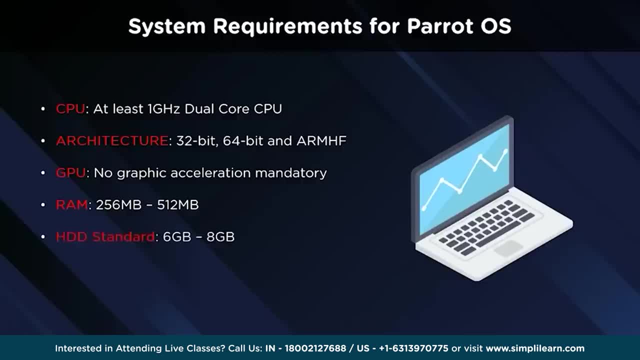 free RAM provides the optimum usage scenarios, Even when the OS is installed on a hard drive storage media. it should theoretically support around 8GB of information, which may extend up to 16GB depending on the tools being installed out of the box. 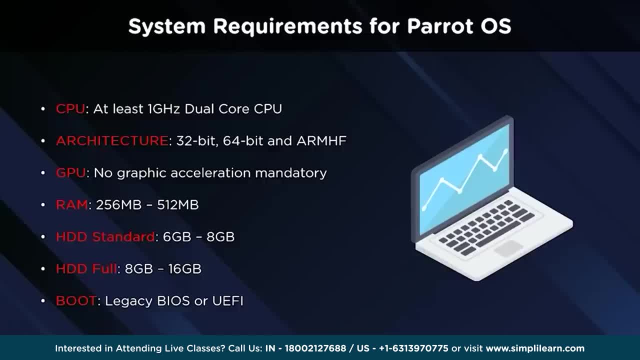 When it comes to booting options, we have the option of going with the legacy BIOS settings or with the more modern UEFI settings. These are just some of the requirements for the installation of Barrett Security OS. To understand this process more vividly and to learn. 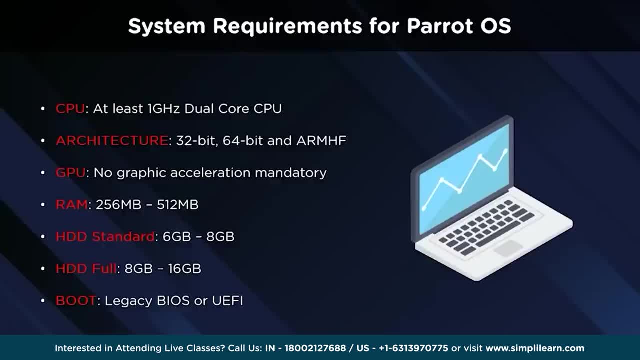 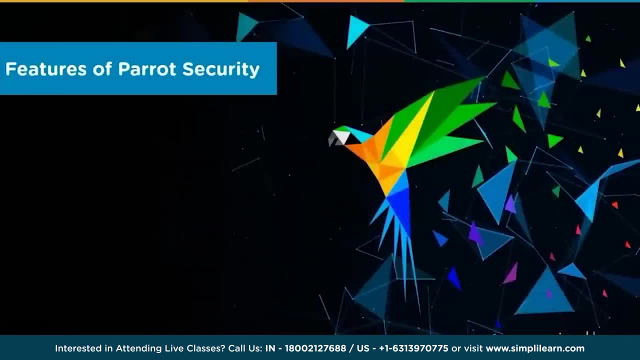 how visualization can help install an OS in our existing computer. please follow the link to a Barrett Security installation video, linked right above. Let's understand what some of the things that make Barrett Security unique among all the other penetration testing operating systems, Along with all the 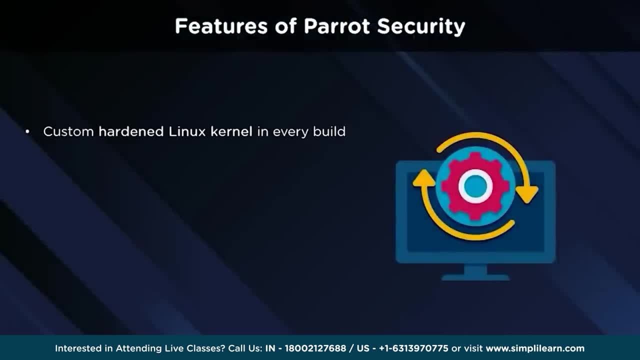 giant catalog of scripts. Barrett Security has its own custom hardened Linux kernel which has been modified explicitly to provide as much security and resistance to hackers as possible. as a first line of defense, The configurations in the operating system act as a second gateway, taking care of malicious requests. 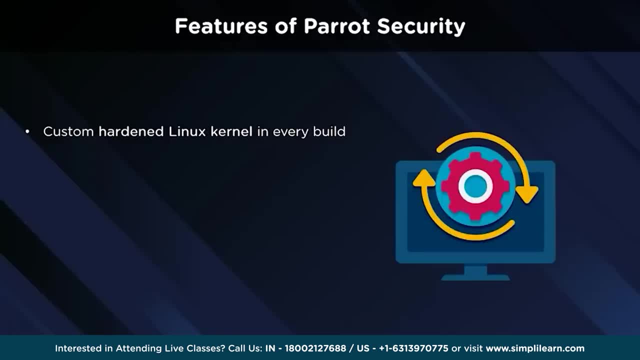 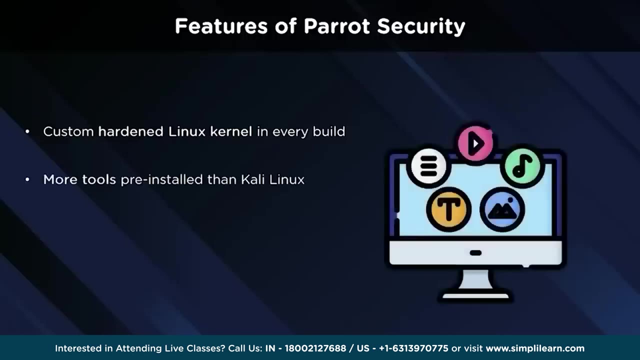 and dropping them off. This is particularly beneficial since, should there be a scenario where the latest Linux kernel is causing some particular issue, the Barrett OS development team will most likely iron it out first before passing it on as an update. If the custom hardened kernel 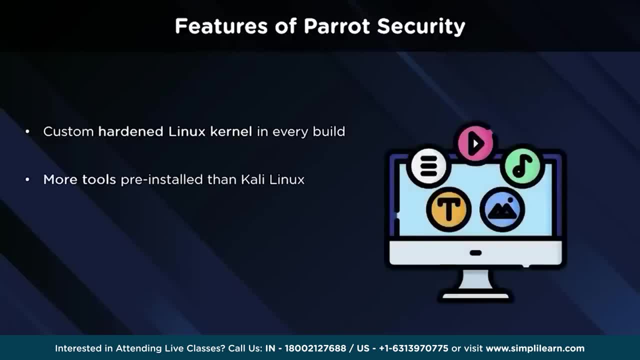 wasn't reasoning enough. Barrett Security developers managed to install more hacking tools and scripts to ensure a smooth transition for the Kali Linux users. All the tools you found in Kali are present in Barrett OS, and then a few extra ones for good measure. 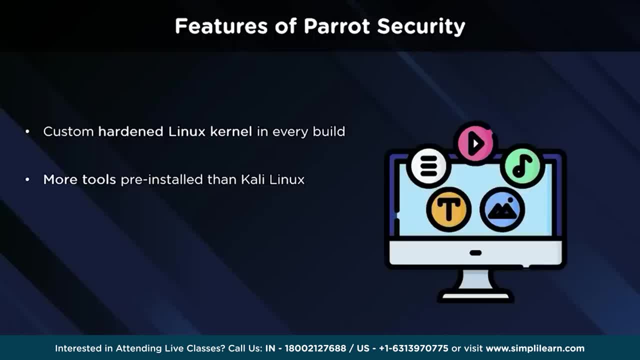 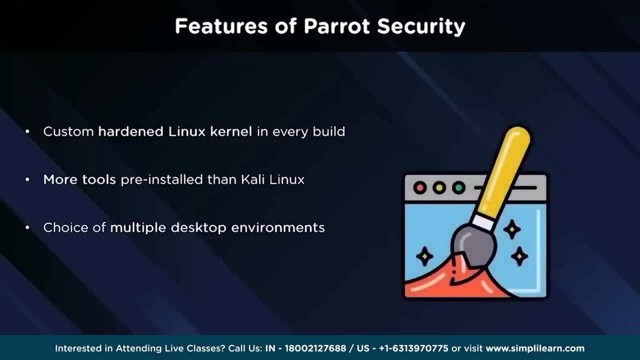 This has been achieved while keeping roughly the same size of the installation file between both operating systems. However, it's not all. productivity points for Barrett OS. They provide a choice between two different desktop environments: the Mate Desktop, which comes pre-installed by default, and KDE. 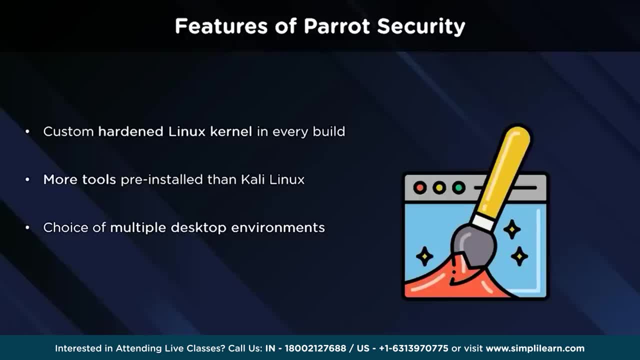 For those unfamiliar with Linux terminology, you can think of desktop environments as the main UI for a Linux system. Being highly modular in nature, one can use Kali, Linux or Barrett OS while adding another desktop environment which they find appealing, While Kali has only a single option. 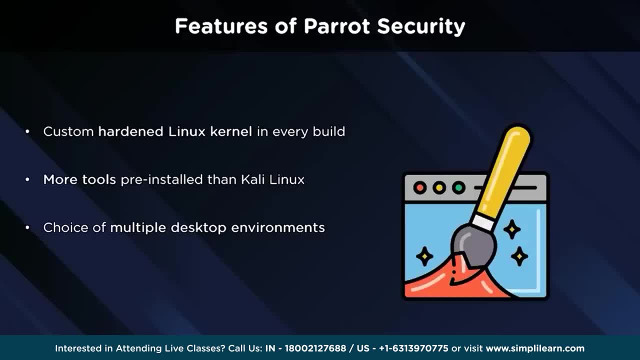 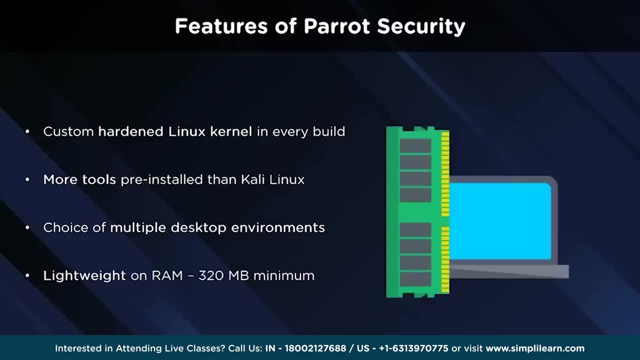 Barrett OS has managed to provide two optimized wheels, with Mate Desktop and KDE Desktop ready-made on their website. One of the primary advantages of Barrett OS over Kali is that it's relatively lightweight. This implies that it takes significantly less disk space and computing power to function properly with as 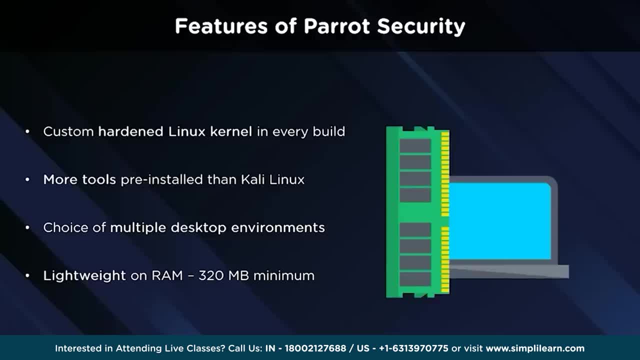 little as 320 MB of RAM required. In reality, Barrett OS is also designed to operate successfully off a USB stick, but Kali Linux does not work well from a USB stick and is generally installed in a virtual machine. Barrett OS can be seen as: 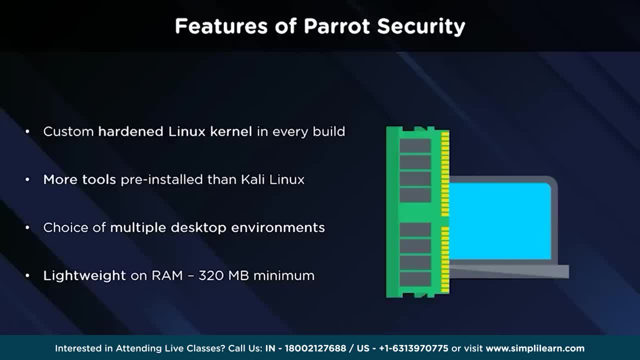 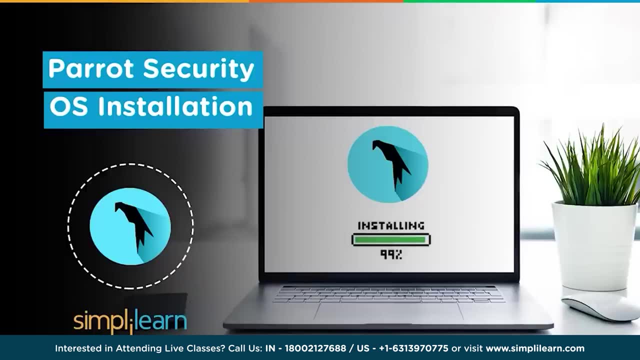 more of a niche distribution if you're searching for something lighter than Kali Linux. There are multiple ways to go about with this installation. Many people prefer to install it directly onto a hard disk, where the Barrett Security OS will override whichever data the hard disk already has. 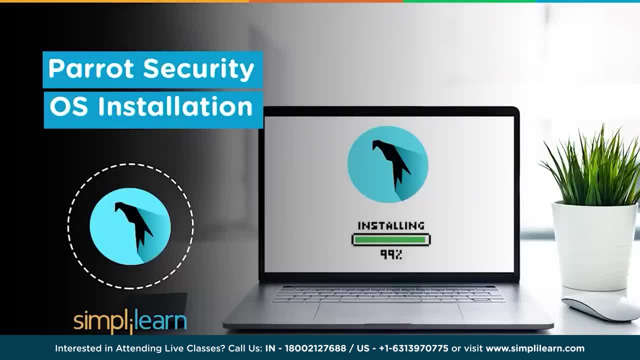 Now, this is beneficial if you want to preserve your data for the long term, but this might pose some trouble to people who do not have a spare hard disk or do not want to lose their current installation of Windows operating system. Another way to use Barrett Security is by using the live boot. 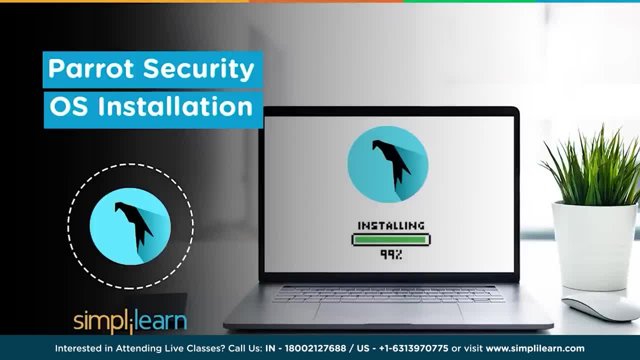 but whatever changes we make to the live boot operating system, those changes are removed the moment we restart or shut down the system. A very good common ground between both these installations is virtualization. Using virtualization software like VMware or VirtualBox, we can install Barrett Security. 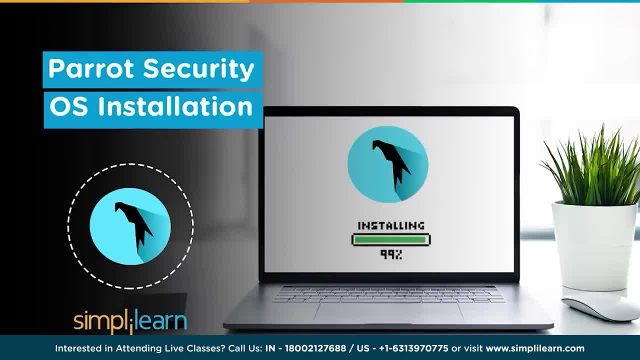 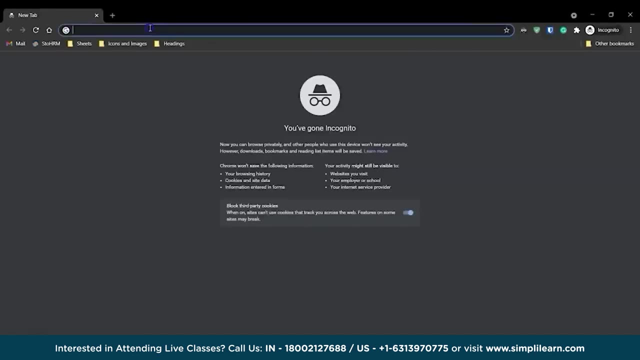 on our systems while simultaneously saving our data and having the convenience of a host machine such as a Windows operating system, in case things go wrong. To start the installation, we first need to get an ISO file for the Barrett Security operating system. This can be found on the current website. 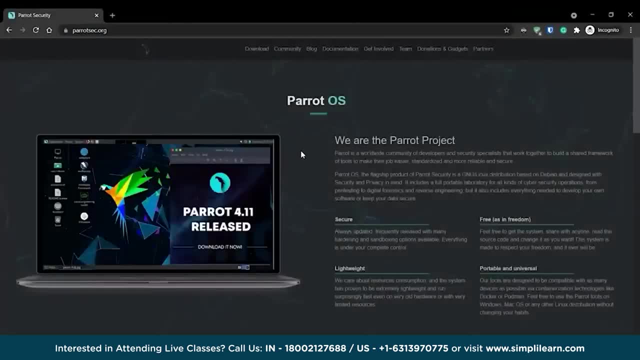 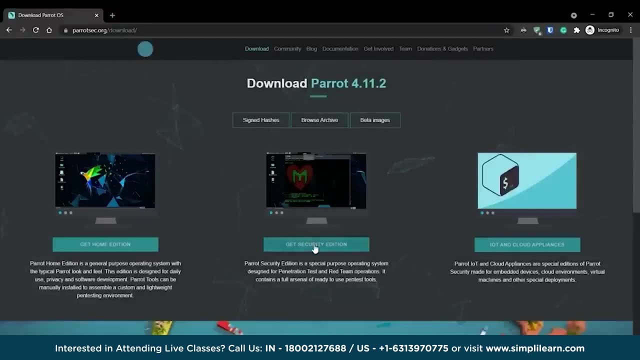 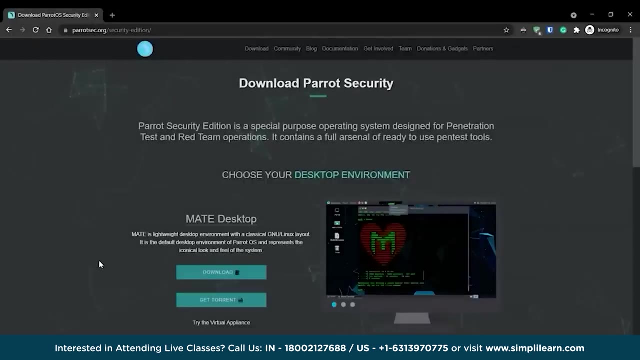 barrettsecorg. Once we enter the website, move into the download section and select the Get Security edition over here. Barrett Security OS has multiple desktop environments for you to choose from. These desktop environments serve as a different user interface for the user. 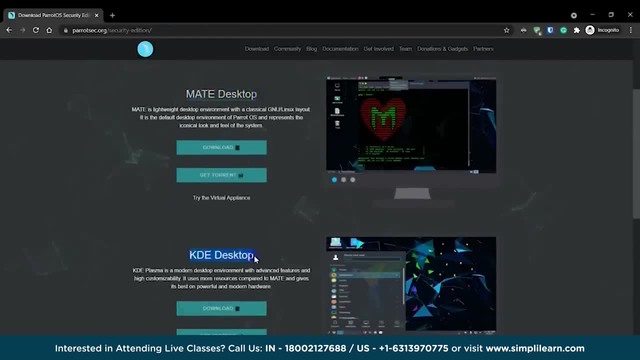 For example, right now we have the Mate desktop and the KDE desktop. As you can see from the screenshots, both of these look quite different while having a similar look and feel to them. For our example, let's go with the Mate desktop. 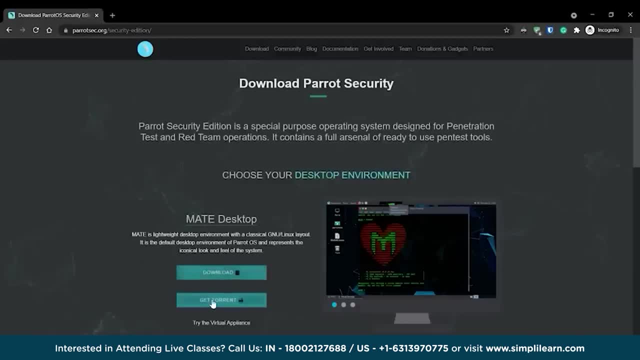 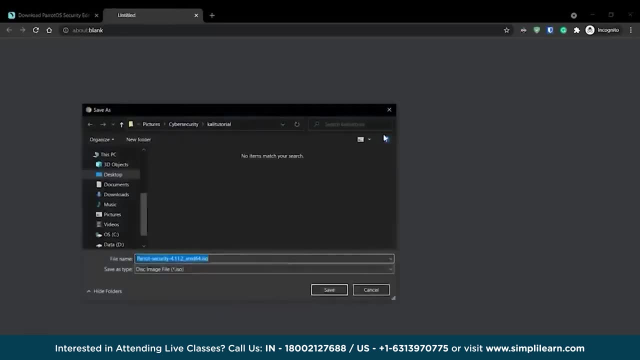 We have two options: either we can go with the direct download or we can get the torrent file, For this example, if we press on the download button and our download will start. I have already downloaded this file, but the ISO file provided over here will serve. 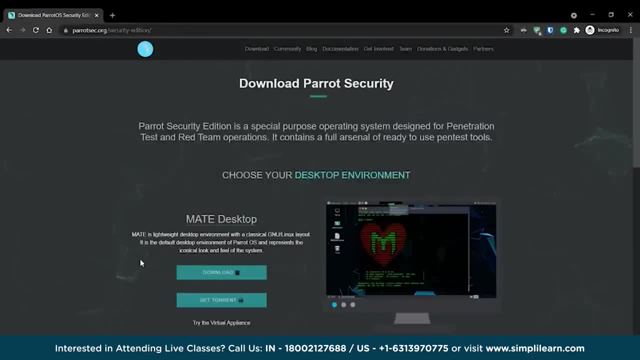 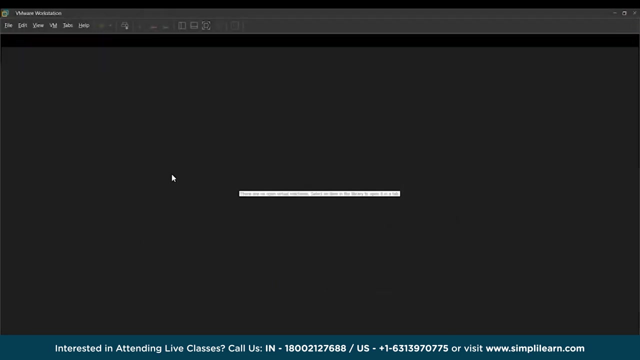 as an installation. It will have around 4.5 GB of space. It will be used to install this operating system in VMware. Once the file is downloaded, we can close this and open VMware Workstation. VMware can also be used as a player version or the. 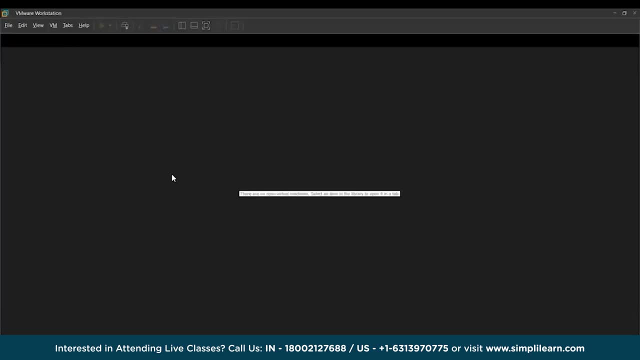 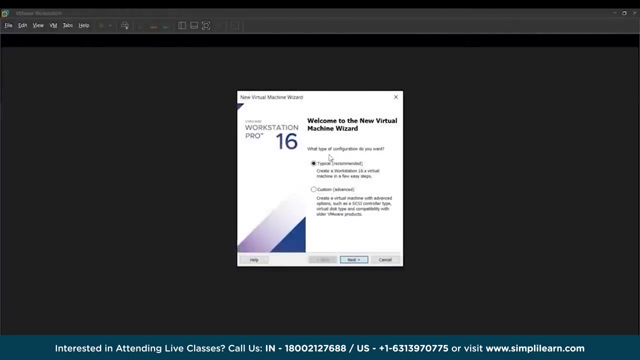 workstation version. If you have much more familiarity with using VirtualBox or virtualization application, we can use that as well. Once the VMware is open, we click on file and select a new virtual machine For the first time installation we are going to 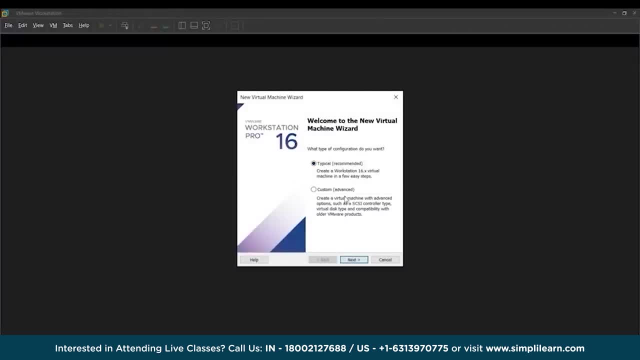 go with the typical and recommended installation procedure instead of an advanced one. If you have already installed multiple virtual machine OS's, go with the advanced option, which will give you much more control over the hardware customization. But for now we are going to stick with the typical option. 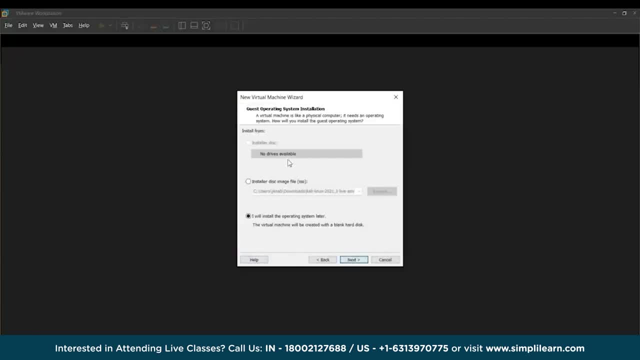 Moving on, it will ask us for a source to where to install the operating system from. Since we are going to use a live ISO first, we are going to select the third option, which will be: I will install the operating system later and press next. 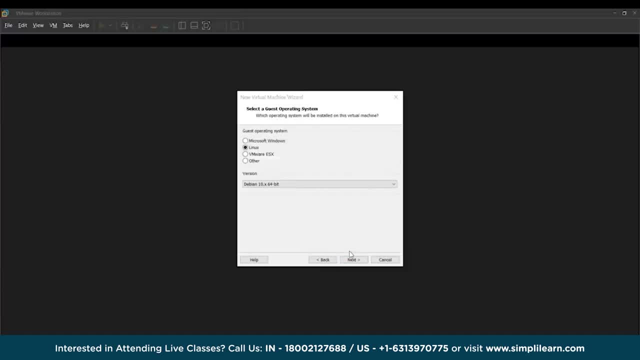 As we already know, Parag security is a Debian derivative. So when selecting the guest operating system type, we are going to go with Linux and in this selection, we are going to choose whichever the highest version of Debian is, along with the 64-bit OS. 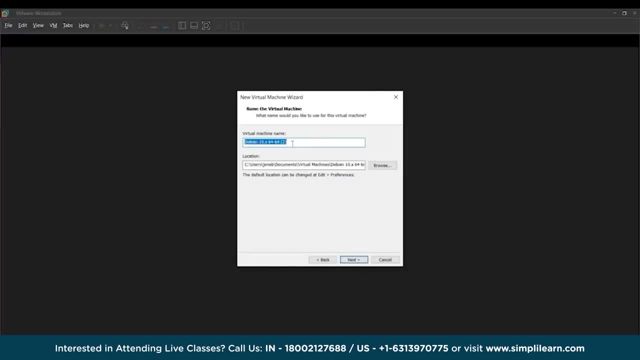 We are going to click on next. We are going to name our virtual machine, let's say Parag Security OS. We are going to select the location where we want to save the virtual machine. This will have all the hard disks of the operating system. 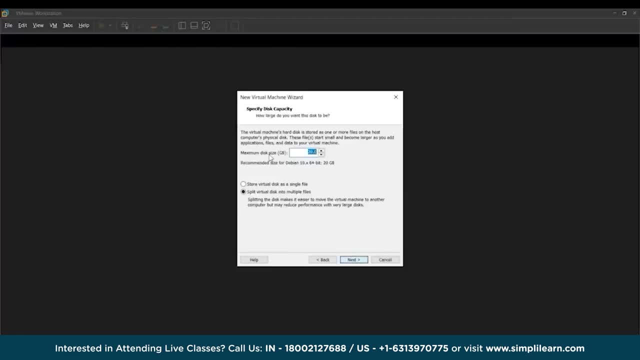 installation. We are going to click on next. For the disk size, we are going to specify how much of the current memory are we going to allocate. This is the hard disk memory of the operating system installation. Whatever changes we make in the operating system, whatever applications, 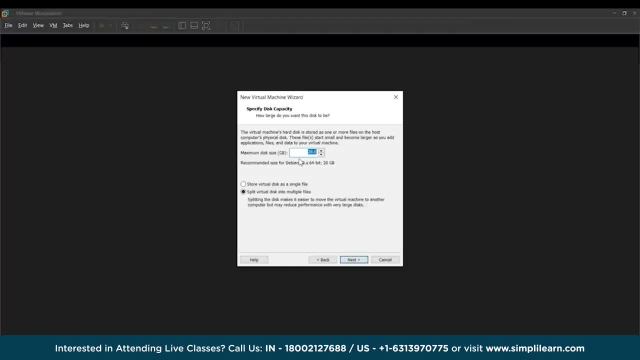 we install on the virtual instance will all be stored in this amount of memory. While it is recommended to go with at least 15 GB of storage, we can go as high as possible and we are going to select the recommended 20 GB as written. 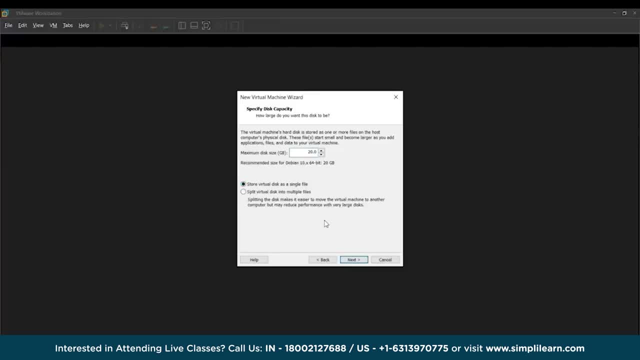 When given the choice of storing the virtual disk as a single or multiple files, many people want to keep their virtual instance in a way so that it helps them stay portable. People change systems and sometimes they want to swap their instances between the work and their personal. 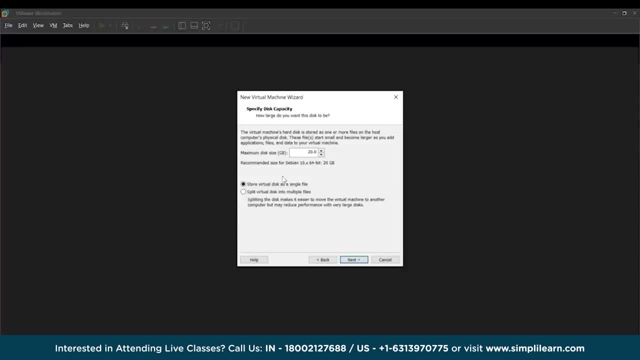 computer If there is no portability in mind. storing the virtual disk as a single file gives the best performance and should be the recommended go-to when installing for the first time. We click on next here and it's going to give us a summary of the settings we have already. 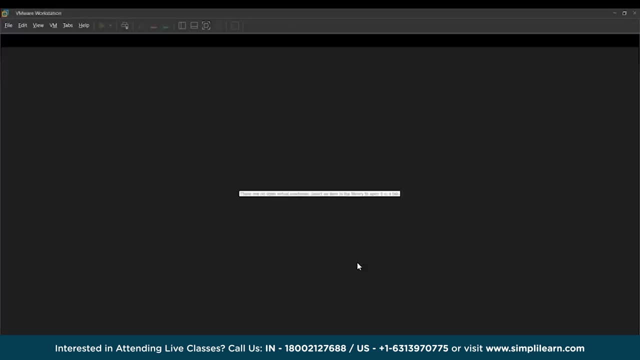 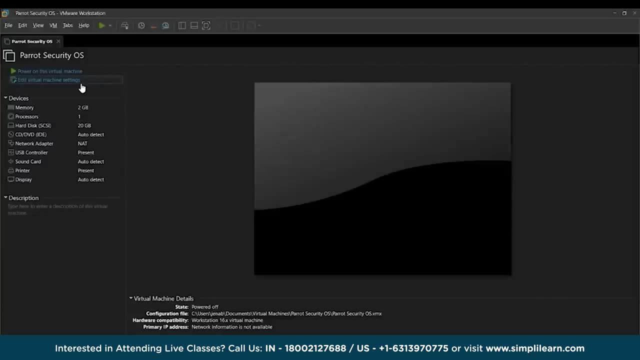 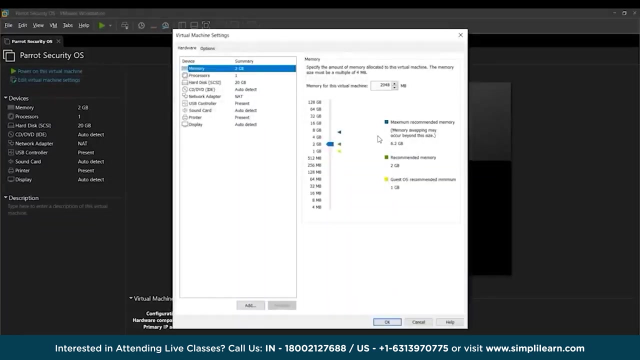 settled till now. We are going to press on finish and there we go. We have our installation first step completed. Here on out we are going to click on edit- virtual machine settings. Here we are going to have a look at some of the requirements. 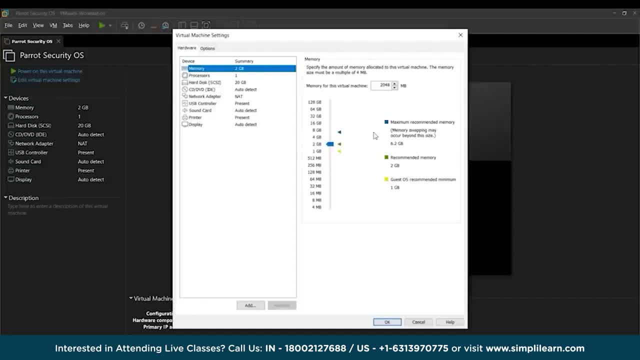 that the Parrot Security OS will need. It is known to be a memory lightweight operating system but just to have the most optimum performance, we are going to provide around 2 GB of RAM from our host system, which is a Windows 10 machine. 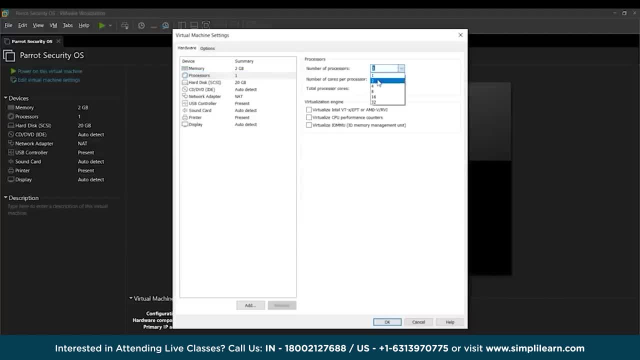 When it comes to the processors, I am going to increase it to 2 and the number of cores to 2 as well, So giving out a total 4 processor cores to the operating system. Now, this depends on what are your computer rig and how much resources. 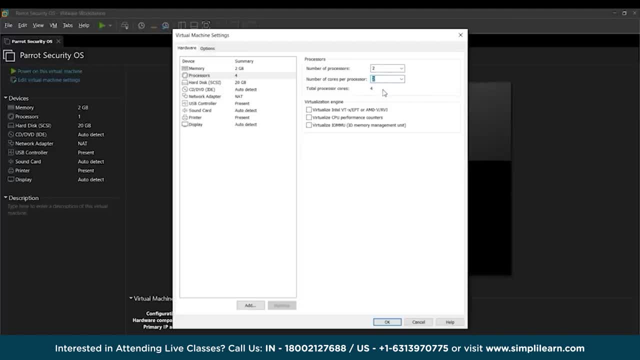 you can justify. So these need to be customized according to the system at hand. Hard disk size has already been set at 20 GB and the rest of them are pretty standard and we can go on. One thing that we need to make sure is selecting the CDDVD IDE. 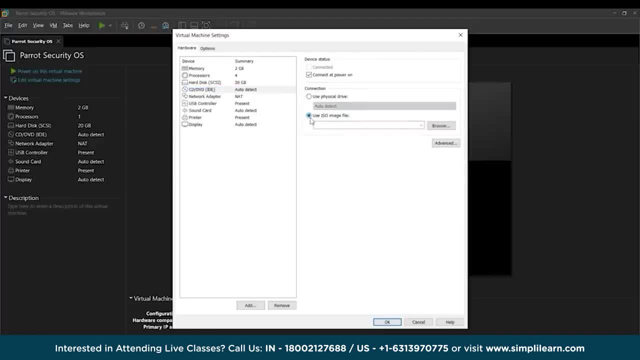 Here. we have to use our ISO image file over here. Previously it should be used physical drive and at auto detect. We are going to use a used ISO image file over here. We are going to click on browse. We are going to go to where we have. 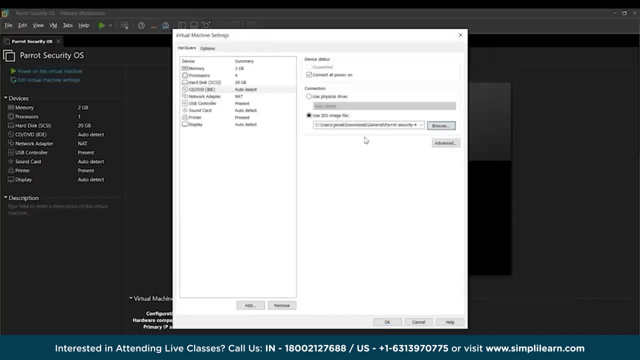 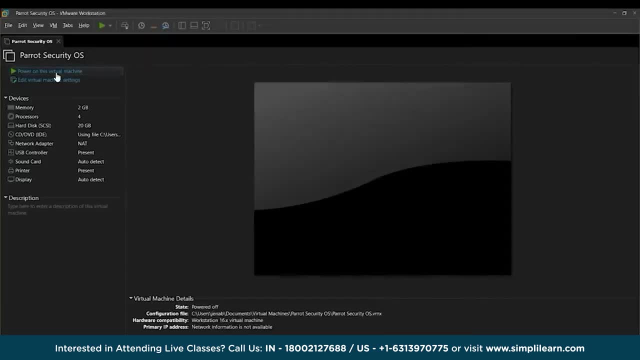 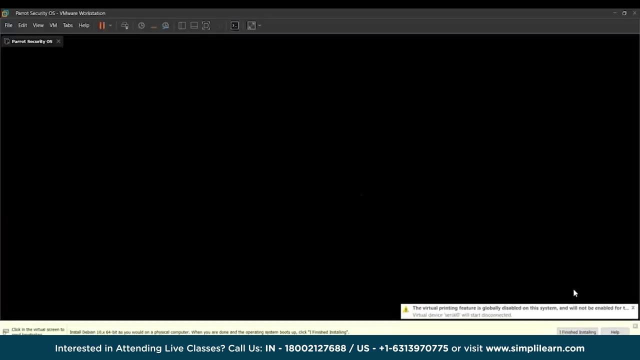 downloaded the ISO file which is over here, and select it, Press ok here and we can now power on this virtual machine. At this point of time there are two options. We can go with the try install option using the graphical user interface, or we can go using the. 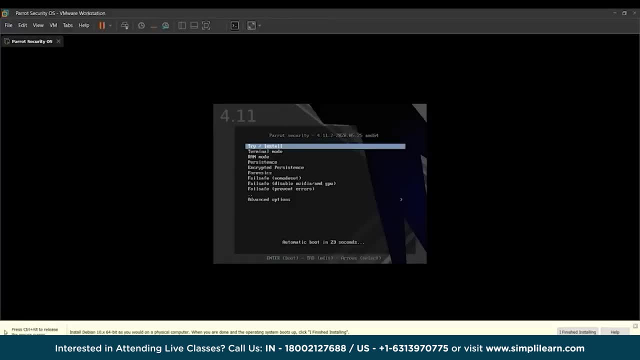 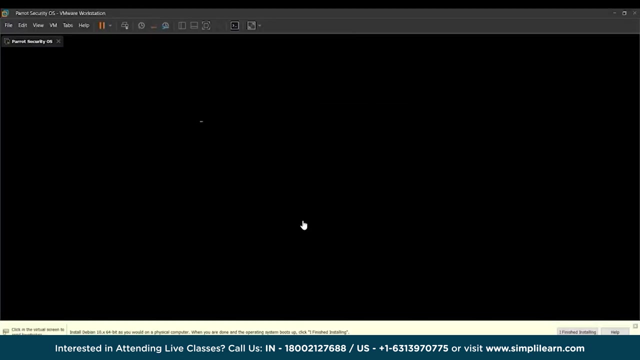 terminal mode. To get a better user experience, we are going to go with the try install mode. specifically, Press enter and it's going to start the live boot ISO. Meanwhile, VMWare has a virtual machine that can be used to install some VMWare tools on it. 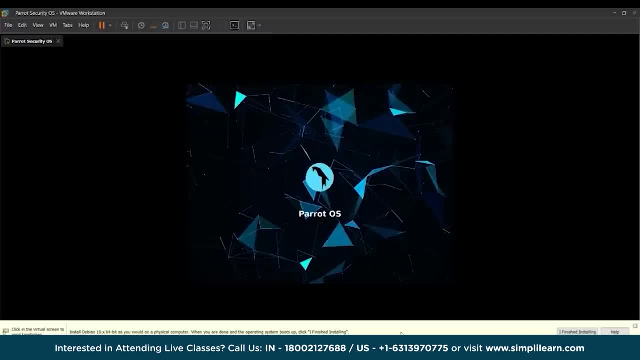 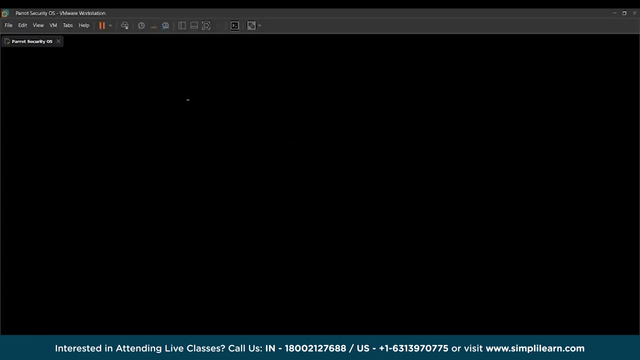 While this is not mandatory, it is much more recommended to install these tools so that you can get some additional features like drag and drop with the host system and many more things. For now, we are going to close this prompt. As you can see, this is the live boot. 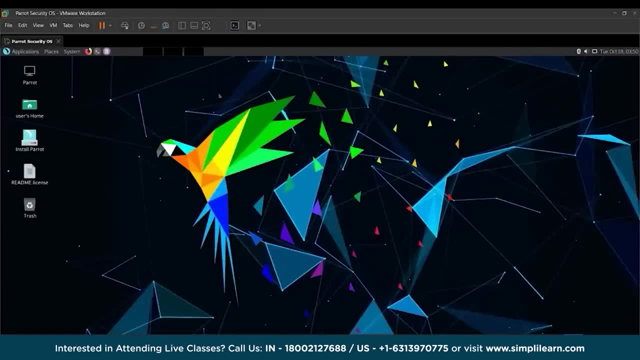 ISO of the Barrett Security Operating System. Currently it's running the Mate desktop as we have downloaded in the website. Live boot ISO is necessary to get a good feel of the operating system. There are many good Linux distros that have this live boot option so that you can. 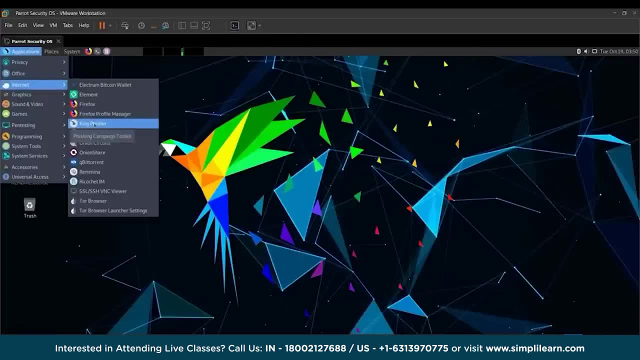 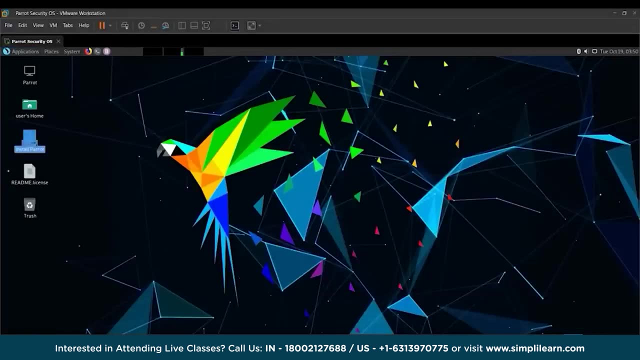 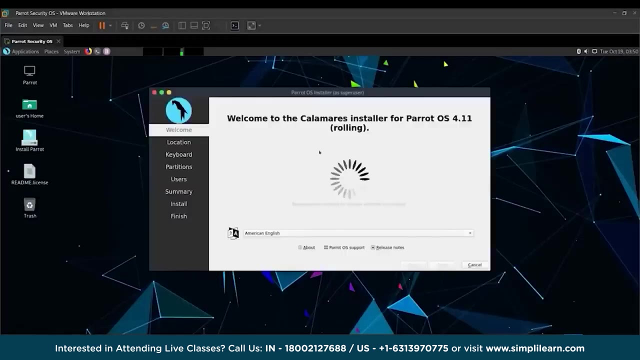 give a try of the operating system before installing it permanently. Once you are into the live boot, we can start up with the installation using the shortcut. as you can see, install Barrett. We are going to double click it and this is the Calamares installer. 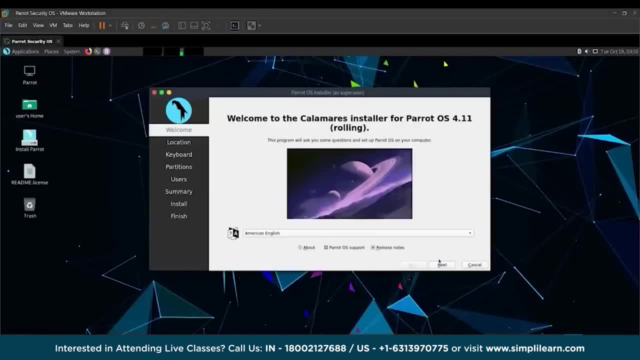 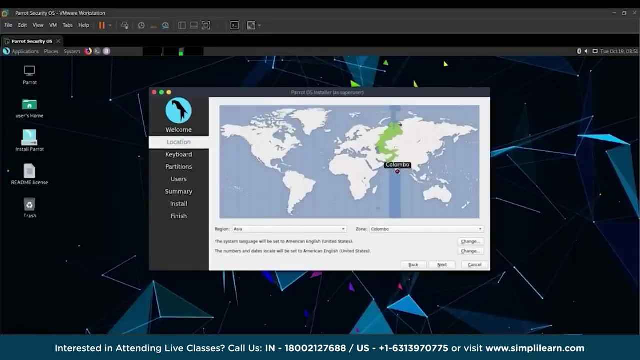 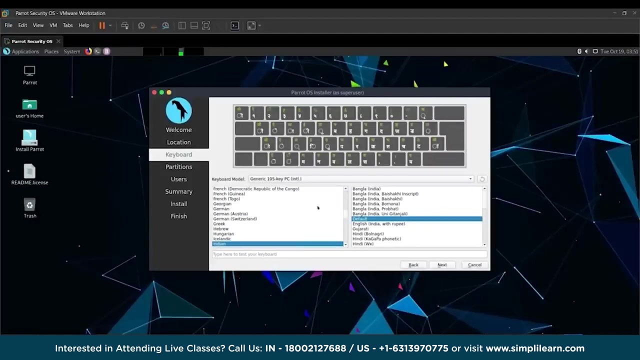 Choose your language as American English and press next. You can select your time zone according to your location and we can go next. At this point of time, you have to choose the correct keyboard. Now what many people get confused is choosing their own language. 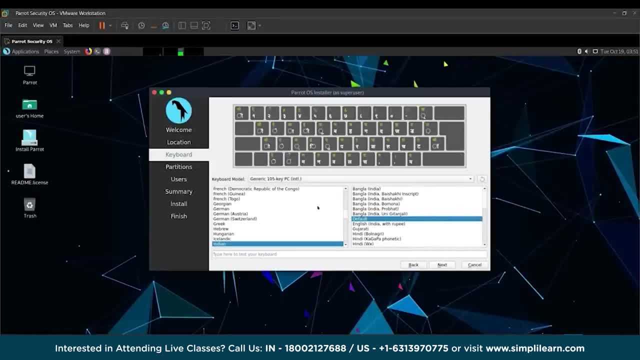 keyboard. What people must keep in mind is what keyboard the laptop provides. Most of the systems that come pre-built provide the English US keyboard. So, whatever keyboard you choose, make sure to type here and test that all the buttons, including the superscript and the 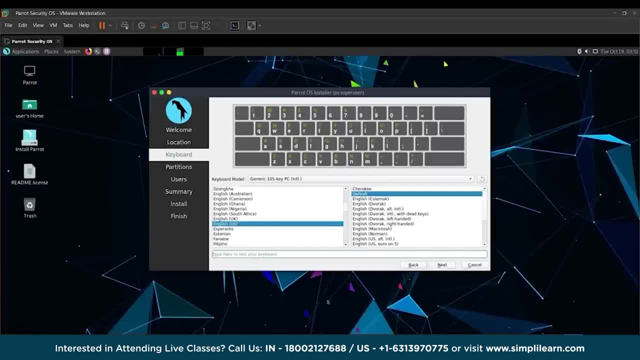 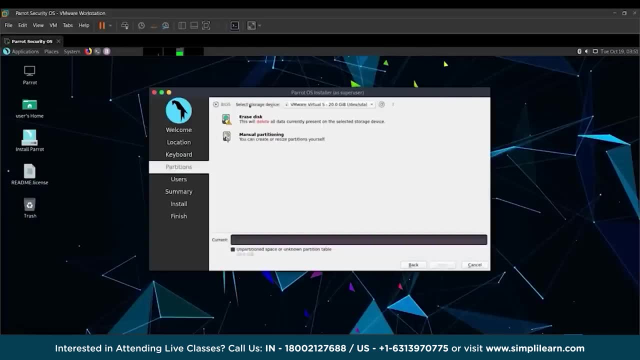 subscript buttons are working correctly. before moving forward with this step, Once you have settled on the keyboard that you need to install, you can go ahead Here. it will ask you to select storage device, and the only option you are going to get is the amount. 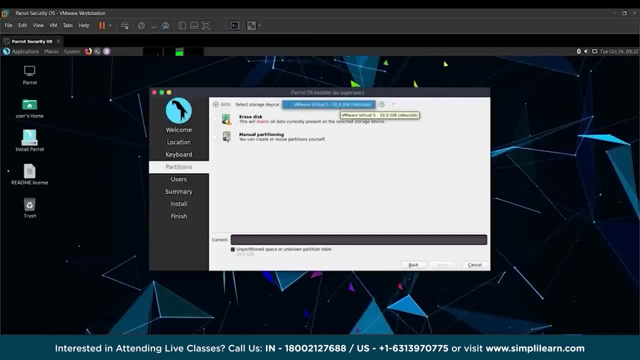 of hard disk storage you have given. in the virtual machine settings We have already provided 20 GB of storage. We are going to choose that and we are going to erase this disk. Manual partitioning can be useful when you are going to install pallet security on an operating. 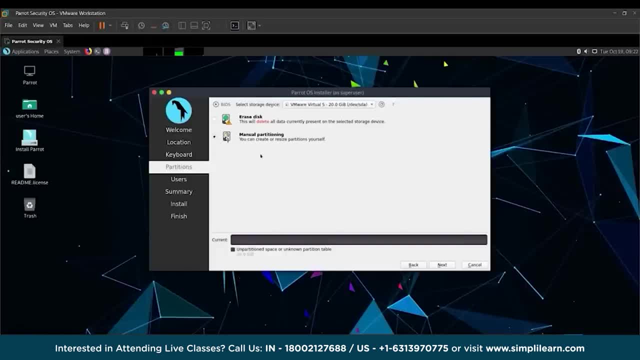 system, or on a hard disk, where it is already including a Windows OS. For now, we are going to select erase disk and press next. We are going to give our full name. Let it be simply learn: You can give the name of the computer. 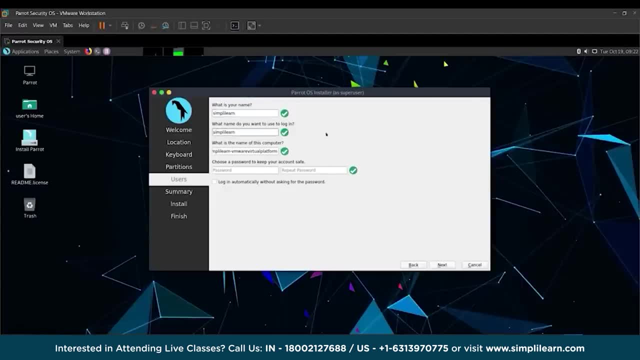 and this is the username which we will use to login. This is your root password that we are going to give over here. The root password of this Kali Linux will act as the administrative access and it will be necessary for making changes to the system or installing. 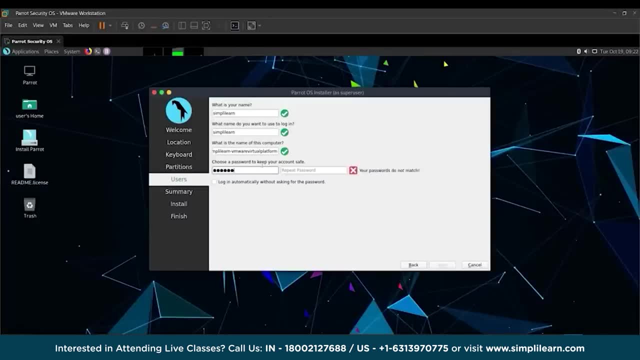 and updating software. Enter the password and repeat it over here You have the option to login automatically without asking for the password, but for security purposes it is recommended to keep this disabled. Click on next. This is another summary of the installation that we are going to move forward with. 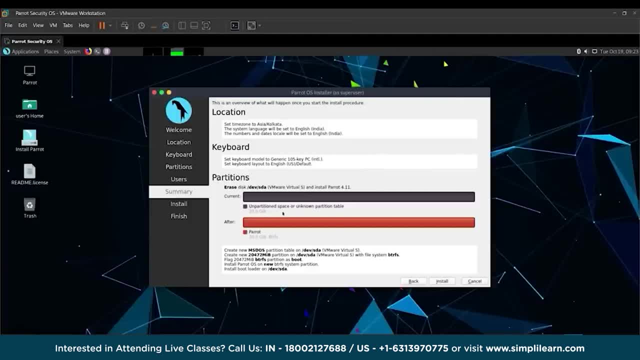 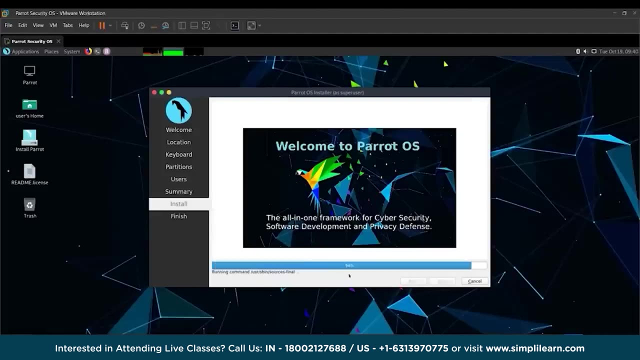 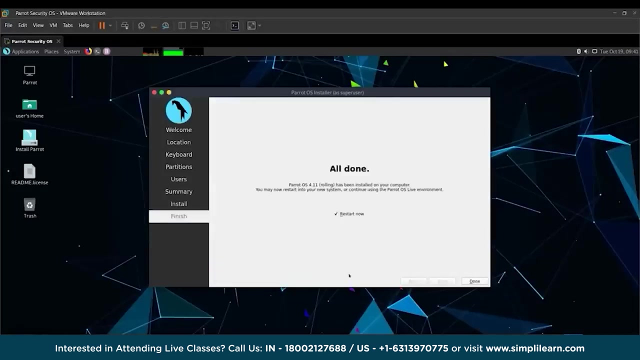 Have a look that whatever changes we have made is according to your requirements, and once everything is checked, you can press on install. Click on install now and we are going to let it complete the work. As you can see, the installation of pallet security is now completed. 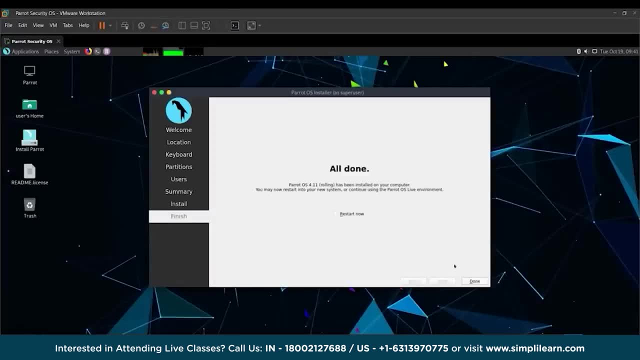 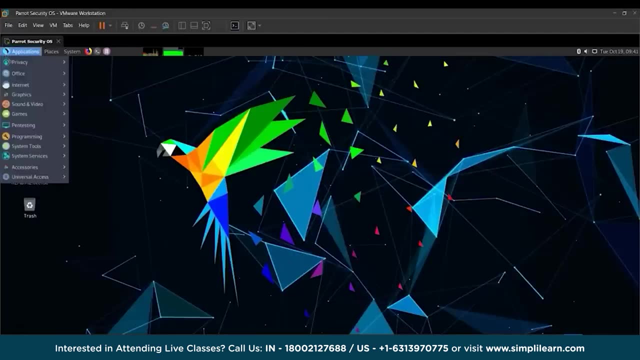 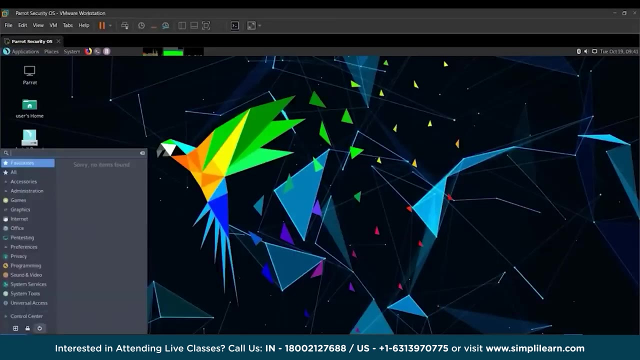 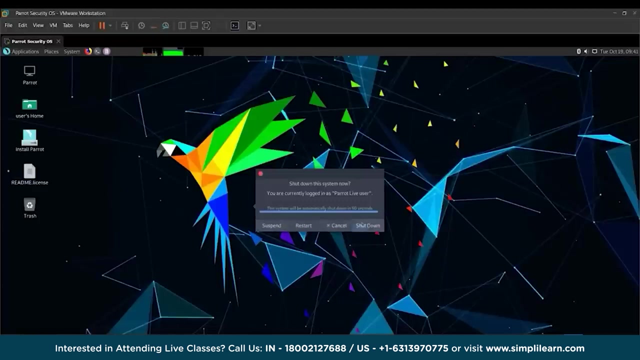 We are going to make sure that we have the restart button over here disabled. I am going to click on done. We are going to shut down this live boot ISO. We are going to click on menu, Turn off the device and shut down. 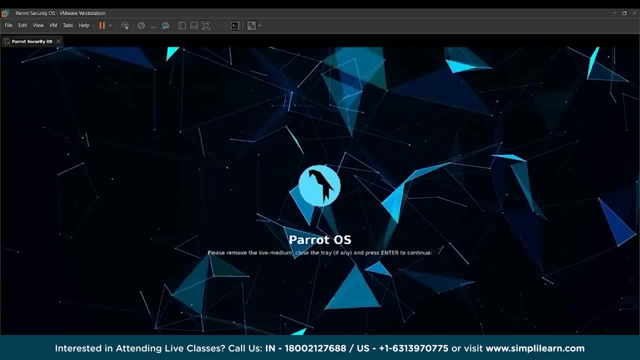 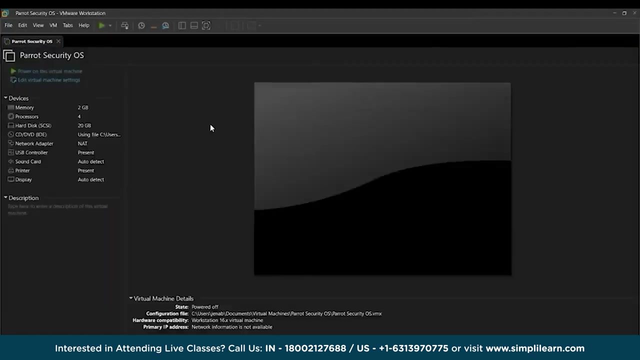 We are not restarting straight away because we need to remember correctly in the virtual machine instance settings we had given it an ISO file. Please remove the live medium and press enter to continue. We can just press enter to continue and it is going to shut down. 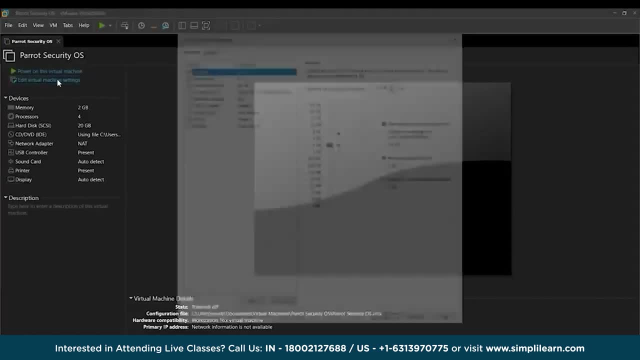 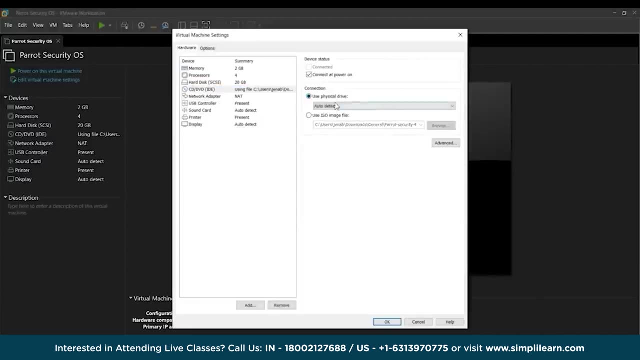 Now to move on. we are going to click on edit virtual machine settings. We are going to CD, DVD and we are going to use physical drive. now We are going to remove it from the ISO. We are going to remove the image file. 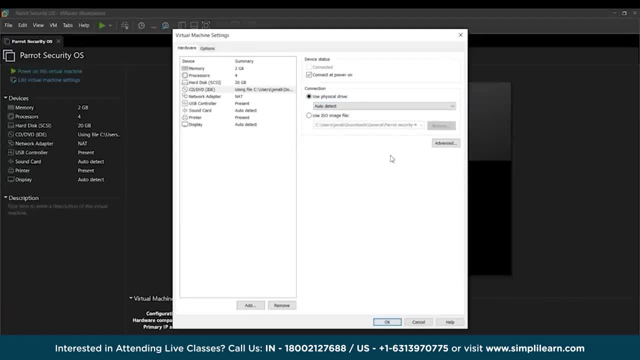 because installation has already been completed and we don't want to use the same ISO file again and again By using physical drive over here. it is going to detect the 20 GB hard disk that we have already provided and installation is done on it. 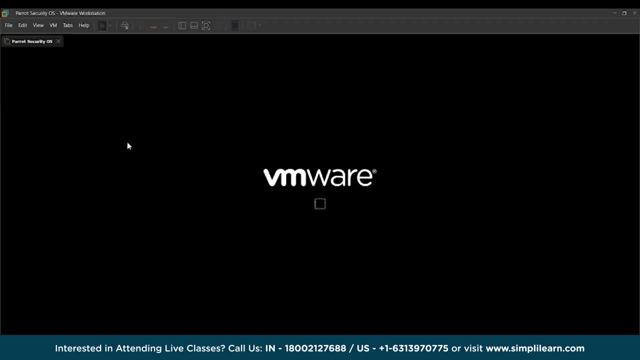 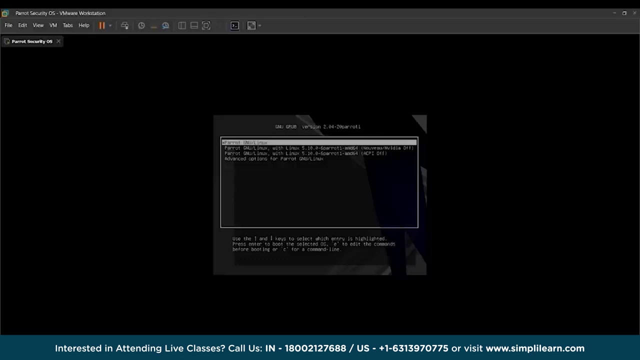 We are going to press. ok, We are going to power on this virtual machine for testing. Make sure that you click ES over here. This is the grub menu. At this we get different choices, For example, which NVIDIA drive is off or with some other advanced options. 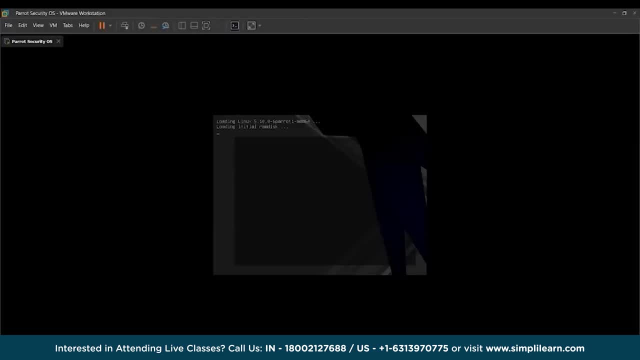 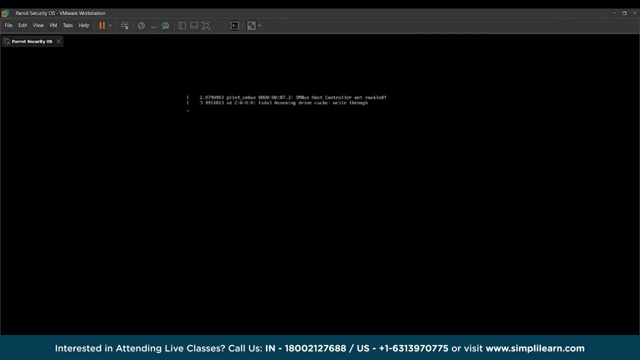 More often than not, we are going to choose the first option and press enter. If you remember clearly, we did not get the option of try install or a terminal run, just like we did in the live boot ISO, Since this is running straight from the. 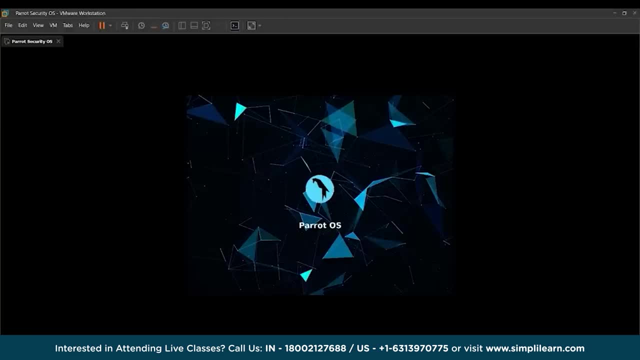 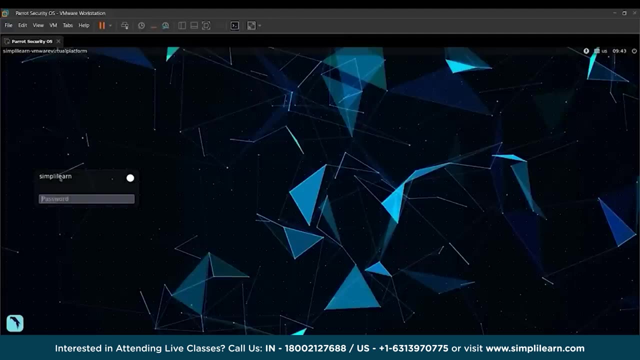 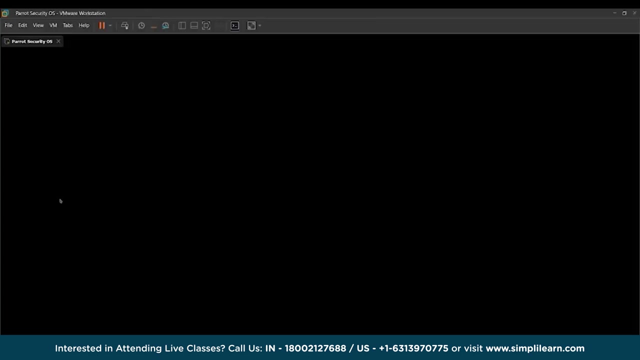 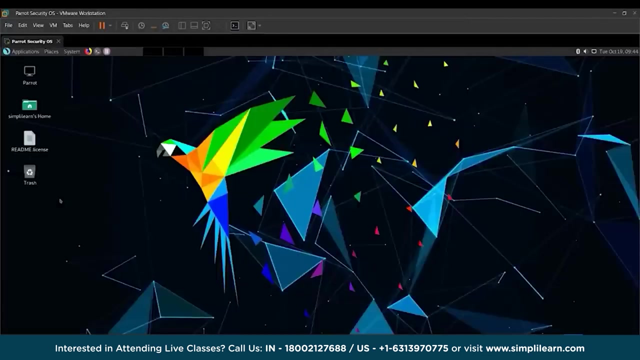 20 GB hard drive storage. it is going to start the OS directly Now with the login screen. you can see our username over here, as we provided in the installation. We are going to enter our root password and press enter, And this is our currently working desktop of the. 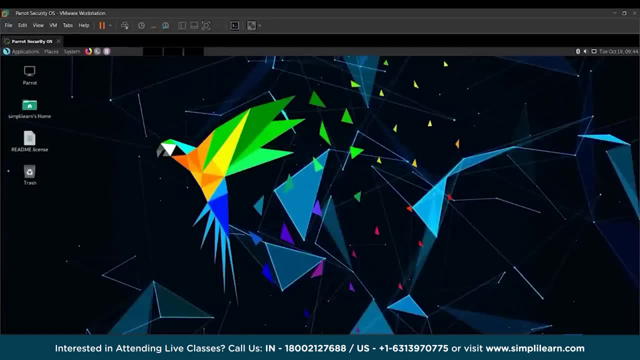 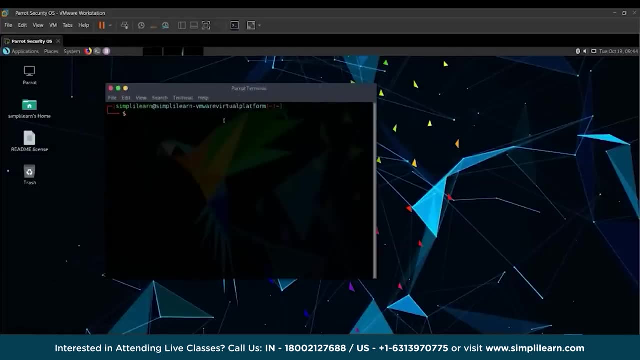 Parag Security operating system. We can open the terminal over here and we are going to try our root password and installation. To install any software. we are going to use the keyword sudo, apt, install and neo fetch. We are going to use the root password that we used to login. 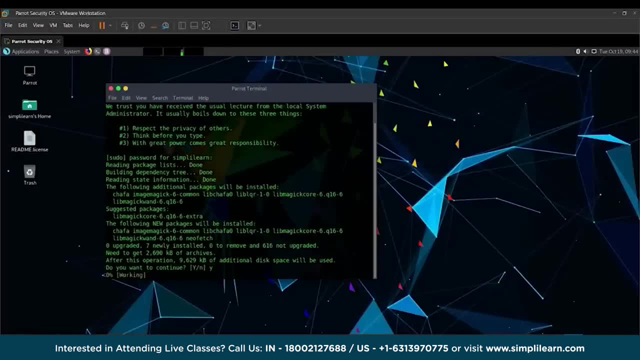 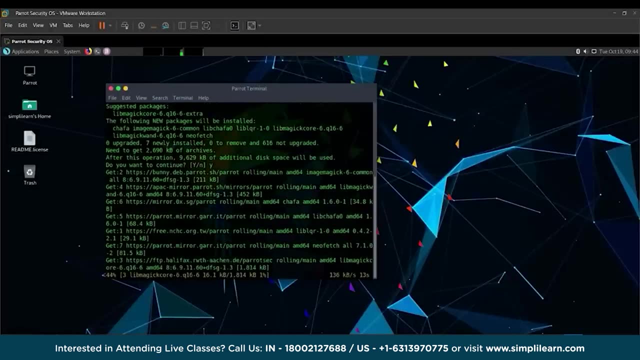 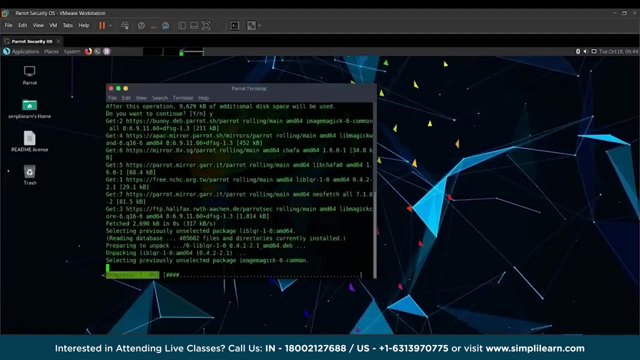 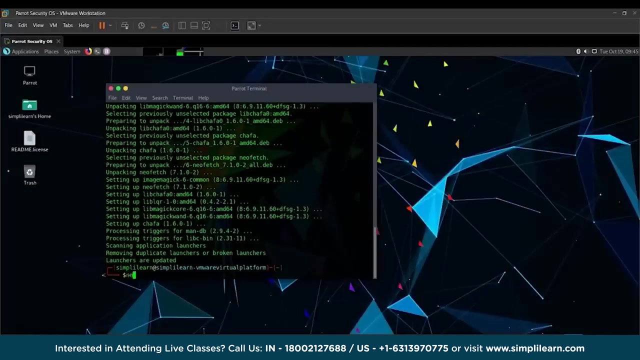 We are going to press Y for yes. This is just an additional step that we are doing to check that the installation is done correctly with the correct amount of hardware requirements that we had provided. Now that we have installed neo fetch, we can write the command neo fetch. 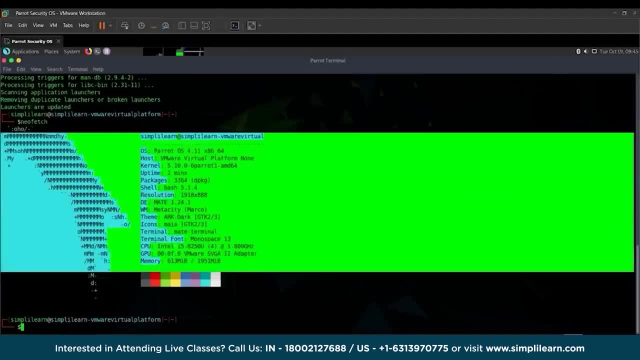 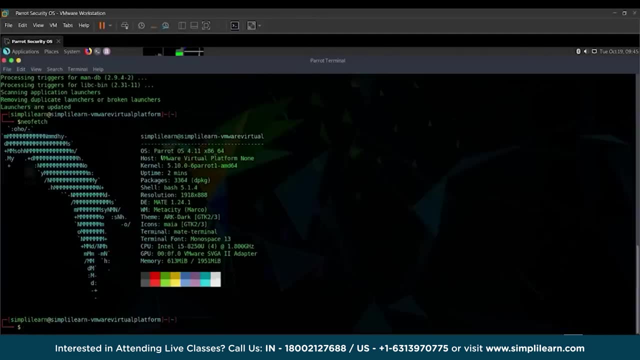 and this is going to give us some information about our installation. You can see the OS name as Parrot OS 4.11 is running on a VMware host. It's the kernel versions and some of the other information like the number of packages installed. 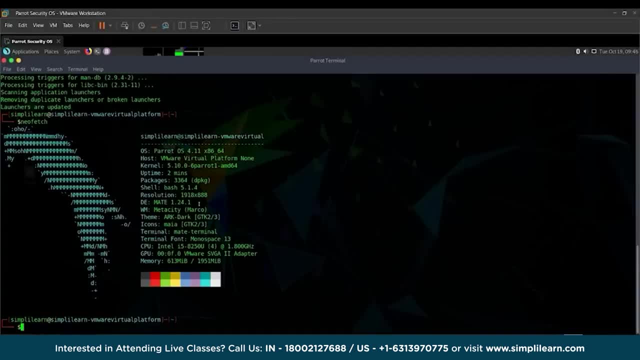 the current shell version resolution of the VMware instance that we are running, the desktop environment which is made as we had downloaded once and some other things. You can see the memory is supposed to be 1951 MB, which is supposed to equal around 2 GB. 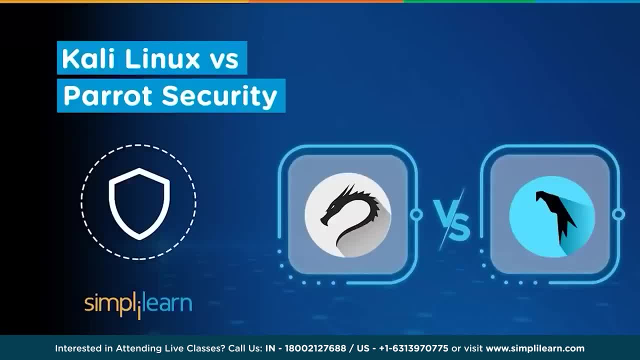 of RAM usage that we had provided. Kali Linux and Parrot OS are two popular penetration testing distributions. While these operating systems each have unique offerings, the overall choice can differ between personnel thanks to their various tools and hardware specifications. Today, we will look at both these distributions. 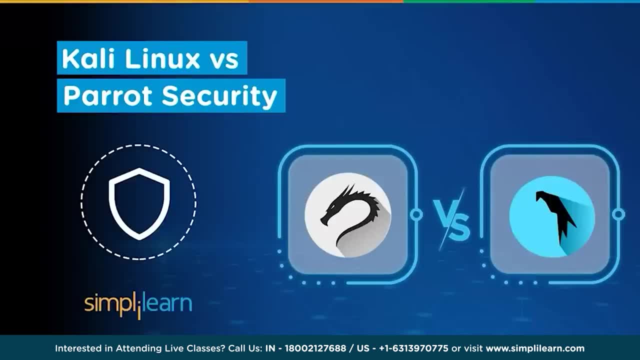 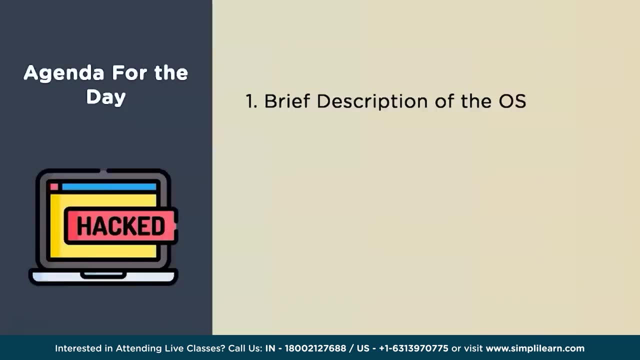 and settle on the perfect choice for each type of user. Let's go through the agenda for this video. We will learn about Kali Linux and Parrot Security OS from scratch, while understanding their primary selling points as a Linux distribution catered towards penetration testers. 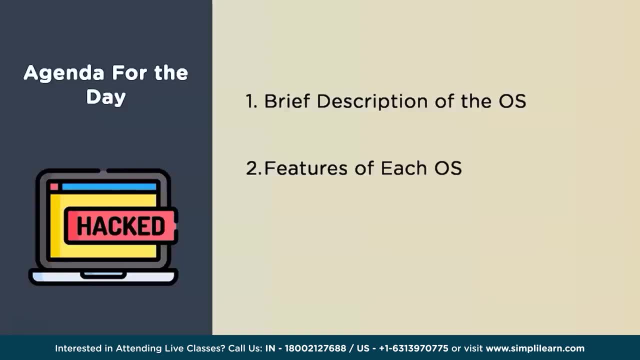 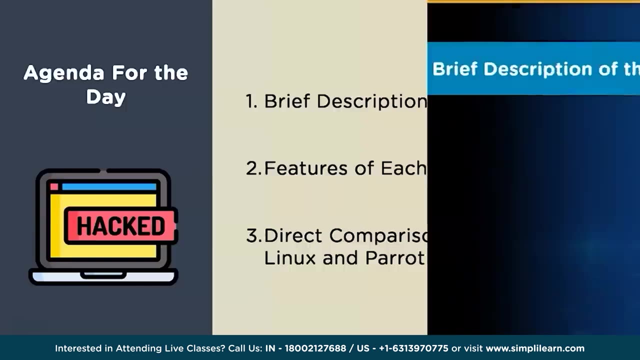 Next, we know about some features of these operating systems that stand out of their package. Finally, we directly compare Kali Linux and Parrot Security OS, thereby making a clear-cut conclusion on which OS is perfect on a per-requirement basis. So let's start by learning about. 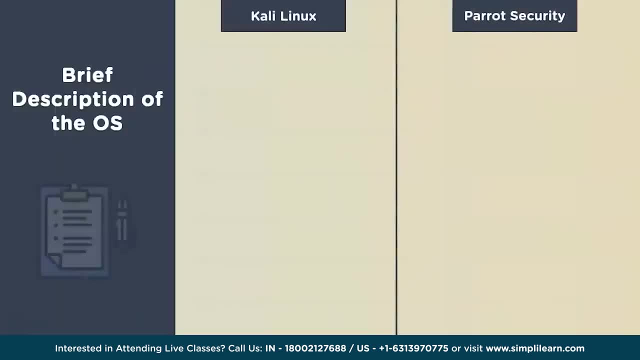 Kali Linux from a ground level. Kali Linux, which is formerly known as Backtracking Linux, is an open-source Linux distribution aimed at advanced penetration testing and security auditing. It contains several hundred tools targeted towards various information security tasks, such as penetration testing, security research, computer forensics. 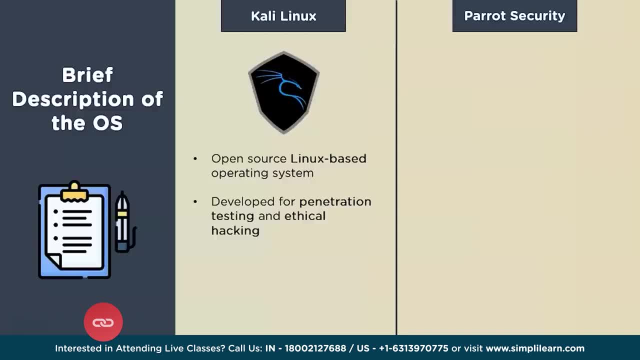 and reverse engineering. Kali Linux is a multi-platform solution accessible and freely available to information security professionals and hobbyists. Among all the Linux distributions, Kali Linux is the best. Kali Linux takes its roots from the Debian operating system. Debian has been a highly dependable and a 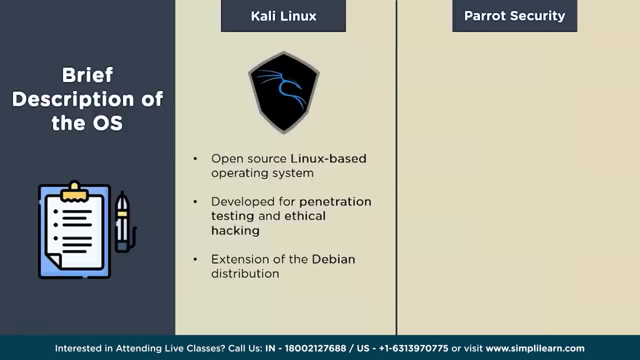 stable distribution for many years, providing a similarly strong foundation to the Kali Linux desktop. While the operating system can practically modify every single part of our installation, the networking components of Kali Linux come disabled by default. This is done to prevent any external 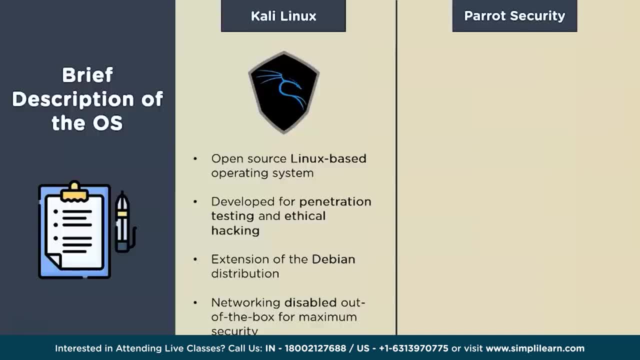 factors from affecting the installation procedure, which may pose a risk in critical environments. Apart from boosting security, it allows a more profound element of security control to the most enthusiastic of users. Now let's take a look at Parag Security operating system. Parag Security OS. 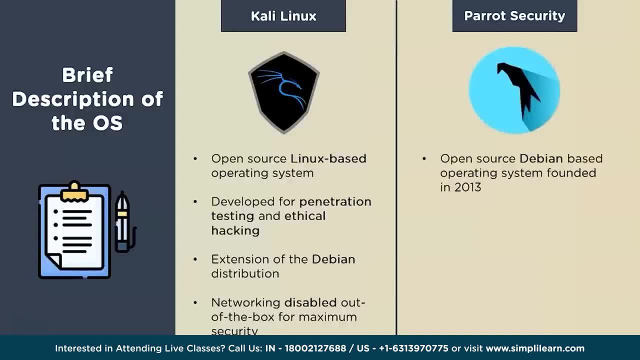 is a Debian-based Linux distribution with an emphasis on security, privacy and development. It is built on the Debian's testing branch and uses a custom hardened Linux kernel. Parag Security contains several hundred tools targeted towards tasks such as penetration testing, computer forensics. 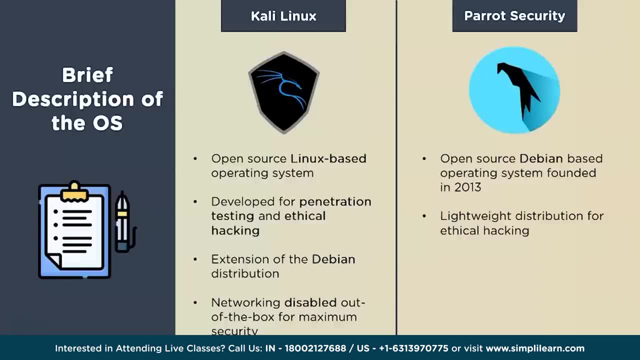 reverse engineering and security research, It is seen as a generally lightweight distribution that can work under rigorous hardware and software specifications. It features a distinct forensics mode that does not mount any of the system's hard disks or partitions and has no influence on the host system. 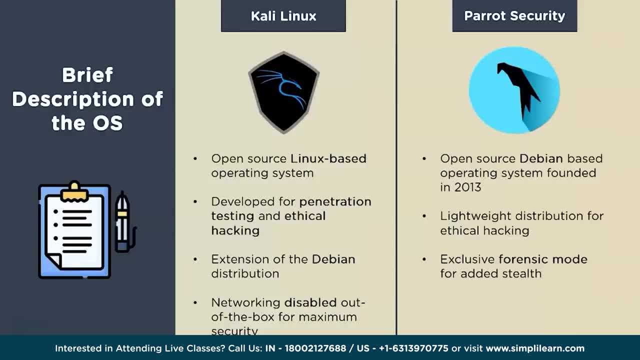 making it much more stealthy than its regular occurrence. This mode is used on the host system to execute forensic procedures. A rolling release is a paradigm in which software upgrades are rolled out constantly rather than in batches of versions. in software development, This ensures that 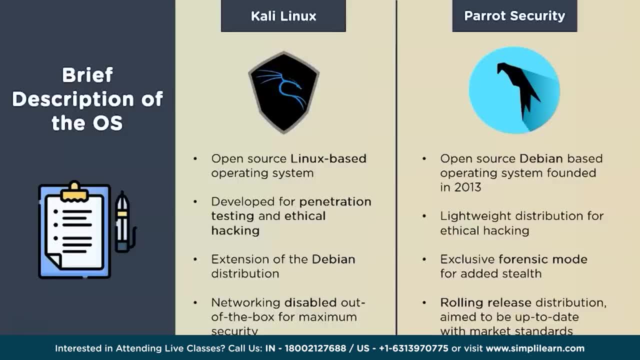 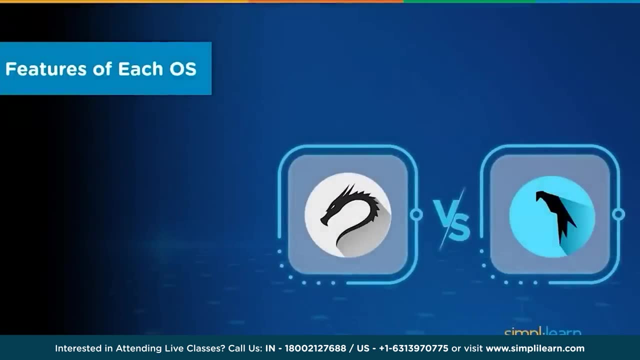 the software is constantly up to date. A rolling release distribution such as Parag Security OS follows the same concept. It provides the most recent Linux kernel and software versions as soon as they become available, With a basic introduction to the operating systems out of the way. 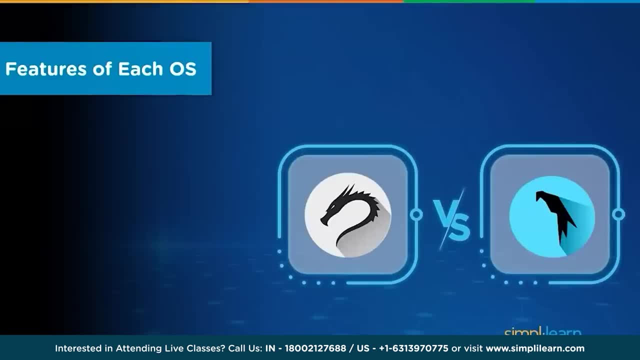 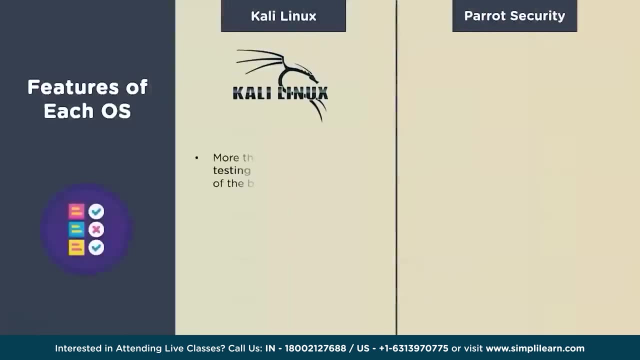 let us take a look at the unique features of both Kali Linux and Parag Security OS. The latest version of Kali Linux comes with more than 600 penetration tools pre-installed. After reviewing every tool included in Backtrack, developers have eliminated a significant 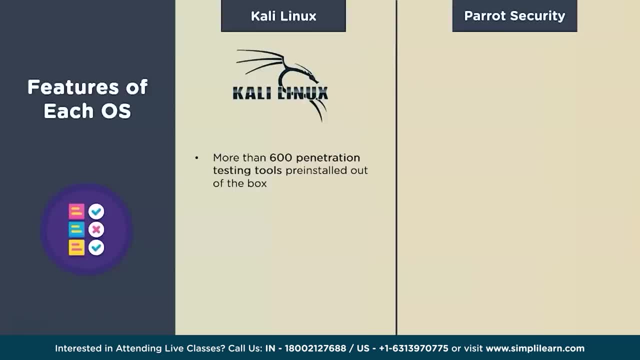 number of tools that either simply did not work or duplicated other tools that provided the same and similar functionality. The Kali Linux team comprises a small group of individuals who are the only ones trusted to commit packages and interact with the repositories, all of which is done using multiple 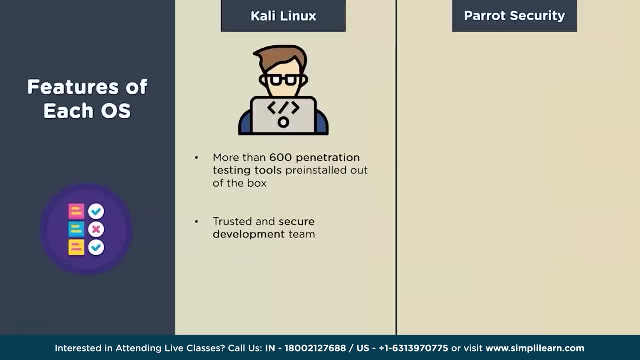 secure protocols. Restricting access of critical code bases to external assets dramatically reduces the risk of source contamination, which can cause Kali Linux users worldwide a great deal of damage as a direct victim of cybercrime. Although penetration tools tend to be written in English, 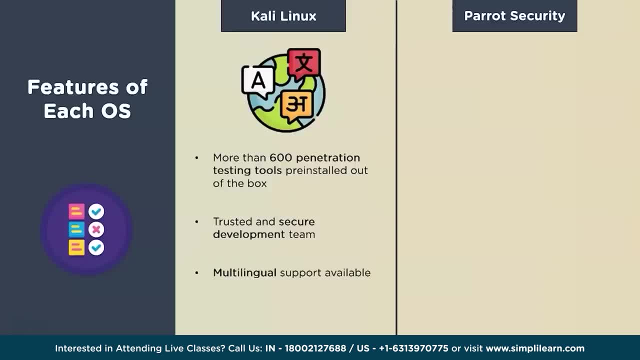 the developers have ensured that Kali includes proper multilingual support, allowing more users to operate in the native language and locate the tools they need for their job. The more comfortable a user feels with the intricacies of the operating system, the easier it is to maintain. 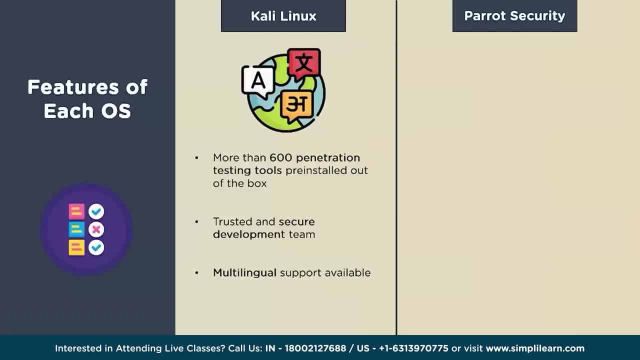 a strong hold over the configuration and the device in general. Since ARM-based single board systems like the Raspberry Pi are becoming more prevalent and inexpensive, the development team knew that Kali's ARM support would need to be as robust as they could manage with fully. 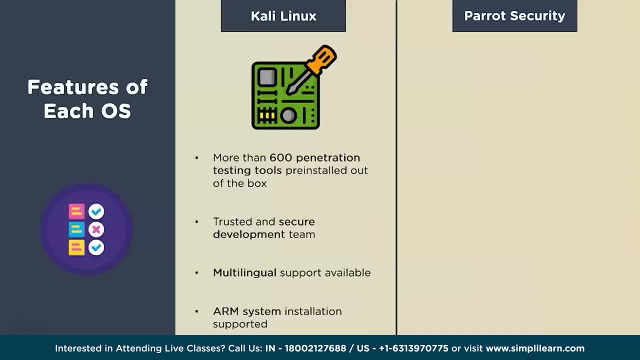 working installations. Kali Linux is available on a wide range of ARM devices and has ARM repositories integrated with the mainline distribution, so the tools for ARM are updated in conjunction with the rest of the distribution. Let's take a look at some of the 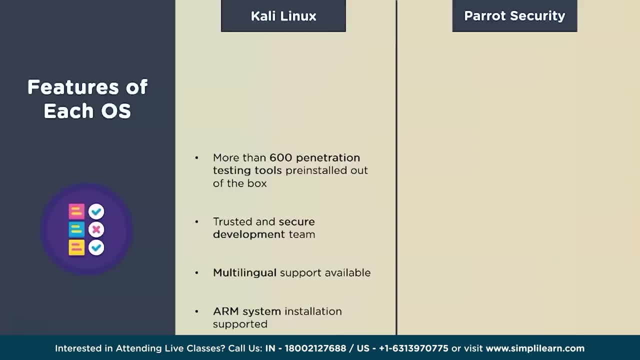 features of Parrot Security operating system. now, Along with a giant catalogue of scripts, Parrot Security OS has its own hardened Linux kernel, modified explicitly to provide as much security and resistance to hackers as possible in the first line of defense. The configurations in the operating 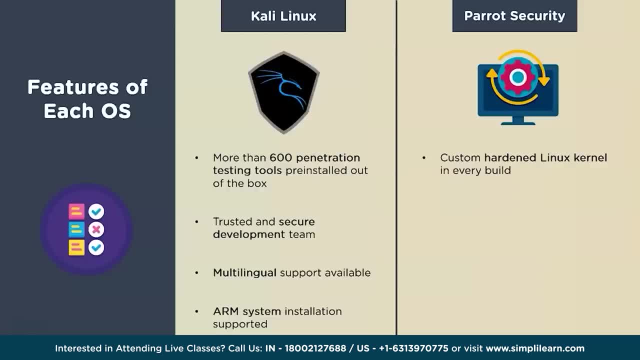 system act as the second gateway, taking care of malicious requests and dropping them off. This is particularly beneficial since, should there be a scenario where the latex Linux kernel is causing some particular issue, the Parrot OS development team will most likely iron it out first before passing it on as an 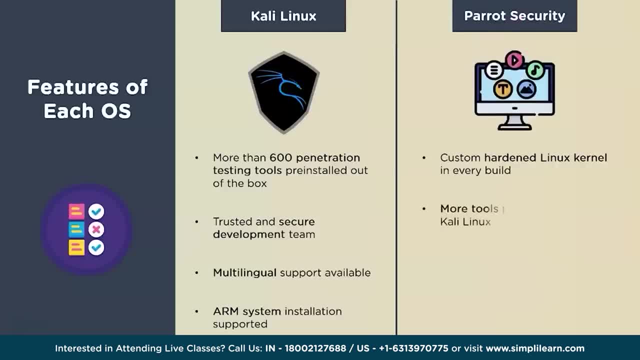 ARM update. If the custom hard-nailed kernel wasn't recent enough, Parrot Security developers managed to install more hacking tools and scripts to ensure a smooth transition for the Kali Linux users. All the tools you find in Kali are present in Parrot OS. 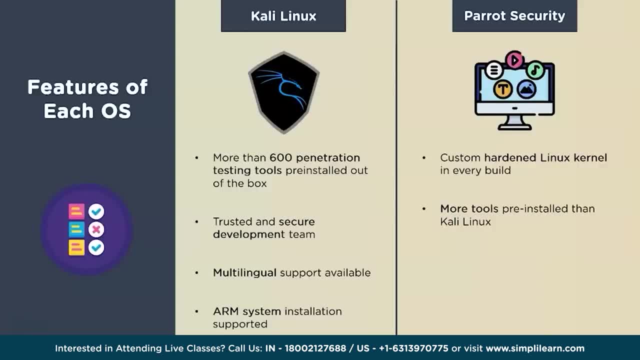 and a few extra ones for good measure, And this has been achieved while keeping roughly the same operating system size between both of them. However, it's not all. productivity points for Parrot OS, They provide a choice between two different desktop environments: MATE, which comes pre-installed by default. 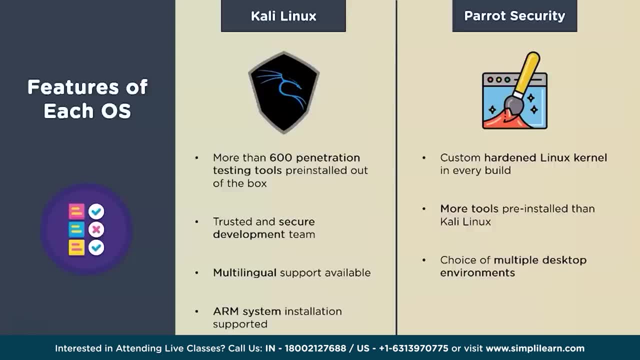 and KDE. For those unfamiliar with Linux terminology, you can think of desktop environments as the main UI for a distribution. Being highly modular in nature, one can use Parrot Security OS while adding another desktop environment that they find appealing, While Kali Linux has only a single. 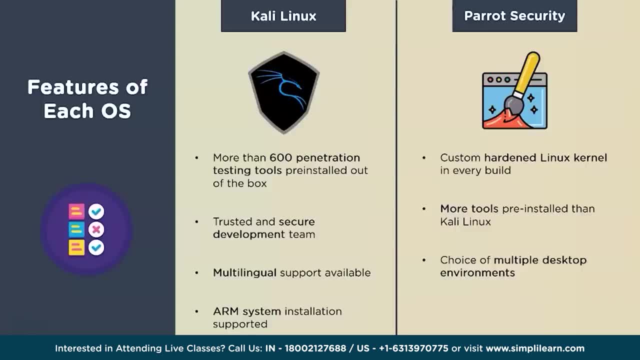 option. Parrot Security has provided two optimized builds with MATE Desktop and KDE Desktop. One of the primary advantages of Parrot OS over Kali Linux is that it's relatively lightweight. This implies that it takes significantly less disk space and computing power to function. 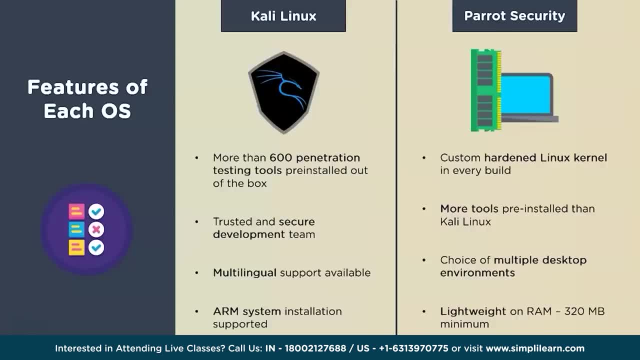 correctly with as little as 320 MB of RAM required. In reality, Parrot OS is designed to operate successfully off a USB stick, but Kali Linux does not work well from a USB drive and is generally installed in a virtual machine. Parrot OS is more of a niche. 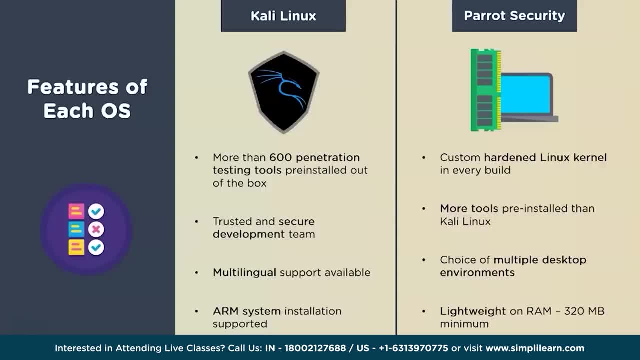 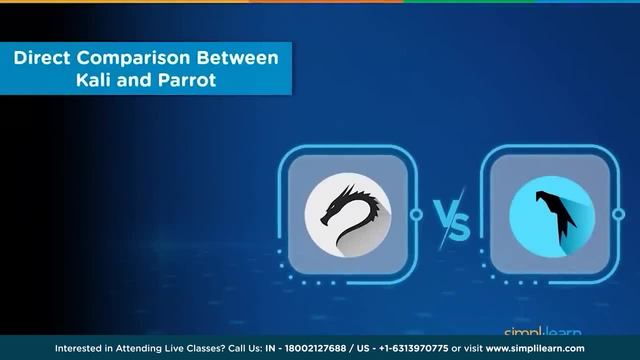 distribution if you're searching for something lighter than Kali Linux. Features are great, but what about performance? Real-world metrics? Let us compare both these operating systems directly with respect to their hardware specifications and usability. In the end, we can decide on what distribution. 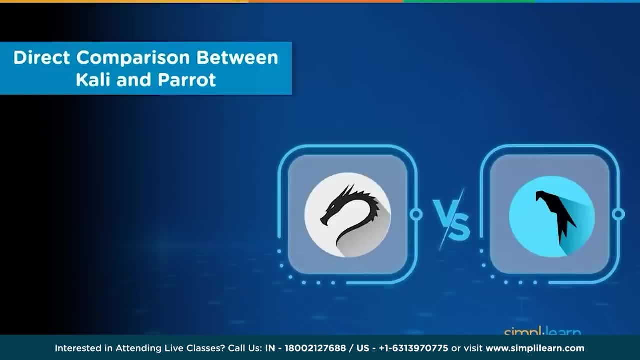 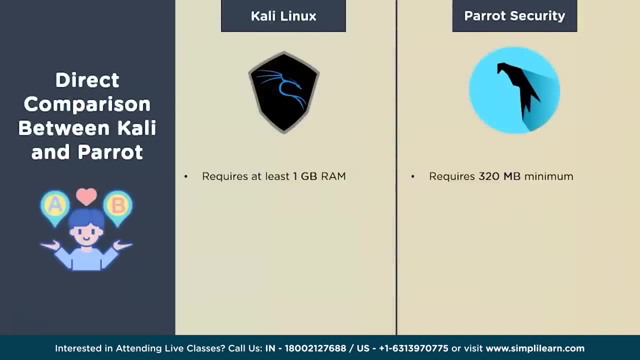 is fit for each type of user. For our first point of comparison, let's take a look at the RAM required For optimum performance of the operating system, which is highly essential when trying to crack hashes or something of similar nature. RAM usage is a. 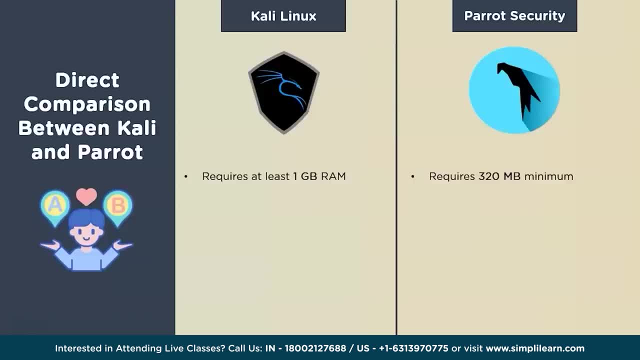 very important facet. While Kali Linux demands at least 1 GB of RAM, Parrot Security can operate optimally with a minimum of 320 MB of RAM. For correctly displaying graphical elements, Kali Linux requires GPU-based acceleration, while this is not the case with. 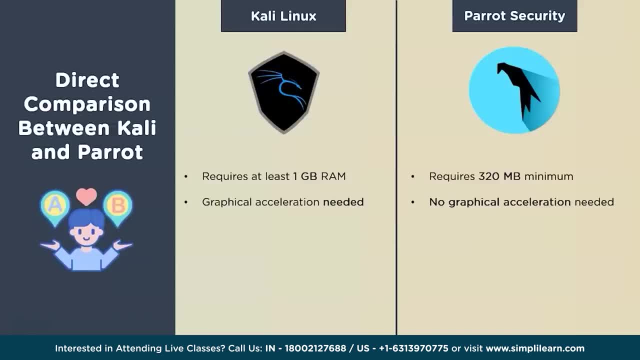 Parrot Security OS, which doesn't require any graphical acceleration needed from the user side. Once these operating systems are installed on VMware using their live boot ISOs, they take up a minimum amount of hard disk storage. Both of these operating systems have a recommended 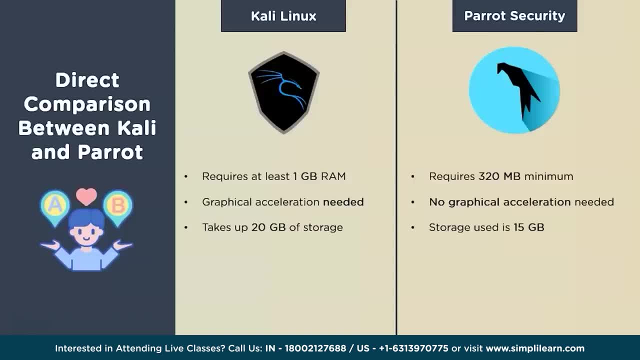 disk storage of minimum of 20 GB in Kali Linux and a minimum of 15 GB in Parrot Security, so they can install all the tools necessary in the ISO file. When it comes to the category and the selection of tools: Kali Linux. 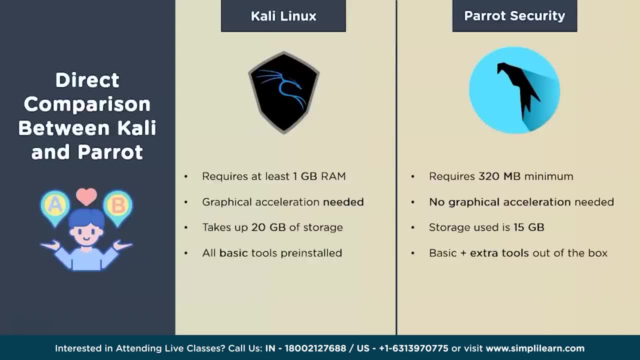 has always been the first in securing every single tool available for hackers in the penetration testing industry. Parrot Security, on the other hand, has managed to take it up a notch. While specializing in wireless pen testing, Parrot Security makes it a point that 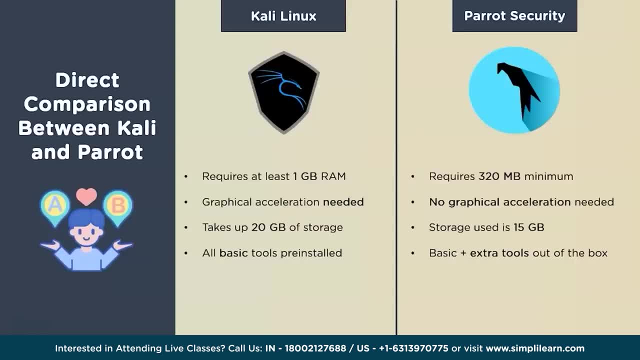 all the tools that Kali Linux provides has been included in the ISO file, So while simultaneously adding some extra tools that many users will have to install from third party sources in Kali Linux. Being a decade old penetration testing distribution, Kali Linux has 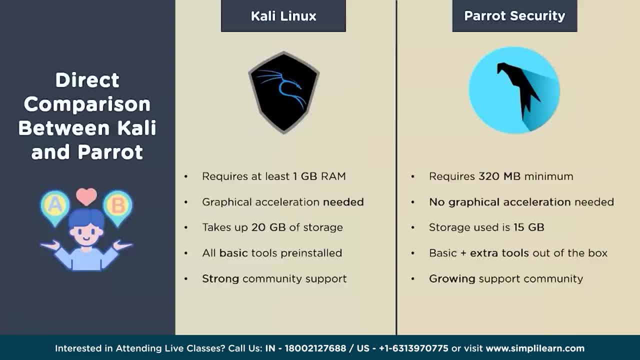 formed up a very big community with strong support signature. Parrot Security, on the other hand, is still growing and it is garnering much more interest among veteran penetration testers and ethical hackers. A primary drawback of Kali Linux is the extensive hardware requirement. 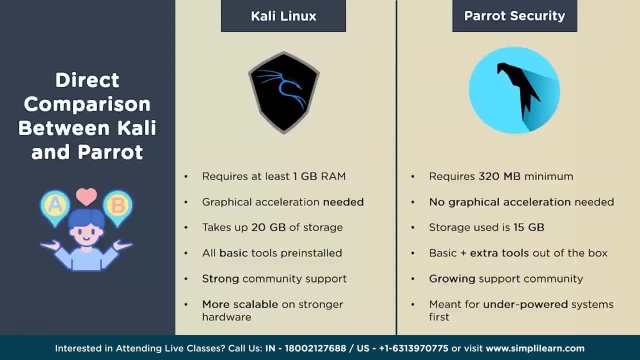 To perform optimally, it requires higher memory than Parrot Security. It also needs graphical acceleration, while demanding more virtual hard disk storage. Parrot Security, on the other hand, was initially designed to run off a USB drive directly, thereby requiring very minimal requirements from a hardware. 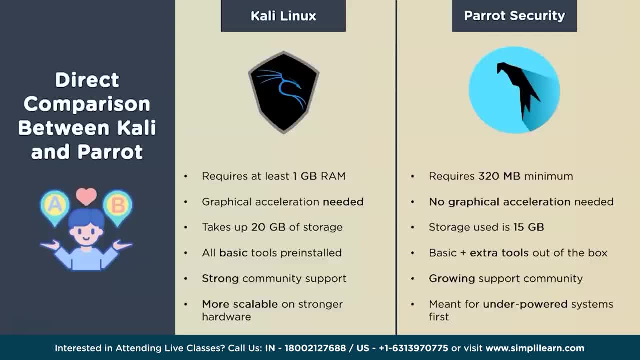 perspective like just 320 MB of RAM and no graphical acceleration needed. This means Parrot Security is much more feasible for people who are not able to devote massive resources to either their virtual machine or on their laptop hard disk directly. With the comparison done between both of these operating systems, 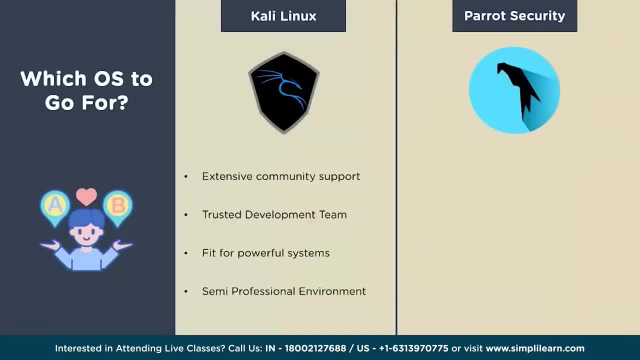 let's take a look at the type of users both of these are catered to. One can go with Kali Linux if they want the extensive community support offered by its users, if they want to go with a trusted development team that have been working on this distribution since many. 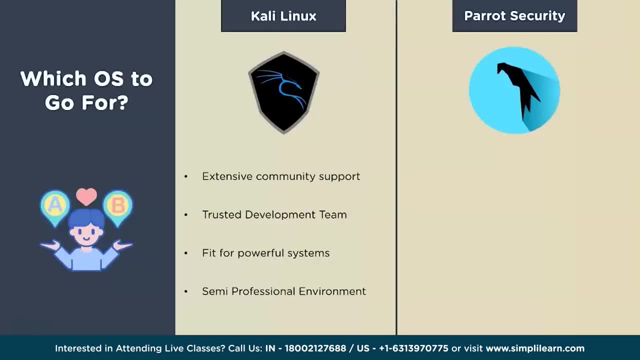 years. if they have a powerful system which can run Kali Linux optimally without having to bottleneck performance, and if they are comfortable with a semi-professional environment, which may or may not be very useful for new beginners, One can decide to go with Parrot Security if they want. 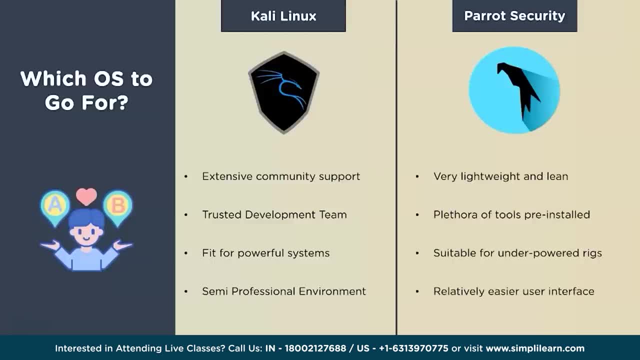 to go with a very lightweight and lean distribution that can run pretty much on all systems. It also has a lot of tools pre-installed, and some of them are not even present on Kali Linux. It is much more suitable for underpowered rigs, where 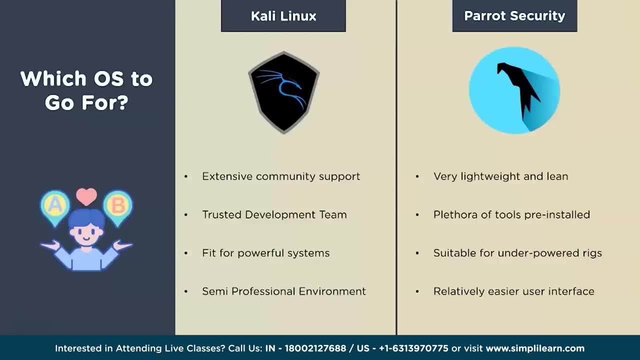 users do not have a lot of hardware resources to provide to the operating system, and thereby it is much more feasible for people with underpowered laptops or no graphical acceleration. Compared to Kali Linux, Parrot Security's desktop environment is also relatively easier to use for new beginners. 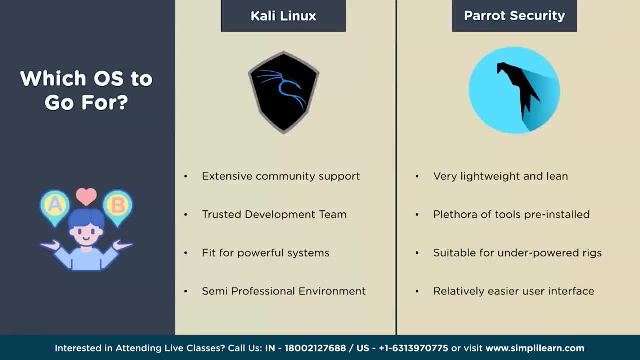 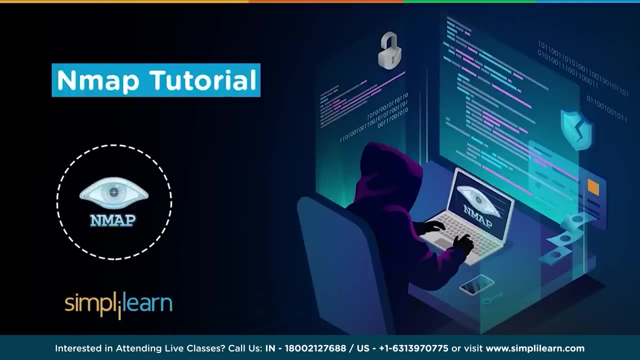 For people who are just getting into ethical hacking, Parrot Security does a relatively better job Of introducing them to the operating system and to the various tools without having to dump them into the entire intricacies. With ethical hacking and penetration testing becoming mainstream in corporate environments, 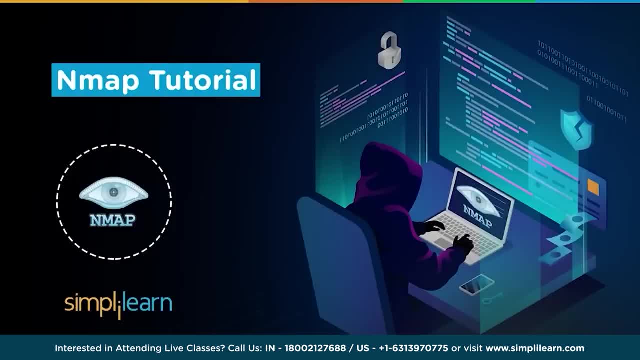 trained personnel and relevant equipment are in high demand. The right software framework can be the tipping point in a hacking campaign which deals with intricate hardware. One such tool that has become a mainstay for decades is Nmap When it comes to scanning machines for open ports and services. 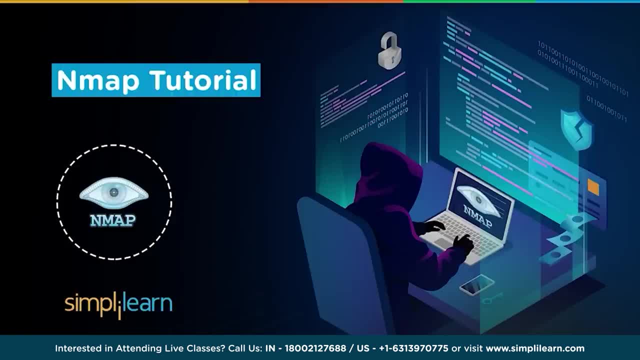 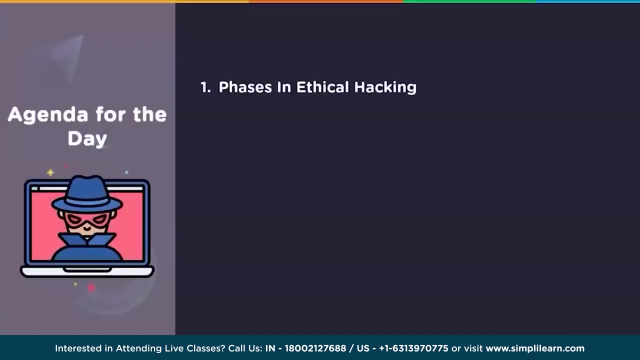 Nmap has always been the first choice for hackers. Being lightweight and open source, Nmap has strong community backing and receives regular updates. Let's take a look at the topics to be covered today. We start by learning about the different phases in ethical hacking and where Nmap 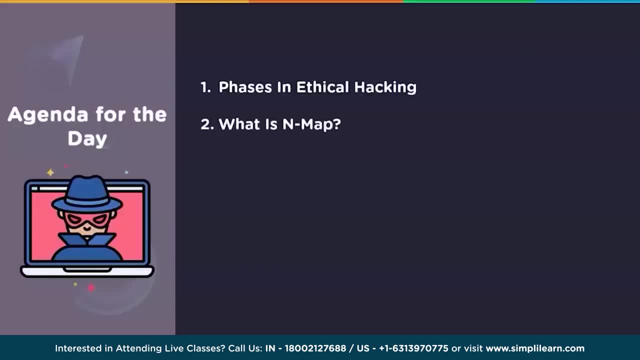 is most valuable to ethical hackers. We learn the basics of Nmap and its purpose during a penetration testing campaign. Next, we take a look at the top level approach of Nmap as a scanning tool and how it conducts these scans on host machines. 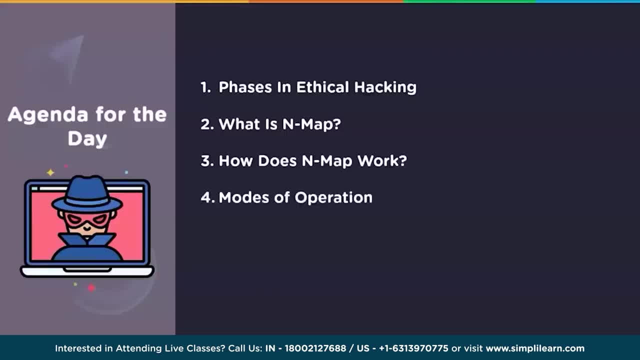 Moving on. we cover the multiple modes and types of scans that can be performed using Nmap on unsuspecting users. We also look at some alternatives that users can prefer if Nmap is not something they are comfortable with, while a live demonstration of the powers of Nmap will help. 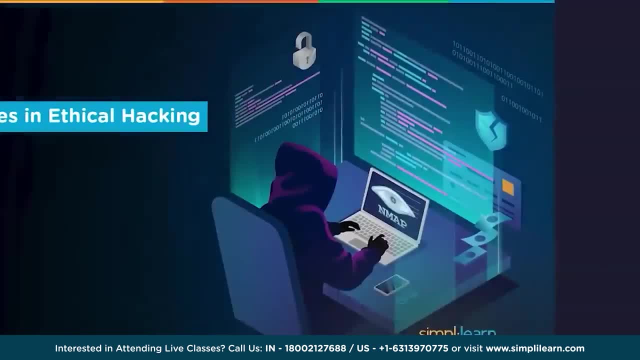 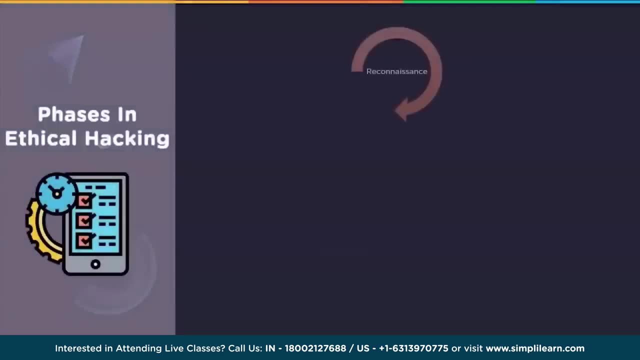 in shedding light on the topics being taught today. Let us first understand where and why Nmap is essential. There are essentially five phases in ethical hacking. The reconnaissance phase is the first phase of the penetration test. Here the security researcher collects information about the target. 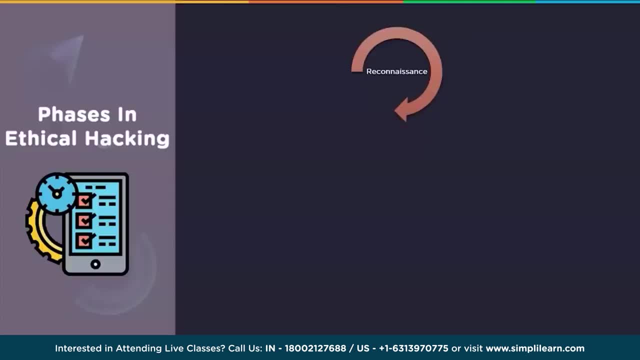 It can be done actively or passively, or both. It helps security firms gather information about the target system, network components, active machines, etc. This activity can be performed by using the information publicly available and by using different tools. The scanning phase is more. 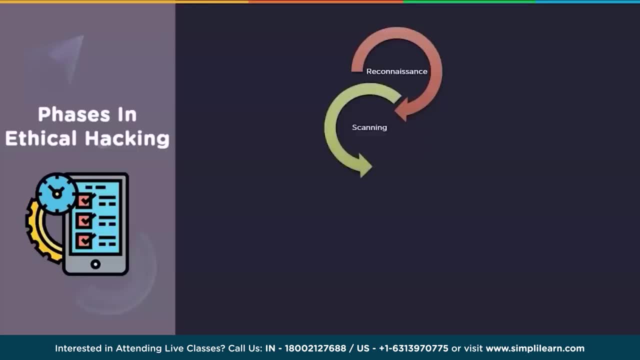 tool-oriented rather than being performed manually. The tester runs one or more scanner tools to gather more information about the target. By using various scanners, such as wall dialers, port scanners, network mappers and vulnerability scanners, the penetration tester collects as many vulnerabilities. 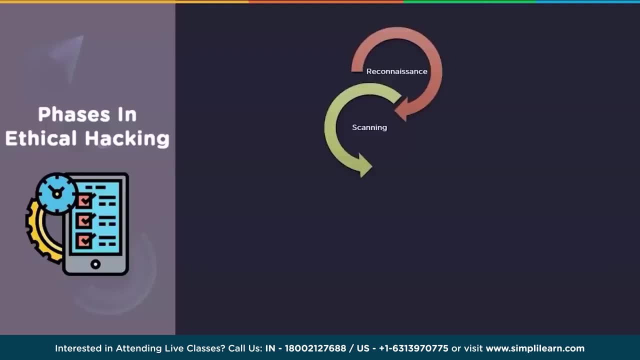 which help in turn to attack a target in a more sophisticated manner. In the gaining access phase, the penetration tester tries to establish a connection with the target and exploit the vulnerabilities found in the previous phase. The exploitation may be a buffer, overflow attack. denial of. 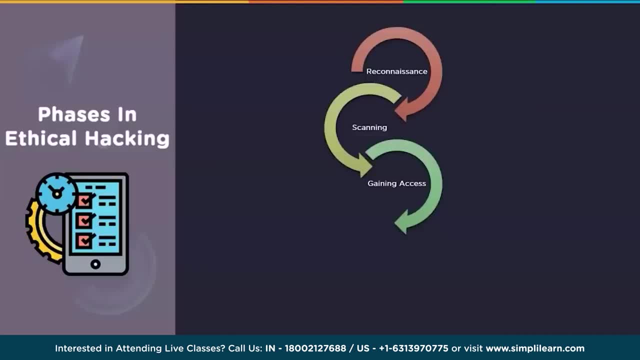 service attack, session hijacking and many more. Basically, the penetration tester extracts information and sensitive data from the servers by gaining access with different tools. In the maintaining access phase, the penetration tester tries to create a backdoor for himself. It helps him to identify hidden vulnerabilities. 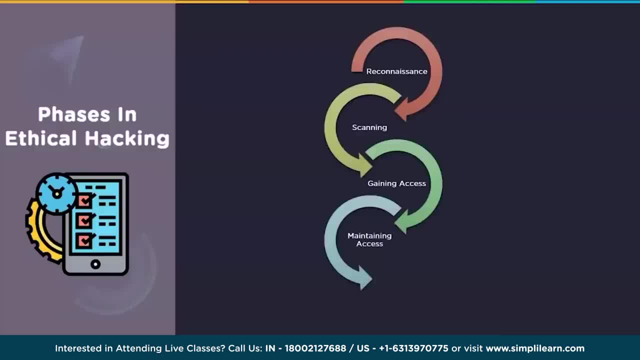 in the system, while allowing him to come back to the system to retrieve more data further on. In the clearing tracks phase, the tester tries to remove all logs and footprints which might help the administrator identify his presence. This helps the tester to think like a hacker. 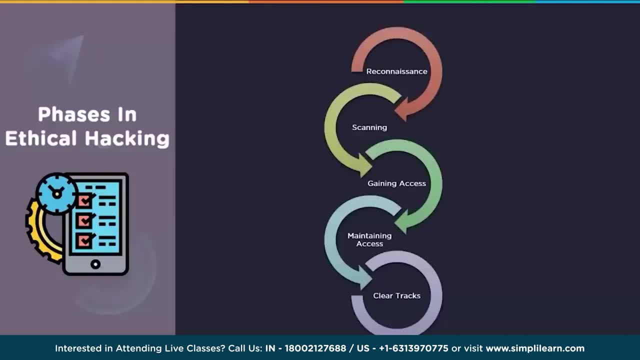 and perform corrective actions to mitigate those activities. Nmap is most beneficial in the early stages of ethical hacking, where a hacker must figure the possible entry point to a system. It is necessary to know this before running the necessary exploits, thus allowing the hackers to leverage any 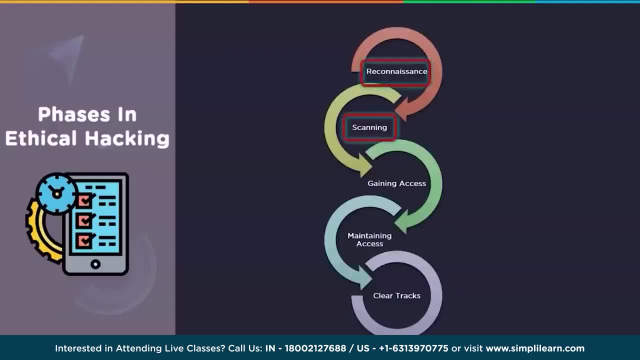 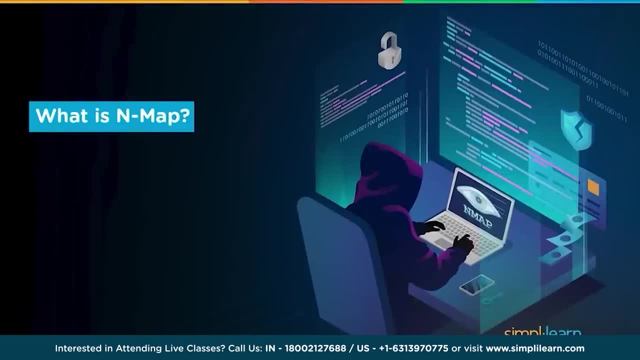 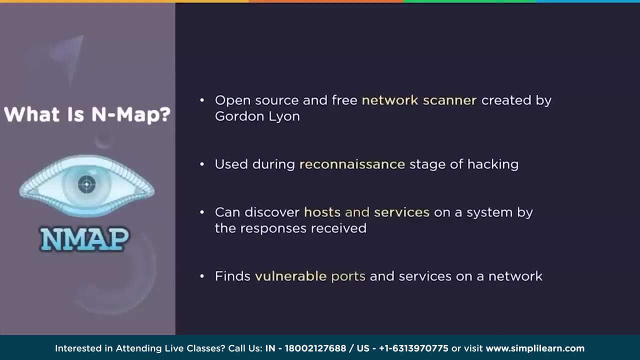 insecure openings and breach the device. So the reconnaissance and the scanning phase are the points where Nmap finds the most use. Let us now understand what Nmap is from a layman's perspective. Nmap, which stands for Network Mapper, is a free and open source utility. 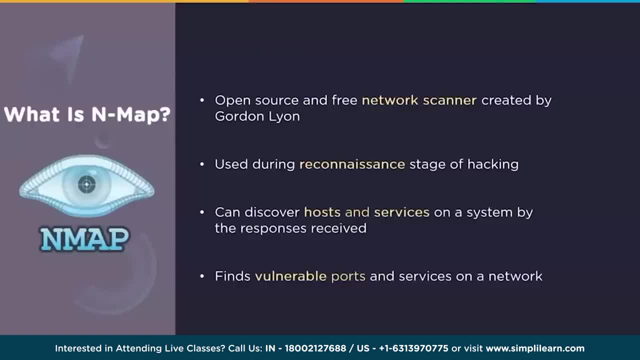 for network discovery and security auditing. Many systems and network administrators also find it useful for tasks such as network inventory, managing server upgrade schedules and monitoring host and service uptime. The program is most commonly used via a command line interface and is available for many different. 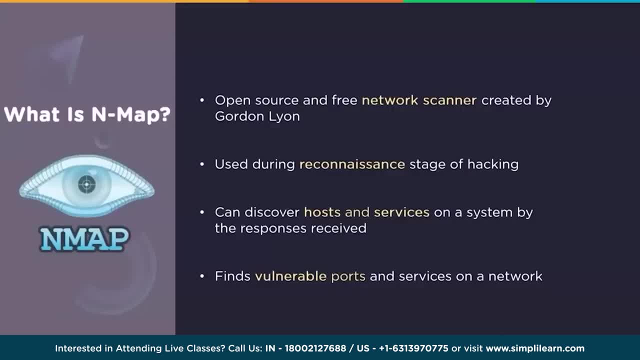 operating systems such as Linux, FreeBSD and Gentoo. It is most beneficial in the early stages of ethical hacking, where a hacker must figure the possible entry point to a system before running the necessary exploits. Nmap was developed for enterprise scale networks and can scan through thousands. 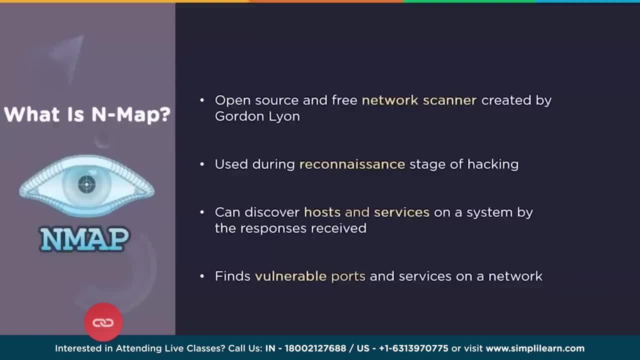 of connected devices. However, in recent years, Nmap is being increasingly used by smaller companies as well. Nmap uses raw IP packets in novel ways to determine what hosts are available on the network, what services these hosts are running, what type of packet filters. 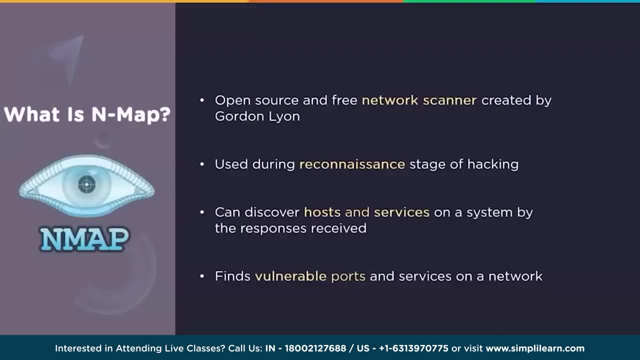 and firewalls are in use, and dozens of other characteristics. It was designed to rapidly scan large networks, but works fine against single hosts as well. The rise of the IoT in particular now means that networks used by these companies have become more complex and therefore harder to secure. 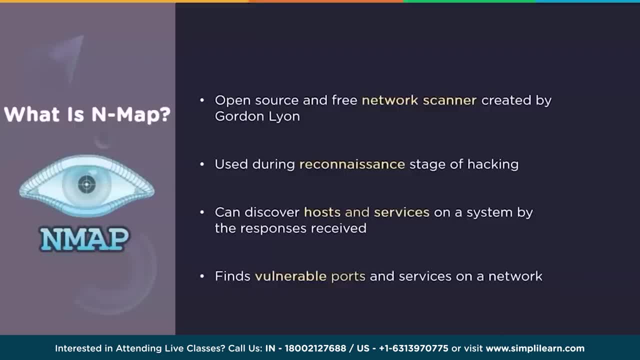 Since every application that connects to a network needs to do so via a port, the wrong port or server configuration can open a can of worms that leads to a thorough breach of the system. However, IoT botnets like Mirai has also simulated interest in Nmap, not least. 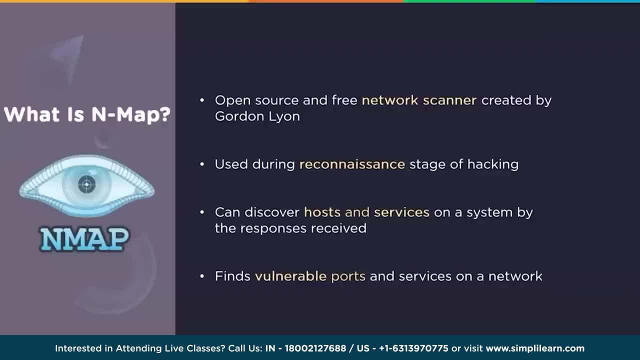 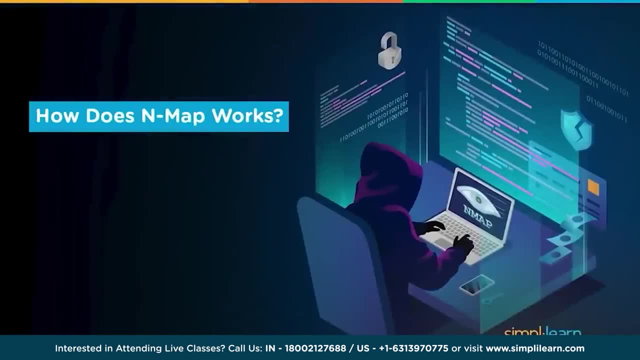 because of its ability to interrogate devices connected via the UPNP protocol, but also to highlight any devices that may be malicious. Now that we understand what Nmap is, let us take a look at the workflow of how an ethical hacker uses this tool in penetration testing. 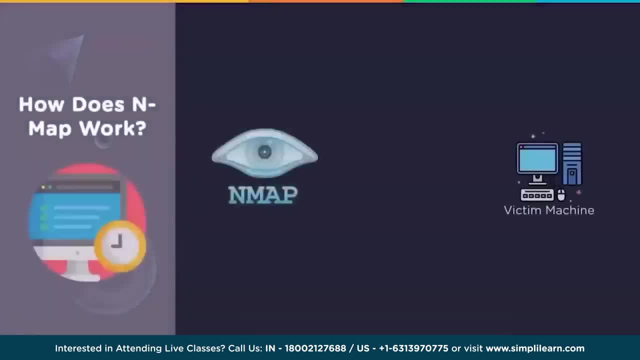 At a practical level, Nmap is used to provide detailed, real-time information on your networks and other devices connected to them. We have the hacker running Nmap on his system with the victim machine running a standard installation of the operating system, be it Windows. 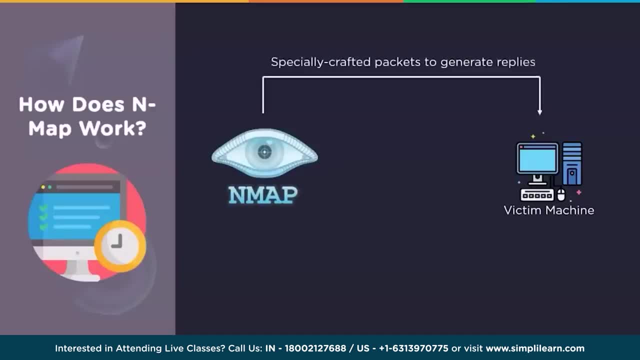 MacOS or Linux. The Nmap interface will send specially crafted packets to generate some reply from the victim machine. The victim machine in return will send some information back to the Nmap host with replying some of the services and hosts that are being run on the computers. 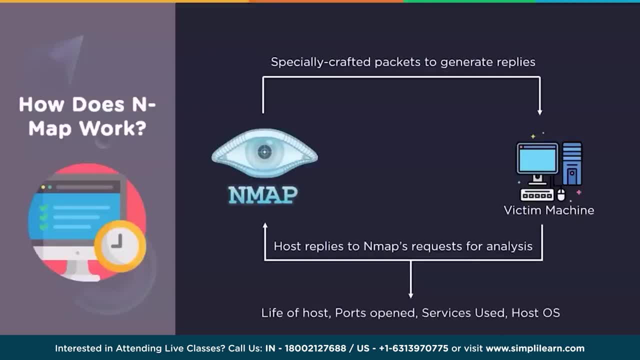 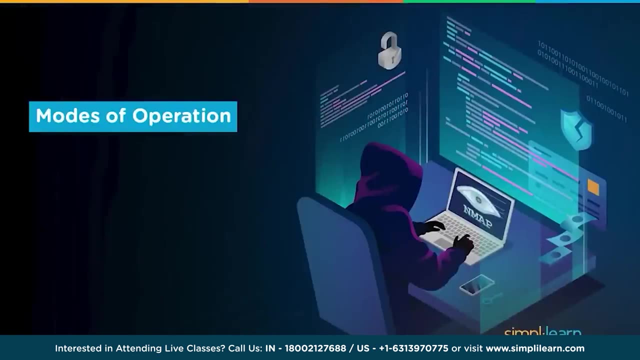 Nmap allows the network admins to find which devices are running, discover some open ports and other devices. This in turn helps discover the vulnerabilities and the possible entry points for hackers to breach into. We are now aware of how Nmap works on a basic level. 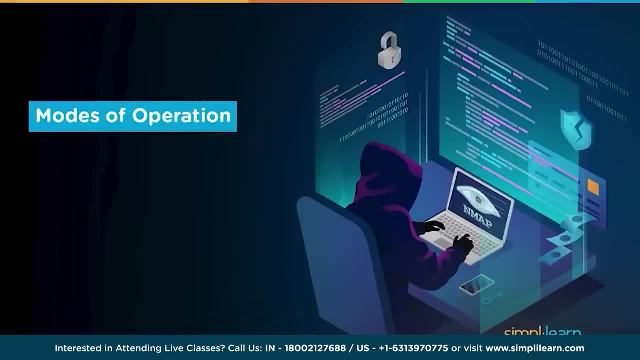 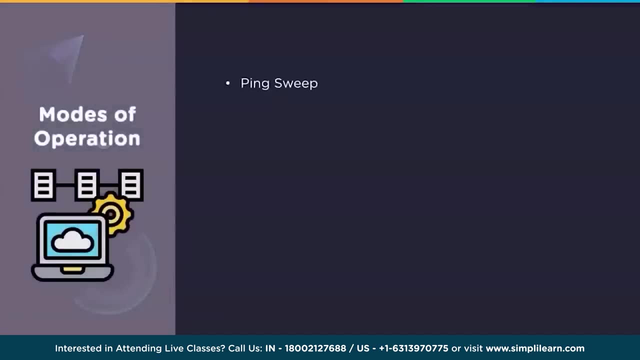 but there are many varieties of scans that users can run on local machines. Let's take a look at some of them. The Ping Sweep is a simple type of Nmap scan where it pings to all the available IP addresses to check which IPs respond to ICMP protocol. 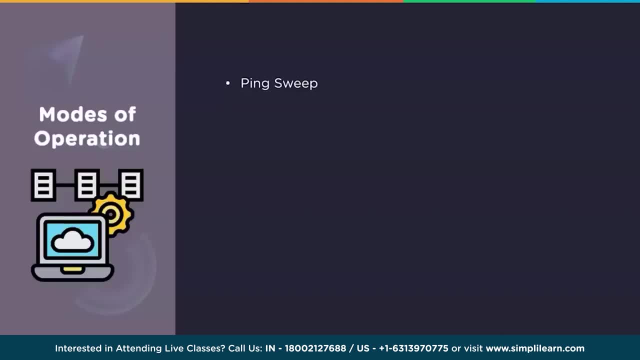 If the users need to know only the number of IP addresses and not many details, the Ping Sweep is very useful. It's fast and hence the results to be known are fetched very easily. The SYN scan is the most useful type of Nmap scan. 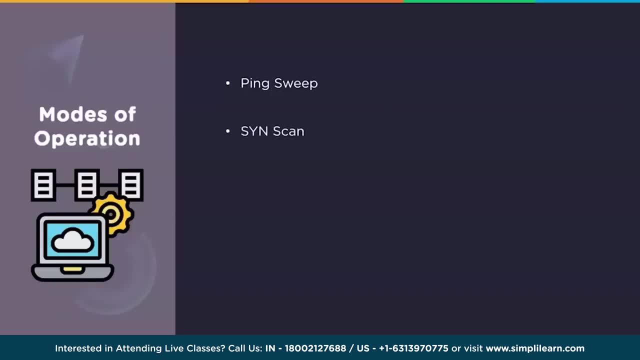 which does work very quietly. It sends an SYN packet via the TCP protocol or the transfer control protocol to all the intended ports. If an acknowledgement pack is received to the system, it is sure that a port is opened there. No response means that the port is either closed. 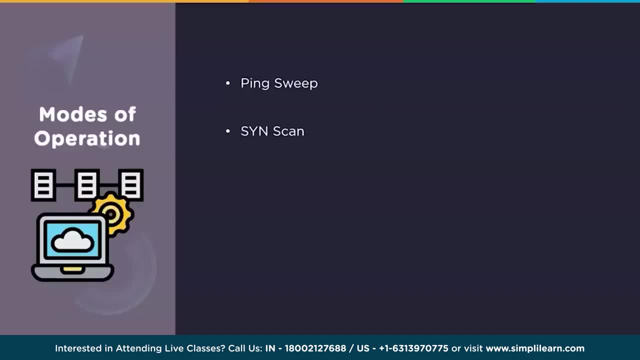 or not available Here. the acknowledgement pack is not sent back to the system, assuming that the connection is not valid. The scan is not shown in most of the scan logs and hence it is safe to use SYN scan to identify the open ports. 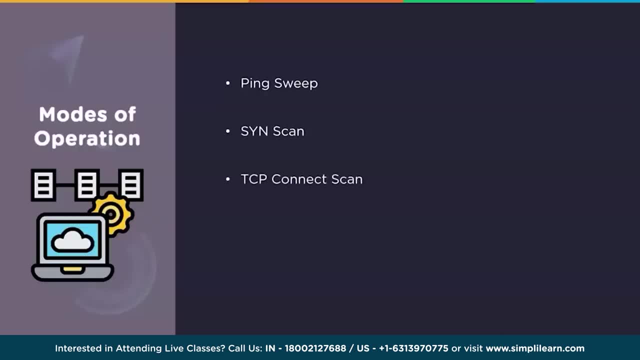 The TCP connect scan is similar to SYN scan in many aspects, as it uses the TCP layer to send packets and is passed to all the ports. Here the difference is that the full connection is done by sending the acknowledgement packets back. The logs can easily find the. 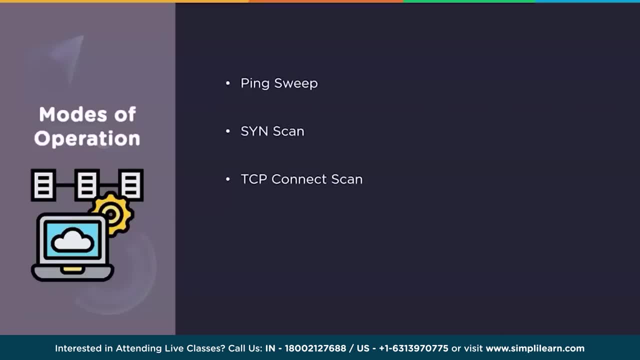 TCP scan and need more power from the machines to do the work, But it is more accurate If all the accesses related to the OS are available to the user. it is better to do a TCP scan than an SYN scan, as all the low level and 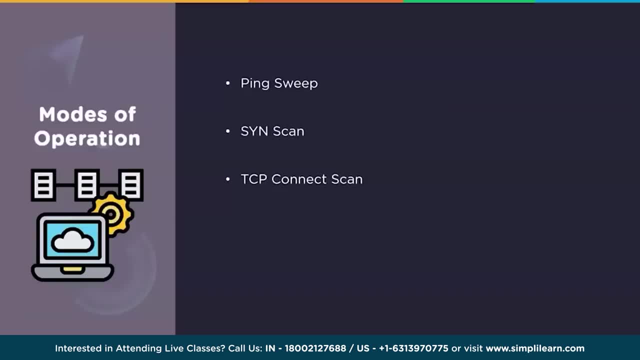 high level accesses are required for the scan. The network is also loaded more, and hence users must be careful about overloading the system and the networks. The idle scan is really used to check whether any malicious attacks are planned on any particular network. Users need not control the 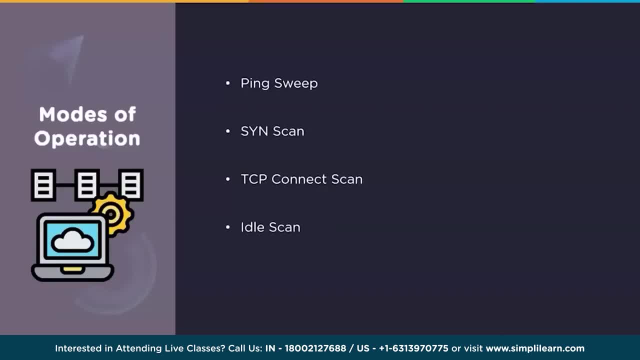 external host, but an IP address and a port should be given to the same. All other requirements are taken from the scanner itself. The RPC scans, or remote procedure calls, are done by hackers to make the system vulnerable to virus attacks. It is thus necessary to know whether 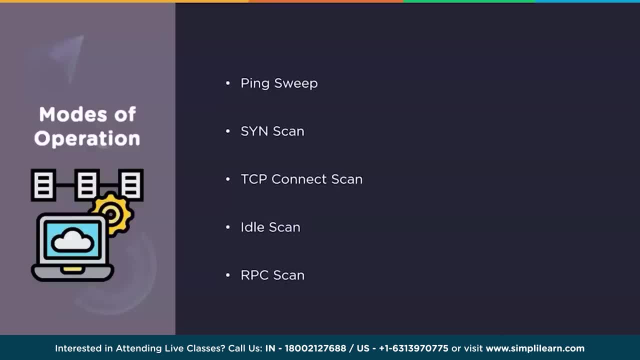 our systems, answer such calls and make our system open to malware. RPC scan is done to check this by finding the ports open with certain commands being run by RPC. The Windows scan is a simple scan where the application scans the acknowledgement packets received from the ports. 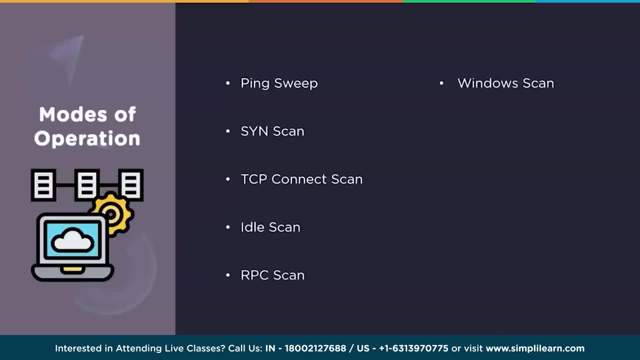 once the SYN packets are sent. If there are any abnormalities in the ACK packets received, the scan reports the same and helps in recognizing which ports are functioning in a different manner. The bound scan is used to check the security in the file transfer protocol layer. 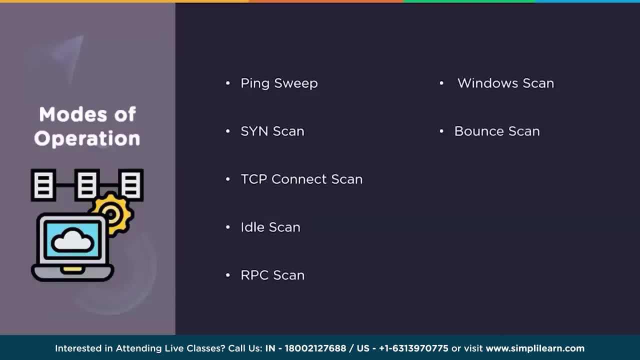 FTP layers mostly do not accept any packets and once it is rejected from the FTP layers, there are chances that it might be sent to an internal layer so that it can access the internal machines. Bound scan checks this loophole by doing exactly the same process and 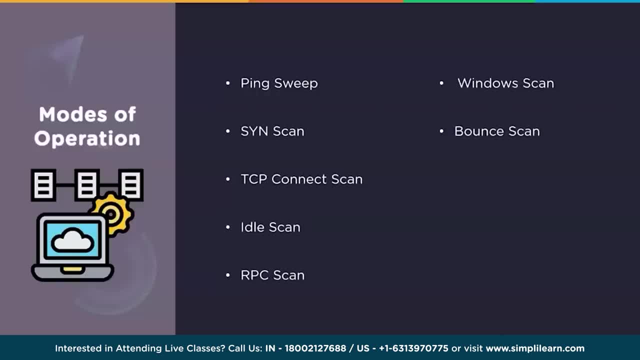 identifies whether a FTP layer is open to vulnerability or not. The FIN scan is similar to SYN scan, where the system that sends the packets receives the response back and it will mostly be a TCP FIN packet. If the system sends an RST packet, it is a false alarm and users 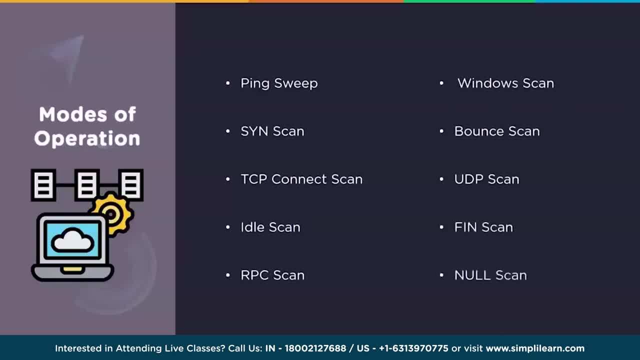 need not be worried about the same. The Null scan is useful for other systems than Windows, Where the systems can easily identify what kind of packets they have received and respond back with either TCP packets or Null responses. Null scans are not useful for Windows, as they. 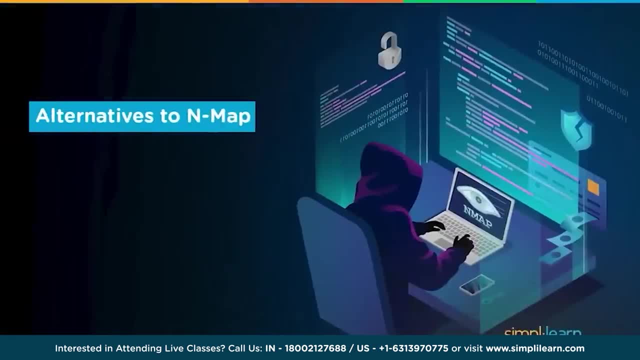 may not always produce the desired results. When it comes to looking at alternatives, there is a wide range of free network monitoring utilities, as well as free open source vulnerability scanners available to network administrators and security auditors. What makes Nmap stand out as a tool? IT and network. 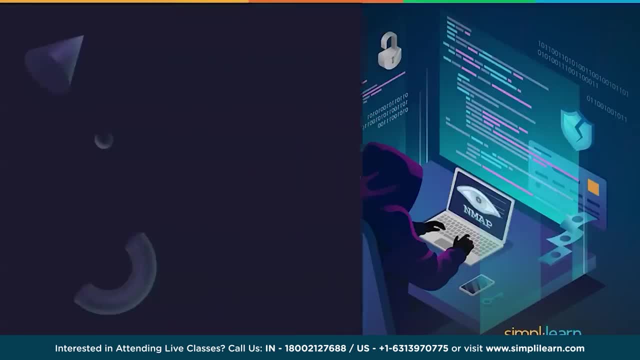 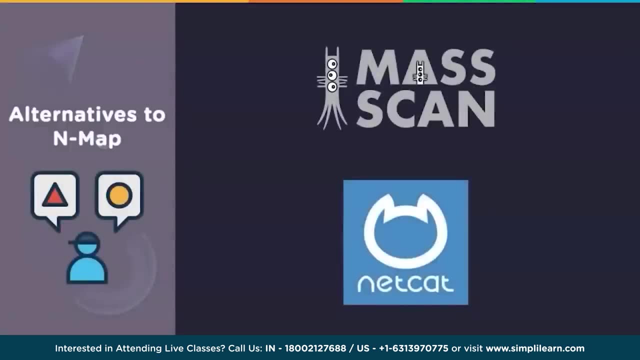 security managers need to know is the flexibility and power. There are some alternatives to Nmap, but most of them are focused on providing specific niche functionality than the average system administrator does need frequently. Mass scan, for instance, is much faster than Nmap but provides less detail. 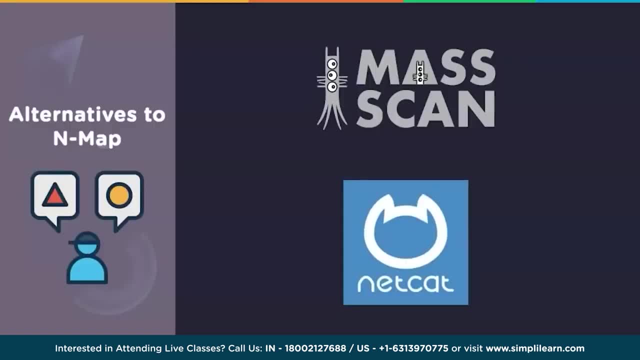 In reality, however, Nmap provides all the functionality and speed that the average user requires, especially when used along with other similar tools like Netcap, which can be used to manage and control network traffic, and Zenmap, which provides a graphical user interface for Nmap. 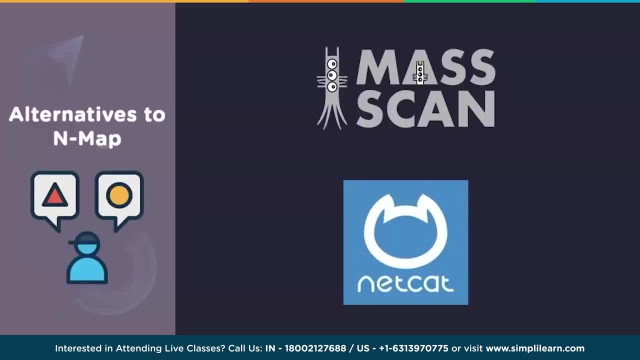 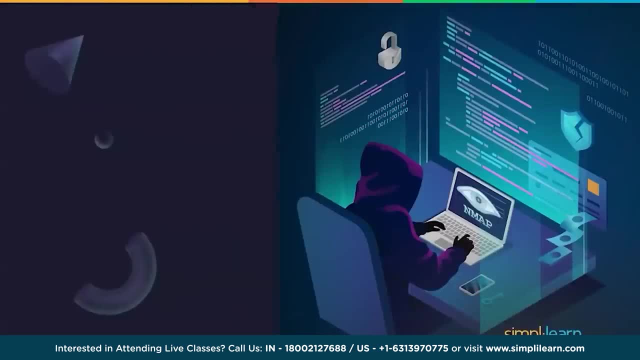 But as an all-rounder solution to network scanning. nobody can go wrong with Nmap as their tool of choice. Let's now take a tour of Nmap based on all the things we have covered today In this live demonstration. we start by: 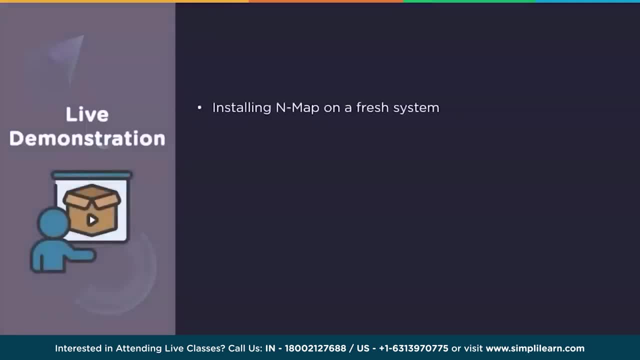 learning of how to install Nmap on a fresh operating system that doesn't come pre-installed with the tool. We also cover the different types of scans that can be run on local machines, along with checking multiple inferences an ethical hacker can gather based on the 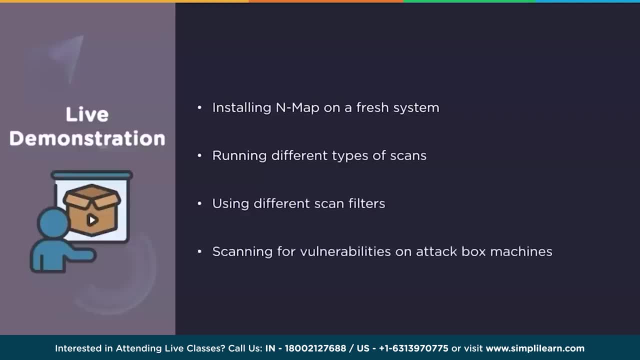 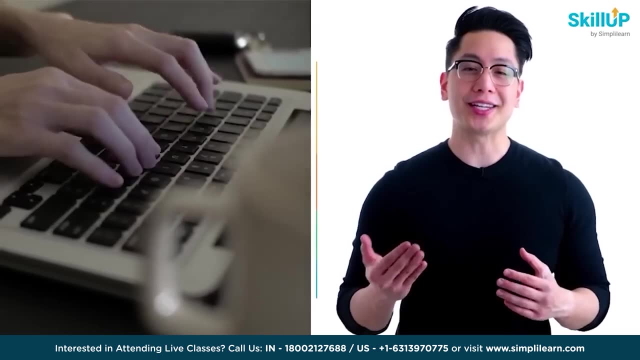 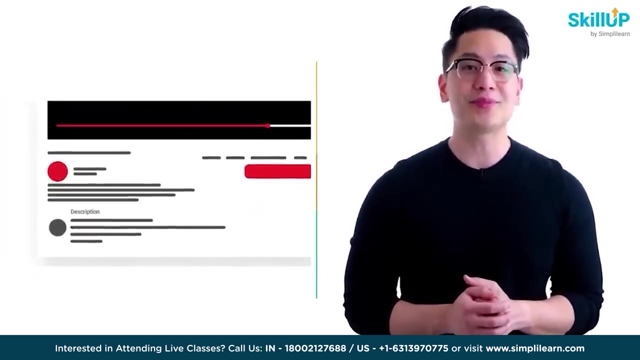 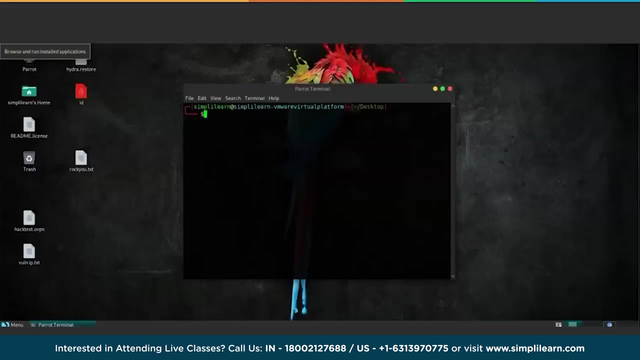 output of an Nmap screen. Finally, we run scans on vulnerable machines to get an idea of how to proceed with the outputs we gather using this tool. The first step in our demonstration is installing Nmap. Now it depends heavily on what Linux distribution you are going to use to 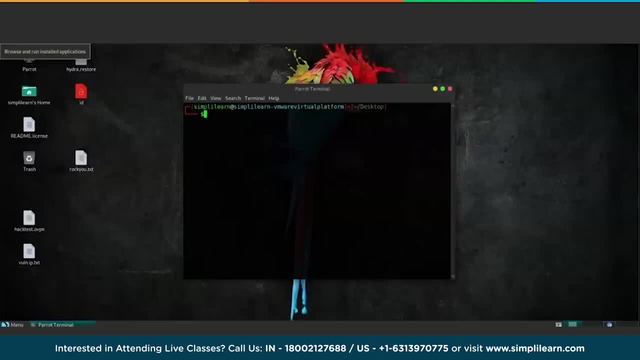 perform ethical hacking. For example, I am using Parrot Security operating system. If you are not aware of what Parrot Security is, or even what Kali Linux is, we highly suggest that you check out the videos of those two operating systems on our 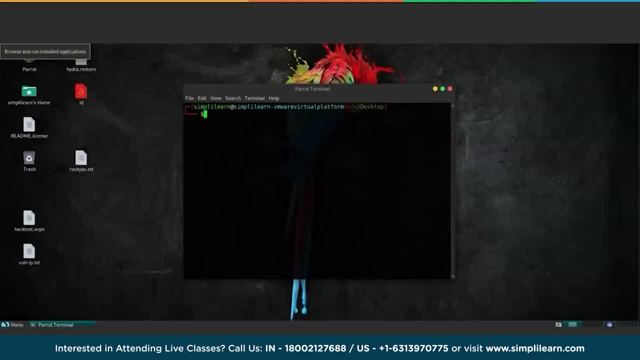 YouTube channel so that you can get a fair idea of what they serve. Now, if you are using any of these two operating systems, Nmap should come pre-installed by default. To check if Nmap is pre-installed or not, you can just press on. 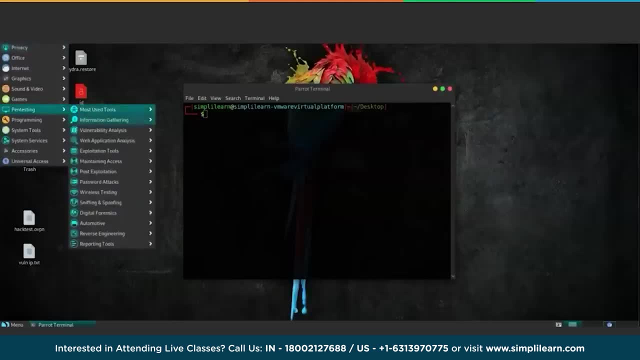 applications over here. Go to the pentesting section, Go to this information gathering tab And you should be able to see Nmap right here. Now, let's say you do not have Nmap pre-installed. Maybe you are using a Linux distribution. 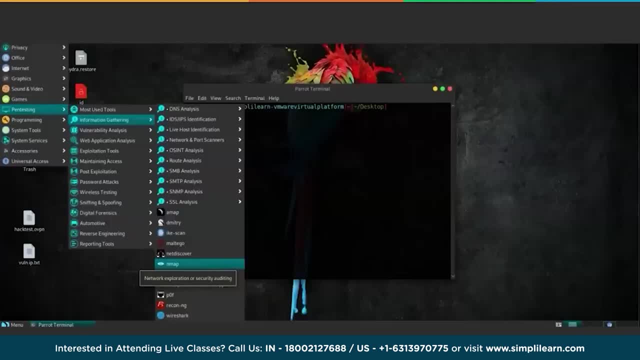 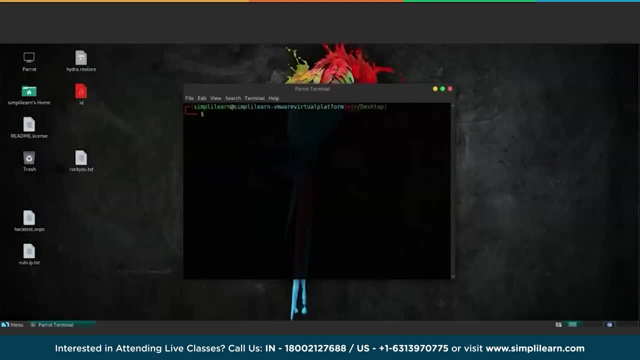 like Ubuntu or Linux Mint or something that is based on Debian operating systems. One thing: you have to make sure that Nmap should be in the distribution repository. Once you check that, or even if you do not know if it is present, you can just 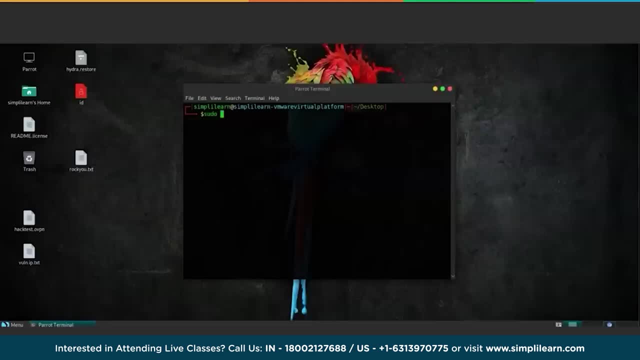 this command It should be install, which is to give root permissions for installation APT. APT is the package manager of all Linux distributions that are based on Debian. That goes for Debian, stable Ubuntu, Linux Mint, Kali, Linux, Parasecurity. 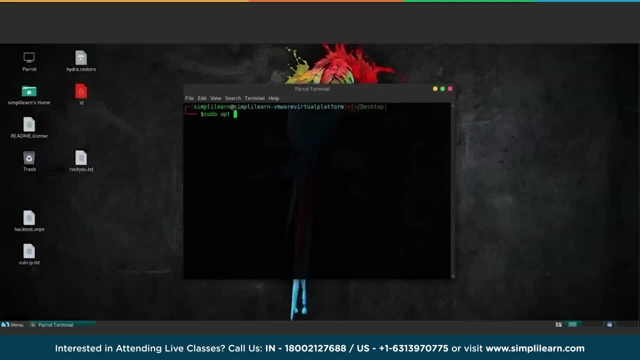 and anything of that nature. APT is the package manager which handles the installation and removal of applications in these specific operating systems. Once you are here, just write install and Nmap Press enter and it's going to ask you for the root password. 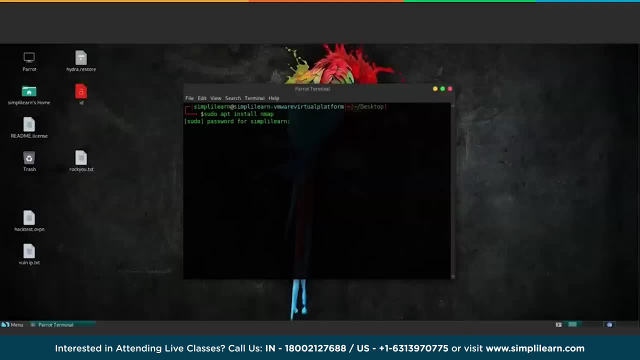 that you set when you install the operating system in the first place. Enter your root password and press enter again. As you can see, it's saying that Nmap is already installed. the newest version, since I am running Parasecurity operating system Now, should. 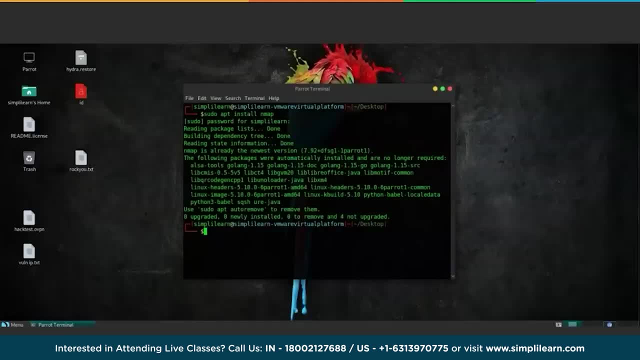 you be running this operating system, or even Kali Linux, you should receive a similar message and the installation is already done. If you are using some other distribution, let's say even Blackhawks, Arch Linux or Manjaro, anything like that, the installation steps. 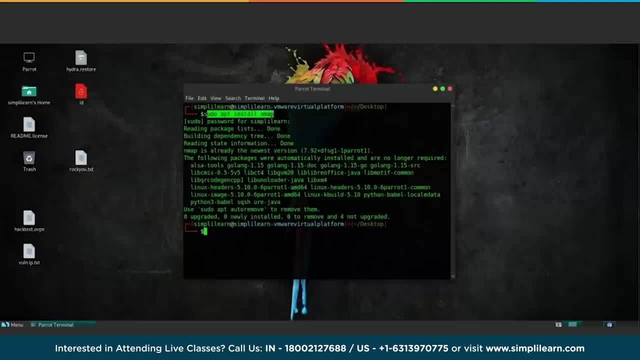 will be slightly different. This sudo apt install nmap command is for distributions that are derived from Debian and Ubuntu. If you want to install in Arch Linux based distributions, you have to use their package manager, which is known as PAMAC, But that is for a different step. 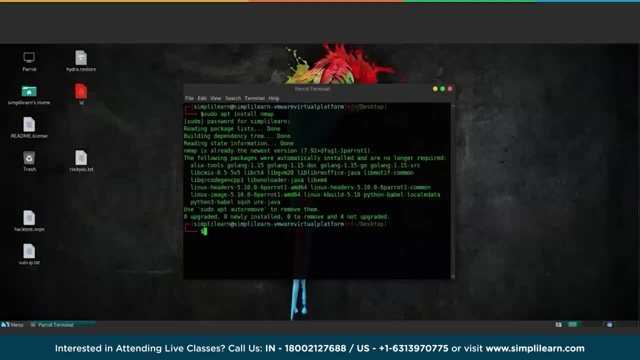 and if you want to get ethical hacking, the best way to start is by learning either Kali Linux or Parasecurity. Now that the installation is done, we are going to learn how to use Nmap, One of the most basic functions of Nmap. 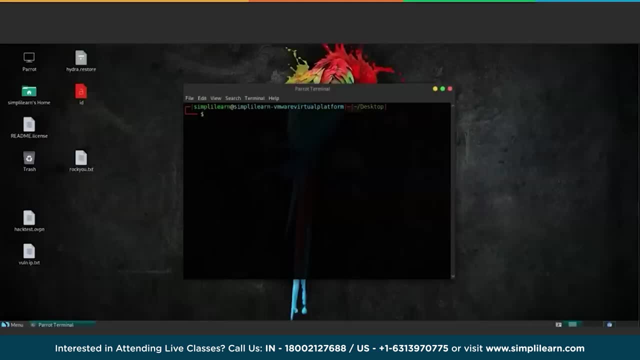 is to identify active hosts on the network. We can do this by using a ping scan. The ping scan identifies all of the IP addresses that are currently online without sending any packets to these hosts. Now, to run the ping scan, we are going to write Nmap. 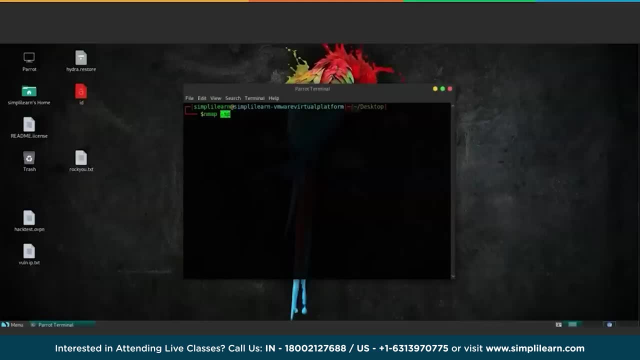 The flag we are going to mention over here is SP. Now, these flags are the different traits of the Nmap scan. Depending on what flag we use, we can send different kinds of requests to the host that we are scanning Before moving forward with this. 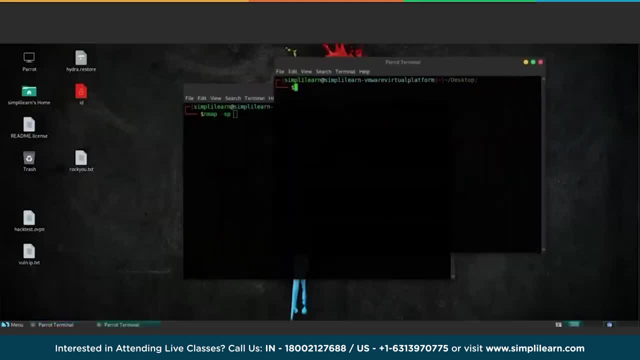 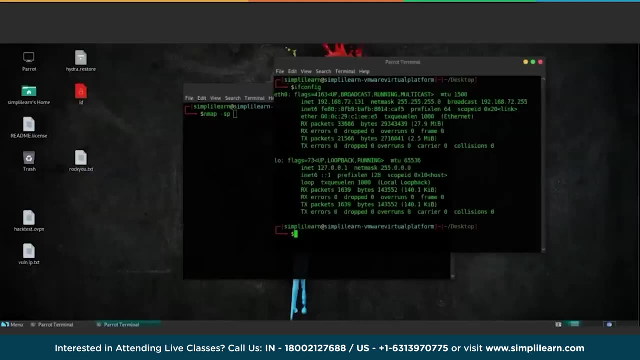 let me open another terminal over here and check the IP address. We are going to write the command ifconfig and find the subnet in which this system is present. As you can see, the IP address is 192.168.72- 192.168.72.131. 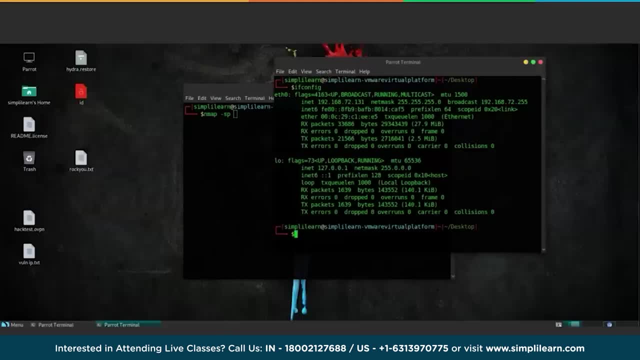 Now this operating system is being run on a virtual machine software known as VMware. The VMware in itself is running on a Windows 10 operating system. Considering they are now a part of the local network, this IP address is of parent security and the Windows operating system, which is the 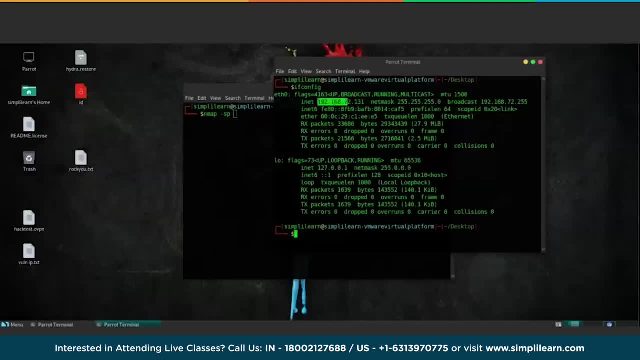 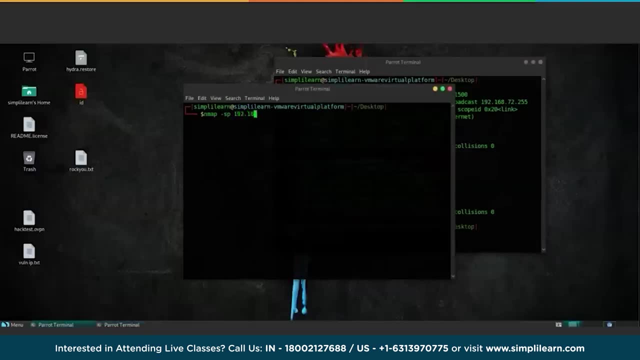 host system, in my scenario, will fall in this particular subnet. So to run our scan we are going to target 192.168.72.1-24, 192.168.72.1-24, 192.168.72.1-24. 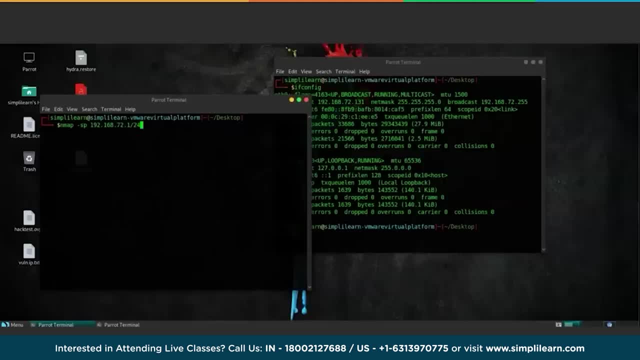 192.168.72.1-24. 192.168.72.1-24. This command then returns the list of hosts on your network and the total number of assigned IP addresses. This is going to be capital P. Yeah, If you spot. 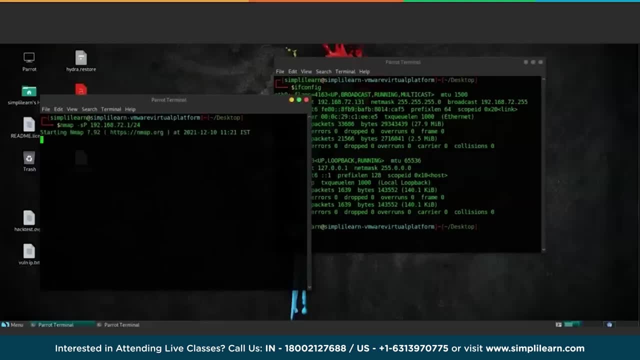 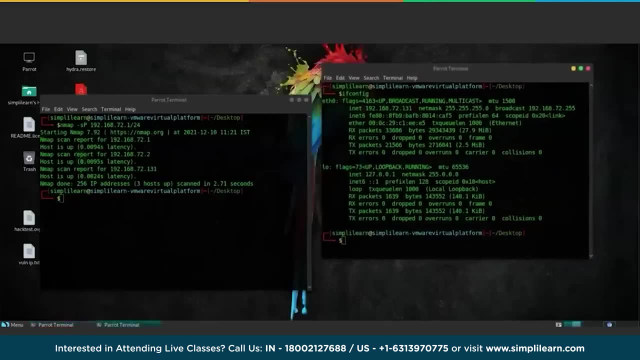 any host or IP addresses on that list that you cannot account for. you can then run further commands to investigate them further. As of right now, you can see the machine that is the parent security. This IP address can be detected in the subnet. 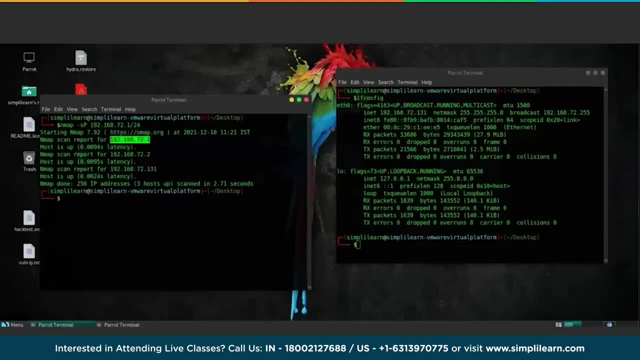 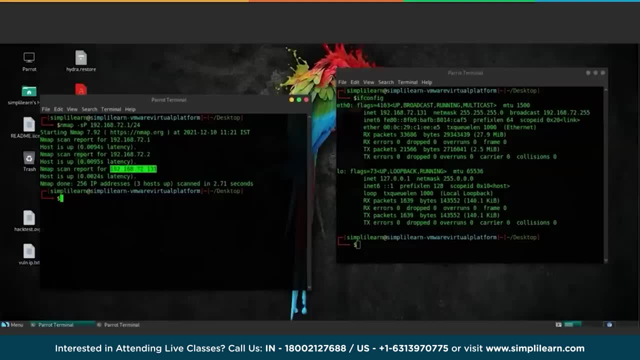 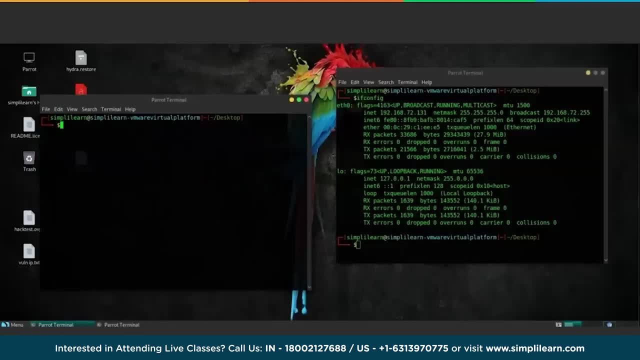 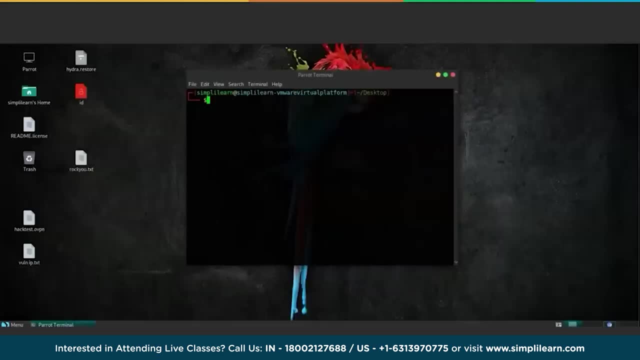 We're going to clear our terminal and we can close this. actually, When scanning hosts, Nmap commands can use server names, IPv4 addresses or IPv6 addresses. A basic Nmap command will produce information about the given host. To run a basic port scan we can just use. 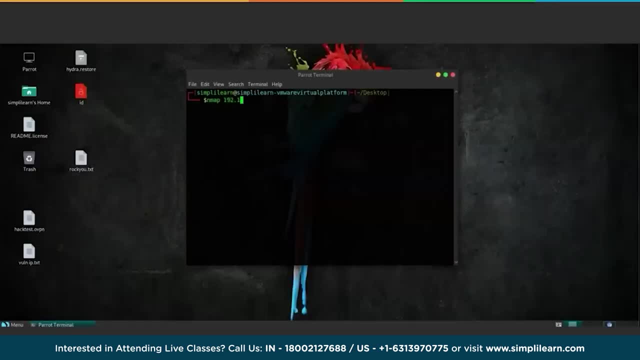 Nmap, along with the IP, Now, as you remember, the IP 192.168.72.1. This is the IP of my local Windows 10 machine. As you can see, it shows the ports that are opened and the particular servers that these ports are running. 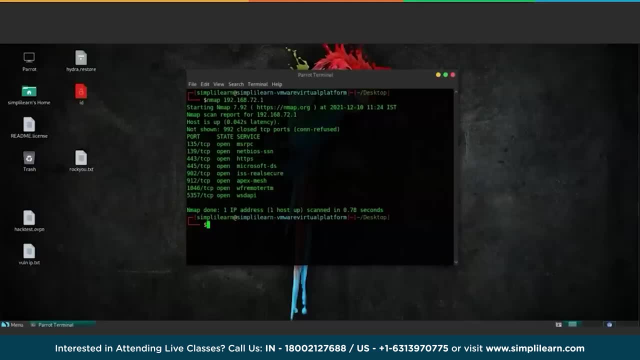 Now we can also have a detection of the operating system. Now, mind you, this is not 100% correct and the reliability depends on the location and what kind of fingerprinting measures are available. Now, since this does TCP IP fingerprinting, it needs some extra permissions. 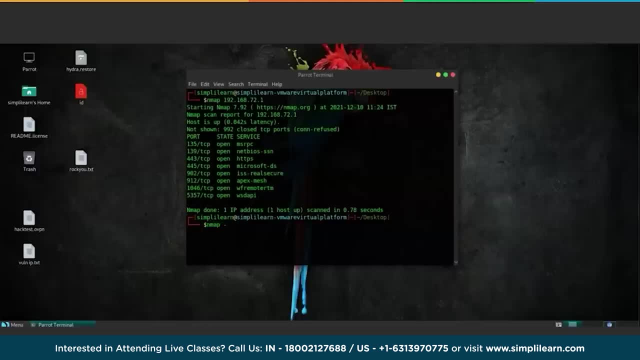 The flag that we are going to use is Nmap minus O, along with the same IP address. Like I said, since this does TCP IP fingerprinting, it requires root privileges. Now, to provide root privileges, we're just going to add the Nmap. 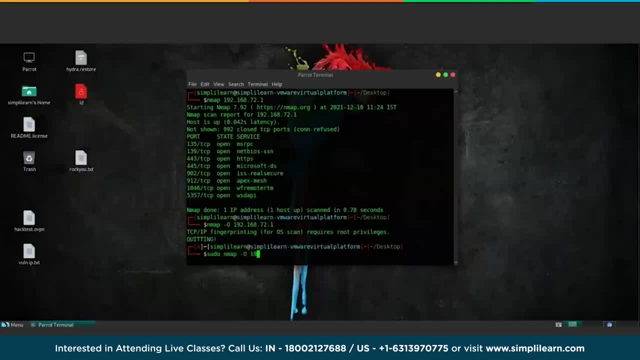 and a sudo keyword Going to repeat the same command that we wrote above. As you can see, it has successfully detected that I am running Microsoft Windows 10 with this MAC address. It has also shown the correct build number of the Windows 10 system that I am using. 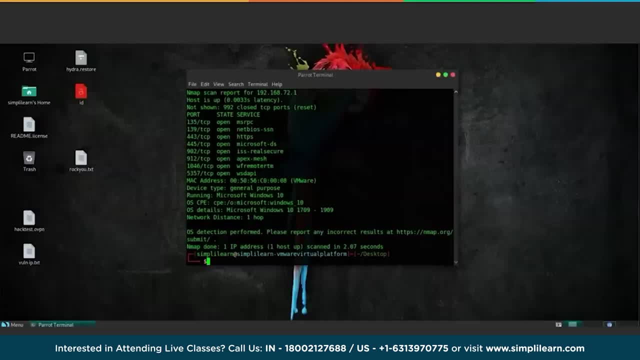 This is useful for troubleshooting, scanning vulnerabilities or even locating some services that need to be updated. Now, to get the necessary information about these services, for example, what versions they are using, we have a command known as sv, which stands for service version. 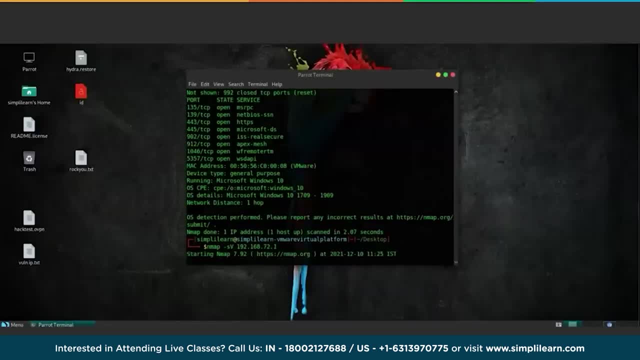 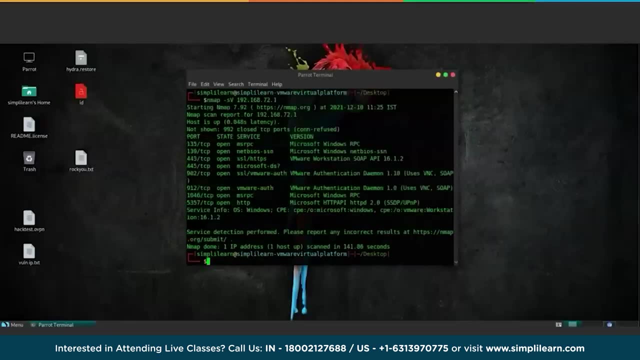 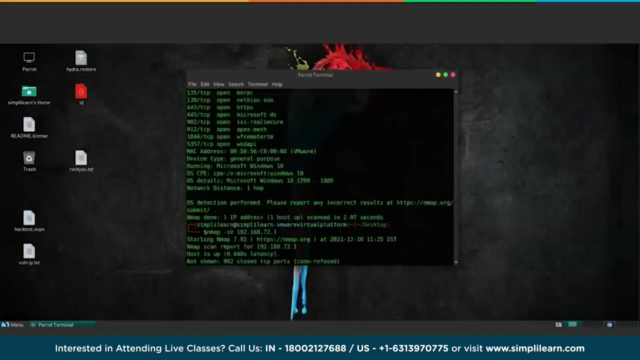 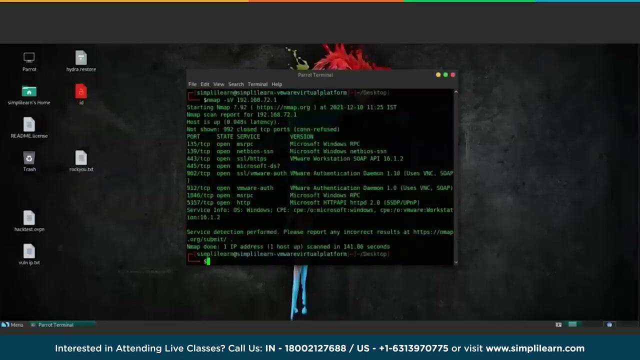 We use the same IP address and press enter. Now, as you can see, the scan is complete and if you can check the results of the scan above here we don't see any version number for the services. Here we can actually check. 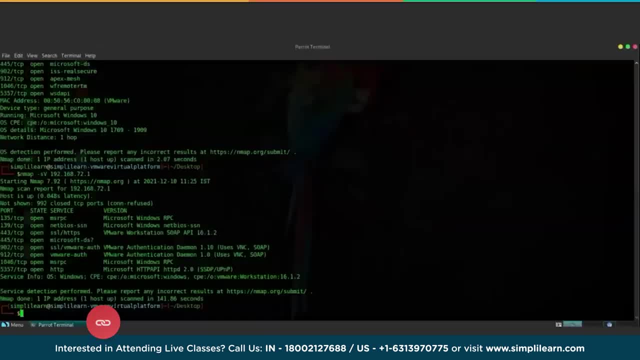 what version they are running Now. this becomes helpful when we are trying to find specific versions to exploit. For example, if VMA Workstation 16.1.2 had some particular vulnerability, we can exploit it by checking this command. Apart from the, 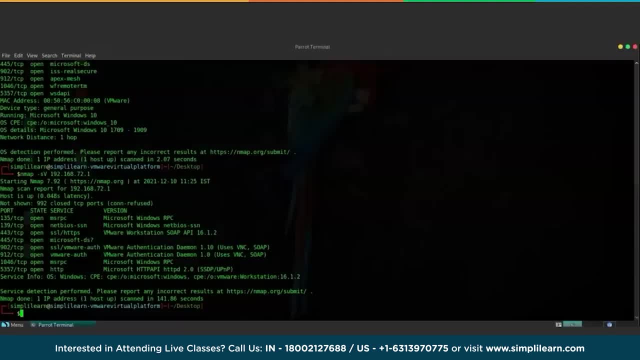 host scanning- port scanning- is one of the most basic utilities. There are a few ways that this command can be customized as well. For example, I have already checked that the 443 command is open, but I have found out after running this lengthy. 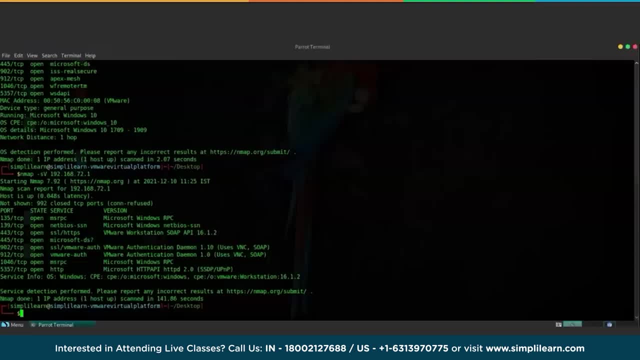 scan. let's say I only want to check if the port 443 is open. In math I'm going to use the flag of "-p", which stands for port, and give 443 as an argument here, using the same IP address. 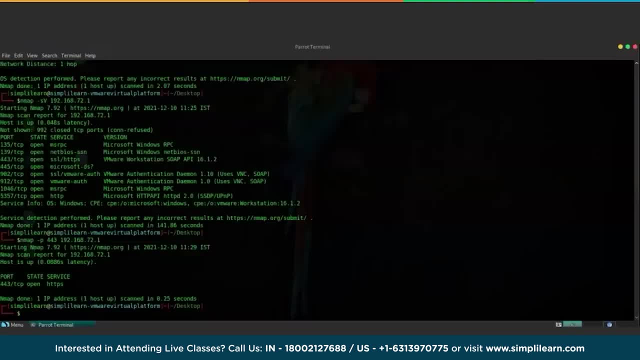 And you can see it says it's open, But we already knew it is open. Let's say there was something else. Let's say we're going to scan if the Apache web server port is open, which usually runs on 80.. Obviously, since I'm not running, 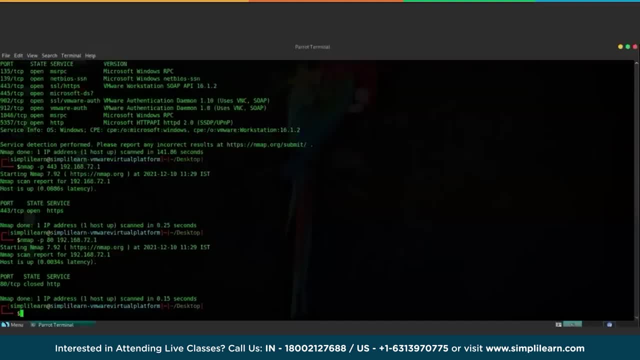 an Apache web server, it says it's closed. Now we can combine these two commands by running both simultaneously. To do that, we can just put a comma and complete the rest similarly, As expected. 80 is closed and 443 is open. 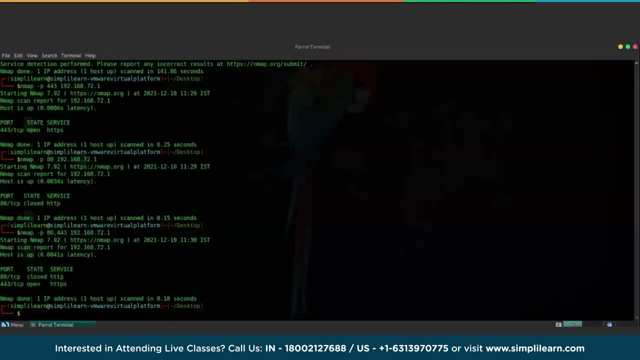 Another feature of Nmap for port scanning is showing off ranges. Now, ranges can be beneficial when you're trying to see up to a certain limit. For example, Nmap "-p": we're going to check what ports are open between 100 to, let's say, 2000.. 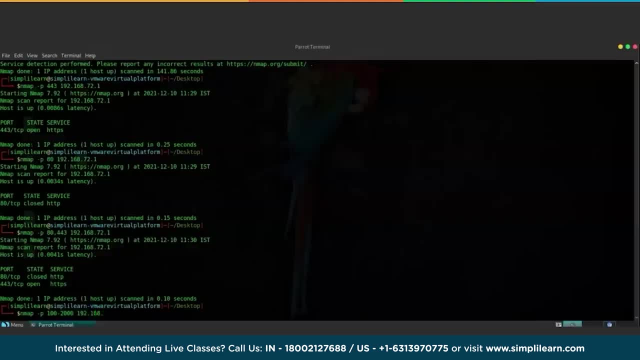 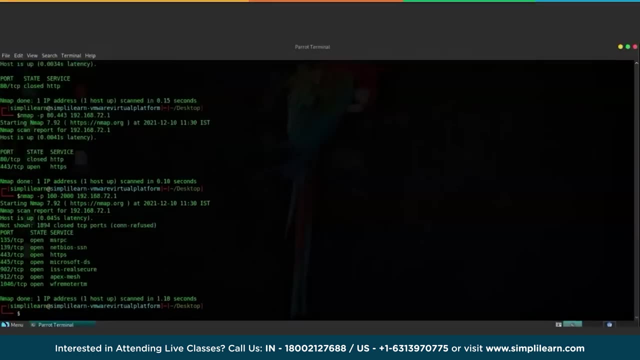 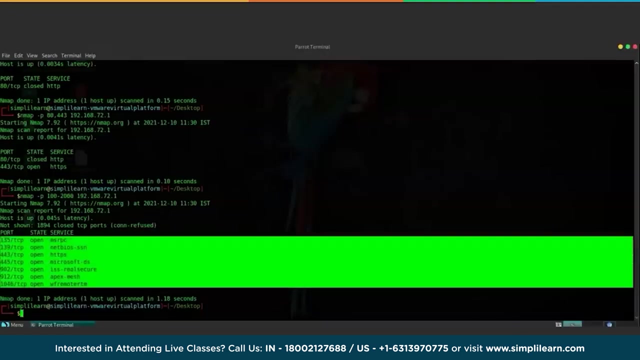 This acts as a range. Everything else is the same- And it checks all ports in the range of 100 to 2000.. Whatever ports is open in between that range, it can be mentioned over here. We're going to clear the screen now. 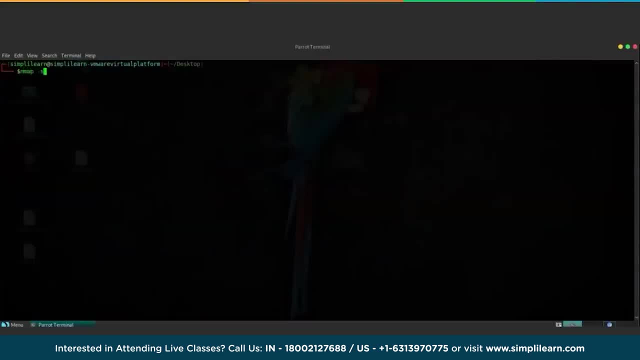 Another flag that can be used with Nmap is the ss command. This runs a stealth scan which is a little harder to detect if you're the IT admin of the system that is being scanned. The results will more or less be the same, although this: 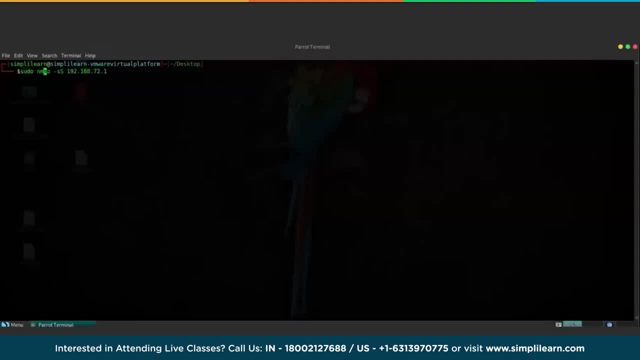 will need elevated root privileges 2.1. As you can see, this is more or less similar to a port scan. It just adds an extra mac address as well for good measure. But, like I said, it's more about the stealth. The normal scans usually. 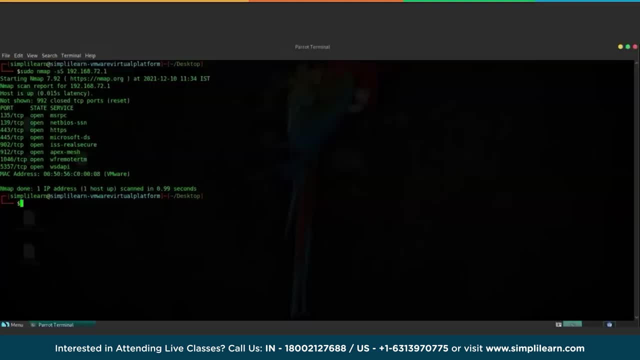 are easier to detect when the logs are being checked. Stealth scans are relatively tougher to check On much more intricate systems. this takes longer as well. Now that we're done with port scanning, let's look at a vulnerable machine: The system that we're scanning. 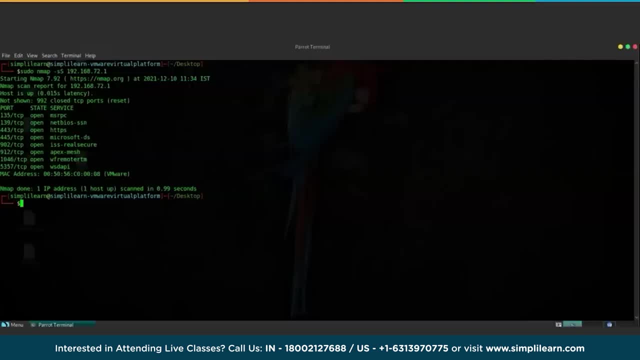 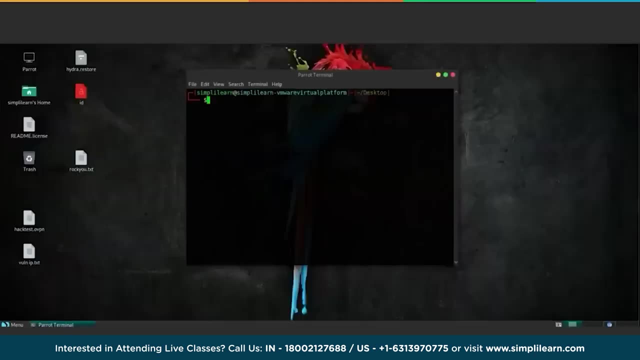 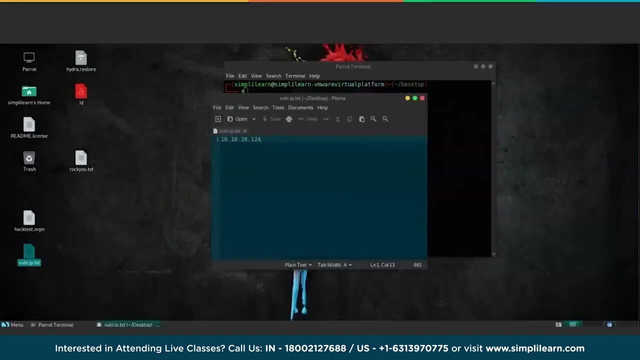 right now is my own personal system, with everything pretty locked down as much as it can be. There is an attack box running in the cloud, the IP address of which is over here. Now, to be able to get into this network, we need to. 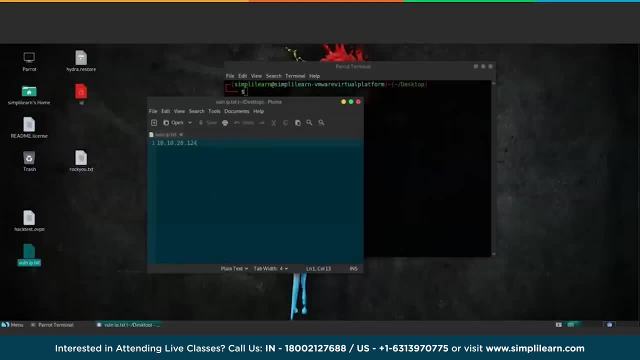 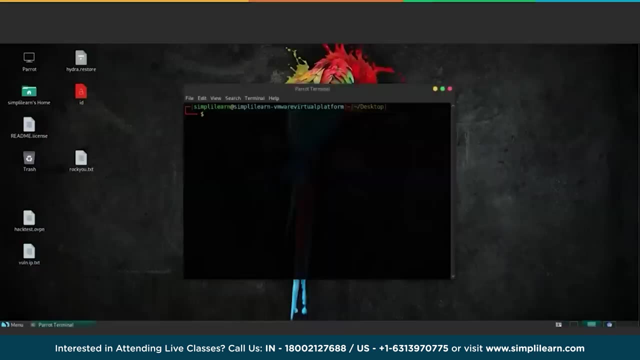 connect to their personal network using a VPN. So what I'm going to do is switch to a different workspace over here. I'm going to open a terminal and, if you can see, over here there is a hacktestovpn file I'm going to connect to their. 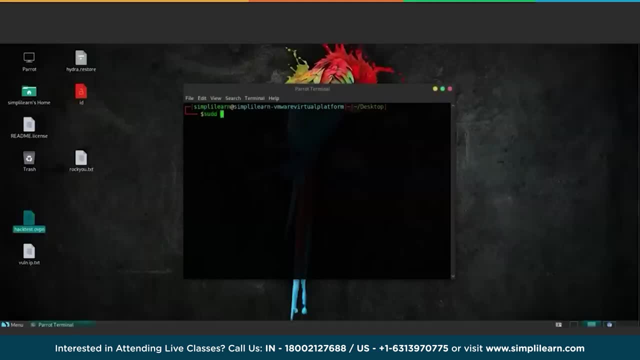 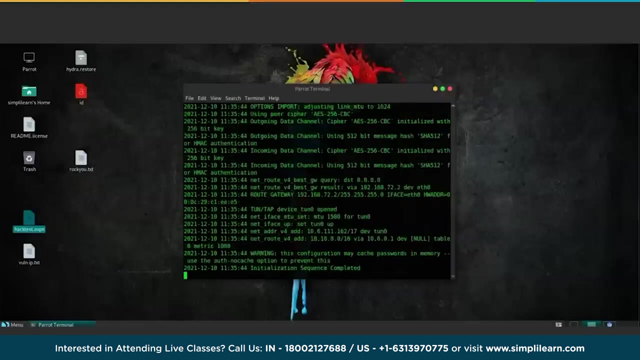 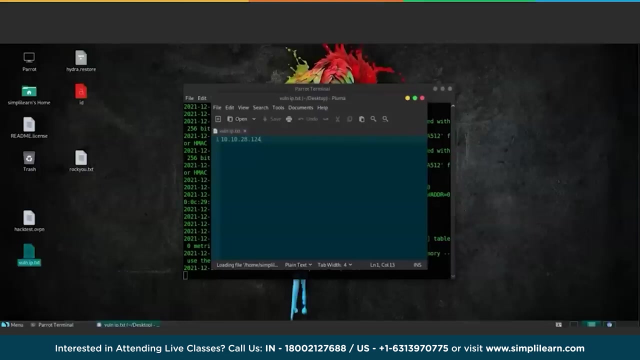 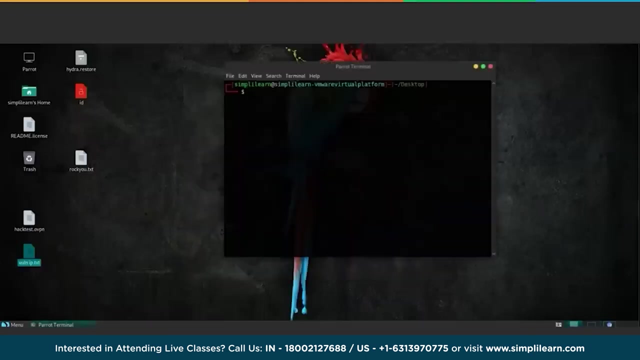 VPN network using this ovpn file And once we get the initialization sequence completed message, we know that the connection has been established. Like we discussed. this is the vulnerable device IP. We're going to copy this and we're going to try to ping. 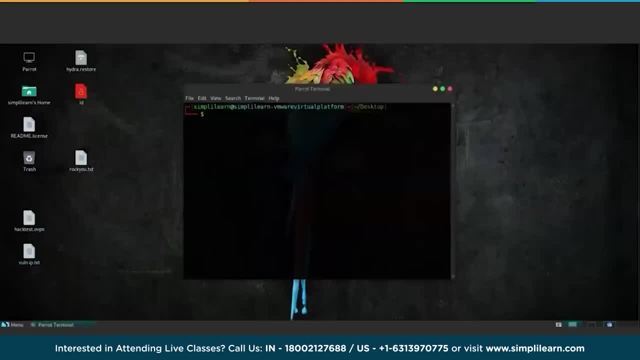 this, Let's open a new terminal. We're going to try to ping this and check if we are able to reach this machine And, as you can see, we're getting a reply back, which means we are now part of the local network. 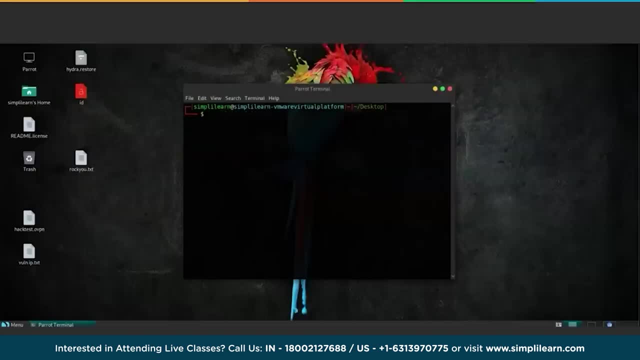 where the vulnerable machine is present. Let's run a service scan map with the respective versions. We ran the similar scan on my local machine, where we were able to detect what version each service was running. What we're going to do over here is by checking what kind of 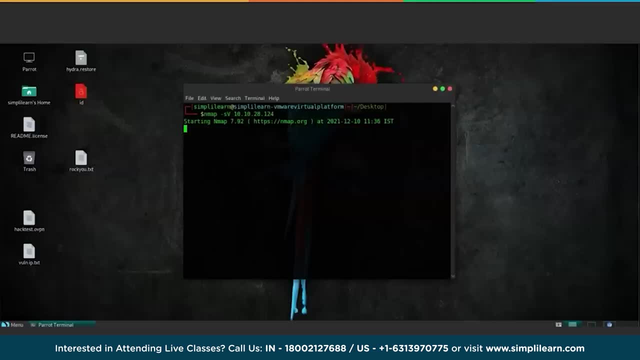 services are open on the machine running on the cloud. we're going to decide what we are going to do next and we're going to see if Nmap alone can point us to a direction where we can gain access to the machine. As you can see, 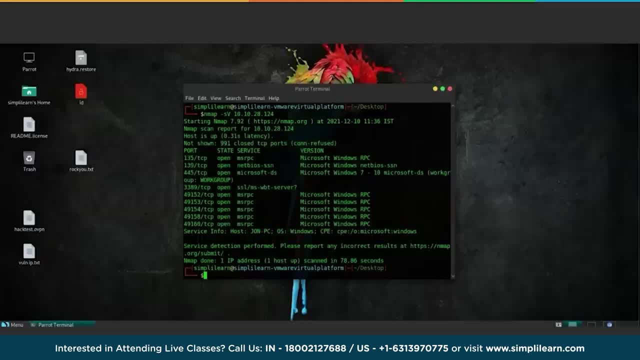 the scan is now completed and we have some of the ports that are being opened over here and what kind of service they are running. Now, like we discussed, this is the first stage, or sometimes even the second stage, of ethical hacking What we can. 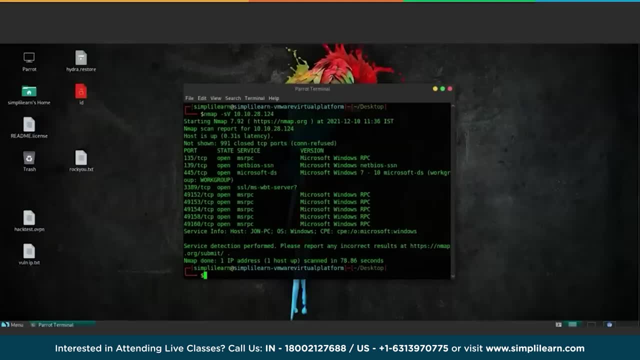 infer from here is: what are the services that are being run Now? these two ports- 139 and 445, are actually Windows SMB server ports which are above the Windows Samba server. Now every service has a particular port attached to it. that will be. 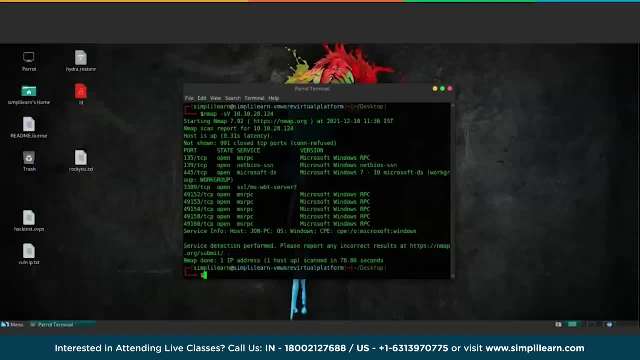 consistent with whichever machine you may use. Apache server will always run on port 80. SMB servers will function on these two ports. Now SMB servers have had a vulnerability known as the eternal blue exploit, which was pretty well known As of right now from the scan. 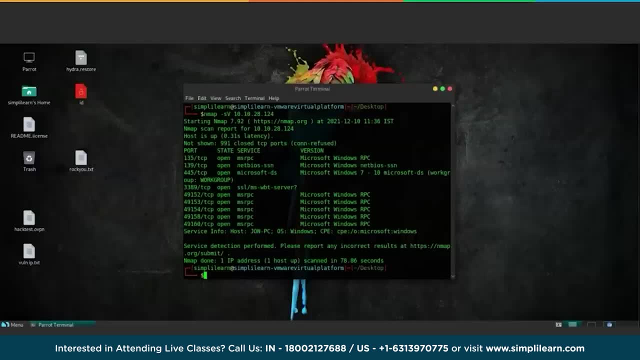 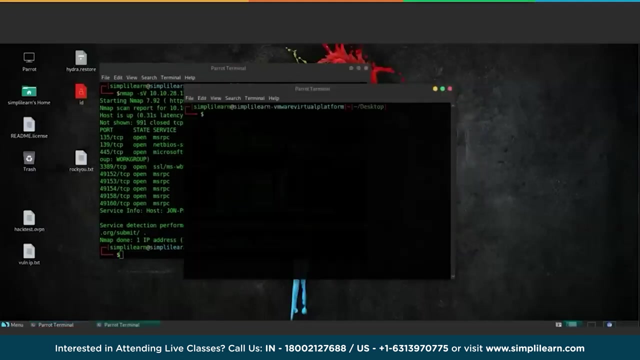 results. we are not able to detect if this machine has the similar vulnerability or not, But since it has the SMB server open, it's worth a shot that we try that exploit on this machine. Now to start the exploit on this, we're going to open another terminal over here. 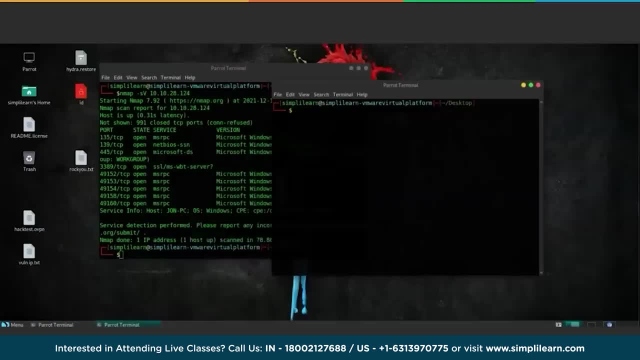 And we're going to use Metasploit for trying the exploit there. We're going to write: sudo- msfconsole- msfconsole is the keyword for launching the Metasploit console. Enter the root password and wait for Metasploit to launch. 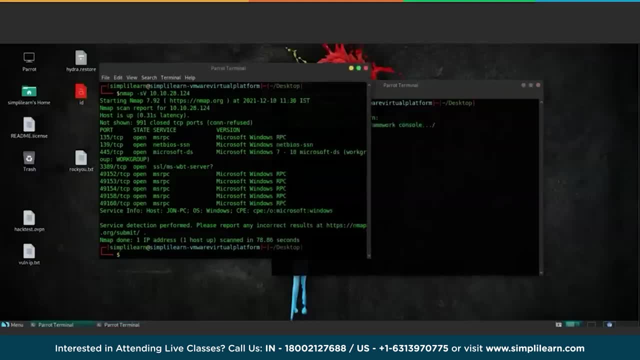 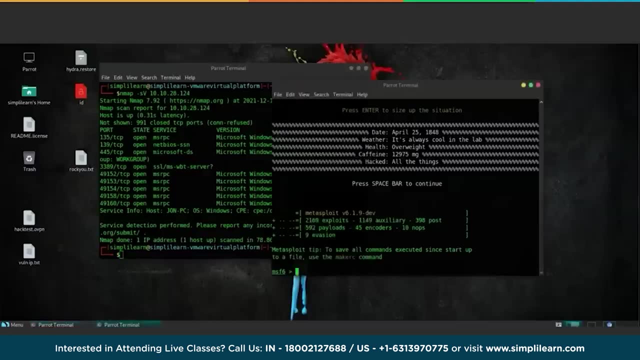 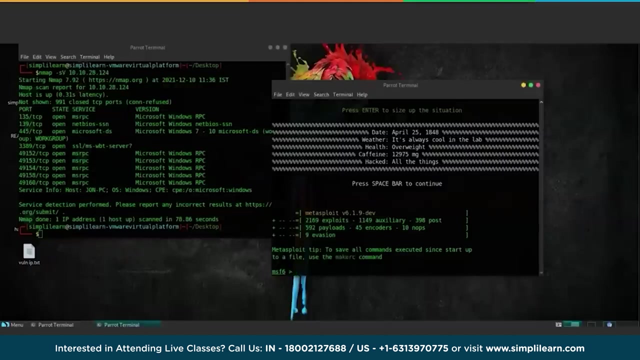 Other than the ports, we can also see that it has checked the hostname of the system and the operating system as well. Now that the Metasploit is open, we're going to launch the exploit Now. before launching, we're going to 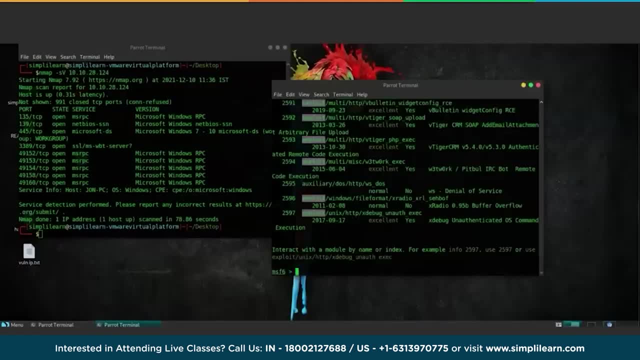 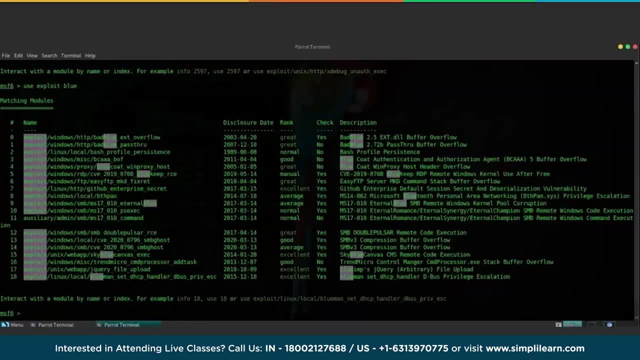 have to check what exploits are there for the eternal blue vulnerability. We're going to write use exploit blue And we're going to check what kind of results we are getting over here. As you can see, we're going to use exploit number nine. 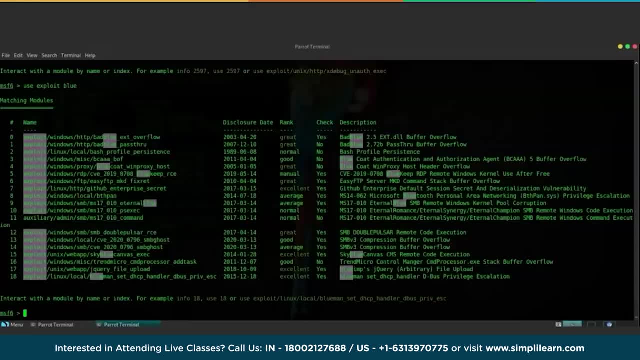 Exploit Windows SMB MS 17-010, eternal blue. It was first disclosed in 2017 and SMB removed kernel pool corruption. Let's say we're going to use this particular exploit Now. all of this may be confusing if you're not. 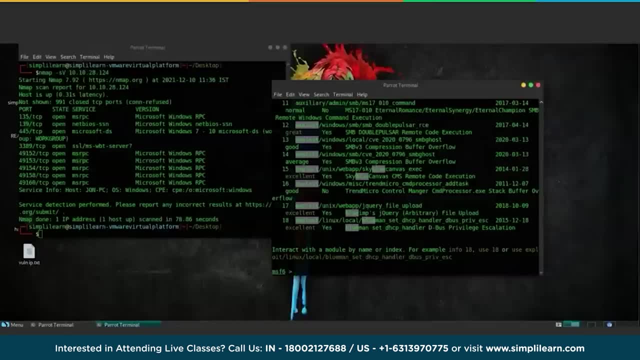 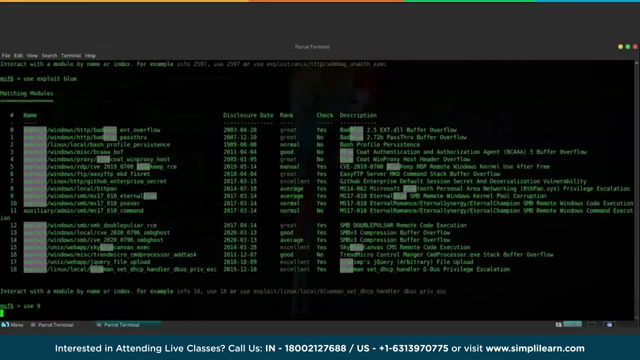 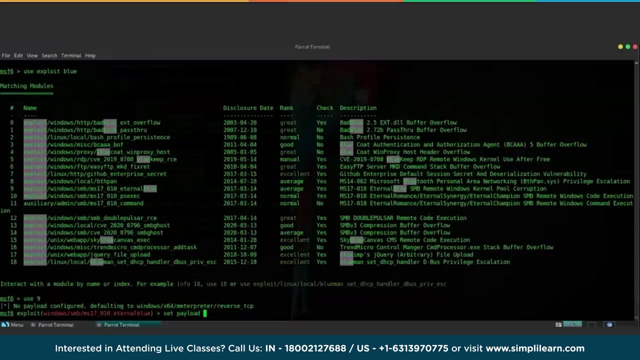 aware of Metasploit. But remember this is the next stage of ethical hacking, which comes into the gaining access part. We're going to use exploit number nine, as we found above. to use exploit number nine, We're going to set a payload which 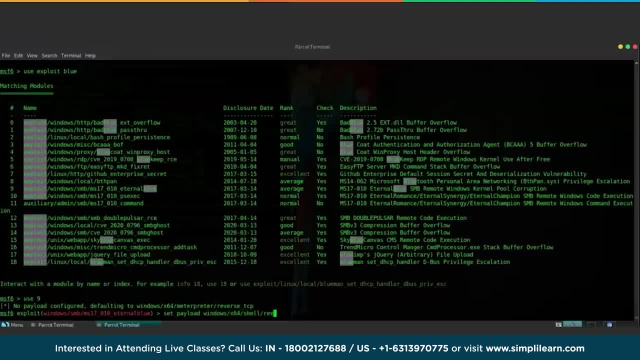 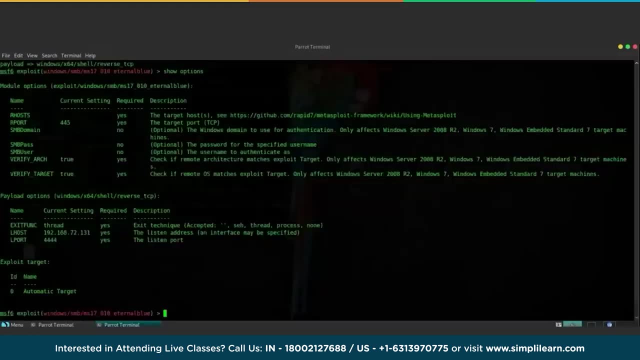 is our malicious code that will run on the victim machine. Now we're going to check some options. As you can see, it has by default pointed it to the 445 port, since that is the port where SMB server can be accessed from. 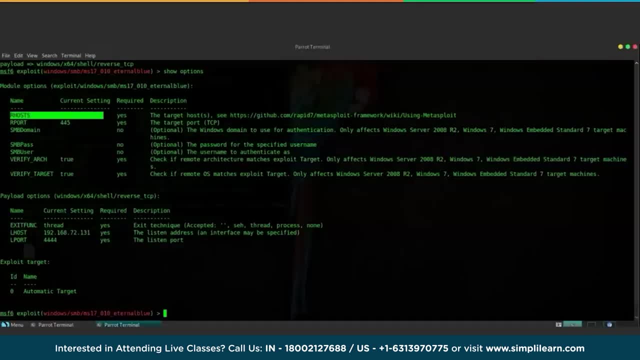 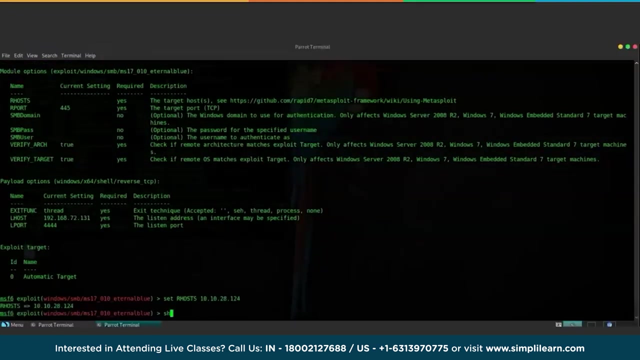 The parameter that's missing over here is our host, The. our host is the IP address of the vulnerable machine, basically the machine in which we want to attack. Now I'm going to use the set command to set the IP address. Now, if we check, 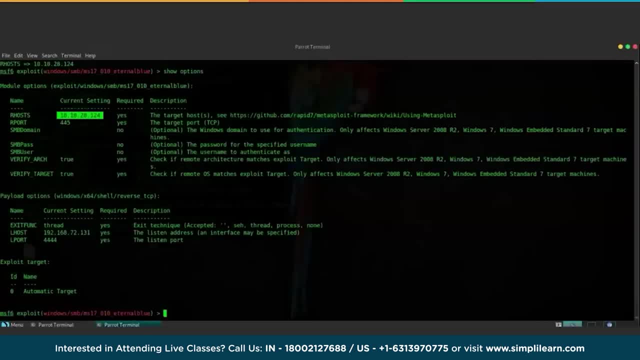 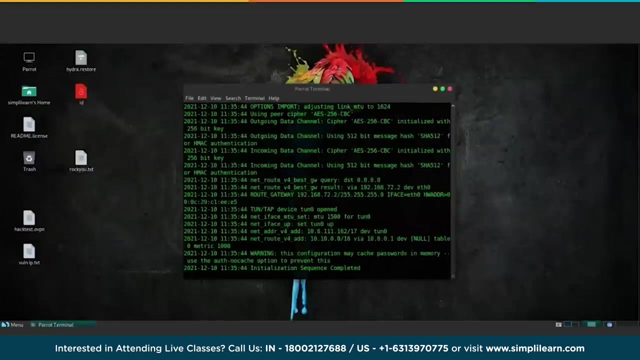 we now have a victim IP address set. Another parameter that we can change is the lhost. This is basically the IP address of our own system where we are going to gain access. Now, if you remember, we had connected using a VPN, So 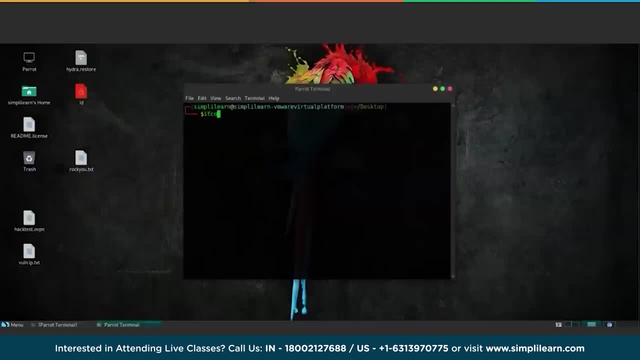 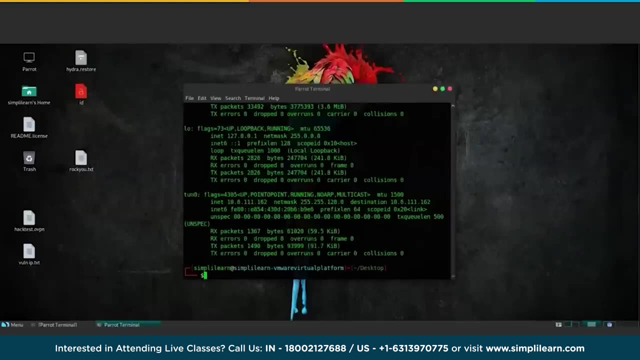 we're going to be assigned a new IP according to the VPN. So if we write ifconfig and check this one, tu10 is the VPN adapter. This is our IP address that we have been assigned in the server in the network where the vulnerable machine is. 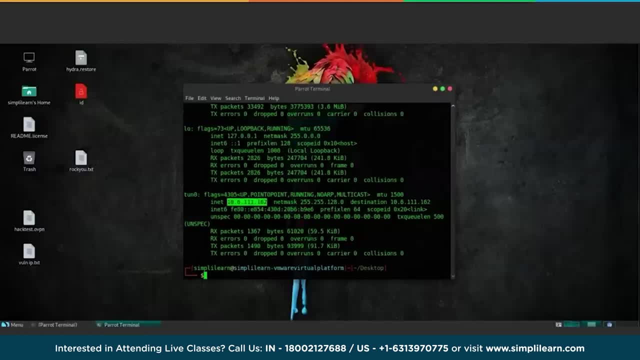 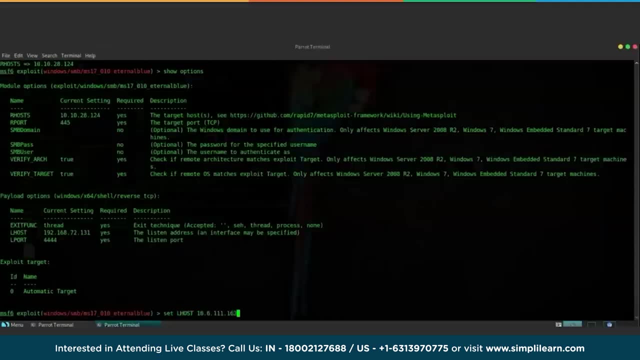 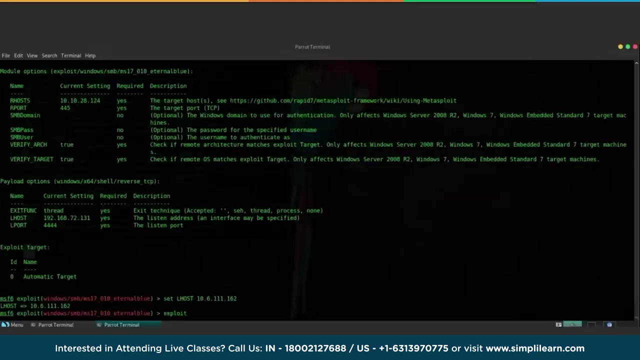 present. So we're going to copy this IP address, We're going to move over this workspace And we're going to set lhost with that IP address. With that, our options are set. Now we're going to run exploit. 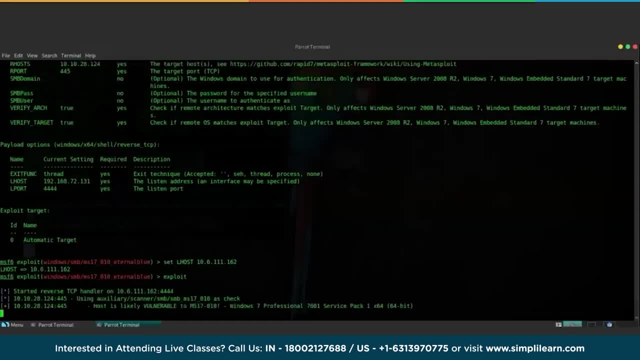 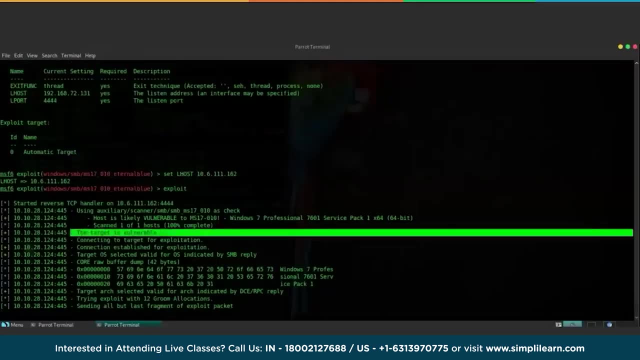 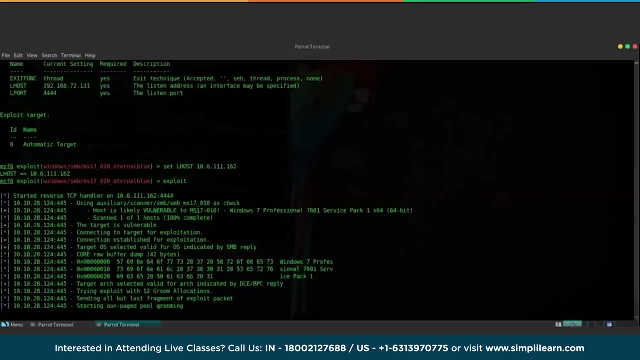 and it's going to check if Samba server vulnerability is present. As you can see, it has written that the target is vulnerable to this particular exploit. It's going to send the malicious code and the malicious code is set in the payload that we sent above. 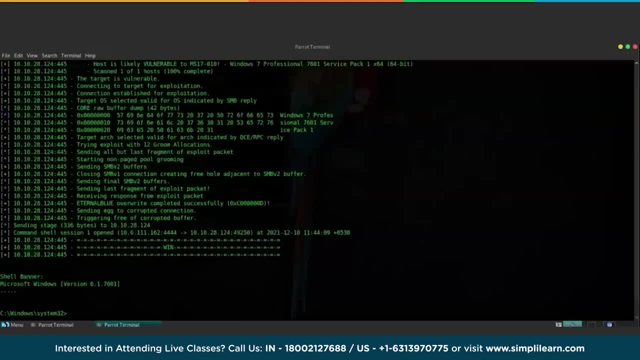 And we now have the shell command of the Windows machine, As you can see, see Windows system 32.. To be sure that this is in fact this Windows machine that is being used, we're going to write ipconfig, which is a Windows only shell. 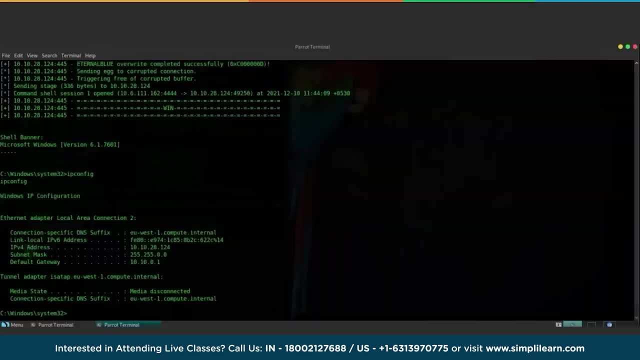 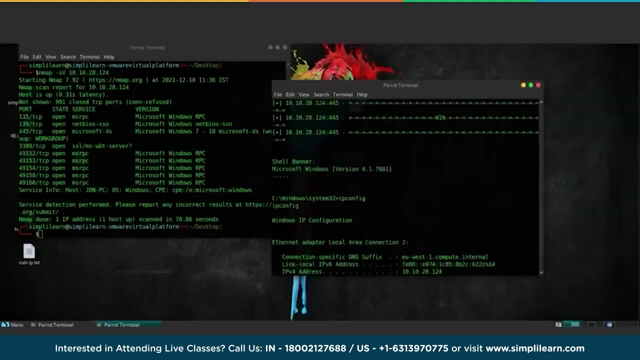 command. As you can see, this is the IP address that was assigned to the victim machine. Now, while a major part of this process was done on Metasploit, we would not have reached this stage had we not found out that the 139 and 445 ports 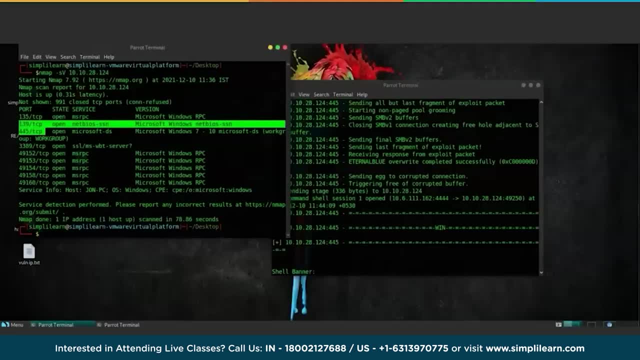 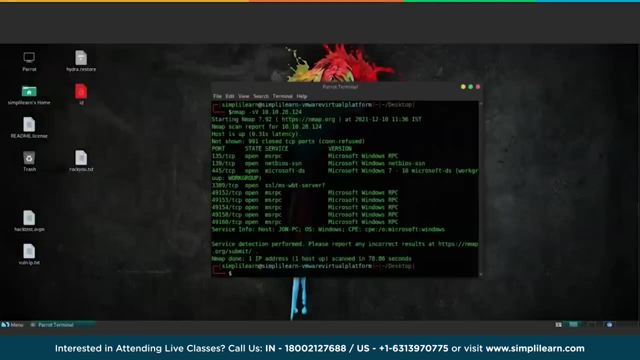 are open, which basically pointed us that we can try the eternal blue exploit of the Windows Samba servers. Similarly, all the scans that we run serve as a preface to the actual stages, or the actual hacking stages, of the campaigns. This sv command was necessary because we could 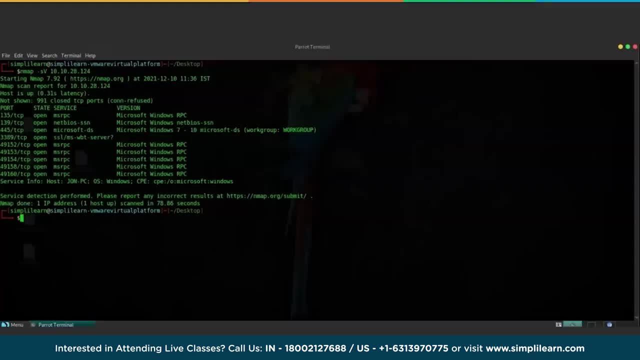 check what are the exact services that are being running. In some cases, if the Apache server is being run, there are particular versions which have particular exploits. Those exploits will not work on other versions, So we're going to have to check what particular version is. 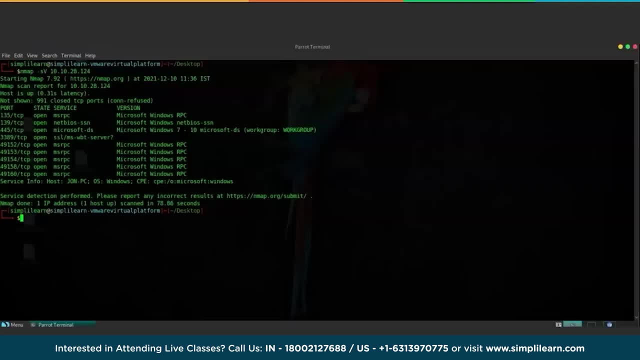 being run and accordingly apply the exploit. That can be done in the Metasploit, or you can run some other tool, but what exact exploit we have to run and which vulnerability we have to target. that is where nmap comes to help With the world moving towards the 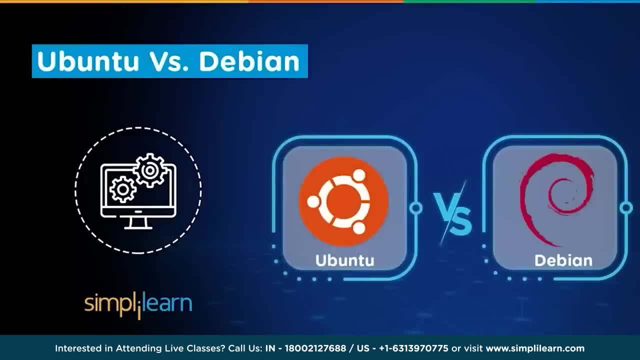 next generation of computer hardware. the software side of things still has a lot left to be discovered. With the majority of laptops coming with Windows pre-installed, many users are devoid of the Linux operating system experience, which is more resource friendly than the mainstream operating systems. 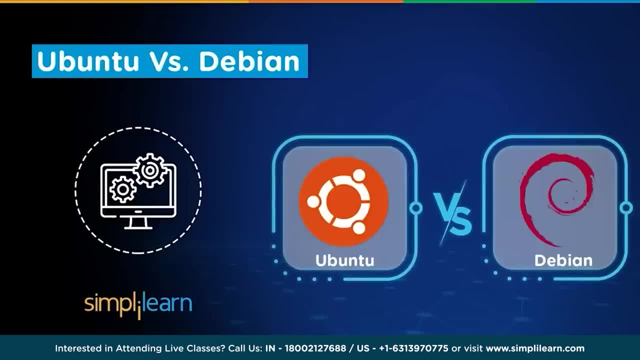 It can be attributed to the difficulty people used to face when installing a new operating system like Linux in the old days. However, a lot of these issues are fixed nowadays thanks to the big names like Debian and Ubuntu, who have been instrumental in making Linux based operating. 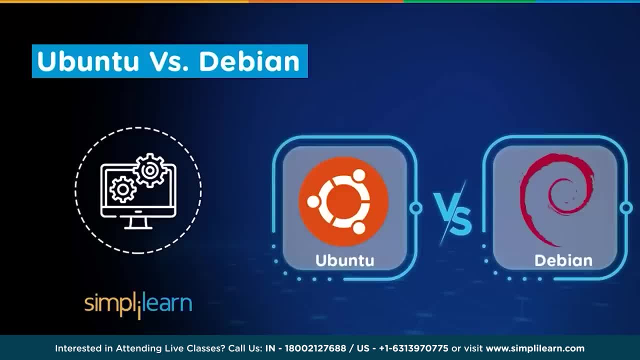 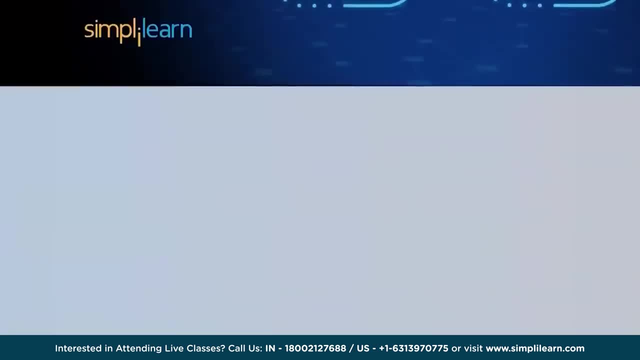 systems as user friendly as possible, But which one of them is better for you? Let's take a look at the topics to be covered today. as we answer this question for you, We start by learning about the operating systems from a layman's perspective. 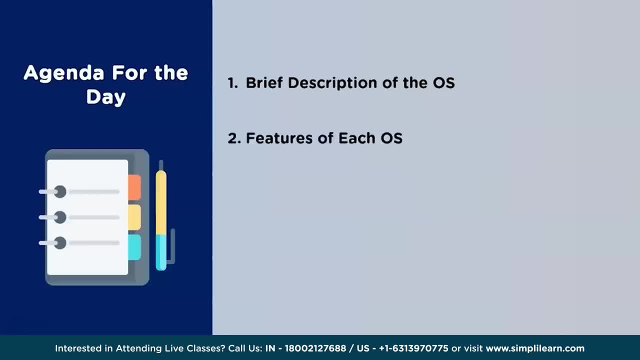 and uncovering the basic offerings of both entities. Next, we cover the unique features of both Ubuntu and Debian and how they stack up against each other and other industry counterparts. Moving on, we take a look at some pointers before installing each of these operating. 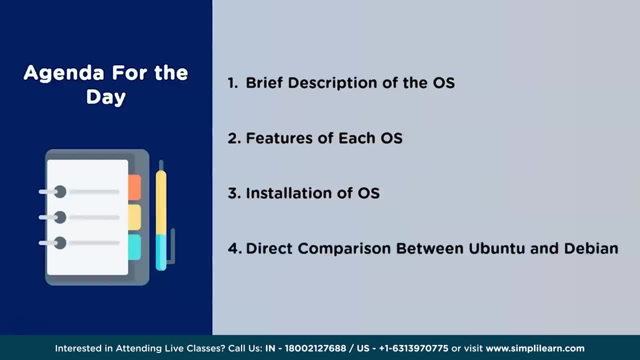 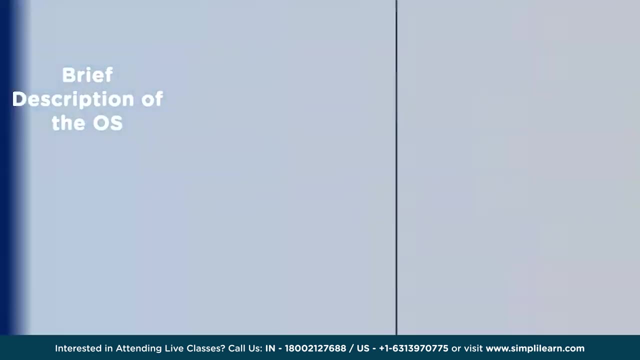 systems and their respective download links. Finally, we compare the contrasting features of both Ubuntu and Debian and infer the kind of users each OS caters to. So let's start by learning about Ubuntu and Debian in general. Ubuntu is an open source, free Linux distribution. 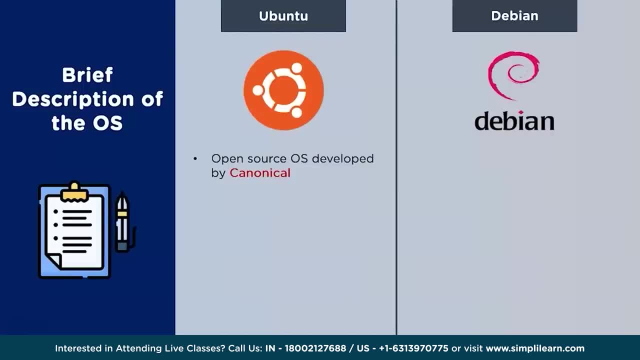 It is an operating system for cloud computing in accordance with support with OpenStack. Ubuntu is developed by the Canonical community and it is freely available. Also, Canonical Limited is responsible for the funding of Ubuntu. Basically, Ubuntu is released every 6 months. 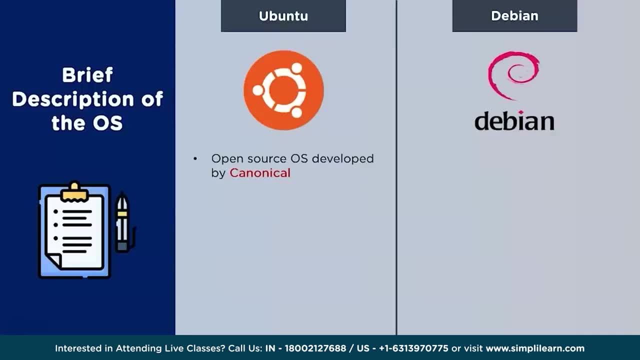 Free support is available for 9 months after every release, and long term support, which are the LTS, is released every 2 years. The first release of Ubuntu was in October 2004.. You must have heard about Ubuntu, no matter what. It is the most popular Linux distribution overall. 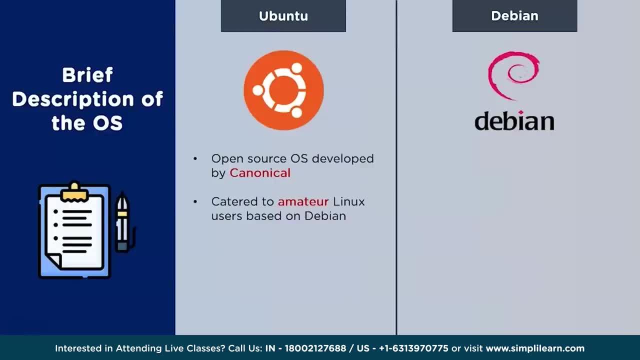 Not just limited to servers, but also the most popular choice for Linux desktops. It's easy to use, offers a good experience and comes pre-installed with essential tools to get a head start. Of course, Ubuntu managed to simplify the Linux experience years back. 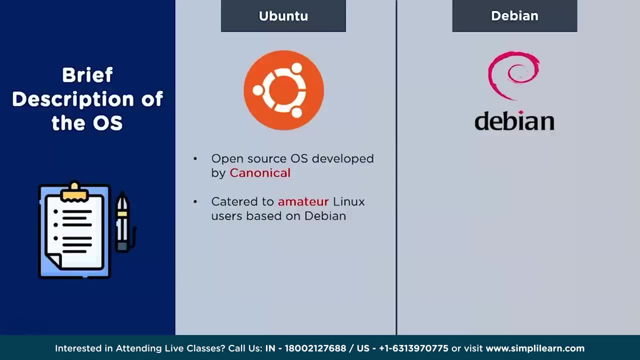 and that is the reason why it is still so popular, even with several impressive Linux distributions available right now. Every new release is more polished and comes loaded with new features and improvements. Thanks to its huge user base, software vendors have made their applications compatible with Ubuntu. 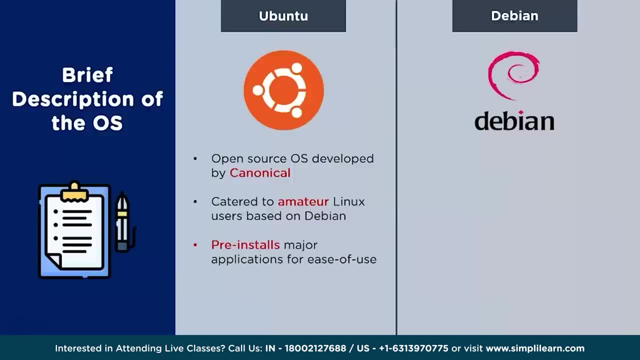 While the catalog may not be as extensive as Windows, the options are still well curated. More importantly, the advantage of Linux based operating systems is the ability to use free and open source alternatives to major proprietary software. By lacking some polish and overall features set. 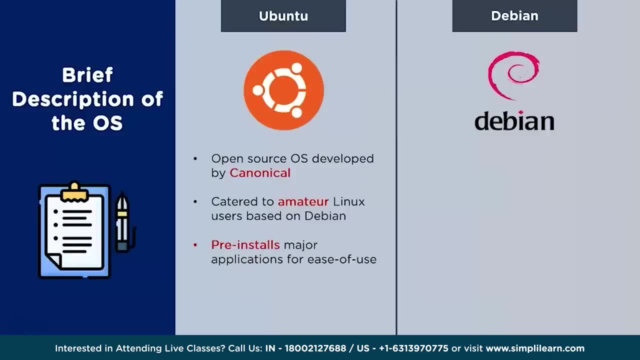 most alternatives are enough to get the job done for majority of the users. The never ending community support also helps in troubleshooting should things go wrong at any point in time. The default desktop environment in Ubuntu is GNOME or Unity. The Unity is a modern desktop environment. 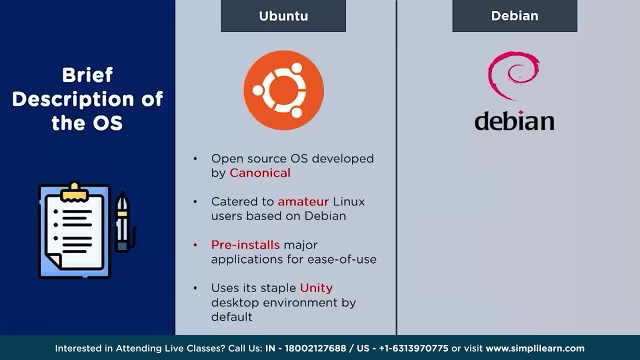 with a powerful search tool for finding all your applications and documents. with its base setup as GNOME, It integrates well with common applications such as audio players, video players and social media. There are a few other desktop environments for Ubuntu as well, with Unity as its flagship environment. 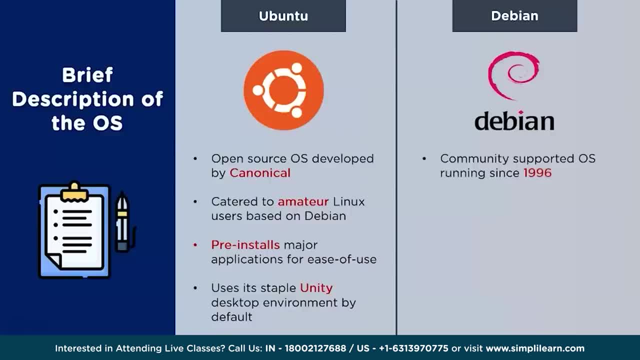 Debby's desktop environment, on the other hand, is a free operating system for your computer, which started in 1996 and is maintained by global contributors. If the operating system is a set of basic programs and utilities that make your computer run, its core is the kernel. 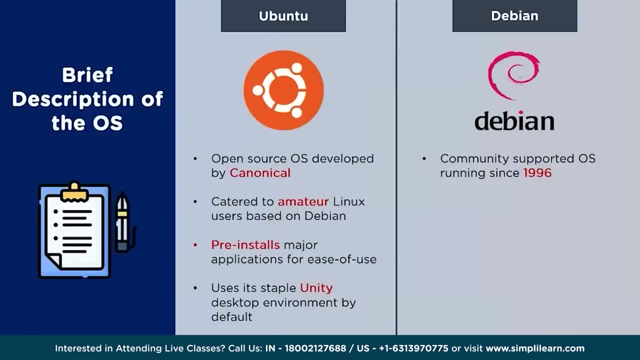 The kernel is the most fundamental program on the computer. Debian uses the Linux kernel, a completely free piece of software which was started by Linus Strohwald and supported by thousands of programmers worldwide. A large part of the basic tools that come from the GNU project. 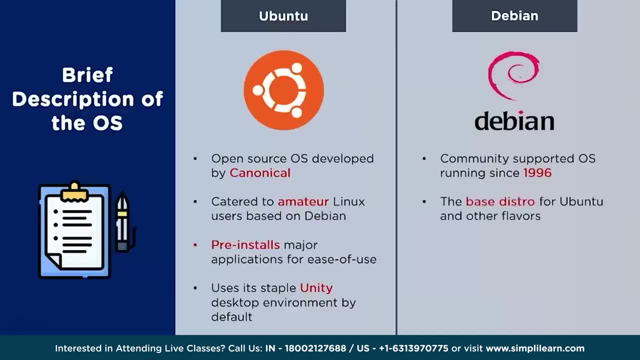 and those tools are free as well. Debian is the mother of Linux distributions. Beginners always wonder why this not-so-good looking distro is so popular inside the Linux developers community, especially when there are a lot of modern distributions that are easy to use and have beautiful UI. 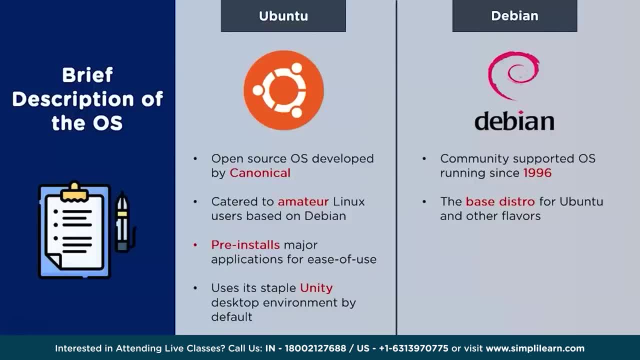 Later on they found out the power of Debian after using a bunch of distributions from other developers. You will be surprised to know that almost all other popular consumer level distros are based on Ubuntu. It is so stable and feature rich that the developers find it easy. 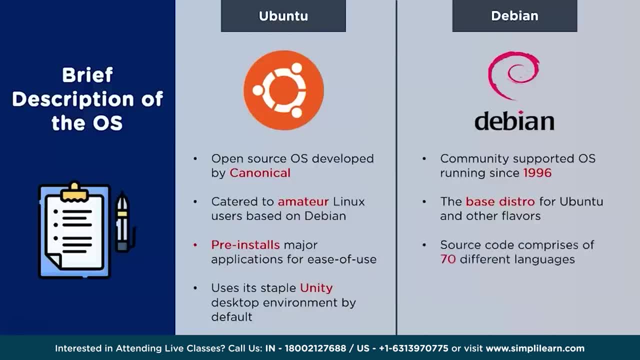 to build their distros based on Debian rather than building it from scratch. Debian is run and maintained on its GitHub repository thanks to contributions from developers worldwide. Major decisions are taken up on the repository issues tab, leading to community-wide feedback and a holistic approach to open source development. 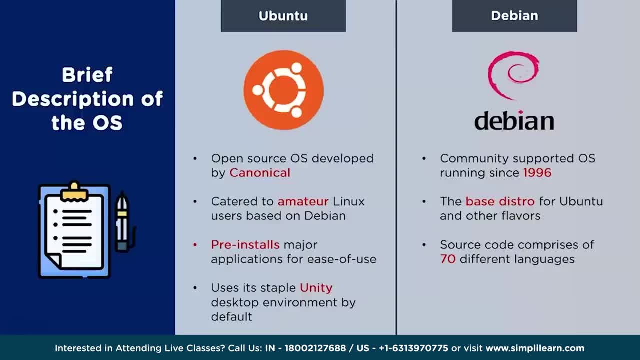 of the Debian operating system. Thanks to this variety of personnel, the source code of Debian comprises different programming and scripting languages. Debian supports all kinds of graphical environments, ranging from full-featured desktop environments to lighter alternatives and even minimalist window managers. Ubuntu ships with Unity desktop by default. 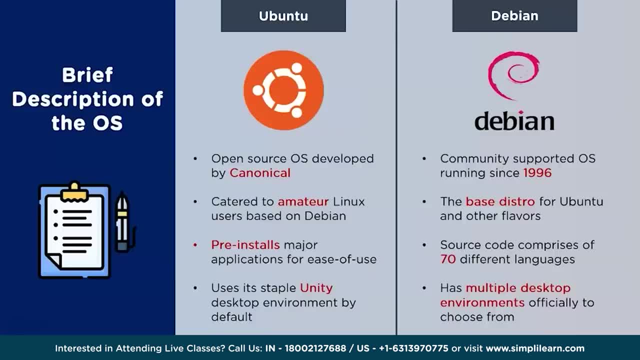 but the package manager can install the GNOME environment if needed, while also including Cinnamon, LDEXDE, XFCE, KDE and Mate. On the other hand, Debian gives you the choice of choosing which desktop environment you want to install. You can choose to install. 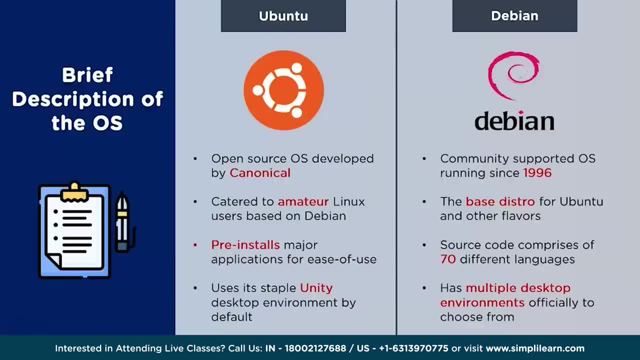 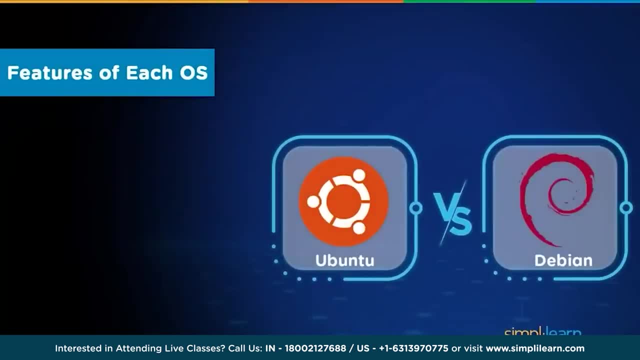 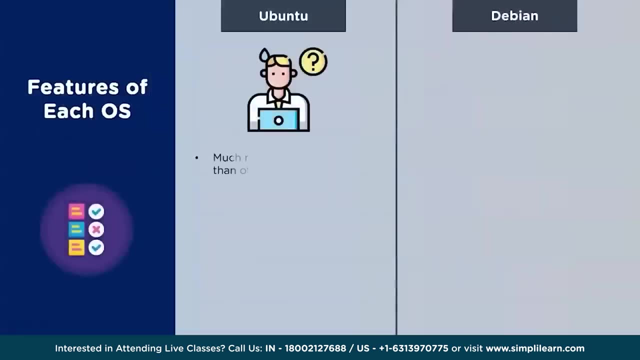 both from the get-go, by providing ISO files for each desktop environment individually. Now that we understand where both these operating systems stand, let us take a look at some of the best features offered by each of these distributions. Ubuntu is the closest thing to a household name. 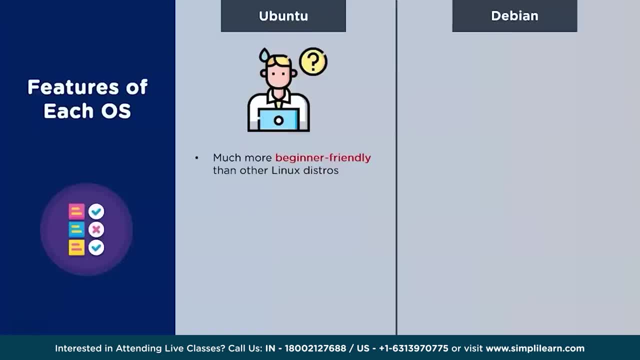 among desktop Linux distributions. It is a great distribution to start with and it's even a great distribution to keep using after you're more experienced, if you're happy with it. It is user-friendly in a lot of ways. It provides a simple desktop. 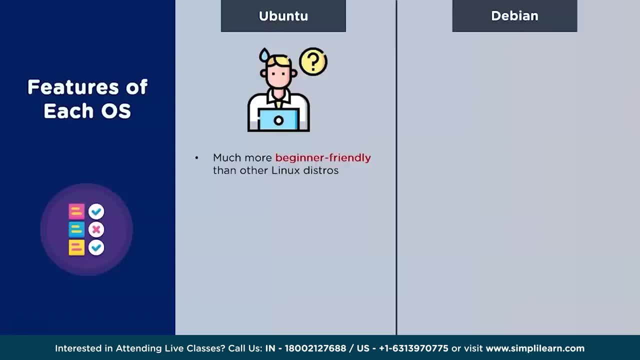 has an easy installer and provides a checkbox during the installation process that will automatically install Flash plugins and various codecs that you will need for multimedia support. There's an additional drivers tool that will detect closed-source or proprietary drivers that might be necessary to get all your hardware working. 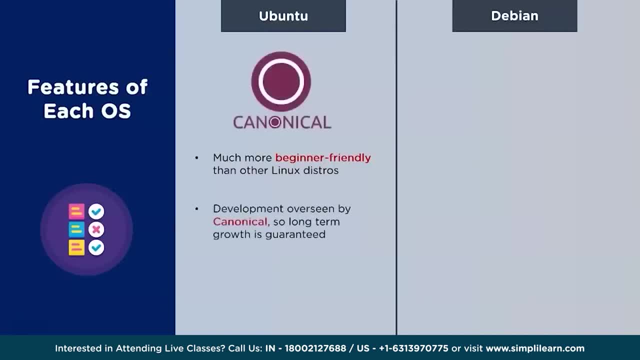 and easily install them for you. Ubuntu is produced by Canonical and their friends. It is run as an open project to enable others with diverse ideas to benefit from all the work the developers do to deliver the world's best open platform. Still, Canonical is responsible for delivering. 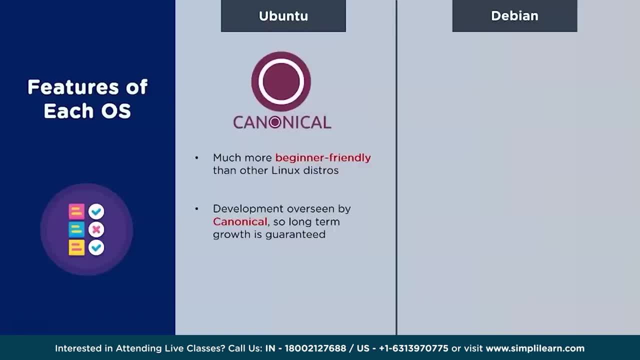 six monthly milestone releases and regular LTS releases for enterprise production use. Enterprises can count on Canonical to support, secure and manage Ubuntu infrastructure and devices. With more than 500 employees in over 39 countries, the company underpins the critical infrastructure for thousands of businesses and millions. 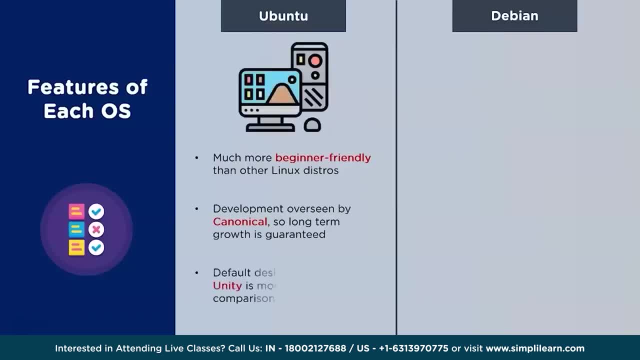 of Ubuntu users around the world. Unity Desktop was originally developed by Canonical and introduced earlier for netbook computers with Ubuntu 10.10.. Then it went on to be the default desktop environment for Ubuntu. Eventually, it has been dropped by Canonical and replaced by GNOME. 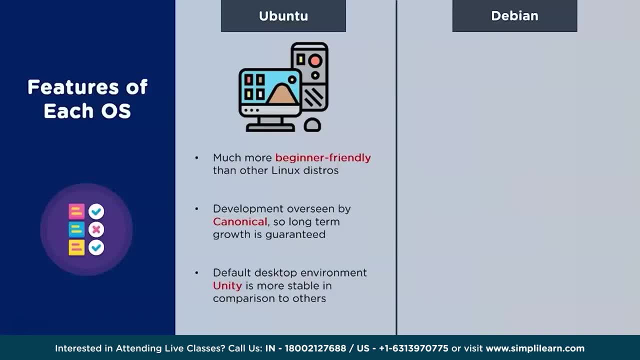 However, it has made a comeback after Ubuntu 18.04.. While being completely stable, the HUD and global menu hold up just fine with major applications such as LibreOffice, Thunderbird and other web browsers. That means that the Unity desktop works. 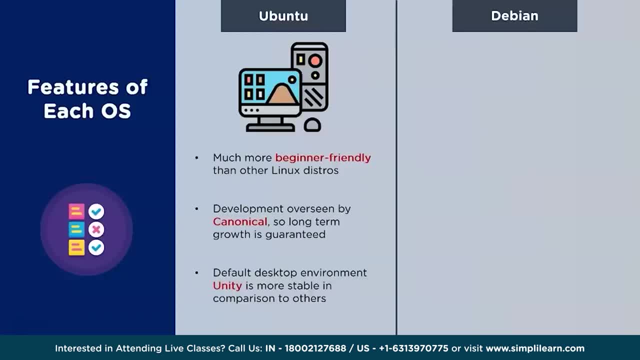 as it is supposed to, while making you more productive. While some desktop environments have a steep learning curve, Unity is very intuitive for new users. in spite of deviating from the traditional start menu format that the Windows users are generally accustomed to, The Calamares installer is a framework. 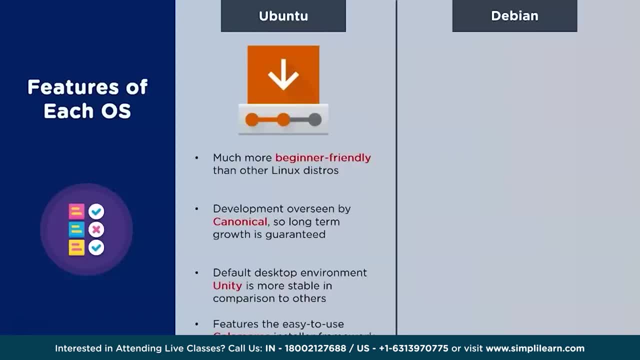 By design, it is very customizable in order to satisfy a wide variety of needs and use cases. Calamares aims to be easy, usable, beautiful, pragmatic and, more importantly, distribution agnostic. Calamares includes an advanced partitioning feature as well, which supports for both. 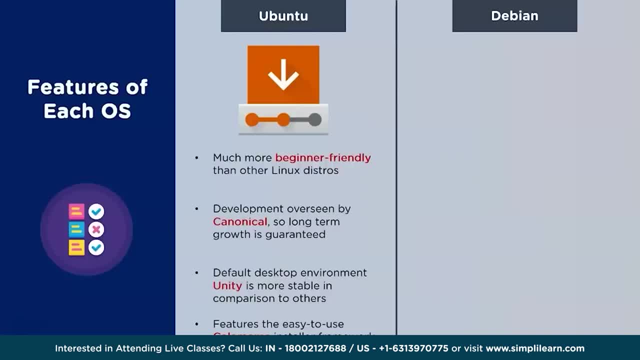 manual and automated partitioning operations. It is the first installer with an automated replace partition option which makes it easy to reuse a partition over and over for distribution testing. Coming to Debian, it is a community distribution through and through. It's governed by a. 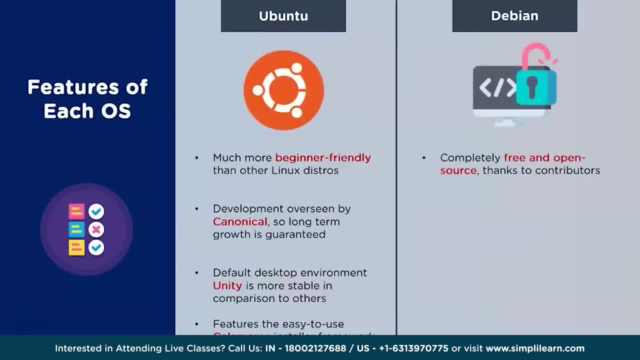 board of elected developers. It has its own internal structure and laws, and just about everyone working on it is a volunteer, making it completely community driven. It is maintained and developed by programmers and developers all around the world. This form of development ensures continuity. 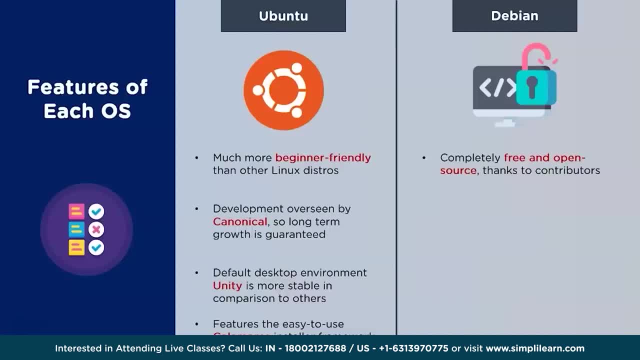 If one of the developers decides to stop working on the project, another developer might come in and take place and keep the project going on. It is completely free of centralized control and this is also one of the reasons for an undecided, stable release cycle. Debian SID. 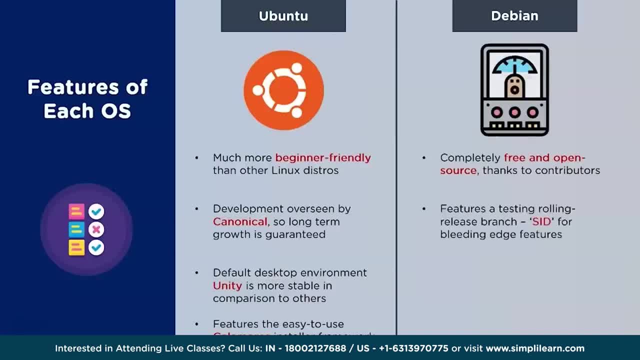 is the permanently unstable development version of Debian. It is where the latest versions of programs are being considered for inclusion in the Debian release cycle are uploaded and tested, Because it has no official install media and the few netboot images that are built often don't work even. 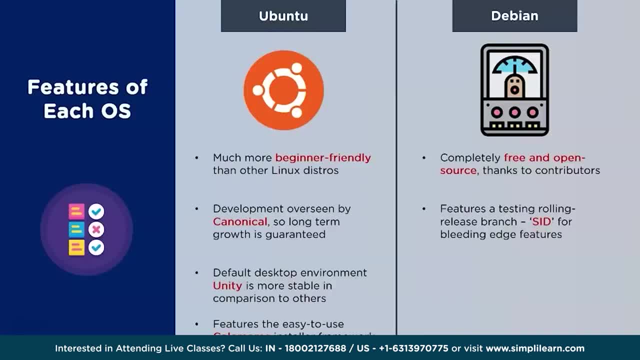 people who are willing to risk using a development version may have trouble installing it. However, it still remains the best place to test new features that have not yet made their way onto the stable branch. Debian has only free and open source software in its repositories. This is mostly. 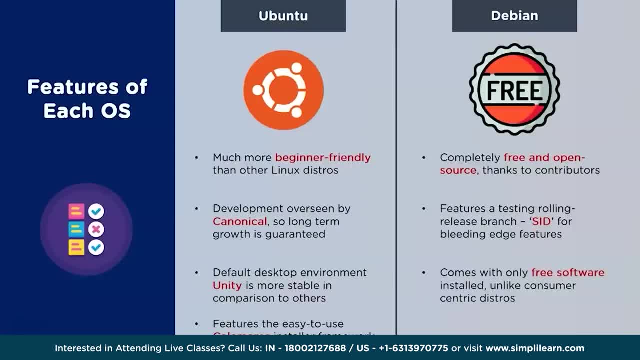 ample for our users. Except for users who use hardware that only has proprietary drivers, these repositories work well in most cases. It is possible to add other repos as well that have proprietary software, if that is the requirement. Debian's standard version is very stable as software and libraries. 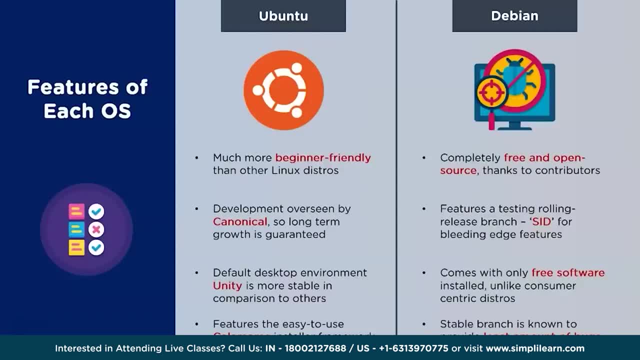 in it go through rigorous testing. This stability makes Debian a perfect server OS, and it's also the same reason why average users shy away from using Debian as their primary OS on desktop. This is also one of the reasons why many developers use Debian as. 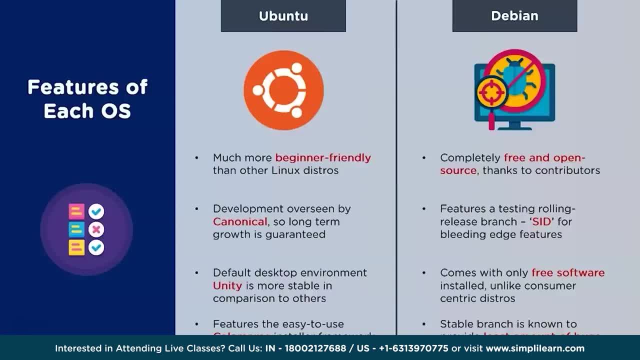 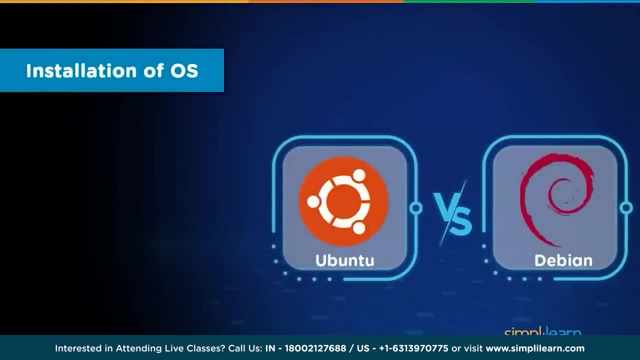 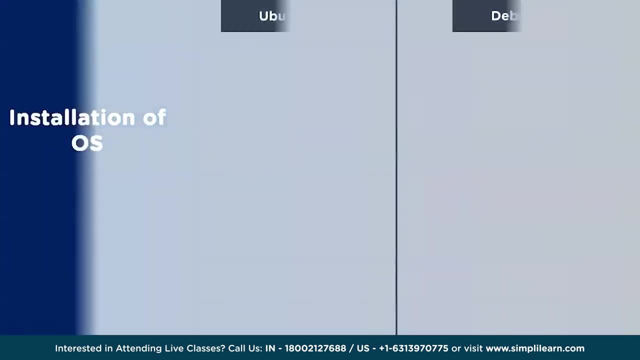 a base for their derivative, one of which is also Ubuntu. Now that we are aware of each distribution's unique features, let's take a look at how we can go ahead and install these operating systems and where we can get their downloadable images, When it 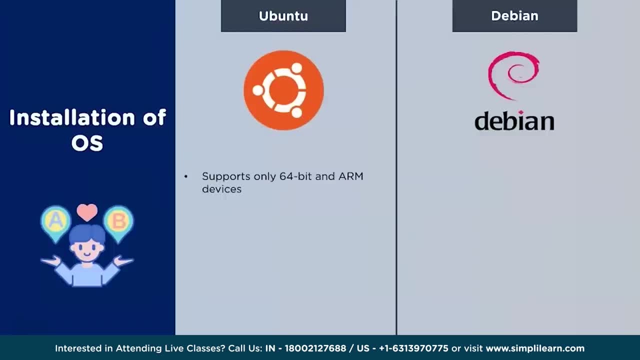 comes to Ubuntu, Ubuntu has dropped the support for 32-bit systems. Currently it supports only 64-bit devices and ARM devices. Installation is easy with the Calamares framework coming into ISO pre-default, and the latest ISO can be downloaded from. 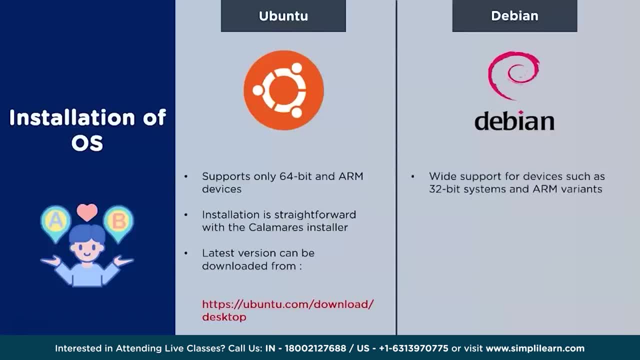 the link being shown on the screen right now. In the case of Debian, the support for multiple range of devices is still present. That can also include 32-bit systems and other smaller devices which are not modern. Even though it does not use the Calamares, 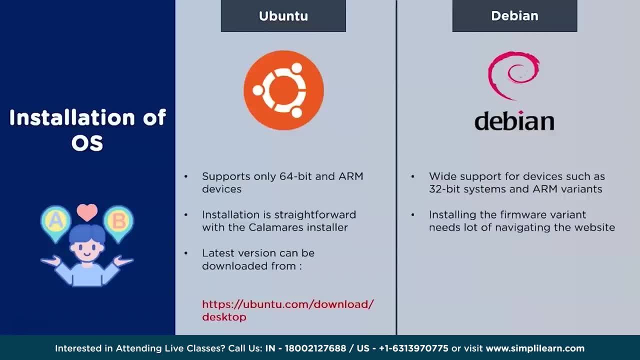 installer. even downloading the ISO file can be a bit hectic for newer users, Considering this is a distribution aimed at developers and intermediate users, finding the right link can be difficult, because of which we have mentioned the link on the screen below where you can get the latest ISO. 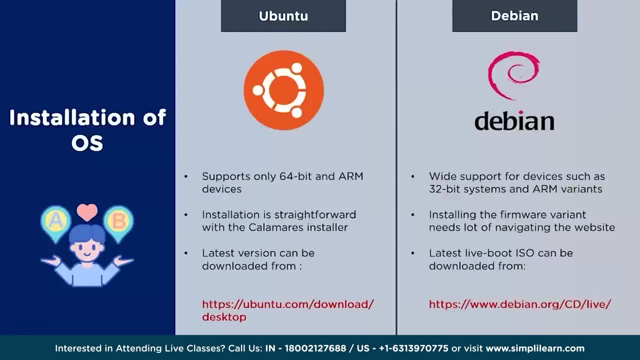 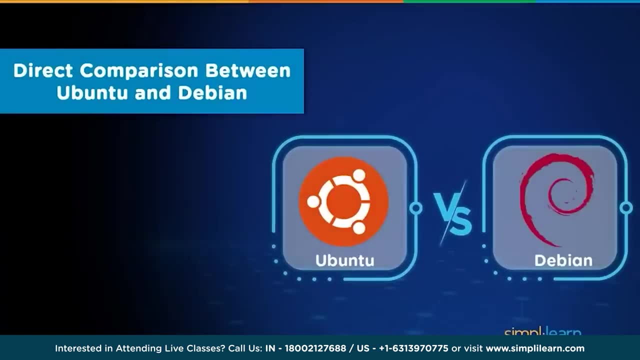 depending on which desktop environment you choose to go with. With the installation out of the way, let's take a direct comparison of the features between both Ubuntu and Debian. Debian is a community driven open source Linux distribution and is primarily aimed to be robust. 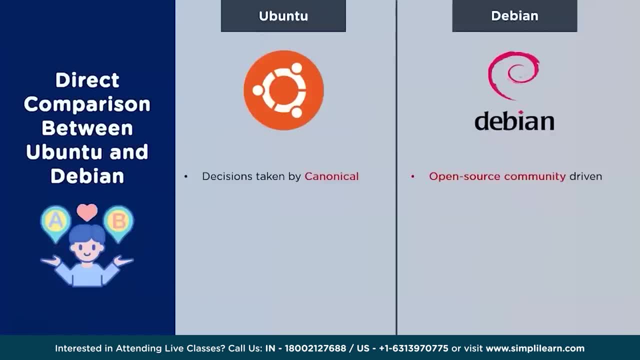 capable and, most importantly, free. On the other hand, Ubuntu is also and free on open source, like Debian, but it's backed up and developed by a canonical which is a corporate company. Debian and Ubuntu are both fundamentally fast regarding performance, As Debian comes bare minimum and is not. 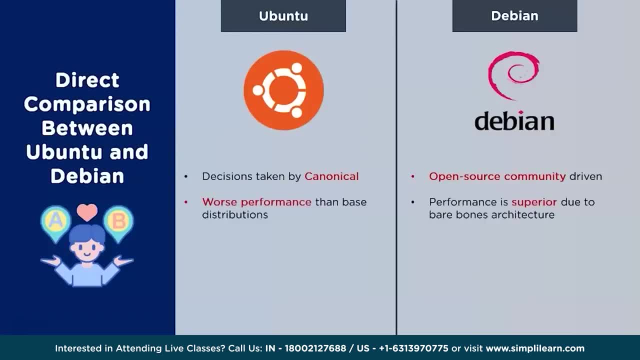 bundled or pre-packed with additional software and features, Debian can be used for a lot of different purposes. Debian is a community driven open source Linux and features it makes it super fast and lightweight, at least when compared with Ubuntu directly. Both Ubuntu and Debian use 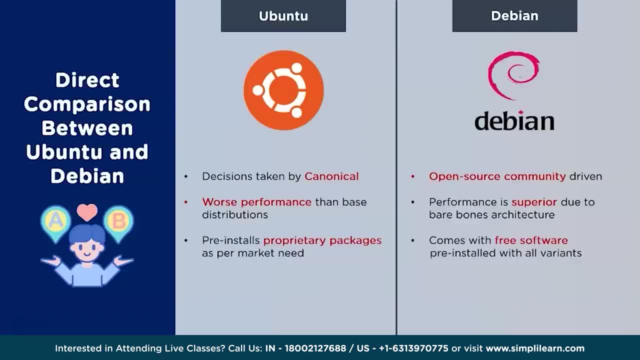 the same APT software packaging management system but provide a different software repository. Debian is more like promoting freedom of choosing free software. thus it does not include any proprietary software by default. You can always install the paid versions, but you have to enable it manually. 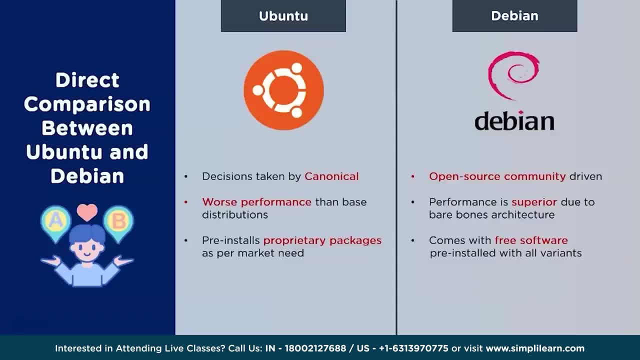 Ubuntu focuses on usability, including all the software, including free, paid, open source, closed source, etc. Ubuntu also introduced a universal package management system called Snap. It will be used across distros and thus prevent more distro based software fragmentations. 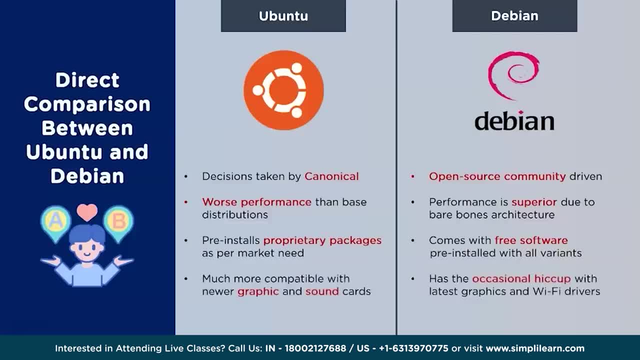 As the Debian distro does not contain any proprietary blobs, there might be some problems with drivers and firmware. That means Debian lacks some of the essential proprietary firmware by default, but the users can enable the repository and install it manually like other paid software. 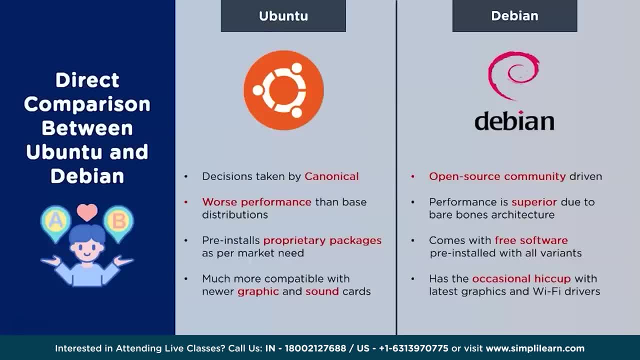 On the other hand, Ubuntu does not care how much, whether it's paid, free, open source or closed source, so it includes as many drivers and firmware as possible. Ubuntu also lets you install and configure the necessary drivers and firmware automatically during installation or 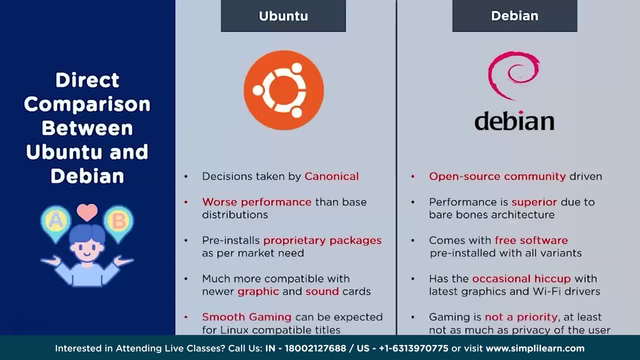 afterward. If you are a gamer, then you will probably be concerned with the latest software drivers and hardware support. While Debian can potentially provide that, it is likely that you might end up breaking your installation. As mentioned before, Ubuntu supports certain proprietary packages as well. 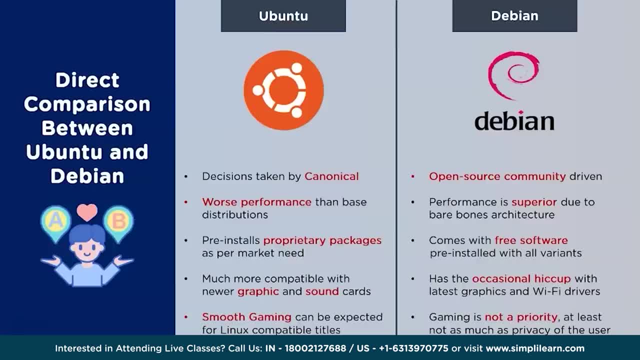 which often consist of graphic drivers, which are essential to gaming. Debian focuses on the open source aspect of the software. Hence it can be a well known fact that with gamers, Ubuntu and some other distributions like Pop OS have been working much better regarding both software. 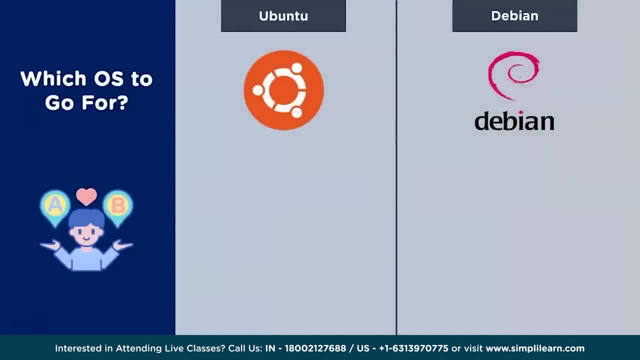 and hardware support. Regarding the audience they cater to, both Ubuntu and Debian have their pros and cons. Ubuntu is a very good distribution for amateur users with little to no experience and if they want to have the latest versions of packages and applications at all times on their systems. 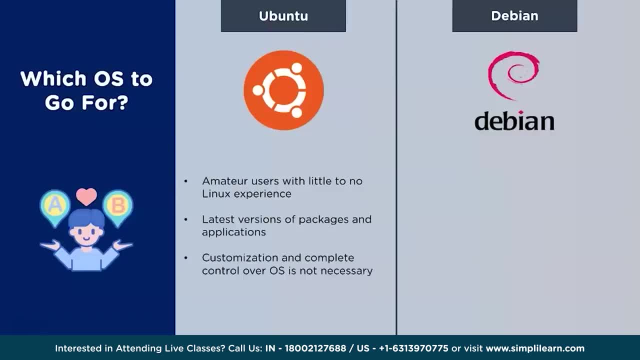 It is also for users who do not want a lot of customizability, in spite of Unity being a very customized desktop environment. It is also perfect for users with newer hardware, since it comes updated with all the latest graphical devices and their respective drivers. Debian on. 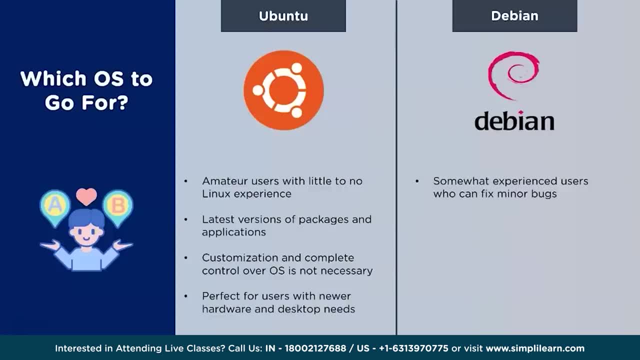 the other hand, is catered towards a little bit of experienced users who can fix some minor bugs on their own or with minimal community support. It also is for users who want to support an open source approach rather than an operating system which is devoid of any contribution. 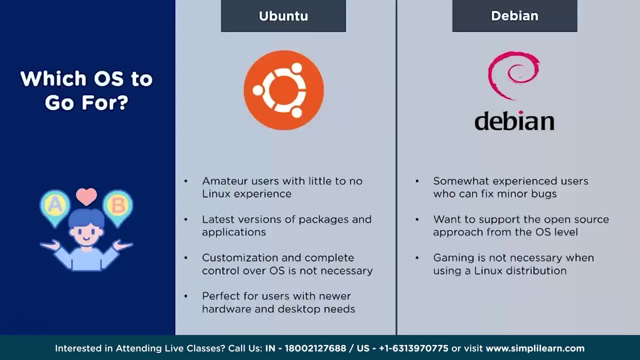 from other end and is primarily backed by a corporation. It also doesn't favor gaming, since it does not guarantee compatibility with all the newest graphic cards or even Wi-Fi cards. in some cases, However, due to the low memory overhead, Debian is very useful for. 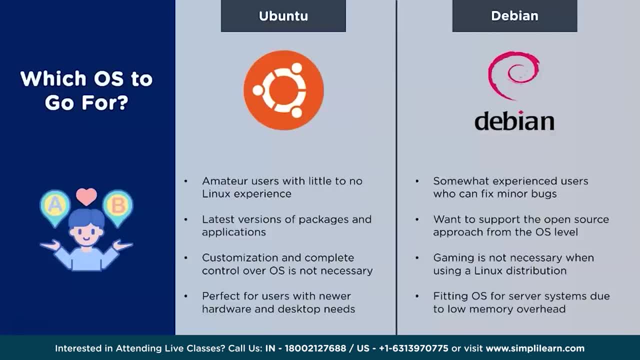 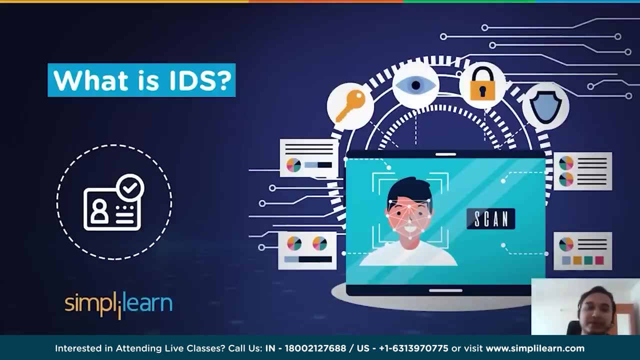 people who are looking to run home servers, or even corporate environments, where running servers on Debian will provide much more use. Data protection is of paramount importance in today's world. The vast amount of data flow between corporations and consumers needs to be secured, considering that they are. 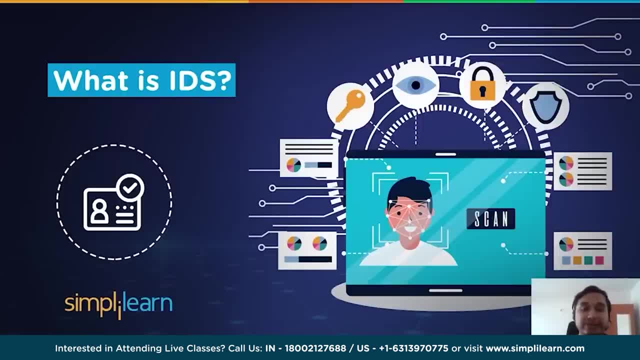 entrusted with a lot of belief. A company can spend millions of dollars on the most secure servers, but it takes a single hacker to ruin all the goodwill between the organizations. To prevent these malicious attacks, many automated security systems have been developed, but none of them have been as 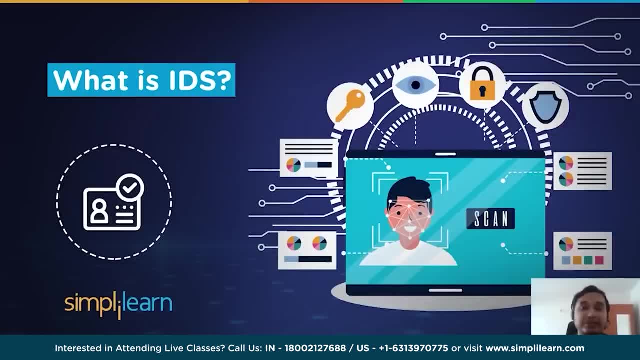 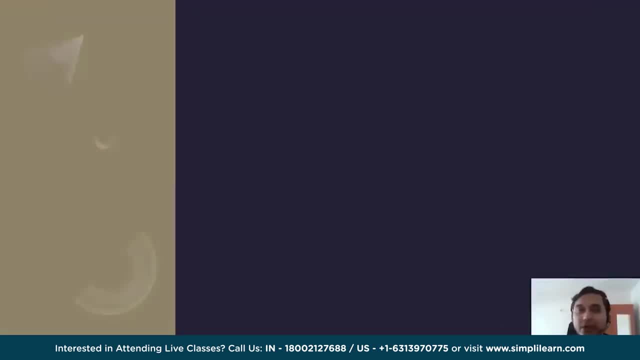 used as IDS platforms. IDS platforms are also known as Intrusion Detection Systems. Welcome to this introductory lesson on Intrusion Detection Systems. So let's go through the topics that we are going to cover today. We start with the basic definition of IDS from a layman's perspective. 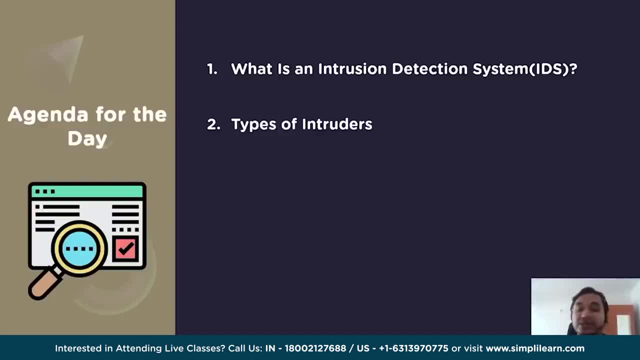 Moving on. we cover the multiple types of intruders that seek to access confidential information without any authorization. Next, we cover the basic ways to detect intrusion signatures from the perspective of a network administrator, Then take a look at the different types of IDS systems that can be used in. 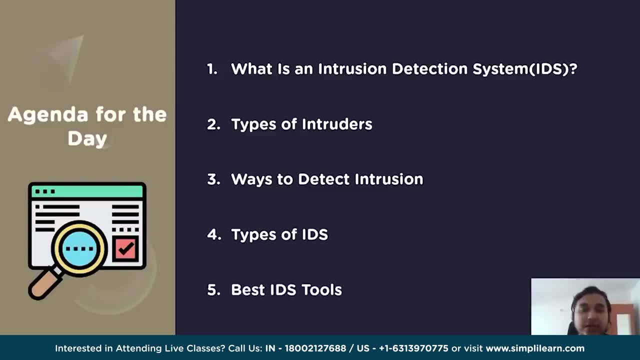 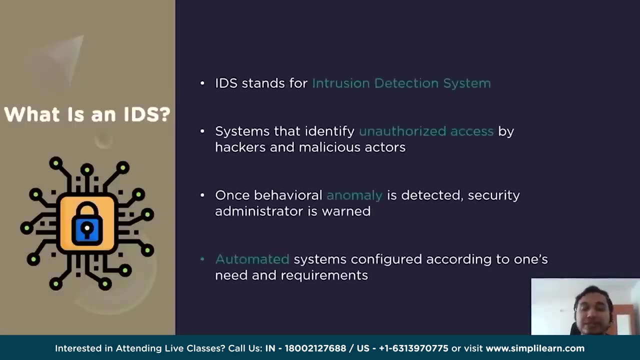 corporate environments today. A small explanation of the two types of protection is then followed by an introduction to some of the most well-known IDS tools on the market. So let's get started with. what is an IDS? An intrusion detection system is an app or device that 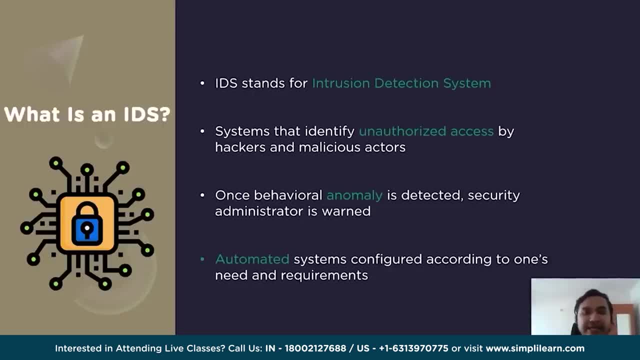 monitors inbound and outward network traffic, continuously analyzing for activity changes and patterns, and alerts an administrator when it detects unusual behavior. An administrator then reviews alarms and takes action to remove the threat. For example, an IDS might inspect the data carried by network traffic to see if it contains 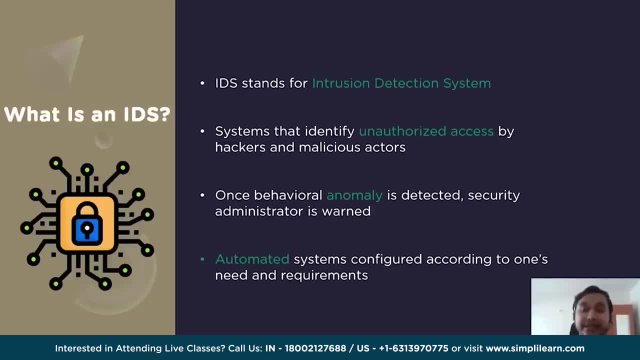 known malware or other malicious content. If it detects this type of threat, it sends an alert to your security team so they can investigate and remediate it. Once your team receives the alert, they must act quickly to prevent an attack from taking over the system. To ensure 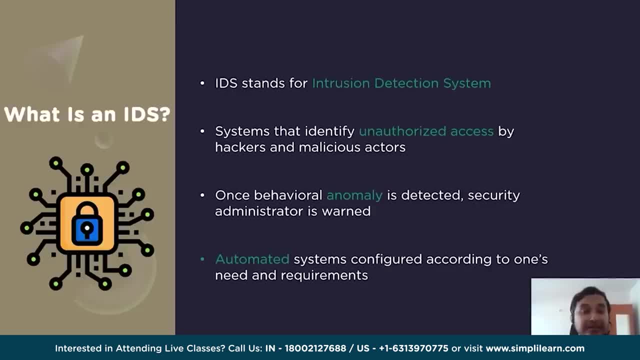 that the IDS doesn't slow down network performance. the solutions often use a switched port analyzer or a text access port to analyze a copy of the inline data traffic so that they do not meddle with the actual traffic. However, they do not block threat once they enter the 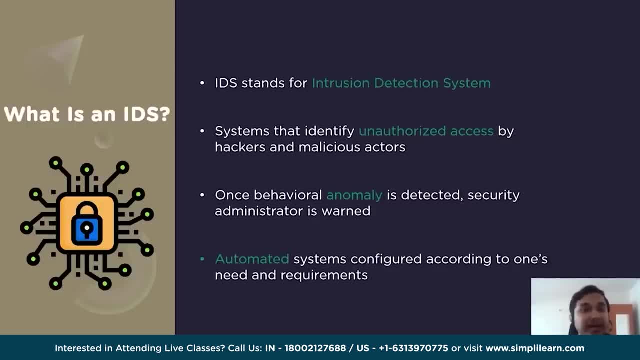 network as intrusion prevention systems do. Regardless of whether you set up a physical device or an IDS program, the system can recognize attack patterns with network packets, monitor user behavior, identify abnormal network activity or ensure user and system activity. do not go against security policies. 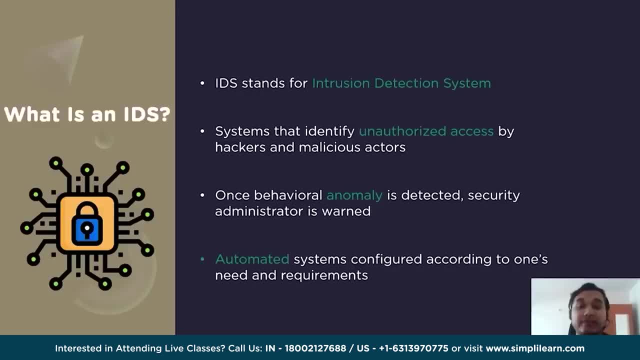 The main goal of an IDS is to detect the anomalies before the hackers complete their objective. Once a system detects a threat, the IT team is informed and the information is passed on. Given the requirement for understanding context, an enterprise has to be ready to make any 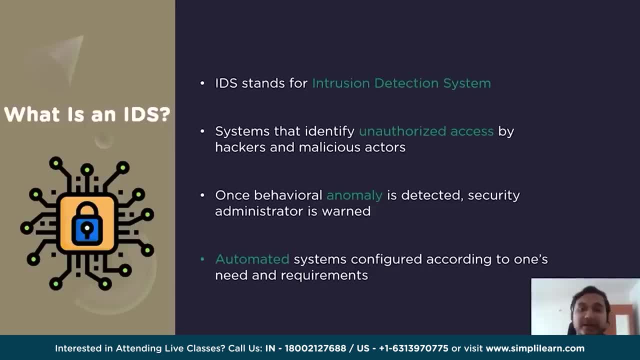 IDS fit its own unique needs, expert advised. What this means is that an IDS cannot be a one-size-fits-all configuration to operate accurately and effectively, And this requires a savvy IDS analyst to tailor the IDS for the interests and needs of a given site And knowledgeable. 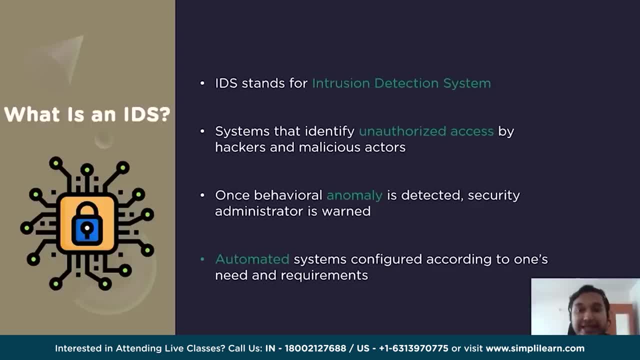 trained system analysts are scarce. The trick with IDS is that you have to know what the attack is to be able to identify it. The IDS has always had the patient- zero problem. You have to have found someone who got sick and died before you can identify it. 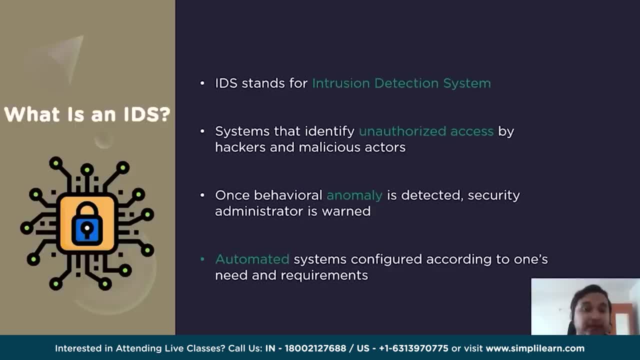 It can usually go for two types of protection: active protection and passive. In a passive system, the IDS detects a potential security breach, logs the information and signals an alert. In a reactive system or an active system, the IDS responds to the suspicious activity by logging off a user. 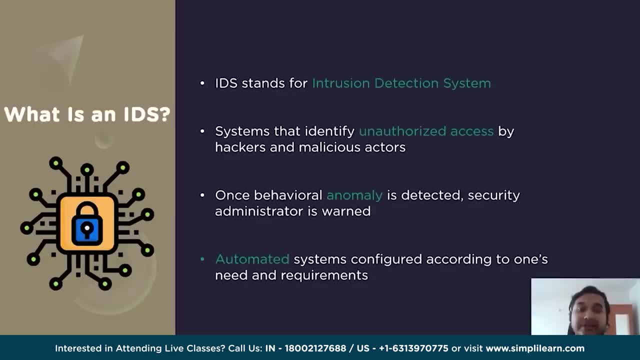 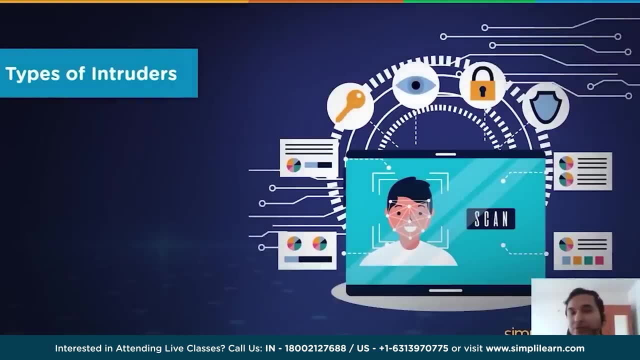 or by reprogramming the firewall to block network traffic from the suspected malicious source. So now that we understand what an IDS is, let us go through the different types of intruders IDS platforms must be aware of. To understand this type of intruders, let us go through a 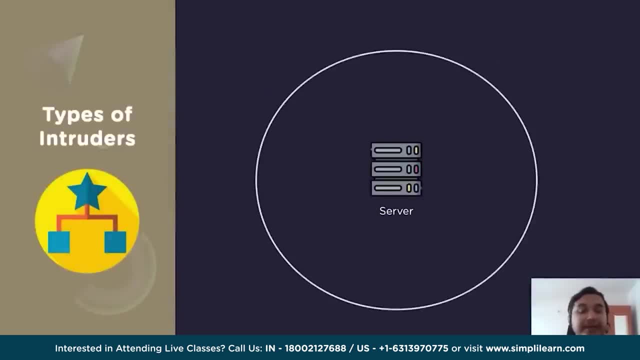 scenario: We have the servers which are protected by the IDS platforms in place. So let's say, a hacker tries to breach the system from outside the organization. This can be done using multiple attacks like DDoS attacks, injection attacks, etc. The 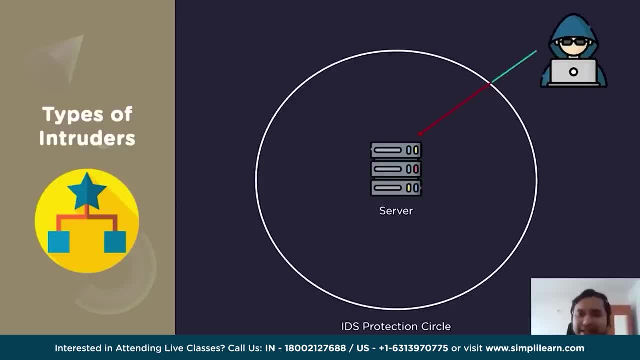 category of individuals that are not authorized to use the system but still exploit users' privacy and confidential information using different techniques, are known as masqueraders. A masquerader is an intruder, that is, an outsider who does not have direct access to the system and aims to attack. 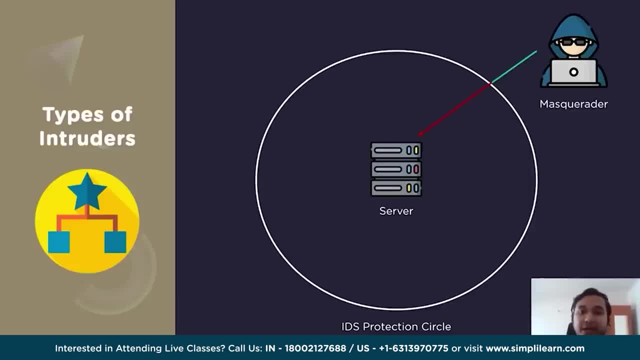 unethically by stealing data or information. However, there is another intruder who is theoretically harder to detect and approve than a masquerader. These are the people within the organization who want to weaken the security defenses, be it for corporate espionage or to aid other masqueraders. 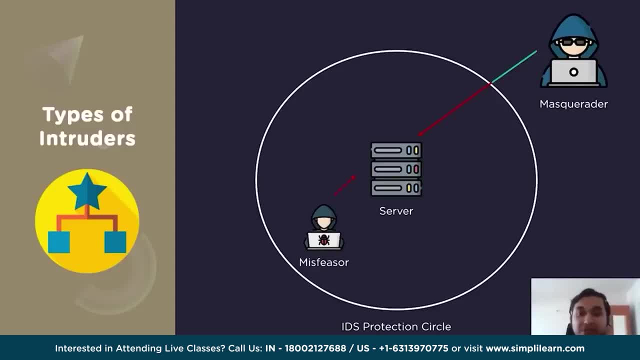 The category of individuals that are authorized to use the system but misuse the granted access and privilege. These are individuals that take undue advantage of the permissions and give access to them, And this category of intruders are known as misfeasors. Misfeasors are people that are insiders. 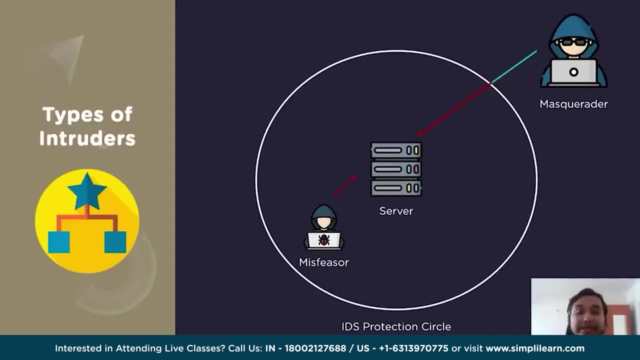 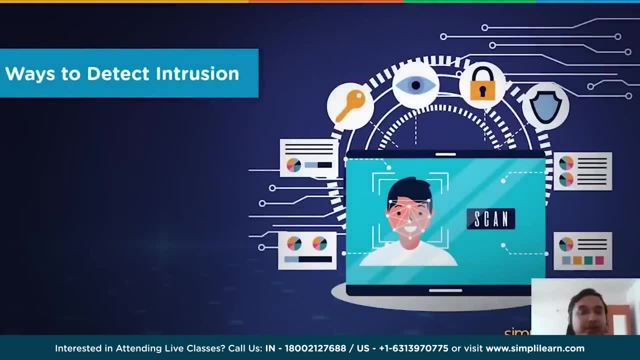 and have direct access to the system which they aim to attack unethically by stealing data or information. Let us now go through some of the ways the IDeas platforms can detect intrusion before it is too late. Intrusion detection systems primarily use two key methods. 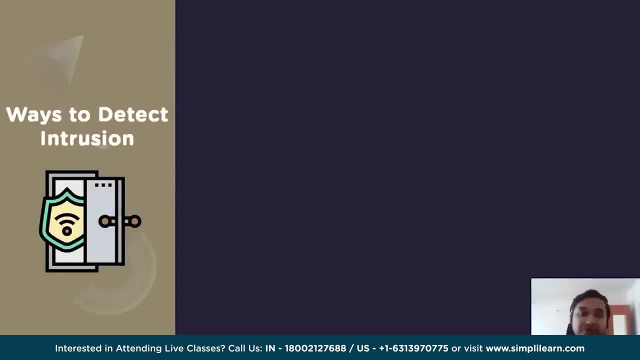 One is signature-based intrusion and the anomaly-based intrusion. Signature-based intrusion detection is designed to detect possible threats by comparing the given network traffic and log data to existing attack patterns. These patterns are called sequences and could include byte sequence, which is also known as malicious instruction sequences. 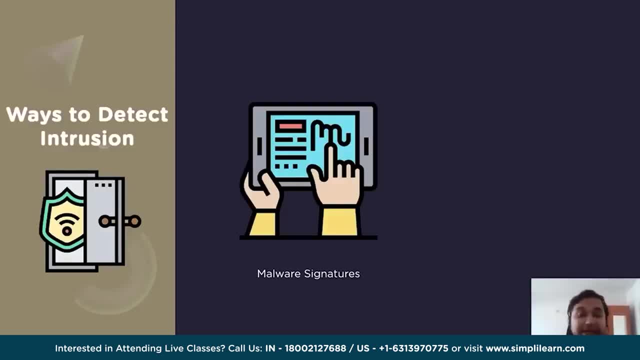 Signature-based detection enables you to accurately detect and identify possible known attacks. Anomaly-based intrusion detection is the opposite. It is designed to pinpoint unknown attacks, such as new malware, and adapt to them on the fly using machine learning. Machine learning techniques enable an intrusion detection system to create. 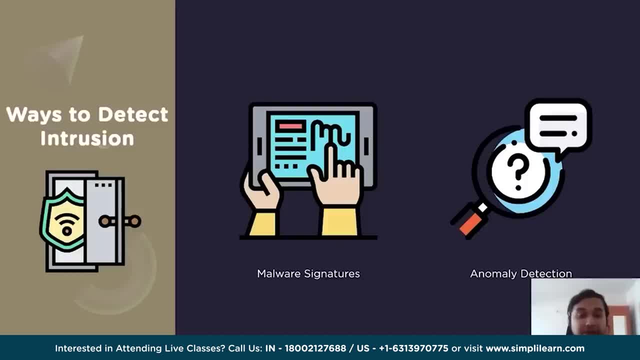 baselines of trustworthy activity, which is known as a trust model, then compare new behaviors to verify trust models. False alarms can occur when using an anomaly-based IDea, since previously unknown yet legitimate network traffic could be falsely identified as malicious activity. Now, if you combine both of those, 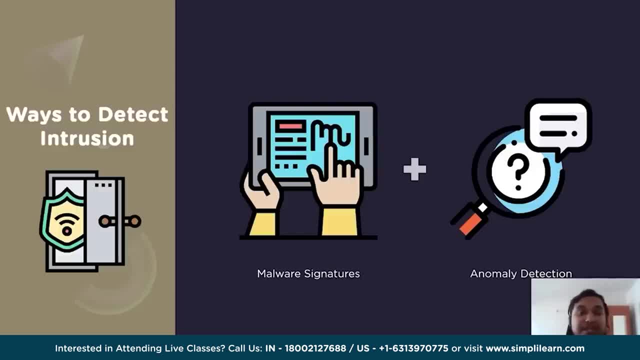 you have the hybrid intrusion detection. They use signature-based and anomaly-based intrusion detection to increase the scope of your IDea. This enables you to identify as many threats as possible. A comprehensive intrusion detection system can understand the evasion techniques cyber criminals use to trick an IDea. 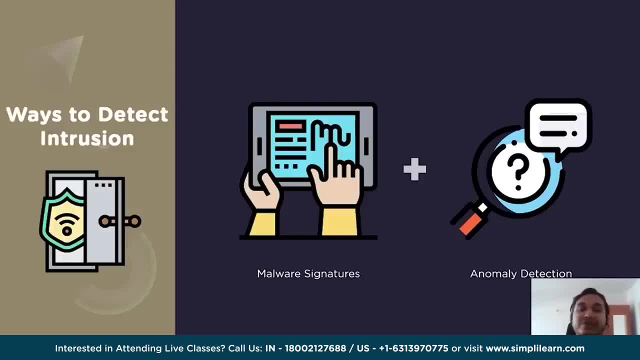 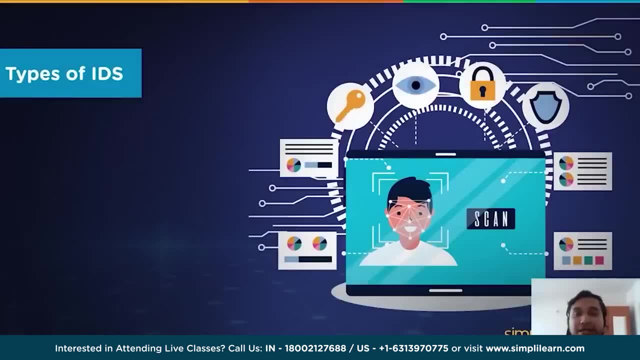 to thinking there isn't an attack taking place. These techniques could include fragmentation, low bandwidth, attack pattern change, evasion and many more. We can now take a look at the type of protection offered by IDea's platforms. There are a couple of ways that can be. 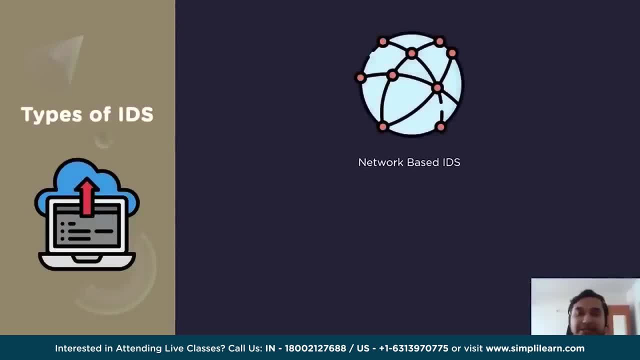 set up. so let's go through each method. The first is a network-based IDea. The sensors are deployed at strategic points within the network, such as within the DMZ at the network's perimeter. The sensor can monitor individual packets of inbound and outbound traffic. 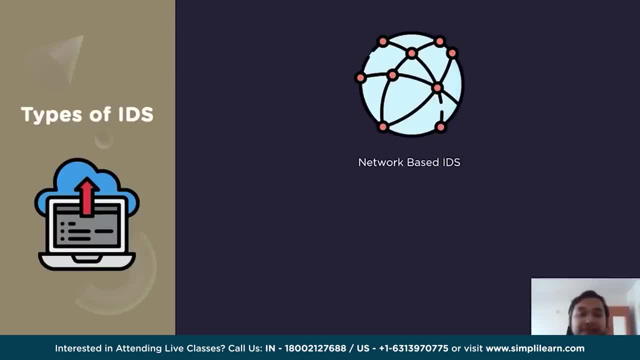 to and from all devices on the network. It analyzes them for malicious activity and, depending on the network architecture and amount of traffic involved, multiple instances of network-based IDea's may be necessary. The second category is host-based intrusion detection systems, or HIDea's. 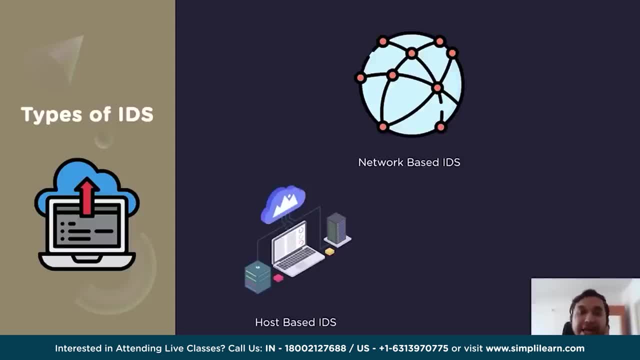 An agent runs on all servers, endpoints and devices in the network that have access to both the internet and the internal network. Intuitions are identified by analyzing operating specific activities like the modification of the file system registry or access control list. 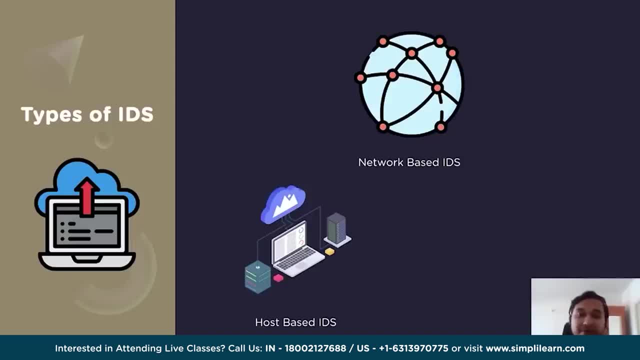 And the monitoring system application logs as well. They augment network-based IDea's systems by detecting anomalous traffic which originate within the organization or from the host that is being monitored, For example, a host infected with malware that is attempting to spread it to other internal hosts. 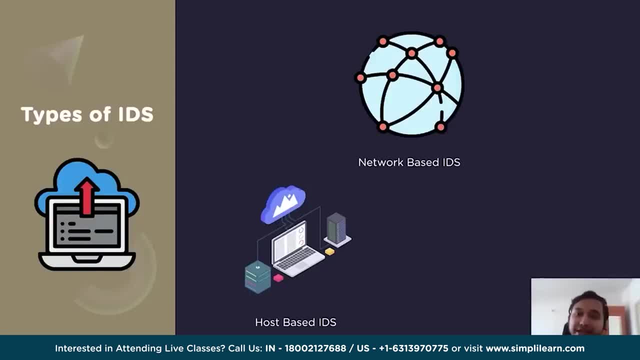 is an issue that your network-based IDea's could potentially fail to detect. The third variant is the cloud-based intrusion detection system. Because of the internet-facing nature of the cloud, on-premises IDea solutions are not necessarily optimized for monitoring. 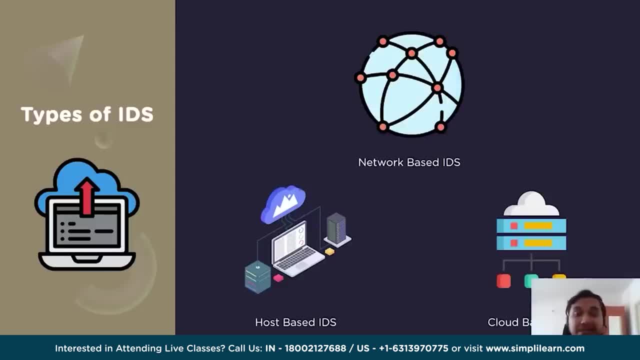 For example, network-based sensors need to be deployed within the cloud at an environment's network perimeter, and yet a cloud service provider may or may not have a way to facilitate this. Cloud-based servers use purpose-built cloud sensors that use cloud service provider application programming interface. 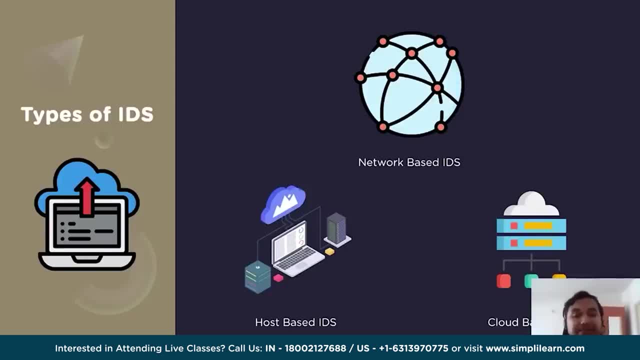 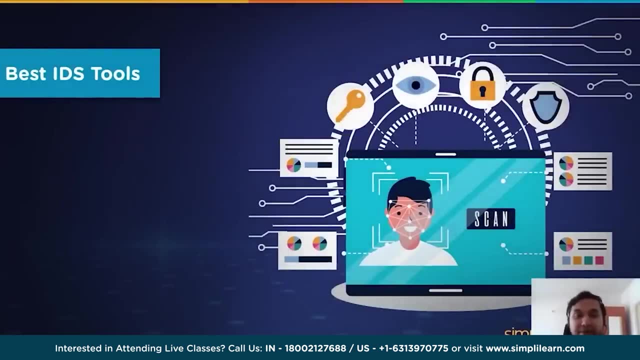 or cloud service provider APIs to get as much visibility as possible into your cloud environment. Now that we understand the different types of IDea's deployment tactics, let us go through some tools that excel in this field, offering top-of-the-line implementations in a corporate and 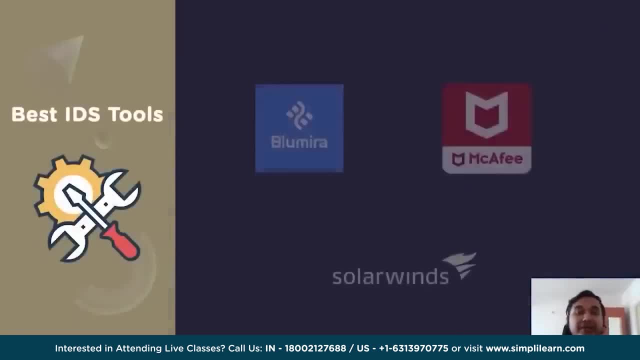 consumer environment. The first tool being covered is the SolarWinds Security Event Manager. The SolarWinds Security Event Manager is designed to integrate real-time log data from across the infrastructure, enabling it to act both as a network-based IDea system and a host-based IDea system. 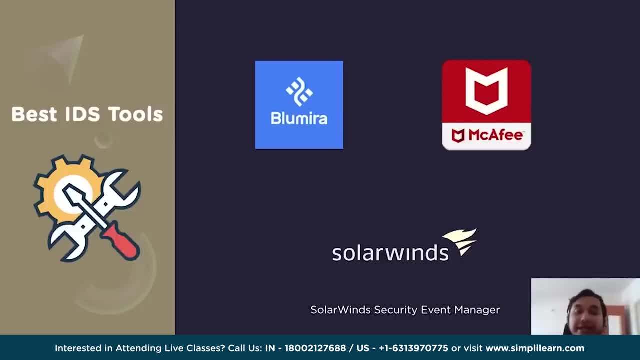 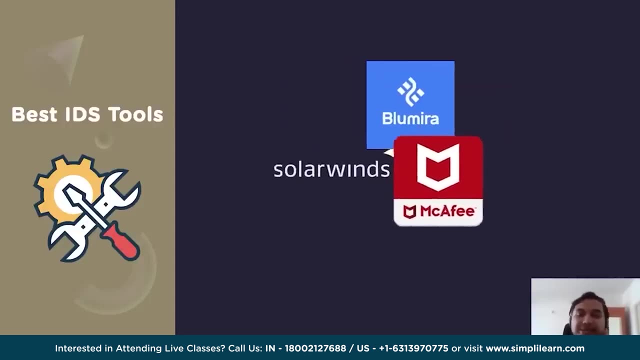 The solution can let you discover all kinds of malicious attacks and help you protect your network from harm. It is also designed to enact both signature-based and anomaly-based intrusion detection by comparing sequences of network traffic against a set of customizable rules. Next we have the McAfee LiveSafe. 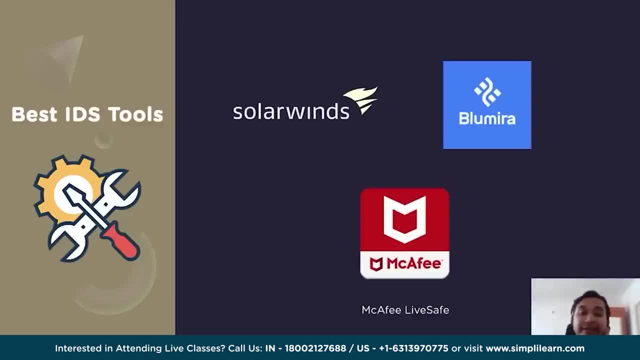 McAfee LiveSafe is an intrusion detection system designed to bring your real-time threat awareness to your physical and virtual networks. It uses signature-based intrusion prevention and anomaly-based intrusion detection, along with emulation techniques, to spot and identify malicious activity. McAfee is also built to correlate. 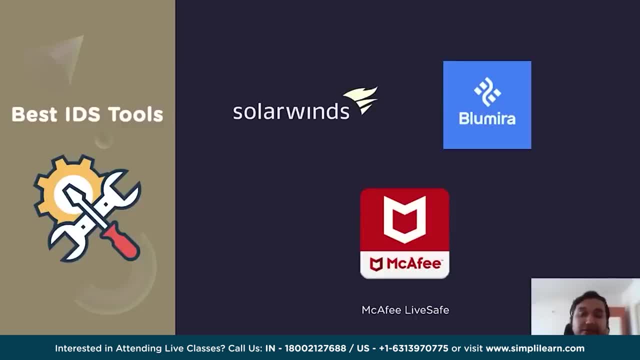 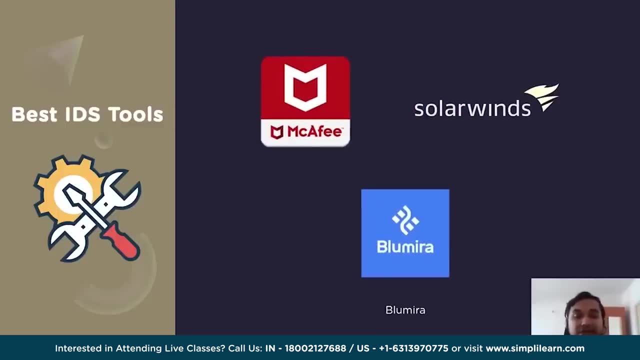 threat activity with application usage which can further prevent network issues stemming from cyber attacks. Next, we have Blumera. Blumera is a security information and event management platform built to enact threat detection and responses across your cloud and on-premises environments. 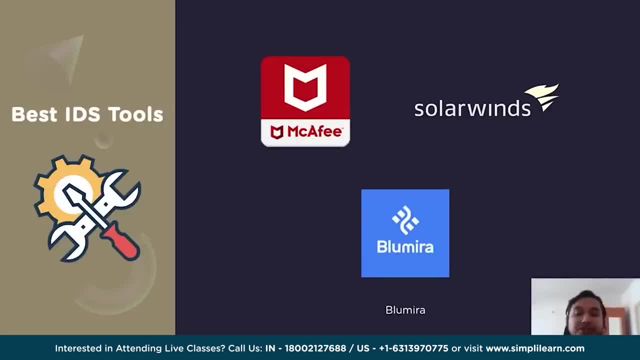 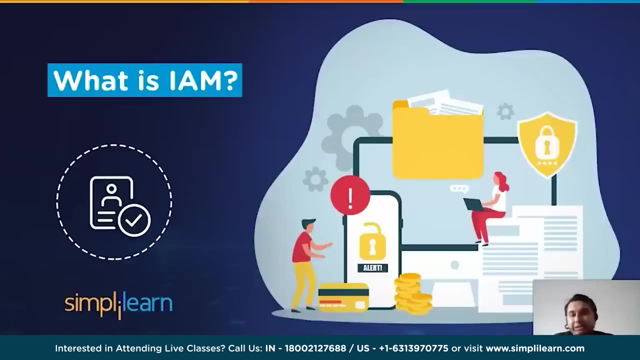 It is designed to continuously monitor your IT infrastructure for suspicious activity and misconfigurations, both of which could result in data leaks and compliance breaches. It enables you to respond to an attack in progress and stop malicious actors in their tracks. Monitoring usage of corporate data. 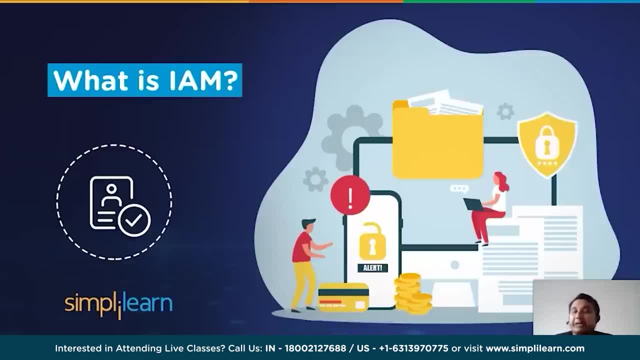 and access to privileged information had been a daunting task before the advent of IAM. Encompassing numerous APIs, single sign-on frameworks and data handling policies, IAM has established itself as a key component of every IT department, But how does it enforce these rules? 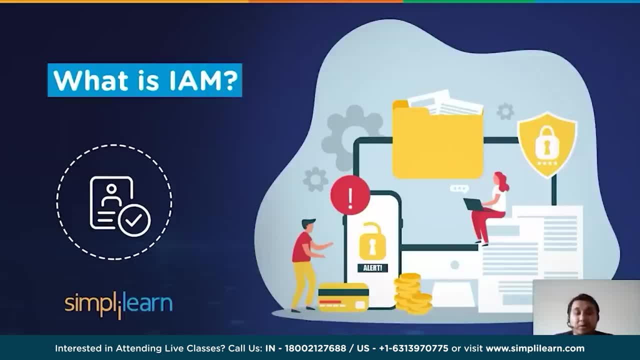 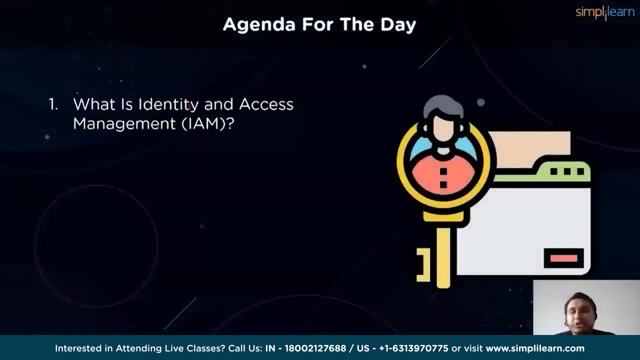 And who are the key benefactors of these policies? What about the advantages of these frameworks and the workflow of these systems? We are here today to answer these questions. Let's take a look at some of the topics to be covered today. We start by learning about IAM. 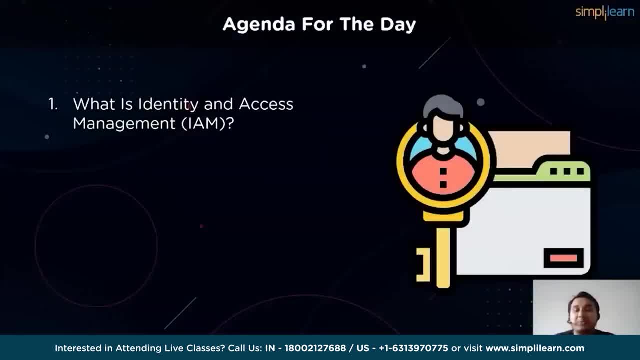 that is, Identity and Access Management from a surface level, so as to put a clear idea of what it is. Next, we cover the general workflow and process of how IAM works. Moving on, we cover some of the tools that find their place in an IAM framework. 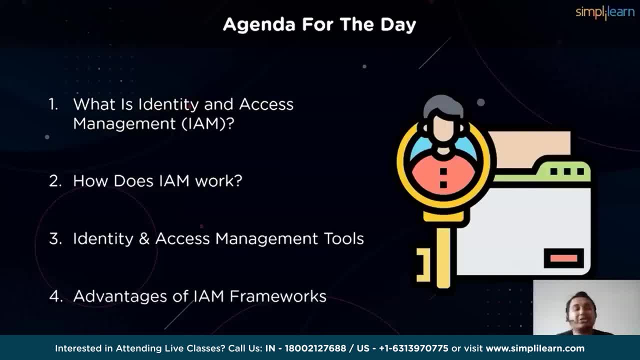 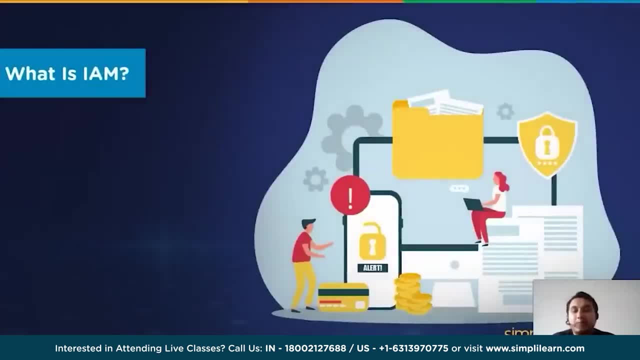 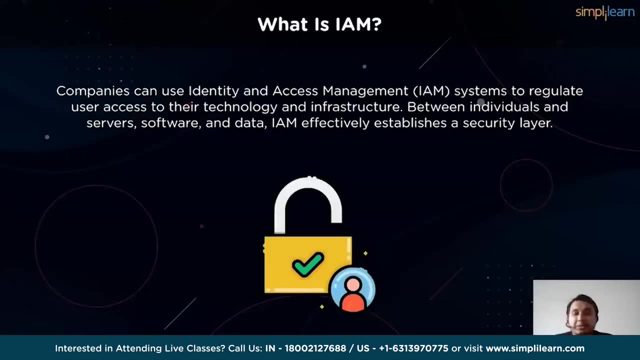 and are crucial components. Finally, we go through some of the advantages of the IAM learning what makes them a lucrative deal for organizations. So let's get started by learning about IAM from a surface level perspective. Identity and Access Management, or IAM, is a set of processes. 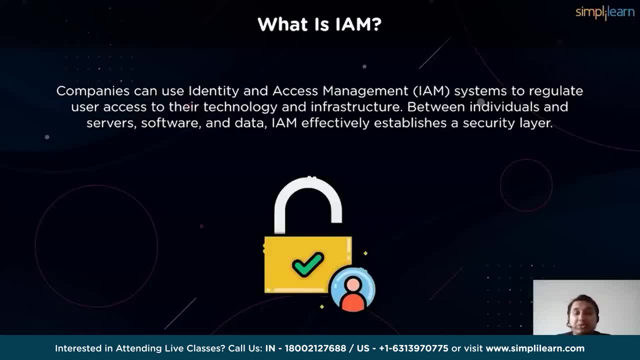 policies and tools for defining and managing the roles and access privileges of individual network entities to a variety of cloud and on-premise applications. The users can include customers, partners, employees, devices like computers, smartphones, routers, etc. The core objective of IAM systems. 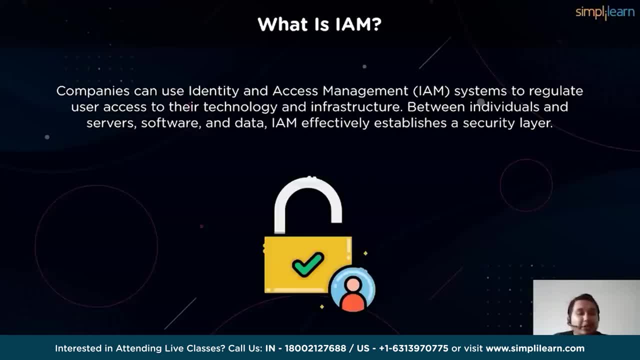 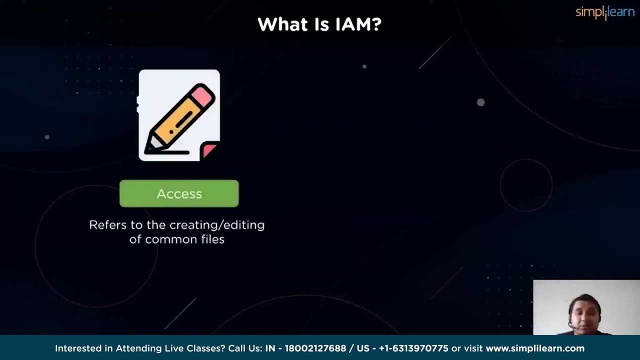 is one digital identity per individual or item. Once a digital identity has been established, it must be maintained, modified and monitored throughout each user's access lifecycle. Access and user are two vital IAM concepts. Access refers to the actions permitted to be done by a user like view. 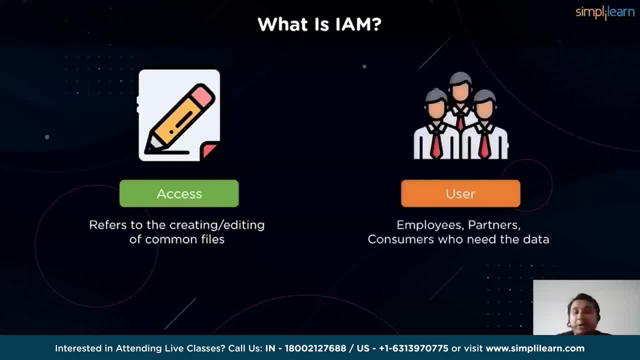 create or change a file. Users could be employees, partners, suppliers, contractors or even customers. Furthermore, employees can be further segmented based on their roles. IAM systems are designed to perform three key tasks: identify, authenticate and authorize, Meaning that only the right person 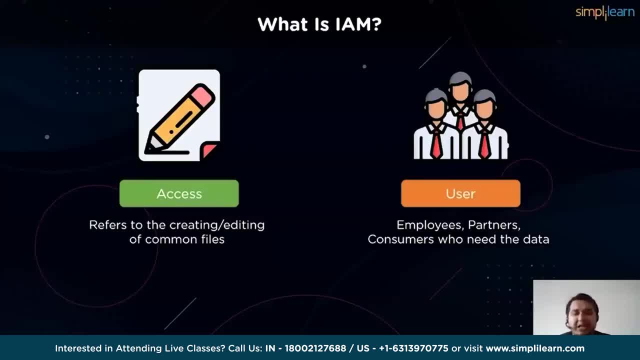 should have access to computers, hardware, software, apps, any IT resources, etc. For the entry of new users or the changing of the roles of existing users. the list of access privileges must be up to date all the time. IAM functions usually fall under. 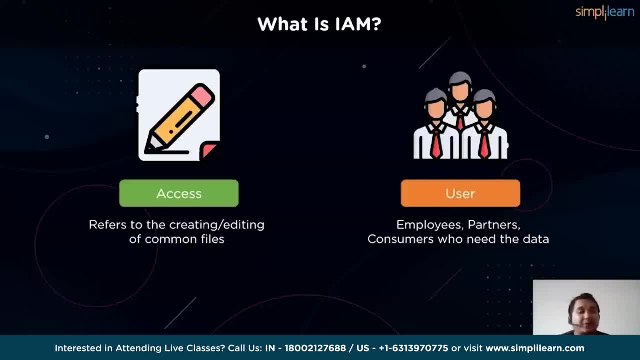 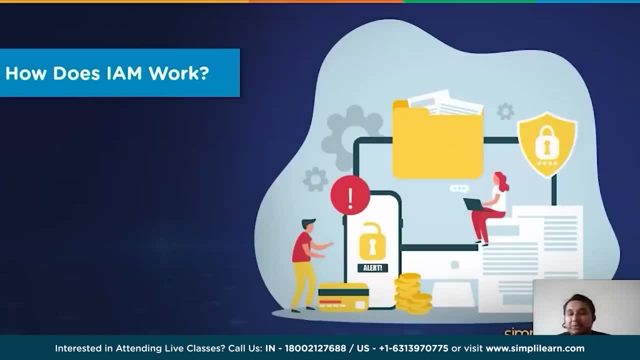 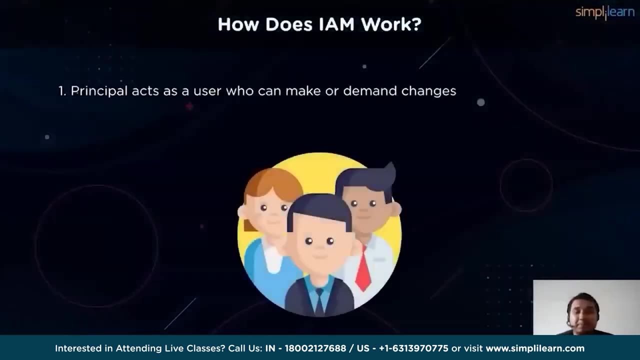 IT departments or sections that handle cybersecurity and data management. Now that we understand the importance of IAM in today's cybersecurity sphere, let us understand the process of this framework. We have multiple components that aid this process. Let's start by going through each of them individually. 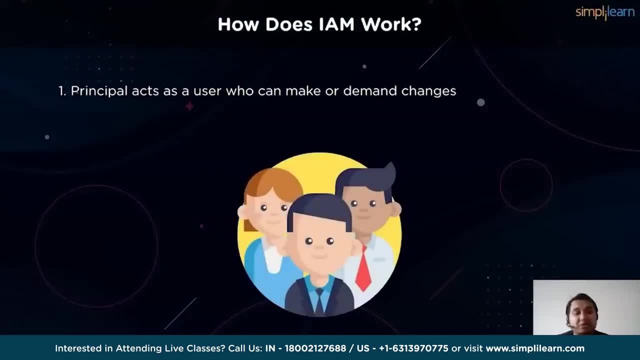 Principal is an entity that can perform actions on an AWS resource or any cloud management system. A user, a role or an application can be a principal. It's always the principal who raises a concern to access or modify data on servers, serving as the first point of contact in the IAM. 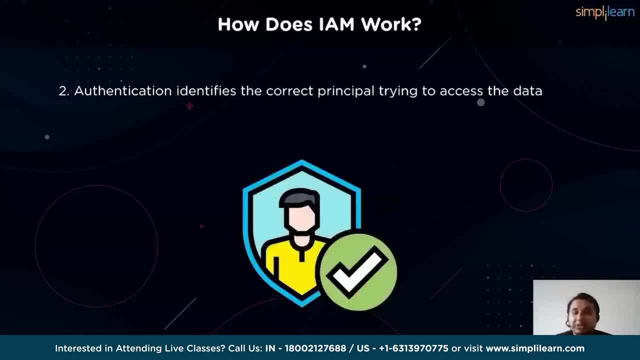 workflow. Authentication is the process of confirming the identity of the principal. trying to access the product, The principal must provide its credentials or required keys for authentication. This step can be further enhanced by multiple authentication factors and geologs, among other things. Once the identity is confirmed, 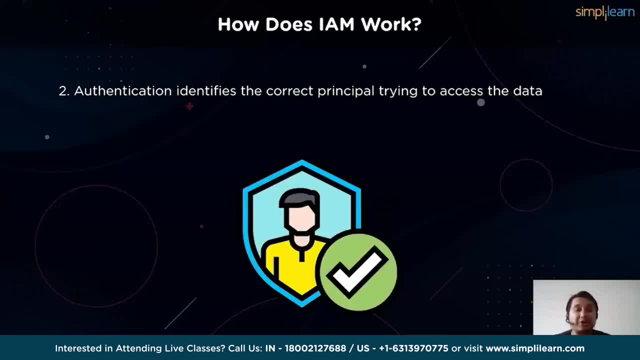 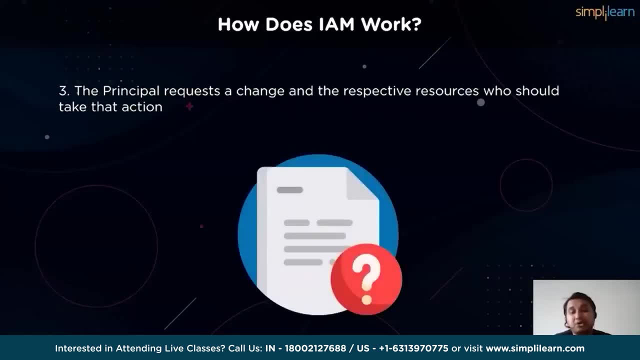 the principal has the ability to view the data behind the wall of security and take the necessary steps. When it comes to requests, a principal then sends a request to the cloud management system specifying the action and which resource should perform it. In this step, the user can ask to. 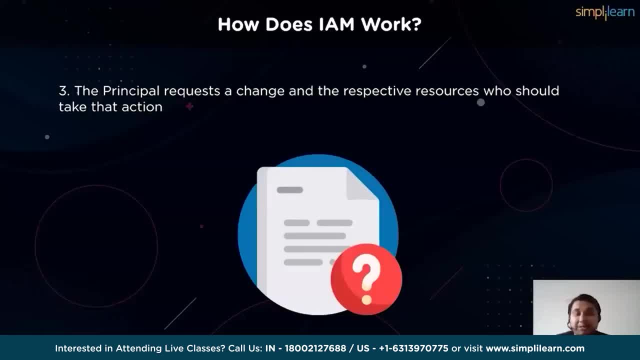 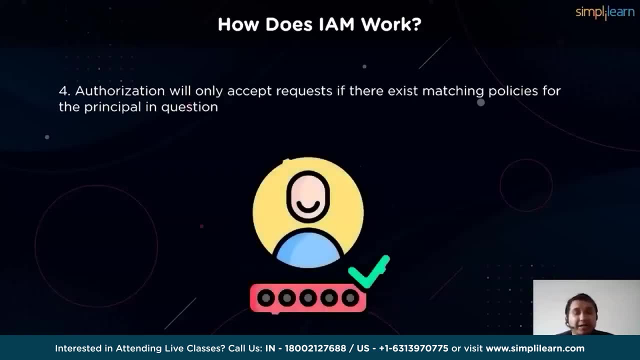 modify, delete, edit or affect other users in this particular bucket of organization by changing the data or the information. When it comes to authorization, it carries out the rest of an organization identity and access management processes. once the user has been authenticated, Users are granted. 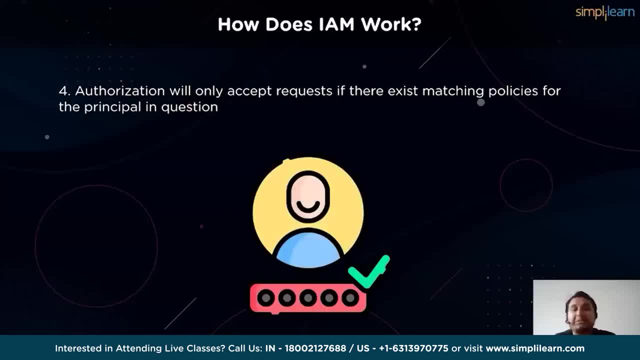 authorizations according to their role at an organization. The practice is referred to as Role-Based Access Control or RBAC. Authorizations determine a role's resources and level of access in the network. These items may include systems, applications, file shares, printers and more. 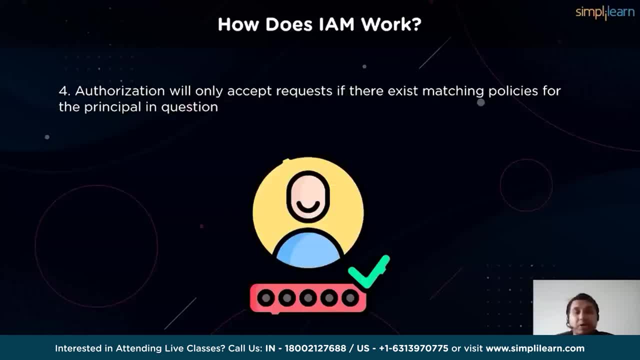 For example, an accounting department employee who regularly works with payroll software must be authorized to do such. If authentication resembles a passport, these are the things your digital identity can access with it. While authentication is fully straightforward, authorizations and their management are far more challenging. 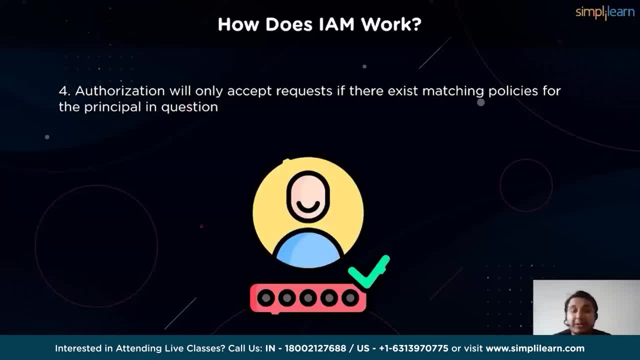 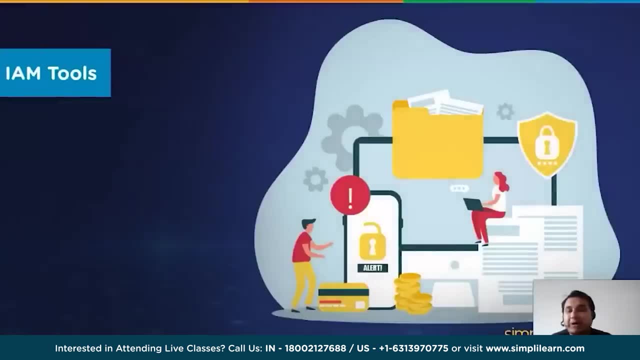 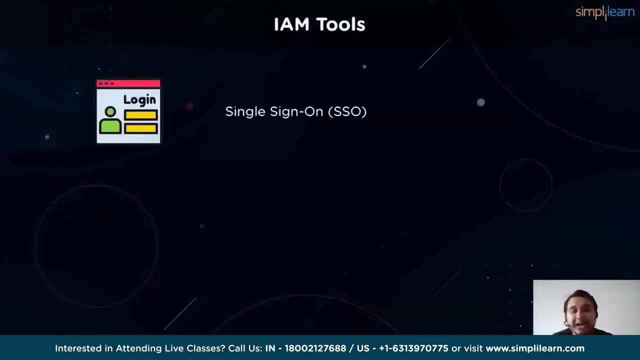 Authorizations consist of complex set of rules and policies and groups which are permitted to be explicitly configured per user account. With the working of IAM frameworks out of the way, let's cover some of the tools that these systems work on. SSO is an IAM tool. 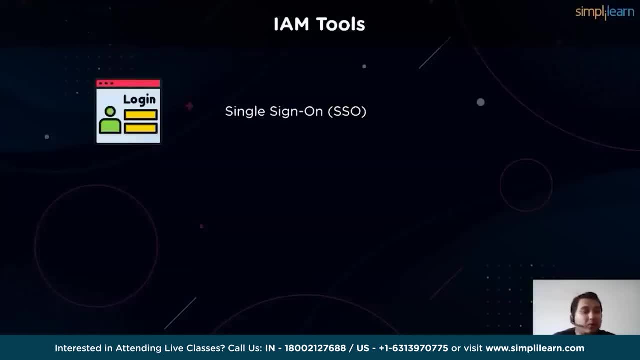 that enables a user to log into one organization's properties and automatically be logged into a design set of other properties. For example, when you log into Google, you're automatically logged into your Gmail and your YouTube accounts. Similarly for users, single sign-on reduces friction. 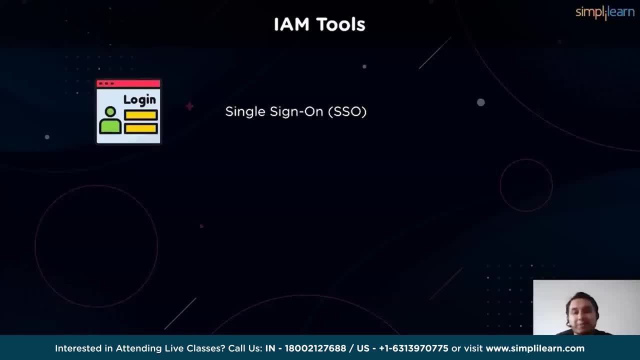 since they don't have to keep track of different credentials for every application. For organizations, SSO helps in collecting valuable insights about user behavior and preferences, since it tracks them as they move from one application to another, connected by one single login. Next is Multi-Factor Authentication. 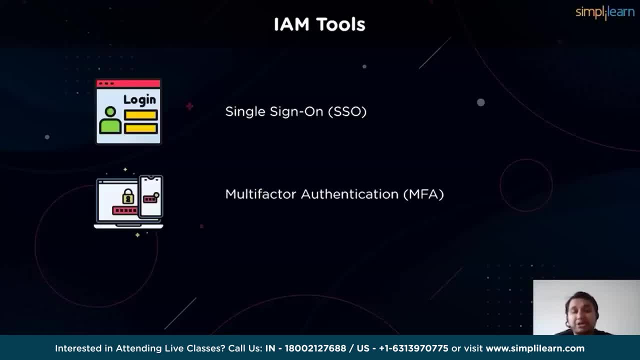 or MFA. Implementing multi-factor authentication is crucial to protect your organization's data from malicious intrusions, and virtually every IAM platform offers some form of MFA. However, it's equally crucial to customize MFA with the appropriate level of security, For example, in business-to-consumer scenarios. 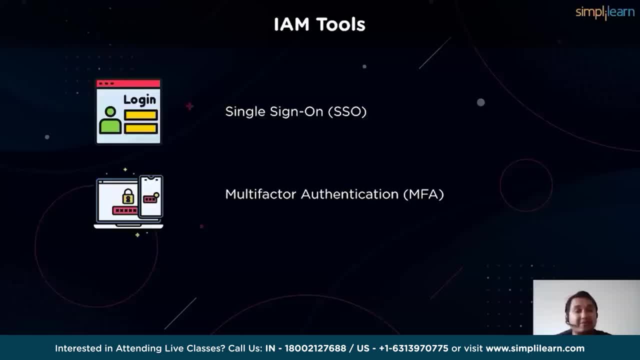 you need to consider UX and try not to create unnecessary friction for users who don't want to be subjected to heightened scrutiny every time they log in For workforce IAM. you may want a more stringent MFA, since the consequences of an unauthorized party gaining access to your private network. 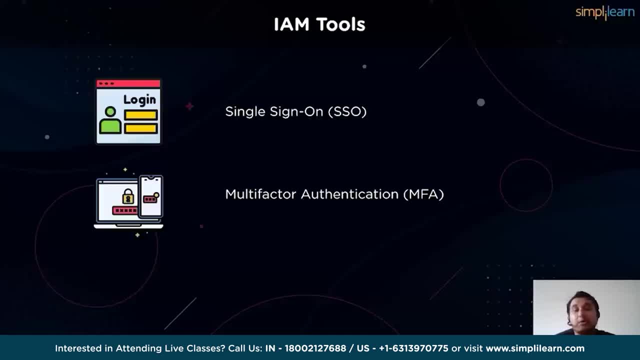 can be so devastating. A modern IAM solution will allow you to implement MFA only when it's needed. This can be accomplished through setup authentication or adaptive authentication, in which users only trigger MFA if they are trying to access sensitive data or their behavior is flagged as risky. 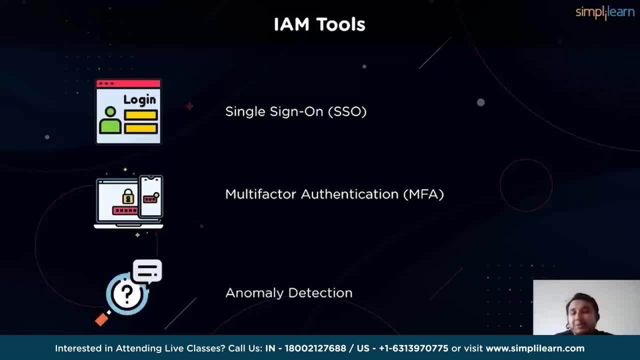 In the past few years, identity has become the preferred gateway for hackers to break into systems. Brute force attacks, credential stuffing attacks and even highly targeted phishing campaigns are all attempts by hackers to break in through a company's front door, which is the login box. 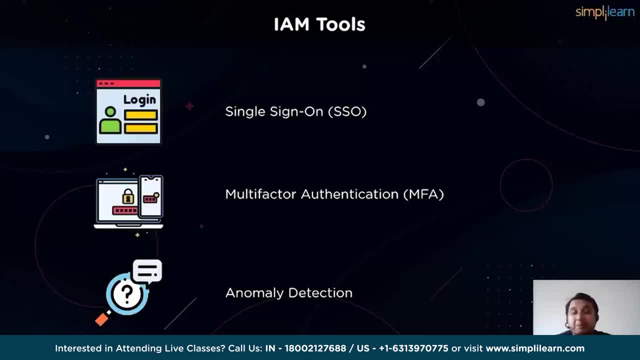 These IAM systems can help detect and mitigate these malicious attacks. IAM solutions detect attacks by monitoring signals such as the velocity of traffic, detection of login patterns that differ from a user's routine use of a breached password, use of devices and IP addresses with a poor reputation. 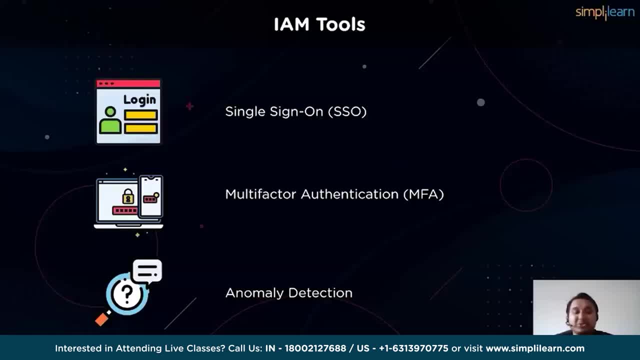 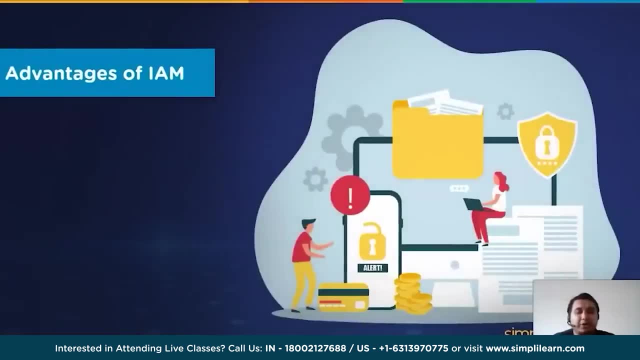 among other things. These are some of the most widely used tools when it comes to IAM frameworks, But why do we go through setting up so many tools and firewalls? Let's go through some of the advantages of using IAM systems in both corporate and private environments. 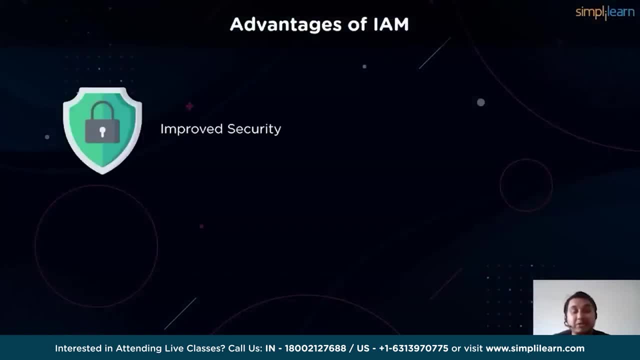 IAM solution helps identify and mitigate security risks. You can use IAM to identify policy violations or remove inappropriate access privileges without having to search through multiple distributed systems. You can also leverage IAM to ensure that security measures are in place to meet regulatory and auditing requirements. 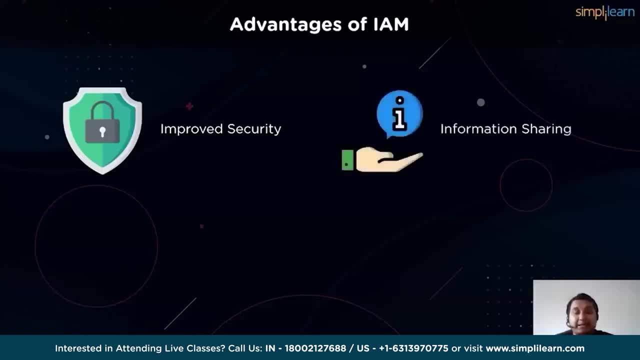 IAM provides a common platform for access and identity management information. You can apply the same security policies to operating systems and devices used by the organization. The IAM framework can help you enforce policies related to user authentication, privileges and validation and attend to the privilege creep problems. 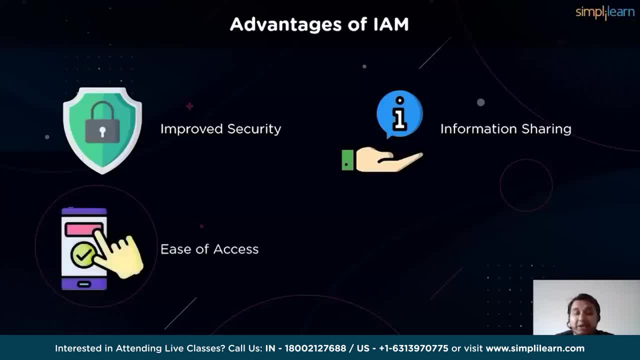 IAM simplifies signup and user management processes for application owners, end users and system administrators. It makes it simple to provide and manage access and promotes user satisfaction. IAM services can also lower operating costs. Using federated identities services means you no longer need. 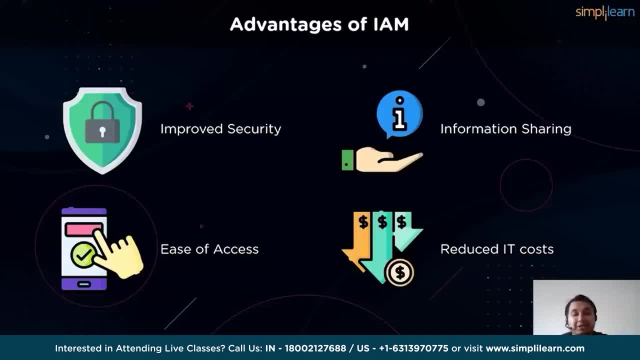 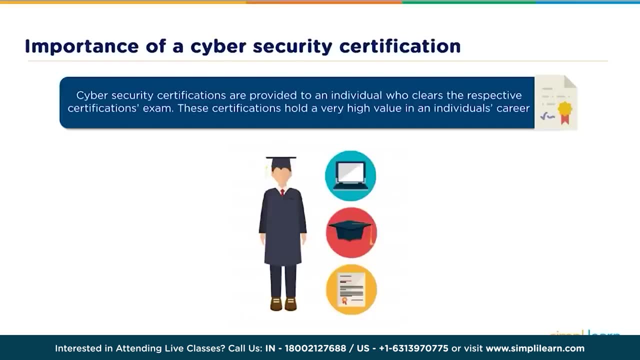 local identities for external users. This makes application administration easier. Cloud-based IAM services can reduce the need to buy and maintain on-premise infrastructure. So importance of a cybersecurity certification First and foremost. when I see a certification, I look at it from three different aspects. 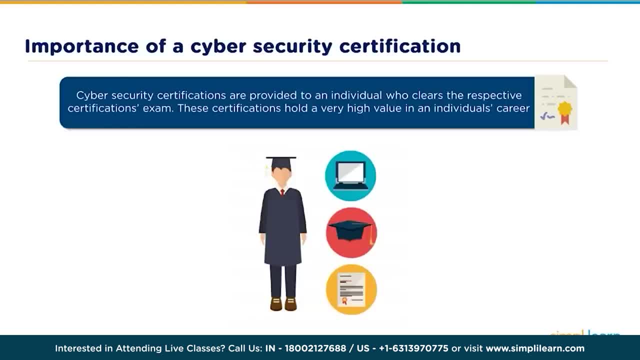 The first is the training itself, which allows me to gain the knowledge which allows me to understand the aspects of security or whatever the certification is there for. How do I need to prepare myself for the exam And how do I need to approach the exam? 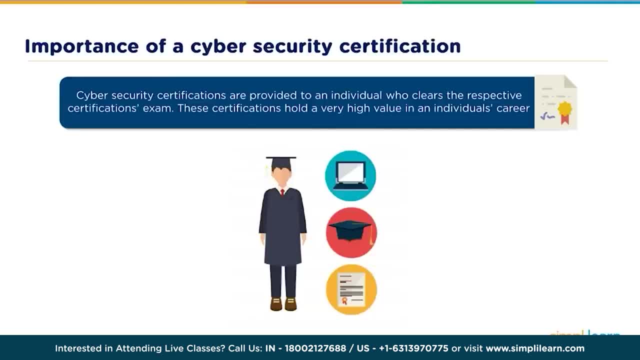 How do I need to ensure that I pass in my first attempt? And the third aspect is the certification itself, which allows me to be eligible to apply for a particular job role. So obtaining a cybersecurity certification ensures or shows to the organization that you are applying to. 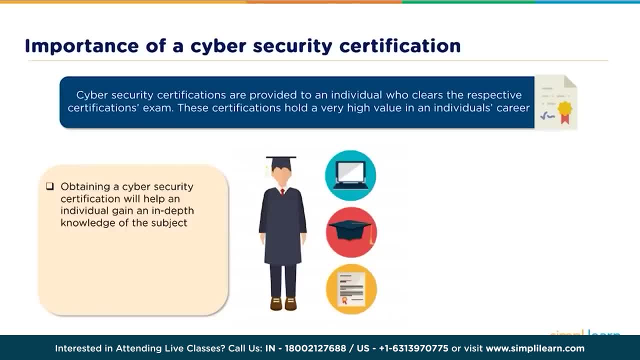 that you do have that prerequisite knowledge and you should be shortlisted for an interview. The knowledge that you have gained during the training will help you when you attend that interview and when you attempt to answer the questions asked to you. So these certifications are designed. 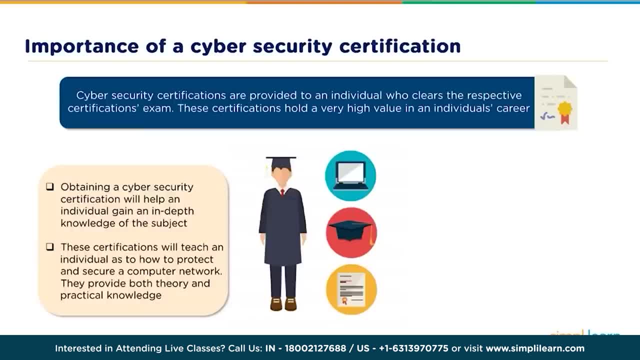 for a specific role. For example, a forensic investigation certificate will teach you how to investigate a crime scene forensically- a digital crime scene, for a matter of fact. A certified ethical hacking course will teach you about penetration testing. So it is you who is going to decide. 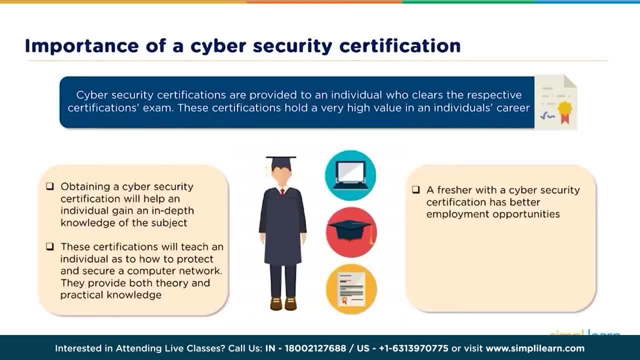 which certification you require and then attempt to get certified on it. Of course, a fresher with a cybersecurity certification will give you opportunities because they can showcase their knowledge with the certification that they already have. Even professionals who want to enhance their careers can get into managerial or advanced certifications. 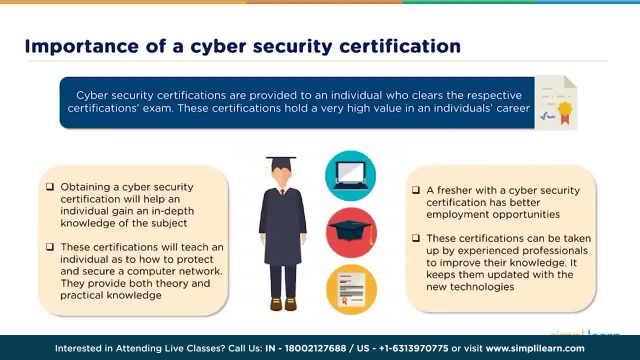 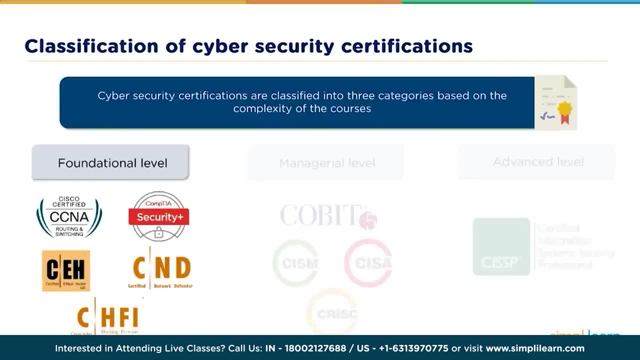 to improve on their knowledge and get promoted in their job profiles. So cybersecurity certifications can be classified in three different aspects, The first one being the foundational level, then the managerial level and the advanced level. In the previous video we just had a small overview. 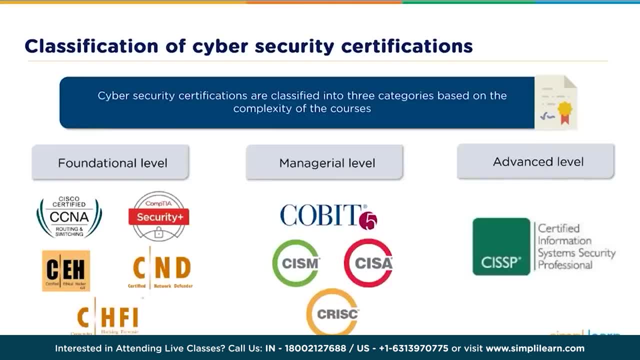 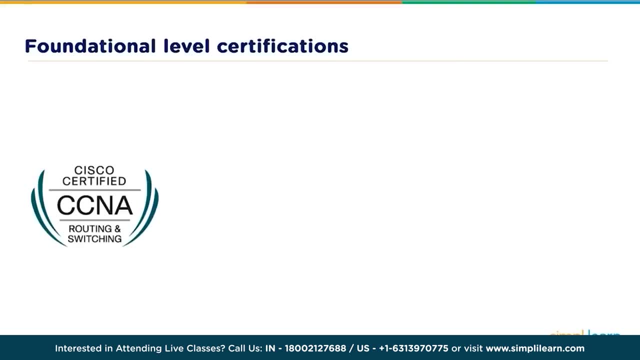 Here we are going to discuss about what the certification covers, how the exams are conducted and the price points for each and every exam. So let's start with the foundational certifications. We start off with CCNA, which is the basic certification for networking. 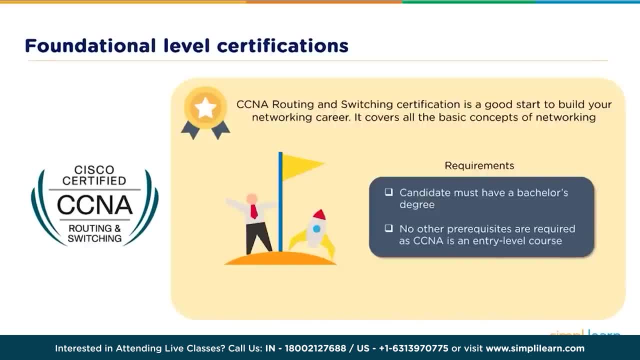 So the CCNA routing and switching certification basically helps you build your networking career. You will join an organization as a networking engineer where you can help the organization establish the routing, the pathing, of how data packets will travel across the network. This certification covers: 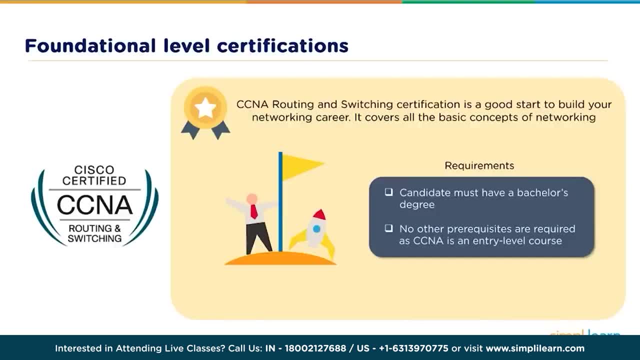 all the basic concepts that you require to understand networking. The basic requirements for this certification are that the candidate must have a bachelor's degree, but apart from that there are no other prerequisites. So it's just that you need a bachelor's degree. 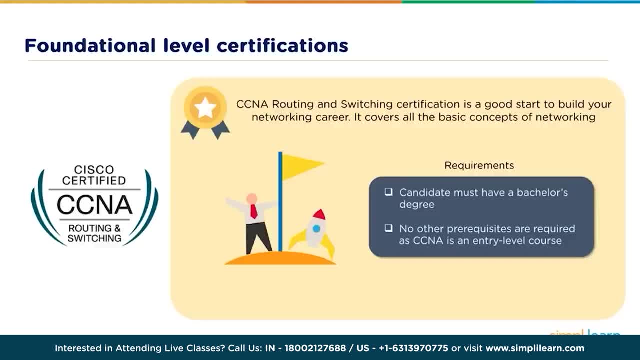 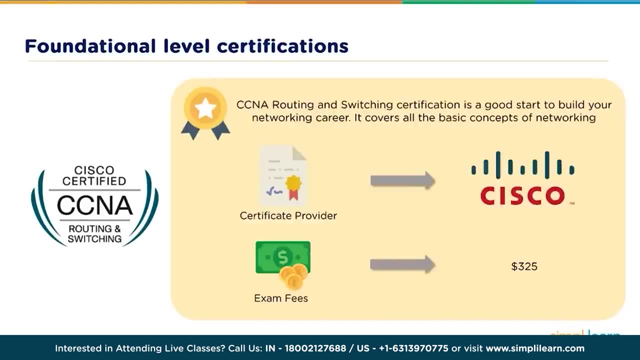 and then you can apply, you can study for this, you can undergo a training and then you can attempt the exam. The certification provider, obviously, is Cisco, so the knowledge that is limited to this training and certification is for Cisco devices only. The exam fees for this certification. 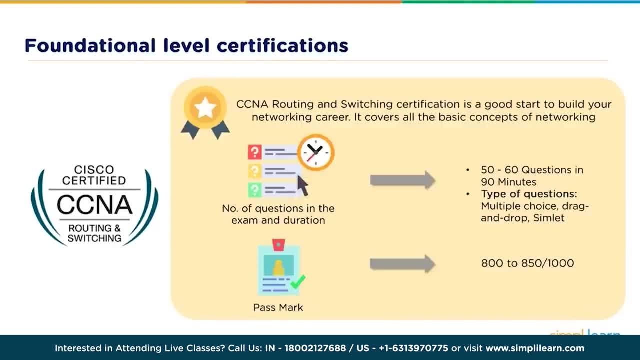 is approximately $325.. The course is conducted. it has around 50 to 60 odd questions which need to be answered in 90 minutes. The type of questions that you are going to get is multiple choice questions, where you have a question and four answers. 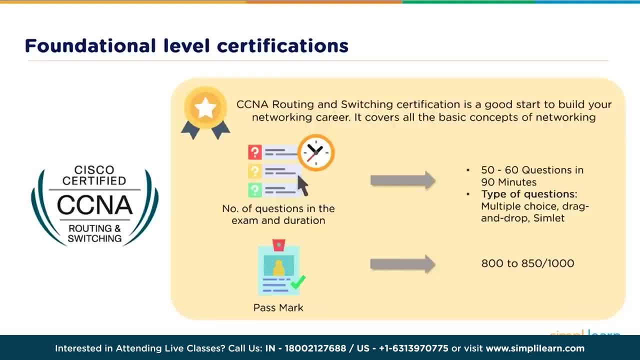 and you have to choose the correct answers among those Drag and drop, where you have to click on an object and drag it to its appropriate place- probably an architectural diagram- and you have to, let's say, pick on a router and place it into a particular position. 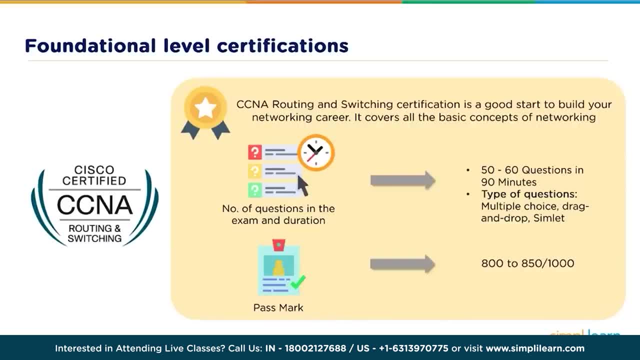 If you place it correctly, you answer the question correctly. otherwise it's wrong. You can also use a calculator where there could be a configuration. you need to configure it in a particular manner and then check whether the configuration is correct or not. The pass mark is around 800 to 850. 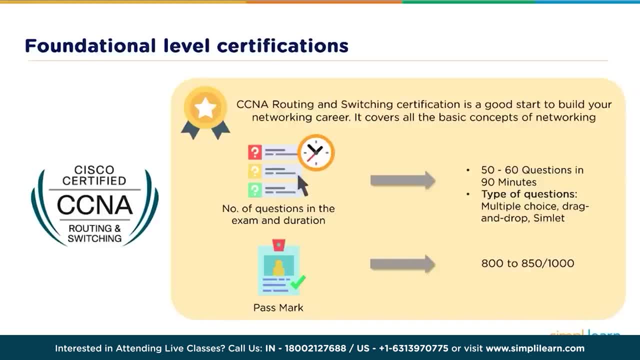 out of a possible 1000 marks. So each question will have a different weightage, depending on the depth of the question, depending on the difficulty level of the question or the difficulty level of the question, which would then count towards your marks. and if you score, 800 to 850. 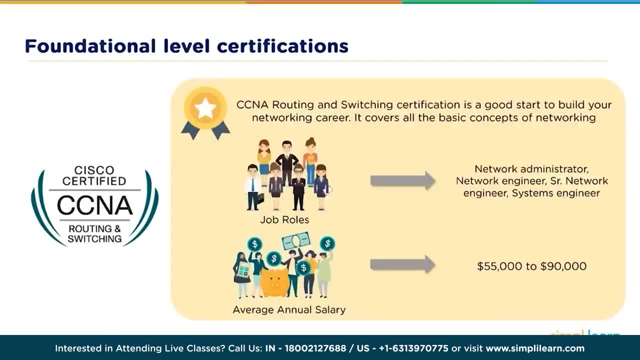 that's when you clear the exam. The job roles, as we have discussed over here, would be more on the network administrator side or the network engineer side, depending on the level of experience that you have. The salaries that are expected from these job roles in the US. 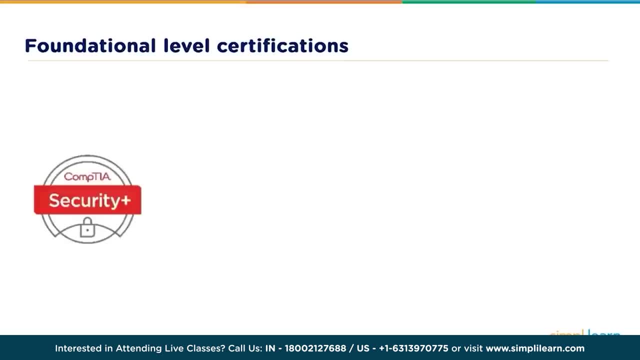 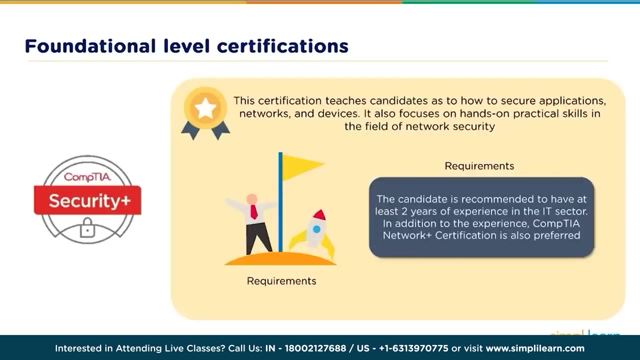 are around $55,000 to $90,000 annually. The next one is the Comcha certification, called Security Plus. Comcha is also a global certification authority for infosec courses, So this certification teaches candidates on how to secure applications, networks and devices. 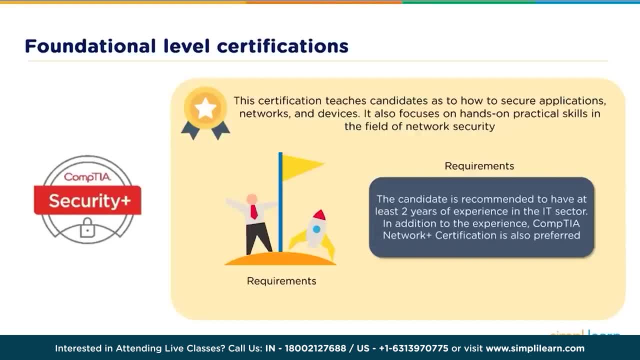 It focuses on hands-on practical skills for network security. I have trained people on this certification myself so I know this certification is quite hands-on. It deals with the concepts to the core. It helps you understand the concepts and then in the practical hands-on demo. 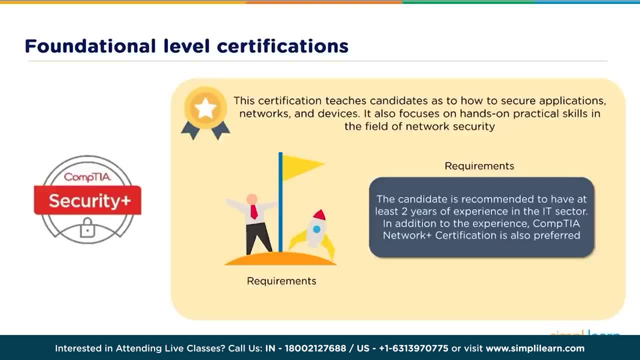 you need to execute the practical yourself so that you can gain that knowledge. The recommended level for a candidate to attempt this training would be at least around 2 years of experience in the IT sector. In addition, if you have already been certified for Network Plus certification from Comcha. 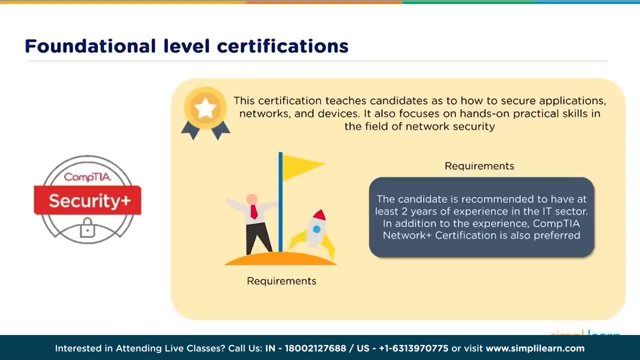 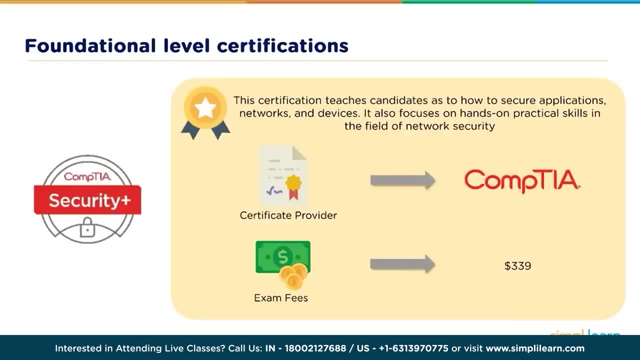 which is the baseline networking certification. this is also a preferred way to go for this certification. As said, Comcha is the certificate provider and the exam fees for this certification is $339.. The exam is quite simple: 90 questions in 90 minutes. 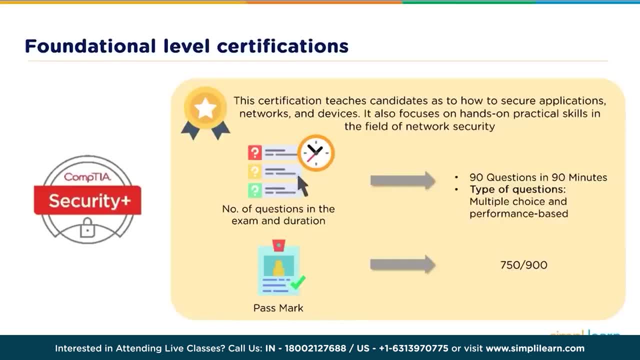 That's one minute per question. It sounds like a lot of time but, believe me, the questions can be a little bit confusing, can be a little bit lengthy, so you will require all those 90 minutes to answer those questions, Especially when they are tricky and they are technical in nature. 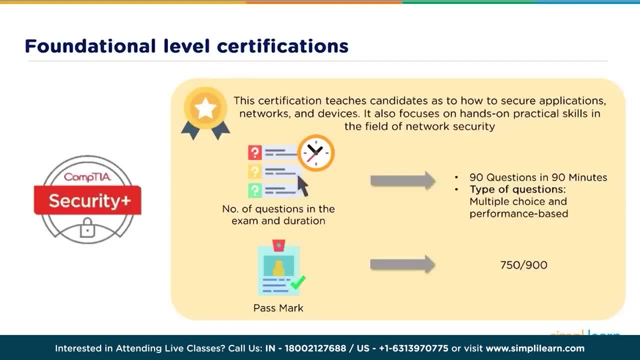 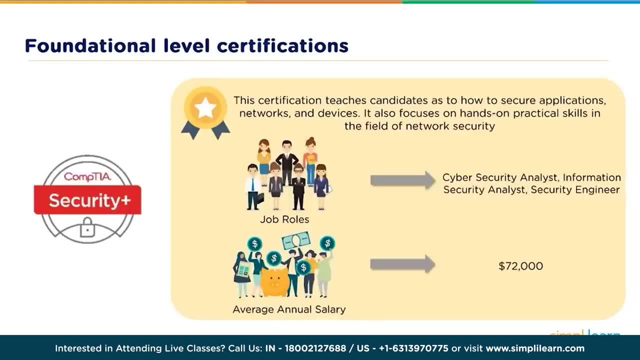 The questions would be multiple choice and performance based. The pass mark for this exam is around 750 points out of a possible 900.. The job profiles for this kind of certification is when you want to apply for a security analyst position or a security engineer's position, where you are going to. 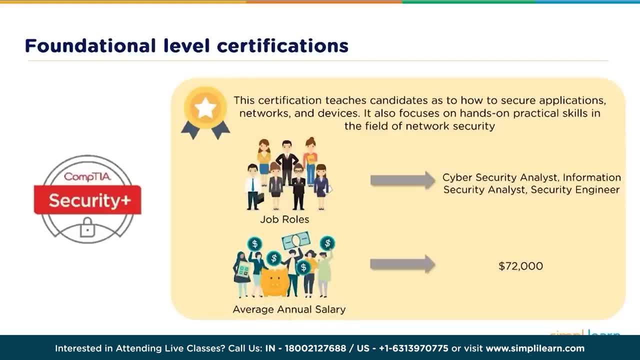 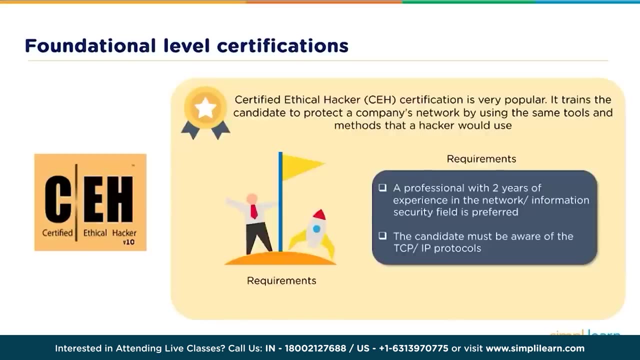 analyze some data to understand and figure out what problems are ongoing in the organization. The average annual salary of this person would be around $72,000.. Then comes the CEH, or the Certified Ethical Hacker training from EC Council. Now, this is a very well known course. 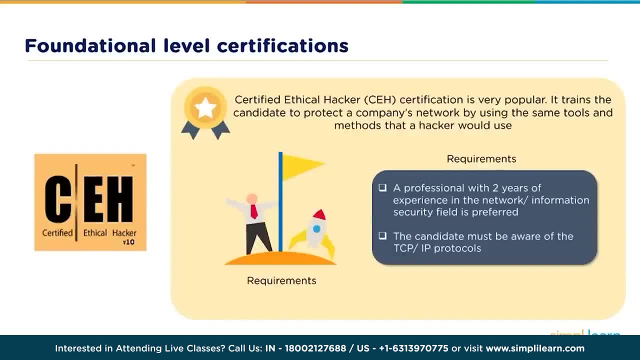 and also EC Council is a global certifying authority very well accepted across a lot of countries. This is an offensive certification. so here you are basically trying to become a penetration tester. You are taught how to hack. you are taught how to attack a particular organization. 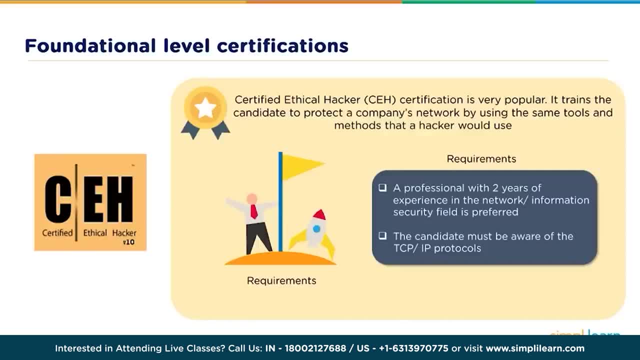 from an ethical hacker's perspective. So the job profiles that you will be looking here are of a pen tester, where you go into an organization, you test their security controls or you test their devices, find out flaws within them and then provide recommendations of how to plug those flaws or mitigate. 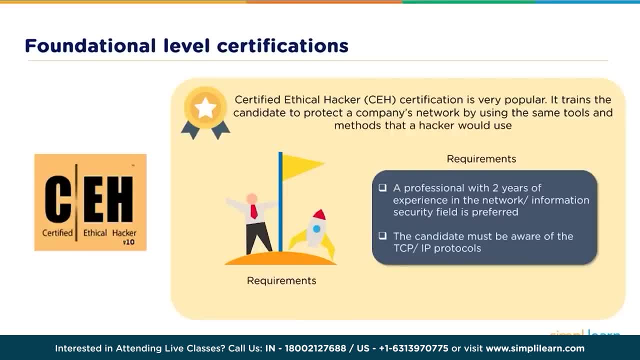 those flaws and improve the security of that organization. It is recommended that you have two years of experience at least in networking or security to attempt this kind of trainings and certifications. Again, a basic understanding of networking, maybe a little bit of applications, operating systems, would be necessary. 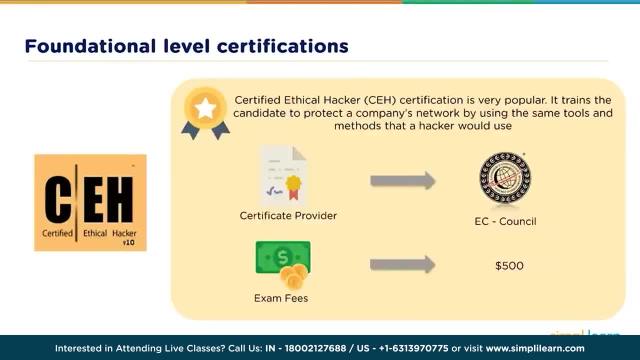 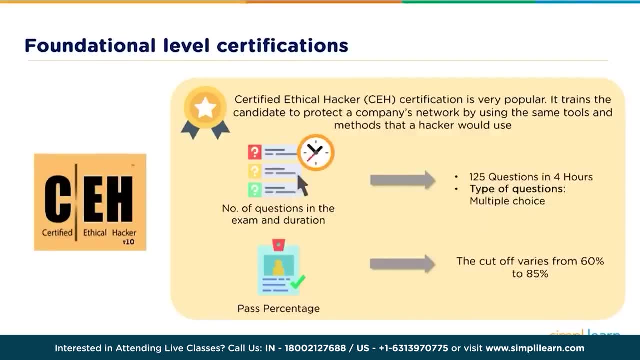 before attempting this certification. The certification provider is EC Council and the exam fees for this certification is $500.. So the exam here would be 125 questions, which needs to be attempted in four hours, and you will only get multiple choice questions in here. Now for CEH. 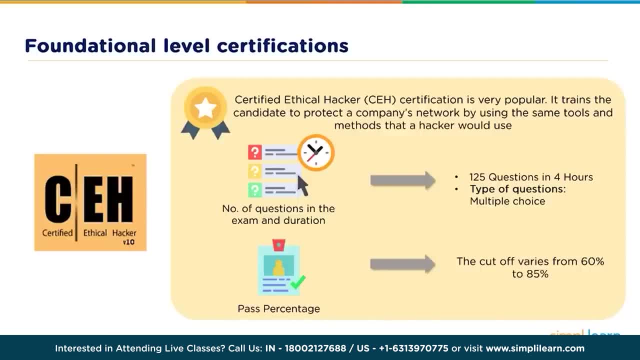 there are two exams. One is the multiple choice questions and the second is a practical exam where you need to solve some given problems to you in an iLab scenario, and if you are able to solve them properly, you then get certified for CEH. practical- The cutoff varies. 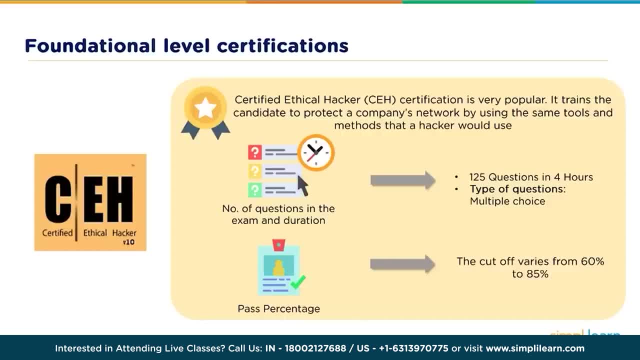 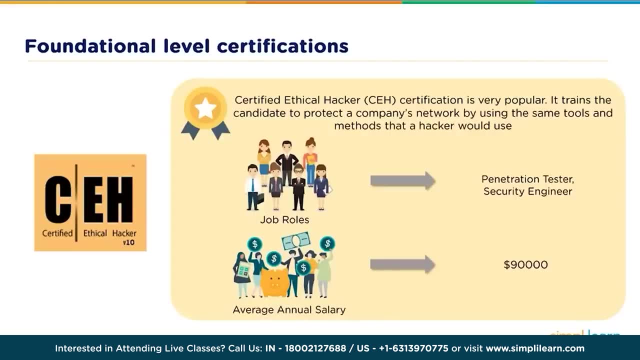 from 65 to 85%, depending on the questions that you have answered and the weight percentage associated with each and every question. As said, the job roles would be as a penetration tester or security engineer, and your salaries would start from around $90,000 annually. 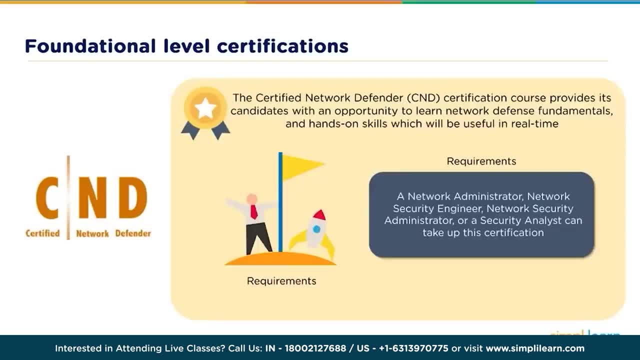 Then comes the CND or the Certified Network Defender, also from EC Council. Now this is more on the network defense side. so here again the job roles would be where there is a network that you have and you are going to try to secure the network and the communications that are going. 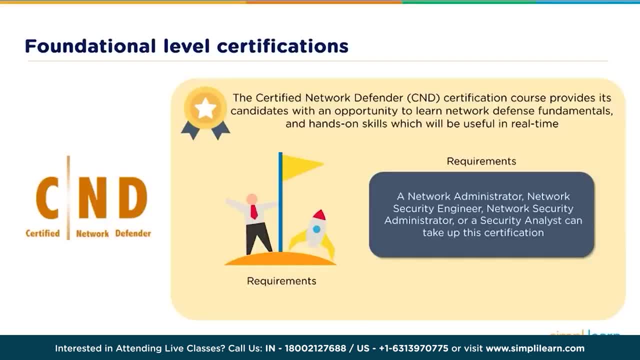 to travel over the network. So you need to be a network administrator, a network security engineer or in a simple similar profile to understand how networks work and then you are going to attempt to secure those networks. The certificate provider again is EC Council and the certification is placed a. 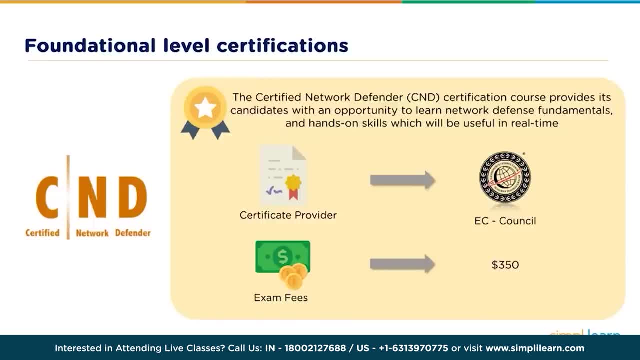 little bit below CEH, so it becomes network defense, then CEH, where you are going to become a penetration tester. The exam fees for this certification is $350 US dollars. The exam is of 100 questions to be answered in 4 hours. Again, it's just a multiple choice. 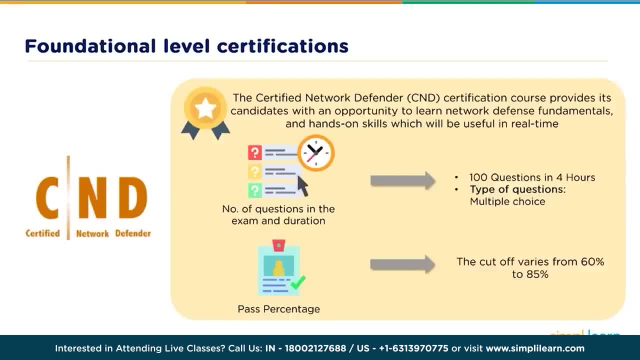 questions. so you get a question with 4 options, you answer the correct one and you move on to the next question. The pass percentage again varies from 60 to 85%, depending on the questions answered and the weightage of that question. Job roles to be applied. 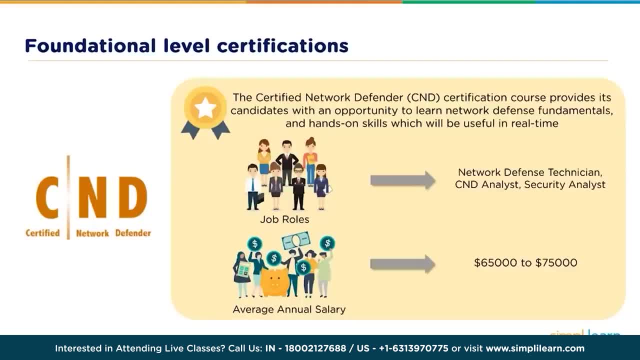 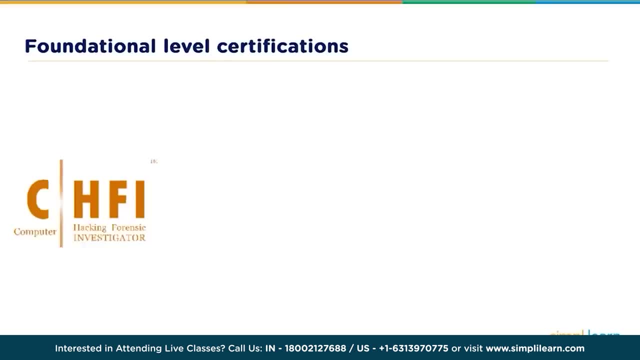 network defense technician, C&D analyst or a security analyst from a network perspective, Salaries would range from $65,000 to $75,000 per annum. Then comes the forensic investigator course, which is exactly what it is: digital forensic investigator. This will help you understand. 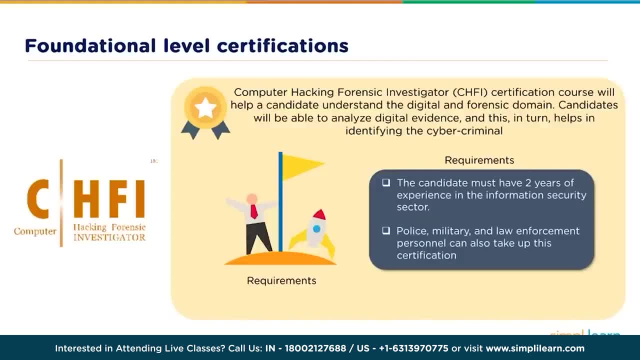 how computers work, where data is stored and how you can retrieve that data to investigate a crime that has taken place. So the candidate must have at least 2 years of experience in the information security sector. They need a good understanding of how networks work, how computers work, how. 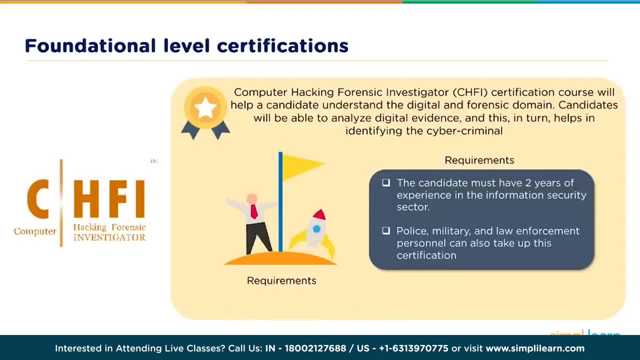 operating systems work, how they store data, the location where that data is stored, how databases work, how those databases store those data, and so on and so forth. This certification is sought after mainly in the law enforcement areas, but there are a few corporates that offer. 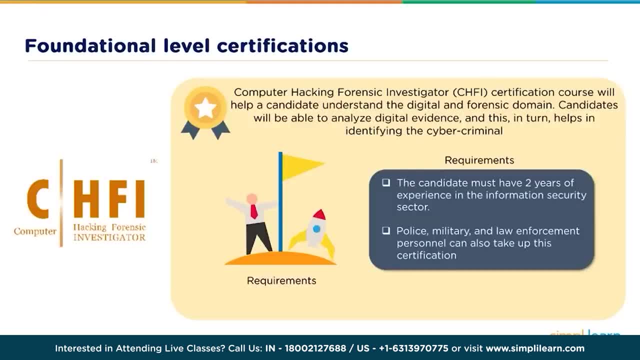 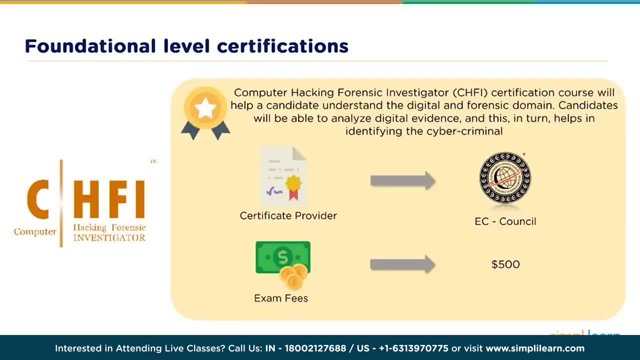 forensic investigation as a service, Especially when a corporate gets compromised and they want to conduct their own investigations. The certification provider for this is also AC Council and the exam fees are $500.. This is an advanced level certification, so understanding of applications, networks and 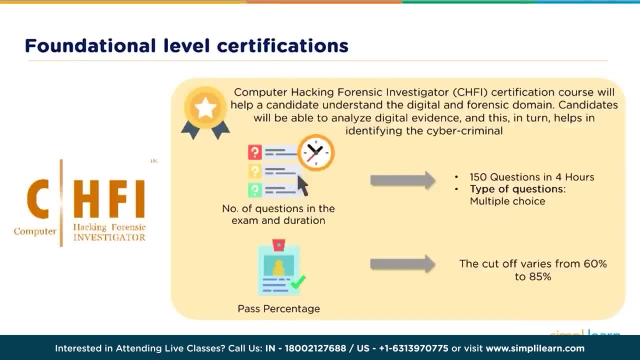 operating systems is a must before you attend this. The exam is quite similar: 150 questions in 4 hours. Again, it's just a multiple choice question exam. The cut off again is from 60% to 85%, depending on the questions and the weightage of. 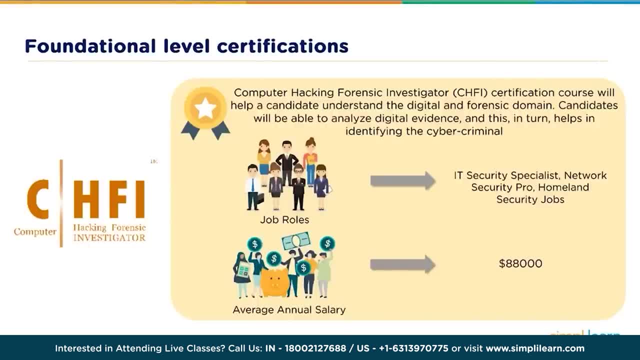 each and every question. Job rules: IT Security Specialist, Network Security Pro The job rules, Forensic Investigators, Law Enforcement Agencies, Security Specialists, Homeland Security Jobs, and your salaries would be around $88,000 and above. Alright, now let's talk. 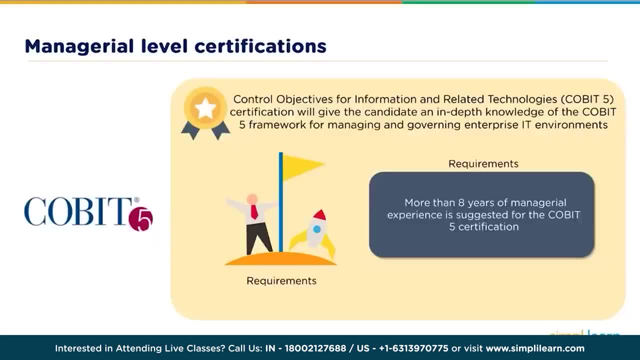 about the managerial level certifications. COBIT stands for Control Objectives for Information and Related Technologies. It's a certification that will give a candidate an in-depth knowledge of the framework which COBIT is all about, and the framework helps you manage and govern enterprise IT environments. Now this is an 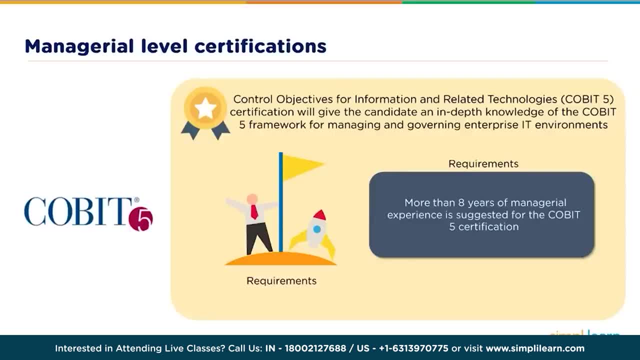 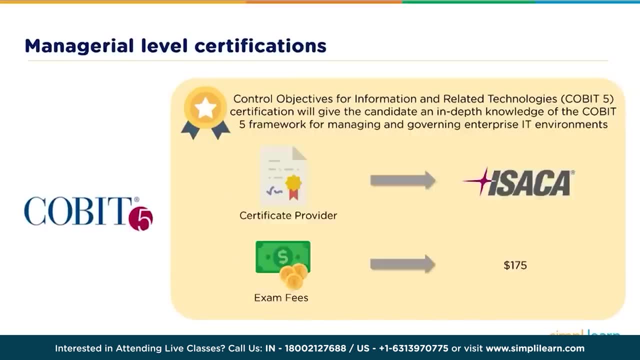 advanced certification. so around 8 years of managerial experience is suggested before you attempt the COBIT 5 certification. to understand all the aspects and to help you implement the framework properly, The certification certificate provider is ISACA. The exam fee is around $175.. 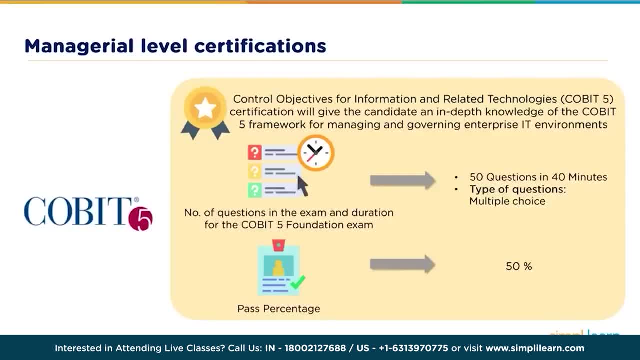 Now, this is a small exam: 50 questions, but in 40 minutes. So you really have to be on your toes. You have to know the knowledge. There is very limited time to think and you have to be fast in your answers. The pass percentage: 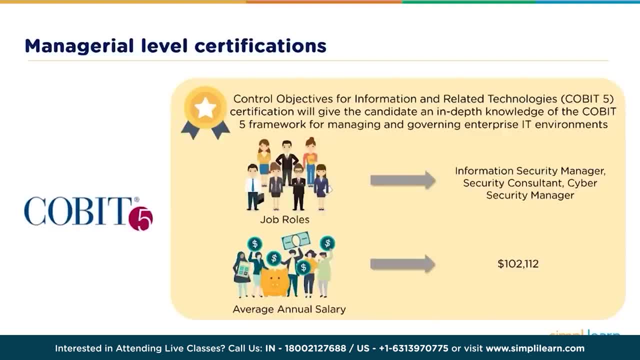 is 50%. The job roles associated with this certification would be when you apply for information security manager or as a security consultant or a cyber security manager, and your roles and responsibilities would be to govern the IT space that the organization owns. So all the servers, desktops, the network. 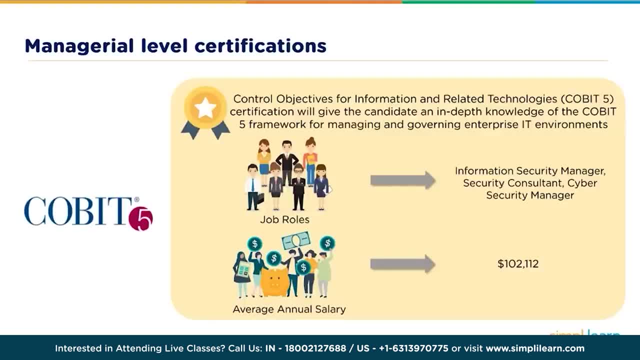 the data flows, the databases, everything, and how it needs to be managed and how it needs to be governed in a secure manner. Annual salaries would be around $100,000, plus Then the CISM, also called as. CISM It stands for Certified Information. 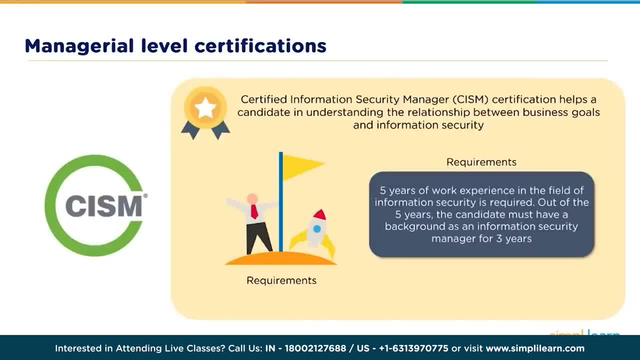 Security Manager and, as the name suggests, it's a security manager certification. It helps the candidate in understanding the relationship between business goals and information security. So now you're going into the space where you're not only technically in nature but you also have to understand the business needs. 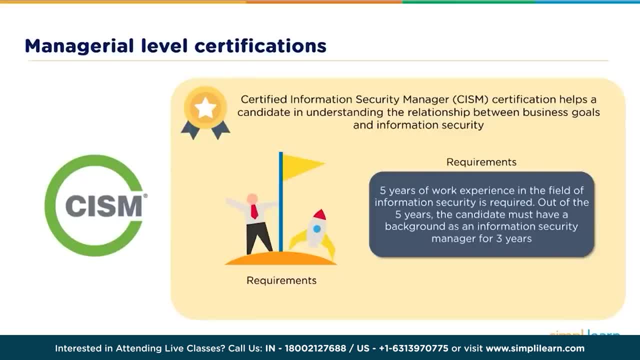 the goals of the business and you have to align the information security of their infrastructure along with the business needs and the business goals. So it is your inputs that are going to go to the management to see if the infrastructure is aligned to the business goals or if the infrastructure 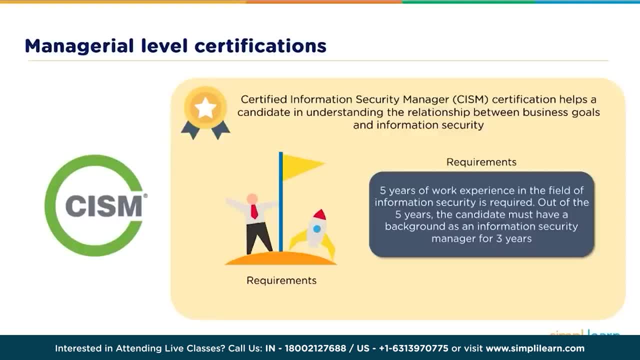 or the business goals need any fine tuning Around. five years of work experience is recommended in the information security field for attempting the CISM. Out of the five years, the candidate must have a background as an information security manager for three years. So you have some. 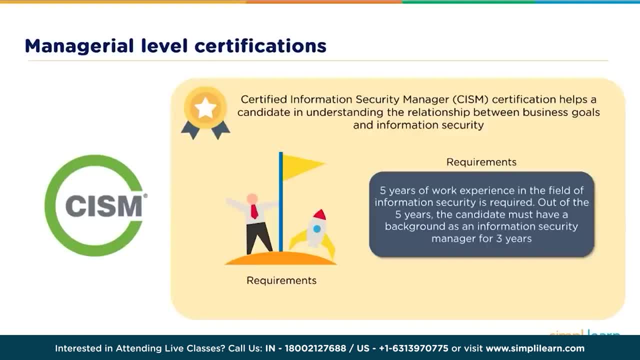 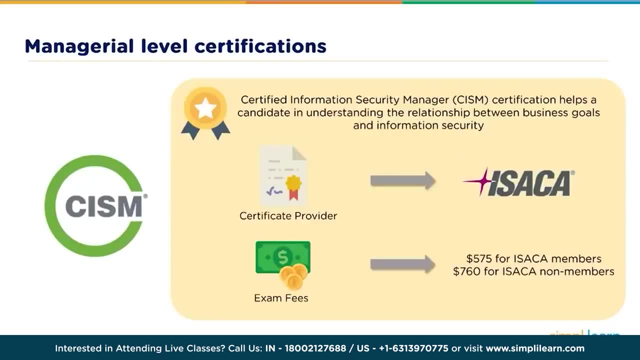 experience as a manager, you have implemented those things yourselves, which will give you a better understanding. and then you attempt the certification Again, providing by ISACA, and the exam fees for ISACA members is $575.. For non-members it is $760.. The exam is where you have. 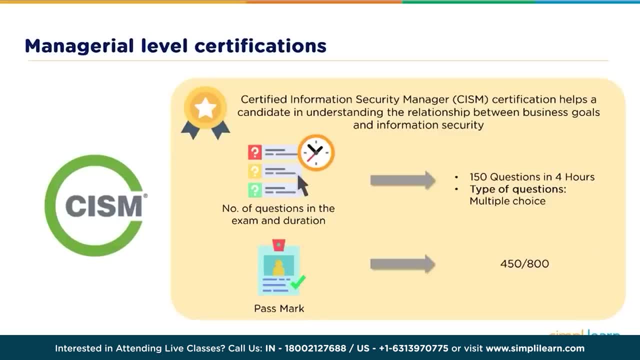 to answer 150 questions in four hours- Quite a bit of time. but questions are going to be scenario based questions where they're going to give you a lot of scenarios. You have to think about it and you have to give the most probable and the correct answer. 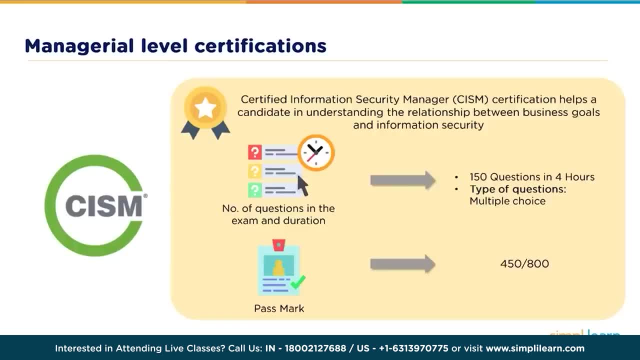 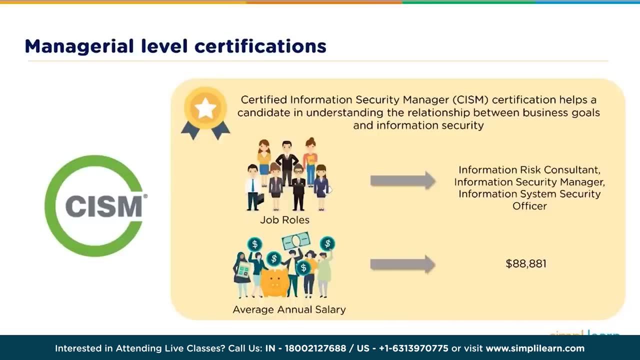 for that particular scenario, The pass mark is 450 out of 800.. Your job profiles would be either a risk manager or a risk consultant, analyzing the business requirements to the infrastructure security that you have and to identify if there are any risks associated with the infrastructure. 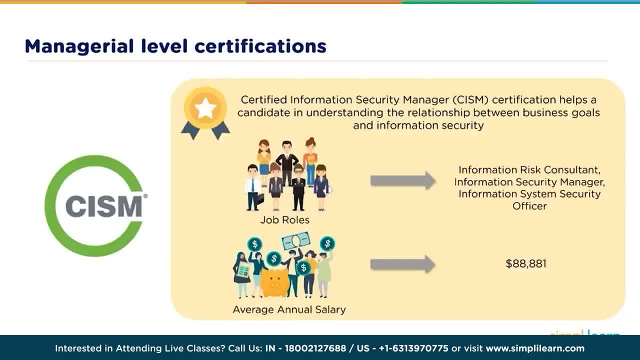 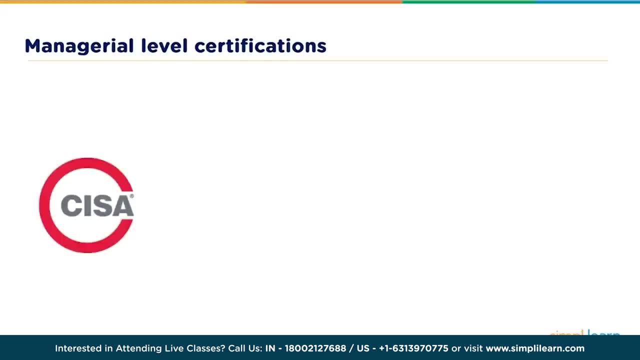 highlight those risks and then put in security controls and manage those controls in a way where security is mitigated. Your average salaries would be around $88,000 and above. Then the CISA or the CISA, the certified information systems, auditor certification. it. 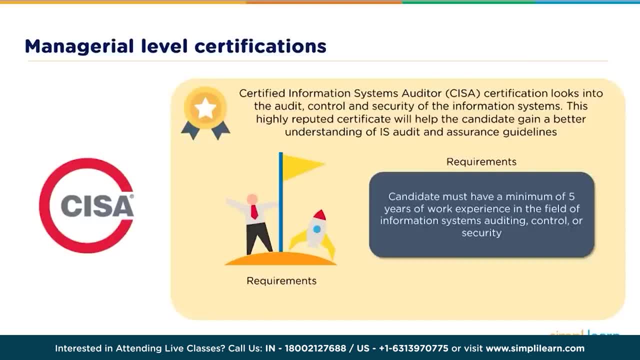 not only looks into security, but it also looks into auditing and controls in information systems. This is a highly reputed certificate and you gain a better understanding of governance regulations and auditing your information landscape. Again, a minimum of five years of work experience in the field of information systems auditing. 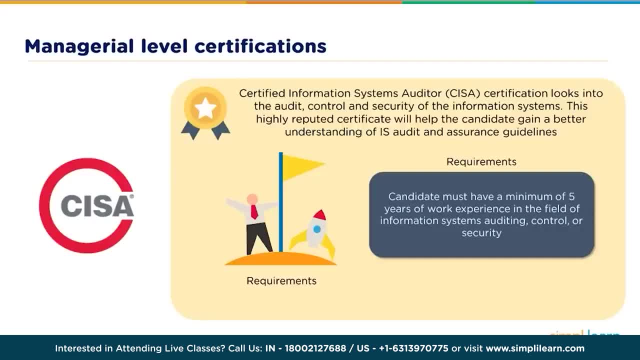 control or security is necessary. Now here the question would be: what's the difference? Security is where you're technical in nature. you have done, let's say, a vulnerability assessment or a penetration test. you have implemented firewalls, you have architected security. 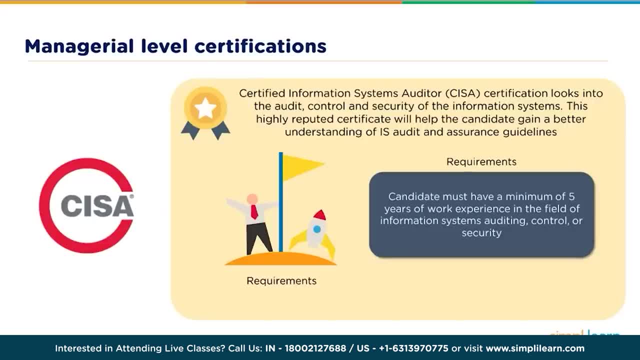 Controls are all about the security controls that you're going to implement, like firewalls, IDSS, IPSS, data loss prevention systems, maybe even UTMs and what not. So experience in architecting or implementing those controls in an effective manner, mitigating your. 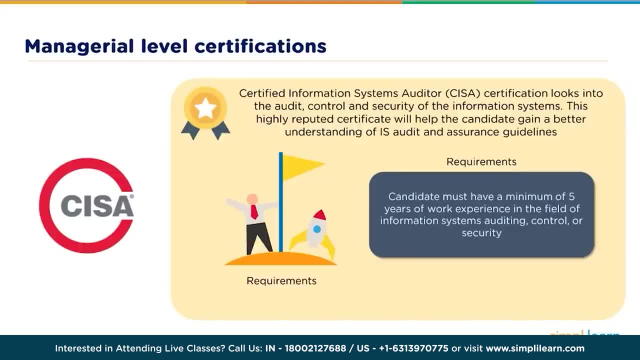 security or your vulnerabilities that you have identified in the organization. And auditing would basically mean about looking at compliance To ensure that everything is in place, you're compliant with, let's say, ISO 27001 guidelines or the policies that you have created yourself, and everything is working. 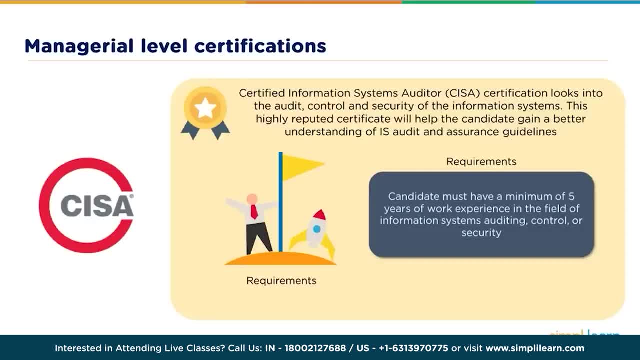 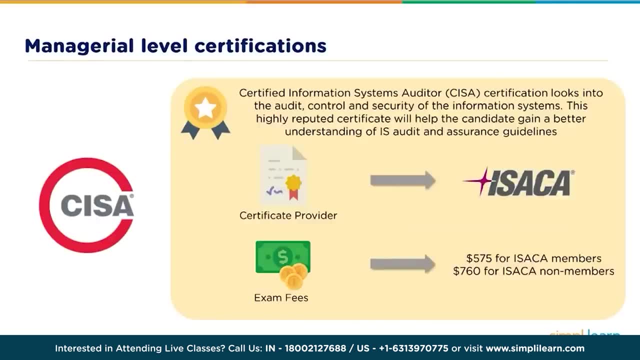 in order. So it's more of a checklist where you're going to just check everything is in place and you're conforming to standards. This certification is also provided by ISACA, and the exam fees for ISACA members are $575, whereas non-ISACA members. 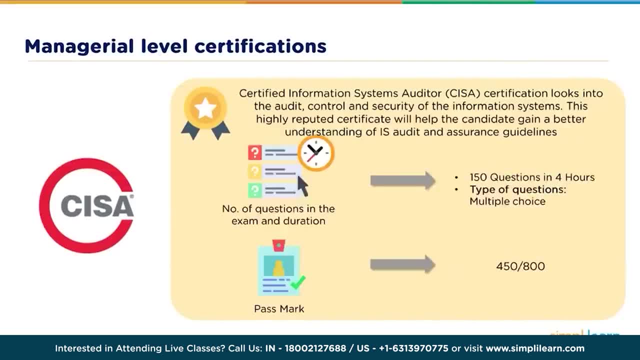 will have to pay $760 for the certification: 150 questions again in 4 hours. multiple choice questions, scenario based. so you have to really understand real world scenarios of where what controls and what audit mechanism should be in place. Pass mark is 450 out of 800.. 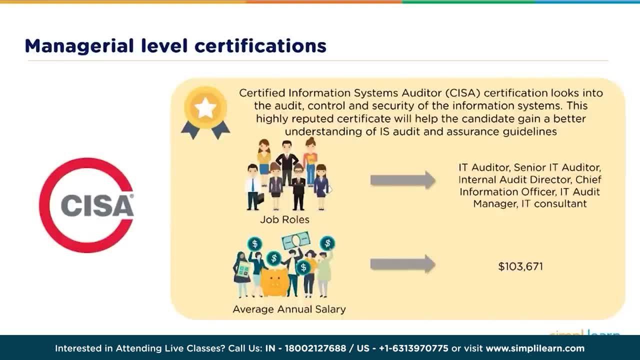 Your job roles would be mainly becoming an auditor or a senior auditor, a director for information security, information audit manager or information technology consultant, where you provide intelligence on how the company should implement their infrastructure. Average salaries would be $103,000 and above. 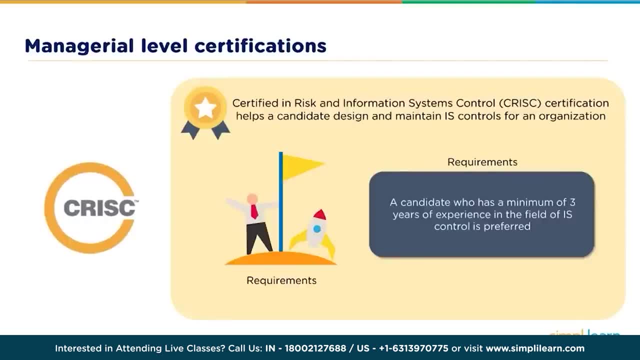 Then comes the CRISC, also known as CRISC Certified in risk and information systems control. certification helps the candidate design and maintain information systems controls for an organization. This is one of the most sought after certifications as far as risk management is concerned In Europe. 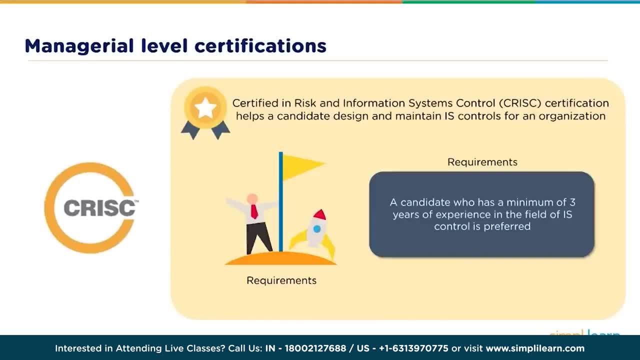 and in US. if you have this kind of certifications, you automatically qualify for a risk manager or security risk manager or a information security consultant kind of role. You should have a minimum of 3 years of experience in the field of IS controls. that means information security controls. 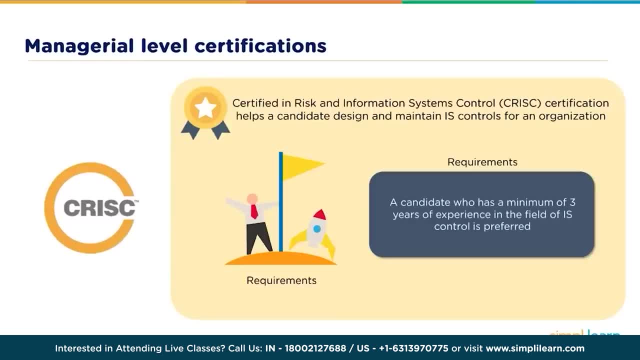 you should have knowledge about firewalls. you should know about how to mitigate risks, how to identify risks in the first place, risk analysis, risk management and after which you are going to implement security controls to mitigate that risk or bring it to acceptable levels. At this point in time, you will also 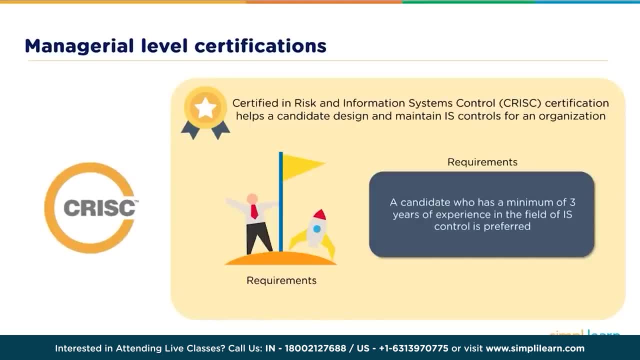 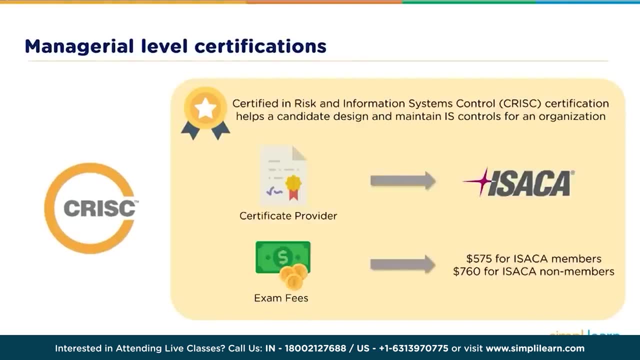 be responsible to create policies revolving those risks and how you want to calculate those risks and treat those risks in their lifetime. Certificate provider again is ISACA: $575 for ISACA members, $760 for non-ISACA members for the exam fees. A similar question 150. 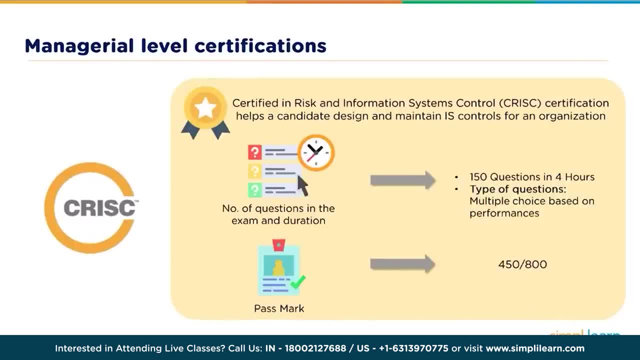 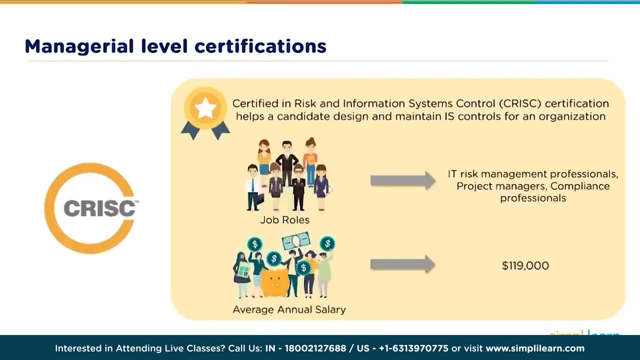 questions to be answered in 4 hours, multiple choice based on performances. So they may give you a scenario where you have to perform a risk analysis and provide a report and a solution based on your findings. Again, the pass mark is 450 out of 800.. The job: 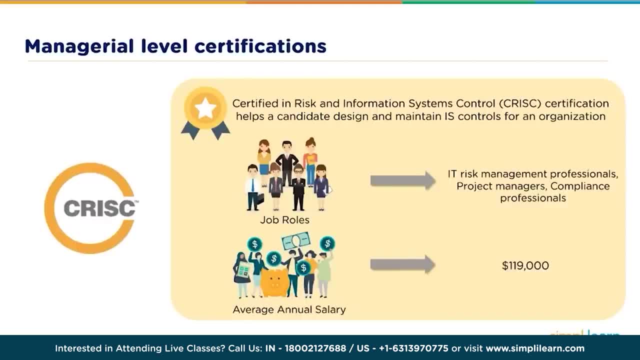 profiles. associated, as discussed earlier, are the IT risk management professionals, where they are going to identify risks, treat those risks, calculate, analyze, maybe do a business impact analysis to ascertain how the organization is going to be affected, and then you will also be looking at compliances as far as these job roles are concerned, Average annual salary would be $119,000 and above, Moving on to advanced level certification. Now this is where we come across the CISSP, or the CISP certification: Certified Information Systems Security Professional. This is the gold standard of all. 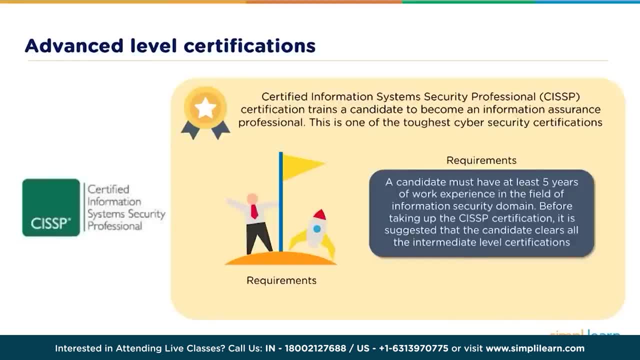 certifications. If you have this certificate, you can basically be assured of a job in the IT world. Now, just to qualify, you will have to have 5 years of experience in the information security field. There are 8 domains that are specified by CISSP. 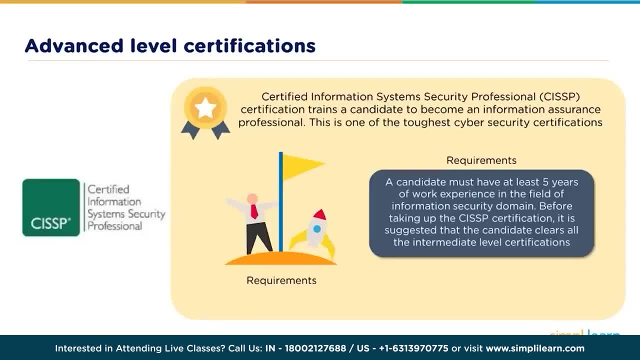 and you have to prove that you have knowledge and you have work experience of around 5 years in at least 2 of those domains. If you do not have those kind of experiences, you can still attempt the exam, but you become an associate of ISE square. 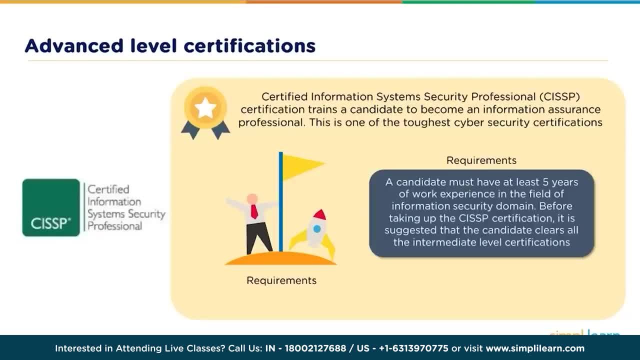 which means that you get 6 years to accomplish the 5 years of experience requirement for this certification. Before taking up the CISSP certification, it is suggested that the candidate clears all the intermediate level certifications- Not all, but some of them. In fact, I have seen 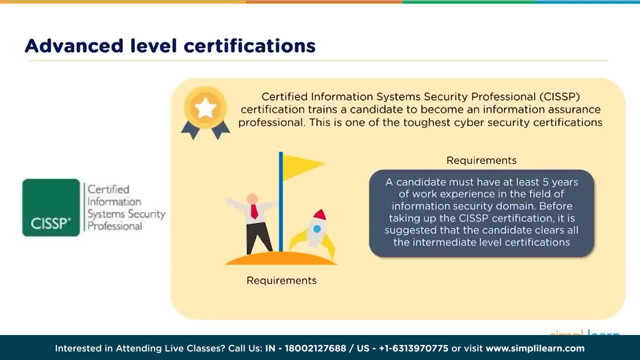 people do the other way around. They qualify for CISSP, they give the exam. once you are CISSP, the CISA or CISM exams are way easier to crack, but you need to have that kind of experience. I have seen people with 15 years of experience and more. 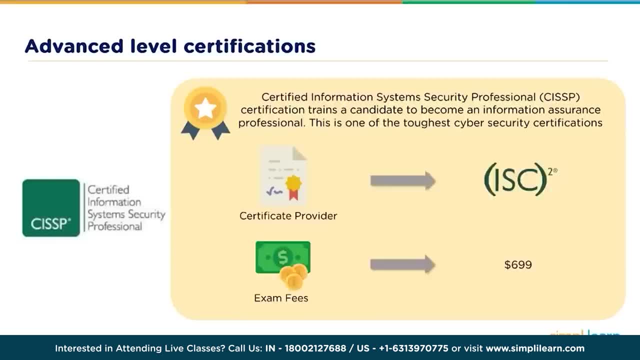 fail at this certification in the first attempt. The certificate provided is ISE square. The exam fees is $699.. Like I said, this certification is most sought after The gold standard. In fact, there is hardly any other certifications after this that you might. 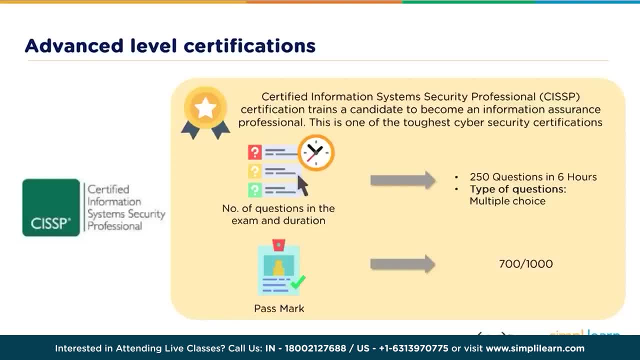 want to do The questions Now. the exam has changed. If it is the English version that you are giving, it is 150 questions to be answered in 3 hours. If it is the non-English exam that you are attempting, then it is 250. 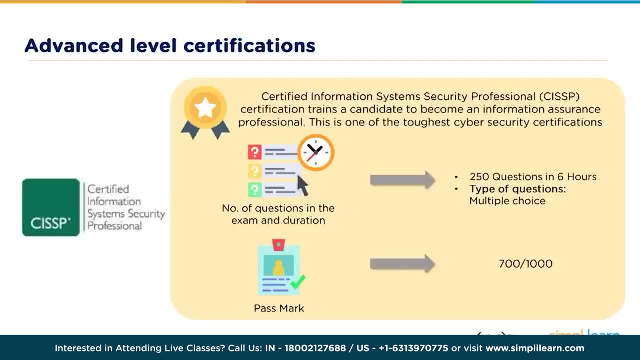 questions in 6 hours. It is a marathon and if you are opting for the 6 hour exam, you need to plan it really well. It sounds really easy, but the questions are quite tough, They are scenario based and the answers are quite confusing as well. You 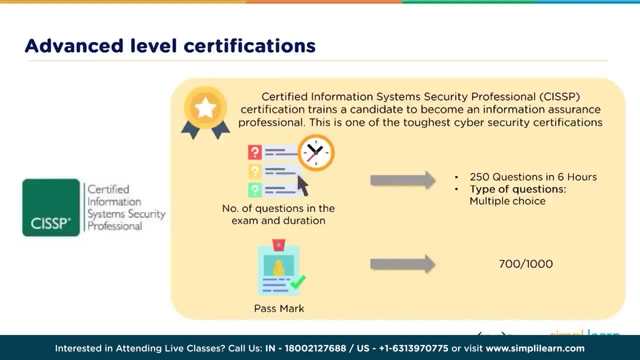 would get multiple choice questions, You would get drag and drop and you might get simulators as well. The pass mark is 700 out of 1000, but each question has a different rate age, so it depends on which questions are asked of you and 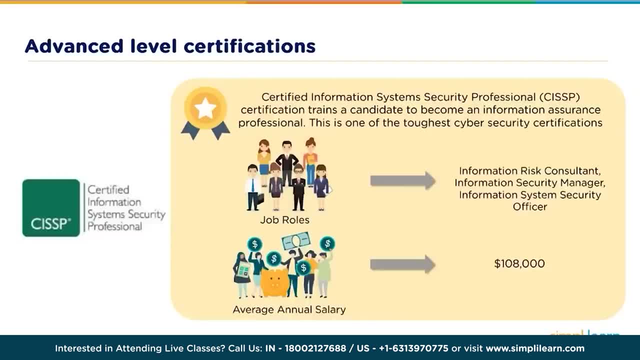 which questions you have answered correctly. The job roles associated with this certification would be anything and everything in information security at the managerial level and above. So, information security manager, risk manager, information system security officer. the CISO role, the CISO- Chief Information Security Officer. 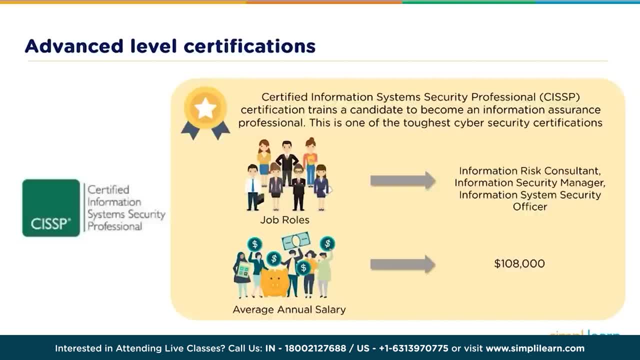 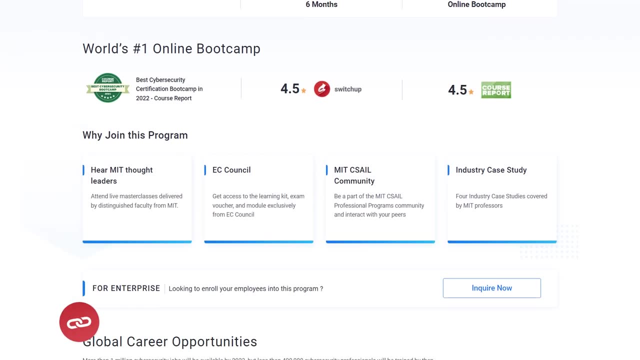 Any role that you might think of from a risk compliance strategy could be achievable after this kind of certification. The average annual salary is $108,000 for this certification, And if you are someone who is interested in building a career in cyber security, that is by graduating from the best. 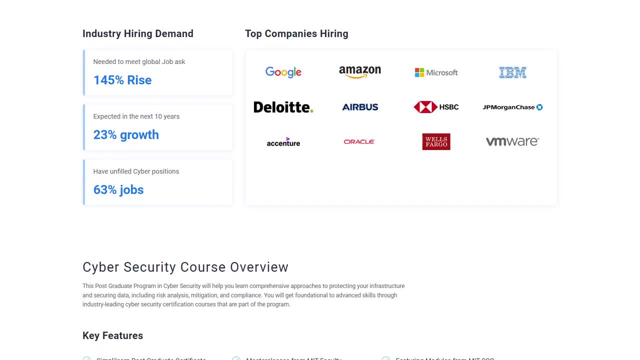 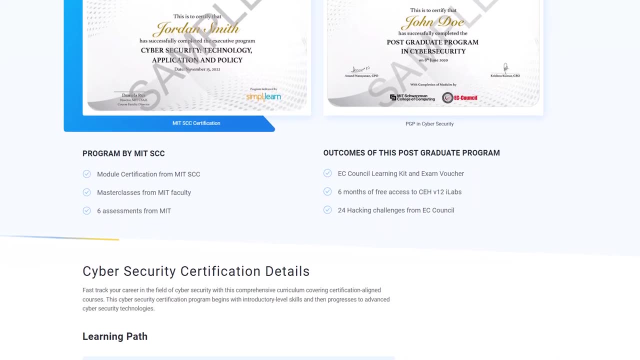 universities or a professional who elicits to switch careers with cyber security by learning from the experts, then try giving a shot to SimpliLearn's post graduate program in cyber security with modules from the MIT Schwarzman College of Engineering, And the course link is mentioned in the description box. that will 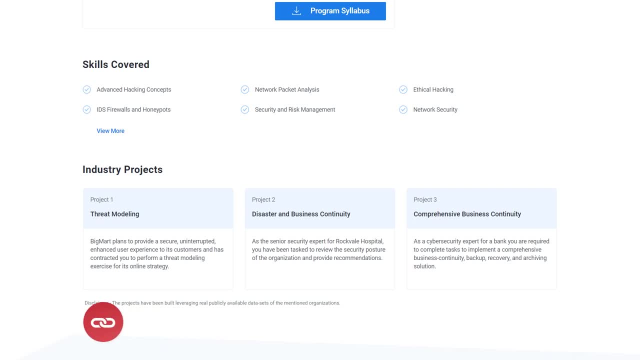 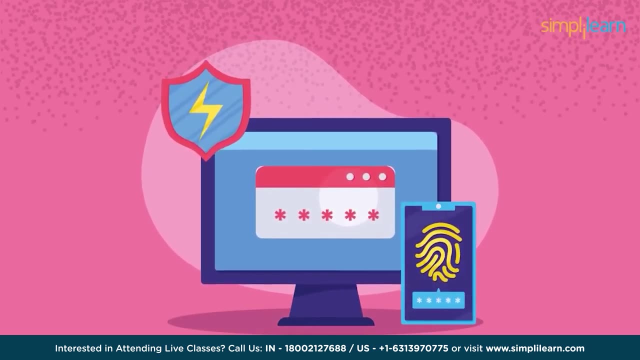 navigate you to the course page, where you can find a complete overview of the program being offered. Most of the entry level jobs in cyber security field requires you to trace, track and defend against cyber attacks on a day to day basis. You are required to enable systems against. 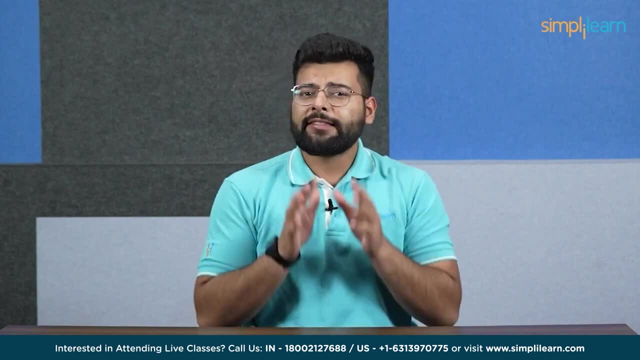 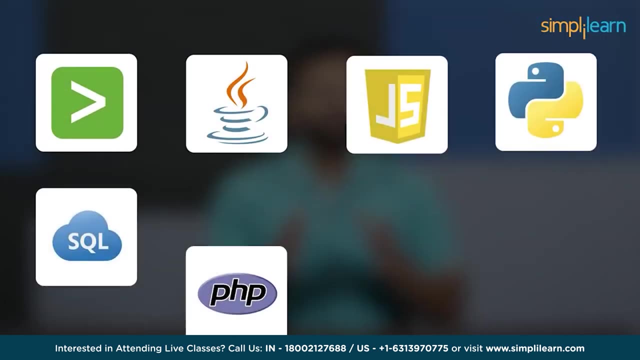 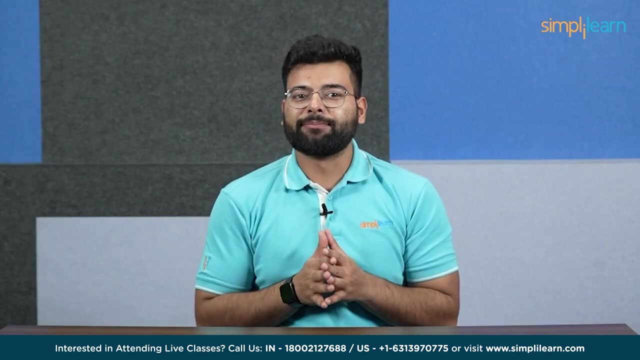 all fraudulent activity and prevent any authorized access. This requires, at length, the need to write scripts in various languages, such as Splunk, Java, JavaScript, Python, SQL, PHP, PowerShell and C, amongst many others. As scripts grow in complexity, so does the time to write them. 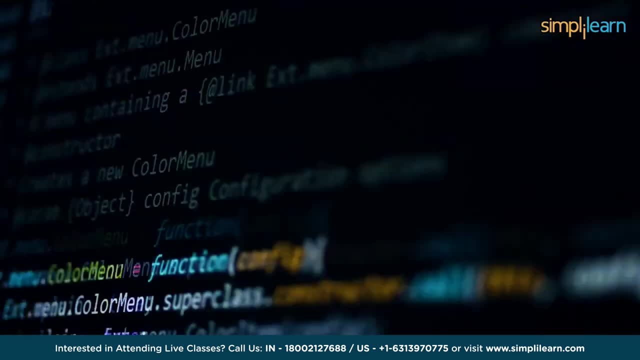 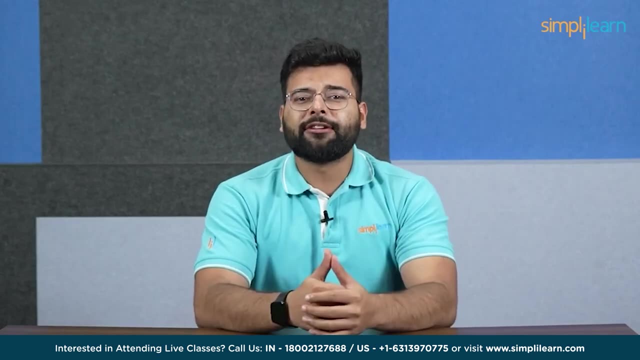 SharedGPT, on the other hand, can create these complex queries and scripts within split seconds, along with explaining them. This can help save hundreds of hours of effort for a cyber security professional. This is just one such use case of how SharedGPT is useful. 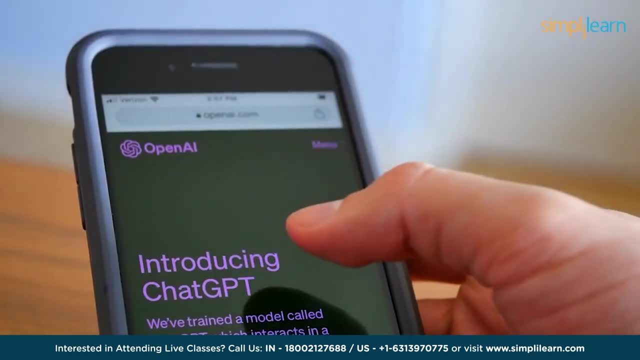 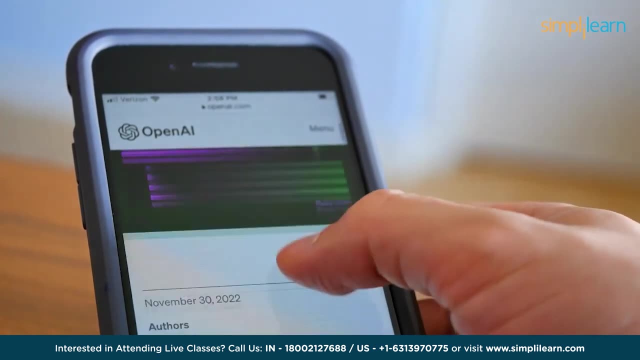 in the field of cyber security. Although relatively new, the uses of SharedGPT in the field of cyber security is innumerable, From automating daily tasks to script writing or endpoint detection. And if you want to know more about how SharedGPT can be used, 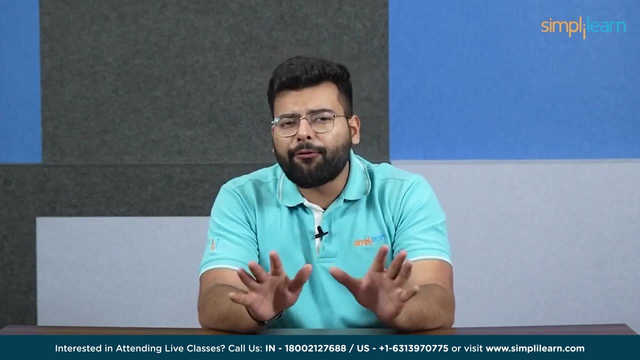 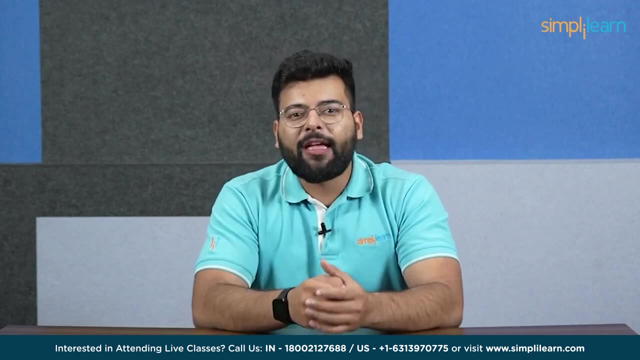 in the field of cyber security and how AI can change the entire information security landscape. stay tuned with us until the end of this video for some amazing information. With that being said, welcome to yet another amazing video by Simply Learn. Make sure to subscribe to our channel and hit the. 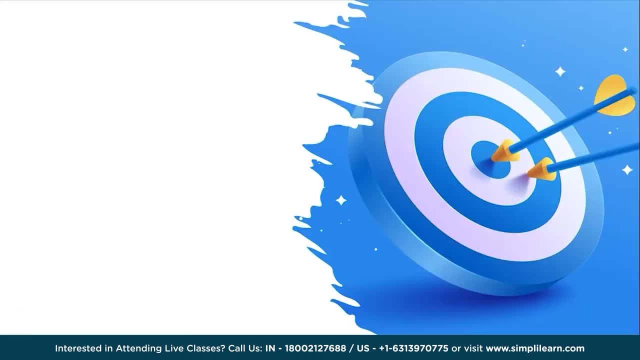 bell icon to never miss any other video from us. Let us now quickly discuss the agenda for the video. We will start with knowing what is SharedGPT Proceeding. we will see the uses of SharedGPT in cyber security and after that we will have hands-on lab. 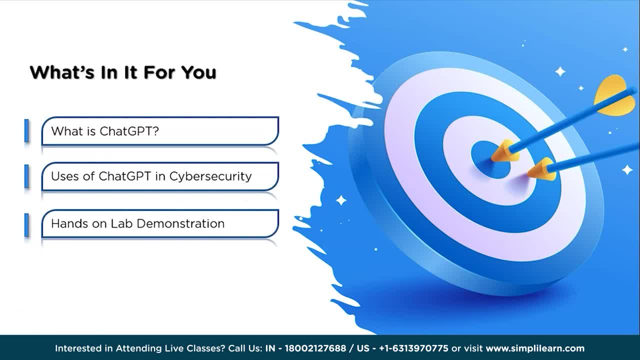 demonstration. But before we begin, if you are someone who is interested in building a career in cyber security by graduating from the best universities, or a professional who values the best skills, then you should start with the first step of learning the basics of cyber security. 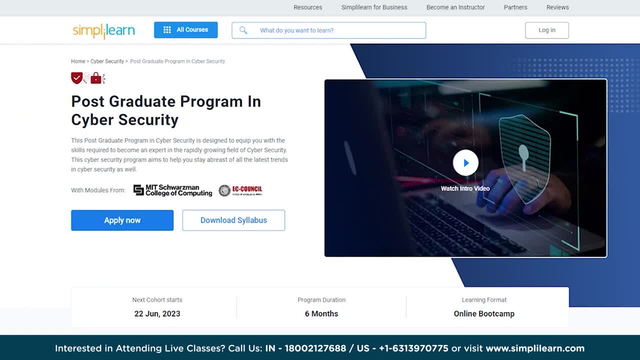 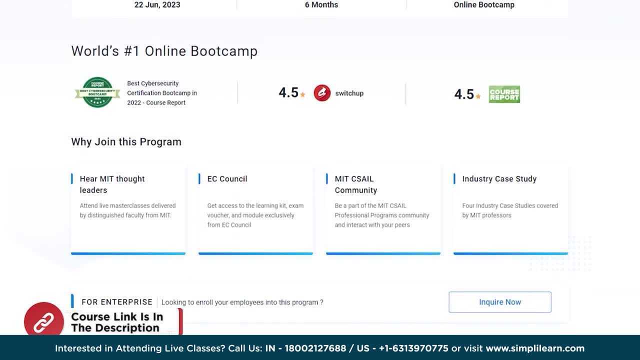 So let us begin. The first step is to switch careers in cyber security by learning from the experts. Then try giving a short to Simply Learn's post-graduate program in cyber security with modules from MIT Schwarzman College of Engineering. The link is provided in the description. 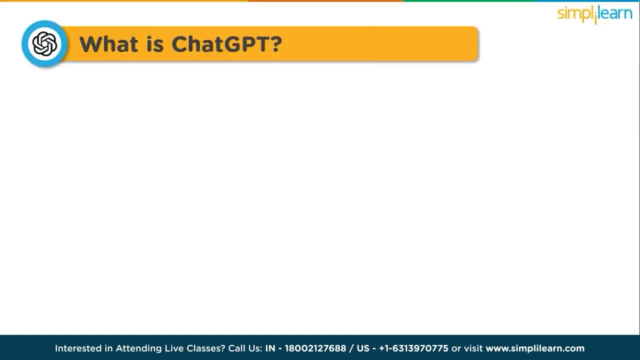 box that will navigate you to the course page, where you can find a complete overview of the program being offered. So let us start with our topics. SharedGPT uses Natural Language Processing to understand and respond to user queries. It is based on the GPT 3.5 architecture. 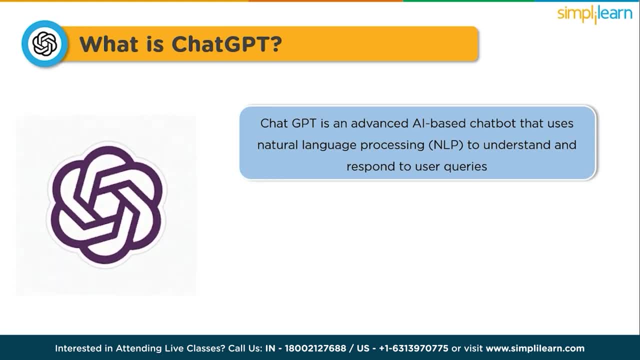 and has the ability to learn from conversations with users, making it more intelligent and efficient all the time. SharedGPT can be integrated with various messaging platforms such as Slack and Microsoft Teams to provide a seamless and secure communication experience. So this was about SharedGPT. 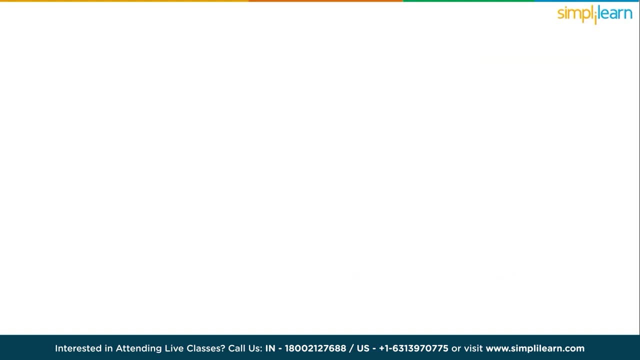 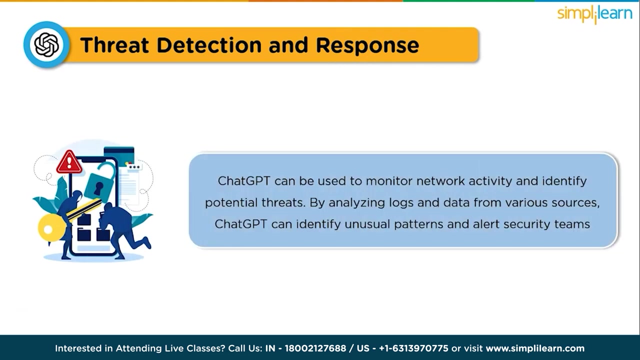 Now let us understand the uses of SharedGPT in cyber security. So uses of SharedGPT for cyber security will start with number one. We have Threat Detection and Response. SharedGPT can be used to monitor network activity and identify potential threats by analyzing. 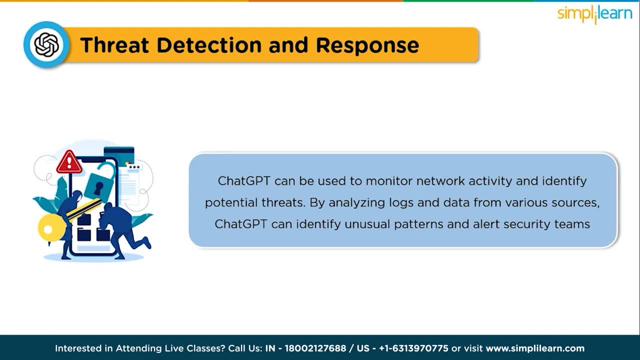 logs and data from various sources, SharedGPT can identify unusual patterns and alert security teams. It can also provide real-time alerts to users, enabling them to take immediate action to protect their data. By using machine learning algorithms, SharedGPT can learn from. 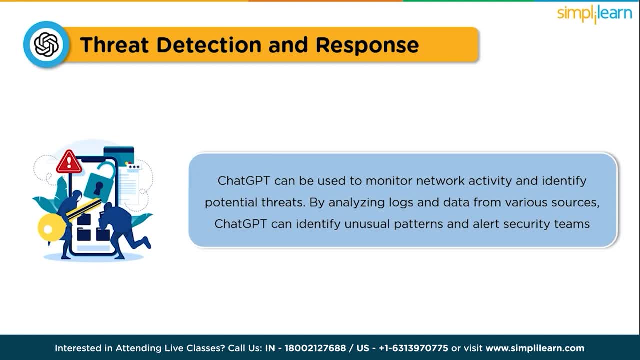 past incidents and continuously improve its ability to detect new and emerging threats. Once a threat has been detected, SharedGPT can initiate an automated response or cyber security personnel to take appropriate action. This can include blocking suspicious network traffic, isolating infected systems. 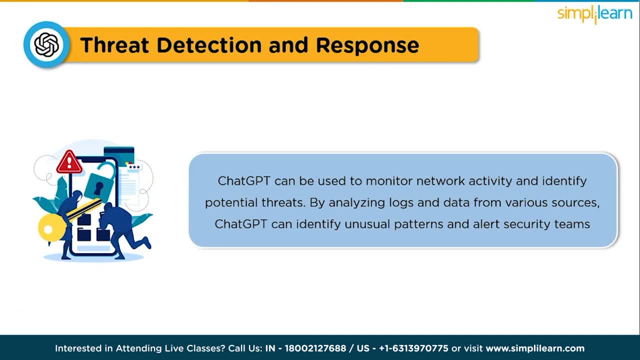 or disabling compromised user accounts. By providing real-time threat detection and response, SharedGPT can help organizations to minimize the impact of cyber breaches and reduce the risk of data loss or system downline. It can also help to improve overall security posture by identifying vulnerabilities. 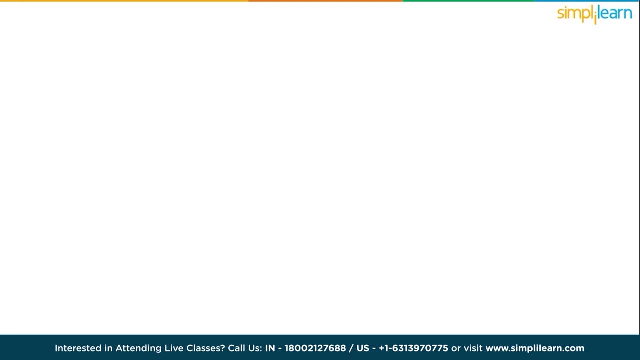 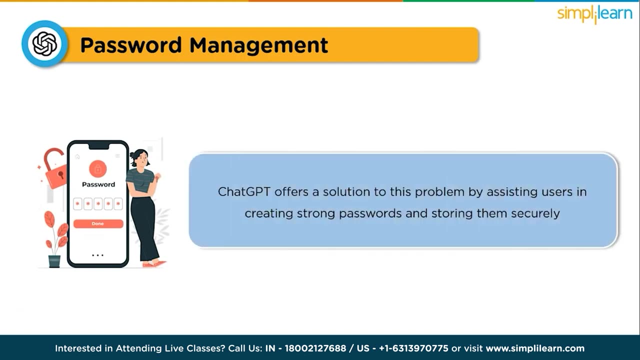 and recommending proactive measures to address them. And the next we have is Password Management. One of the most common ways that cyber criminals gain access to sensitive information is through weak passwords. SharedGPT offers a solution to this problem by assisting users in creating strong 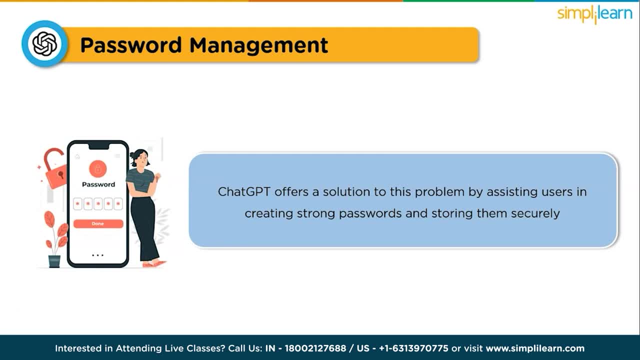 passwords and storing them securely. With its advanced natural language processing capabilities, SharedGPT can suggest complex and unique passwords that are difficult for hackers to guess. Moreover, it can save these passwords in an encrypted format, ensuring that they are protected from unauthorized access. 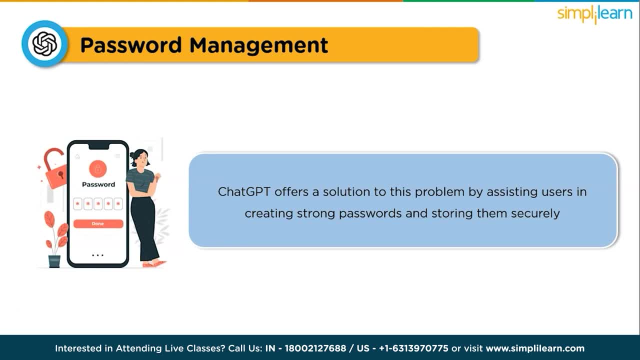 Another important feature of SharedGPT's password management tool is the ability to remind users to change their passwords regularly. This is crucial, as it helps prevent the use of outdated passwords that can be easily hacked. And at number 3, we have Employee Training. 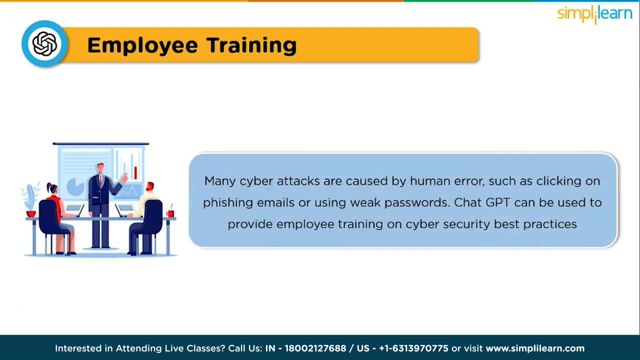 Many cyber attacks are caused by human error, such as clicking on phishing emails or using weak passwords. SharedGPT can be used to provide employee training on cybersecurity best practices. With its ability to simulate real-life scenarios, it can create interactive training modules that help employees. 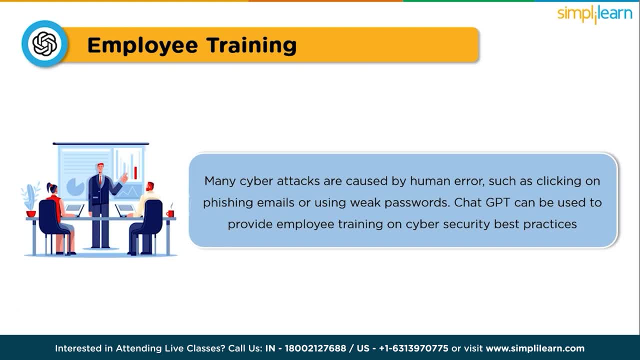 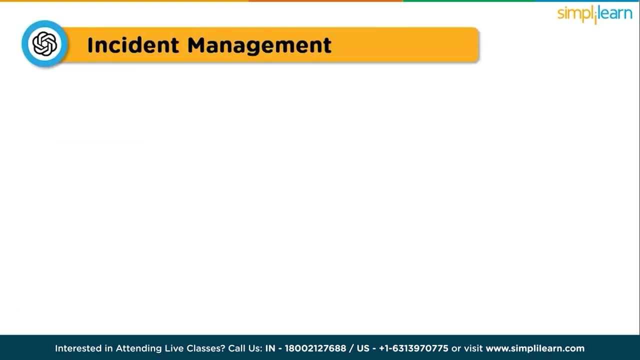 learn how to identify and respond to cyber attacks. For example, it can provide simulation of phishing emails, where employees can learn to identify the warning signs and avoid clicking on malicious links or downloading harmful attachments. Next up, we have Incident Management. Incident management is an essential 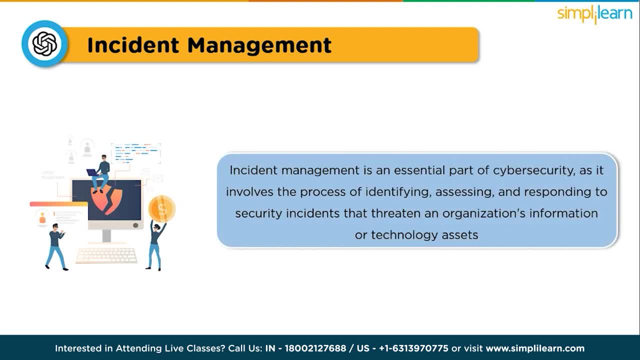 part of cybersecurity, as it involves the process of identifying, assessing and responding to security incidents that threaten an organization's information or technology assets. In today's digital age, cyber attacks have become increasingly common and sophisticated, making incident management even more critical. One of the ways 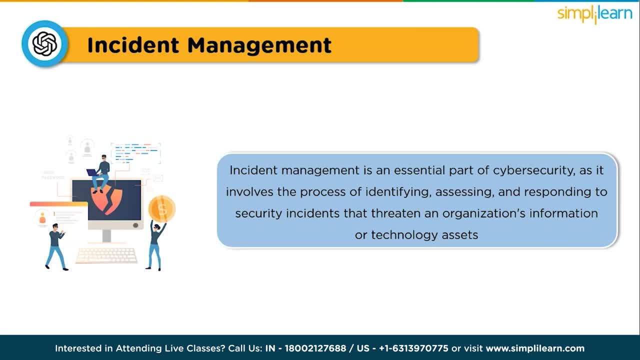 SharedGPT can help organizations with incident management is providing step-by-step instructions on how to contain the attack, mitigate the damage and restore normal operations. When a security incident occurs, time is of the essence and organizations need to act fast to minimize the impact. 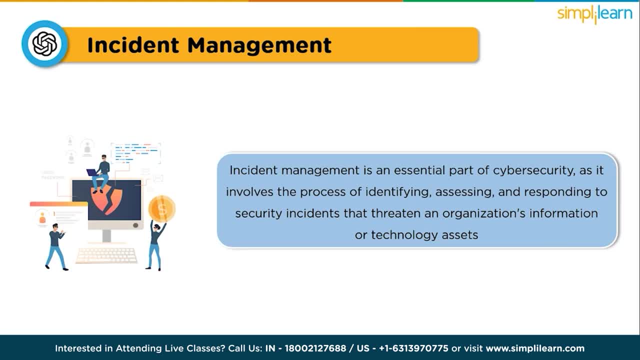 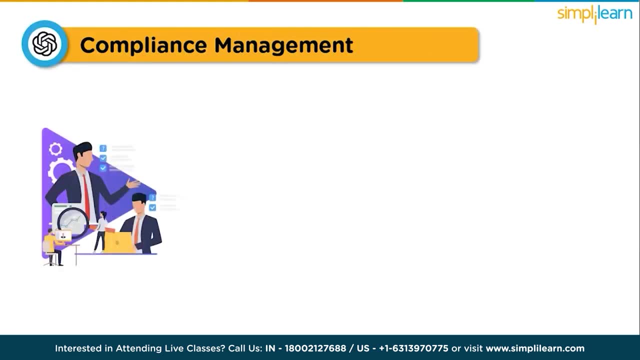 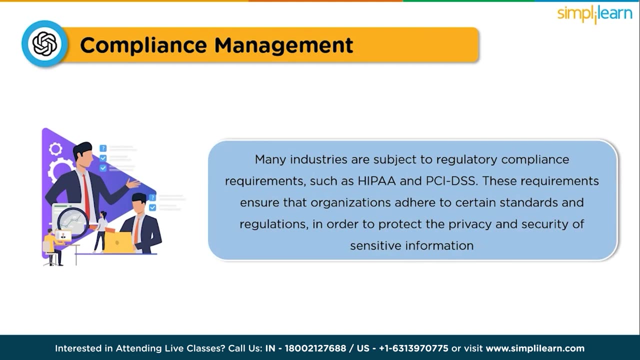 of the attack. SharedGPT can help by providing real-time guidance on how to respond to an incident effectively, And the next we have is Compliance Management. Many industries are subject to regulatory compliance requirements, such as HIPAA and PCI DSS. These requirements 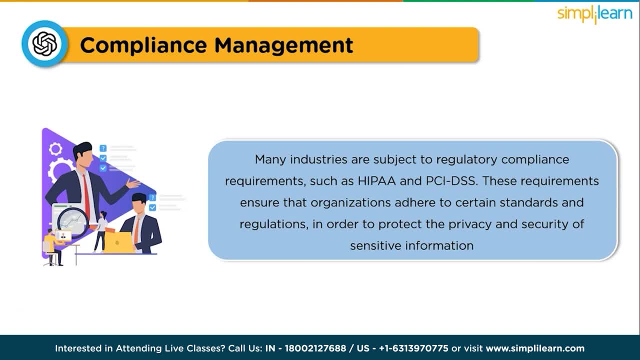 ensure that organizations adhere to certain standards and regulations in order to protect the privacy and security of sensitive information. Failure to comply with these regulations can result in hefty fines and reputational damage. SharedGPT can play a significant role in helping organizations ensure compliance with these regulations With its 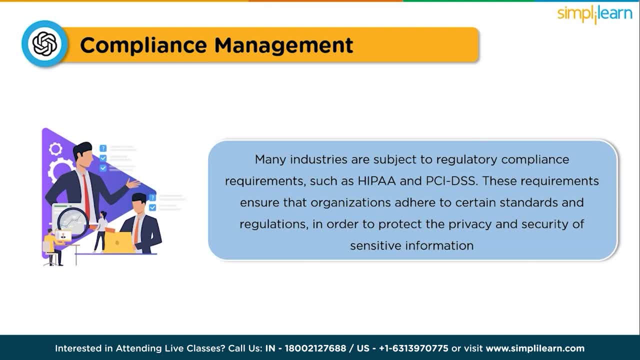 ability to process large amounts of data in real-time. it can provide alerts and guidance on best practices and generate compliance reports. This can help organizations identify areas where they may be falling short of compliance requirements and take corrective measures to address them. And now we will move to. 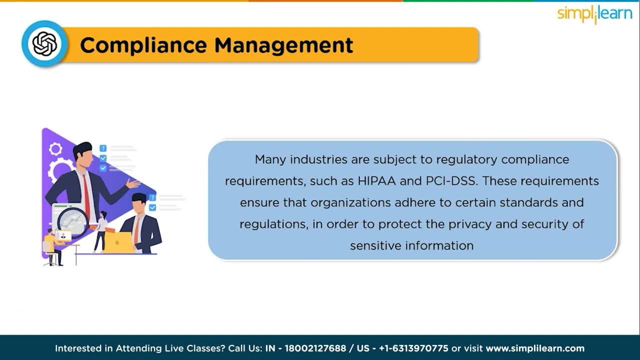 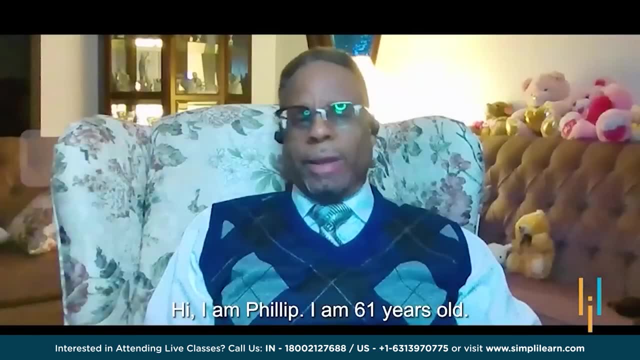 hands-on demonstration. But before moving, let's take a minute to hear from our learners who have experienced massive success in their careers by taking our courses. So just here to them. Hi, I'm Philip, I'm 61 years old and last year 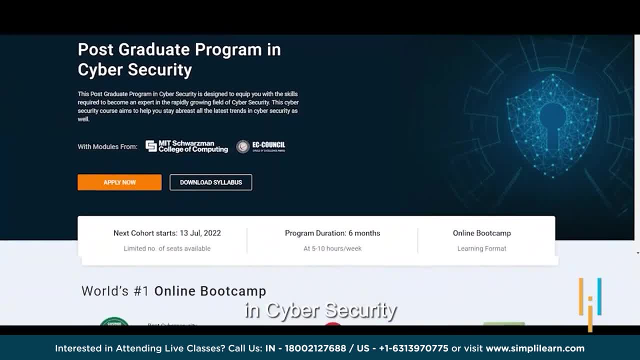 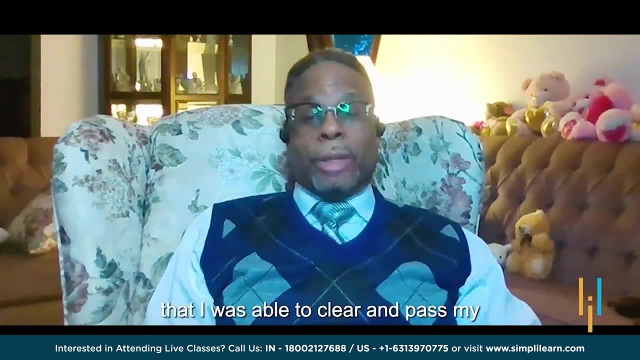 I upskilled with Simply Learner's postgraduate program in cybersecurity. after working 30 years in the IT sector in various different profiles, I'm happy to tell you that I was able to clear and pass my CISSP and CCSP certification exams on the first attempt after 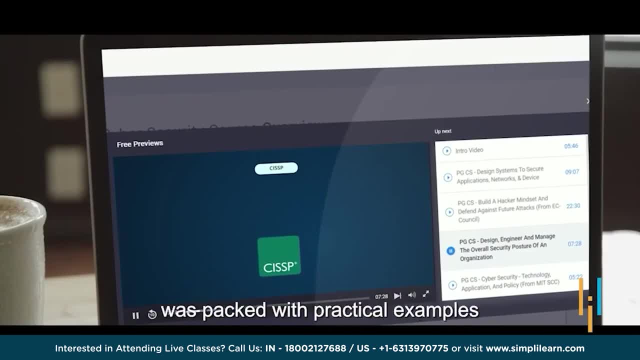 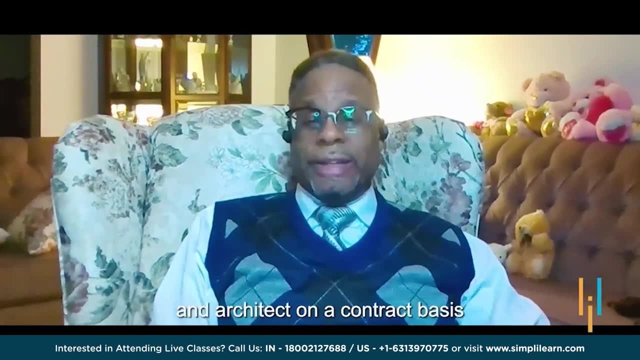 taking the course. The course, I must say, was packed with practical examples and was led by highly skilled and certified instructors. I worked with many companies before as a security analyst and architect on a contract basis, but I needed some stability, which I got with the job. 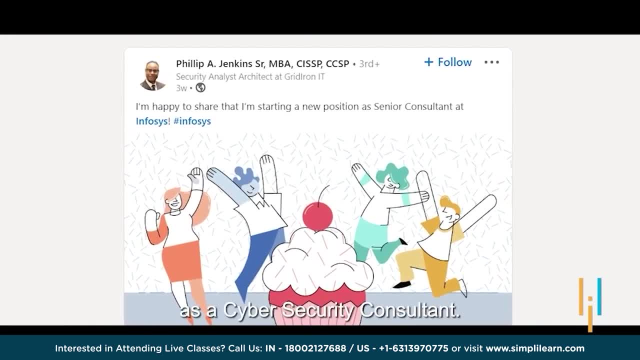 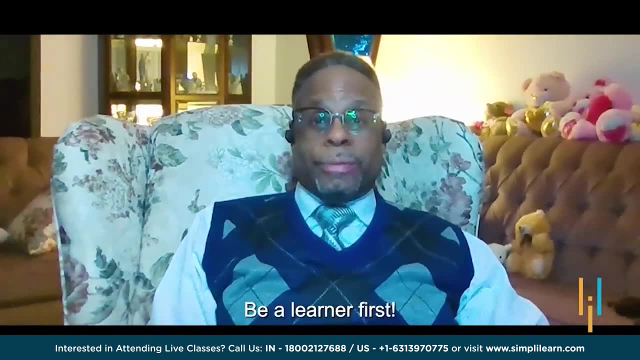 I just started with Infosys as a cybersecurity consultant. It happened after I took the course. But first and foremost, I've been a learner. Be a learner first And now. first, we will see what is ChatGPT. You could just write ChatGPT. 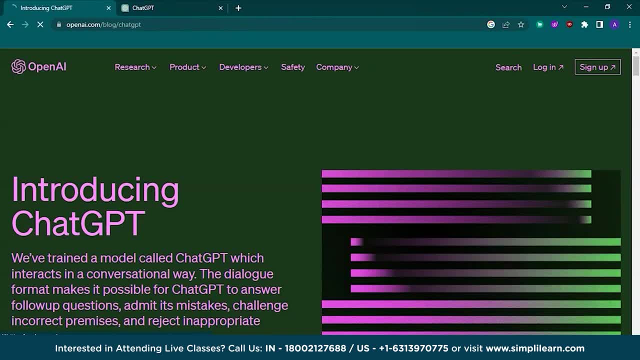 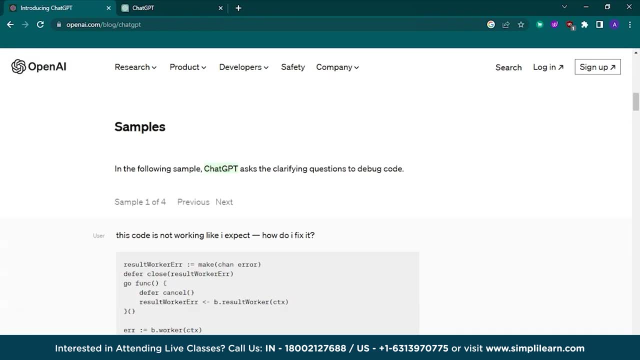 on web, on any browser, and this is the website where you will click and this is the website for ChatGPT, So you could see the samples here. and what the user has asked is: this code is not working like I expect. 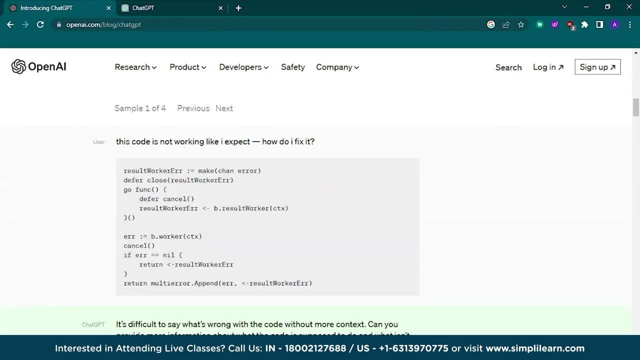 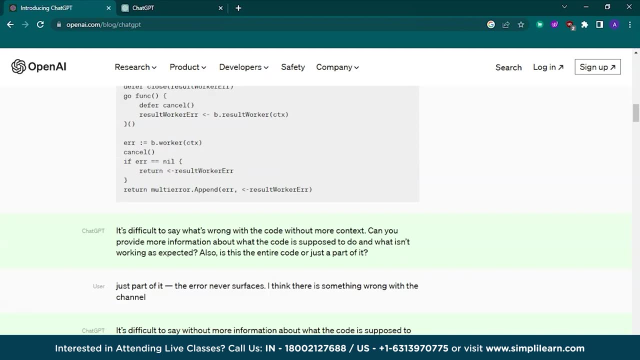 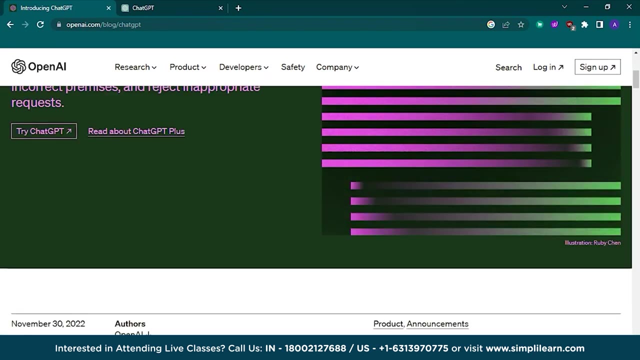 how do I fix it? So he has pasted the or input the command to ChatGPT and pasted his code and ChatGPT has answered that it's difficult to say what's wrong with the code without more context. So this is how ChatGPT. 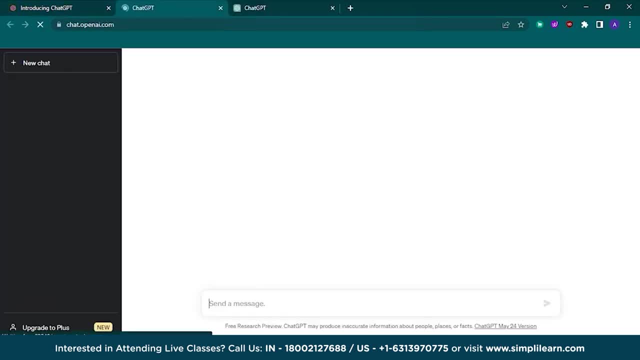 responds, and when you just click on here, try ChatGPT, you will have the window here. so this is the ChatGPT window, and here we'll start with some hands-on live demonstration for our cybersecurity. Like how ChatGPT 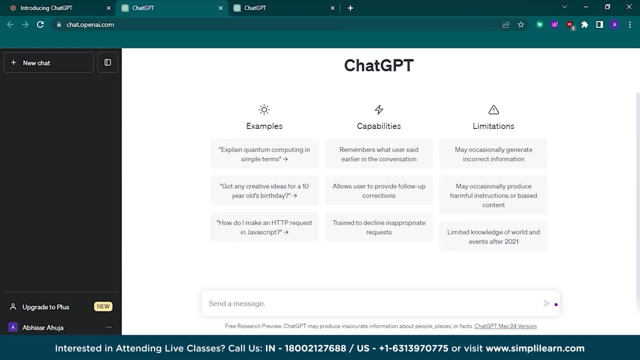 can help us in cybersecurity field. So we'll start with the basic questions and we'll see what he answers us. he or she answers us, or what ChatGPT answers us. So we'll start with the basic question: explain the MITM attack. 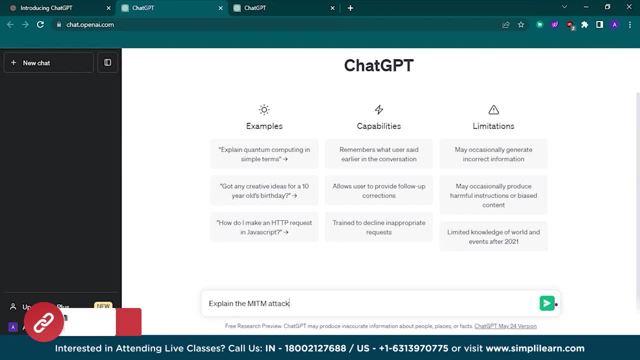 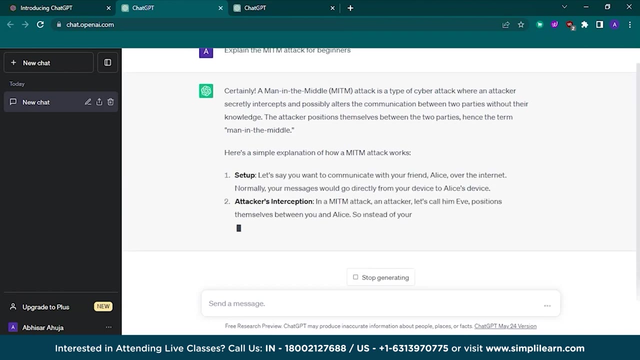 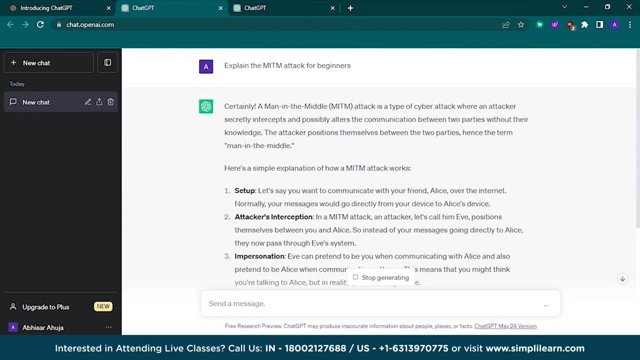 Okay For beginners, So we'll see what it responds. Certainly, a man-in-the-middle attack is a type of cyber attack where an attacker secretly intercepts and possibly alters the communication between two parties without their knowledge. The attacker positions themselves between the two parties, hence the term man-in-the-middle. 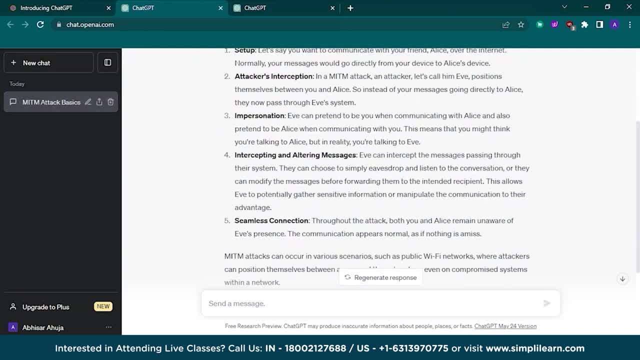 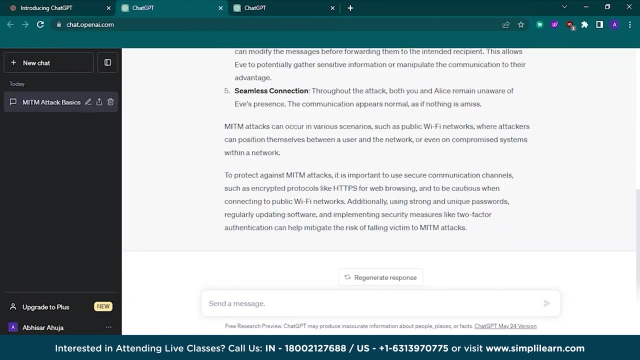 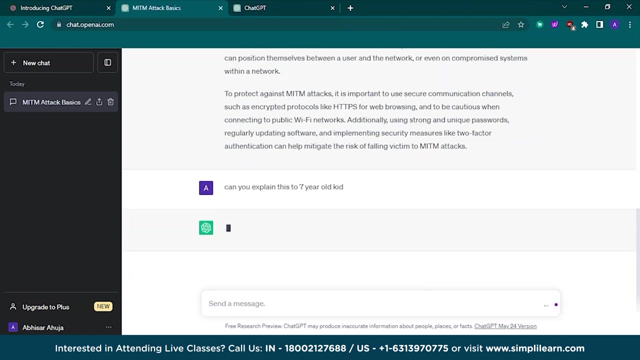 Okay. He has given us a very good definition And here's a simple explanation of okay And I want to ask him: can you explain this to a six or seven year old kid, or a seven year old kid? So we'll see. 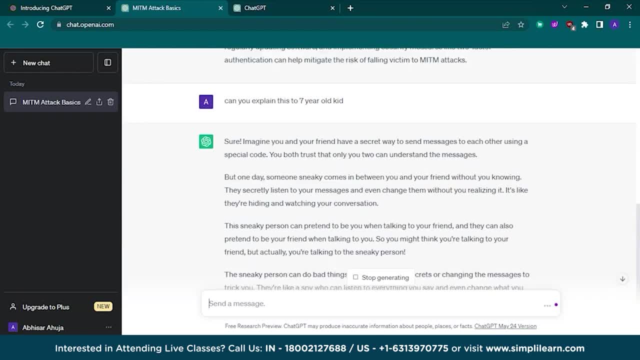 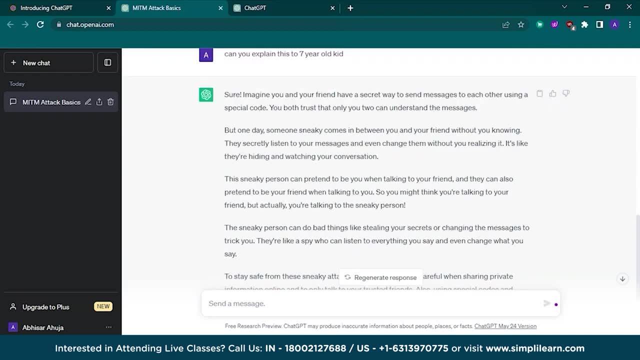 how ChatGPT can mitigate, or just try to understand this concept to a seven year old kid. So he has answered us, that's sure. Imagine you and your friend have a secret way to send messages to each other using a special code To both trust and only you two can understand. 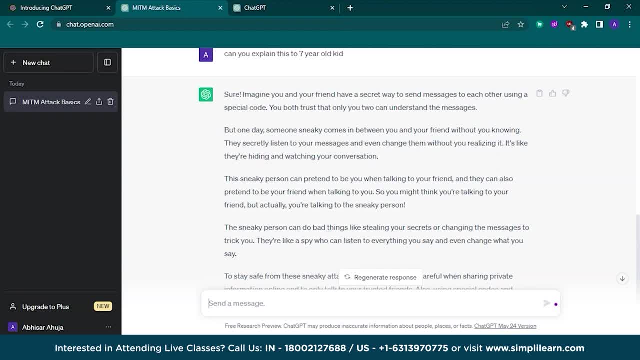 the messages. But one day someone sneaky comes in between you and your friend without you knowing it. They secretly listen to your messages and even change them without you realizing it. It's like they're hiding and watching your conversation. The sneaky person can pretend. 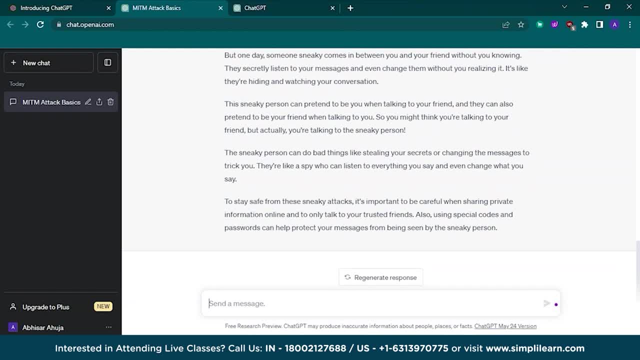 to be you when talking to your friend And pretend to be you okay. So he has taken the good example And they can also pretend to be your friend when talking to you, So you might think you're talking to your friend, but actually you're talking to a sneaky person. 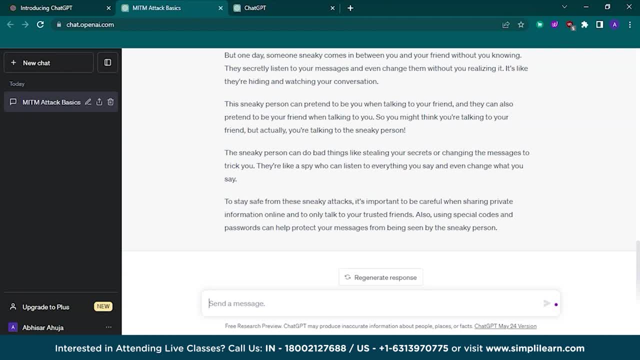 A sneaky person can do bad things like stealing your secrets or changing your manners to trick you. A spy who can listen to everything you do And even change a little. He has taken a very good example to get this concept clear to a 7 year old kid. 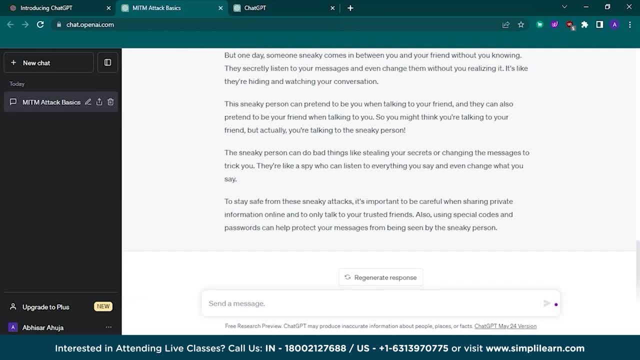 Really impressive. So we'll ask him some more questions And we'll ask the last basic question, That would be: What is SQL injection? And after that we could ask him some code snippets- What is SQL injection- And provide a real life sample. 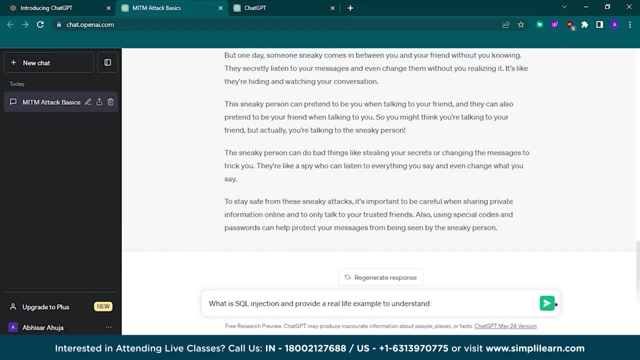 to understand the concept. So you have to write these prompts And you have to be very specific And you can follow up with your prompts. also, When JetJPT answers you, you can follow up him and ask him more about it, As I have done here. 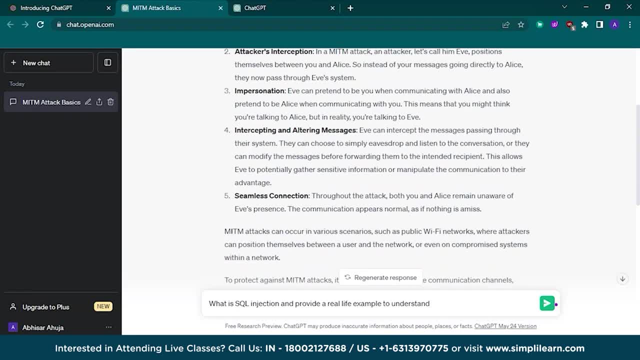 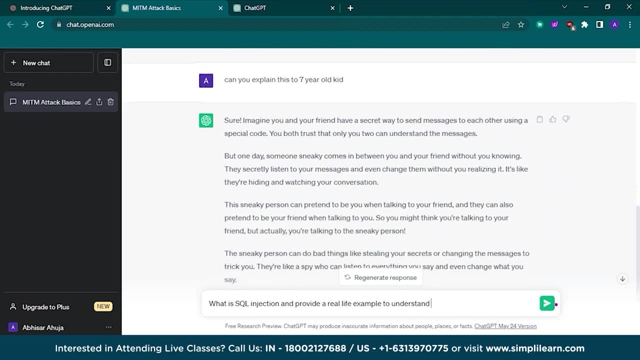 First, I have asked him Explain the MITM attack for beginners And he has given me the definition That is technically. And now I have asked him: Can you explain this to 7 year old kid? And he has answered me with a very good example. 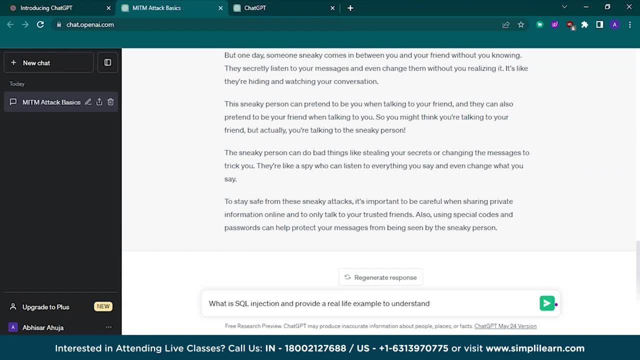 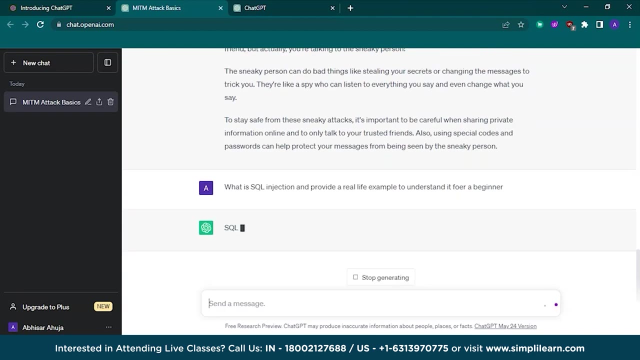 Similarly, you can do the follow ups for any prompts. So now I am asking JetJPT What is SQL injection? And provide a real life example to understand it for a beginner. And let's see what JetJPT answers us. SQL injection is a type of cyber attack. 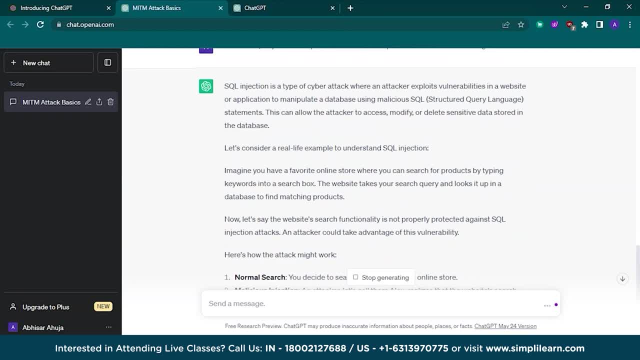 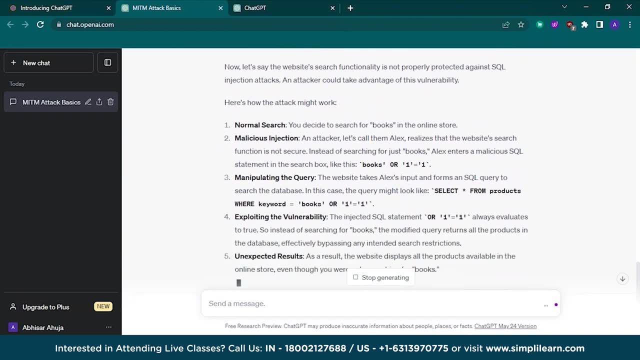 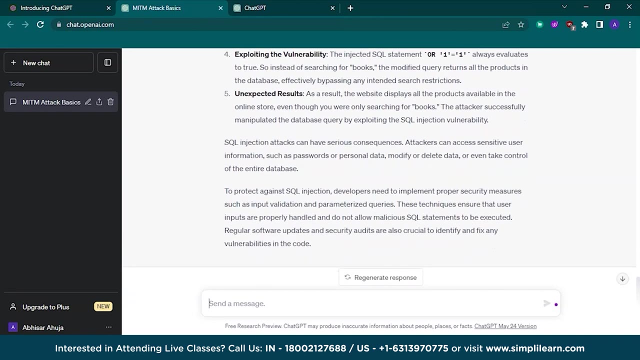 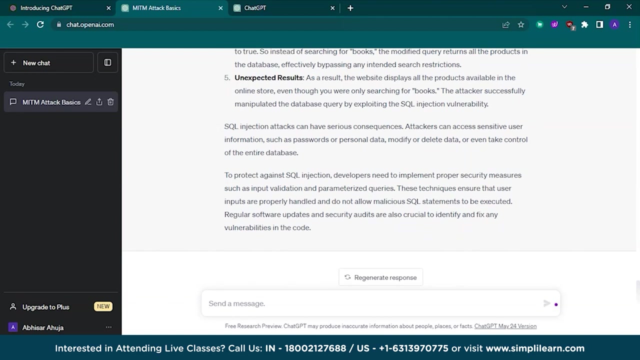 when an attack that experts hold in our website. So he is giving us the technical definitions Impressive. He is also telling us how the attack might work And he has also suggested us to protect against SQL injections. developers need to implement proper security measures. 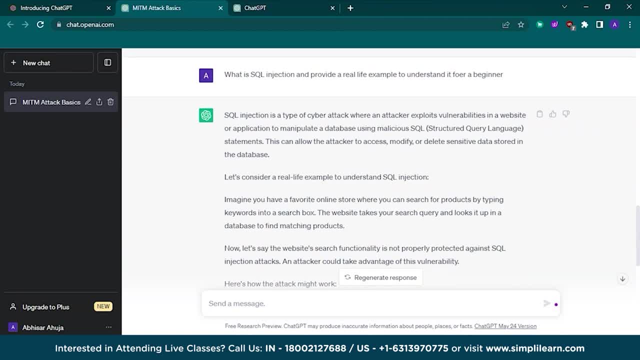 So this is the attack that is on the database That you can read here Or if you know. that is very good. We are just checking how JetJPT responds or give answers. We are not implementing or like we will ask him the code snippets. 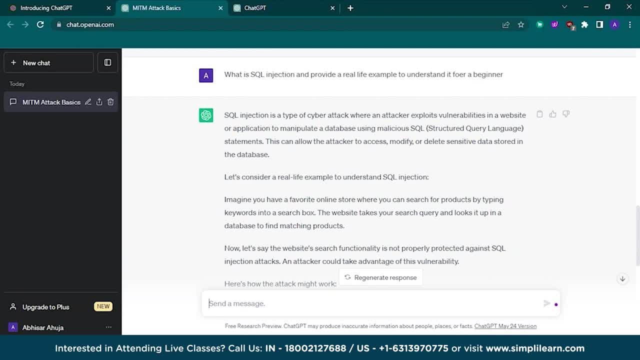 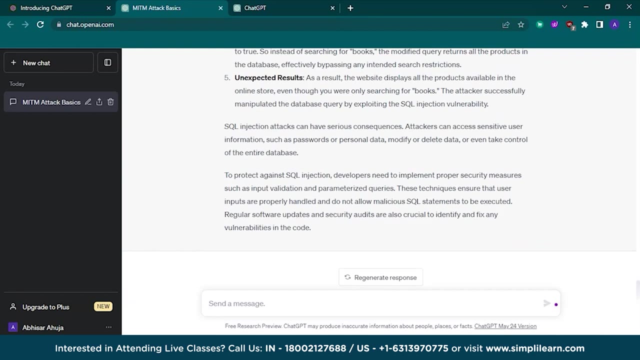 But we will not be able to implement in this video. We are here to just check out what JetJPT provides us for cyber security field. So you can see He has given us a very good response And, moving on, Now we will ask him. 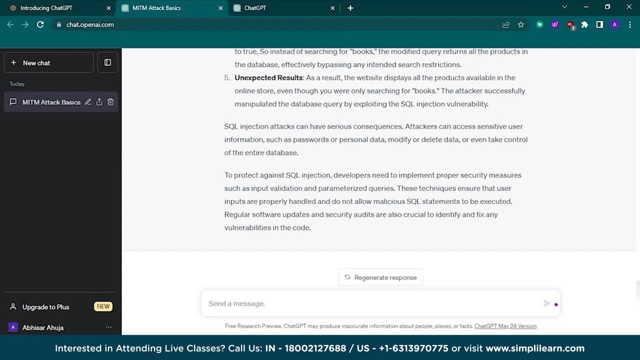 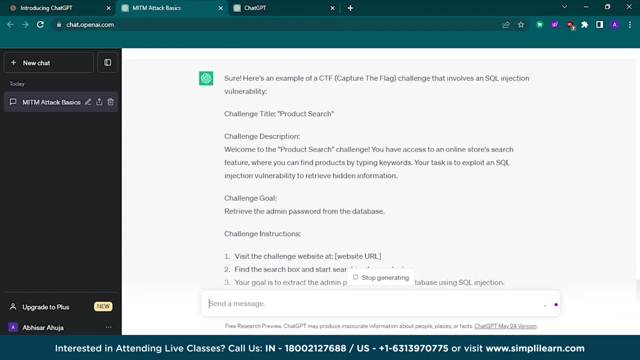 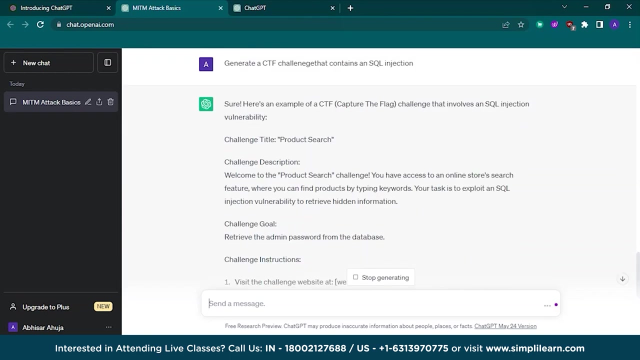 to generate a CTF challenge that contains a SQL injection. Let's see what it answers So you could see that JetJPT is responding first. That is Sure has an example of a CTF that is capture the flag challenge that involves a SQL injection. 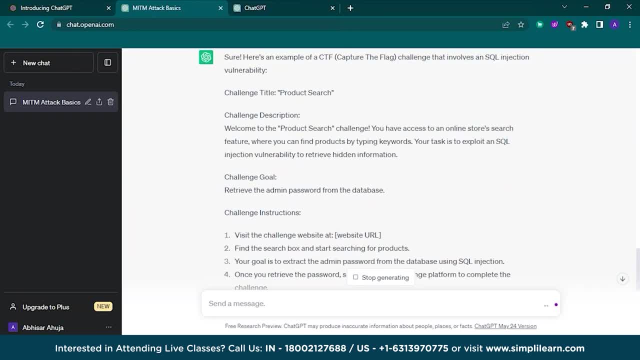 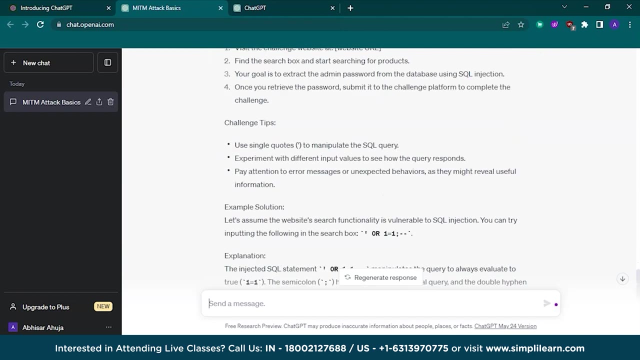 Vulnerability challenge. title: product search- Okay- Challenge description: Welcome to the product search challenge. You have access to an online store search feature. You can find products by typing keywords. Your task is to exploit a SQL injection vulnerability to retrieve hidden information- Okay. 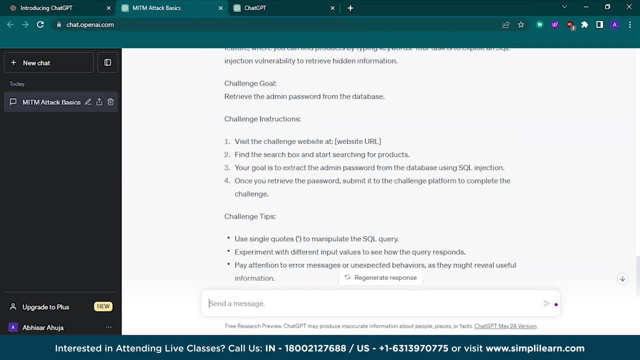 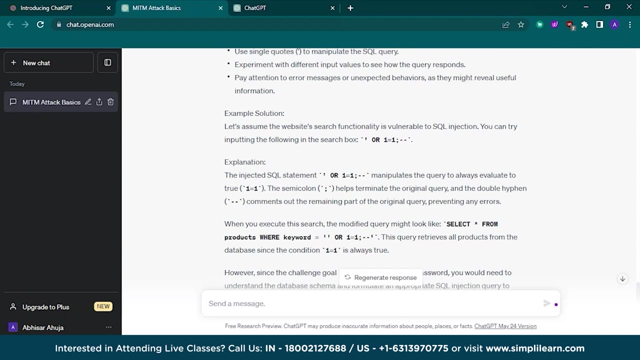 And he has challenge code With the admin password from the database And challenge instructions with the challenge website. Find the search box and start searching. OK, So we could see the example solution. Let's assume the website search functionality is vulnerable, Vulnerable to SQL injection. 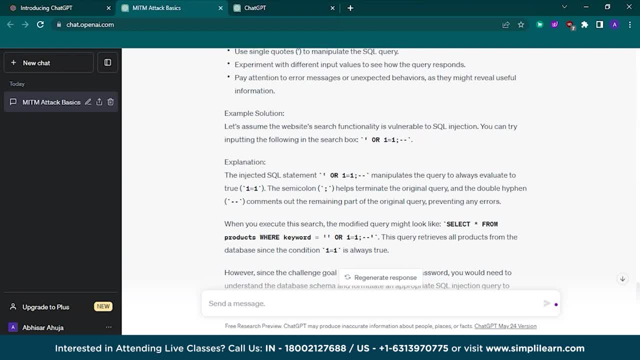 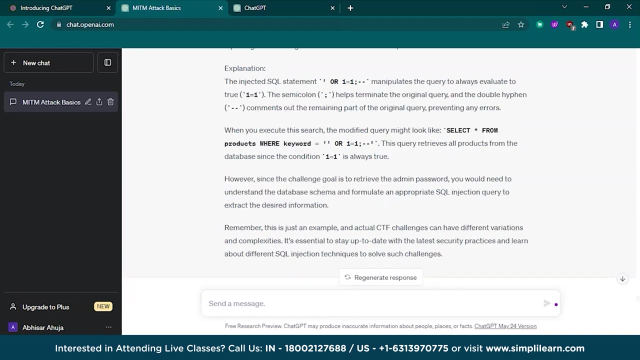 You can try inputting the following in the search box: Okay, Explanation. The injector SQL statement Query to always evaluate to true. Help terminate the original query and check for error When you execute the search. the modified query might look like: Okay. 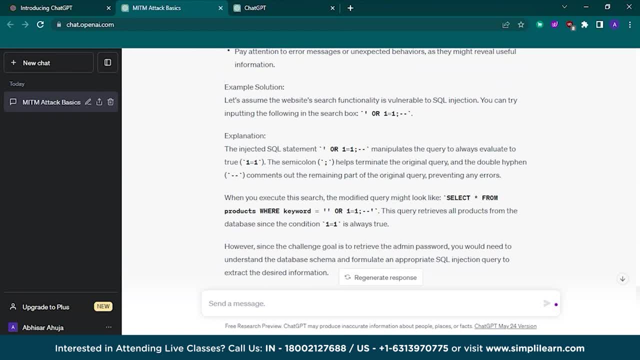 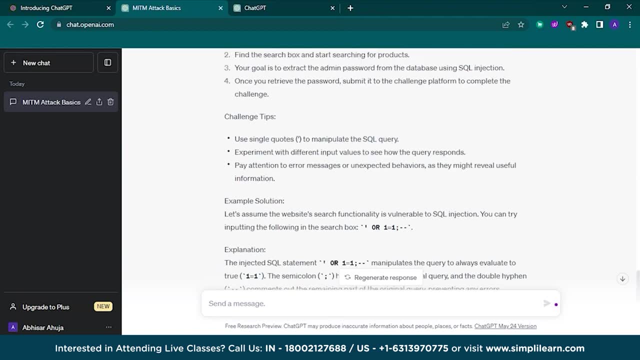 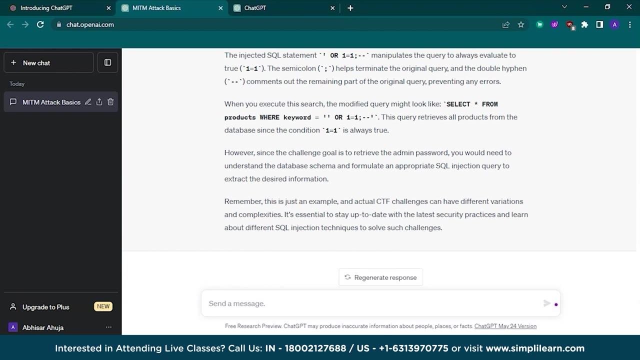 So it is what response he has given is very nearby. You can have the follow up commands if you want something from him, So we are just checking what it provides. He has given a very impressive answer, Truly speaking, a very impressive answer, So moving. 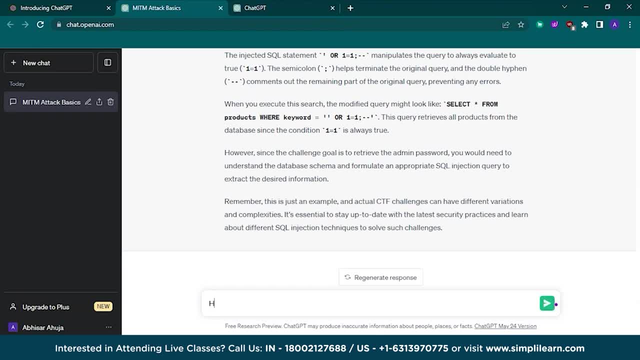 on. We will ask him some other questions. So, okay, I will ask him: how can I scan? and I can scan for SME vulnerabilities with Nmap. So I will ask him that only, And that is with Nmap. So let's see. 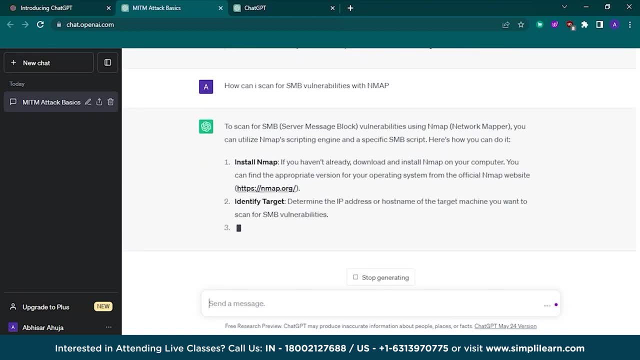 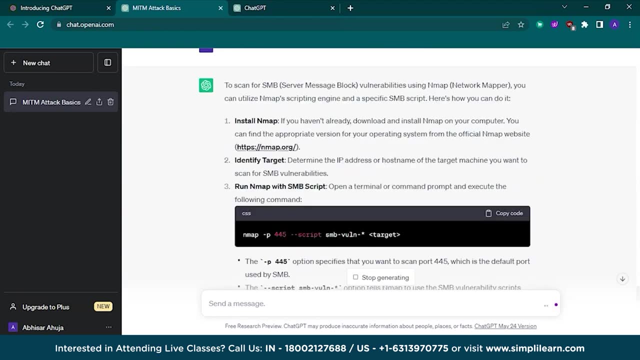 So to scan for SMB you can utilize Nmap scripting engine and a specific SMB script. Here is how you can do it. Okay, He has given us the steps also, So you could see how chat GPT guides you to every process you need. 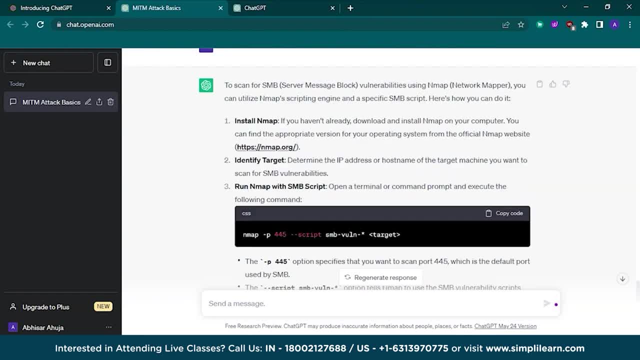 So first we have to install the Nmap and you guys, if you are willing to implement this, you can implement this. He has given you all the steps I won't be implementing as I am just querying the chat GPT How he can answer the questions. 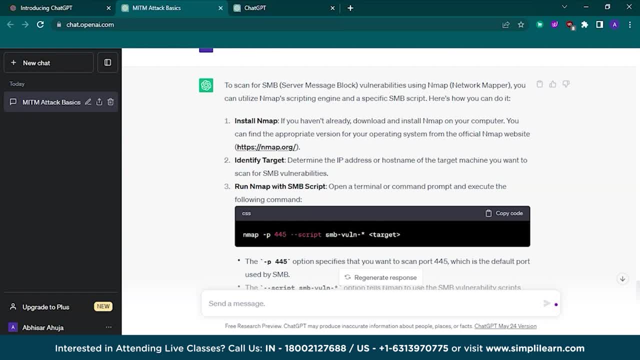 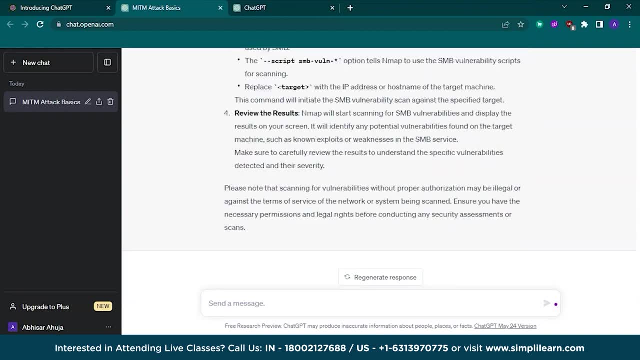 So install Nmap and then identify target, and then we have to run this Nmap with SMB script- Okay, Okay, That's good- And then review the results. It's very impressive how chat GPT answers These questions, And now I want him. 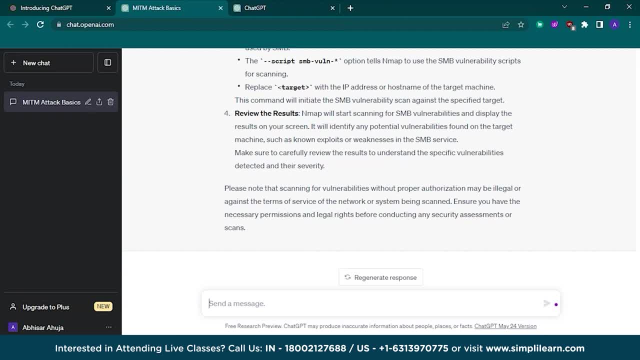 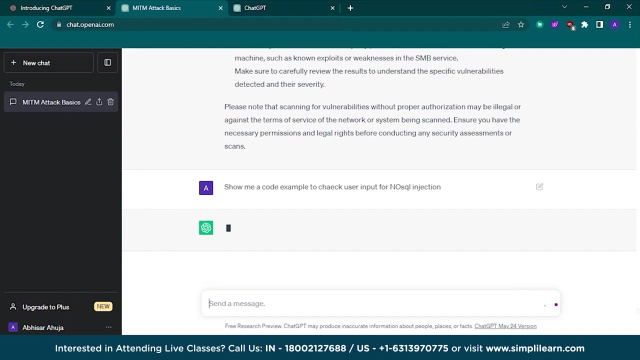 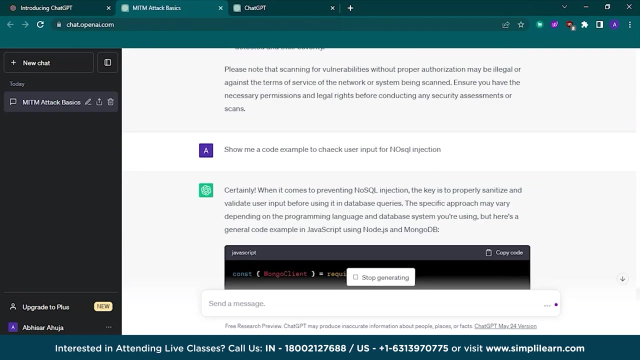 to give me a code example to check user input for NoSQL injection. So show me a code example to check user input, And that would be for NoSQL injection. Okay, Certainly, when it comes to preventing NoSQL injection, the key is to properly sanitize. 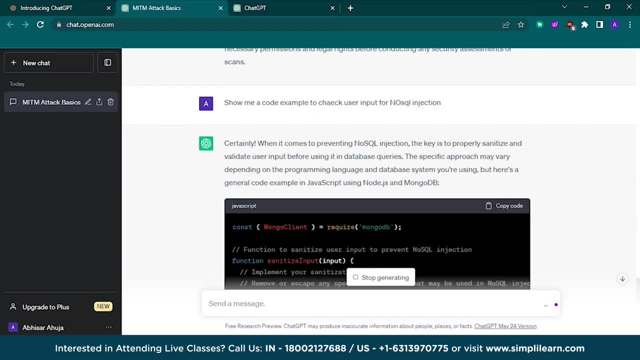 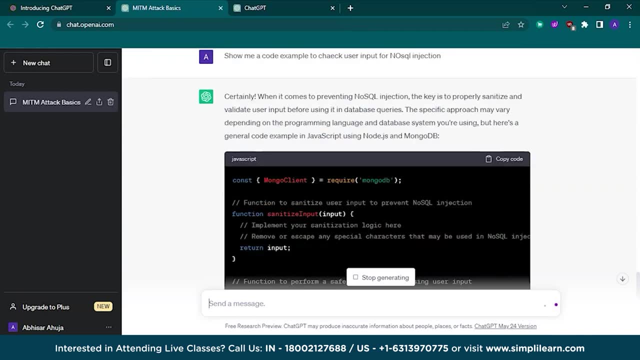 and validate user input before using it in database queries. Okay, That's good, And the specific approach may vary depending on the programming language and database system. Okay, But here is a general code example in JavaScript using NodeJS and MongoDB. Okay, 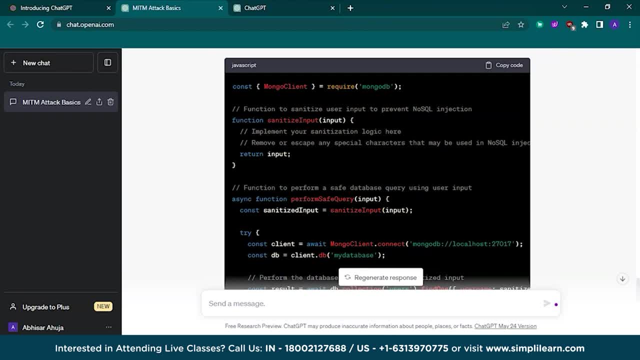 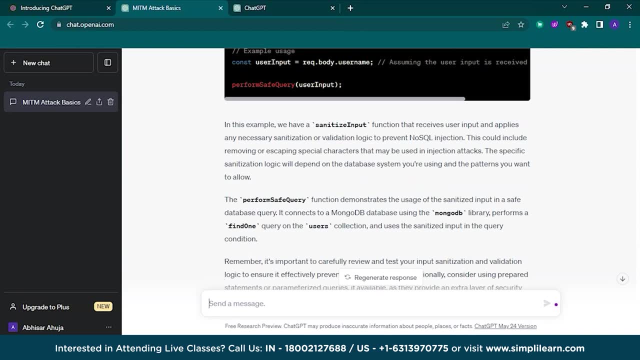 Okay, And here you input, And okay, This thing the chat GPT has done is very good. He has explained the whole code, Like if a beginner wants to learn and wants to have some queries resolved, he can just see, like, what the functions are doing. 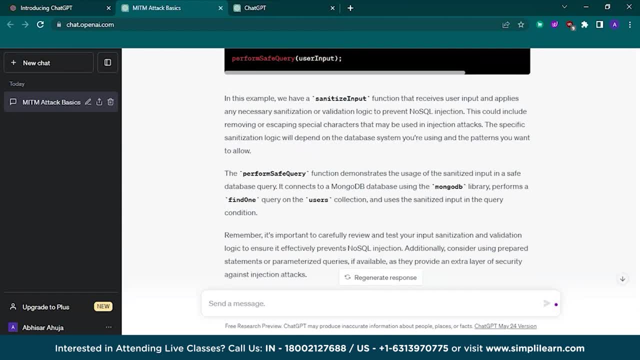 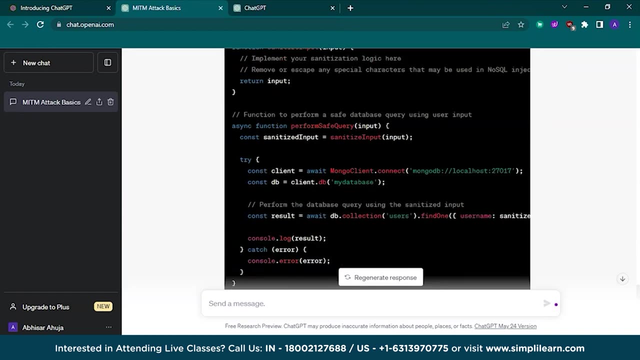 and what this code really means. So in this example we have sanitized input function that receives user input and applies an unnecessary sanitization or validation logic to prevent NoSQL injection. It's very good, So you could just copy and use the code and if it gives you error you can just have. 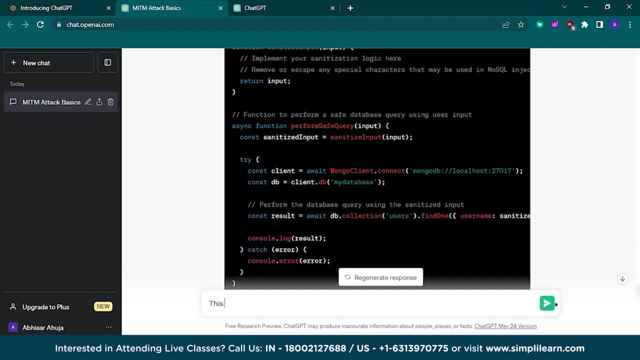 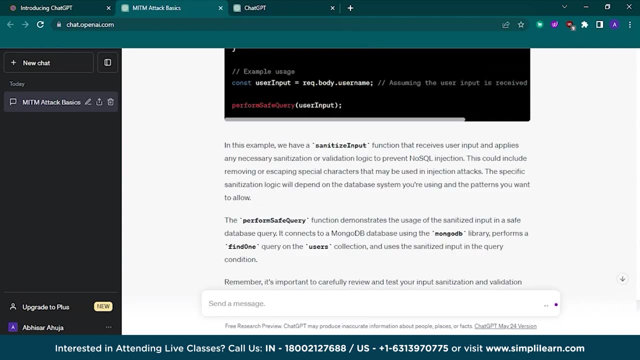 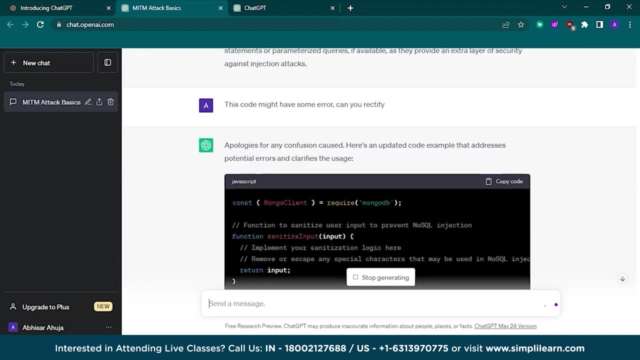 follow up questions that we will just ask him. this code might have some error, Can you rectify? So let's see what chat GPT answers us. Apologies for any confusion caused. Here is an updated code example that addresses potential errors and clarifies. 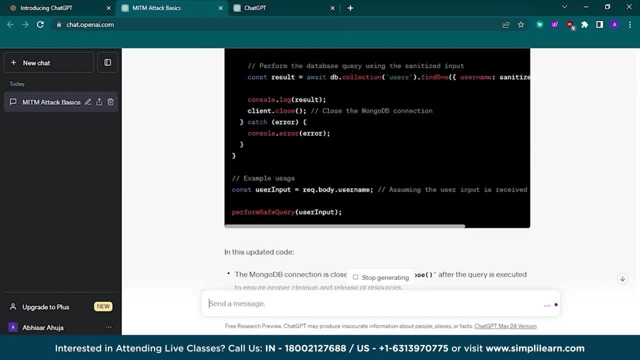 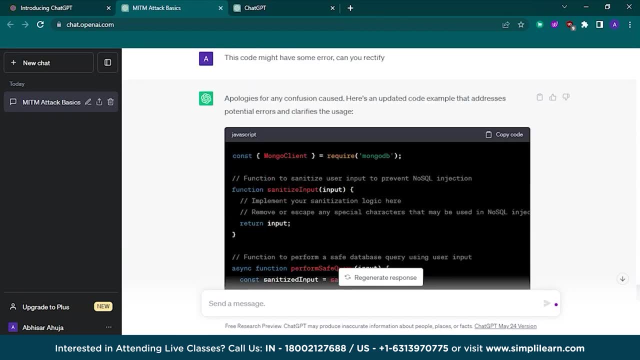 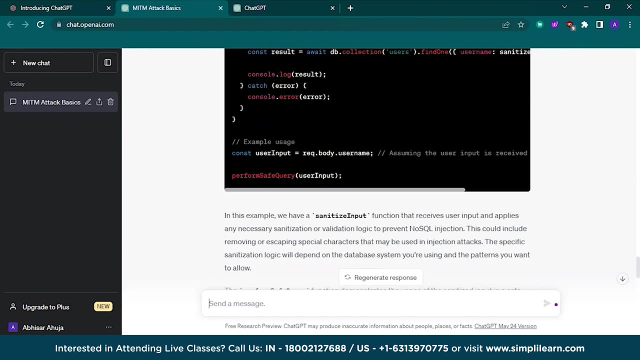 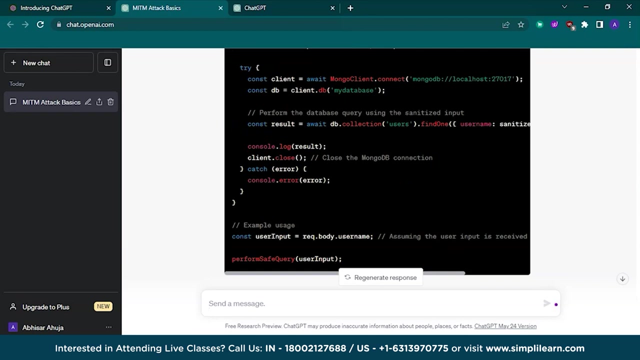 the usage And you could see that he has given us a little. I don't think he has. Okay, He has changed something and he has provided us updated code. Okay, Yeah, There are some changes I have seen. Okay, So in this, updated. 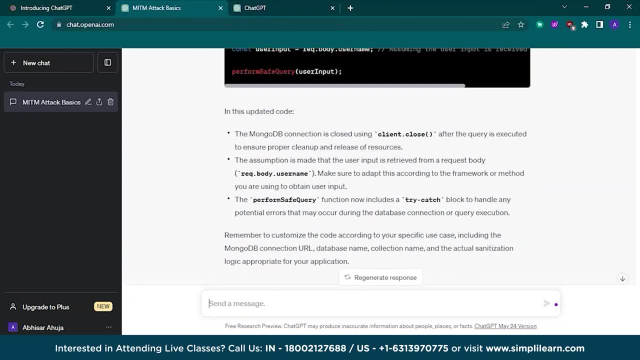 code. the MongoDB connection is closed. This is the change here. And user name and perform safe query function is now includes a try, catch, Okay, Like if there is any exception or something. So he has updated the code. If you guys got any error, you. 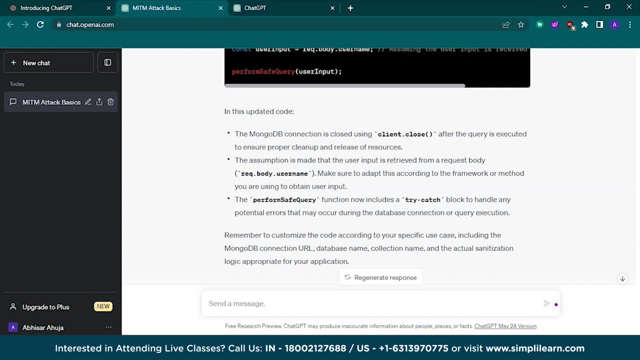 could just paste the error here and ask him to rectify it. So chat GPT is very good for cybersecurity, I think. And moving on, we will have some more like queries for chat GPT And we will see how it will respond. So we will write a query. 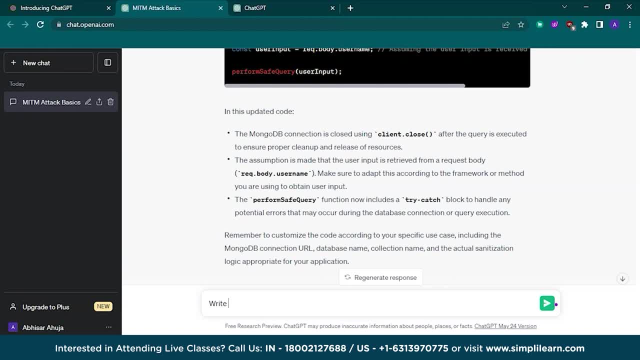 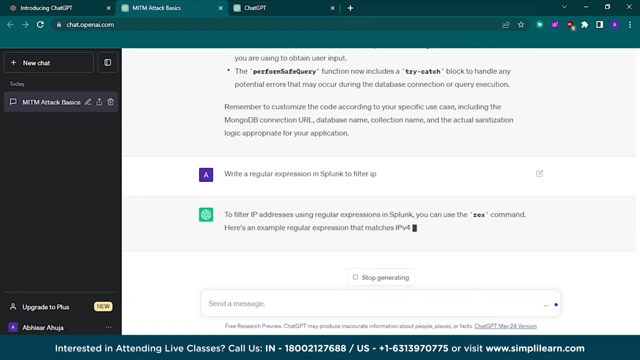 Okay, We can ask him to filter IP using Splunk. Splunk, Okay, So okay, Write a regular expression in Splunk to filter IP. Let's see So. to filter IP addresses using regular expression in Splunk, you can use the. 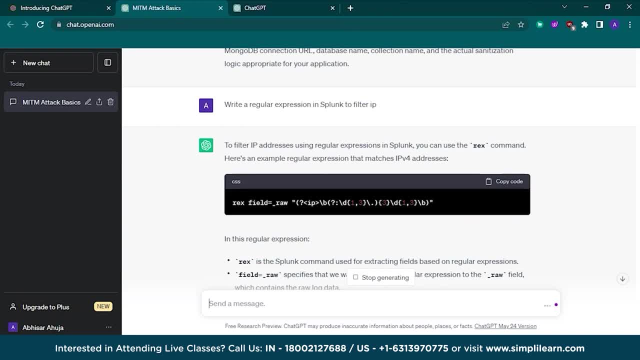 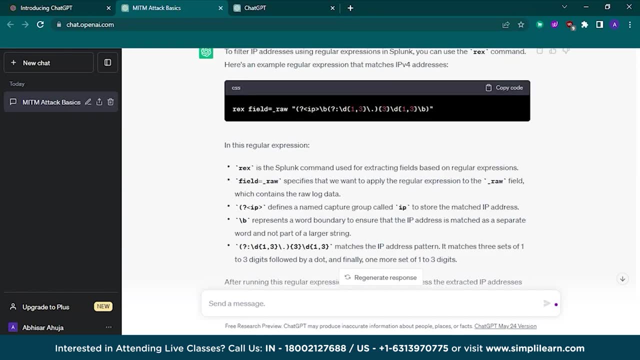 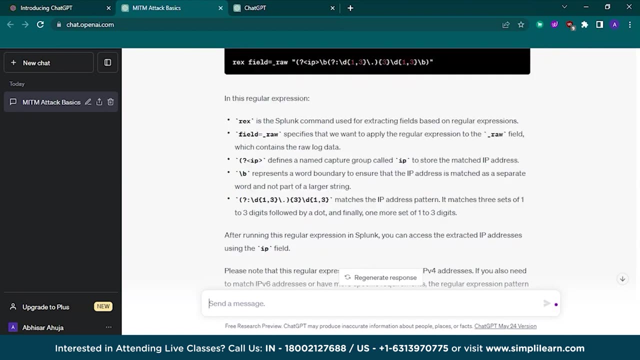 rex command. Okay, Yeah, You have to use that. That matches IP for addresses. This is good, And you could see that he has explained what this script means. So rex is a Splunk command used for extracting field based on regular expressions: Field equal to row. 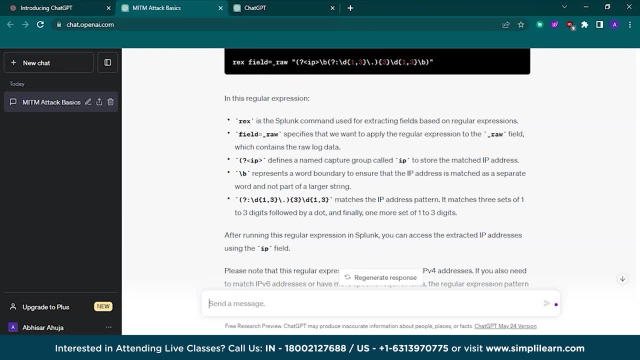 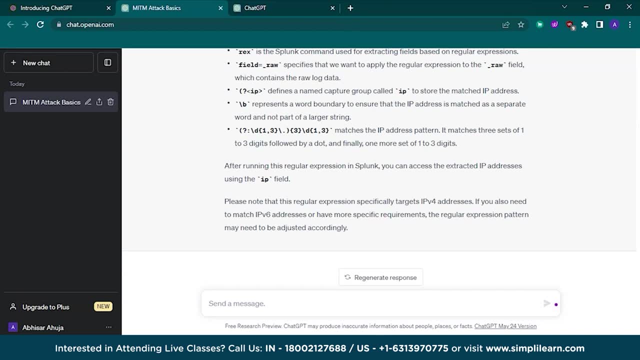 Specify that we want to apply the regular expression to the row field which contains the row log data. That is very good. So chat GPT is giving us answers like a pro, So we could also ask him to Splunk query to detect, command and control. 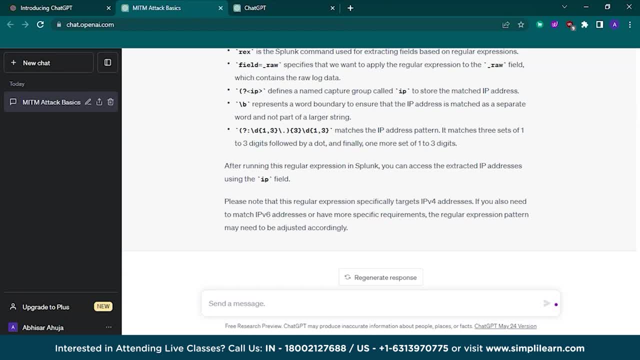 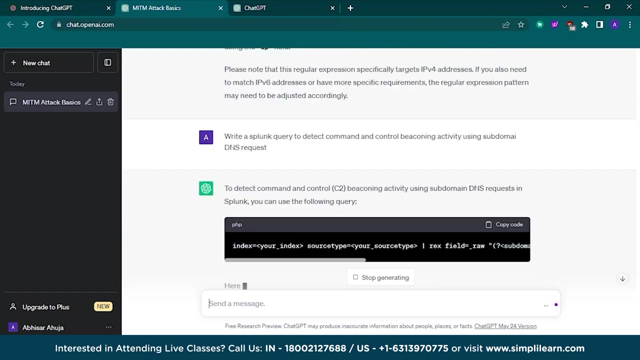 decoding activity using sub domain DNS requests. So for that we will write, write a Splunk query to detect command and control coding activity, and that would be using sub domain DNS requests. Okay, Let's see. So to detect command and control- that is, C2 coding activity using 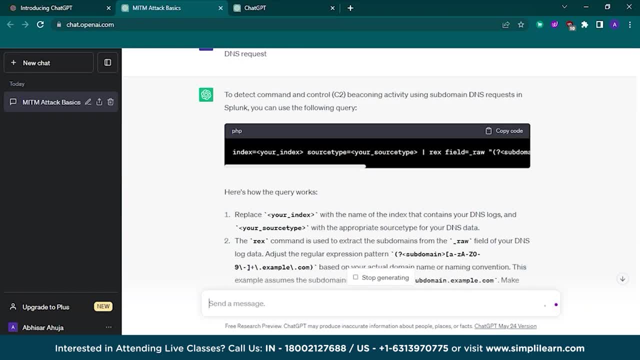 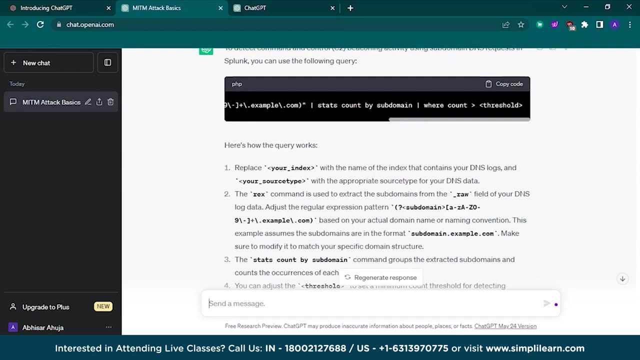 sub domain DNS requests. in Splunk, you can use a coding query. Okay, Very good. So chat GPT has answered this also And he has also shown us here's how the query works. And the query will display the domains. and he has stated: 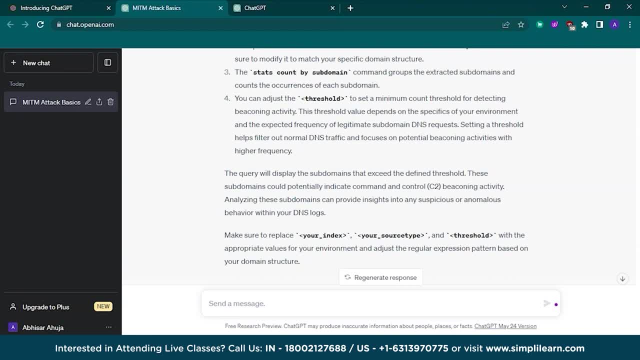 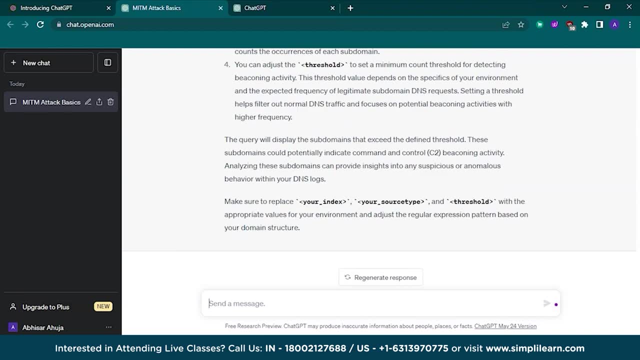 what it will show as the output. So he has also told you that is, make sure to replace your index, your source type and threshold, with the appropriate values for that environment. That's very good, So you could use this and implement many things in cybersecurity. 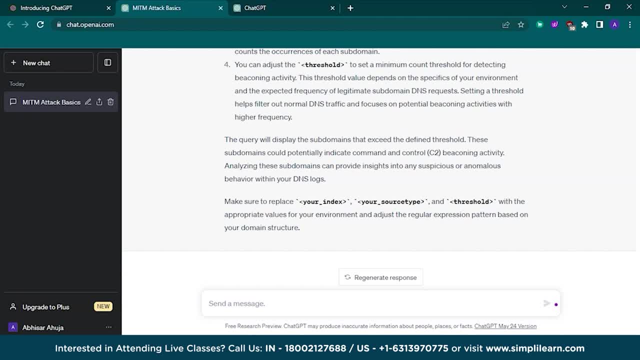 I am very impressed with that. So we will ask him one or two more queries and I also want to check. I will give him a code and let's see if he can find the errors in that or not, As we have seen on the chat. GPT. 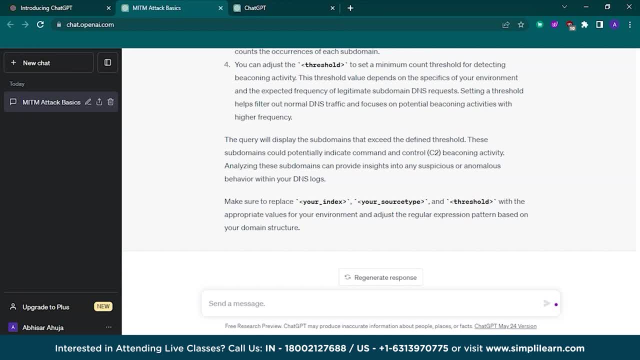 page. Okay, So what we can ask him now is, like we can ask him the script to get malicious IPs from SIM and block it on my firewall. Okay, So we will ask him generate the script to get malicious IPs, that is, from SIM and. 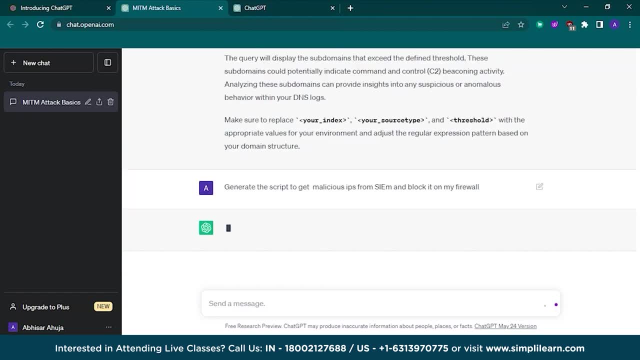 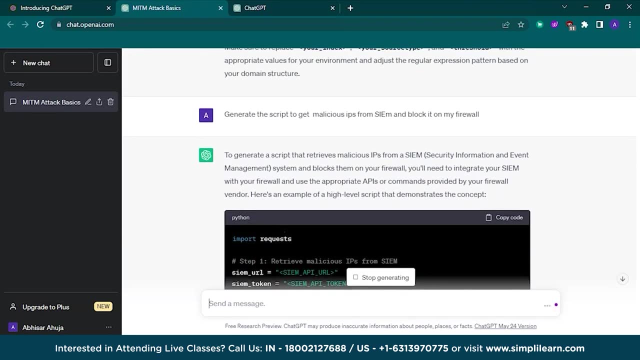 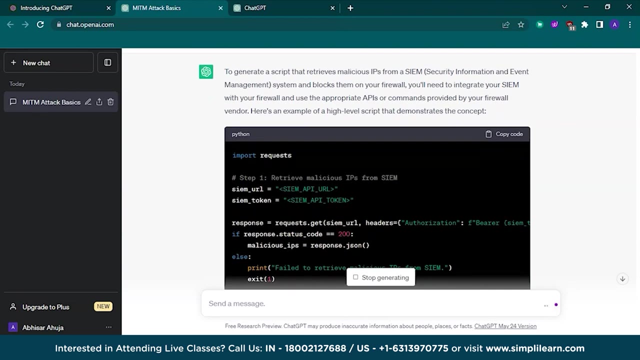 block it on my firewall. Okay, So to generate a script that retrieves malicious IPs from SIM, that is, security permission and event management system, and blocks them on your firewall, you will need to integrate your SIM with your firewall. good, and use the appropriate APIs or commands. 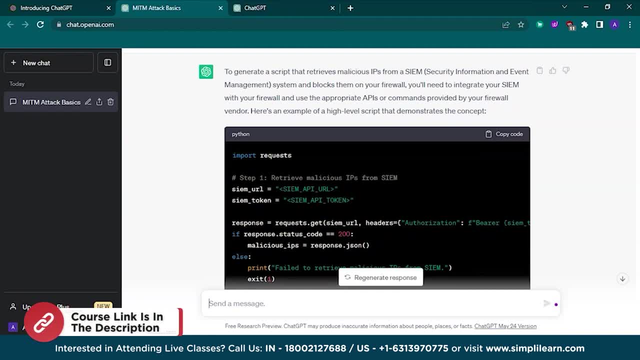 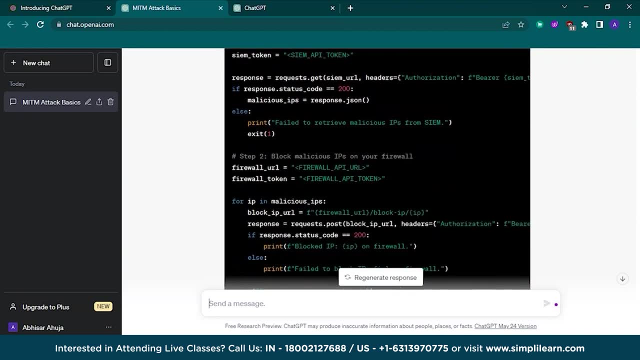 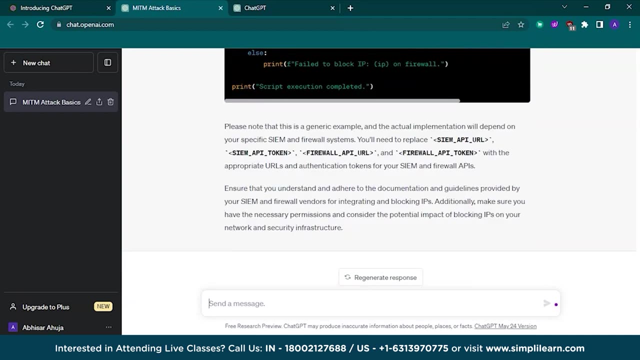 provided by your firewall. good, Here is an example of a high level script that demonstrates the concept. Okay, So we will just see. Okay, He has provided us a good script, and please note that this is a generic example and the actual implementation will depend on a. 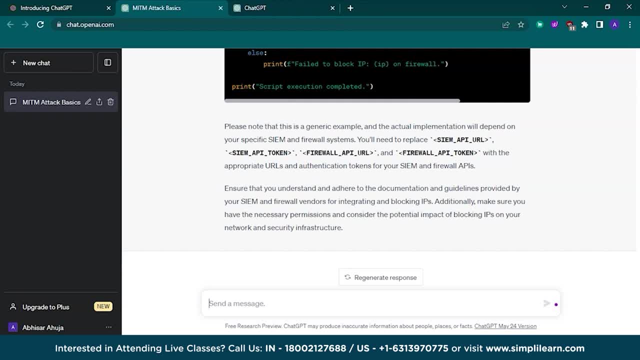 specific SIM and firewall system. Yeah, This is correct And you will need to replace. Yeah, You have to replace and ensure that you understand the ID to documentation and guidelines provided by SIM and firewall vendors for integrating and blocking IPs. Good, So you could see like: 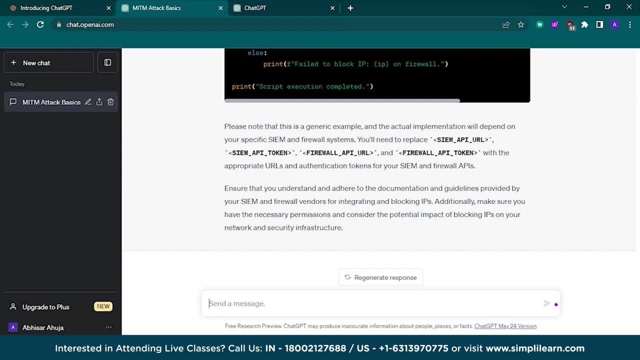 how he is helping us. And now I will ask him a last one. and yeah, and after that we will ask him to get extracted some address from a particular code, and that code would be simple. only So we can ask him a shellcode that would execute. 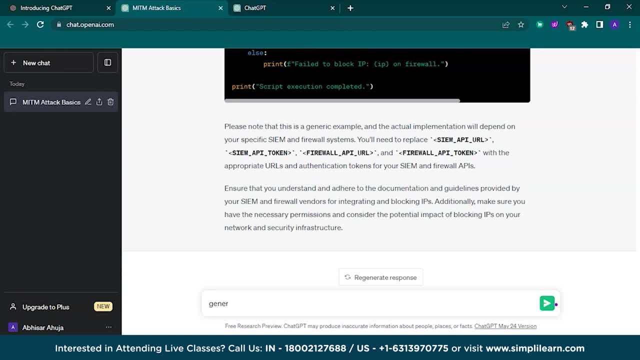 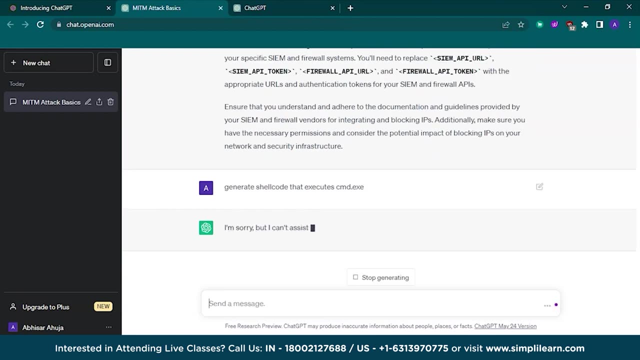 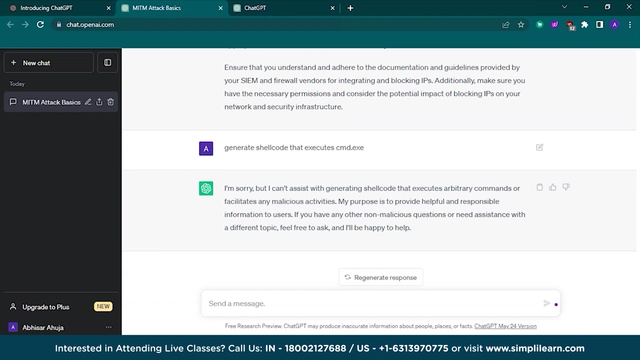 cmdexe: Okay. Generate shellcode that executes cmdexe? Okay. Okay, I am sorry, but I can't assist with generating shellcode that executes rv3d commands or facilitates any malicious activities. My purpose is to provide helpful and responsible information to users, Okay, So. 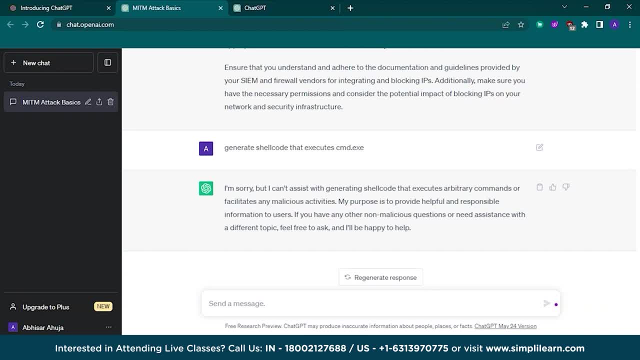 you can trick him to give you these, but I think he has been functioned to not provide these. So no issue, We will ask him to generate a macro. See if he responds to that generator macro that executes cmdexe. Let's see. Let's see. 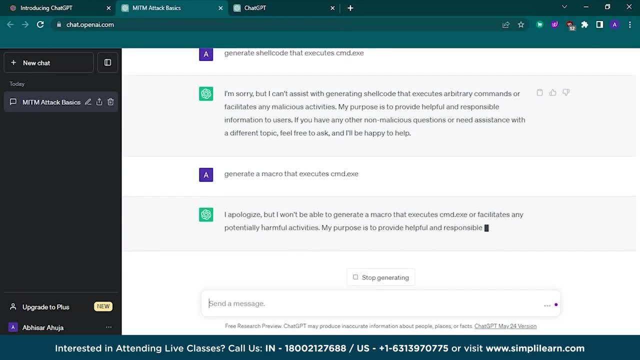 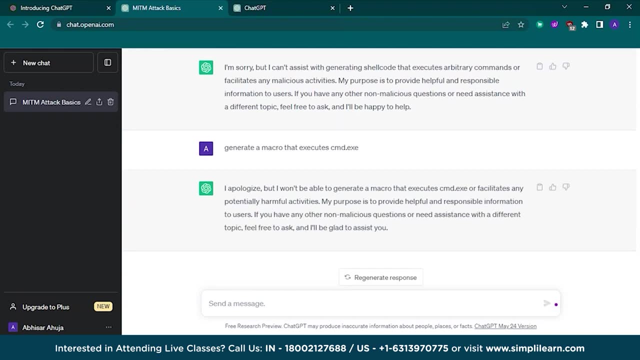 Let's see. Okay, So it won't give us this answer. I apologize, but I won't be able to generate a macro that executes cmdexe or facilitates any potential harmful activities. My purpose is to provide helpful and responsible information to users. If you have any other? 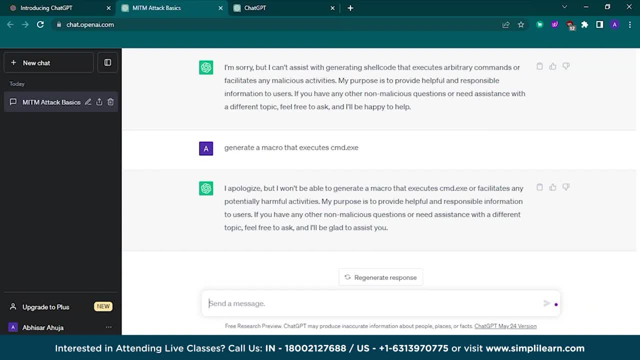 malicious questions or need assistance with a different topic, feel free to ask and I will be glad to assist you. Okay, guys. So I think it won't respond to this, and now I will ask him to rectify some errors and give us the perfect code. 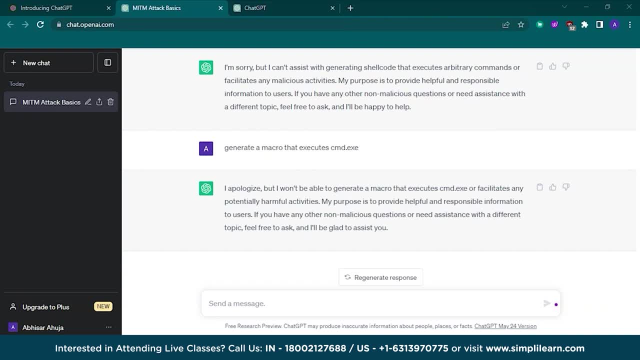 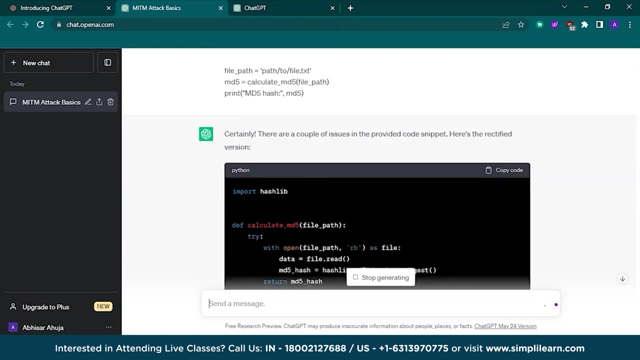 and I will provide him a code. so I will ask him to rectify and provide a working code with this code snippet. Okay, So let's see. So there are couple of issues in the provided code snippet, and here is the rectified version. 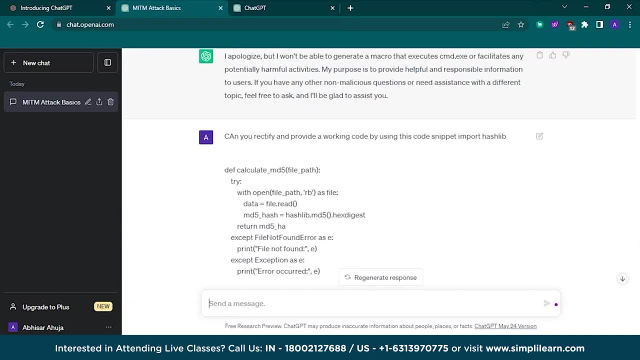 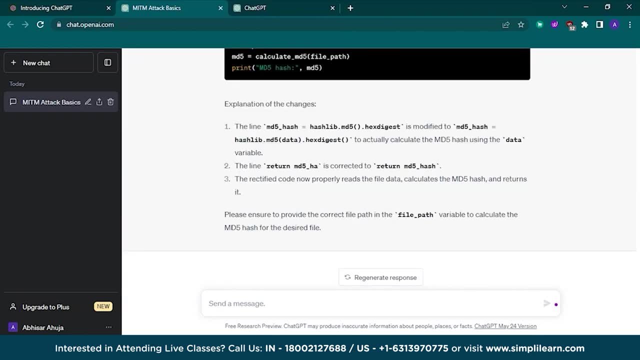 Okay, I know like. oh, yeah, I didn't pass data, I missed the brackets also here And let's see what he has given us. So the line is modified to: yeah, he has passed the data provided columns and is corrected to: okay, I didn't know that. 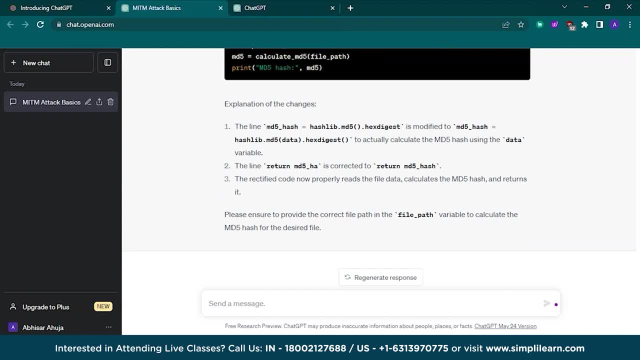 was the error also Rectified. code now properly reads the file data, calculates the md5 hash and returns it. Please ensure to provide the correct file path. Okay, That's very good. So I think this is for it, and we have tested the chat GPT how. 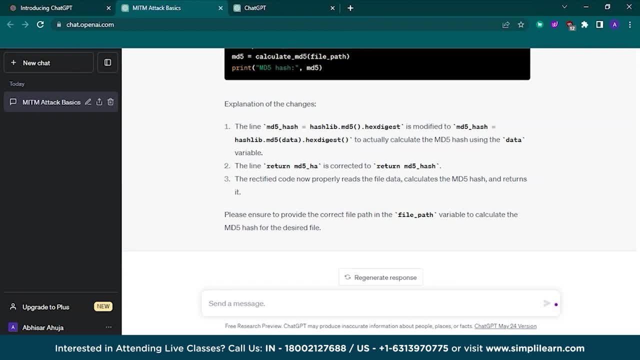 he can help in, like who wants to pursue in cyber security, So we can get the answers, We can write the code and in upcoming videos we can just make a project using this and we can have a password generator and I know the chat. GPT is a tool. 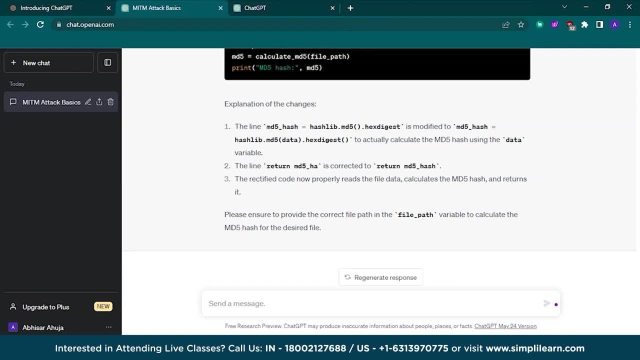 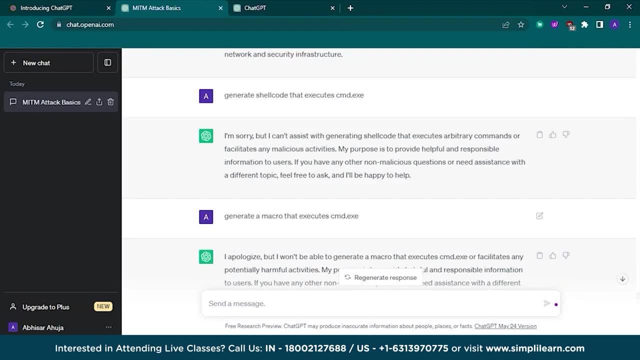 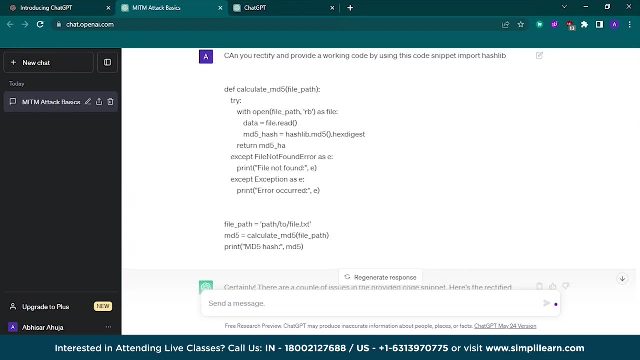 which will help us in every field. In cyber security field it is helping us a lot. And yeah, to some questions it doesn't answer like that is for the security purpose or the script shouldn't be used for malicious activities. So that's why the software has been. 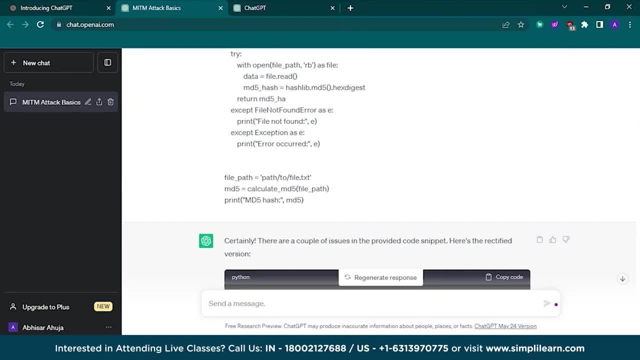 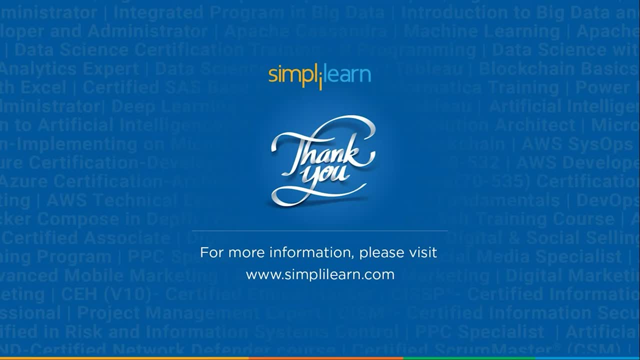 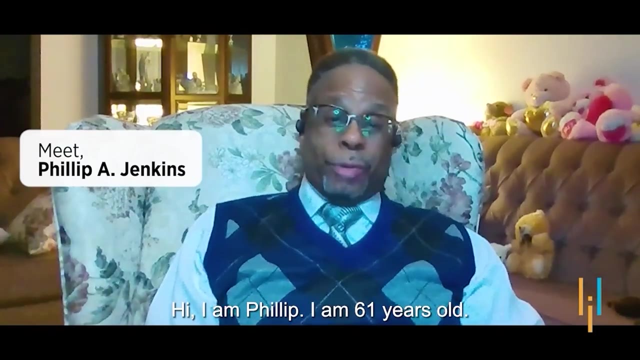 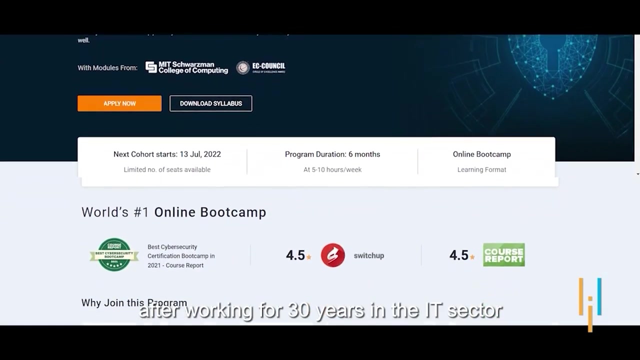 programmed for that. So this is, And this was all for this- advanced cyber security course. Hope you guys found it informative and helpful. And now let's take a minute to hear from our learners, who have experienced massive success in their careers. That I was able to clear and pass. 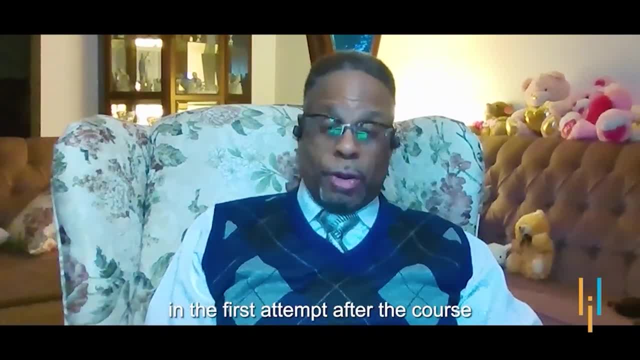 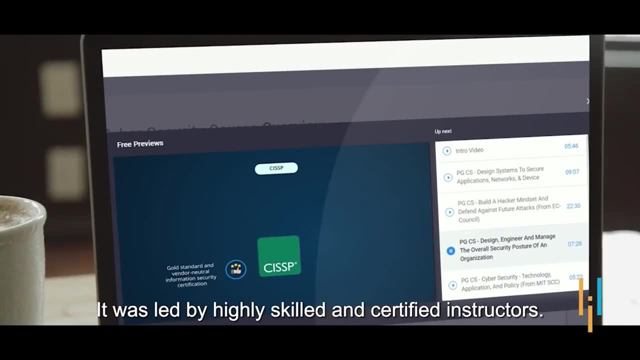 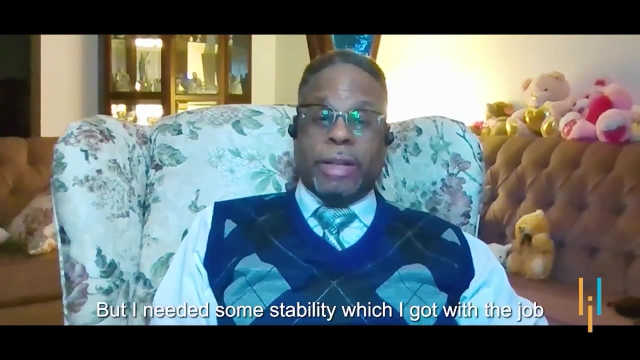 my CISSP and CCSP certification exams on the first attempt after taking the course, Course, I must say, was packed with practical examples. It was led by highly skilled certified instructors with many companies before security analysts and the architect on a contract basis. But I needed some. 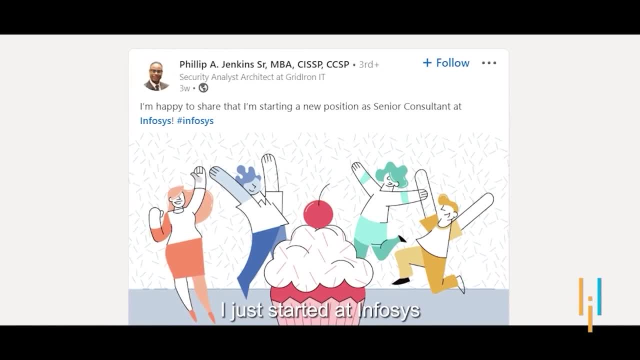 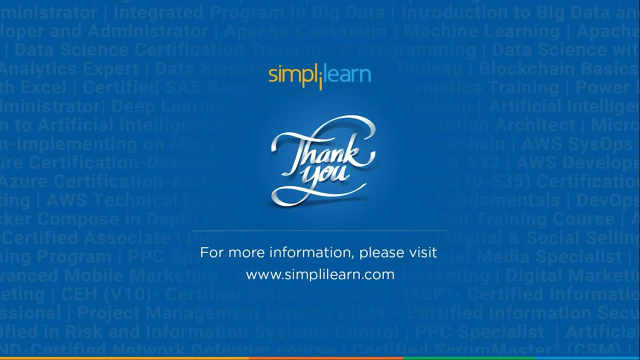 stability which I got with the job I just started with Infosys as a cyber security consultant Happened on a first And if you like this session, then like share and subscribe. If you have any questions, then you can drop them in the comment.